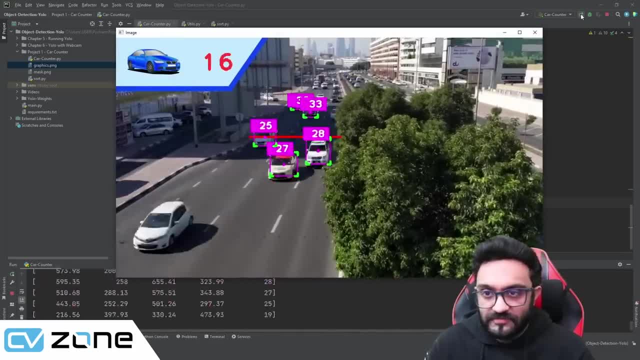 Hey everyone, welcome to my channel. This is the Object Detection 101 course. In this course we will cover everything to get you started with object detection, along with four exciting and real-world projects. We will first start with the theory and have a look at its brief history. 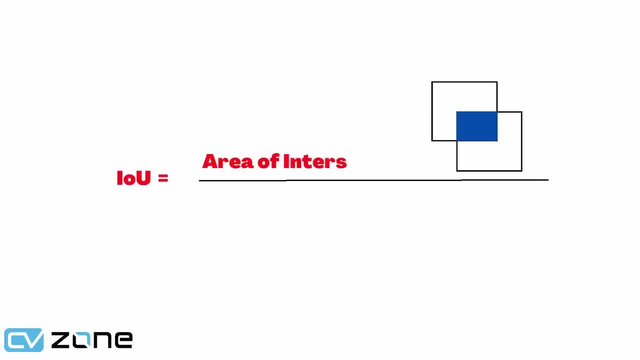 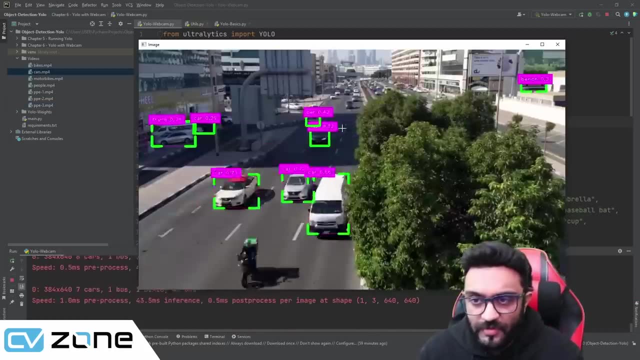 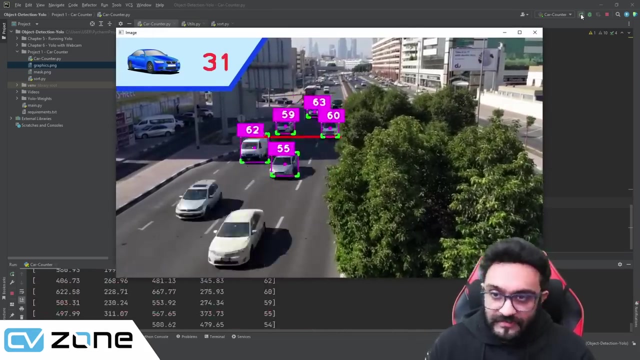 Then we will understand the working of object detection, along with its evaluation matrix. From there we will install everything from the start and run the YOLO version 8 Object Detection pre-trained models. Using these models we will create two projects: Car Counter and People Counter. Here we will learn how to implement object tracking along 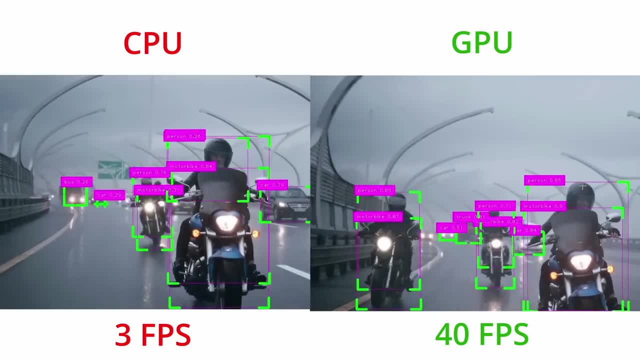 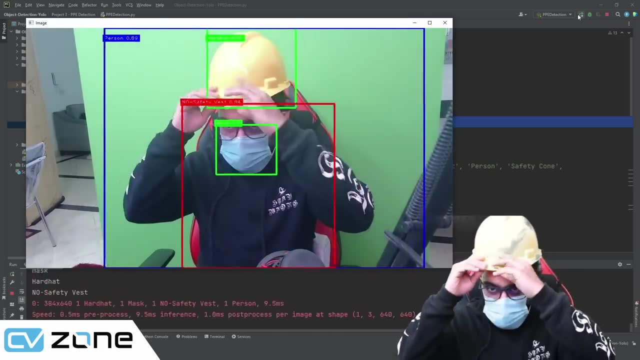 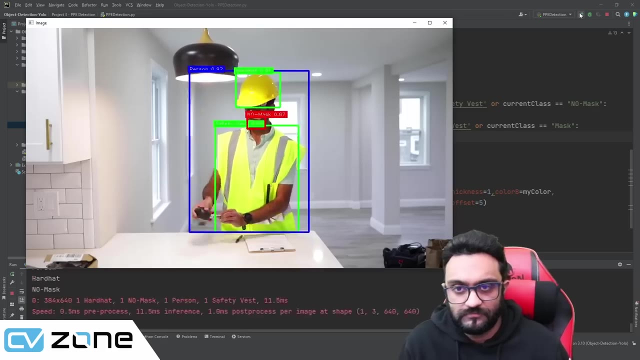 with object detection. We will also install and run YOLO with our GPU for better performance. Later we will learn how to train a custom YOLO model using our own dataset and create two projects using our own training. The first one will be Personal Protective Equipment Detector. 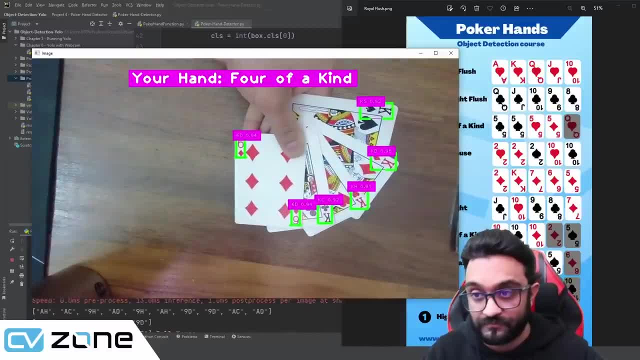 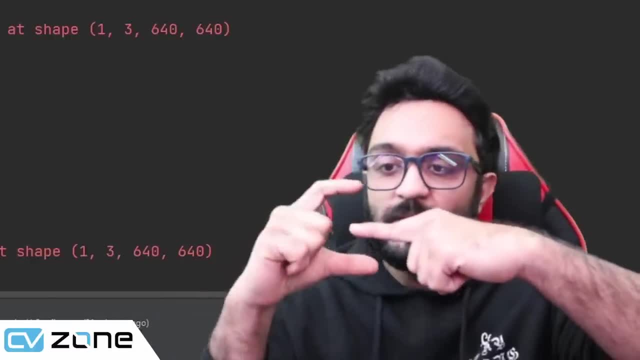 and the second one will be Poker- Poker Hand Detector, where we will first detect the playing cards and then create a classifier to classify the correct poker hands. If you are a beginner, don't worry, this course is for you. We will go step by step, so it is easy. 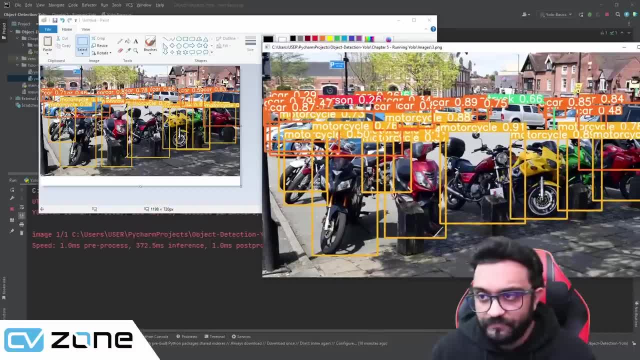 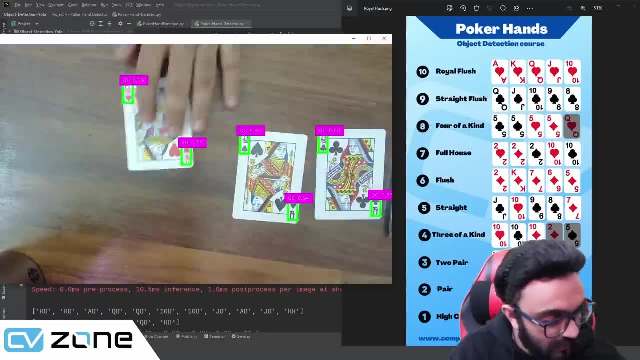 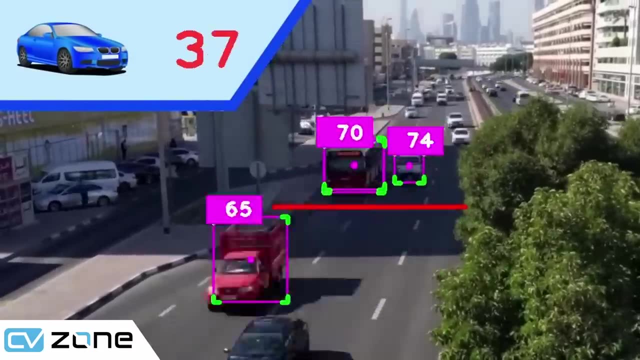 to follow. This is an information-dense course that will provide you with maximum knowledge without wasting your time. Learning Custom Object Detection is a superpower that can allow you to solve real-world problems, and it can be easily completed over a weekend. So buckle up and get your nerdy glasses on, and let's get started. 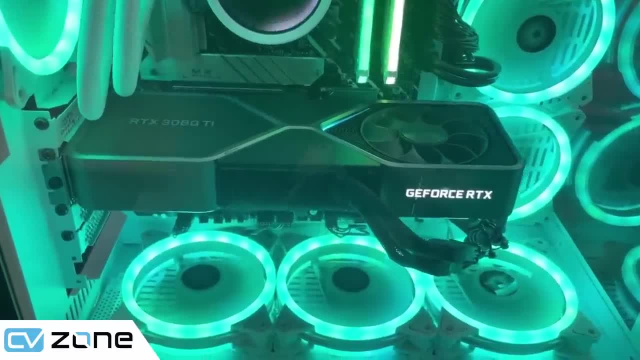 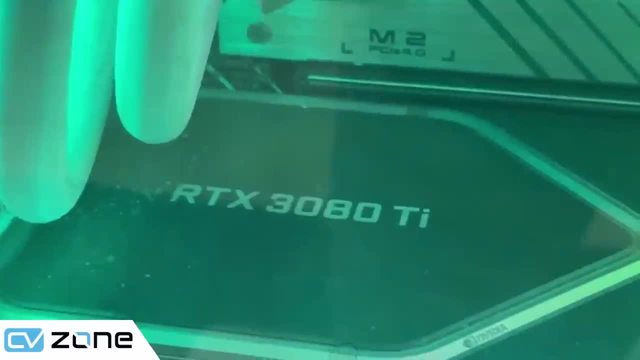 But wait, we are going to use NVIDIA's 3080Ti graphics card in this course. Now my question to you is: would you like to have one too? If yes, then you are in luck. I will be giving away a 3080Ti graphics card, and all you have to do is register to NVIDIA's. 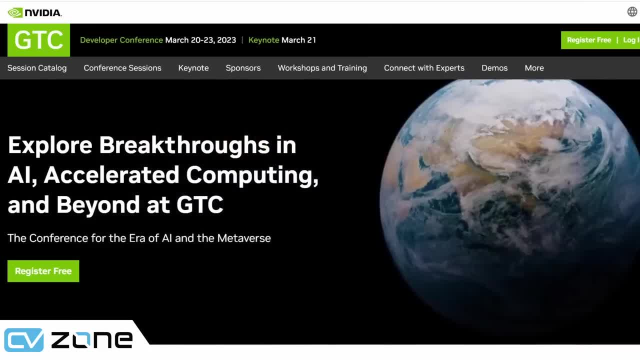 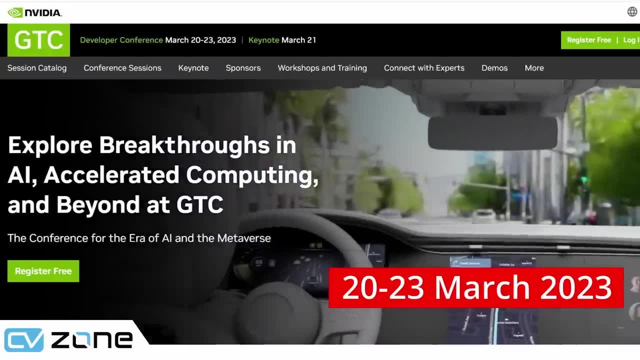 GTC 2023 conference through my link in the description and attend one of their sessions to enter the giveaway automatically. The conference will be held from 20-23 March 2023.. This is a great place to learn new things and keep up with the trend. 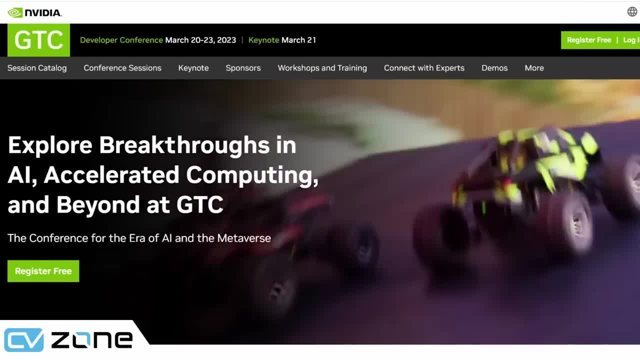 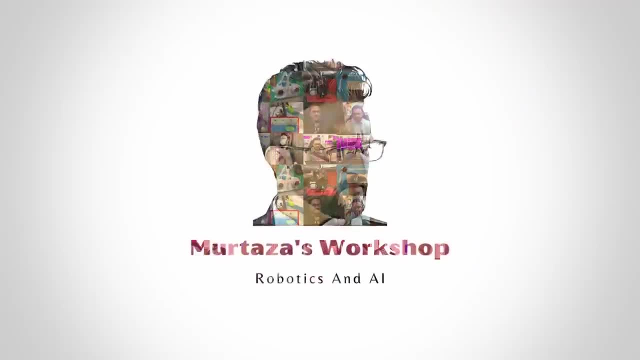 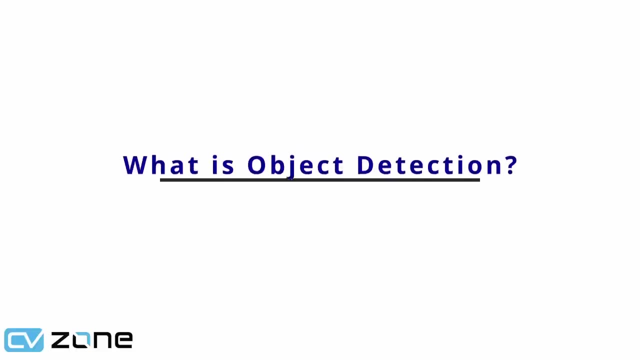 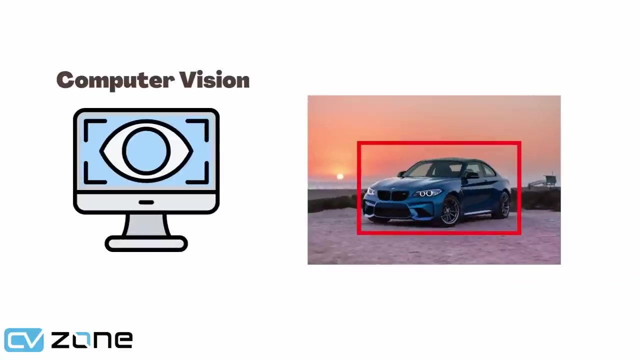 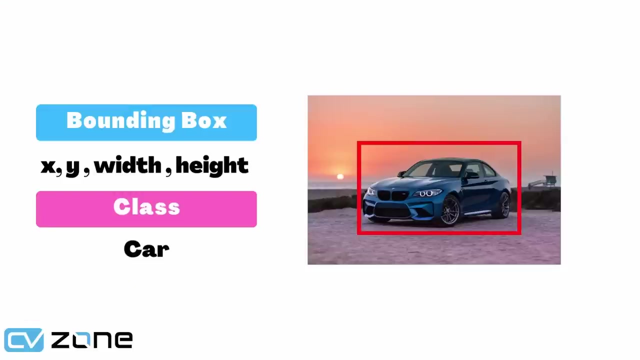 So sign up today and I will see you there. What is Object Detection? Object Detection is a computer vision technique for locating objects in an image or a video. Object Detection gives us the bounding box information of the object, well as the classification of that object. What is Object Detection? Object Classification: 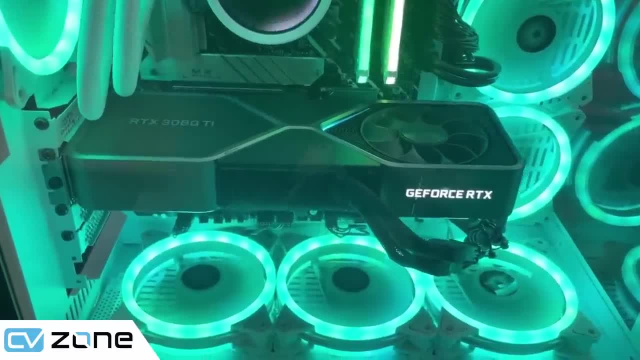 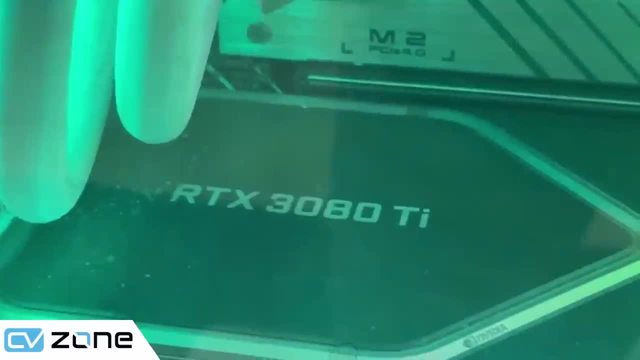 But wait, we are going to use NVIDIA's 3080Ti graphics card in this course. Now my question to you is: would you like to have one too? If yes, then you are in luck. I will be giving away a 3080Ti graphics card, and all you have to do is register to NVIDIA's. 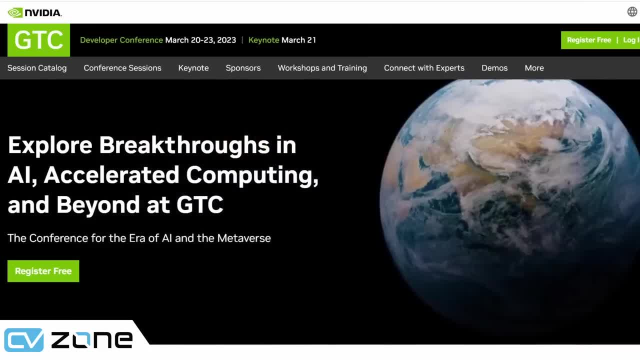 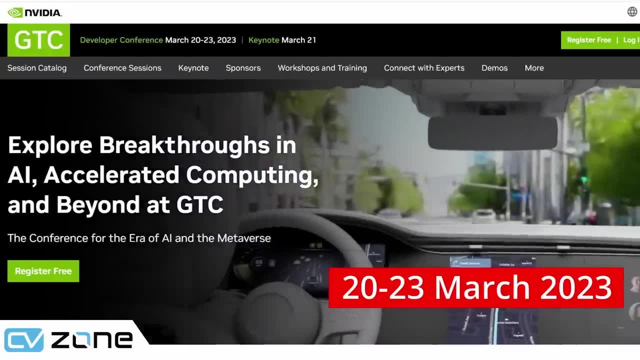 GTC 2023 conference through my link in the description and attend one of their sessions to enter the giveaway automatically. The conference will be held from 20-23 March 2023.. This is a great place to learn new things and keep up with the trend. 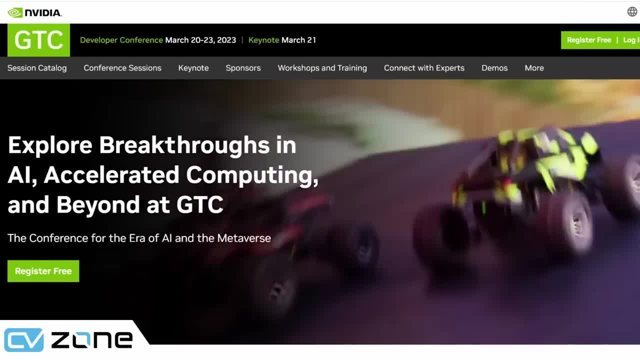 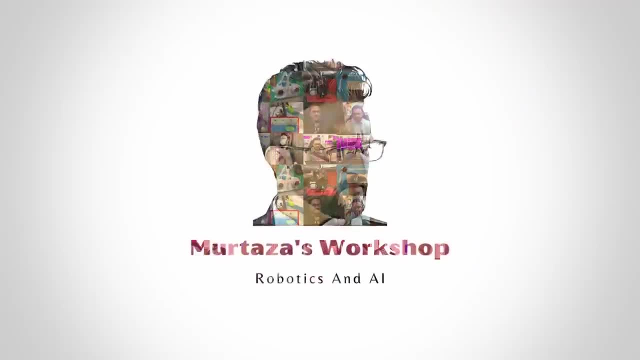 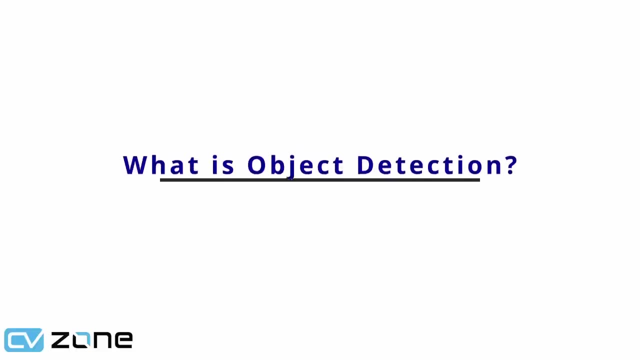 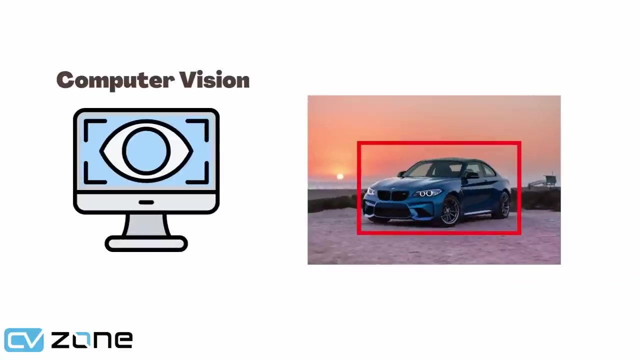 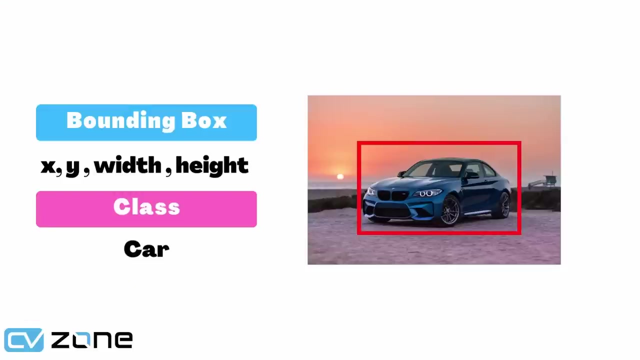 So sign up today and I will see you there. What is Object Detection? Object Detection is a computer vision technique for locating objects in an image or a video. Object Detection gives us the bounding box information of the object, as well as the classification of that object. What is the difference between Object Classification? 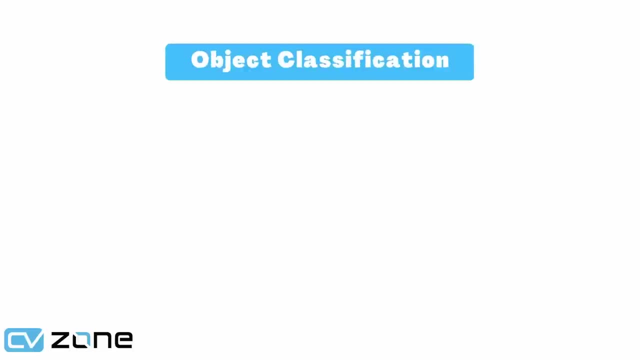 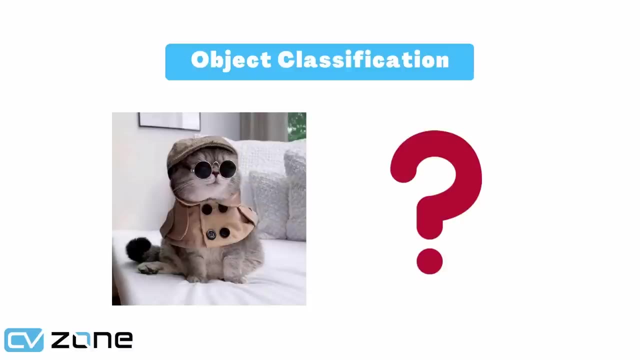 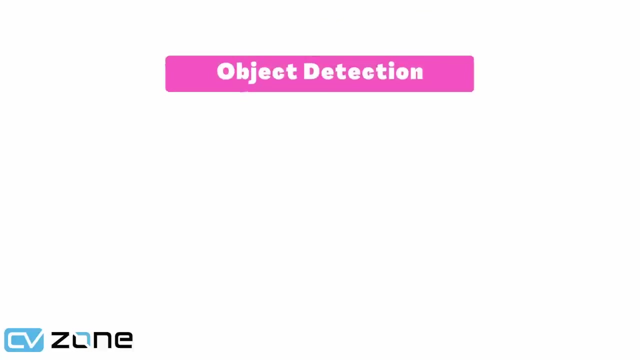 Object Detection and Object Segmentation. Object Classification is a type of image recognition that identifies what type of object is present in an image. Here the complete image is sent for classification, So the output is single class. Object Detection is a type of image recognition that is used to identify and locate the presence. 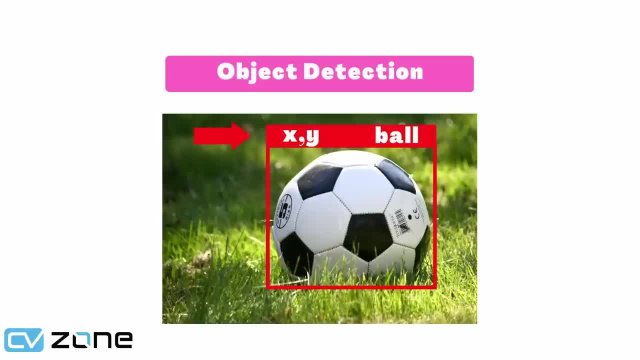 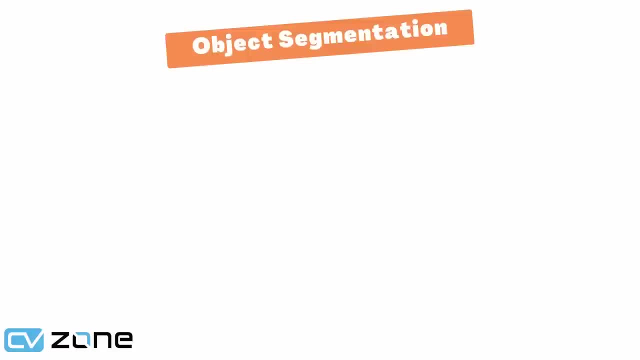 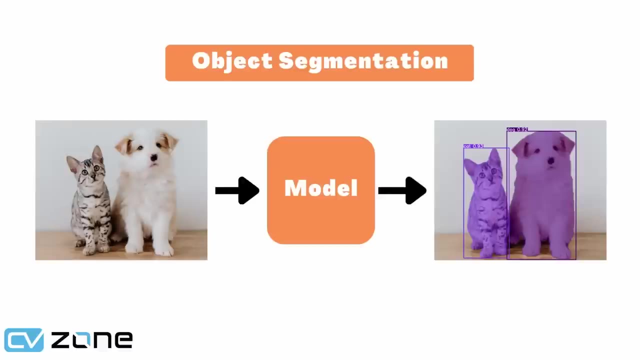 of an object in an image. this gives us the bounding box information and the class as well. here the results can be multiple bounding boxes and classes. object segmentation is the type of image recognition that is used to identify and separate the distinct objects in an image on a. 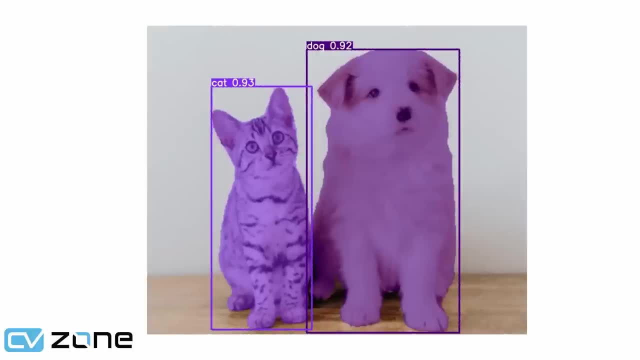 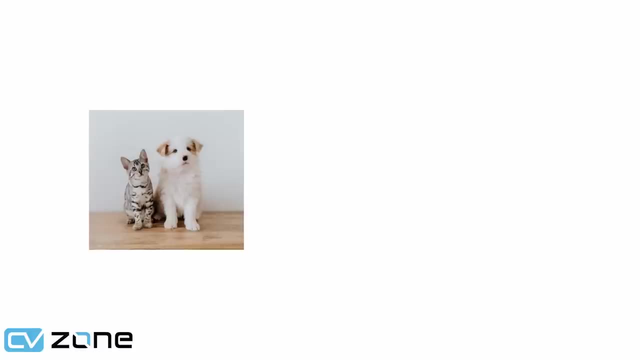 pixel level. here we get the exact shape of the object detected rather than just the bounding box. although image segmentation provides more information, image detection is still the first choice for most computer vision applications, since it is less computationally expensive. a brief history of object detection. object detection was first started in the 1970s. 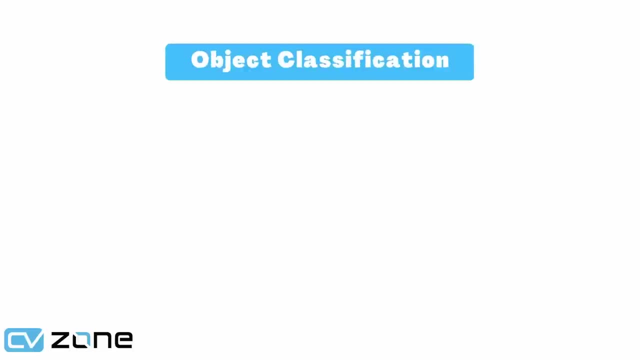 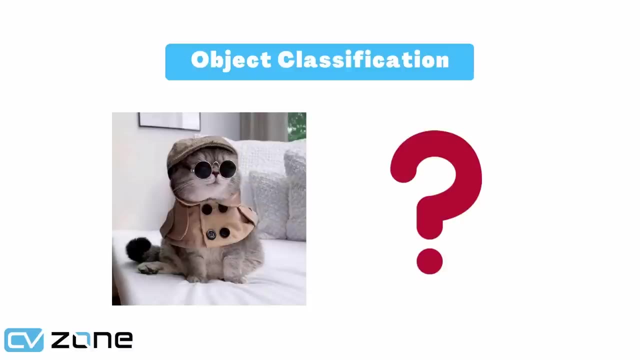 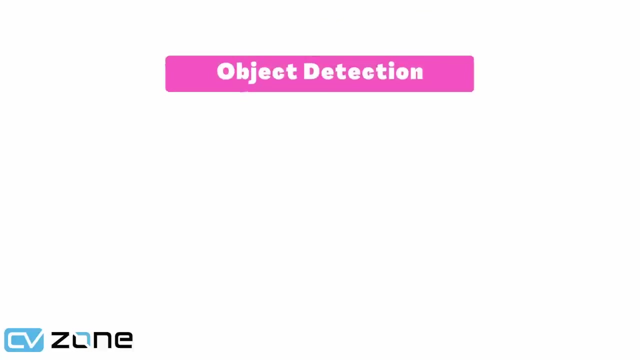 Object Detection. Object мал Detection is a type of image recognition that identifies to what type of object is present in an image. Here the complete Image is sent for classification, So the output is single class. Object detection is a type of image recognition that is used to identify and locate the presence. 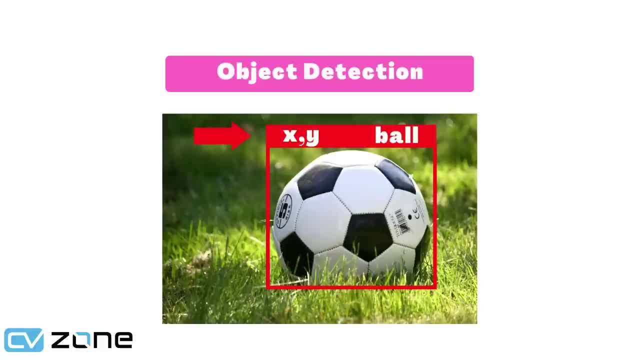 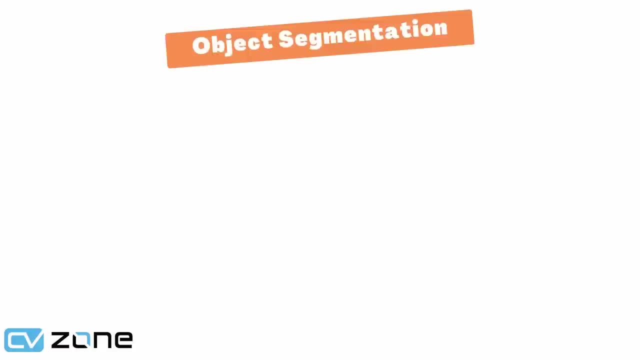 of an object in an image. Object Detection equals being able to go straight to a tenimclip of an image in an image. This gives us the bounding box information and the class as well. Here the results can be multiple bounding boxes and classes. Object segmentation is the type of 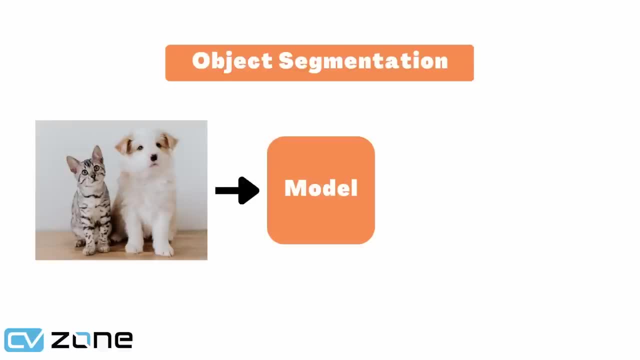 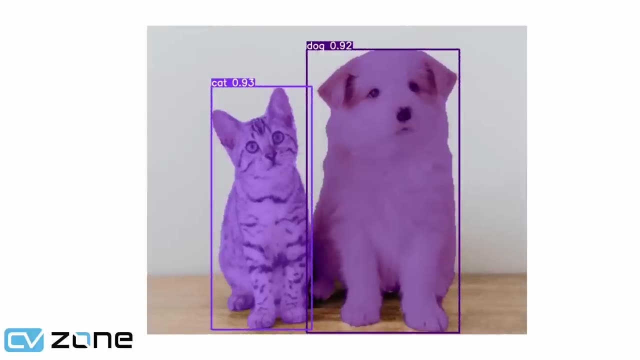 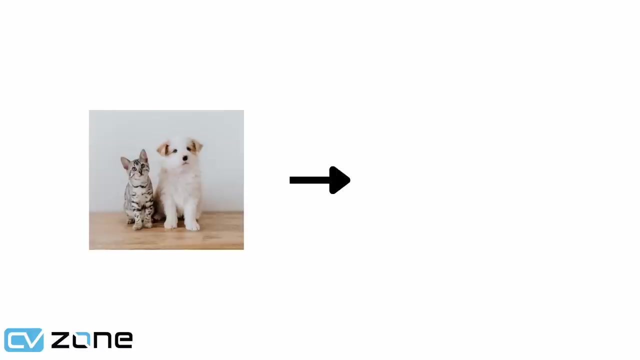 image recognition that is used to identify and separate the distinct objects in an image on a pixel level. Here we get the exact shape of the object detected rather than just the bounding box. Although image segmentation provides more information, image detection is still the first choice for most computer vision applications, since it is less computationally. 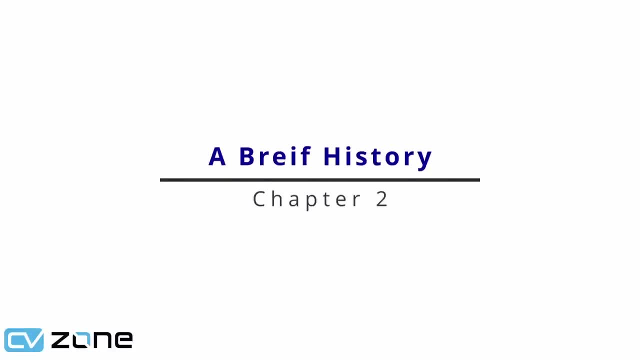 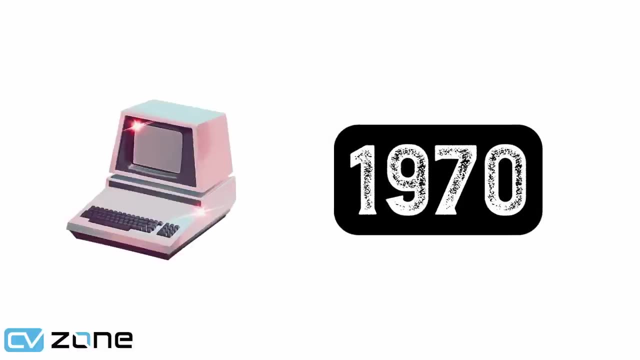 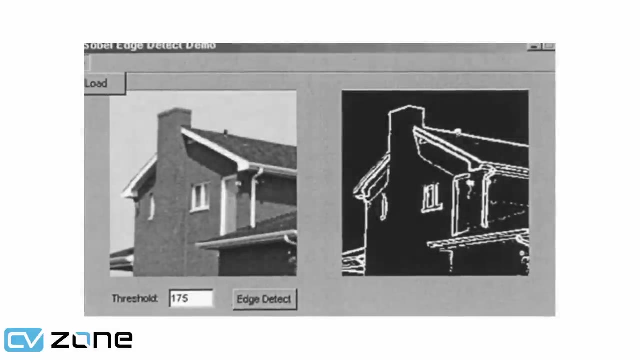 expensive. A brief history of object detection. Object detection was first started in the 1970s. Researchers started to develop automated methods for object detection. The first automated object detection algorithm were based on the method of object detection, The first method of object. 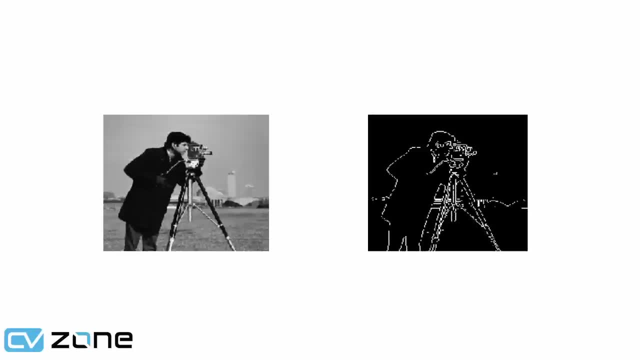 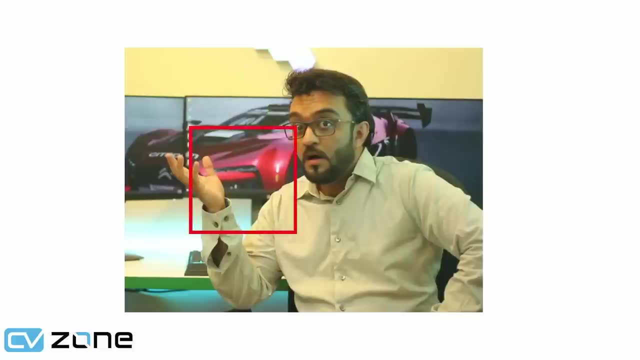 detection was the method of object detection. The first method of object detection was the method of object detection on simple features such as edges and corners. The first real object detection was Viola Jones, developed in 2001.. It used sliding windows to search for heart-like. 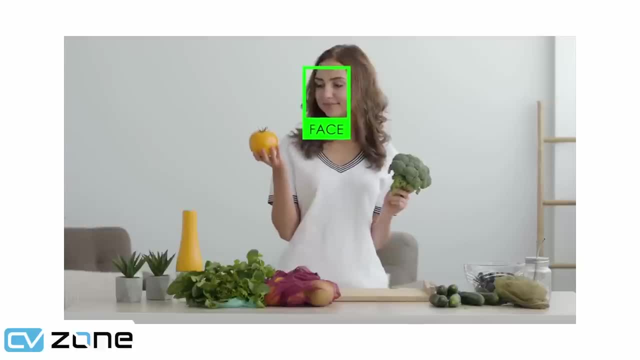 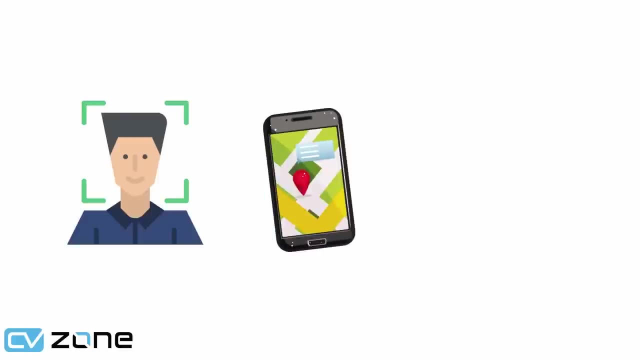 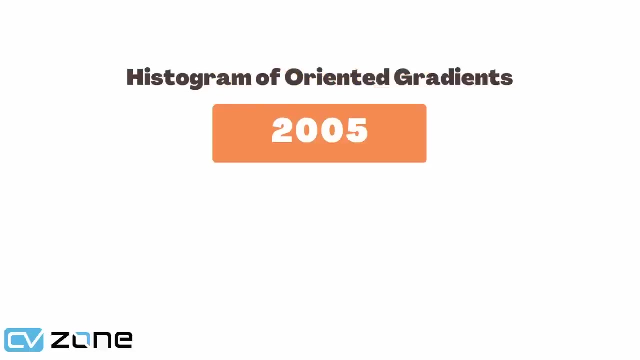 features, which are simply rectangular features. This method became popular since it was real-time For the longest time period. this method was used for face detection in smartphones and cameras. The histogram of oriented gradients was another method released in 2005.. That focus 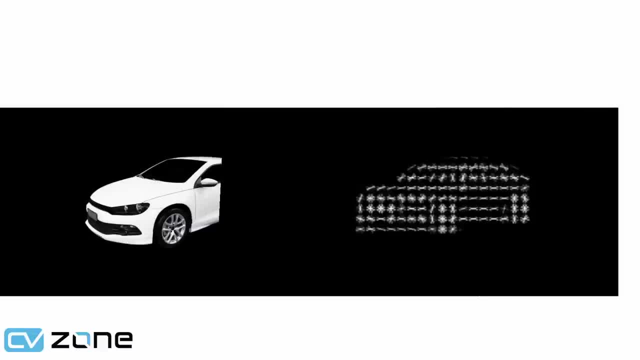 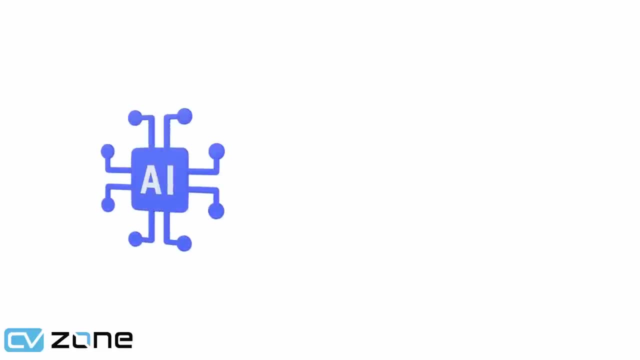 on the shape of the object. It worked by extracting the gradient and orientation of the edges. This method was mostly used to detect humans in an image. Then came the revolution of AI, with neural networks gaining popularity. The true potential was seen with convolutional neural. 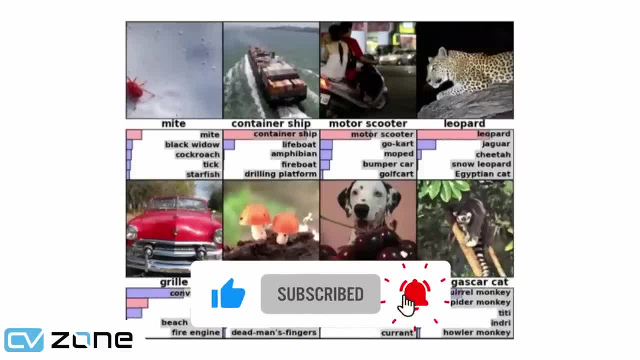 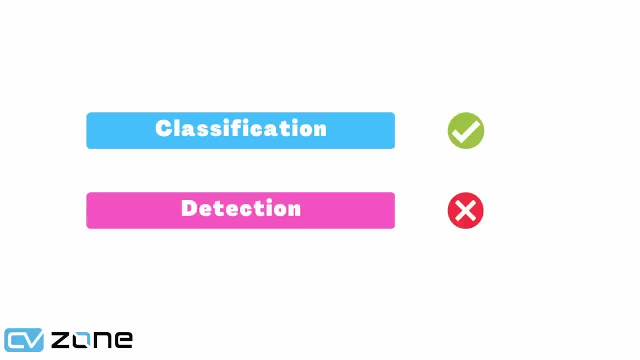 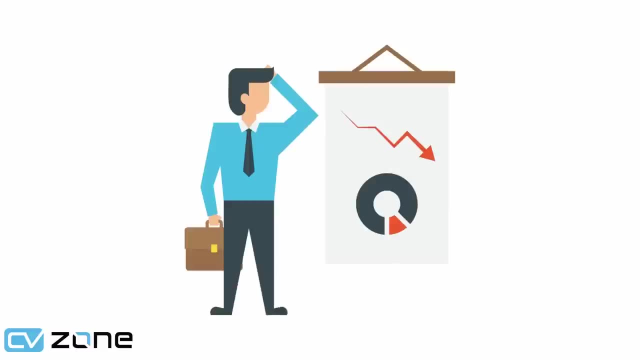 networks when LXNet won the ImageNet Large-Scale Vision Recognition Challenge in 2012.. But this solved a classification problem and not detection. Later, bruise force methods were used to reproduce the CNN models to work as detection models. This was a very inefficient approach. So soon after, 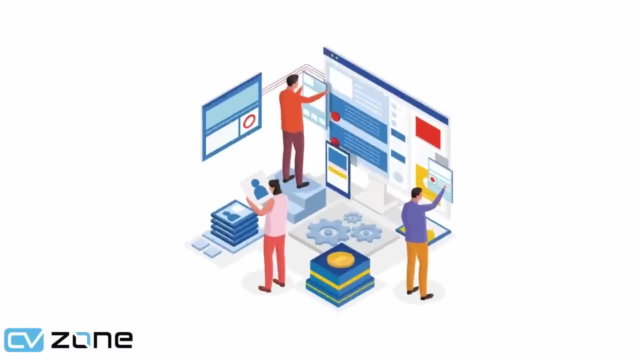 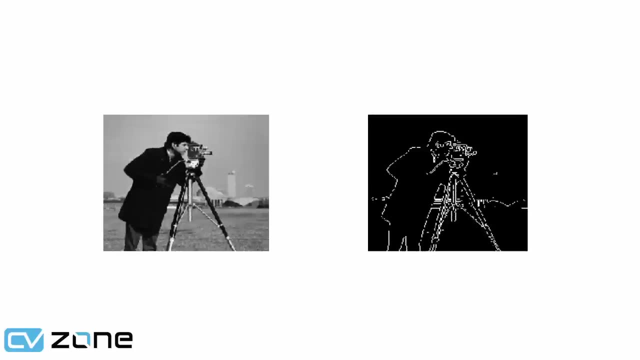 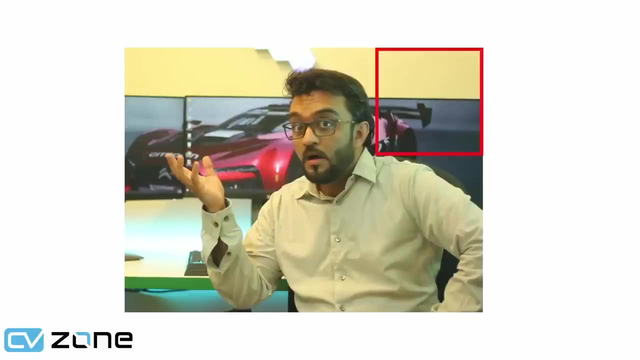 researchers started to develop automated methods for object detection. the first automated object detection algorithm were based on simple features such as edges and corners. the first real object detection was viola jones, developed in 2001.. it used sliding windows to search for har like features which are simply. 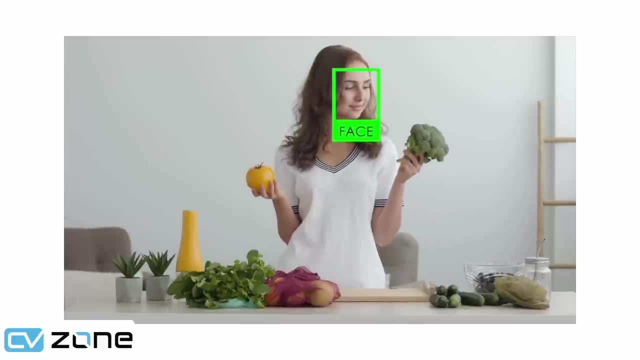 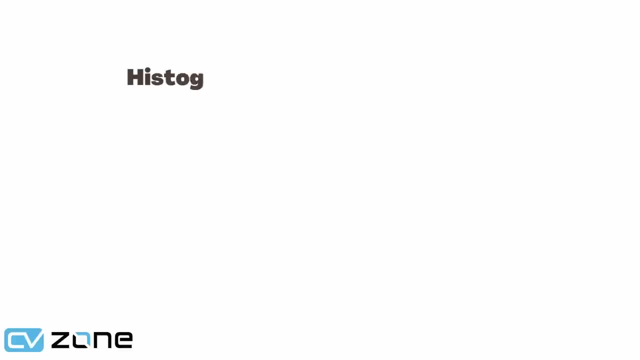 rectangular features. this method became popular since it was real time for the longest time period. this method was used for face detection in smartphones and cameras. the histogram of oriented gradients was another method released in 2005.. this method was used on the shape of the object. it worked by extracting the gradient and orientation. 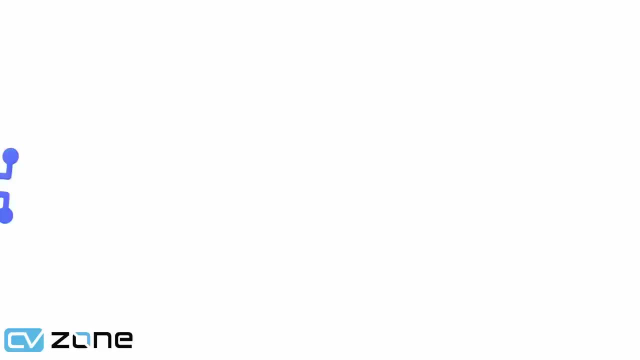 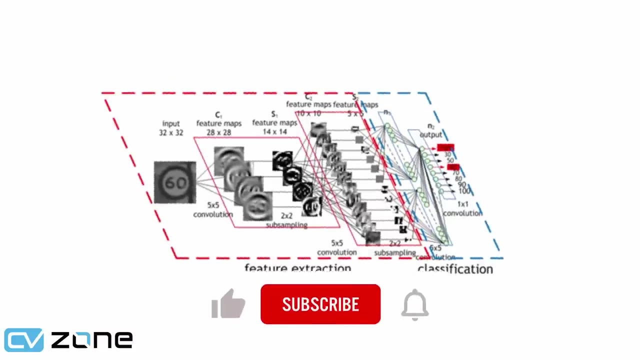 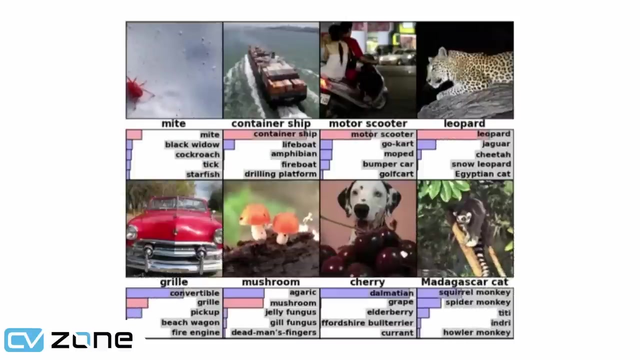 of the edges. this method was mostly used to detect humans in an image. then came the revolution of ai, with neural networks gaining popularity. the true potential was seen with convolutional neural networks when lx net won the image net large-scale vision recognition challenge in 2012. but this 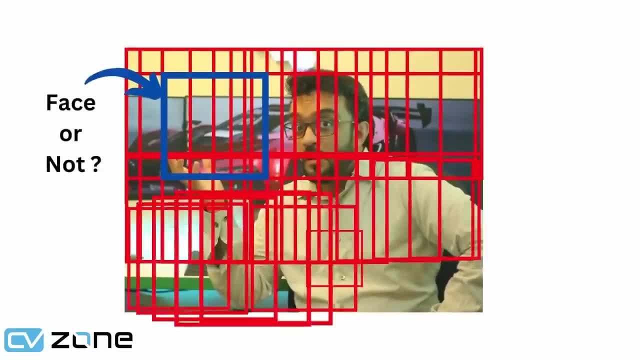 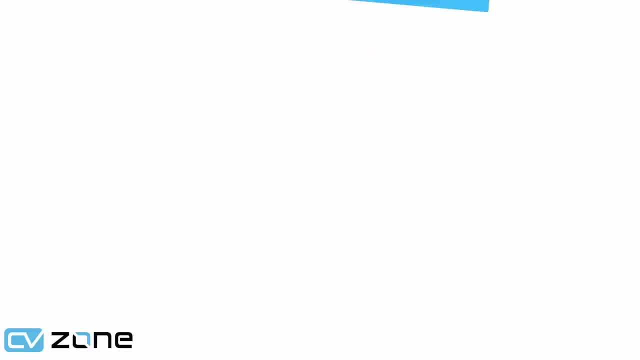 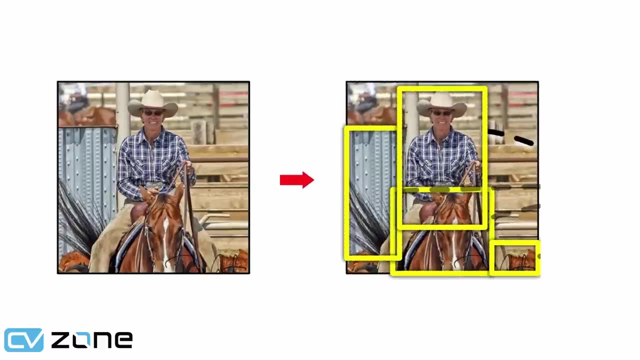 solved a classification problem and not detection. later, bruce force methods were used to repurpose the cnn models to work as detection models. this was a very inefficient approach. so soon after came the rcnn regions with cnn that used selective regions to apply the classifiers. this gave good results, but 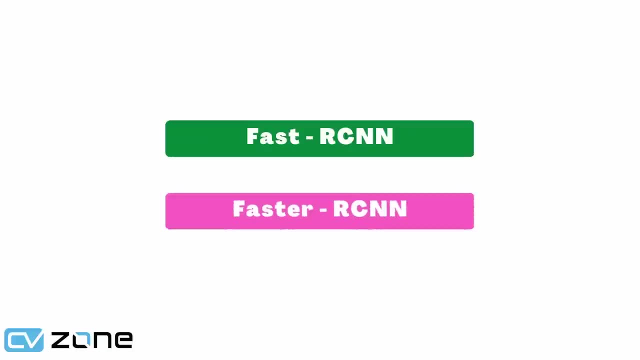 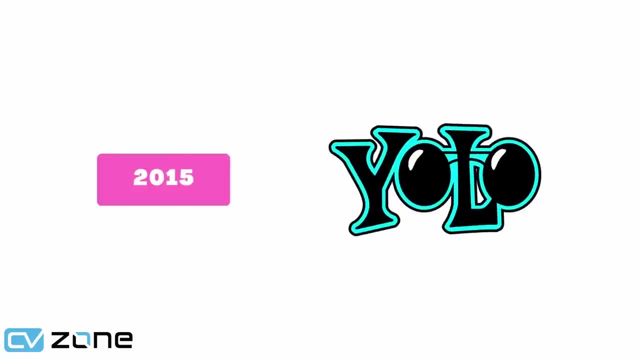 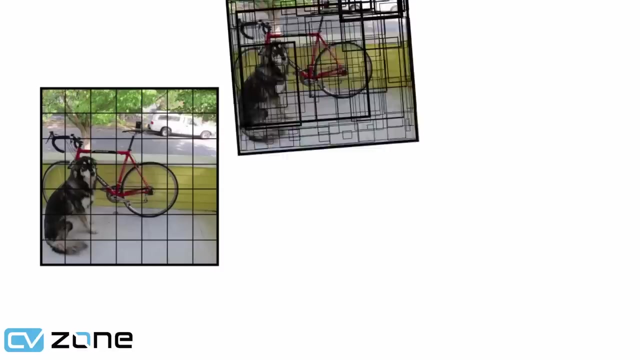 it was slow. so then came the fast rcnn and the foster rcnn, which were faster but still not real time. in 2015 came the breakthrough of yolo. this outperformed all the other models and ran object recognition. this was a different approach as it used single pass of the input image to make 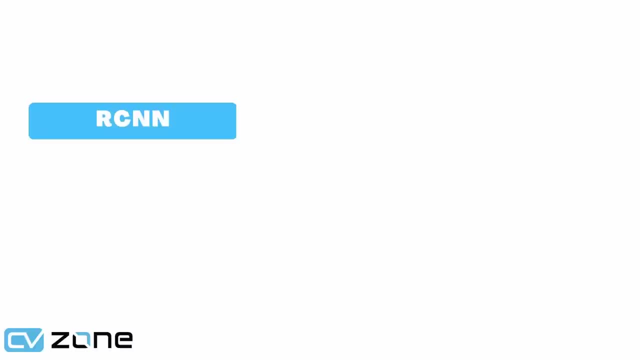 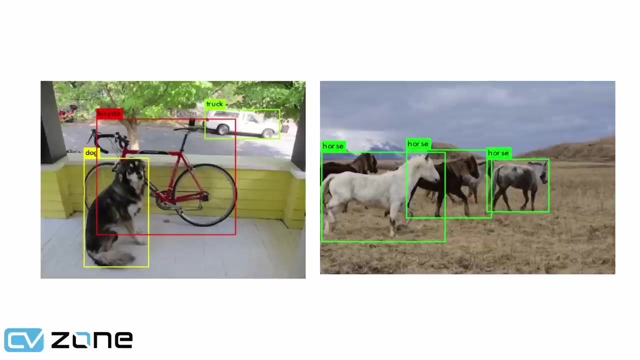 predictions of the objects. methods like rcnn used regional proposal to perform multiple iterations for the same image, while yolo gets it done in a single iteration. this makes yolo more efficient, even though the architecture of yolo is based on convolutional layers similar to its predecessors. 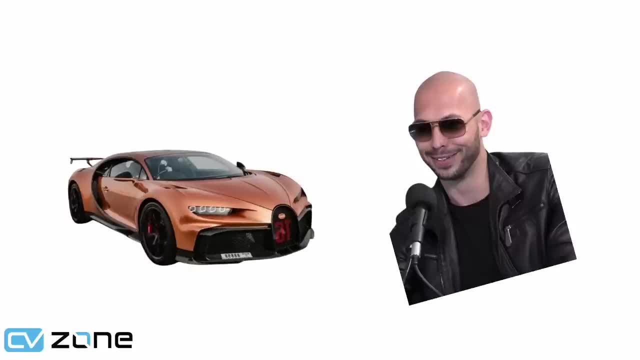 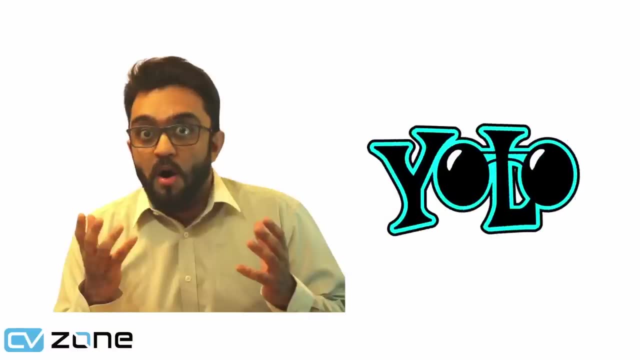 since then, yolo versions have been releasing faster than android dates. five million dollar bugatti's. every time i come back from the toilet i have to check if a newer version of yolo was already released. but don't worry, the change between each iteration is not always very significant. 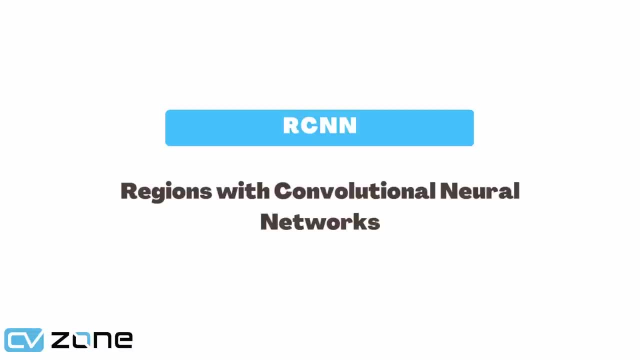 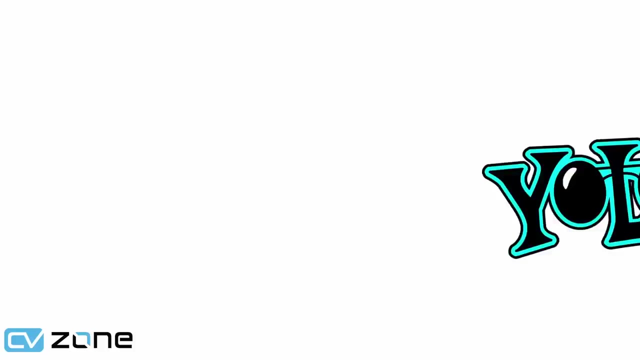 came the RCNN Regions. with CNN That used selective regions to apply the classifiers. This gave good results, but it was slow. So then came the FOSTRCNN and the FOSTRRCNN, which were faster but still not real-time. In 2015 came the breakthrough of YOLO. This outperformed all the 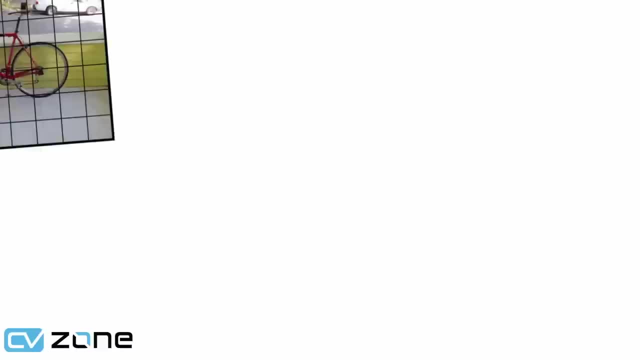 other models and ran object detection in real-time. In 2015,- the breakthrough of YOLO- This outperformed all the other models and ran object detection in real-time. This was a different approach as it used single pass of the input image to make predictions of the objects. 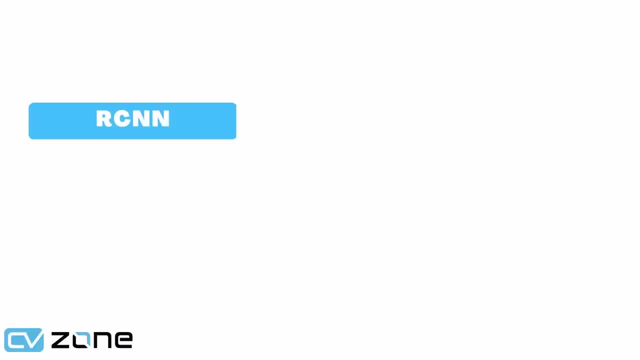 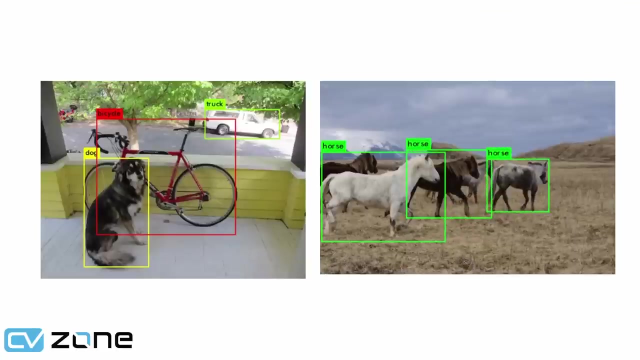 Methods like RCNN used regional proposal to perform multiple iterations for the same image, while YOLO gets it done in a single iteration. This makes YOLO more efficient, even though the architecture of YOLO is based on convolutional layers similar to its predecessors. Since then, 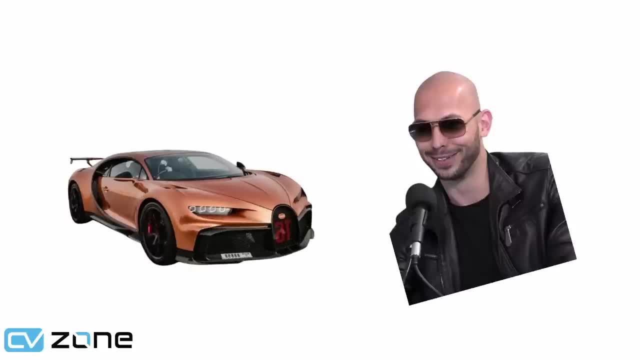 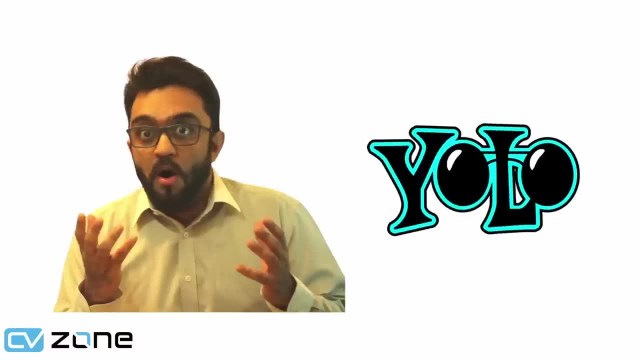 YOLO versions have been releasing faster than Andrew Tate's 5 million YOLO versions have been releasing faster than Andrew Tate's 5 million Bugattis. Every time I come back from the toilet I have to check if a newer version of Yolo was already released. But don't worry the change between each. 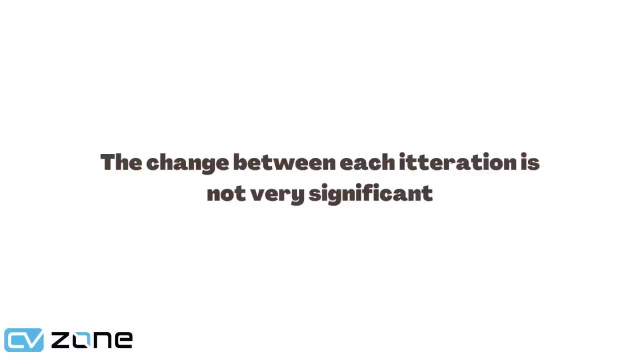 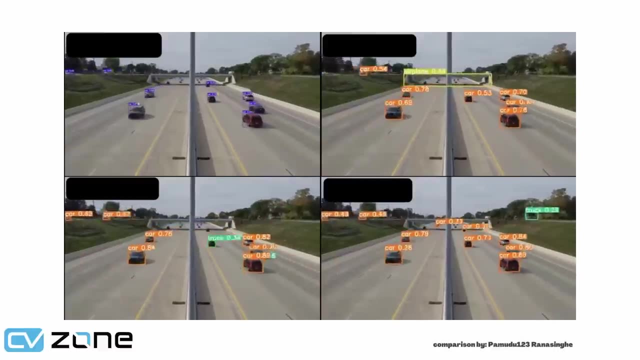 iteration is not always very significant. It's like Apple telling us how their latest iPhone design is completely different from the previous one. If you don't believe me, have a look at these results. Can you guess which is the latest model? Absolutely not. So even if a newer version comes in the previous. 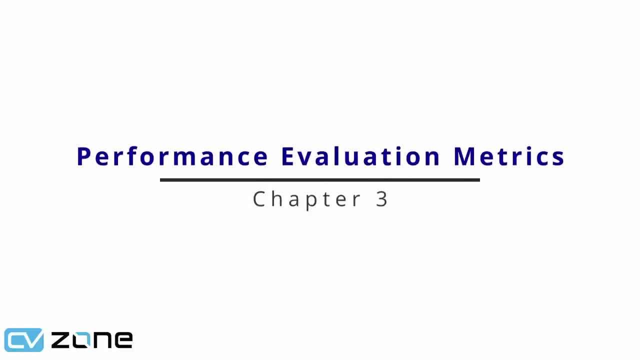 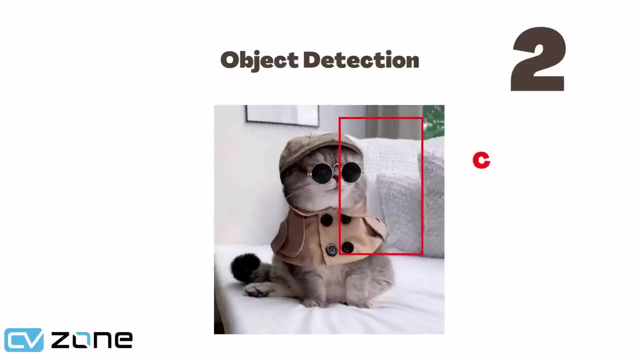 versions don't go out of date. Performance Evaluation Metrics. In order to evaluate our object detection models, there are two main metrics that we need to understand. One is to evaluate how good is the location, and the other is how good is the classification. First is 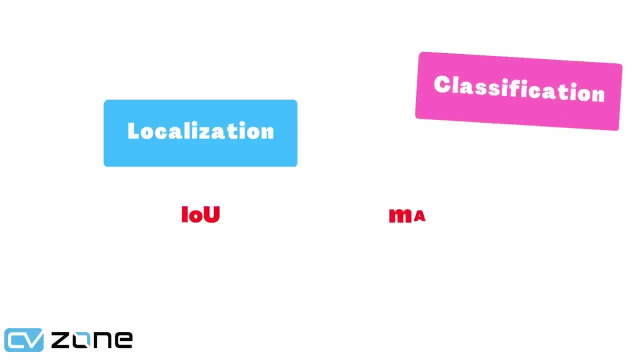 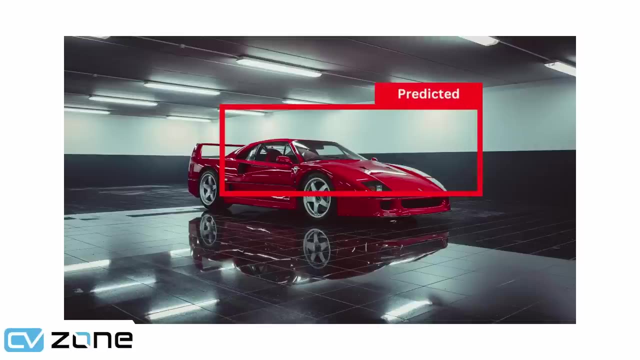 the IOU to measure the localization and the second is the MAP for classification. IOU stands for Intersection Over Union. It tells us how close the predicted bounding box is to the ground truth. It's a value that we can use to measure the location and the classification. It's a 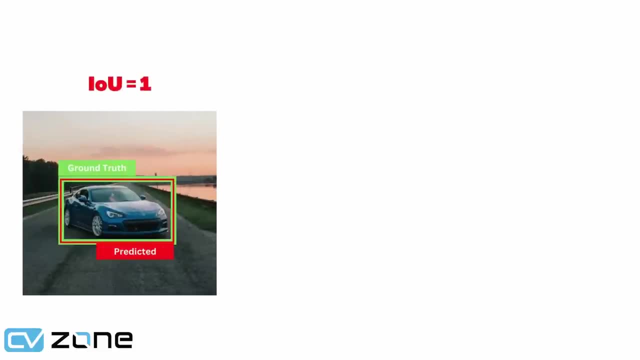 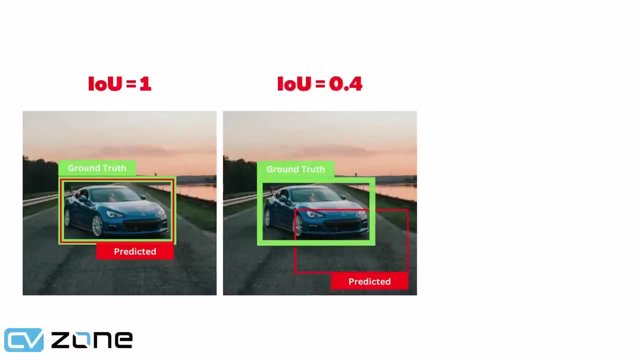 value between 0 and 1.. If the boxes overlap, then it's a perfect detection with an IOU of 1.. If the boxes have some overlap, then the values are between 0 and 1, depending on how much the overlap is. If there is no overlap, then the IOU 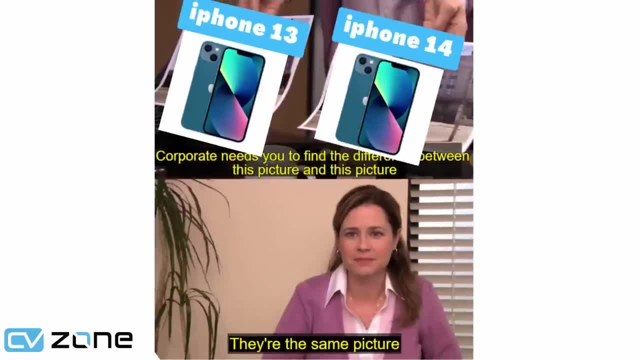 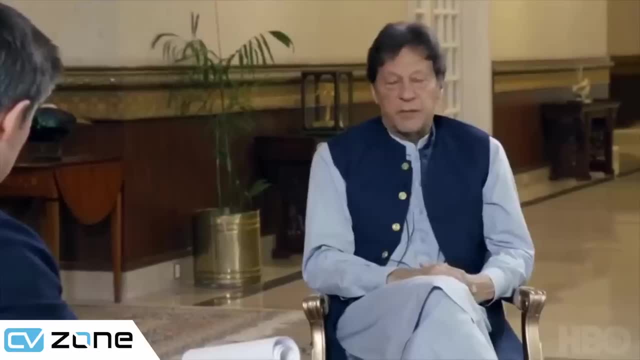 it's like apple telling us how their latest iphone design is completely different from the previous one. if you don't believe me, have a look at these results. can you guess which is the latest model? absolutely not so. even if a newer version comes in, the previous versions don't go out of date. 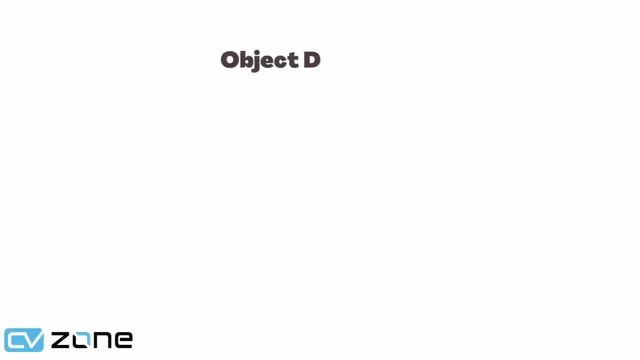 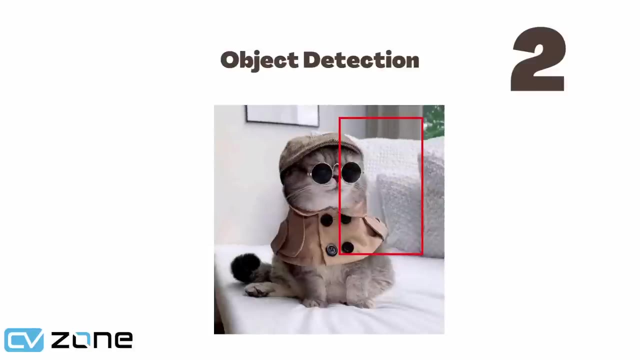 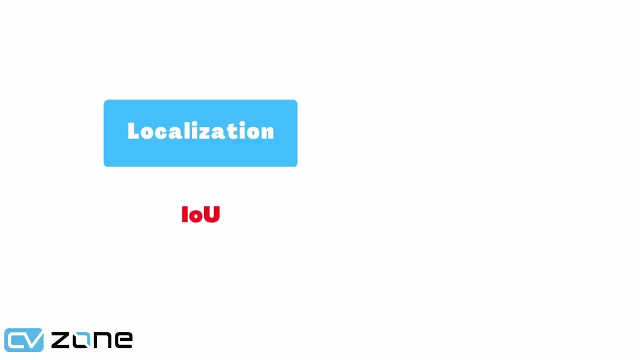 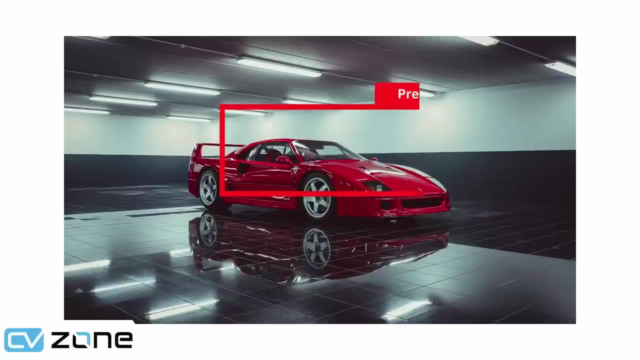 performance evaluation metrics. in order to evaluate our object detection models, there are two main metrics that we need to understand. one is to evaluate how good is the location and the other is how good is the classification. first is the iou to measure the localization and the second is the map for classification. iou stands for intersection over union. it tells us how close. 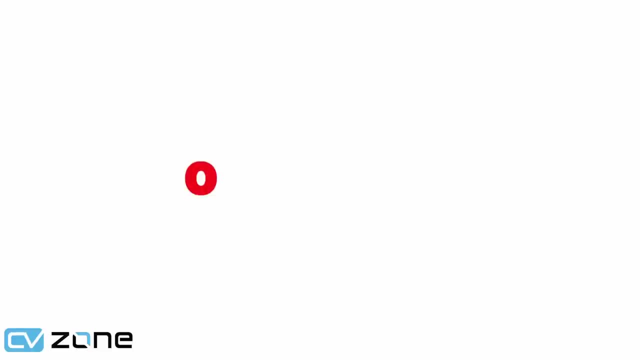 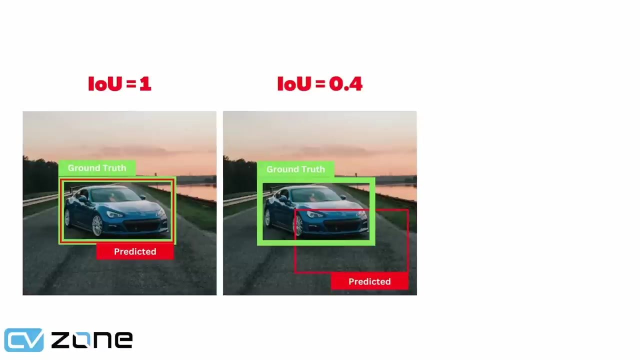 the predicted bounding box is to the ground truth. it's a value bounding box between 0 and 1.. if the boxes overlap, then it's a perfect detection with an iou of 1.. if the boxes have some overlap, then the values are between 0 and 1, depending on how much the overlap is. 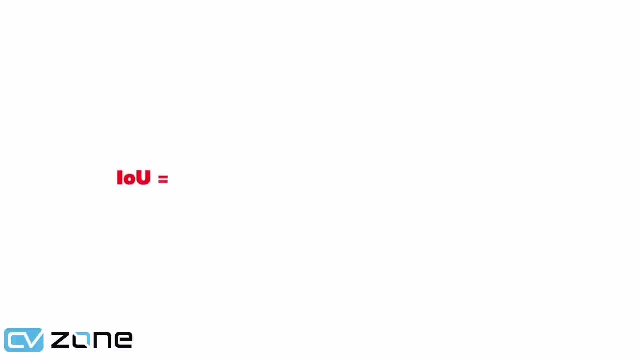 if there is no overlap, then the iou is 0.. the value of iou is calculated by taking the ratio between the area of the intersection and the area of the union of bounding boxes. in order to understand average precision, we need to know confusion matrix. 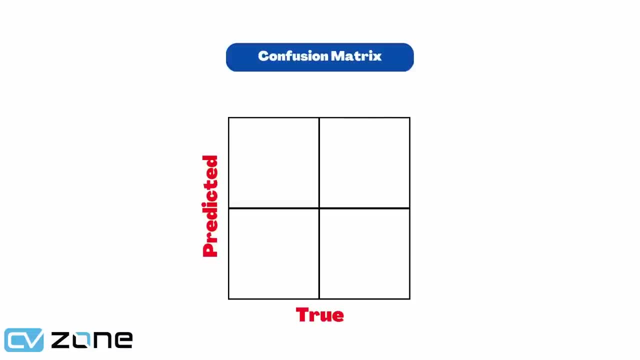 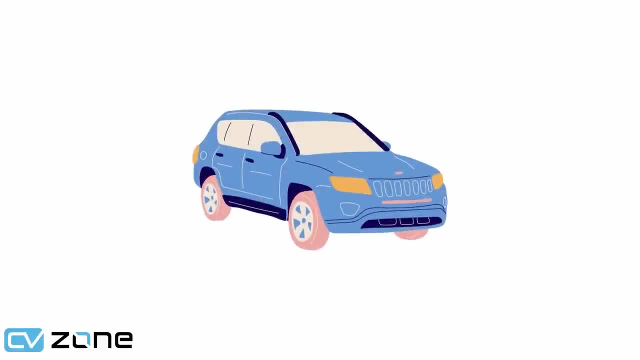 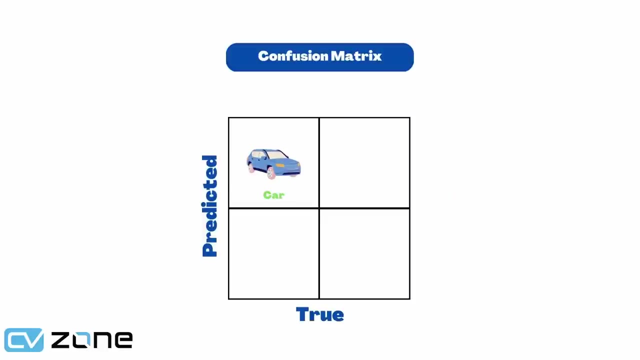 precision and recall confusion. matrix is a simple table that consists of actual classes on one side and the predicted classes on the other. let's have a look at an example of a car classifier. in the first cell, the actual class is of a car and the model predicted it as a car. 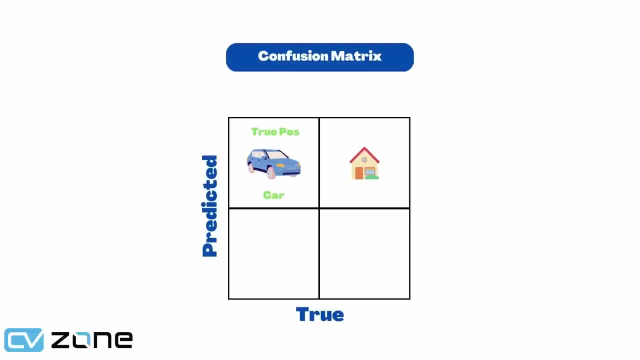 so it's a true positive. in the second cell, the actual class is a house, but the model predicted it as a car, so it's a false positive. in the third cell, the actual class is a car, but the model predicted it as not a car, so it's a false negative. in the last: 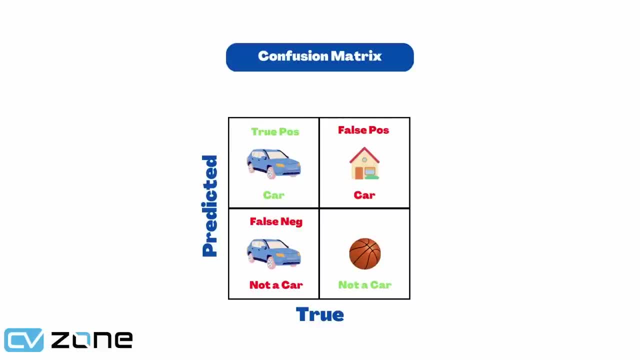 cell. the actual class is ball and the model predicted it as not a car, so it's a true negative. this value corresponds to not predicting a bounding box and is usually the background, so it is not used in the matrix calculations. using these values we can calculate the precision and 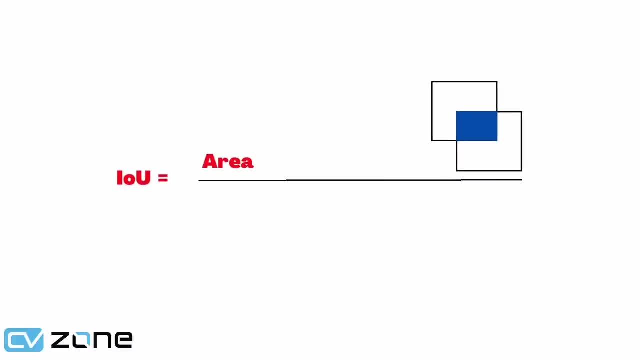 is 0.. The value of IOU is calculated by taking the ratio between the area of the intersection and the area of the union of bounding boxes. In order to understand average precision, we need to know confusion, Confusion math whose segundo cell has the name midpoint of H. 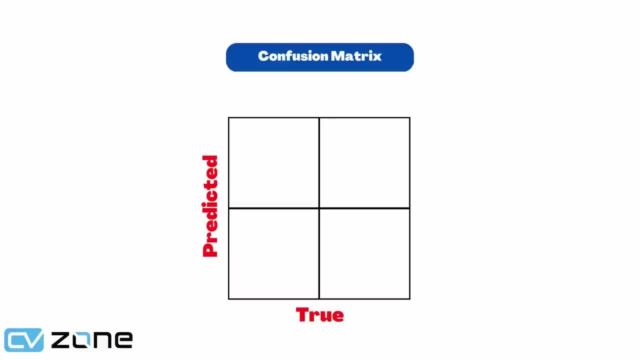 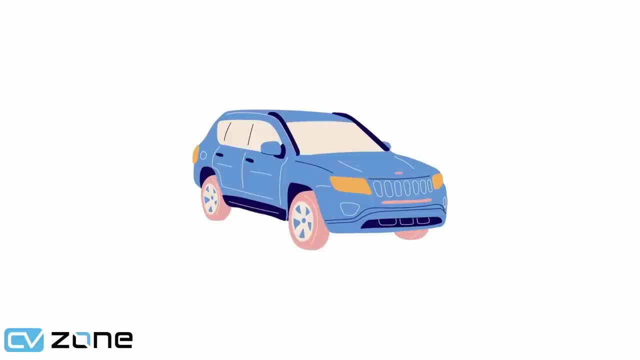 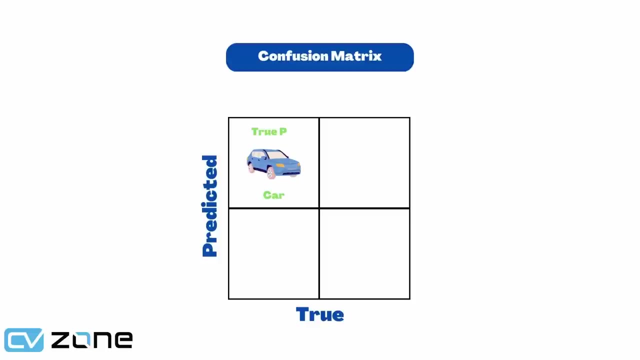 is called a relationship, so it worrying through an subsequent data. It's a proof of information The herself tell usовit is true, positive. It's a predictative tag dance between a random goal and an expectии. Actual is terms Tá. 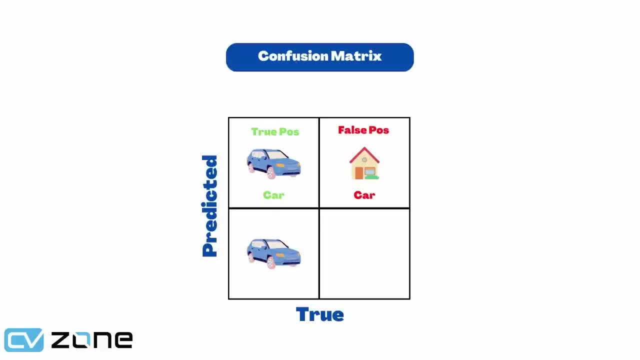 res are from models, so they are random�onia. In order to predict the dog, we need to know cell. the actual class is a car, but the model predicted it as not a car, so it's a false negative. in the last cell, the actual class is ball and the model 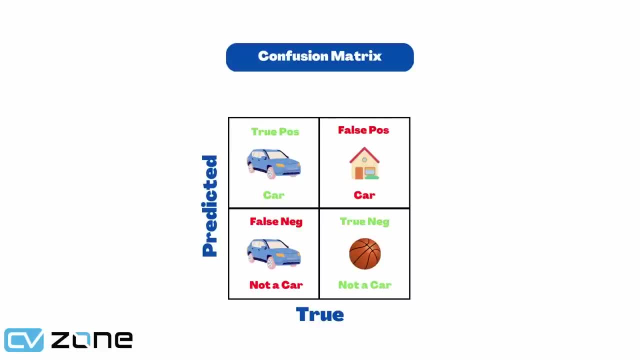 predicted it as not a car, so it's a true negative. this value corresponds to not predicting a bounding box and is usually the background, so it is not used in the matrix calculations. using these values we can calculate the precision and the recall. precision is the total positives out of the total positive predictions. 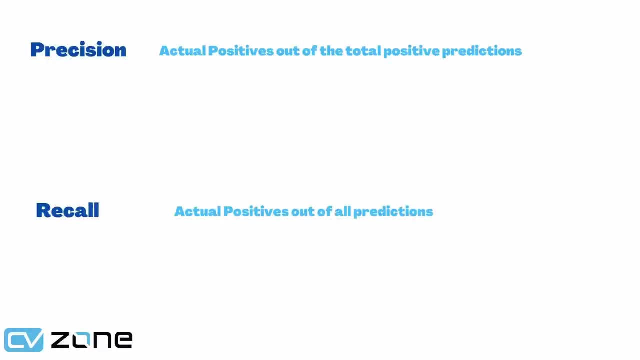 recall is the actual positives out of all predictions. in mathematical terms, precision is true positive divided by true positive plus false positives. recall is true positive divided by true positive plus false negatives. since both matrix provide us valuable information, we combine them to one called the precision average. this is the area under the precision recall curve. the precision recall curve. 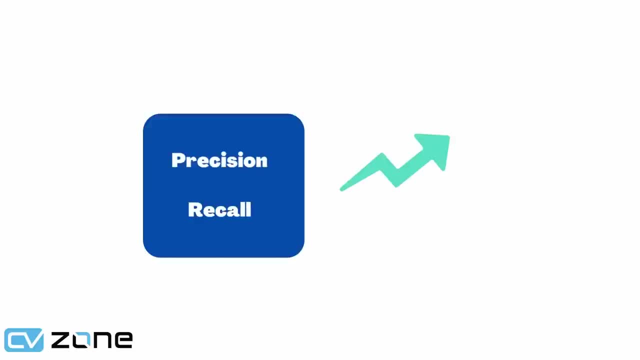 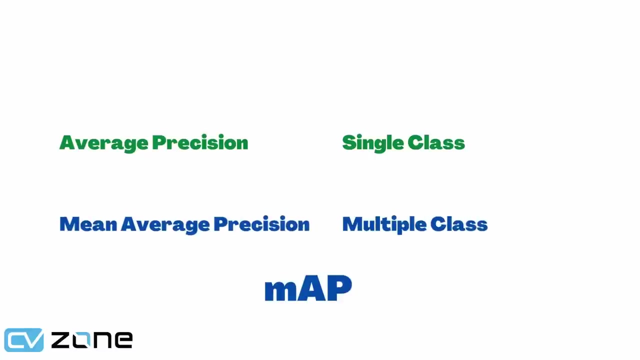 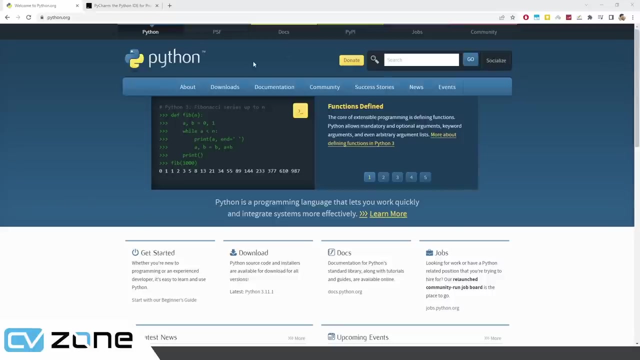 maximizes the effects of both the matrix and give us a better idea of the overall accuracy of the model. this average precision is of a single class. if we have multiple classes, then the mean of these precision values is the mean average precision, also known as MAP. so the first thing we will do is to download Python. 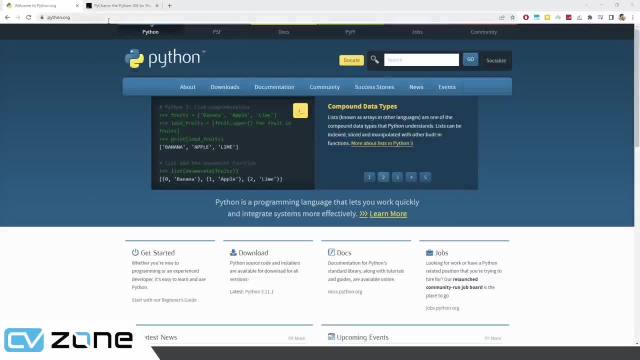 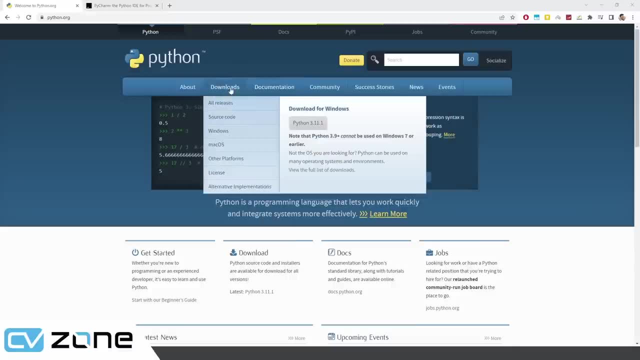 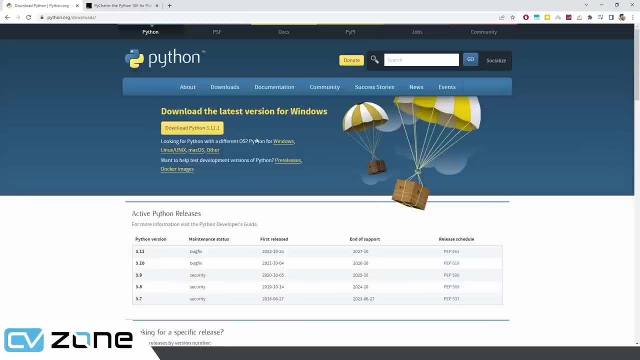 and to do that we can go to pythonorg. so we will simply go to downloads and here you can see, you can download the latest version. but that is not recommended because it might have some errors or it might need some bug fixes. so we'll go to all releases and here we'll go down and you can see Python 3.11. 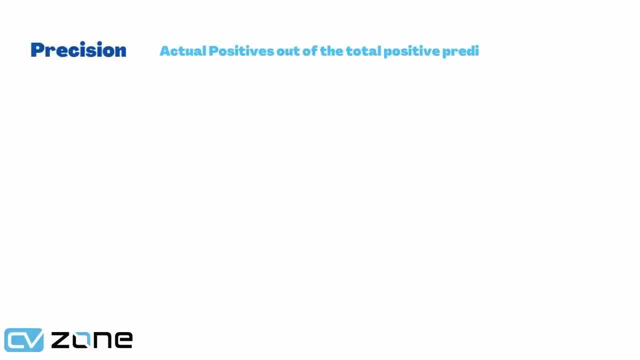 the recall. precision is the total positives out of the total positive predictions. recall is the actual positives out of all predictions. in mathematical terms, precision is true positive divided by true positive plus false positives. recall is true positive divided by true positive plus false negatives, since both matrix provide us valuable information. 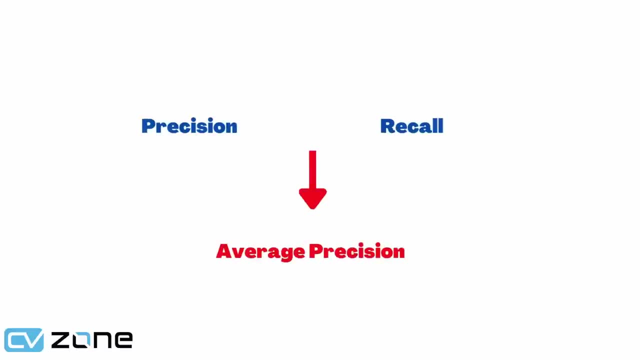 we combine them to one called the precision average. this is the area under the precision recall curve. the precision recall curve maximizes the effects of both the matrix and Give us a better idea of the overall accuracy of the model. This average precision is of a single class. if we have multiple classes, 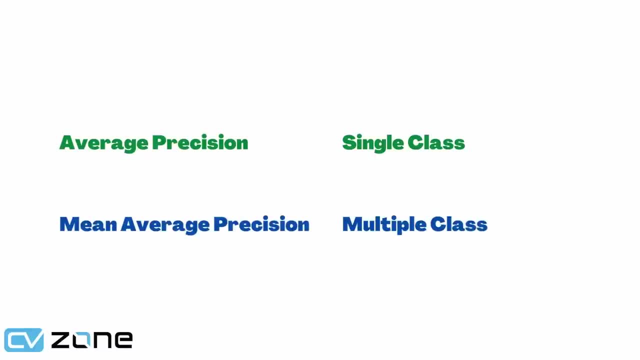 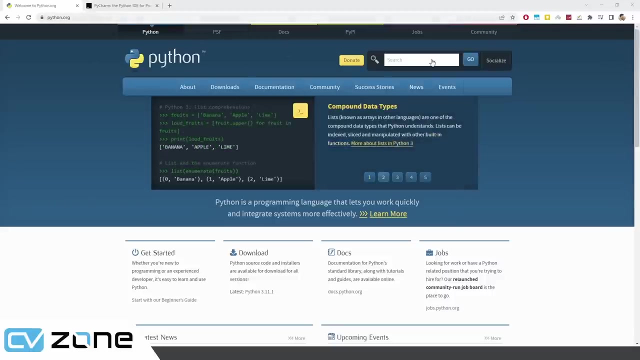 Then the mean of these precision values is the mean average precision, also known as MAP. So the first thing we will do is to download Python, and to do that we can go to pythonorg. So we will simply go to downloads and here you can see, you can download the latest version. But that is not recommended because it might have some errors or it might need some bug fixes. So we'll go to all releases and here we'll go down and you can see. Python 3.11 Will have support till 27. Python 3.10 will have till 26. 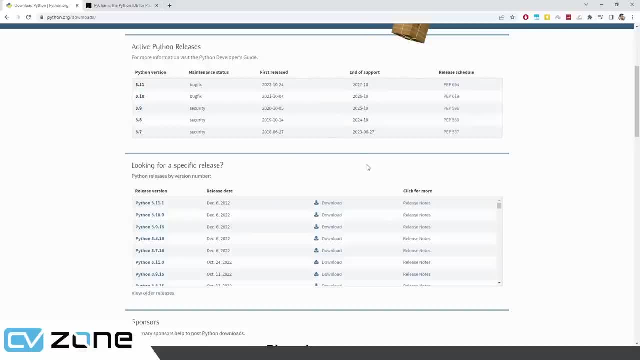 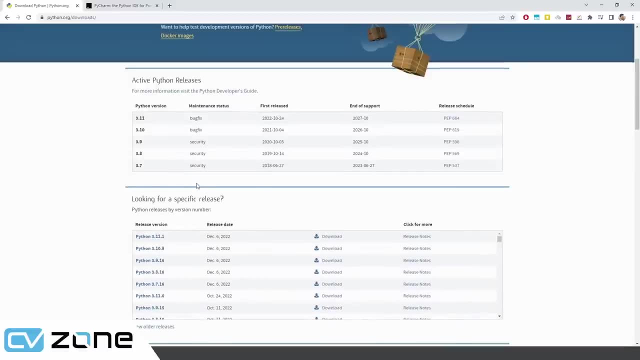 So you can see the information here. So this is basically the long-term support. So here in the release version I would suggest to go: Don't go for the latest one, go for the one that is one below the latest one. So, for example, here you can see three points, ten, point nine, so we can download this. we can simply press on download and 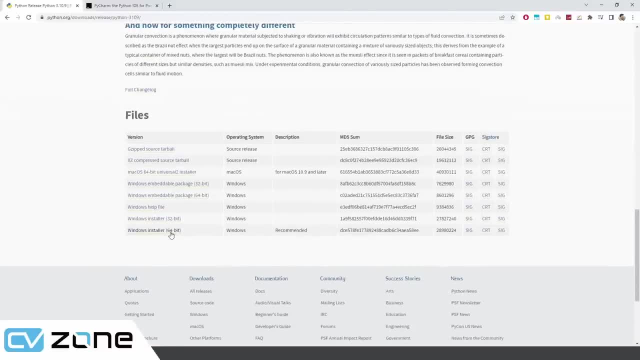 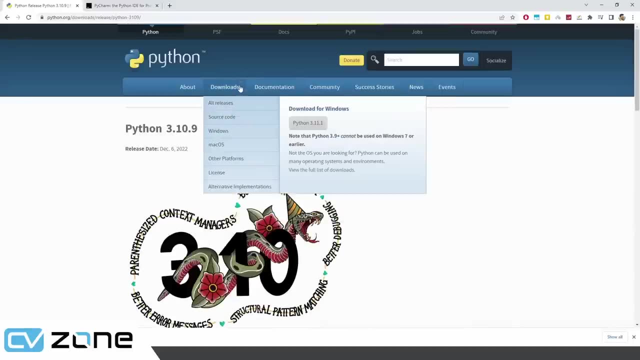 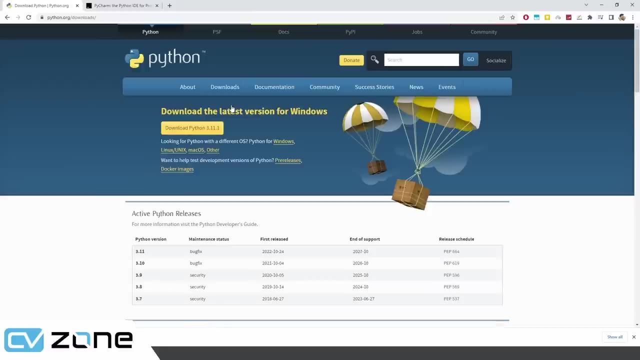 Here you will go to Windows 64-bit and you will click on that so it will start the download. Now you can have multiple versions of Python as well, So you can have the same project running on different Python versions, So you can see which one is more stable, which one gives you better results. 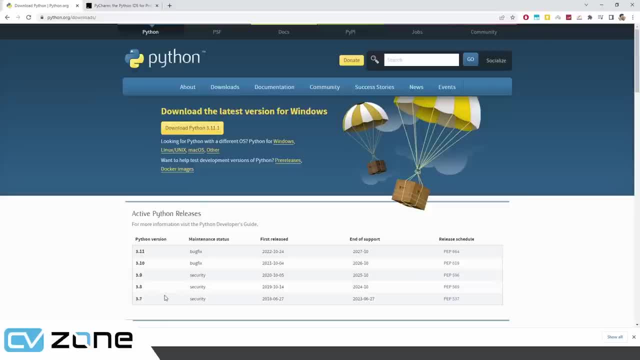 So I will show you how you can do that, because We have Python 3.7.6, Which I have been using for the longest time period, and I will also show you how you can use python 3.10 in this case. so we will be using python 3.10, but if we have to, will have support till 27. Python 3.10 will have till 26. so you can see the information here. so this is basically the long-term support. so here in the release version I would suggest to go. don't go for the latest one, go for. 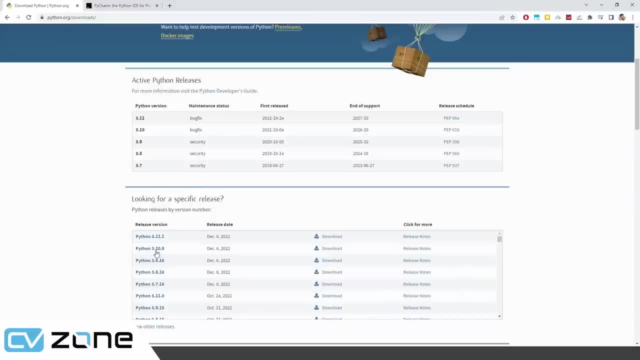 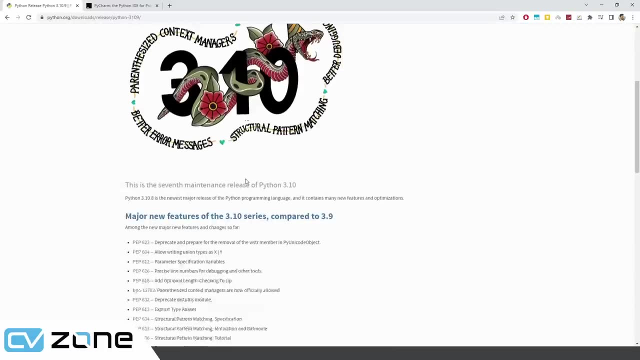 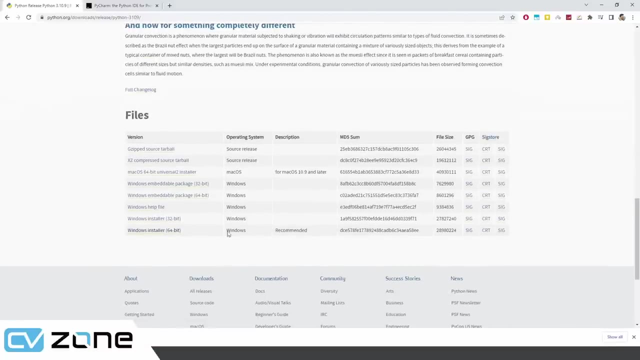 the one that is one below the latest one. so, for example, here you can see 3.10.9, so we can download this. we can simply press on download and here you will go to Windows 64-bit and you will click on that so it will start the download now. 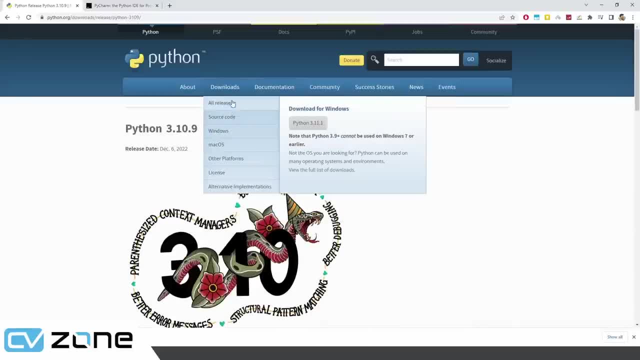 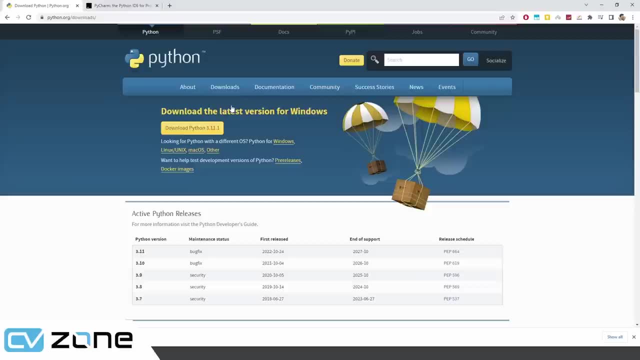 you can have multiple versions of python as well, so you can have the same project running on different python versions so you can see which one is more stable, which one gives you better results. so I will show you how you can do that, because I already have python 3.7.6 which I have been using for the 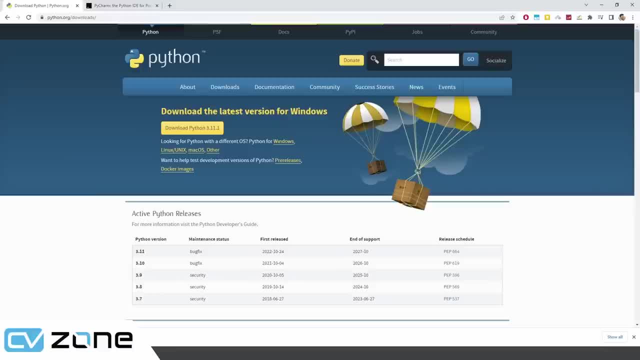 longest time period, and I will also show you how you can use Python 3.10 in this case. so we will be using Python 3.10, but if we have to downgrade, I will you how you can do that. or if we had to upgrade, i will show you how to do that as well. so what? 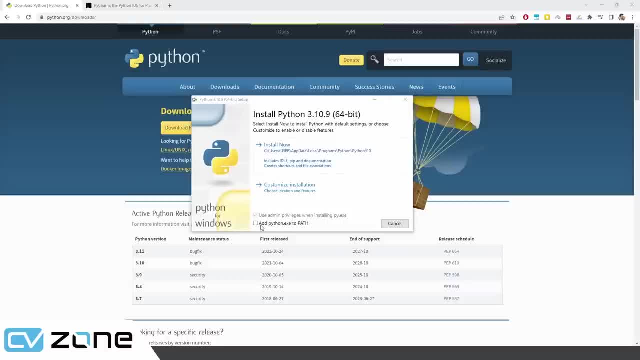 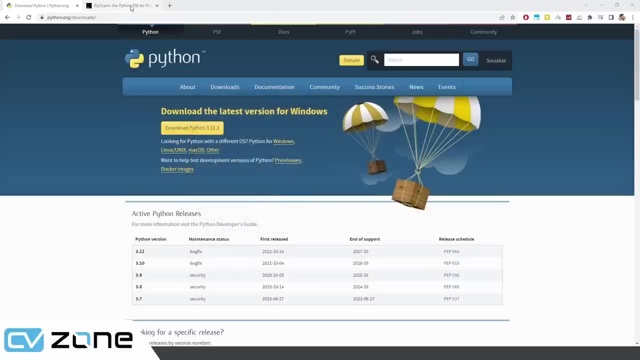 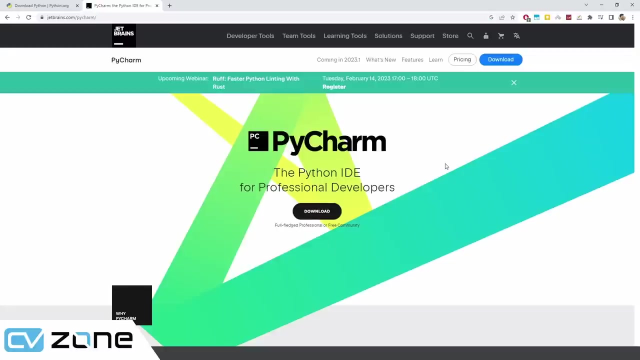 you will do is you will click on python. so here, make sure that you add pythonexe to the path- and you will click on install now. okay, so the setup is done and we can close. now we will go to pycharm, which is our ide. now, if you are not familiar with ide, it stands for integrated development environment. it's basically: 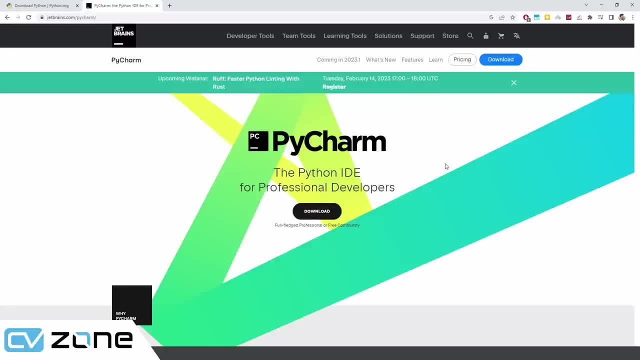 a notepad where you can write code. but it will help you out to write the code, it will tell you where the problems are, how to fix the bugs and all that. so what you will do is you will go to pycharm- so this is jetbrainscom, pycharm- and you will go to download and in the downloads, 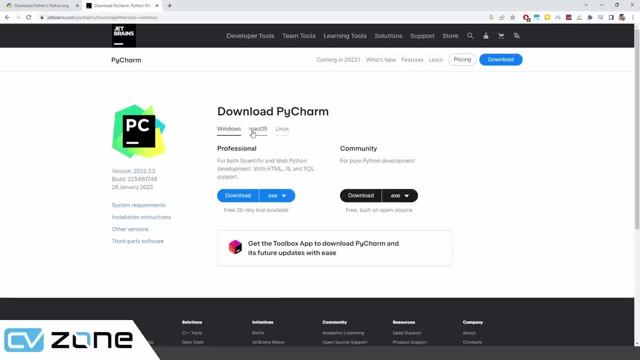 there is a professional version and there's a community version, so you have from mac os and linux as well. so we will be working on windows, so we will download for that. so for the community version, you can simply hit download, because it is free and it is more than enough. 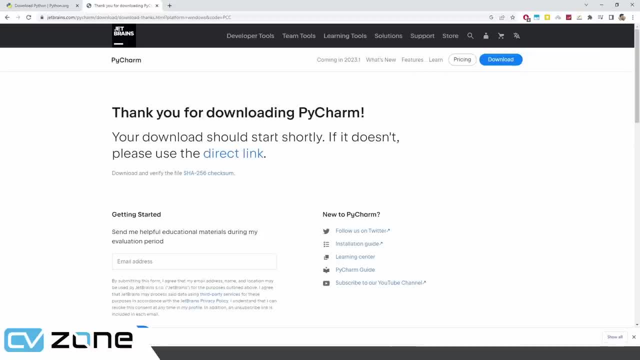 for what we need. so now the download has started and we will wait for it to finish. so now the download is complete and we will hit on pycharm community, we'll click on next next and we will associatepy files with that. we'll add bin folder to the paths and pycharm community edition. 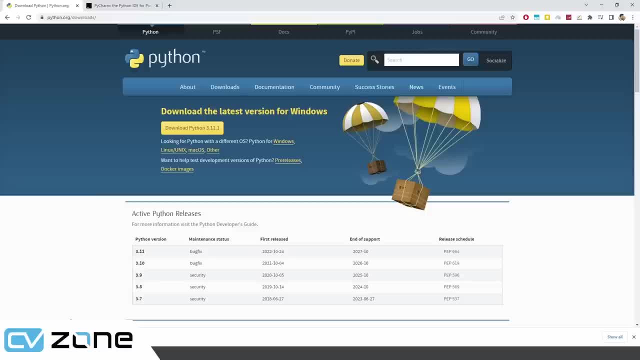 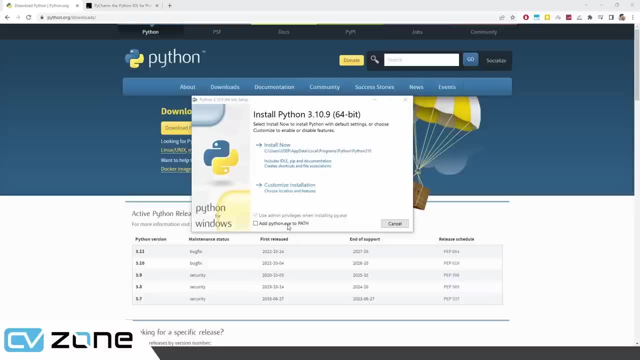 downgrade. I would you how you can do that. or if we had to upgrade, i will show you how to do that as well. so what you will do is you will click on python. so here, make sure that you add pythonexe to the path, and you will click on install now. 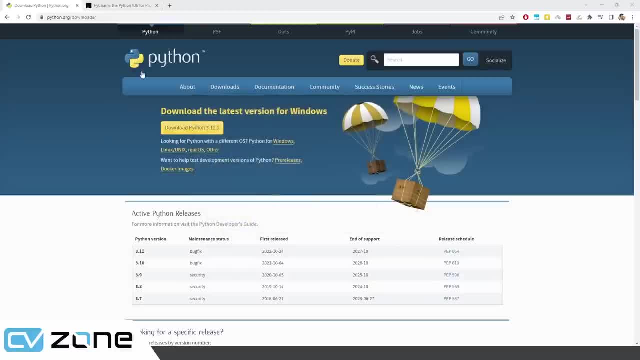 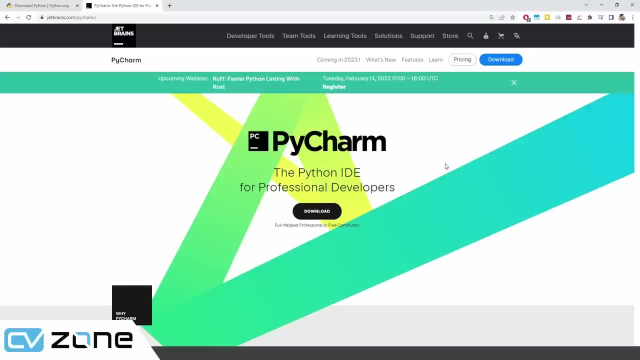 okay, so the setup is done and we can close. now we will go to pycharm, which is our ide. now, if you are not familiar with ide, it stands for integrated development environment. it's basically a notepad where you can write code, but it will help you out to write the code. it will tell you. 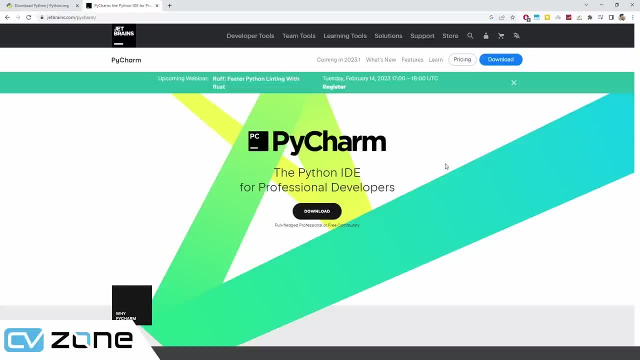 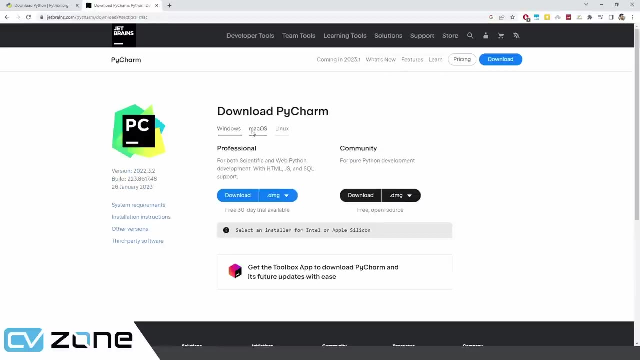 where the problems are, how to fix the bugs, and all that. so what you will do is you will go to pycharm- so this is jetbrainscom, pycharm- and you will go to download, and in the downloads there is a professional version and there's a community version. so you have from. 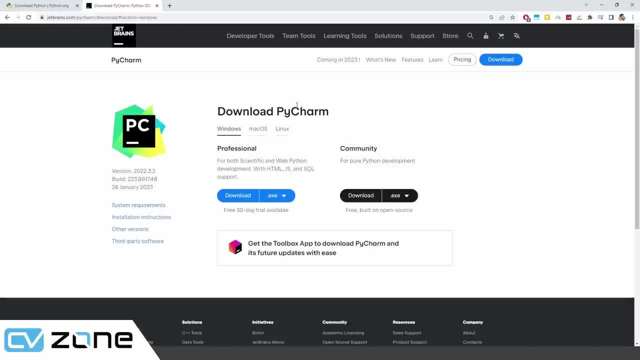 mac os and linux as well. so we will be working on windows, so we will download for that. so for the community version, you can simply hit download, because it is free and it is more than enough for what we need. so now the download has started and we will wait for it to finish. 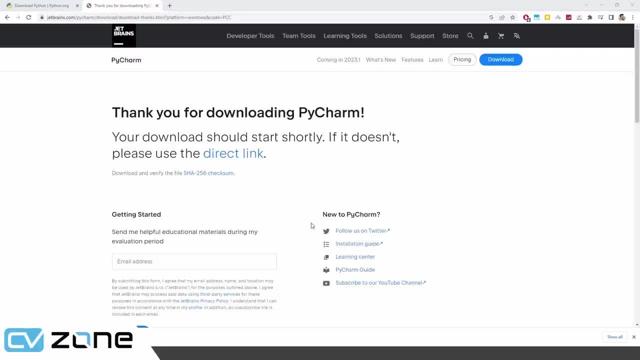 so now the download is complete and we will hit on pycharm community, we'll click on next, next and we will associatepy files with that. we'll add bin folder to the paths and pycharm community edition will create the desktop icon as well. install. then we are going to restart our computer and hit finish and then we are going to open up. 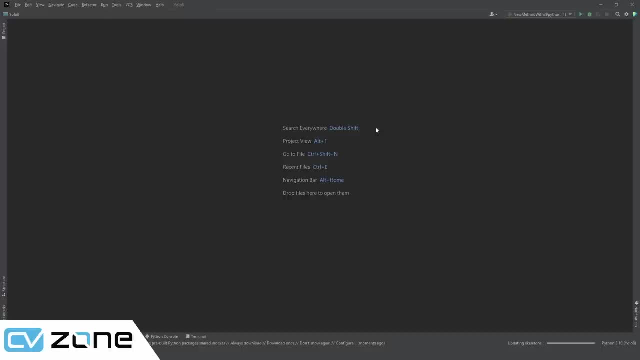 pycharm. so this is not the first time i am installing pycharm, so it has some memory of what i've been doing, so it has some of the default parameters. so i'm going to open up pycharm and i'm going to ask what it's created by the very first time here. so that's what we need to build and 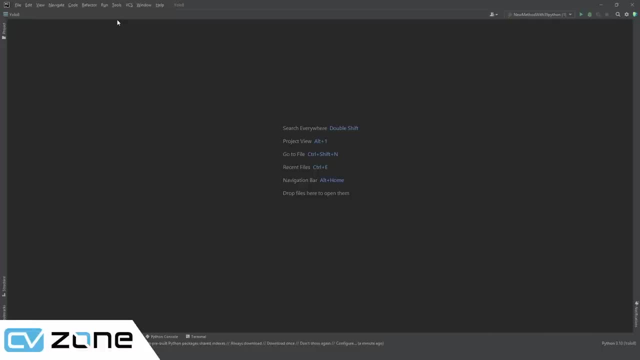 we are going to do is create this Yamaha system. this is that, the scale from file's. we have a package, so let's call it drive. i am going to use the, the file's file summary, and we are going to add some projects here, so here we can decide. each one click on. 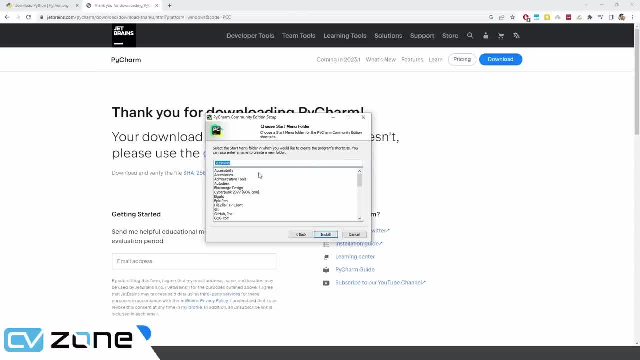 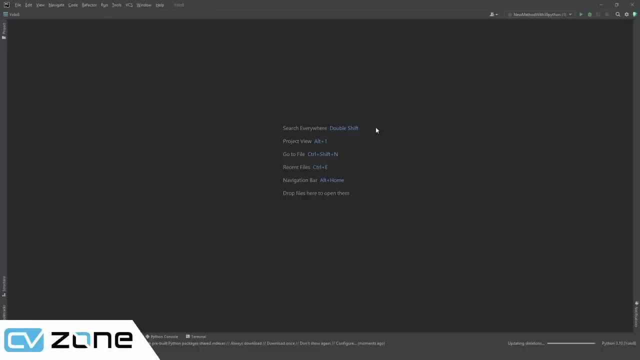 will create the desktop icon as well. install. then we are going to restart our computer and hit finish, and then we are going to open up pycharm. so this is not the first time i am installing pycharm, so it has some memory of what i've been doing, so it has some of the default parameters. so i'm going to open up pycharm and i'm 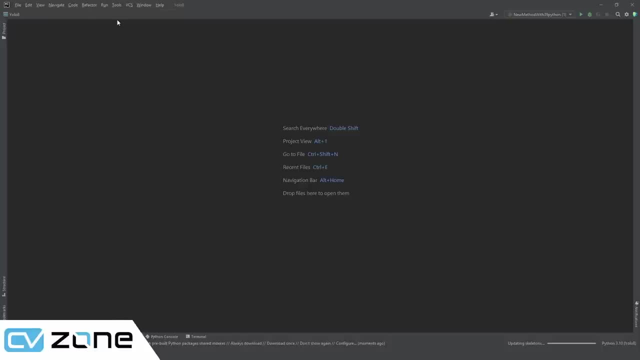 going to assign the default bitrate and you have a block file, which i have because i'm using the iste initial, but of course that's not my main project and i think it's not going to be a hard project and as stuff is elementary files, i should actually have a bit more manual work. 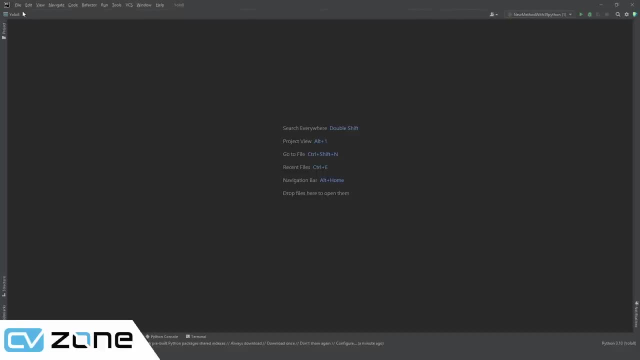 on that. so this is an environment possible so you can withiders, but you can need something different. so i would love to cover performance setting for it like a lot of vmятся, and so you do have time or want to do some more work, but if you do not want to do that, you can use this. 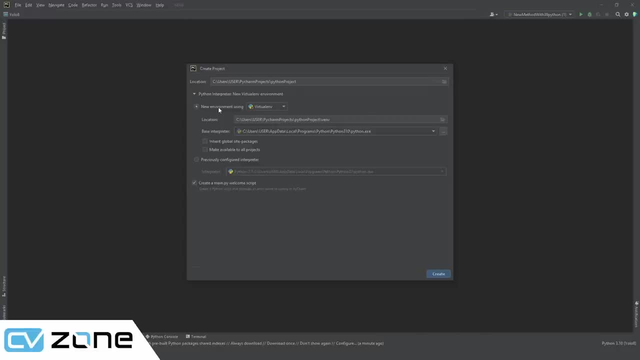 suite because there is so many infrastructure that can be set up and you can do many things. so here is the säger talks aboutfia style. so you will click on file and you want to set up a map so you might read a few python and you copy that, basically, and you create a virtual environment that is separate to 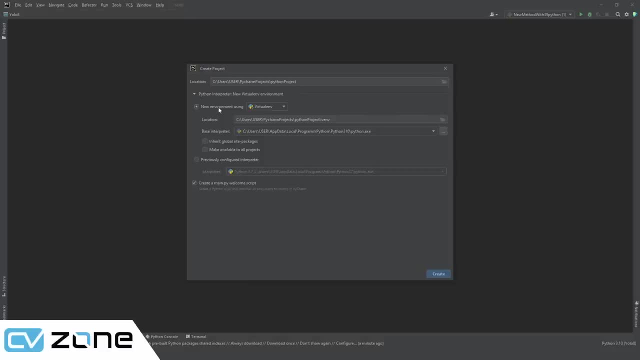 everything else. so this project will have its own environment and whatever you install will be installed in this environment. so this is based on a specific version of python. so here the base interpreter you have to mention. so right now the base interpreter is python 3.1.0, so you can also. 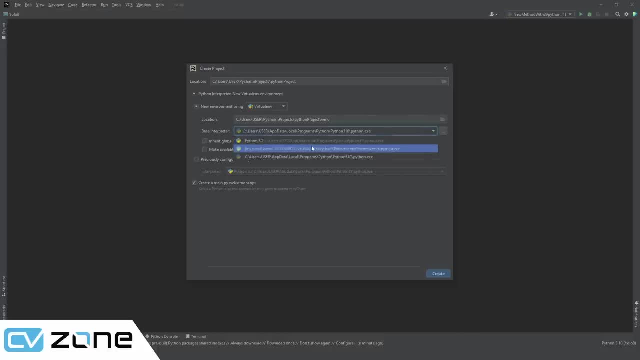 have python, for example, 3.7. so i have these two, python 3.7 and python 3.10, so i can choose between these two. so for now, i'm going to choose, for example, this one. so what i will do is, when i'm 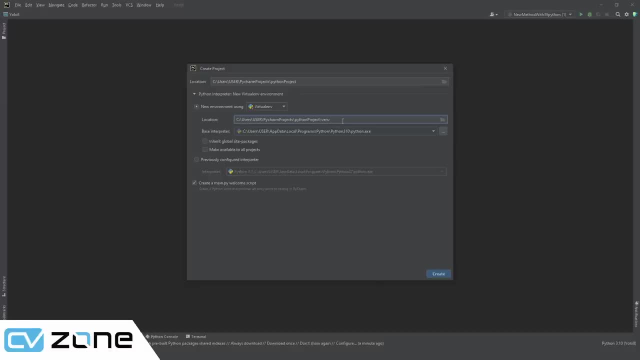 creating the environment. i'm putting down the name and i can write environments and i can write 3.1.0, so this has a version as well. so here we'll just name it python project and we are going to hit create. so we will use the same window to create this project. and here we 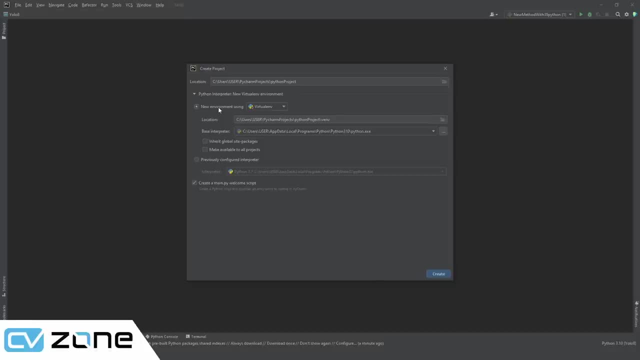 the actual python and you copy that, basically, and you create a virtual environment that is separate to everything else. so this project will have its own environment and whatever you install will be installed in this environment. so this is based on a specific version of python. so here the base interpreter you have to mention. so right now the base interpreter is python. 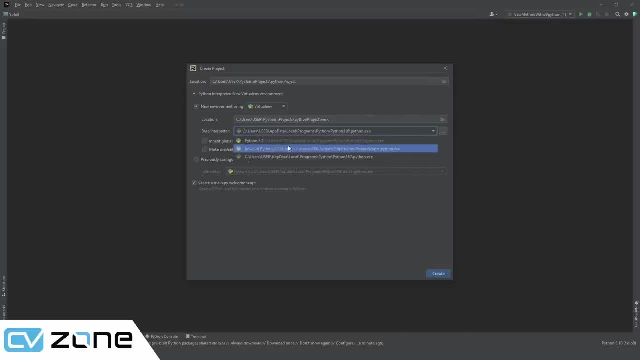 3.1.0, so you can also have python, for example, 3.7. so i have these two, python 3.7 and python 3.10, so i can choose between these two. so for now, i'm going to choose, for example, this one: 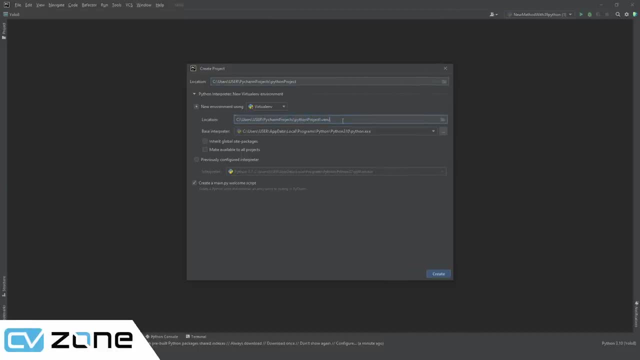 so what i will do is, when i'm creating the environment, i'm putting down the name and i can write environments and i can write 310. so this has a version as well. so here we'll just name it python project and we are going to hit create. 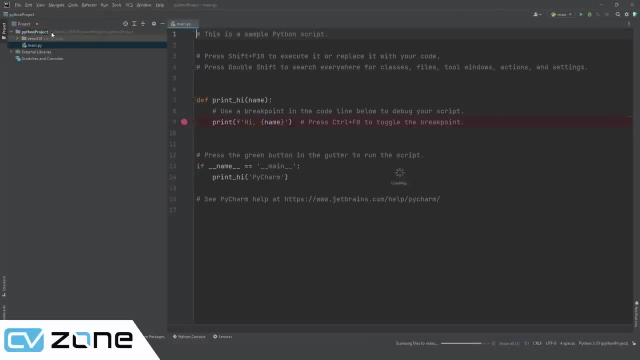 so we will use the same window to create this project, and here we have our python project, and that is created with the main file and you can see the virtual environment 3.10 has been created. so what i can do is i can remove all this and i can simply write: print: hello world. so let's go. 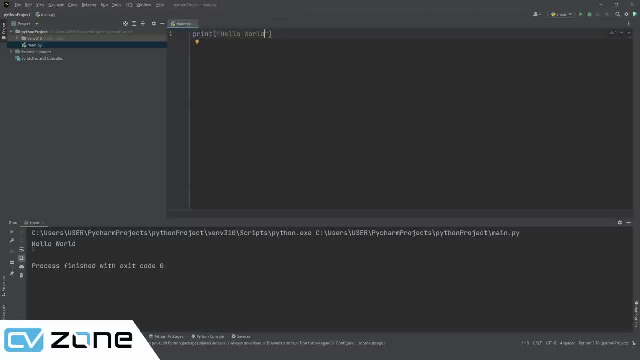 and right click and we are going to run main and this will give us hello world. so this is running python 3.10. how do i know this is because you can see, here we have python 3.10, we don't have python 3.7. so what we will do is we are going to go to file and any package that we 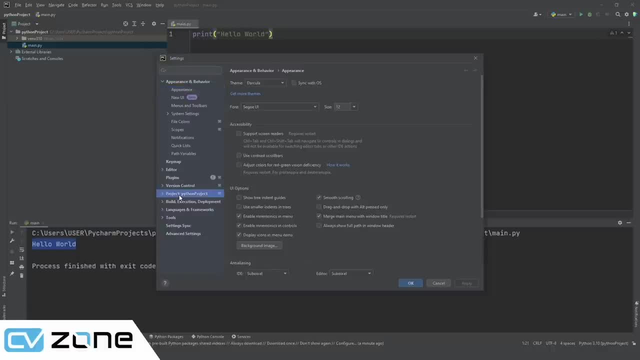 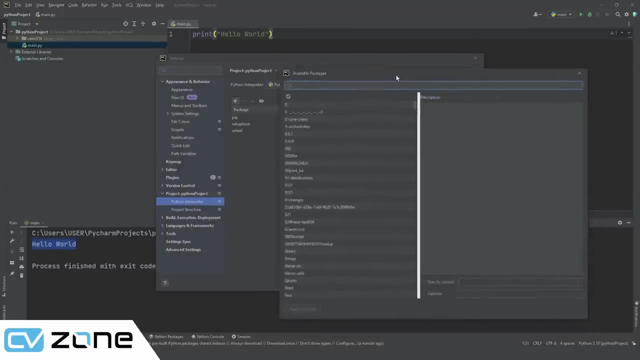 want to install, we can go to settings, and then we will go to project, python project and we'll go to interpreter, and here we can add any package that we want, whether it's opencv, whether it's cv zone, whether it's ultralytics, whatever it is, you can install here. so, for example, we can go ahead and 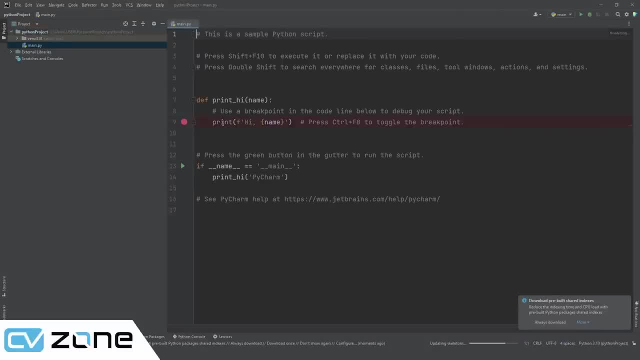 have our python project and that is created with the main file and you can see the virtual environment 3.10 has been created. so what i can do is i can remove all this and i can simply write: print: hello world. so let's go ahead and right click and we are going to run main and this will 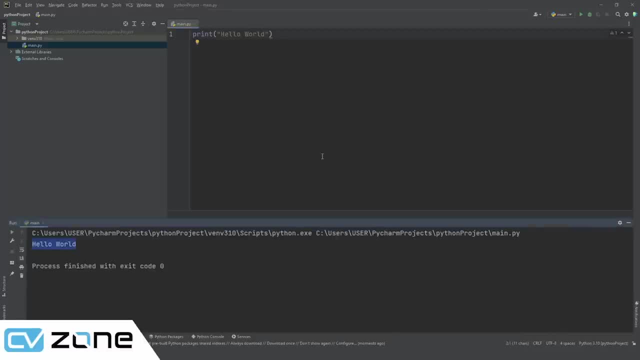 press the button that to go to the world so you can see python 3.1 hold. so this is running python 3, point 1: 0. how do i know? this is because you can see here we have python 3.1: 0, we don't have python 3.7, so 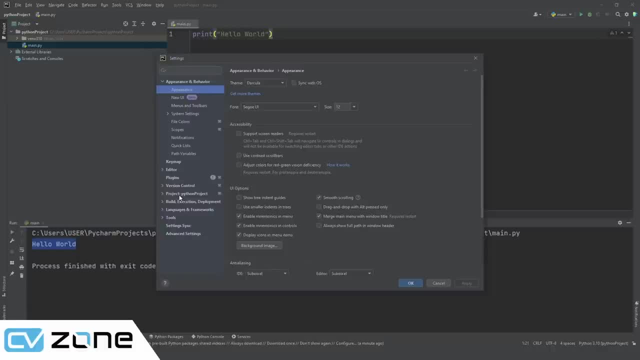 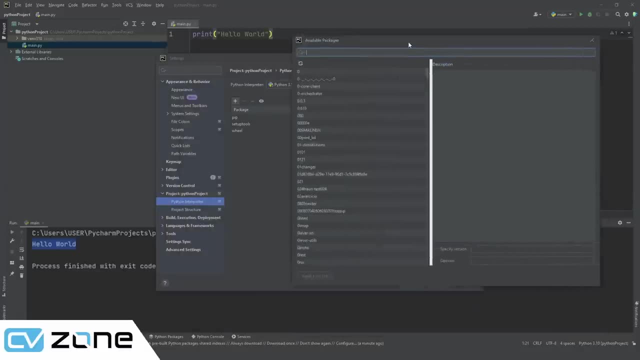 what we will do is we are going to go to file and any package that we want to install, we can go to settings and then we will go to project, python project, and we'll go to python interpreter and we want, whether it's opencv, whether it's cvzone, whether it's ultralytics, whatever it is, you can. 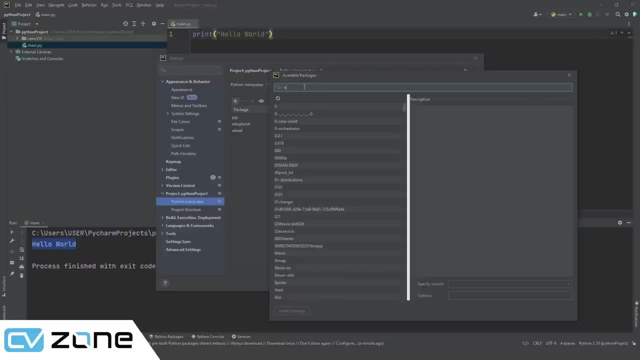 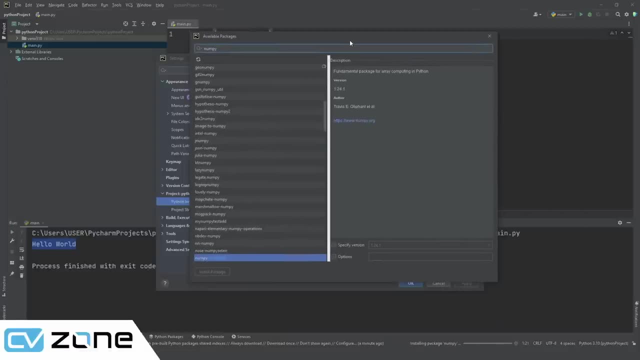 install here. so, for example, we can go ahead and install numpy, numpy. so we will click on install package and it will take a while, and you can also specify which version of numpy do you want to install. we are installing the latest one that is available right now, so we can hit close and here. 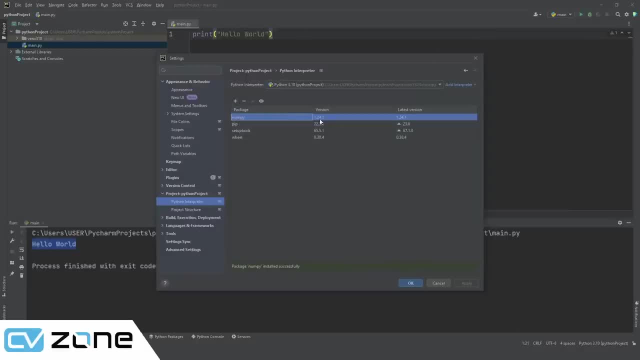 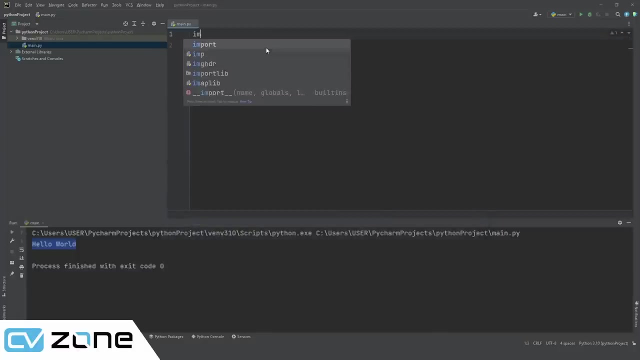 you can see now in the packages, we have numpy installed. this is the current version and this is the latest version, so they are up to date. so these three are already installed, so you don't have to worry about those. then we can simply click: ok. so here, if i write imports numpy. 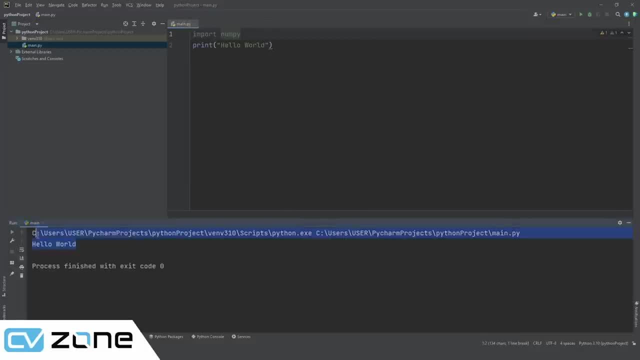 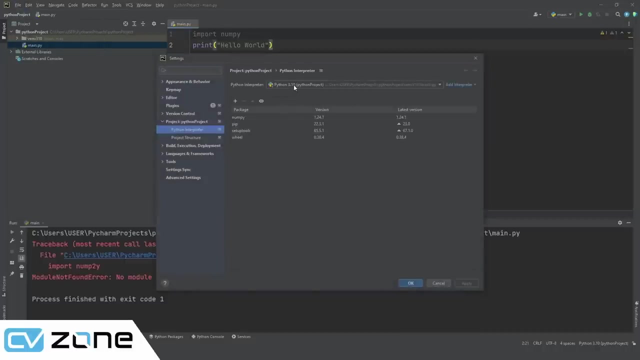 and if i run this, it will not give me any error, which means numpy has been installed. if i write anything else, it will give me an error because there is no library called numpy2y, right? so that's the basic idea. so this is import numpy. now if i go to file and if i go to settings, i can create a new virtual environment if i wanted. 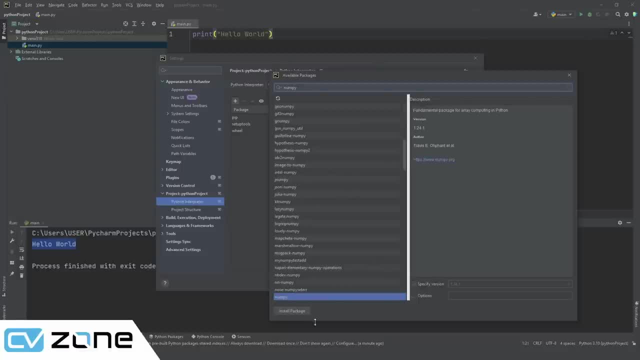 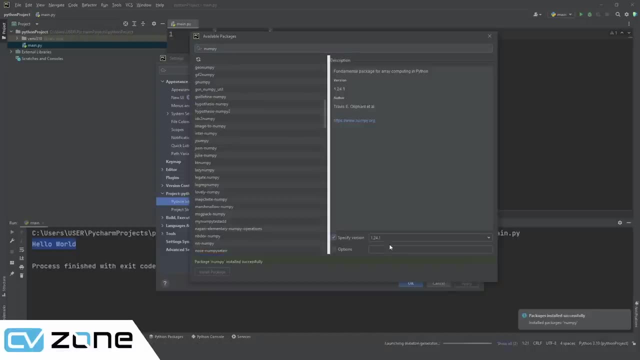 install numpy, numpy. so we will click on install package and it will take a while and you can also specify which version of numpy do you want to install, the latest one that is available right now so we can hit close. and here you can see now in the packages we have numpy installed. this is the 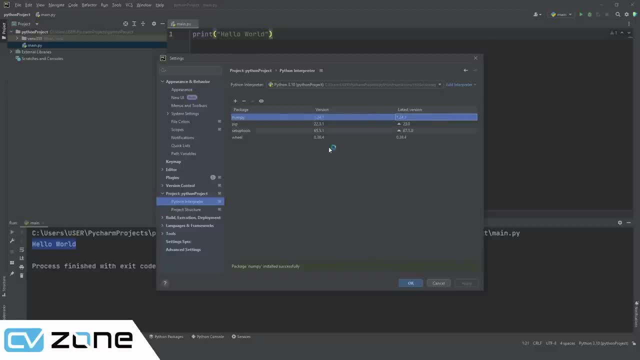 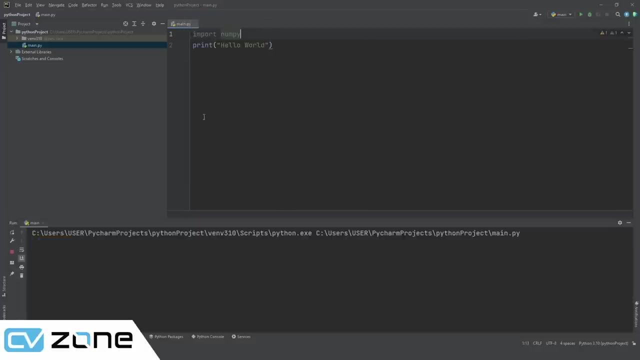 current version and this is the latest version, so they are up to date. so these three are already installed, so you don't have to worry about those. then we can simply click. ok, so here, if i write imports numpy and if i run this, it will not give me any error, which means numpy has been installed. 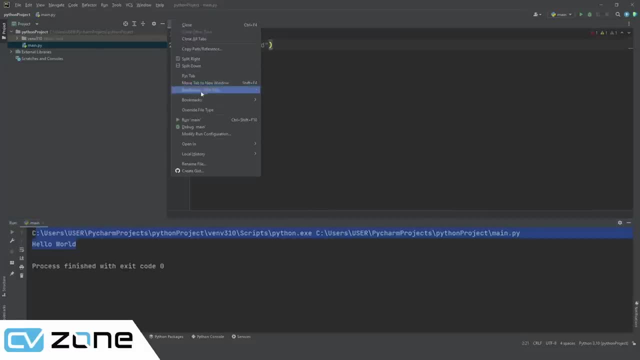 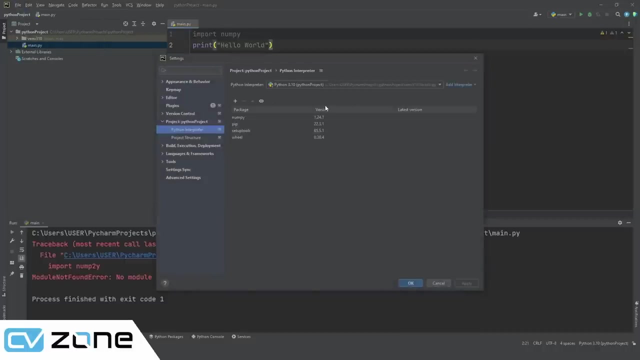 if i write anything else, it will give me an error because there is no library called numpy2y, right? so that's the basic idea. so this is import numpy. now, if i go to file and if i go to settings, i can create a new virtual environment. if i wanted to use two different pythons, i could create a new. 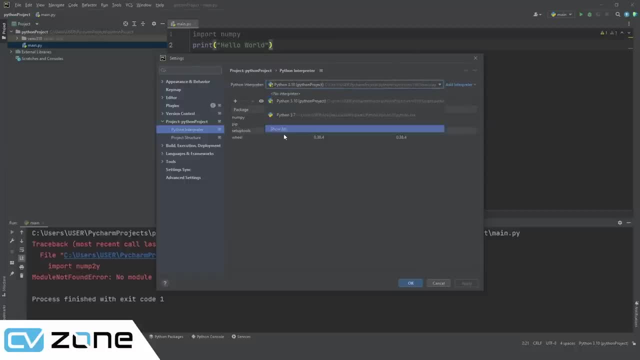 virtual environment. to do that, you can click here. you can go to show all and over. here we can click on add. so here we can create a new environment and here we will create for 3.7. so we will select 3.7 as our brace interpreter and we have named the virtual environment 3.7. 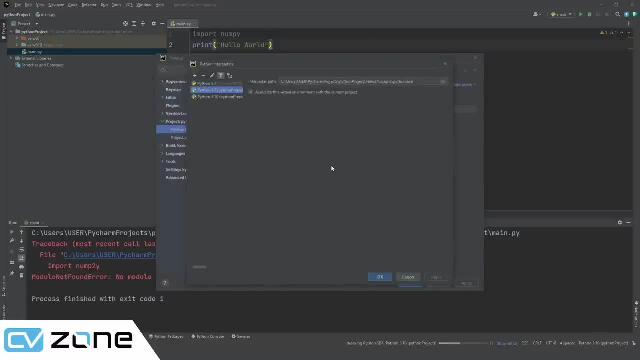 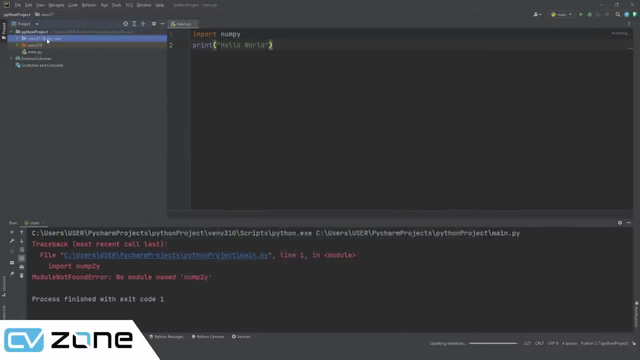 and then we'll press ok. so now it will create and it will shift it to 3.7. we'll hit ok. but now you can see that we installed numpy earlier, but it was installed in the virtual environment of 3.10 but now it's not installed in 3.7 because we are now using 3.7 as the main. 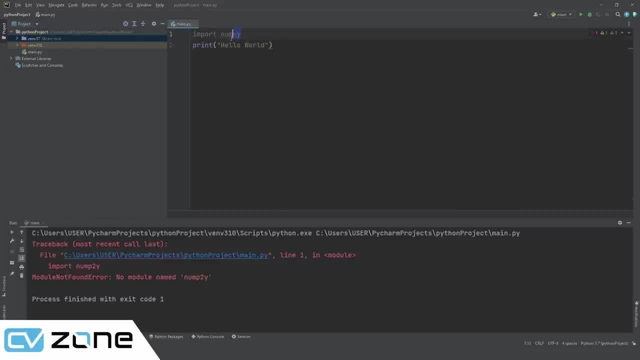 environment, so that's why it is giving us an error over here. so if i run this now, it will give me an error that there is no numpy, but if i click here and go to 3.10 and then it will load up, and if i run it again, it will not give me an error, because 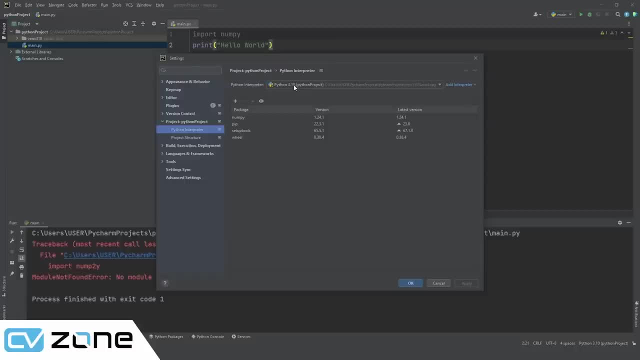 to use two different pythons. i could create a new virtual environment. to do that, you can click here. you can go to show all and over. here we can click on add. so here we can see the new virtual environment. we can create a new environment, and here we will create for 3.7. 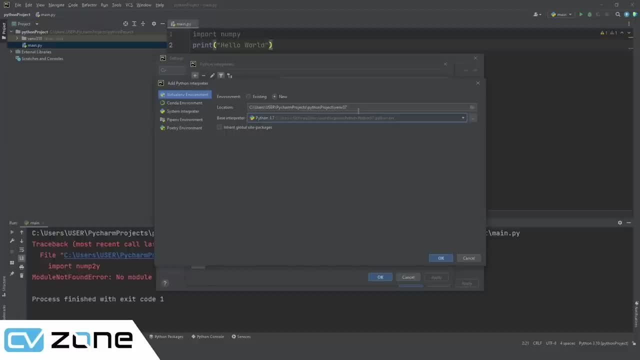 so we will select 3.7 as our brace interpreter and we have named the virtual environment 3, 7 and then we'll press ok. so now it will create and it will shift it to 3.7. we'll hit ok, but now you can see. 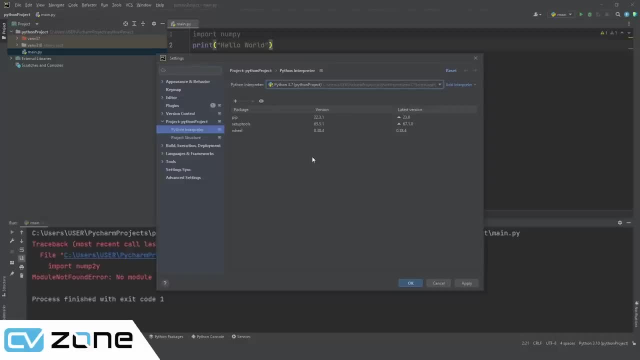 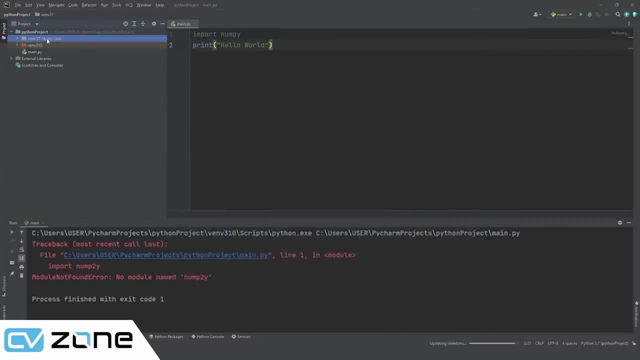 that numpy has been installed in the virtual environment, but it was installed in the virtual environment of 3.10, but now it's not installed in 3.7 because we are now using 3.7 as the main environment. so that's why it is giving us an error over here. so if i run this now, it will give me an. 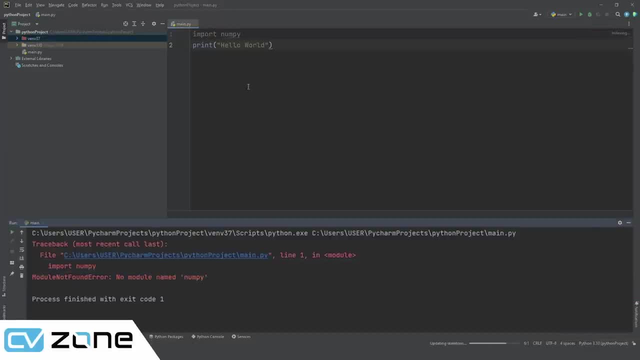 error that there is no numpy. but if i click here and go to 3.10 and then it will load up and if i run it again, it will not give me an error because numpy is already installed. so you have to make sure that your libraries are installed if you are trying different versions of python. so here you can go. 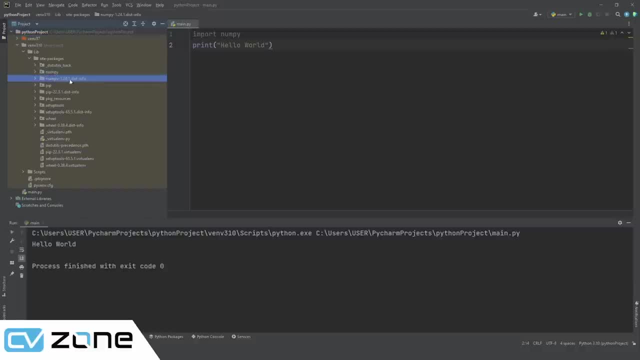 to library and you can see you have numpy installed. so here in 3.7 you will not see numpy. so what you can do is, if you wanted to use in 3.7, you will make sure it's 3.7 over here and you will go to file settings and here you are going to install numpy. 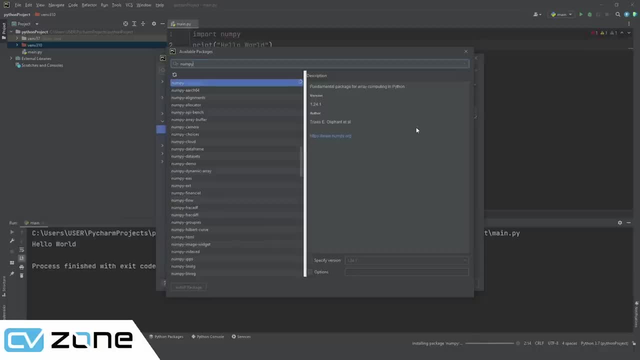 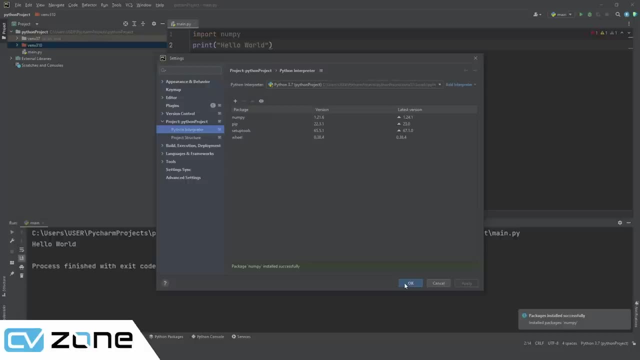 now it will install it to 3.7 as well. so the reason i'm telling you this is because later on you might face some issue in, for example, 3.12 or 3.15, and you might you might want to downgrade, or you might want to upgrade later on. so instead of creating a new project and then 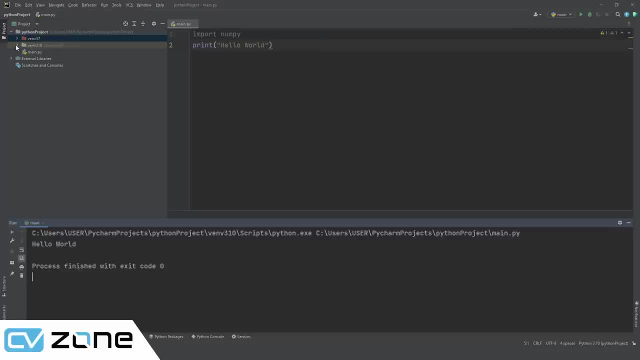 numpy is already installed. so you have to make sure that your libraries are installed if you are trying different versions of python. so here you can go to library and you can see you have numpy installed. so here in 3.7 you will not see numpy. so what you can do is, if you wanted, 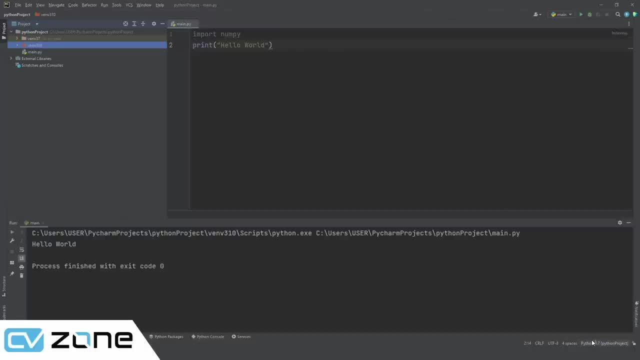 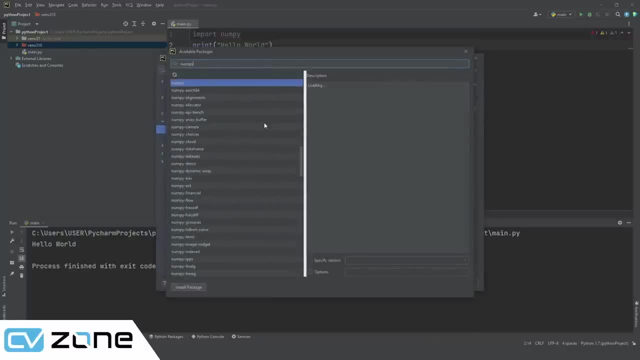 to install numpy. you will make sure it's 3.7 over here and you will go to file settings, and here you are going to install numpy. now it will install it to 3.7 as well. so the reason i'm telling you this is because later on you might face some issue in, for example, 3.12 or 3.15 and you want. 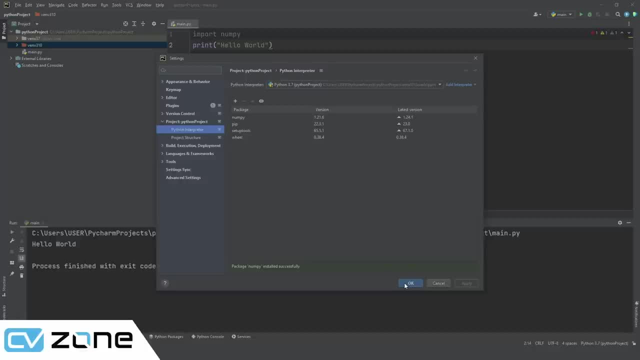 you might want to downgrade, or you might want to upgrade later on, so if you want to upgrade later on. so instead of creating a new project and doing all of these things together again, what you can do is you can simply have a new virtual environment and have the same project running. so it will not. 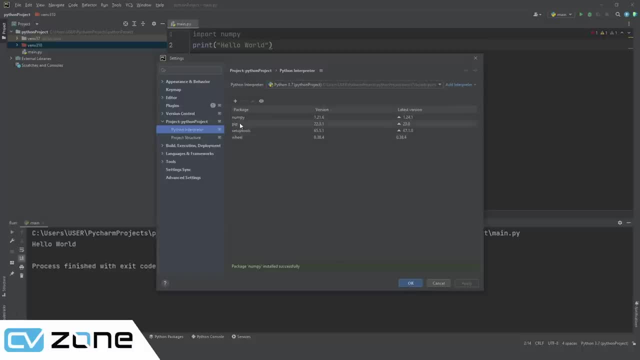 be very difficult to debug. so here you can see we have installed numpy for 3.7 as well. so now if i run with 3.7 or 3.10, it will run with both. so for most project we are only going to use. 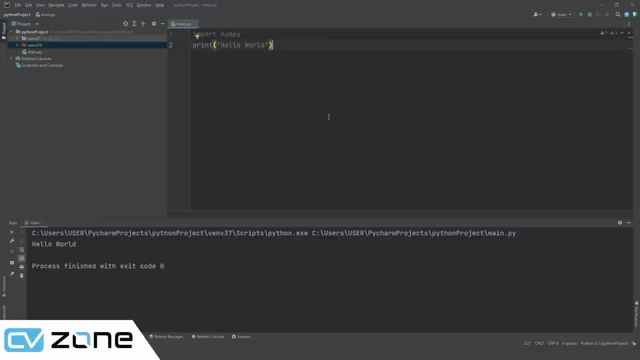 one python environment, we will usually use the higher one, unless there are some major issues in that. so then, in that case, we are going to downgrade. so now that we understand how to install pycharm and how to install python, you can add more python versions. now we can simply: 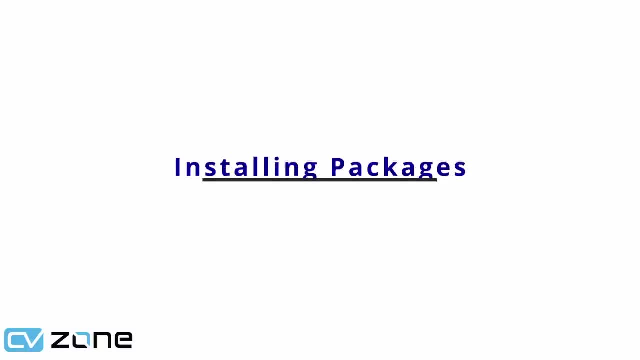 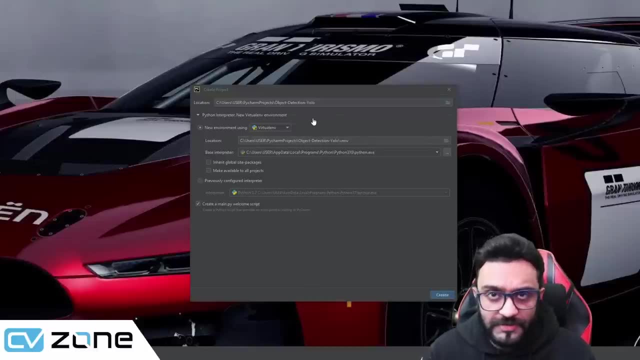 go ahead and start working on our project. so here we are going to create our pycharm project, which is object detection yolo, and we are creating a new virtual environment, and the environment is based on the base interpreter of python version 3.1.0, so 3.10. so it is up to you which python 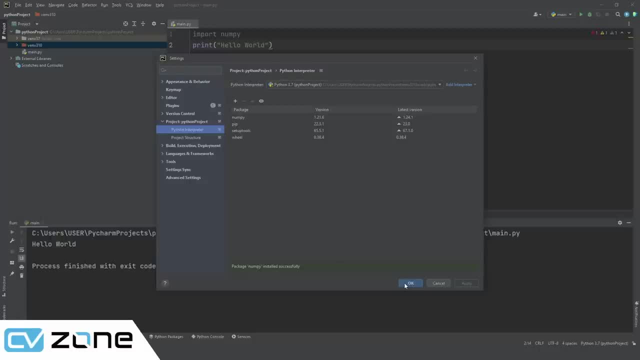 load it in vmware project and doing all of these things together. again, what you can do is you can simply have a new virtual environment and have the same project running, so it will not be very difficult to debug. so here you can see. we have installed numpy for 3.7 as well. so now if i run with 3.7 or 3.10, 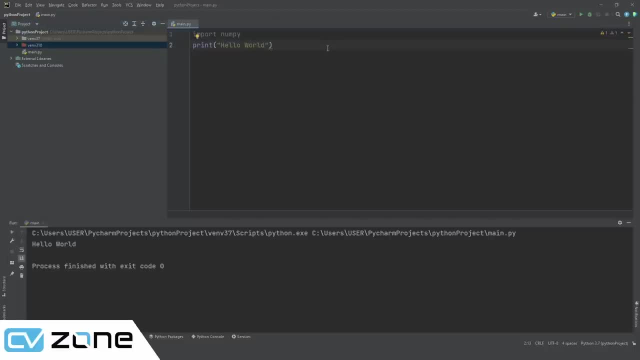 it will run with both. so for most project we are only going to use one python environment. we will usually use the higher one, unless there are some major issues in that. so then in that case we are going to downgrade. so now that we understand how to install pycharm and how to install python, 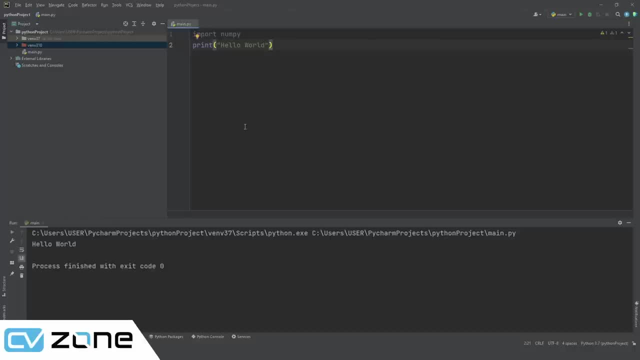 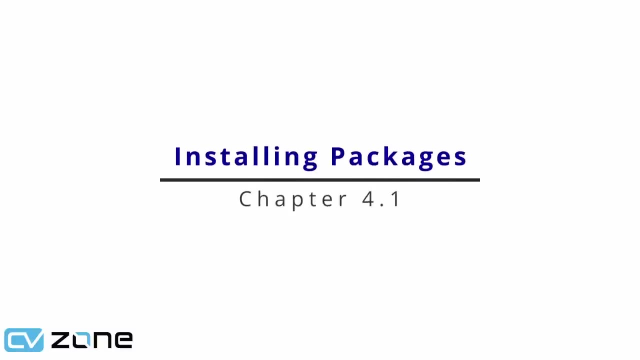 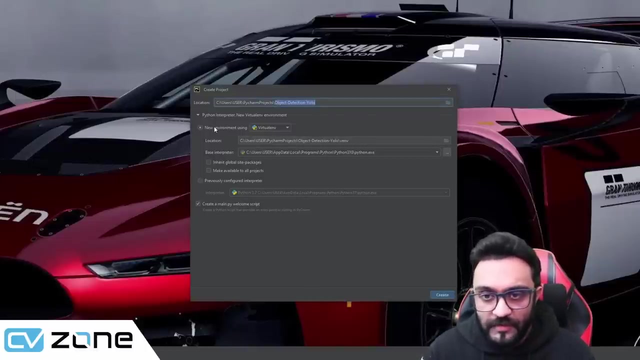 you can add more python versions. now we can simply go ahead and start working on our project. so here we are going to create our pycharm project, which is object detection yolo, and we are creating a new virtual environment, and the environment is based on the base interpreter. 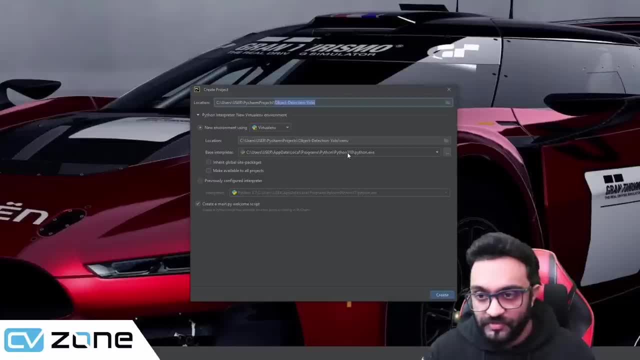 of python version 3.1.0, so 3.10. so it is up to you which python version you want to use. so we are using 3.10. if you have a newer version you can use that too, but don't use the latest. 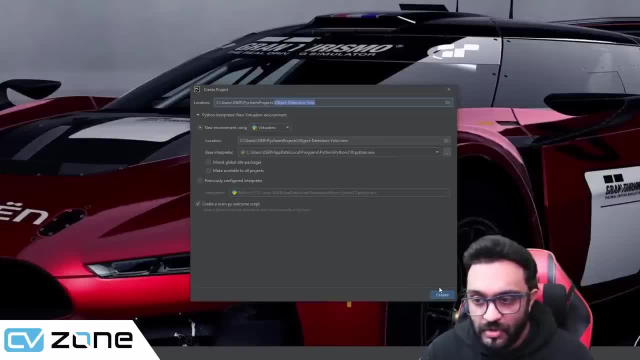 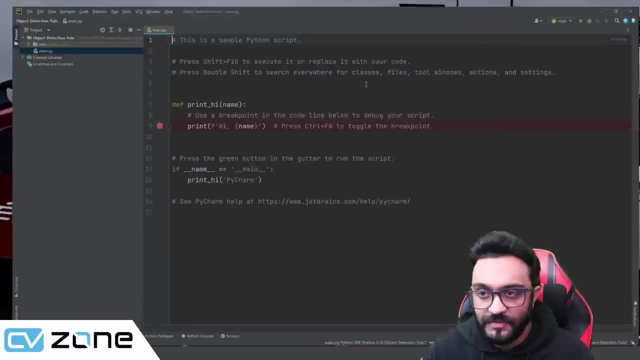 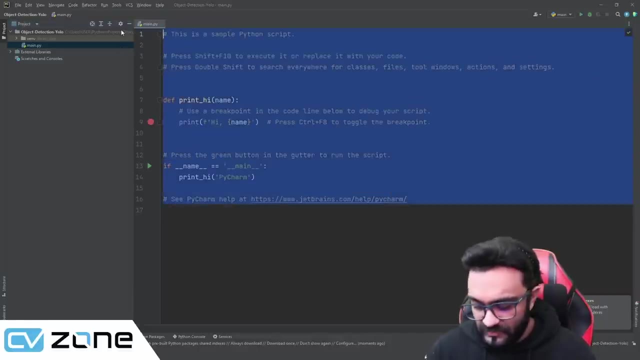 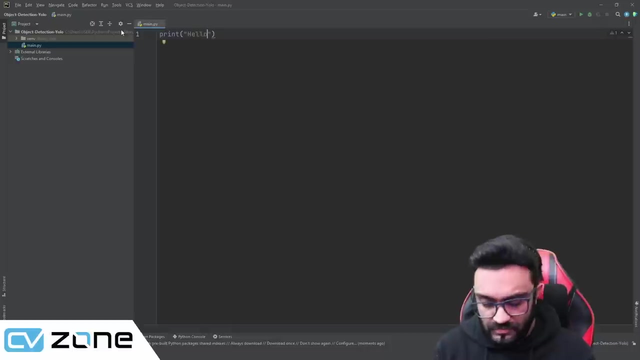 one, because it might yield some errors. so what we'll do is we'll simply hit on create and there you go, we have our project, and here we have a main file. so what we can do is we can use this main file to test our code. we can simply write: print, print hello world, and we can. 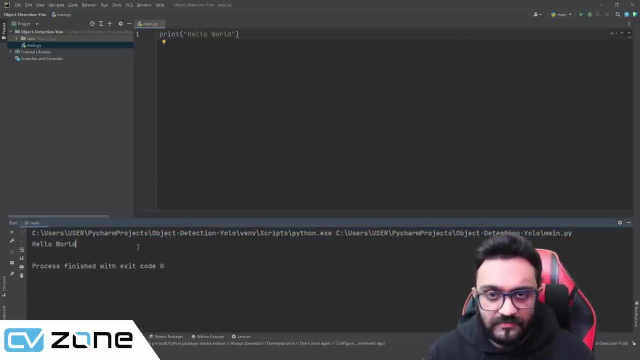 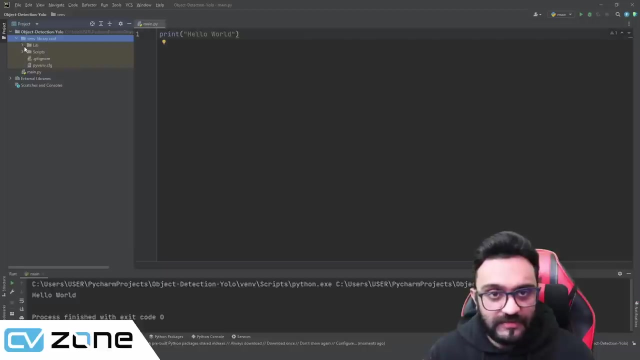 run it just to see if everything is working, and it's working fine. so in order to get started, what we have to do is we have to do some installations on this virtual environment. so if you look at this folder, we have the virtual environment. if you click on that in the libraries, these are: 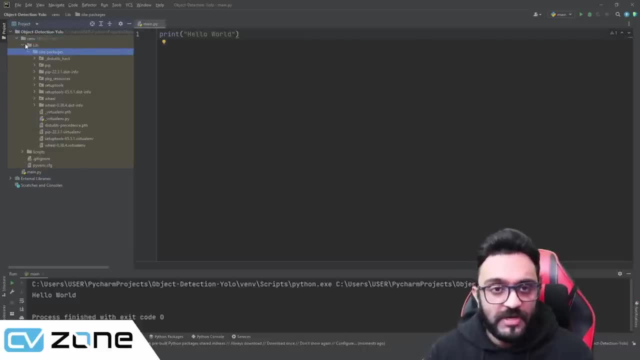 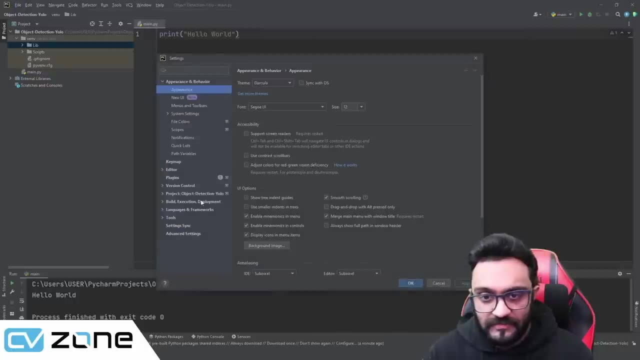 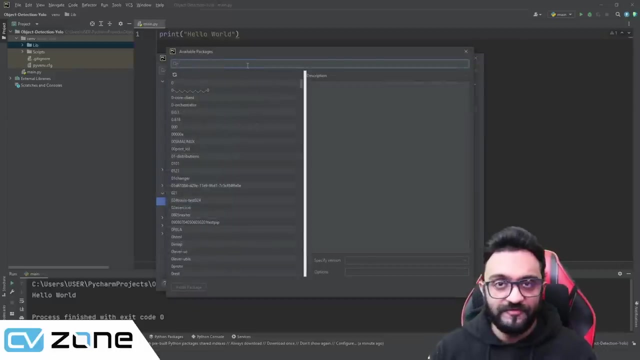 the site packages. we need to install some packages in order to run our project. so how can you do that? you can go to file settings and in the project python interpreter you can click on add. you can type in the version, for example. you can type in the site package name, for example cv zone. 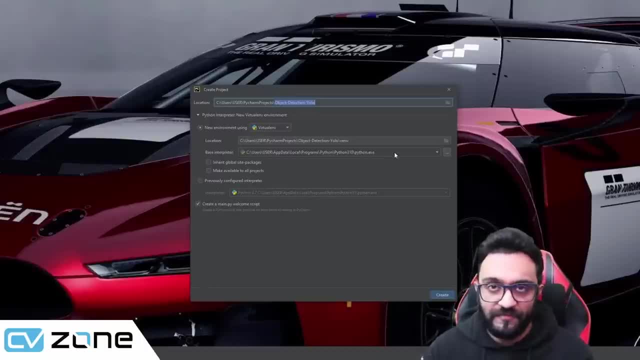 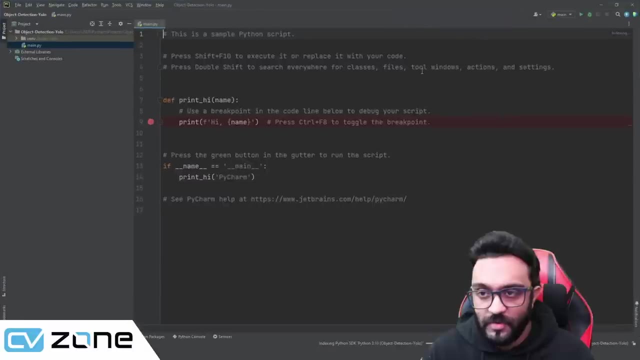 version you want to use. so we are using 3.10. if you have a newer version, you can use that too, but don't use the latest one, because it might yield some errors. so what we'll do is we will simply hit on create and there you go: we have our project, and here we have a main file. so what we can do is we can. 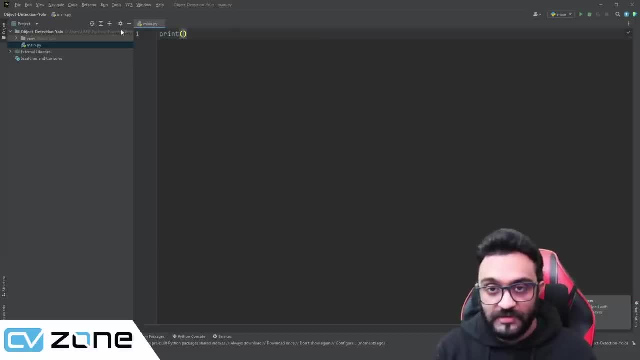 use this main file to test our code. we can simply write, print, print hello world, and we can run it just to see if everything is working, and it's working fine. so, in order to get started, what we have to do is we have to do some installations on this virtual. 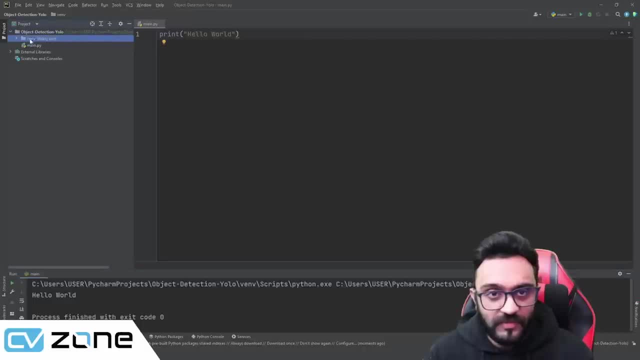 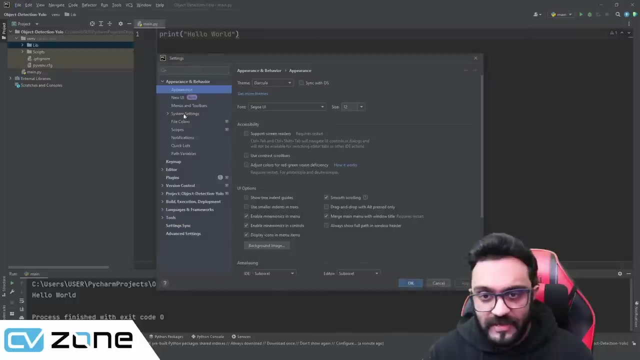 environment. so if you look at this folder, we have the virtual environment. if you click on that in the libraries, these are the site packages. we need to install some packages in order to run our project. so how can you do that? you can go to file settings and in the project python interpreter you. 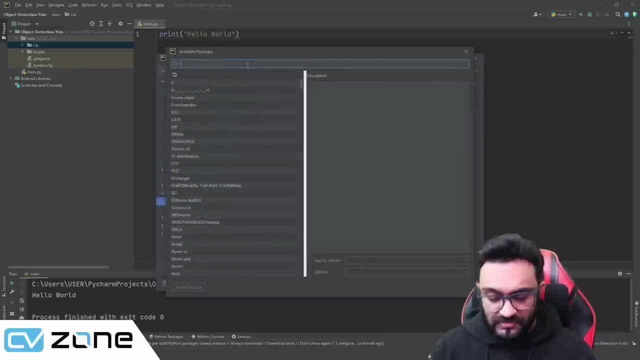 can click on add, you can type in the version, for example. you can type in the site package name, for example CV zone, and you can hit install. now, when we are working with object detection, there's a lot of libraries that are working at the back end, so installing them one by one will take a lot of time. 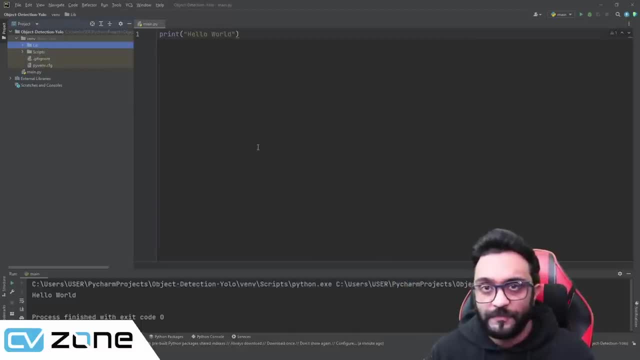 so what you can do is a simple way of doing this is copying a requirements file, or you can create your own file as well. so here, this is a standard version. this is a standard way of doing this, so what you can do is you can simply paste. 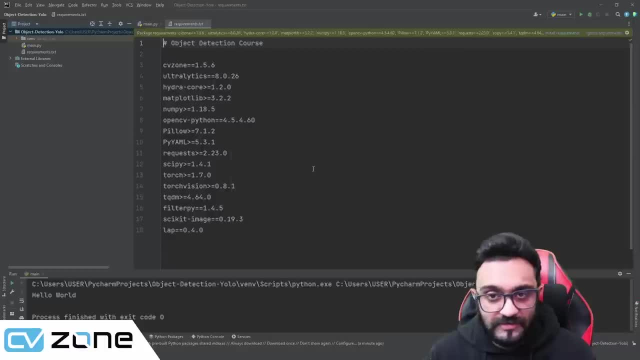 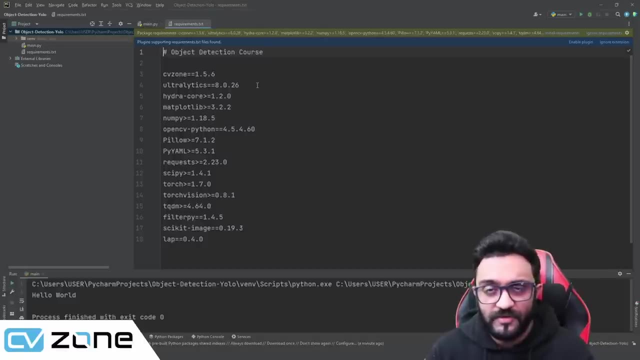 requirementstxt in this project. so where do you get this requirementstxt? you can download it from our website computervisionzone. it is free to download. all you have to do is sign up. if you already have signed up, just sign in with your account, go to the course page and there you can. 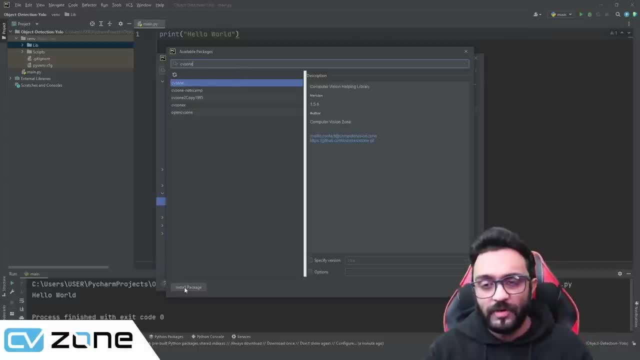 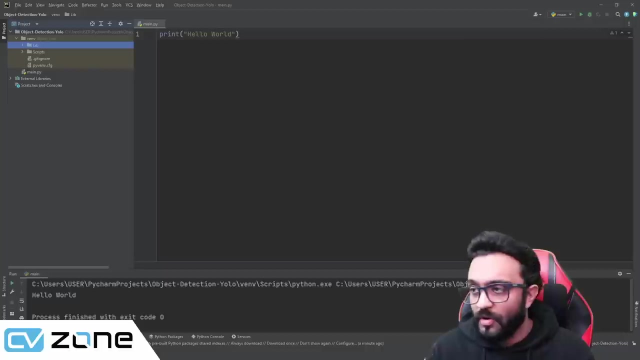 and you can hit install. now, when we are working with object detection, there's a lot of libraries that are working at the back end, so installing them one by one will take a lot of time. so what you can do is a simple way of doing this is copying a requirements file, or you can create. 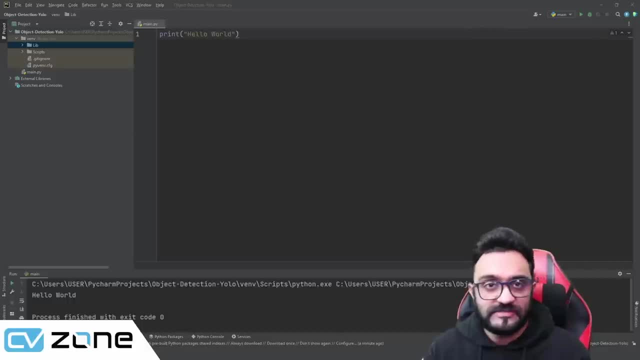 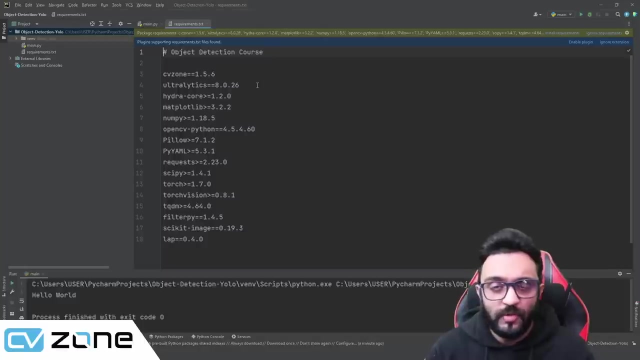 your own file as well. so here, this is a standard version. this is a standard way of doing this, so what you can do is you can simply paste requirements dot text in this project. so where do you get this requirementstxt? you can download it from our website, computervisionzone. it is free to download. all you have to do is sign up, if you. 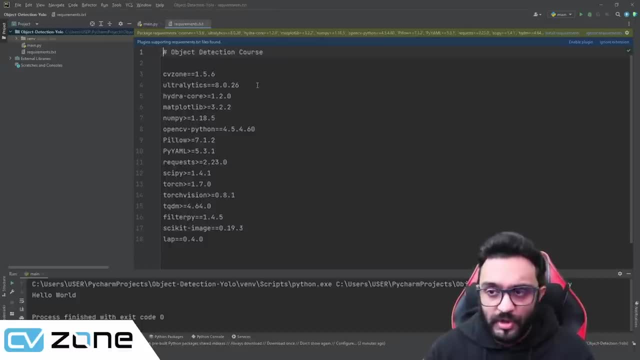 already have signed up, just sign in with your account, go to the course page and there you can download everything related to the course absolutely free. so you don't have to pay anything, you can just download and you can copy it here. so here you can see as soon as we copy the requirements. 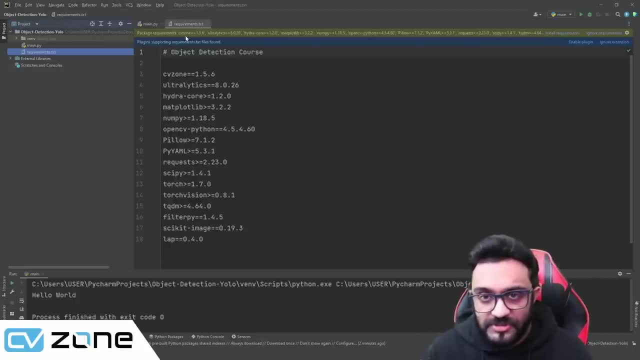 file. it will give us a notification package requirements. all of these packages have not been installed, so what you can do is you can click on install requirements and it will install all the requirements that you need. so what do these mean? so, for example, cv zone double equals 1.5.6. this 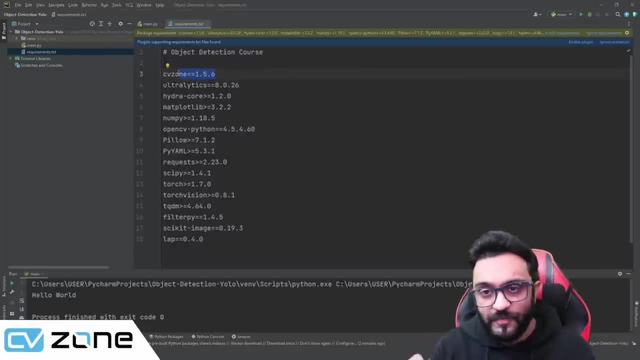 means: use the exact same version, 1.5.6. don't use anything above it. don't use anything below it. the following single file: lower case and, as such, only write向ing. to be the case, however, you need to use the same, only�리. 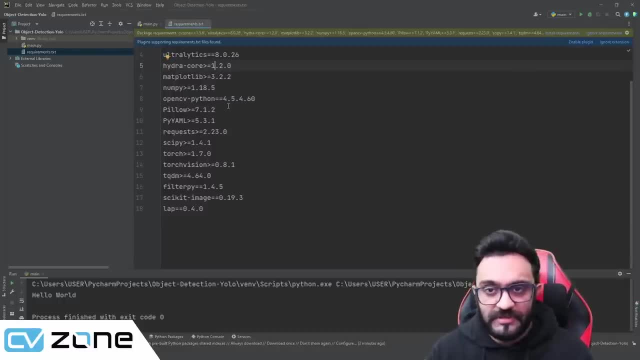 1.5 at the last. so in everything else we use the same version 1.5.. this means to be Fans shell, so that we can actually peruse something. we simply open it. everything else we won't, but in audiobook or something like that, here in a være. ます. so right now i'm using python 3.10, so with this, all of these versions should work fine. now, when it is greater than or equals to, then it means that use this at the very least, or if there is a newer version, use that instead. so this can be a little bit dangerous or tricky, because if the newer version is not compatible it might not work. so you have to be careful. which ones are you? hard coding of the written hiç. 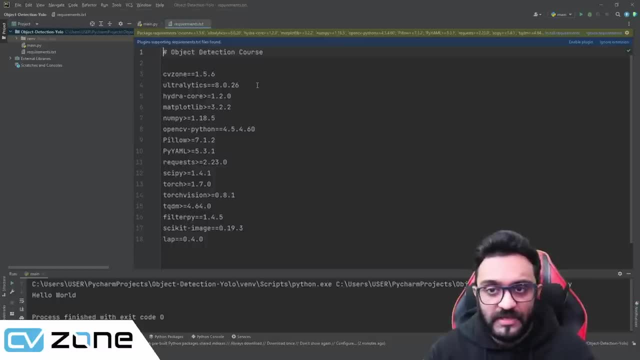 download everything related to the course absolutely free. so you don't have to pay anything. you can just download and you can copy it here. so here you can see. as soon as we copy the requirementstxt file, it will give us a notification package requirements all of these: 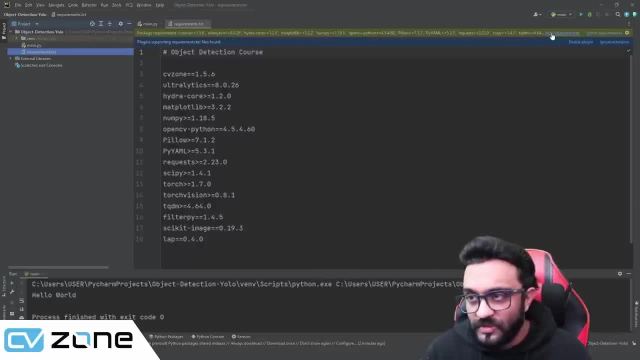 packages have not been installed. so what you can do is you can click on install requirements and it will install all the requirements that you need. so what do these mean? so, for example, CV zone double equals 1.5.6. this means: use the exact same version, 1.5.6. don't use anything above it. 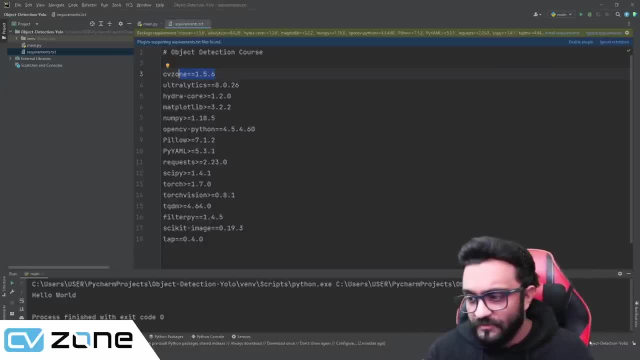 anything below it, the exact same version. so right now I'm using python 3.10, so with this, all of these versions should work fine. now, when it is greater than or equals to, then it means that use this at the very least, or if there is a newer version, use that instead. so this can be a little. 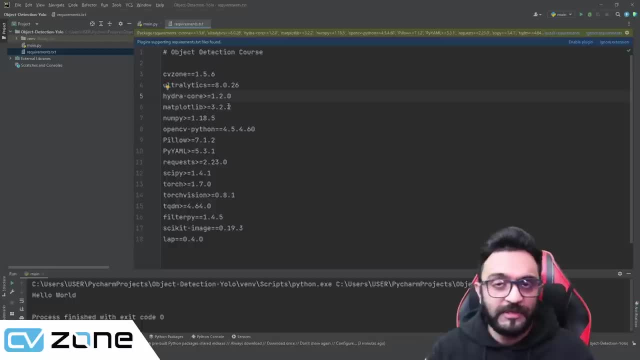 bit dangerous or tricky, because if the newer version is not compatible it might not work. so you have to be careful which ones uh are you hardcoding to be exact same version and which ones are using. for example, here for python, we have hardcoded it to the exact same version. normally it's not done like this, but 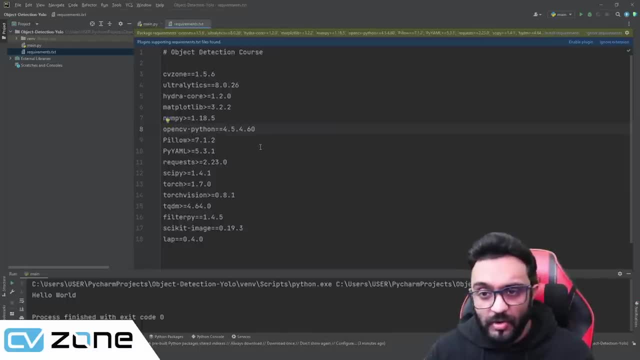 because the latest version has some issues in auto um correcting. we are going to use uh dot 60. this is the version that does not have this issue, so that's why I have hardcoded it to be this exact version. now, if you have a later version that works fine for you, that's okay, but if it doesn't, then it's better if you use. 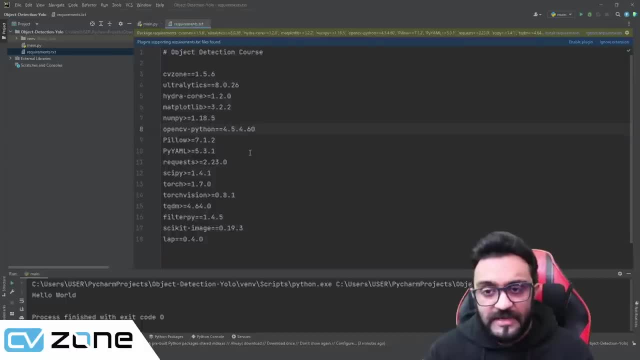 the exact same thing. now, sometimes what happens is that you install everything, but some of them do not install, and again that might be the issue of that. it's not compatible, they don't have a version that satisfy the satisfies, the requirement. so what you can do is you can downgrade or you can. 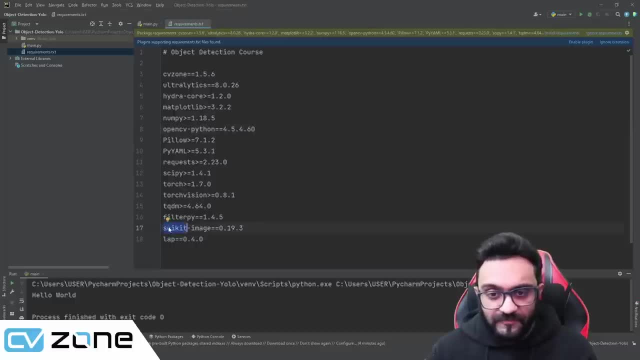 upgrade. it's based on that. for example, uh, scikit learn. for example, this scikit image, let's say it doesn't work, or we can simply comment it and it will remove it from the install installations. so later on, if I give it a wrong number, let's say like that, it will give us an. 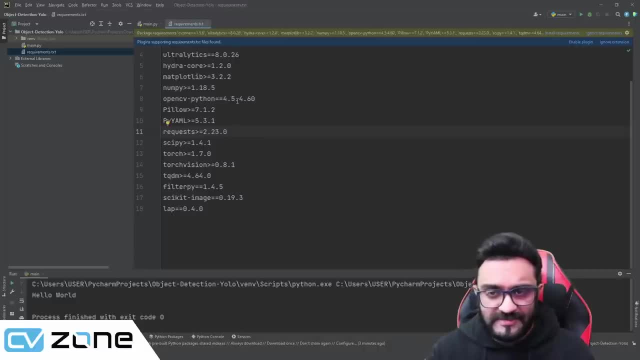 ones are you hardcoding to be exact same version and which ones are you using, For example, here for Python? we have hardcoded it to the exact same version. Normally it's not done like this, but because the latest version has some issues in auto correcting, we are. 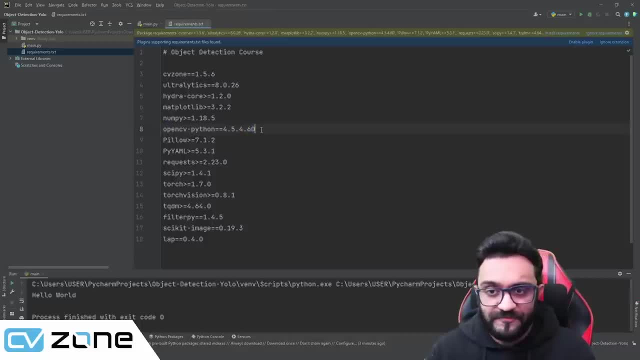 going to use .60.. This is the version that does not have this issue, So that's why I have hardcoded it to be this exact version. Now, if you have a later version that works, fine for you, that's okay, But if it doesn't, then it's better if you use the exact same. 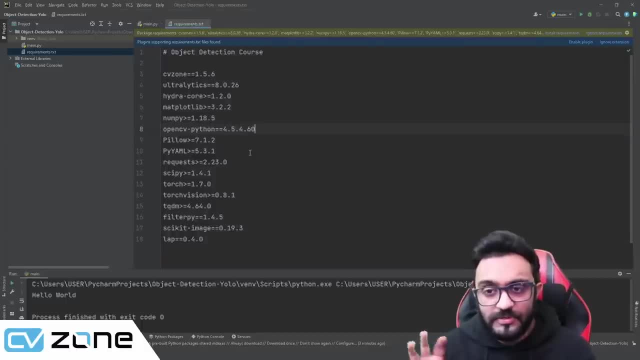 thing. Now, sometimes what happens is that you install everything, but some of them do not install, And again that might be the issue of that. it's not compatible. They don't have a version that satisfies the requirement. So what you can do is you can downgrade or 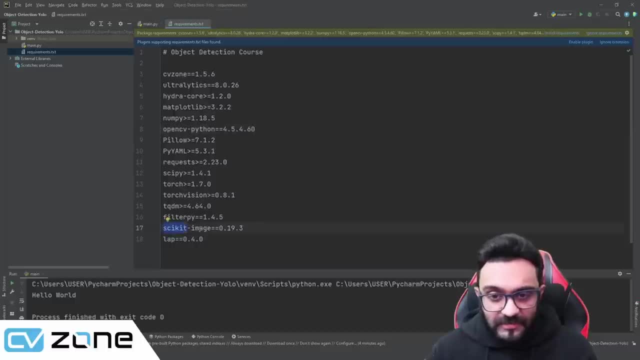 you can upgrade. It's based on that, For example, scikit-learn, for example, this scikit image, let's say it doesn't work, or we can simply comment it and it will remove it from the install installations. So later, 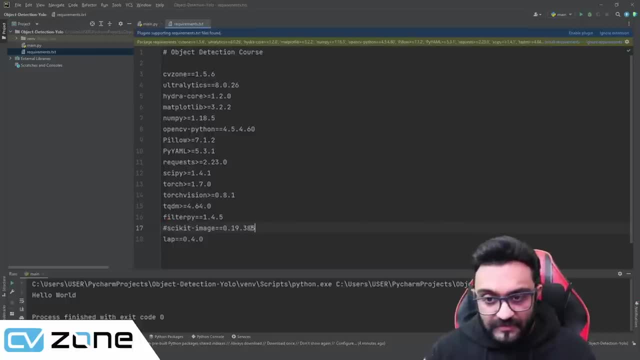 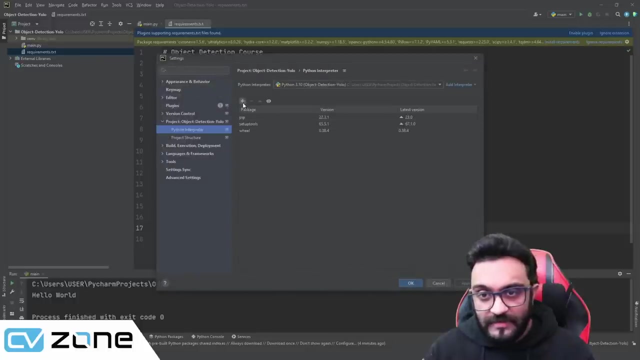 on. if I give it a wrong number, let's say like that, it will give us an error that it was unable to install. So in that case, either you can come here and fix the number here based on the version, or you can go to file, you can go to settings and in add you can. 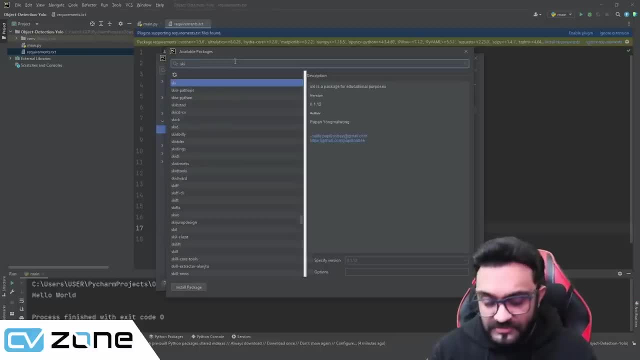 you can search for sci. what was the spelling scikit? I believe no. S, C, I, K, I, T. dash image. Yeah, so you can click on that. You can specify version and you can select which version do you need. It might be a higher version, it might be a lower version. So if the latest 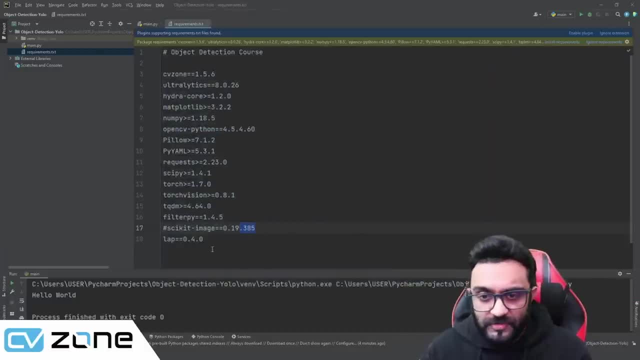 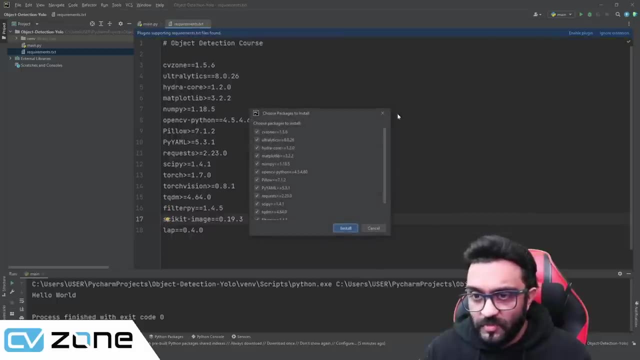 one doesn't work, go to the previous one by default, Okay. so, that being said, let's just install everything. we will click on install requirements. it will ask us that you want to install all of these. we will say yes, install, and then we are simply going to wait for the. 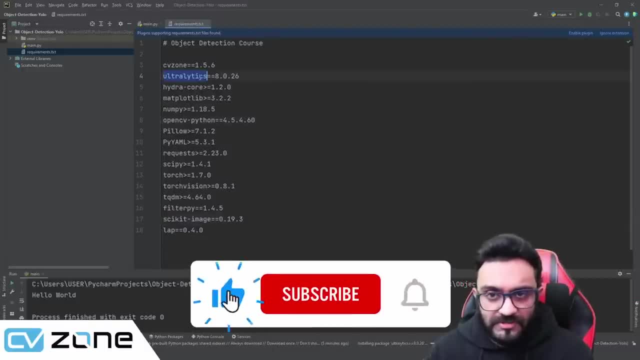 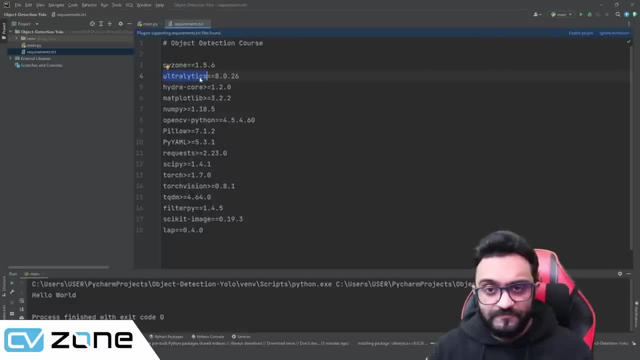 installation to complete. so the main library that we are using is ultralytics. that will provide us with the yolo package and it will download the yolo weights for us as well. so we will be using version 8 of yolo and if later versions come up, you can use those two, depending on whether they 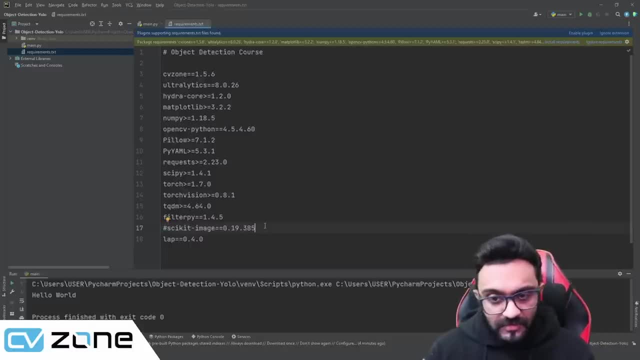 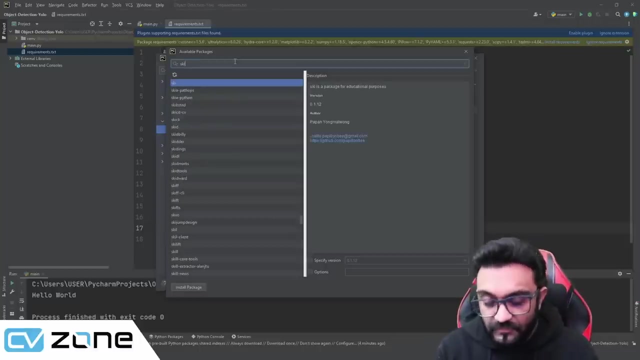 error that it was unable to install. so in that case, either you can come here and fix the number here based on the version, or you can go to file, you can go to settings and in add you can. you can search for psi. what was the spelling? scikit? I believe no. s-c-i-k-i-t dash image. yeah, so you can click on that. you can specify version. 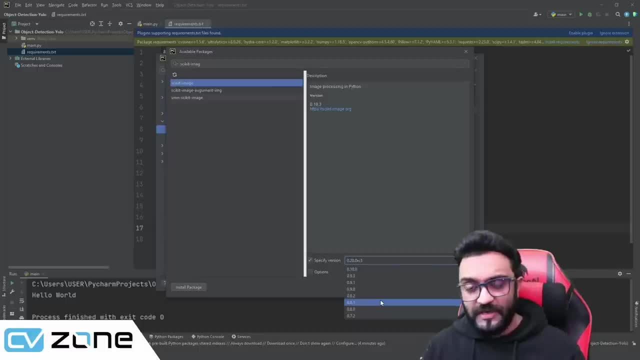 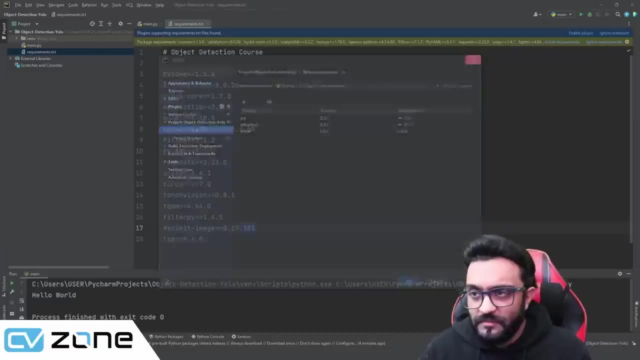 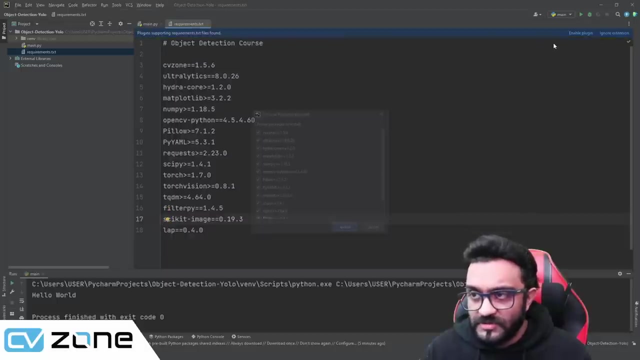 and you can select which version do you need. it might be a higher version, it might be a lower version. so if the latest one doesn't work, go to the previous one by default, okay, so, uh, that being said, let's just install everything. we will click on install requirements it. 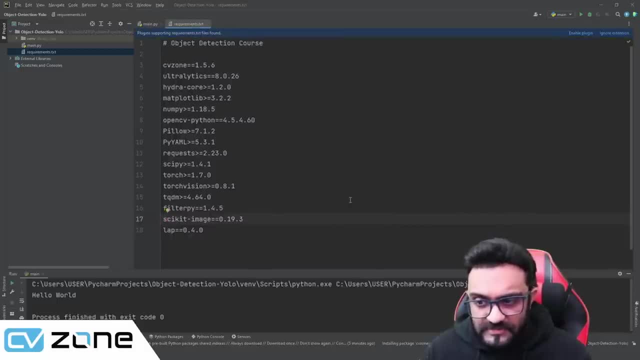 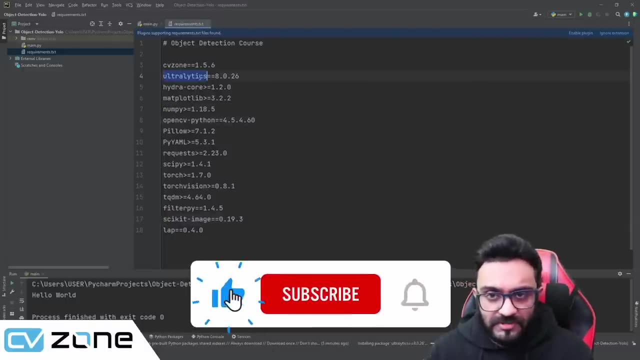 will ask us that you want to install all of these. we will say, yes, install, and then we are simply going to wait for the installation to complete. so the main library that we are using is ultralytics. that will provide us with the YOLO package and it will download the YOLO weights for 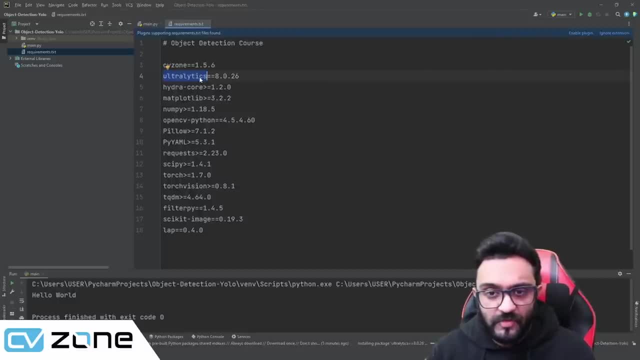 us as well. so we will be using version 8 of YOLO, and if later versions come up, you can use those too, depending on whether they are um, are related to ultra analytics or not. so all of these packages are being installed and let's wait for it to finish. 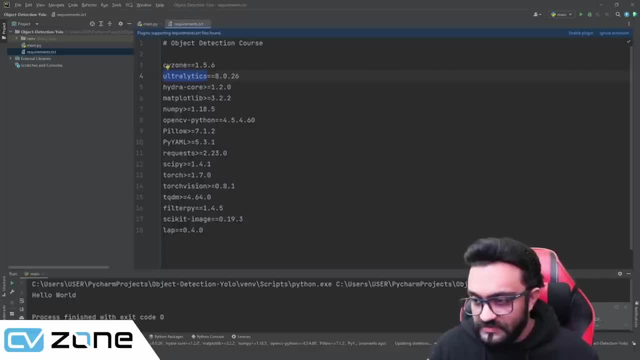 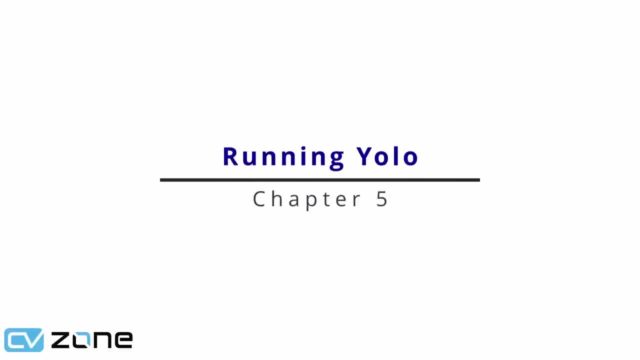 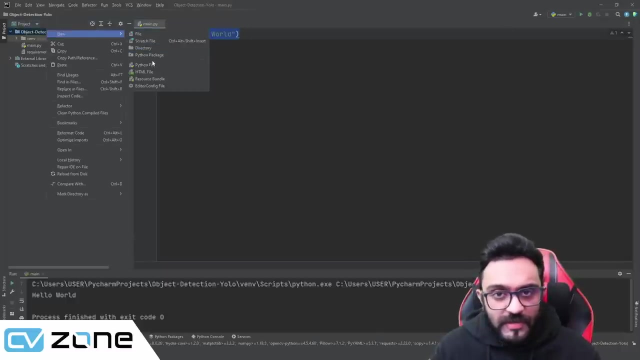 so all the packages have now been installed. as you can see, all of them are installed and we are good to go. so what we can do is we are going to create a new folder and we are going to call it chapter 5, and within chapter 5, we are going to say running YOLO. 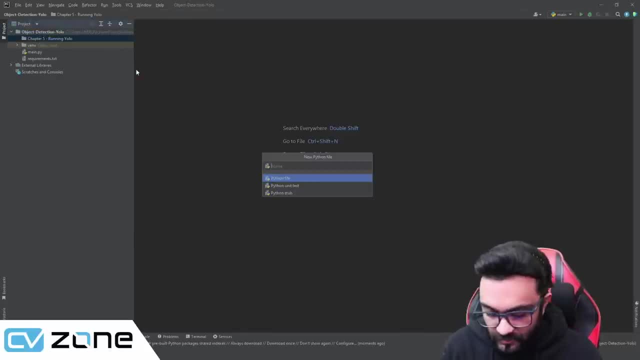 so then we will right click and we will create a new python file and we will call it YOLO- basics- basics. so there you go, we have our first file, and all we have to do is we have to test whether the YOLO uh will work or not, and how exactly can we run it. so, in order to test YOLO, we 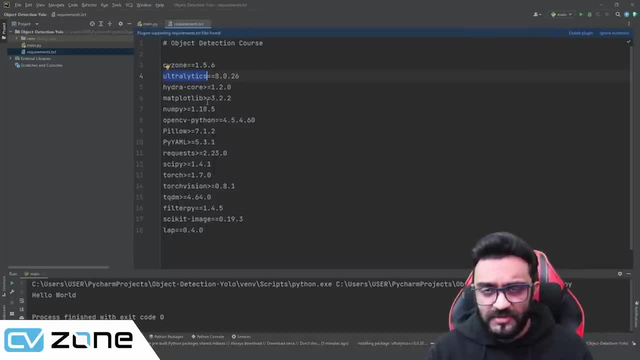 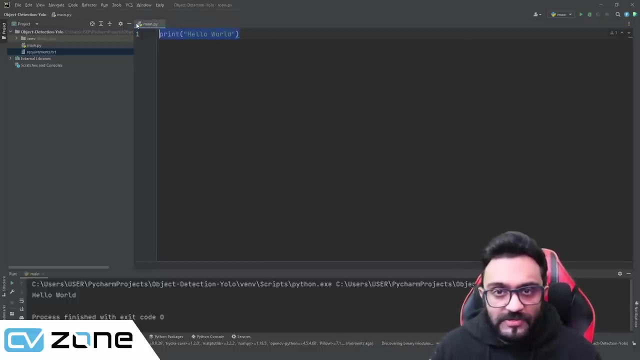 are are related to ultralytics or not. so all of these packages are being installed and let's wait for it to finish. so all the packages have now been installed, as you can see, all of them are installed and we are good to go. so what we can do is we. 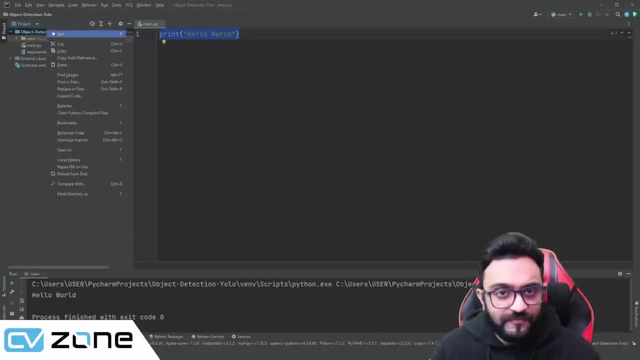 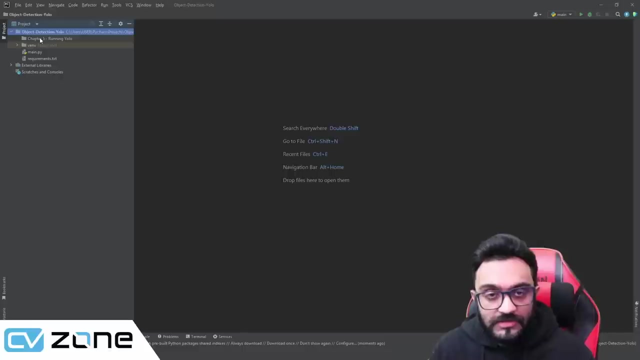 are going to create a new folder and we are going to call it chapter 5, and within chapter 5 we are going to say running yolo. so then we will right click and we will create a new python file and we will call it yolo- basics, basics. so there you go. we have our familiar version of ultralytics. 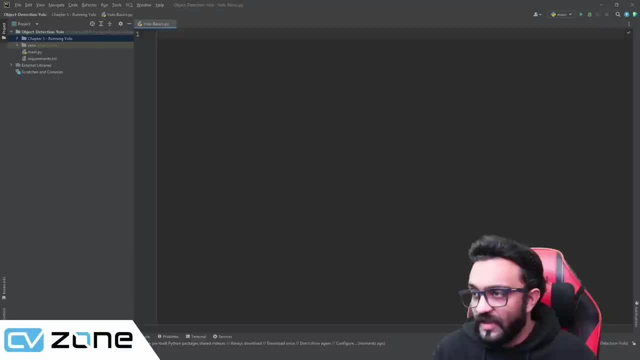 which we have previously analyzed, and we are going to start by earning some money by using file and all we have to do is we have to test whether the YOLO will work or not and how exactly can we run it. so in order to test YOLO, we need to have some 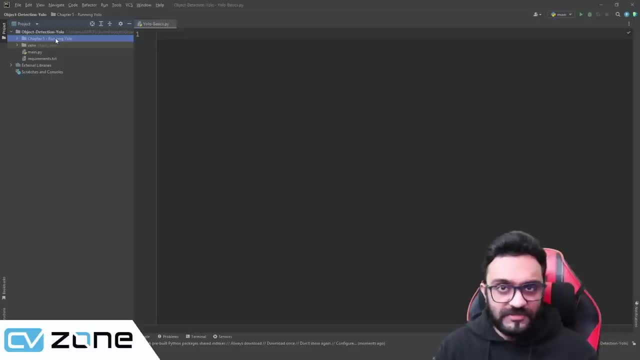 images. so we are going to run it on images first, once we know it it works. then we are going to try it with webcam in the next chapter. so we have some images again. you will find this on our website. once you download the zip file, everything will be included in it. so here you will see we have images and if 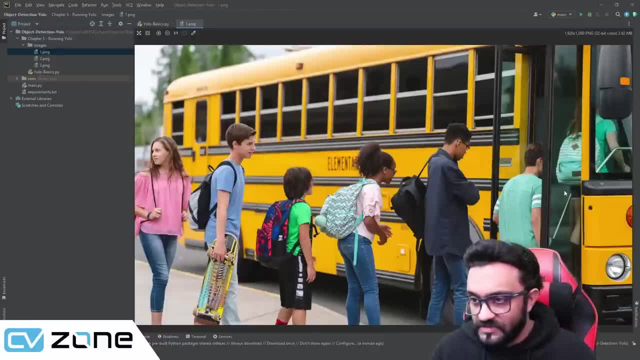 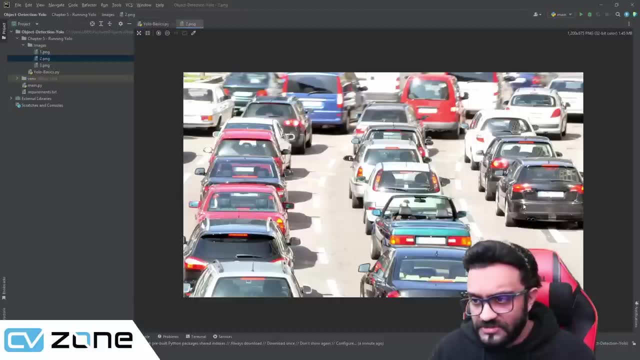 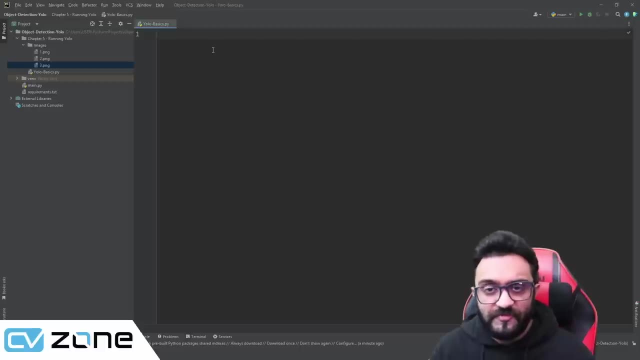 you open up images. the first image is of a school bus, with some kids going into the school bus. then the second image is of cars and the third image is of some bikes, so motorbikes. so these are the three image images that we are going to. 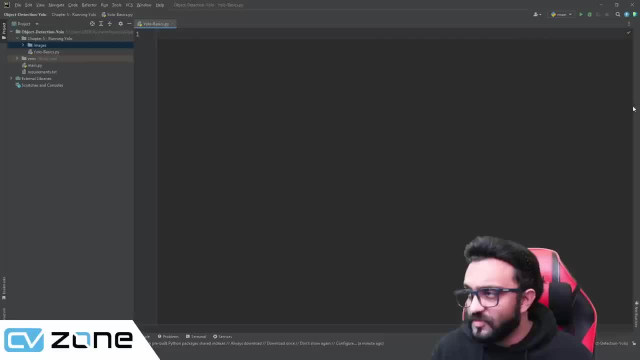 test on. so once we have that, now what we have to do is, first of all we have to import the zip file, and then we have to import the zip file, and then we have to import the zip file, and then we have to import the cel pills. snakes and I draw. 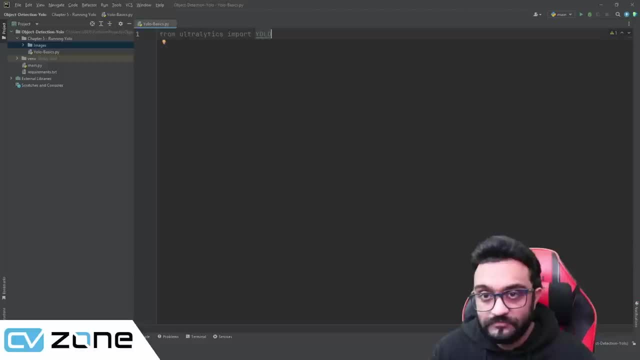 a bullet. you will see how, why we name it. so this is a very simple model. I call this model called ultra latex, which means what ultra latex? so we are going to write: from ultra latex imports Yolo, so that is what we are going to import. and then we also need to import cv2, and I will tell you why. okay, 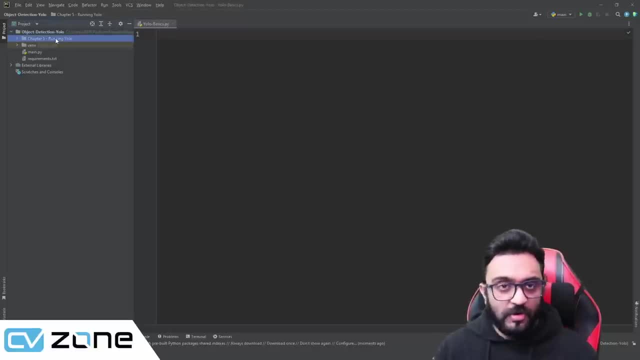 need to have some images, so we are going to run it on images first, once we know it it works. then we are going to try it with webcam in the next chapter. so we have some images again. you will find this on our website. once you download the zip file, everything will be included in it. so here you. 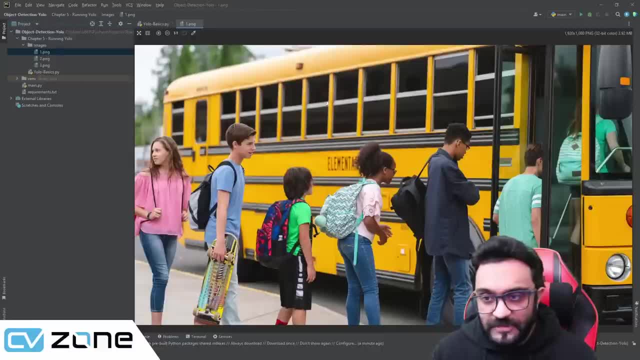 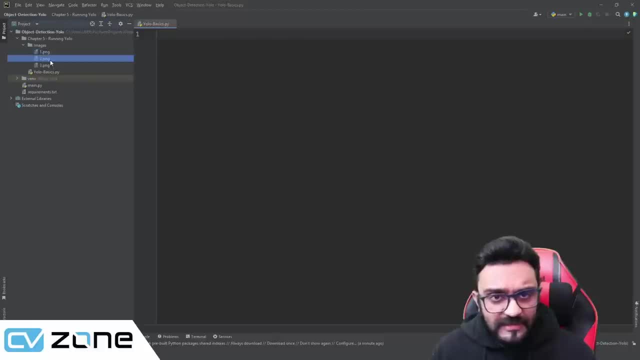 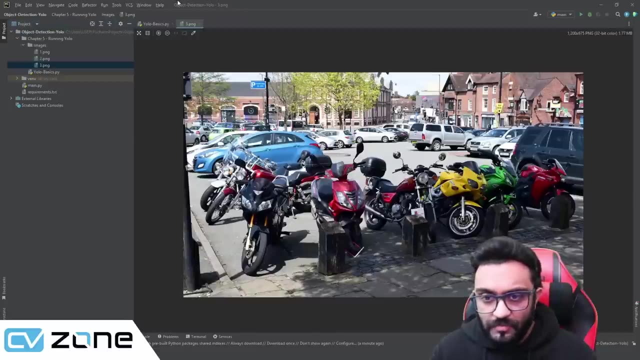 will see. we have images and if you open up images, the first image is of a school bus with some kids going into the school bus, then the second image is of cars and the third image is of some bikes, so motorbikes. so these are the three image images that we are going to test on. so once we have that, 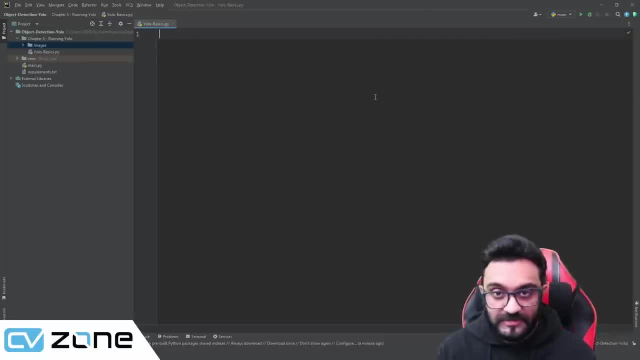 now what we have to do is, first of all, we have to import ultralytics, so we are going to write: from ultralytics imports yolo, so that is what we are going to import. and then we also need to import cv2, and i will tell you why. okay, let's just run it, and i will tell you why later on. 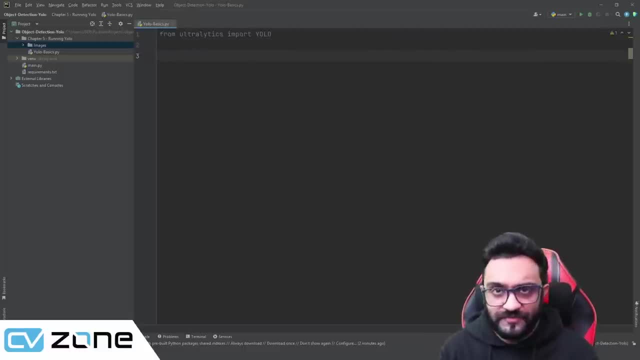 so it is very simple. with only two lines of code, you can simply run your mod. so first of all we are going to create the model we'll call model equals yolo, and then we are going to give in the weights. so there are different types of weights. you have the nano, the 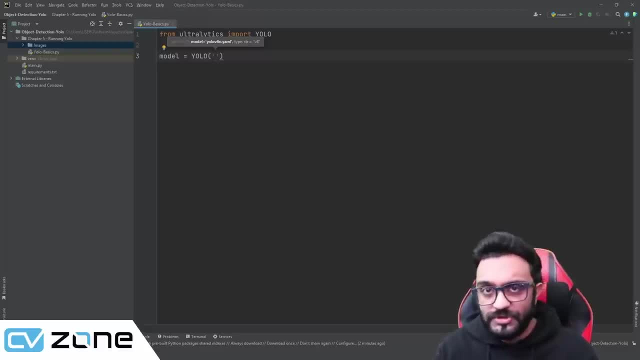 medium, the large- it's based on you- which you want to use. now, the good thing about this method is that you just type in the name of the, the weights that you need, and it will download the weights for you. so, for example, we will write yolo version 8 and we are going to write n for nano. so this: 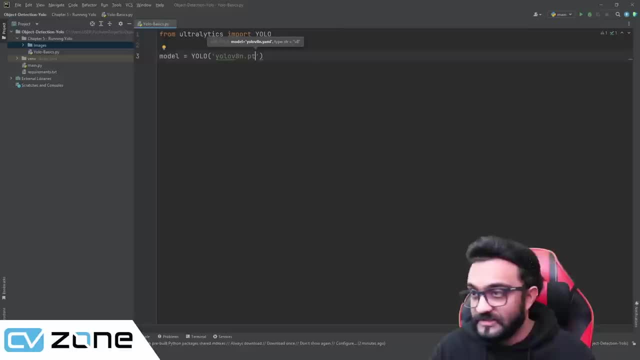 will download the nano version 8 and we are going to write n for nano, so this will download the nano version, so we'll write here pt. then we simply have to write results equals model and then we have to give in the source of the image. so the image source is basically images slash and we can write. 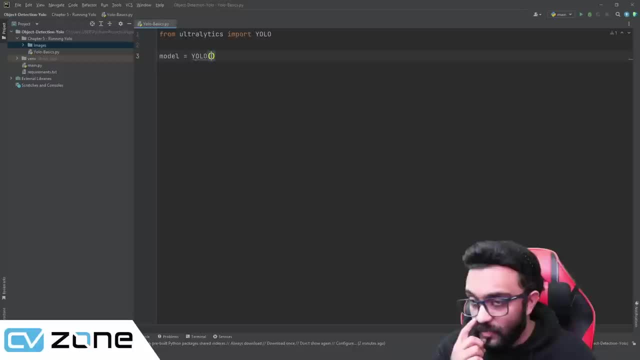 call model equals yolo, and then we are going to give in the weights. so there are different types of weights. you have the nano, the medium, the large. it's based on you which you want to use. now, the good thing about this method is that you just type in the name of the: the weights. 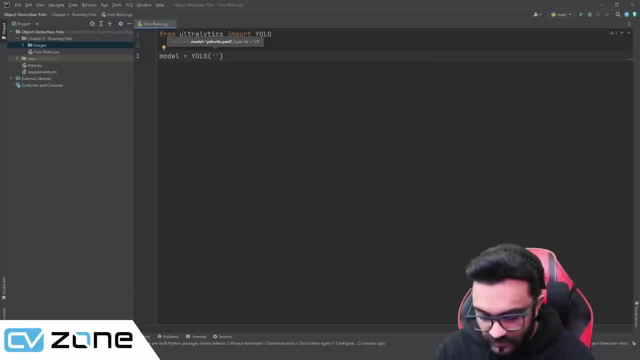 that you need and it will download the weights for you. so for example, we will write yolo version 8 and we are going to write n for nano, so this will download the nano version. so we'll write here pt. then we simply have to write results equals model and then we have to give in the 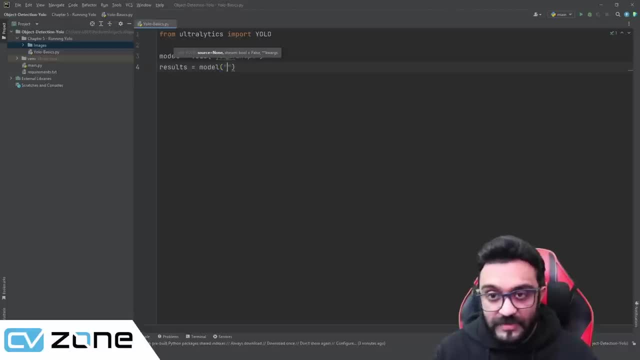 source of the image. so the image source is basically images slash and we can write one dot png. so this is our image, and then all you have to do is you have to write: show equals true. so we want to see the image at the end. so there you go. so if we run this now, right click yolo basics, we are going to run it. 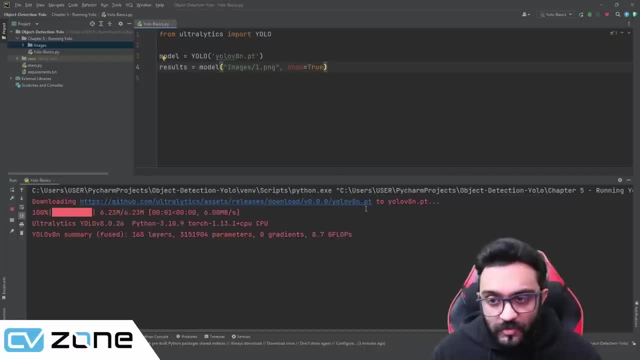 let's see what happens. first of all, it will download the weights. once it's downloaded, it will tell you that it is running on cpu. so that is another thing we are going to discuss later on- how to run it with gpu. but for now nothing happened. it did run the image. it told us that it is running at this. 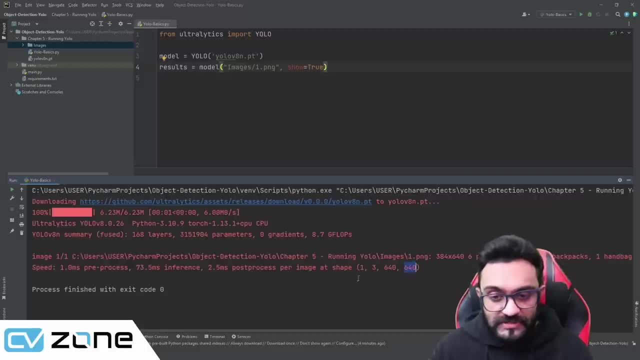 speed and this is the size, but it didn't actually show us anything. so what exactly happened? it actually opened up the image and it closed very quickly because there was no delay. it just opened up and closed. so we need to stop it. so here we go and we have to run the grid. 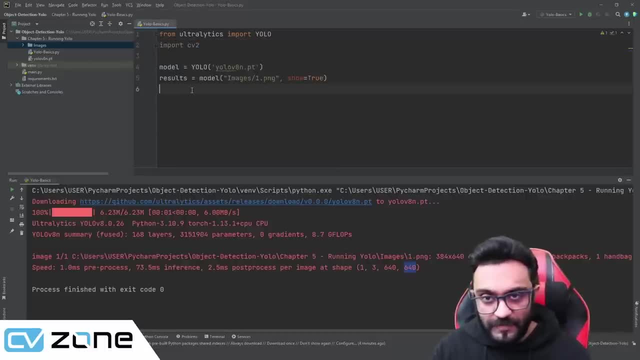 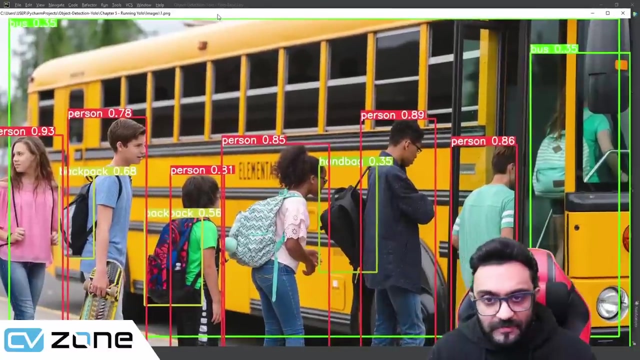 will write import cv2 in order to stop it. we will simply write cv2, dot wait key and will give the delay of zero. zero means that unless the user inputs don't do anything. so if we run this now, this time around, when we run it, this is the image that we get. so we have the bus being detected. we 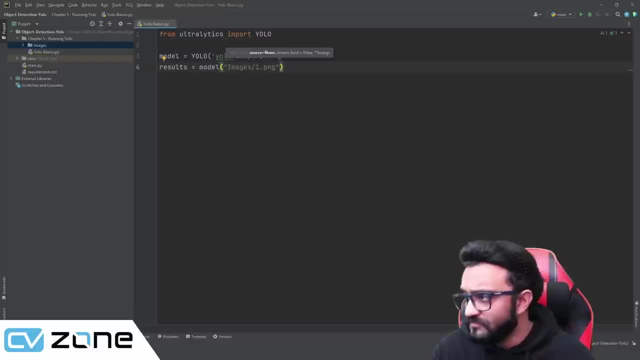 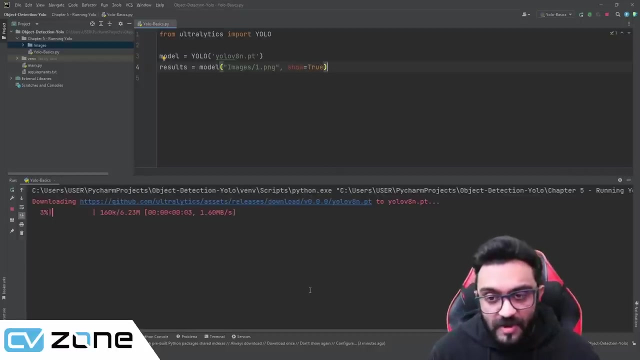 one dot png. so this is our image. and then all you have to do is you have to write: show equals true. so we want to see the image at the end. so there you go. so if we run this now, right click yolo basics. we are going to run it. let's see what happens. first of all, it will download the weights once. 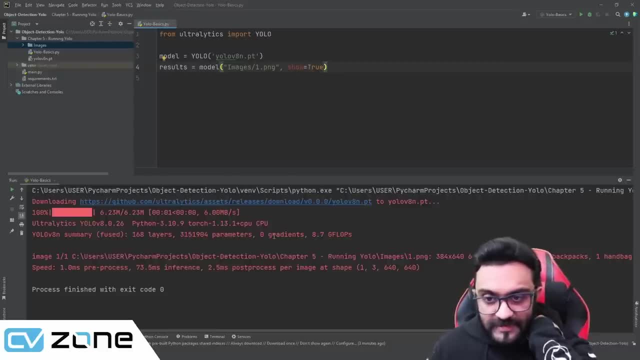 it's downloaded, it will tell you that it is running on cpu. so that is another thing we are going to discuss later on, how to run it with gpu. but for now nothing happened. it did not run the image. it it told us that it is running at this the speed and this is the size. 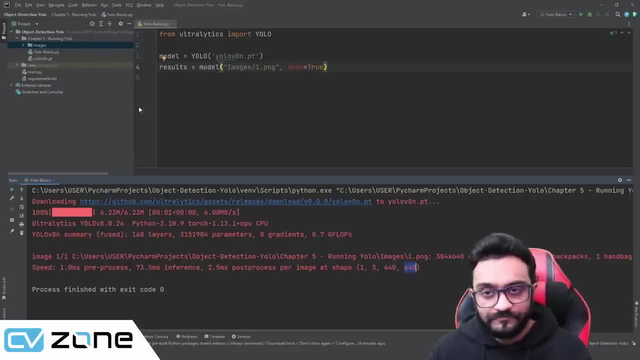 but it didn't actually show us anything. so what exactly happened? it actually opened up the image and it closed very quickly because there was no delay. it just opened up and closed. so we need to stop it. so here we will write import cv2. in order to stop it, we will simply write cv2 dot. 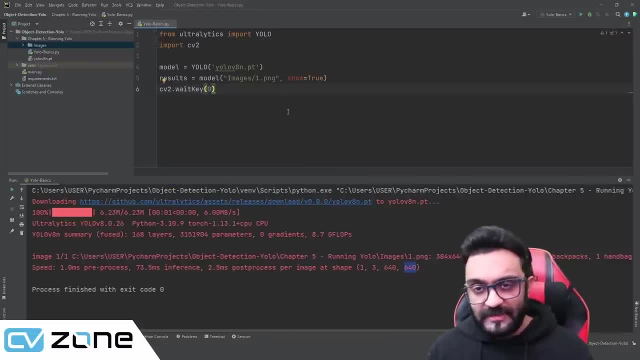 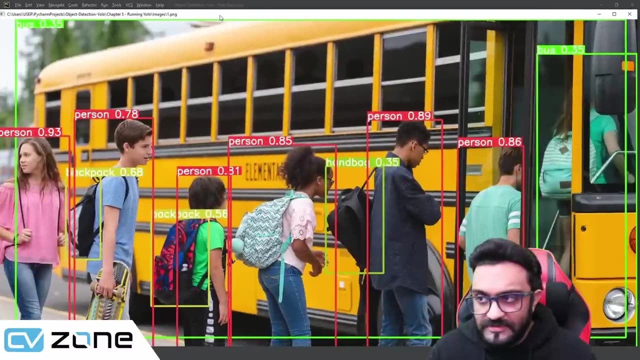 and we'll give the delay of 0.. 0 means that unless the user inputs don't do anything. So if we run this now, this time around, when we run it, this is the image that we get. So we have the bus being. 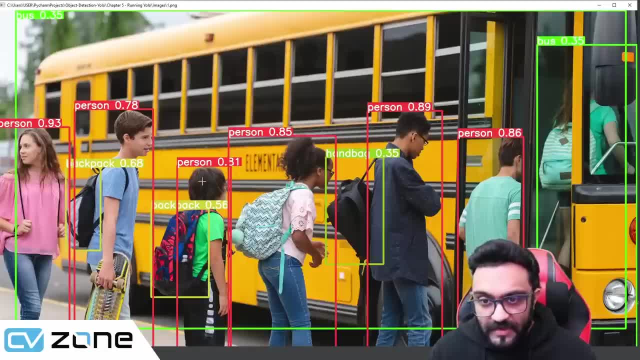 detected. we have the person being detected handbag, backpack, backpack. So there's a lot of good detections here. and they are also giving you the confidence level of each of these, So 0.35, 0.78.. Of course, the higher the confidence value, the better the detection is. So this is quite 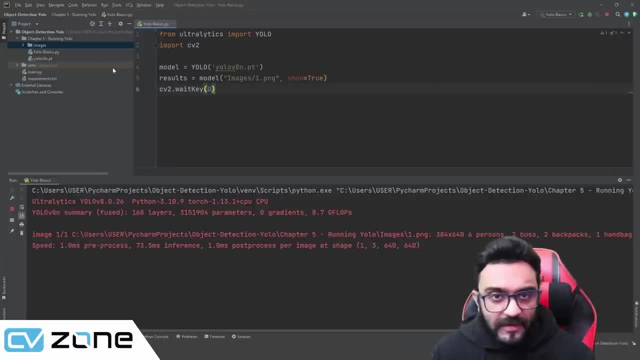 good, We can close that. But here again, you can see that we have downloaded the weights and they are in our chapter five folder Now, in order to make it a little more efficient, we don't want to download it for each chapter, because each chapter or each project we are going to have some weights. 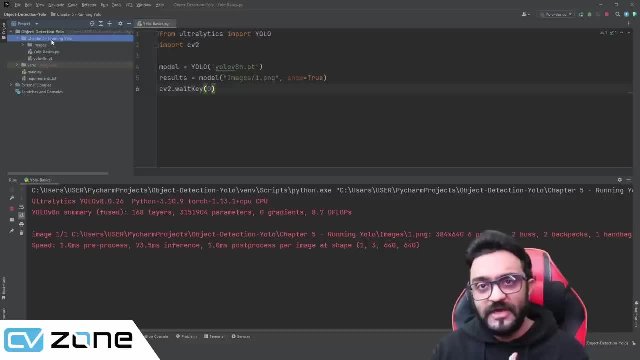 So if we are using the same weights, we should not have it being downloaded every single chapter. So what you can do is you can create a new folder in the object detection YOLO. We will create a new directory and we will call it YOLO weights And we are going to put our weights within YOLO. 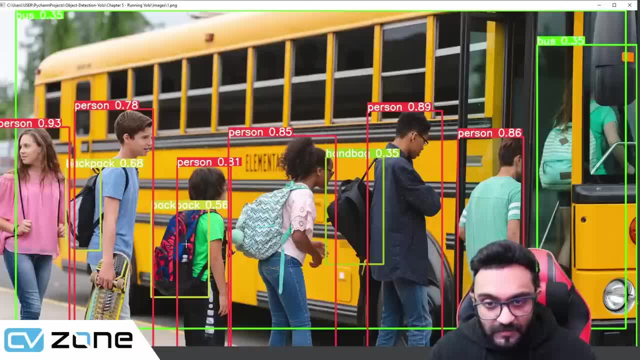 have the person being detected handbag, backpack, backpack. so there's a lot of good detections here and they are also giving you the confidence level of each of these, so 0.35- 0.78. of course, the higher the confidence value, the better the detection is. so this is quite good. we can close that. but here 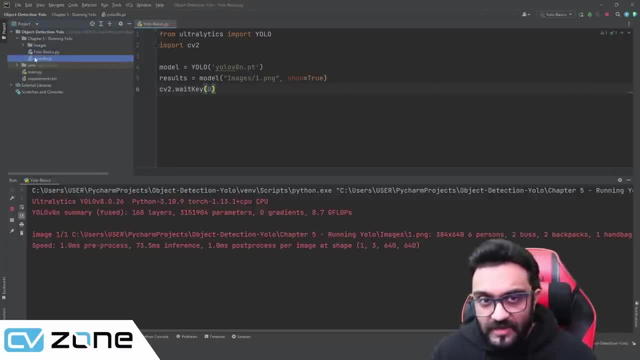 again. you can see that we have downloaded the weights and they are in our chapter 5 folder now in order to make it a little more efficient. we don't want to download it for each chapter, because each chapter has its own weight, and we don't want to download it for each chapter because each chapter 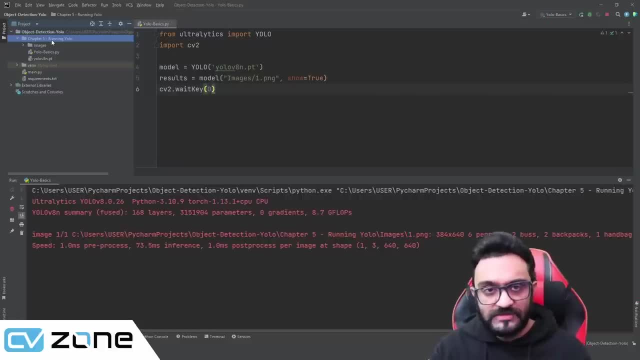 or each project. we are going to have some weights, so if we are using the same weights, we should not have it being downloaded every single chapter. so what you can do is you can create a new folder in the object detection. yolo, we will create a new directory and we will call it. 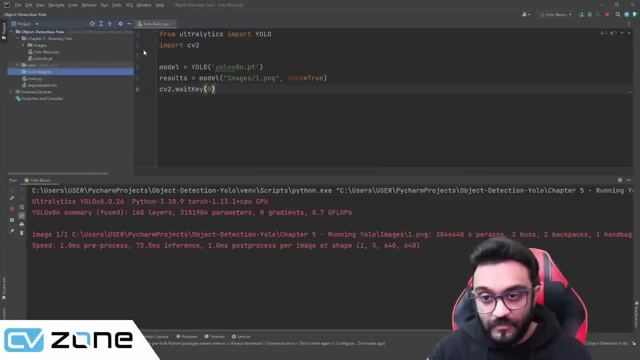 yolo weights and we are going to put our weights within yolo weights when we refactor it. now it's in the yolo weights, so here we can go back. double dot slash, that means go back, and then we will write yolo dash weights, slash. yolo eight, nine, uh, 8n. so if we run this now, it will run. 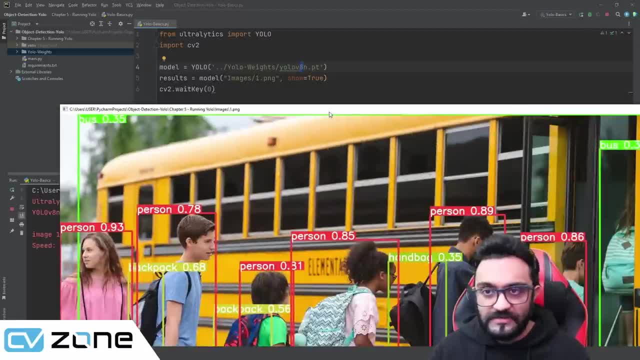 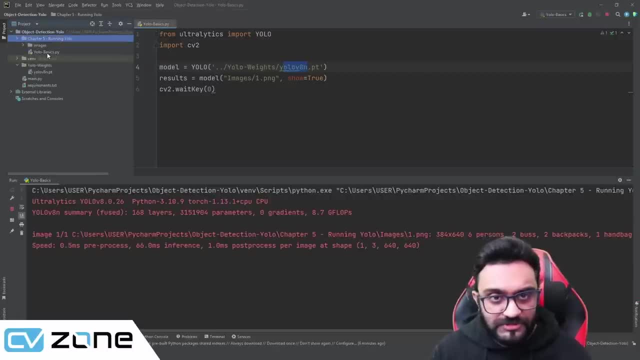 exactly the same way, because it is able to find, uh, this file within this folder. so if you want to try out different uh, what do you call versions of the yolo weights- you can go to the yolo weights folder and you can simply change the name here and you can write, for example, large, and we can try to run. 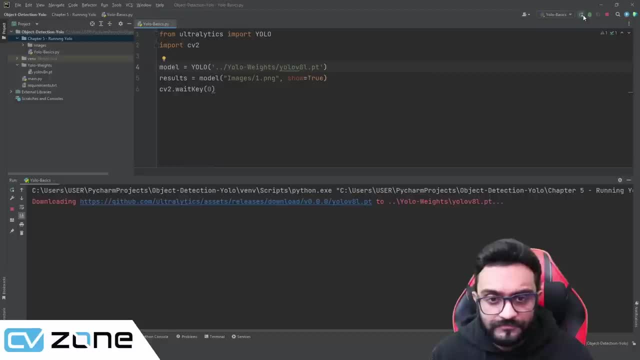 it and see if it works. so it is downloading now and once it's downloaded it should give us the results. so nano will be faster, medium will be a bit slower, large will be slower, and you can check out the other versions as well, which one will be faster and which will be slower. so we will. 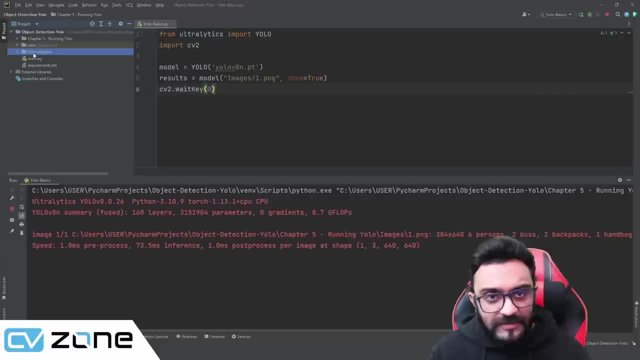 weights When we refactor it. now it's in the YOLO weights. So here we can go back to the YOLO weights And then we can go back double dot slash, That means go back. And then we will write: YOLO dash weights slash YOLO eight, nine, eight N. So if we run this now it will run exactly the. 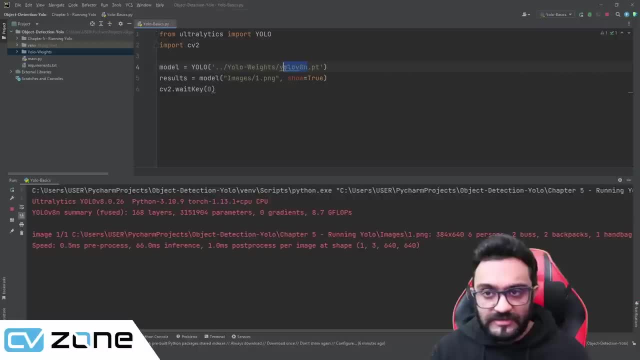 same way, because it is able to find this file within this folder. So if you want to try out different- what do you call versions, you can simply change the name here And you can write, for example, large, and we can try to run it and see if it works. So it is downloading now. 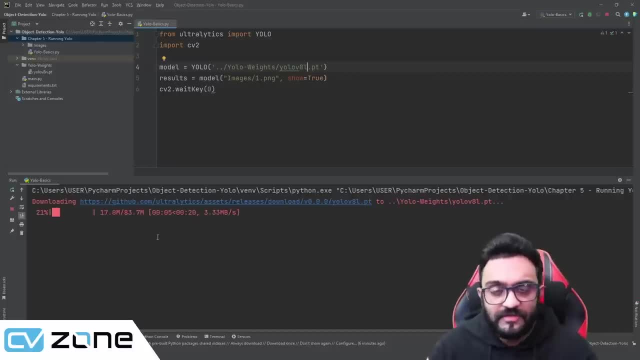 And once it's downloaded, it should give us the results. So nano will be faster, medium will be a bit slower, large will be slower, And you can check out the other versions as well. Which one do you prefer? So this version is 83.. 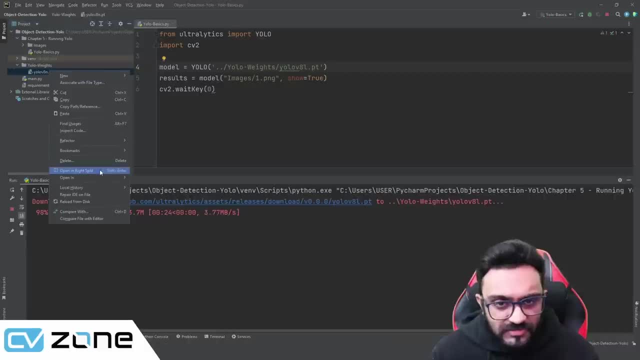 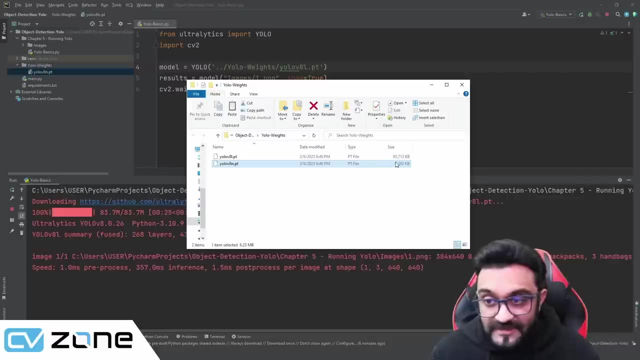 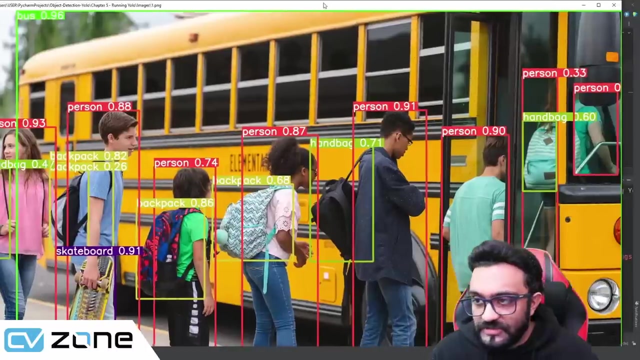 I'm not sure how much was this. Let's open that up. Okay, this one was six MB, So it's a huge difference in terms of weights. So there you go. it has been downloaded And now you can see we are getting better results. We have multiple results here. We also found the skateboard. 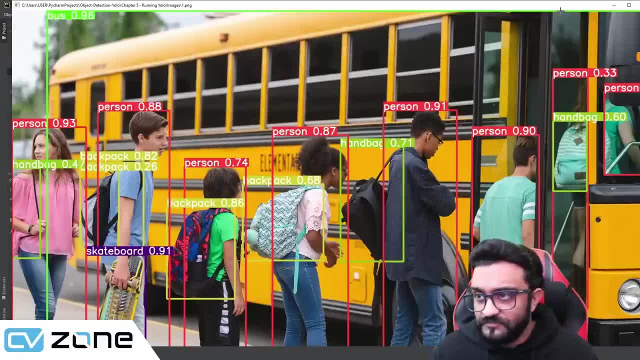 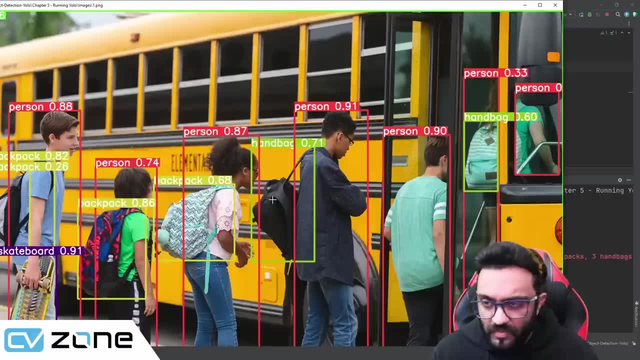 which was not found with the nano version, And there was a wrong detection here for the buzzer. So we are getting better results. We have multiple results here. We also found the bus. that is not detected as well, But here it's saying handbag when it's a backpack. So that is. 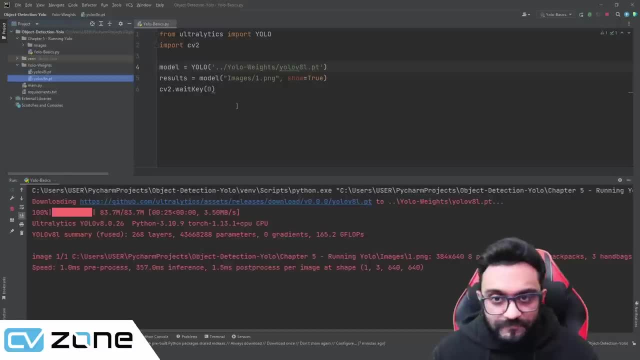 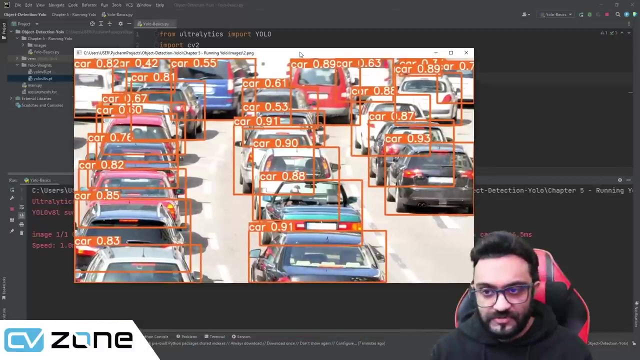 still a mistake, but it works fine. So there you go. So this is how you can download and you can run the models. So what we can do now is we can run imagespng2.. So let's see how that works. So there you go. So you have lots of cars being detected. 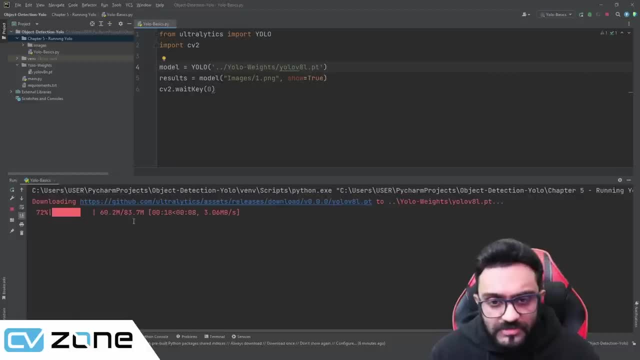 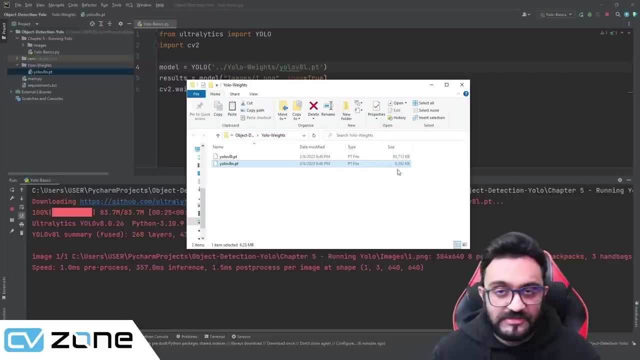 see which one, uh, do you prefer? so this version is 83 mbs. i'm not sure how much was this. let's open that up. okay, this one was 6mb, so it's it's a huge difference in terms of weights. so there you go, it has been downloaded and now you can see. 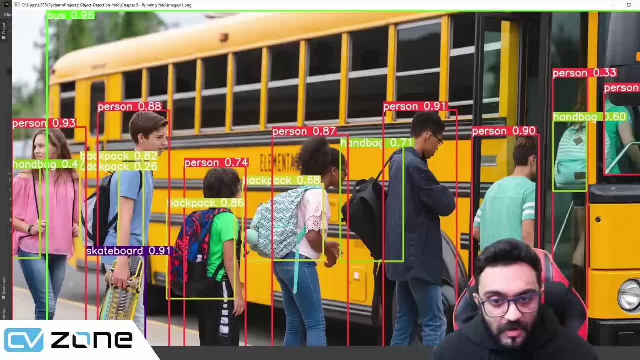 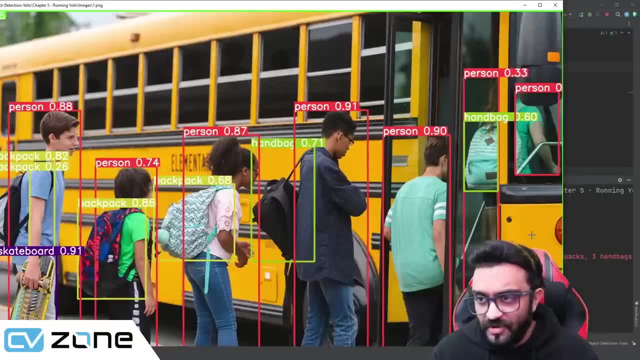 we are getting better results. we have multiple results here. we also found the skateboard, which was not found with the nano version and there was a wrong detection here. for the bus that is not detected as well, but here it's saying handbag when it's a backpack. so that is still a mistake, but it 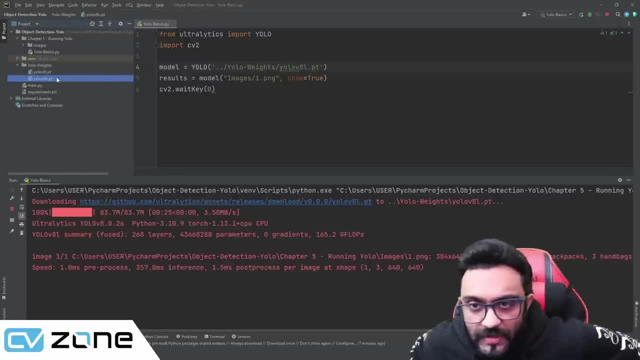 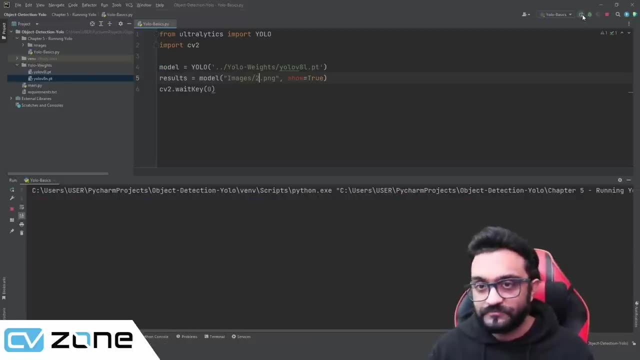 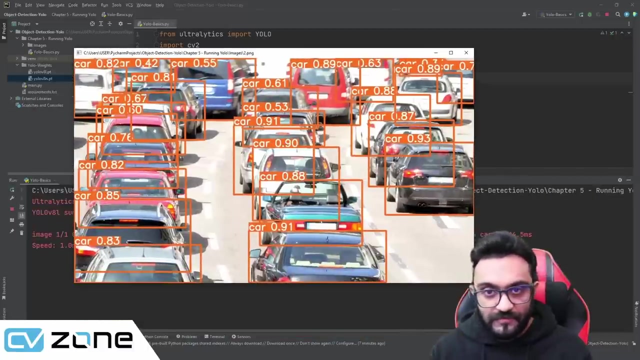 works fine. so there you go. so this is how you can download and you can run the models. so what we can do now is we can run images dot PNG 2, so let's see what that how that works. so there you go. so you have lots of cars being detected, some with confidence of 0.88, some with 0.85, some with 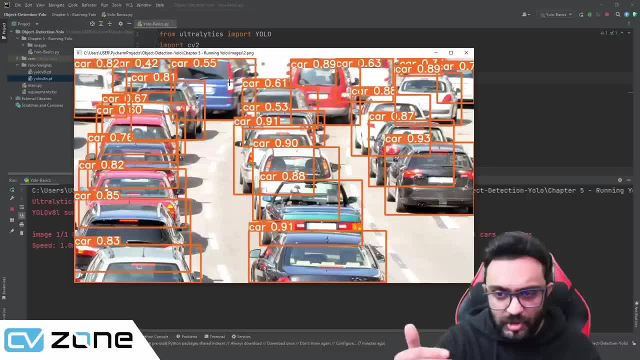 0.67, you can. you can see the pattern. the closer it is to the camera, it actually detects it very well. the further it is from the camera, it might not detect. basically, the idea is, how clear is the sight of viewing? so if it's able to detect, if it's, 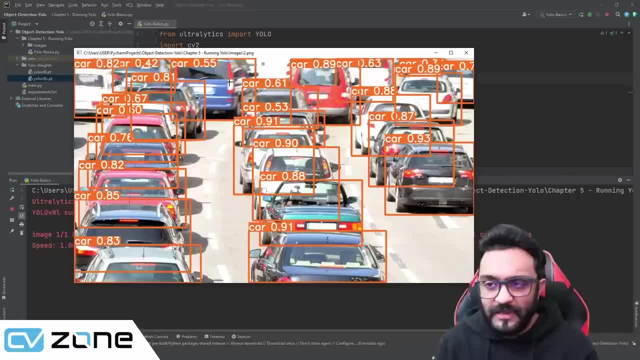 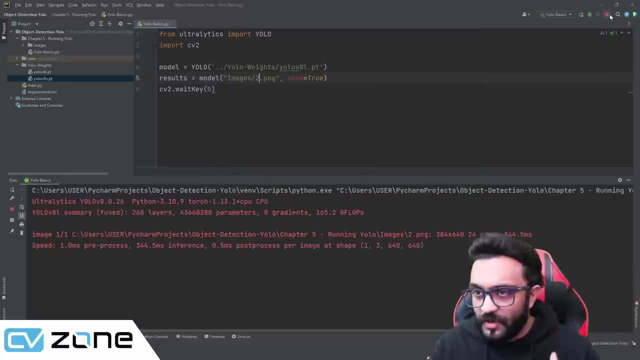 able to find the car a bit more. it will be easier to classify, it will be easier to detect and the confidence level will be higher. but if it's far, if it's blur, then of course the confidence level will not be that much. so that's the basic idea, and then we'll go to images 3 and let's see how. 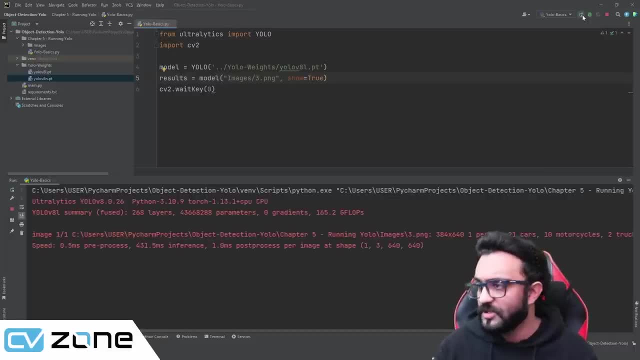 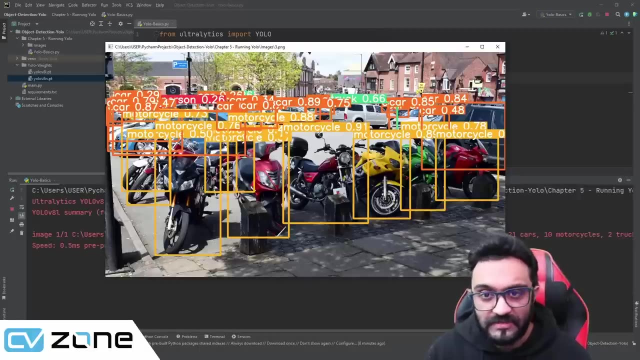 that works out. so right now we are using the large version and you can use the Nano version as well. okay, there you go. so here we have a lot of detections, motorcycles and we have a truck. at the back, we have a person and they are overlaying on each. 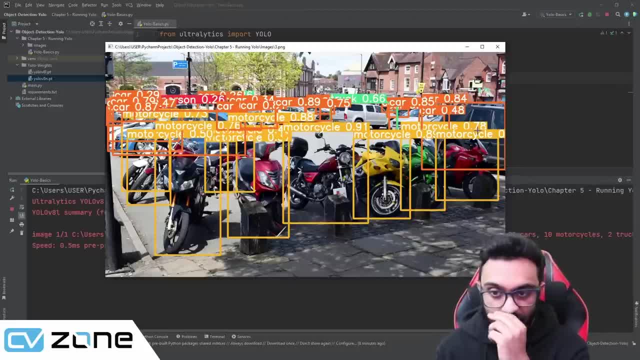 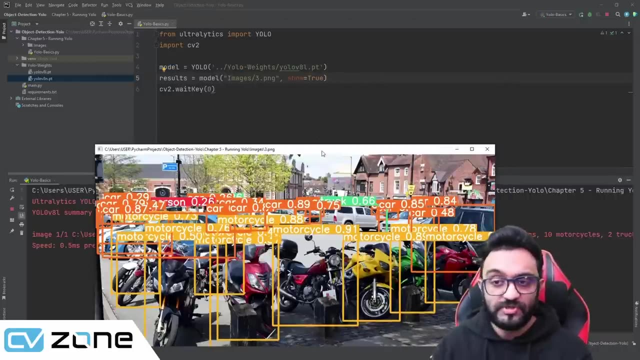 other and it's a little bit difficult to see what exactly is going on. and right now we are not really detect, we are not really telling the system, um, that put these bounding boxes and put the names and the confidence level. this is done by default. when you are saying show equals true, then it's. 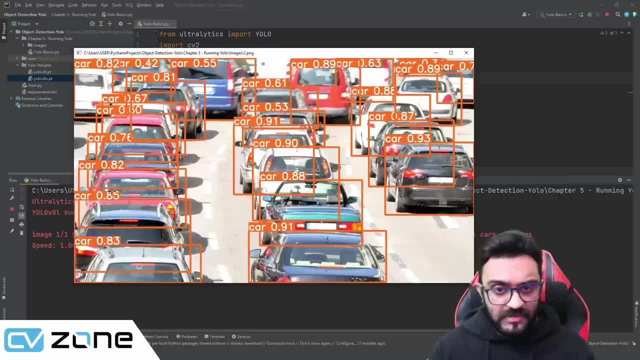 Some with confidence of 0.88, some with 0.85, some with 0.67.. You can see the pattern. the closer it is to the camera, it actually detects it very well. The further it is from the camera, it might not detect. Basically, the idea is: how clear is the site of viewing? 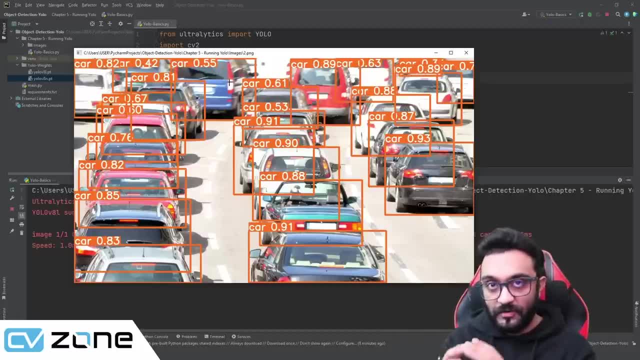 So if it's able to detect, if it's able to find the car a bit more, it will be easier to classify, it will be easier to detect And the confidence level will be higher. But if it's far, if it's blur, then of course 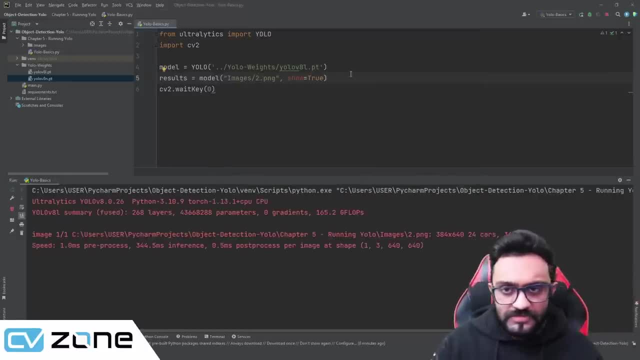 the confidence level will not be that much. So that's the basic idea, And then we'll go to images three And let's see how that works out. So right now we are using the large version And you can use the nano version as well. Okay, there you go. So here we have a lot of detections. 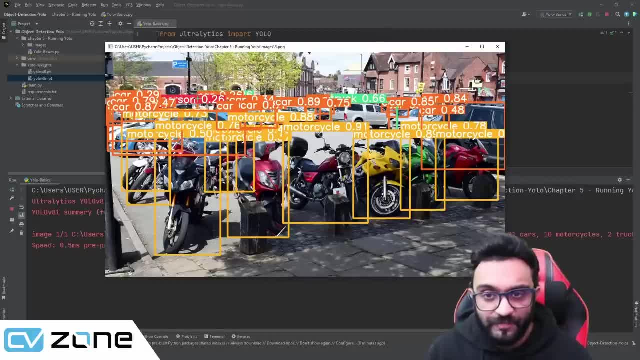 motorcycles and we have a truck, at the back We have a person, and they are overlaid on each other And it's a little bit difficult See what exactly is going on. And right now we are not really detect, we are not really telling. 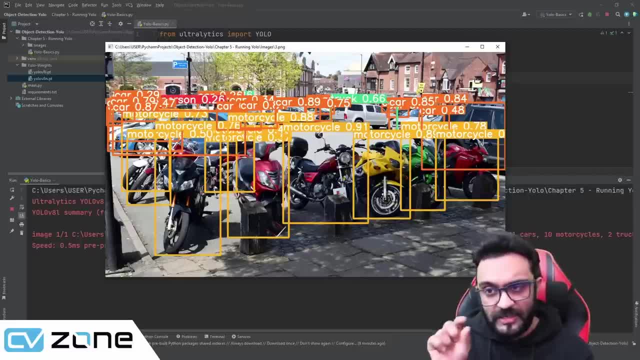 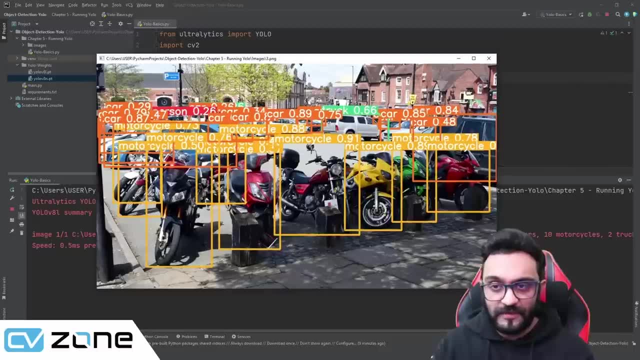 the system that put these bounding boxes and put the names and the confidence level. This is done by default. When you are saying show equals true, then it's doing all of that. So what later on? what we'll do is in the in the next chapter, we are going to put all of these manually ourselves. 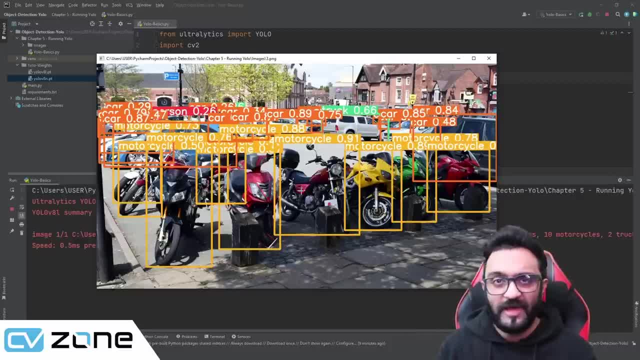 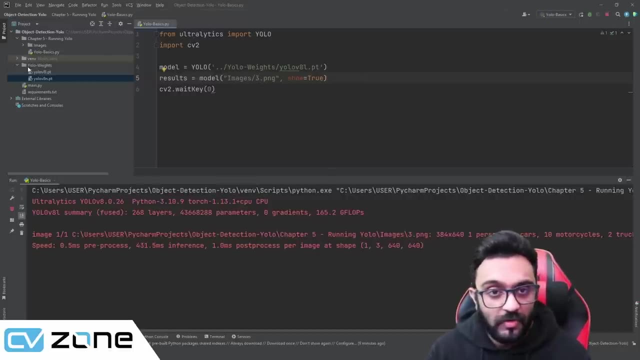 we will not use the default version, And that way we will have much more control on how we can see what's going on. So right now they are overlaying on each other and it's not very clear, So it's not very useful in terms of viewing. So that's the basic idea. That's how we can run different. 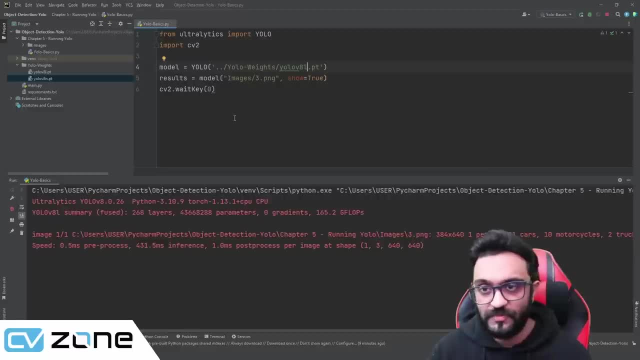 versions of YOLO: The large, the nano, the small, the medium. So here, if we write M, by the way, I wanted to check if we run it with the nano, what exactly happens. How many detections do we get? 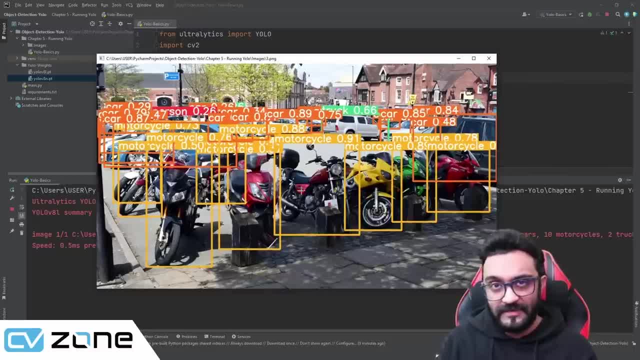 done, so what? later on? what we will do is, uh, in the, in the next chapter, we are going to put all of these manually ourselves. we will not use the default version, and that way we will have much more control on how we can see, because right now they are overlaying on each other and it's not 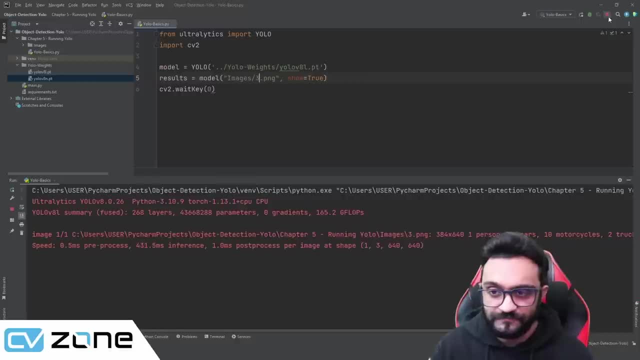 very clear, so it will. it's not very useful in terms of viewing. so that's the basic idea. that's how we can run different versions of Yolo uh- the large, the Nano, the small, the medium. so here if we write M? uh. by the way, I wanted to. 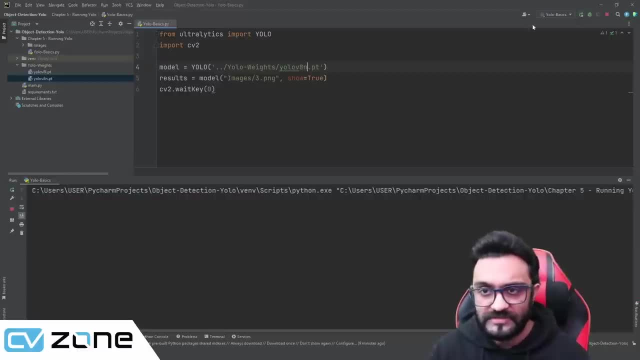 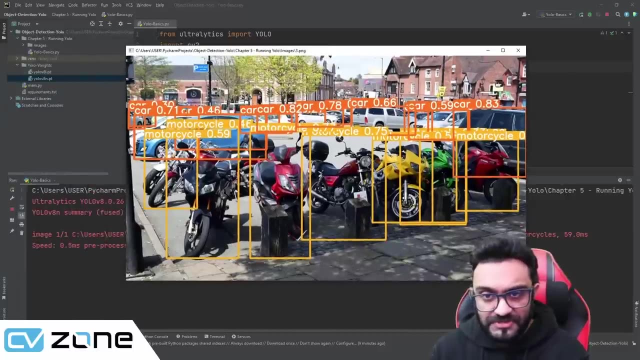 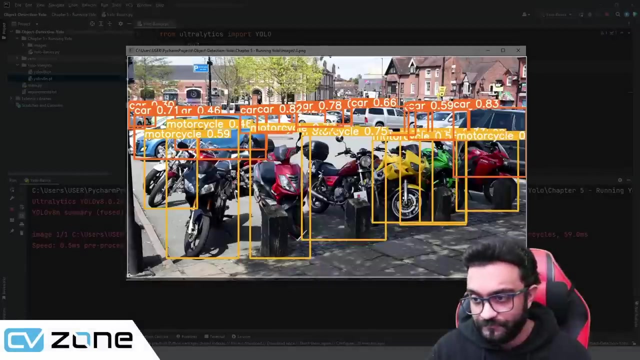 check if or we run it with the Nano, what exactly happens? how many detections do we get? so there you go. so it says a car, car, and the person is not detected. that was detected earlier. and actually, let me, let me take a screenshot of this and I will open it up in paint. 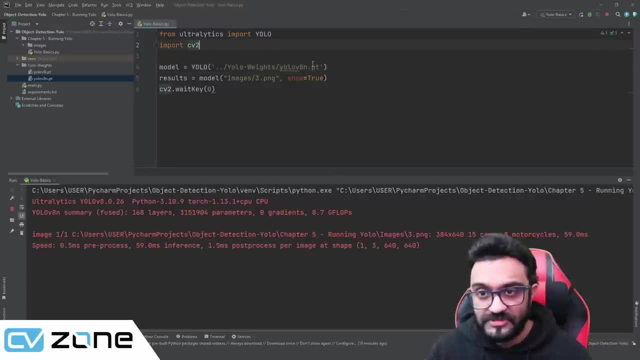 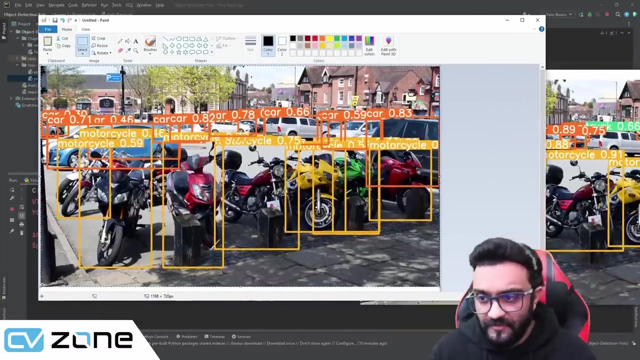 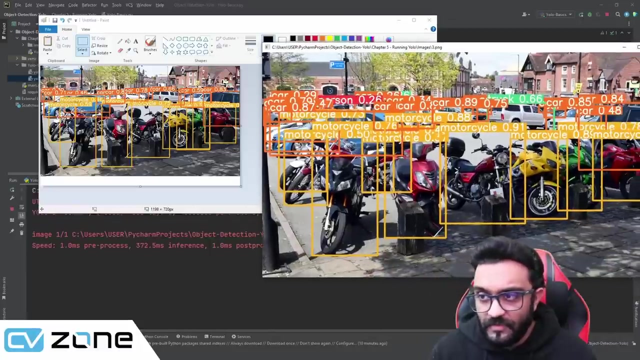 so this is the one with the Nano, and let's run it with large and then we will compare. that will be a fun experiments. uh, exactly how much are we getting when we are using the heavier version? okay, so here you can see. we do have, can we? yeah, so here you can see. we don't see the truck. uh, we have some motorcycles. 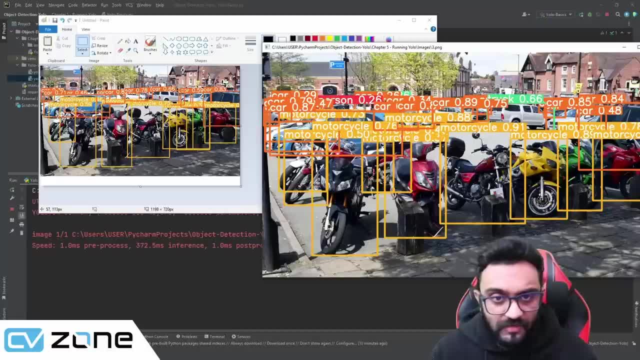 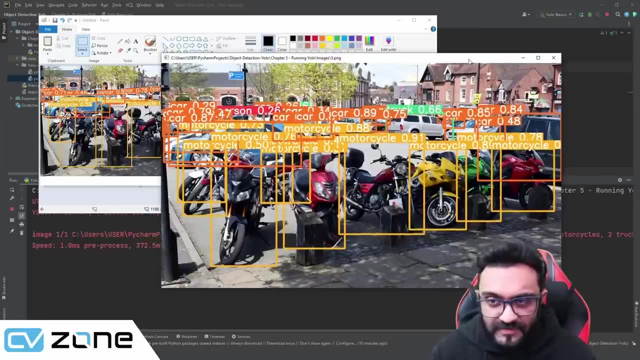 cars are limited here. here we have more cars, here we have less, and here we have a red which is for a person, here we don't, and here there's another truck at the back which is green. we don't get that. so, yeah, definitely we are getting more, but is it correct or not? that is yet to be seen. so, based on 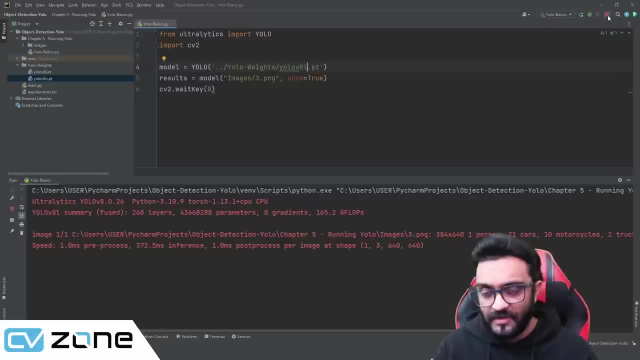 your requirement, whether you want it fast or whether you want it highly accurate. again, all of these methods, all of these versions, they are good, not in a very general sense, but if you have a controlled environment, for example, you're detecting cars or you're detecting uh pedestrians in in a fixed environment with a 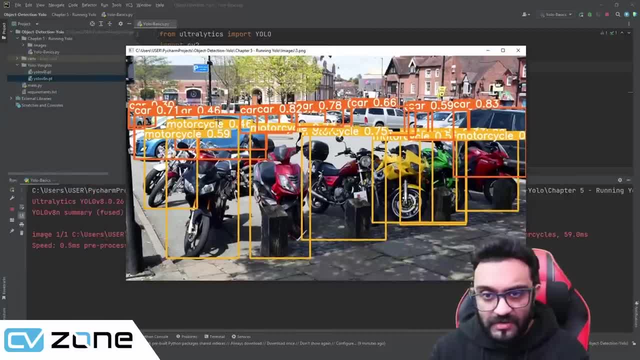 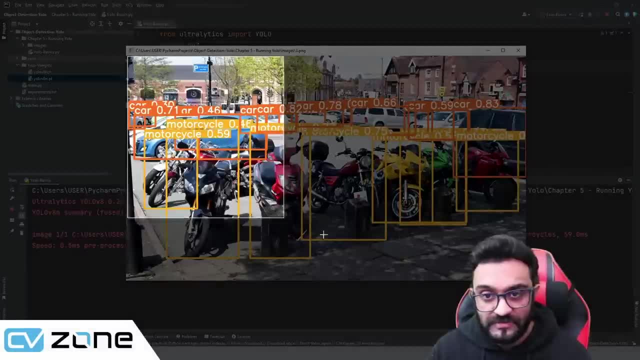 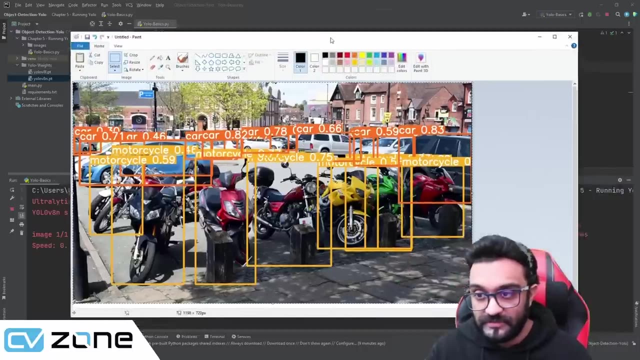 So there you go. So it says a car, car, and the person is not detected. that was detected earlier And actually, let me, let me take a screenshot of this And I will open it up in paint. So this is the one with the nano And let's run it with large and 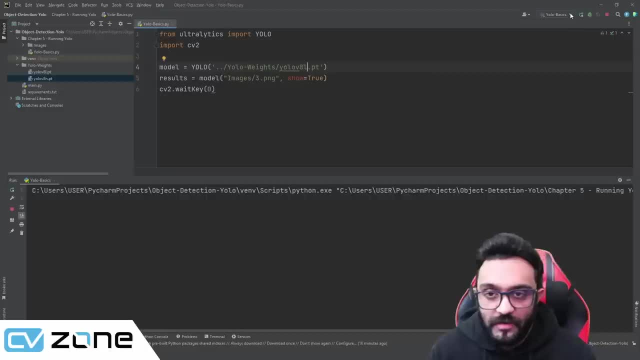 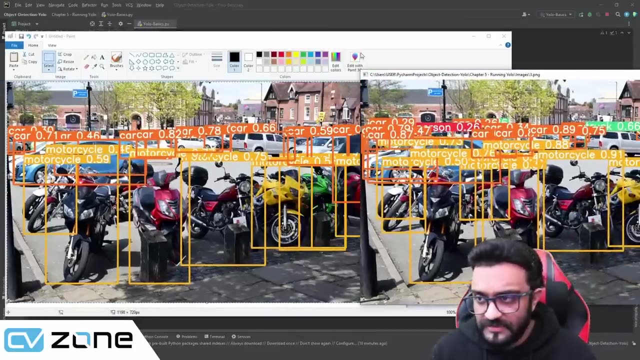 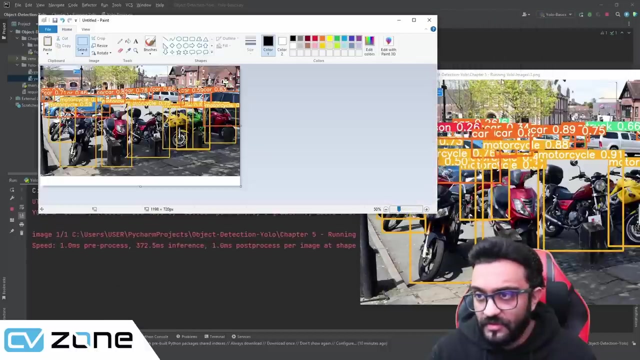 then we will compare. that will be a fun experiments. Exactly how much are we getting when we are using the full version? Okay, so here you can see we do have, can we? Yeah, so here you can see. we don't see the truck. 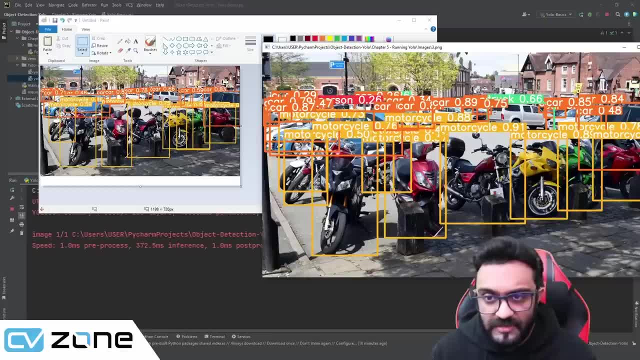 We have some motorcycles. the cars are limited here. Here we have more cars, here we have less. And here we have a red which is for a person, here we don't. and here there's another truck at the back which is green. 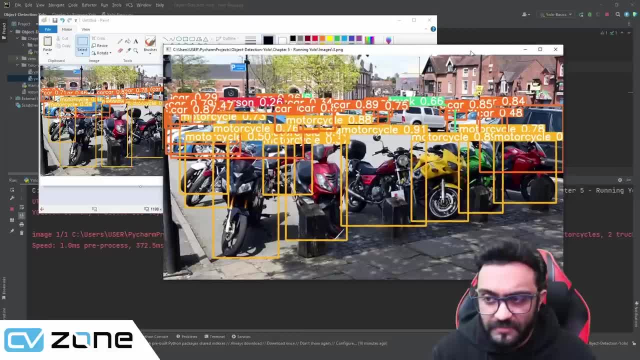 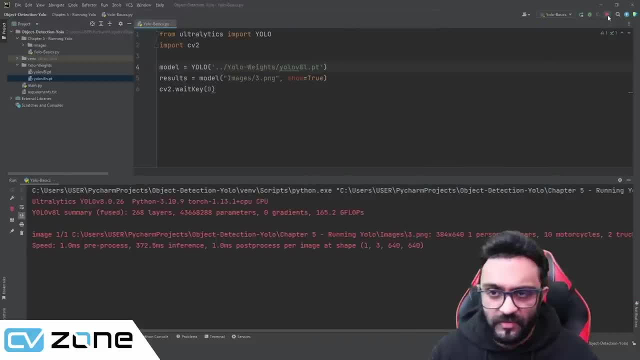 We don't get that. so, yeah, definitely we are getting more, but is it correct or not? that is yet to be seen. so, based on your requirement, whether you want it fast or whether you want it highly accurate, again, all of these methods, all of these versions, they are good, not in a very general sense, but if you have 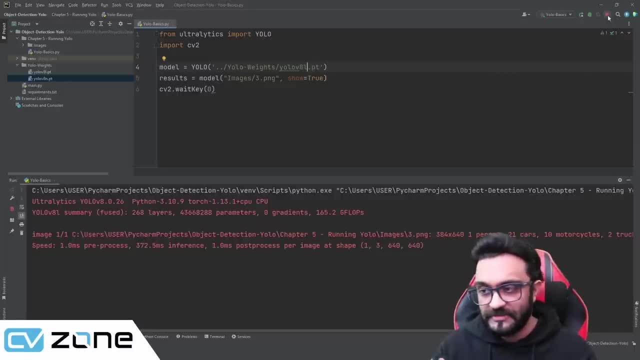 a controlled environment, for example, you're detecting cars or you're detecting pedestrians in in a fixed environment with a fixed camera, then, yes, it can be very useful. you can have certain limitations, certain constraints, some certain constants that this, this will always be this. you can add a mask that do not detect in these regions, only detect in these regions. 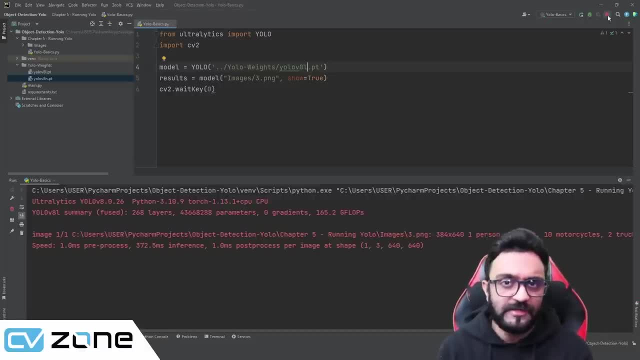 and things like that. it will definitely be useful to put it in your project. so that is exactly what we are going to do. first of all, we are going to run it with our webcam, and then later on we will try it with our webcam, and then, later on, we will try it with our webcam, and then later on, we will 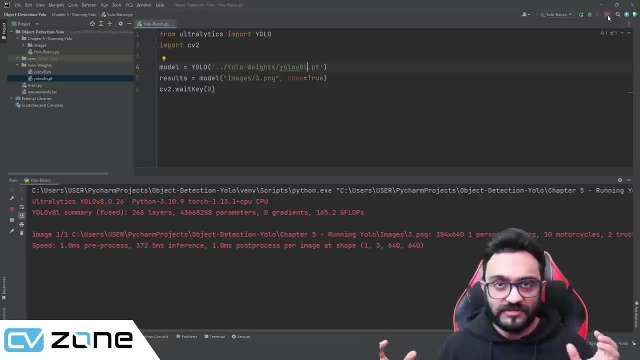 fixed camera, then, yes, it can be very useful. you can have certain limitations, certain constraints, some certain constants that this will, this will always be this. you can add a mask that do not detect in these regions, only detect in these regions, and things like that. it will definitely be. 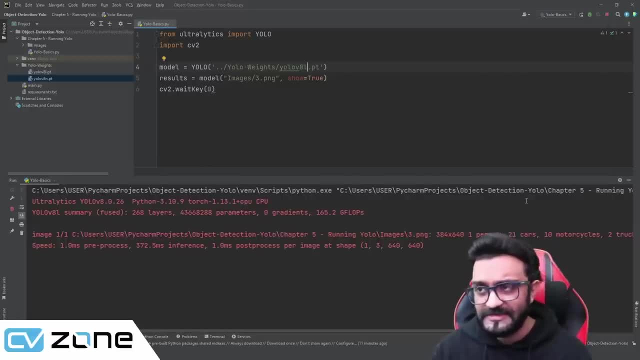 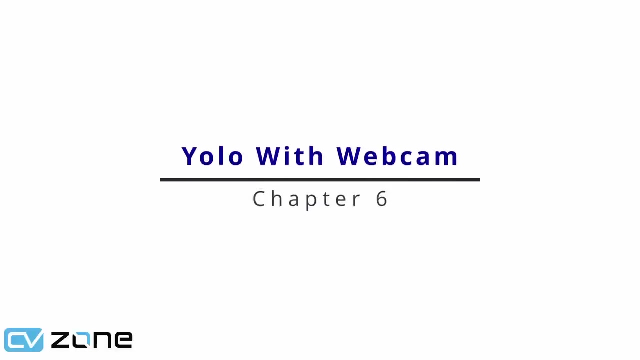 useful to put it in your project. so that is exactly what we are going to do: first of all, we are going to run it with our webcam, and then, later on, we will try it with different projects- how we can implement this in real time. so now, in chapter number six, we are going to run Yolo with our webcam. 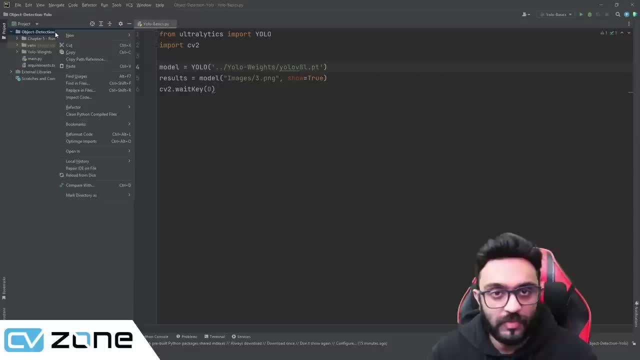 so let's see how we can do that. so we are going to need the help of open CV in this case, and we are going to put bounding box ourselves manually so that it is easier for us to decide what to display and what not to display. so what we'll do is, first of all, we'll go to, we'll go to new and directory. 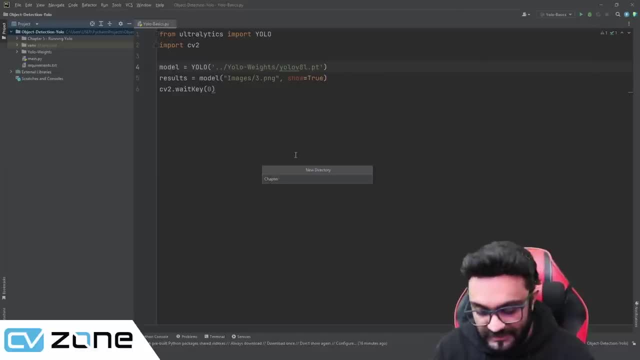 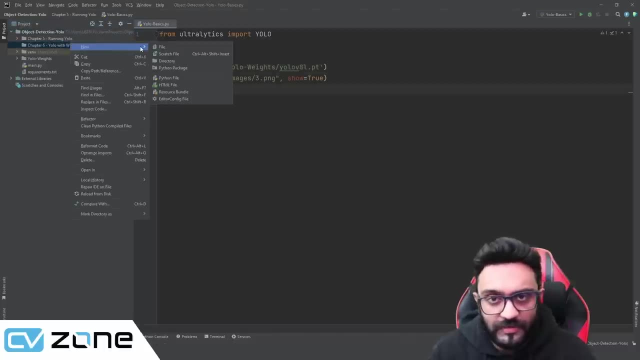 and then we are going to write chapter six, and chapter six is Yolo with webcam. so then we are going to right click and we are going to create a new python file and we will call it Yolo webcam. so first of all, we are going to import ultralytics, as we did earlier, and we also have to import 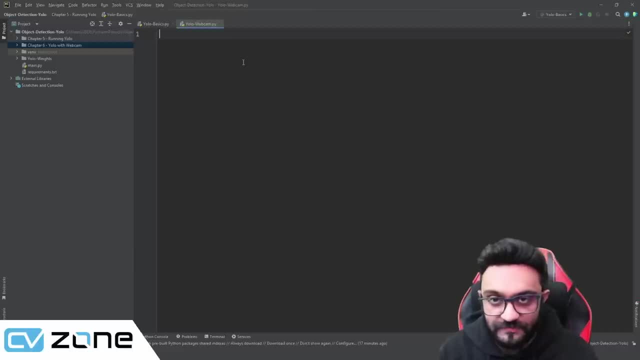 python. so we will uh, not python, open CV. so we will write: from ultralytics, import Yolo, and then we will write uh, imports, imports, CV2, and then we will also import CV zone. so CV zone we will be using to actually display all these, um, what you call Detections, it. 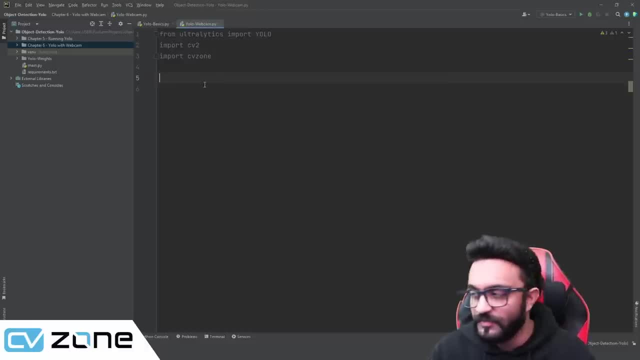 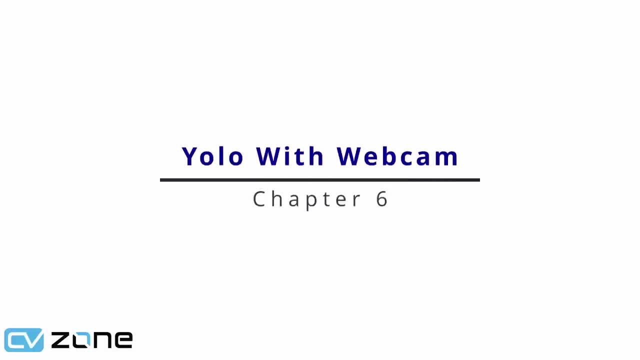 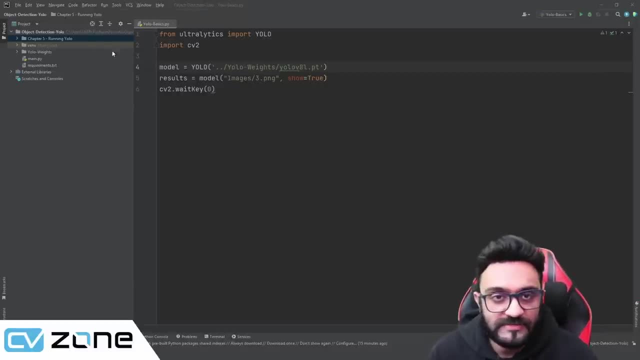 so now in chapter number six, we are going to run yolo with our webcam, so let's see how we can do that. so we are going to need the help of opencv in this case and we are going to put bounding box ourselves manually, so that it is easier for us to decide what to display and what not to display. 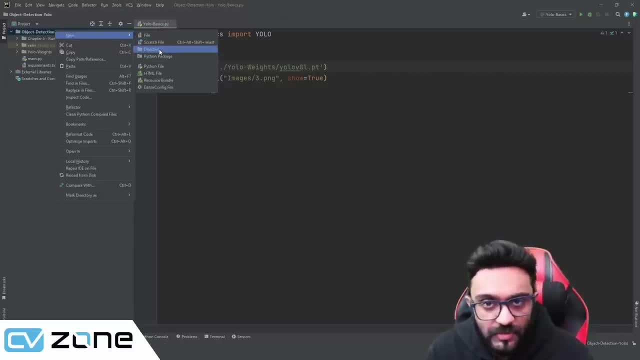 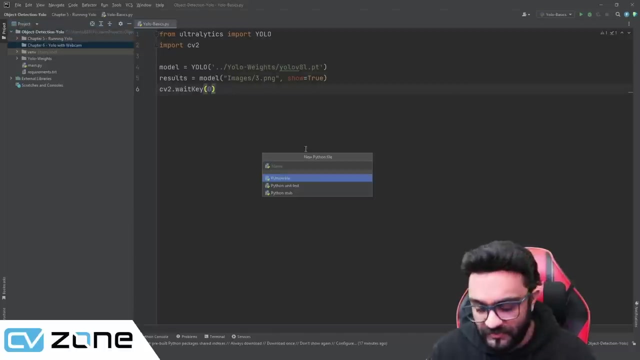 so what we'll do is, first of all, we'll go to, we'll go to new and directory, and then we are going to write chapter six, and chapter six is yolo with webcam. so then we are going to right click and we are going to create a new python file and we will call it yolo webcam. so first of all, 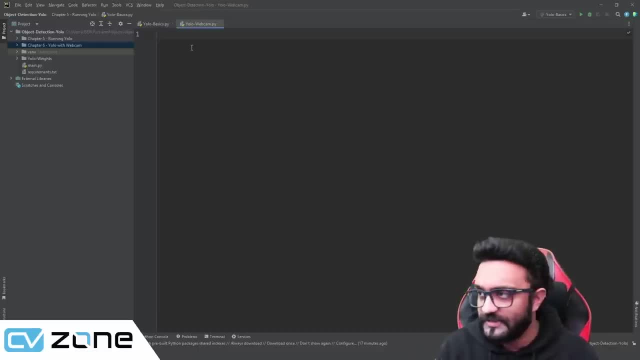 we are going to import ultralytics, as we did earlier, and we also have to import python. so we will uh, not python, opencv. so we will write: from ultralytics, import yolo, and then we will write uh, imports, imports, cv2. and then we will also import uh cv zone. so cv zone we will be using to actually display. 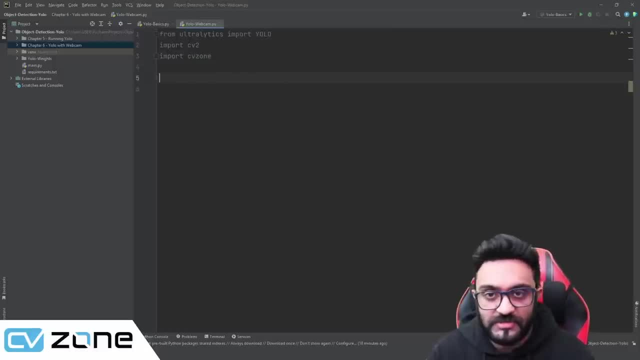 all these, um, what do you call them? we will call detections. uh, it will make it a little bit easier. you don't have to, but it will make a little bit easier. so the first thing we will do, we will create the webcam object. so we'll write: cap equals uh, cv2, dot, video capture. so this is what i was referring to earlier. so, if you are, 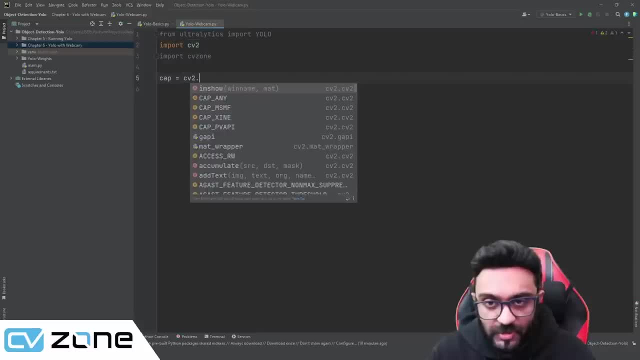 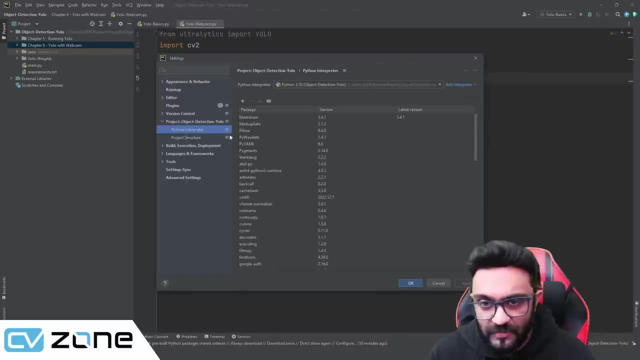 not getting any suggestions. so if you write dot video and you don't get any suggestions, then it means you probably are using a newer version of of opencv. so- and this is the issue that we are getting with the newer versions, so where is it? opencv, opencv. 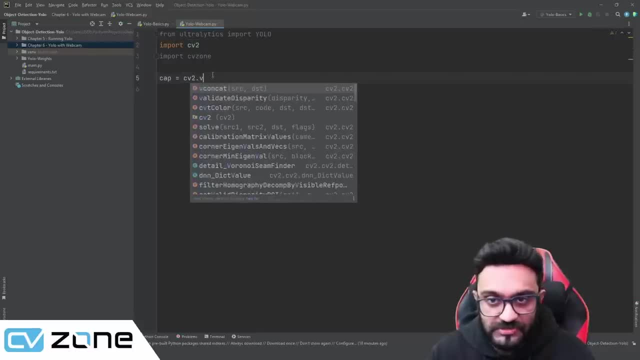 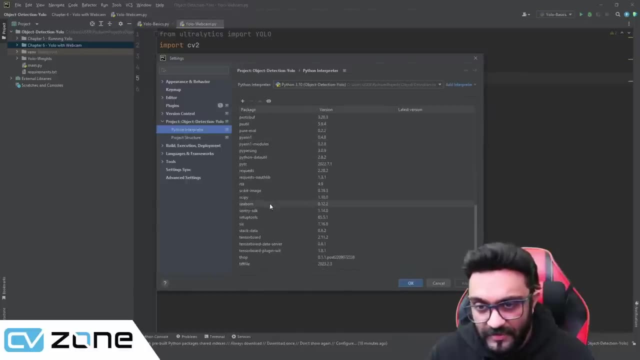 you will write dot video and you don't get any suggestions, then it means you probably are using a newer version of python of open CV. so- and this is the issue that we are getting with the newer versions- so where is it? open CV, open CV, there you go. so open CV. as you can see, we are using version. 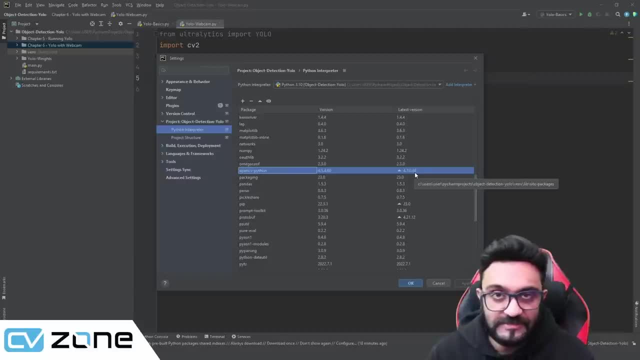 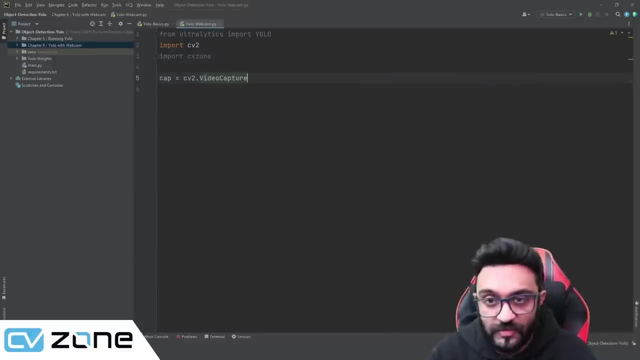 4.60, whereas 6: 8 is the latest version. still 6, 8 has this issue. that's why we are using 6: 0.. so we will write CV2 dot video capture and the video capture ID. basically, you have to give in the ID number for your webcam. I'm using multiple. 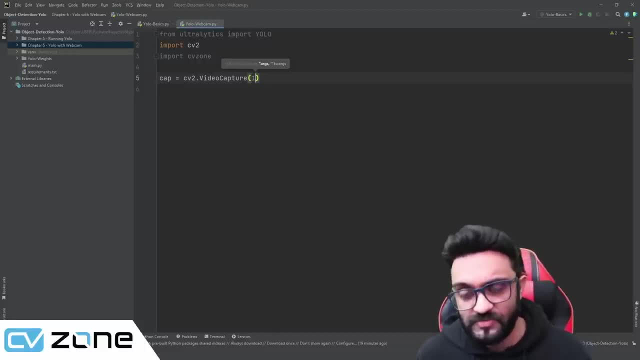 webcams. so I will give the ID number one, because that is what I am going to use. but if you are using only one webcam, if you don't have multiple webcams installed, then you should write zero instead of one. so I will write here one and then you can specify cap dot set. you are going. 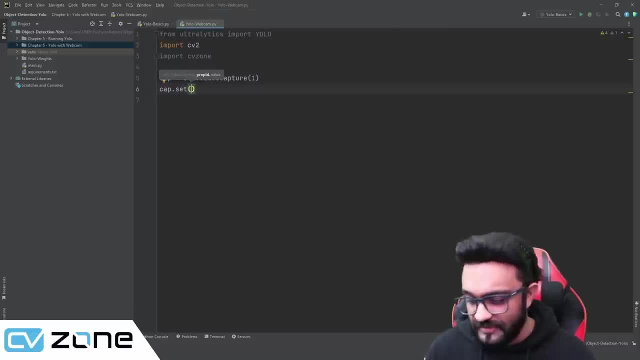 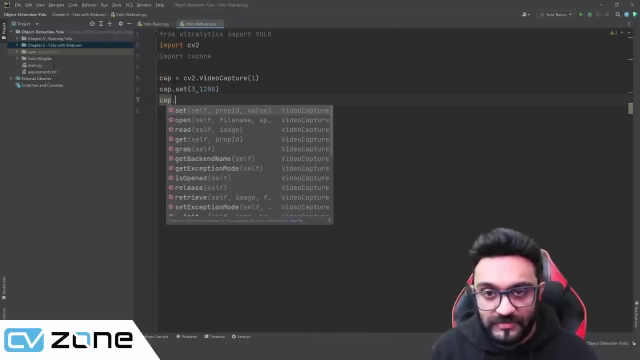 to set the width and the height. so the width, uh, basically, is prop ID number three, so you can write 1280. this is the width, and cap dot set. that is the prop ID number four, that is 720.. so this is the height and we are going to set it at 720.. so this is the basic idea and again, if you wanted, 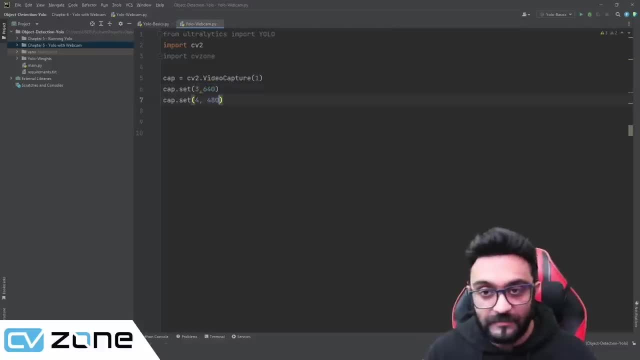 to. there's another one which is mostly used in webcam: 640 by 480. these dimensions are commonly used, so it's up to you which one you want to use. then we are going to write while true, and we are going to write success, and the image equals cap dot read. and then we 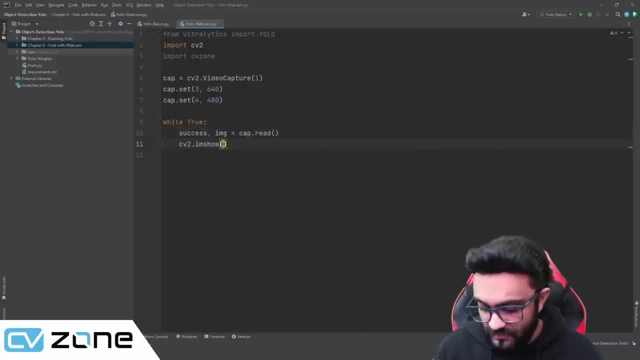 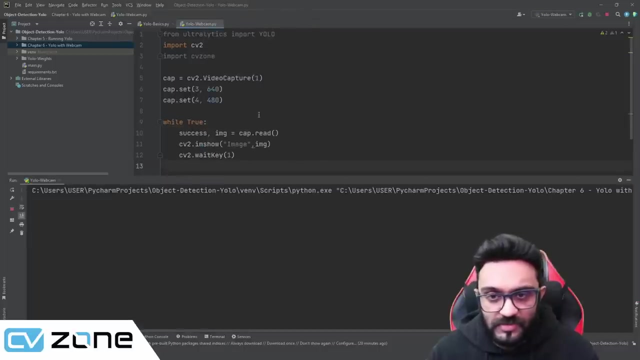 are going to write cv2 dot im show. we want to show the image. so we will write image and img- that is the image we want to show- and cv2 dot wait key, because we want to give it one millisecond delay. so this should run our webcam by default. so if we right click and run, we should have our webcam. 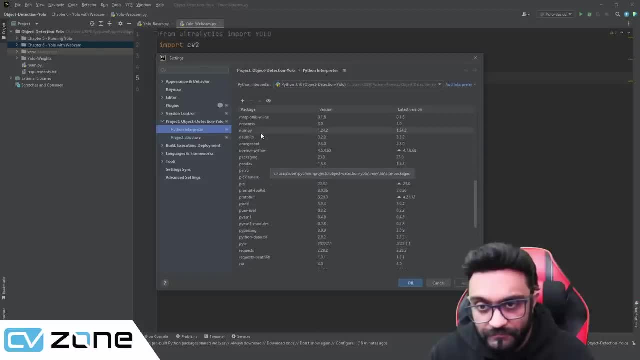 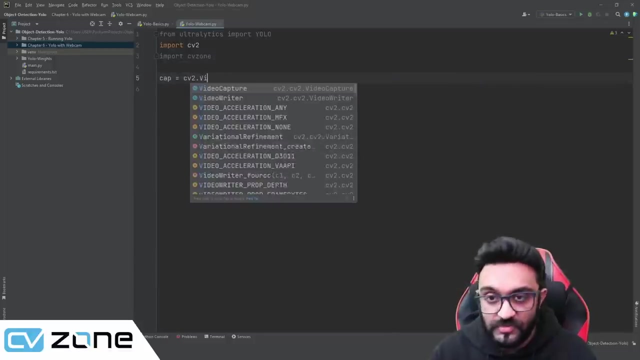 there you go. so opencv. as you can see, we are using version 4.60, whereas 6.8 is the latest version, but still 6.8 has this issue. that's why we are using 6.0. so we will write cv2 dot video. 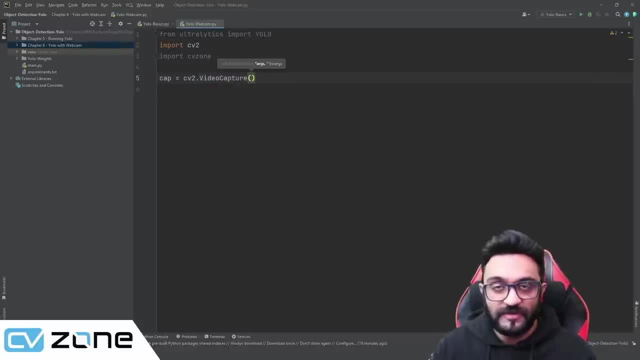 capture and the video capture is going to be the latest version of the new version, of the new version, with two hé entries and we will have two after ender and minutes based option. so this is where we'll have to make our cv2 Culture object under the front onions. we're going to make a new 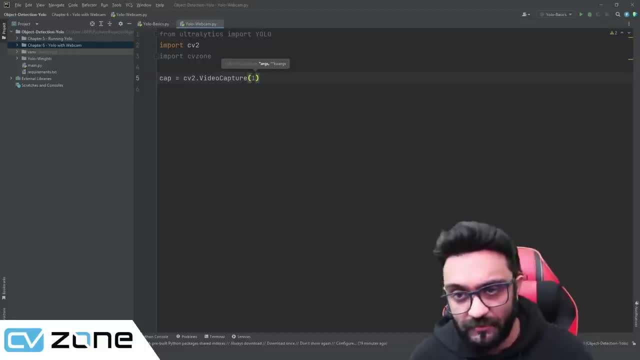 h었어, and it's really, really hard to get that step before we go to other projects, because we just want to keep the. we want to keep the image steady. so if you are looking to permission, support your windows, but if you want to capture your video camera, şek sujet çevurek. and that's what we have. and here is how to create your video capture object using the opencv object. so basically have the name of the video capture object on your video capture. i'm using multiple web cams, so i will give the id number one, because that is what i'm going to. 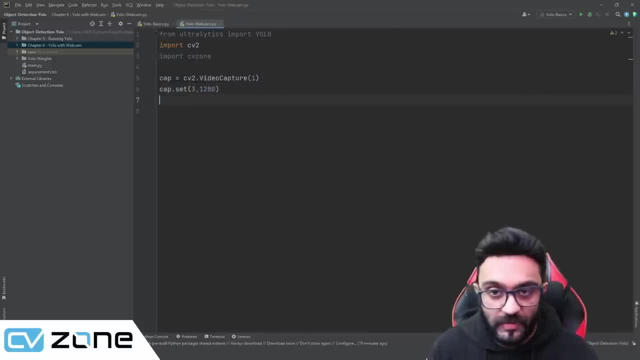 put it down here, because there are a lot of ways to fineala. that's why we would use that right now. but let's go to contact是什麼 function and we will use that one. So you can write 1280.. This is the width and cap dot set. That is the prop ID number four. That is. 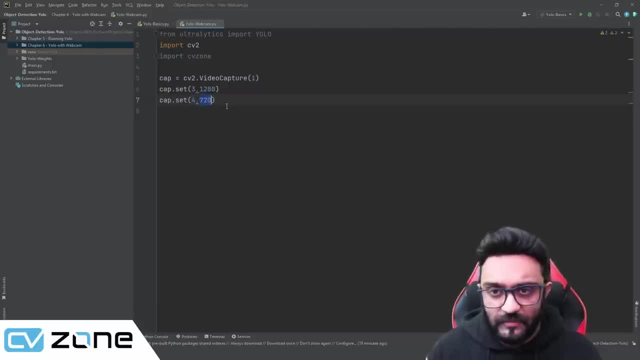 720.. So this is the height and we're going to set it at 720.. So this is the basic idea. And again, if you wanted to, there's another one which is mostly used in webcam: 640 by 480.. These dimensions: 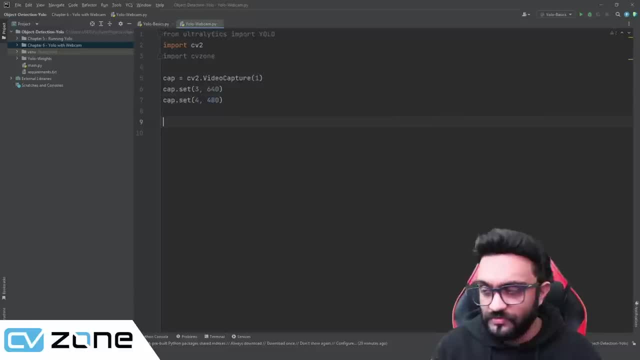 are commonly used, So it's up to you which one you want to use. Then we are going to write while true And we are going to write success and the image equals cap dot read. And then we are going to write cv2 dot. im show. We want to show the image, So we will write image and img That. 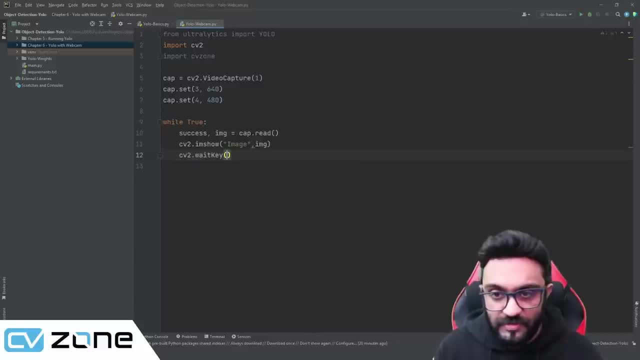 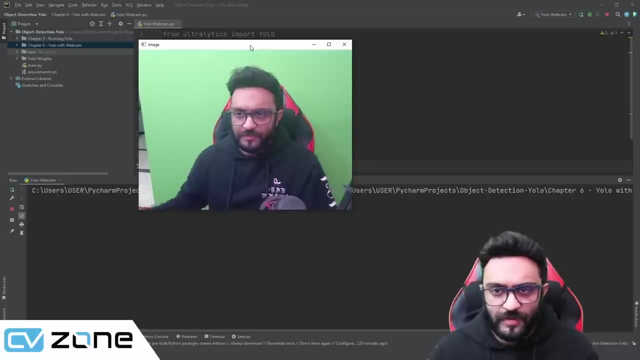 is the image we want to show And cv2 dot wait key, because we want to give it one millisecond delay. So this should run our webcam by default. So if we right click and run, we should have our webcam running. There you go. So this is the webcam, As you can see me. 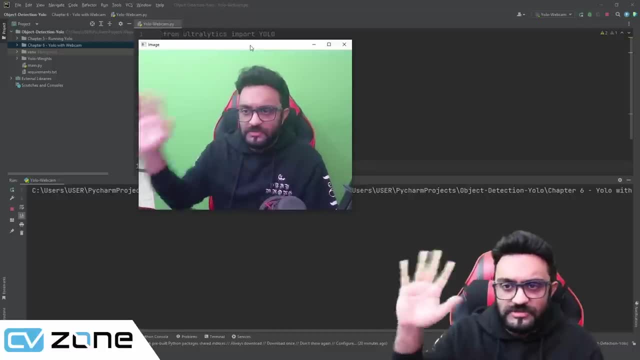 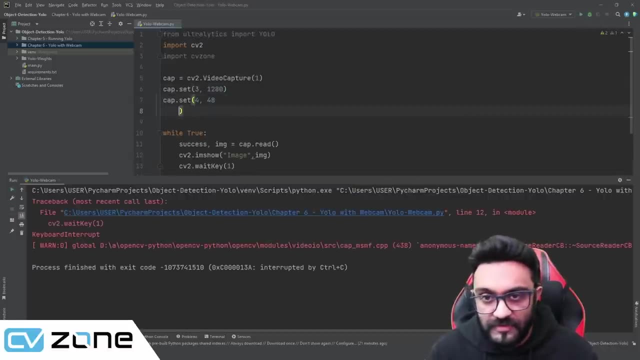 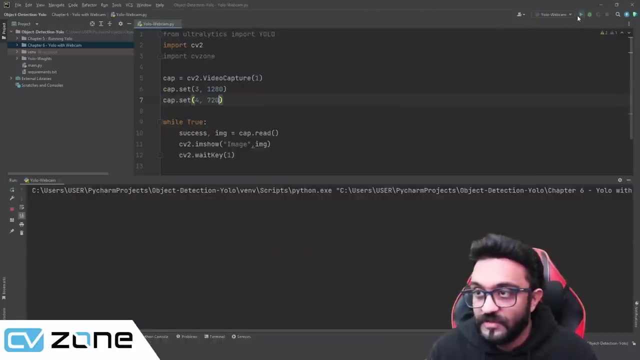 running. there you go. so this is the webcam, as you can see me. it's running live, so we can close this and, if you wanted to, you can write 1280 by 640 and oh, not 640, 720, my bad, 1280 by 720, and that should. 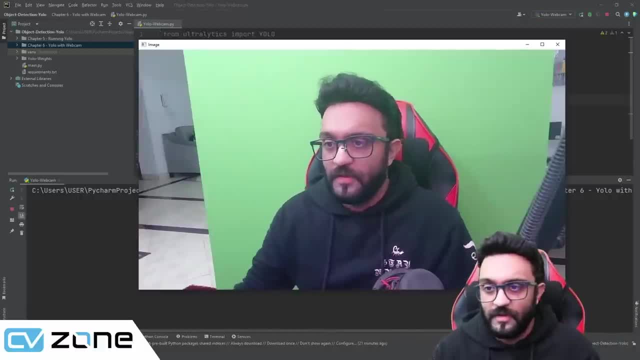 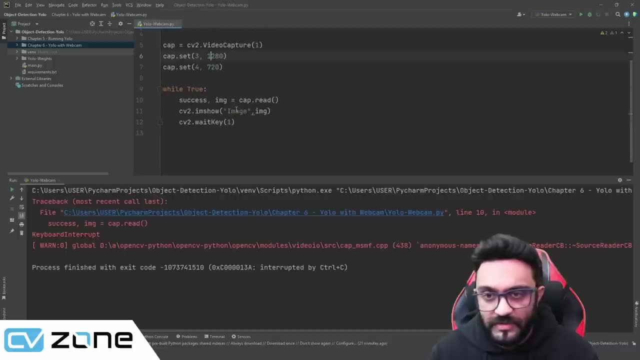 work as well. there you go. so now you have a bit more area to work with. so again, it's up to you which one you want to use. so we'll keep it on this and let's go ahead and create our model. so the model as we. 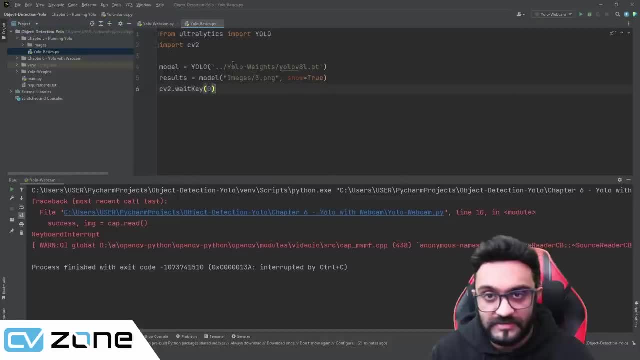 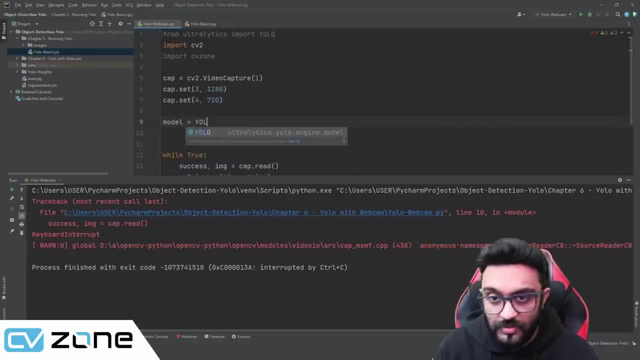 have seen earlier. if you go to Yolo basics here you can see this is how you can create your Yolo model and then you can find the results like this: so here we are going to write model equals, we are going to write Yolo and then we have to give in the weights. so the weights we are going. 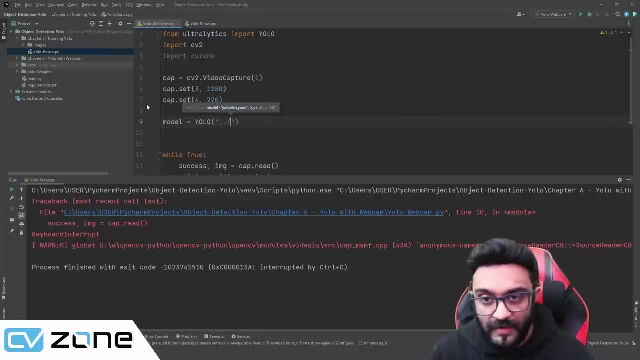 to use Nano for this purpose. so we will go back, we will write Yolo, Yolo, dash weights and then we will write the version. so this is Yolo, version 8 and Nano. so Yolo, version 8 and Nano. so I wrote the one by extra. so version 8 and Nano dot PT. so here we will go down and we will write: 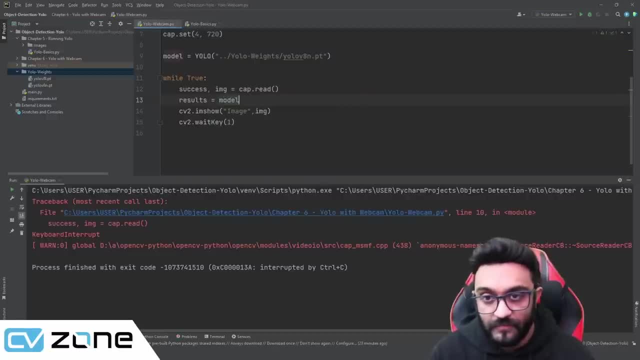 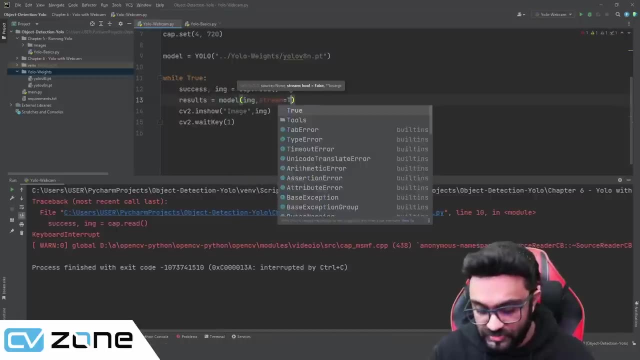 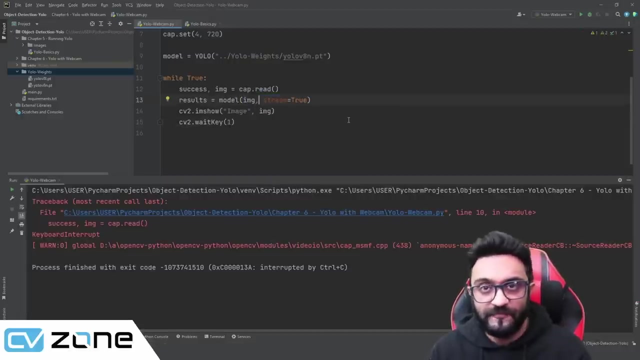 the results equals model and we are going to give in our image and we are going to write stream equals true. now, if you write stream equals two, it will use generators and that will be a bit more efficient than without it. so it is recommended to use stream equals true. so if we run this now, 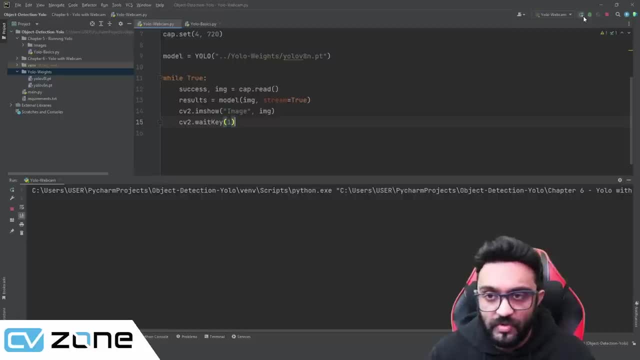 let's see what happens, so we should not get any errors. that's what we are trying to check. if we are getting any errors, it means we are heading in the wrong direction. there you go. we are not getting any error, so that is good. so now, once we have the 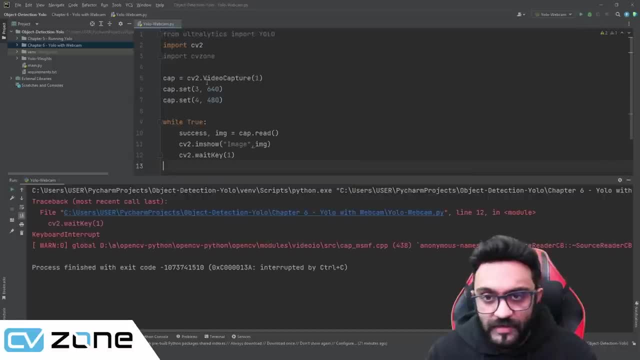 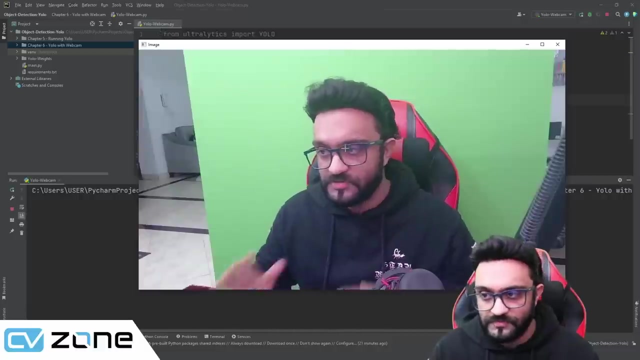 it's running live, So we can close this And, if you wanted to, you can write 1280 by 640. And not 640- 720.. My bad, 1280 by 720.. And that should work as well. There you go, So now you. 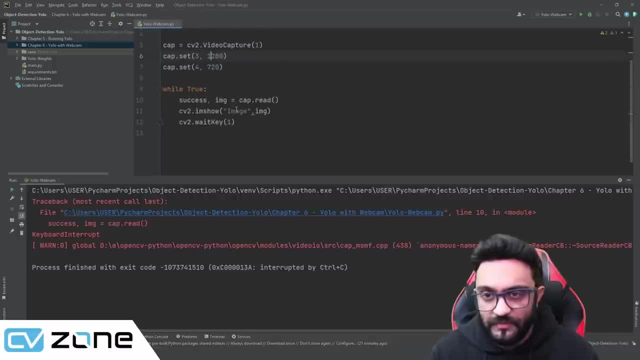 can see the image is running. So, again, it's up to you which one you want to use. So we'll keep it on this And let's go ahead and create our model. So the model as we have seen earlier, if you go to, 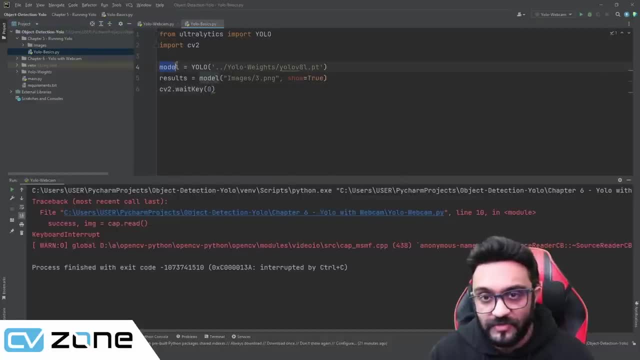 Yolo basics. here you can see. this is how you can create your Yolo model, And then you can find the results like this: So here we are going to write model equals, we are going to write Yolo, And then we have to give in. 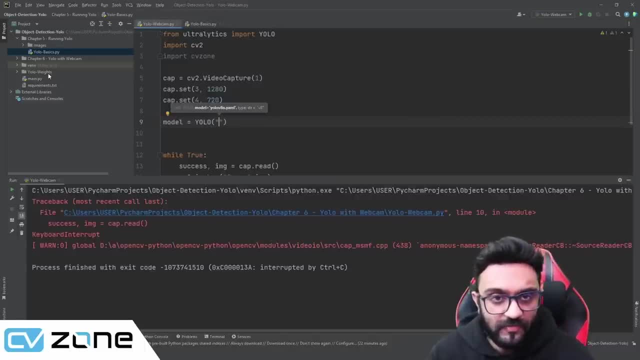 The weights. So the weights, we are going to use nano for this purpose, So we will go back, we will write Yolo, Yolo, dash weights And then we will write the version. So this is Yolo version eight and nano, So Yolo version eight and nano. So I wrote one by extra. 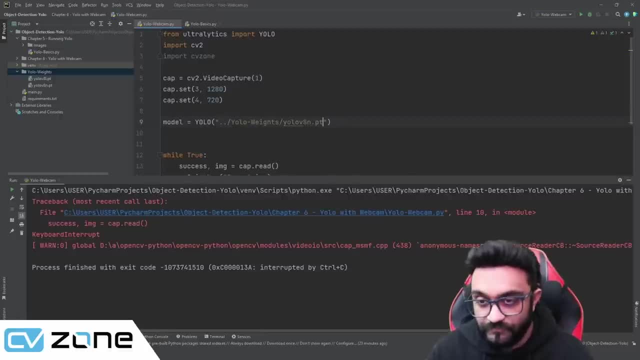 So version eight and nanopt. So here we will go down and we will write the results: equals model And we are going to give in our image And we are going to write: stream equals true. Now, if you write stream equals two, it will use generators and that will be a bit more efficient than without it. So it is. 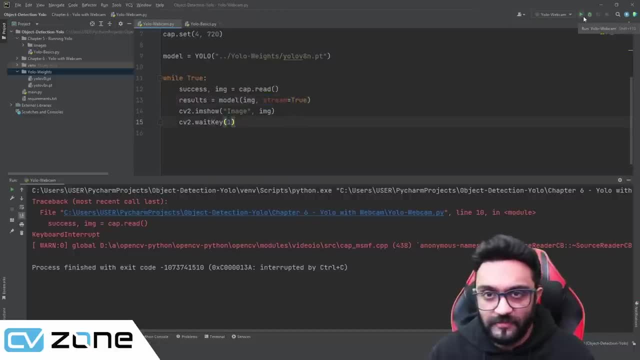 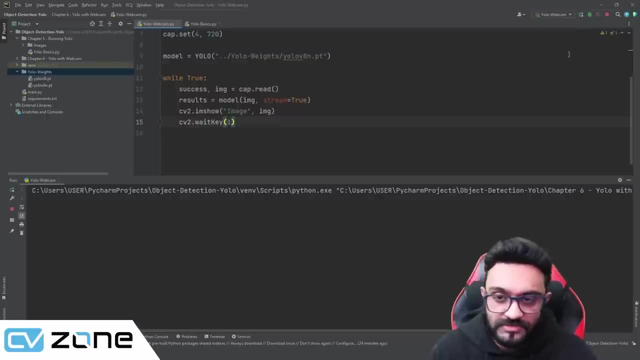 recommended to use stream equals true. So if we run this now, let's see what happens. So we should not get any errors. That's what we are trying to check. If you're getting any errors, it means we are heading in the wrong direction. 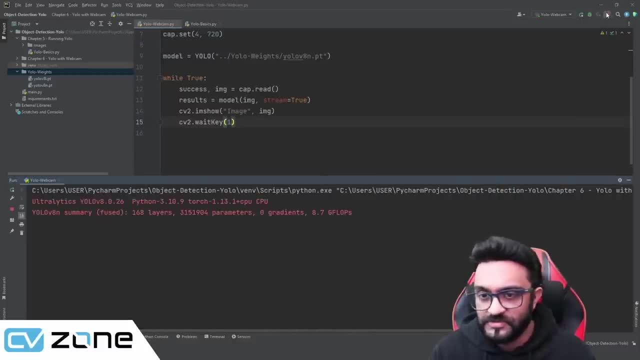 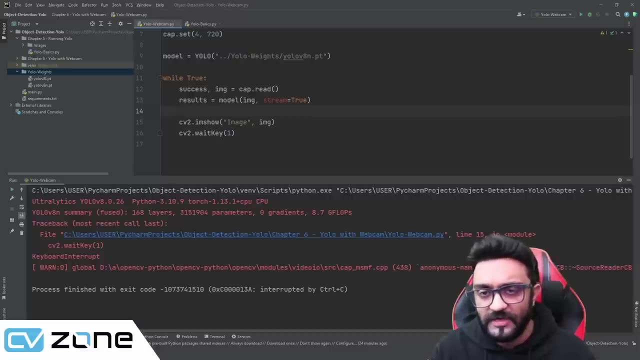 There you go. we are not getting any error, So that is good. So now, once we have the result, what we can do is we can check for individual bounding boxes and see how well it performs. So here, once we get the results, we are going to loop through. 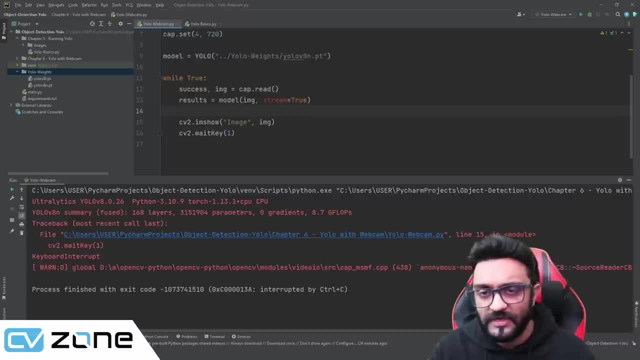 result. what we can do is we can check for individual bounding boxes and see how well it performs. so here, once we get the results, we are going to loop through them. so we are going to write for R in results. uh, we are going to get the bounding box of each. there's each of the results, so we will write here. 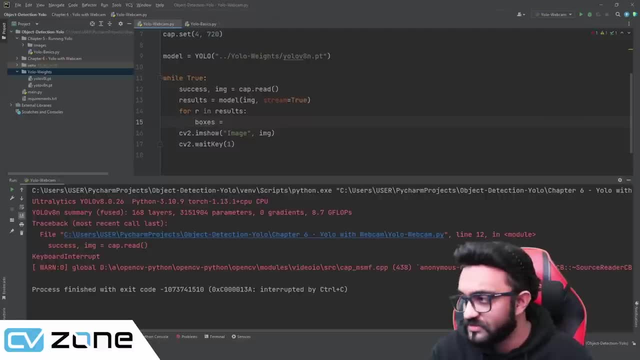 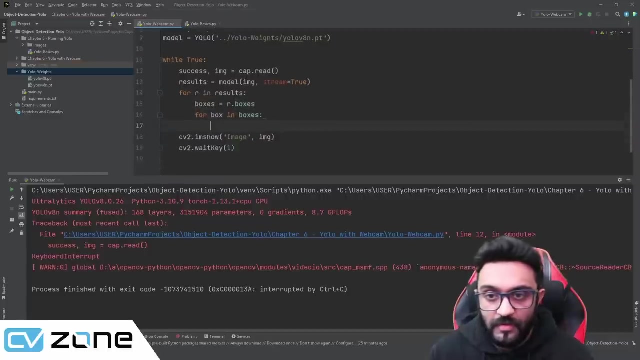 box is equals R dot box, and now we have to loop through the boxes, so we will write for box in boxes. we are going to find the X? Y of each of the bounding boxes. so there are two methods. uh, you can use X Y, X Y, which means X 1 Y 1, X 2 Y 2, or X 1 Y 1 and width and height. so which format? 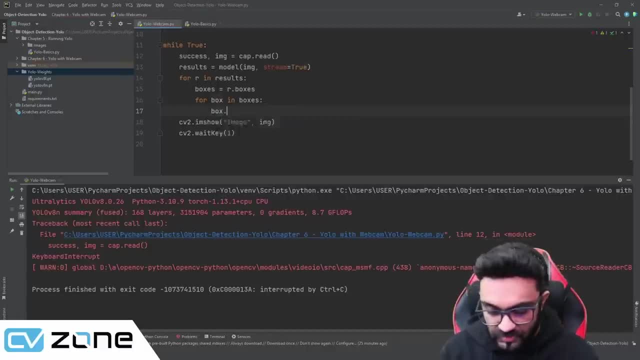 do you need? it depends on you. so here you can write dot X Y, X Y, or you can write box dot X, Y with height. so which one do you want? so I would recommend X Y, X Y, because it will be easier to input directly. to open. 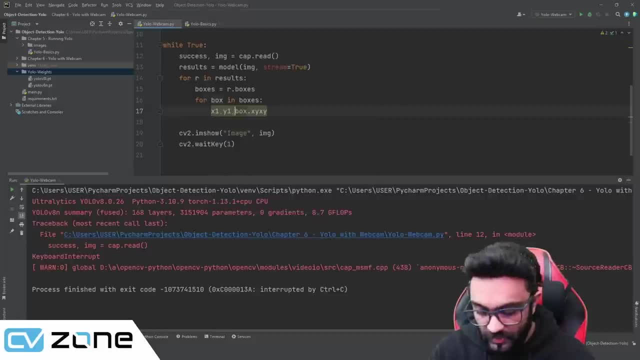 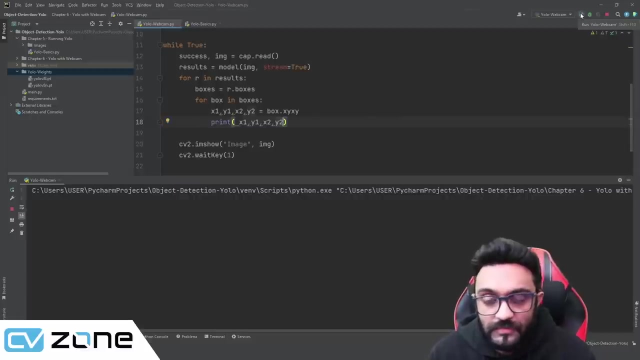 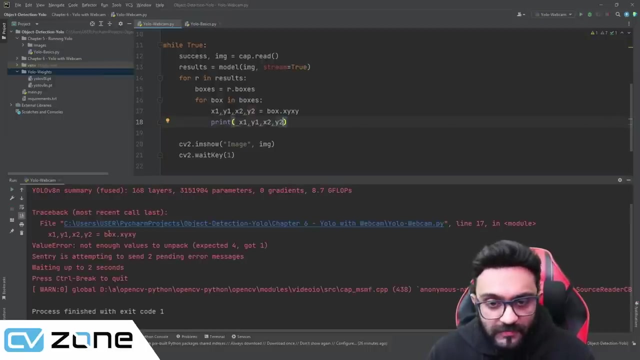 CV. so we will write here: X 1, Y 1, then X 2 and Y 2 equals this, and what we can do is we can print these values. so we will copy these and we are going to simply print them. so let's see what do we get? so we are getting an error, not enough. 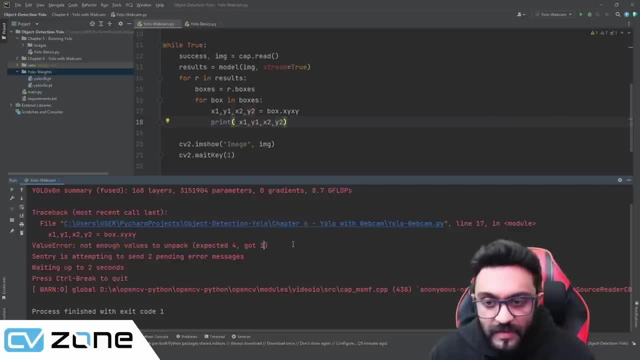 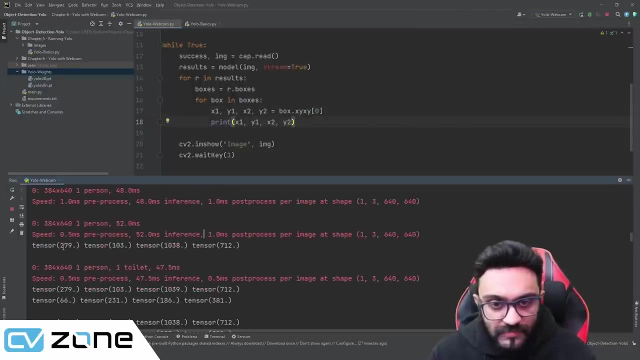 values to unpack. expected for got one. so it means they are just packed in sides. so what we need to do is we just need to get the first element of it, so hopefully that will work out. there you go. so this is what we are getting. so we are getting. 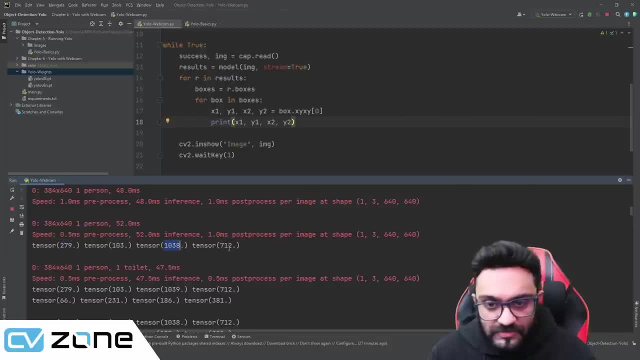 the value of 279: 1, 0, 3, 1 0, 3, 8 and 7, 1, 12. so again, then we have multiple detections, then we are getting two values. so here we are getting X 1, Y 1, X 1, X 2 and Y 2, so these: 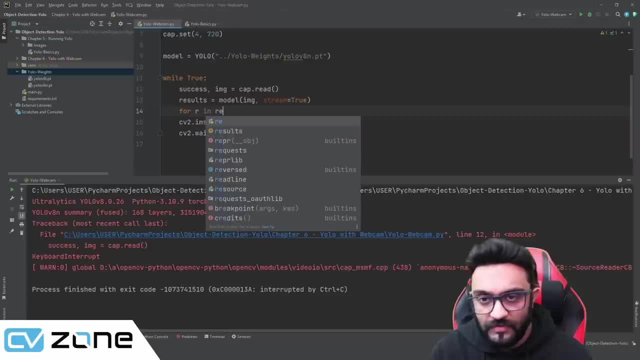 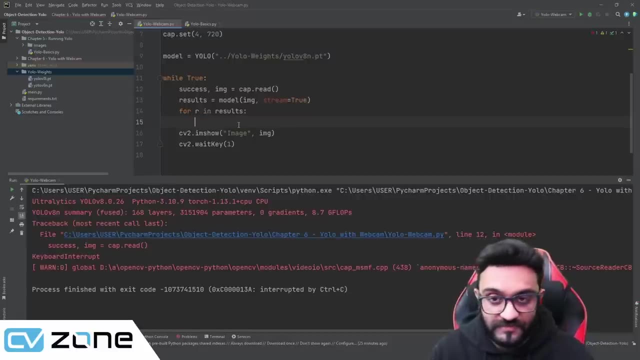 them. So we are going to write for R in results. We are going to get the bounding box of each of the results, So we will write here: box is equals R dot boxes. And now we have to loop through the different bounding boxes, So we will write for box in boxes. We are going to find the X, Y of each of. 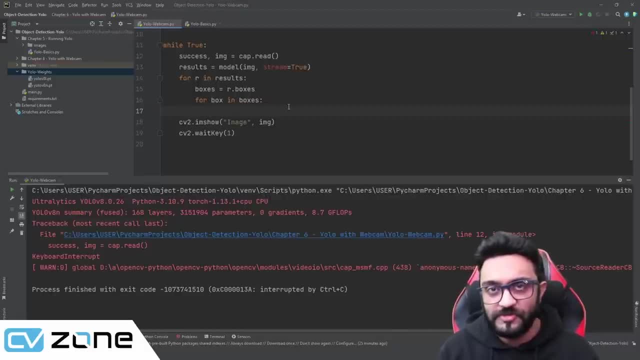 the bounding boxes. So there are two methods. You can use XP, X- Y, which means x one, y one, x two, y two, or x one y one, and width and height. So which format do you need? it depends on you. So here you. 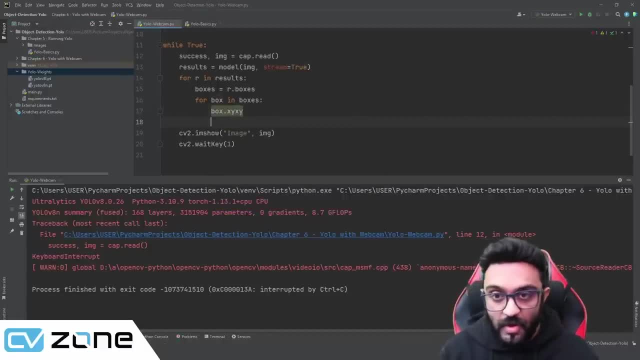 can write box dot x, y, x y, or you can write box dot x, one y, one x y, width height. so which one do you want? so i would recommend x y, x y, because it will be easier to input directly to opencv. so we will write here: x 1, y 1, then x 2 and y 2 equals this and what we. 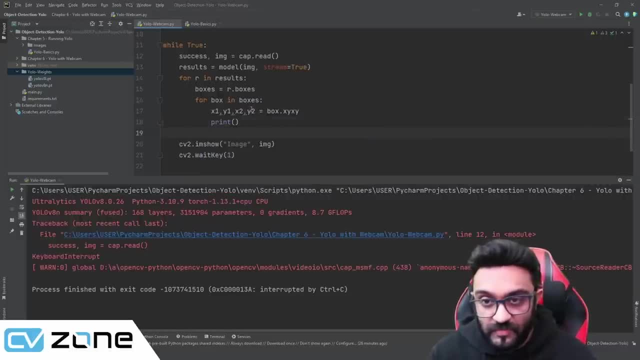 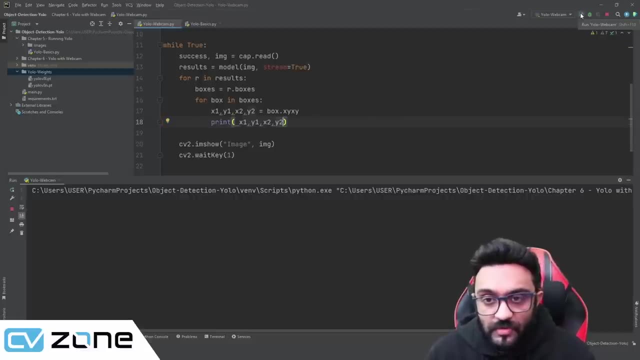 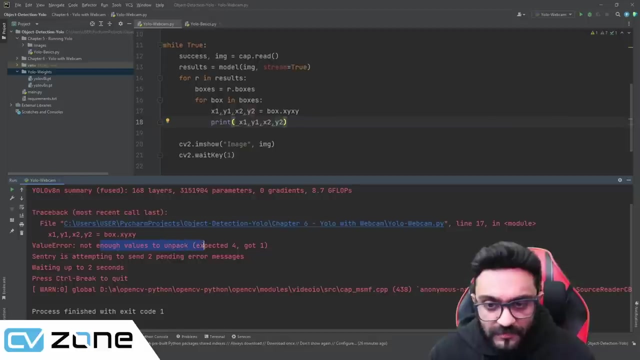 can do is we can print these values, so we will copy these and we are going to simply print them. so let's see what do we get. so we are getting an error: not enough values to unpack, expected for got one, so it means they are just packed in sides. so what we need to do is we just need to get the first element of it. 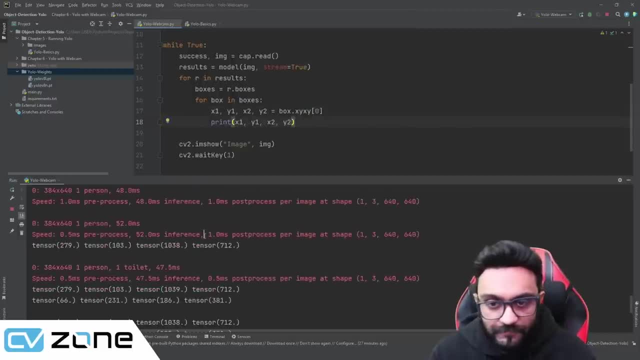 so hopefully that will work out. there you go. so this is what we are getting. so we are getting the value of 279. so we are getting the value of 279. so we are getting the value of 279. one zero three, one zero three, eight and seven, one twelve. so again, then we have multiple detections. 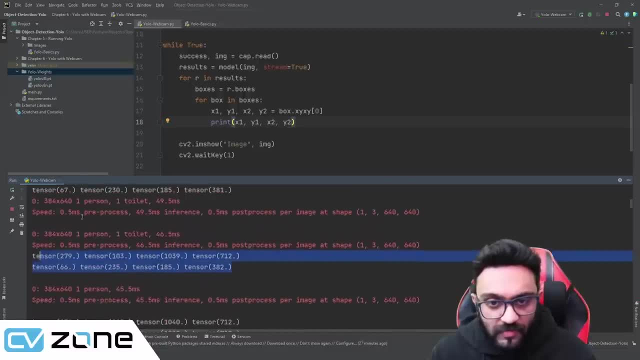 then we are getting two values. so here we are getting x 1, y 1, x 1, x 2 and y 2. so these are the values that we are getting. so what we need to do is we need to convert them into integers so that we 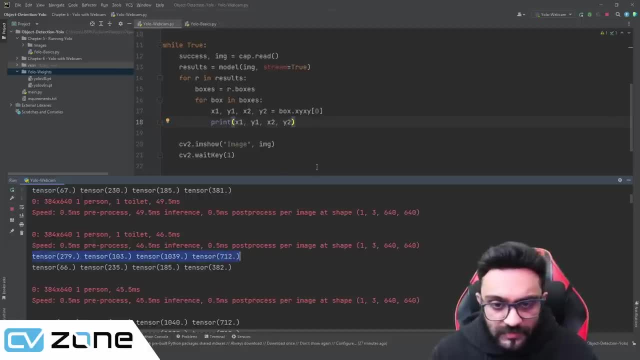 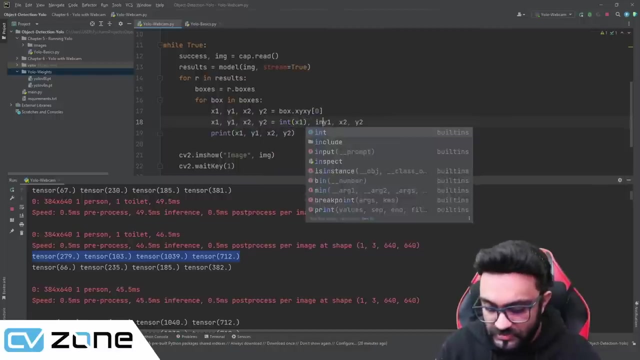 are the values that we are getting. so what we need to do is we need to convert them into integers so that we can actually use them. so we can copy this part and we can paste it, and then we can put it into integer, convert it into integer, and integer and integer. there you go. so let's run it and 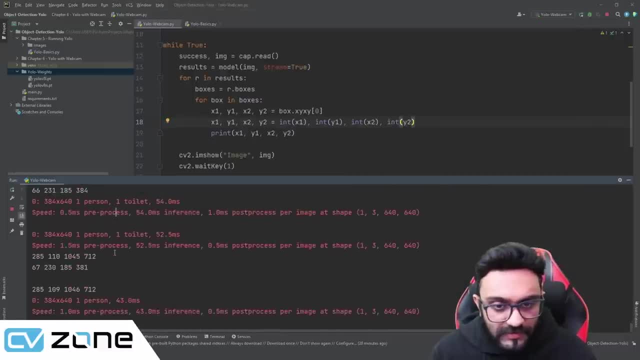 see if it works. so there you go. now we are getting the values you can see here we are getting the actual values that we can use with open CV. so let's go ahead and create a rectangle to actually find out if we are getting the correct bounding box. 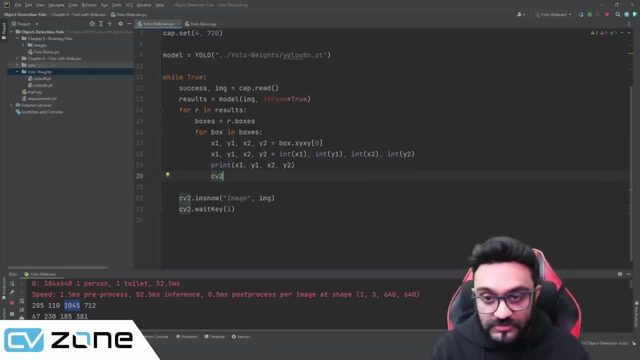 or not. so here we will write CV 2 dot rectangle, rectangle and we will give in our image. and then we have the points, so X 1 and Y 1, then we have the X 2 and X 2 and the Y 2. so these are the points that we will give in and then we have the 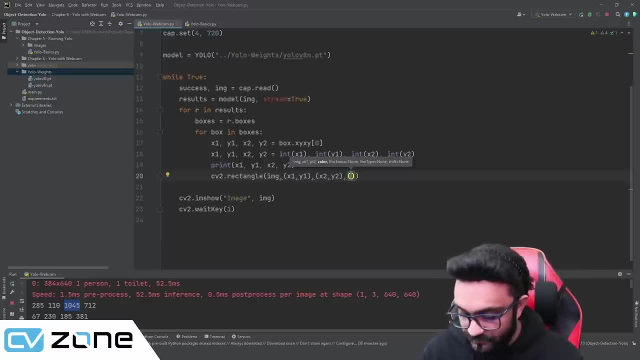 color, so color, let's put it. it's B, so let's put it at 0. green is let's 200 and 0, or let's make it purple. so 2, 5, 5, 0, 2, 5, 5, that will make it purple. okay, then we have the. 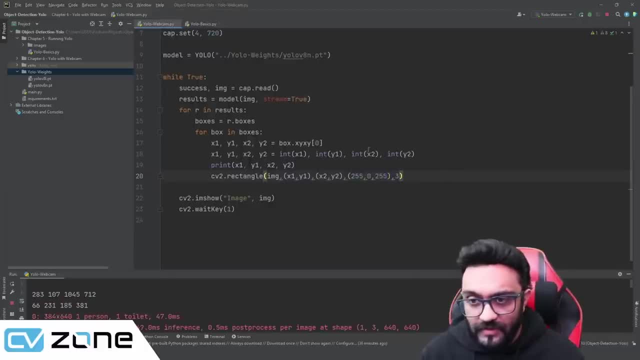 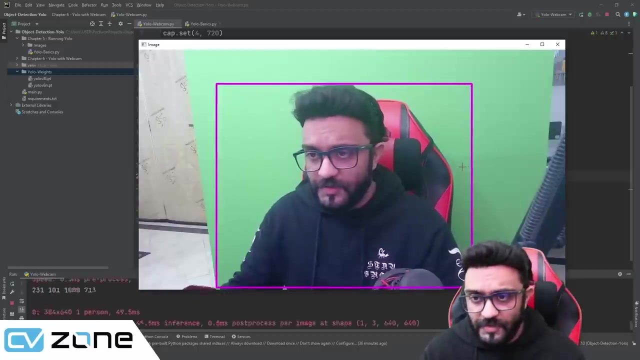 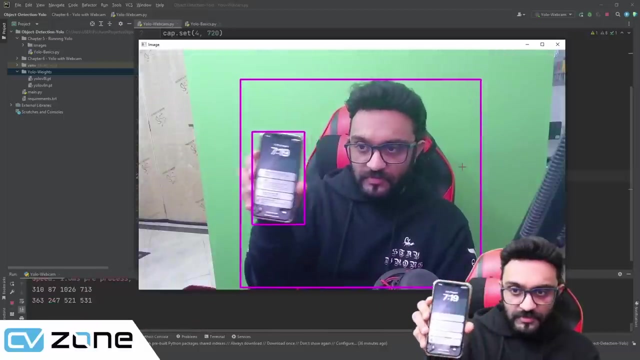 thickness, let's put it at 3. and yeah, that's pretty much it. so let's run it and see if it works. and there you go. so we are detecting. so if I bring in my phone, you will see there's a bounding box around it and it shows that it is working fine. so let's. 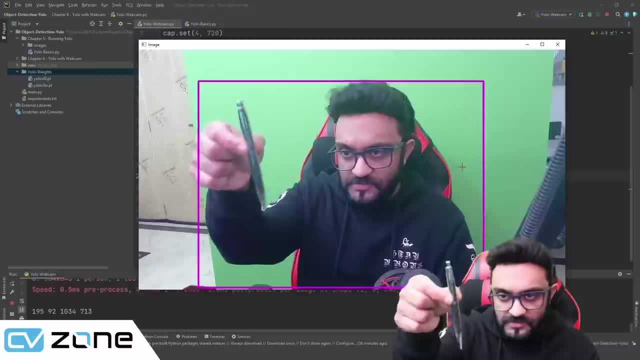 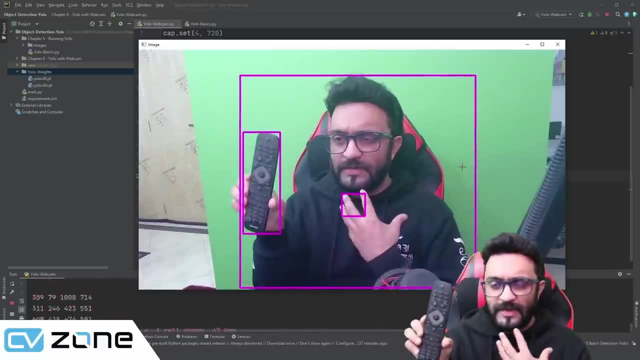 try a pen. can I detect a pen? yeah, to text a pen as well. it detects the phone. and let's try the remotes defects that we mode as well. but again, we are not actually going to do so long until the remote is active, so it's not going to be. 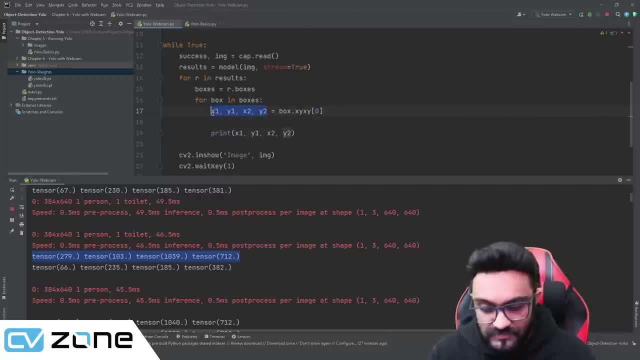 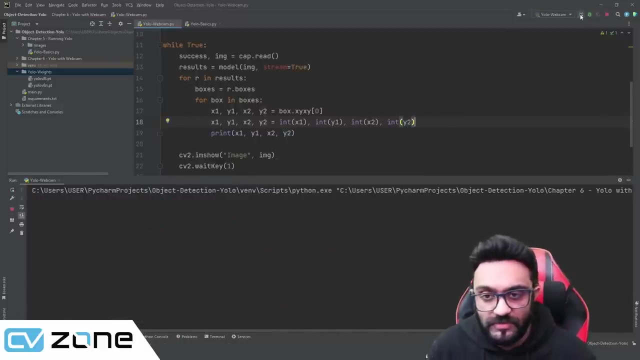 can actually use them. so we can copy this part and we can paste it, and then we can put it into integer, convert it into integer, and integer and integer. there you go. so let's run it and see if it works. so there you go. now we are getting the values you can see. here we are getting the actual values that 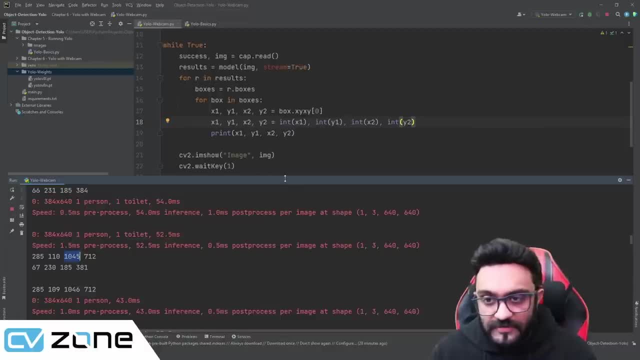 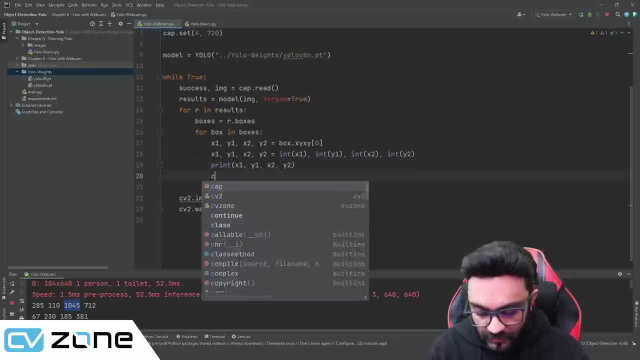 we can use with opencv. so let's go ahead and create a rectangle to actually find out if we are getting the correct bounding value. so let's go ahead and create a rectangle to actually find out boxes or not. so here we will write cv2 dot rectangle, rectangle and we will give in our 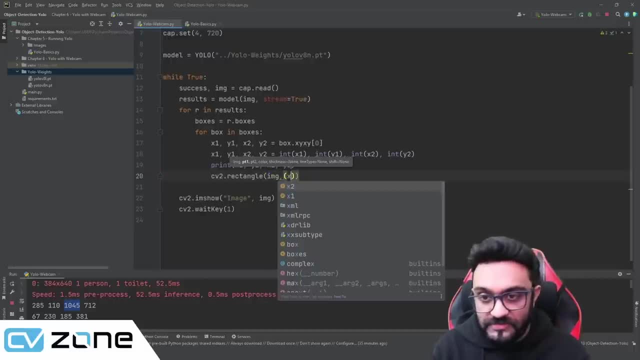 image. and then we have the points, so x1 and y1, then we have the x2 and x2 and the y2, so these are the points that we'll give in. and then we have the color. so color, let's put it: um, it's b, so let's put it at zero. green is let's 200 and zero, or let's make it. 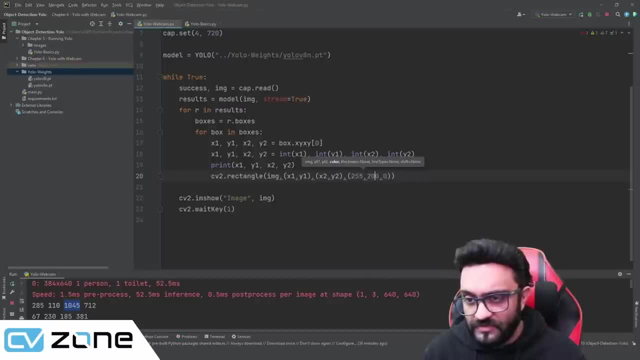 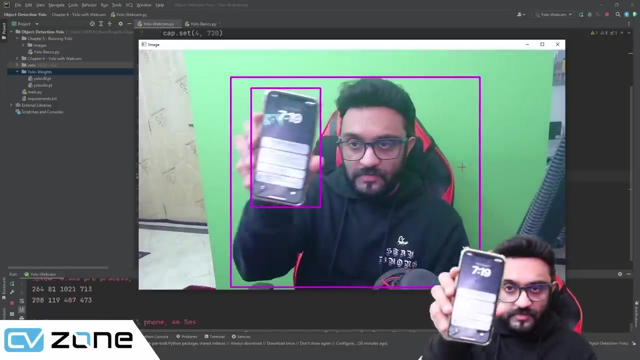 purple. so two five five, zero, two five five, that will make it purple. okay, then we have the thickness, let's put it at three and yeah, that's pretty much it. so let's run it and see if it works. and there you go. so we are detecting. so if i bring in my phone, you will see there's a bounding box. 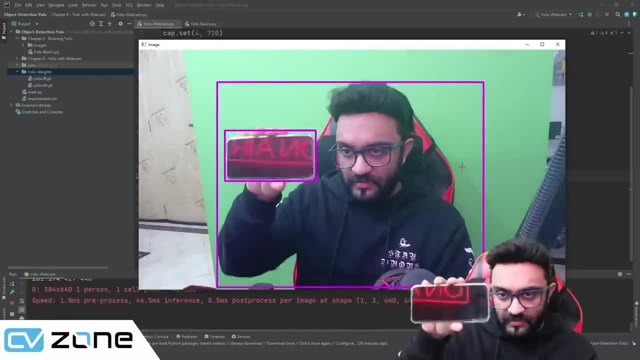 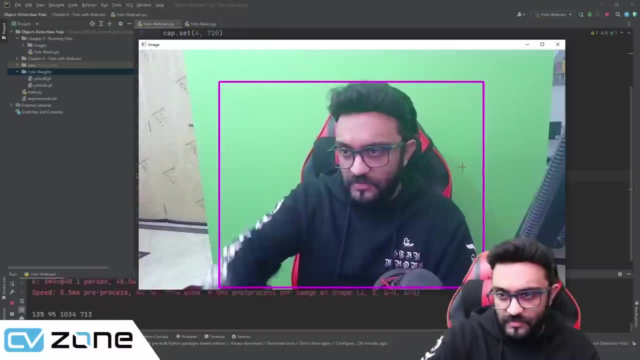 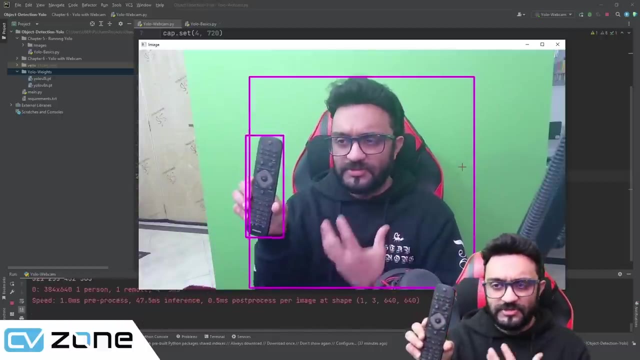 around it and it shows that it is working fine. so, um, let's, let's try a pen. can it detect a pen? yeah, it detects a pen as well. it detects the phone. and let's try the remote. it detects the remote as well, but again, we are not actually using the remote. so let's try the remote and 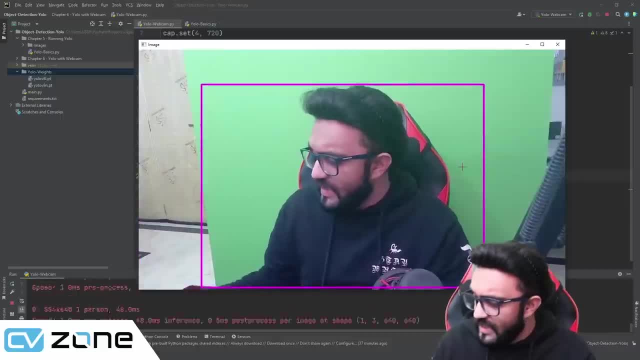 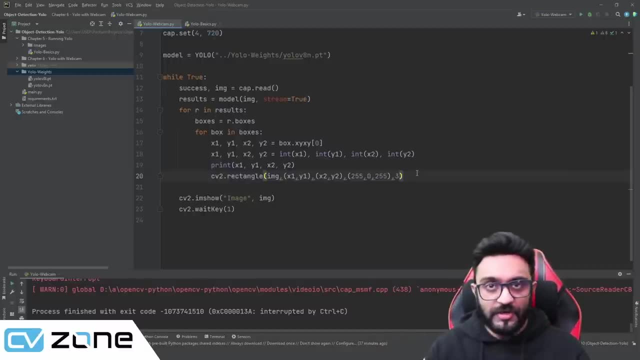 actually getting, uh, the feedback of what exactly the class is and, uh, how confident it is. so we are going to detect those as well. now, uh, as i mentioned earlier, you can use a fancy rectangle as well, which we provide in cv zone package. so in order to do that, you can simply write cv zone dot. 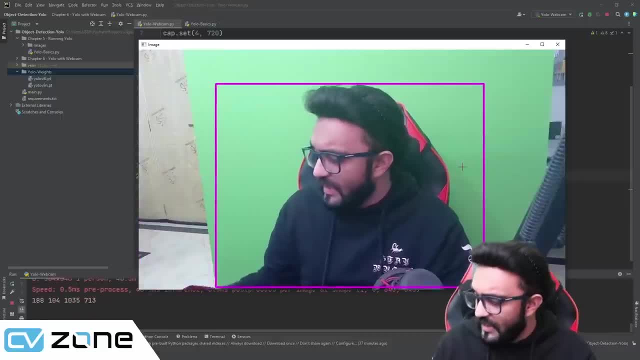 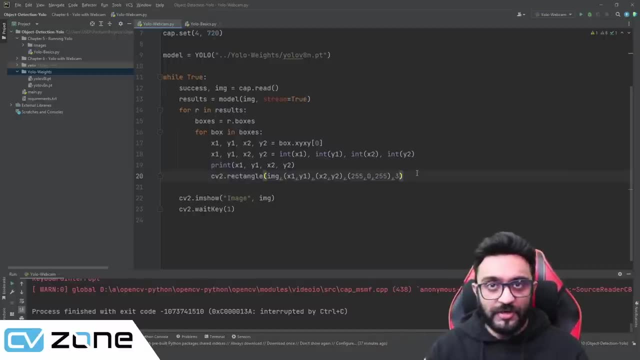 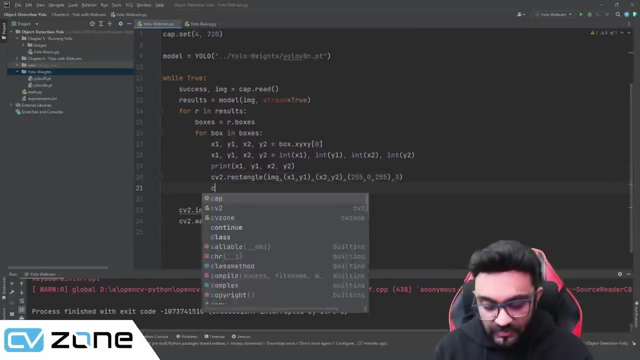 getting the feedback of what exactly the class is and how confident it is, so we are going to detect those as well. now, as i mentioned earlier, you can use a fancy rectangle as well, which we provide in cv zone package. so in order to do that, you can simply write cv zone dot. corner rectangle. 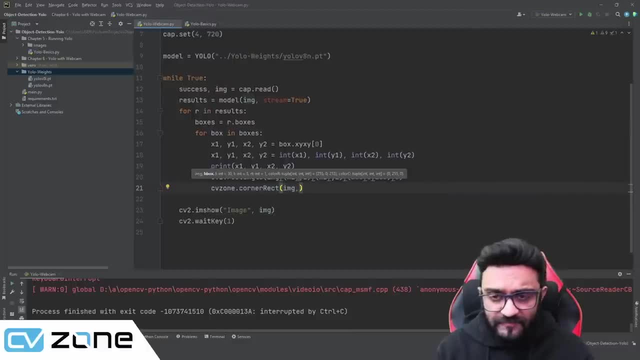 and you will give in the image and all you have to do is give in the bounding box so you can write here: bounding box, bb box. so where is this bounding box coming from? this is actually x, y, width and height, so we can get that too. so we can write here: bounding box, x, y, width, height, and this will give. 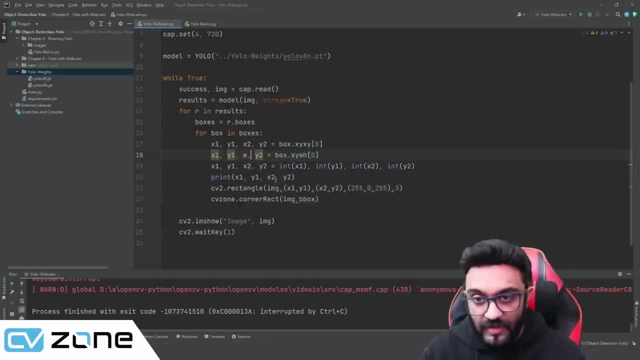 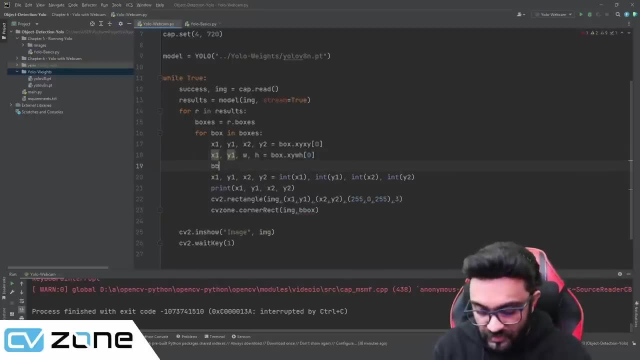 us, the x1, y1 will be the same and then we will have the width and the height, and then what we can do is we can put it in the bounding box and we can write here: bounding box x, y, width, height in bounding box. so bbox equals uh, this: 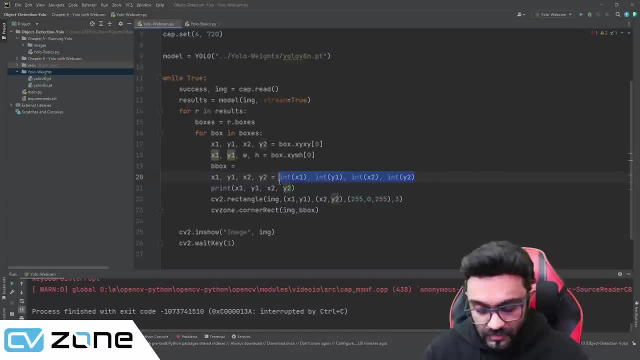 we'll convert it into integers, and there you go. so this will be width and this will be height. there you go. now. this is a repetition, so again, we can use one of them. we don't have to use both of them at the same time, so so, 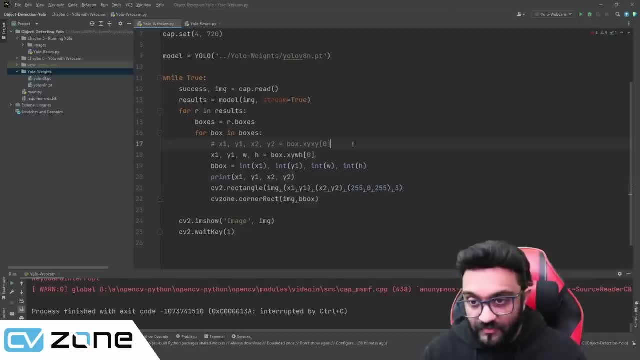 so let's put this one over here, so this one, and let's put this with it so you can use either one of them, so not both of them at the same time, because that would be weird. we can remove that. so this one is for open cv and this one is for cv zone. let's run that and see if it works. 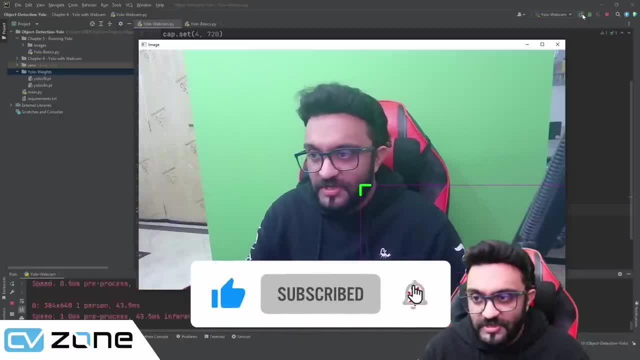 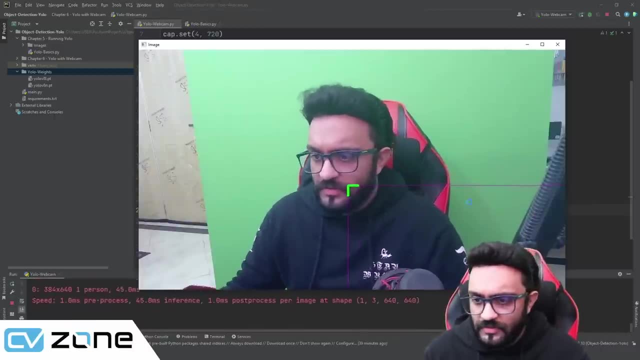 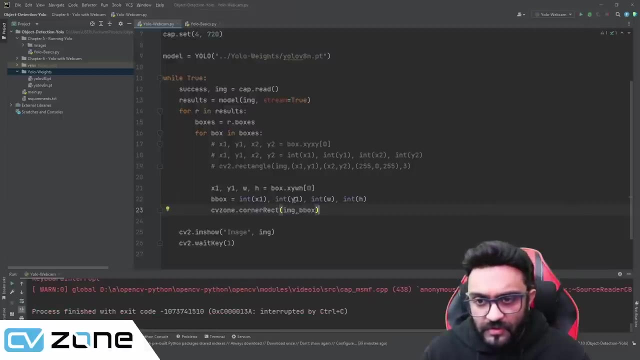 and there you go, we are getting something, but it is wrong. so why exactly is it wrong? so we are getting x1, um, what happened here? so x1, y1 and then w and h. so okay, something seems wrong. so let's try that. let's just get these values and we can subtract to get the width and height. 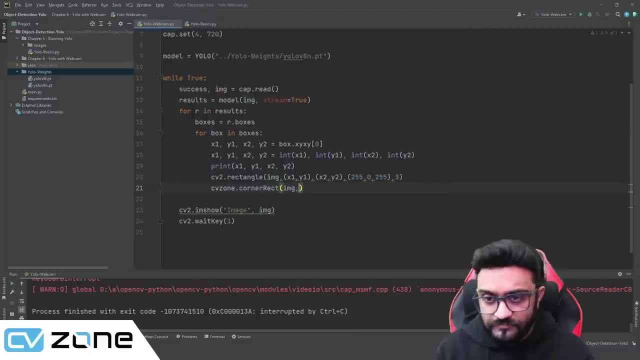 corner rectangle and you will give in the image and all you have to do is give in the bounding box so you can write here: uh, bounding box b, b, b o, x. so where is this bounding box coming from? uh, this is actually x, y, width and height. 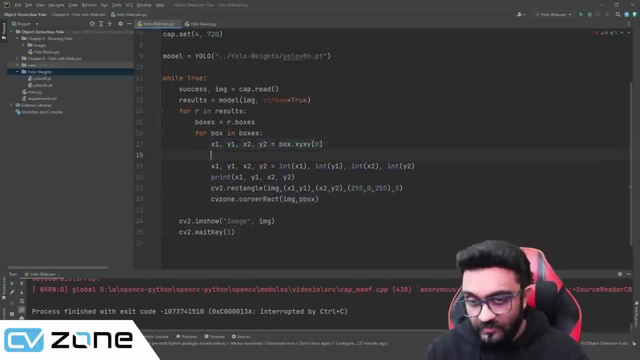 so we can get that too. so we can write here a bounding box x, y worth height, and this will give us the x, 1, y, 1 will be the same, and then we will have the width and the height, and then what we can do is we can put it in bounding box. so b, b o x. 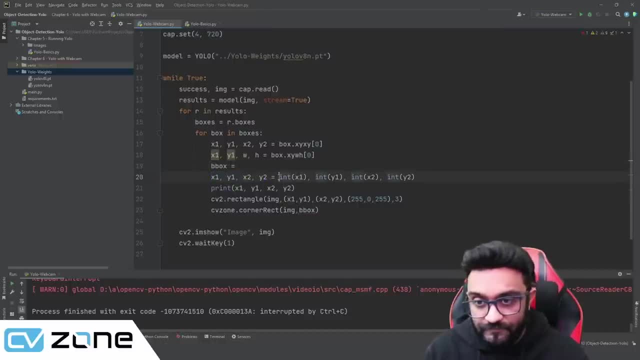 equals uh, this, we'll convert it into integers, um, and there you go. so this will be width and this will be height. there you go now. this is a repetition, so again, we can use one of them. we don't have to use both of them at the same time. so let's put this one over here. 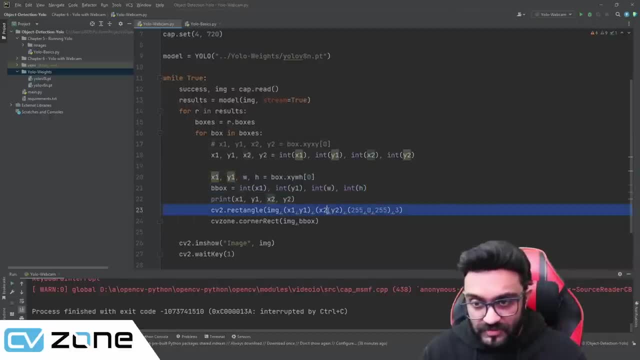 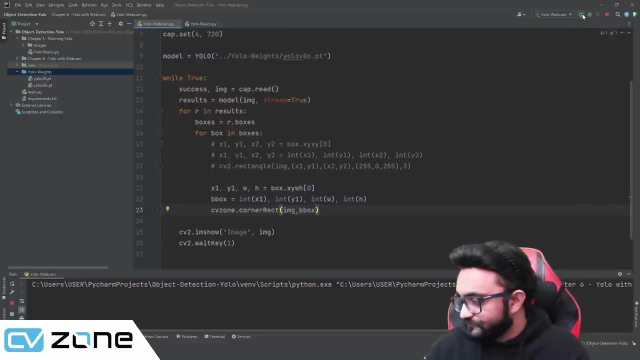 so this one- and let's put this with it, so you can use either one of them, so not both of them at the same time, because that would be weird. we can remove that. so this one is for open cv and this one is for cv zone. let's run that and see if it works, and there you go, we are getting something. 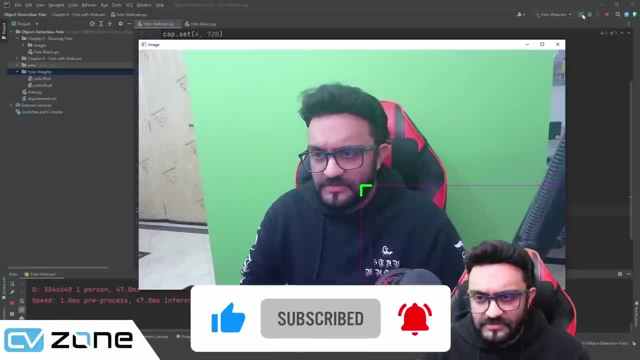 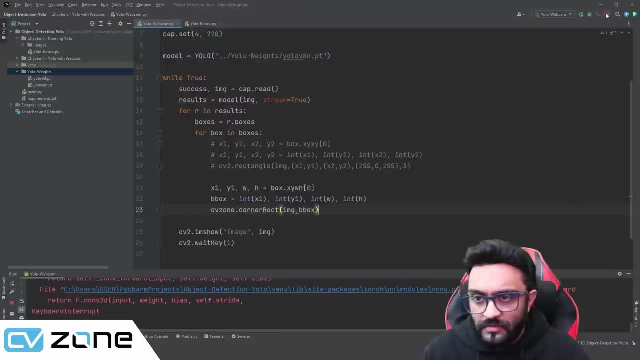 but it is wrong. so why exactly is it wrong? so we are getting x1, um, what happened here? so x1, y1 and then w and h. so, okay, something seems wrong. so let's try that, um, let's just get these values and we can subtract to get the width and height. 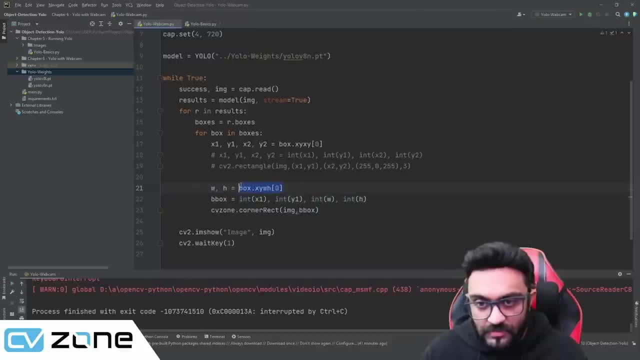 so the width and height equals x2 minus x1 and then y2 minus y1, and hopefully that will work out. so let's open this up and we can remove this, and here for the bounding box we can simply write x1, y1 and width and heights. let's try it this way. hopefully it will work. 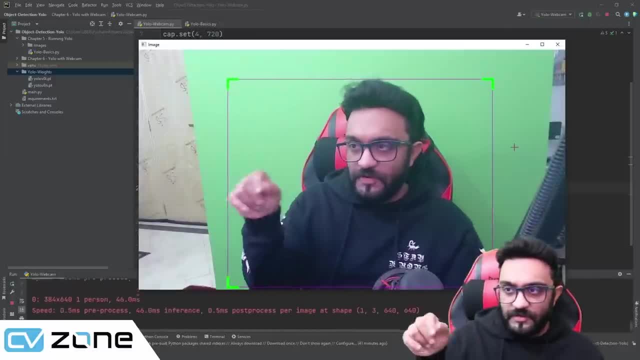 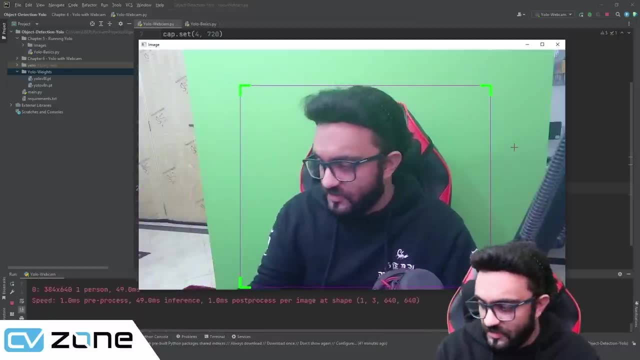 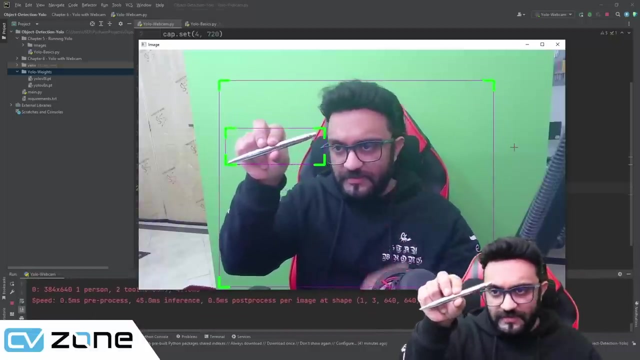 there you go, so it works now. so we have the green boxes, and then we can also have, for example, for the phone. you can see it's a little bit fancier again. you can change the colors, uh, the colors of these edges, you can change the color of the inner rectangle, and all of that. 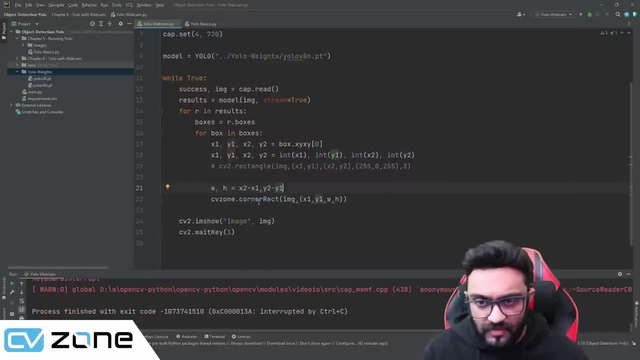 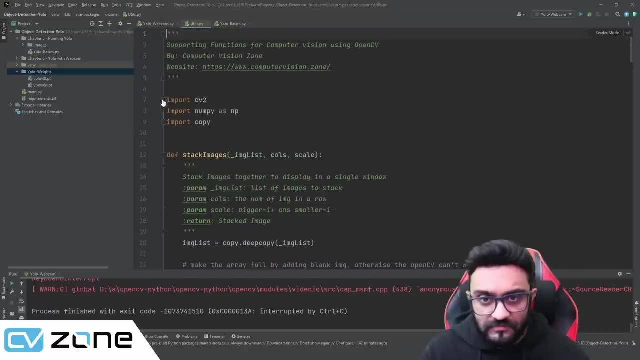 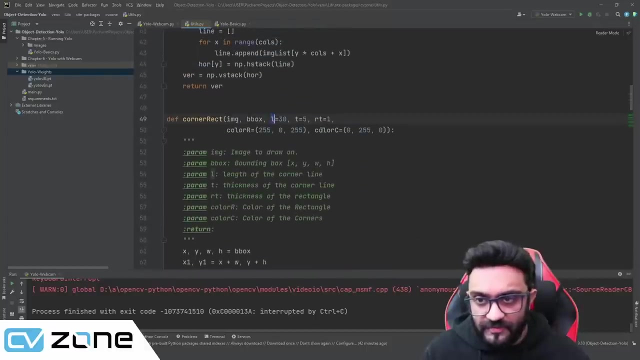 all of this information is given here. if you click on the control and click on corner rectangle here you will see: uh, where is it? is it's corner rectangle. there you go, so it will show you. this is the length and this is the color for the corner. 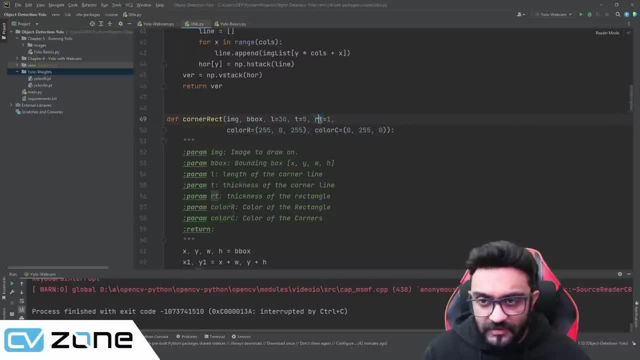 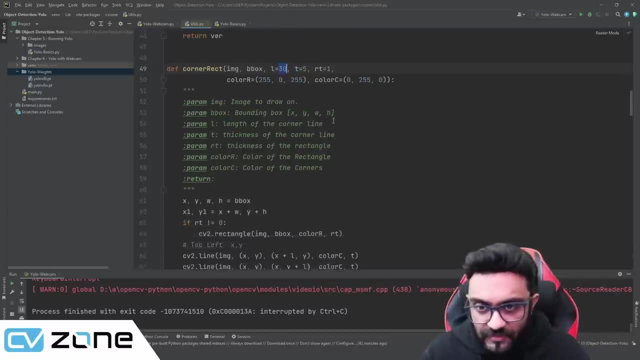 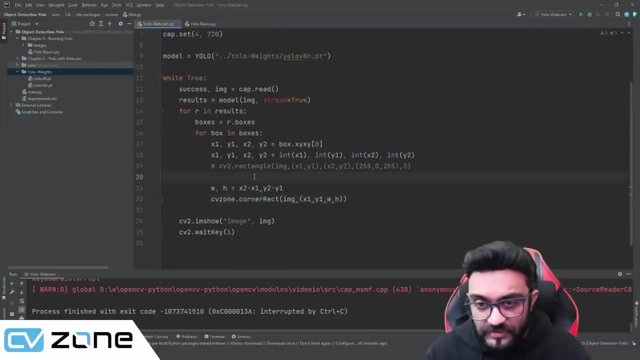 the color for the rectangle and the rectangle thickness and the thickness of the corner, and all of these details are given here so you can check here and, based on that, you can apply this. okay, so this is good. so the next step would be to actually get the confidence values and the class names, so we don't have the class names of 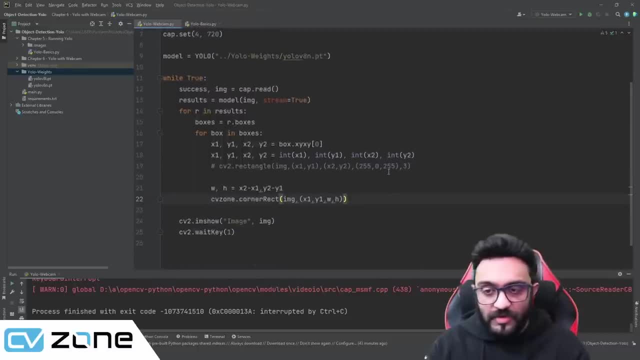 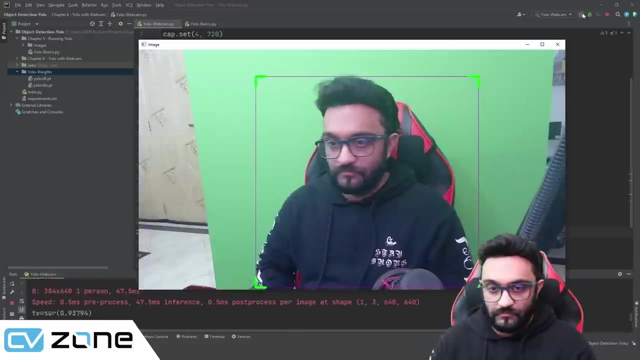 yet. so we only are showing the bounding box. so let's find out the confidence first. so the confidence is: conf equals bounding box, conf zero. so this is the confidence. so let's print that out and see if it works. so if we go down and there you go, you can see the confidence values. 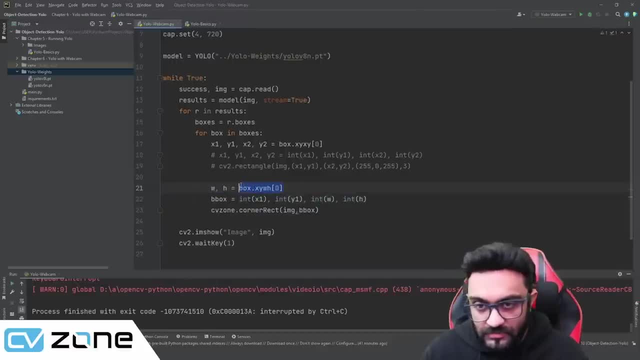 so the width and height equals x 2 minus x 1, and then y 2 minus y 1, and hopefully that will work out. so let's open this up and we can remove this, and here for the bounding box we can simply write x1, y1 and width and height. 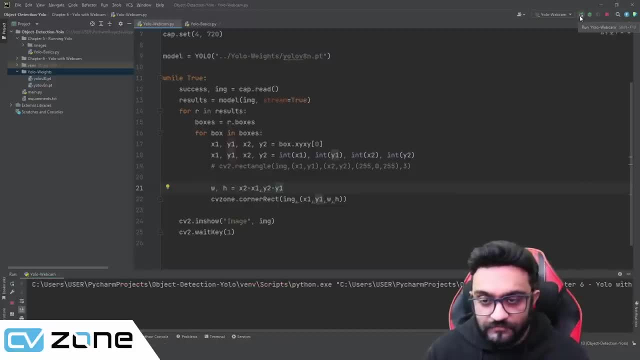 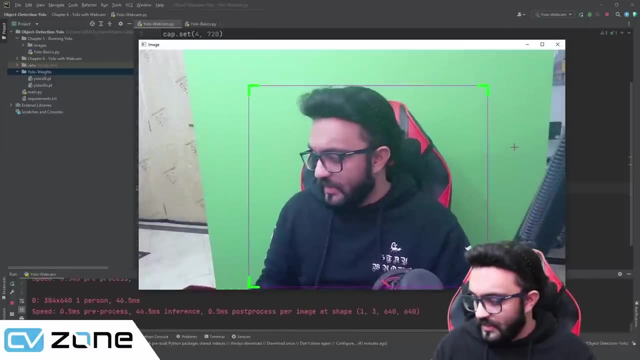 let's try this way. hopefully it will work. there you go. so it works now. so we have the green boxes and then we can also have so, for example, for the phone. you can see it's a little bit fancy little guys. so this is a little way like sciences that we would want to go into, and if you want to move into something, for example, using a phone, it looks like this: 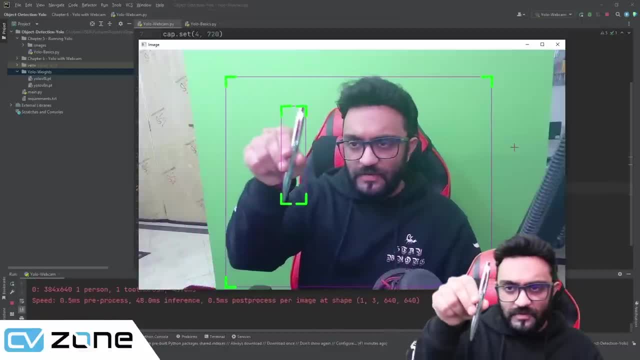 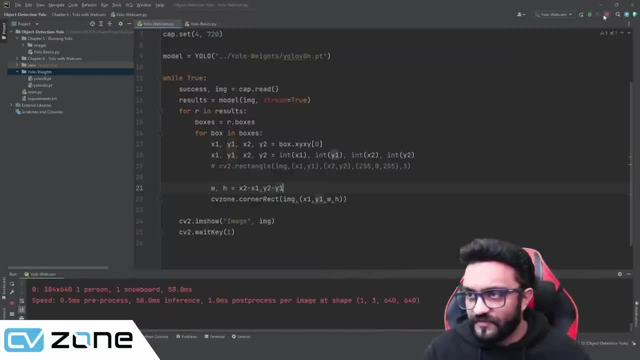 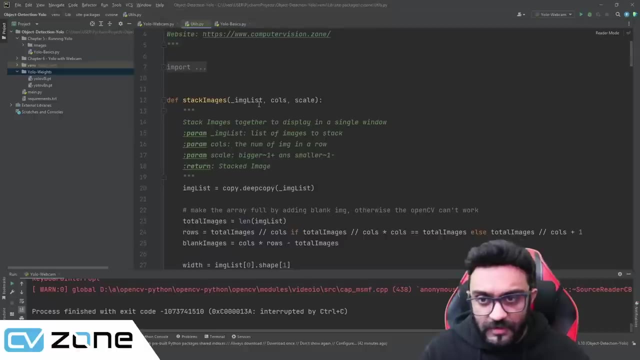 a little bit fancier again. you can change the colors, the colors of these edges, you can change the color of the inner rectangle and all of that. all of this information is given here. if you click on the control and click on corner rectangle here you will see: uh, where is it? is it's corner. 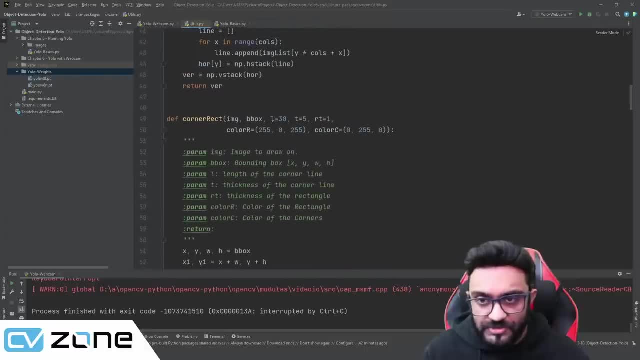 rectangle. there you go, so it will show you this is the length and this is the color for the corner, the color for the rectangle and the rectangle thickness and the thickness of the corner, and all of these details are given here so you can check here and, based on that, uh, you can apply. 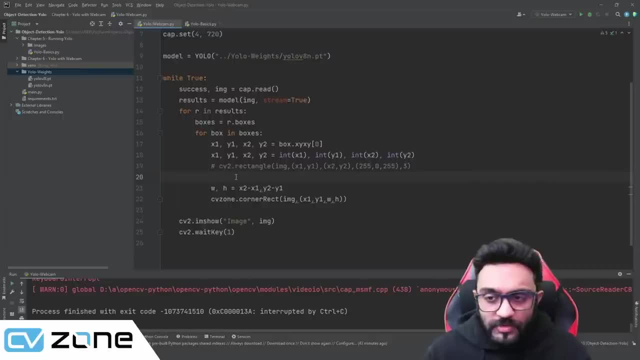 this okay, so this is good. so the next step would be to actually get the confidence values and the class names. so we don't have the class names of yet, so we only are showing the bounding box. so let's find out the confidence first. so the confidence is conf, equals bounding box- conf. 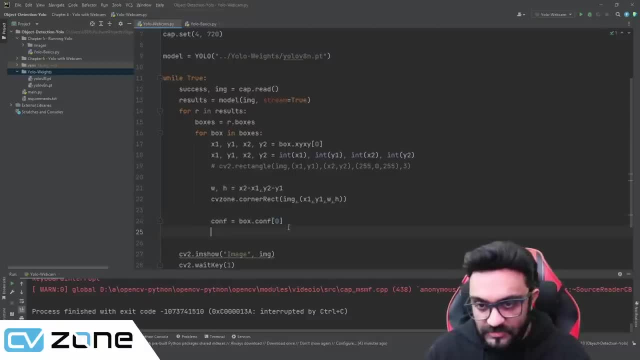 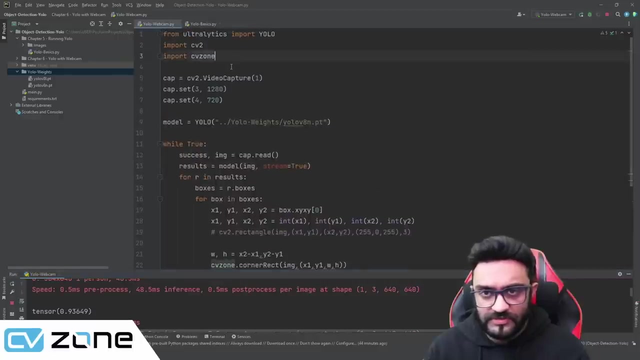 zero. so this is the confidence. so let's print that out and see if it works. so if we go down, and there you go, you can see the confidence values. but we want it to be rounded. so what you can do is you can use math. so import, import math. 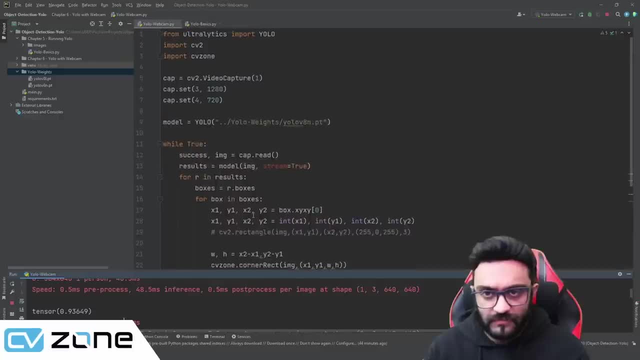 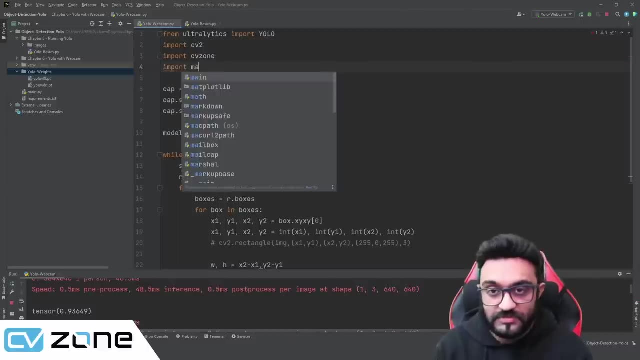 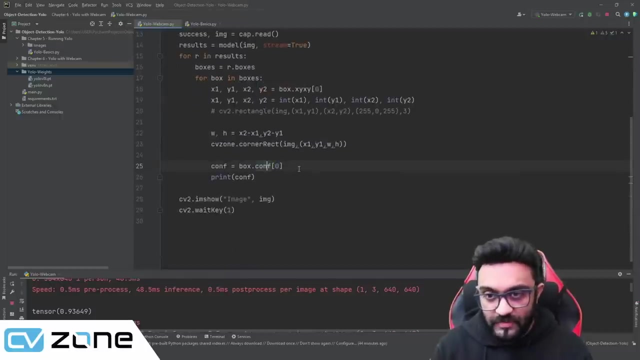 so, but we want it to be rounded. so what you can do is you can use math. so imports, imports math, and then over here you can change this value. so here we can write math dot. uh, you can write ceiling or floor, it's up to you. so seal and that's it, or 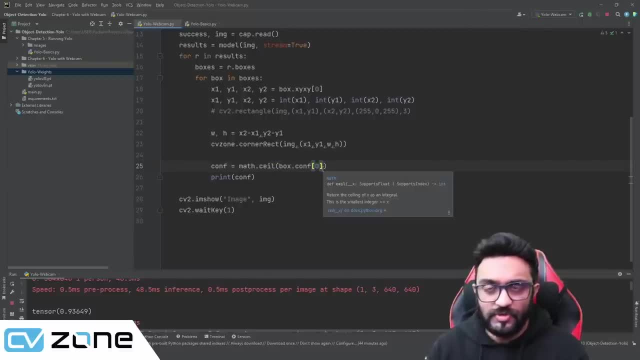 we, and based on what exactly do you want to round it off? so we want to round it to two decimal places. so we are going to multiply it by 100 and then we are going to divide it by 100. so that's the idea. so if we check the confidence values now, it will be two decimal places. 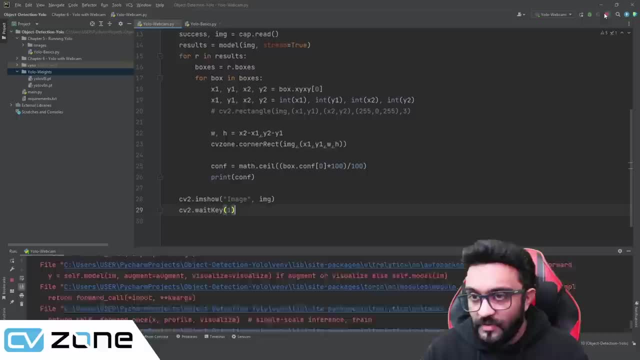 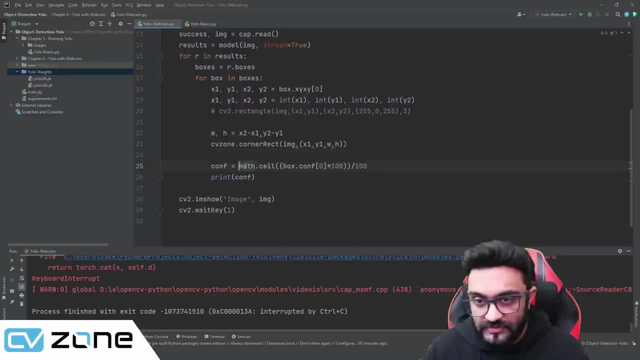 so hopefully that should be good. and we are getting one because we made a mistake here. it should be, the bracket should be here. so you are doing the ceiling for this and then you are dividing it by 100. there you go. so now you're getting 0.94. so that is good. uh, now we can display it. so to display: 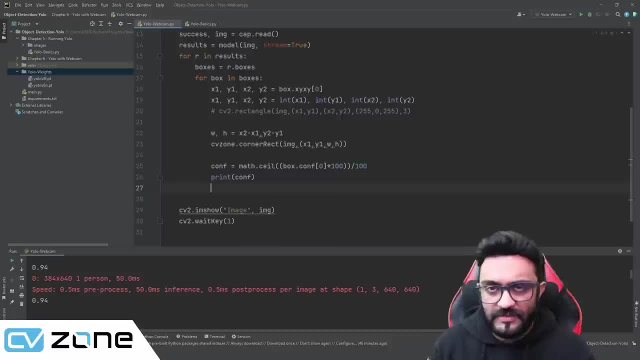 we are going to use cv zone. uh, now, what exactly are we going to display? we are going to display the confidence and the class name. so we need a box, a rectangle, on top of which we can display this, because if we just display it on the image, it is not very clear, depending on the background. so if 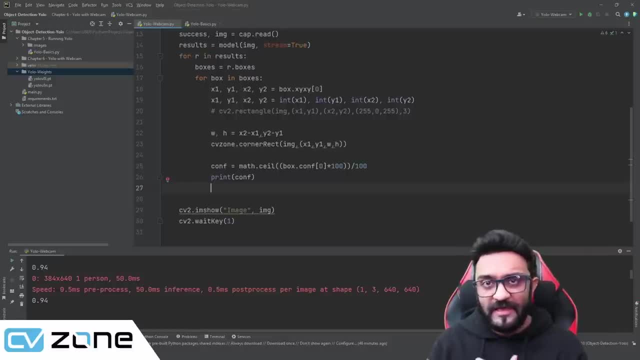 the background is in contrast, it will actually display well, if our, if they are pretty much the same color, it will fade away. so that's why we want a rectangle, and on top of the rectangle we want a text. now, uh, if we create a rectangle using opencv and then we put the text on it, then it won't be. 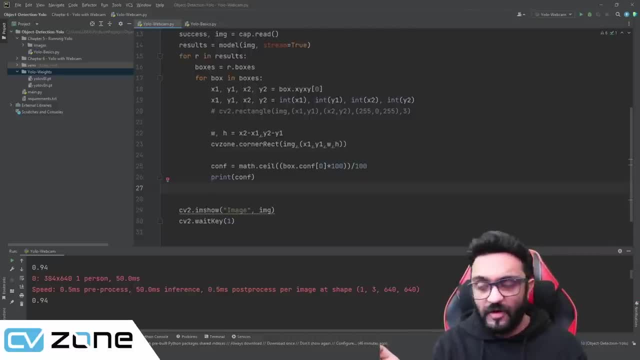 centered. uh, if the text is bigger, it will move away, it will move out of the box, and things like that. so in order to fix that, we have a function in cv zone that will create the rectangle, it will put it: uh, it will put the text on the rectangle and it will center it based on the length of the text. 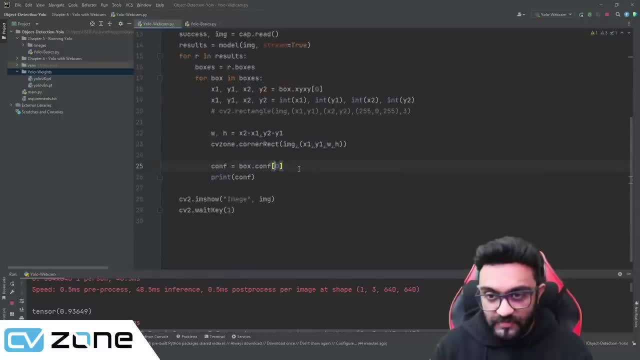 and then over here you can change this value. so here we can write math dot, you can write ceiling or floor, it's up to you. so seal and that's it, or we, and based on what exactly do you want to round it off? so we want to round it to two decimal places, so we are going to 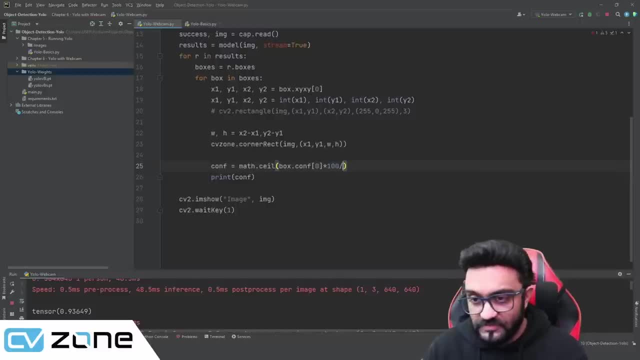 multiply it by 100 and then we are going to divide it by 100.. so that's the idea. so if we check the confidence values now, it will be two decimal places. so hopefully that should be good and we are getting one because we made a mistake here. it should be. 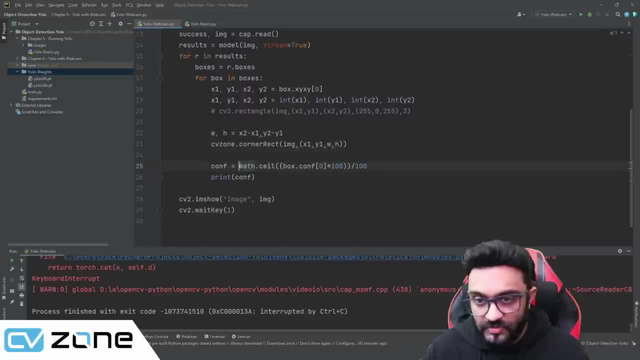 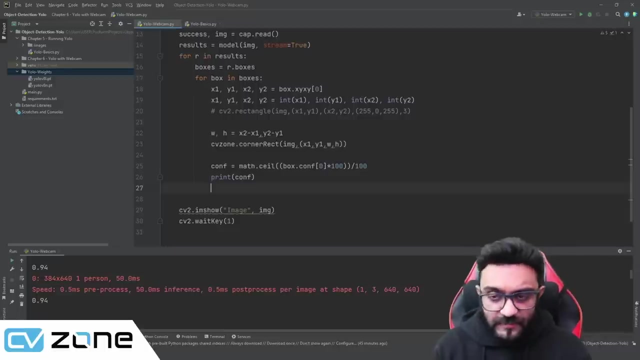 the bracket should be here. so you are doing the ceiling for this and then you are dividing it by 100.. there you go. so now you're getting 0.94. so that is good. uh, now we can display it. so to display: we are going to use cv zone. uh, now, what exactly are we going to display? we are going to. 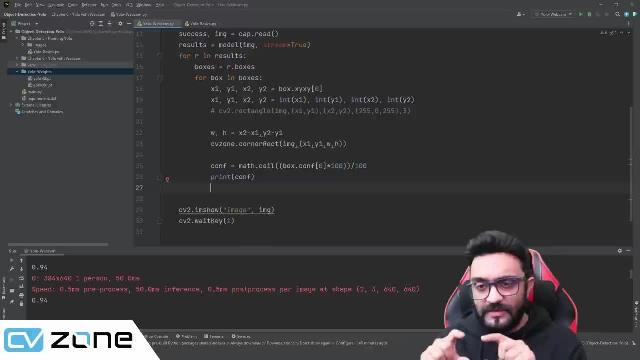 display the confidence and the class name. so we need a box, a rectangle, on top of which we can use cv, and then we can display this, because if we just display it on the image it is not very clear, depending on the background. so if the background is in contrast it will actually display well. 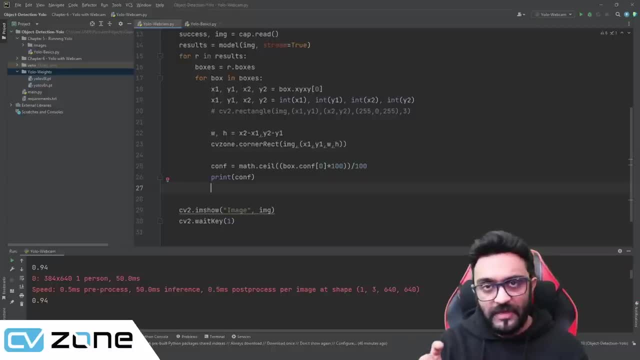 if our, if they are pretty much the same color, it will fade away. so that's why we want a rectangle and on top of the rectangle we want a text. now, if we create a rectangle using opencv and then we put the text on it, then it won't be centered. uh, if the text is bigger, it will move over the rectangle and 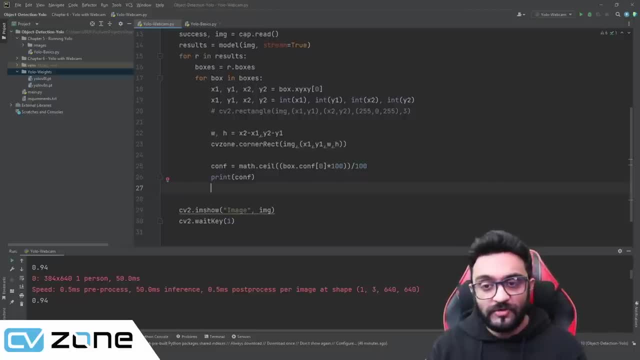 away, it will move out of the box and things like that. so in order to fix that, we have a function in cv zone that will create the rectangle, it will put it- uh, it will put the text on the rectangle and it will center it based on the length of the text. and all of this is done automatically so we can write. 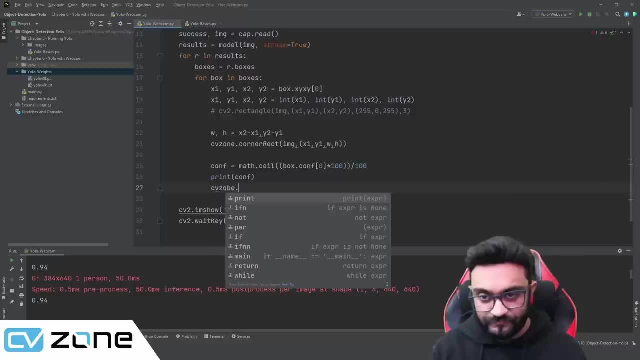 and all of this is done automatically so we can write here cv on cv zone dot. uh. put text correct and we are going to give in our image and then we have to give in the text. so the text. let's put it an f string for now, because later on. 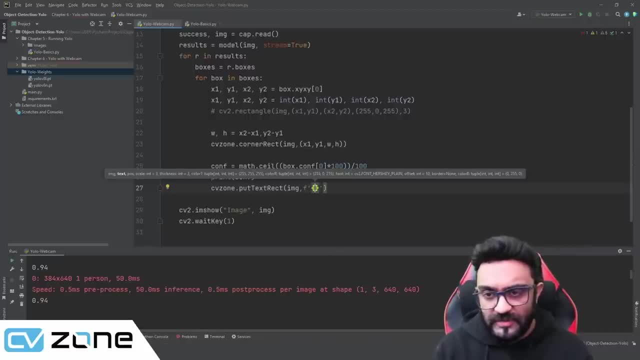 we are going to add some stuff to it, so the f string will contain the confidence for now, and then we'll give in the position. now the position should be the starting value of our x and y, so it will be x1 and y1, but because y1 will bring it a little bit down, we wanted to push it up a little bit. 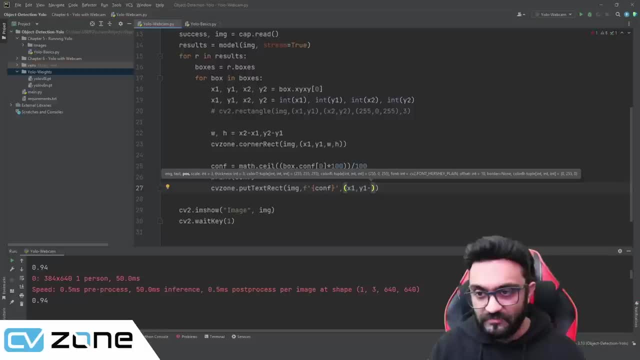 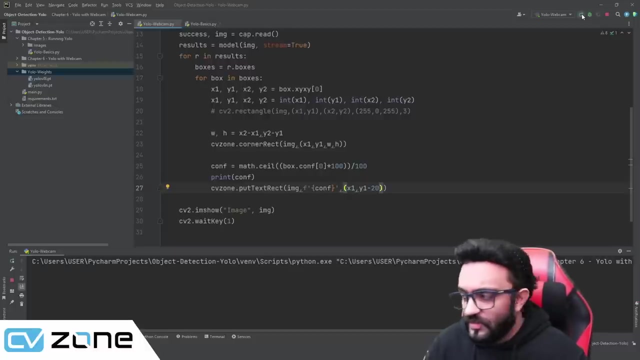 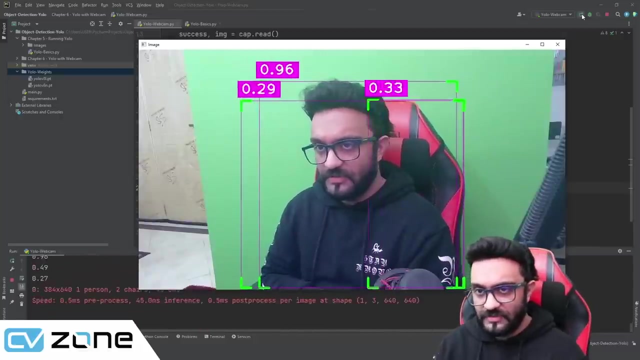 so we can say minus. let's say 20 or 30 or 50, let me check something like that. so let's run that and see if it works. now this will give us an issue and i will tell you what that is. there you go. now it's giving us 0.96 and if i bring 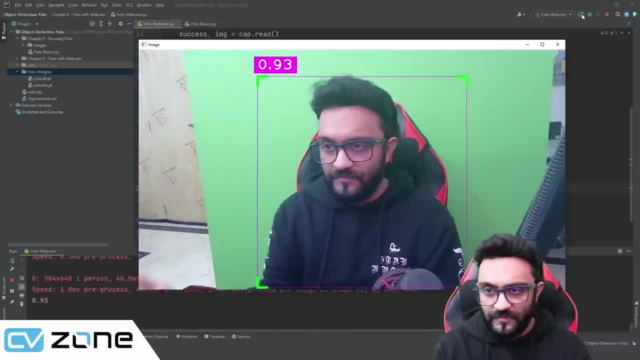 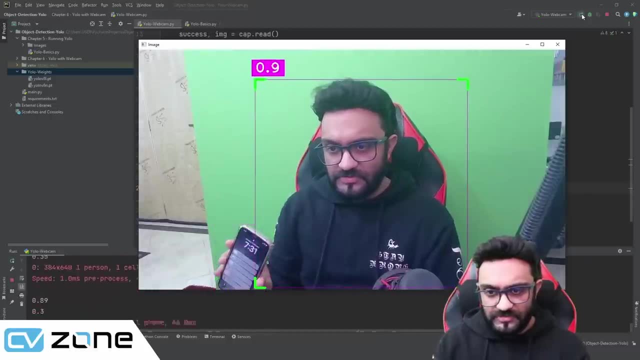 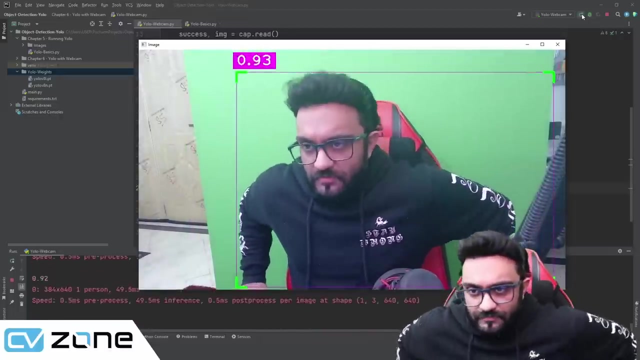 this in 0.94. that's good. if i bring in my phone, there you go. if i push it up, it goes up. if i bring it down, it goes down- there you go. so if i go up a bit, there you go. so that's the idea. but 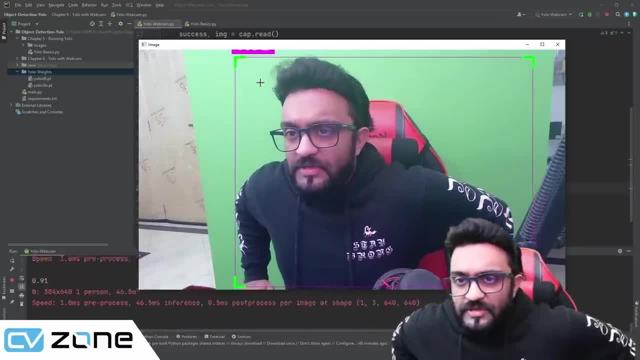 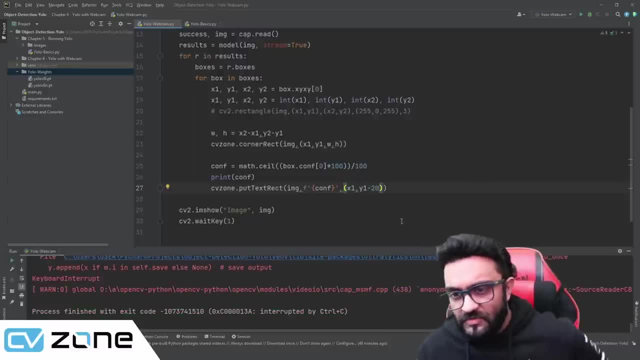 here. the problem is that if i go up, you can see the the text actually goes out and that that is not what we want. uh, we want it to display. so what we can do is we can write here: take the max, whether it's zero or this value. 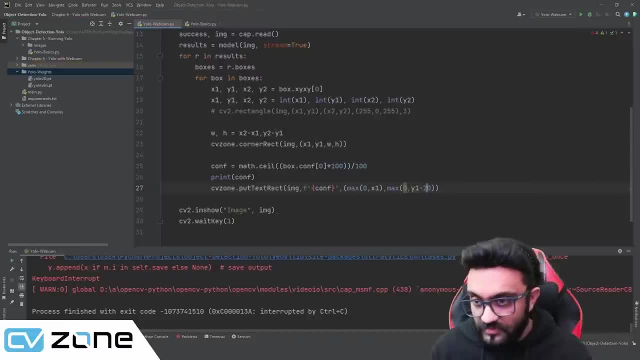 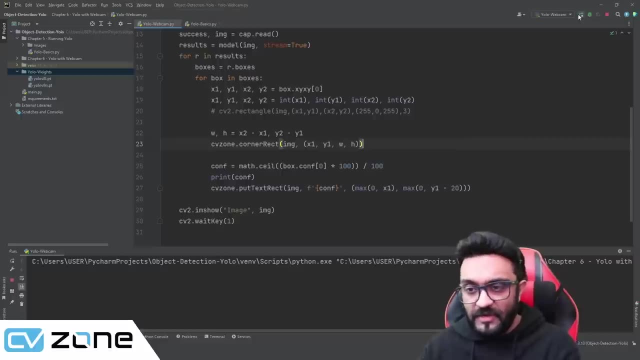 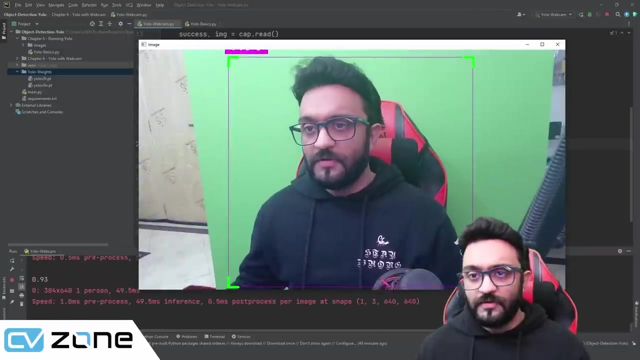 and take the max, whether it's zero or this value, and then we can write here: so whichever one is bigger, because if it goes in minus, then use zero, so it will not go above that, it will stay within. so let's try that out. there you go. 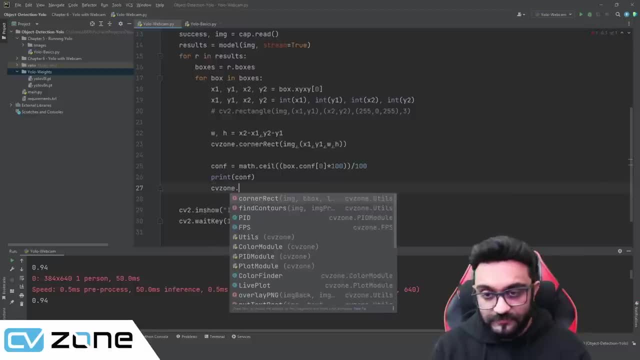 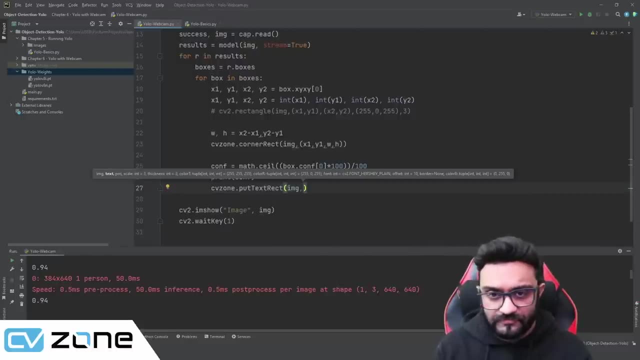 here: cv zone, cv zone, dot. uh. put text correct and we are going to give in our image and then we have to give in the text. so the text- let's put it an f string for now, because later on we are going to add some stuff to it. so the f string will contain the confidence for now and then we'll give in the position. 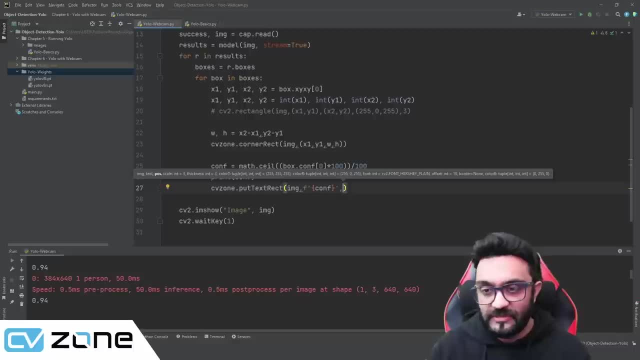 now the position should be the starting value of our x and y, so it will be x 1 and y 1, but because y 1 will bring it a little bit down, we wanted to push it up a little bit so we can just go to the exactly people, which is兽 and one of my favorite projects, isivia. 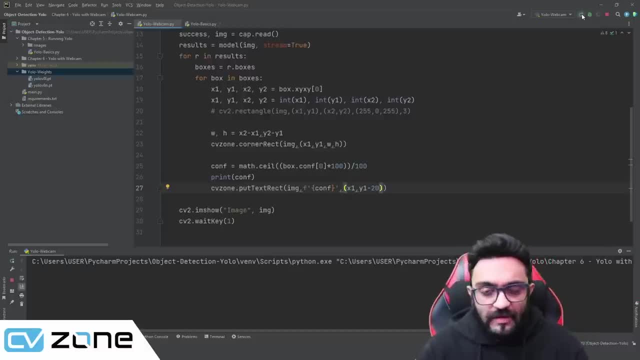 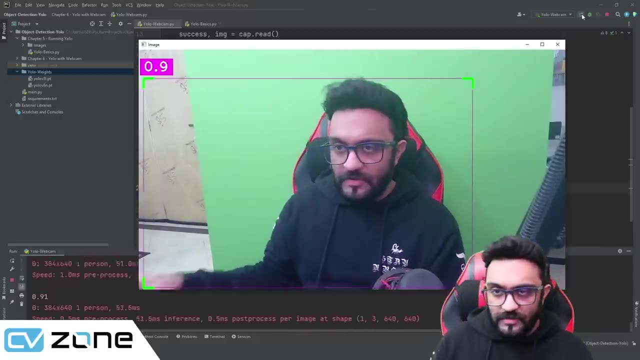 which was slip of the tongue. we're going to have a little thread here. now the thread of the card is saved in a way that it can beперaced here, for example. so i'll put it like this: okay, and now it will call octa for the background. and this is how we have Harmonia file game. we're going to call it theporximля and this thingきっisaleition. we can see minus, let's say everywhere, 30 or 30 or 50. let me check something like that. so let's run that and see if it works. now this will give us an issue. i will tell you what that is. there you go. now it's giving us 0.96 and if, if i bring this in, 0.94, that's good. if i bring thexx in, that's good. if if i bring the 1, 7 and 7 and discard, that's good. if i bring the 6 and the next, we get x�. masih living machine passwork prevention. 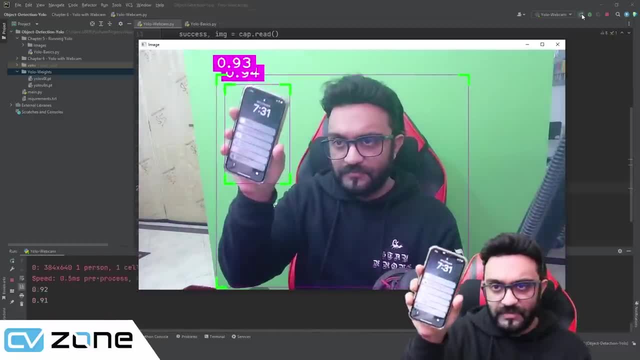 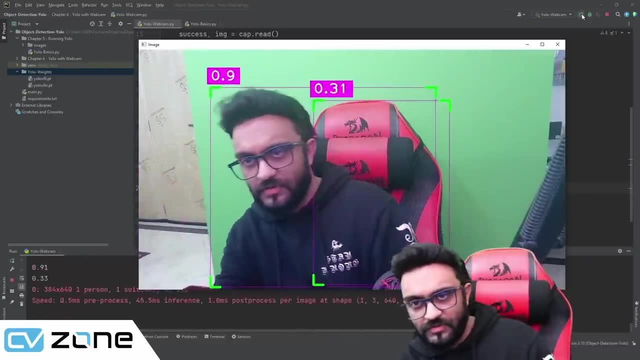 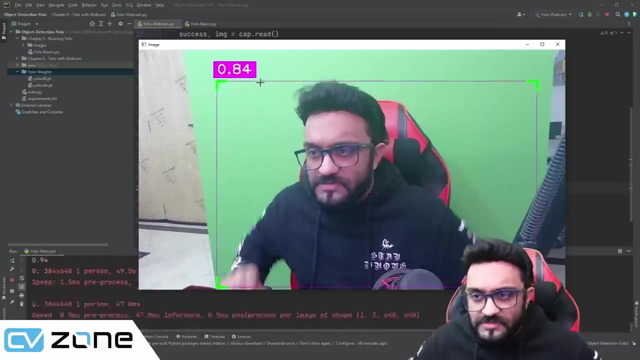 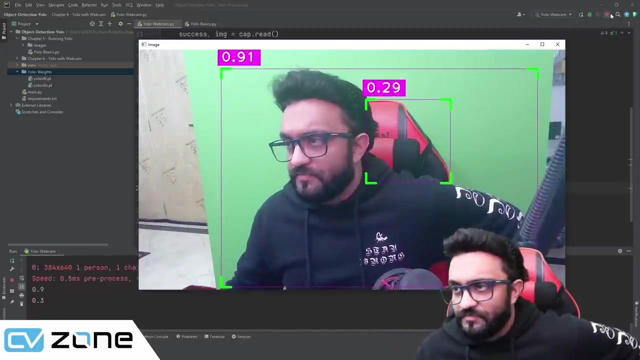 in my phone, there you go. if i push it up, it goes up. if i bring it down, it goes down- there you go. so if i go up a bit, there you go. so that's the idea. but here the problem is that if i go up you can see the. the text actually goes out: um, and that that is not what we want. uh. 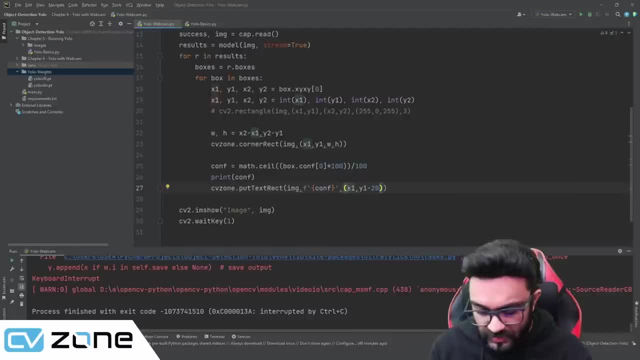 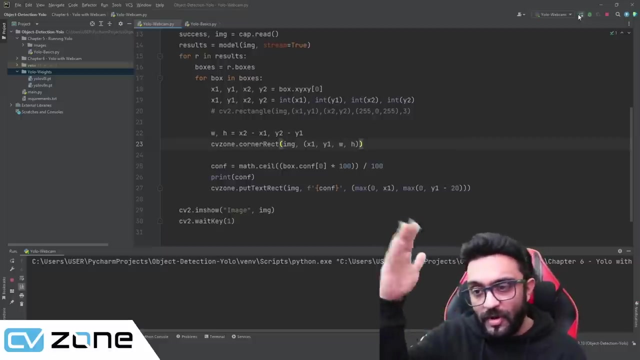 we want it to display. so what we can do is we can write here: take the max, whether it's zero or this value, and take the max, whether it's zero or this value, so whichever one is bigger, because if it goes in minus, then use zero, so it will not go above that, it will stay within. so let's try that out. 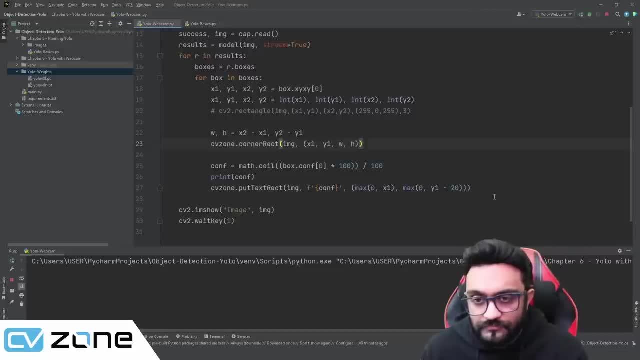 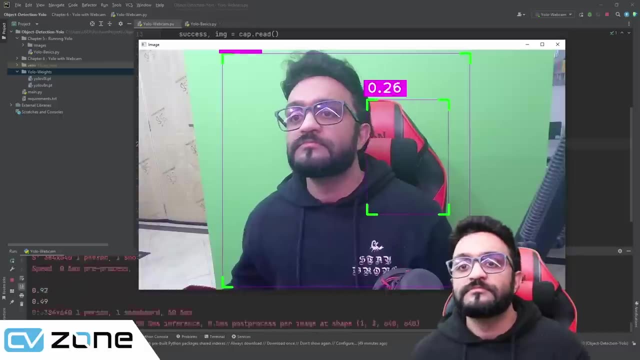 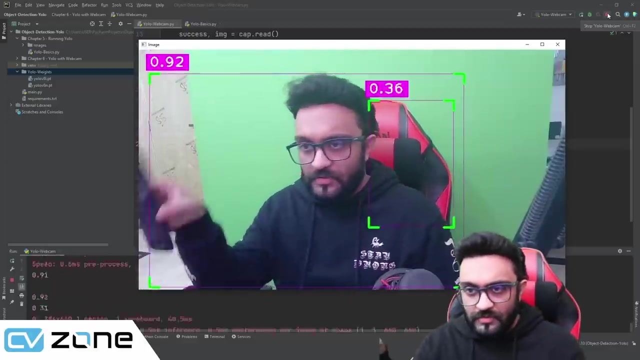 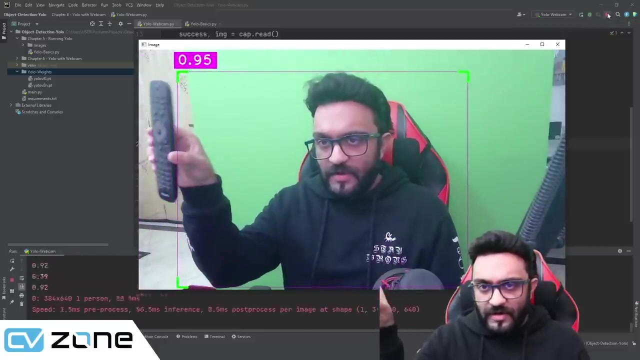 let's see if it works. there you go, it doesn't seem to work very well. uh, if we go here, uh, if we go to the side, it it's working on the side, but it's not working on the why? um, because we already have a minus 20. 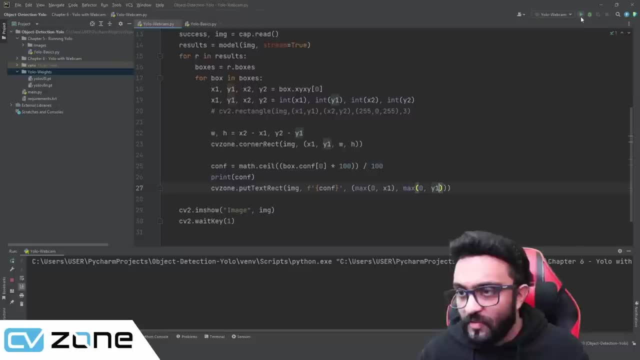 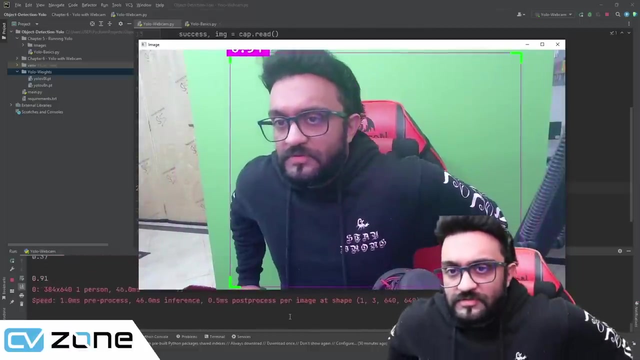 in there. so let's remove the minus 20 and hopefully this will work better, or or what we can do is we can put here 20.. so if we go up, let me just go like this. yeah, it's not working very well, so let's try. 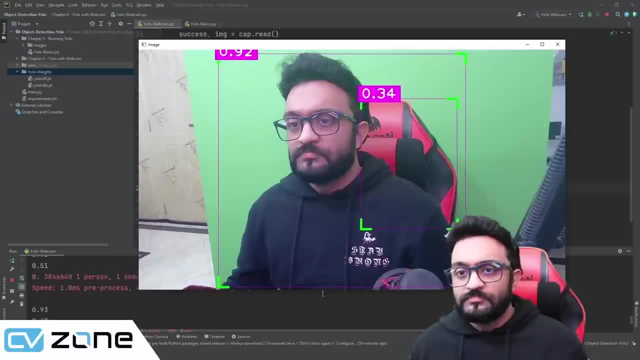 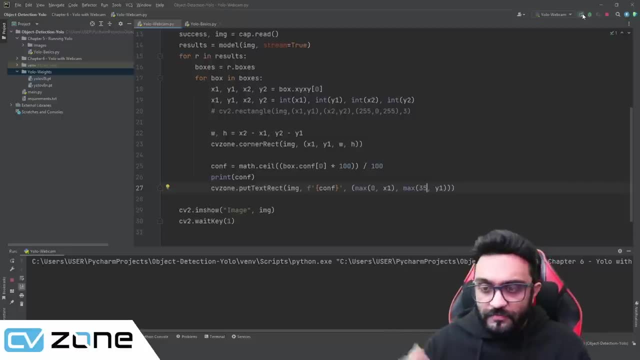 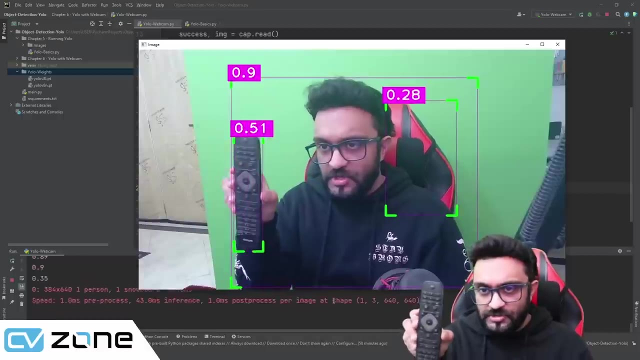 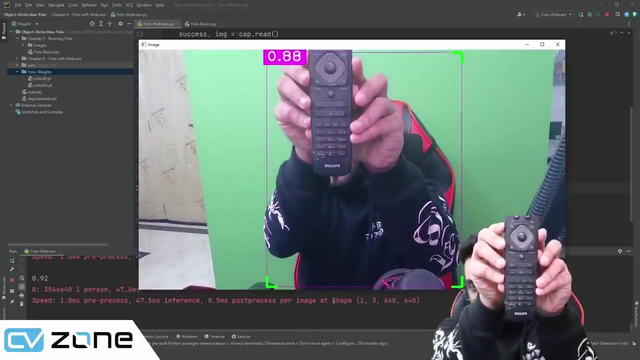 20 or y1. yeah, now it's better, so maybe make it 35, so it doesn't go beyond that. there you go, so now it's actually showing us. so if i have this remote and if i push it up, the confidence level stays there even though it's going out of. 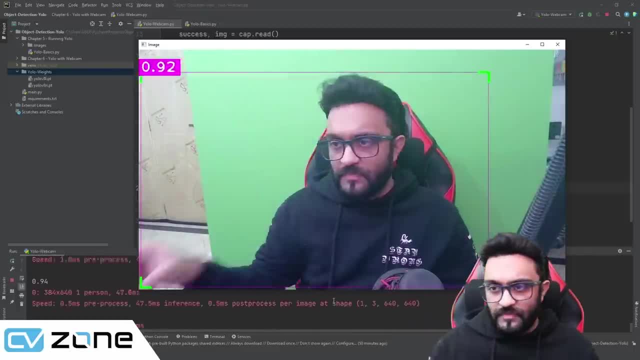 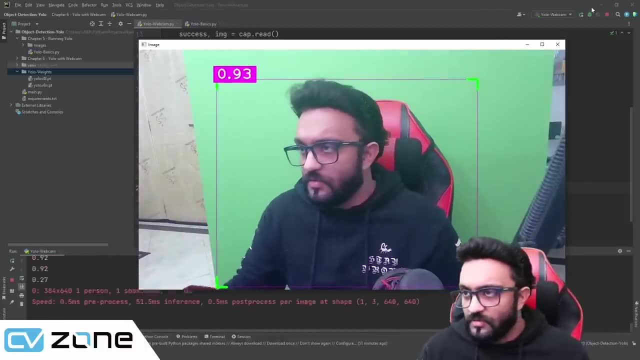 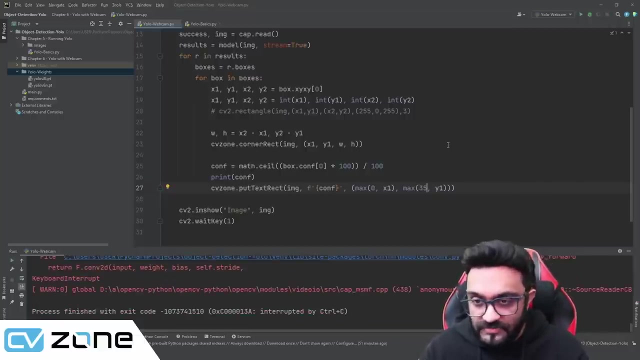 the image. there you go. so that's that's good, that's good. let's see the phone. yeah, it's working fine, okay, so this is good. now what we need is the class. so we need to know what class are we detecting. is it a person, is it a car? is it a bike? what exactly are we detecting? so this is: 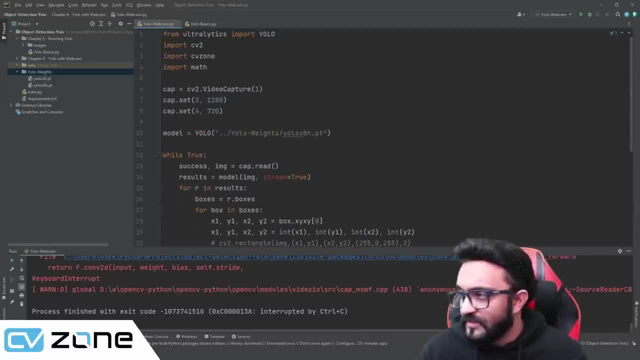 based on the poco data set, and what we can do is we can get the class names for that, so i've already created um what do you call a list? this is a class name and we can get the class names for that, because i've already created um what you call a list, so we just 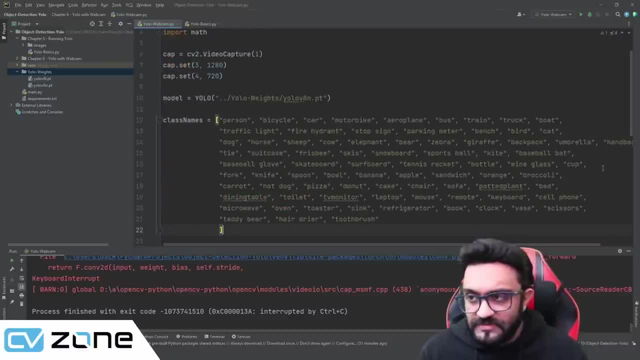 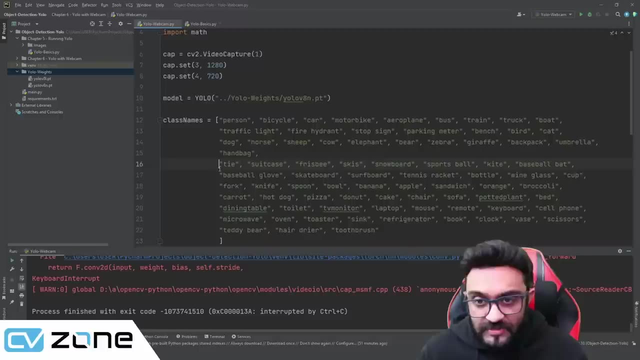 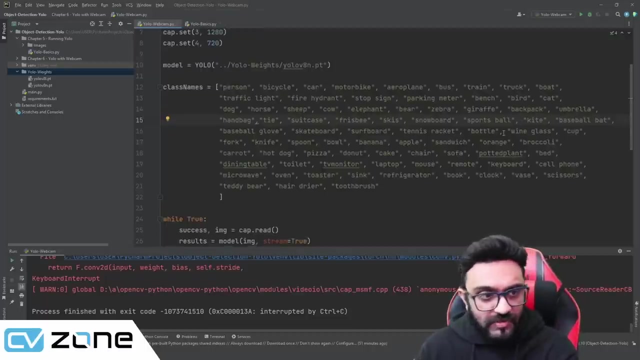 and you can get this list from our website again. you can download it for free now. if you don't want to do that, the other thing you can do is you can simply type it from here. so right now you can see it's showing the complete thing on the screen. so if you want to go ahead and simply type it out, 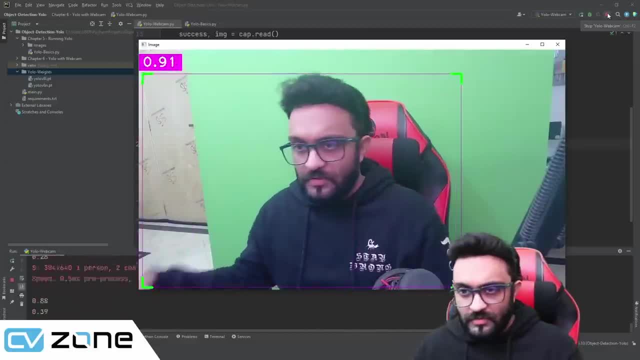 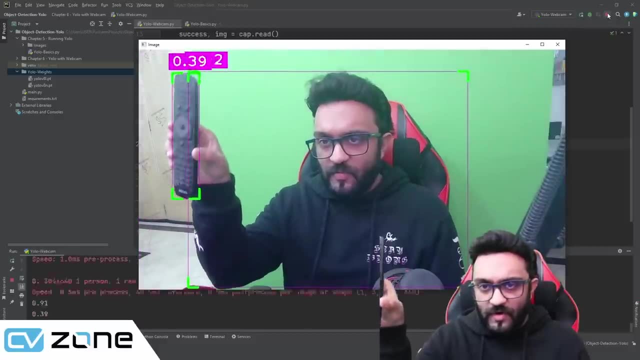 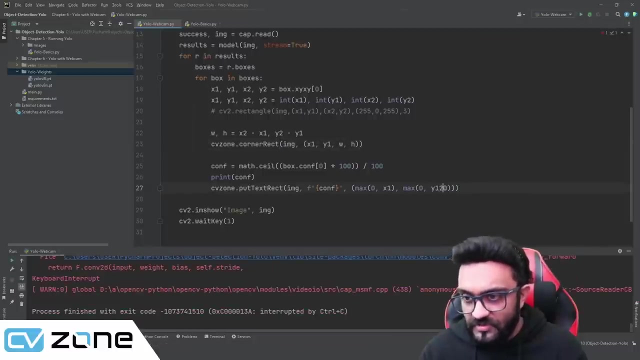 it doesn't seem to work very well. if we go here, uh, if we go to the side, it's working on the side, but it's not working on the y? uh, because we already have a minus 20 in there. so let's remove the minus 20 and hopefully this will work better. 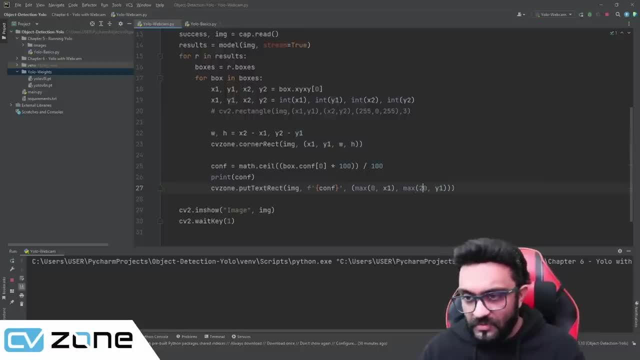 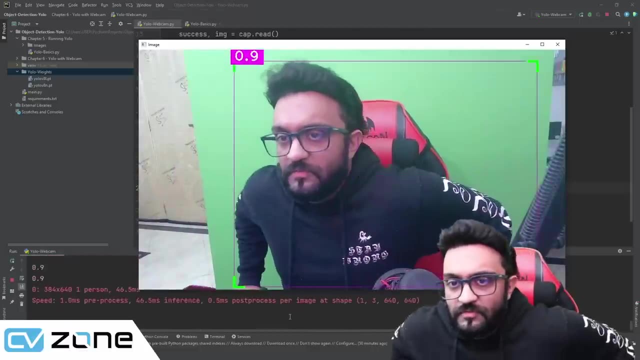 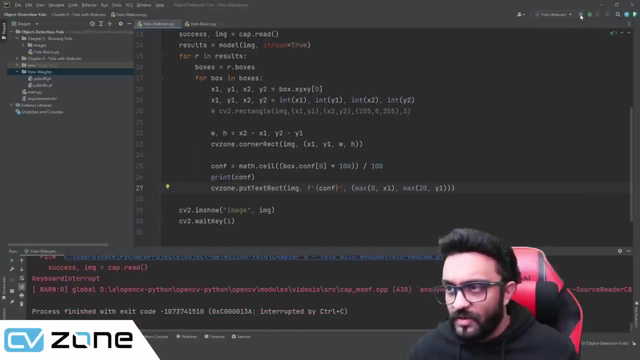 or, or. what we can do is we can put it here: 20.. so we go up. let me just go like this: yeah, it's not working very well, so let's try 20 or y1. yeah, now it's better, so maybe make it 35, so it doesn't go beyond that. 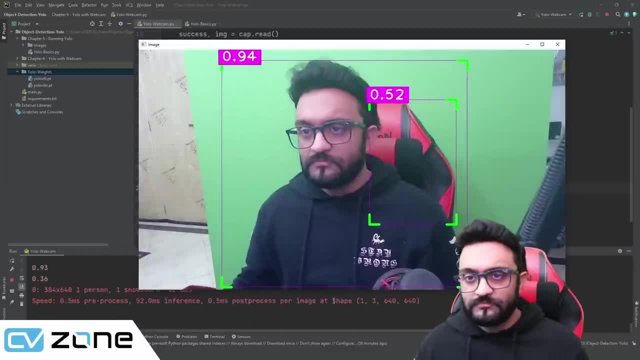 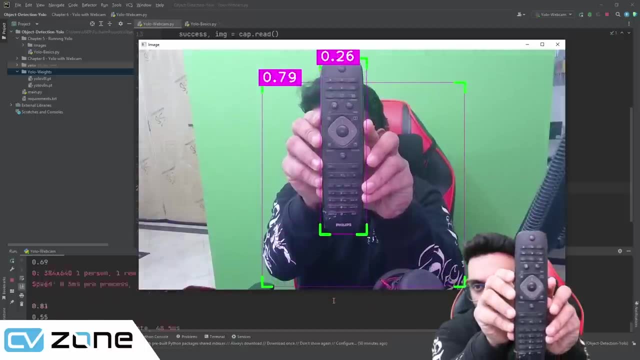 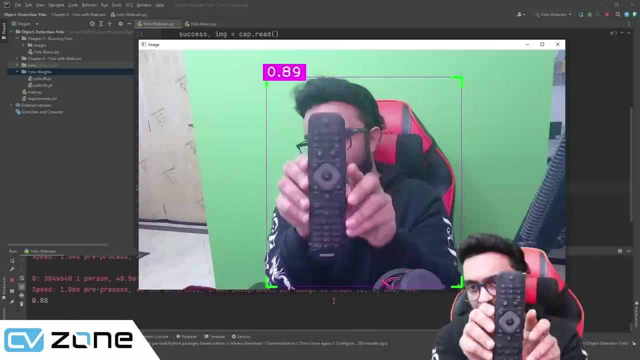 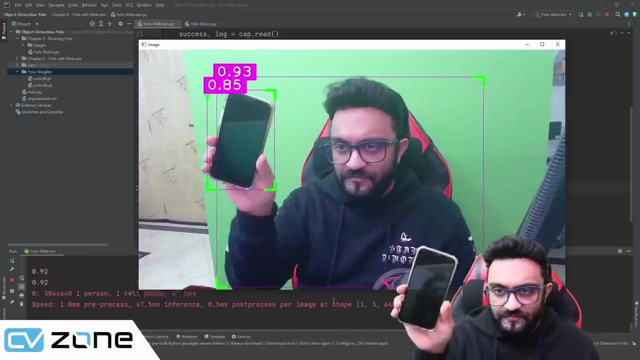 there you go. so now it's actually showing us. so if i have this remote and if i push it up, the confidence level stays there, even though it's going out of, uh, the image. there you go. so that's that's good, that's good. let's see the phone. yeah, it's working. 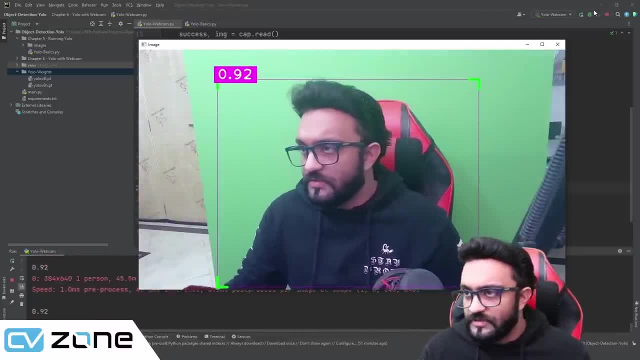 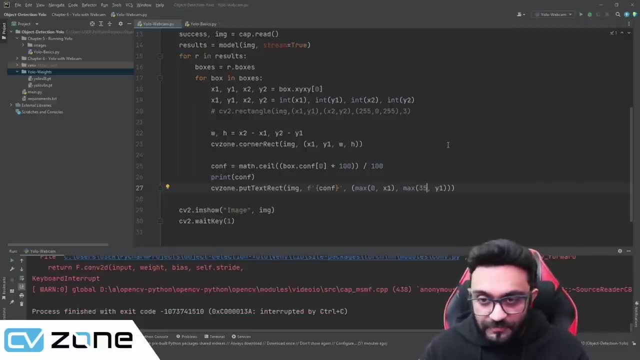 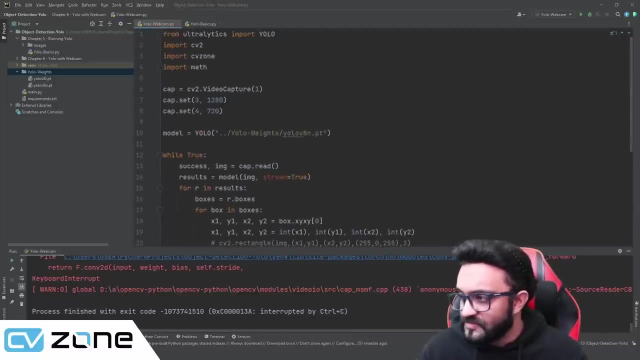 fine, okay, so this is good. now what we need is the class. so we need to know what class are we detecting. is it a person, is it a car, is it a bike? what exactly are we detecting? so this is based on the coco data set, and what we can do is we can get the class names for that. so i've already created. 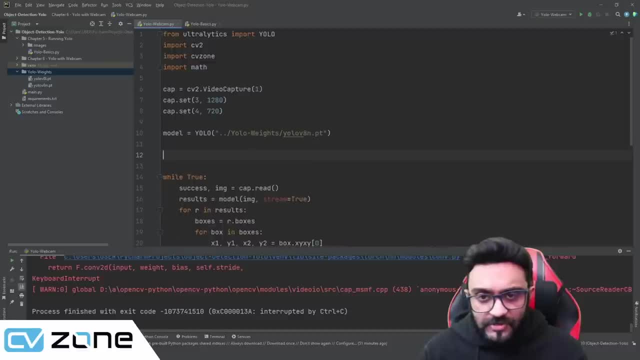 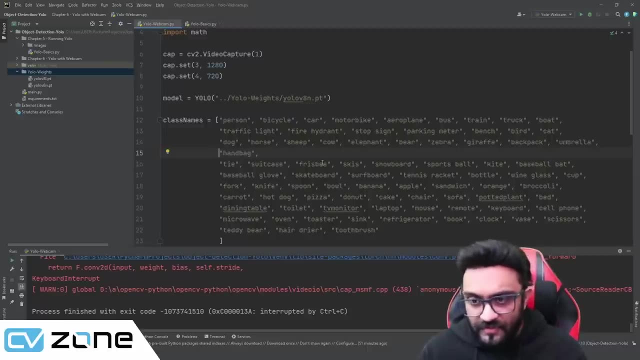 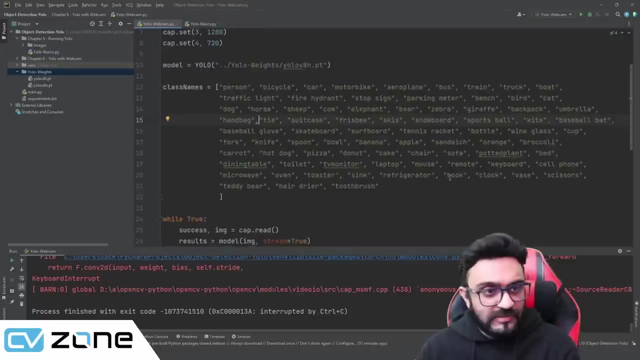 um, what you called a list, and you can get this list from our website again. you can download it for free now. if you don't want to do that, the other thing you can do is you can simply type it from here. so right now you can see it's showing. 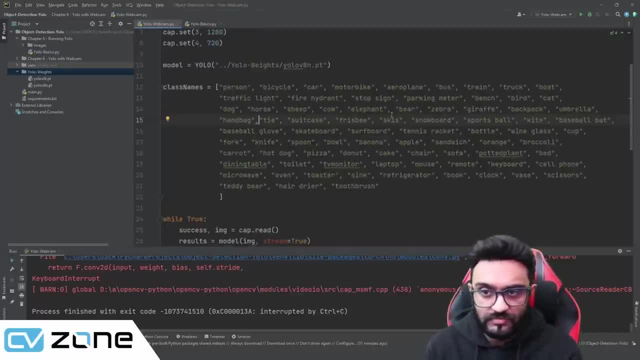 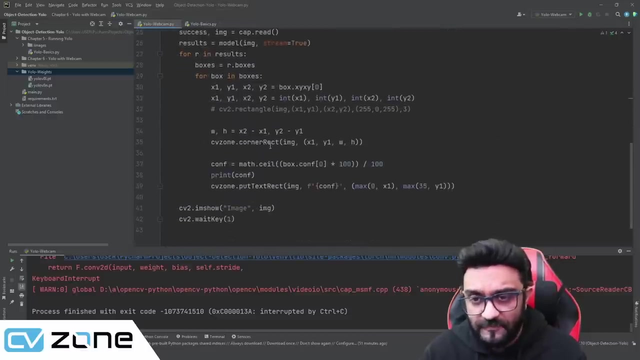 the complete thing on the screen. so if you want to go ahead and simply type it out, you can type all these 80 classes so person, bicycle, car, motorbike, airplane, blah, blah, blah and all of these. so it should be in a list called class names. so once we have that, we need to find the id number. 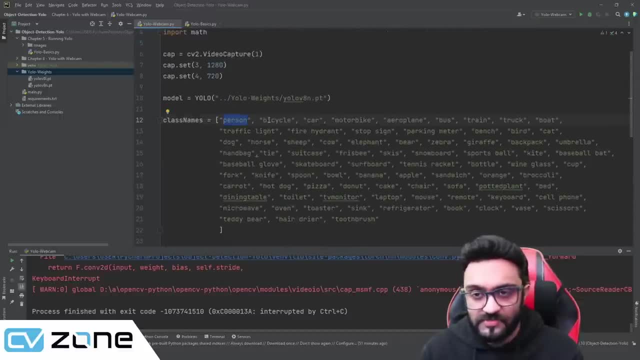 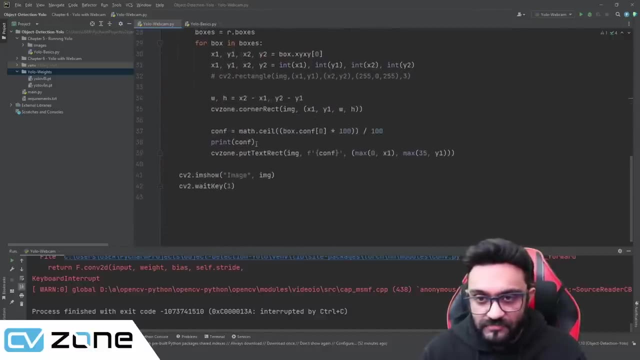 so if the id number is zero, it will be a person, if the id number is one, it will be a bicycle, id number two is a car, and so on. so what we need to do is we need to find the confidence, uh sorry, the the class. so here we. 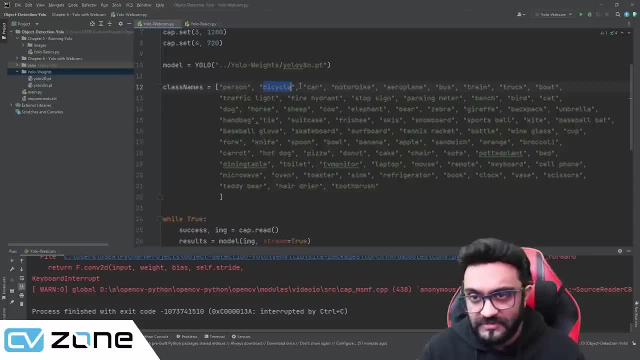 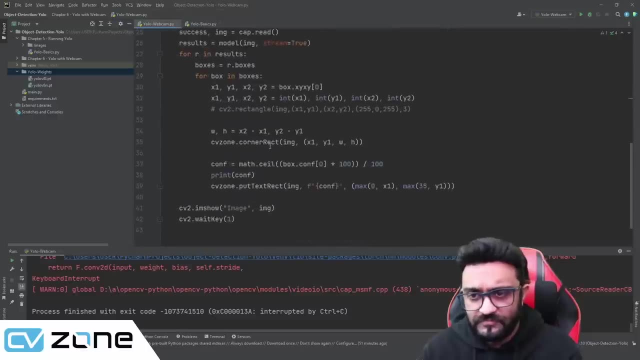 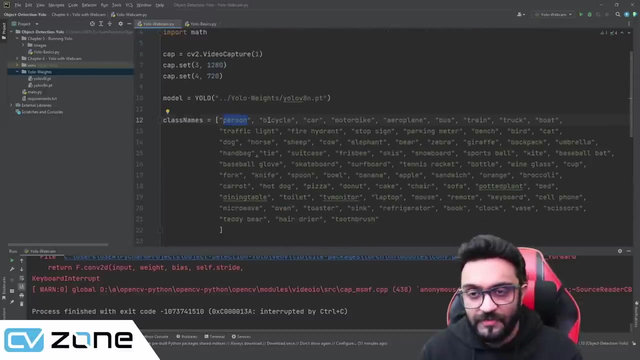 you can type all these 80 classes so: person, bicycle, car, motorbike, airplane, blah, blah, blah and all of these. so it should be in a list called class names. so once we have that, we need to find the id number. so if the id number is zero, it will be a person, if the id number is one, it will be a. 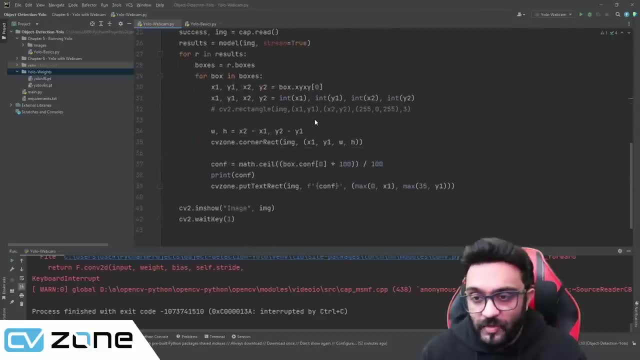 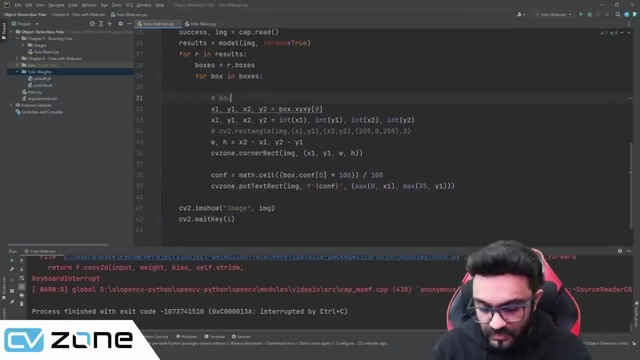 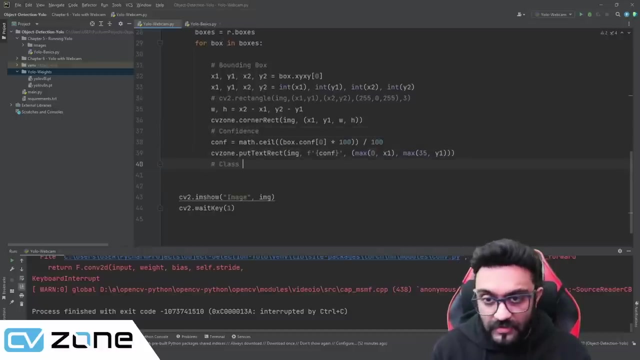 bicycle. id number two is a car, and so on. so what we need to do is we need to find the confidence, uh sorry, the the class. so here we found the bounding box. this is for bounding box, let's write here so box. this here is for the confidence, and now we are going to do it for the class name. 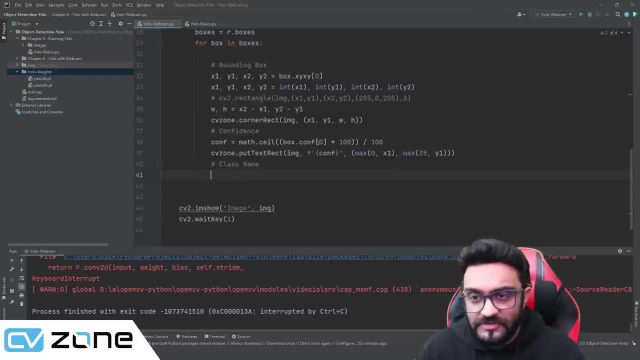 so for the class name, what you have to do is you are going to use the same format. you will write cls. you can't write class because- because you can't use class for obvious reasons. so here you will write class, cls, and then box and you will write here, cls. so that will give you the class name. so let's print it out. 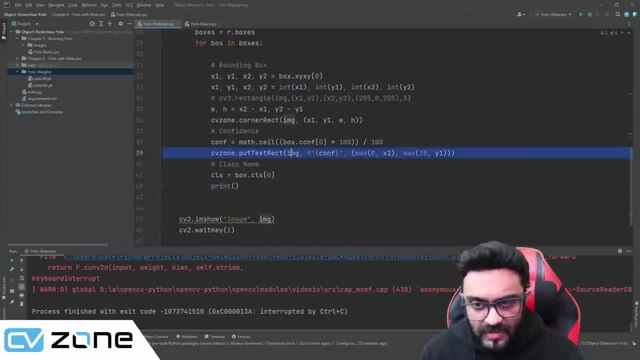 or let's put it on the rectangle. so let's remove it here and we will put it directly on the rectangle. we will write here: cls, we'll give it a space and then this. there you go. so this is for the confidence, this is for the class, and let's see if that works out. so let's print it out and then. 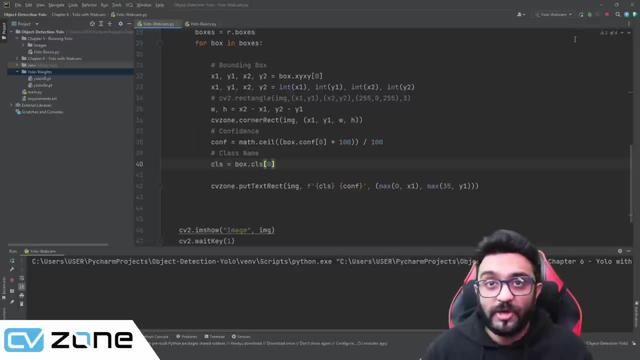 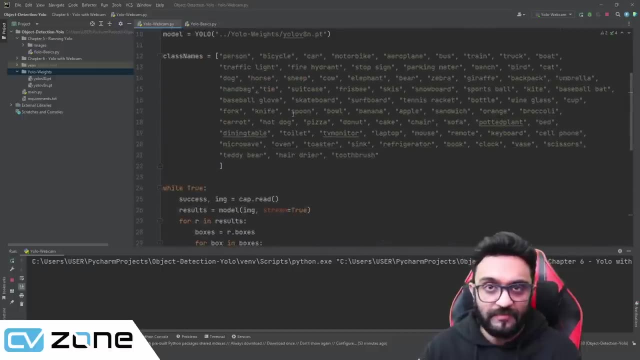 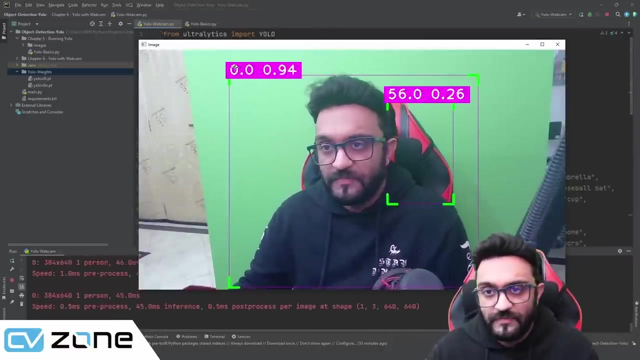 box out. so right now it will give us the class id. it will not give us the actual name because we are not referring it to our list. once we refer it to our list, it will give us the name as well. so for now it will just give us. it should give us id number zero. so here you can see 0.0. uh, it's decimal. 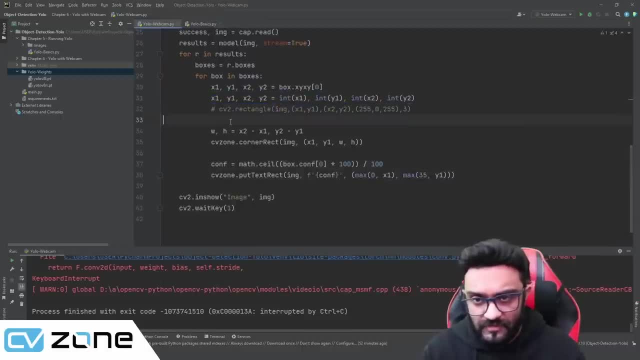 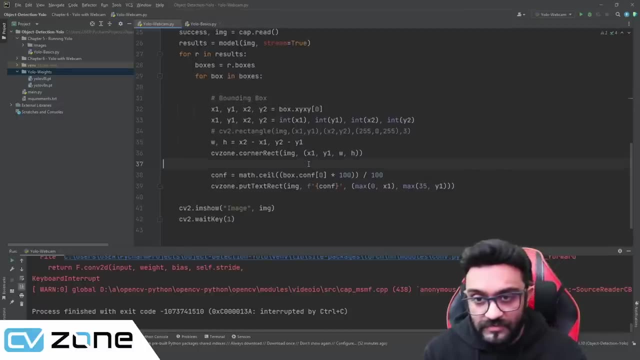 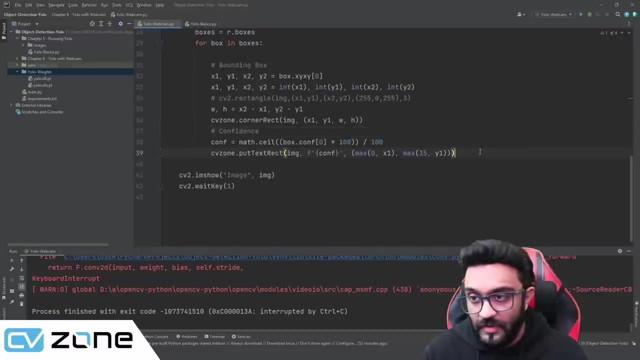 found the bounding box. this is for bounding box. let's write here: bounding box. this here is for the uh confi dense. and now we are going to do it for the class name. so, for the class name, what you have to do is you are going to use the same format. you will write cls. you can't write class because, because, 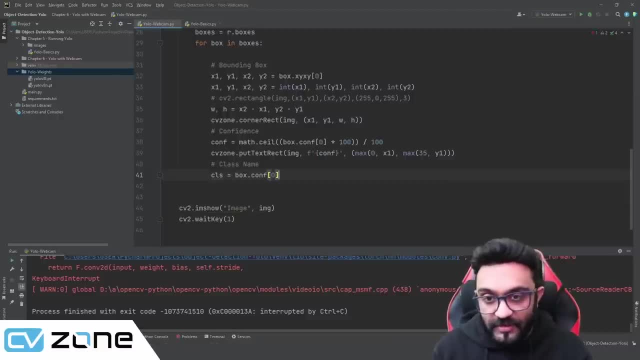 you can't use class for obvious reasons. so here you will write class cls and then box and you will write here, cls. so that will give you the class name. so let's print it out, uh. or let's put it on the rectangle. so let's remove it here and we will put it directly on the rectangle. we will write. 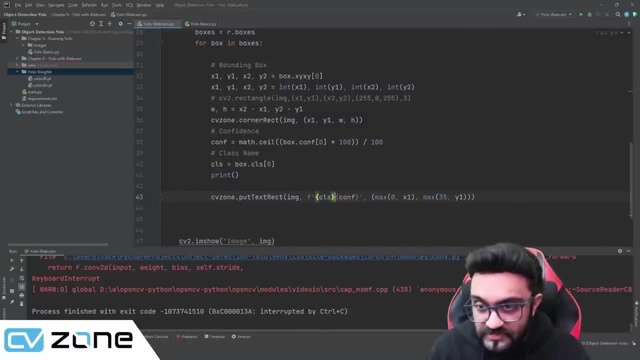 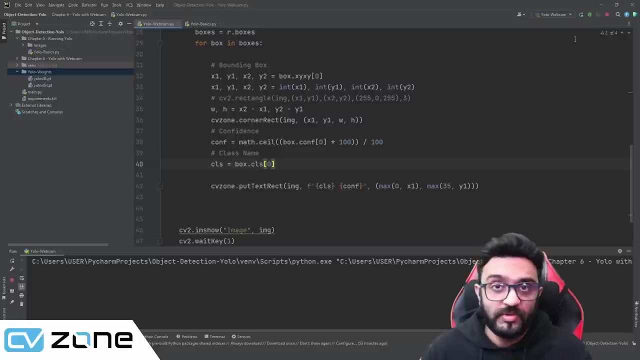 here. uh, c l s, we'll give it a space and then this. there you go. so this is for the confidence, this is for the class, and let's see if that works out. so right now it will give us the class id. it will not give us the actual name because we are not referring it to our list. once we refer it to our 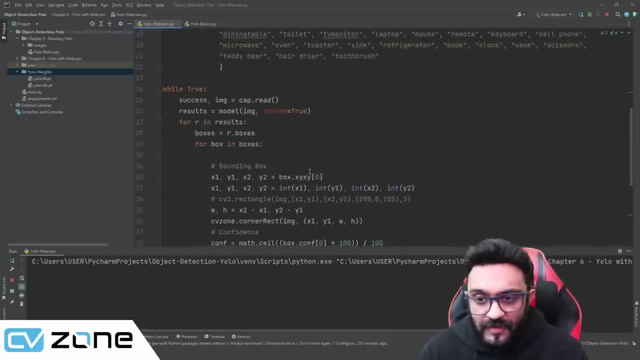 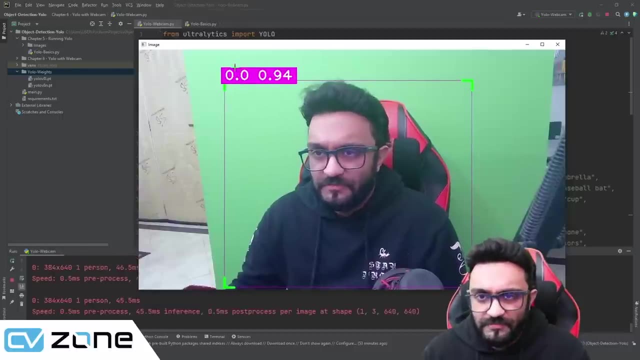 list. it will give us the name and we will give it the class name. so let's remove it here and let's put the name as well. so for now it will just give us it should give us id number zero. so here you can see 0.0. uh, it's decimal places. i'm not sure why, but uh, we will figure that out. the phone is 67. 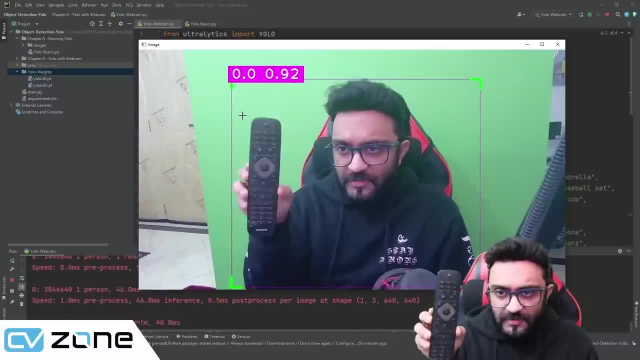 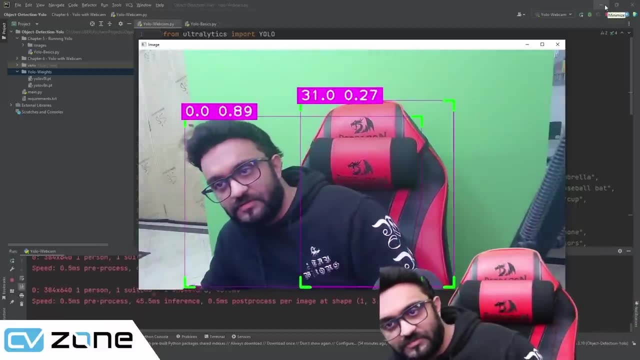 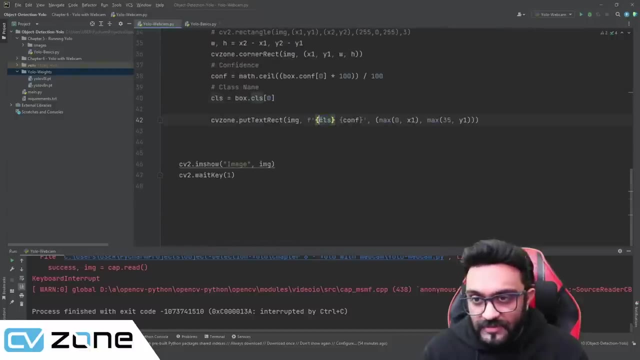 that's a very high class. remote is 65. so what about the chair? can you find the chair? can you find the chair? it's confused about the uh, about the chair anyways. so what we have to do is, instead of class, what we will write here. we'll write here class names. 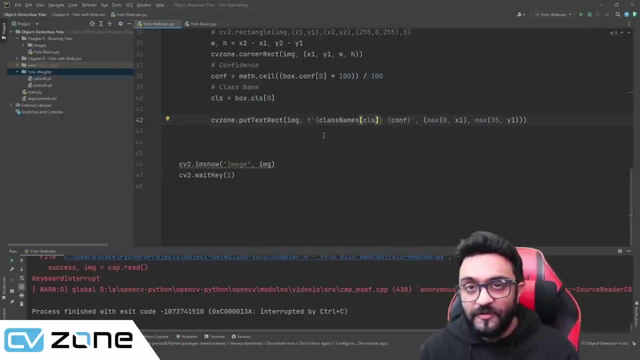 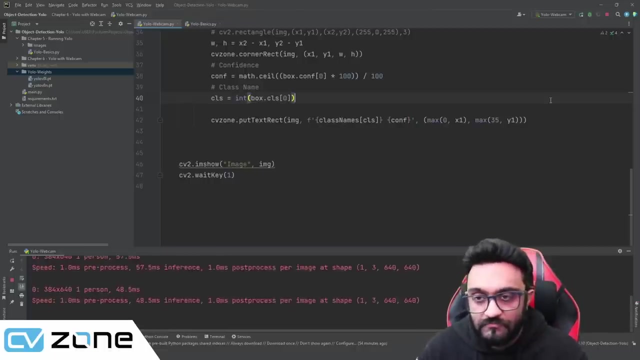 and then we will put in here class. but if you remember, it was a floating value, so we have to convert it into integer. so we'll put it here as integer and then if we run this now, this time around, it should give us the class name as well. so if we open this up, here you go, person 0.96. 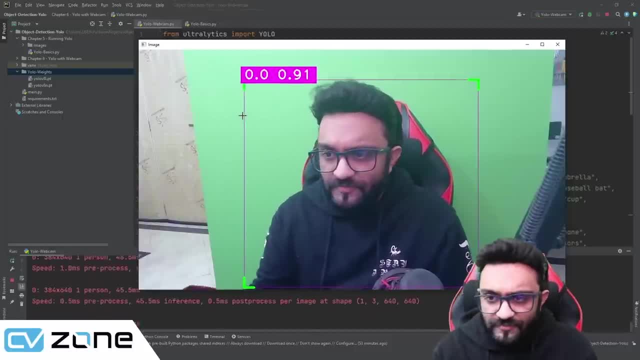 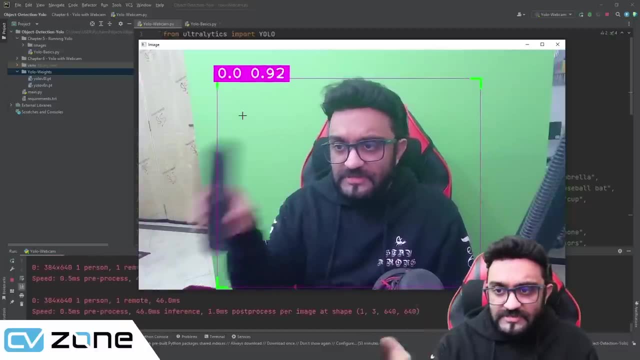 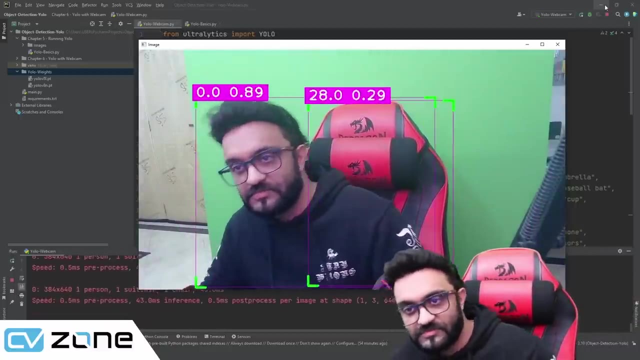 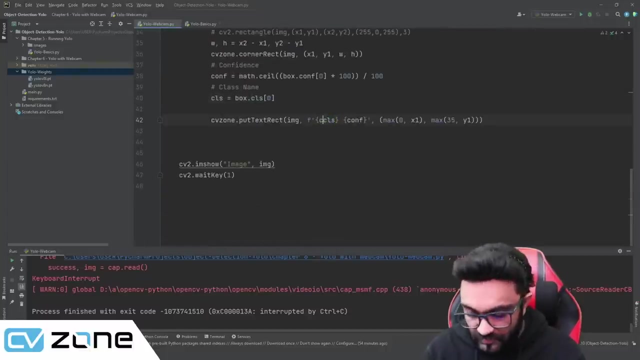 places. i'm not sure why, but, uh, we will figure that out. the phone is 67 and that's a very high class. remote is 65. so what about the chair? can you find the chair? can you find the chair? confused about, about the chair, anyways. so what we have to do is, instead of class, what we will write here. we'll write here. 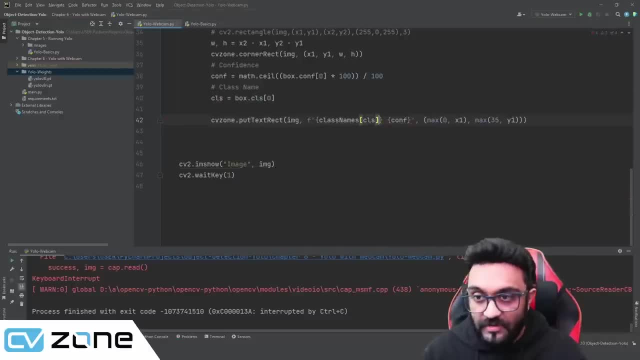 class names and then we will put in here class. but if you remember, it was a floating value so we have to convert it into integer. so we'll put it here as integer and then if we run this now, this time around it should give us the class name. so let's put it here and then we will put it here and then. 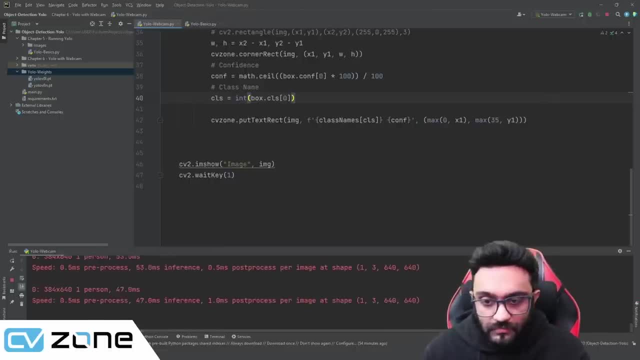 we will put it here, and then we will put it here and then me. so if we would close this up and then we'll rising and then? so this is the window, so we'll easily find it. uh, what does it look like to see the class name aproximadamente again? so we will never see this on here, but 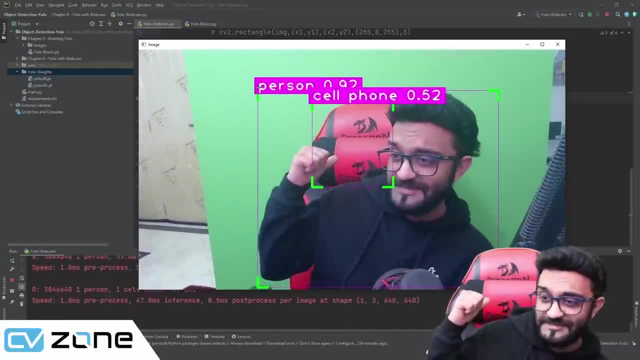 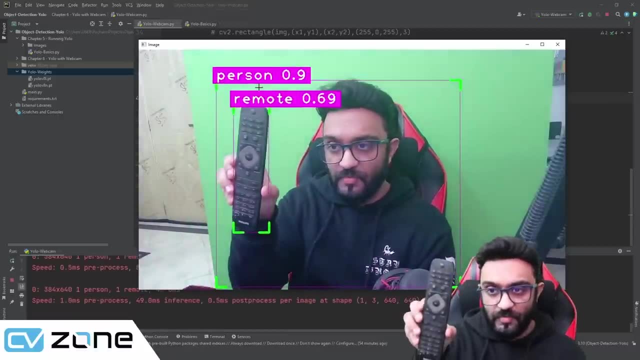 then if we have- don't see it, it does look like that. it looks like a class name as well. so if we open this up, here you go. person 0.96: confidence if we move around, uh, that's a suitcase, i'm not sure why. uh, so sometimes it's a chair, and then we have the remote. that's. 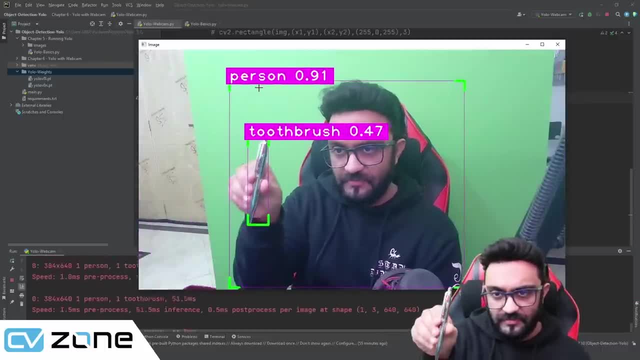 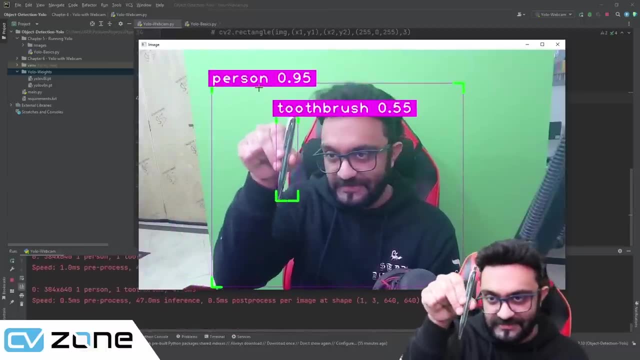 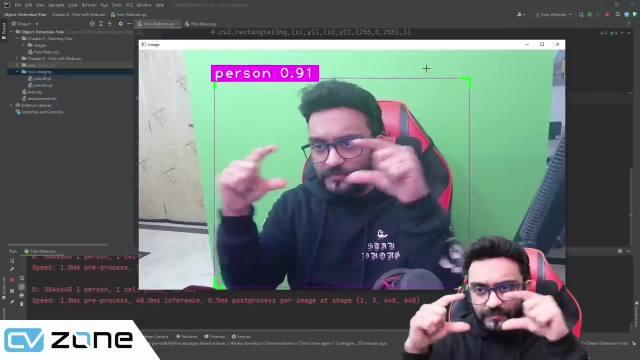 very good. uh, then we have the phone, the cell phone. that's very good. a toothbrush. i didn't know that. so it is actually detecting this as the toothbrush. that's fine, okay. so, uh, if you wanted to check it on a video, you can do that too, and if you wanted to make these, 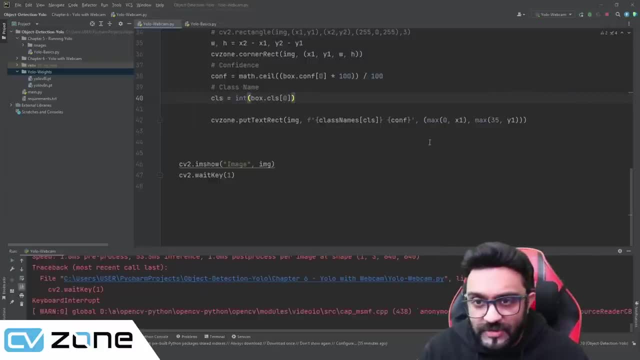 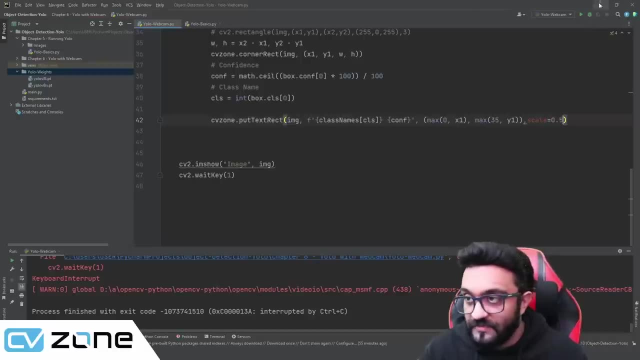 uh, names these labels a bit smaller. you can do that too. so here input text rect. here you can write scale and you can give in, let's say, 0.5, so that will squeeze everything down and make it smaller. uh, this will be helpful in case you have a lot of detections. for example, you have a lot of. 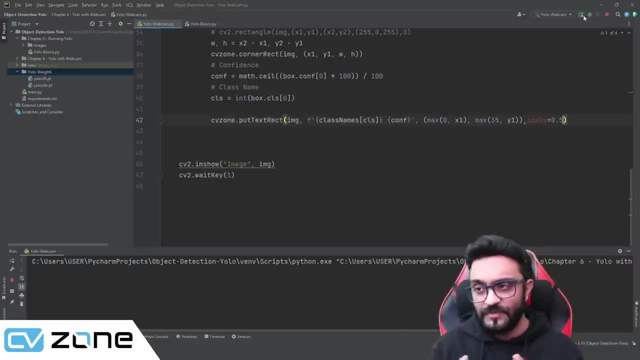 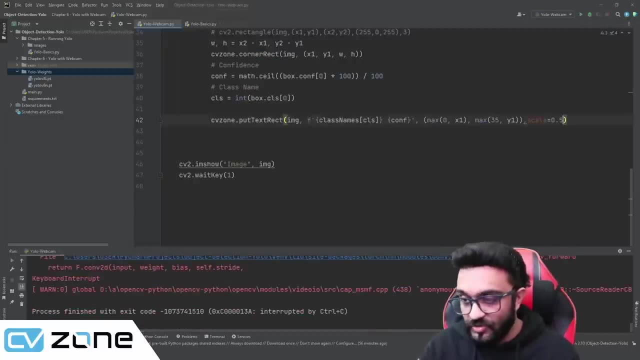 cars on a highway, or you have a lot of p, a lot of people being detected, so this will make it easier. so there you go, but then it's, it's a little bit harder to read, so you have to change. let's say, we'll put 0.7, then you also have to change the threshold, sorry, the thickness, the thickness, let's. 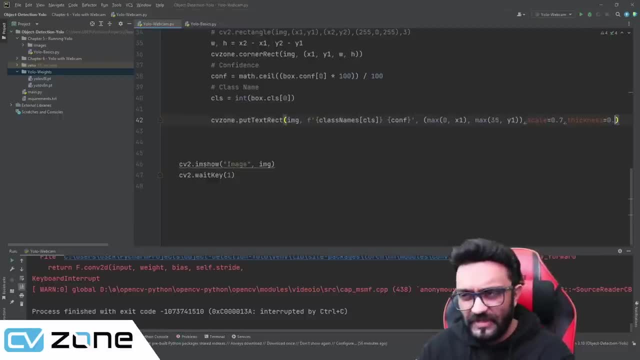 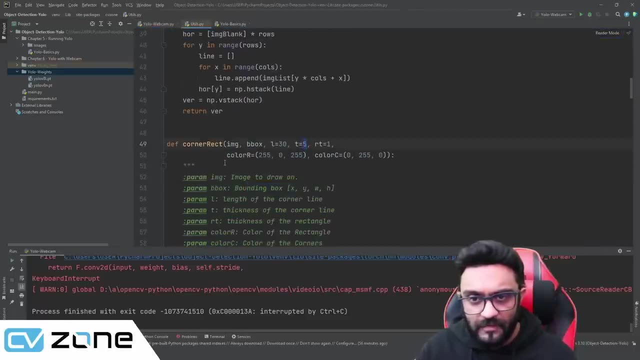 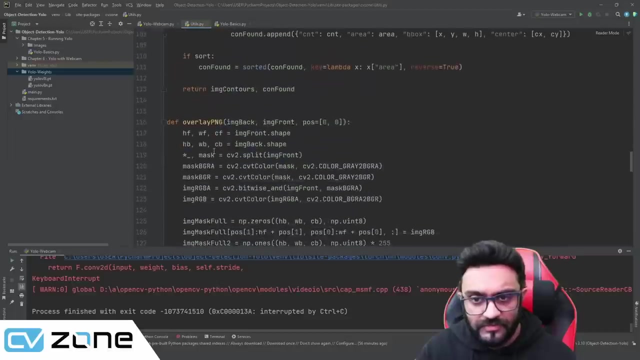 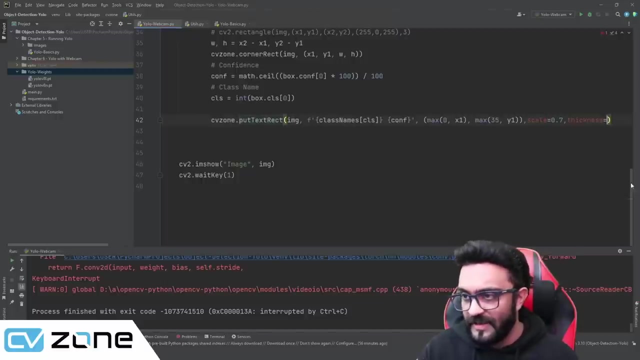 put it as 0.5. actually, the thickness is not 0.5. uh, if we check the default thickness it is: uh. no, this is not not the corner rect. where is put text right put text rect is here. the default thickness is three. so let's put it as: 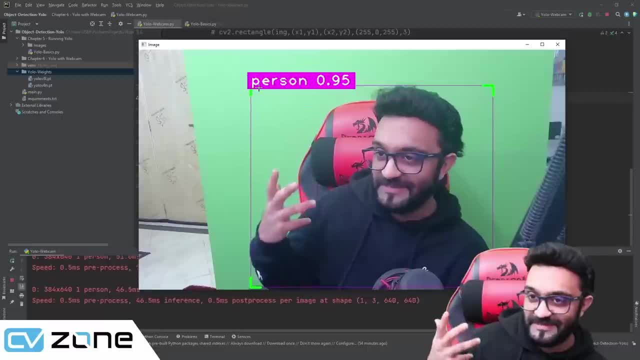 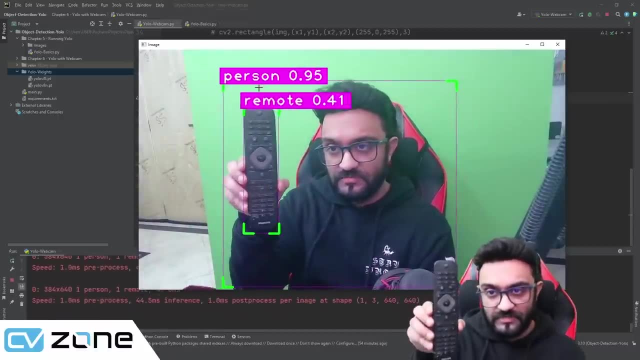 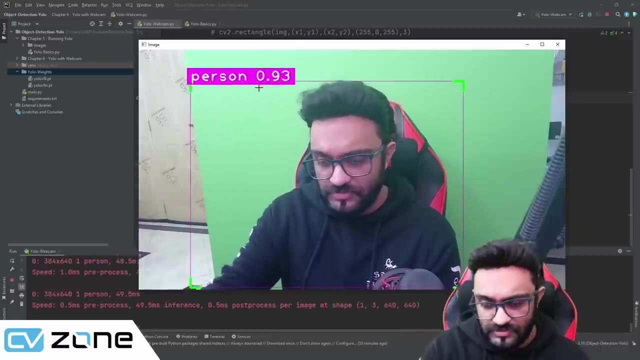 confidence if we move around. uh, that's a suitcase, i'm not sure why, uh, so sometimes it's a chair. and then we have the remote. that's very good. uh, then we have the phone, the cell phone. that's very good. so that's the basic idea, and let's 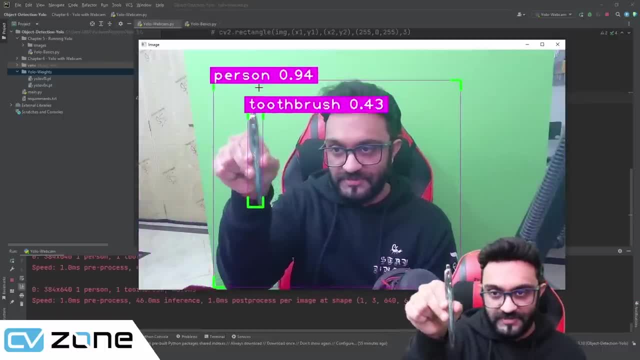 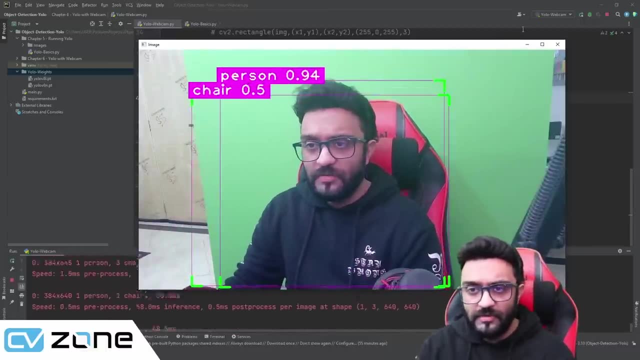 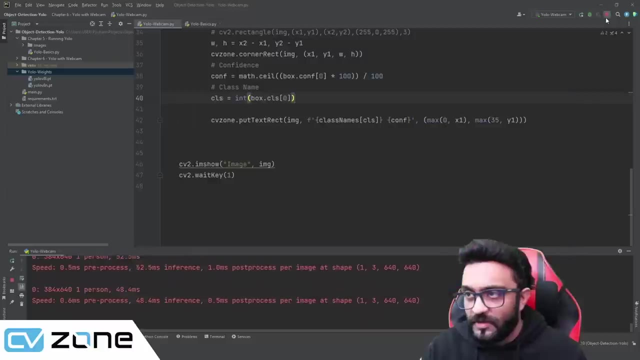 see the pen, oh, it's actually a toothbrush. i didn't know that. so it is actually detecting this as the toothbrush. that's fine, okay. so, uh, if you wanted to check it on a video, you can do that too. and if you wanted to make these uh names, these labels, a bit smaller, you can do that too. so, here, 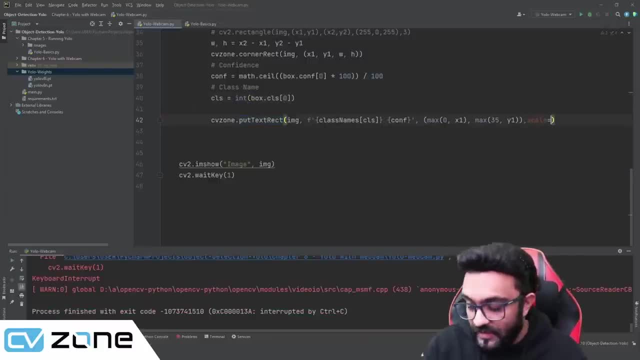 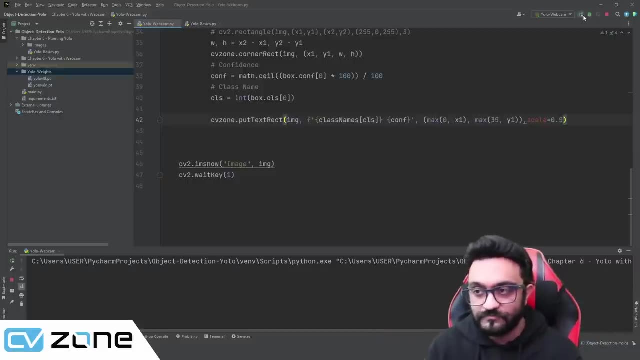 input text: rect. here you can write scale and you can give in, let's say 0.5, so that will squeeze everything down and make it smaller. uh, this will be helpful in case you have a lot of detections. for example, you have a lot of cars on a highway or you have a lot, of, a lot of people being detected. 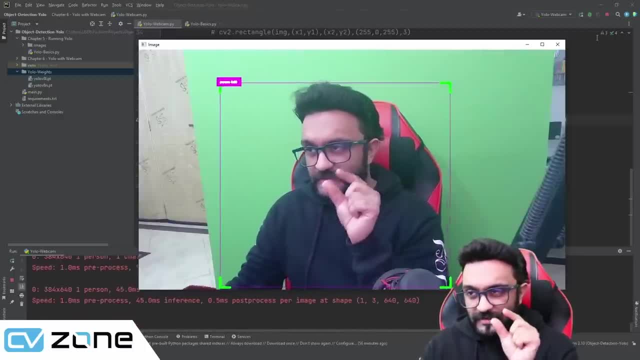 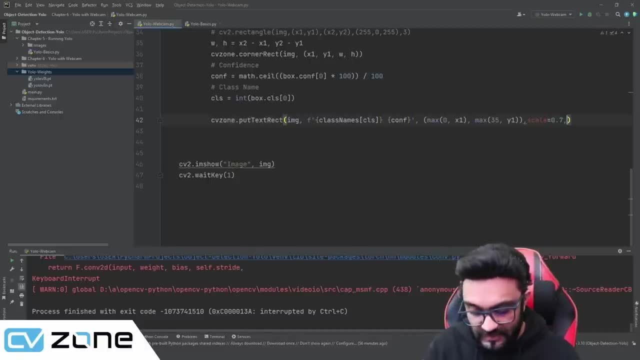 so this will make it easier. so there you go, um, but then it's, it's a little bit harder to read, uh, so you have to change. let's say, we'll put 0.7, then you also have to, uh, change the threshold. sorry, the thickness, the thickness. 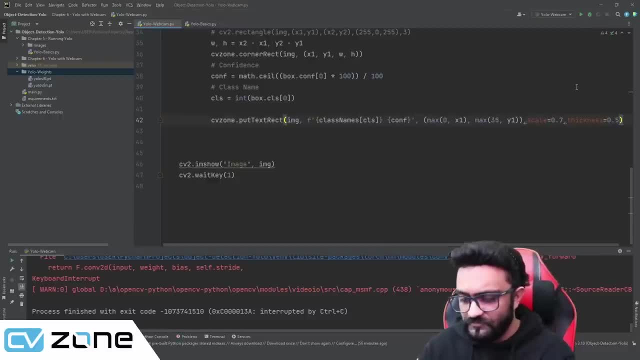 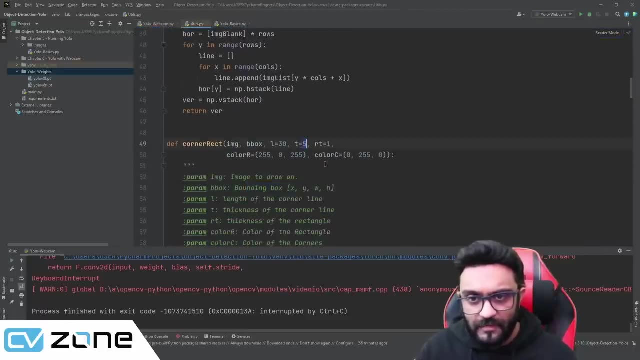 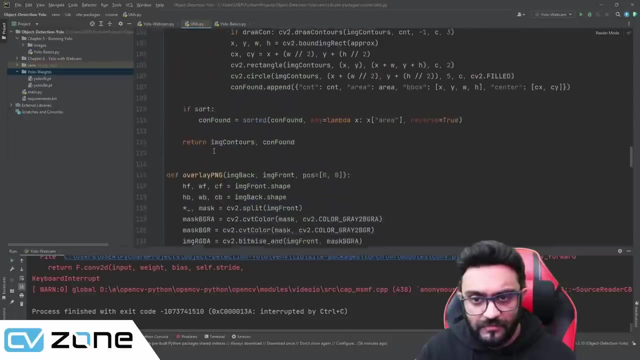 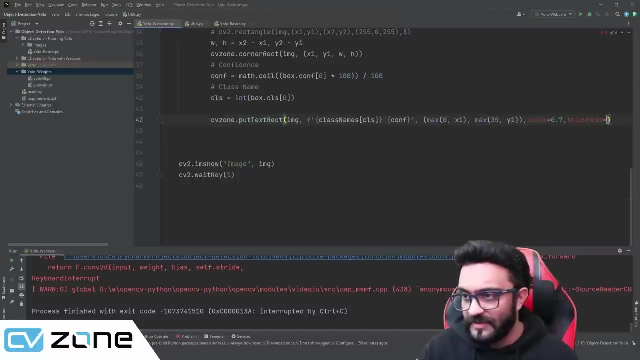 let's put it as 0.5. actually, the thickness is not 0.5. uh, if we check the default thickness, it is: uh. no, this is not the corner right. where is what text right? what text correct is here? the default thickness is three, so let's put it as one. 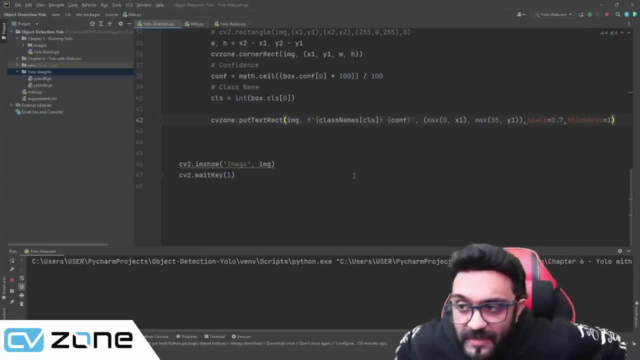 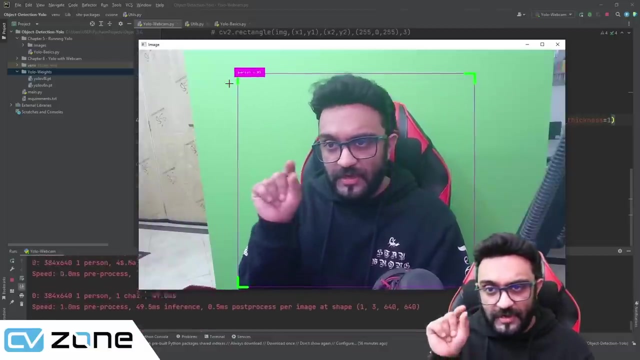 so if you put it as one, hopefully we'll be able to read it, uh, even if it's a bit smaller, because we have, uh, drastically reduced the scale from three to 0.7, so the thickness, well, I don't think we can go below one, I'm not sure. so there you go. now you can actually read person 0.9, 0.6. so if you 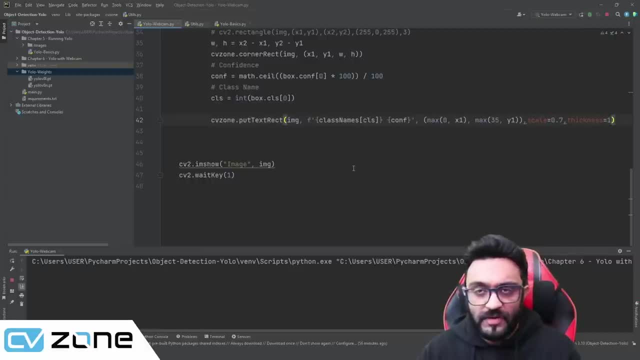 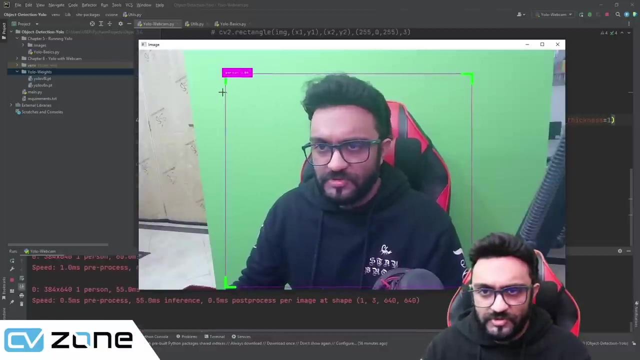 one. so if you put it as one, hopefully we'll be able to read it, even if it's a bit smaller, because we have, uh, drastically reduced the scale from three to zero point seven, so the thickness, well, i don't think we can go below one, i'm not sure. so there you go. now you can actually read person 0.9: 0.6. 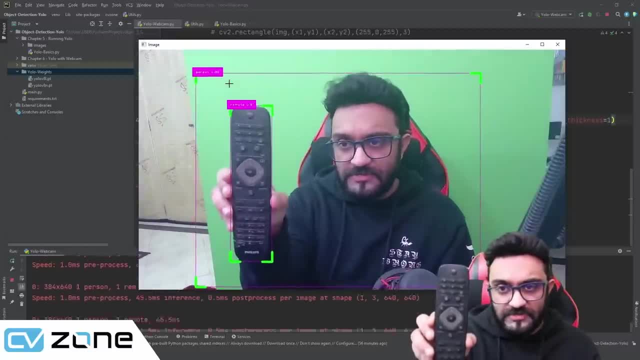 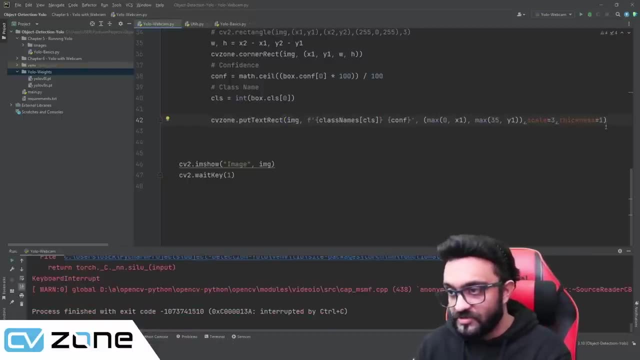 so if you bring in the remote, you can actually read it. so that's how you can, uh, increase and decrease the scale for it. by default, it's three and three, so it's up to you if you wanted to check that, okay. so, um, actually, let's keep it there because we are going to 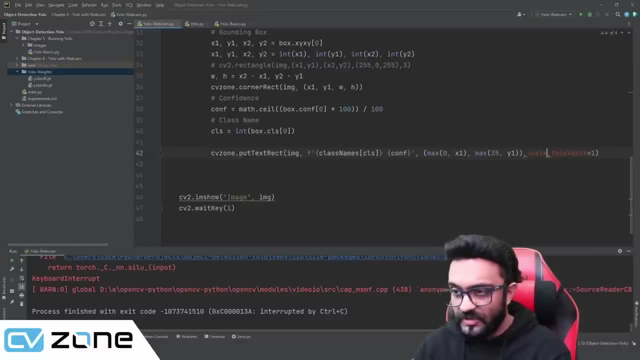 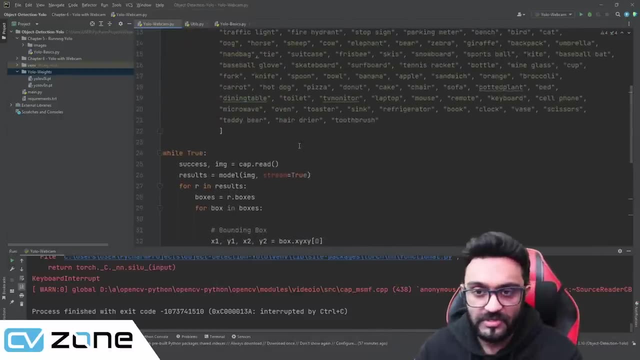 try it with the video and videos. they usually are bigger. so let's put scale as one, just a little bit bigger, and you saw that the box actually scales up and scales down automatically. so that's the best part of this function, okay. so let's try it with some videos. so what we will do is we will. 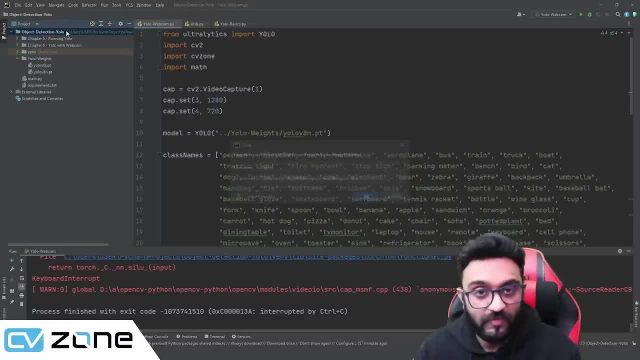 copy and we are going to paste our videos folder in object: detection yolo. so here we have some videos: bikes, cars, motorbikes, people, ppe2, pp3. so all of these options are available in object: detection yolo. so here we have some videos: bikes, cars, motorbikes, people, ppe2, pp3. so all of these. are all available on the object element and when we go into the object minus, we fallen in the option allows point and size there, and now we are going to copy this and then we are gonna choose dose we're going to have, which option we i'll give you to excuse. 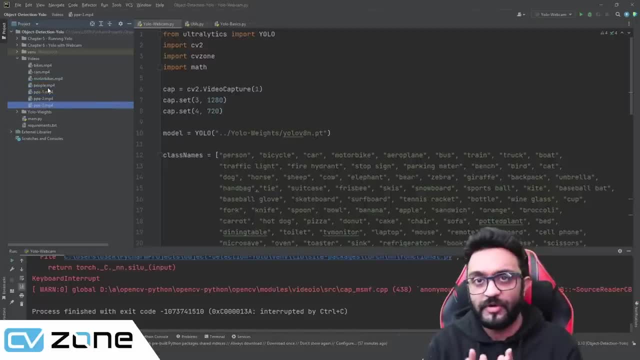 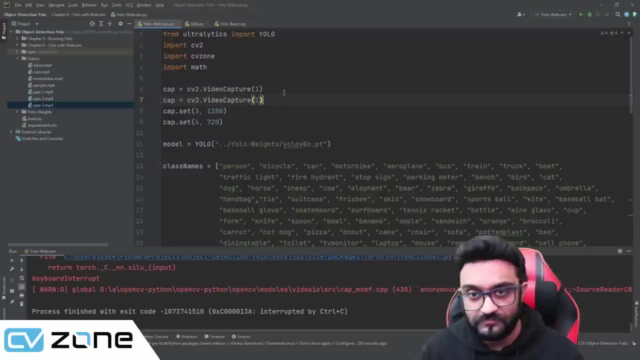 what i meant going to do is, like i Mans performance, speedchill or race or And with are. these are different videos we are going to use throughout the course, so we have all of them in one folder. so here, instead of video capture one, let me copy that and i will write here for web. 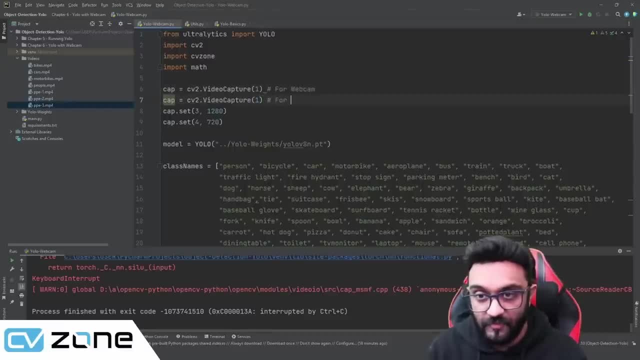 webcam and here we will write for video and we will remove. for the webcam and for the video all we have to do is we have to point it to the correct path. so here, if we go back, we will go to videos and in the videos let's try, let's try bikes. 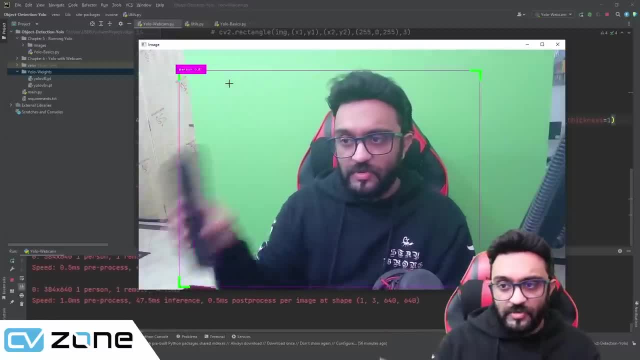 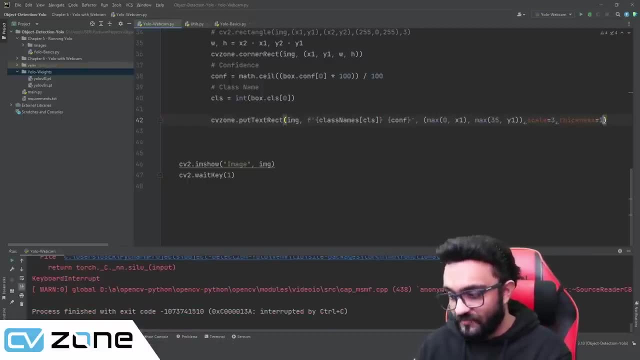 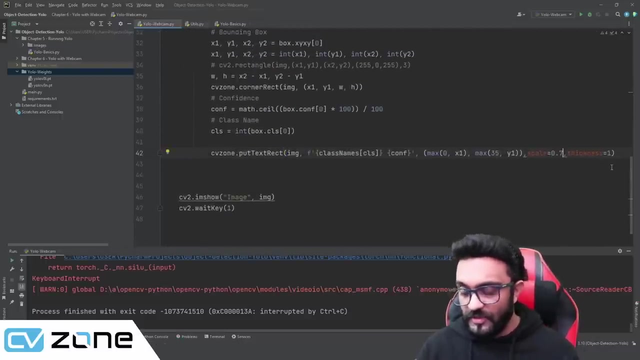 bring in the remote, you can actually read it. so that's how you can, uh, increase and decrease the scale for it. by default, it's three and three, so it's up to you if you wanted to check that, okay, so, um, actually let's keep it there because we are going to try it with the video, and videos they usually are bigger, so 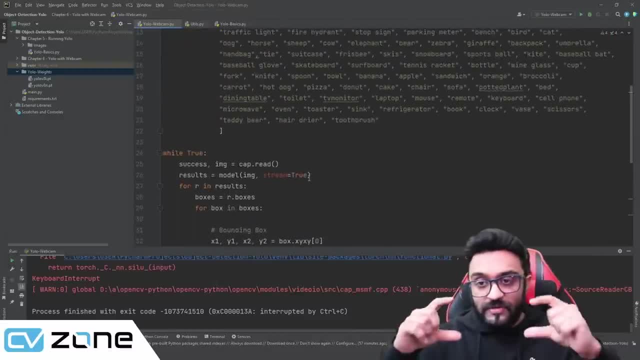 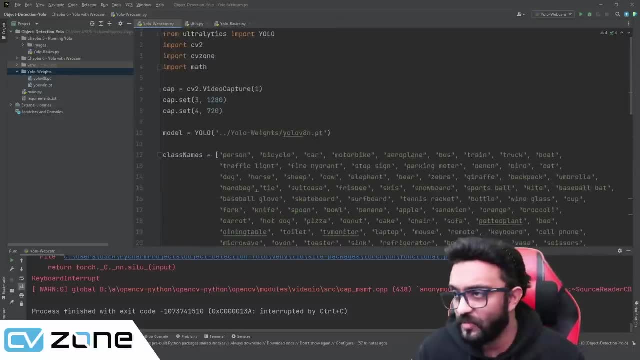 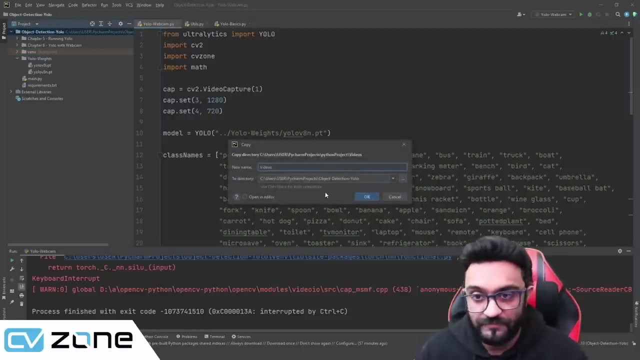 let's put scale as one just a little bit bigger, and you saw that the box actually scales up and scales down automatically. so that's the best part of this function. okay, so let's try it with some videos. so what we will do is we will copy and we are going to paste our videos folder in object. 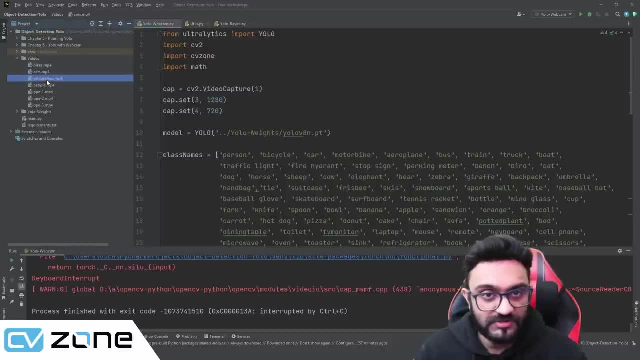 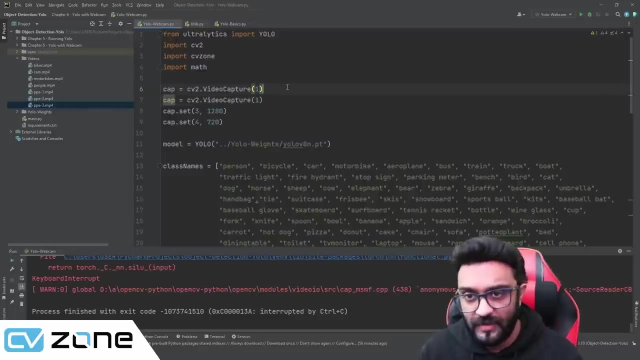 detection, Yolo. so here we have some videos: bikes, cars, motorbikes, people, ppe2, ppe3. so all our these are different videos we are going to use throughout the course, so we have all of them in one folder. so here, instead of video capture one, let me copy that and I will write here for web webcam. and here we 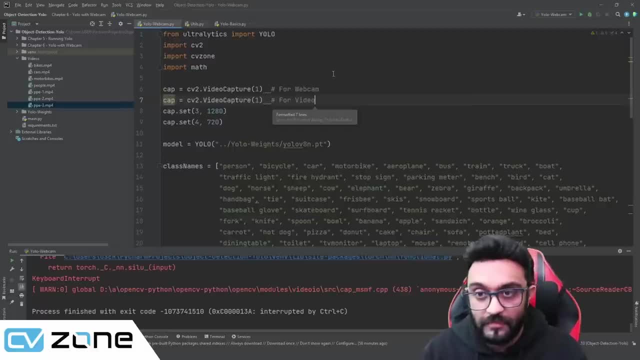 will write for video and we will remove for the webcam and for the video. all we have to do is we have to point it to the correct path. so here, if we go back, we will go to videos and in the videos, let's try, let's try bikes. 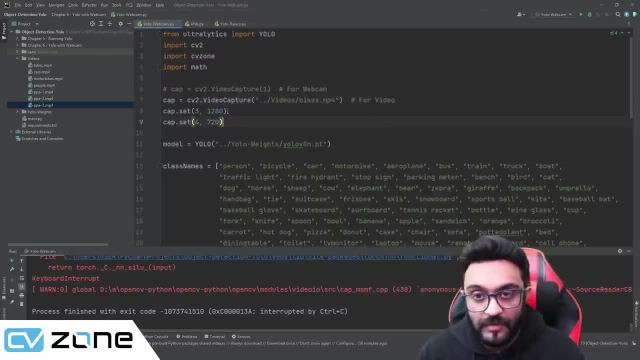 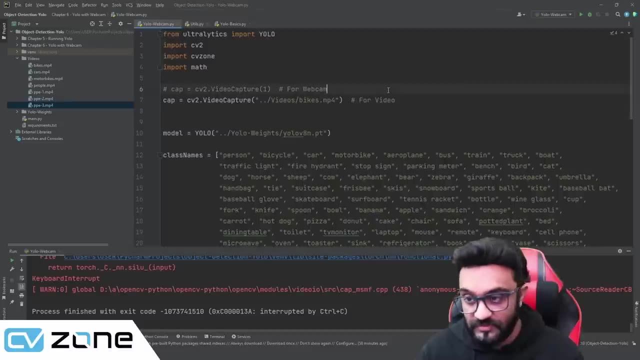 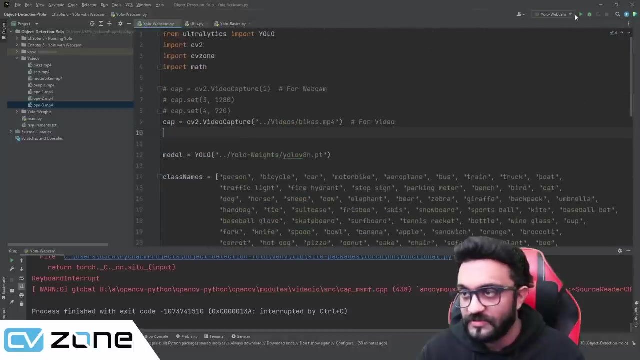 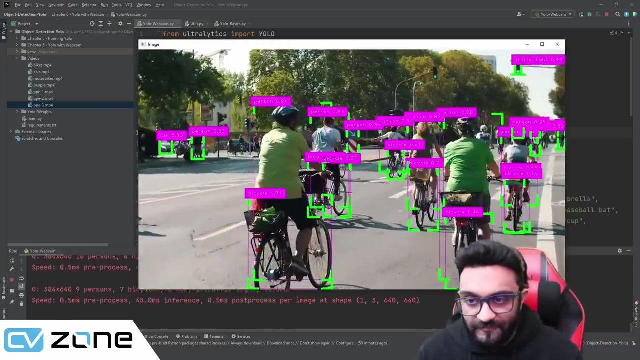 bikesmp4 and this is the size and all that. so in in case of the video, you cannot actually set the size, so let's put it here with the webcam, like that. so for the video, that is good. let's run it and see if it works. there you go. so we have a lot of people and we have bicycle. we have person. 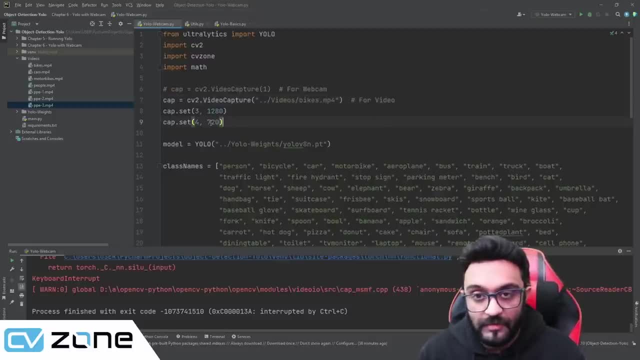 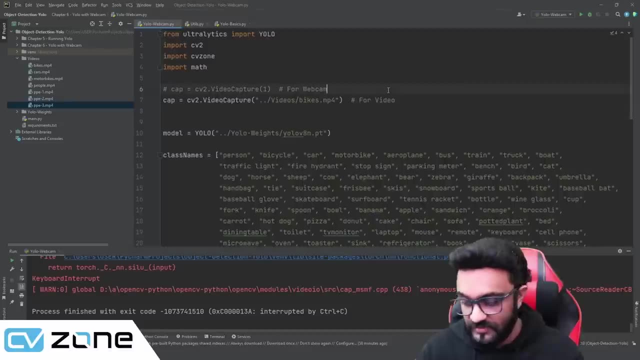 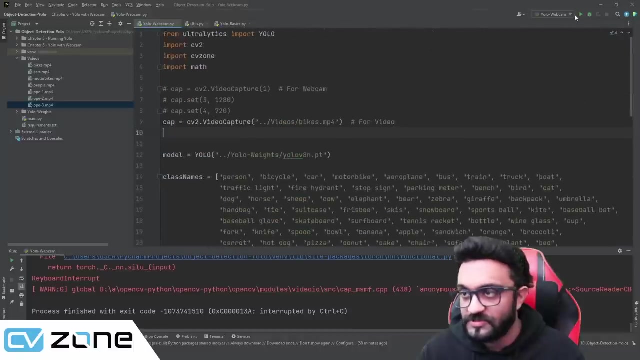 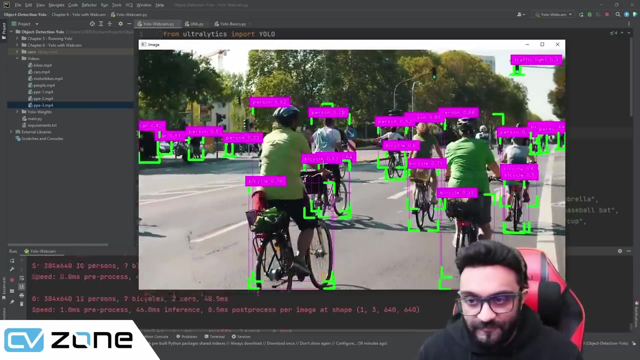 bikesmp4 and this is the size and all that. so in in case of the video, you cannot actually set the size, so let's put it here with the webcam, like that. so for the video, that is good. let's run it and see if it works. there you go. so we have a lot of people and we have bicycle, we have person, we have 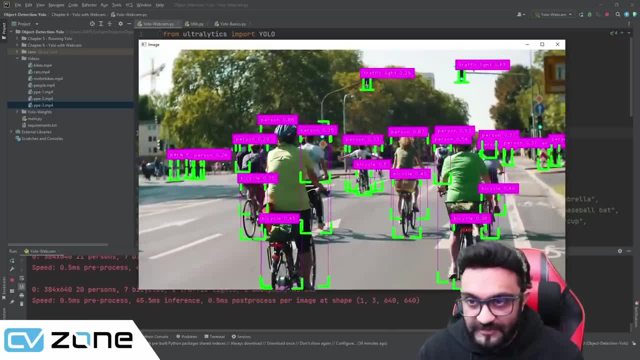 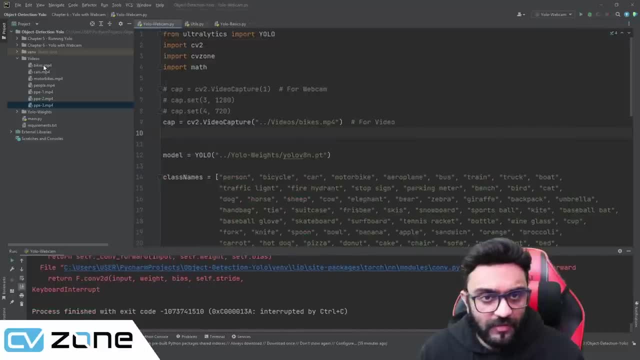 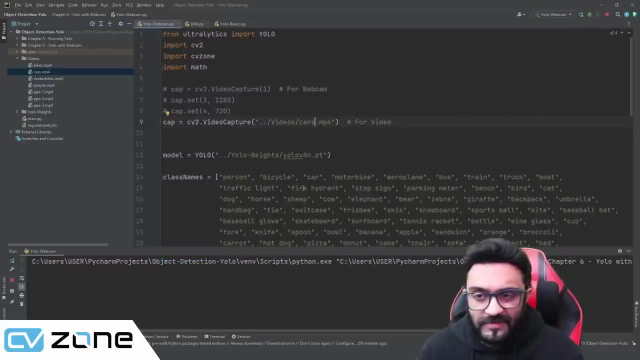 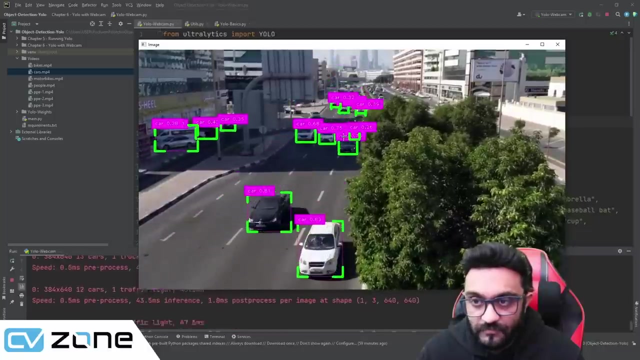 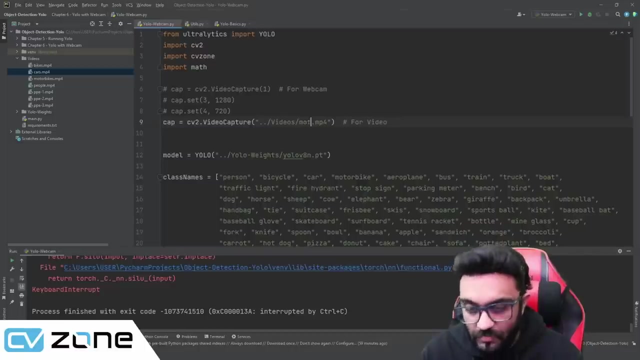 car. there's a lot of detections. we have traffic light being detected as well, so that's pretty good. and then let's try with um, cars, cars- again. you can try with different versions. so there you go, we have some cars being detected, looks pretty good. and then we can try with motorbikesmp4. 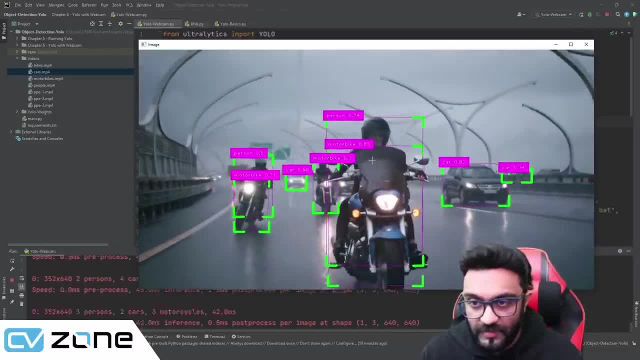 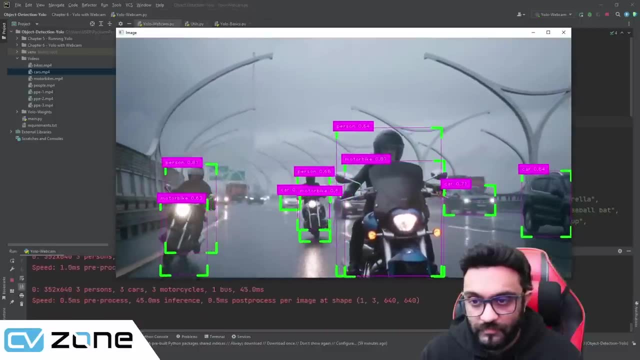 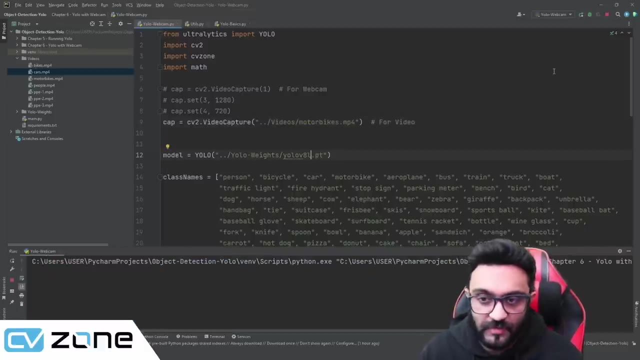 there you go. so we have some cars being detected, we have motorbike, we have person. so those are some pretty good results. let's try it with the large version- same video with the large version- and see what happens. uh, most probably it will be a lot slower. there you go. 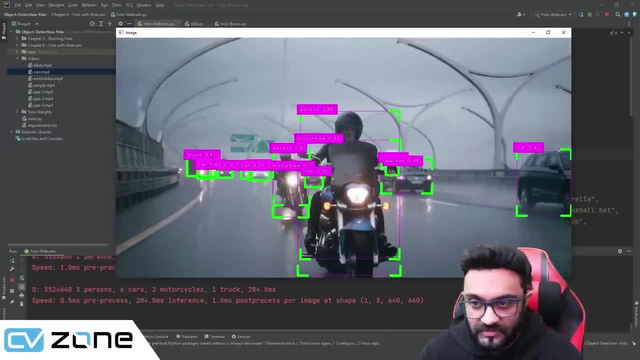 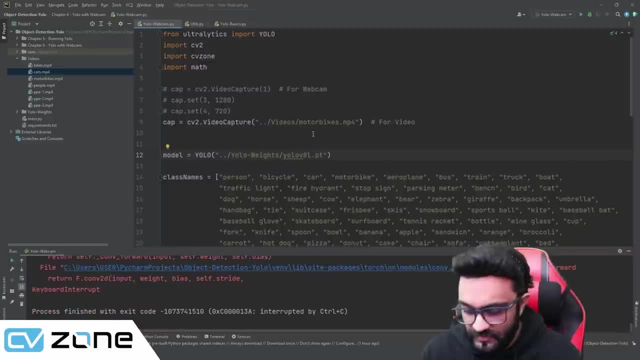 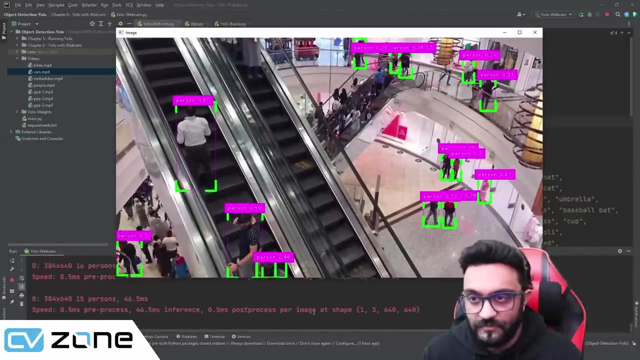 and we, but we are getting better results in terms of detections, so that's good, okay, and uh, then let's put it back to nano and the people. let's try people, p-e-o-p-l-e people, and let's run that. there you go. so we are detecting people as well, and that's pretty good. so this is the basic idea. 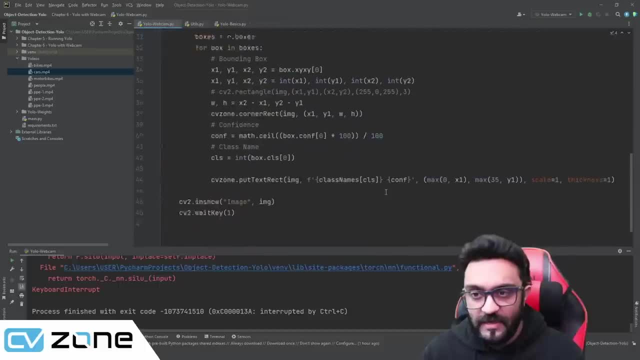 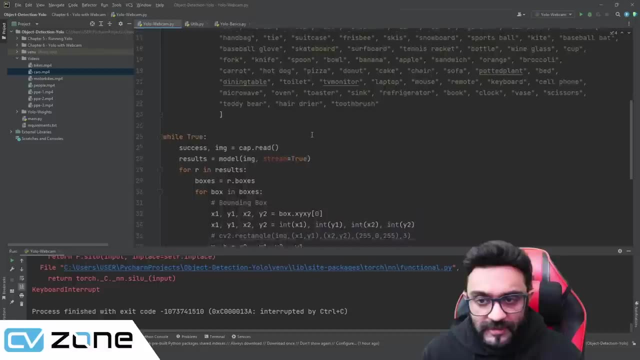 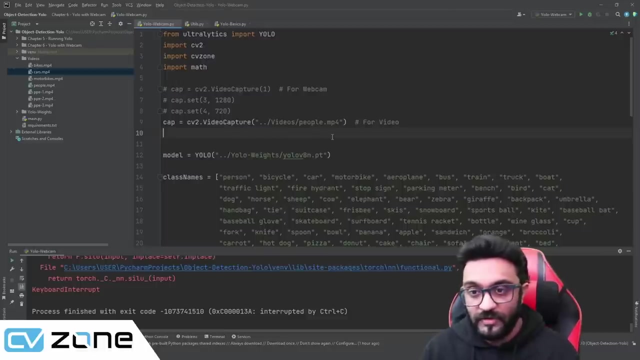 of how you can use webcam with yolo version 8 to detect these different objects, and this is quite an efficient way to do it. so later on we are going to use it. so right now we are actually using it with cpu, so that's why when we go to the large version it actually is very slow. so in the 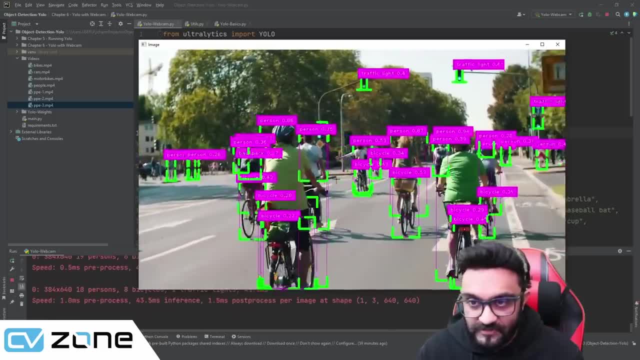 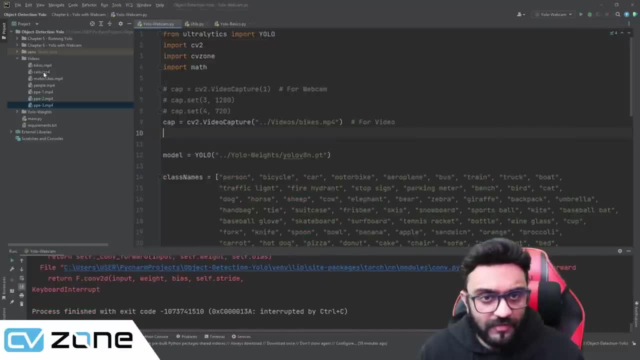 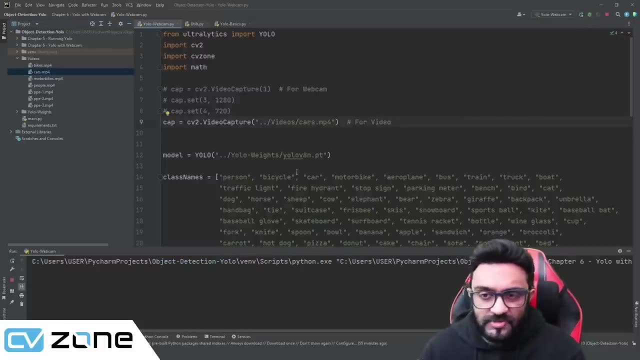 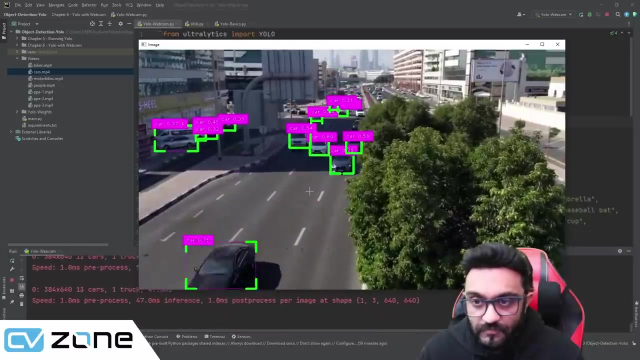 car. there's a lot of detections. we have traffic light being detected as well, so that's pretty good. and then let's try with um, cars, cars- again. you can try with different versions. so there you go. we have some cars being detected. looks pretty good. and then we can try with 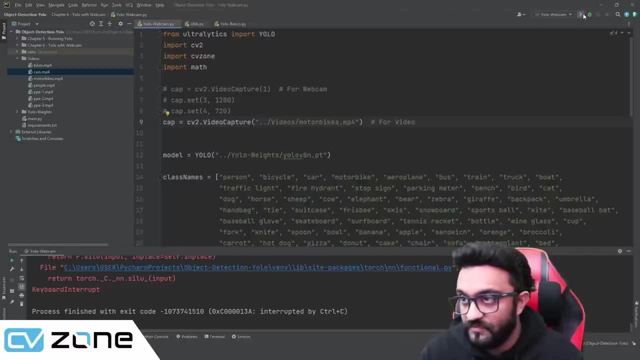 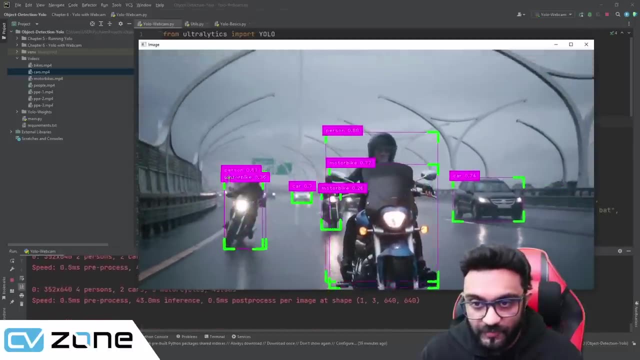 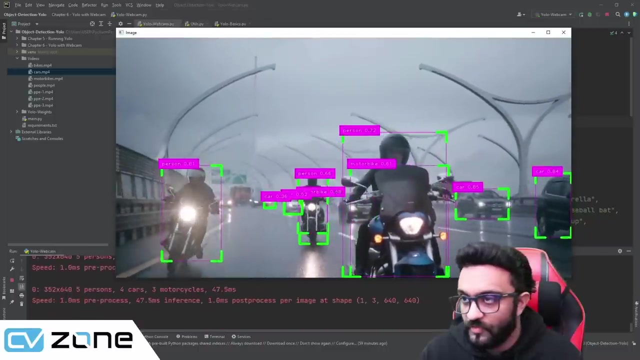 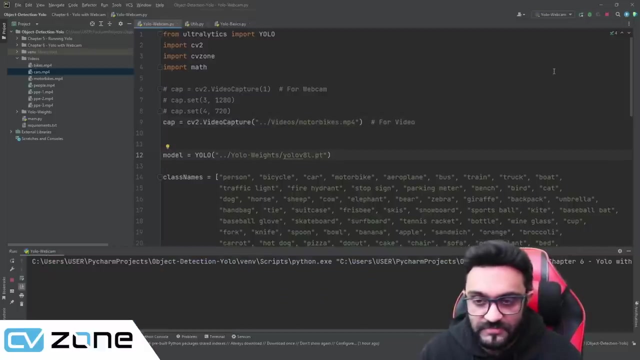 motor bikesmp4. there you go, so we have some cars being detected, we have motorbike, we have person. so those are some pretty good results. let's try it with the large version- same video with the large version- and see what happens. uh, most probably it will be a lot slower. there you go, and 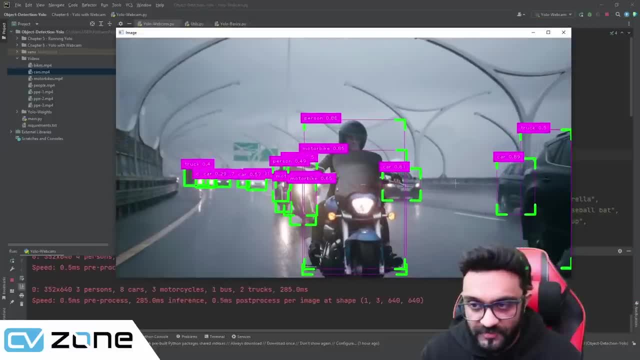 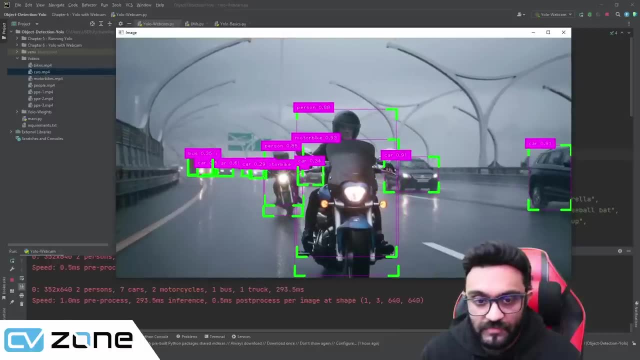 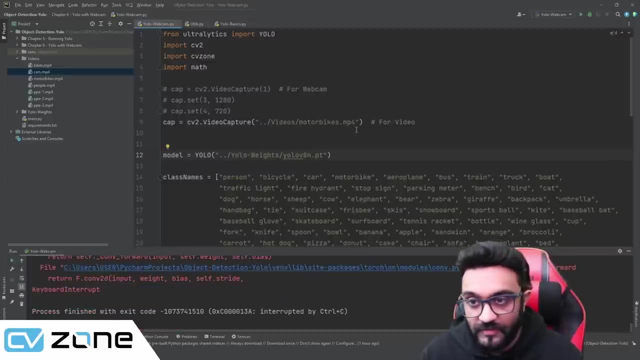 we have some cars being detected, we have motorbike, we have person. uh, most probably it will be a lot slower there you go and we. but we are getting better results in terms of detections. so that's good, okay, and uh, then let's put it back to nano and the people. 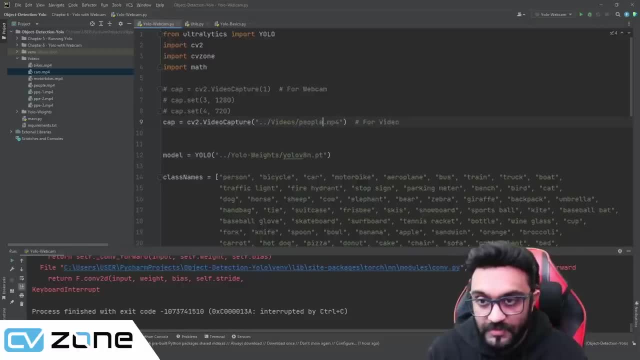 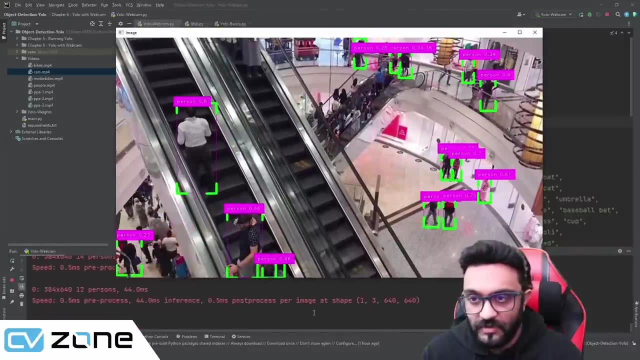 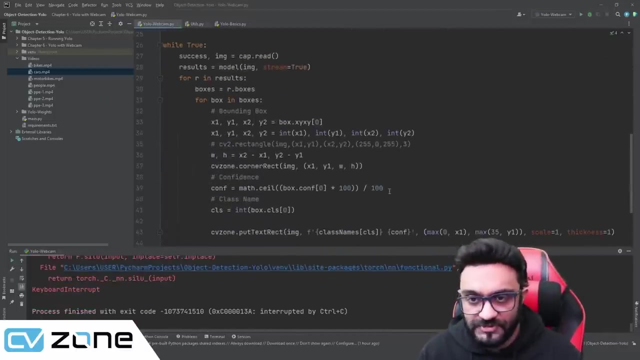 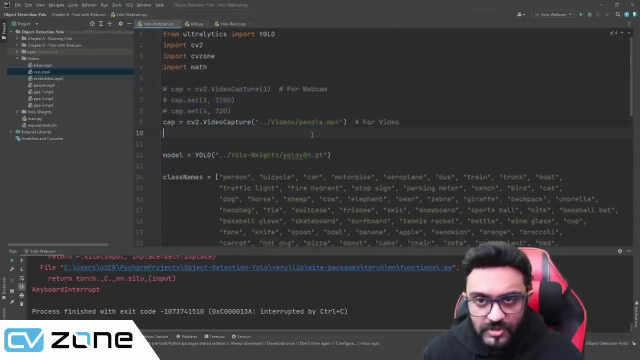 let's try people- p o p l e people- and let's run that. there you go. so we are detecting people as well, and that's pretty good. so this is the basic idea of how you can use webcam with yolo version 8 to detect these different objects, and this is quite an efficient way to do it. so later on we 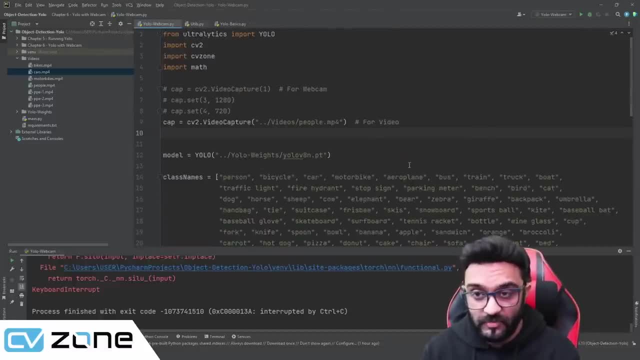 are going to use it. so right now we are actually using it with cpu, so that's why when we go to the large version, it actually is very slow. so in the next chapter we are actually going to use the same code, but we are going to run it with the gpu. 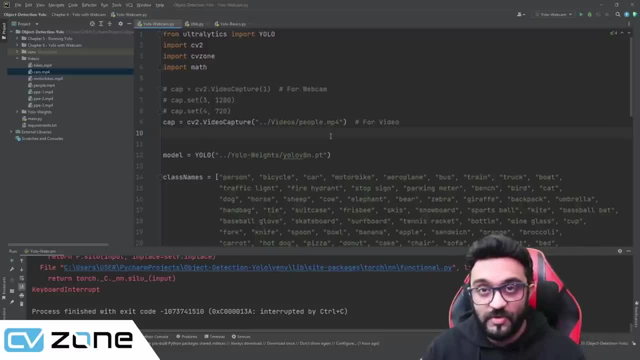 so it will be much faster than this. so let's go ahead and try that out now. in the previous chapter we saw that how we can run uh yolo version 8 with our webcam and we we took the help of opencv to actually do it. now the problem that we saw that it is using a cpu to 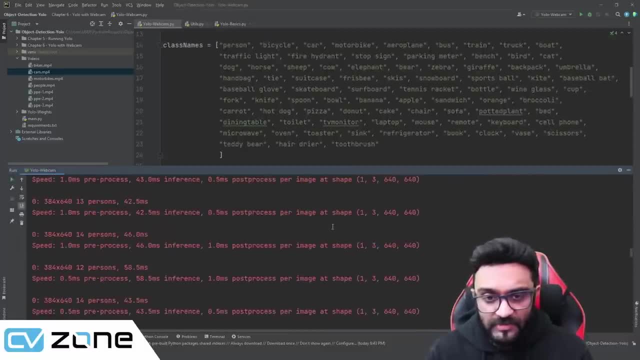 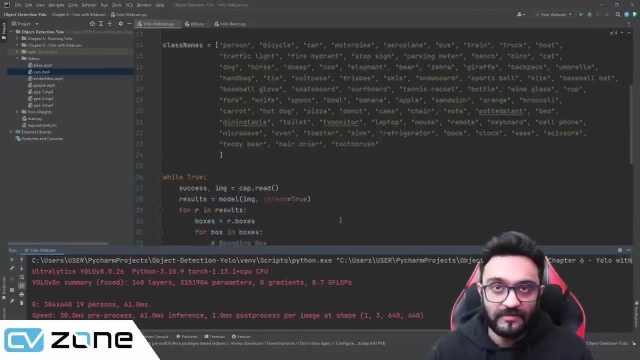 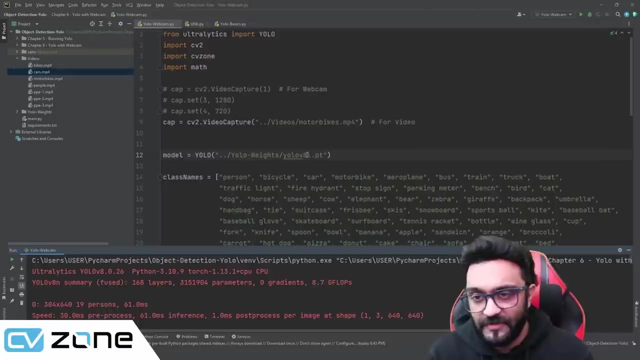 actually run all the computation and while i do have a very good cpu, which is core i9 and it is 12th generation, it is still unable to handle real-time information. when it comes to the large version, when we are using nano version, it's fine, but when it comes to large or medium version, 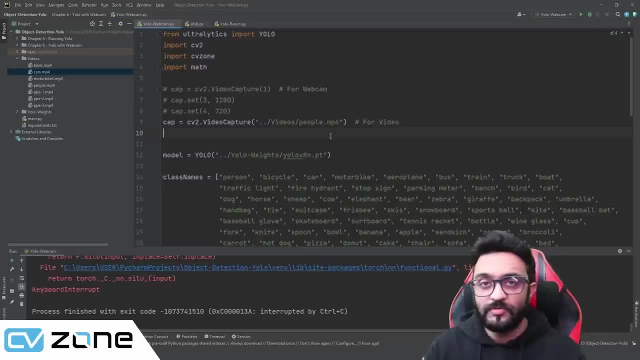 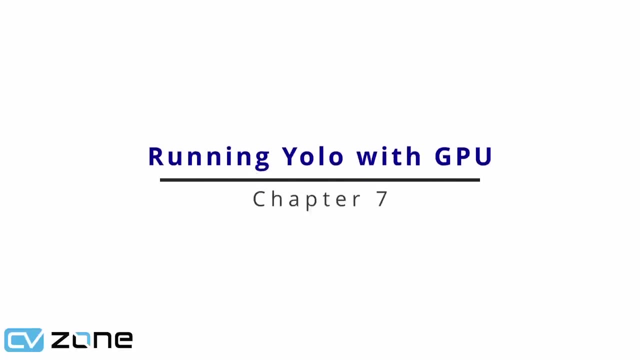 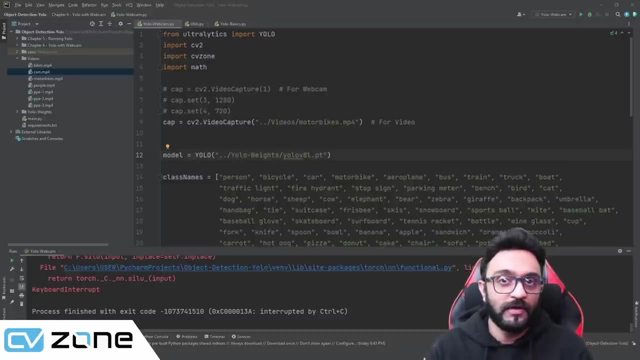 next chapter we are actually going to use the same code, but we are going to run it with the gpu, so it will be much faster than this. so let's go ahead and try that out now. in the previous chapter we saw that- how we can run yolo version 8 with our webcam, and we we took the help of opencv. 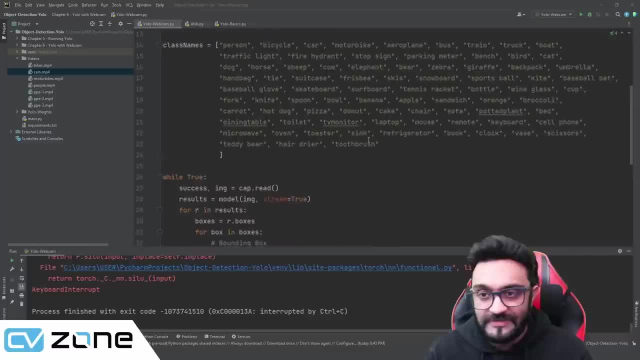 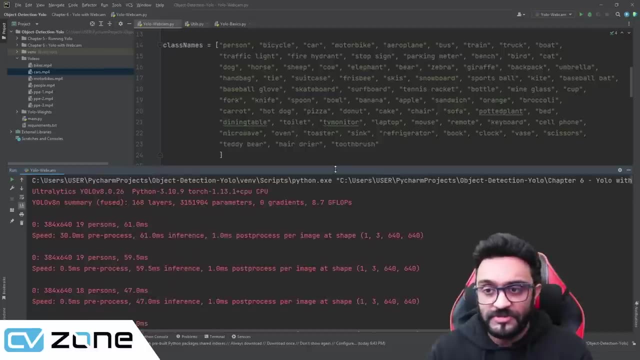 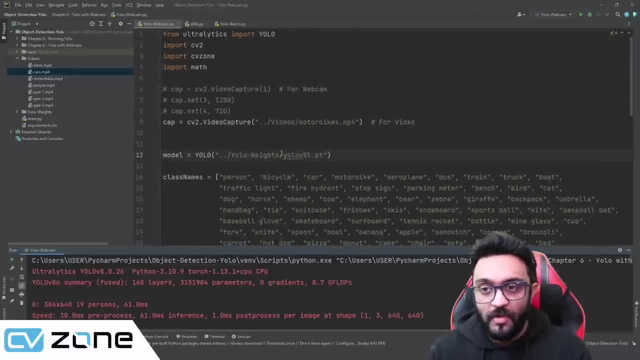 to actually do it. now, the problem that we saw that it is using a cpu to actually run all the computation and while i do have a very good cpu, which is core i9 and it is 12th generation, it is still unable to handle real-time information when it comes to the large version, when we are using nano version. 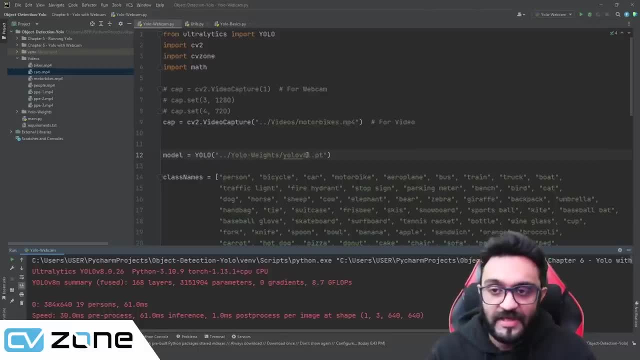 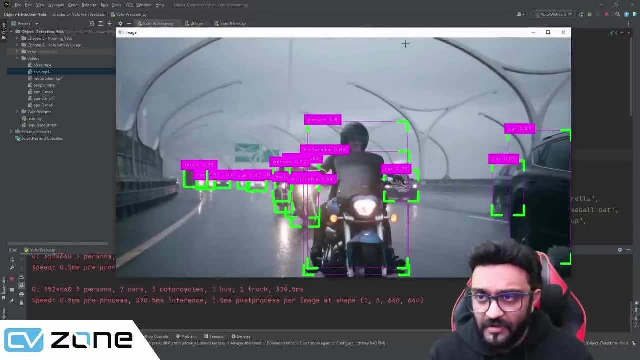 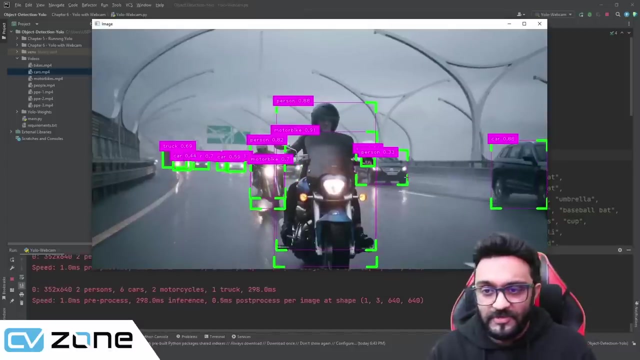 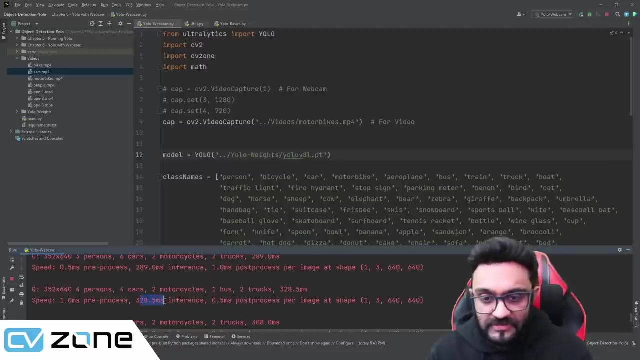 it's fine, but when it comes to large or medium version then it lags very much. so, as you can see here, if we run it right now, we are detecting a video, and then we are. we are running a video with version 8, large model, and you can see the lag is very much, so it takes almost 300 milliseconds. 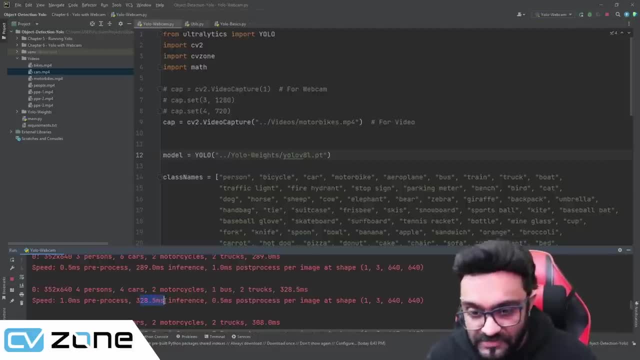 to run an inference. so only three frames per second. you can say: so that's not very good. so what exactly can we do? we can use our gpu to actually run it and hopefully the gpu will give us real-time results. so how exactly can we run a gpu? so first of all, you need to have 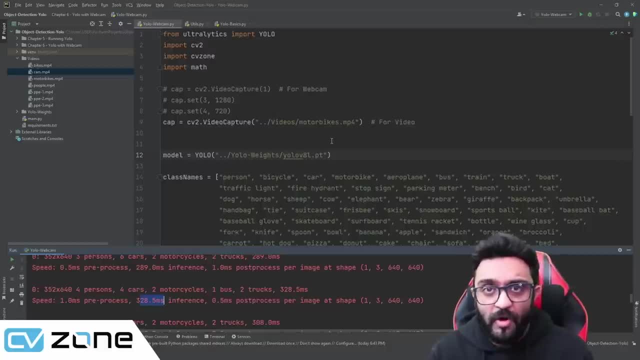 a gpu. you can check the gpu level on their website- the compute capability- and based on that, it will perform very good or very bad, based on how powerful it is. now, when it comes to installations, there's a lot of installations required to run the gpu, but it is all well worth it, because when once you, 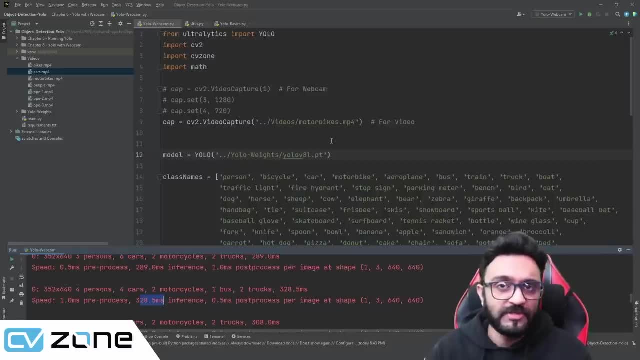 actually get it running. you will be able to run your gpu and you will be able to run your yolo version 8 in real time, and that is something that is very good to know. so i've listed down everything in detail, so let's go ahead and follow those steps. 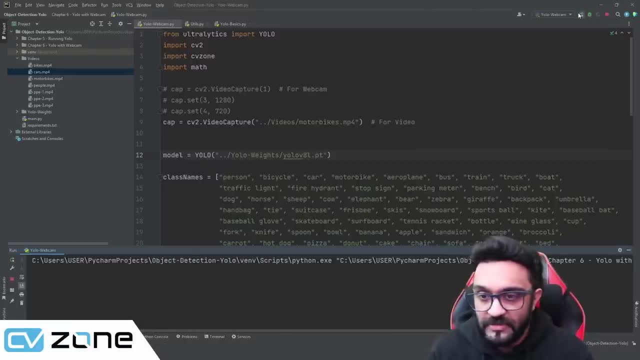 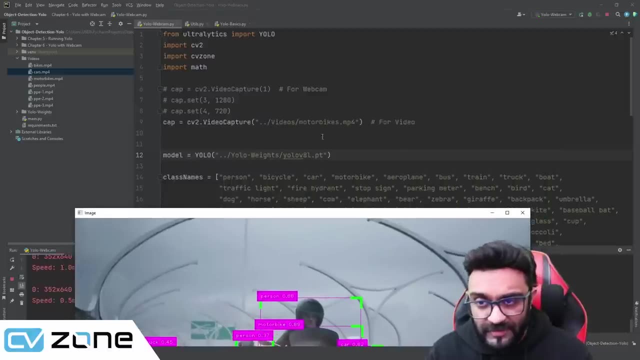 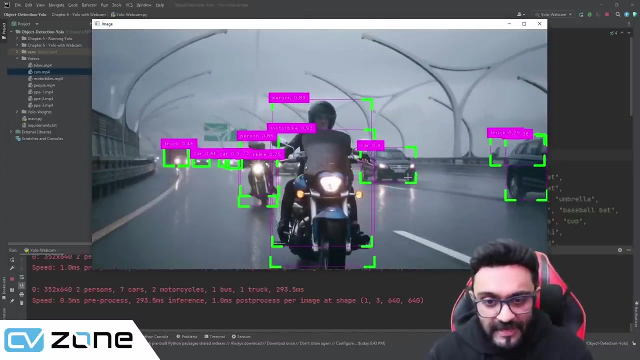 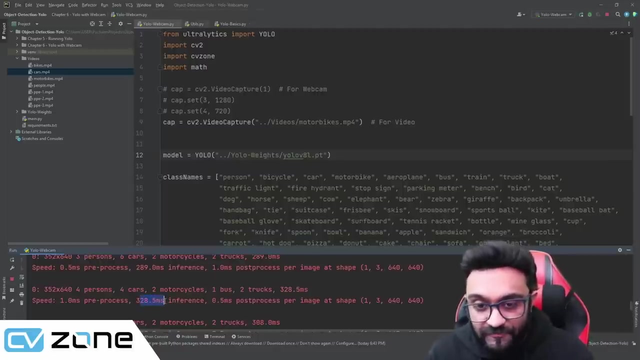 then it lags very much. so, as you can see here, if we run it right now we are detecting a uh video and then we are. we are running a video with yolo version 8 large model and you can see the lag is very much. so it takes almost 300 milliseconds to run an inference, so only three frames per second you. 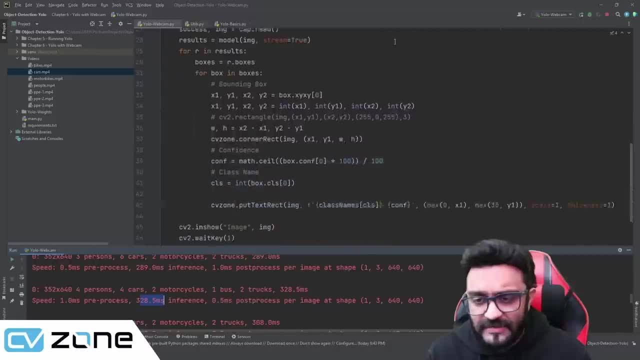 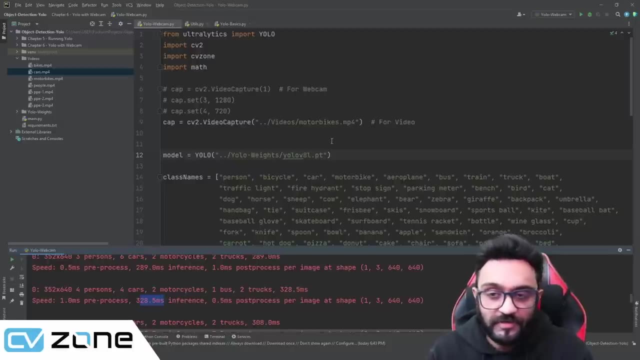 can say: so that's not very good. so what exactly can we do? we can use our gpu to actually run it and hopefully the gpu will give us real-time results. so how exactly can we run a gpu? so first of all, you need to have nvidia's gpu. you can check the gpu level on their website, the. 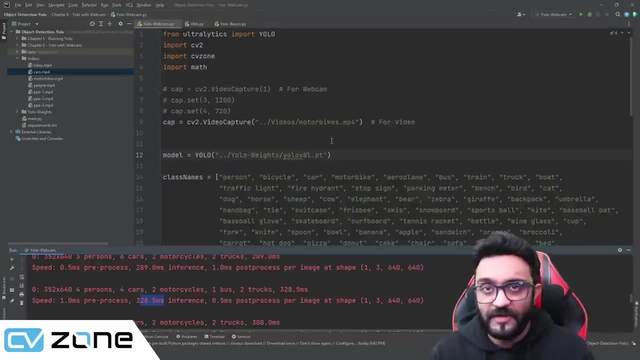 compute capability and, based on that, it will perform very good or very bad, based on how powerful it is. now, when it comes to installations, there's a lot of installations required to run the gpu, but it is all well worth it, because once, once you actually get it running, you will be able to. 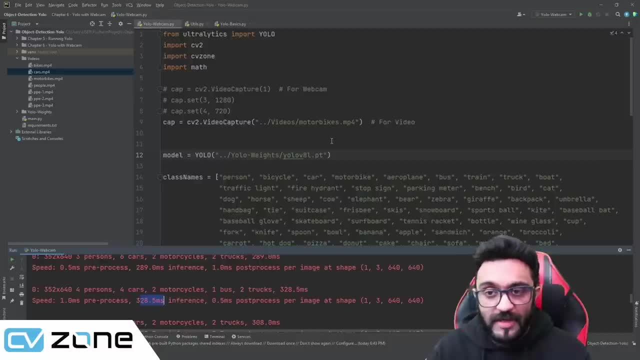 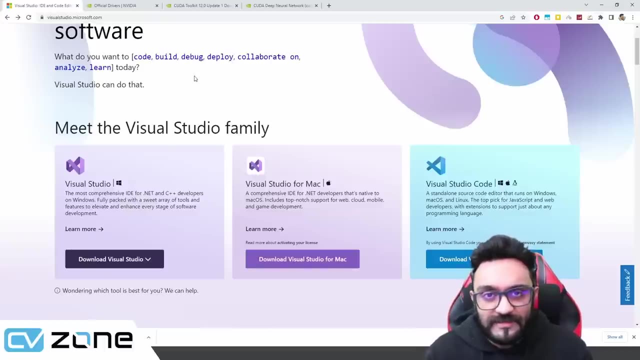 run your gpu and you will be able to run your yolo version 8 in real time, and that is something that is very good to know. so i've listed down everything in detail, so let's go ahead and follow those steps. first thing you will need is visual studio, so you have to install visual studio. this is the 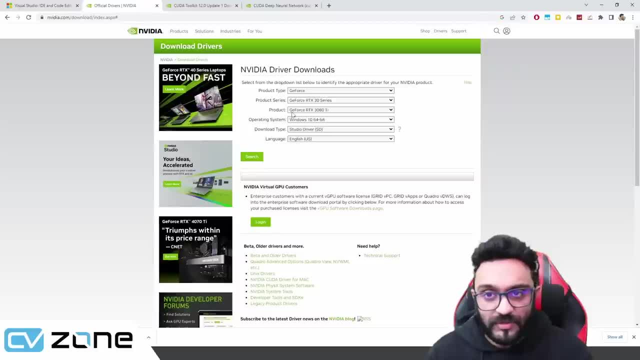 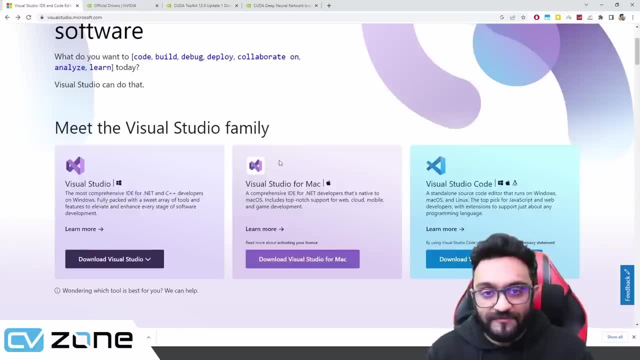 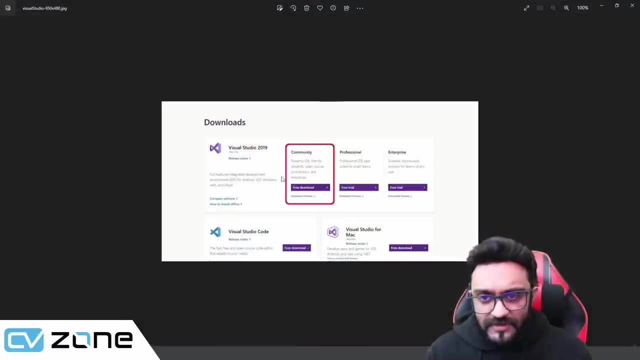 requirement for the cuda toolkit. so this is the cuda toolkit, so this is the requirement of this kit. so you have to install this first. so visual studio. but what exactly do we need in visual studio? once you run it, you have to download the community version. so whichever one is the latest one you can. 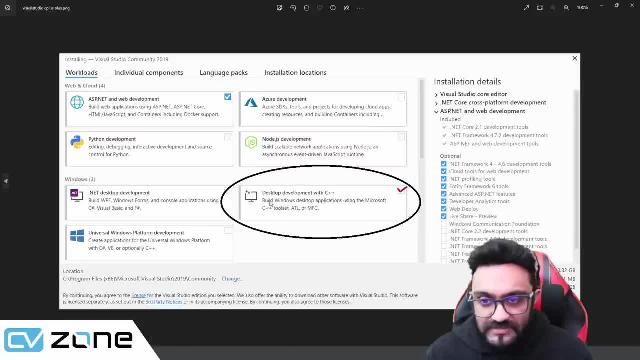 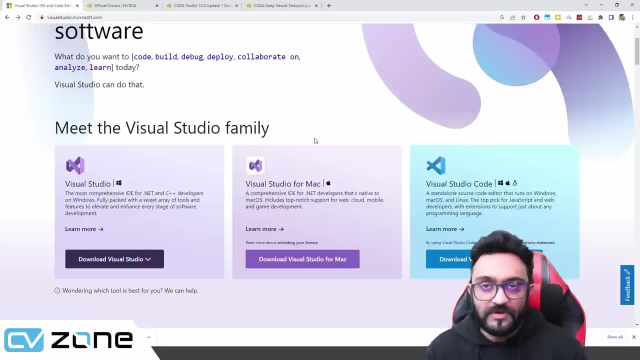 download that, but then the the biggest thing that we need is the development with c plus plus, so you will need that to install that as well. so make sure you run uh, install it. so once we have that, then you have to go ahead and this will take a while because it's uh quite a few gbs, so it will take a while to download and 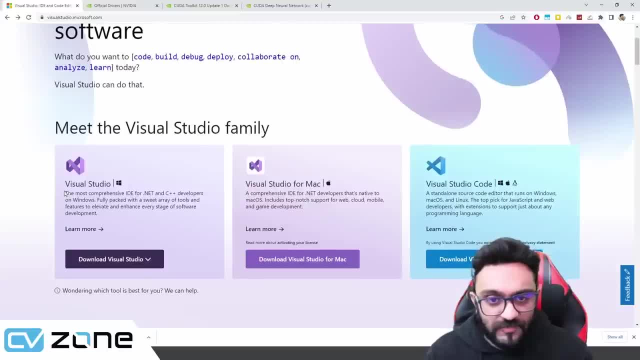 the first thing you will need is visual studio, so you have to install visual studio. this is the requirement for the cuda toolkit. so this is the cuda toolkit, so this is the requirement of this kit. so you have to install this first. so visual studio. but what exactly do we need in? 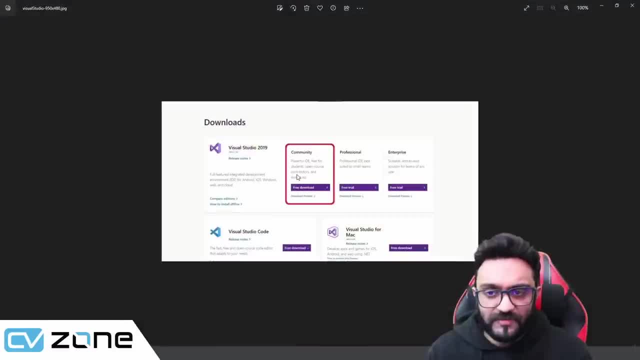 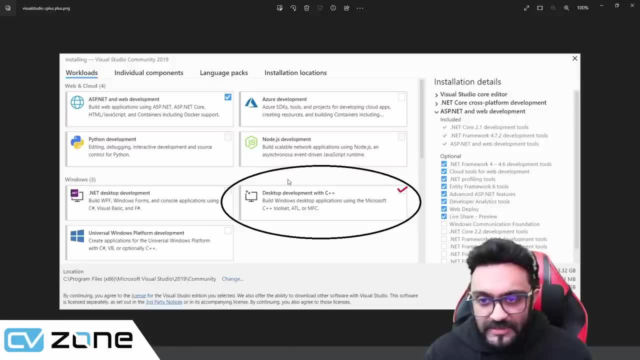 visual studio. once you run it, you have to download the community version. so whichever one is the latest one, you can download that. but then the the biggest thing that we need is the development with c plus plus. so you will need that to install that as well. so make sure you run, install it. so once we have that, then you have to go ahead, and this will take. 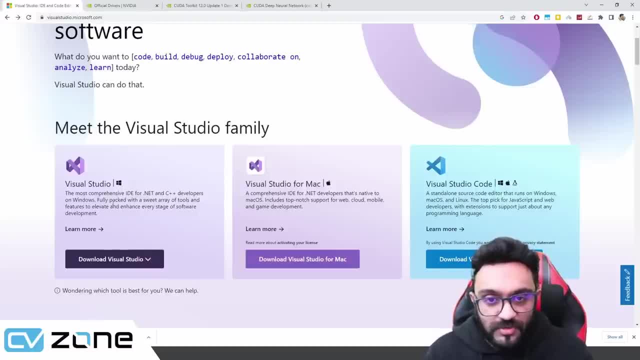 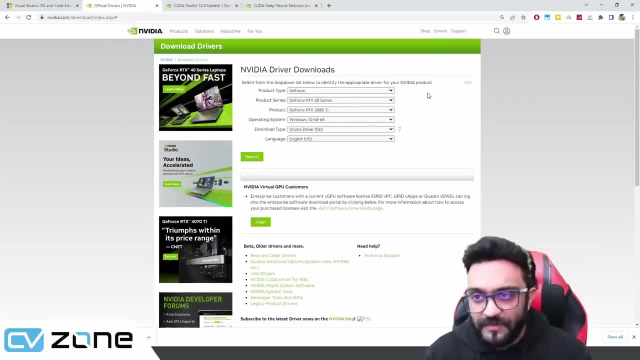 a while because it's quite a few gbs so it will take a while to download and install. once that is done, you will go to the official nvidia's drivers. so, for example, i have a have the nvidia's um rtx 3080 ti, so i will select the geforce in geforce. i will select the. 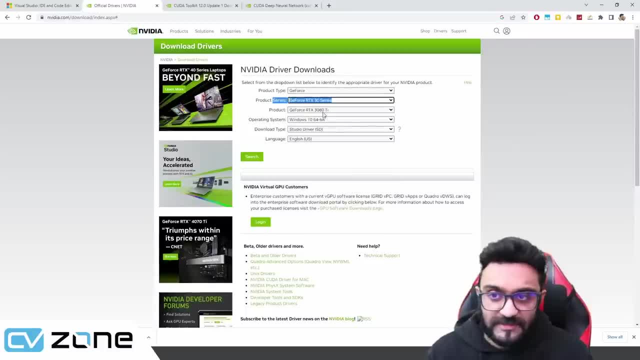 30 series and then geforce rtx 3080 ti, and i'm using windows 10, so i will select that. you will select the studio driver and english, and you will search and you are going to download it. now. this is a simple wizard. you have to click next, next, next, and it should install quite easily once that. 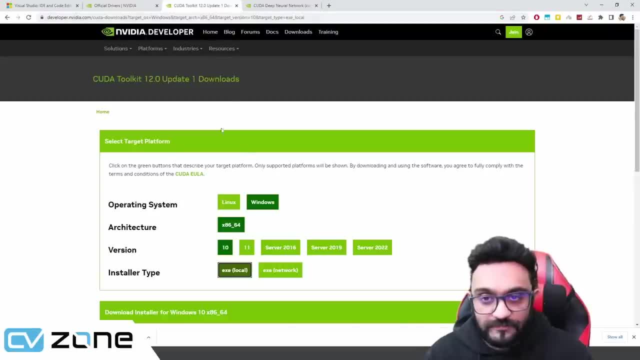 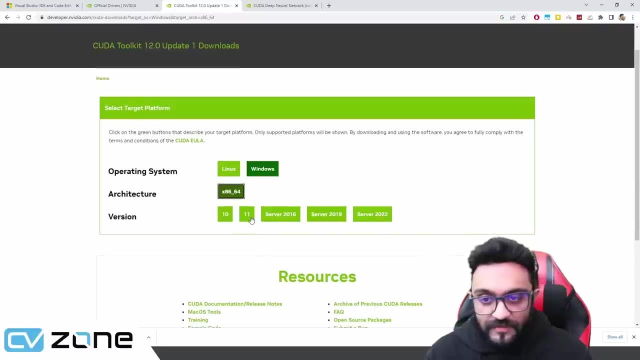 is done, you will go ahead and install cuda toolkit. so to the to, not to, the cuda toolkit you can install by going to their website. so this is for the nvidia developer. you will click on windows, then x86, 64, then you will click on 11 and then you will download the local version. 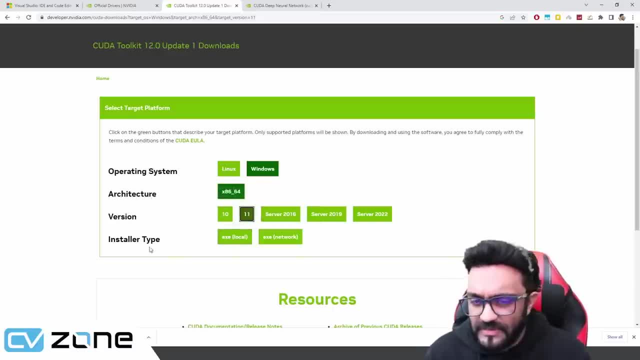 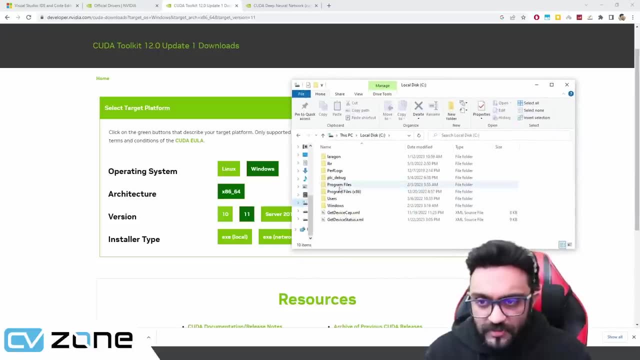 so i have, i believe, cuda 11.6. let me check. so once you download it will install, and i will check my version as well. so it will install in program files and if you go down nvidia gpu computing toolkit and if you go to cuda, this is 11.5. so i have 11.5, based on the version. 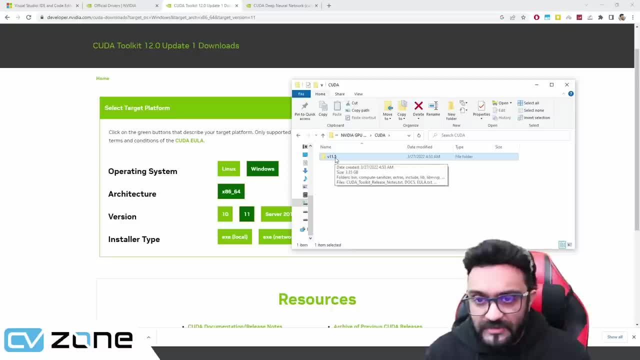 the latest version you can download as well. so here it's 11.5. we will open that up and you can see again. this will be an installer. it will be a wizard you have to click next, next. next, install it in c and in c. this is where you will find the software that you want to install and you will 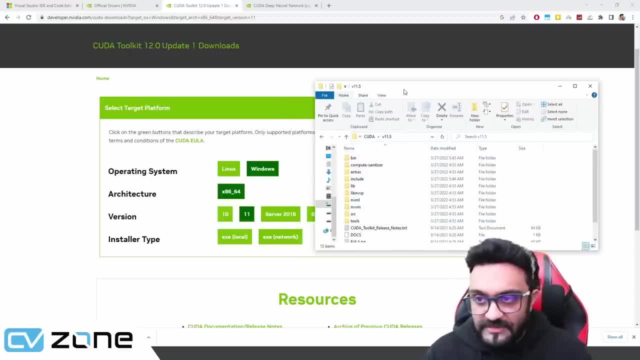 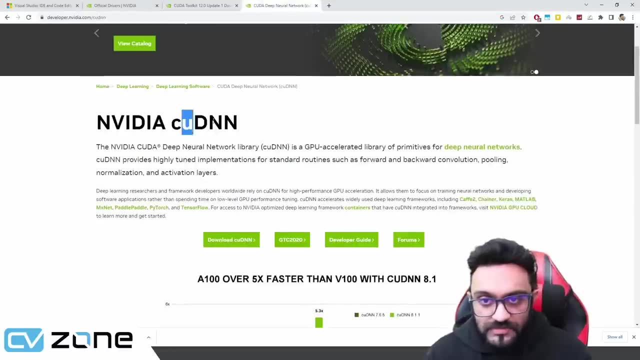 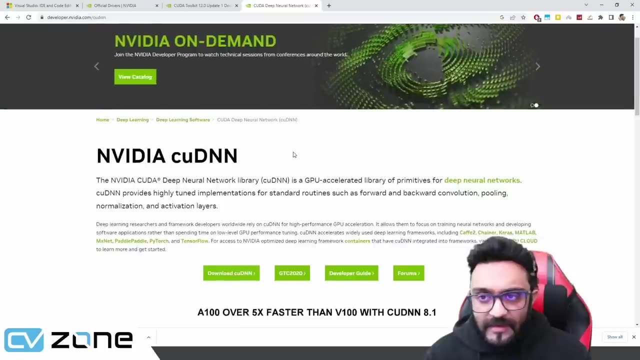 find all the files. so keep this folder open, because next we are going to install cuda dnn, which is which stands for deep neural networks, cuda, deep neural networks. so again you have to click on download, uh, the cuda dnn, and this will need, uh what you call the registration. 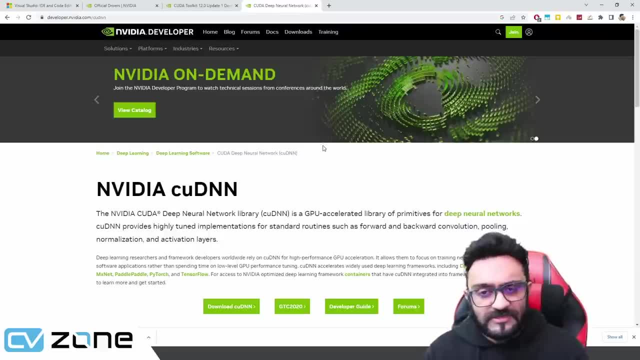 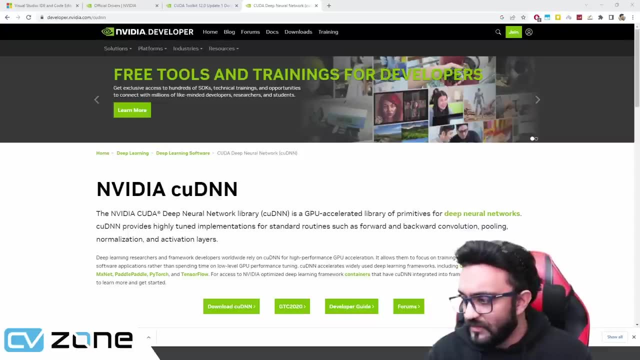 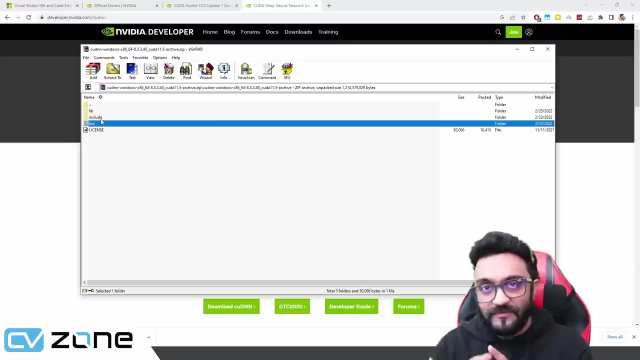 on their website. so make sure you have registered and it is free to download. so just make sure that you have registered and it will let you download. uh, the cuda dnn. so once you download that, this is what you will get. so make sure the versions are. 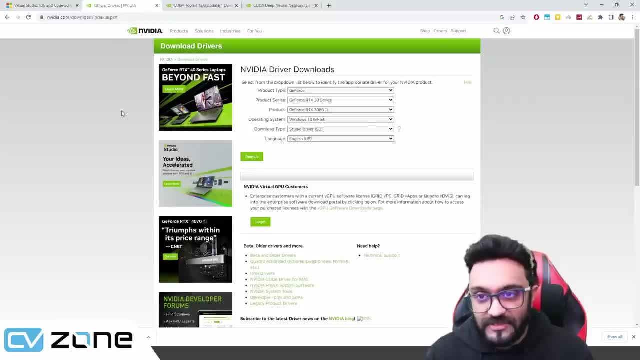 install. once that is done, you will go to the official nvidia's drivers. so, for example, i have the nvidia's um rtx 3080 ti, so i will select the geforce. in geforce, i will select the 30 series and then geforce rtx 3080 ti. 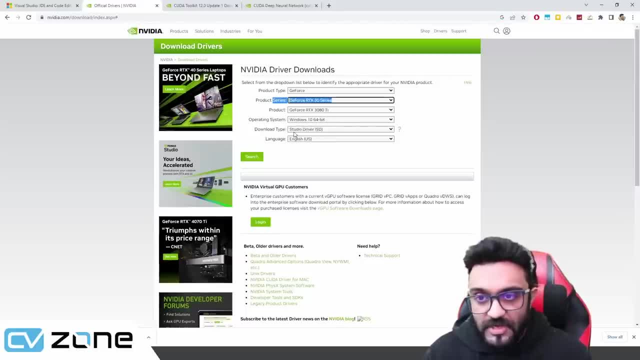 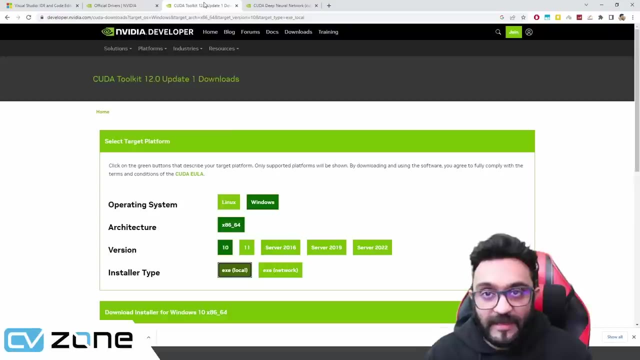 and i'm using windows 10, so i will select that. you will select the studio driver and english and you will search and you are going to download it now. this is a simple wizard. you have to click next, next, next, and it should install quite easily. once that is installed, you will go ahead and install. 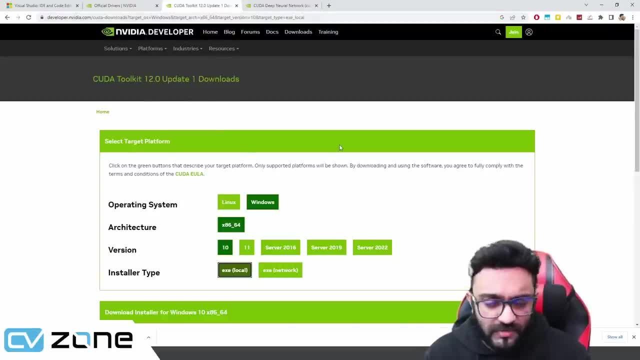 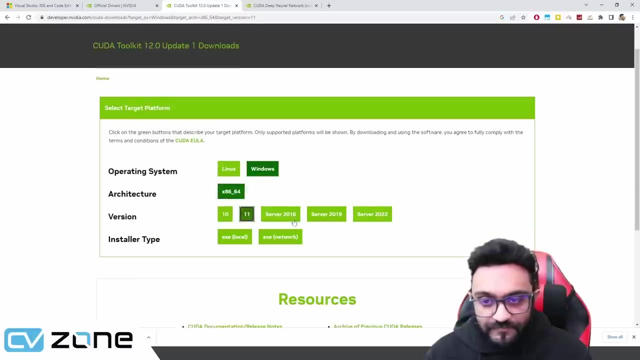 cuda toolkit. so tuda do not tuda. cuda toolkit you can install by going to their website. so this is for the nvidia developer. you will click on windows, then x8664, then you will click on 11 and then you will download the local version. so i have, i believe, cuda 11.6. let me check so once you download it. 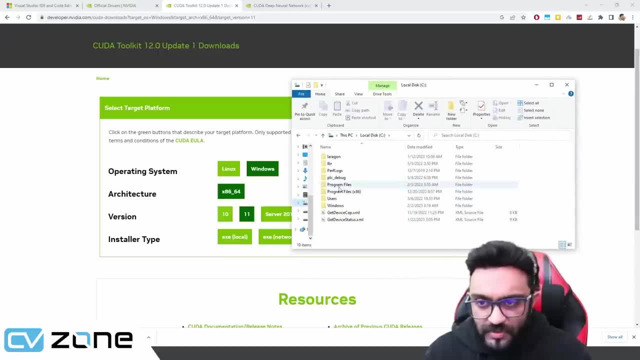 will install and i will check my version as well. so once you have installed that, you will click on my version as well. so it will install in program files and if you go down nvidia gpu computing toolkit and if you go to cuda, this is 11.5. so i have 11.5 based on the version, the latest version. 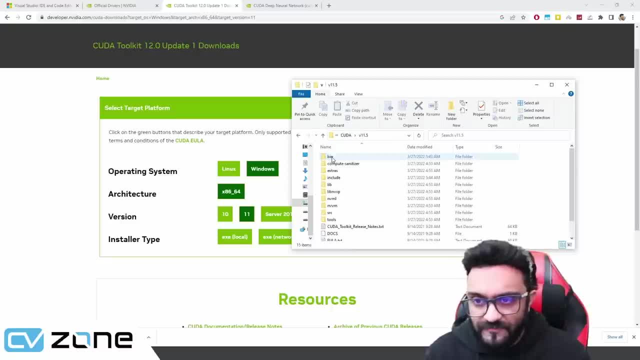 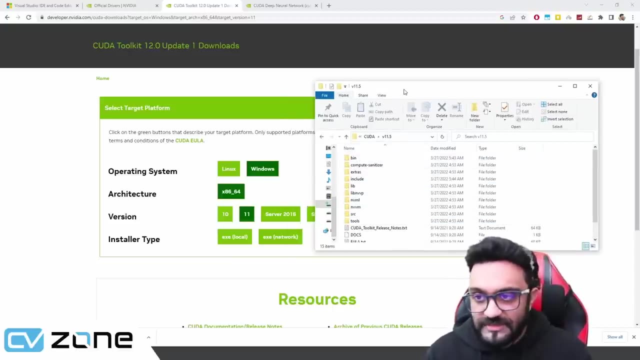 you can download as well. so here it's 11.5. we will open that up and you can see again. this will be an installer. it will be a wizard you have to click next, next, next, install it in c, and in c this is where you will find all the files. so keep this folder open, because next we are going to install. 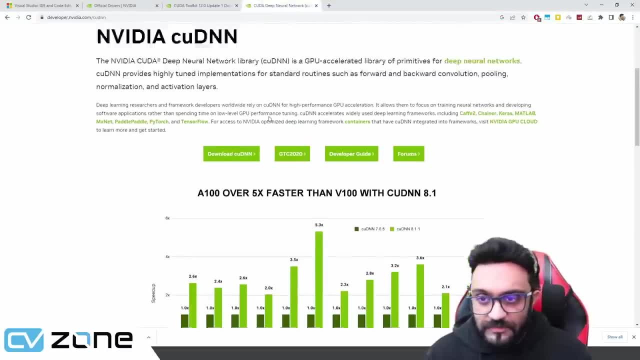 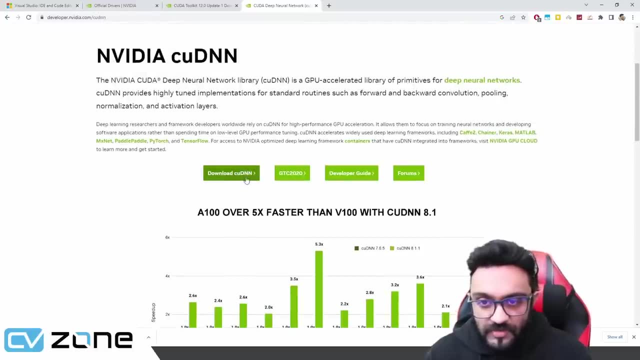 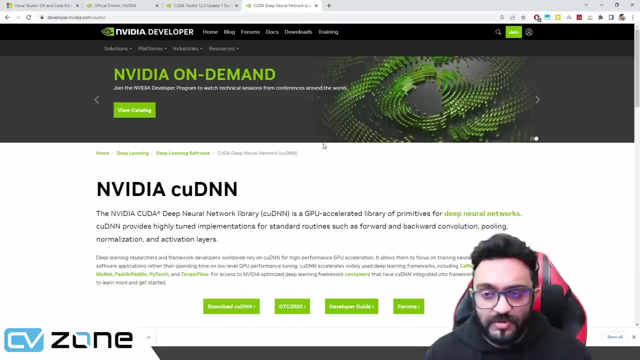 cuda dnn, which is which stands for deep neural networks, cuda, deep neural networks. so again you have to go click on download, uh the cuda dnn, and this will need, uh, what you call the registration on their website. so make sure you have registered and it is free to download. so just make sure that. 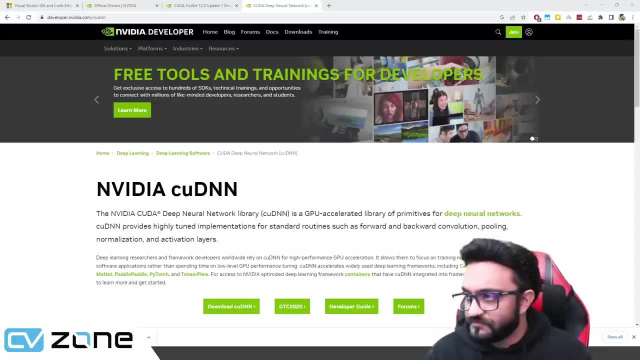 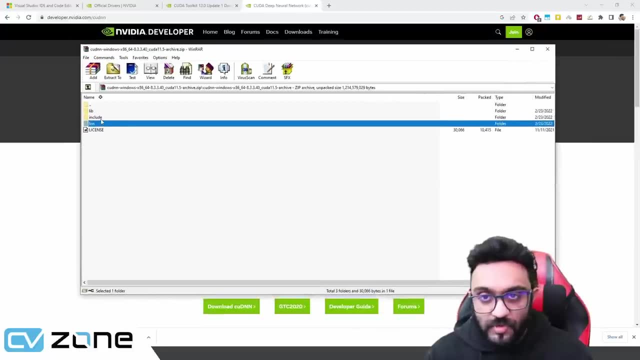 you have registered and it will let you download, uh, the cuda dnn. so once you download that, this is what you will get, so make sure the versions are compatible. so right now, this is for 11.5, which i installed as the toolkit, so i have to. 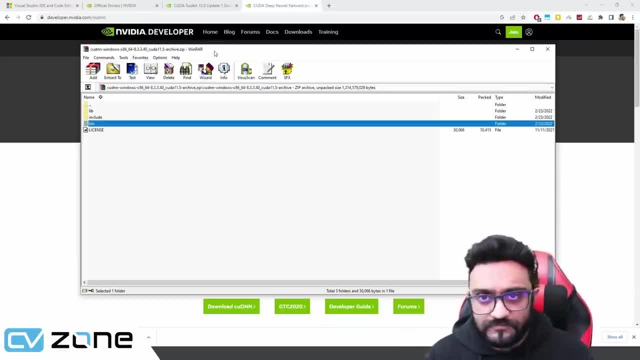 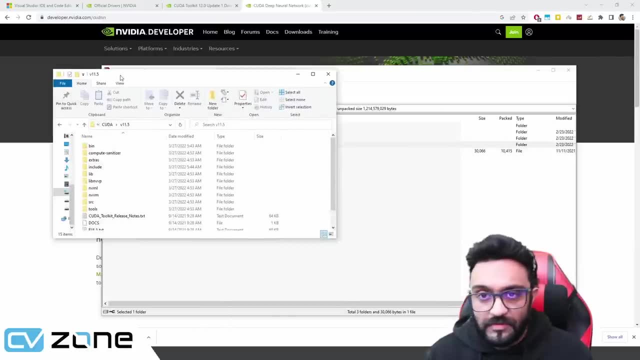 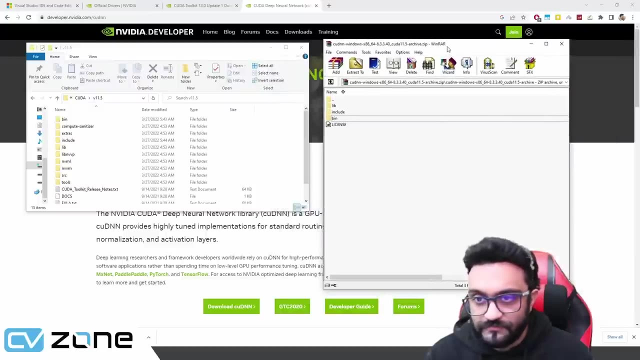 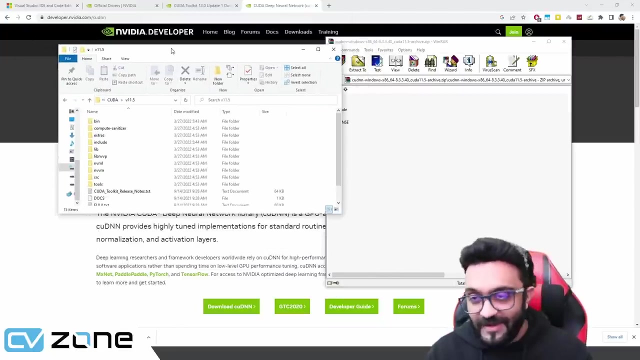 download it for 11.5. uh, the cuda dnn. so this is what you will get. so if we open up our folder to install this, all you have to do is you have to open up your folder here, so you will see, here you have a bin folder. so this is the cuda toolkit. i don't know why it's. 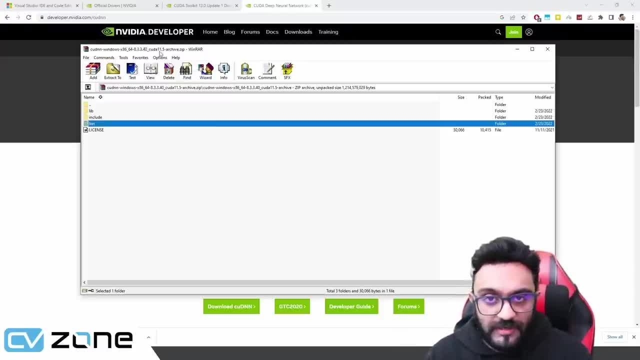 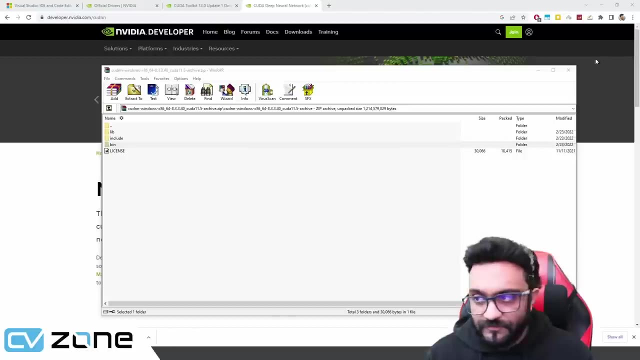 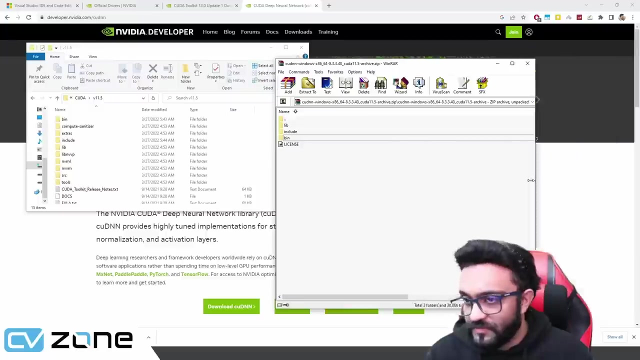 compatible. so right now, this is for 11.5, which i installed as the toolkit. so i have to download it for 11.5 and the cuda dnn. so this is what you will get. so if we open up our folder to install this hats, check it out, alright, in here. so what we will see in here is: this is the cuda tool kit. 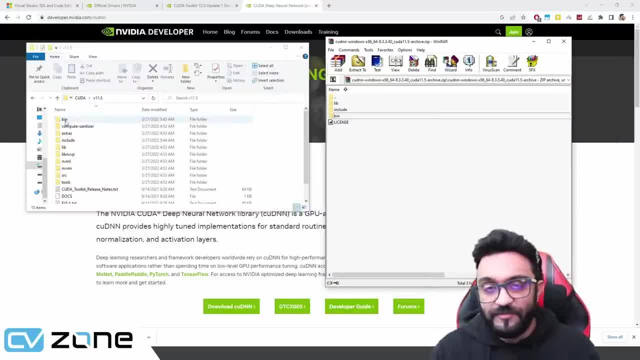 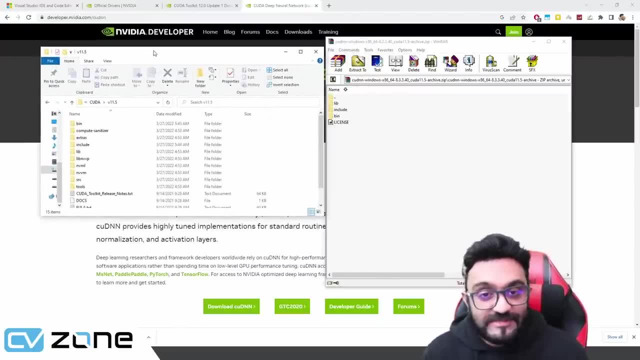 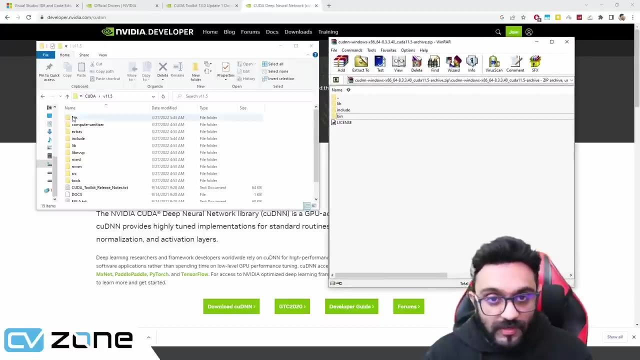 so here you have to do is you have to open up your folder here. so you will see, here you have a bin folder. so this is the quda tool kit. i don't know why it's so hard to pronounce this. so this is the cuda tool kit. so this is that and this is the dnn. so if you go to bin, 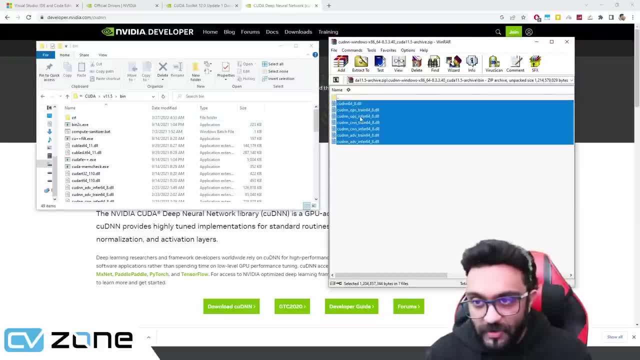 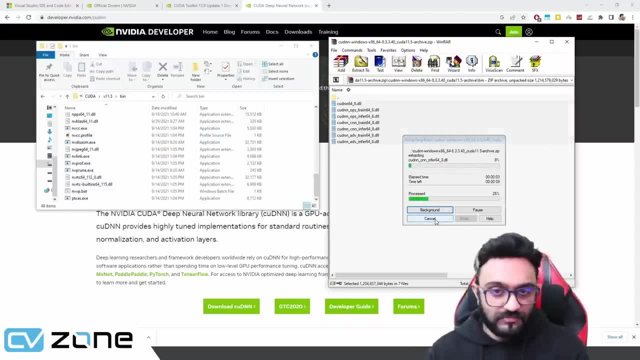 here you have a bin folder, here you have a bin folder and copy all of these files and paste it here. so just drag and drop. so i have already done that. so it will ask me to do it again. i will not do that again. so then you will go back, then you will. 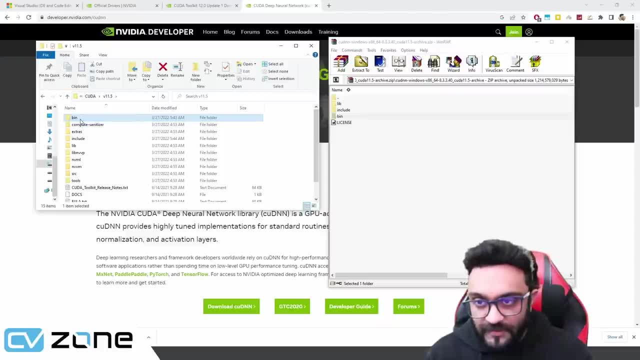 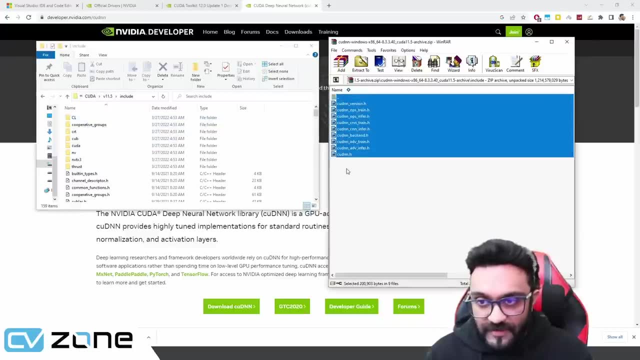 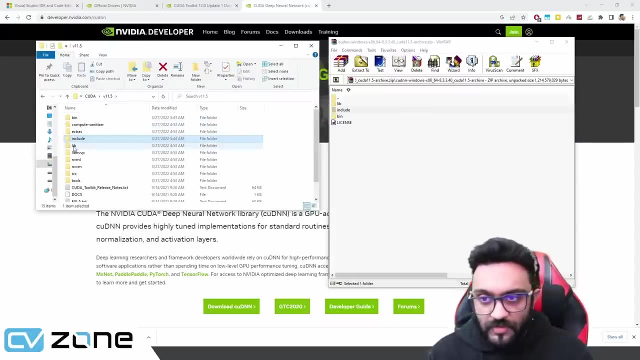 go back and you will go back here. we have already done the bin. then you will go to include, so in include again you will open, include here, copy all these files, drag and drop them here, so in the main folder, like that. so then you will go back and then you will go to lib and inside lib 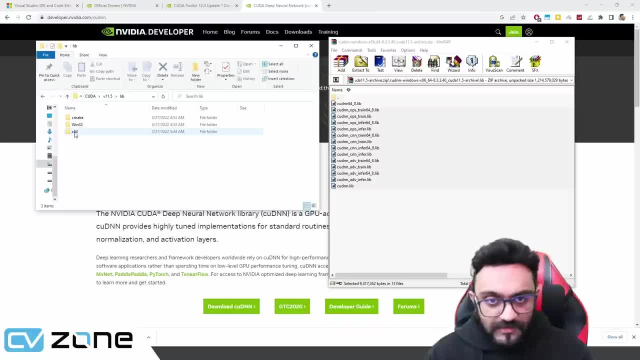 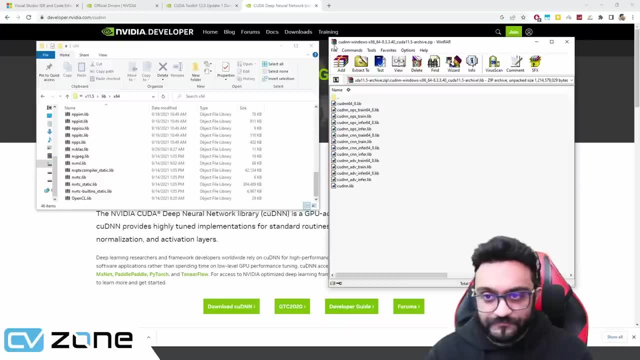 you will see all these files, but here you will not paste them directly. you will go to x64 and over here you are going to paste all these. so drag and drop all these over here. so this way it will install your cuda toolkit along with the cuda deep neural networks, cuda dnn. so this: 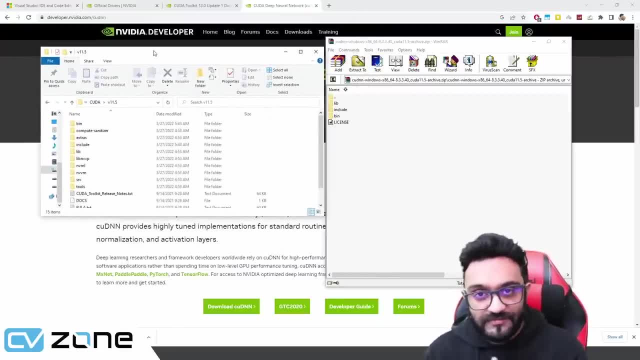 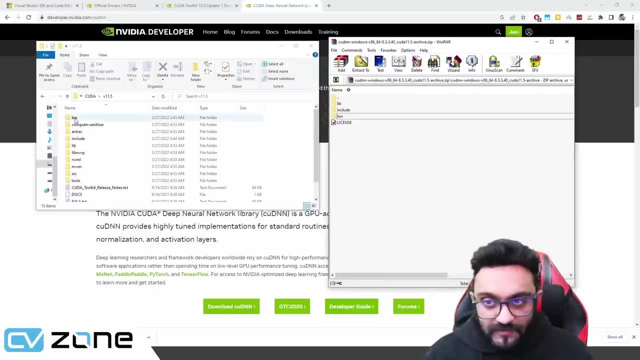 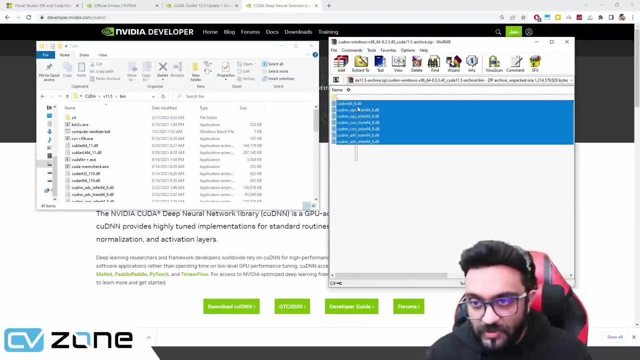 so hard to pronounce this. so this is the cuda toolkit. so this is that and this is the dnn. so if you go to bin- here you have a bin folder, here you have a bin folder, open up bin and open up bin and copy all of these files and paste it here. so just drag and drop. so i have already done that. 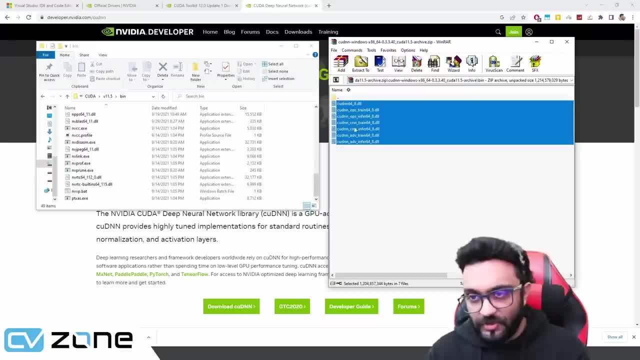 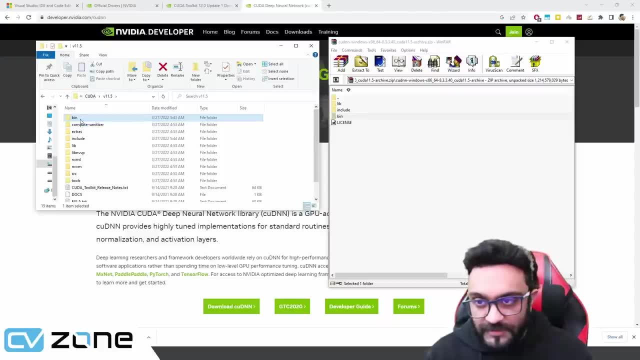 so it will ask me to do it again. i will not do that again. so then you will go back. then you will go back and you will go back here. we have already done the bin. then you will go to include, so in, include again. you will open, include here, copy all these files, drag and drop them here. so in the main, 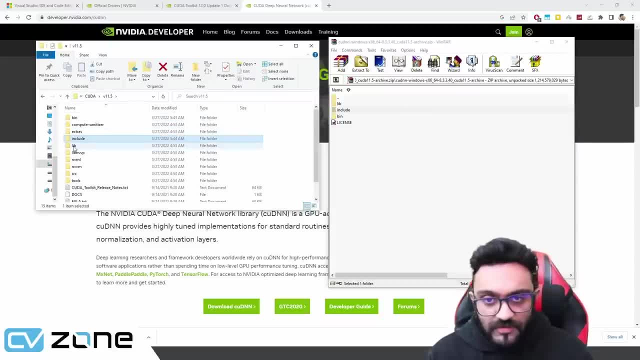 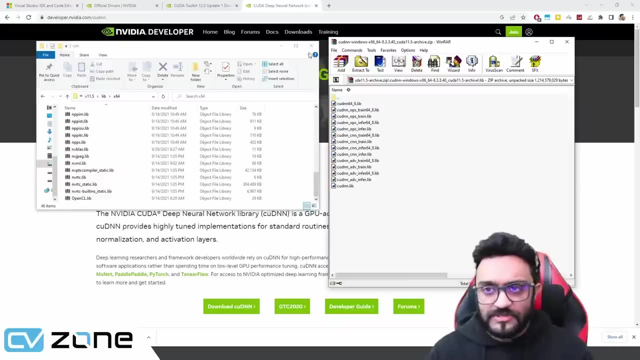 folder like that. so then you will go back and then you will go to lib and inside lib you will see all these files, but here you will not paste them directly. you will go to x64 and over here you are going to paste all these. so drag and drop all these over here. so this way it will install. 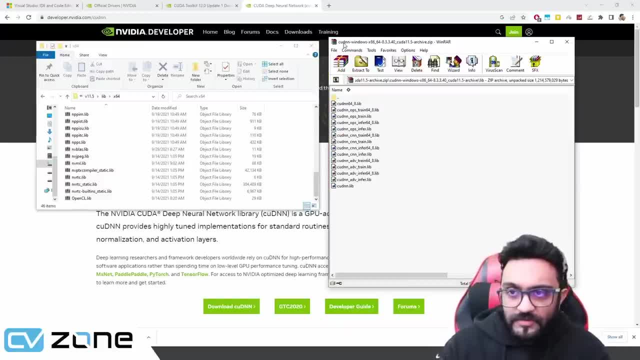 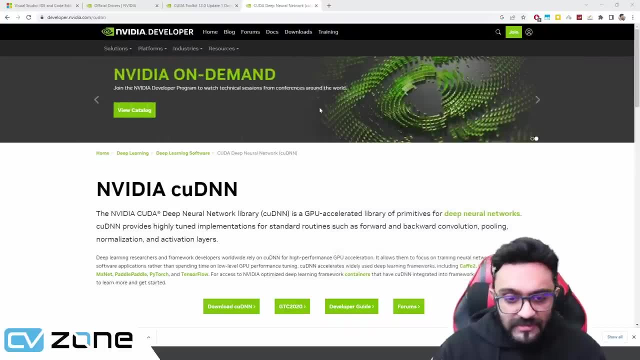 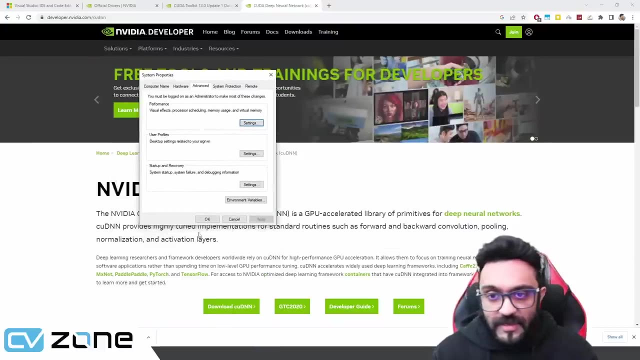 your cuda toolkit, along with the cuda deep neural networks, cuda dnn. so this is basically the installation. and one last thing you have to do is you have to go to your environmental variables. so you will click on edit system variables and here you will go to environment variables, and over here you will go to cuda path. 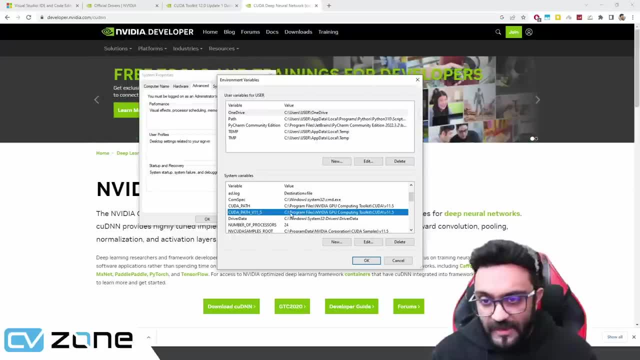 11.5. so this is the version that i have and you will make sure that it points to the correct directory. so, if you remember, we had it in program files: nvidia, gpu, computing toolkit, cuda and then version 11.5. so make sure this and this they are pointing to the right path. 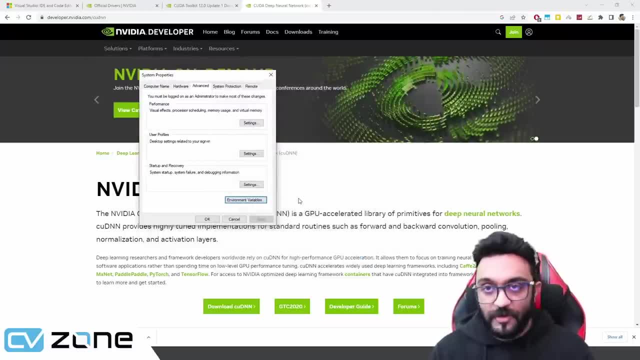 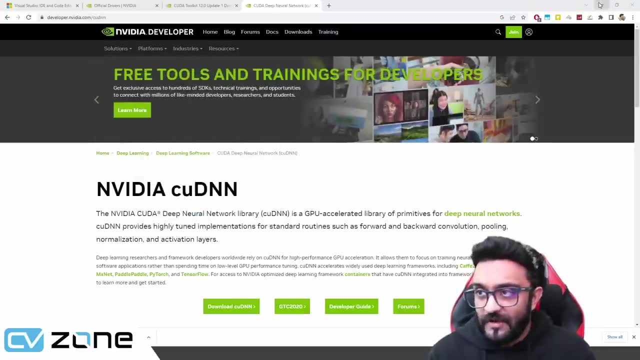 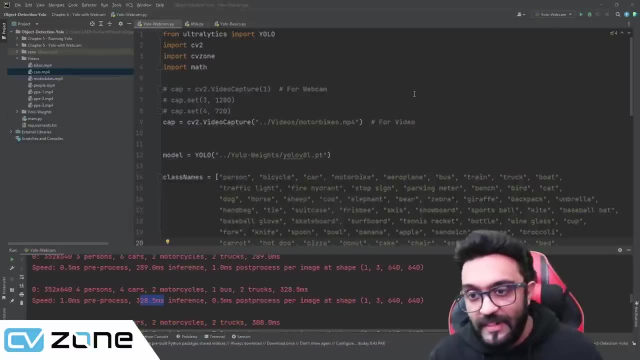 so if they are pointing, then it's fine. if they are not, type it in. make sure they are in the correct path. so you hit ok and that is it. so now the, the drivers and the cuda toolkit and the cuda deep neural network is installed. but there is one more step. we do need to install pytorch, which 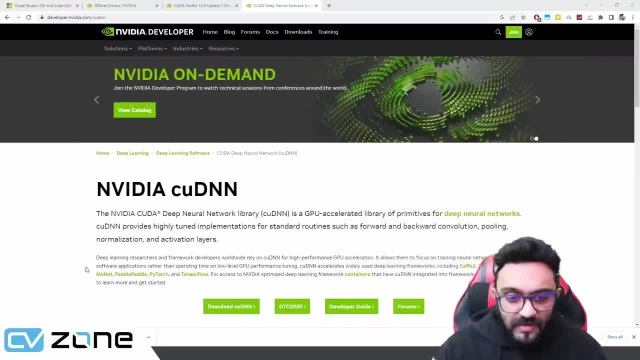 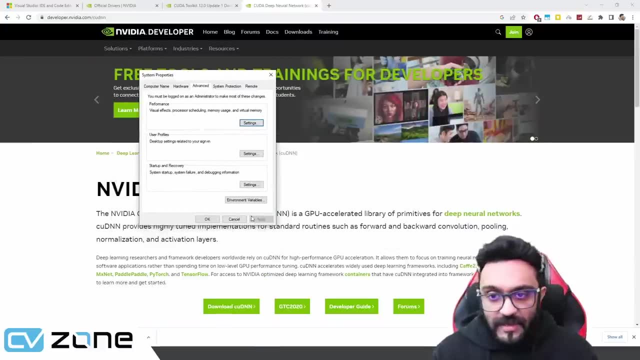 is basically the installation. and one last thing i want to mention is that if you want to install cuda dnn you have to do is you have to go to your environmental variables. so you will click on edit system variables and here you will go to environment variables and over here you will go. 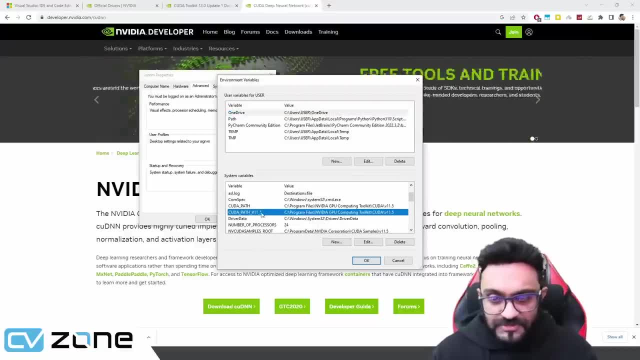 to cuda, path 11.5. so this is the version that i have and you will make sure that it points to the correct directory. so, if you remember, we had it in program files: nvidia, gpu, computing toolkit, cuda and then version 11.5. so make sure this and this they are pointing to the right path. 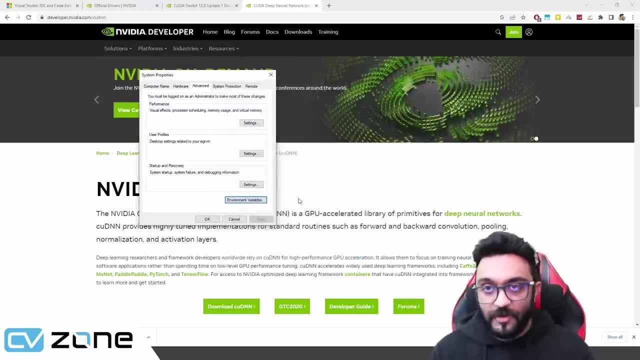 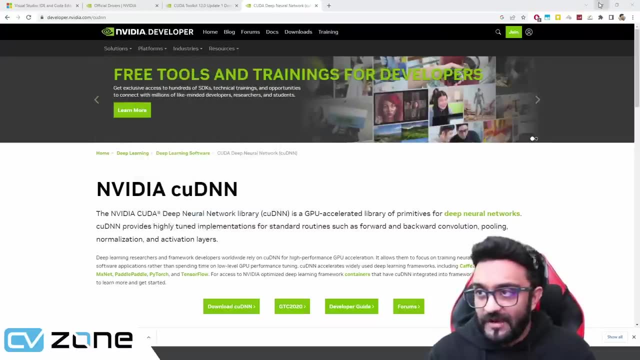 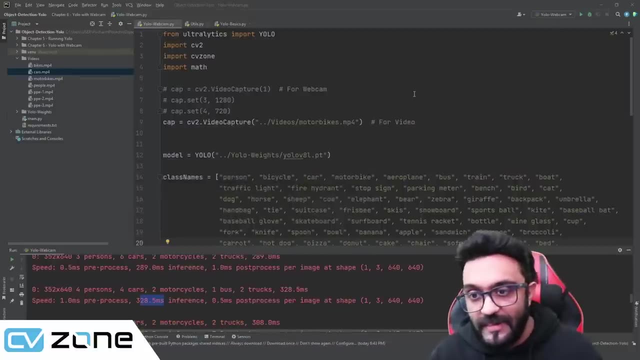 so if they are pointing, then it's fine. if they are not, type it in. make sure they are in the correct path. so you hit ok and that is it. so now the, the drivers and the cuda toolkit and the cuda deep neural network is installed. but there is one more step. we do need to install pytorch. 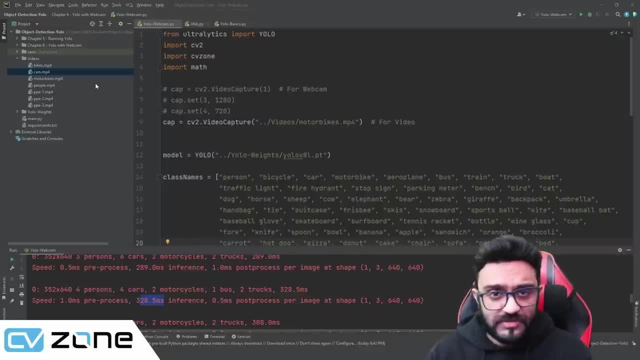 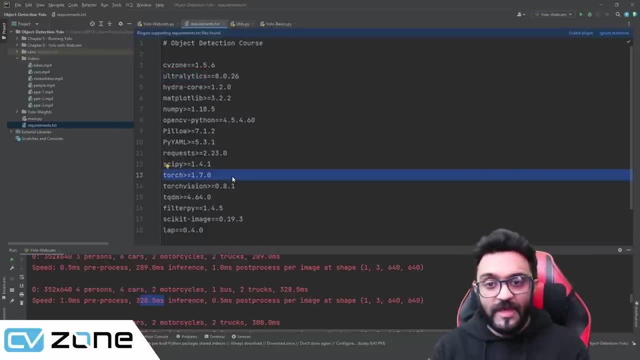 which is compatible with cuda. so here you can see in the requirements: we have already installed torch, but now we have to install the torch which is compatible with the gpu or with cuda. so how can you do that? we can go to their website. so this is the pytorch website. 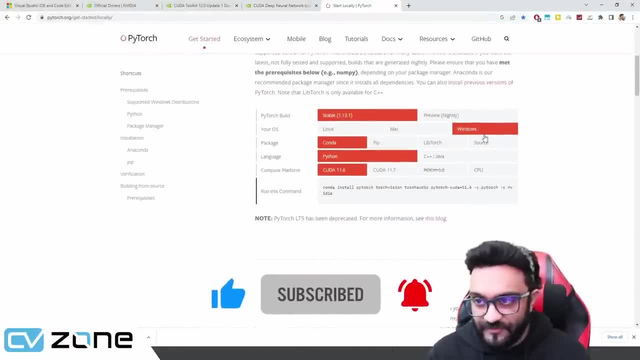 and this is how we can install. so we are using the stable version for windows, we are going to use pip to install and we are installing it on python and we are installing for cuda 11.6 and this is the command that we need to run. so we are going to copy that again. i will share this command. 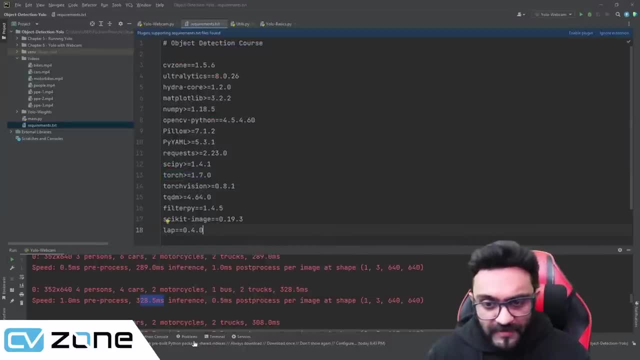 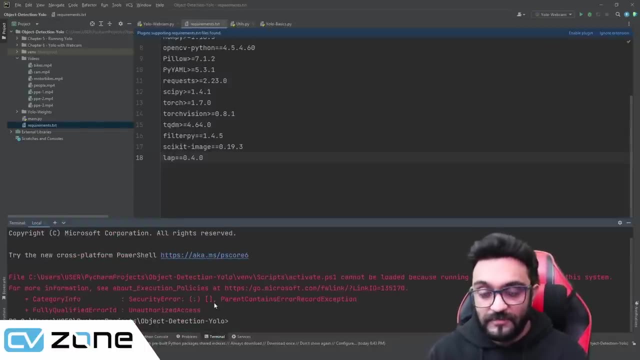 so that it's easier for you to install. so you will copy that and here at the bottom you are going to go to terminal. now this is very important because some of you might make this mistake and it is very frustrating. if you make this mistake, make sure you are not in local. click on this down arrow and select command prompt. 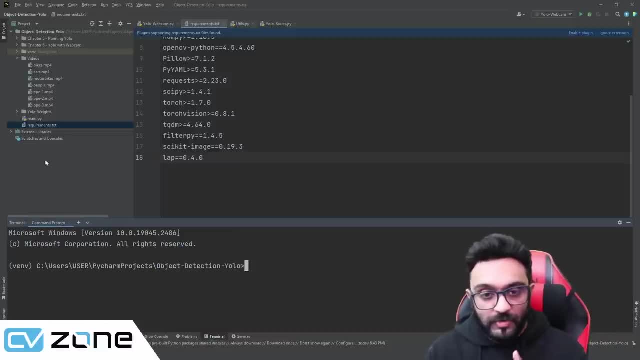 If you are at local, it will install it globally. We want to install it in this virtual environment, So you have to go to the command prompt and here you can see it's installing it in the virtual environment. So here we are going to paste our link and we are going to press OK or we are going to 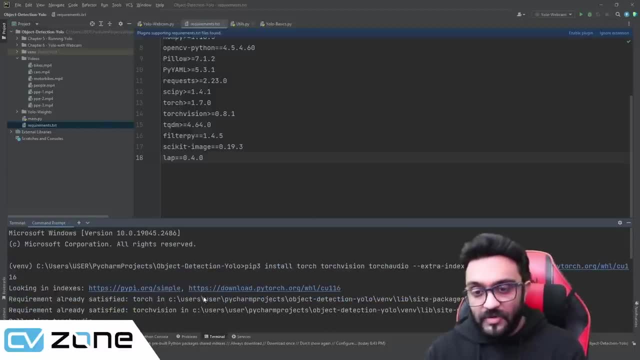 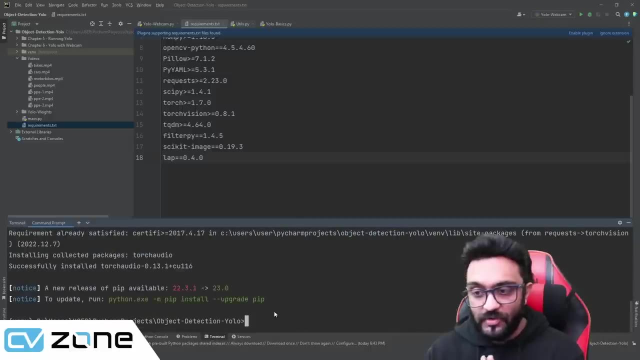 hit enter. So this will take a while because I have done this already. It has all these files archived in the cache, So that's why it is able to install this very quickly. Otherwise, it will take a while to actually install all of these. 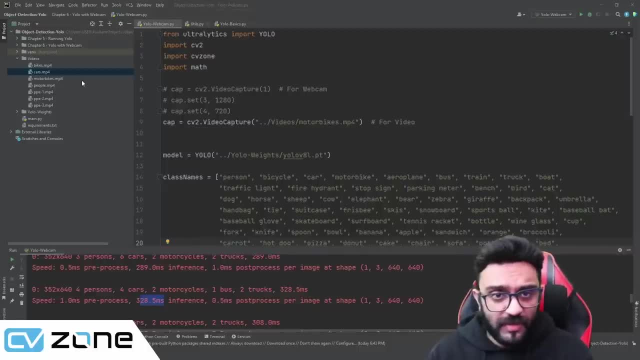 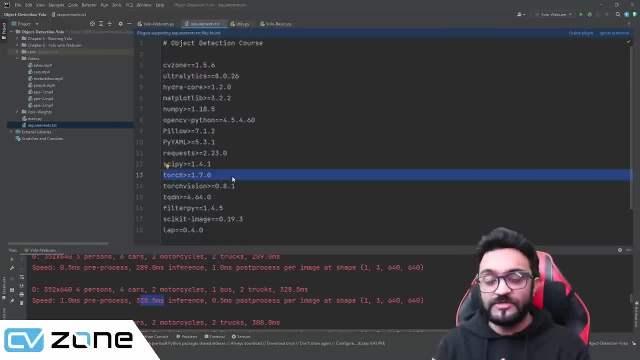 is compatible with cuda. so here you can see in the requirements: we have already installed torch, but now we have to install the torch which is compatible with the gpu or with cuda. so how can you do that? we can go to their website. so this is the pytorch website and this: 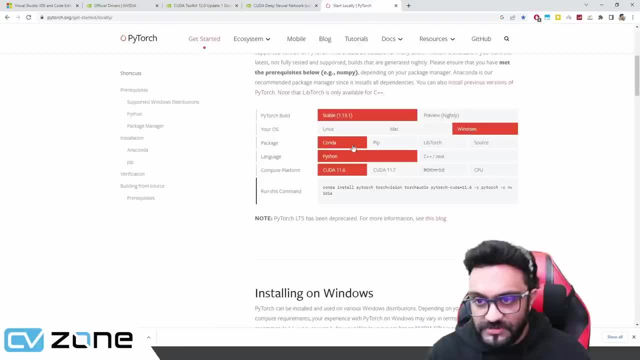 is how we can install. so we are using the stable version for windows, we are going to use pip to install and we are installing it on python and we are installing for cuda 11.6 and this is the command that we need to run, so we are going to copy that again. I will share this command so that 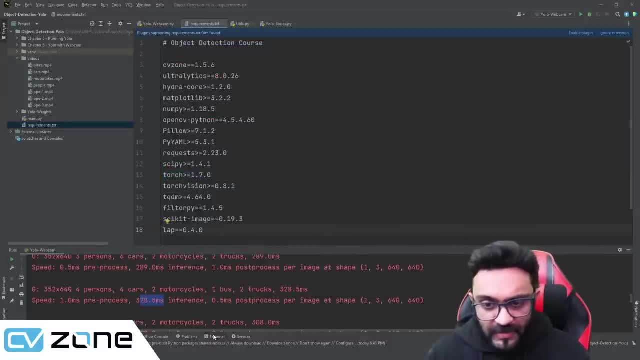 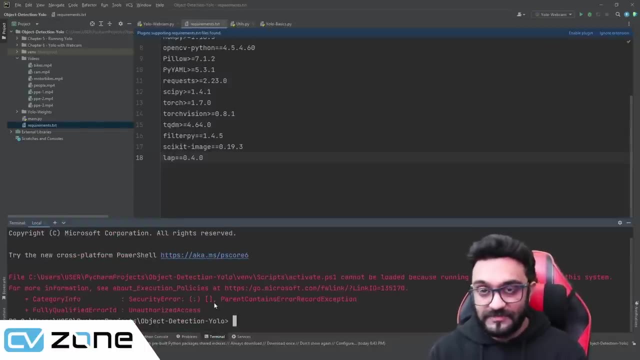 it's easier for you to install. so you will copy that and here at the bottom you are going to go to terminal. now this is very important because some of you might make this mistake and it is very frustrating. if you make this mistake, make sure you are not in local. click on this down arrow and 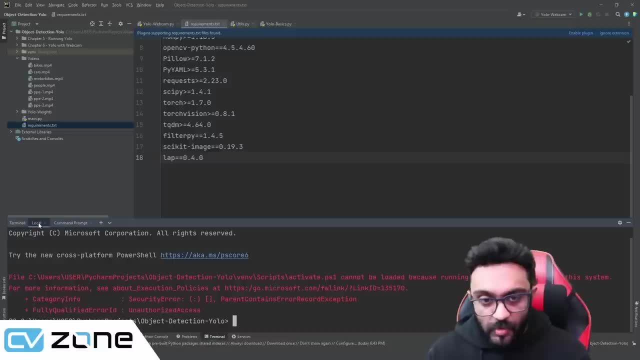 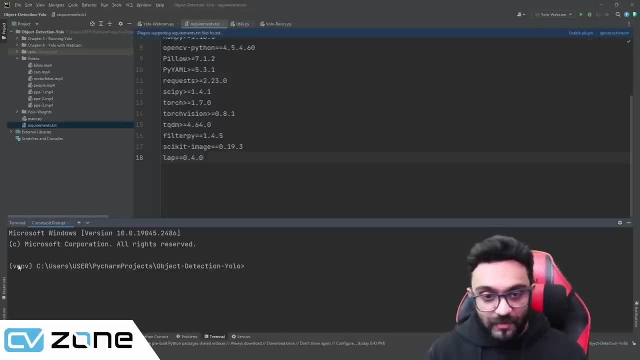 select command prompt, because if you are in that local it will install it globally. we want to install it in this virtual environment, so you have to go to the command prompt and here you can see it's installing it in the virtual environment. so here we are going to paste our link and we are going to press OK or we are going to hit enter. so 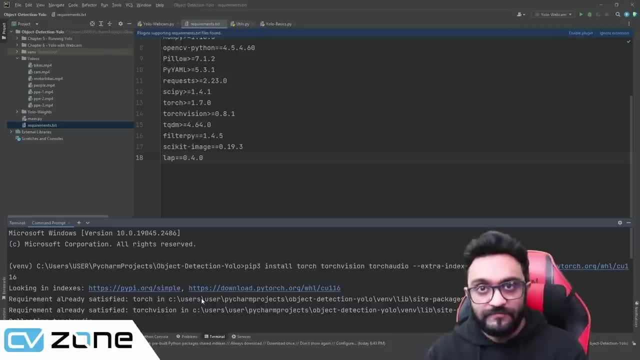 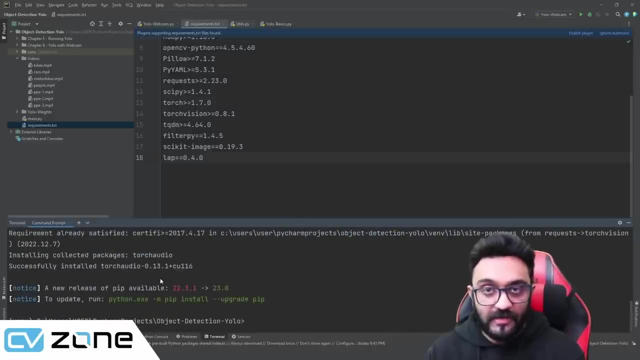 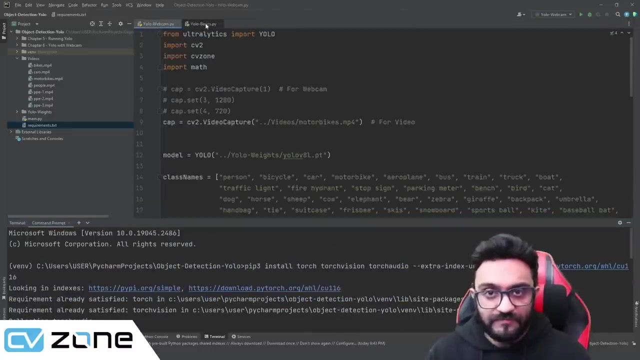 this will take a while because I have done this already. it has all these files archived in the cache, so that's why it is able to install this very quickly. otherwise it will take a while to actually install all of these. so once it is done, we can go back and we can go to, we can close all of these and here in. 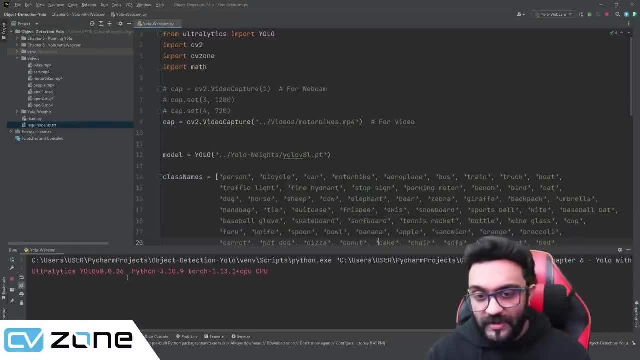 the webcam, we can right click and we can run Yolo. so if it's actually using the GPU, then it will right here GPU. so right now it's not actually showing GPU, it means there is something wrong. it did not install it properly. so if we go to file settings- 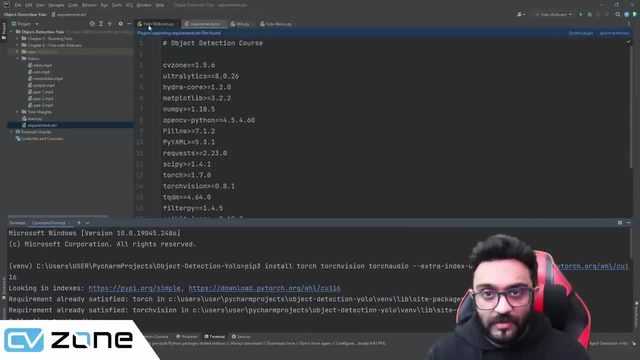 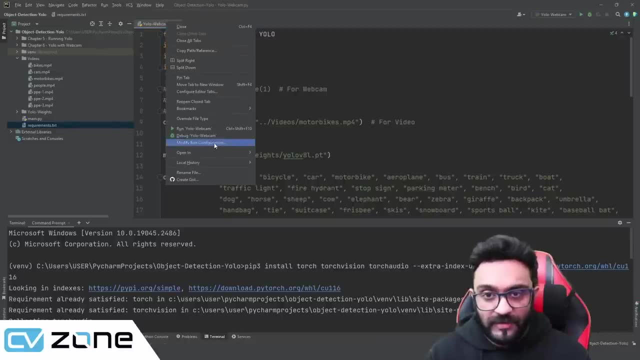 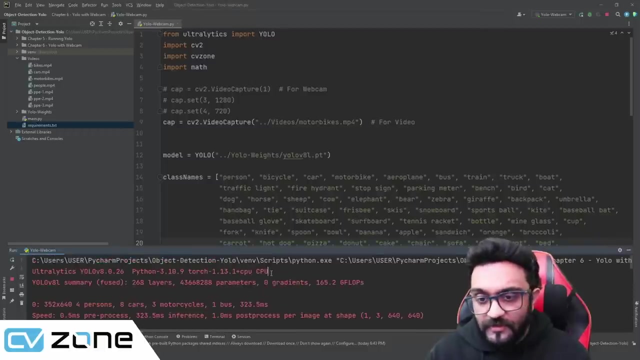 So once it is done we can go back and we can close all of these, and here in the webcam we can right click and we can run YOLO. So if it's actually using the GPU, then it will write here GPU. So right now it's not actually showing YOLO. 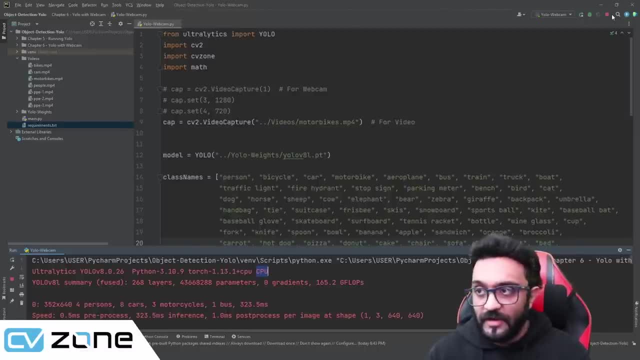 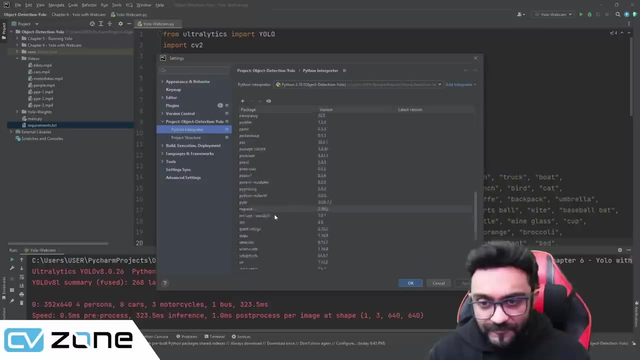 It's showing GPU, So it means there is something wrong. It did not install it properly. So if we go to file settings and interpreter, if we go to the torch over here, it is using the same torch that we had earlier, So it's probably not using it properly. 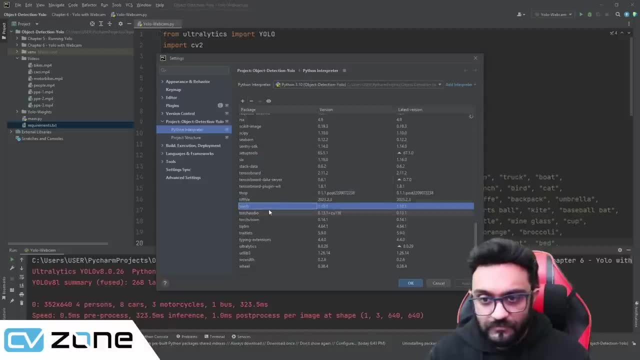 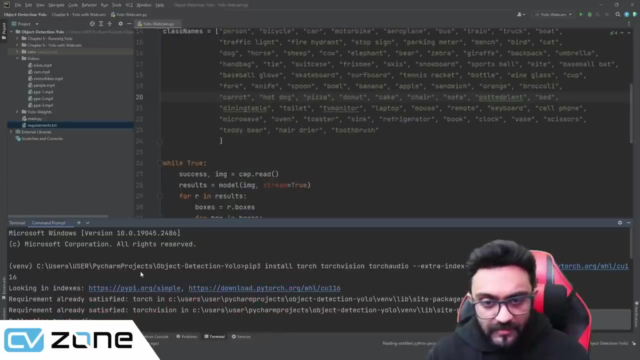 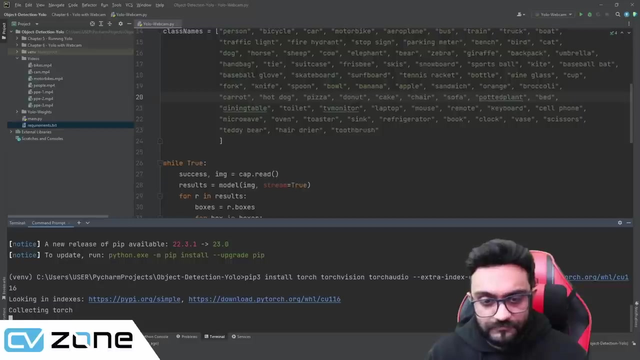 So what we can do is we can uninstall, Just to make sure, And we can uninstall the torch audio and the torch vision. We can uninstall those, will press OK and then we'll go to our terminal and then we will run the command again. 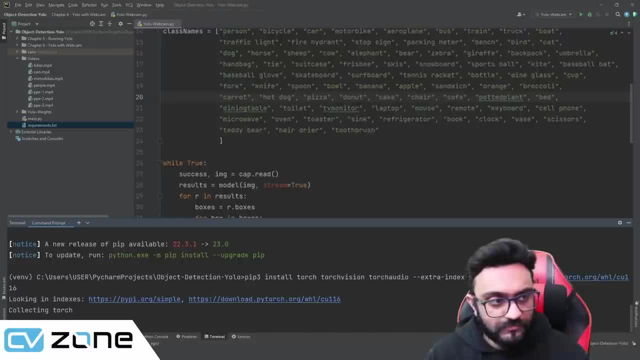 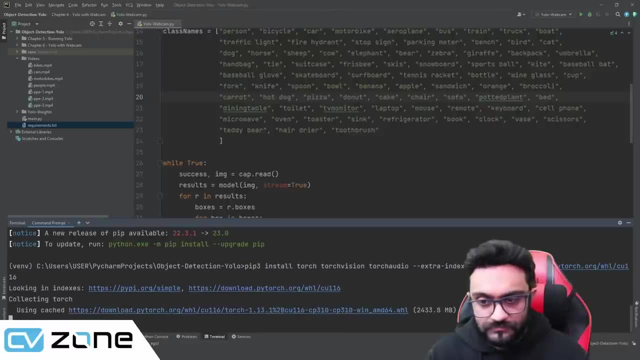 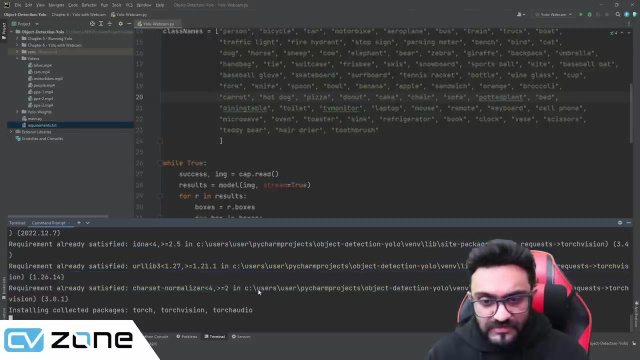 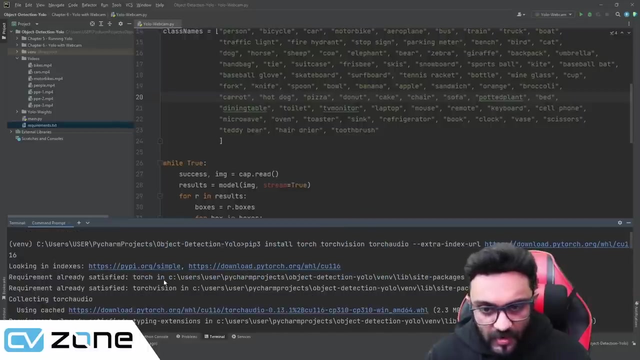 So again you can see it is using the cached, otherwise it is quite a big file. It's almost 2.4 GB, So it will take a while to download and install. I think what happened earlier was that all the requirements were already satisfied. 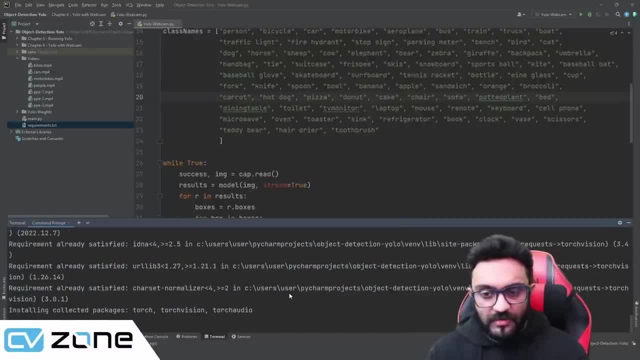 The torch was there, Vision was there, So it didn't actually Reinstall. It didn't install anything. So I believe that's what happened. So you need to uninstall and install again. So it is currently installing. So let's see how it works. 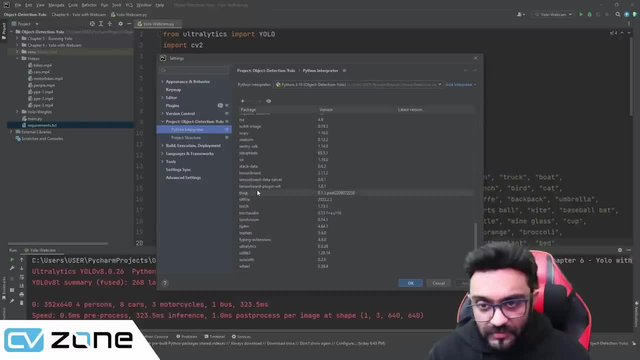 an interpreter. if we go to uh the torch over here, it is using the same torch that we had earlier, so it it's probably not using it properly. so what we can do is we can uninstall, just to make sure we can uninstall the torch audio and the torch Vision. we can uninstall those. 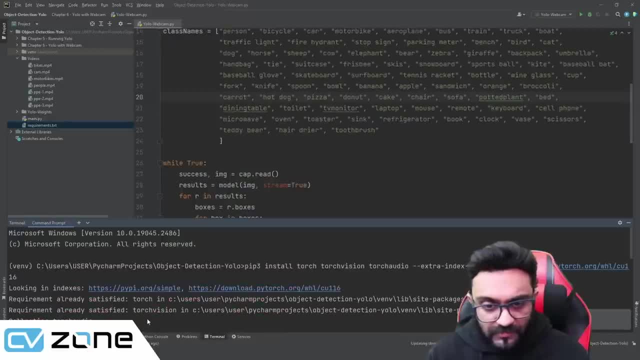 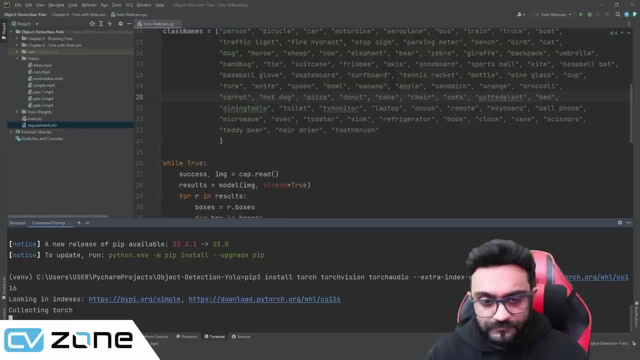 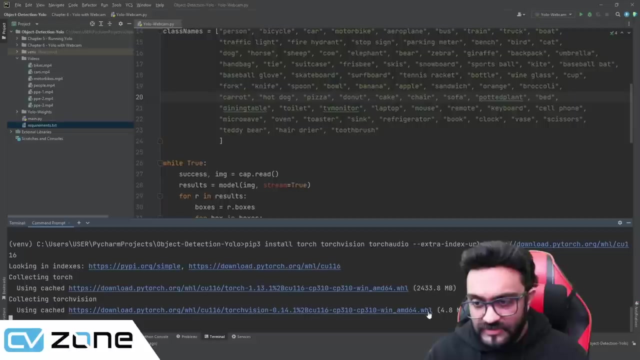 we'll press OK and then we will go to our terminal and then we will run the command again. so again you can see it is using the cached. otherwise it is quite a big file. it's almost 2.4 gbs, so it will take a while to download. 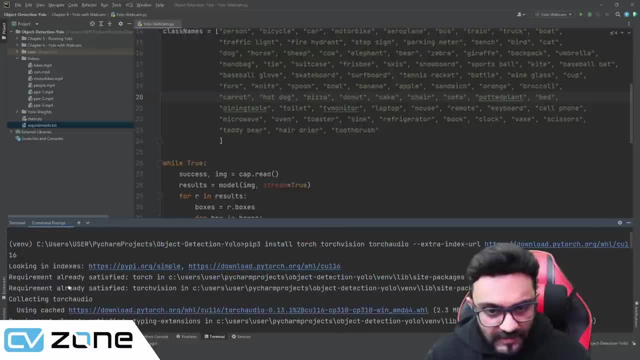 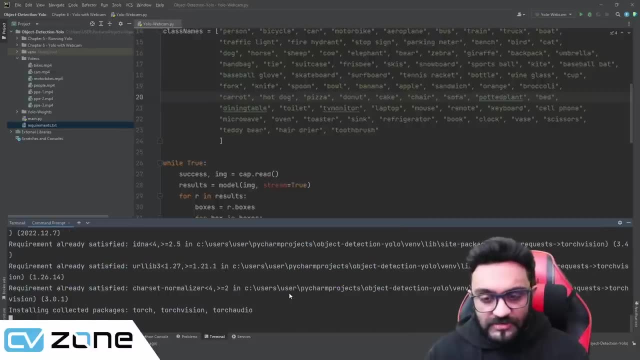 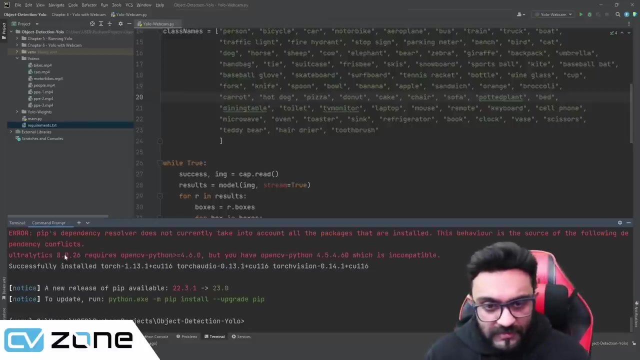 and install. i think what happened earlier was that all the requirements were already satisfied: the torch was there, vision was there, so it didn't actually reinstall. it didn't install anything. so i believe that's what happened. so you need to uninstall and install again. so it is currently installing, so let's see how it works. so it is saying that requires a later. 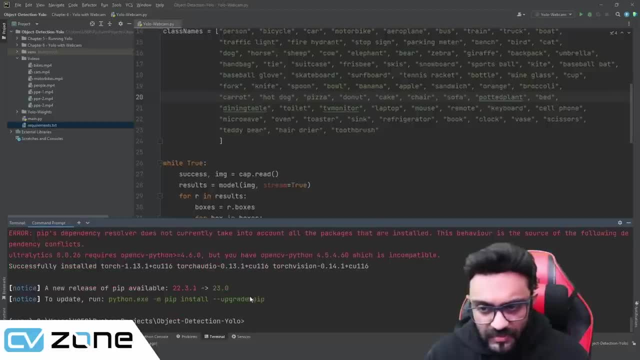 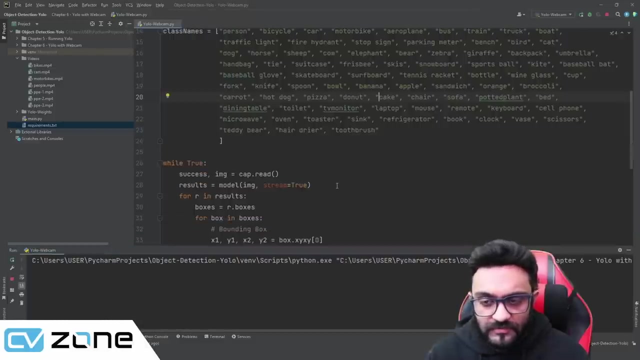 version of opencv. we are using this um. i believe it should be fine, so otherwise it has installed. so let's run that and see if we are getting so it is updating. that's why it's not running. let's run that again. there you go. so now you can see. 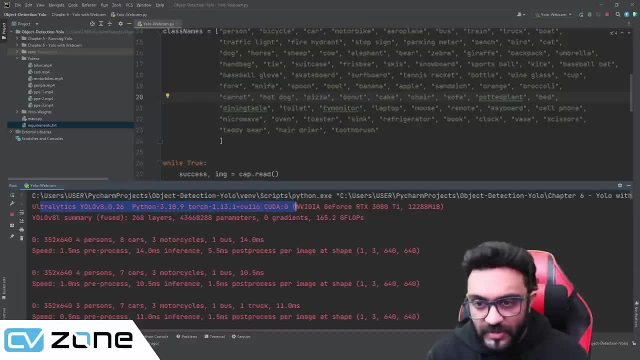 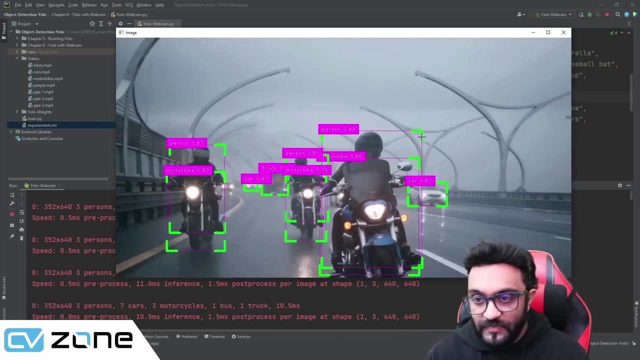 it says ultralytics, yolo, python, blah, blah, blah, cuda, zero, nvidia geforce uh 3080 ti. so this means now it's not using the cpu, it's actually using the gpu and if we open up, there we go. now it's lighting fast, so it is using the gpu. earlier it was using the cpu and it was dead slow. 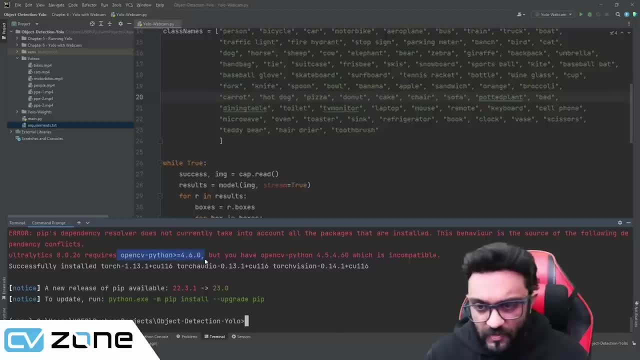 So it is saying that requires a later version of OpenCV. We are using this. I believe it should be fine. So otherwise it has installed. So let's run that and see if we are getting. So it is updating. That's why it's not running. 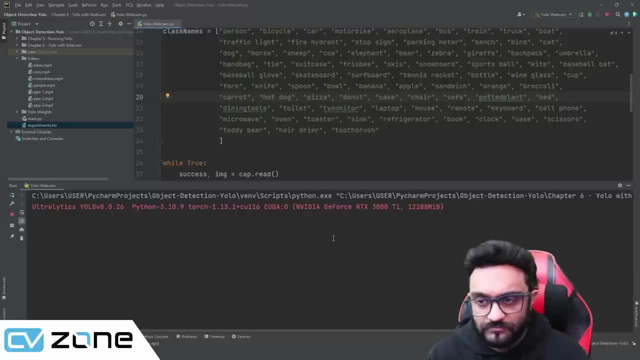 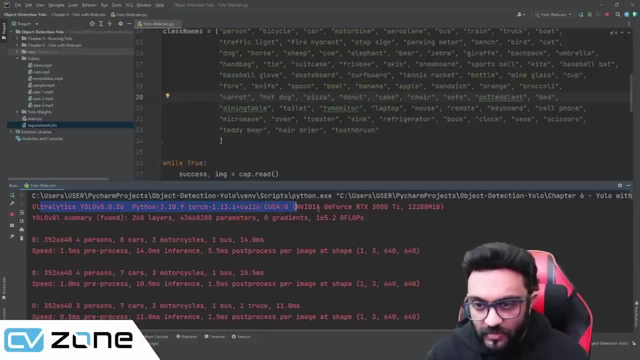 Let's run that again. There you go. So now you can see it says Ultralytics, YOLO, Python, blah, blah, blah. CUDA 0, NVIDIA GeForce 3080 TI. So this means now it's not using the CPU, It's actually using the GPU. 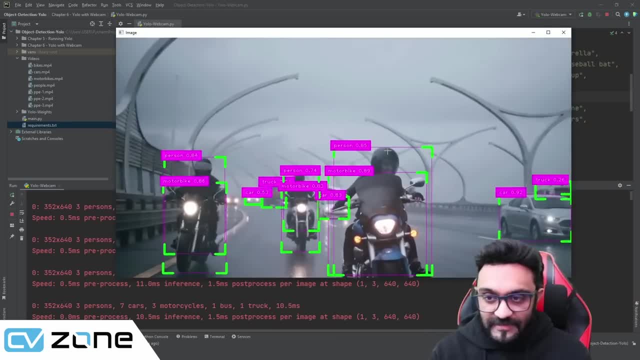 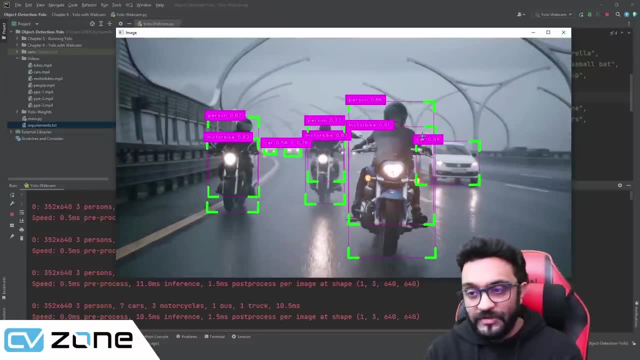 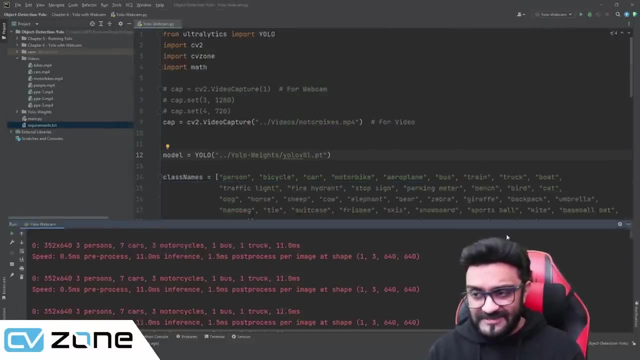 And if we open up, Open up, There you go. Now it's lighting fast, So it is using the GPU. Earlier it was using the CPU and it was dead slow, But now it's using the GPU. And remember, we are using the large version for this demonstration and still it is running. 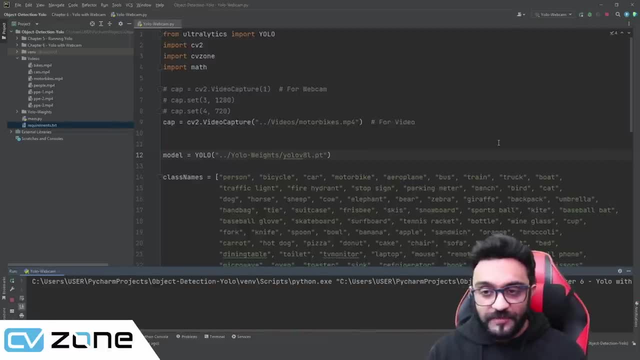 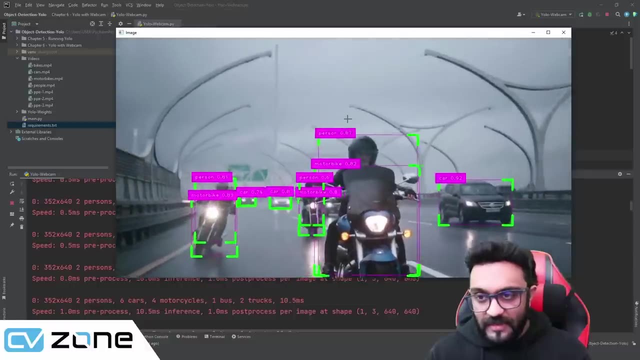 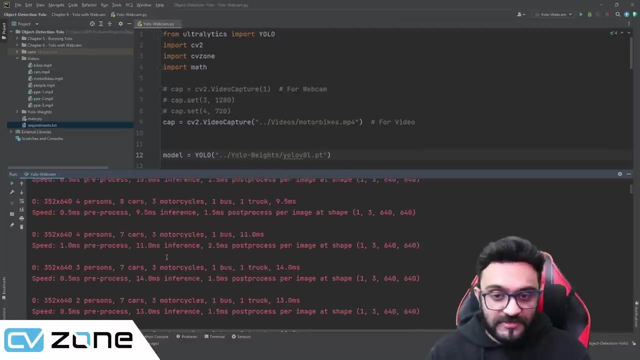 real time. So that is very good. It means the GPU has been running properly and it has accelerated our video, our inference, and that's how it's running. So right now, 10.5.. So 10 milliseconds earlier, the inference was 300 milliseconds. 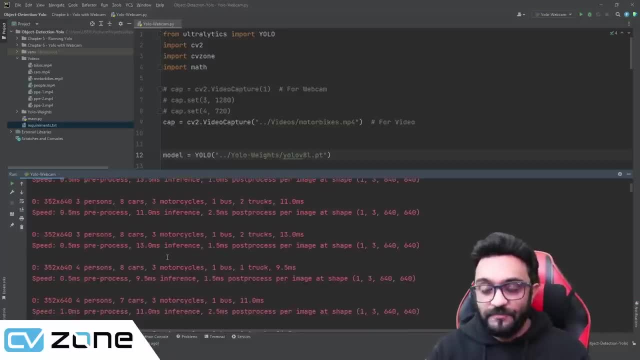 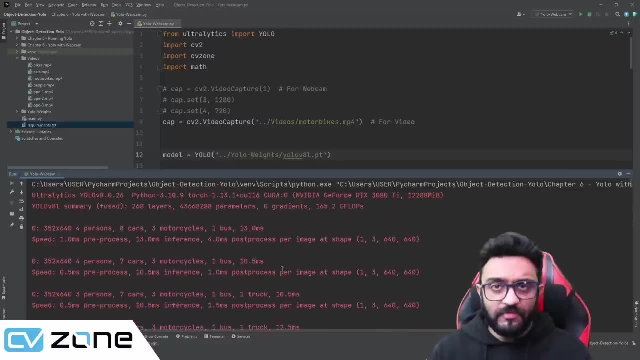 So that is a difference of 30 X. So that is a very big, big difference when we are using the GPU. So that's great. And again, if you run into any issues, go back and check the video again, follow through. 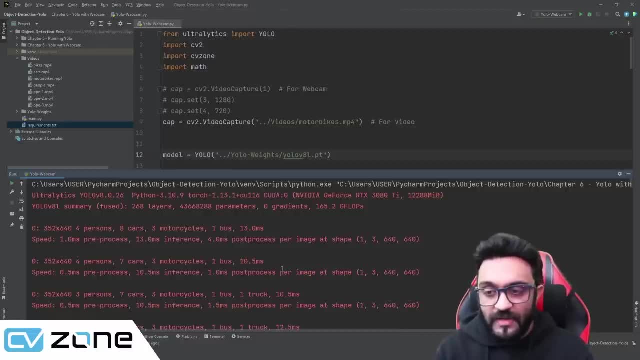 the steps one by one, and it should work fine at the end. So again, it's a big difference. So it's Well worth trying this And if it runs properly, you will have a much faster system that will be running Yolo in. 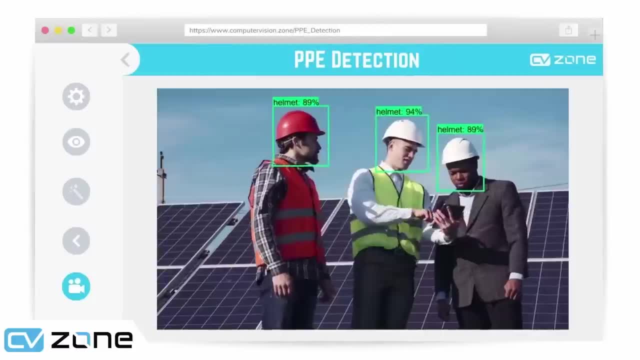 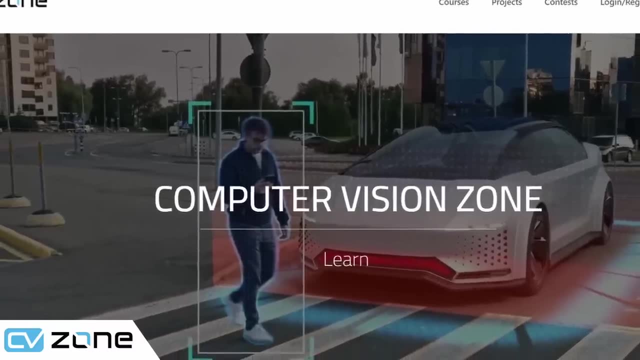 real time. Do you want to implement your computer vision ideas to solve real world problems or upgrade your resume by enhancing your computer vision skills? Then the computer vision dot zone is the perfect platform for you. CV zone is a one-stop computer vision platform with over a hundred thousand users with courses. 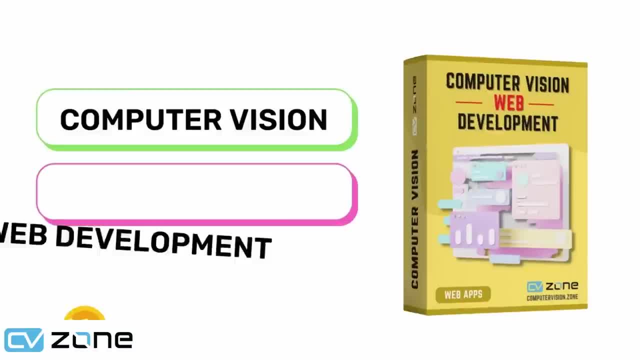 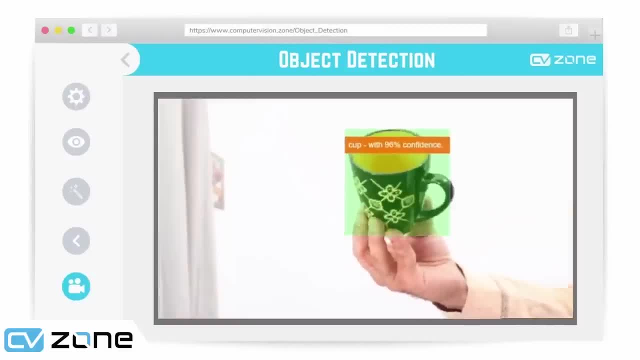 sold in over 80 different countries. If you want to commercialize your computer vision ideas, Then the computer vision web development course is the perfect course for you. here You will learn the basics of web development and computer vision, as well as how to integrate. 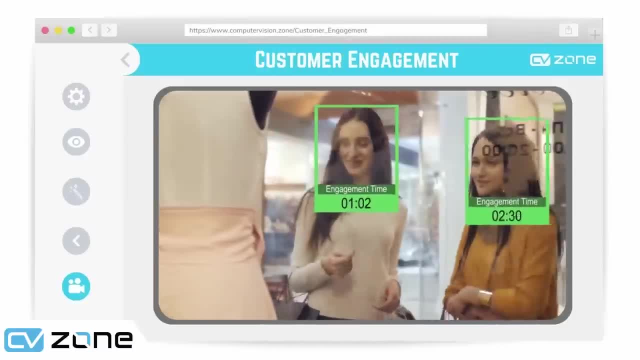 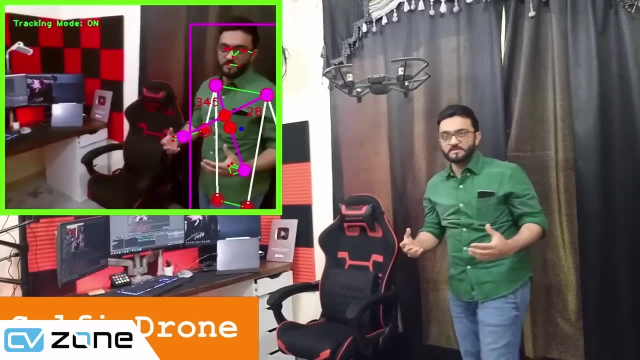 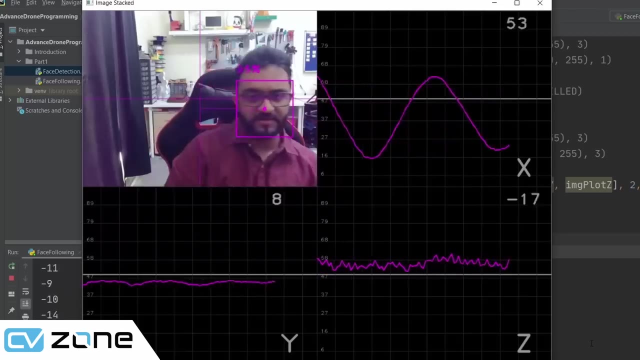 them to solve real world problems like customer engagement, car counter, face attendance, shirt size measurement and a lot more advanced. stone programming is another great course that focuses on the practical implementation. Here you will learn the basics of drone programming as well as advanced concepts like face following. 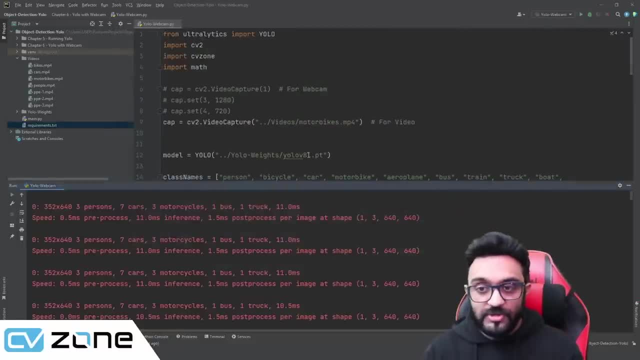 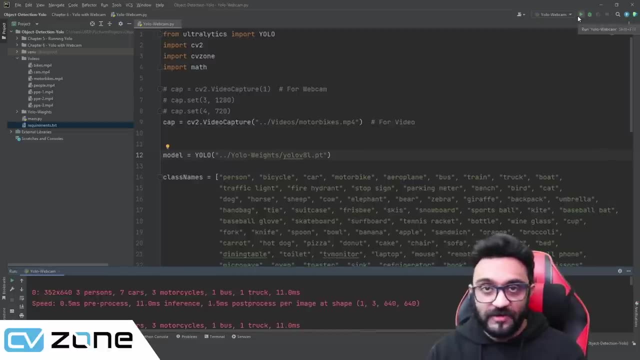 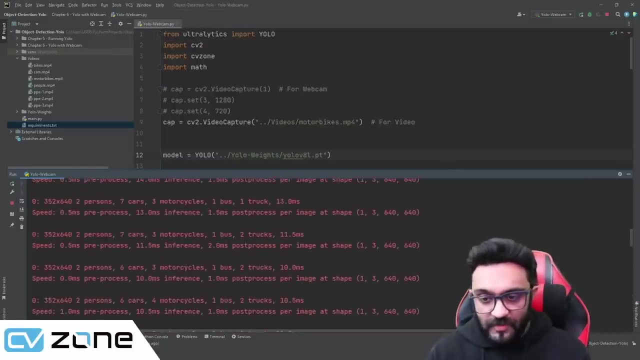 but now it's using the gpu- and remember we are using the large version for this demonstration and still it is running real time. so that is very good. it means the gpus has been running properly and it has accelerated um, our video, our inference, and that's how it's working running. so right now the inference is: 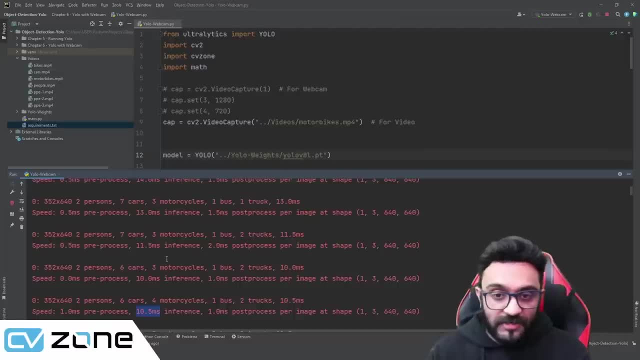 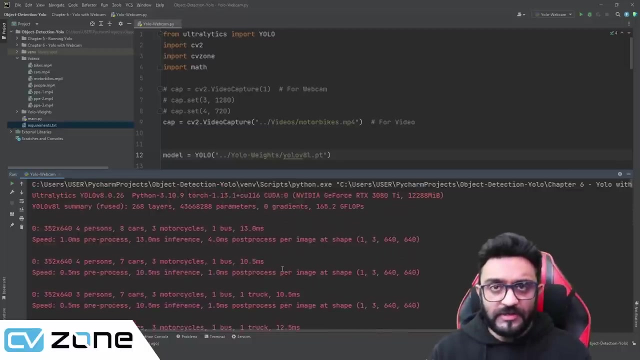 10.5, so 10 milliseconds. earlier the inference was 300 milliseconds, so that is a difference of 30x. so that is a very big, big difference when we are using the gpu. so that's great and if you run into any issues, go back and check the video again. follow through the steps one by one. 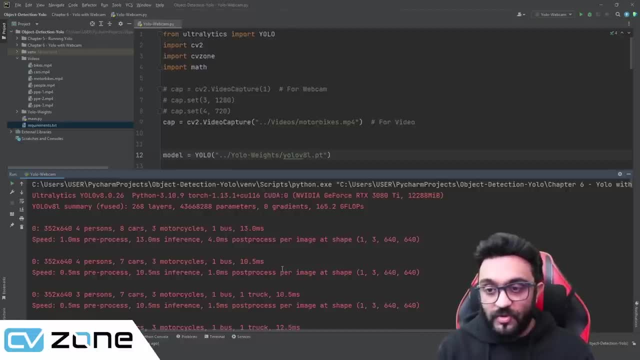 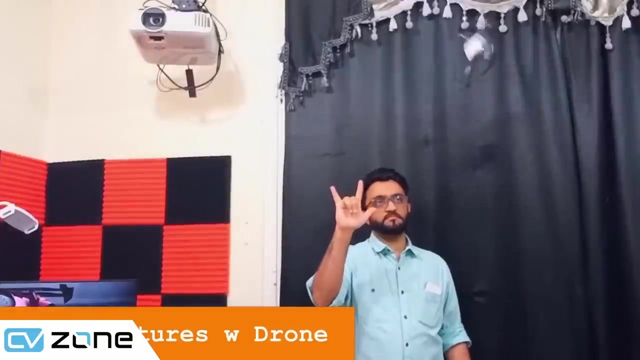 and it should work fine, uh, at the end. so again, it's a big difference. so it's well worth trying this and if it runs properly, you will have a much faster system that will be running yolo in real time. do you want to implement your computer vision ideas to solve real world problems? 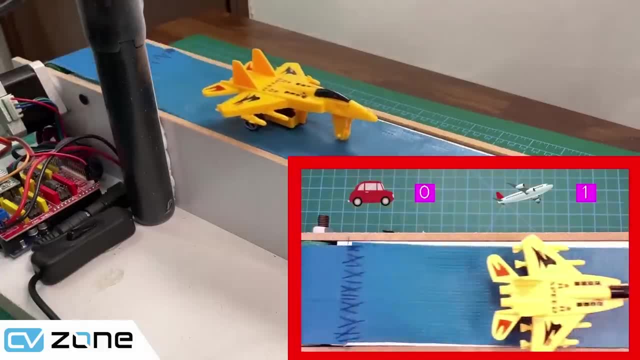 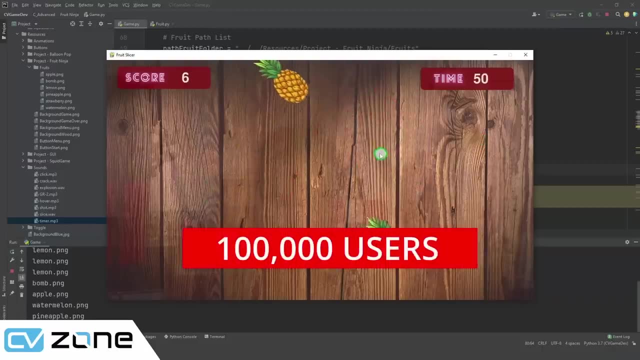 or upgrade your resume by enhancing your computer vision skills, then the computer visioncom is the perfect platform for you. cvzone is a one-stop computer vision platform with over 100 000 users with courses sold in over 80 different countries. if you want to commercialize, 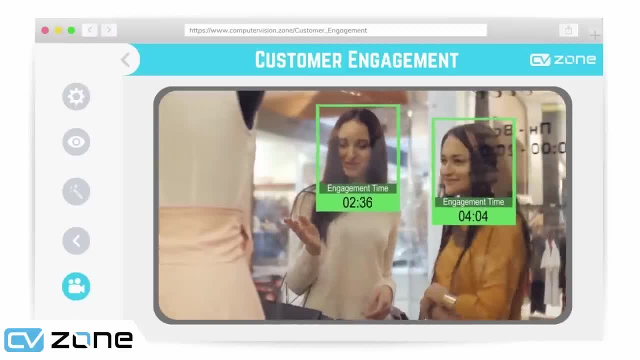 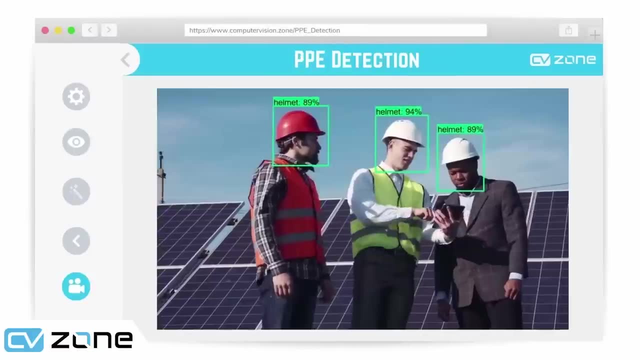 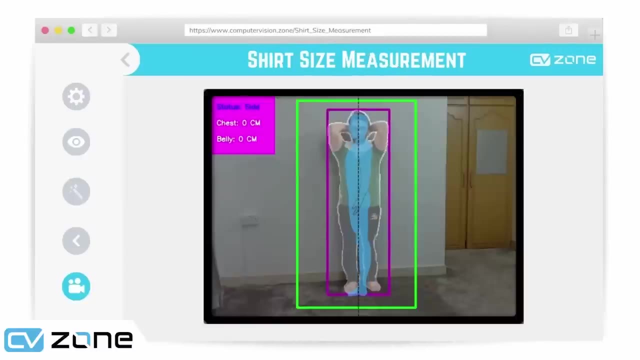 your computer vision ideas, then the computer vision web development course is the perfect course for you. here you will learn the basics of web development and computer vision, as well as how to integrate them to solve real world problems like customer engagement, car counter, face attendance, shirt size measurement and a lot more. 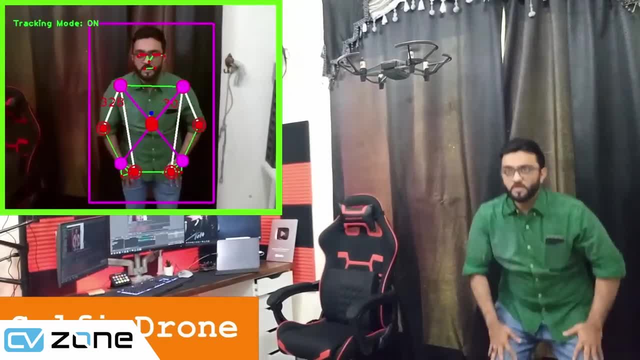 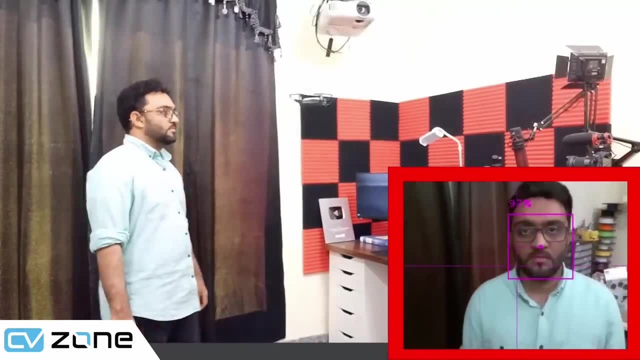 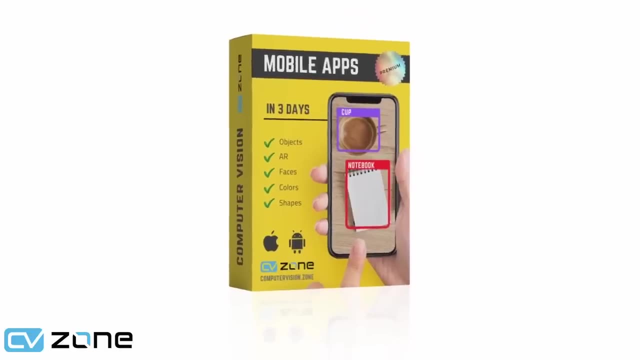 advanced tone programming is another great course that focuses on the practical implementation. here you will learn the basics of drone programming, as well as advanced concepts like face following, body following, gesture control and a lot more. if developing mobile apps is your thing, then check out our computer vision mobile apps course. here you will learn. 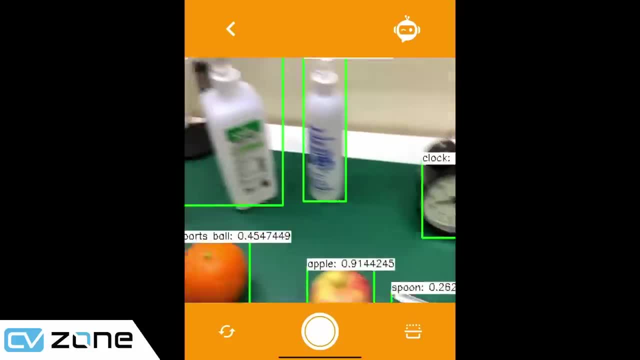 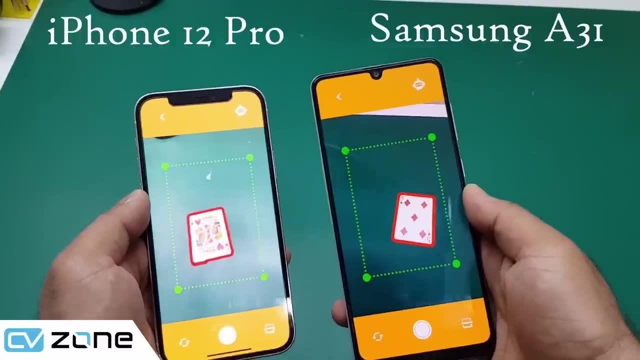 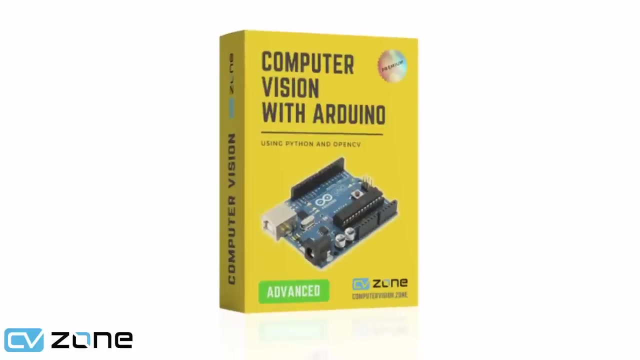 the basics and create several apps, including object detection, augmented reality, face detection, document scanner and a lot more. the best part is that you will create a single app that will work both on ios and android. if you are passionate about integrating hardware with software, then check out our computer vision arduino course. here you will learn the basics. 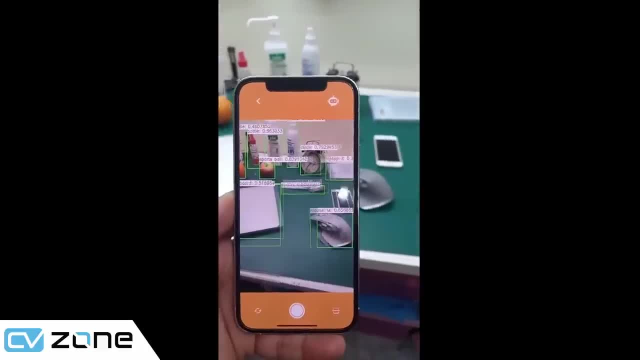 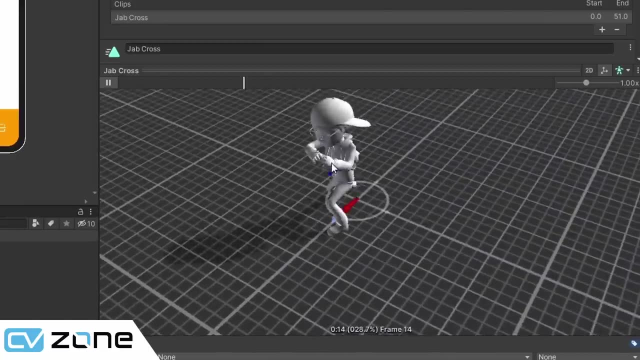 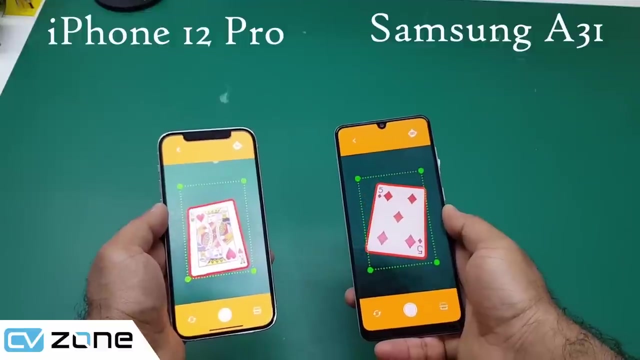 body following. If developing mobile apps is your thing, then check out our computer vision mobile apps course. Here you will learn the basics and create several apps, including object detection, augmented reality, face detection, document scanner and a lot more. The best part is that you will create a single app that will work both on iOS and Android. 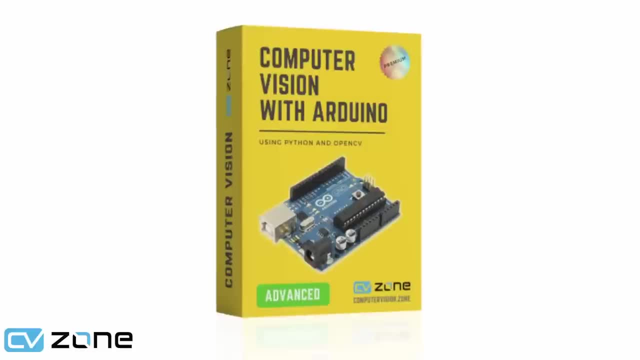 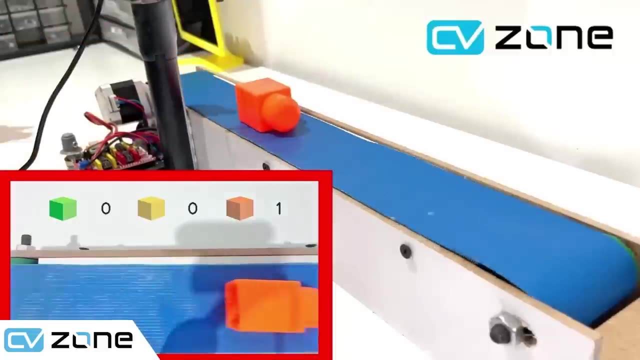 If you are passionate about integrating hardware with software, then check out our computer vision Arduino course. Here you will learn the basics along with amazing projects. Thank you, The game software is particularly good for software development, such as conveyor belt assembly, face tracking, lamcester control, door lock and a lot more. 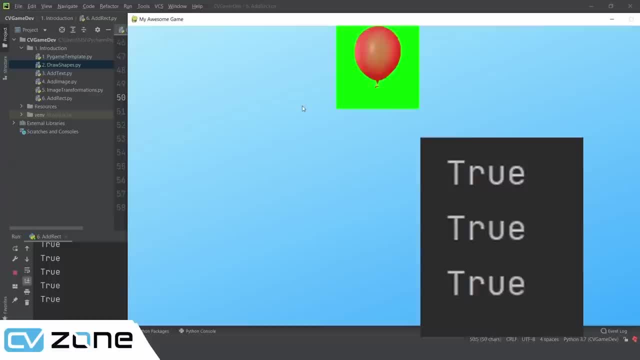 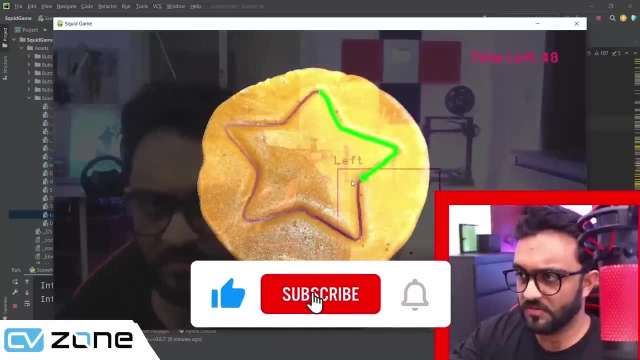 The computer vision game development is another great course where fun meets programming. Here you will learn to create games such as fruit ninja, balloon, pop squid game, cookie cutter-, all using the latest computer vision techniques. Not only that else: will learn to compile your awesome game to an exe file to make it. 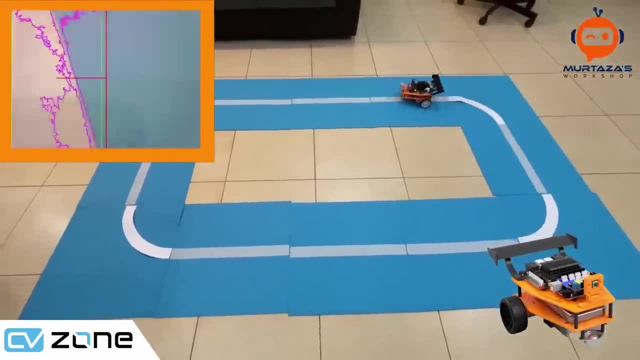 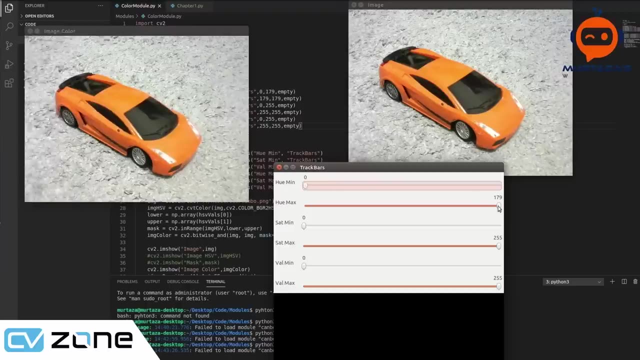 accessible to all. You can also learn to implement computer vision on embedded devices with you using Jet Het, a way to store nothing or any otheromethat doesn't take up much space Nano course: Here you will learn the basics of Jetson, Nano and computer vision, along with creating exciting 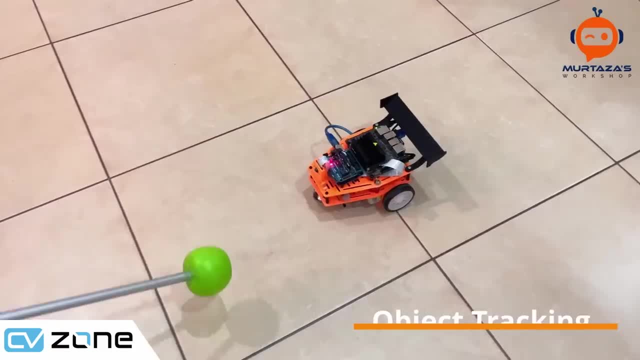 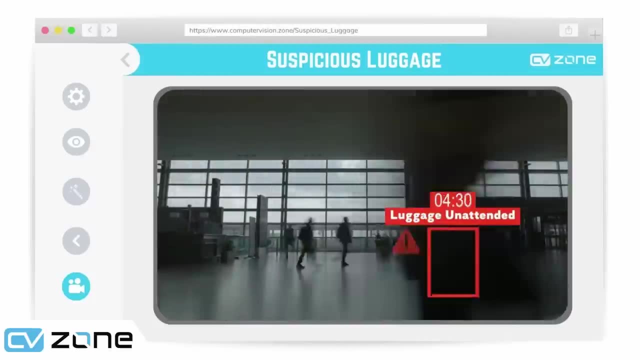 projects like lane following, robot eye tracking, object following and a lot more. All these courses have a clear path from basics to advanced with maximum knowledge in a short amount of time. So check out the links in the description to get started with your computer vision journey. 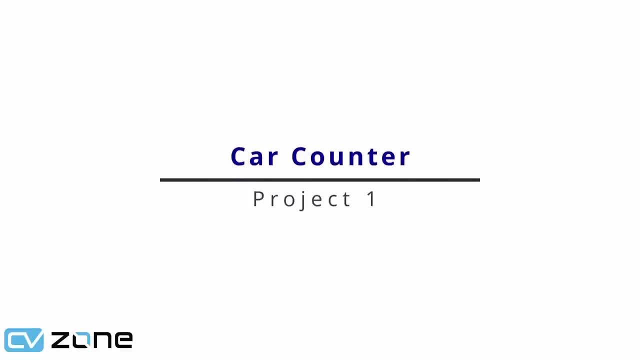 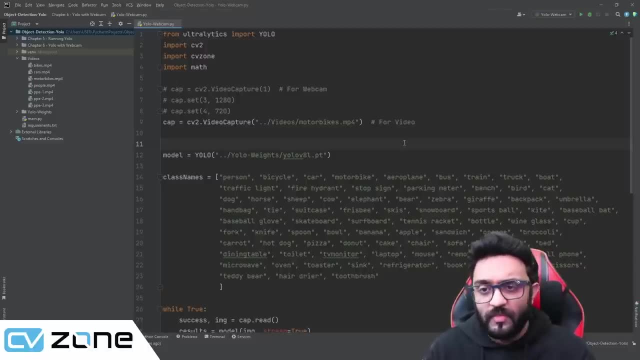 today. So now that we understand how to run YOLO and how can we run using GPU, we are going to create some projects out of this. So the first project that we are going to do is a car counter. So within a video, we are going to count the number of cars that pass a certain region. 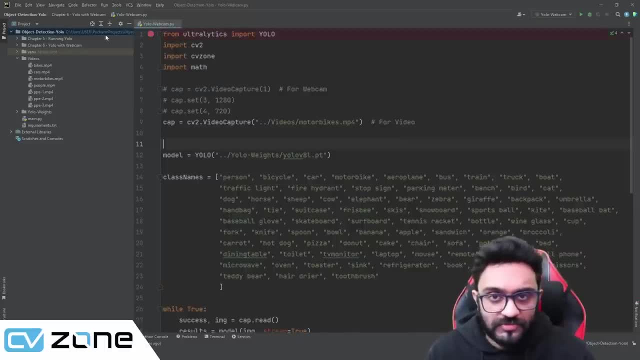 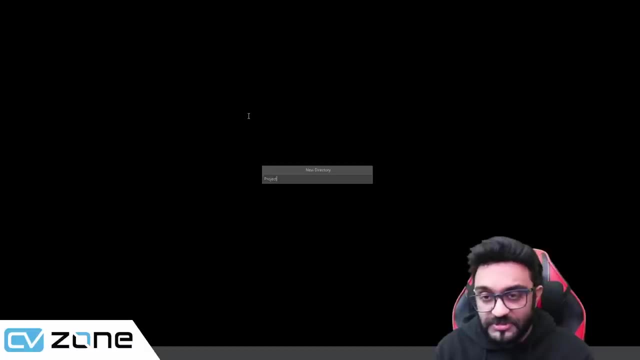 So to do that, we will first create a new folder. we'll go to- Oh, not a new file, we'll go to new and we'll click on directory. And here we are going to write project one and the name of this project. we are going. 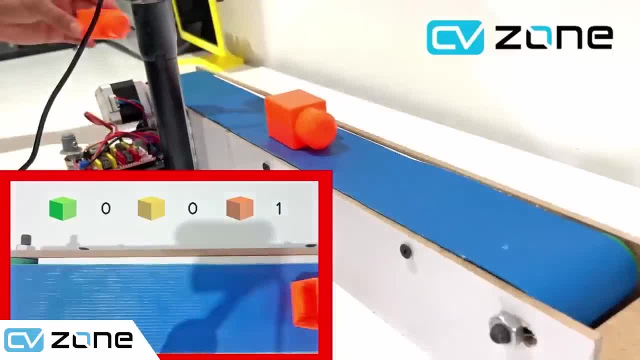 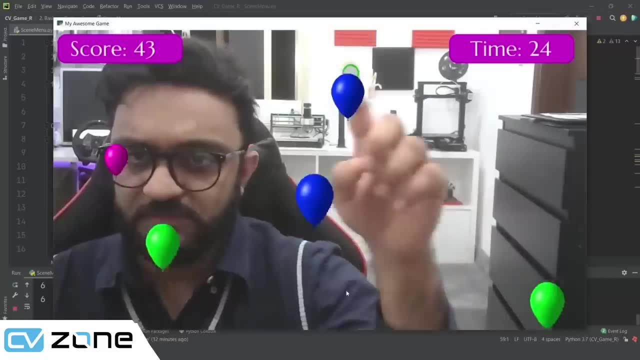 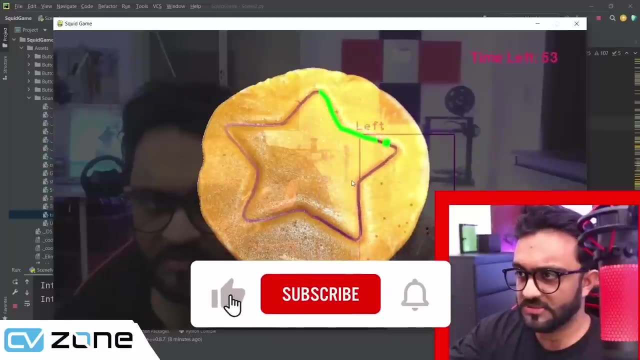 along with amazing projects such as conveyor belt assembly, face tracking, lamp gesture control, face door lock and a lot more. the computer vision game development is another great course where fun meets programming. here you will learn to create games such as fruit ninja, balloon, pop, squid game, cookie cutter, all using the latest computer vision software. so if you want to learn more about computer, 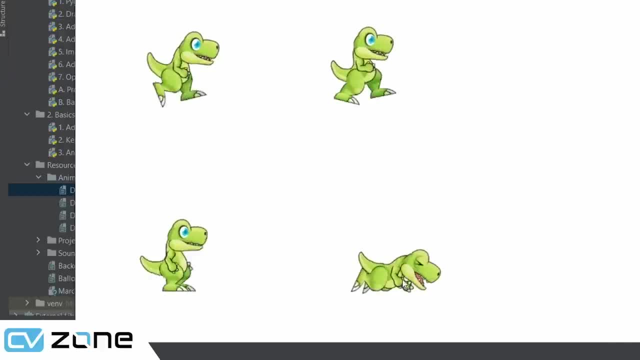 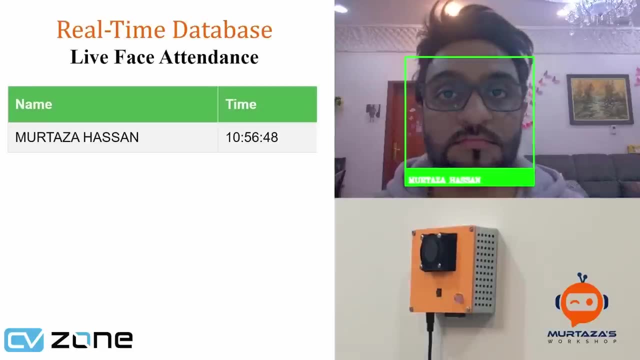 vision techniques. not only that, you will learn to compile your awesome game to an exe file to make it accessible to all. you can also learn to implement computer vision on embedded devices with our computer vision, with jetson nano course. here you will learn the basics of jetson nano and 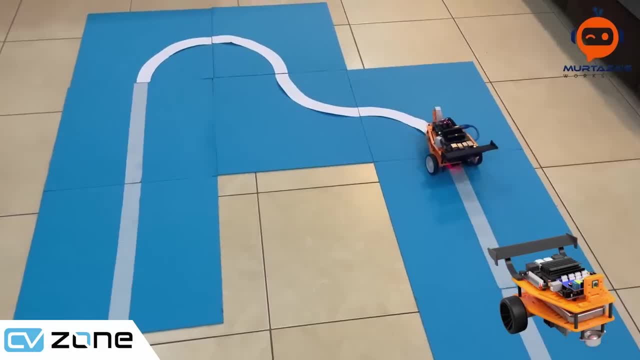 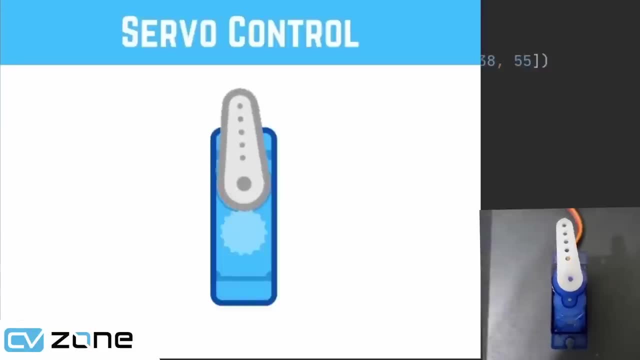 computer vision along with creating exciting projects like lane following, robot eye tracking, object following and a lot more. all these courses have a clear path from basics to advance with maximum knowledge in a short amount of time. so check out the links in the description to get started with your computer vision journey today. 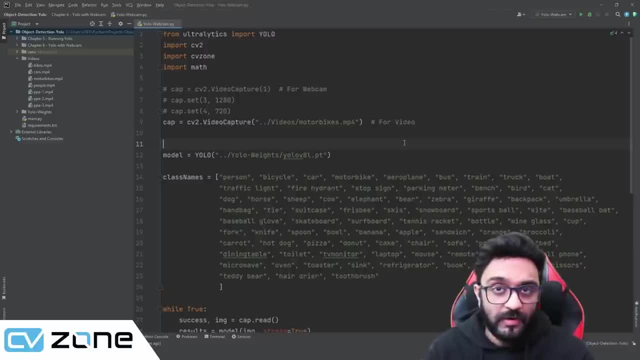 so now that we understand how to run yolo and how can we run using gpu, we are going to create some projects out of this. so the first project that we are going to do is a car counter. so within a video we are going to count the number of cars that pass a certain region. so to do that, we will 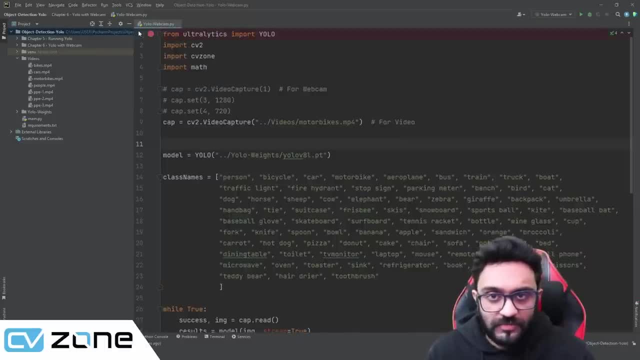 first create a new folder. we'll go to- oh, not a new file. we'll go to new and we'll click on directory and here we are going to write project one and the name of this project. we are going to call it car counter. so within our car counter, we are basically going to copy the code of yolo webcam. so we will copy. 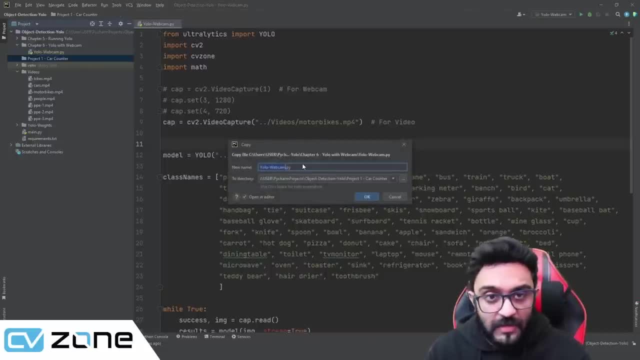 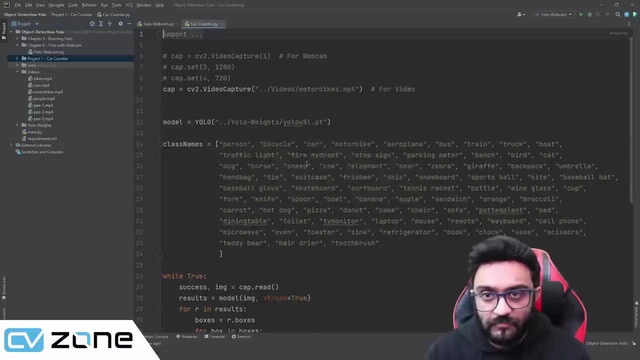 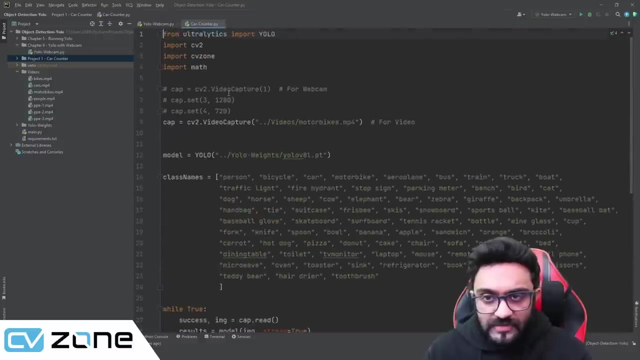 yolo webcam and we are going to paste it in the project project one. so here we will call it car dash. let's write it capital: car dash, counter dot pi. so we will have the exact same code that we were running earlier, and all we have to do is we have: 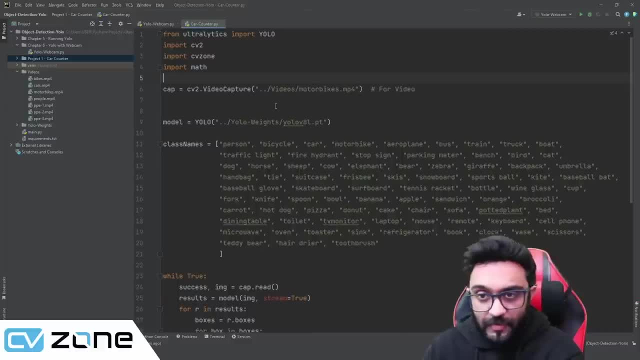 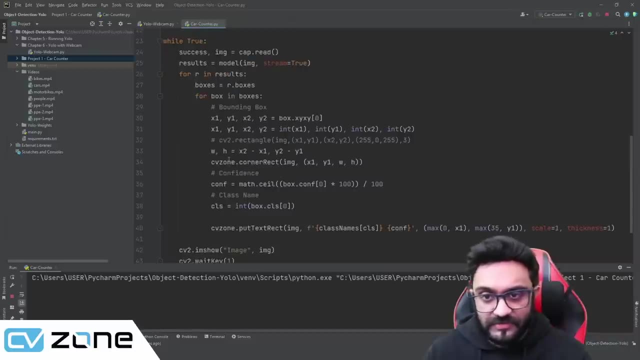 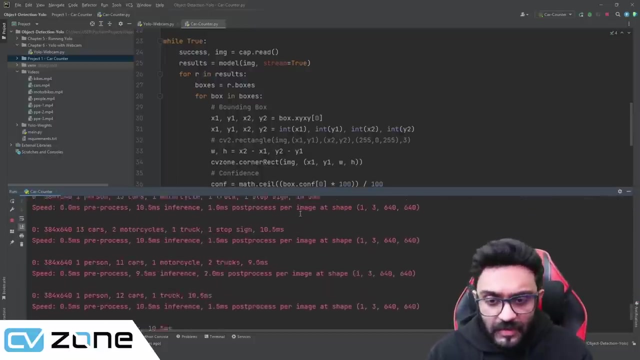 to make sure it's running with the videos, we can remove the webcam part and we are going to run carsmp4. so we will have a lot of things done and set it up already while we start this project. so right now you can see it's running on gpu, it's using 3080 ti and there you go, we are getting. 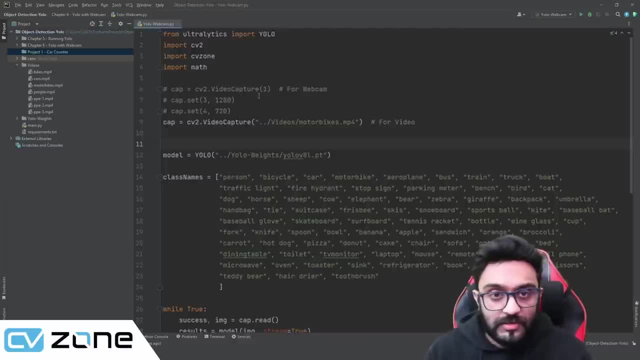 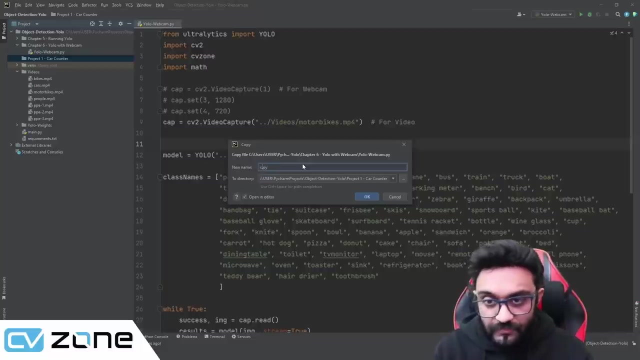 to create. We will call it car counter. So within our car counter we are basically going to copy the code of Yolo webcam. So we will copy Yolo webcam and we are going to place it in the project project one. So here we will call it car dash. 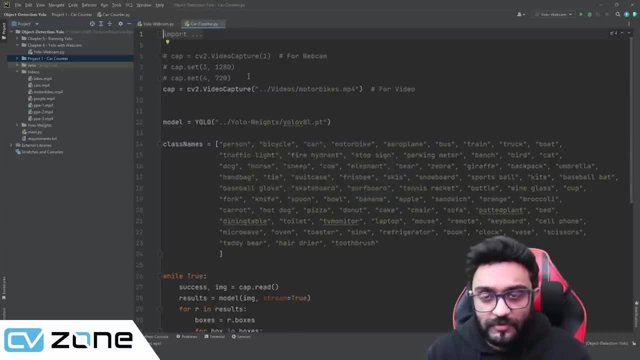 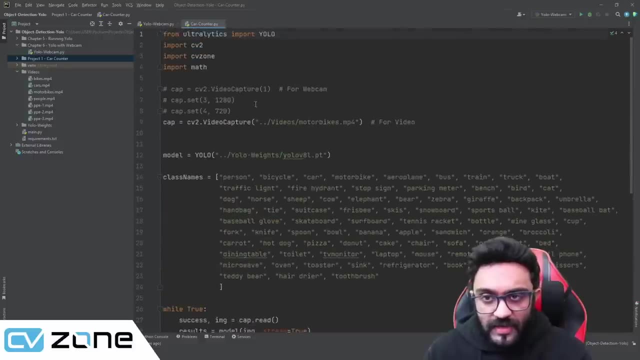 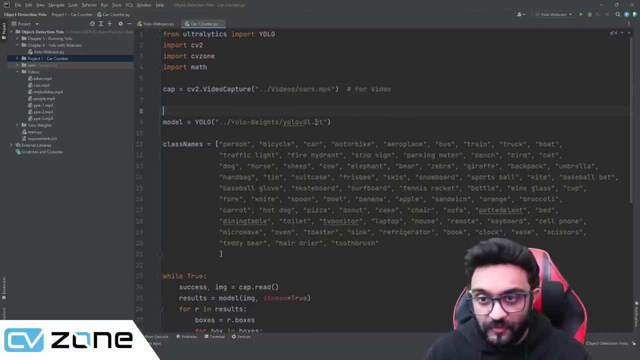 Let's write it capital: car dash counter dot pi. So we will have the exact same code that we were running earlier And all we have to do is we have to make sure it's running. With the videos, we can remove the webcam part and we are going to run cars dot mp4. 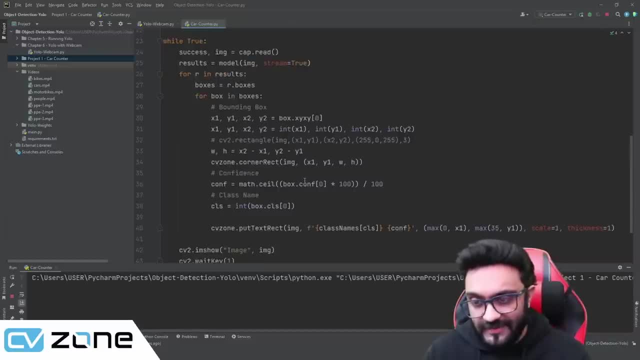 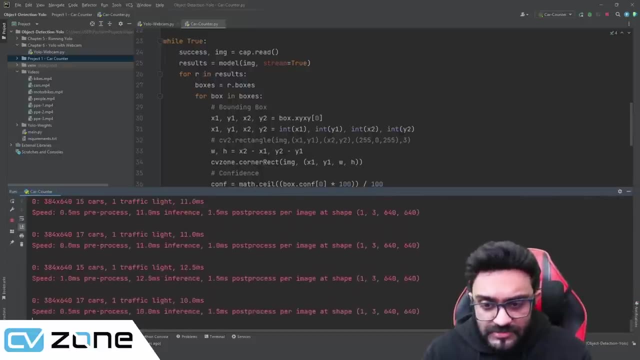 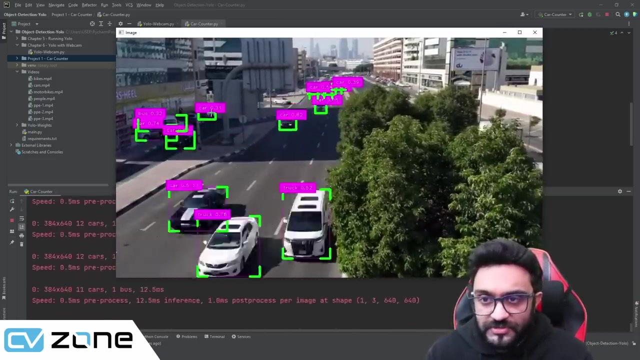 So we will have a lot of things done and set it up already while we start this project. So right now you can see it's running on GPU, It's using 3080 TI And there you go, we are getting the cars and we are getting their bounding box information. 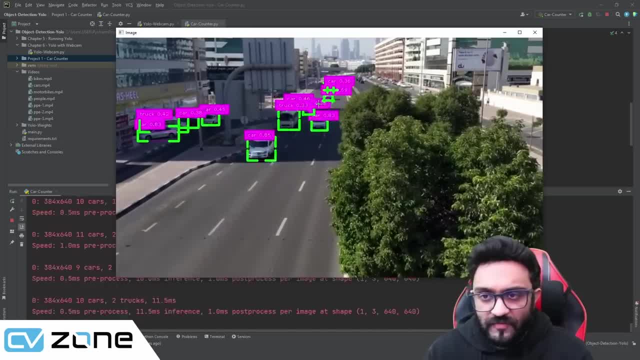 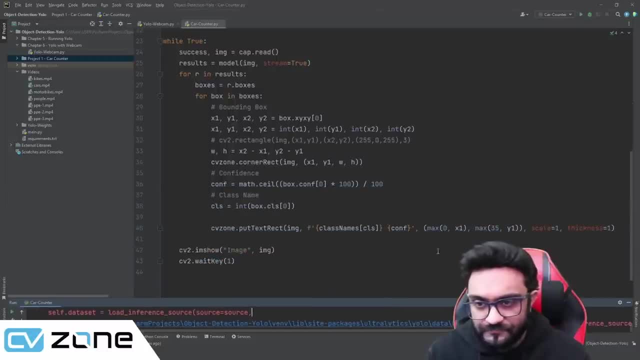 their class, their confidence, and you can see when, when it's too small, it's not actually putting the corner rectangle properly. So what we can do is, first of all, let's fix that. So here, where is it corner rectangle? what we can write is: the length equals, I think. 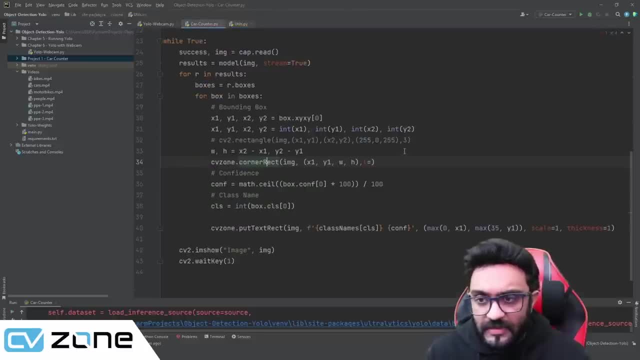 by default, it's 30.. Yeah, it's 30 by default. Let's put it at 15.. So this is the length of the corner, So the green part that you see, that is what we are referring to, So we can make it smaller. 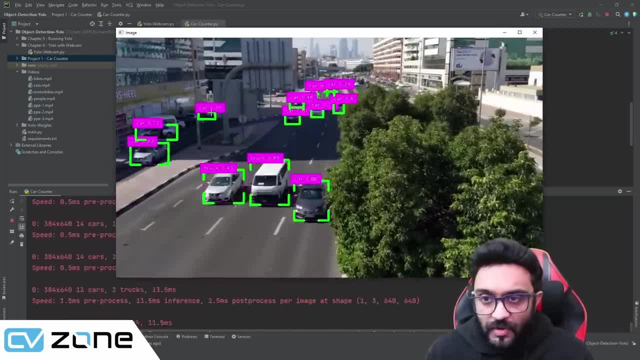 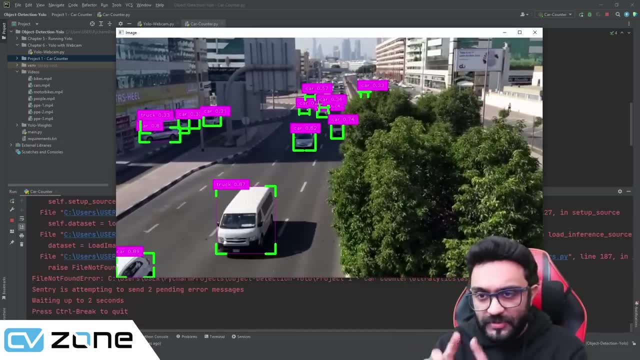 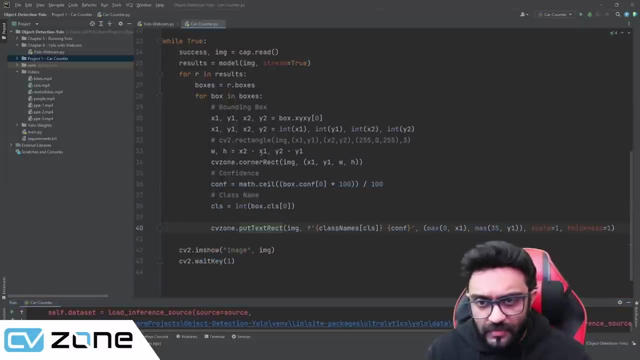 the cars and we are getting there bounding box information, their class, their confidence, and you can see, uh, when, when it's too small, it's not actually putting the corner rectangle properly. so what we can do is, first of all, let's fix that. so here, uh, where is it corner rectangle? uh, what we can write is the. 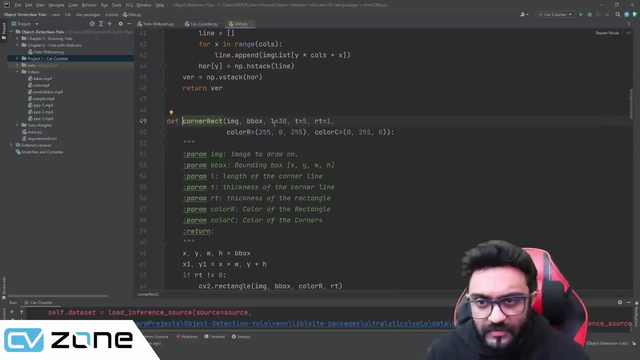 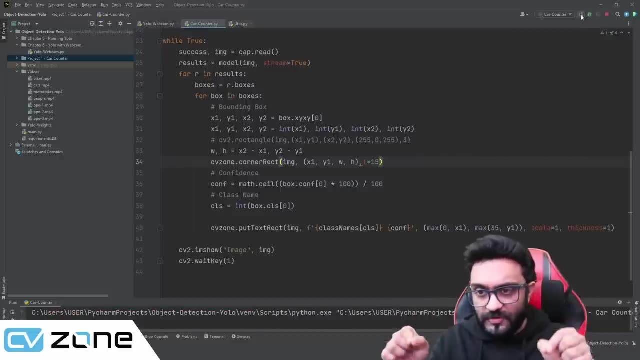 length equals, i think by default it's 30. yeah, it's 30 by default. let's put it at 15.. so this is the length of the corner. so the green part that you see, that is what we are referring to, so we can make it smaller. yeah, so there you go now. 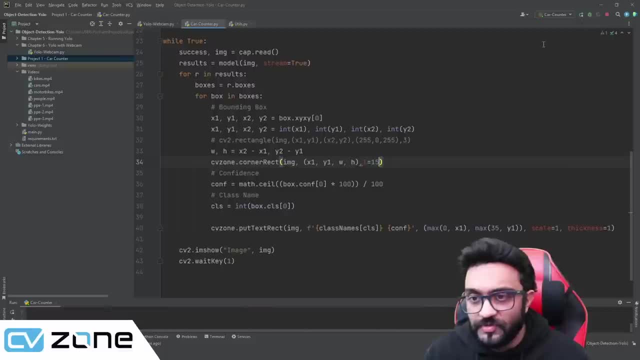 it's smaller. so the green part, and if you wanted to, you can even reduce it further. you can make it, let's say five, then it will be really small. uh, let's see how that works out. there you go: um, it's too small, maybe eight or nine. let's say: 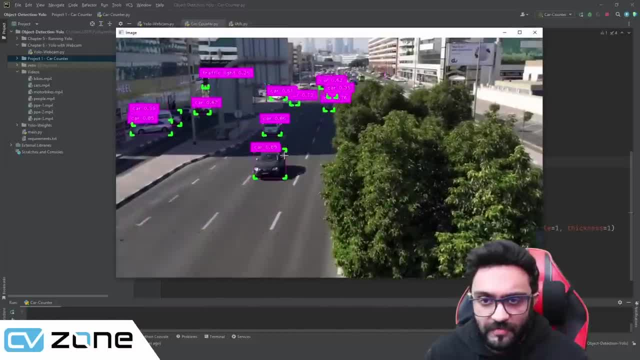 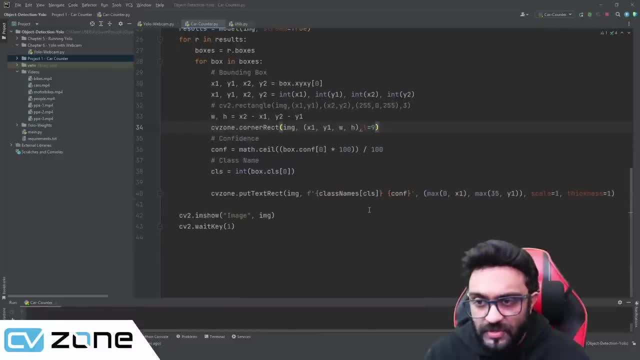 maybe five. okay, so how about that? yeah, you can do a little bit of the same. there you go. i think this is better, okay, so we have the cars coming in, we have the rectangle on top of it. we can actually make it smaller, so that, uh, we can see it better. so let's make it 0.3, or let's say 0.6. 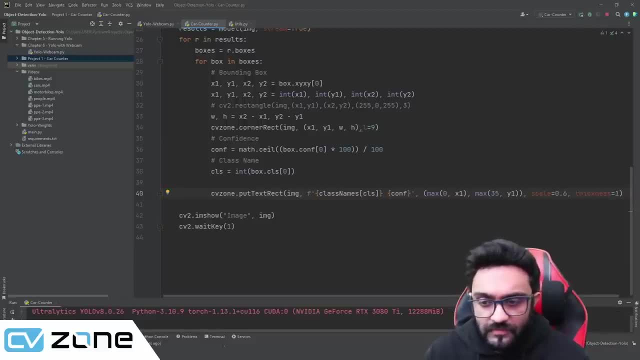 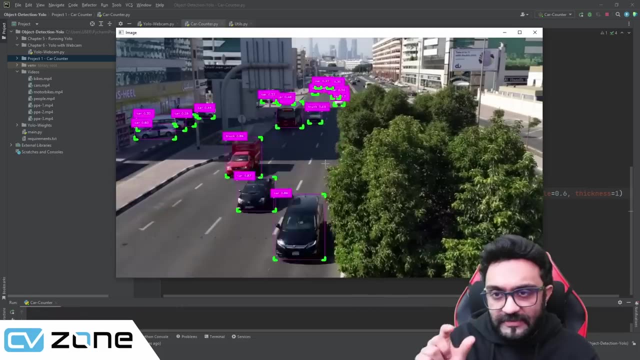 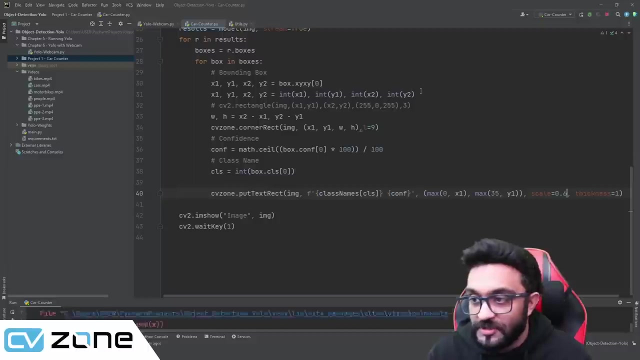 and the thickness is still one- we cannot reduce it further, i believe- so smaller, but you can see the, the, the title itself is smaller, but there is some offset around the region which is quite huge, so we can reduce that too. so there is a very there's a variable called 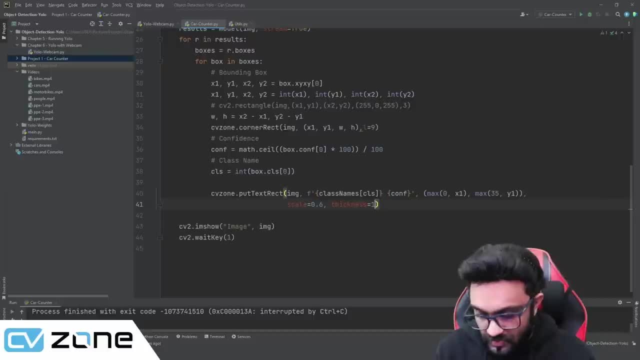 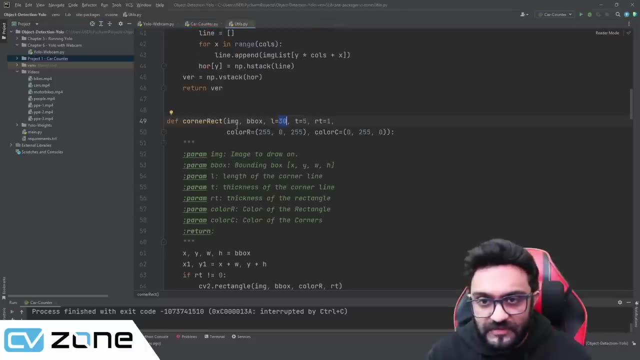 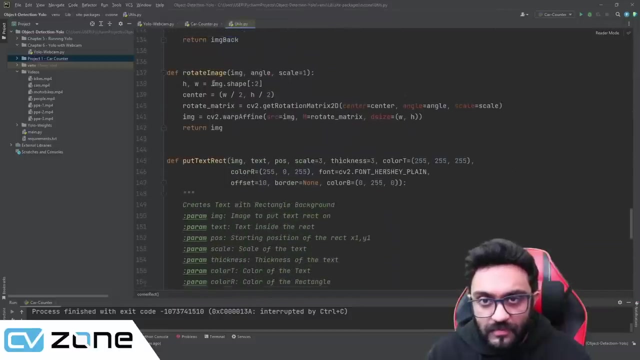 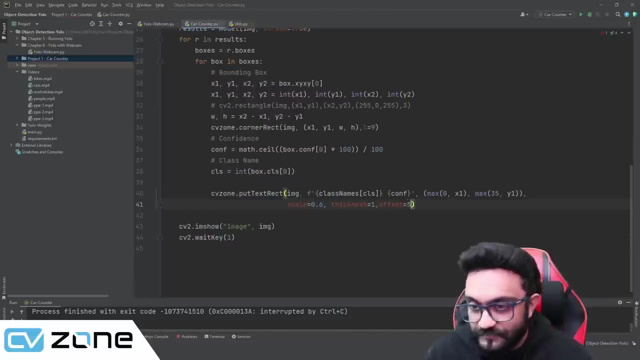 offset. uh called offset and by default, i believe it's 15.. do we have an offset here? no, the bounding box. um, yeah, put text correct. we have offset as 10.. so let's make it five or let's put it three, because we don't want a huge offset. we want the cars to be visible. 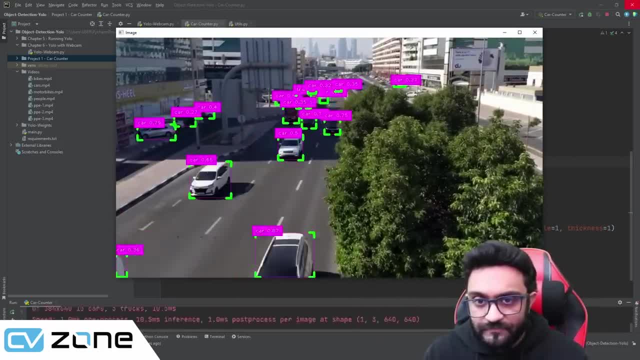 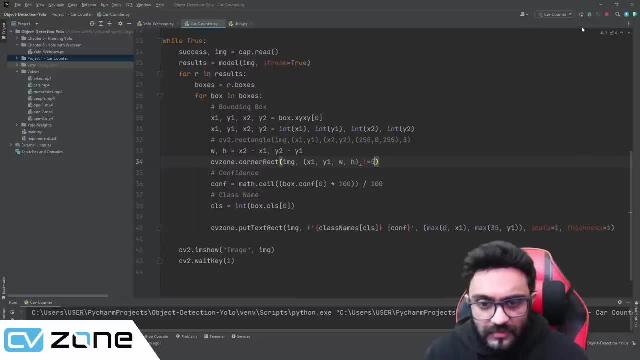 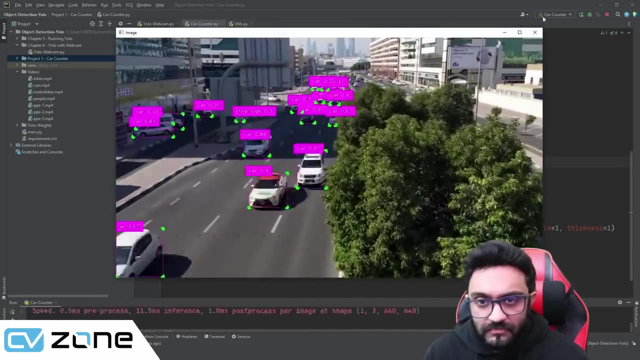 Yeah, so there you go. Now it's smaller And if you wanted to, you can even reduce it further. you can make it, let's say, five. then it will be really small. Let's see how that works out. There you go. 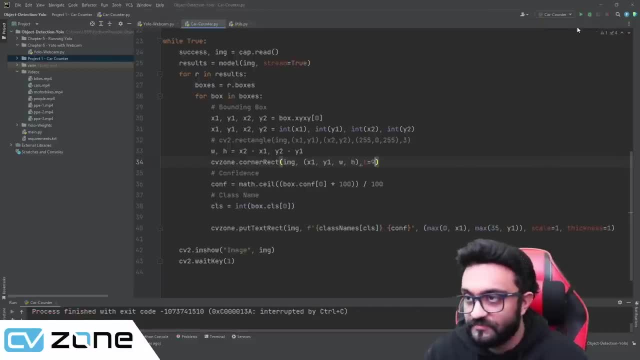 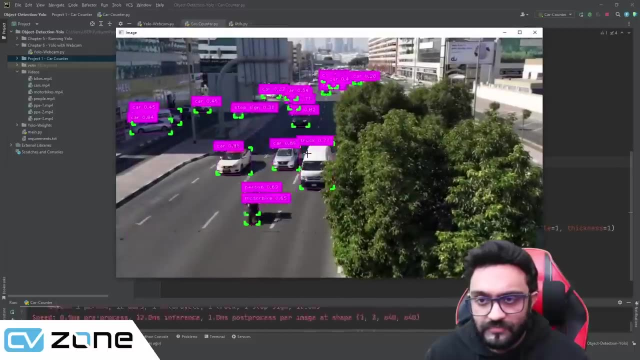 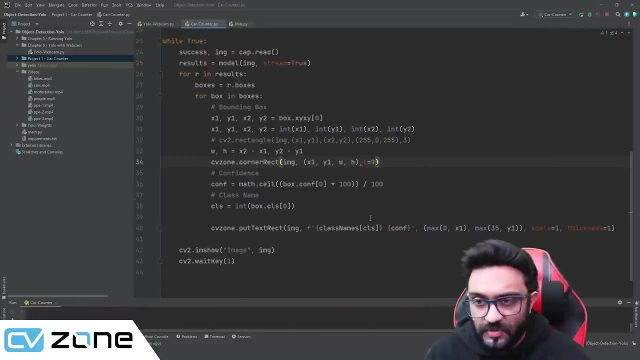 It's too small, maybe eight or nine, let's say: there you go. I think this is better. Okay, so we have the cars coming in, We have the rectangle on top of it. we can actually make it smaller so that we can see. 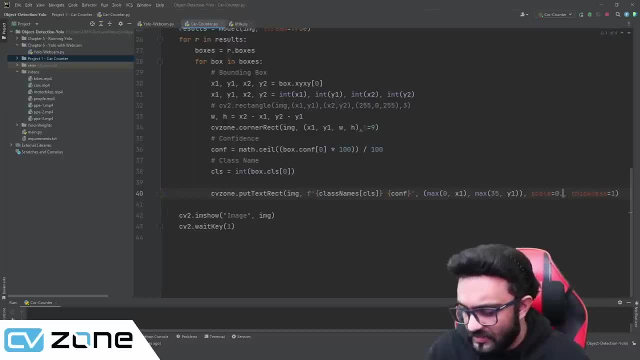 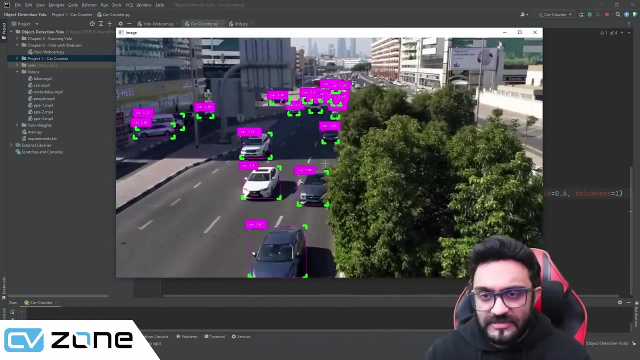 it better. So let's make it 0.3.. Or let's say 0.6.. And the thickness is still one cannot reduce it further, I believe. So there we have it. Now we have it smaller, But you can see the. the. the title itself is smaller, but there is some offset around the. 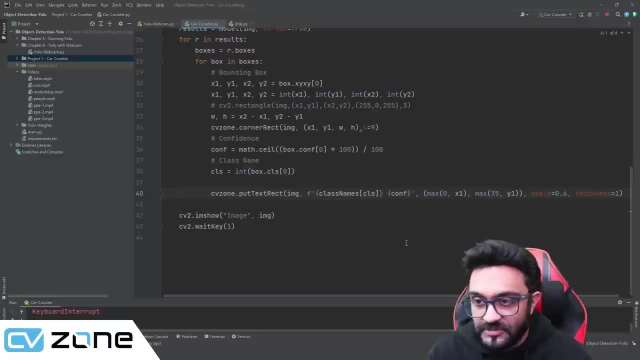 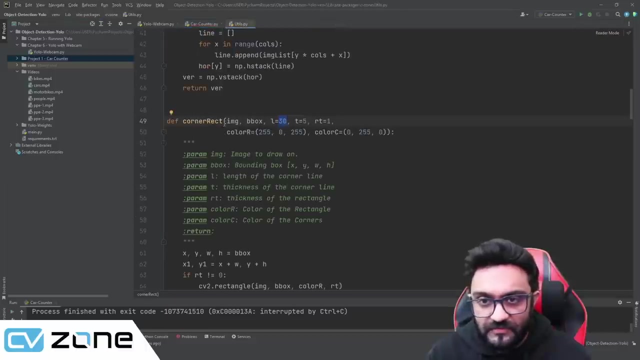 region, Which is quite huge, So we can reduce that too. So there is a very there's a variable called offset, called offset, And by default I believe it's 15.. Do we have an offset here? No, the bounding box. 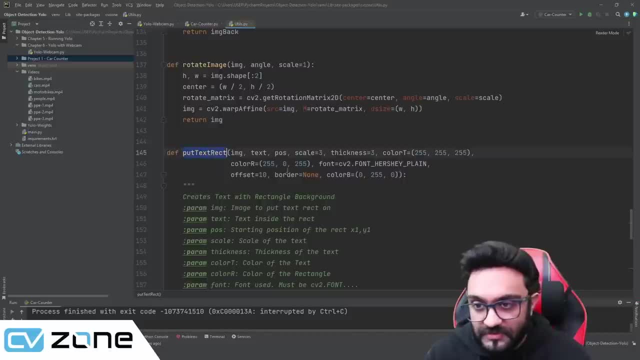 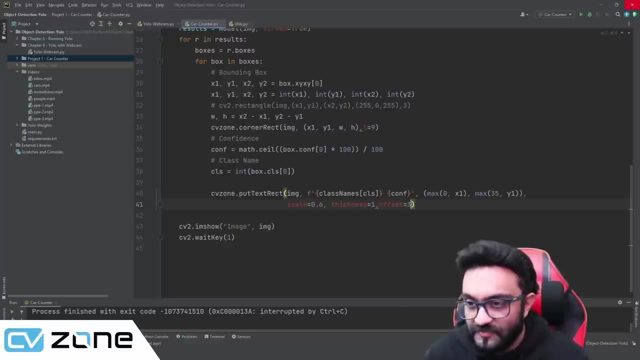 Yeah, put text right. we have offset as 10.. So let's make it five Or let's put it three, because we don't want a huge offset. we want the cars to be visible. There you go. So now it's much better. 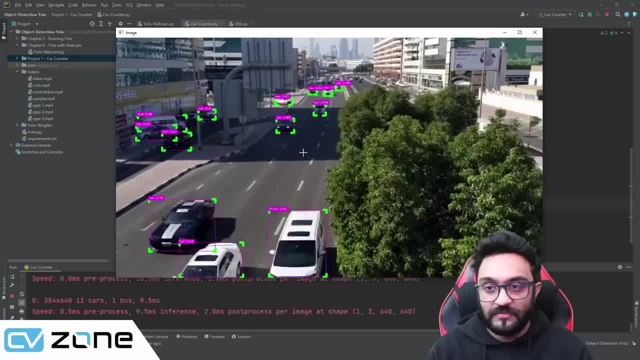 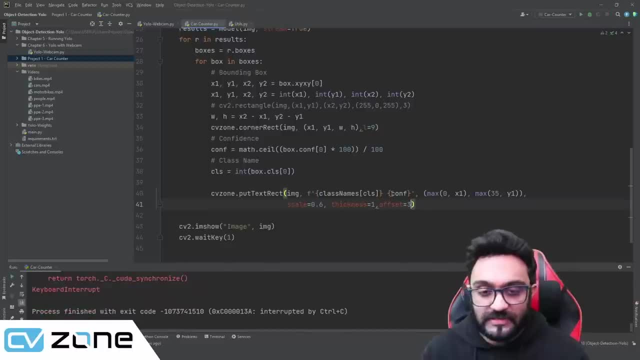 You can see, we have the offset and we can see the cars coming in. Looks good, Okay, so this is the basic idea: that we have these cars coming in. Now the thing is that it might not be a car, it might be a truck, but then what exactly? 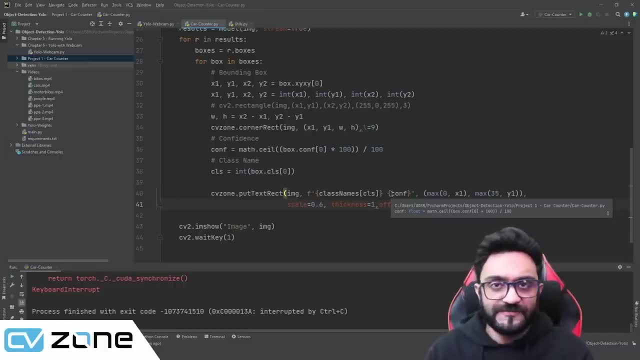 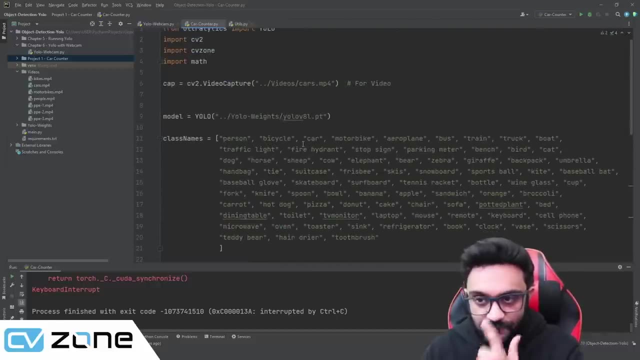 are we trying to find. So if you just want to do cars, you can add a if statement that if it's a car, then detect it. Otherwise we can find out what are the vehicles that we want to find. For example, in our case, let's say we will detect the car, will detect motorbike will. 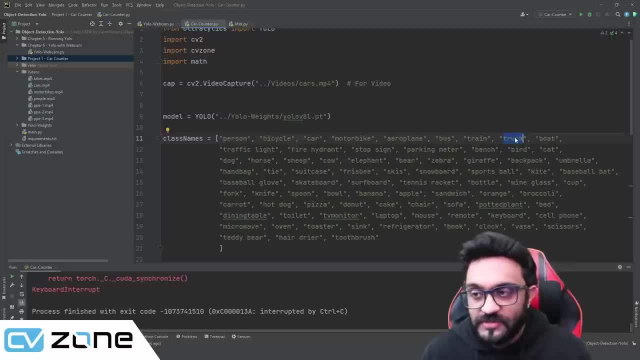 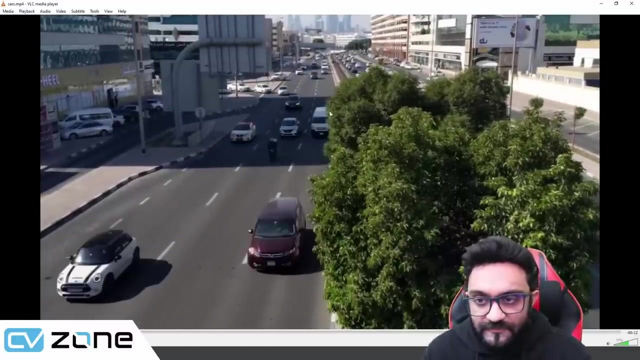 detect bus and then we will detect truck. So these are the four categories that we are going to detect. So if we go to our cars video- let's open that up- There you go. So if we go a little bit back, there you go. I believe this will be detected as a truck. 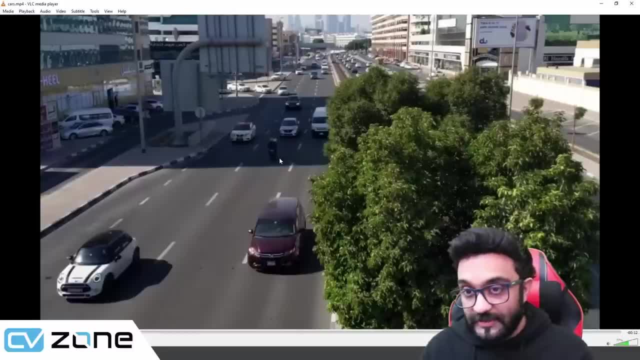 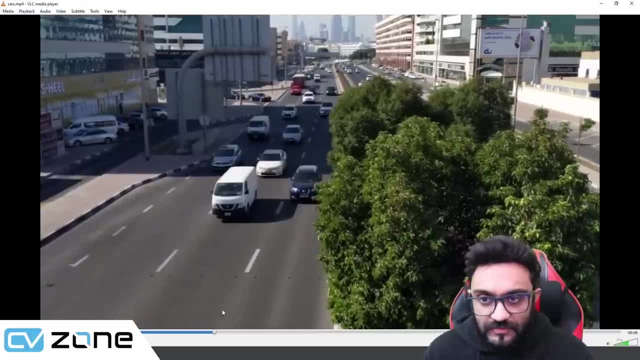 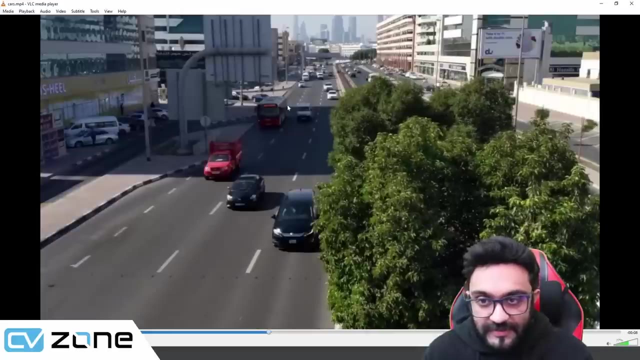 This is a car, that's fine. This is a motorbike, So we want to detect that too, And then later on we also have. Yeah, I believe this will be detected as truck as well, And this should be detected as a bus. 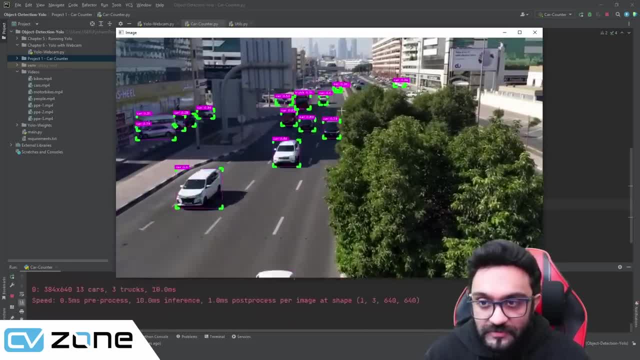 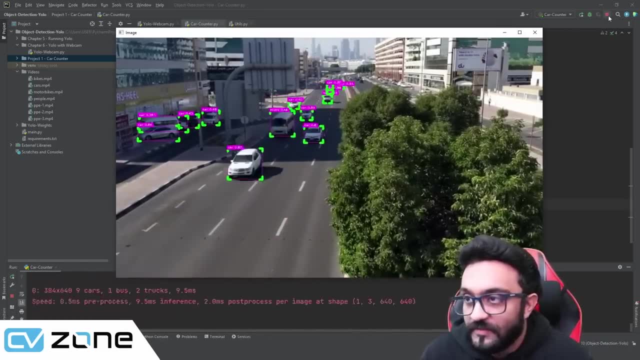 there you go. so now it's much better. you can see we have the offset and we can see a little bit that there is that offset from um thequez. as you can see, the cars coming in looks good, okay. so this is the basic idea: that we have these cars coming in. 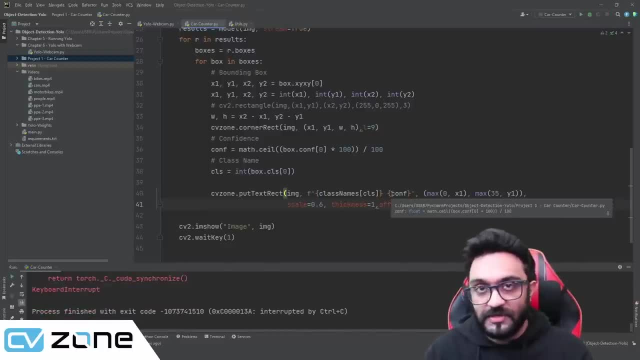 now, the thing is that it might not be a car, it might be a truck, but then what exactly are we trying to find? so if you just want to do cars, you can add a if statement that if it's a car, then detect it. otherwise we can find out what are the vehicles that we want to find. for example, 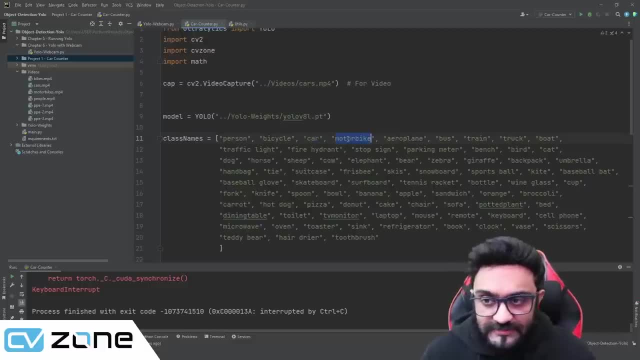 in our case, let's say we will detect the car, we'll detect motorbike, we'll detect bus and then we will detect truck. so these are the four categories that we are going to detect. so if we go to our cars video, let's open that up. 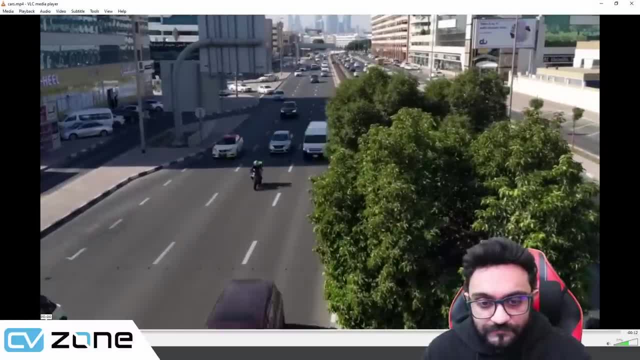 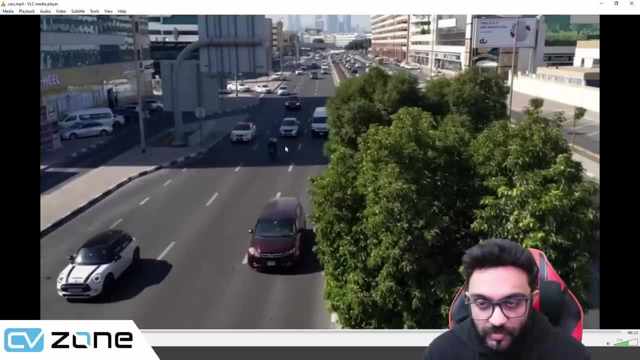 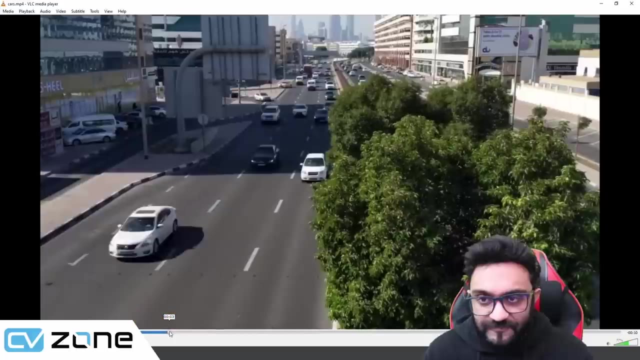 there you go. so if you go a little bit back, there you go. i believe this will be detected as a truck. this is a car, that's fine. this is a motorbike, so we want to detect that too, and then later on we also have. uh yeah, i believe this will be detected as truck as well. 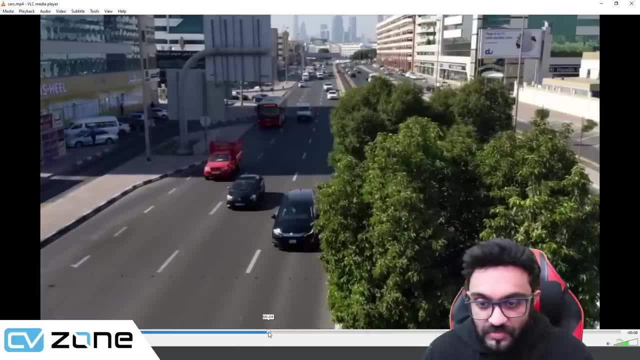 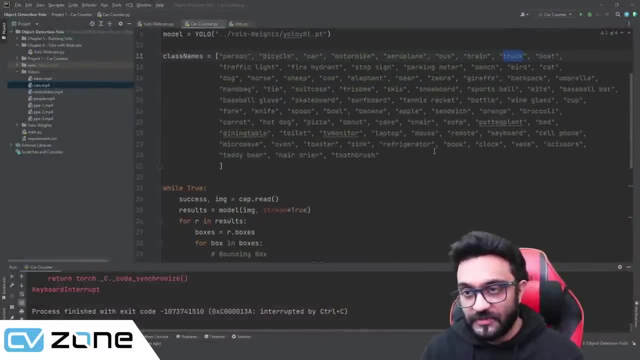 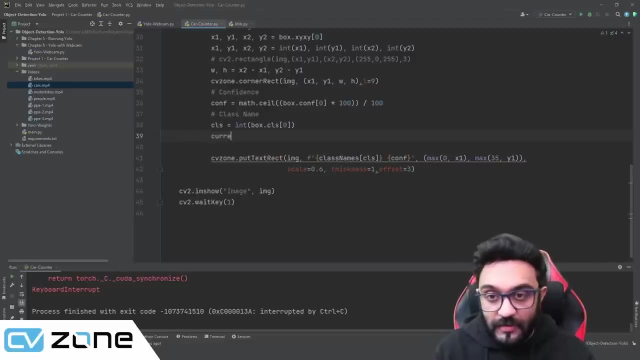 and this should be detected as a bus. so we have these different categories and we want to detect all of them. so in that case, first of all, we have to give an if statement that only detect these categories. so here what we can do is we can write here: current class. 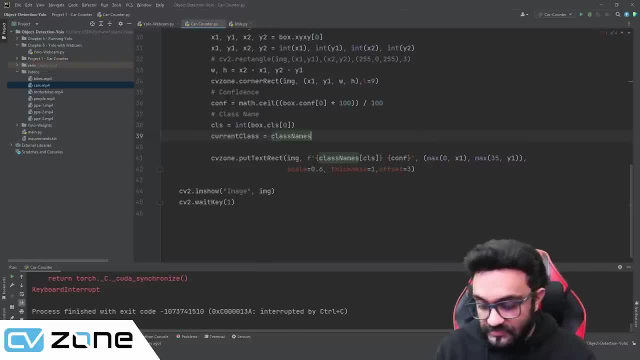 equals uh class names at cls, so this will give us the class name. so over here as well, instead of writing this, we can write current class. and over here we can write: if the current class equals car, then only we are going to display it. so in case of motorbike and in case of the truck it will not get detected and what we can do is 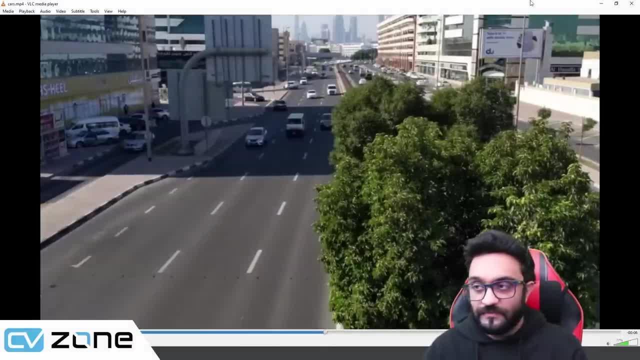 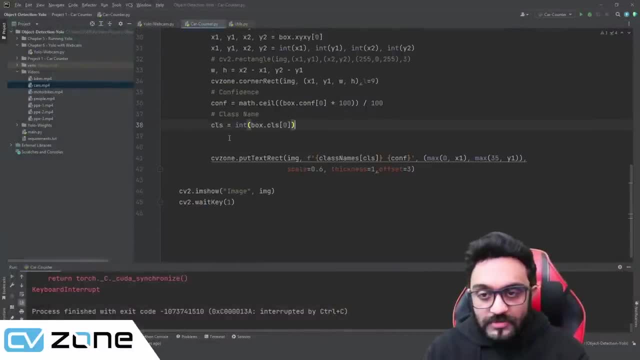 So we have these different categories and we want to detect all of them. So in that case, we want to detect all of them, Okay, So first of all we have to give an if statement that only detect these categories. So here what we can do is we can write here: current class equals class names at CLS. 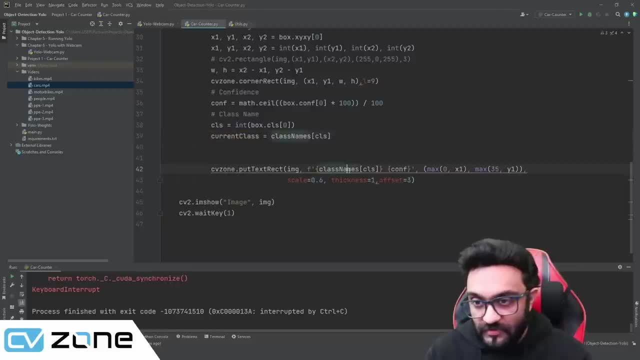 So this will give us the class name. So over here as well, instead of writing this, we can write current class, And over here we can write: if the current class Equals car, then only we are going to display it. So in case of motorbike and in case of the truck it will not get detected. 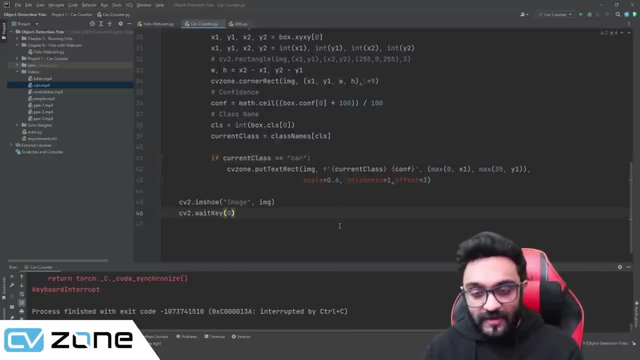 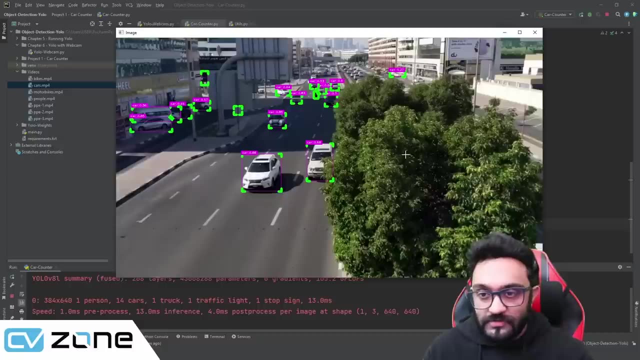 And what we can do is we can put a zero here. So every time we press the keyboard button it will go forward. Otherwise it will not go forward by its own. So there you go, Let's. I will keep pressing, Okay. 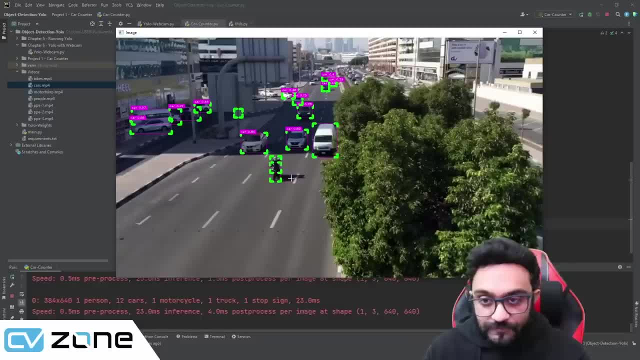 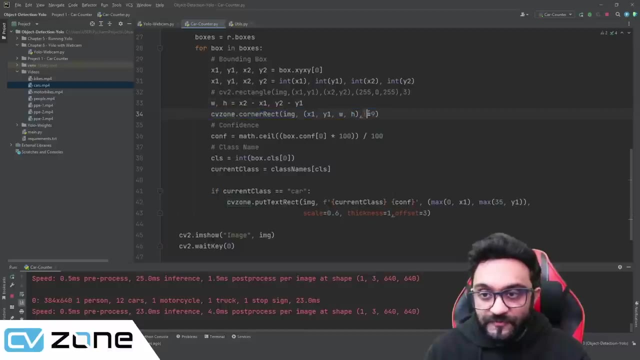 And let's move forward. And here you can see it is detecting it, but it is not displaying the confidence and the class value over here as well. It's not because we are displaying the rectangle. The rectangle is displayed here. The rectangle is. if you wanted to remove that as well, we can do that. 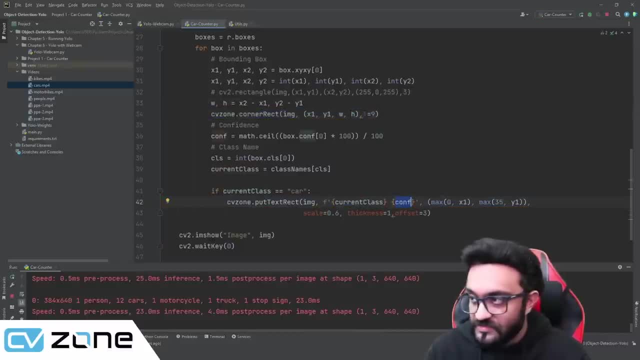 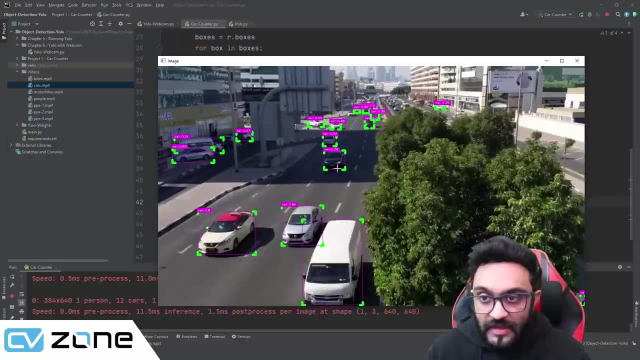 But right now it is not displaying the confidence and the class values. So that is what we are trying to do. So here it's not detecting it. So it means the motorbike is not being detected. And then here the truck, as I mentioned, it's not being detected. 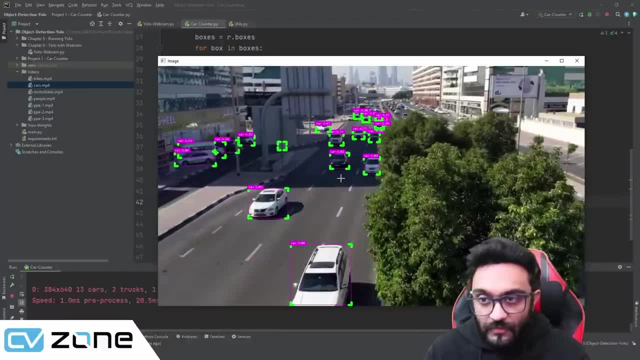 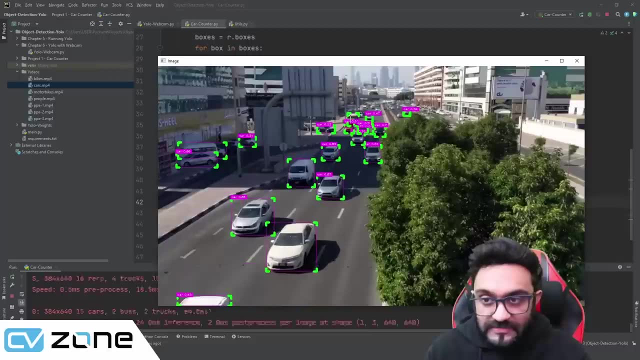 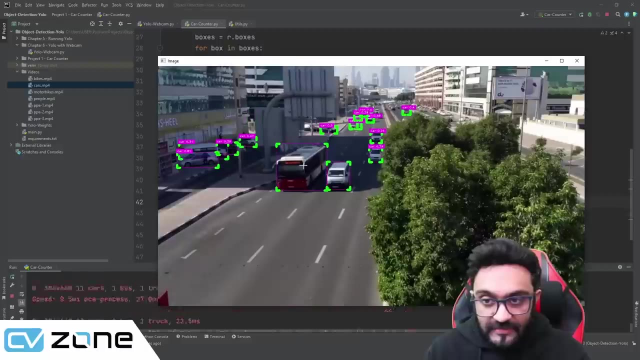 Then let's move on to the bus. So, as you can see, the bus is detected here. You can see it is detected, but it is not classifying it, because we said that only when it's a car. So this is a bus and this is a truck. 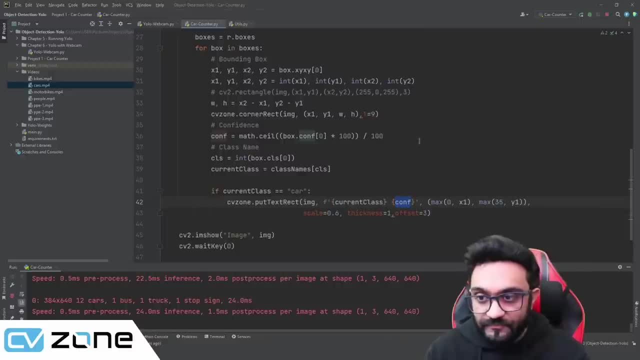 It's not detecting these two because we did not classify it, We did not define them. So here we can see and we can also put the confidence level. So if the confidence level is very low, then you should not display. So here we can write: and confidence is greater than at least 0.3.. 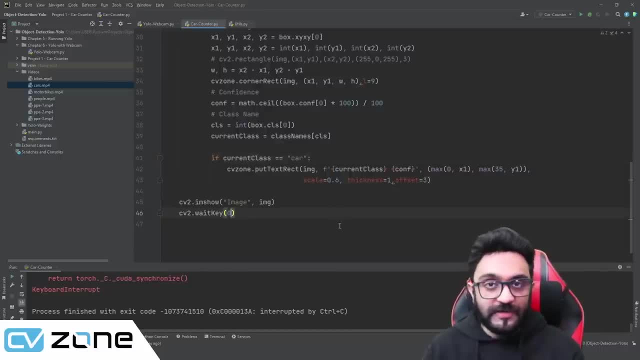 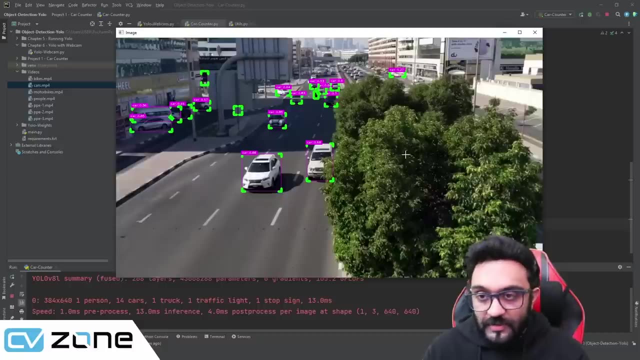 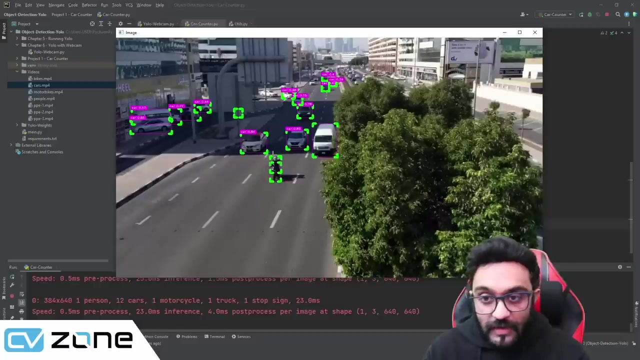 we can put a zero here. so every time we press the keyboard button it will go forward, otherwise it will not go forward by its own. so there you go, let's- I will keep pressing and let's move forward. and here you can see, it is detecting it, but it is not displaying the confidence and the class. 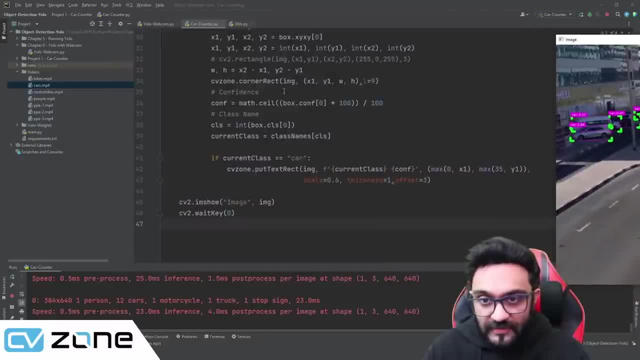 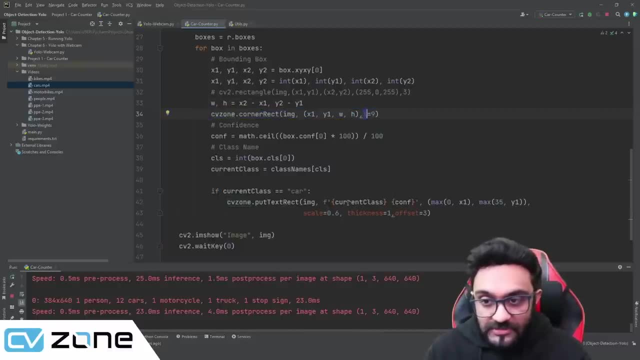 value over here as well. it's not as because we are displaying the rectangle. the rectangle is displayed here, the rectangle is. if you wanted to remove that as well, we can do that, but right now it is not displaying the confidence and the class values. so that is what we are trying to do, so here. 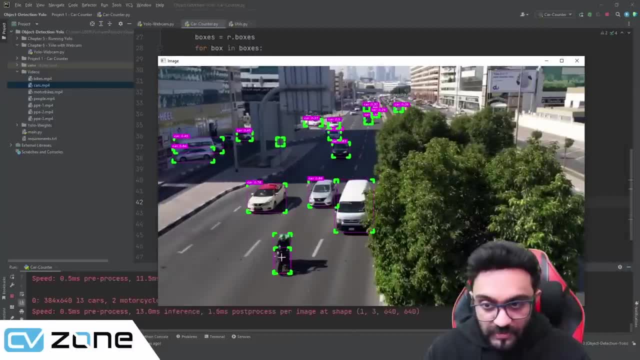 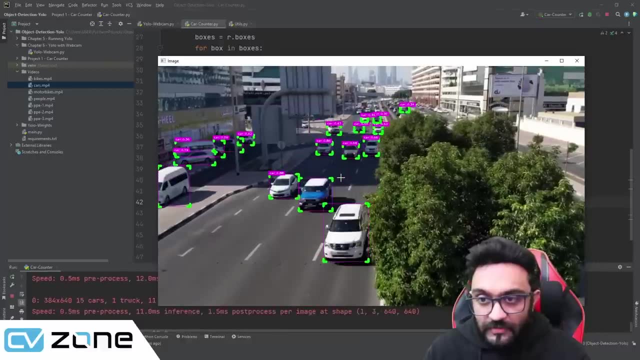 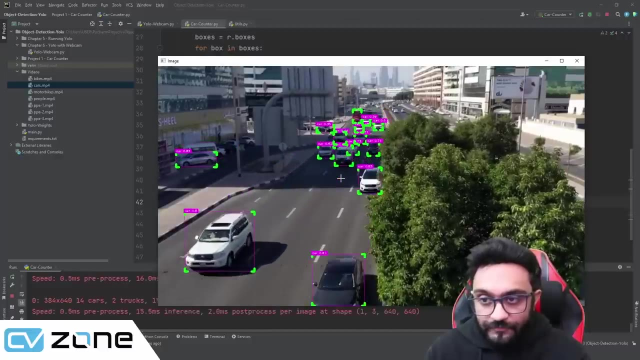 it's not detecting it. so it means the motorbike is not being detected. and then, here we are, the truck, as I mentioned, it's not being detected. then let's move on to the bus. so, as you can see, the bus is detected. here, you can see it is detected, but it is not. 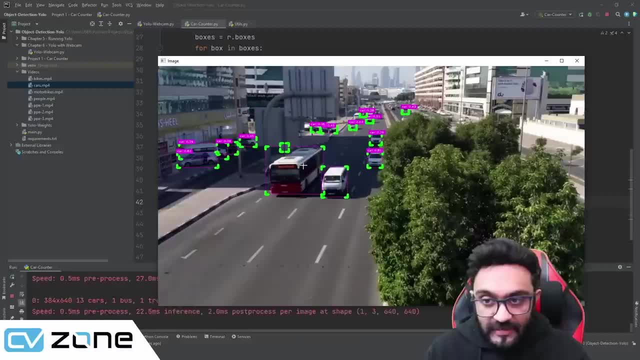 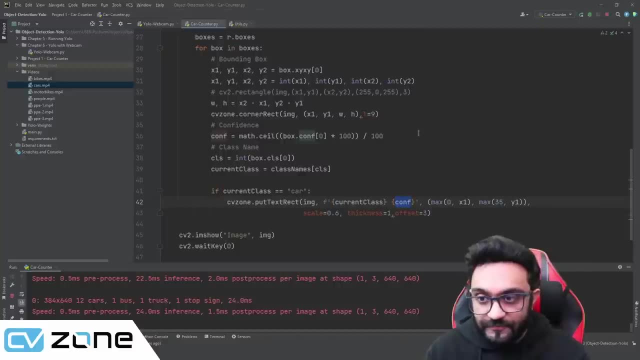 classifying it because we said that only when it's a car. so this is a bus and this is a truck. it's not detecting these two because we did not clarify, we did not define them. so we are not going to define the bus, because we are not going to define the vehicle, because we 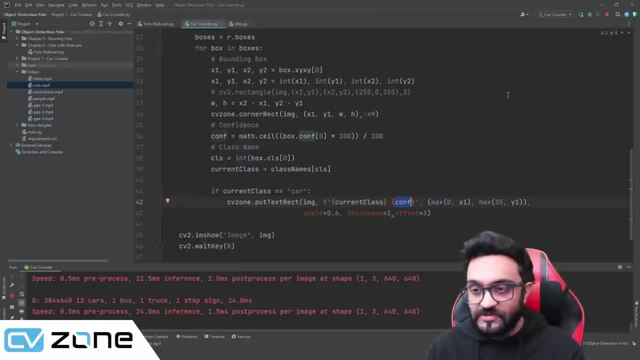 so here we can say, and we can also put the confidence level: so if the confidence level is very low, then you should not display. so here we can write: and confidence is greater than at least 0.3. so that's what we are writing here, that if the confidence is greater than 0.3, and it's a 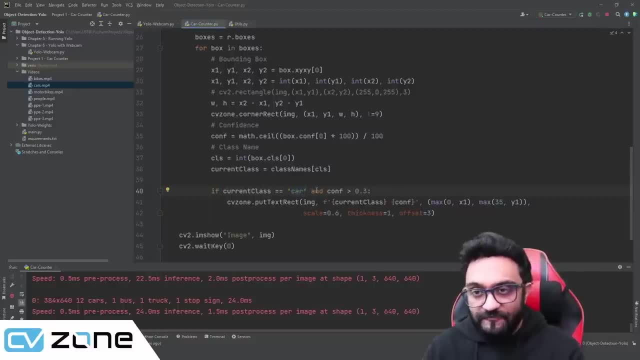 car, then only you can detect it. so we have four categories, so we will write for all four of them. so we'll write here: it's a car, or it's a truck, uh, or it's a bus, or uh, it's a motorbike. so let's go down. or it's a motorbike. 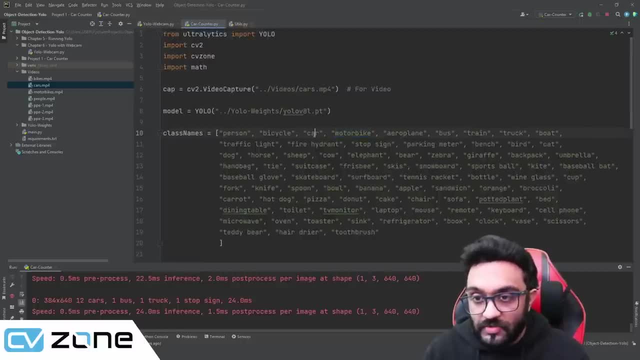 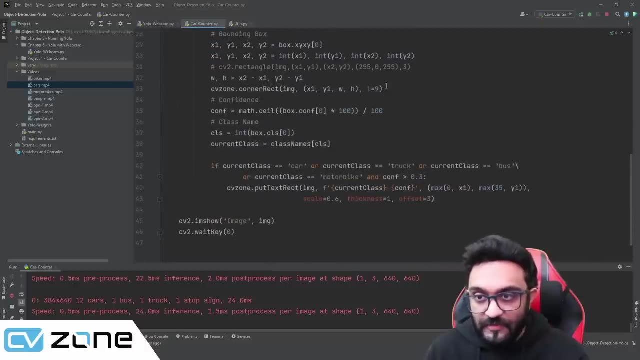 we have motorbike, right, we have motorbike. so car, motorbike, uh, bus and truck. so these are the ones that we're detecting. rest of them we will not detect and we will not even put the rectangle around them. so we can bring it down here in the if statement and we can paste it here. so 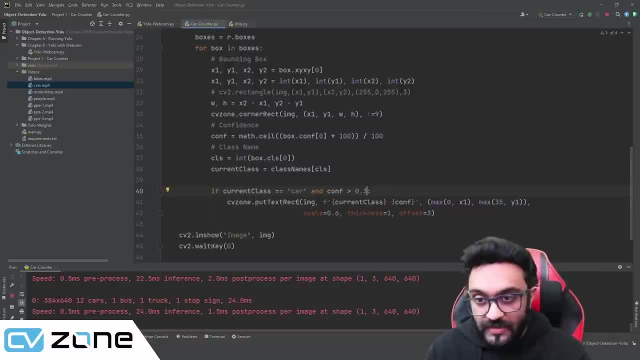 So that's what we are writing here: that if the confidence is greater than 0.3 and it's a car, then only you can detect it. So we have four categories, So we will write for all four of them. So we'll write here: 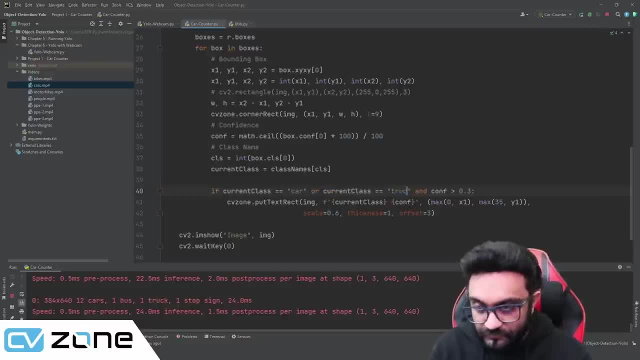 It's a car, Or it's a truck, Or it's a bus, Or it's a motorbike, So let's go down. Or it's a motorbike, We have motorbike, right? Yeah, we have motorbike. 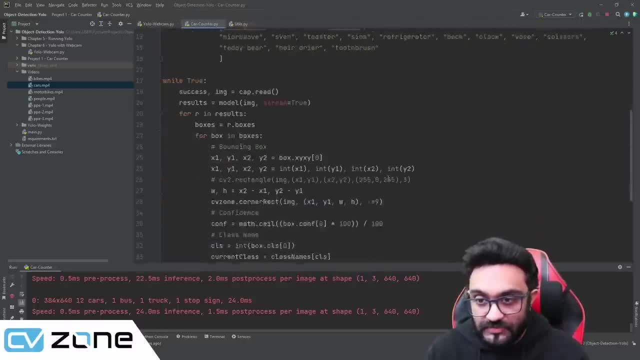 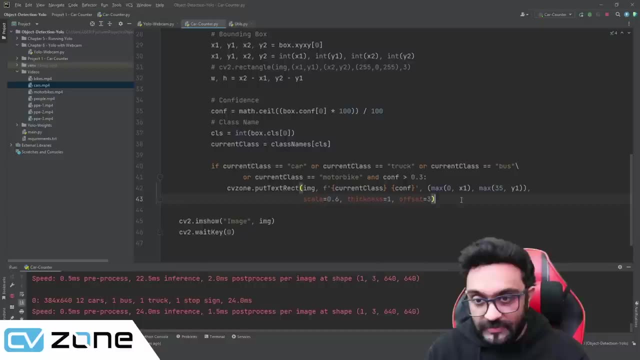 So car, motorbike, Bus and truck. So these are the ones that we're detecting. Rest of them we will not detect and we will not even put the rectangle around them. So we can bring it down here in the if statement and we can paste it here: 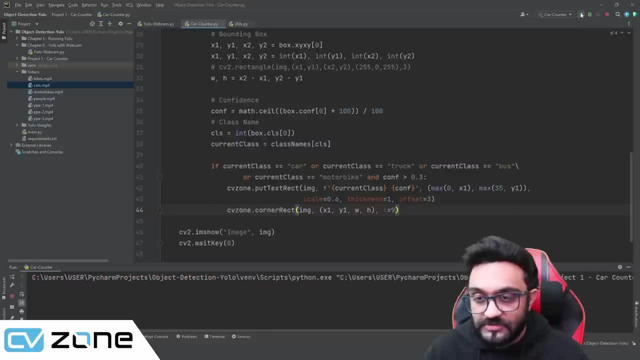 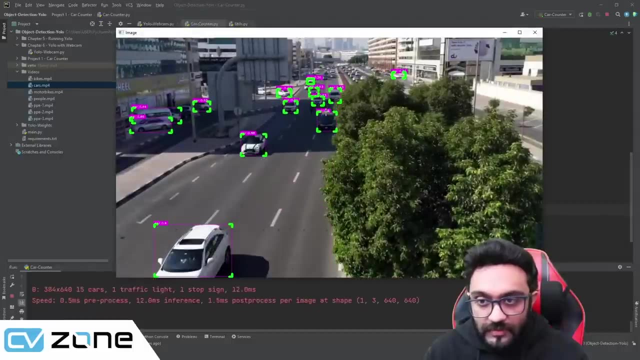 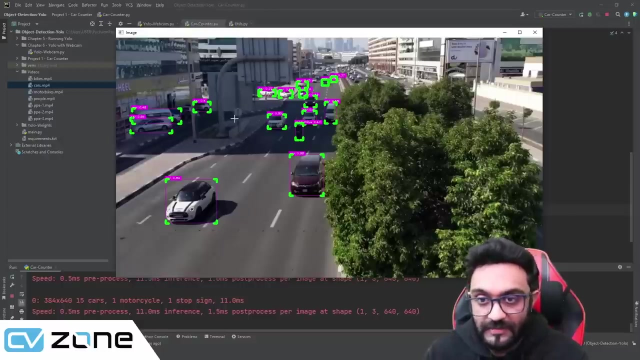 So let's run it and see how it works. So now it will detect only those. So here you can see it was detecting something here. It was detecting probably a traffic sign, but now it's not detecting that because it's not part of it. 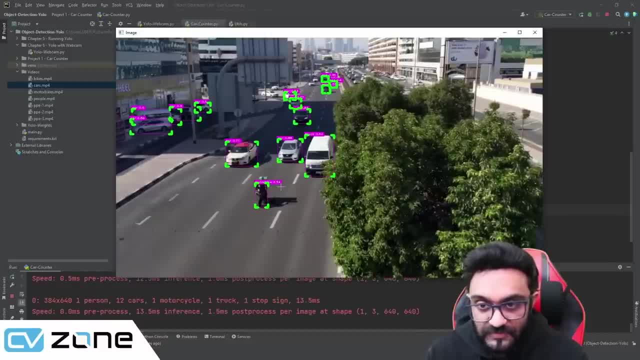 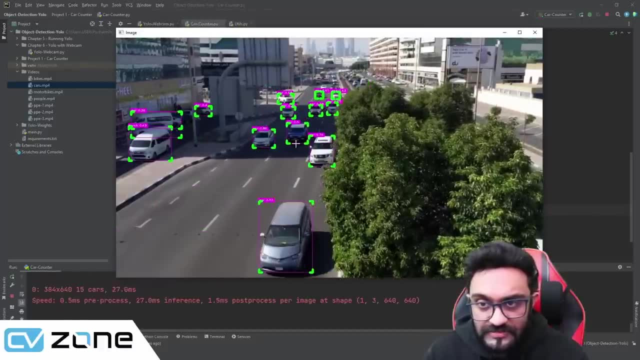 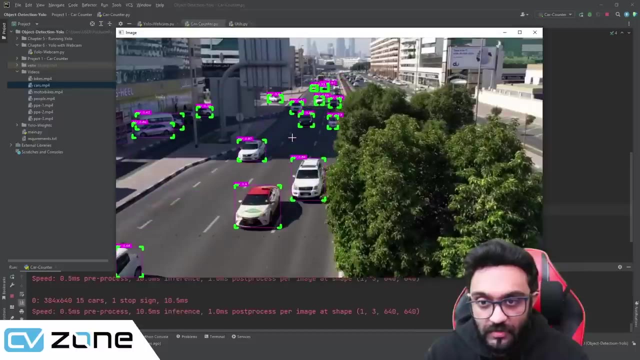 And here you can see it says motorbike at 0.56 or 59% confidence. So 59% confidence. So here you can see car: This is detected as a truck. This is also detected as a truck. So then we'll move forward and we wait for the bus. 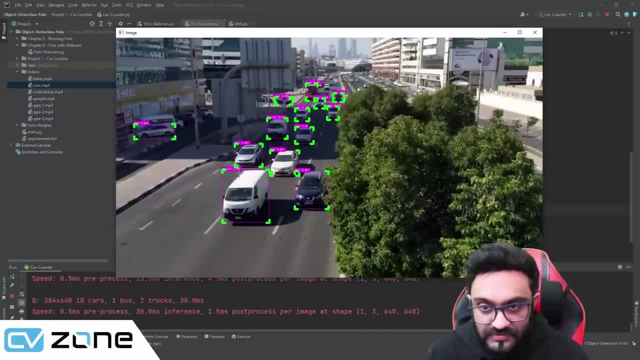 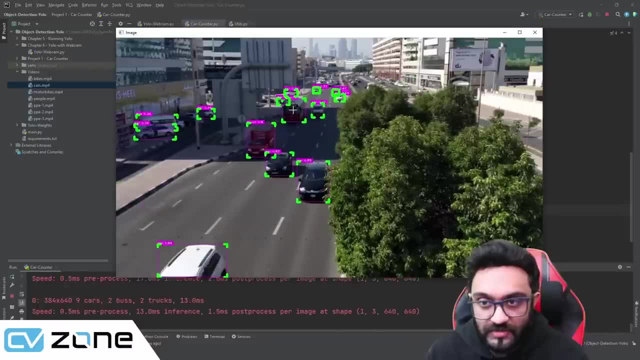 Whether it's detected as a bus or a truck. So this is truck as well, And this is truck as well. Then there you go, We have the truck. So earlier it was detecting as a truck, but here it's detecting as a bus. 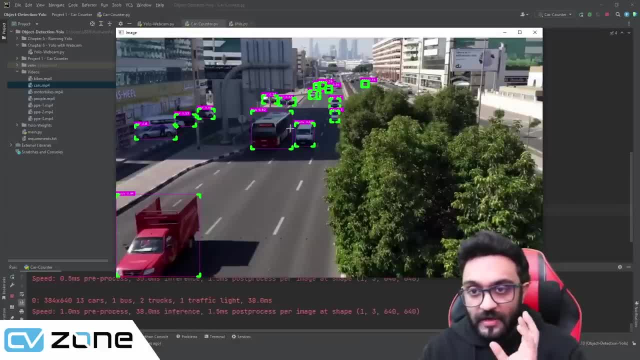 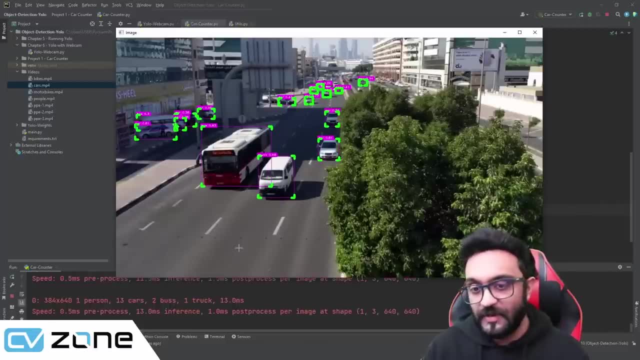 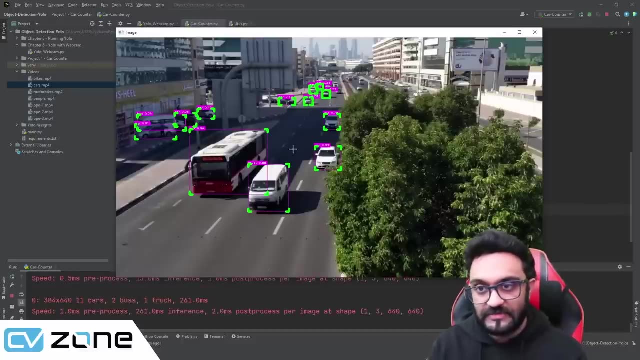 So actually this gives us a good point that this point is actually where most of the cars will be classified properly. At the very end it might not classify properly. At the very back It might not classify properly, But at the middle it should detect and classify properly. 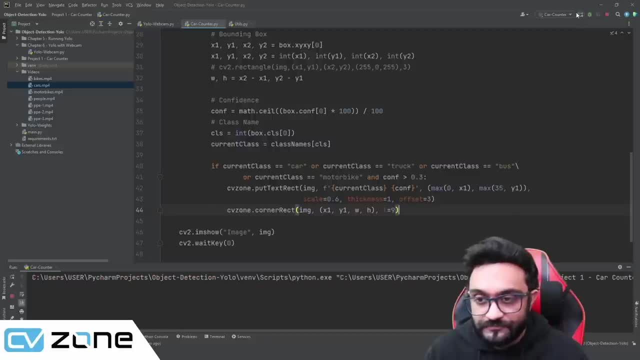 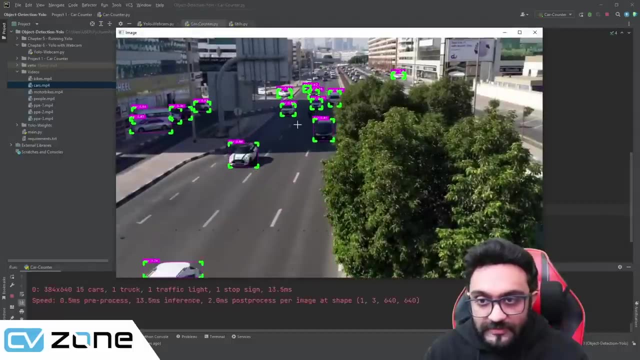 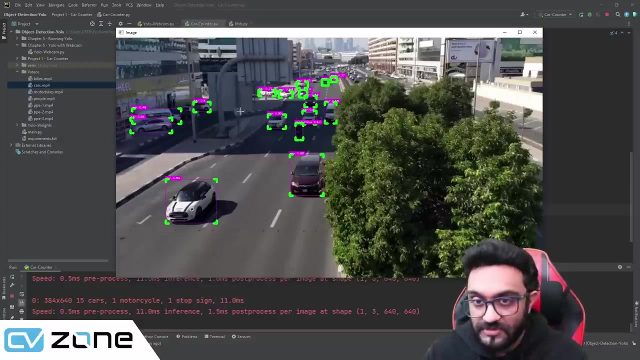 let's run it and see how it works. so now it will detect only those. so here you can see it was detecting something. here it was detecting probably a traffic sign, but now it's not detecting that because it's not part of it. and here you can see it says motorbike. 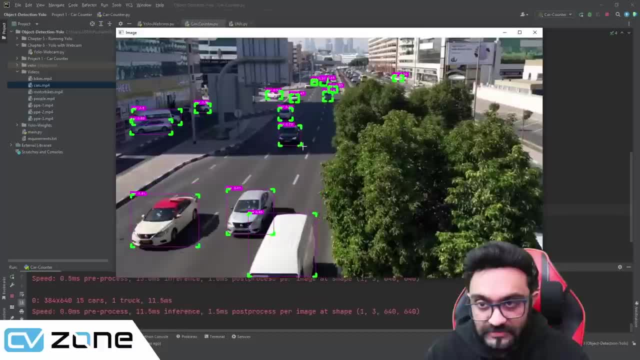 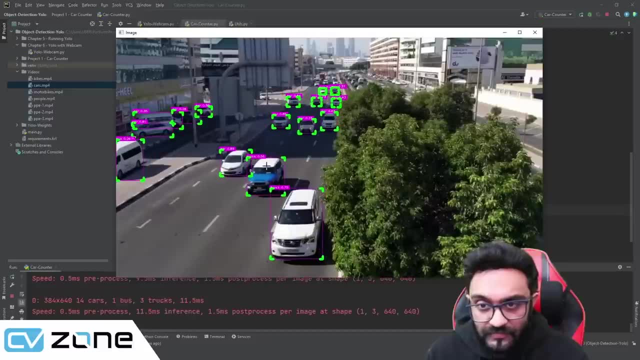 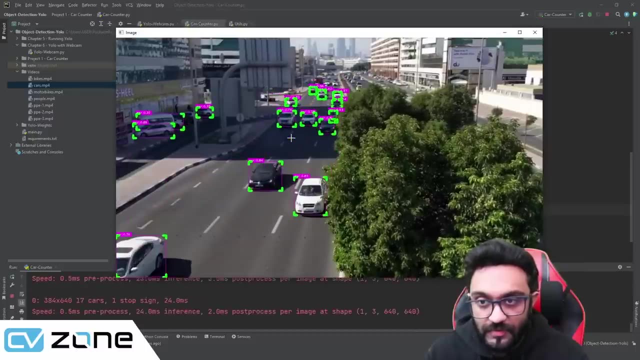 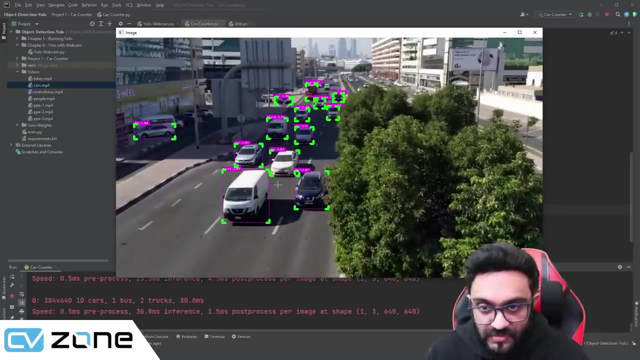 at 0.56 or 59 percent uh confidence. so 59 confidence. so here you can see car um. this is detected as a truck. this is also detected as a truck. so then we'll move forward and we wait for the bus, whether it's detected as a bus or a truck, so this is truck as well. 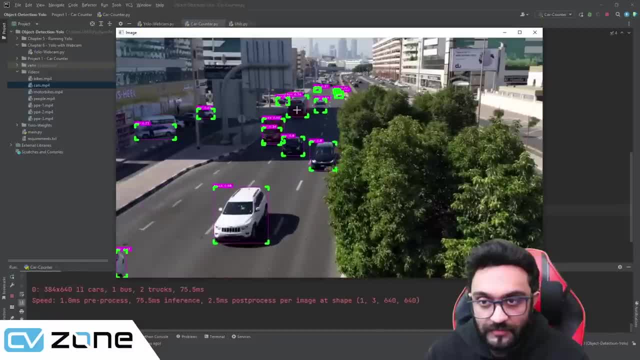 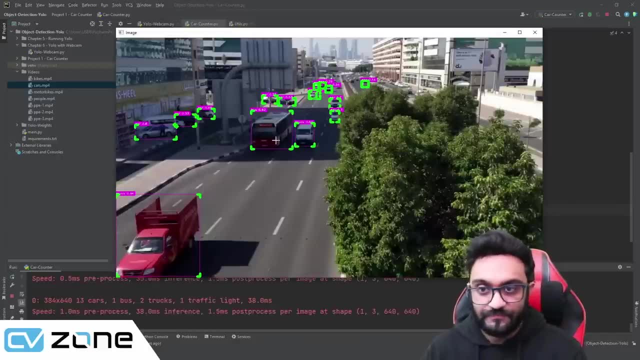 and this is truck as well. then there you go, we have the truck. so earlier it was detecting as a truck, but here it's detecting as a bus. so actually this gives us a good point, that this point is actually where most of the cars will be classified properly. at the very end it might not classify. 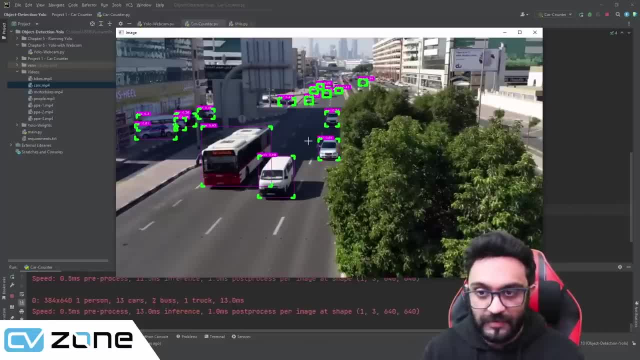 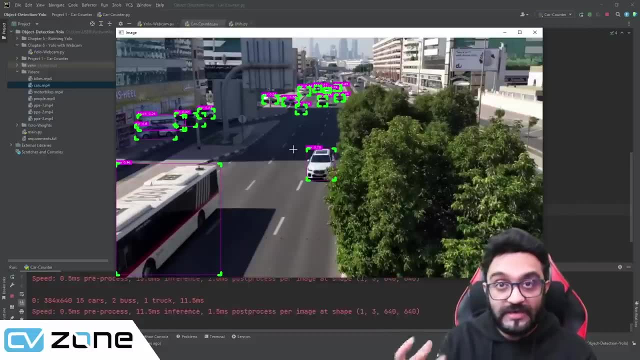 properly. at the very, the very end there are cars would be classified correctly. at the very back it might not classify properly, but at the middle it should detect and classify properly. so that is the region where we should count. so this is where it gives us the idea. so if you are trying to find, 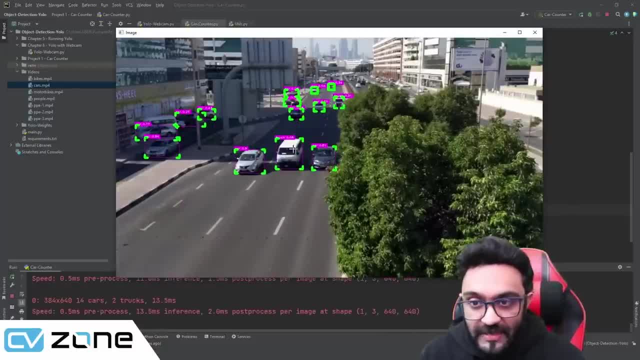 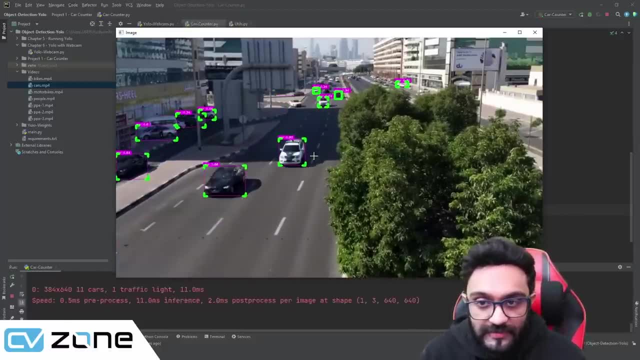 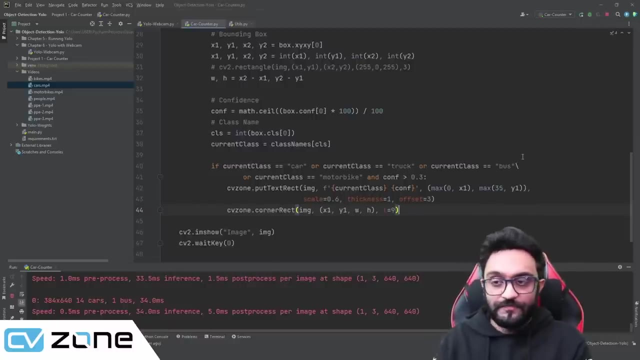 that position. try to loop through these images and try to find that correct position where the detections are correct. so that's how you can tell: oh, the good position where the good position is okay. so that's done. so we have the cars now, but, as you can see, we have it in the wrong places, as 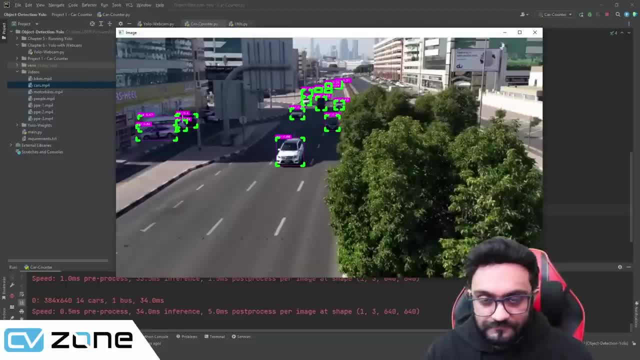 well. so, for example, we don't care about what's happening here. if we have some counts over here, it will interrupt our count. for example, if a car is come going out from here. we don't want to detect that, we just want to detect at this point on the main road. so you have to constrain your. 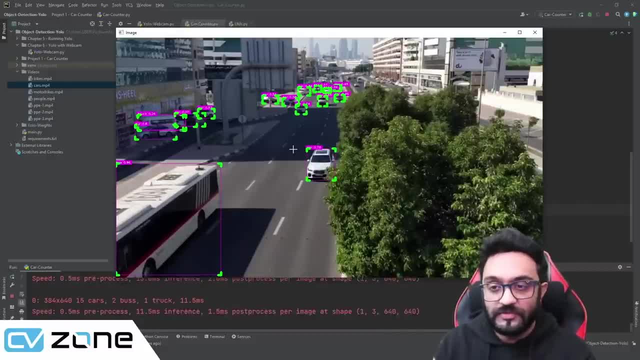 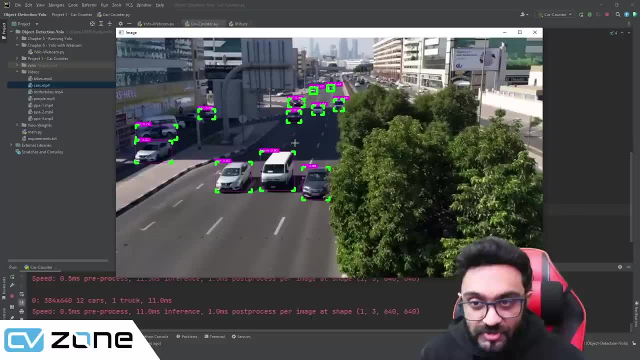 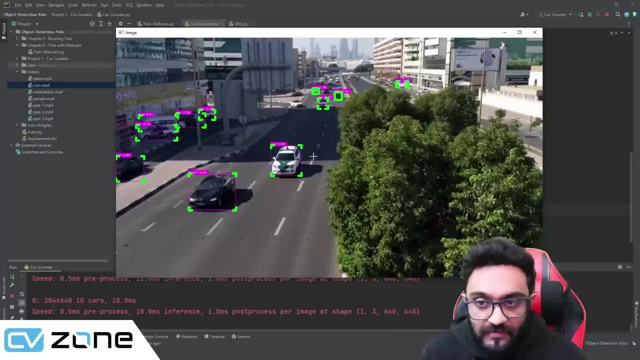 So that is the region where we should count, So this is where it gives us the idea. So if you're trying to find that position, try to loop through these images and try to find that correct position where the detections are correct. So that's how you can tell the good position where the good position is. 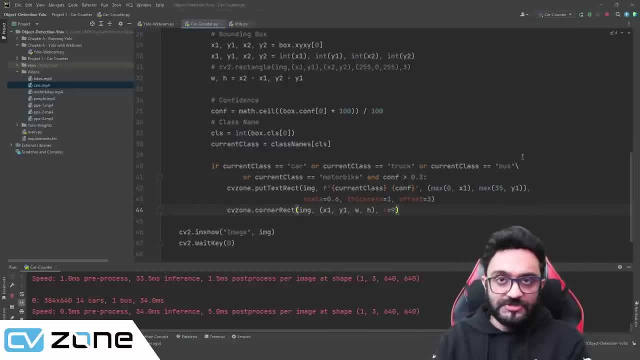 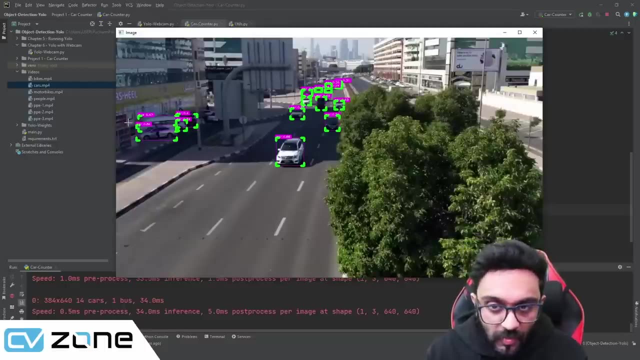 Okay, so that's done. So we have the cars Now, but, as you can see, we have it in the wrong places as well. So, for example, we don't care about what's happening here. If we have some counts over here, it will interrupt our account. 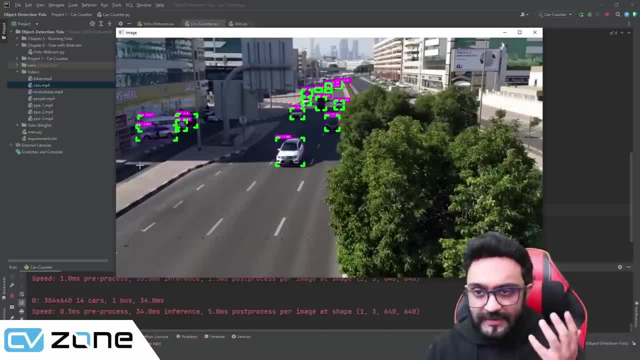 For example, if a car is going out from here, we don't want to detect that, We just want to detect at this point on the main road. So you have to constrain your values So to get good results. otherwise, if it's completely open, it's not constrained at all. 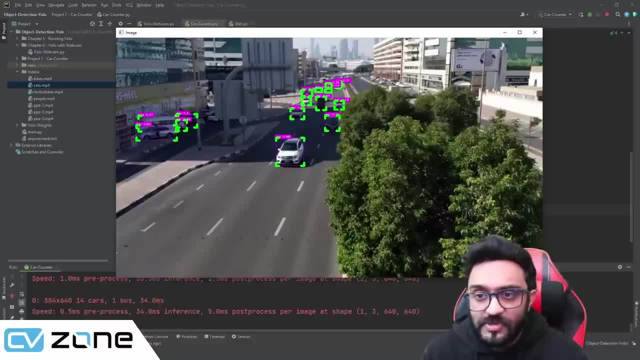 You might not get the best results. Okay, So how can we constrain this? How can we make sure that only this region you detect? what do you call the cars or whatever the object is? So one thing you can do, which is very simple and that you can do within OpenCV or within 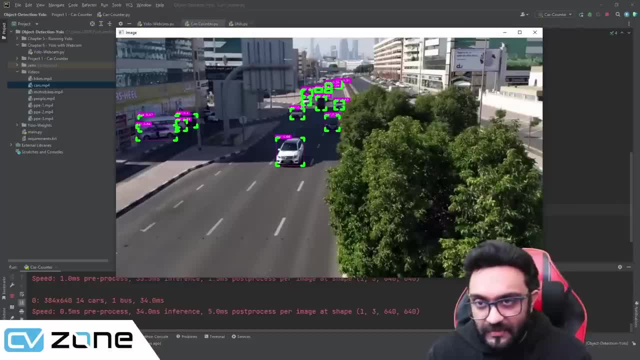 this PyCharm environment is that you can create a rectangle So you can crop this image. You can create this rectangle here And you can say, okay, only detect in this. And how can you say that You will crop that image and that image you are going to send it to your detector. 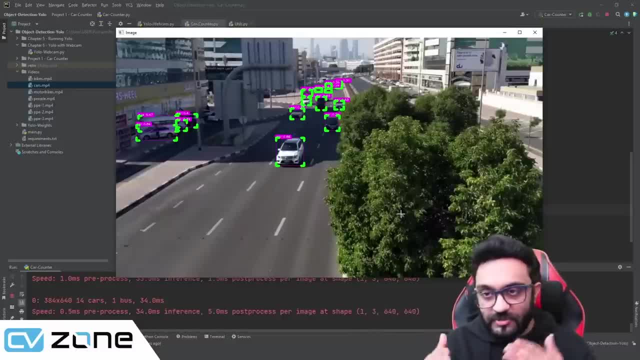 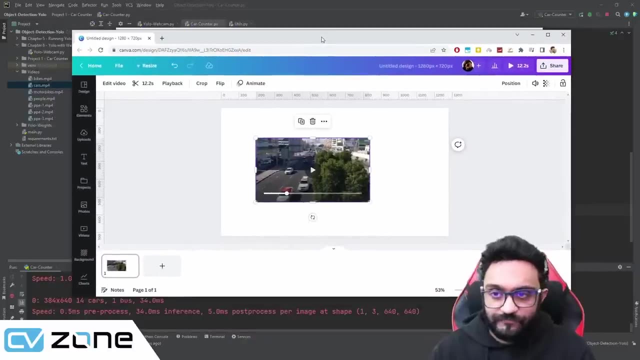 But that is not a very good idea, because the shape over here is not rectangular or not square, So what we want is the exact shape. So how can we do that? Now? it is very simple: We will go to canvacom and we are going to create a new design. 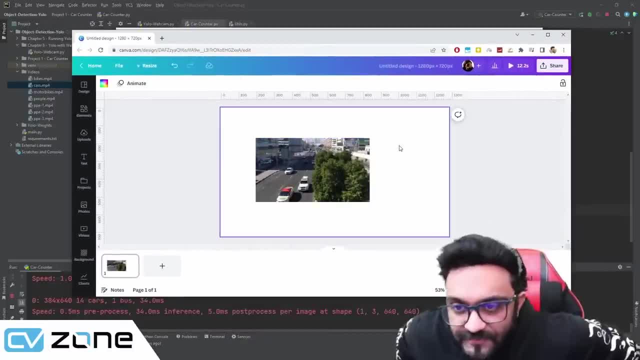 And in this new design. This design is 1280 by 720.. So this is the size of our video and that is exactly the size of the design, And then we are going to import this video. So here, this is the video. 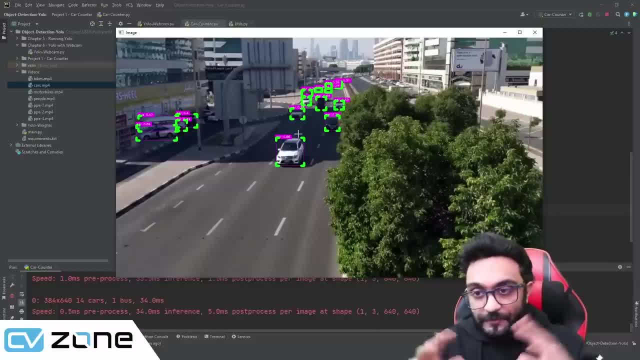 values so to get good results. otherwise, if it's completely open, it's not constrained at all, uh, you might not get the best results. okay, so how can we constrain this? how can we make sure that only this region, uh, you detect? uh, what do you call the cars or whatever the object is? so, once, one thing you can do, which 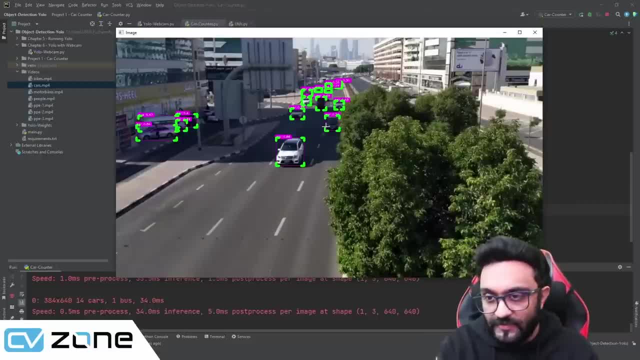 is very simple and that you can do within opencv or within the spy charm environment, is that you can create a rectangle so you can crop this image. and you can create a rectangle so you can crop this image, you can create this rectangle here and you can say: okay, only detect in this and how can? 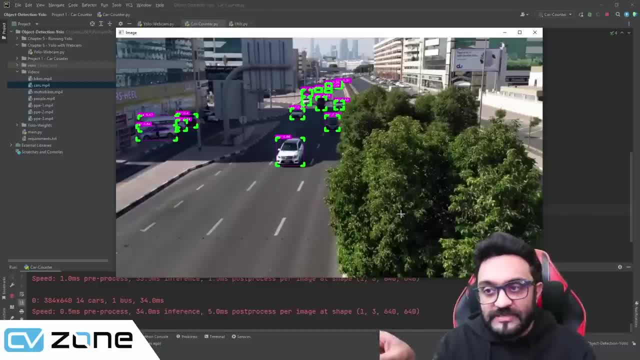 you say that you will crop that image and that image you are going to send it to your detector, but that is not a very good idea, because the shape over here is not rectangular or not square, so what we want is the exact shape. so how can we do that now? it is very simple: we will go to canvacom. 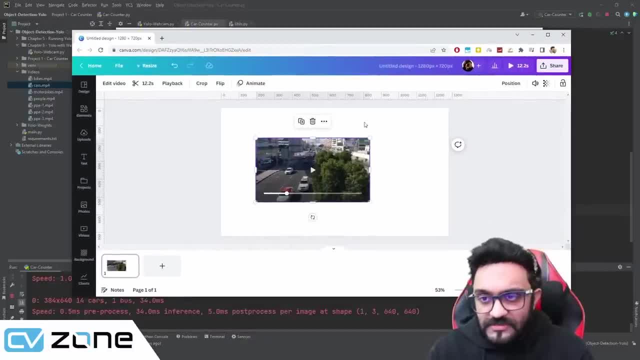 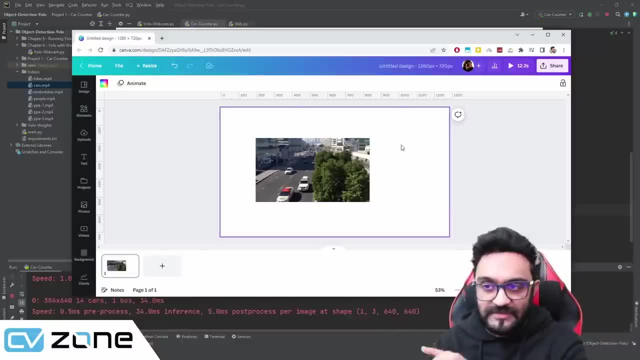 and we are going to create a new data and we are going to create a new design, and in this new design, this design is 1280 by 720, so this is the size of our video and that is exactly the size of the design, and then we are going to import. 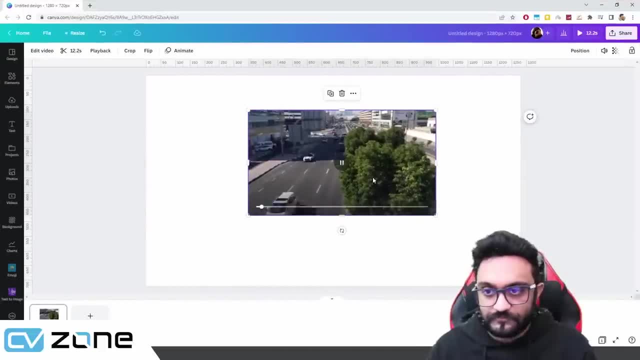 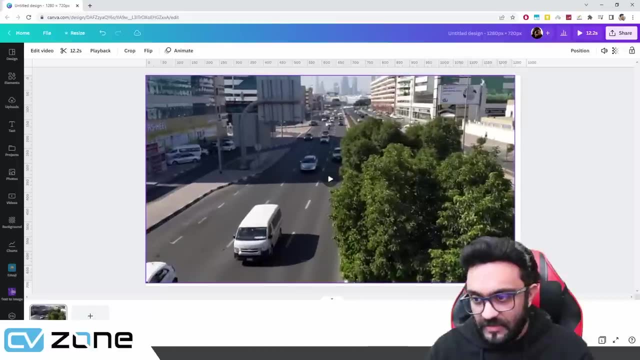 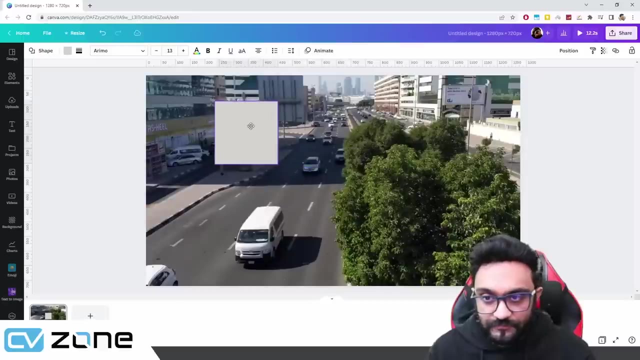 this video. so here, this is the video you can see. it's the exact same one. now, what you will do is you will resize it so that it is the correct size. it fills up the whole screen and then you are going r. that will give you a rectangle. so, with this rectangle, what you have to do is you have to. 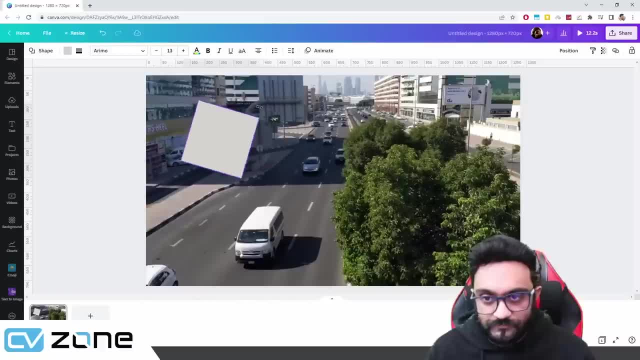 determine the region. so we are going to rotate it and we are going to align it with this dotted line, this lane. we are going to align it with this and for the other one, we are going to align it with this lane. so let's go ahead and do that, so we will align. we will try to align it as. 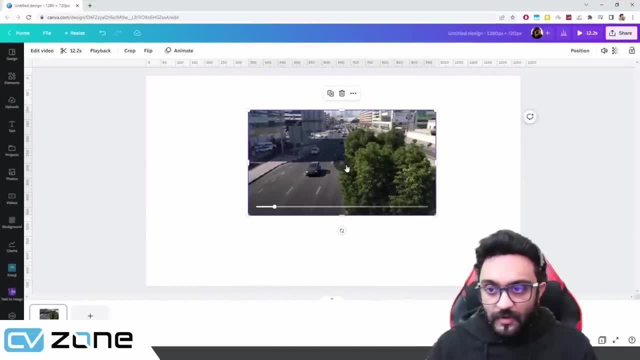 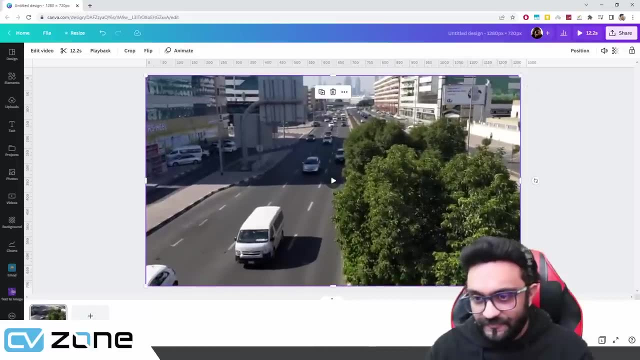 You can see, it's the exact same one. Now, what you will do is you will resize it so that it is the correct size. It fills up the whole screen and then you are going to press R. That will give you a rectangle. So, with this rectangle, what you have to do is you have to determine the region. 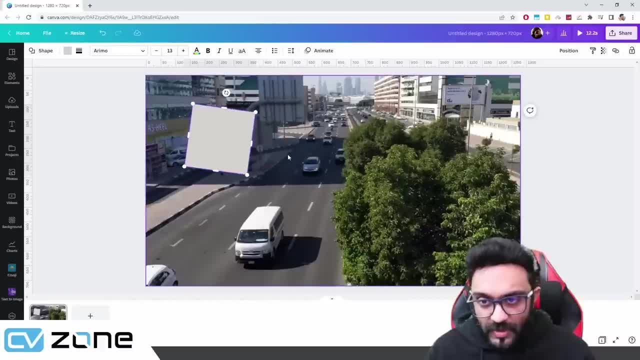 So we are going to rotate it and we are going to align it with this dotted line, This lane, We are going to align it with this and for the other one, we are going to align it with this lane. So let's go ahead and do that. 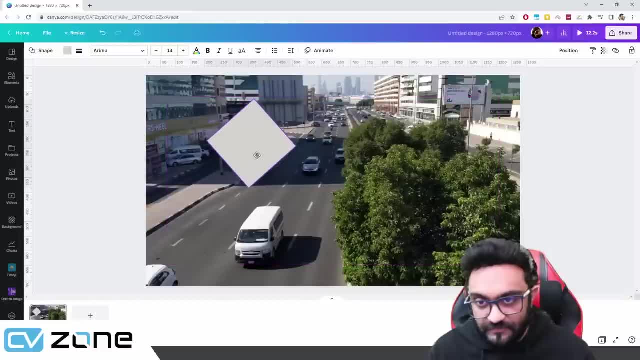 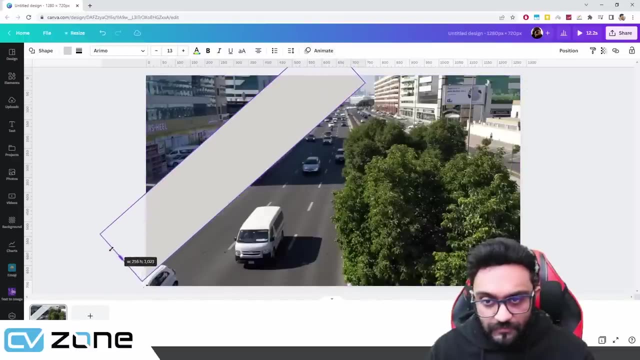 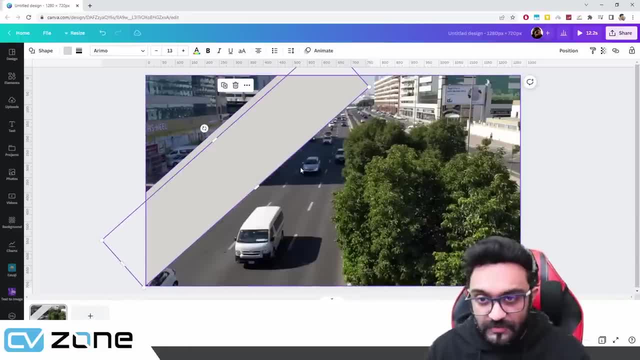 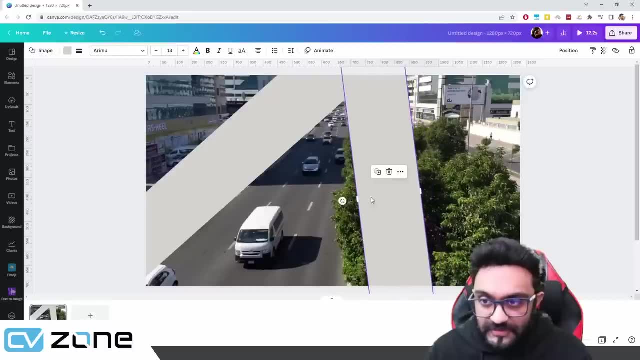 There you go. So this is the first one and the second one we are going to. basically, what we are trying to do is we are trying to create a mask so that it only views in that mask region. So we are going to put another image here. 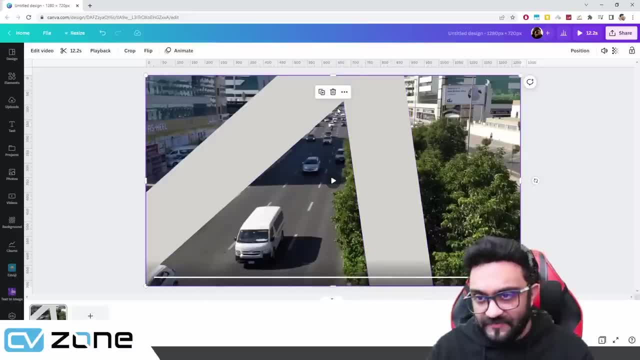 There you go, Another rectangle here. this area again is very small and it's not very useful, so we are going to remove that as well. so we'll create another rectangle and we'll put it over here, something like that, and at the bottom as well. we don't want to detect. 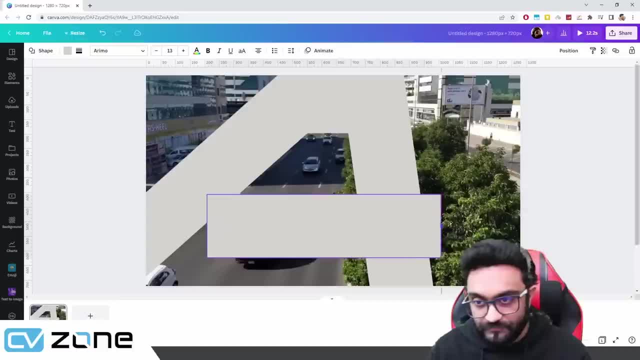 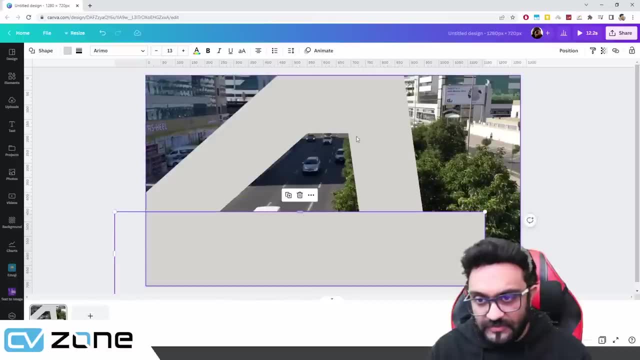 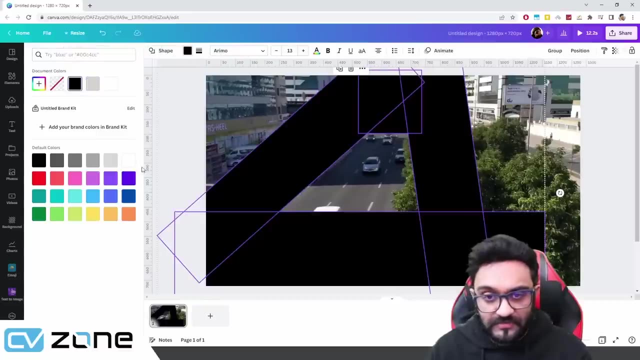 so we'll create another one and we will put it here. something like that: so, depending on which region you are trying to detect, you can create this. so the then you are going to select all of them and you are going to change the color to black- you can do that in the beginning as well- and then we are going to extend. 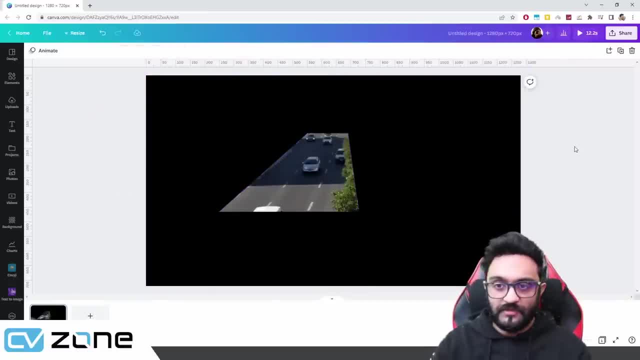 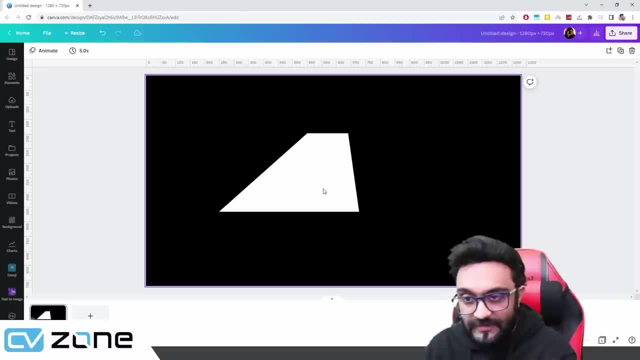 it so that only that region is visible. there you go. that's how simple it is. that's how you can create this mask, and all you have to do now is click on the video and delete it. that will give you the white region, so then you can simply share, download, and you don't need transparent. 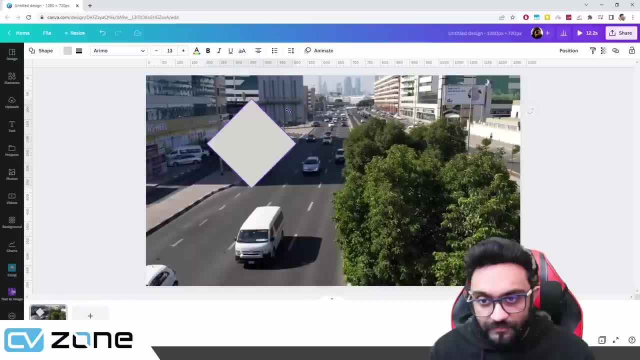 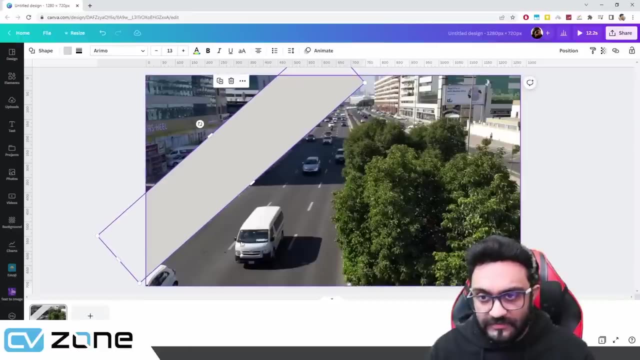 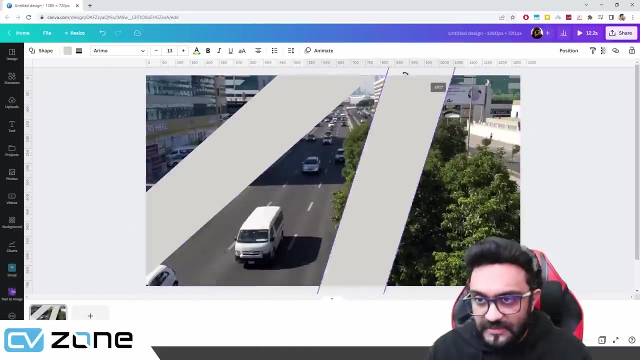 much as we can. so something like that, something like that. so there you go and you can move it around like that, there you go. so this is the first one and the second one we are going to. basically, what we are trying to do is we are trying to create a mask so that it only views in that mask. 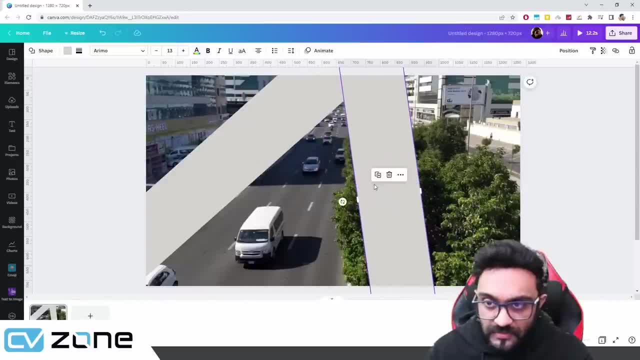 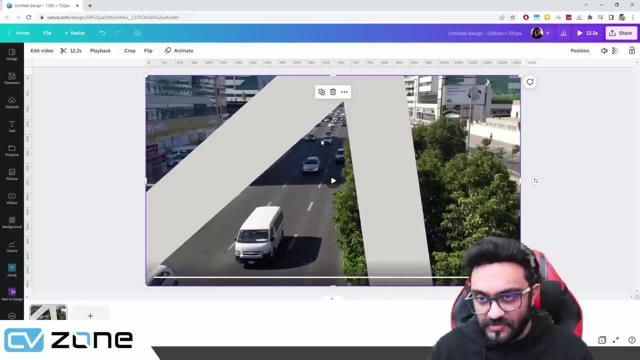 region. so we are going to put another image here. there you go, another rectangle here and then this area again is very small and it's not very useful, so we are going to remove that as well. so we'll create another rectangle and we'll put it over here, something like that, and at the bottom as 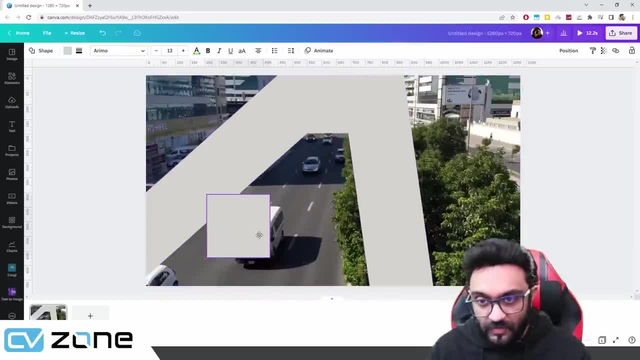 well, we don't want to detect, so we'll create another one and we will put it here, something like that. so, depending on which region you are trying to detect, you can create this. so then you are going to select all of them and you are going to change the color. 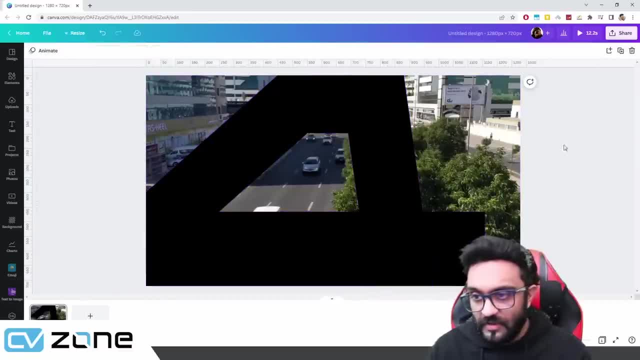 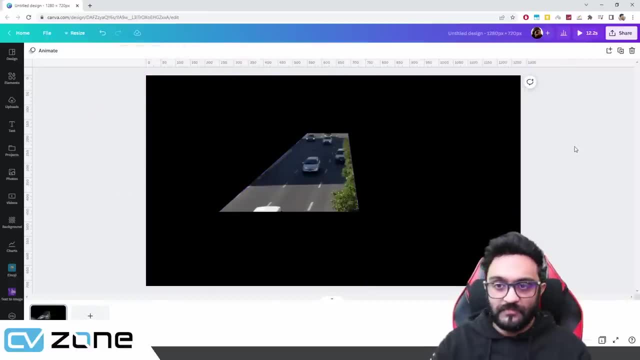 to black. you can do that in the beginning as well, and then we are going to extend it so that only that region is visible. there you go. that's how simple it is. that's how you can create this mask, and all you have to do now is click on the video and delete it. that will give you 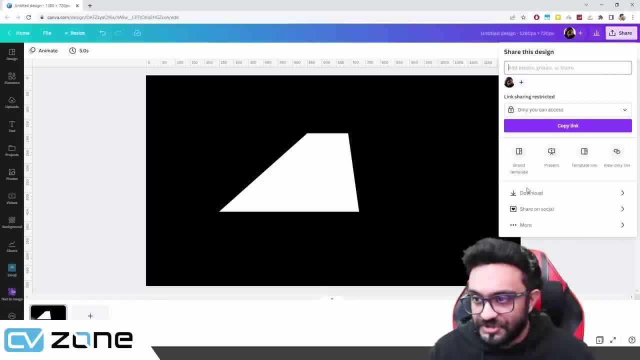 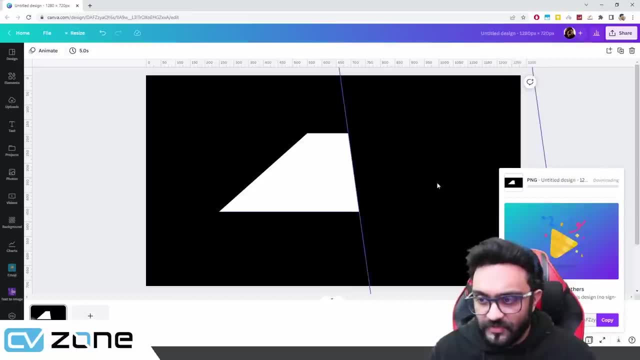 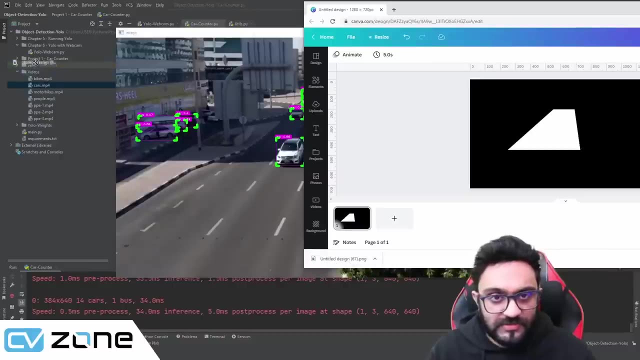 the white region. so then you can simply share download, and you don't need transparent background, you don't need to compress. all you have to do is you have to download the image. once it's downloaded, we are going to import it. so here is the downloaded file. we are going to bring it to our project. so project one car. 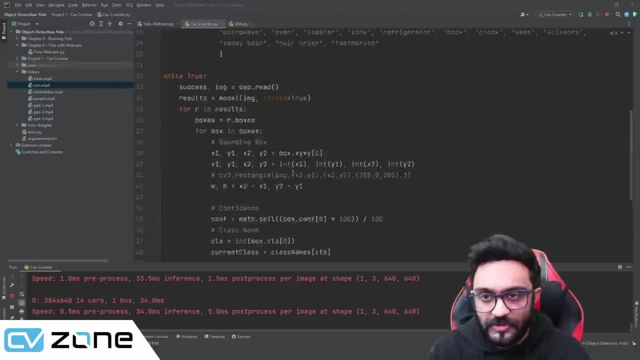 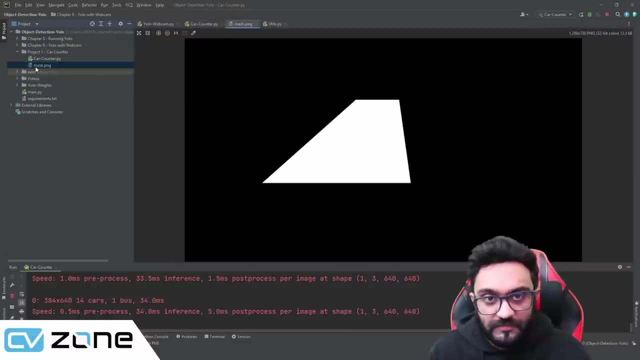 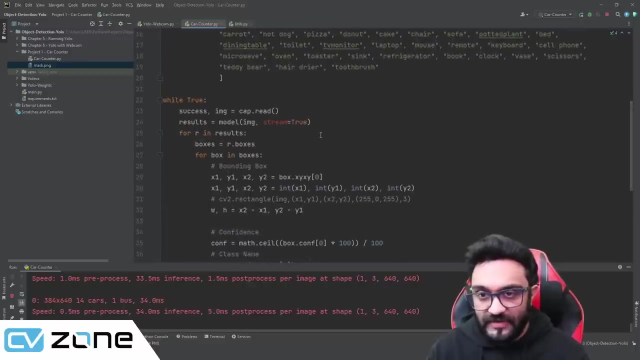 counter, and we are going to name it mask dot png. so if we open that up in projects, let's close the others. so here, mask dot png, this is our mask, so we can remove that. and now what we have to do is we have to overlay these images so that only this region is detected and we only find the cars. 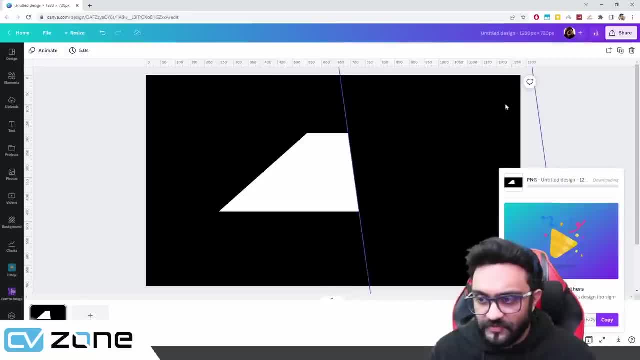 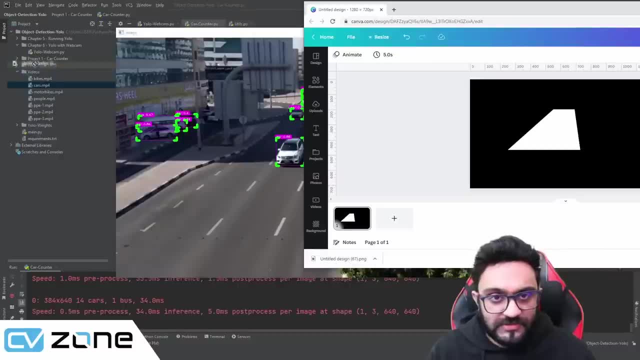 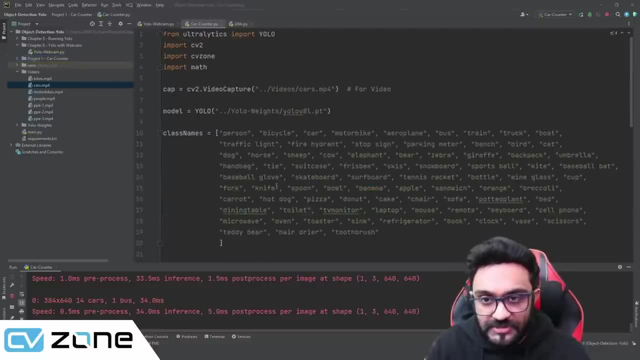 background. you don't need to compress. all you have to do is you have to download the image. once it's downloaded, we are going to import it. so here is the downloaded file. we are going to bring it to our project. so project one car counter, and we are going to name it mask dot PNG. so if we open that up in 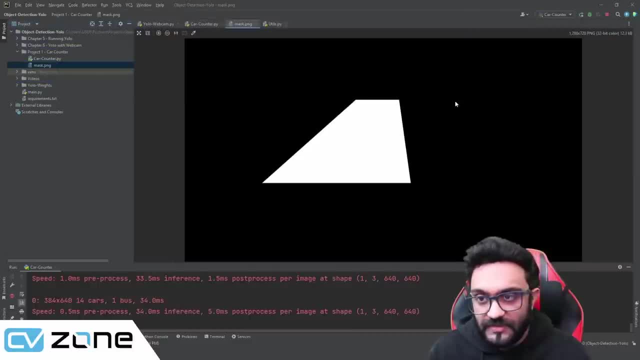 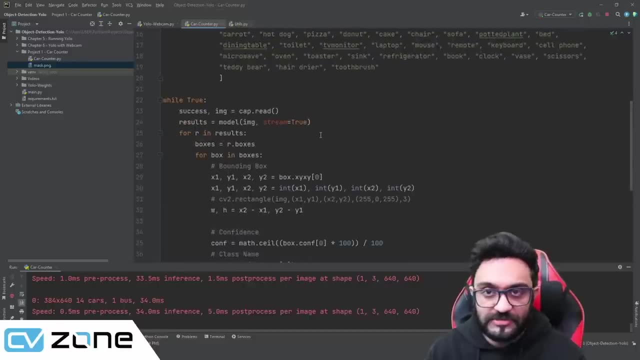 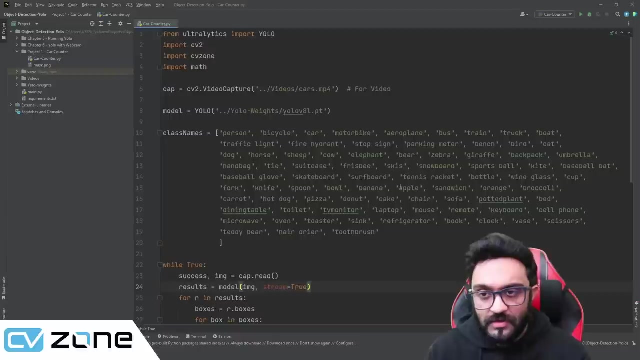 projects. let's close the others. so here: mass dot, PNG. this is our mask, so we can remove that. and now what we have to do is we have to overlay these images so that only this region is detected and we only find the cars within these regions. so now what we need: 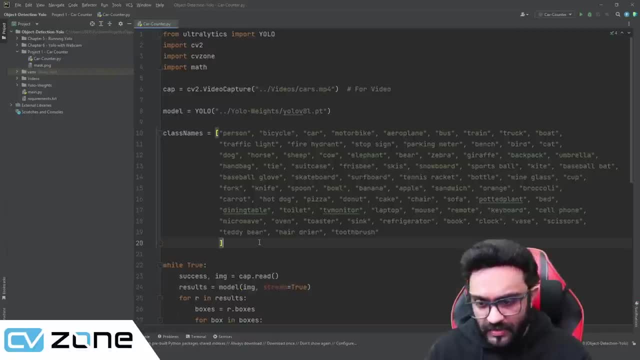 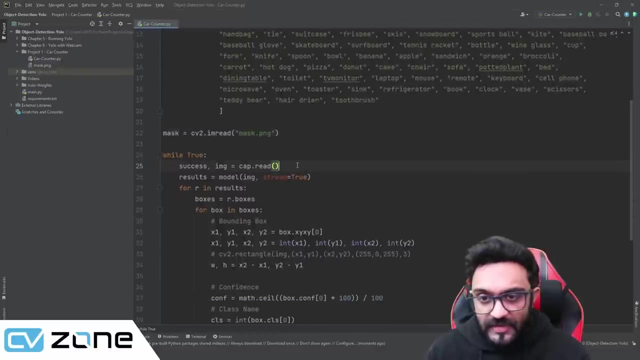 to do is we need to import this mask. so here at the bottom we are going to say: mask equals cv2 dot. I am read and we are going to read from our image. so we will write mass dot, PNG. and once we have that and we get our webcam image or we 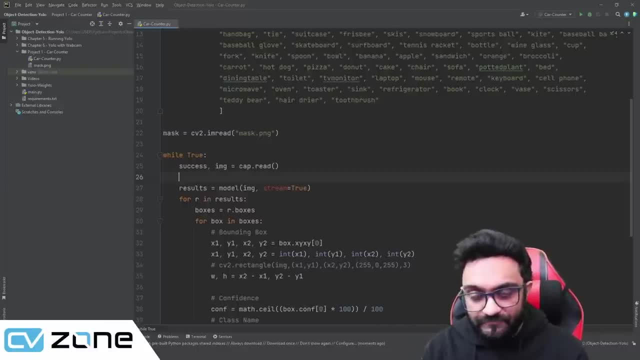 get our video image, then we are going to use the mask dot PNG and we are going to overlay the mask on our main image. we are going to use a bitwise operation of and that will give us only that region. so we are going to say we are going to 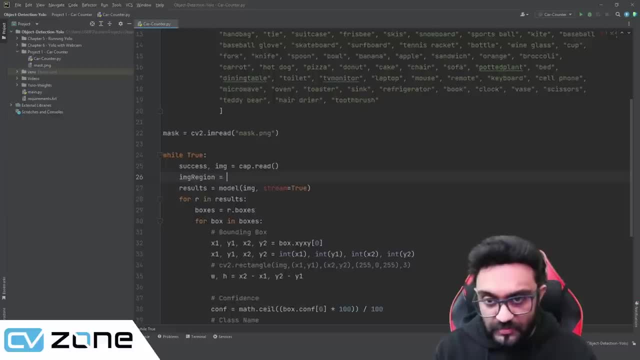 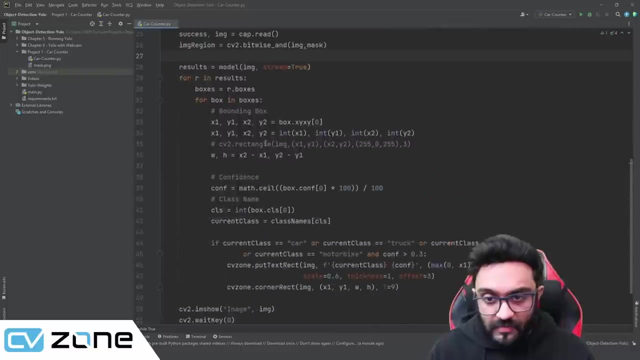 say, image re gen equals cv2 dot bitwise. and and we are going to give in our image and we are going to give in our mask, and this will give us the IMG region and we are going to display that image region. so let's copy that and paste it here so we will write it. 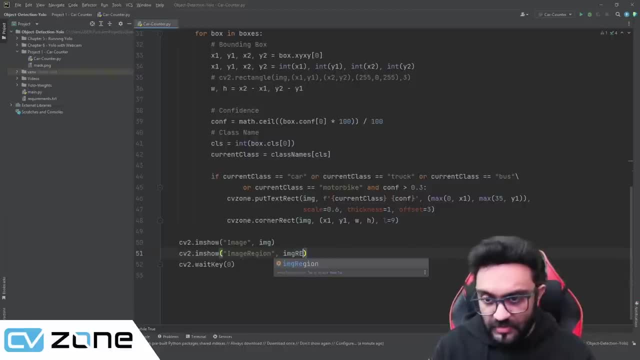 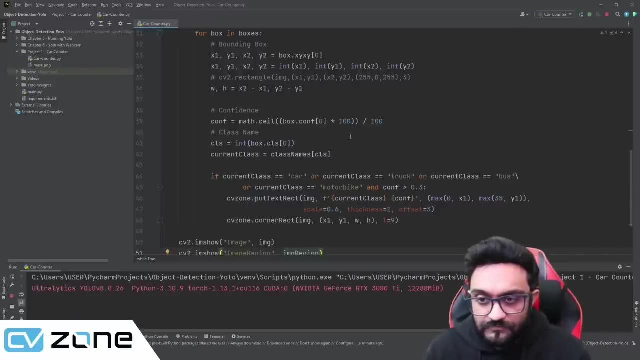 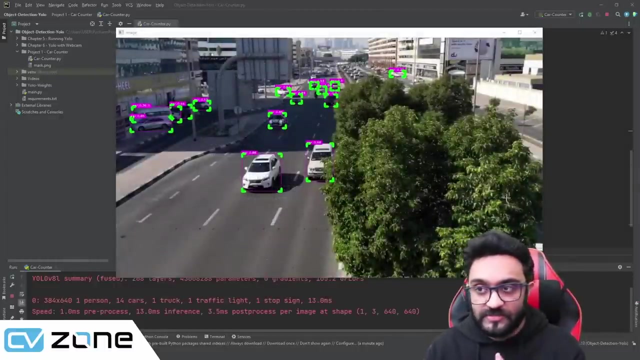 as region and we will write image region. so let's run that and see if we get that region as well and make sure they are of the same size. if they're not of the same size, it will not work. uh, right now i know it's 1280 by 720. that's why we have created the image of 1280 by 720. 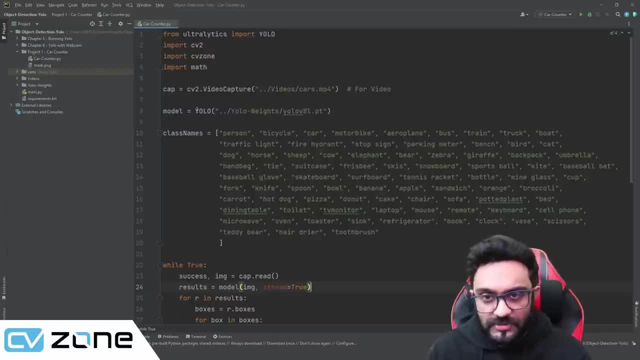 within these regions. so now what we need to do is we need to import this mask. so here at the bottom we are going to say: mask equals cv2, dot. im read and we are going to read the from our image. so we will write mass dot png. and once we have that, uh, and we get our webcam image. 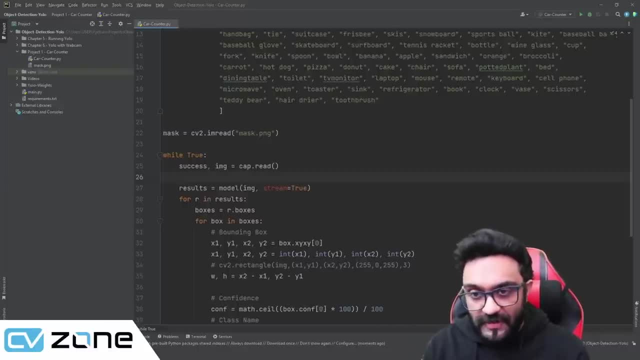 or we get our video image, then we are going to overlay, uh, the mask on our main image. we are going to use a bitwise operation of and that will give us only that region. so we are going to say we are going to say image region equals cv2 dot bitwise. 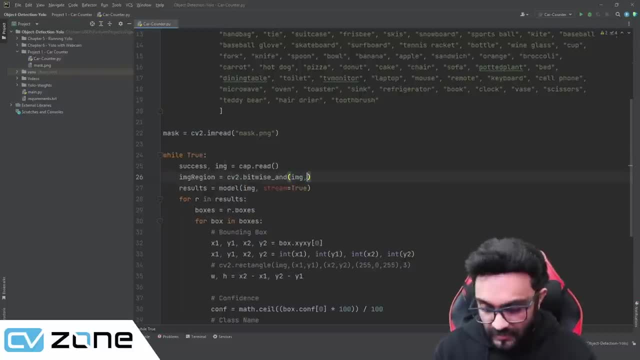 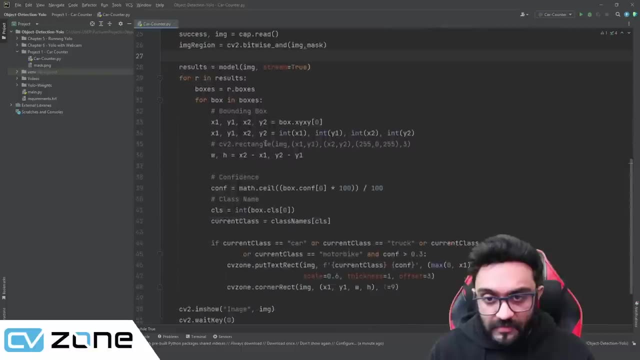 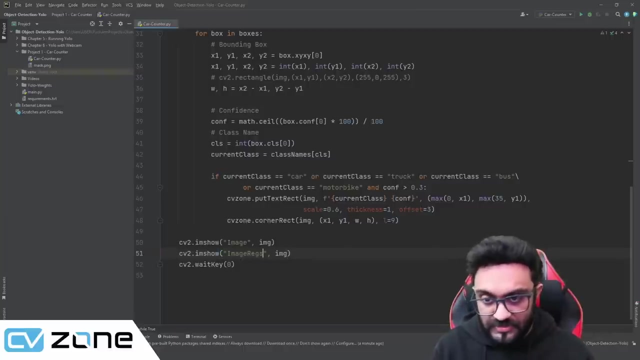 and and we are going to give in our image and we are going to give in our mask and this will give us the img region and we are going to display that image region. so let's copy that and paste it here, so we'll write it as region and we will write image region. 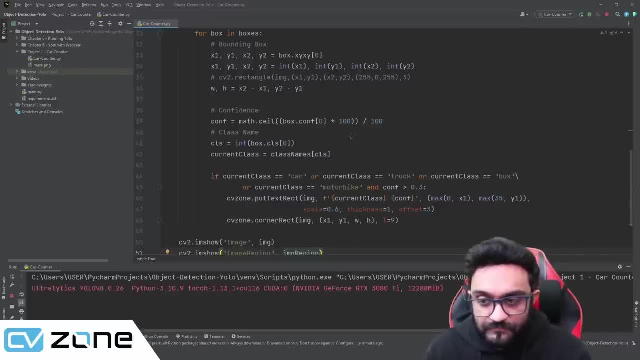 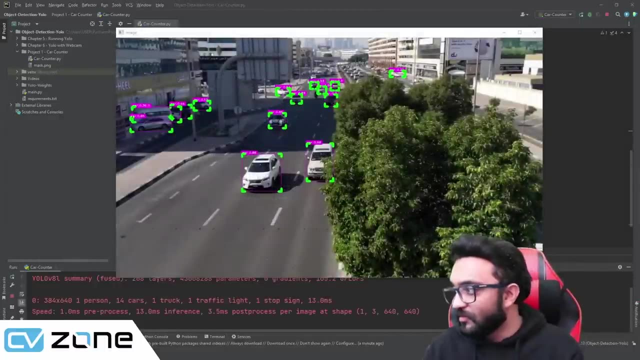 so let's run that and see if we get that region as well and make sure they are of the same size. if they're not of the same size, it will not work. right now i know it's 1280 by 720. that's why we 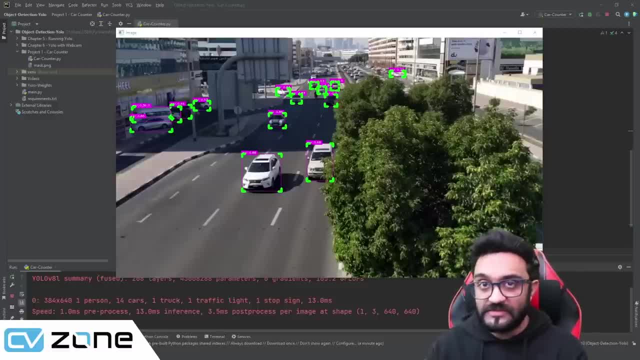 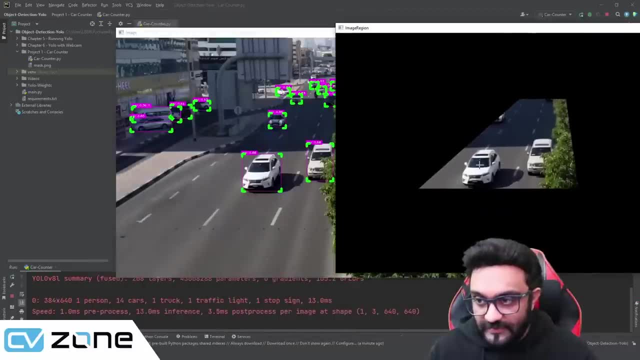 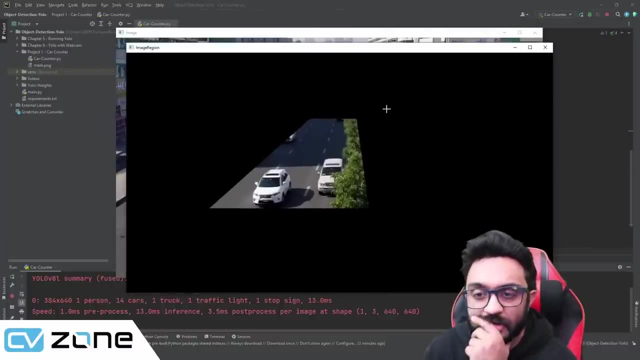 have created the image of 1280 by 720 of the mask, otherwise it will not work. so there you go. this is your mask, this is the image region and, as you can see, it will only detect in this region. that's what we need now, so we want to detect only in this part. actually, the mask is wrong. um, it's, it's not. 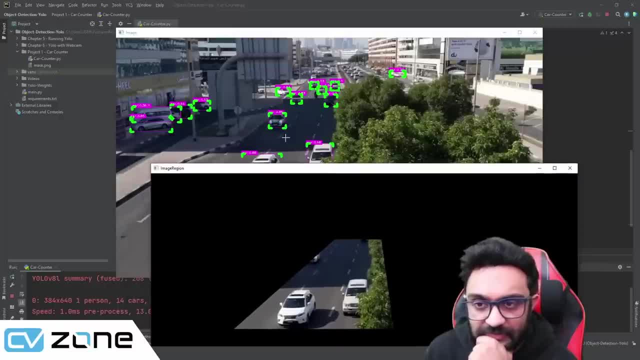 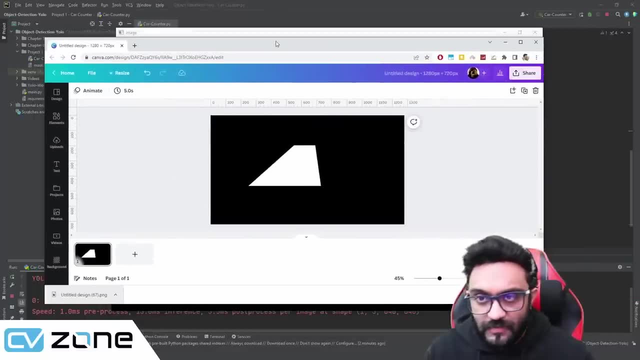 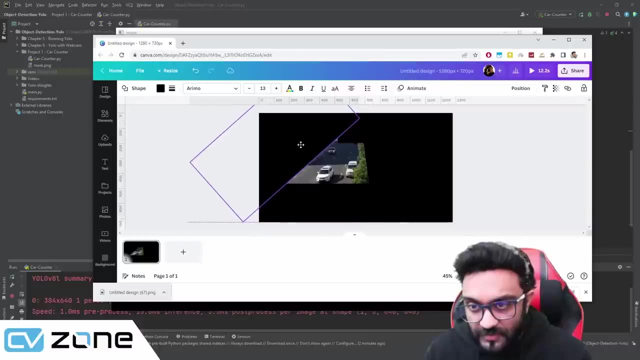 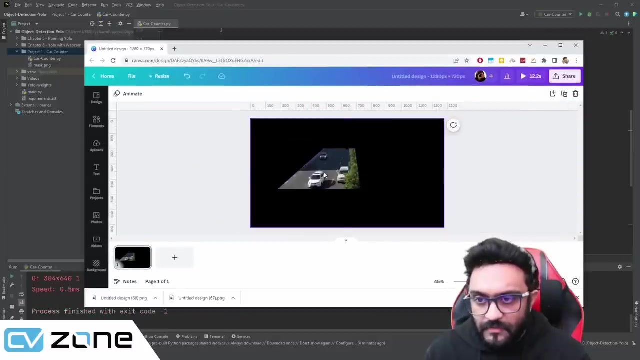 perfect, because this car is is not visible. so this is not correct. something is wrong. let's go back to canva and let's undo: yeah, this is not correct. we need to go a little bit higher. there you go. i guess this is a better representation. there you go. so then we are. 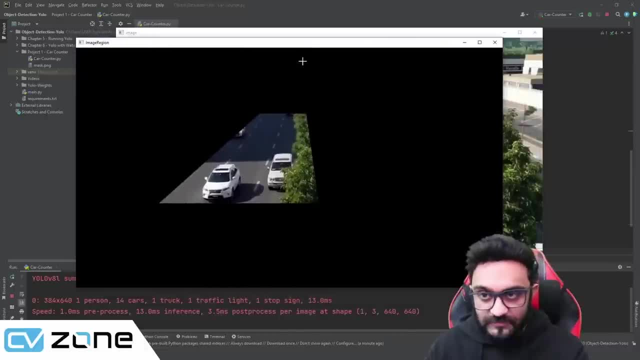 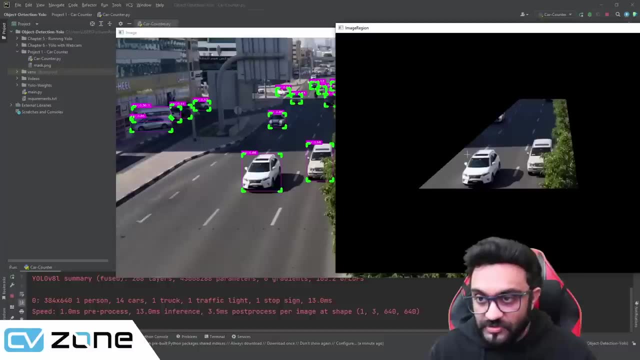 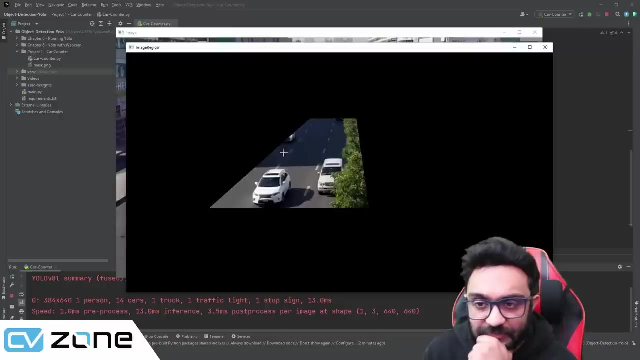 of the mask, otherwise it will not work. so there you go. this is your mask, this is the image region and, as you can see, it will only detect in this region. that's what we need now, so we want to detect only in this part. actually, the mask is wrong. um, it's, it's not perfect because 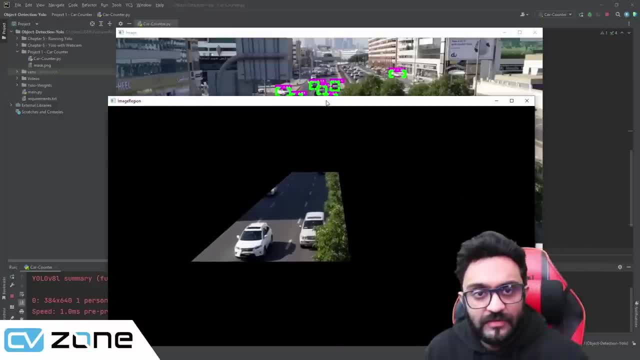 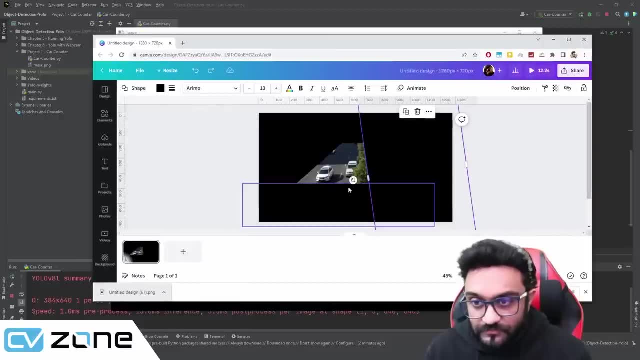 this car is is not visible, so this is not correct. something is wrong. let's go back to canva and let's undo. yeah, this is not correct. we need to go a little bit higher. there you go. i guess this is a better representation. there you go. so then we are going to delete this. 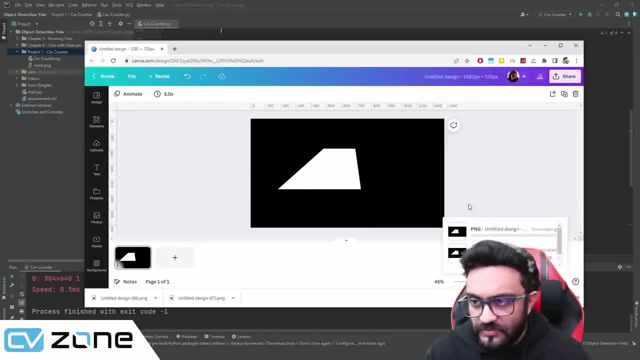 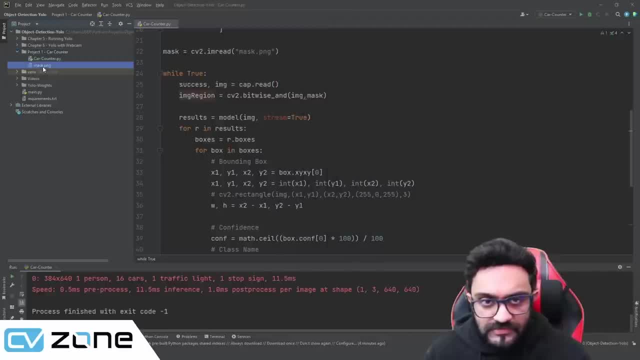 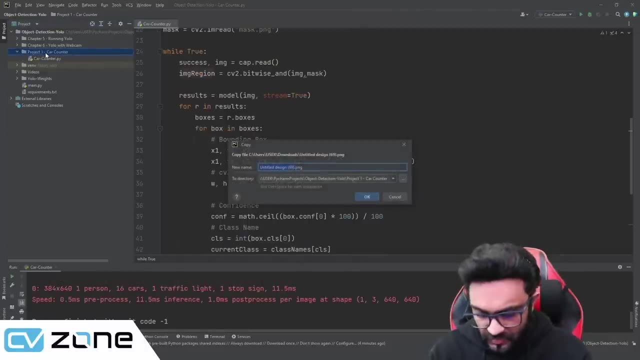 so now it is our new mask, then we are going to download and then we are going to delete this previous mask and we are going to drag in our new mask and we will call it mask mask dot png, and then we are going to run it again. 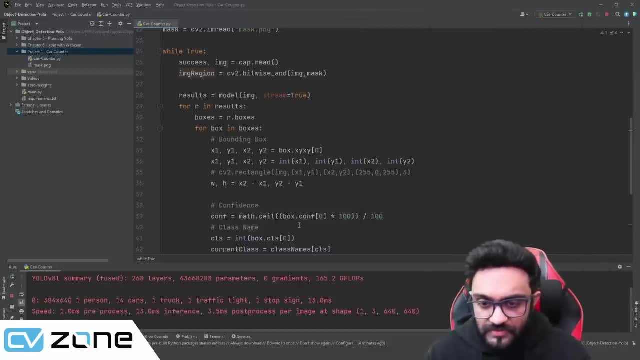 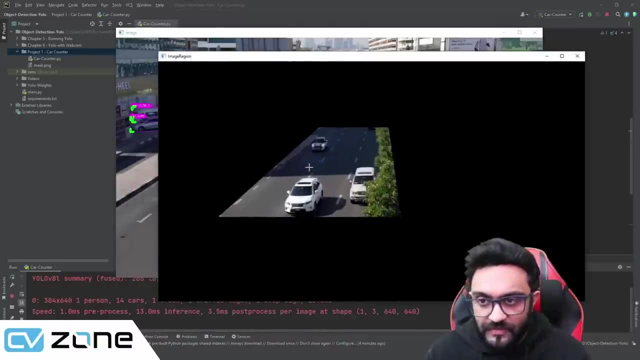 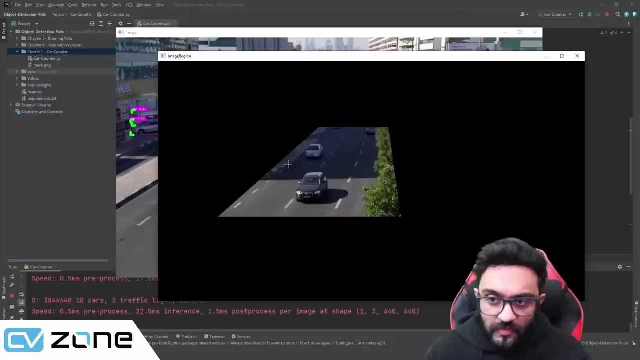 and hopefully this time around we will not face the same issue. okay, so this is our image and this is our mask. there you go. so if we play it, that seems fine to me. yeah, that's good. okay, so now we will send only this image to our 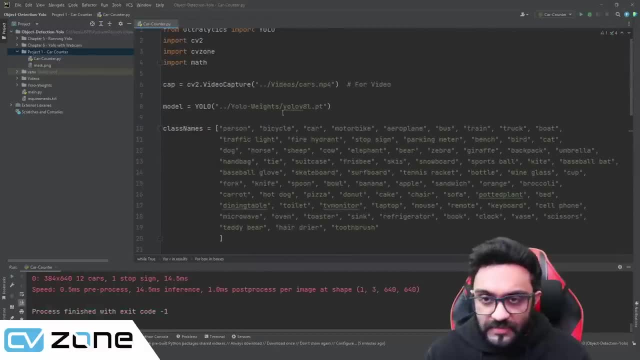 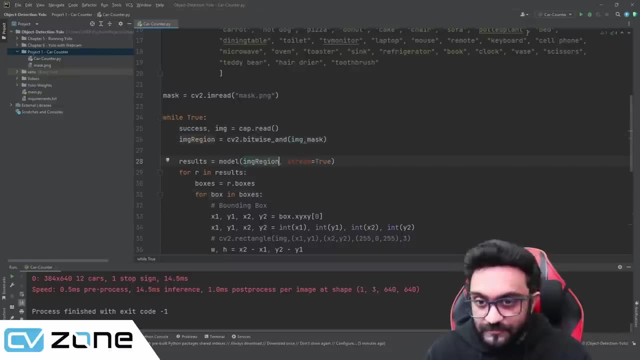 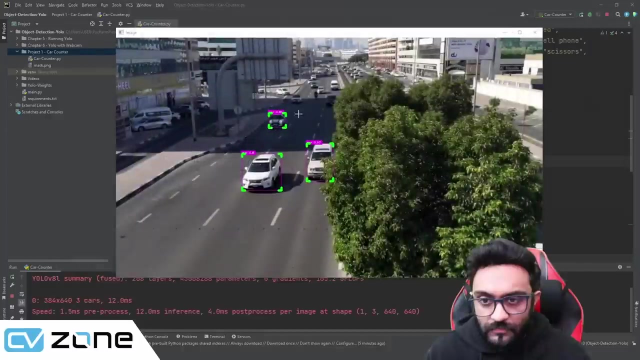 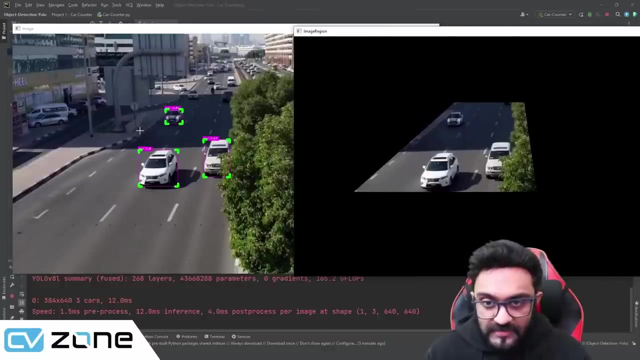 system. so in terms of computation, it will be more efficient as well. so instead of image, we will send image region. that's how simple it is. so let's run that, and there you go. so, based on our image region, as you can see, only this area is being detected as. 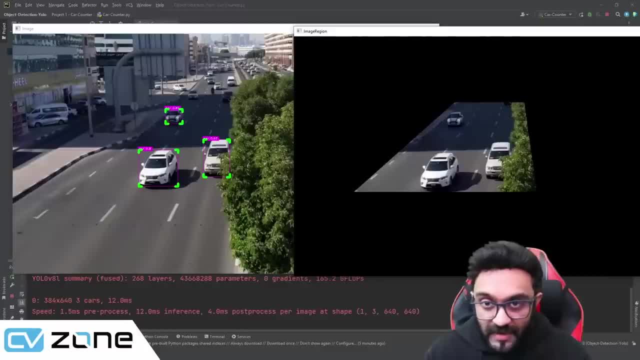 cars. so within this region we are detecting cars behind the car right now we are detecting cars. it we are not getting it on the side, we are not getting it. so only in the middle, in the specified region, we are getting the detections. so if i plate, once it reaches that region it detects it. 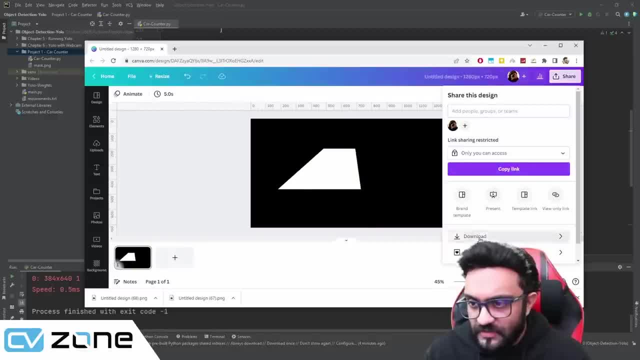 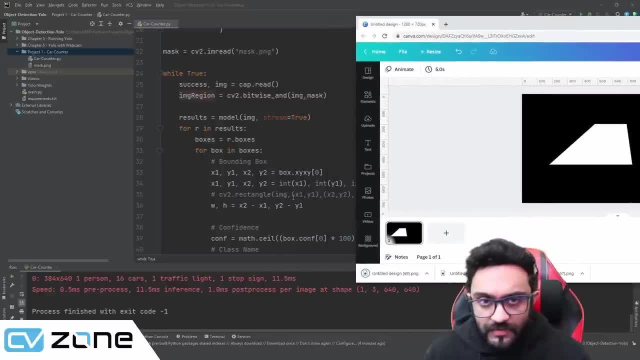 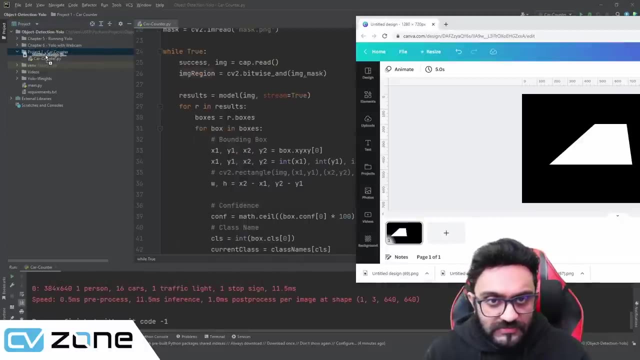 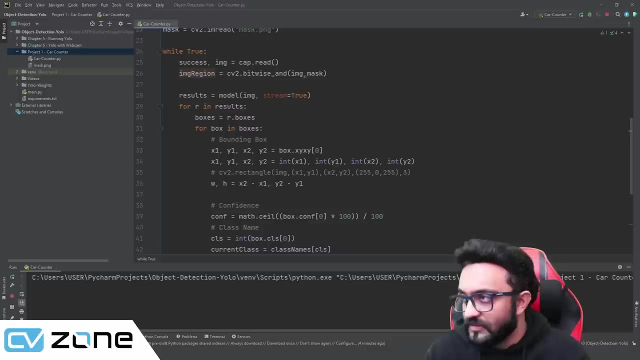 going to delete this. so now it is our new mask, then we are going to download you and then we are going to delete this previous mask and we are going to drag in our new mask and we will call it mask mask dot png, and then we are going to run it again. 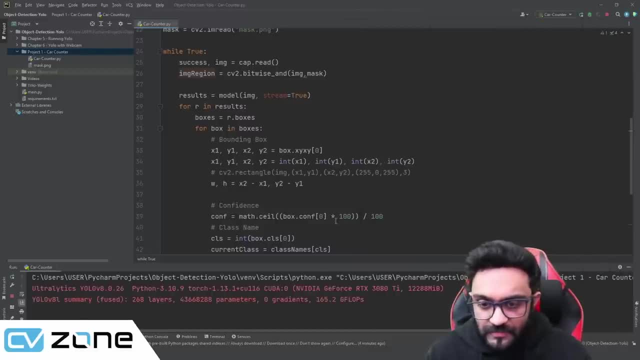 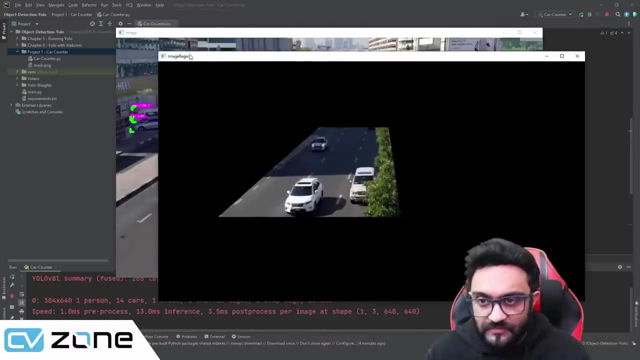 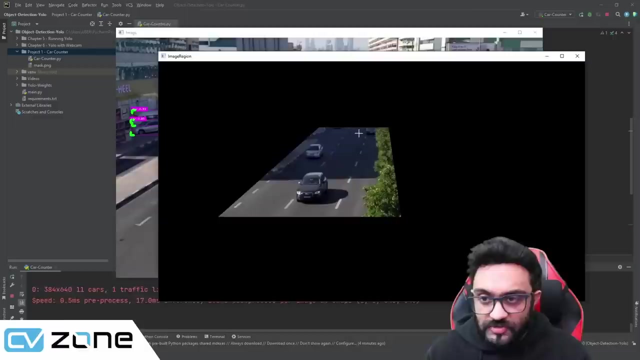 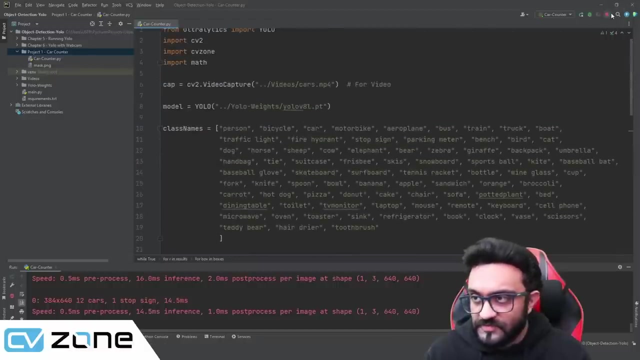 and hopefully this time around we will not face the same issue. okay, so this is our image and this is our image mask. there you go. so if we plate, that seems fine to me. yeah, that's good. okay, so now we will send only this image to our system. so in terms of computation, it will be more efficient as well. 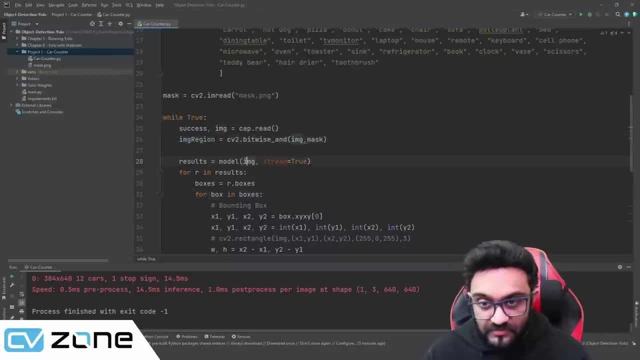 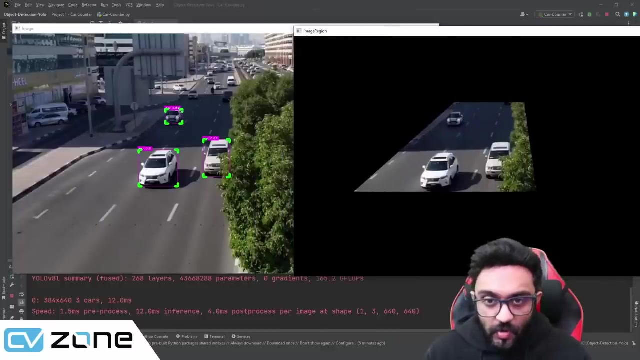 so instead of image, we will send image region. that's how simple it is. so let's run that and there you go. so, based on our image region, as you can see, only this area is being detected as cars. so within this region, we are detecting cars. behind it. we are not getting it on the 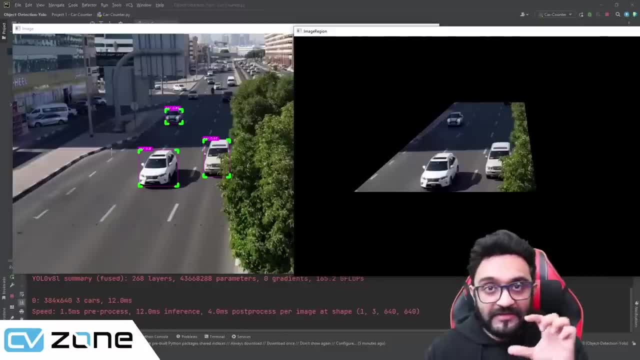 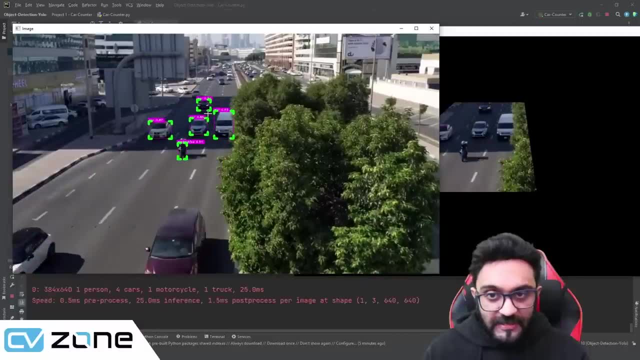 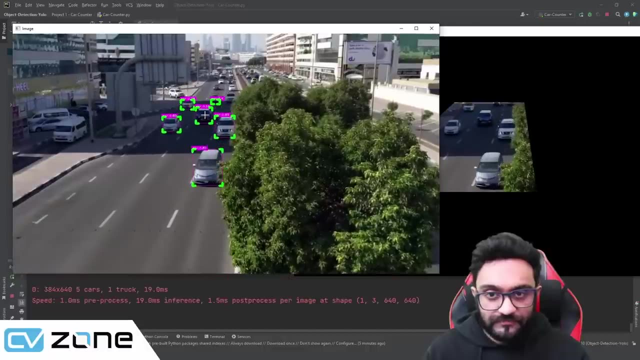 side we are not getting it. so only in the middle, in the specified region, we are getting the detections. so if i plate, once it reaches that region it detects it as a car or a bike and all that. so that's good. as you can see, it looks good. 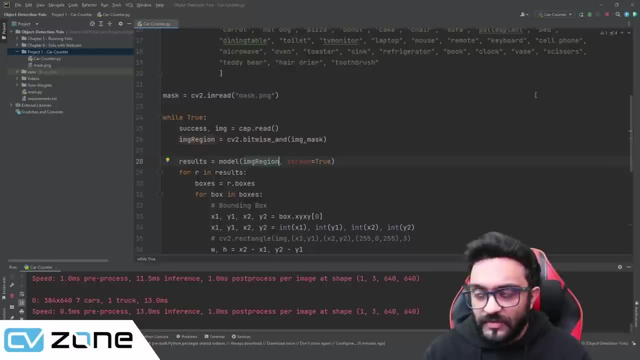 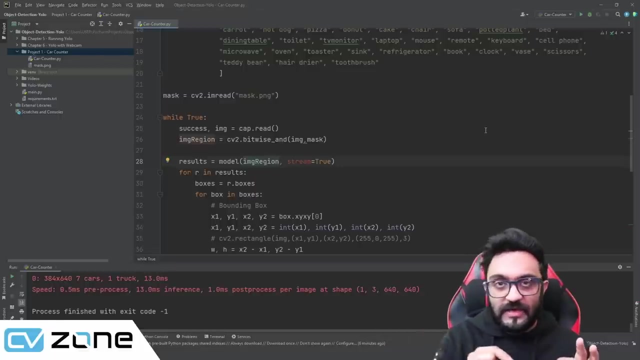 yeah, okay. so now that we have a specified region and we can see all the cars being detected, now we need to count them. so in order to count, we need to have a certain region that this is the line. when it passes this line, we will consider it as counted. 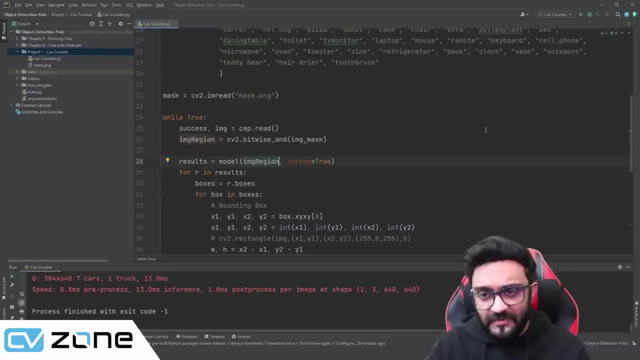 so we need to know that. Second thing we need is an actual tracker. So right now what we are doing is we are detecting the cars, but in the next frame we do not know where the car has gone. So what we need is a tracking ID. So if we detect a car in the first frame, we need to know where did? 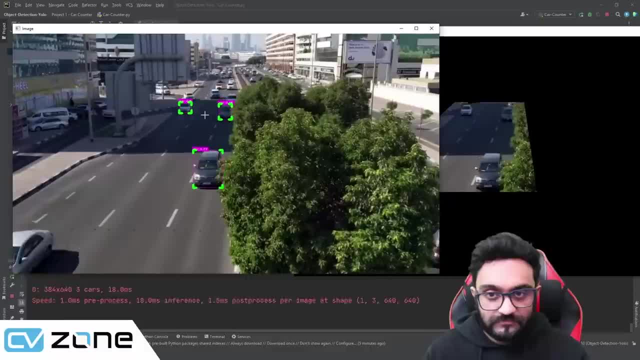 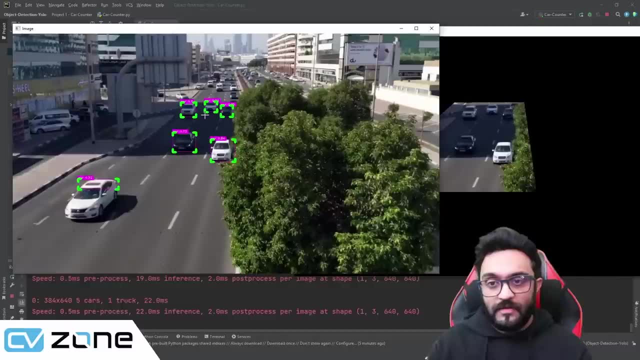 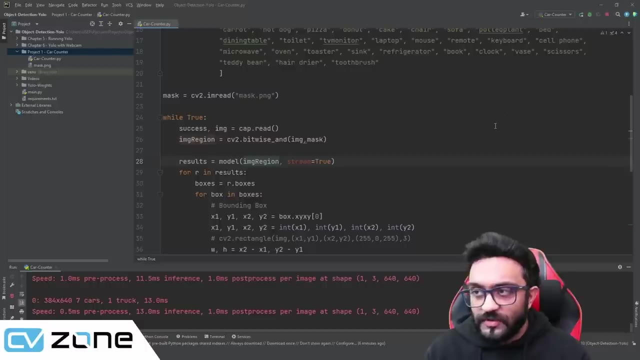 as a car or a bike and all that. so that's good. as you can see, it looks good. it yeah, okay, so now that we have a specified region and we can see all the cars being detected, now we need to count them. so, in order to count, we need to have a certain region. that 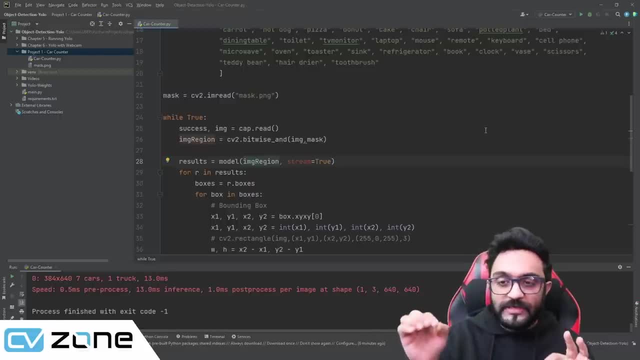 this is the line. when it passes this line, we will consider it as counted. so we need to know that. second thing we need is an actual tracker. so right now what we are doing is we are detecting the cars, but in the next frame we do not know where the car has gone. so what we need is a tracking id. 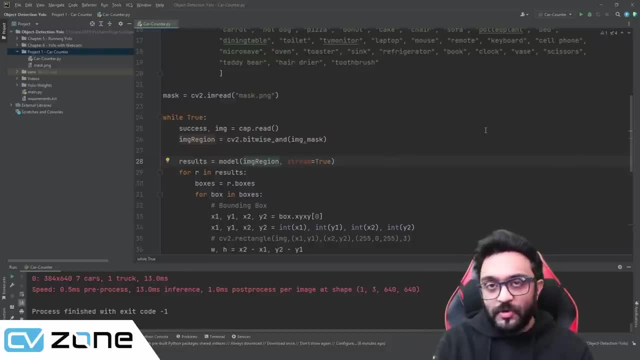 so if we detect a car in the first frame, we need to know where did that car go in the next frame so that we can assign it the same id. so in the first one if it's id number one in the second frame it should remain id number one. it should not go to id number two or 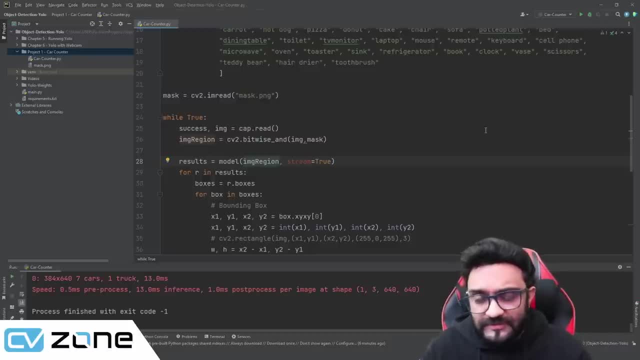 so it's not going anywhere in the next frame, but doesn't matter, because it's always there three or four or five. so this is basically a tracking problem. so within the consecutive frames we need to find out where is our object moving to, so that we can assign them unique ids, so to count. 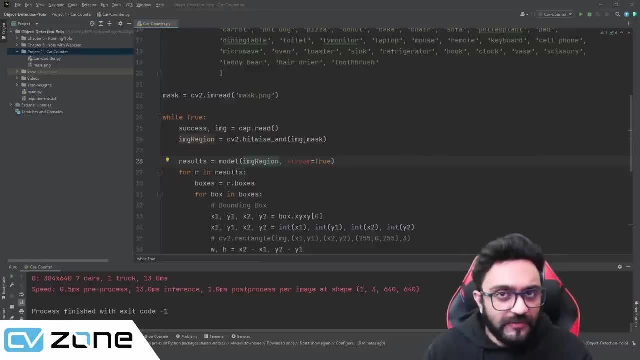 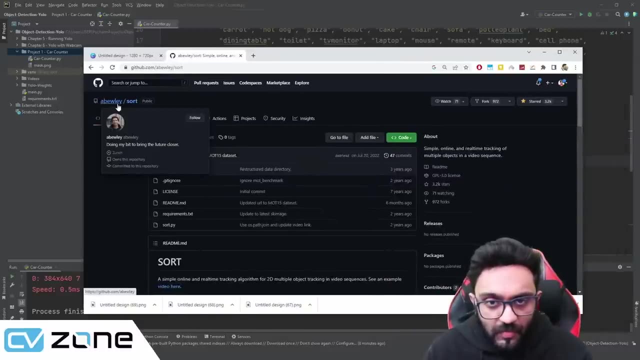 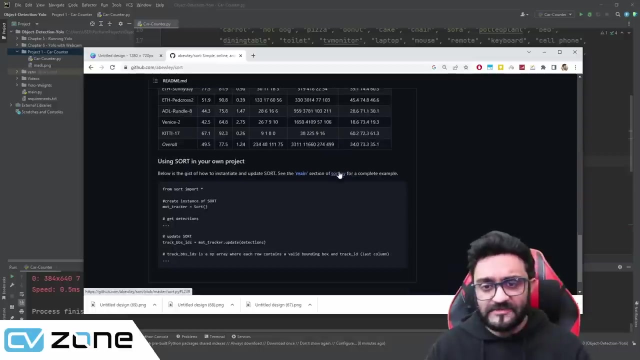 we need to find first a tracker. so the tracker that we are going to use is called sort and you can find it on github and here you can see it's by abby welly and thanks to him and the contributors who actually created this tracker and it is very easy to use, and here they are showing us. 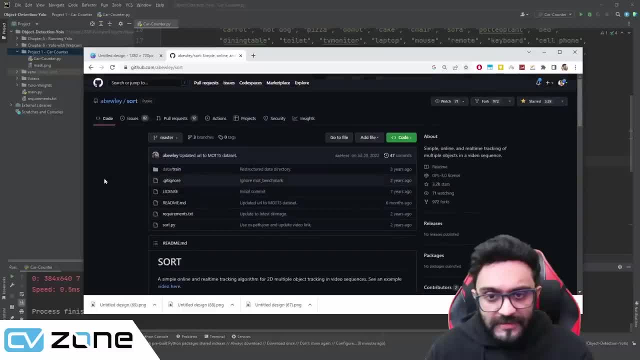 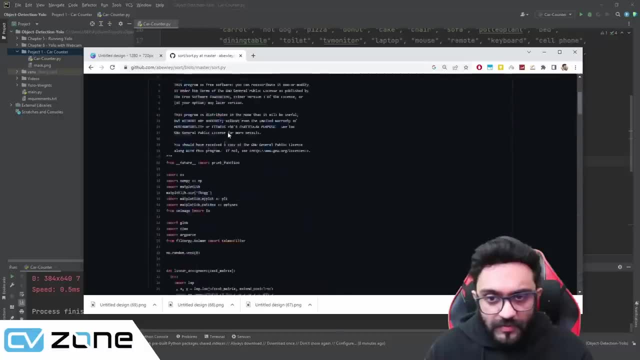 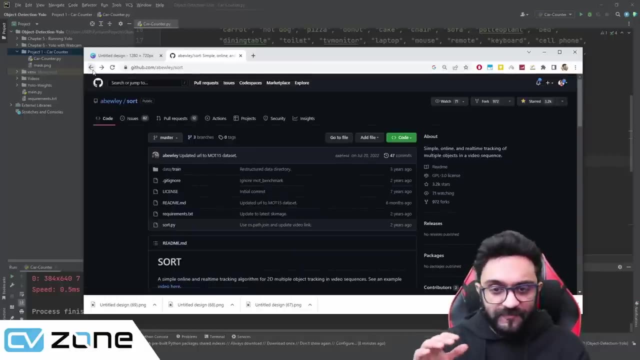 how to use as well. so all we need is this sortpy. so if we click on that, this is the code. what we will do is we will download this file. of course, this file will also be available with our zip file, so you can find it there, or you can come to github and download it from here. 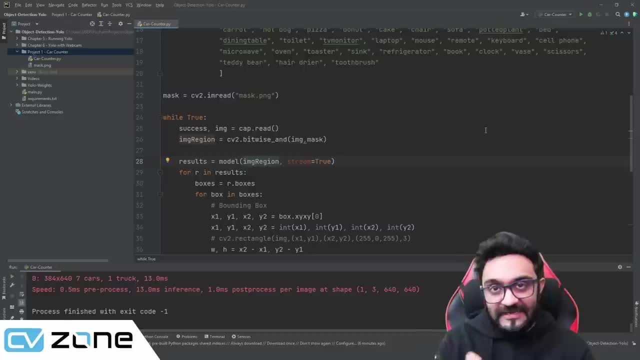 that car go in the next frame so that we can assign it the same ID. So in the first one if it's ID number one, in the second frame it should remain ID number one. It should not go to ID number two or three or four or five. So this is basically a tracking problem. So within the consecutive frames. 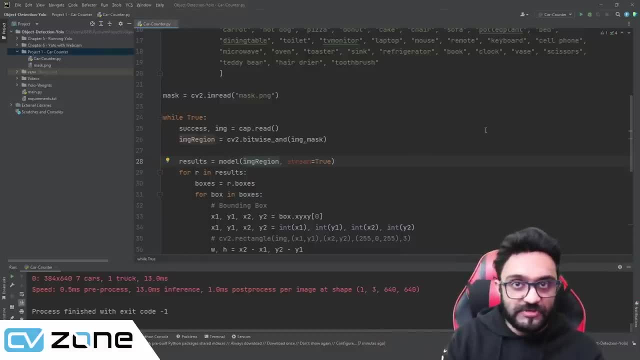 we need to find out where is our object moving to, so that we can assign them unique IDs. So, to count, we need to find first a tracker. So the tracker that we are going to use is called sort, and you can find it on github. 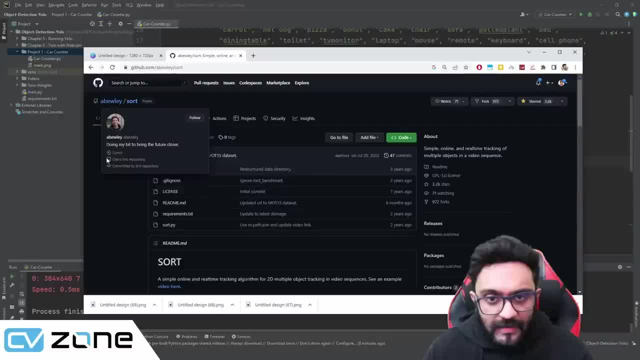 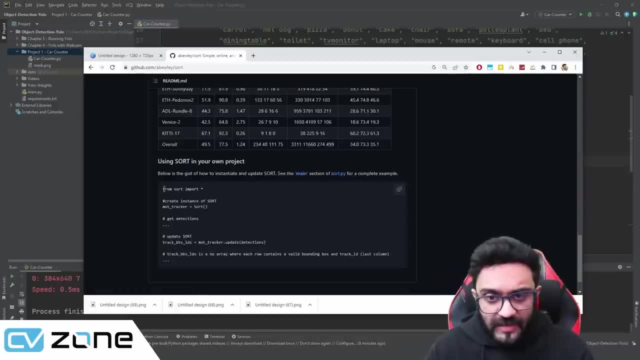 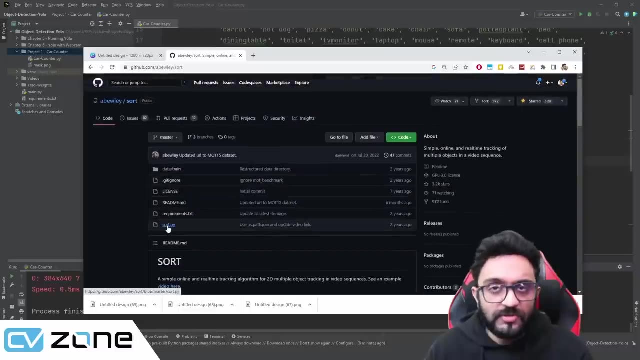 You can see, it's by Abby Welly and thanks to him and the contributors who actually created this tracker, and it is very easy to use, and here they are showing us how to use as well. So all we need is this sortpy. So if we click on that, this is the code. What we will do is we will download this. 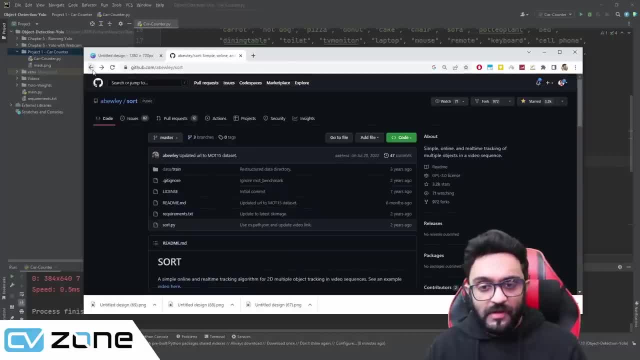 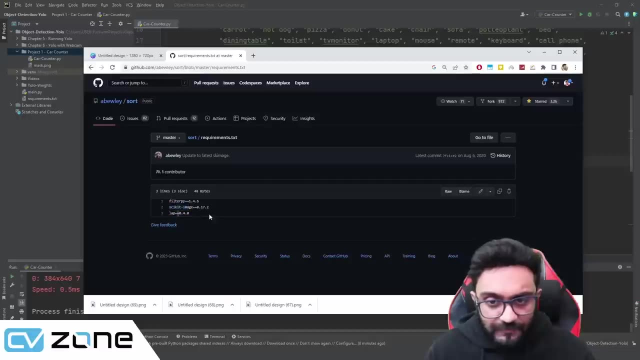 file. Of course, this file will also be available with our zip file, So you can find it there or you can come to github and download it from here. So we also have some requirements: filterpy, scikit-image and lap. So these requirements are already fulfilled because 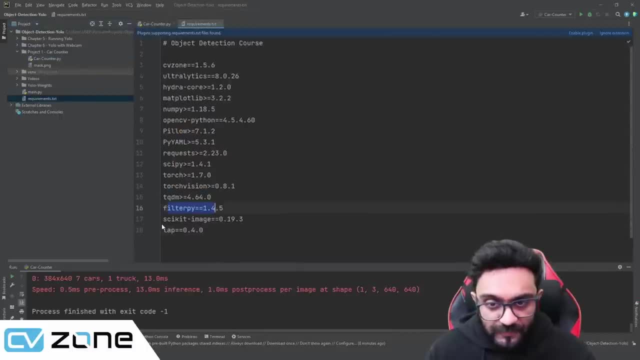 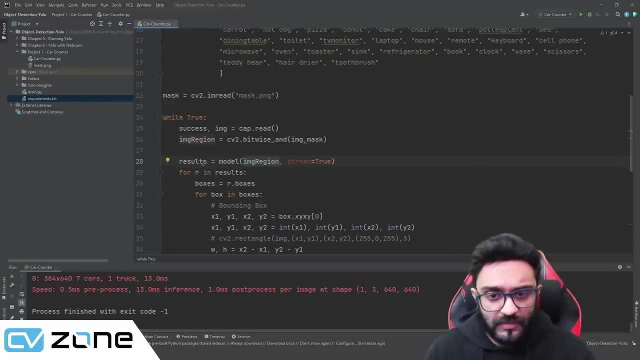 we added that in our requirements as well. So filterpy, scikit-image and lap, So these are the ones that we have already installed. So what we need to do is we need to bring in the file. So let me do that And I will bring it here into our project one. and this is a simple sorter, a simple. 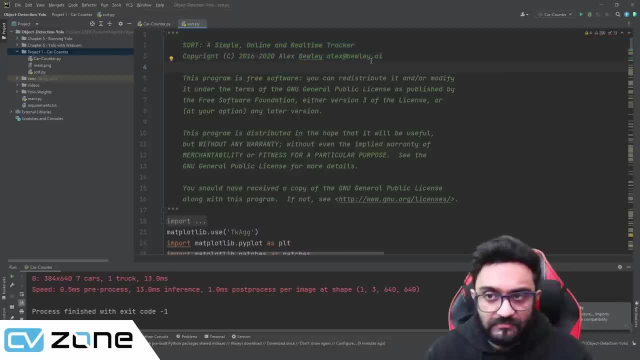 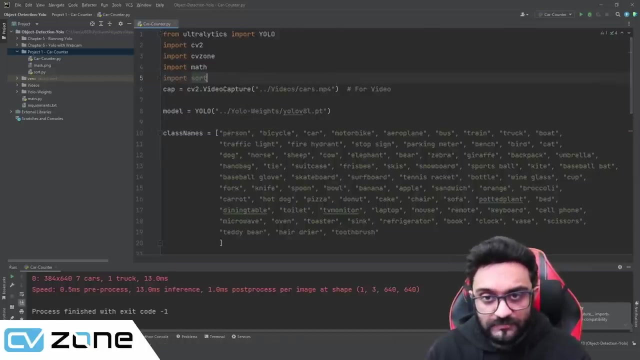 online and real-time tracker. Copyright: Alex Beverly. You can see here. So this is all the code. We are not going to do anything to this. All we have to do is we need to know how to use it. So here to import, we are going to write: import sort. 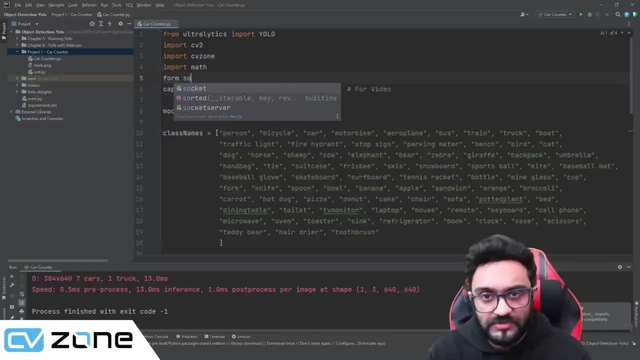 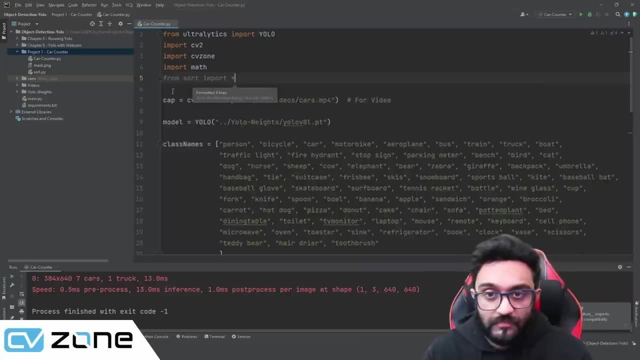 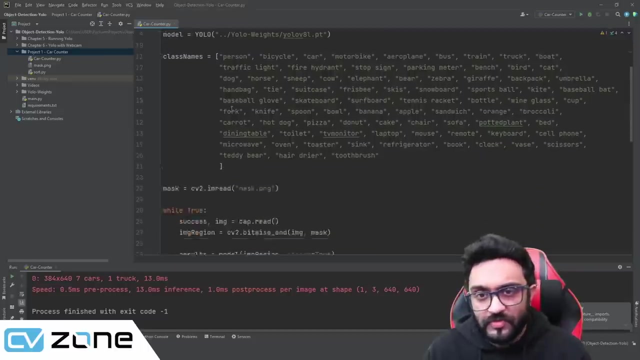 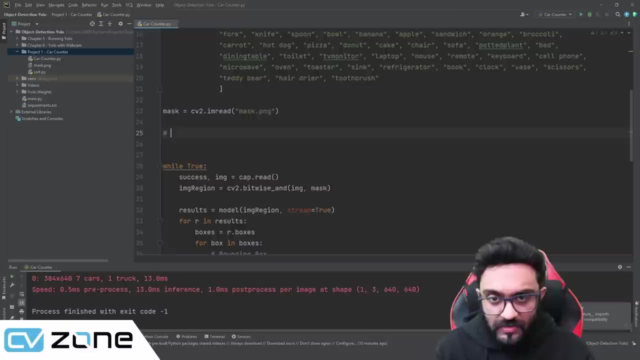 Or actually, what we can do is we can write from sort, from sort, import everything, So it will be easier for us to work with. So this is what we are going to do, And then we are going to create an instance for the sorter. So what we will do is sorting, or let's call it tracking. 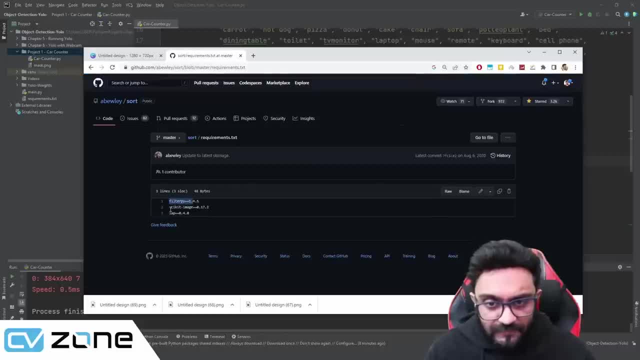 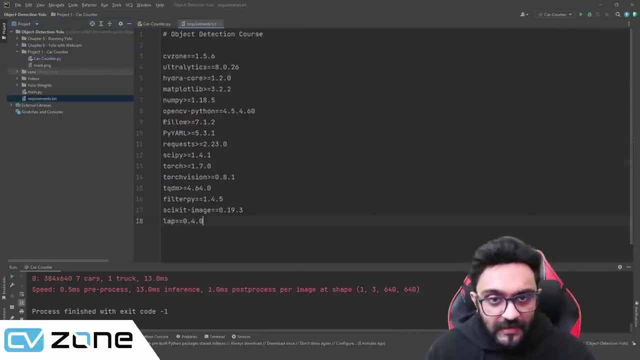 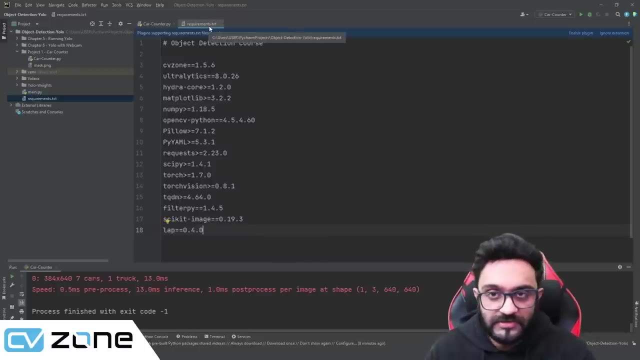 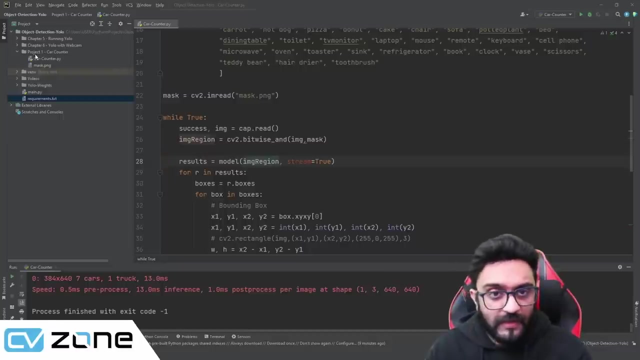 so we also have some requirements- filter by psychic image and lap. so these requirements are already fulfilled, because we added that in our requirements as well. so filter by psychic image and lap- so these are the ones that we have already installed. so what we need to do is we need to bring in the file. so let me copy that and i will bring it here into our project one. 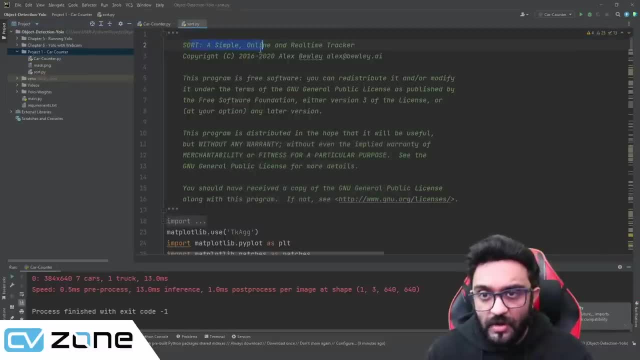 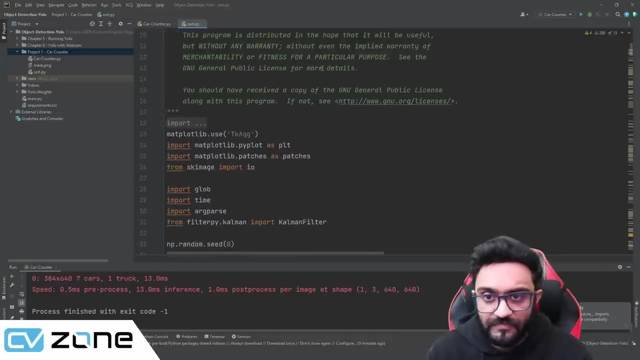 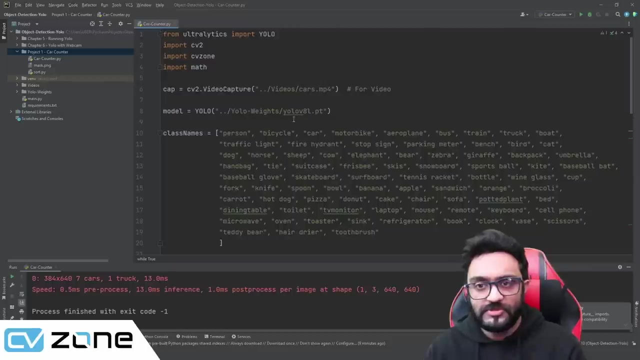 and this is, uh, a simple sorter, uh, a simple online and real-time tracker. uh, copyright alex beverly. you can see here. so this is all the code. we are not going to do anything, uh to this. all we have to do is we need to know how to use it. so, here to import, we are going to write: import sort. 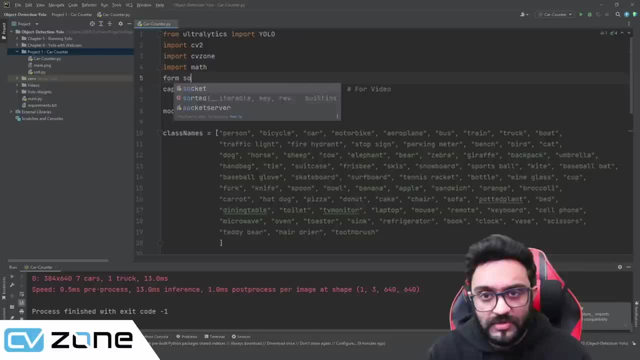 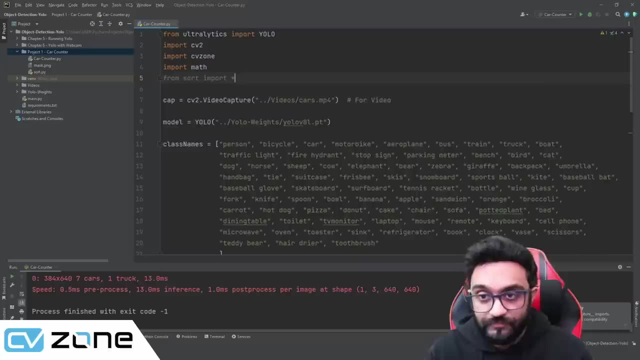 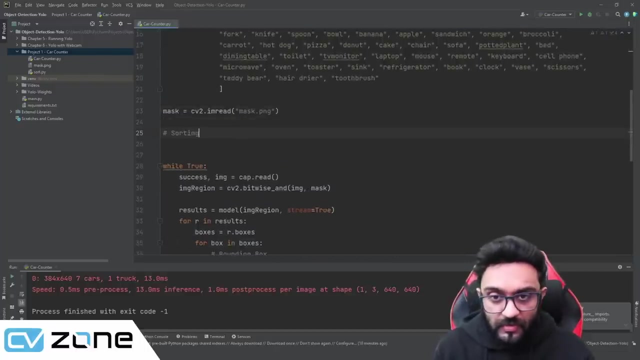 or actually, what we can do is we can write from sort, from sort, import everything, so it will be easier for us to work with. so this is what we are going to do, and then we are going to create an instance for the sorter. so what we will do is sorting, or let's call it tracking. 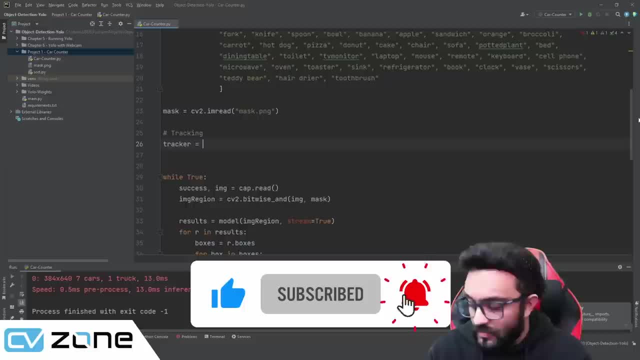 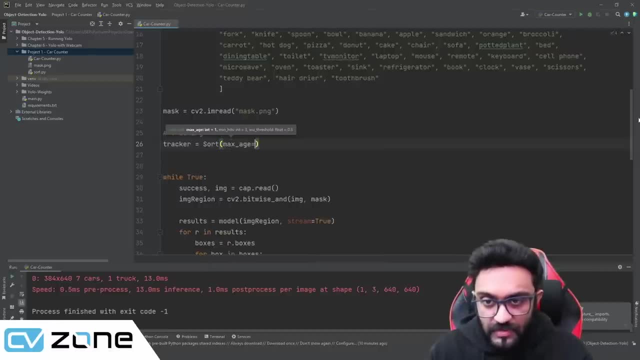 tracker equals sort, and then we have to give in the maximum age. so what is the limit of the number of frames? uh, that it is gone and we still recognize it within that region. so if id number one is lost, how many frames do we wait to detect it back? so the higher, the longer it will wait for it to come back. so maximum age. 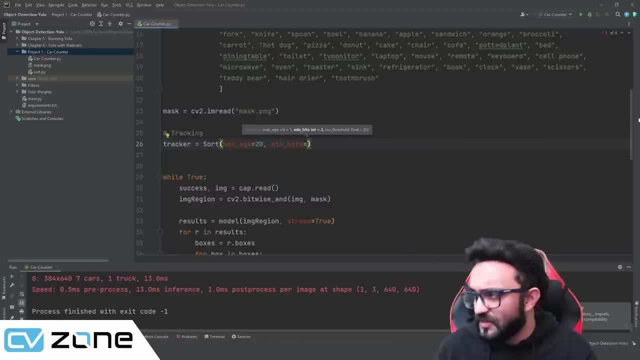 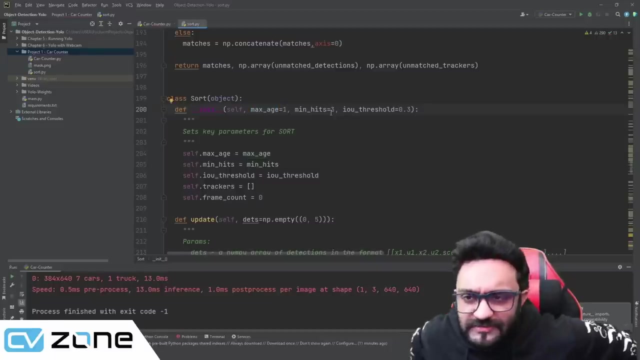 let's put it as 20 minimum hits, let's put it as two, and then we have the iou threshold again. these are parameters that you can change, but they have default values as well. if you go to sort, maximum age is one which is really bad. uh, it's not really useful. then we have minimum. 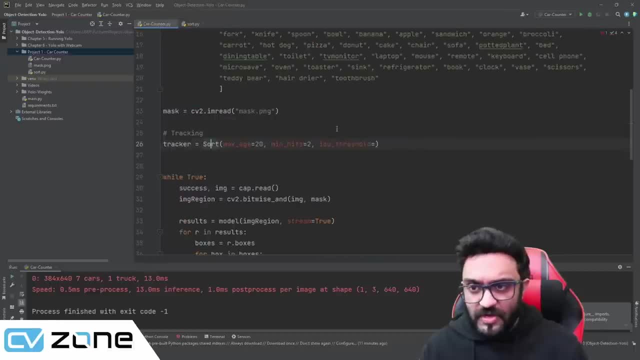 hits as three and the iou threshold as 0.3. so i will, i will keep them the same. uh, let's put it as three and iou threshold is 0.3. so again, um, this we have explained in the theory part, so if you're not, 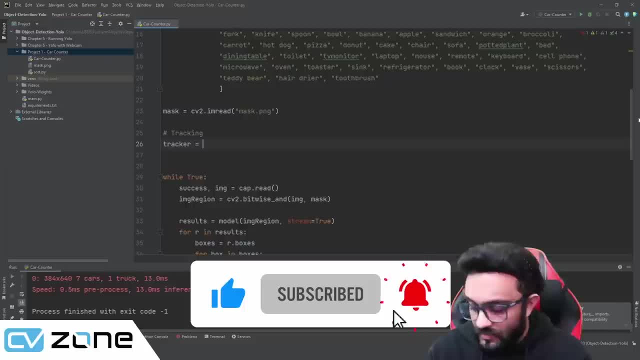 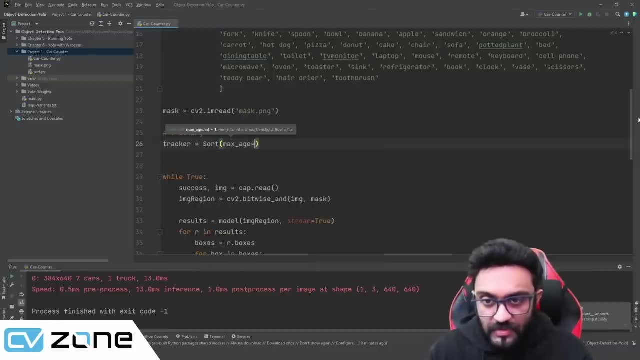 Tracker equals sort, and then we have to give in the maximum age. So what is the limit of the number of frames that it is gone and we still recognize it within that region? So if ID number one is lost, how many frames do we wait to detect it back? 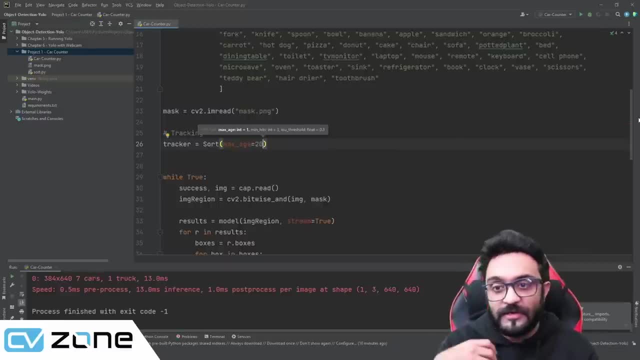 So the higher, the longer it will wait for it to come back. So maximum age: Let's put it as 20.. Minimum hits: Let's put it as two. And then we have the IOU threshold. Again, these are parameters that you can change, but they have default values as well. 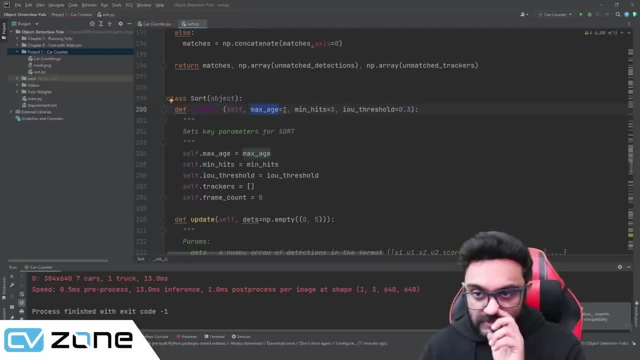 If you go to sort, maximum age is one which is really bad. It's not really useful. Then we have minimum hits as three and the IOU threshold as 0.3.. So I will keep them the same. Let's put it as three. 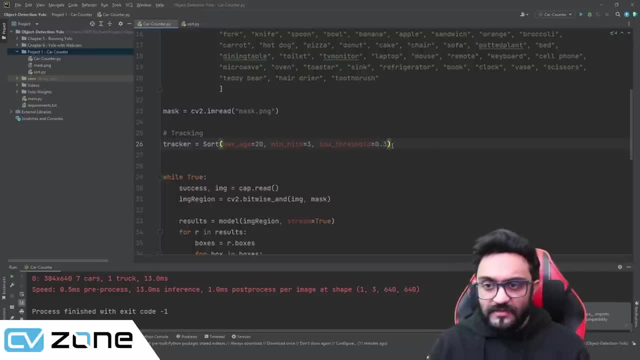 And IOU threshold is 0.3.. So again, this we have explained in the theory part, So if you're not familiar with this, go ahead and check that out. This is the intersection over union threshold to find how good the overlap of the bounding boxes is. 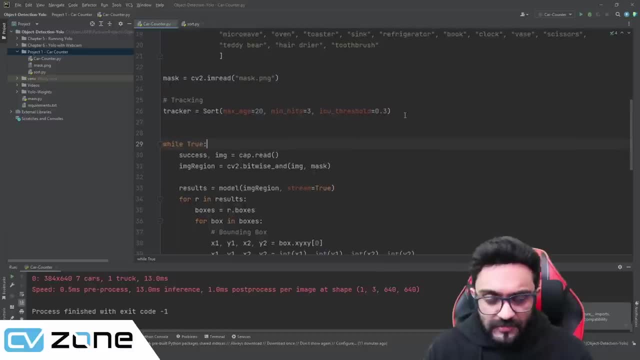 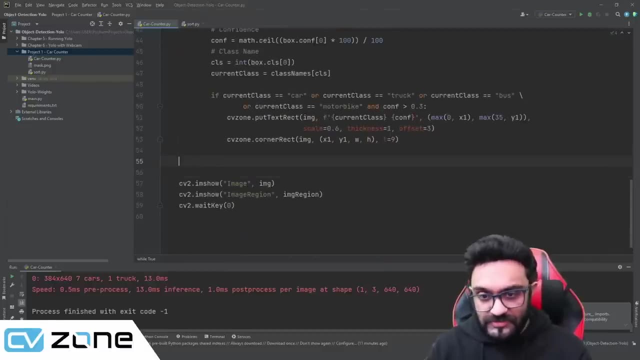 So these are the values. you can play around with them and see what type of results you get. Now, in order to run this, it's very, very simple. All you have to do is you have to write tracker dot- update And that's it. 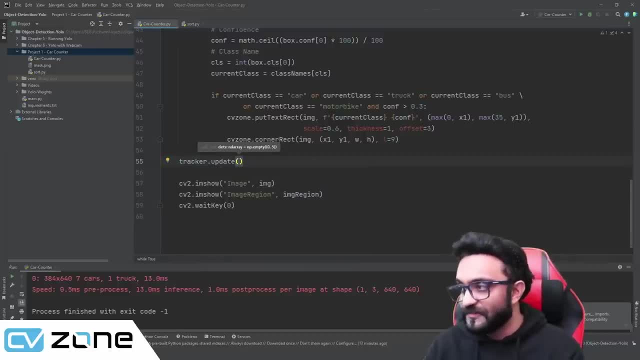 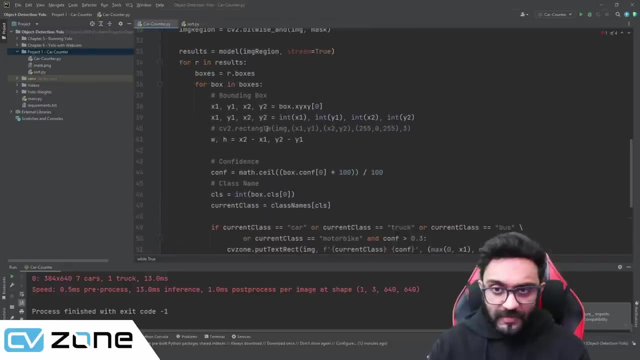 So you need to update it with a list of detections. So we will write here detections. Now we need to find these detections, which we already have, by the way, because here we have the bounding boxes, But what we need to do is we need to put them in an array. 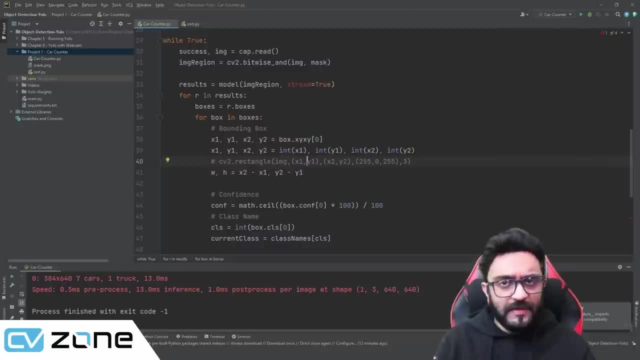 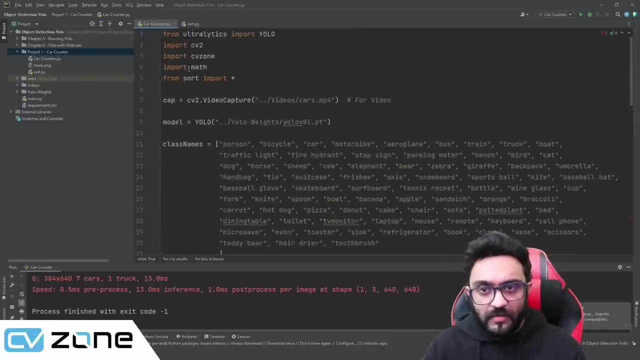 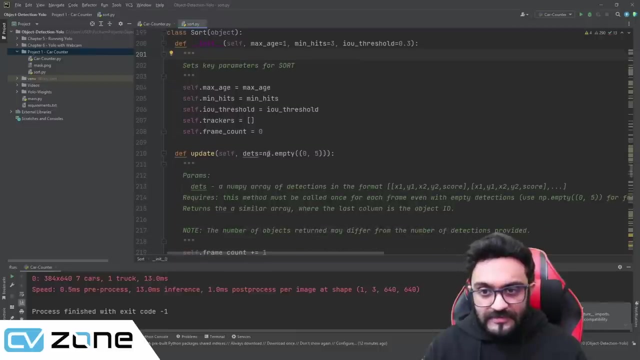 We need to put them in a list And we need to make sure that the format is exactly what this requires. So what format does it need? We don't know. We can go into the sort and we can check here. So in the update it says this is a numpy empty. 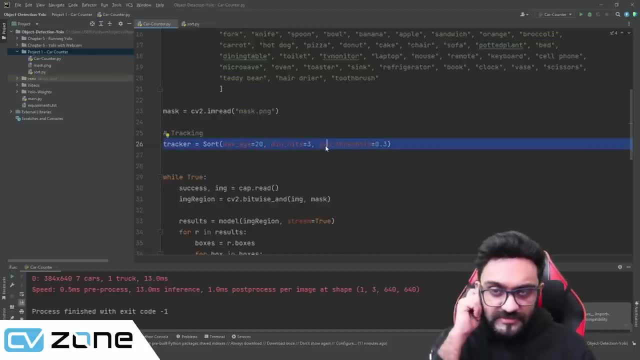 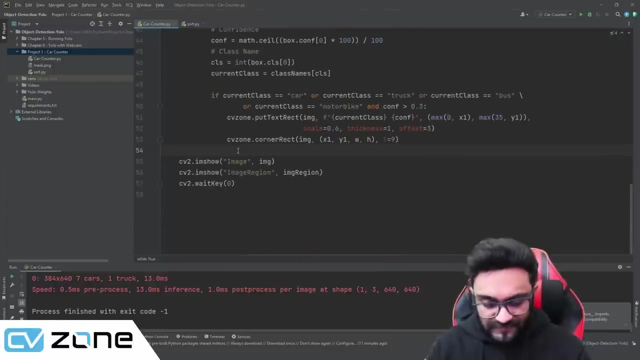 familiar with this. go ahead and check that out. uh, this is the intersection over union threshold to find how good the overlap of the bounding boxes is. so, uh, these are the values. you can play around with them and see what type of results you get. now, in order to run this. it's very, very. 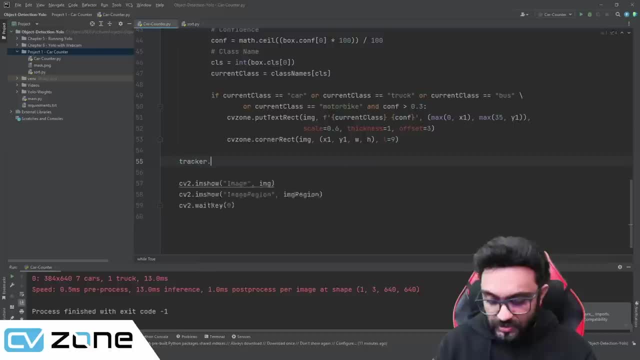 simple. all you have to do is you have to write tracker dot update and that's it. so you need to update it with a list of detections. so we will write here detections now. we need to find these detections, which we already have, by the way, because here we have. 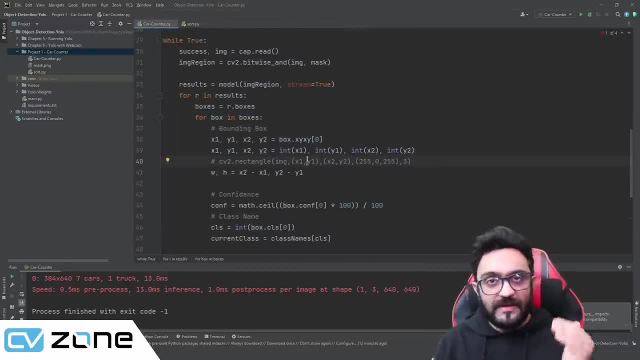 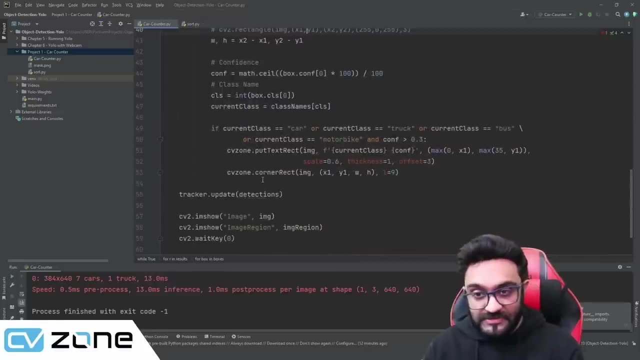 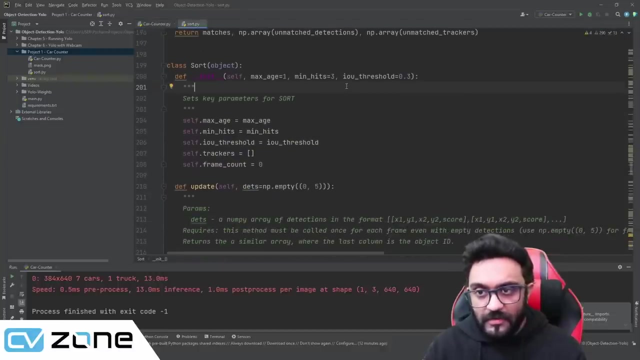 the bounding boxes, but what we need to do is we need to put them in an array, we need to put them in a list and we need to make sure that the format is exactly what this requires. so what format does it need? we don't know. we can go into the sort and we can check here. so in the update it says: 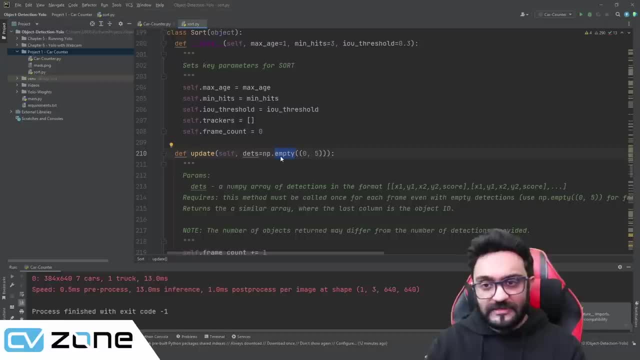 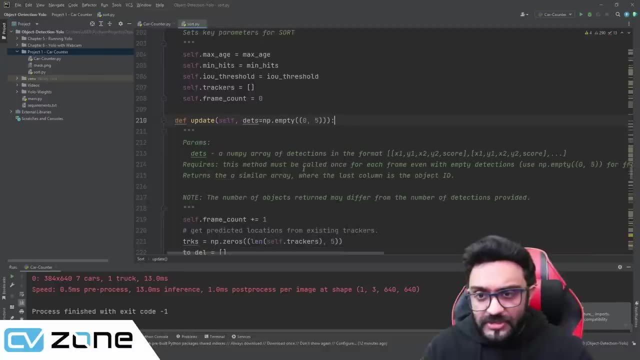 this is a numpy empty, so by default it's a numpy array of 0 by 5.. so this is the dimension, so we have five values. so, uh, the format is x1, y1, x2, y2 and the score. so this is what we have to feed in, and what do we get out of it? we get erect. 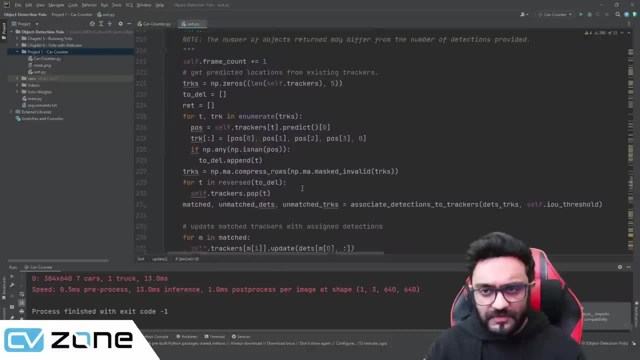 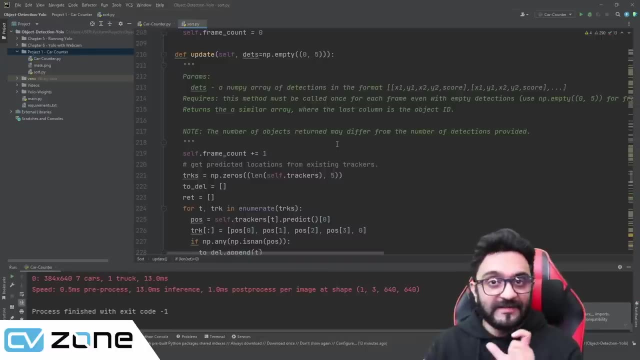 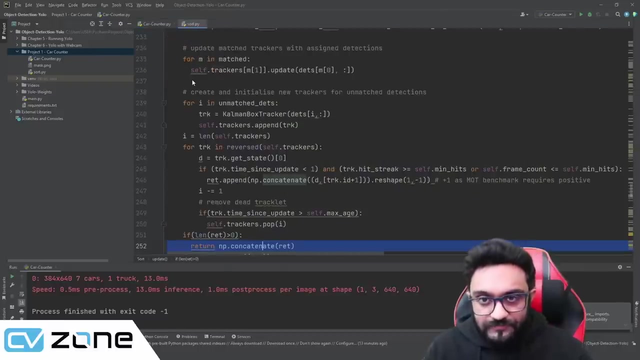 concatenated. um, maybe it's not mentioned here. what we get as the output or the return is x1, y1, x2, y2, and then we also get the main thing, which is the id number. so that is what we need, so let's just copy that. so where is the update here? so our detections by default, if we don't? 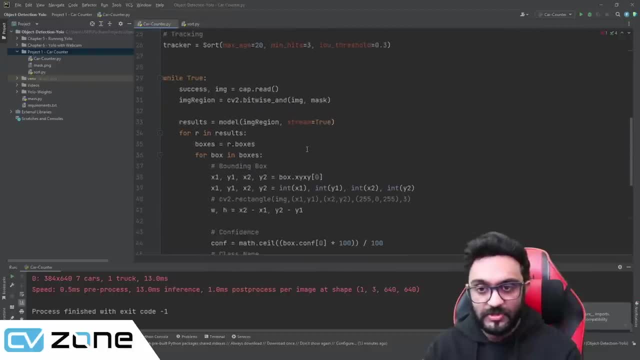 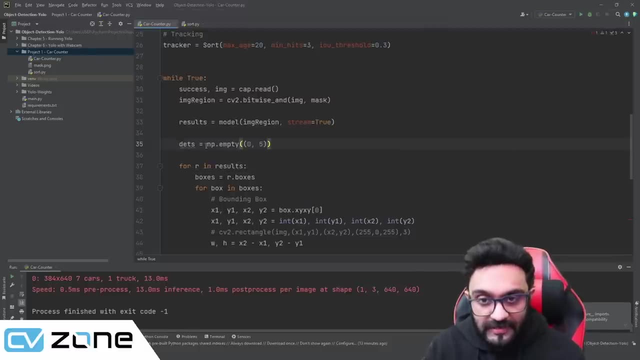 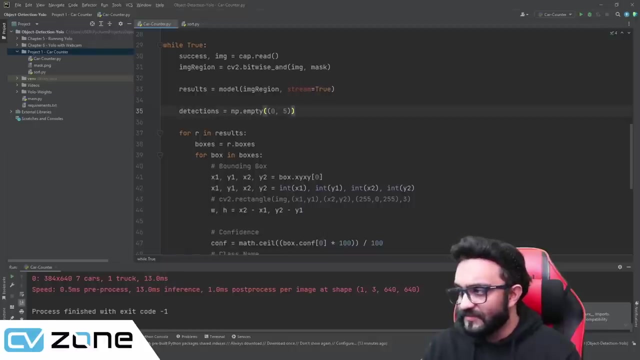 have any detections. this should be our type, so we should have a numpy list. so right after we get the results, we are going to create a list or a array of detections, detections, and this will be empty: uh, 0 by 5.. so that is the idea, and once we have that, 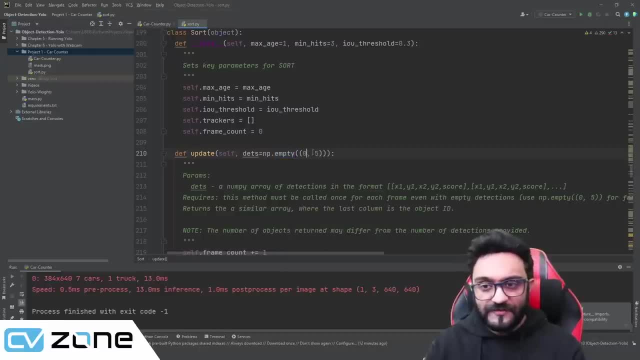 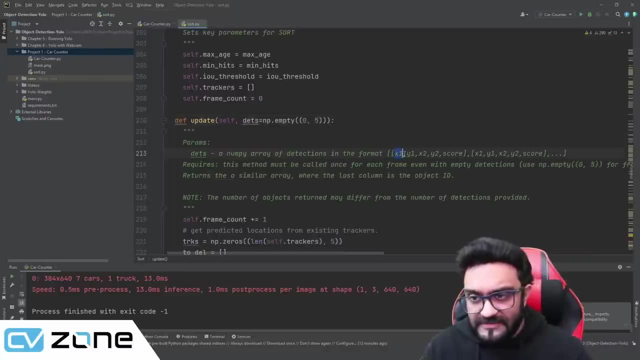 So by default it's a numpy array of zero by five. So this is the dimension, So we have five values, So the format is X1, Y1, X2, Y2, and the score. So this is what we have to feed in. 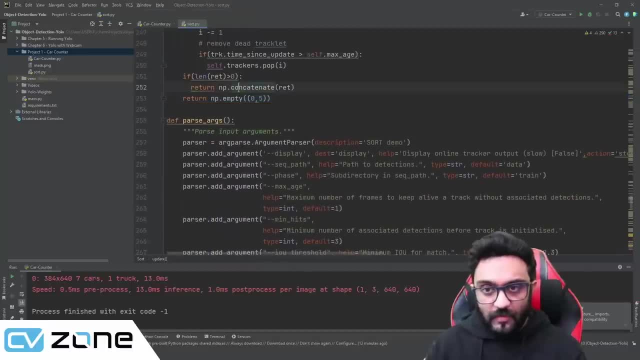 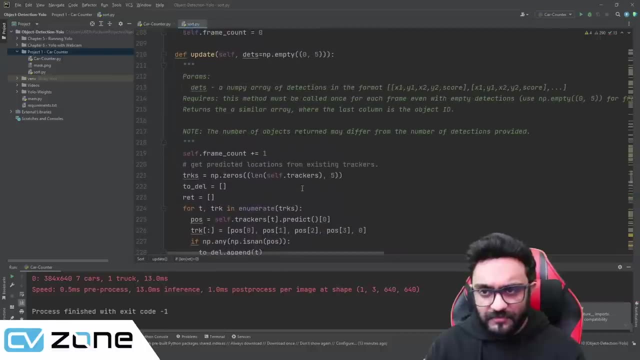 And what do we get out of it? We get erect concatenation. Maybe it's not mentioned here. What we get as the output or the return is X1, Y1, X2, Y2.. And then we also get the main thing, which is the ID number. 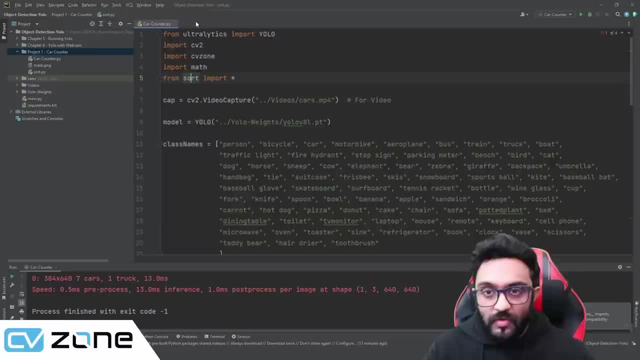 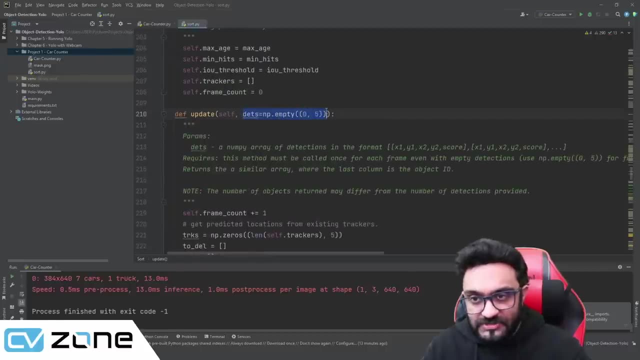 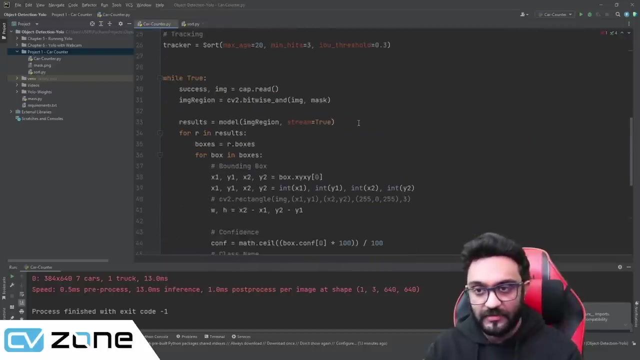 So that is what we need, So let's just copy that. So where is the update here? So our detections by default. if we don't have any detections, this should be our type, So we should have a numpy list. So right after we get the results, we are going to create a list or an array of detections. 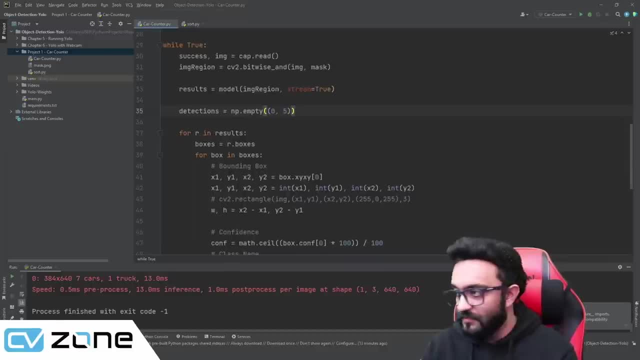 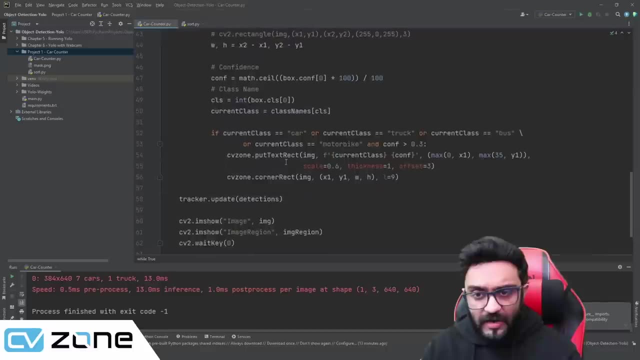 And this will be empty, zero by five. So that is the idea, And once we have that, then we are going to. once we detect it as a car or a truck or a bus or a motorbike, and the confidence is greater than 0.3,. 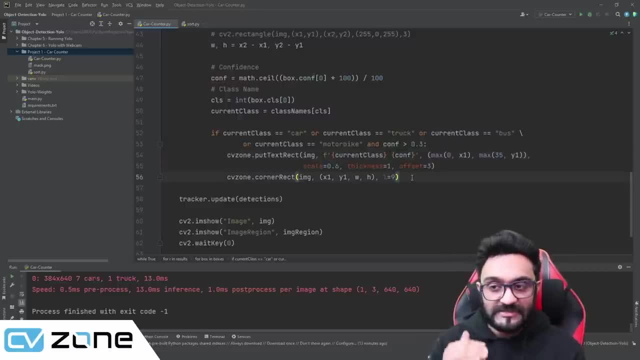 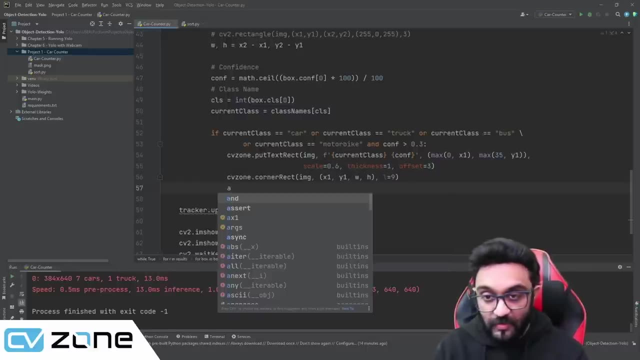 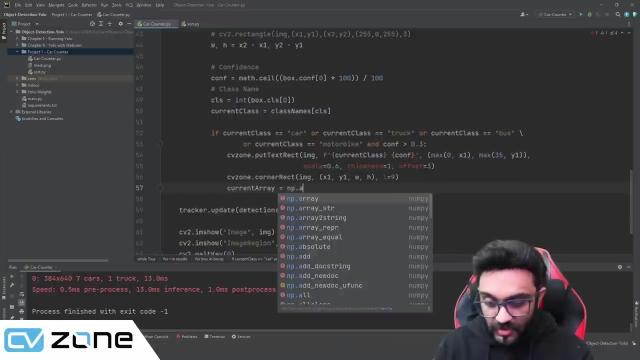 then only we are going to save it to our detection list or detection array. So then, what we are going to write? we are going to write that our current array equals numpy dot array, And we are going to give in the X1,, X1, Y1,, X2, and Y2.. 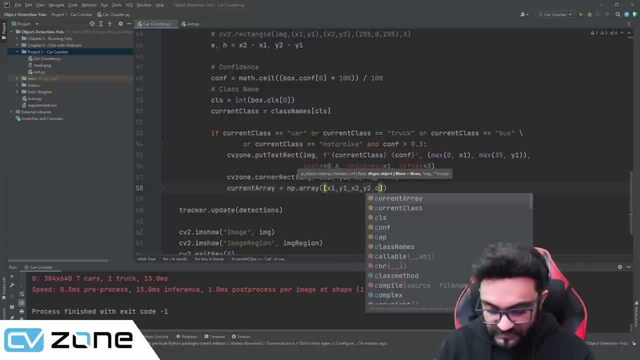 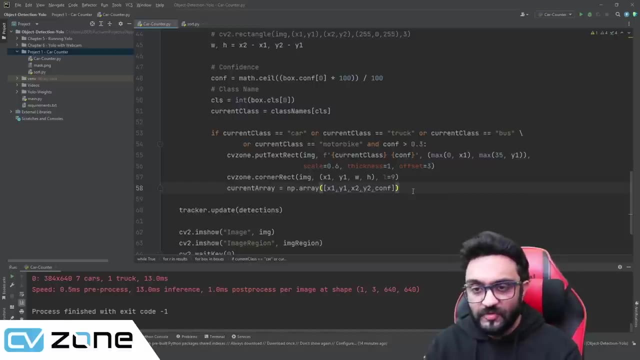 And we will also give in the confidence value. So these are the five values that it requires. And then what we have to do is: so, normally, if we have a list, what we do is we write dot append. So if you want to add it to the list, you just write append. 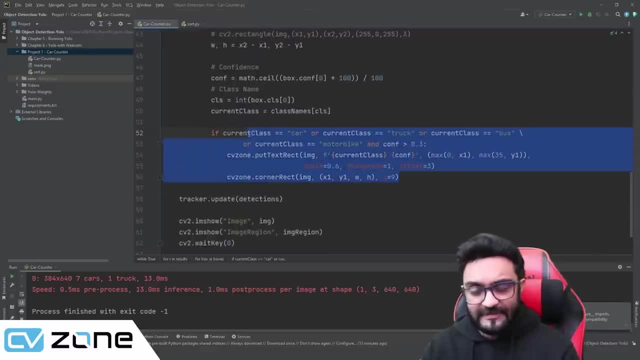 then we are going to, once we detect it as a car or a truck, or a bus or a motorbike and the confidence is greater than 0.3, then only we are going to save it to our detection list or detection array. so then, what we are going to write? we are going to write that 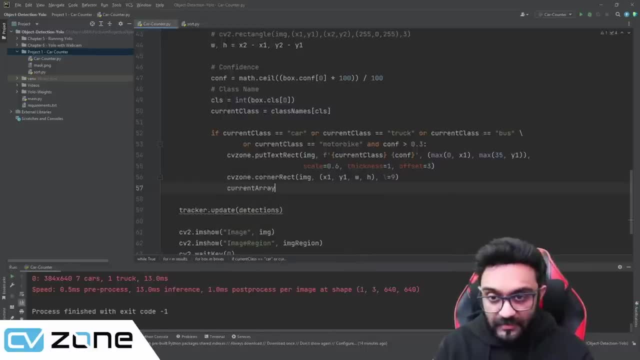 our current array equals numpy dot array and we are going to give in the uh x 1, x 1, y 1, x 2 and y 2, and we will also give in the confidence value. so these are the five values that it requires, and then what we have to do is: so, normally, if we have a list, what we do is we write dot, append. so 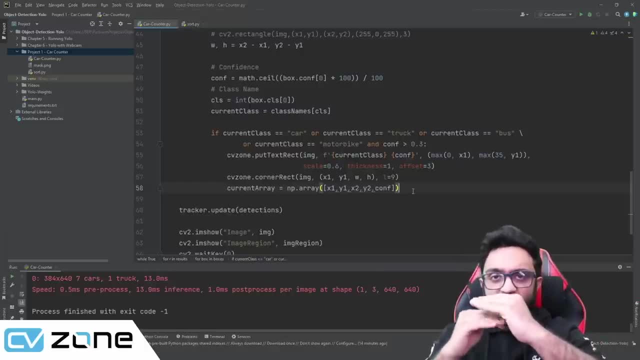 if you want to add it to the list, you just write append, it goes down, it goes down, goes down, like that. but in in a numpy array we don't write append, what we do is we stack. so we will do a vertical stack. that's how simple it is. so we'll write: detections: equals numpy dot, vertical stack. 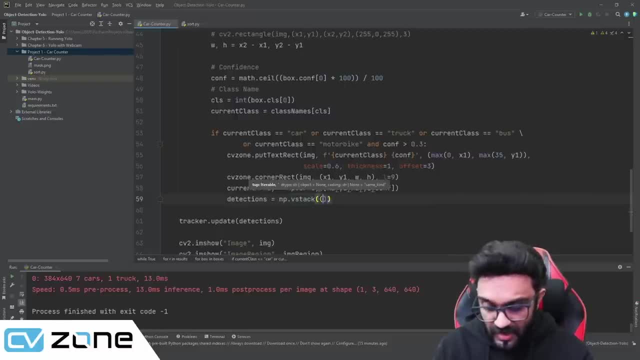 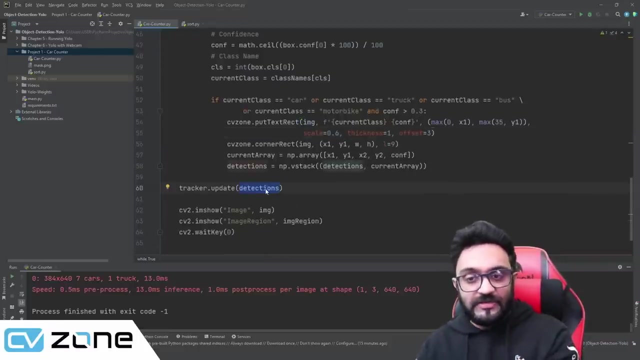 and we have to give in: uh, our current detection, the old detections that we already had, and the current array, the current array. so we stack them together. so that's the idea. so once we have these detections now, we can simply send it to the updates and again. 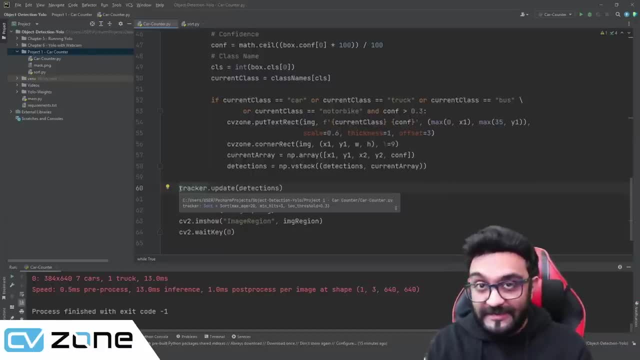 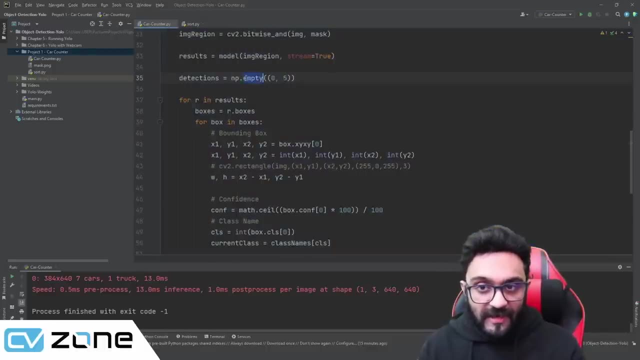 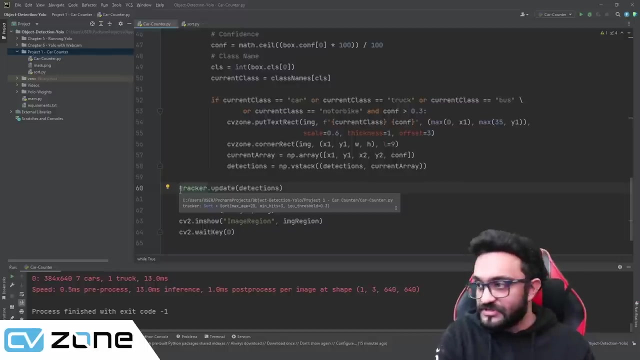 this update is not dependent on what did we detect new, because we need to keep updating it from the previous times as well. so we already have an empty one and it will keep updating. so here we have the detections and then we need to get the results of this so we can write here results for the tracker. 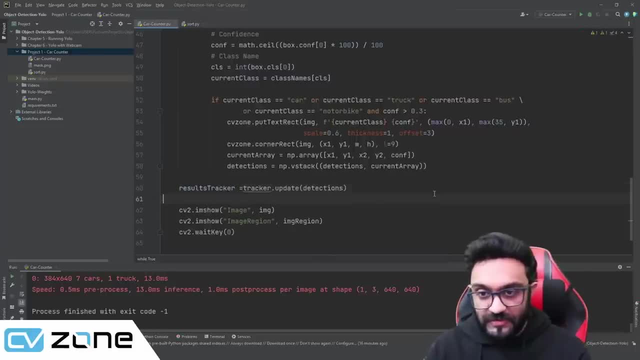 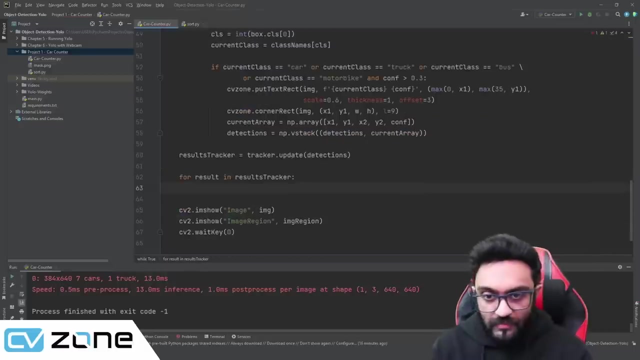 equals this, results of the tracker equals this and then we can loop through the results of this tracker so you can write, for example, for results in results tracker. we are going to get the x1, y1 and the x2 and the y2 and the id, so which is the most? 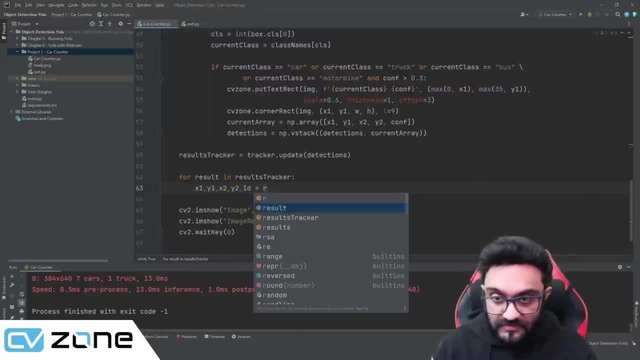 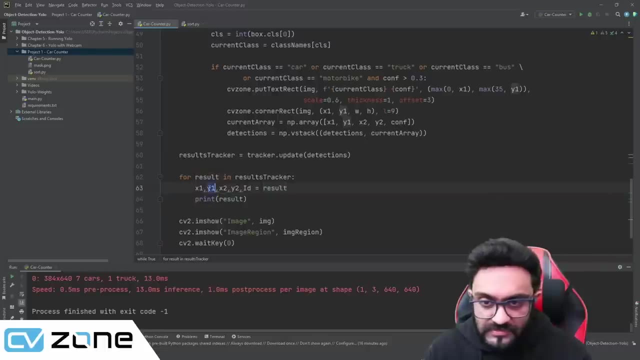 important thing that we get the id and that is basically the result. so let's print out the results. actually, we can print out this as well. later on we are going to use this. that's why we are writing it like that. so let's run that and see if we get something. hopefully there are no errors, um. 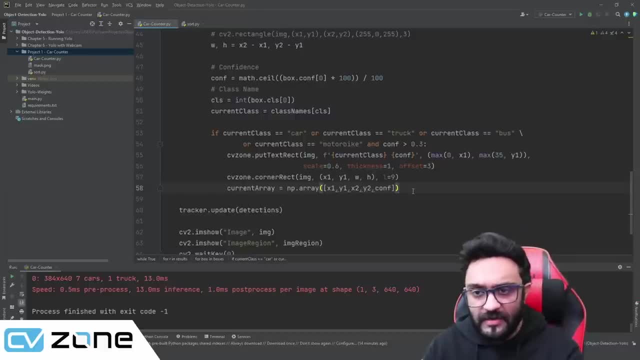 It goes down, it goes down, it goes down, like that. But in a numpy array we don't write append. What we do is we stack, So we will do a vertical stack. That's how simple it is. So we'll write: detections: equals numpy dot vertical stack. 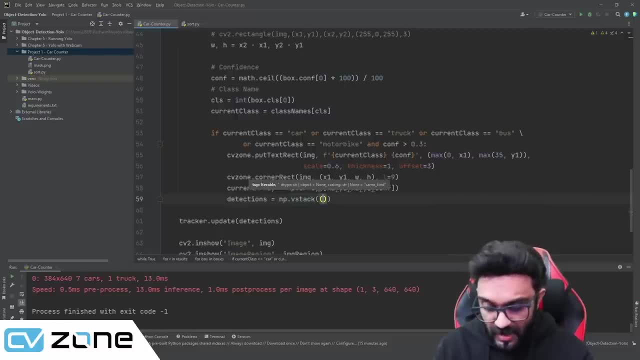 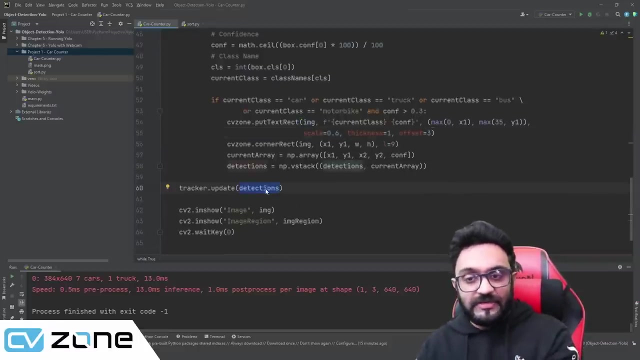 And we have to give in our current detection the old detections that we already had And the current array The current array. So we stack them together. So that's the idea. So once we have these detections now, we can simply send it to the updates. 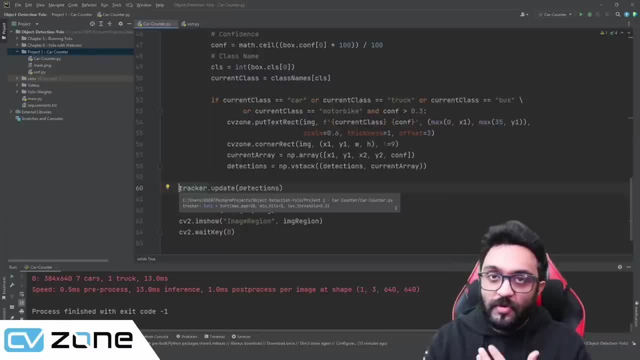 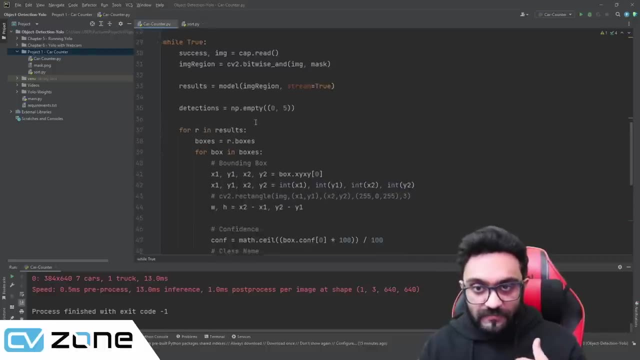 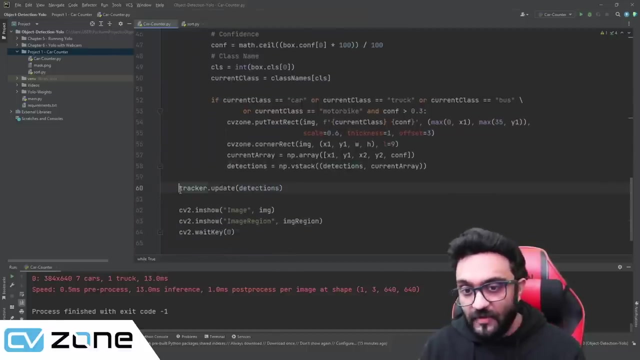 And again, this update is not dependent on what did we detect new, Because we need to keep updating it from the previous times as well. So we already have an empty one and it will keep updating. So here we have the detections, And then we need to get the results of this. 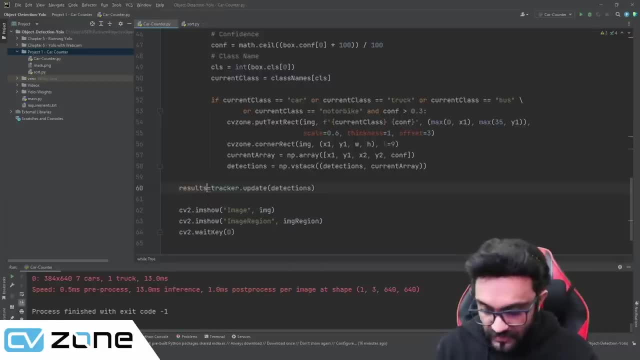 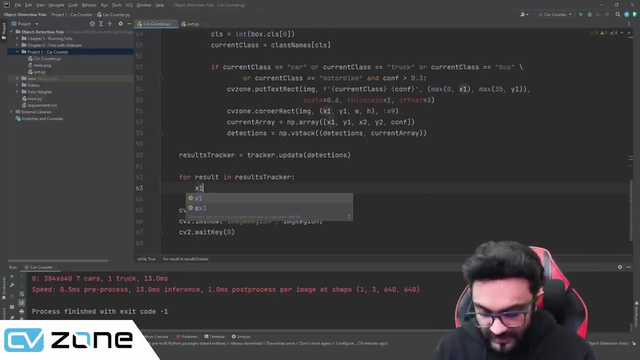 So we can write here: results for the tracker equals this, Results of the tracker equals this, And then we can loop through the results of this tracker. So you can write, for example, for results in results tracker, we are going to get the X1, Y1. 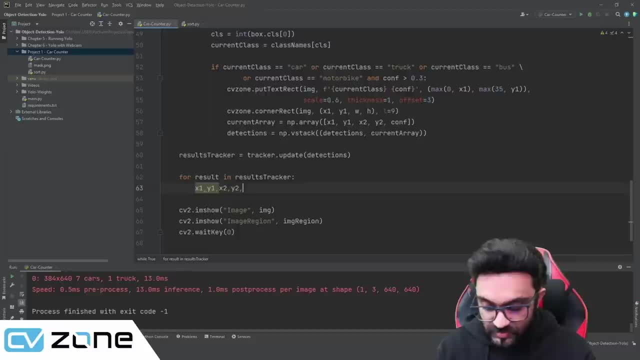 And the X2 and the Y2 and the ID. So, which is the most important thing, that we get the ID And that is basically the result. So let's print out the results. Actually, we can print out this as well. Later on we are going to use this. 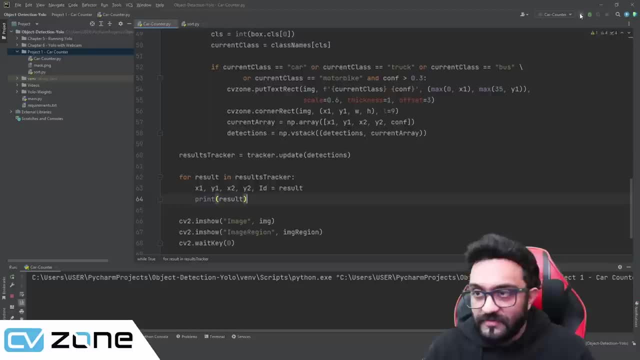 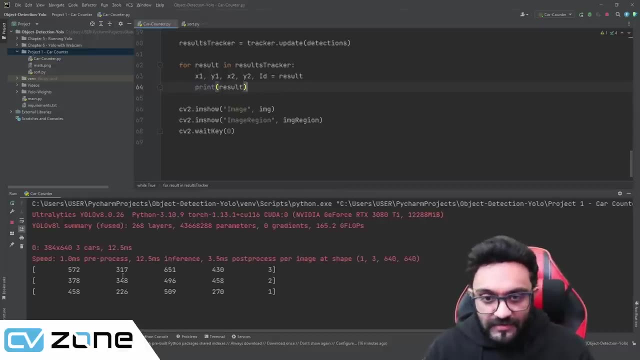 That's why we are writing it like that. So let's run that and see if we get something. Hopefully there are no errors, Otherwise we are heading in the wrong direction. Okay, there you go. So now we have our three IDs. 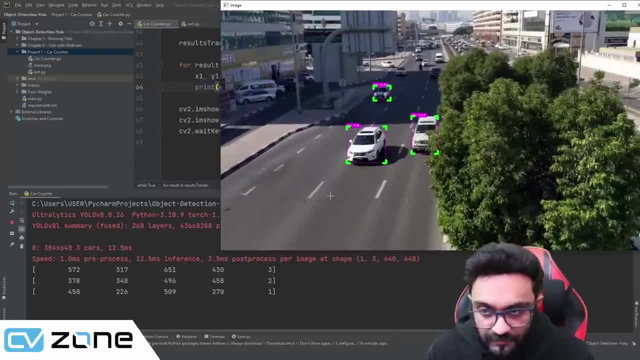 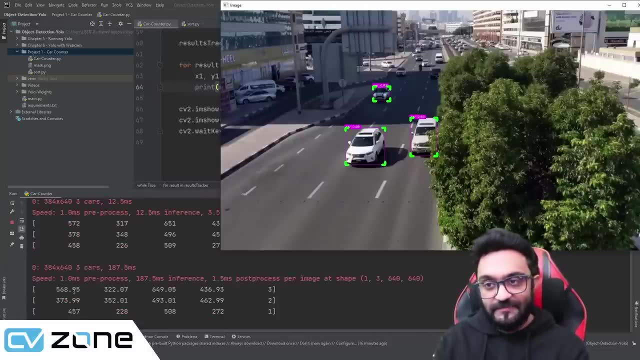 Perfect. So we have ID number 1, ID number 2, ID number 3.. Let's press spacebar And then again it is moving on to the next one And you can see it's the same ID. Then it moves on to the next one. 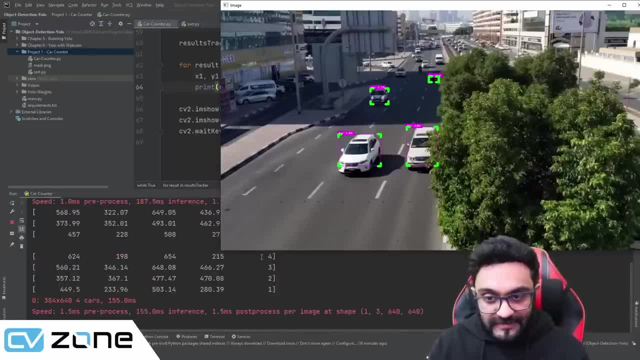 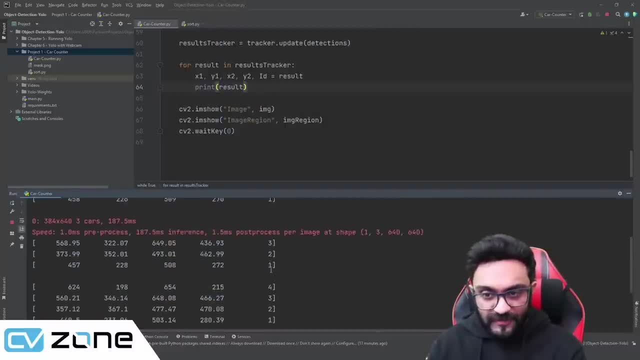 And you can see the fourth one has come up And it has increased the ID. There you go, And then the fifth one comes in And it shows It couldn't find probably the other two And that's why it's showing only three. 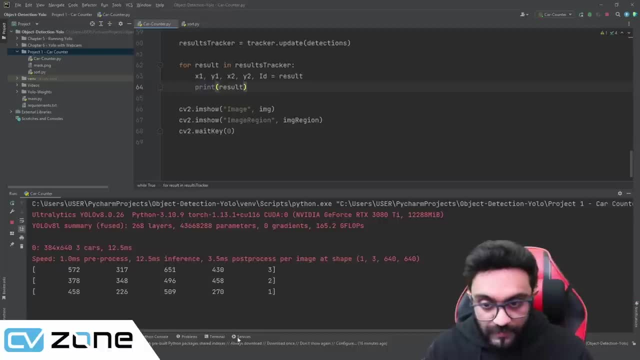 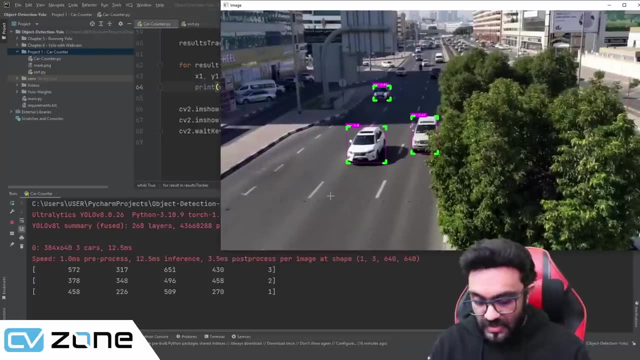 otherwise we are heading in the wrong direction. okay, there you go. so now we have our three ids. perfect, so we have id number one, id number two, id number three. let's press spacebar and then again it is moving on to the next one and you can see it's the same id. 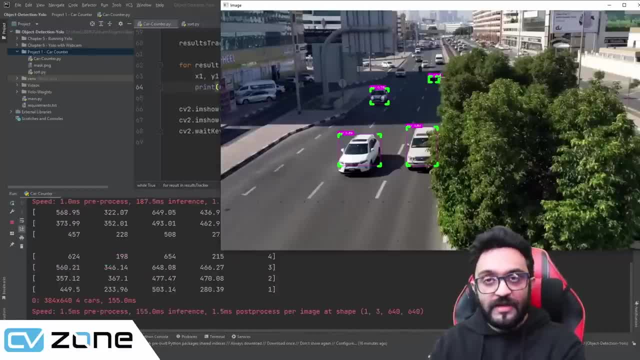 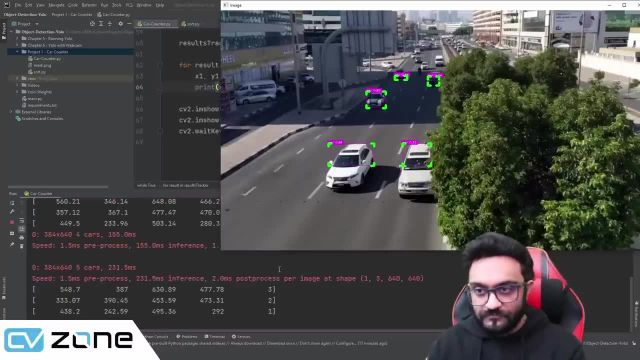 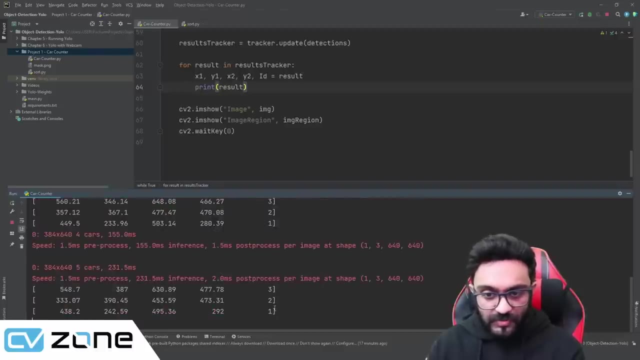 then it moves on to the next one and you can see the fourth one has come up and it has increased the id. there you go, and then the fifth one comes in and it shows: so it couldn't find probably, uh, the other two, and that's why it's showing only three. okay, so in order to understand this better, 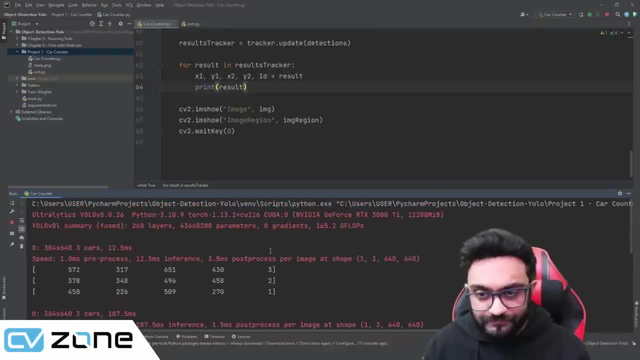 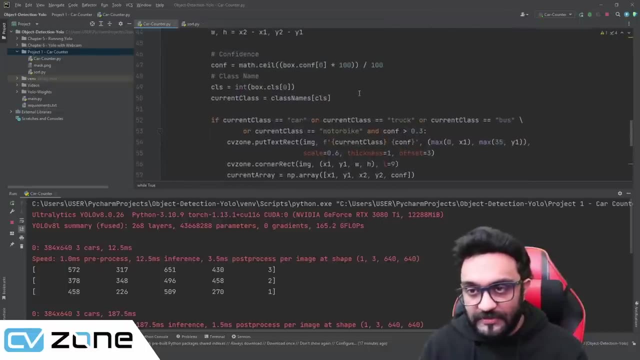 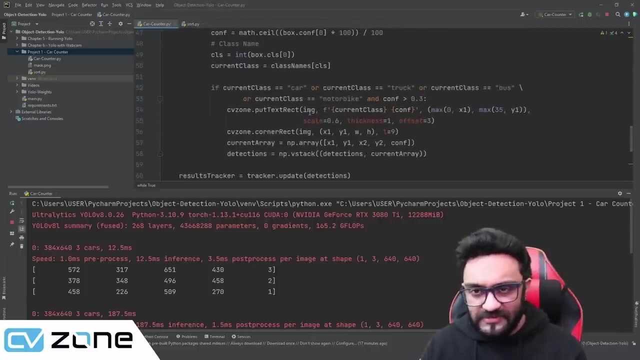 what we are going to do. uh, we are going to display these id numbers, so it will become easier. so, instead of uh showing it here, or let's do both, we'll show it here and we will show it here as well. we'll keep the thickness of this bigger. so we are talking about the rectangle, so the rectangle. 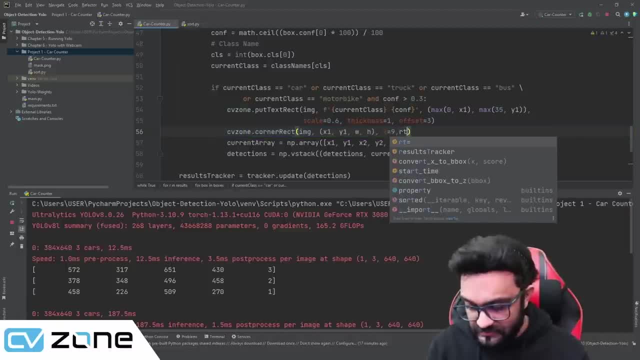 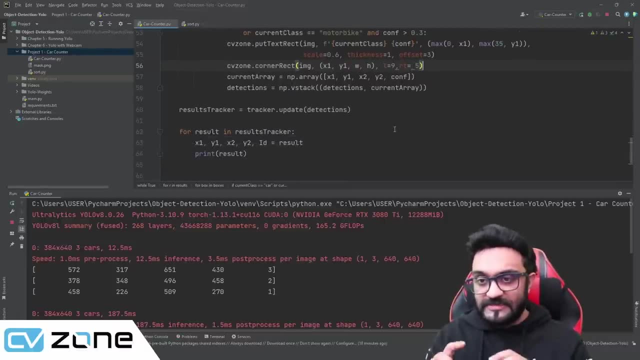 thickness here. so rectangle thickness equals, let's say, five, and for the other one we will make it a little bit smaller, so we can see what is the actual detection and what does it think. where is the tracking part? so how well the tracker detects the bounding box. so let's, let's try to. 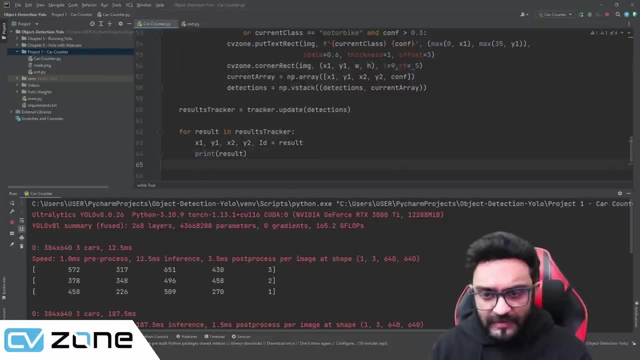 find that. so what we'll do is: uh again, what? uh? we will simply use these values. are they integers? yeah, they seem to be integers. so what we can do is we can simply uh, create our corner rectangle. so we will write here: uh, cv zone dots corner rectangle. 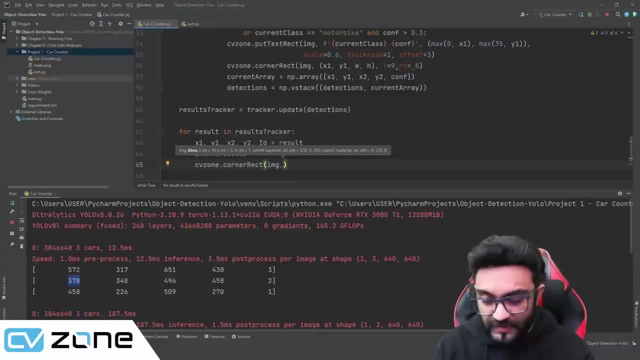 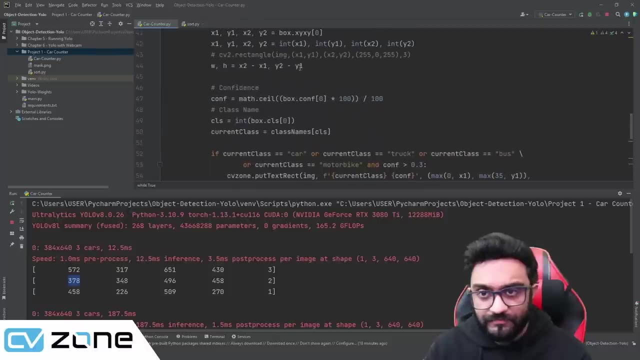 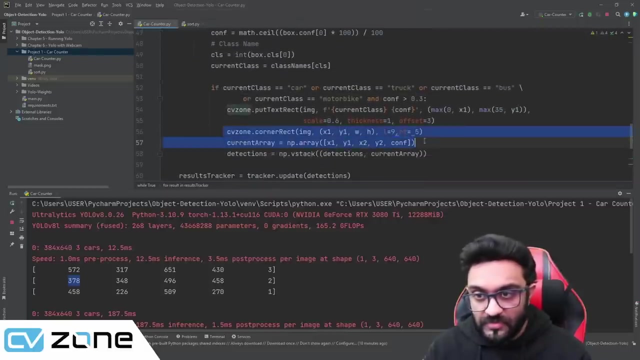 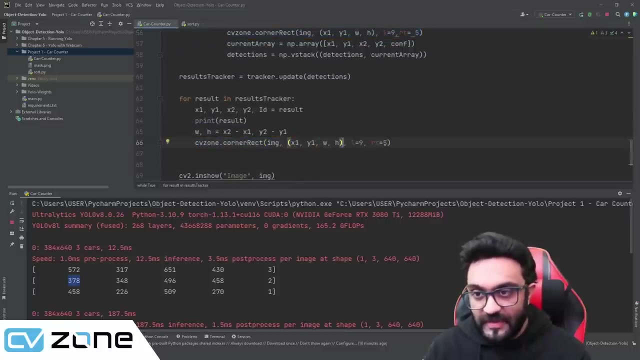 image and we have to give in the bounding box information. so the bounding box information, uh, will be like we did here, let's copy that. and uh, actually, let's copy this corner rectangle because we're lazy. so there you go. so x1, y1, width and height, and this time around we'll put the rectangle as: uh, let's say two. 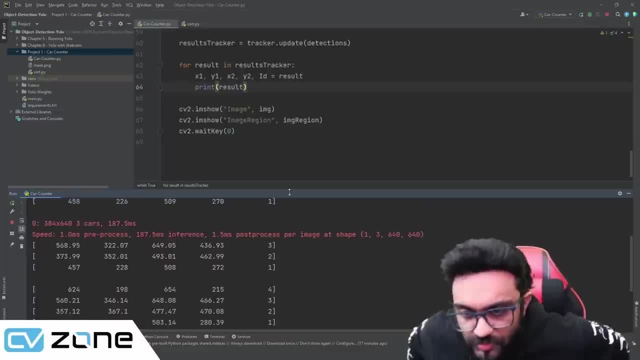 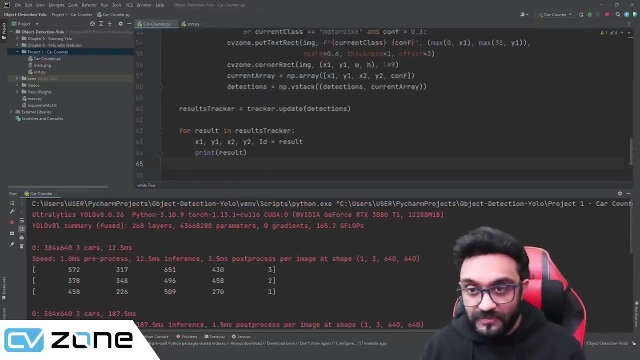 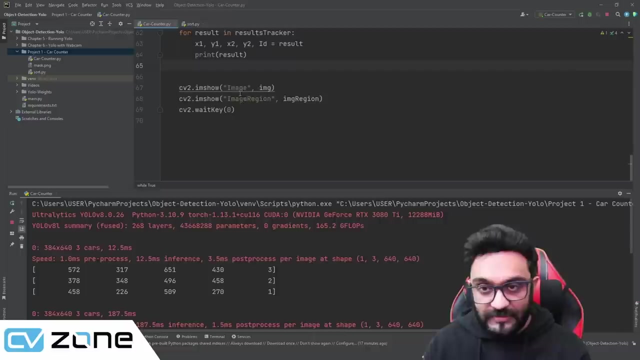 Okay. So in order to understand this better, what we are going to do, we are going to display these ID numbers, So it will become easier. So, instead of showing it here, or let's do both, We will show it here and we will show it here as well. 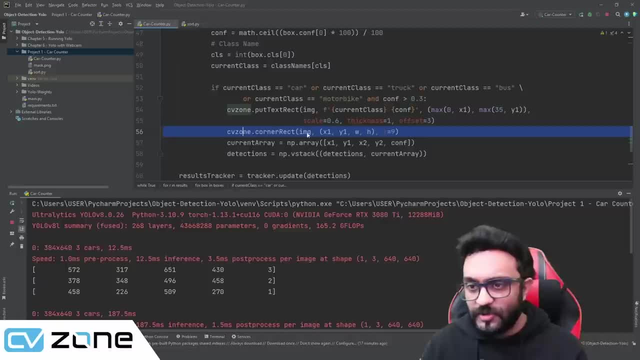 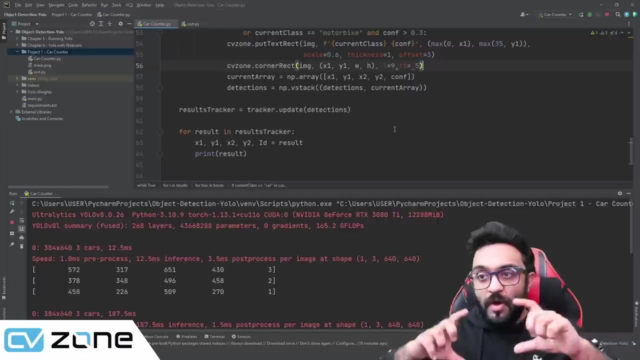 We will keep the thickness of this bigger. So we are talking about the rectangle, So the rectangle thickness here. So rectangle thickness equals, let's say, 5. And for the other one we will make it a little bit smaller So we can see what is the actual detection and what does it think? where is the tracking part? 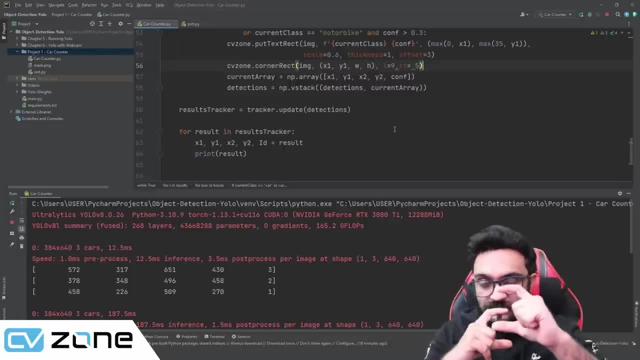 So how well, the tracker detects the bounding box. So let's try to find that. So what we will do is We will simply use these values. Are they integers? Yeah, they seem to be integers. So what we can do is we can simply create our corner rectangle. 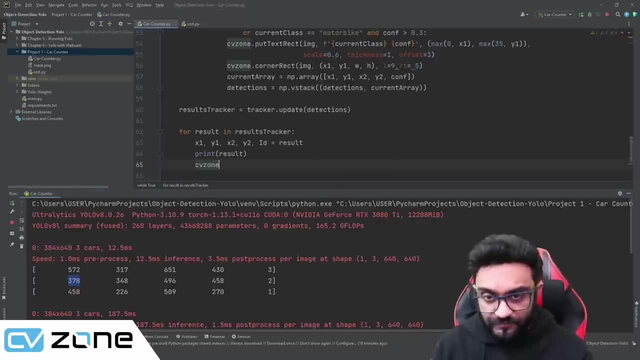 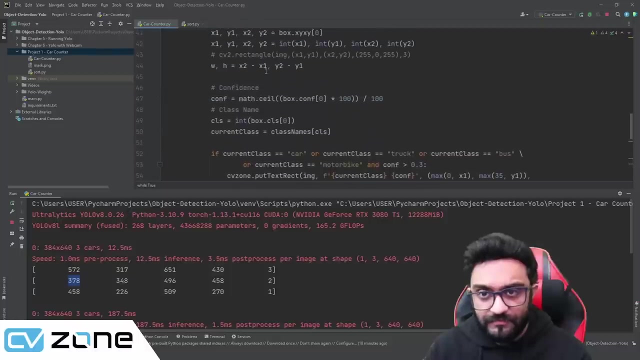 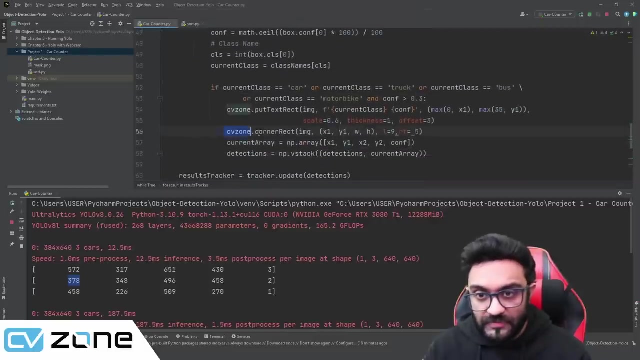 So we will write here CV zone dots- corner rectangle image And we have to give in the bounding box information. So the bounding box information will be like we did here. Let's copy that And actually let's copy this corner rectangle, because we're lazy. 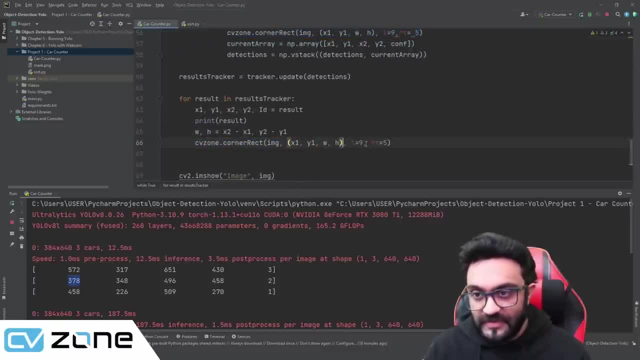 So there you go. So X1, Y1, width and height, And this time around, we'll put the rectangle as, let's say, 2.. And we will put it as blue, the color. So the color for the rectangle, Let's put it as 2550 and 0.. 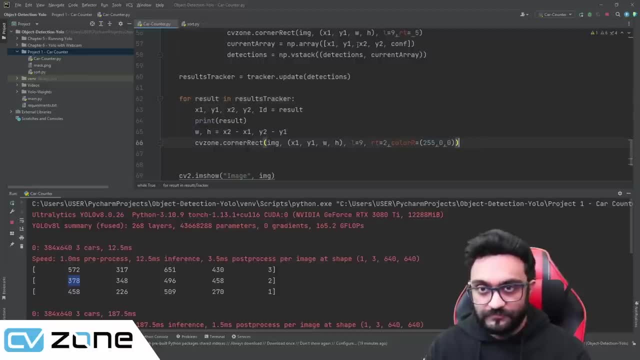 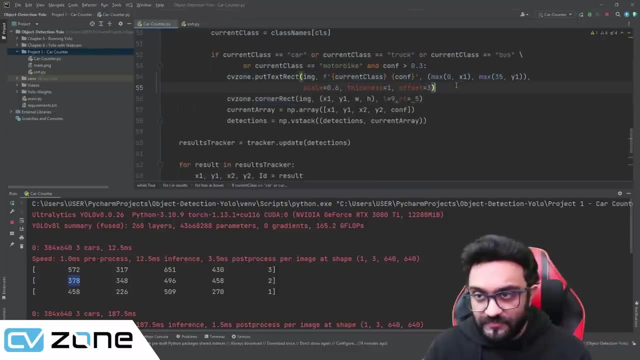 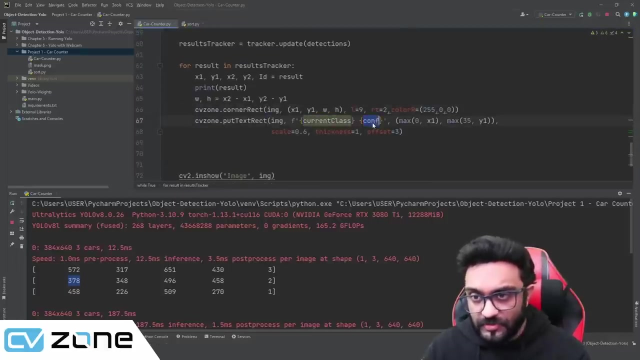 And let's show the ID as well. So Here we are showing using Put text right. So we will copy that And we will paste it here And instead of confidence and current class, we are going to display ID. It didn't show. 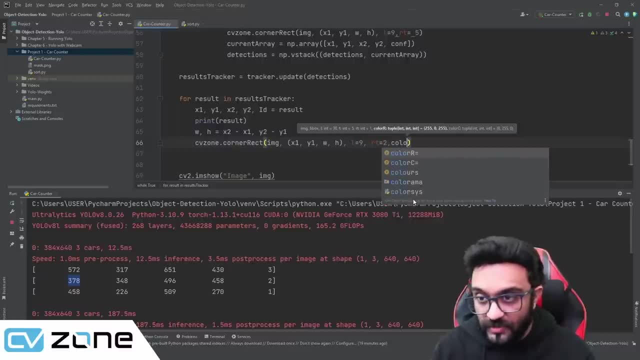 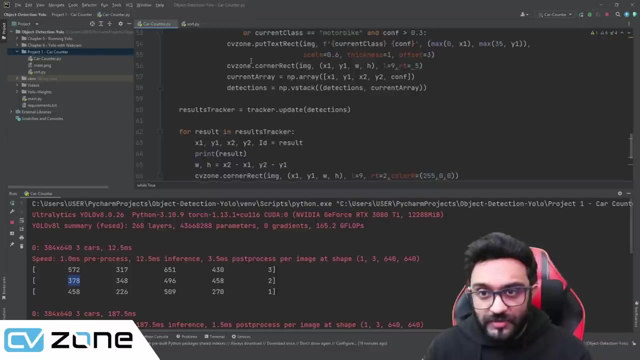 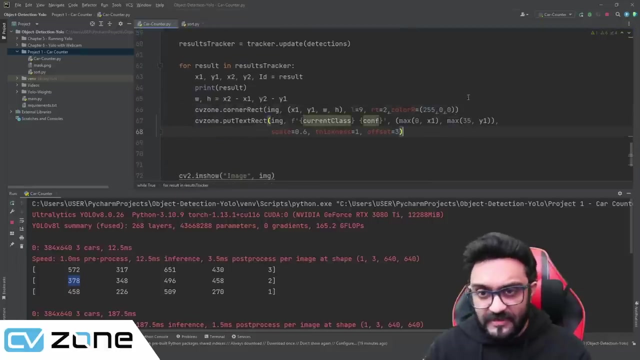 and we will put it as blue the color, so the color for the rectangle. let's put it as 255, 0 and 0.. and let's show the id as well. so here we are showing using uh, put text rect right, so we will copy that and we will paste it here. and instead of confidence and current class, we are going to 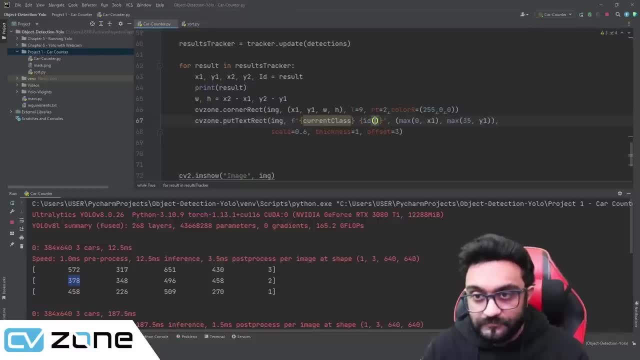 display id. so we will copy that and we will paste it here and instead of confidence and current class, we are going to display id. it didn't show. oh, the i is capital. my bad, so this here: why did i put i capital? let's put it small id. 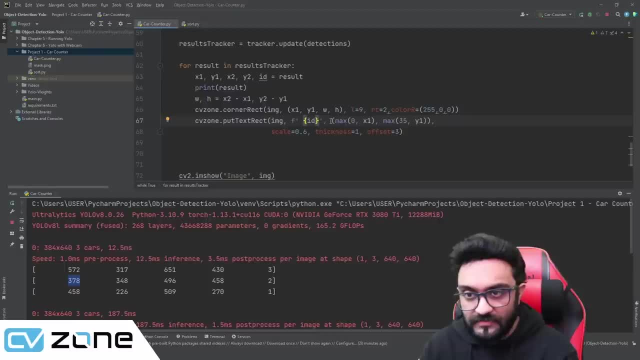 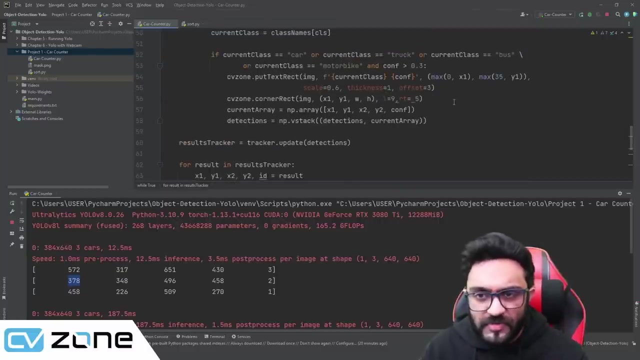 like that. okay, so id and yeah, that's fine. and the positioning is x1- y1, so x1- y1 is already bugged like it's. something is already there. we have the confidence and all the at. let's remove that, because we know already, we have the classes and all that. uh, it's car or. 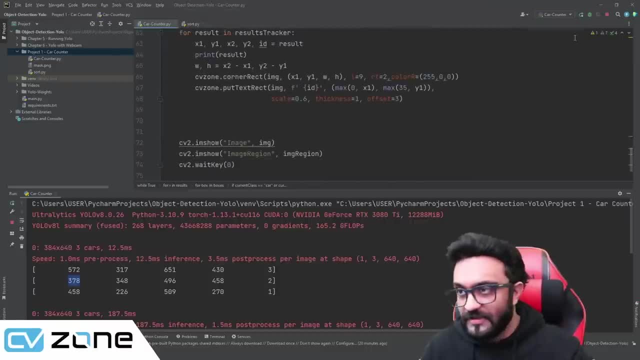 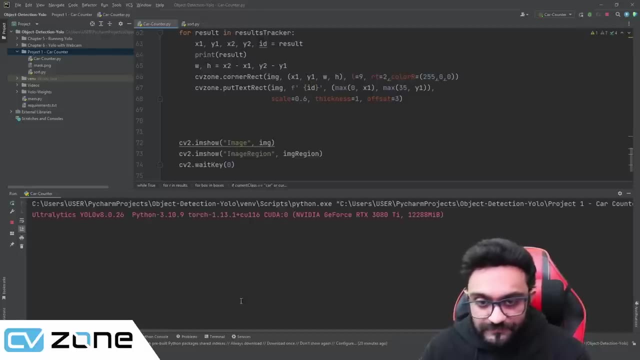 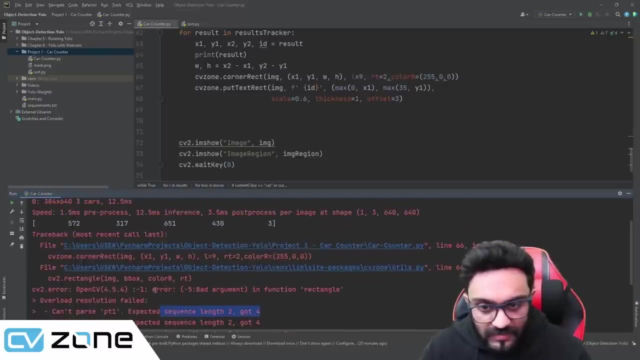 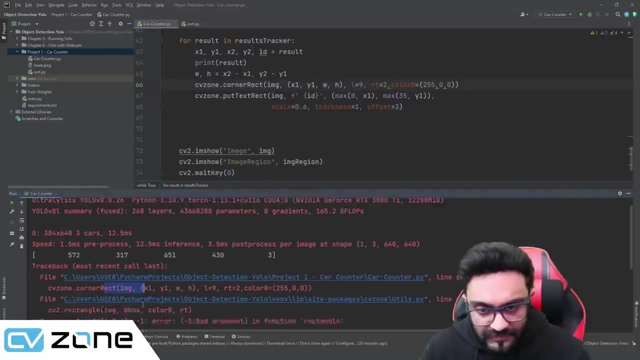 bus or whatever. so we can remove that and now we'll get the id instead of that. okay, so let's run that and hopefully we'll get some good results. so, expected sequence length 2 got 4.. uh, what is happening here? um, so it detected something. then it said corner rectangle. we have an issue. 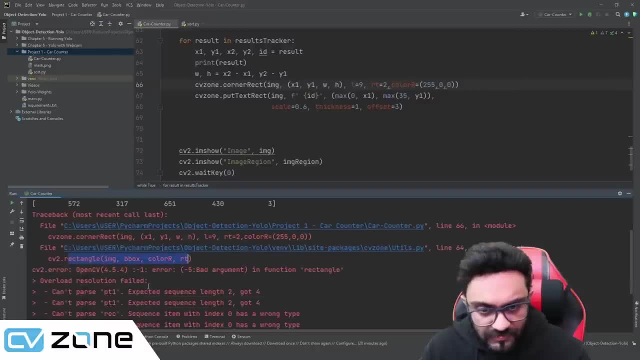 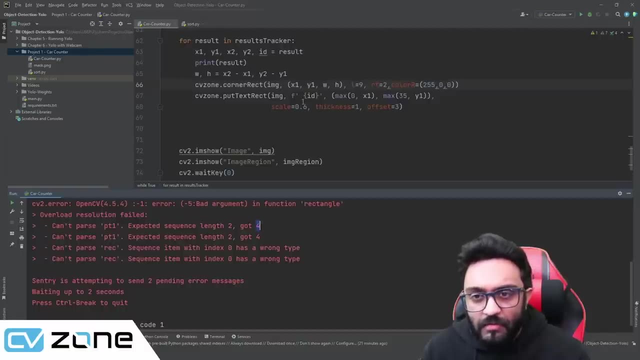 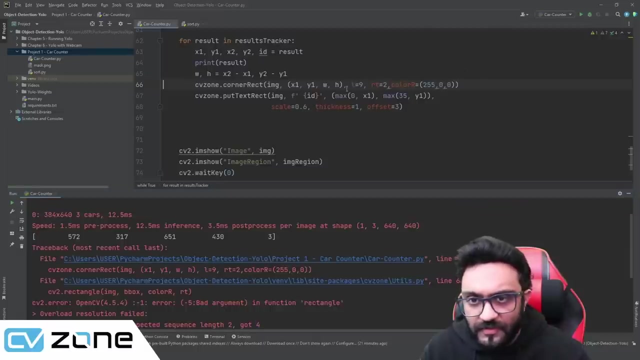 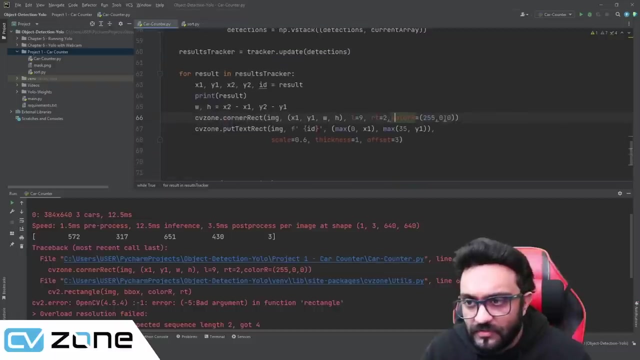 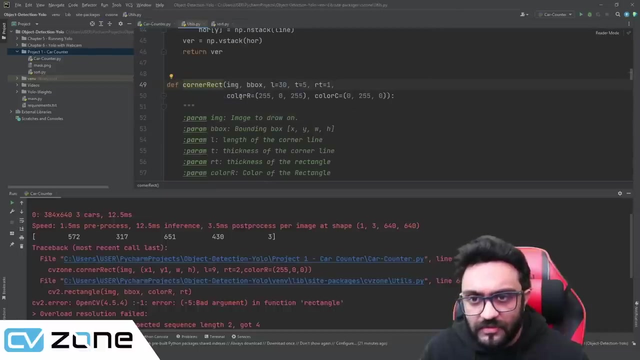 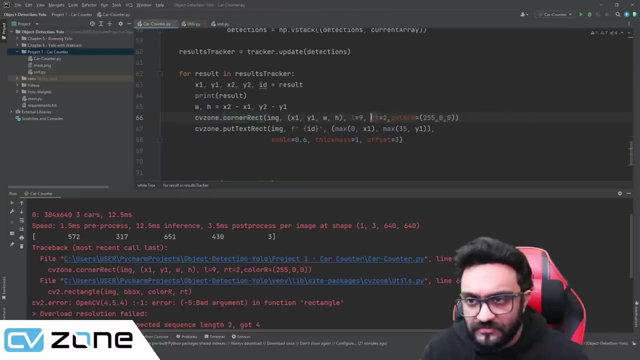 image: color rt. open cv by argument: rectangle expected length 2 got 4.. okay, um, so we are getting an error here, the corner rectangle. uh, why are we getting an error here? uh, let me check the corner rectangle. color r and color c: rt, or is it tr? it's rt, yeah, rt. and is this? uh, let's, let's print out. print out x1. 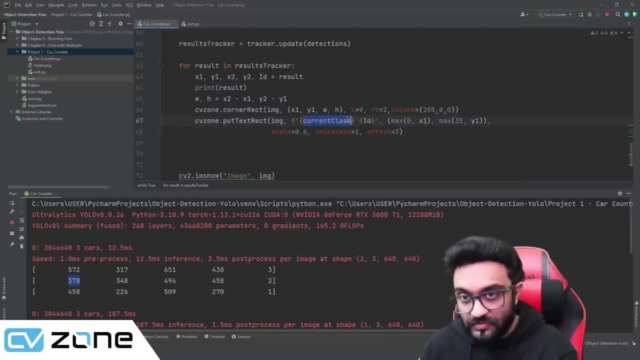 Oh, the I is capital, My bad. So this here: Why did I put I capital? Let's put it small ID. My God, Okay, So ID, And yeah, that's fine. And positioning is X1, Y1.. 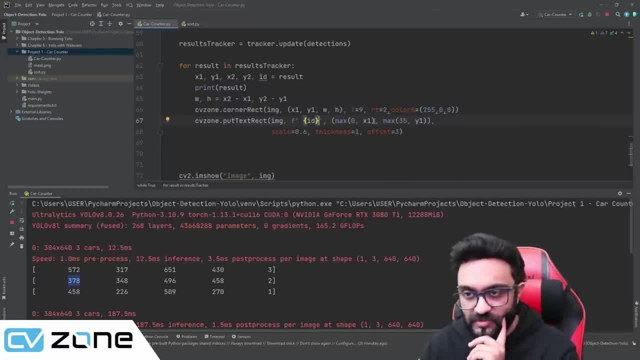 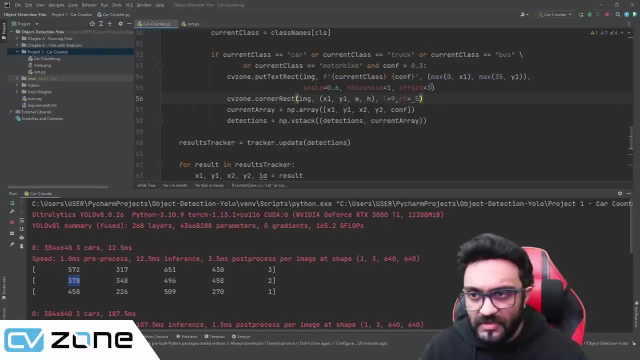 So X1, Y1 is already bugged, Like something is already there, We have the confidence and all that. Actually, let's remove that, because we know already we have the classes and all that. It's car or bus or whatever, So we can remove that. 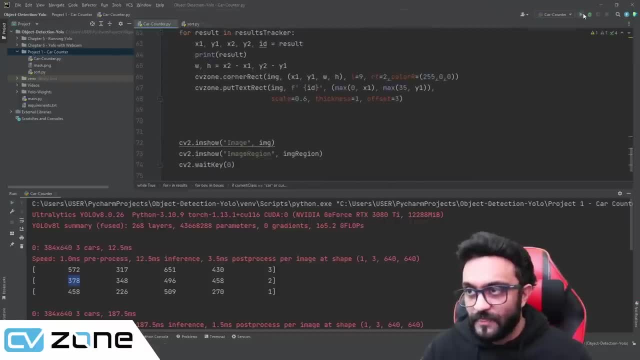 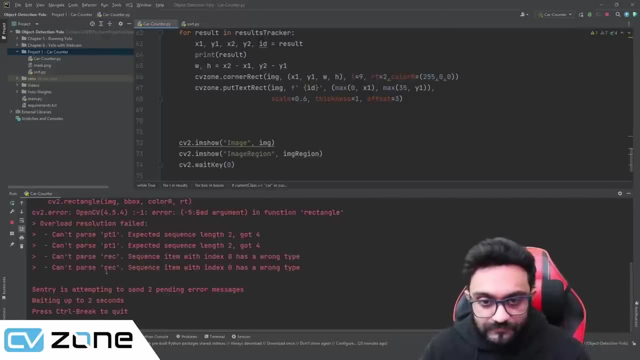 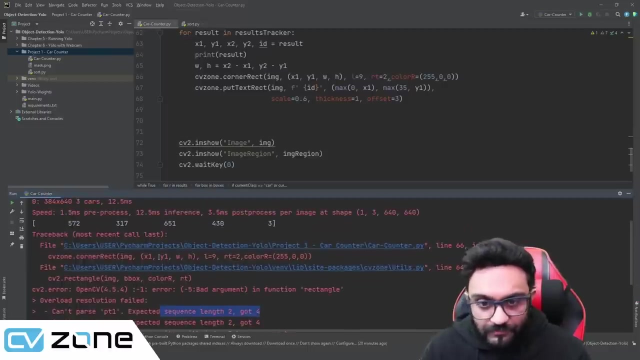 And now we'll get the ID instead, Instead of that. Okay, So let's run that And hopefully we'll get some good results. So expected sequence length two, got four. What is happening here? So it detected something. Then it said corner rectangle. 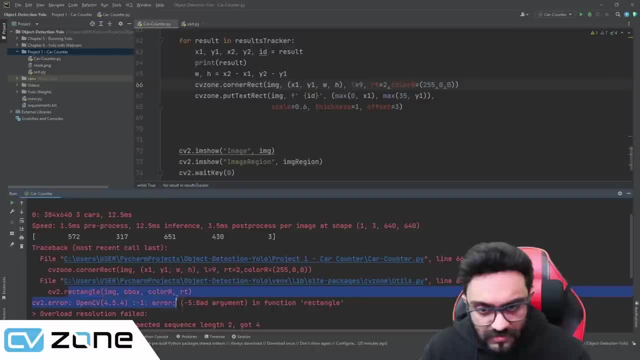 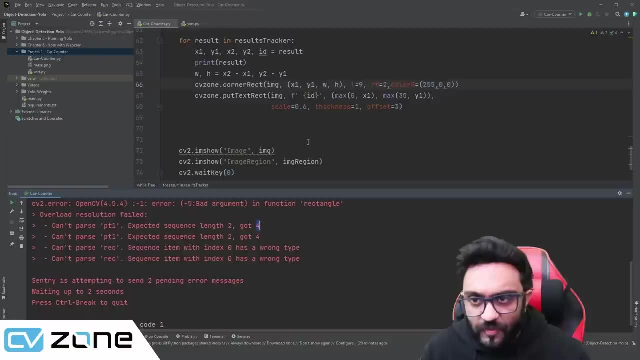 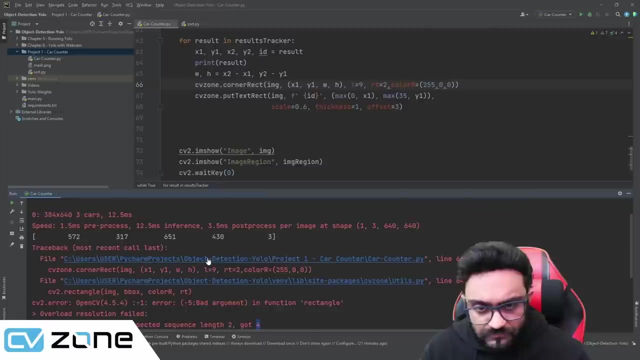 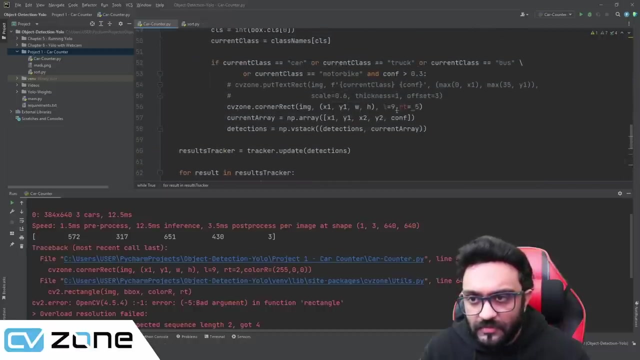 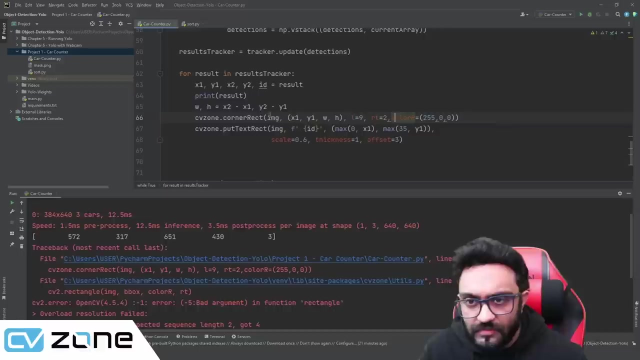 We have an issue. Image color RT Open CV by argument: rectangle: Expected length: two got four. Okay, So we are getting an error here. The corner rectangle. Why are we getting an error here? Let me check the corner rectangle. Color R. 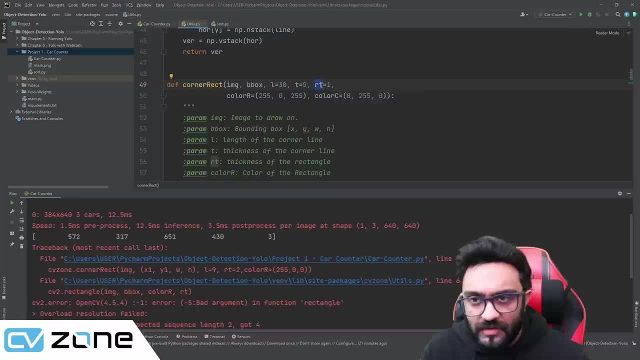 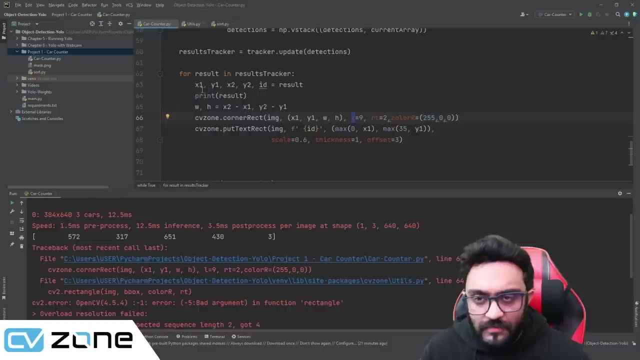 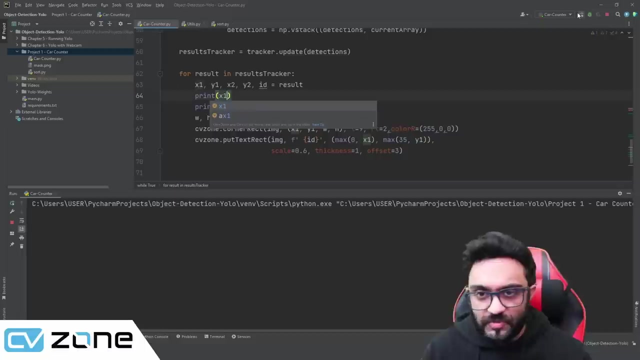 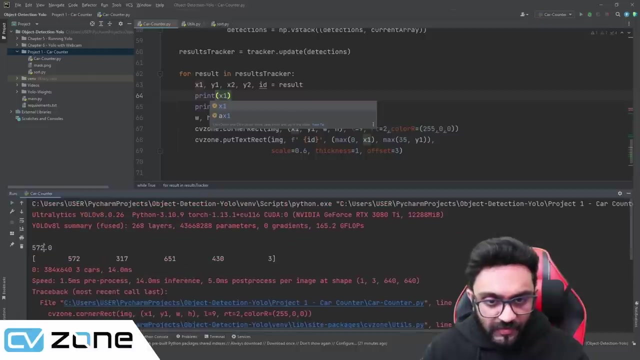 Color C, RT or is it TR? It's RT. Yeah, RT Length is this. Let's print out. Print out X1.. I just want to make sure that X1 is actually an integer and not a floating value, Because if it is, then we have a problem. 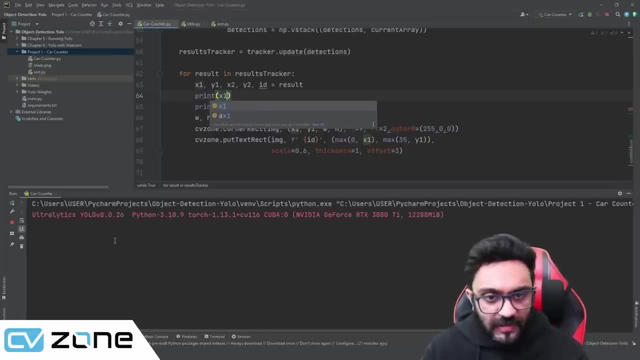 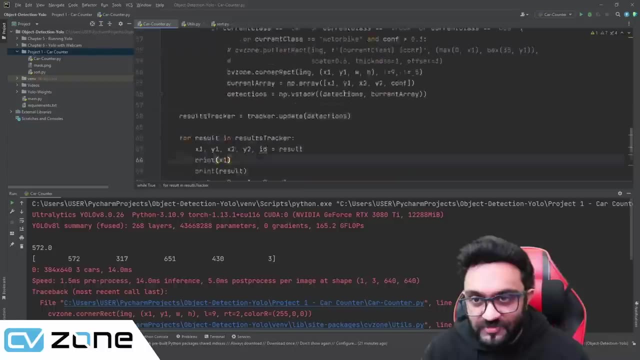 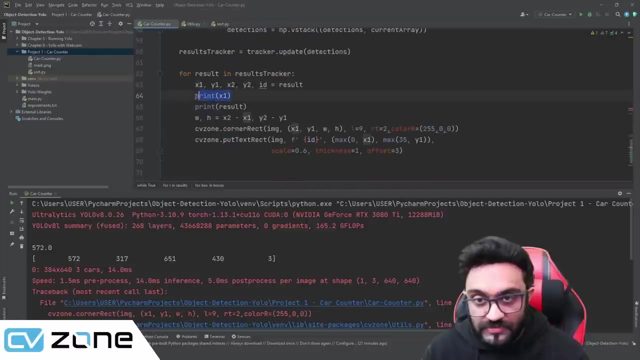 i just want to make sure that x1 is actually an integer and not a floating value, because if it is, then we have a problem. there you go, that's why. yeah, that's the issue. so we have to do the same thing we did earlier. uh, we have to do this. we have to convert them into integers. 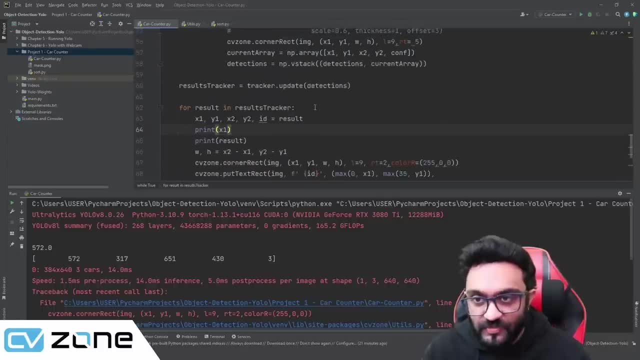 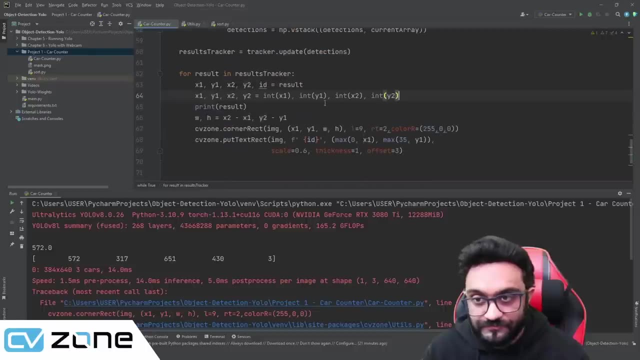 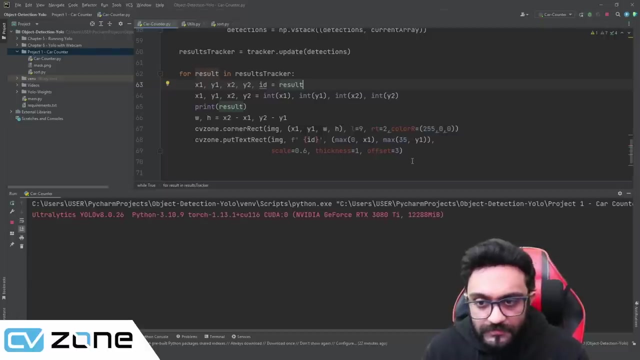 There you go. That's why. Yeah, that's the issue. So we have to do the same thing we did earlier. We have to do this. We have to convert them into integers. There you go. So let's run that and hopefully it will be fine now. 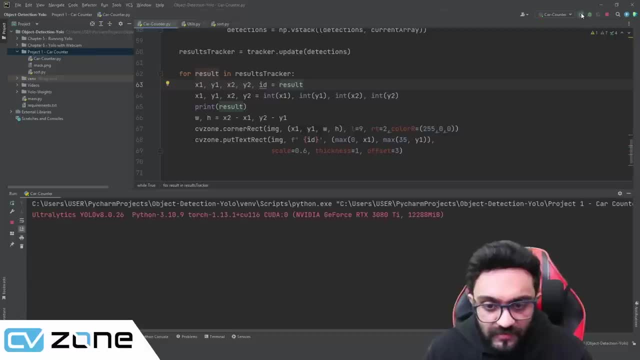 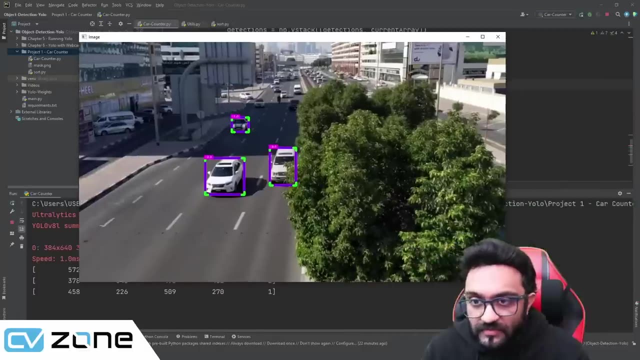 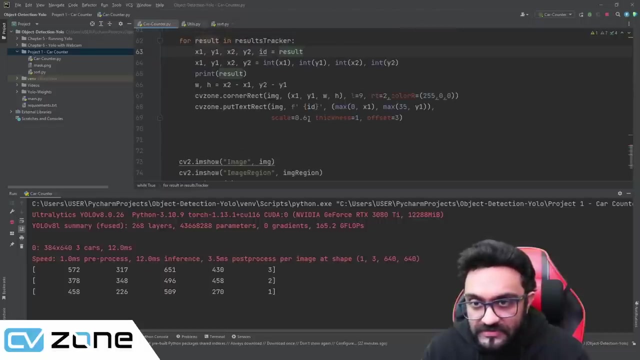 there you go. so let's run that and hopefully it will be fine now, there you go. so now it's showing us: okay, the ids are very small, let's make them bigger. so put x: rect. id max is this and that scale: let's put it as 2. 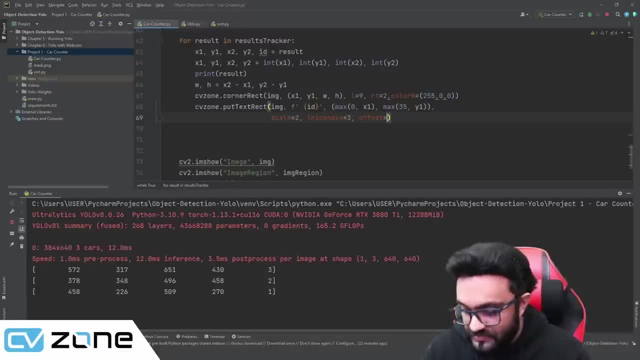 and thickness. let's put it as 3, offset, let's put it as 10.. so it will be big values. we can clearly see what's going on. there you go: uh point, ah, hit the point. so id: we need to convert the id into integer as well, so let's. 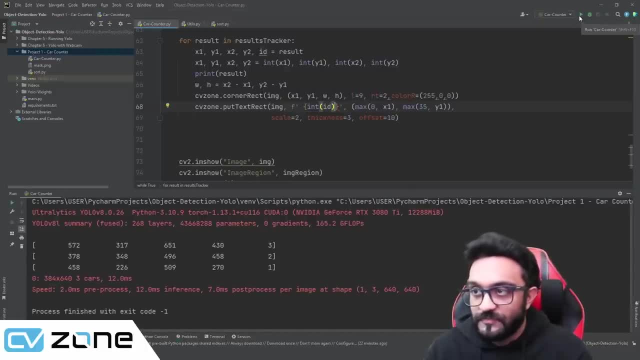 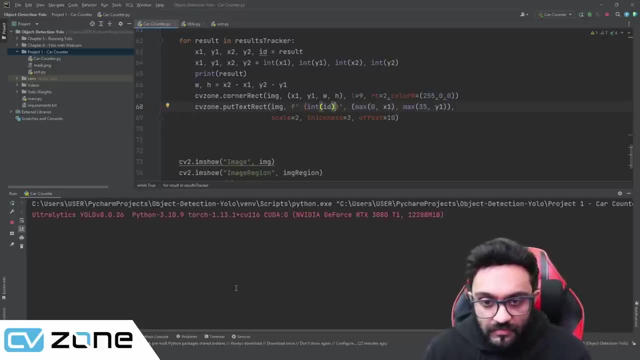 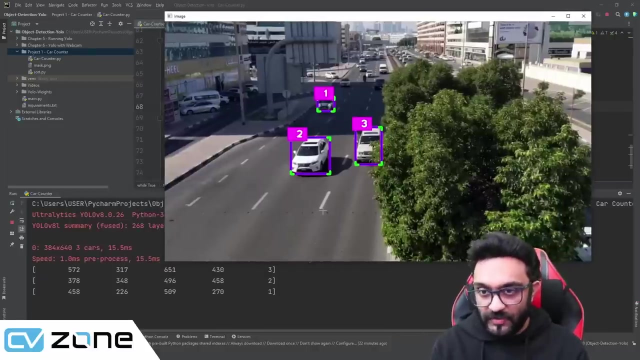 just do it here: integer id. okay, so there you go. so this is id 1, id 2, id 3.. now is the moment of truth. so if we go to the next one, these ids should remain same. if they flip around, it means it's not tracking. 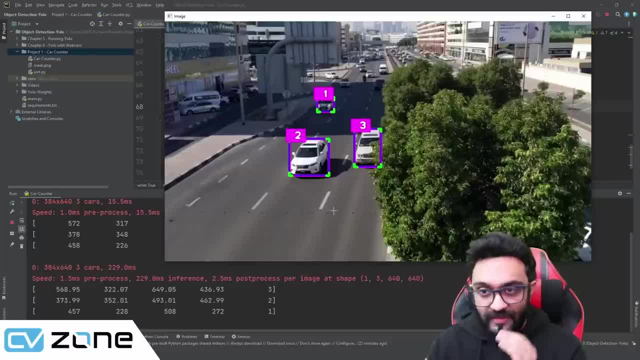 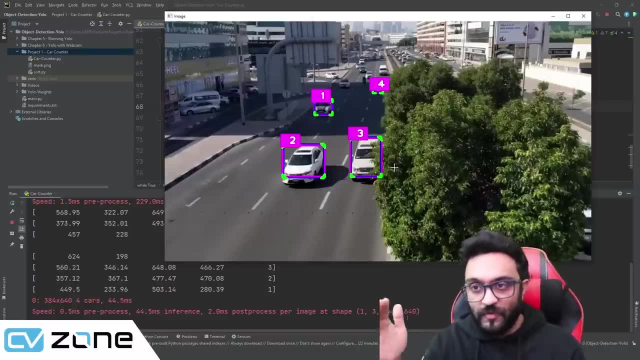 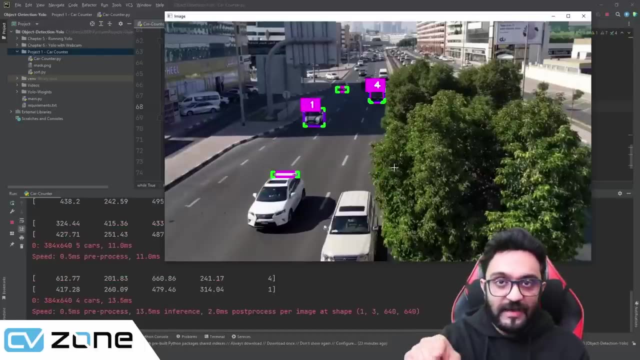 it's only detecting. so if i press spacebar, and there you go, it's the same. so if i press spacebar again, again it's the same. so one, two, three, four, if i keep pressing, there you go. so the four was lost, but it kept it. uh, it brought back the four from where it left off and you can. 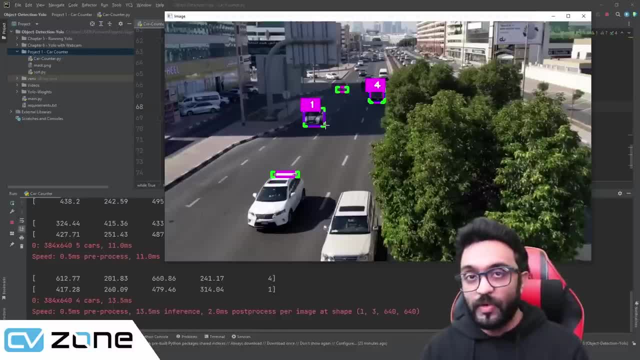 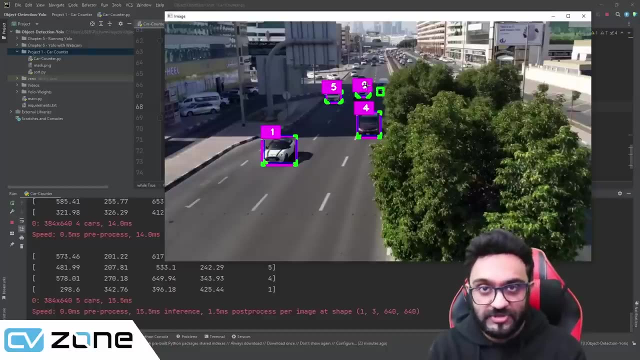 also see the blue line. the blue line is basically what the tracker is detecting and the purple one is what the detector or the yolo is detecting. so if we keep going forward, you can see this is now five and this one is nine. now this is not an issue, because if it doesn't go to five it might. 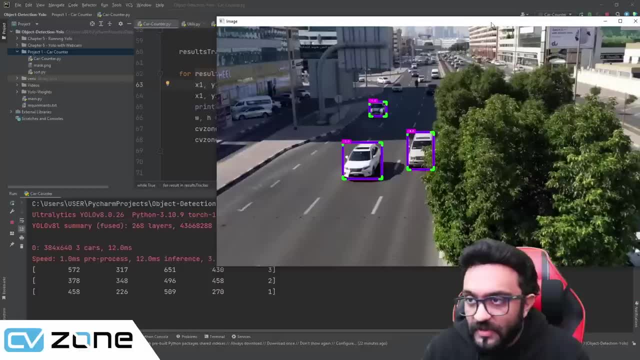 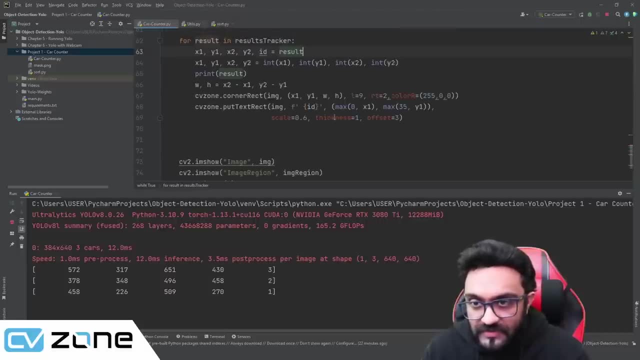 There you go. So now it's showing us: okay, the IDs are very small, Let's make them bigger. So put text rect: ID max is this and that. Scale, let's put it as two, And thickness, let's put it as three. 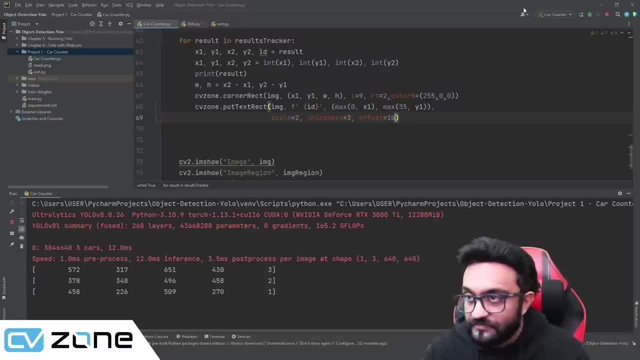 Offset. let's put it as 10.. So it will be big values. We can clearly see what's going on. There you go Point, Hit the point. So ID: we need to convert the ID into integer as well, So let's just do it here. 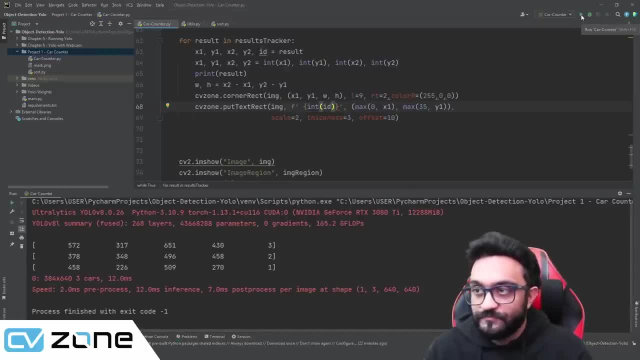 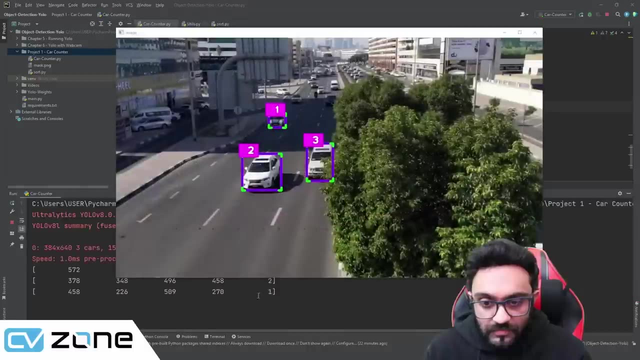 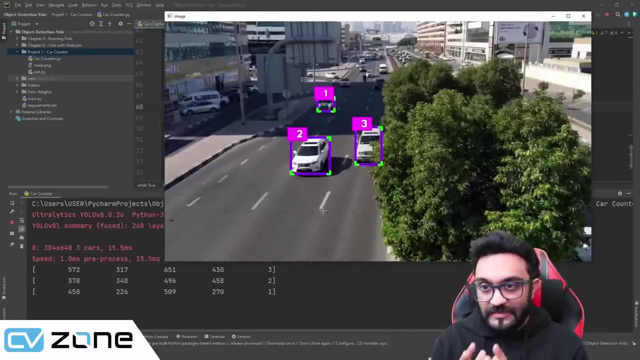 Integer ID. Okay, So There you go. So this is ID 1, ID 2, ID 3.. Now is the moment of truth. So if we go to the next one, these IDs should remain same. If they flip around, it means it's not tracking. 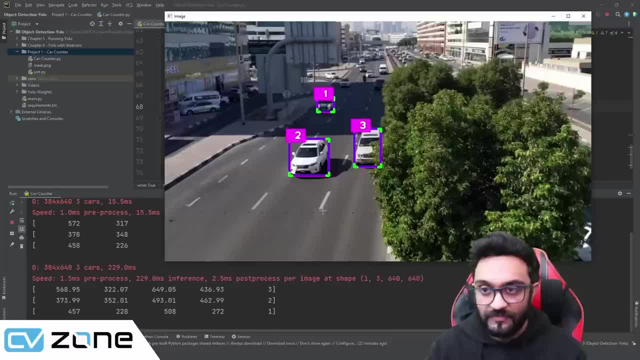 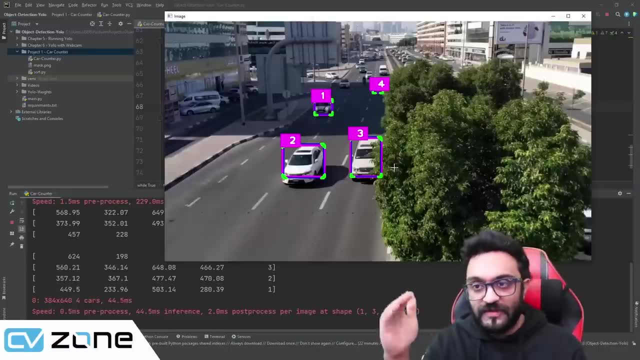 It's only detecting. So if I press spacebar, and there you go, It's the same. So if I press spacebar again, again it's the same. So 1,, 2,, 3,, 4.. If I keep pressing, there you go. 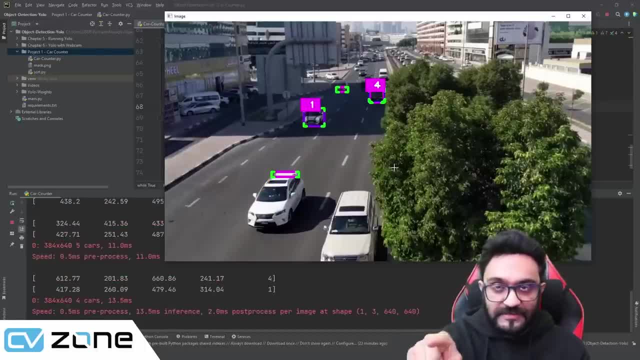 So the 4 was lost, But it brought back the 4 from where it left off. And you can also see the blue line. The blue line is basically what the tracker is detecting And the purple one is what the detector, or the YOLO, is detecting. 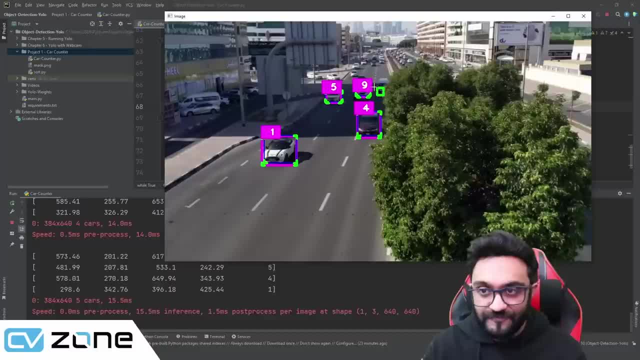 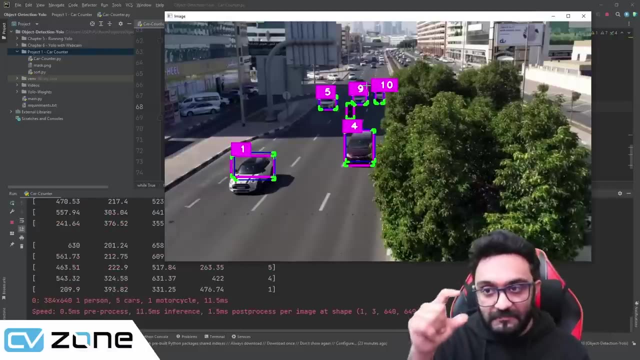 So if we keep going forward, you can see this is now 5. And this one is 9.. Now this is not an issue, Because if it doesn't go to 5, it might have detected some wrong IDs, But as long as the ID remains the same, if 9 remains 9, then it's fine. 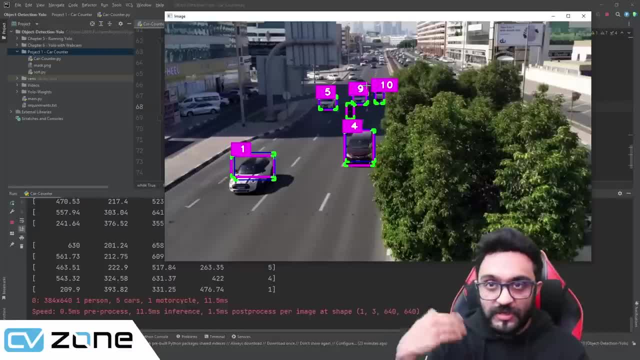 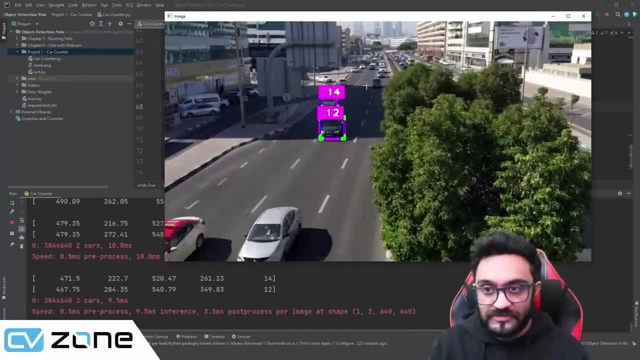 Because we will have a line after which we cross, we will detect it or we will count it, So that's fine. So there you go, It's 14 is 14.. 12 is 12.. 18 is 18.. 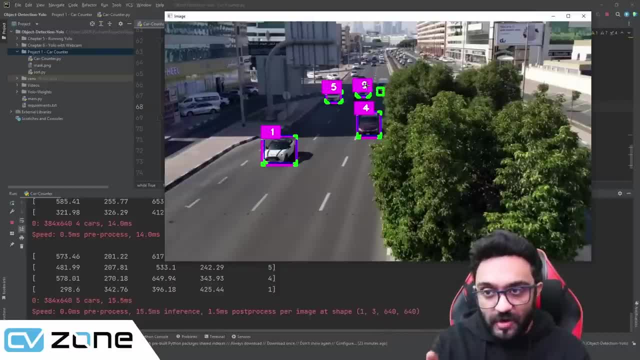 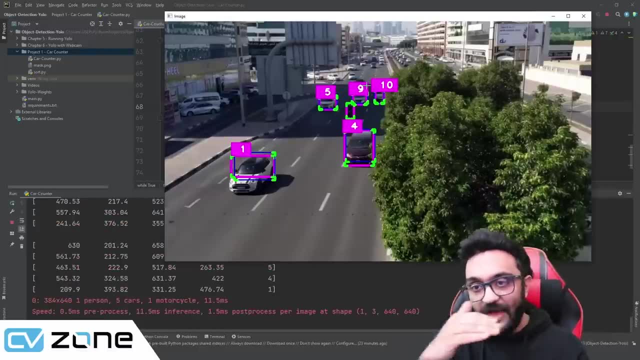 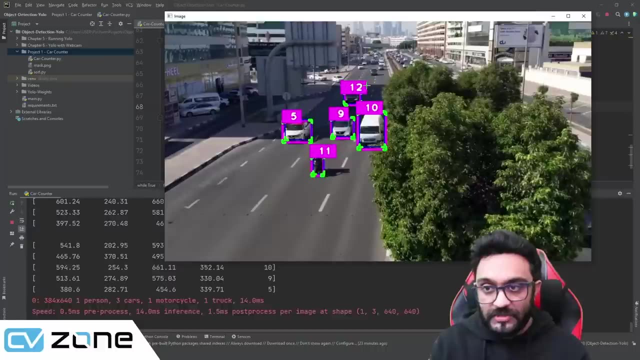 have detected some wrong ids, but as long as the id remains the same, if nine remains nine, then it's fine, because we will have a line after which we cross, we will detect it or we will count it. so that's fine. so there you go. it's. 14 is 14, 12 is 12, 18 is 18. 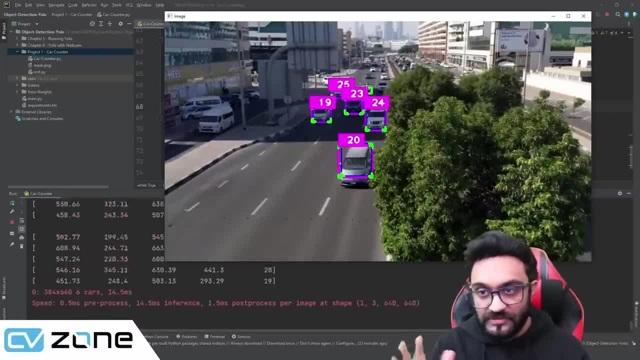 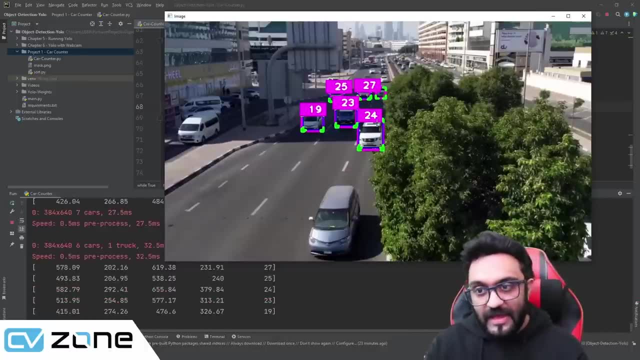 19 is 19, 20 is 20, 23 is 23, 24 is 24 and that's all good. so we can make a line here. we can make a line here and whenever that line crosses, whenever that id crosses that line, we are. 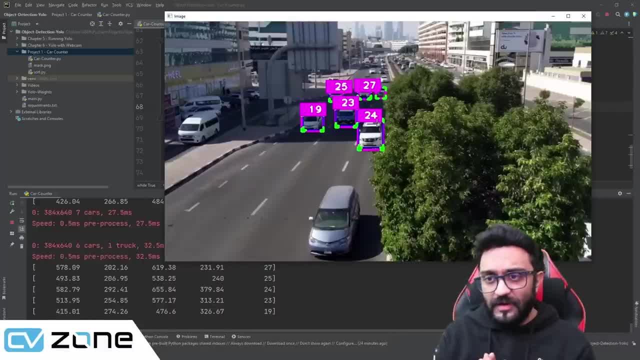 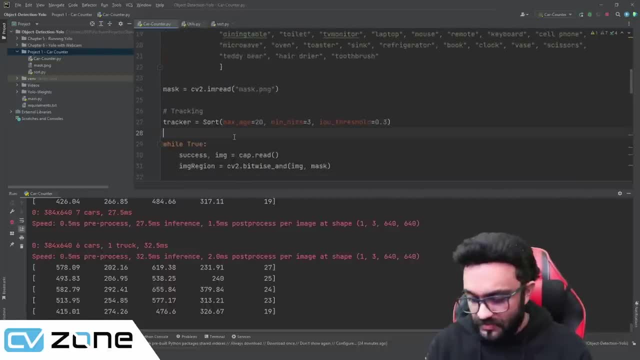 going to detect it as a count. now, how can we do that? it's very simple. all we have to do is we have to first of all create the line, so we are going to write here that our line equals. so this value should be actually. there's image region coming here. let's remove that, because we 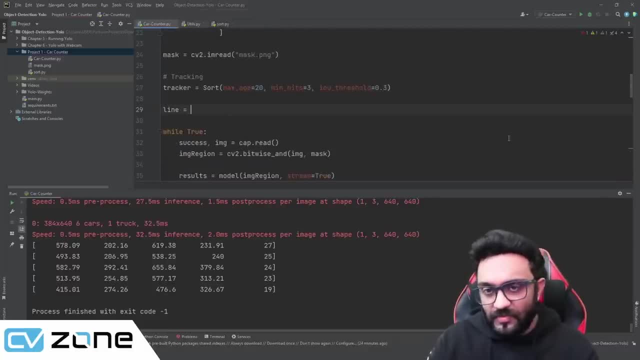 don't need that anymore. now this line: uh, i have checked the values already, so we are going to put that: uh, let's call it limits, let's call it limits instead. and then we are going to write here: 423, 297, 673 and 297. 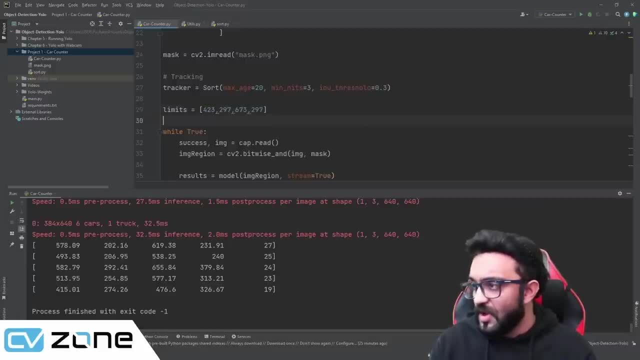 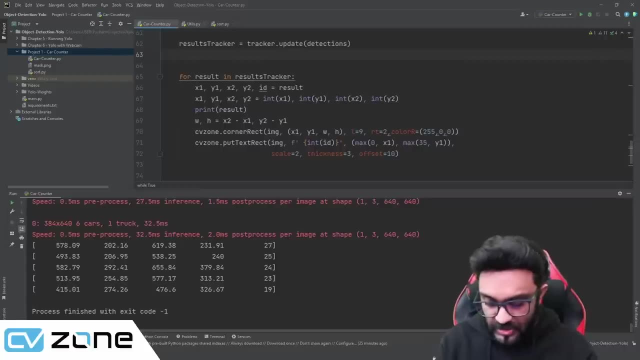 so these are the limits, and using these limits, uh, we are going to create a line. so this line, let's draw it after the tracker. so here we'll write cv2 dot line and we'll give in the image, and then we have to give in the points. so the points are basically limits at zero and limits at one. 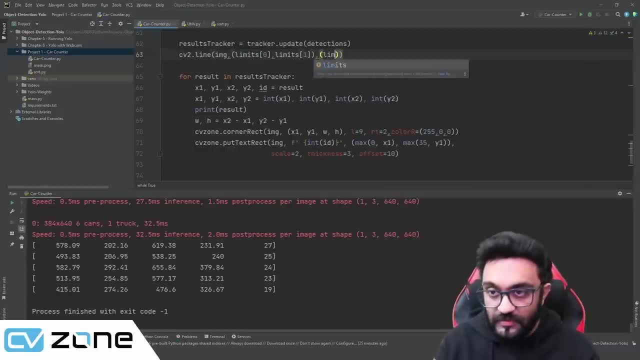 then the second point will be limits at zero, uh sorry, limits at two and uh, limits at three. and then what do we need? then we need the color. so the color: let's put it as red. so it will be uh, zero, zero, bgr, so 255. and then we have the thickness: let's put it as five, and that should. 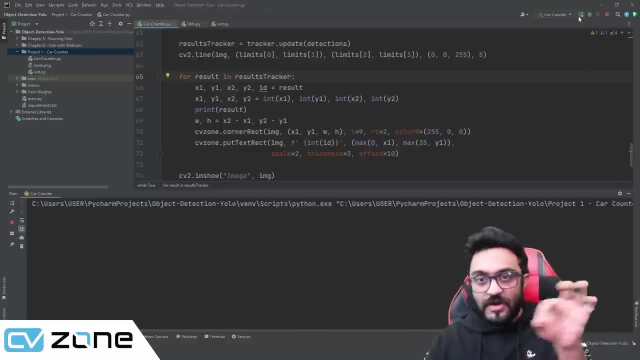 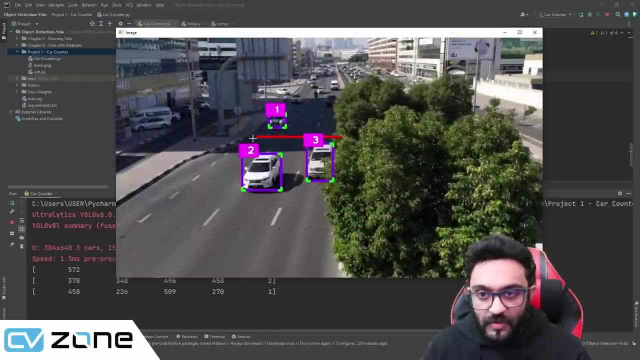 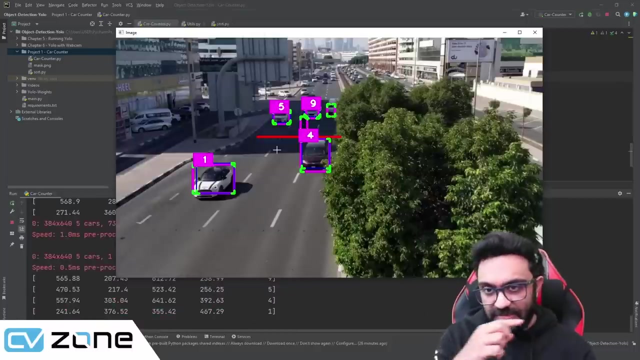 be good. so if we run this now, we should have a line right in the middle of our road. so there you go. so this is our line. if these IDs, if any of these cars, they cross this line, then it will be detected as- um, what do you call detection? actually, what we can do is we can extend it to the left a little. 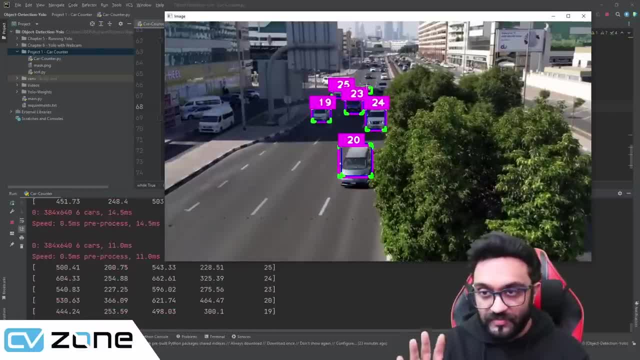 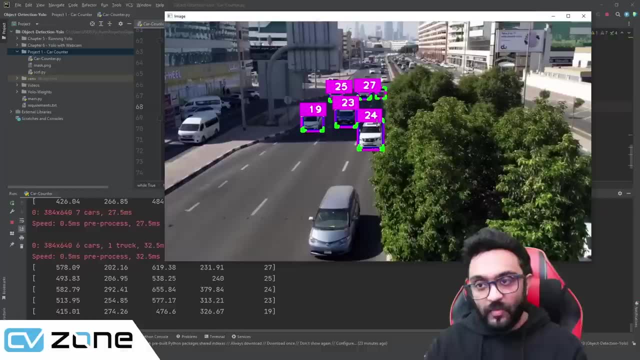 19 is 19.. 20 is 20.. 23 is 23.. 24 is 24.. And that's all good. So we can make a line here. We can make a line here And whenever that line crosses, whenever that ID crosses that line, we are going to detect it as a count. 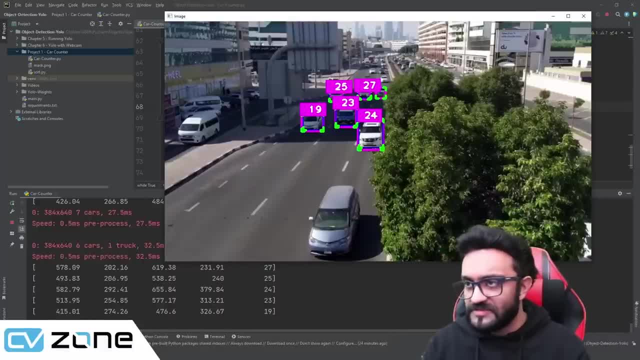 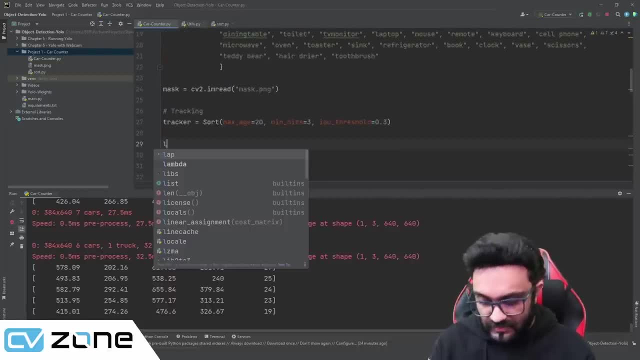 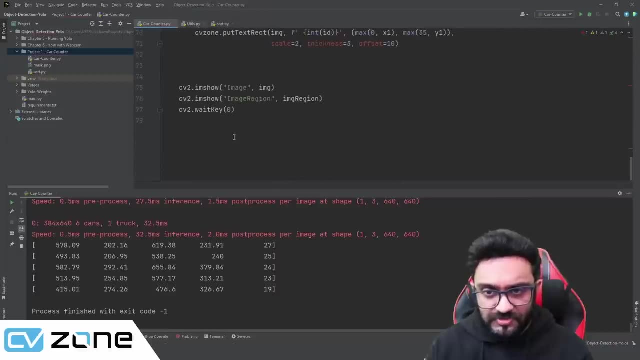 Now, how can we do that? It's very simple. All we have to do is we have to first of all create the line. So we are going to write here that our line equals. So this value should be actually. there's image region coming here. 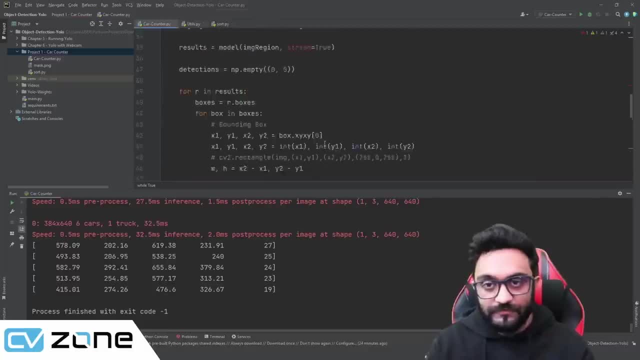 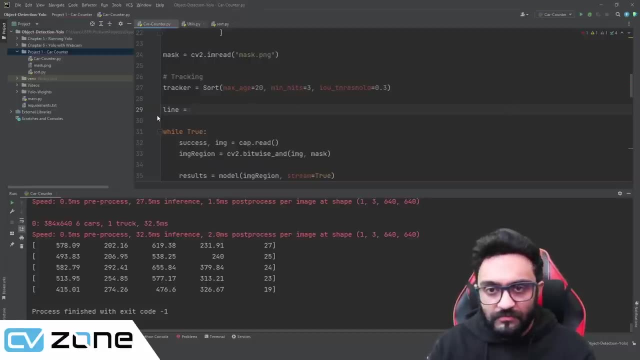 Let's remove that, Because we don't need that. We don't need that anymore. Now this line: I have checked the values already, So we are going to put that. Let's call it limits. Let's call it limits instead. 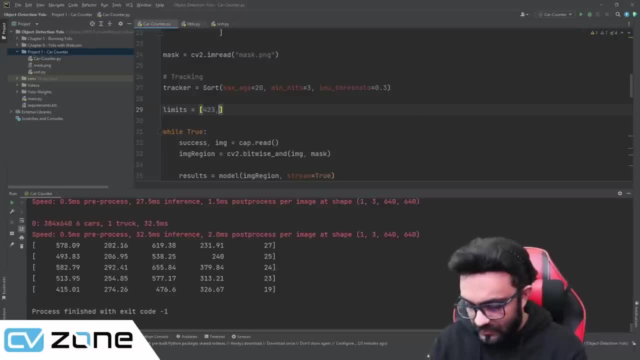 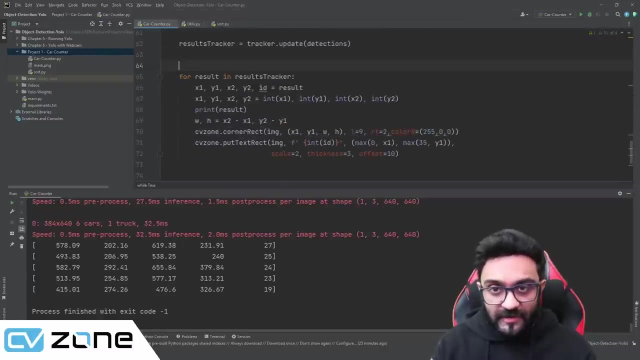 And then we are going to write here: 423, 297,, 673, and 297.. So these are the limits And using these limits, we are going to create a line. So this line, Let's draw it after the tracker. 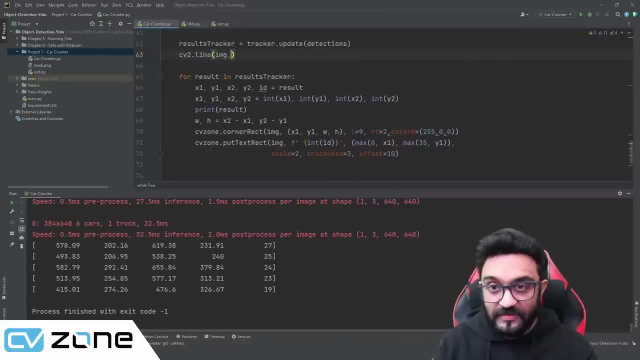 So here we will write cv2.line And we will give in the image, And then we have to give in the points. So the points are basically limits at 0 and limits at 1.. Then the second point will be limits at 0.. 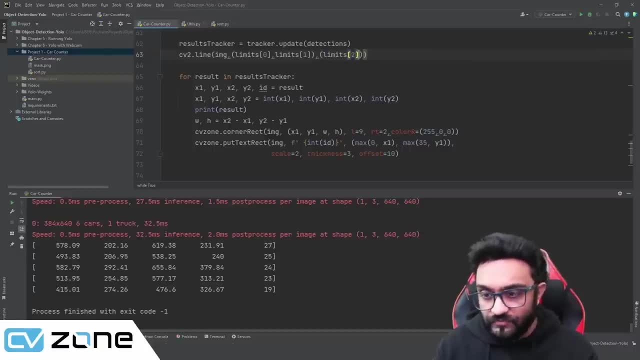 Sorry, limits at 2.. Limits at 3.. And then what do we need? Then we need the color. So the color, let's put it as red, So it will be 00BGR, So 255.. And then we have the thickness. 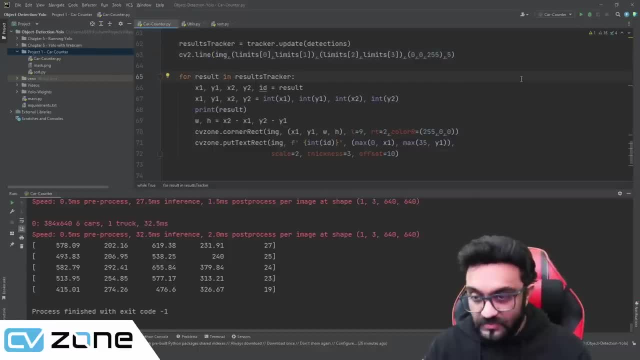 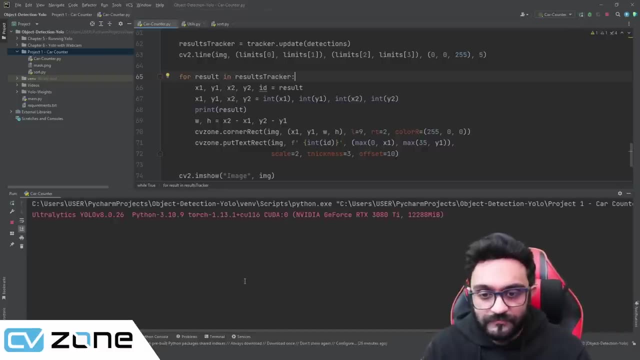 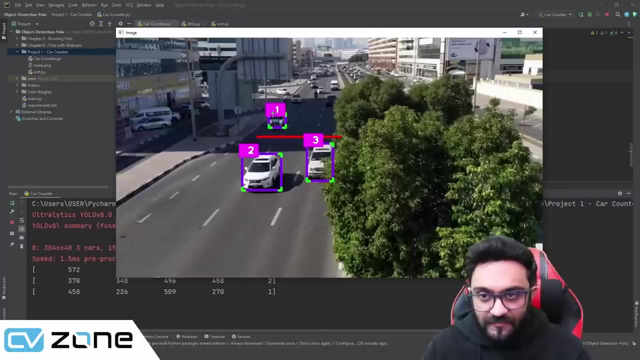 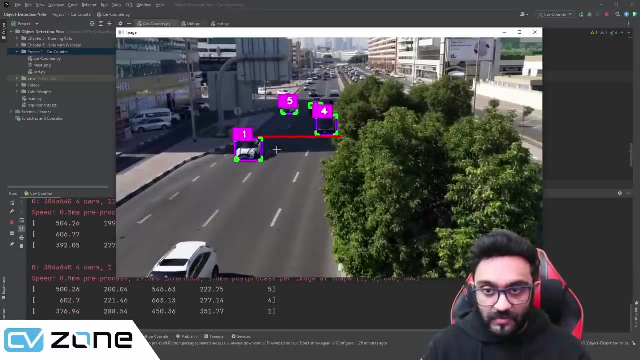 Let's put it as 5. And that should be good. So if we run this now, we should have a line right in the middle of our road. So there you go, So this is our line. If these IDs, if any of these cars, they cross this line, then it will be detected. as what do you call detection? 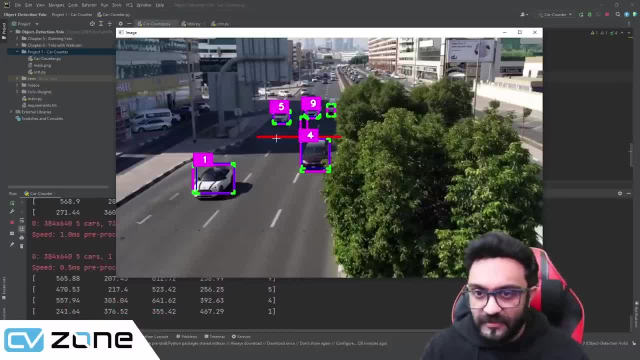 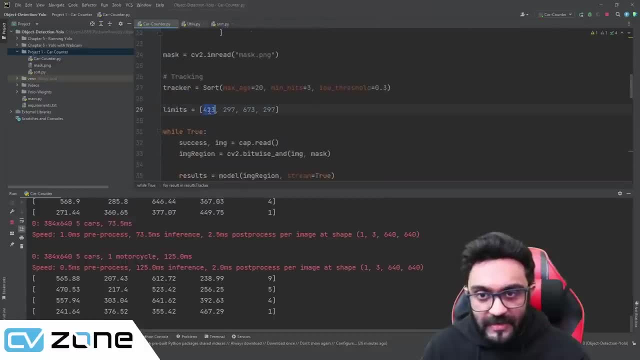 Actually what we can do is we can extend it to the left a little bit, because there's a gap here. So let's go over here to the limits And in the X we can make a line. In the X we can make it, let's say 400.. 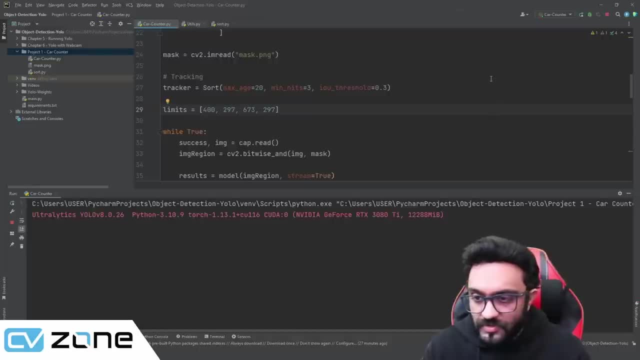 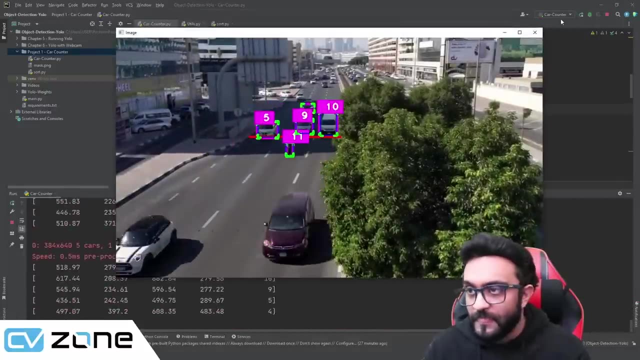 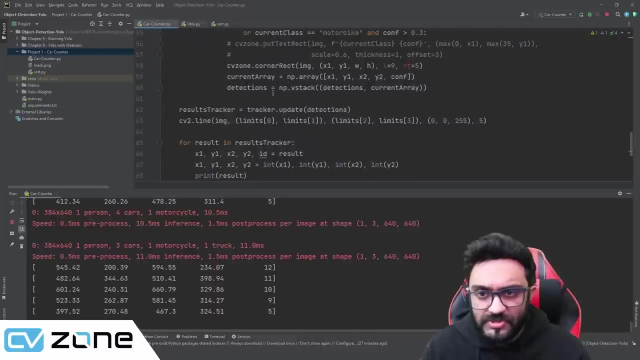 We'll move back 20 pixels, 23 to be exact. Yeah, now it's perfect, So now it should be fine. Now what we need to do next is: let's remove the detection part, So we don't need to draw the rectangles when we are detecting, only for the tracker. 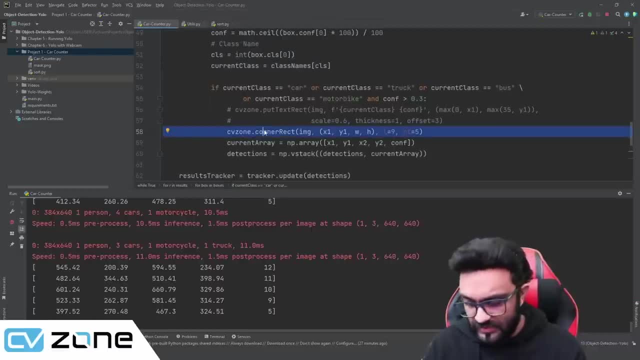 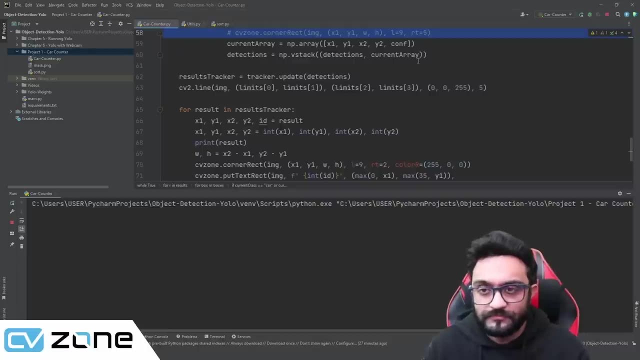 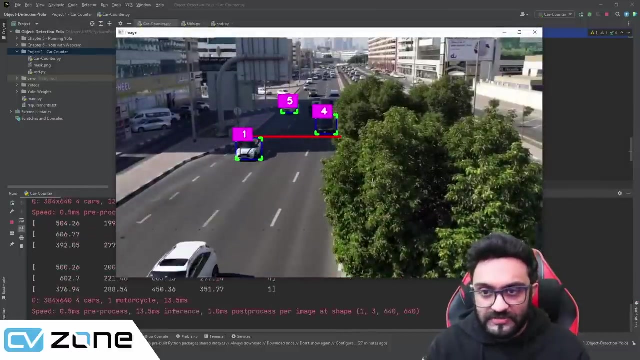 So here the corner rectangle. we can remove that. So now it will only show us the blue ones. There you go. Now it's only showing us the blue ones. Actually, I like the purple color better. Let's make it purple. 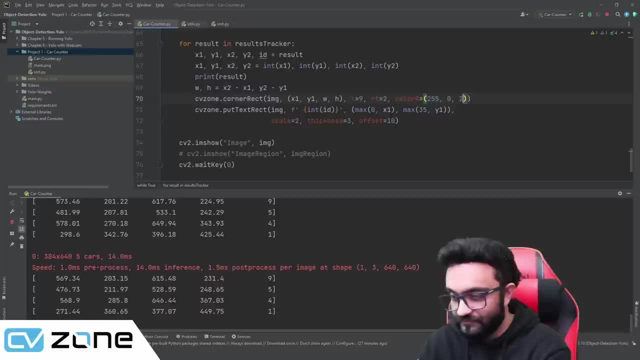 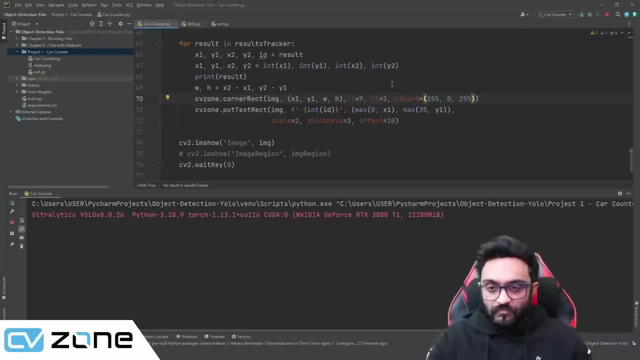 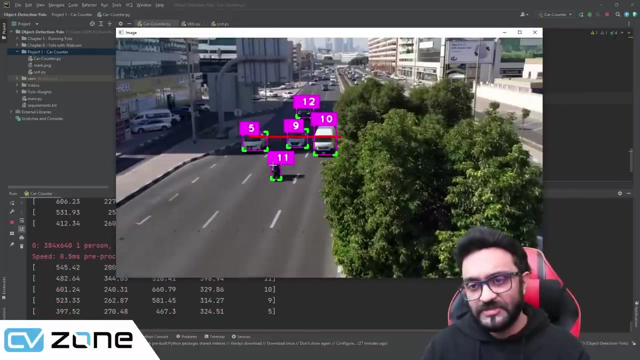 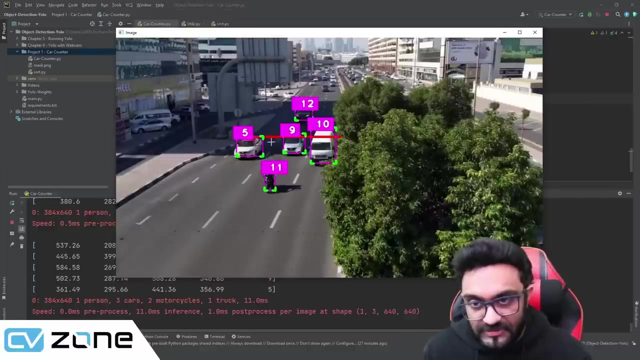 255 and make this 255 as well. So now the rectangles will be purple. There you go. So yeah, I like that better. So the next step is to find the center point. So once we have those center points, we need to check if that center point actually touched this line. 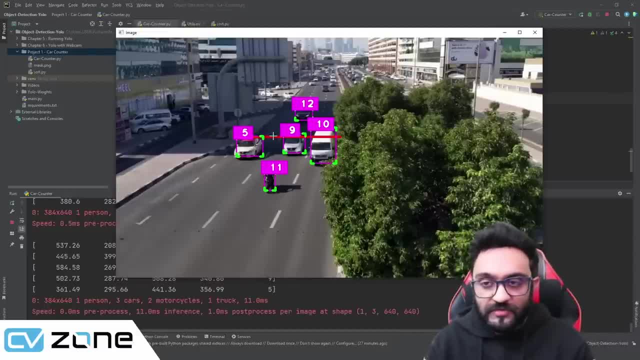 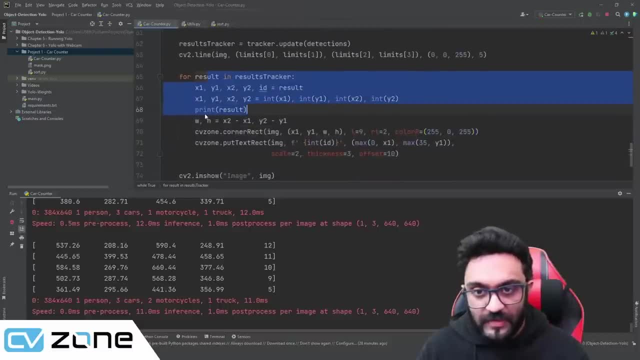 If it touched the line, then we are going to say it was a count, So that's the idea. So how can we find this? This is our results. We have the X, we have the Y, we have the width, we have the height, we have everything. 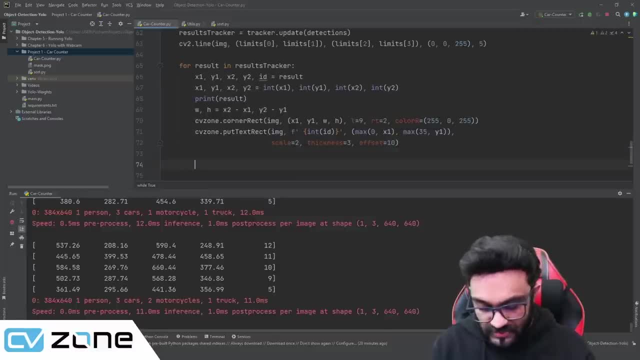 All we need to do is we need to find the center, So we will call it CX and CY. This is the center X and the center Y. And how can we find it? It will be X1 plus the width divided by 2.. 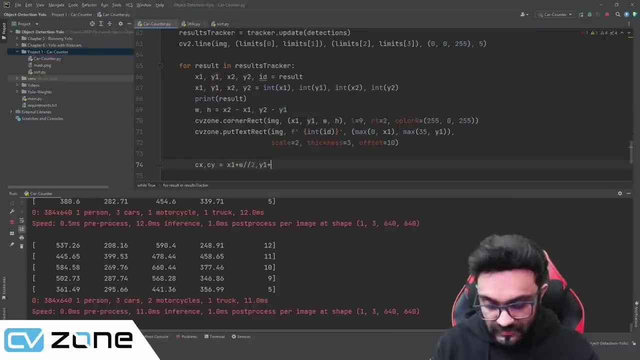 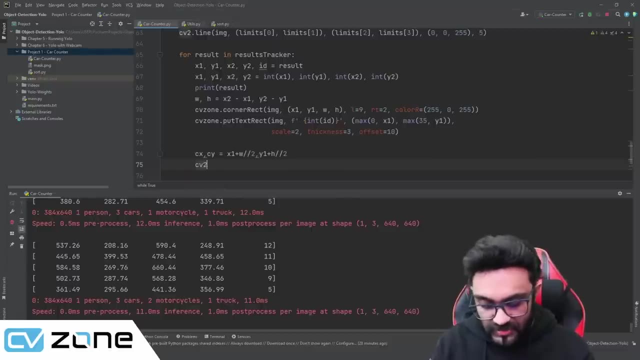 And it will be Y1 plus the height divided by 2.. So just to make sure that we are headed in the right direction, we can draw it CV2 dot circle And we will give in the image, We will give in the CX and the CY. 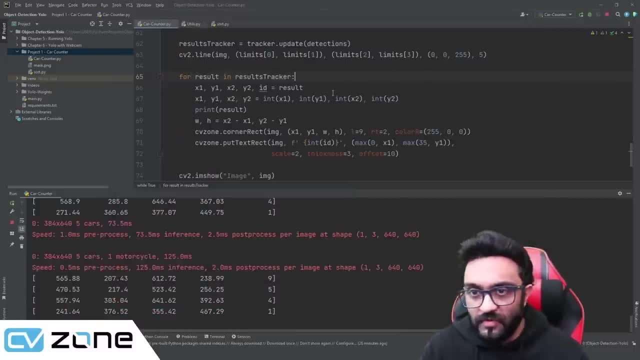 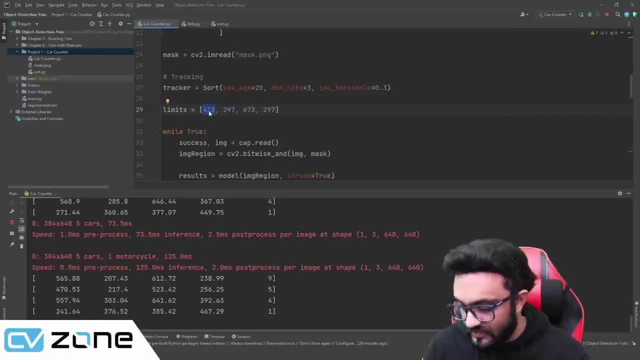 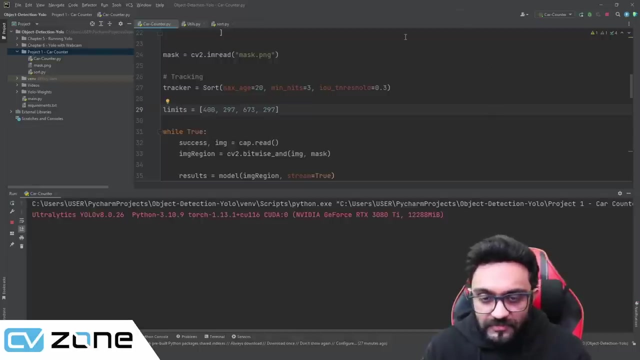 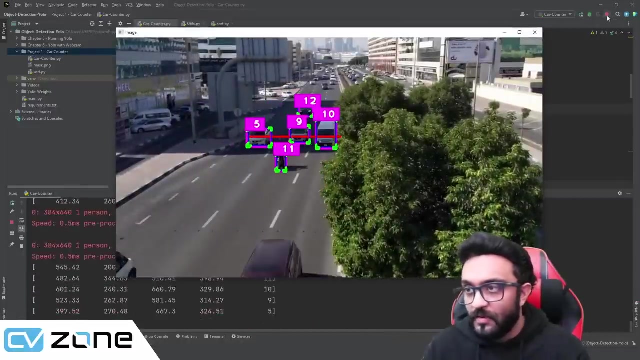 bit, because, uh, there's a gap here, so let's go over here to the limits and in the uh X we can make it. let's say 400, we'll move back 20 pixels, 23 to be exact. yeah, now it's perfect, so now it should be fine. uh, now, what we need to do next is, uh, let's remove the. 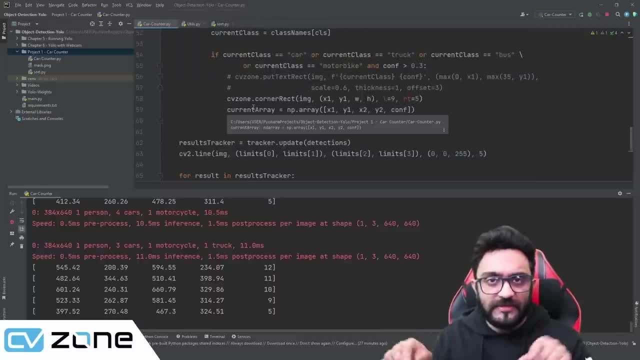 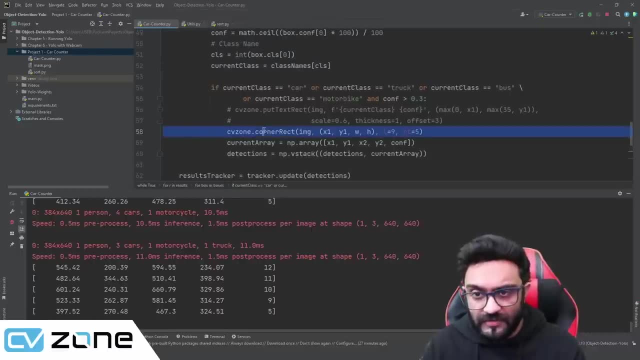 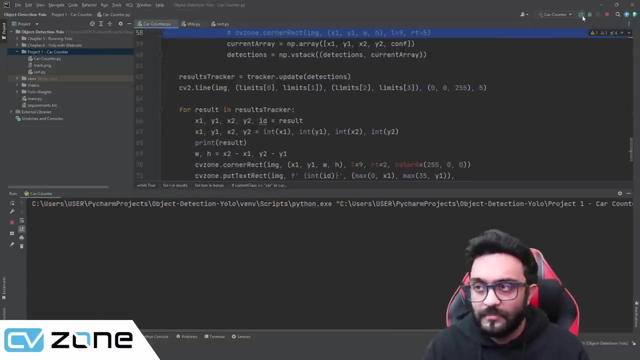 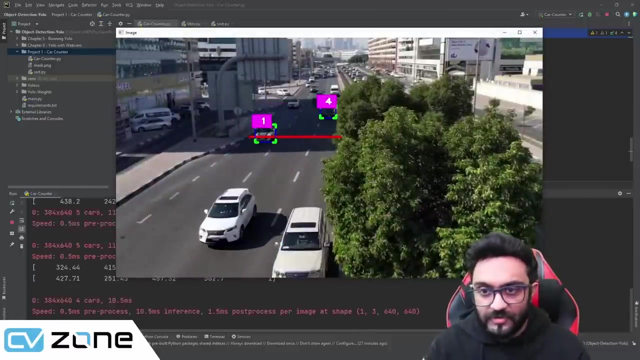 the detection part so we don't need to draw the uh, the rectangles detecting only for the tracker. so here the corner rectangle. we can remove that. so now it will only show us the blue ones. there you go. now it's only showing us the blue ones. actually, I look, I like the. 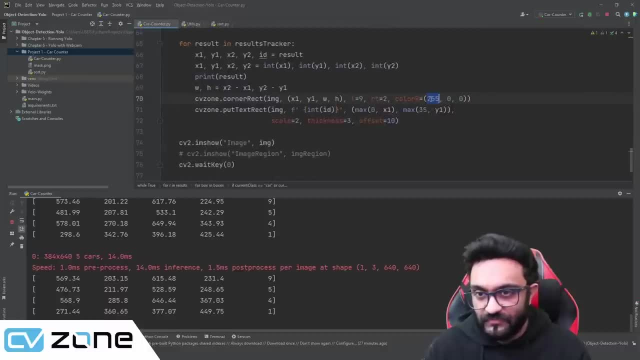 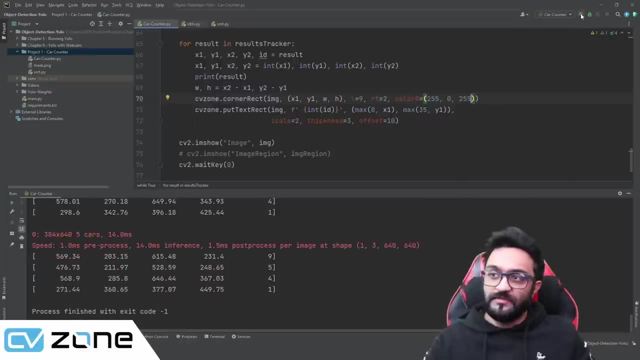 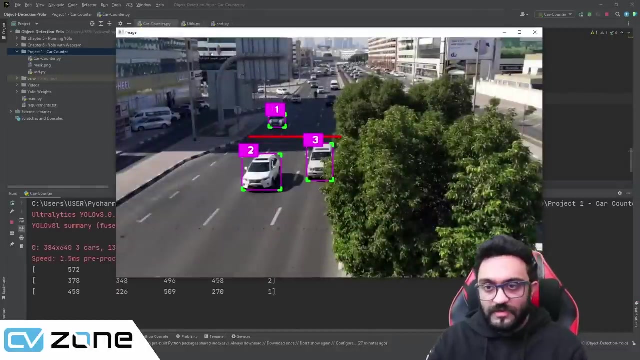 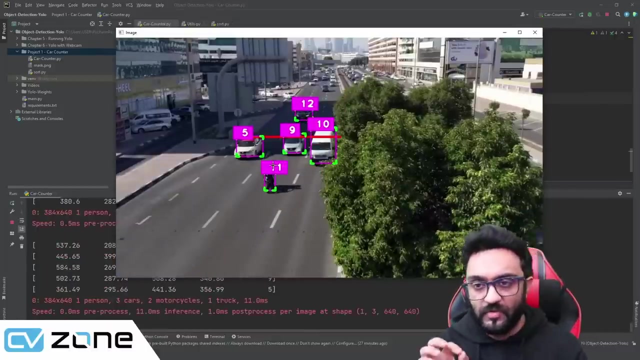 purple color better, let's make it purple 255 and make this 255 as well. so now the the rectangles will be purple. there you go. so yeah, I like that better. so the next step is to find the center point. so once we have those center points we need 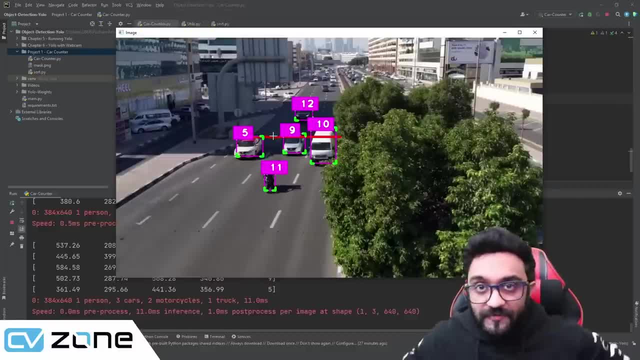 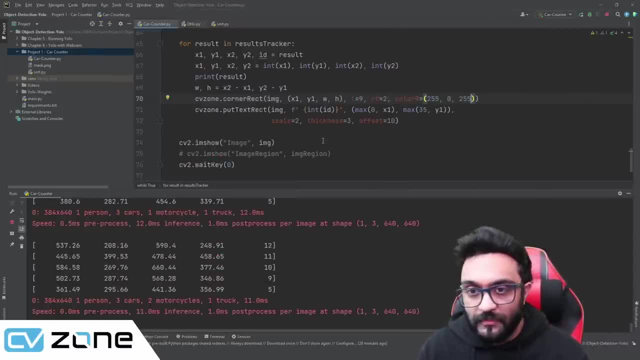 to check if that center point actually touched this line. if that center point actually touched this line, if that center point actually if it touched the line, then we are going to say it was a, it was a count. so that's the idea. so how can we find this? this is our results. we have the X, we 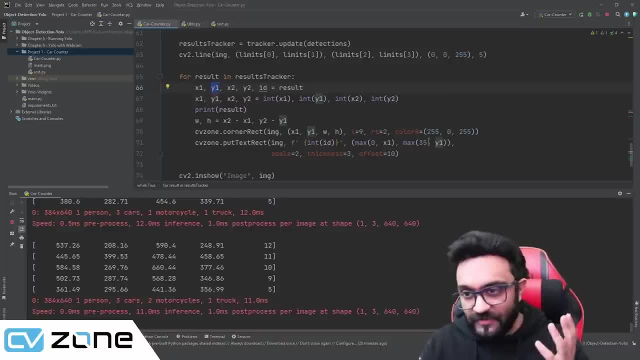 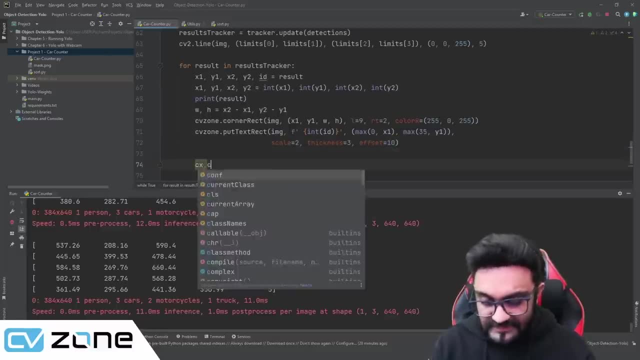 have the Y, we have the width, we have the height, we have everything. all we need to do is we need to find the center. so we will call it C X and C Y. this is the center X and the center Y. and how can we find it? it will be X 1 plus. 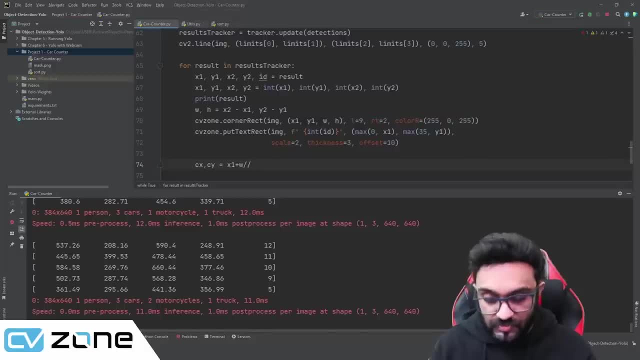 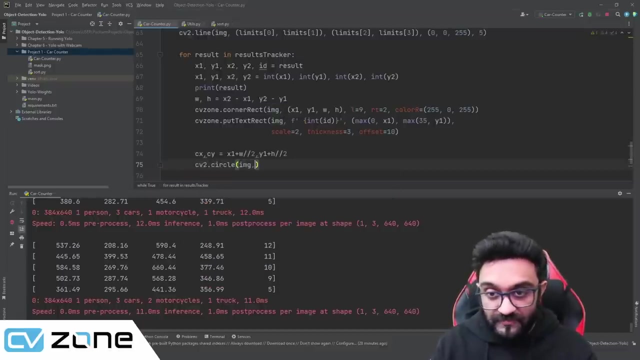 the width divided by 2 and it will be Y 1 plus the height divided by 2. so just to make sure that we are headed in the right direction, we can draw it CV 2 dot circle and we'll give in the image we will give in the C X and the C Y and 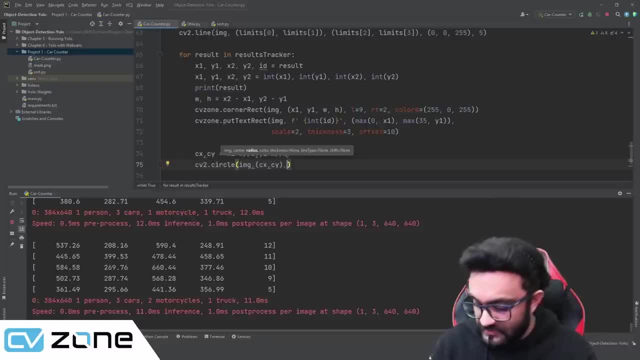 And then we are going to give in the radius. Let's give it 5.. I don't know why I'm giving everything 5 today. So then we will give in the color: 5,, 0, and 255.. Purple again. 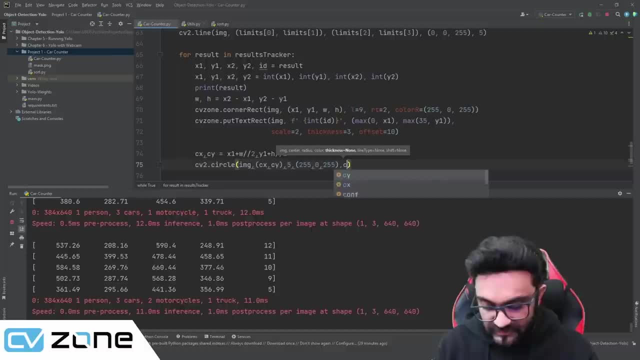 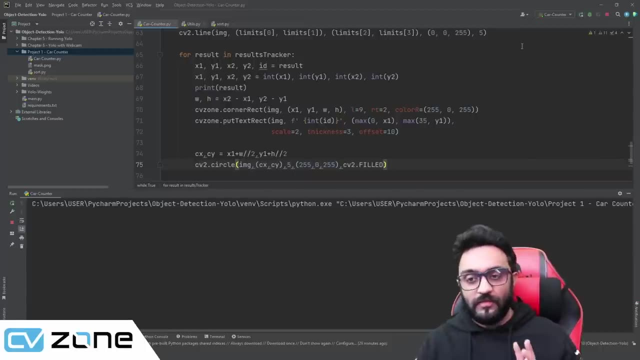 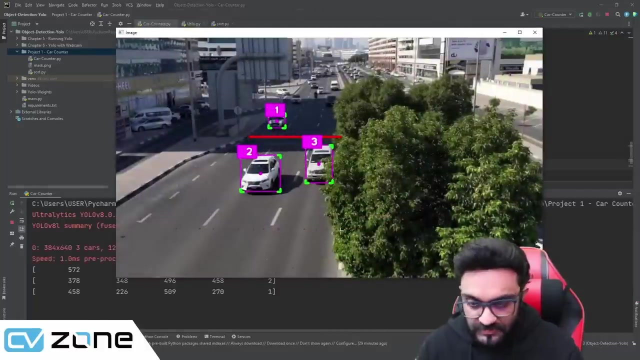 And the thickness, let's put it as CV2 dot filled. So we want it filled completely. So just to make sure that the circles are at the correct position, we are going to draw them And there you go. So here you can see the circles. 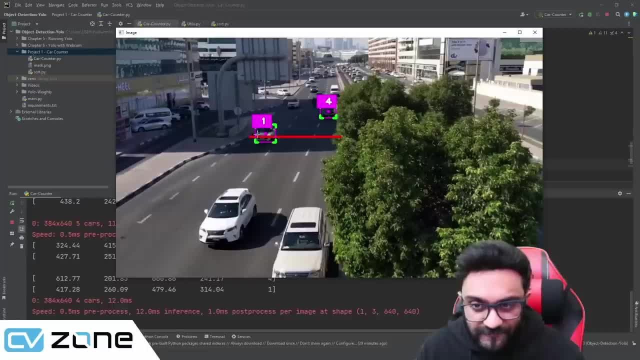 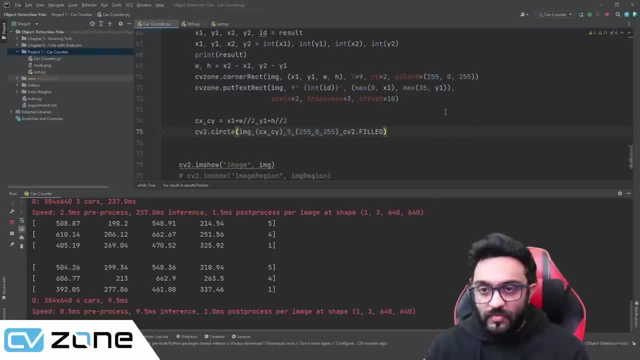 And as soon as this circle actually falls in this region, we are going to count it as detected 1.. There you go. So how can we do that? We can write that if we need to check the limit of the X and we need to check the limit of the Y. 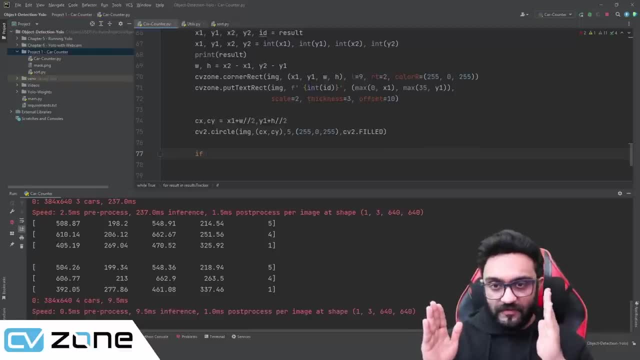 Now the limit of the X is straightforward. We have starting from here, ending till here. It should be within this region. That's simple enough. So we can write that. the limits at 0,. this is our first limit And the limits at 1.. 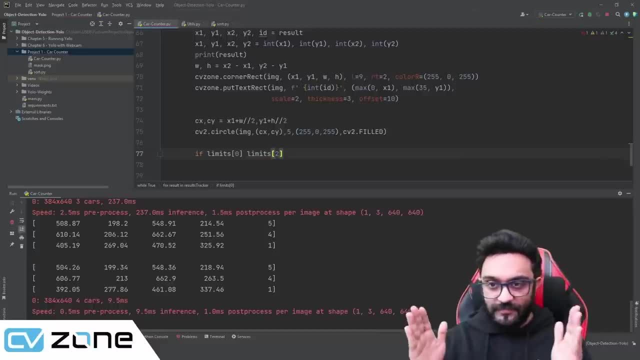 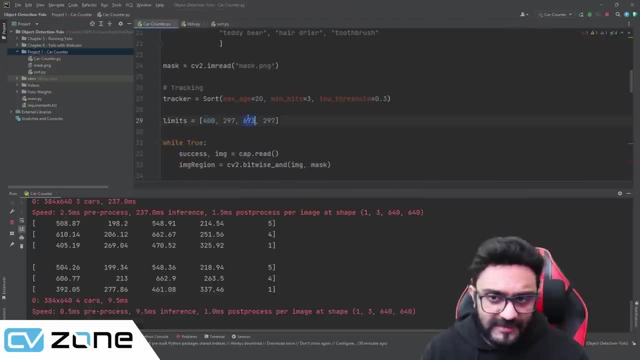 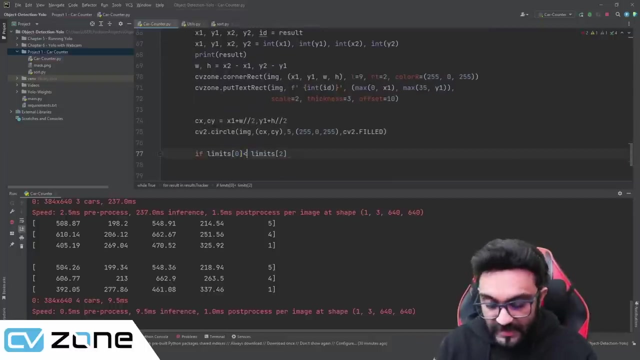 No at 2.. This is the second limit. So X and X, these are the two limits. So the first one is 400.. The second one is 673.. So that's the idea. So we are going to say that if CX is in between that and CY is in between, what limit? 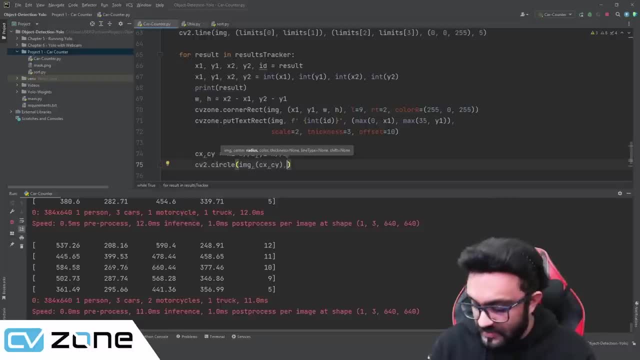 then we are going to give in the radius. let's give it 5. I don't know why I'm giving everything 5 today. so then we'll give in the color: 2, 5, 5, 0 and 2, 5, 5 purple again, and the thickness. let's put it as CV 2 dot filled. so we want it. 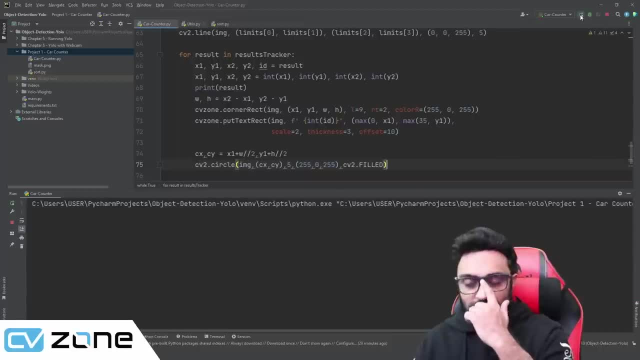 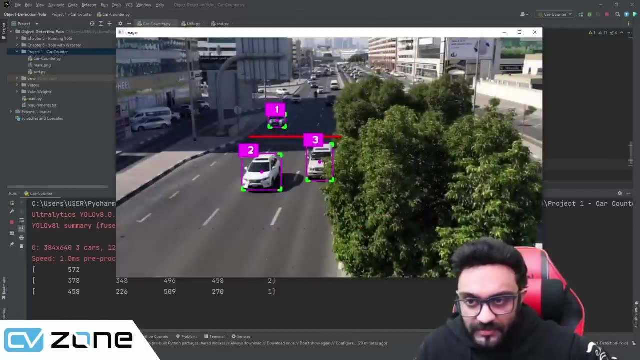 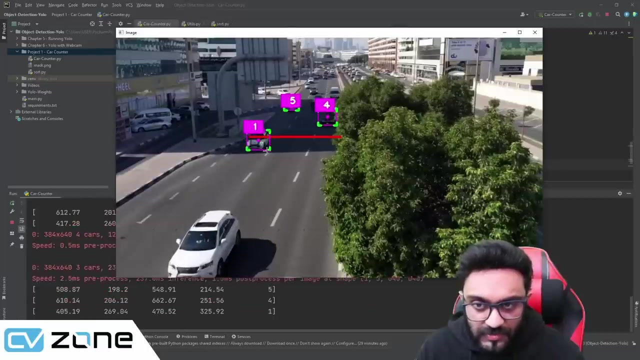 filled completely. so just to make sure that the circles are at the correct position, we are going to draw them and there you go. so here you can see the circles, and as soon as this circle actually falls in the middle of the circle, we are going to mark our circle in preciseALimit. 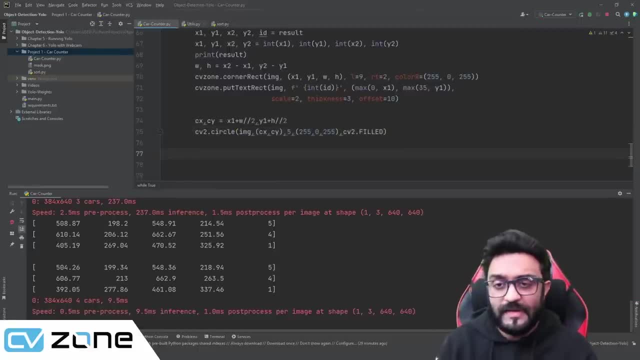 by about 1 .0. so in this region we are going to count it as detected 1. here you go. so how can we do that? we can write that if we need to check the limit of the X and we need to check the limit of the Y, now the limit of the X is. 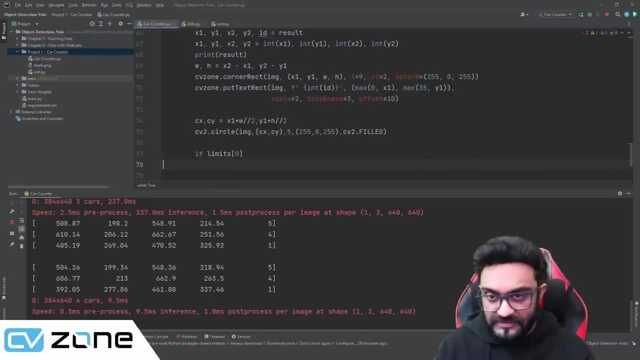 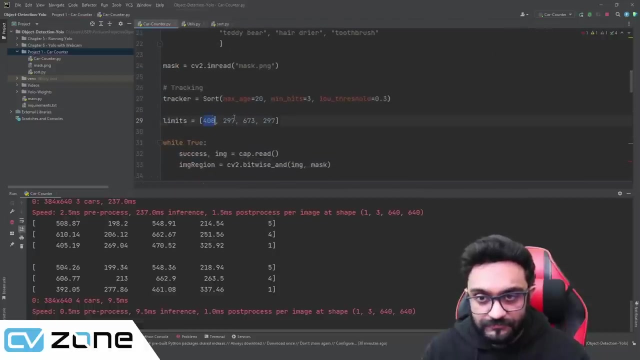 straightforward. we have starting from here, ending till here. it should be within, and the limits at one, no at two. this is the second limit. so x and x, these are the two limits. so the first one is 400, the second one is 673. so that's the idea. 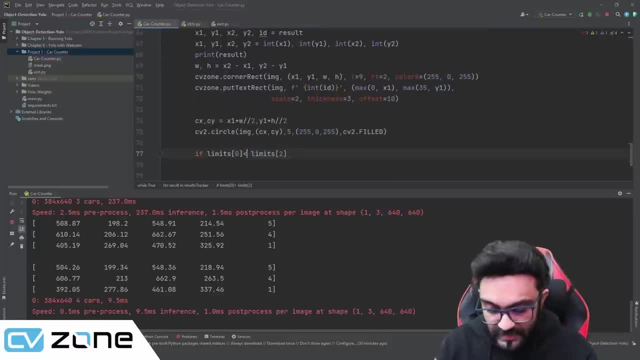 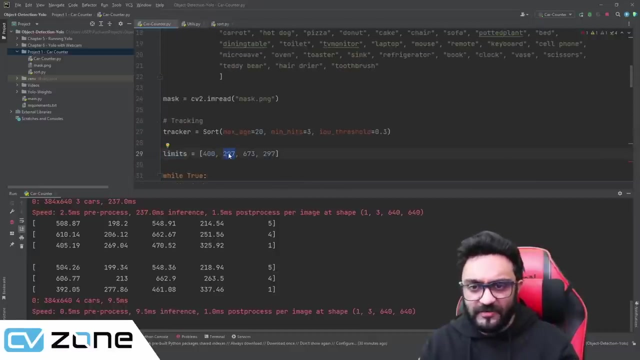 so we are going to say that if cx is in between that and cy is in between, what limit? now we don't want to say if cy equals, uh, the exact value of our limit, no, we don't want to say that, because this is just single value. the height is a single value, 297. so we don't want to say if the 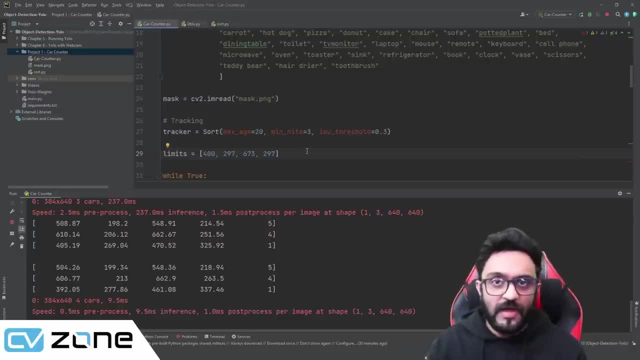 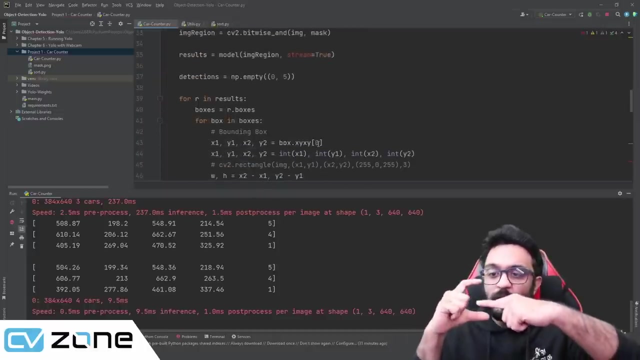 value is exactly 297, then detect it as a count, because sometimes, uh, the car may be fast and it might not touch that uh pixel value, so putting it one as one pixel value might be a problem. so what we need to do is we need to create a region. so this is our line. we. 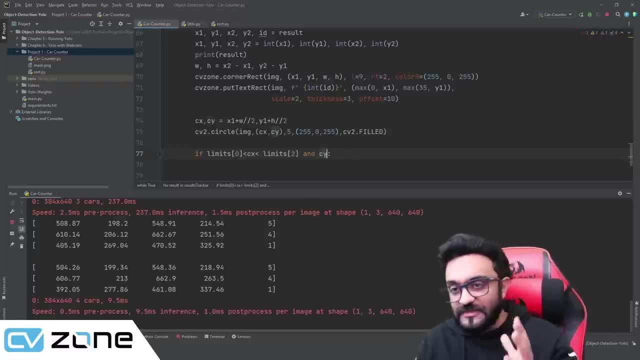 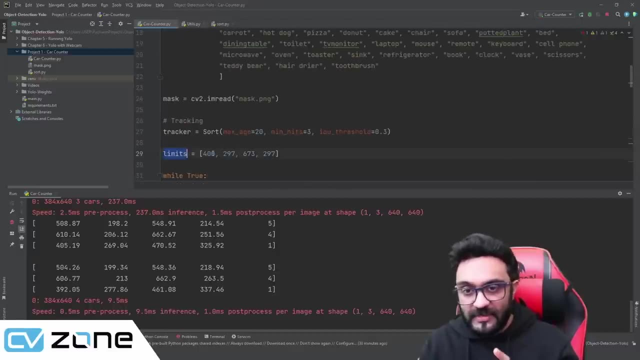 Now we don't want to say if CY is in between, that. We don't want to say if CY equals the exact value of our limit, No, we don't want to say that, because this is just a single value. The height is a single value: 297.. 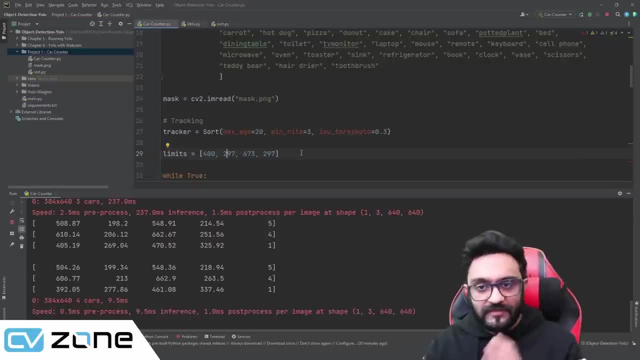 So we don't want to say: if the value is exactly 297, then detect it as a count, Because sometimes the car may be fast and it might not touch that pixel value, So putting it as one pixel value might be a problem. So what we need to do is we need to create a region. 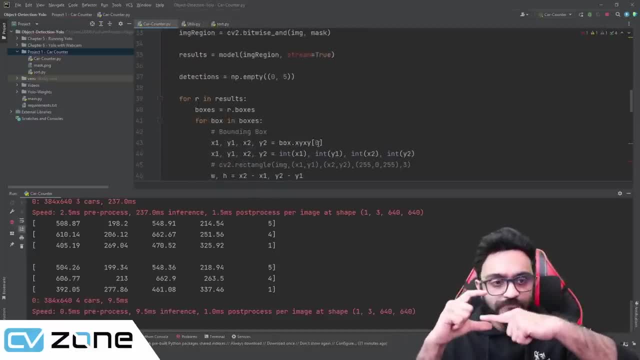 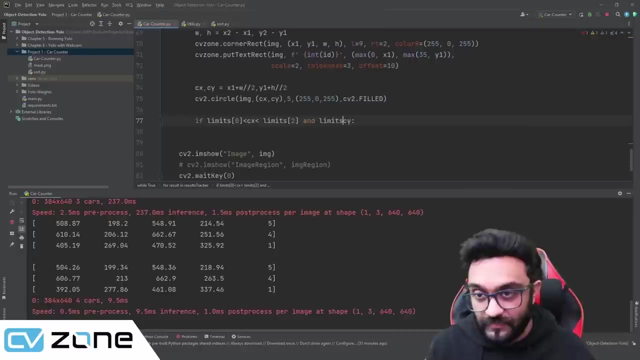 So this is our line. We will have this region, Can you see? Yeah, So you will have this region in which, if it lies, then it is detected as a count. So what we can do is we can simply write that limits at 1 plus 20, or for this instance, 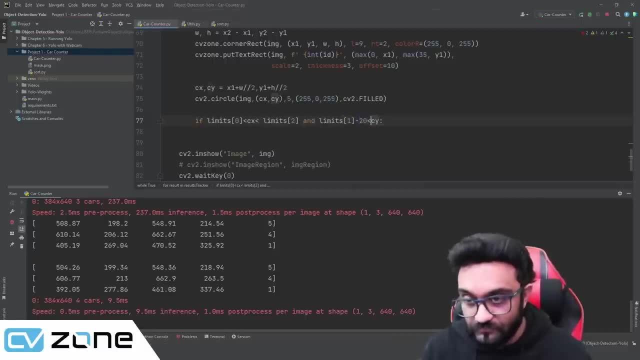 minus 20.. And for the next limit we are going to say 0. And for this one we can say plus 20. So if it falls in that region, then only it will detect it as detected. So then we are going to say that total counts plus equals 1.. 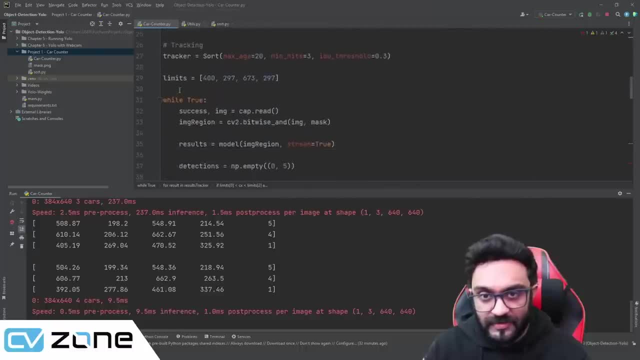 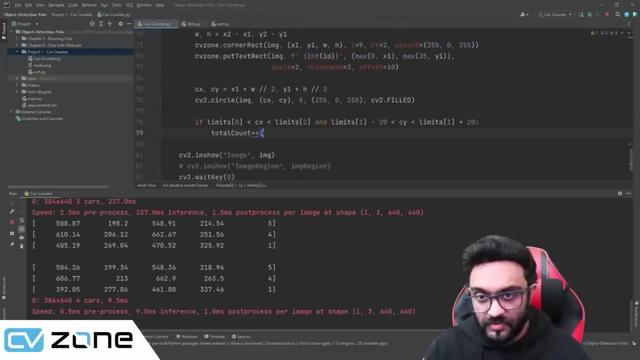 And we didn't define total counts. So we will write here after tracking. We will write here: Total count equals 0.. So total count plus equals 1.. And all we have to do is now we have to show the total count. 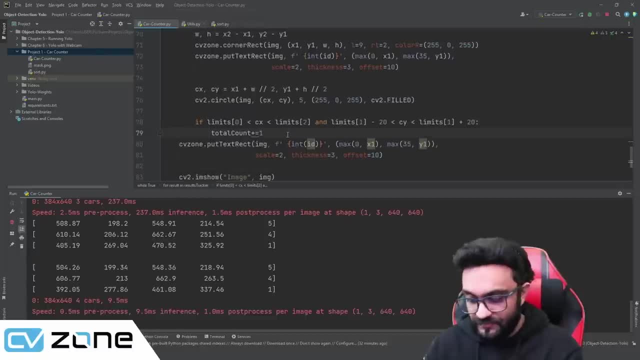 So let's copy this CVZone function, We will put it on the image, We will write count and colon And then we will write total count. It's already integer, so we don't need to worry about that, And we will give in the value of x, as let's say 50, and y, as let's say 50 as well. 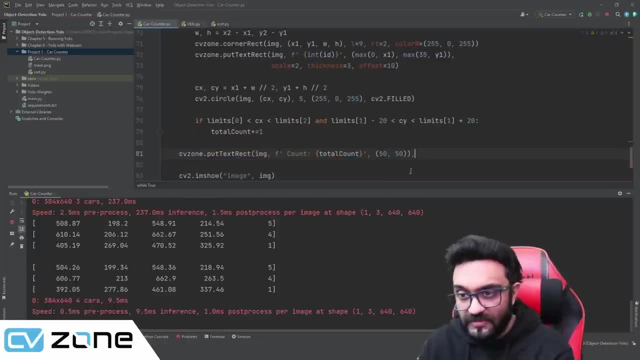 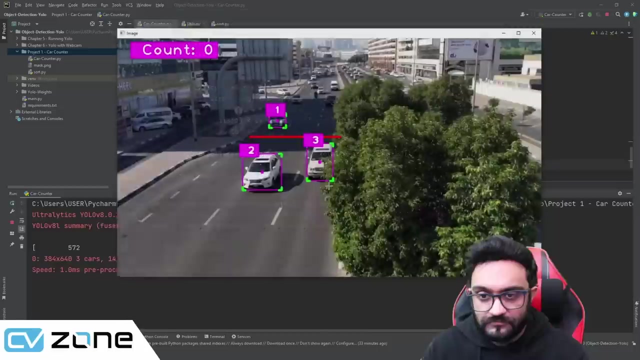 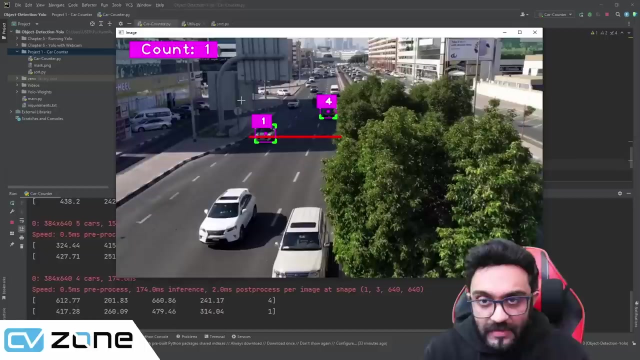 So 50,, 50. And the rest we will keep at default. What happened? OK, So let's run that. There you go. So the total count right now is 0, because nothing passed that region. So if we keep pressing, and there you go. 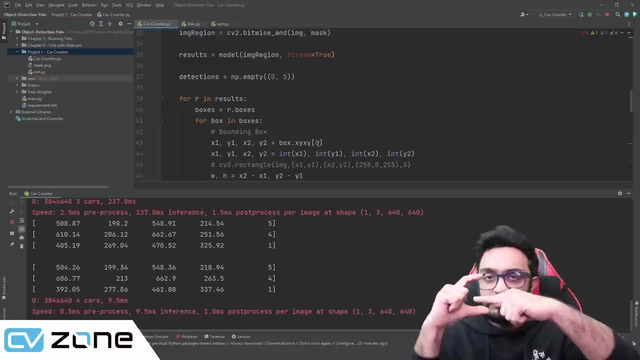 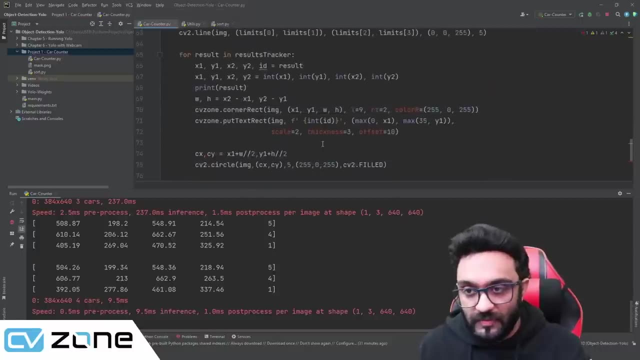 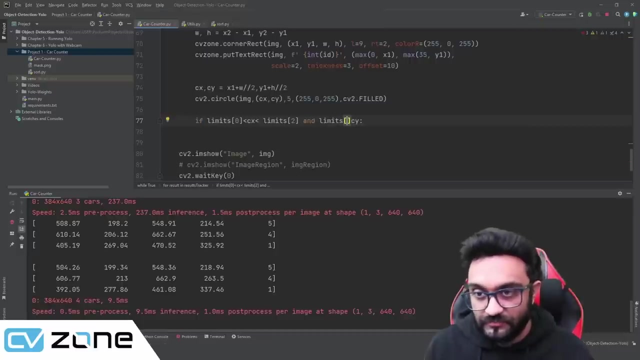 will have this region, can you see? yeah, so you will have this region in which, if it lies, then it is detected as a count. so what we can do is we can simply write that limits at 0, no, at 1 plus 20, or, for this instance, minus 20 and for the next. 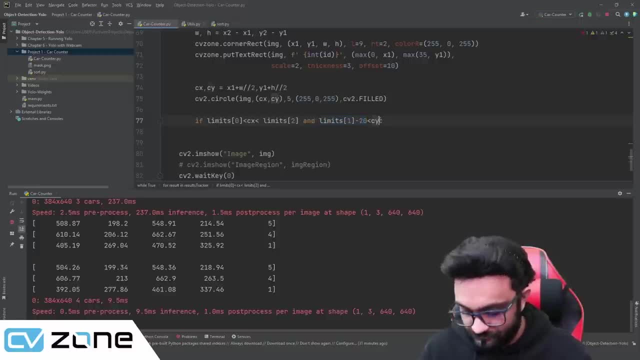 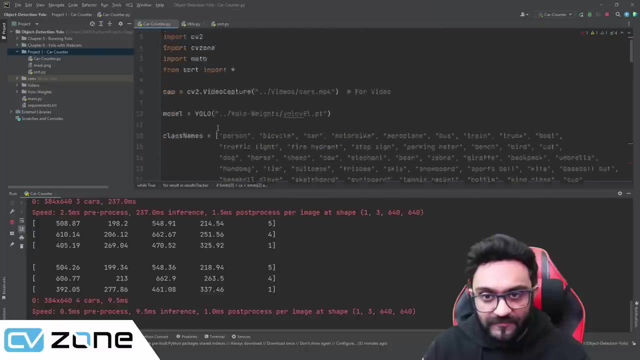 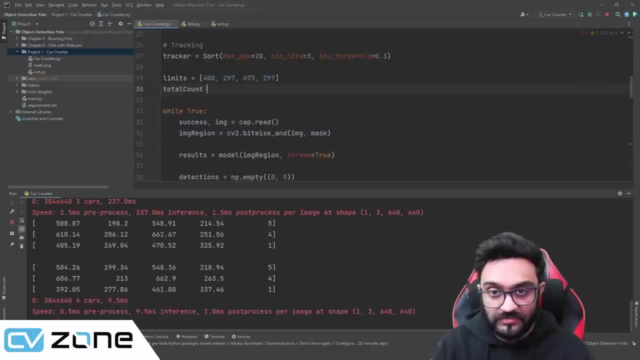 one, we can say plus 20, so if it's, if it falls in that region, then only it will detect it as detected. so then we are going to say you that total count plus equals 1 and we didn't define total count. so we will write here after tracking, we will write here: total count equals 0, so total count. 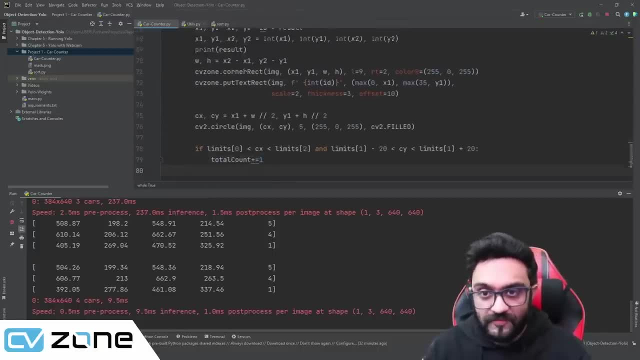 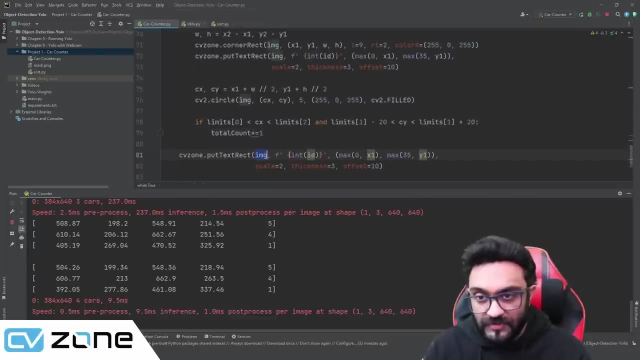 plus equals 1, and all we have to do is now we have to show the total count. so let's copy this CV zone function. we will put it on the E, we will put, we will write count and colon and then we will write total count. it's already integer, so we don't need to worry about. 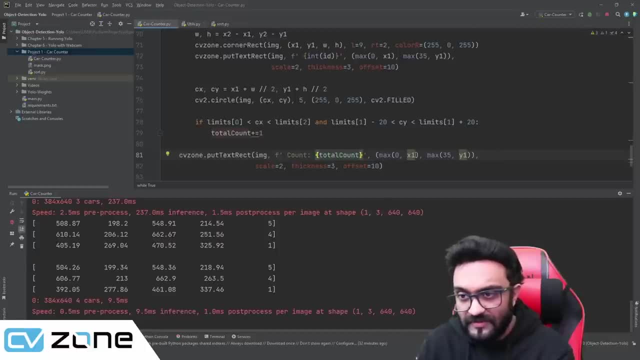 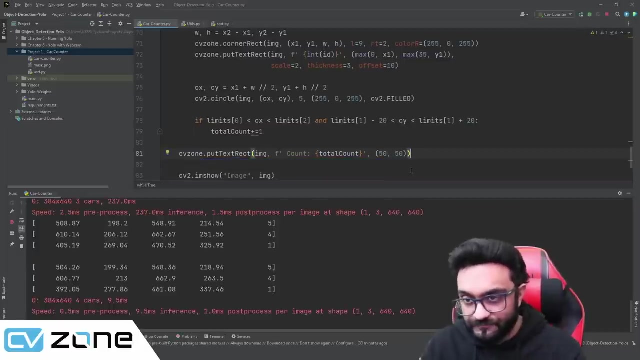 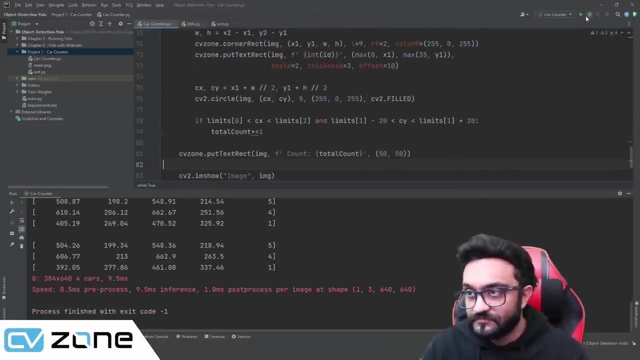 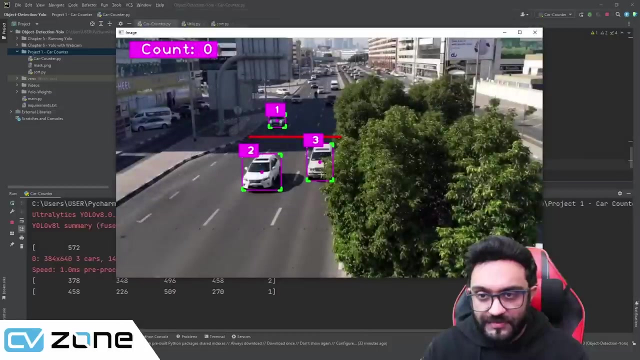 that, and we will give in the value of x, as let's say 50, and why, as let's say 50 as well. so 50, 50 and the rest we will keep at default. uh, what happened? okay, so let's run that. there you go. so the total count right now is zero, because nothing passed that region. 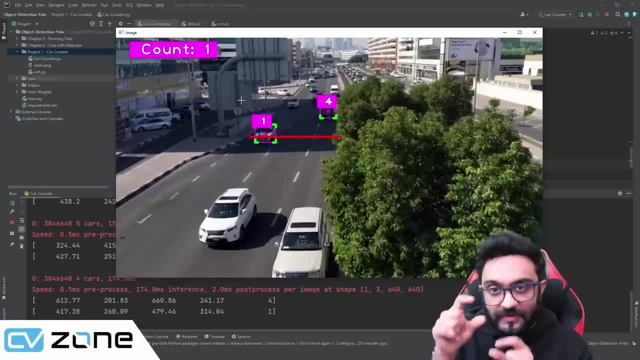 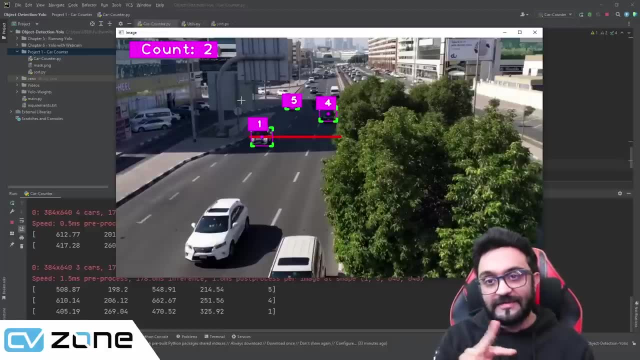 so if we keep pressing, and there you go, now it entered that region and it counted as one. but now you will see an issue if i press again. it counted it as two because it is still in that region. uh, because it's not just a single line, it's a region where it lies. so because it's already, 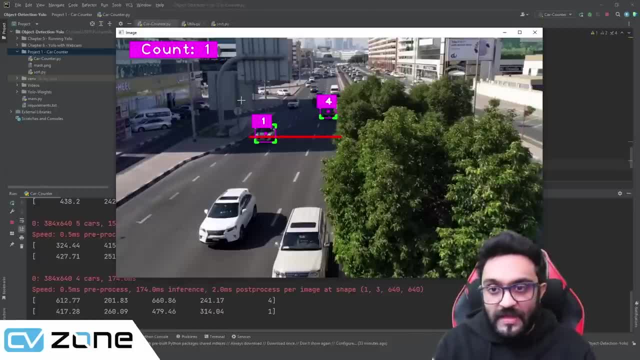 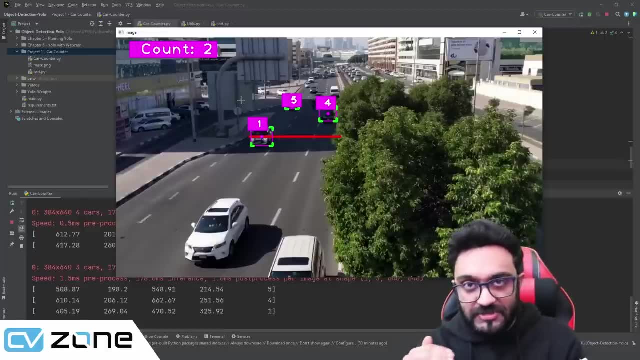 Now it entered that region and it counted as 1.. But now you will see an issue If I press again. it counted it as 2 because it is still in that region, because it's not just a single line, It's a region where it lies. 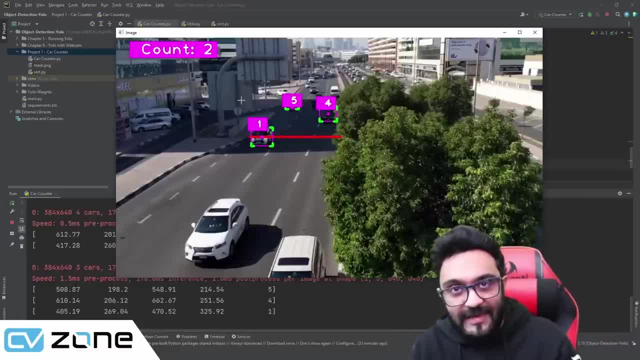 So because it's already there, It's counted it as 2.. Now if we make this region very small, it might not count it at all because it's very low, But if we make it very big, then it will have multiple counts. 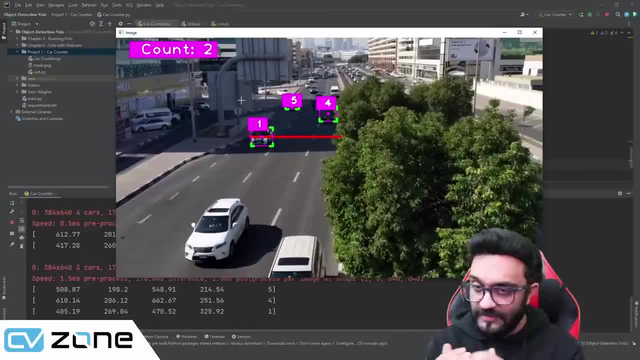 So we need to have a balance. First of all, we need to have the balance, And the second thing that we do need is we need to check if this ID is already counted or not. If it's already counted, we will not add it to the counter. 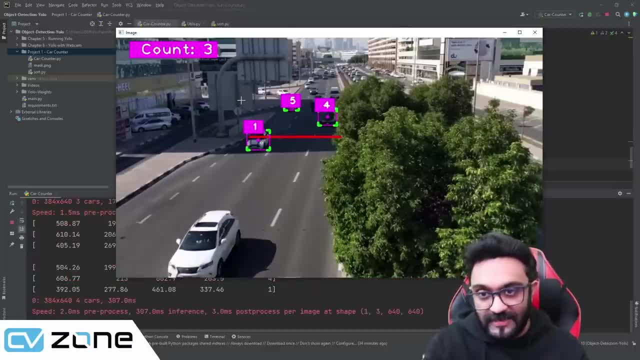 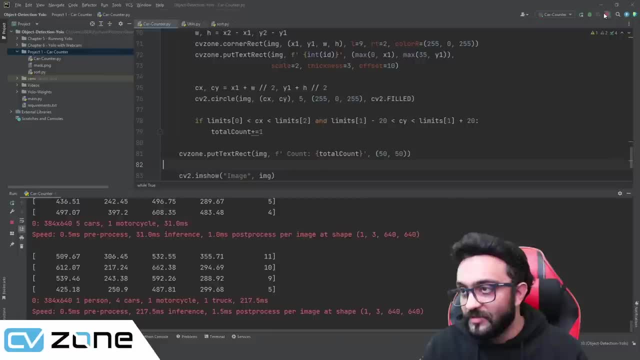 That's how we will fix this issue, Because if I run it again at the same point, it has counted three times, So that's not good. OK, so how can we do that? Instead of making it a variable, we will make it a list. 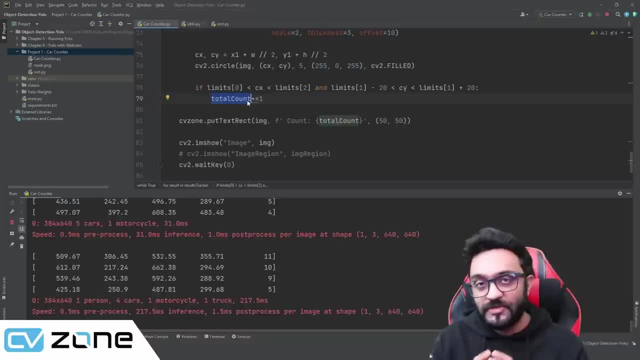 I'm talking about the total count. So instead of making total count a variable, we'll make it a list, And in that list we will put IDs, So 1,, 2,, 5,, 8,, 9,, things like that. 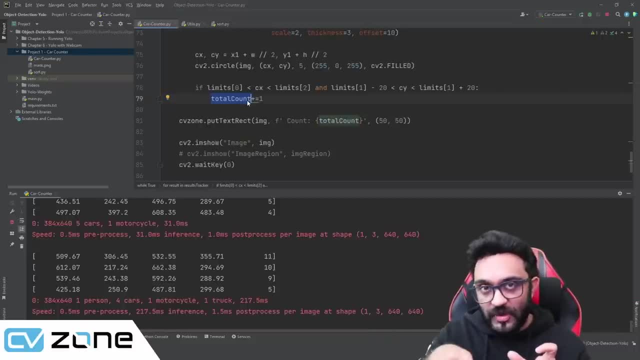 So then, whenever we do that, When we detect a new count, we will check if that ID is already present, We will not count it. If it's there, we will not count. If it's not there, we will add it. 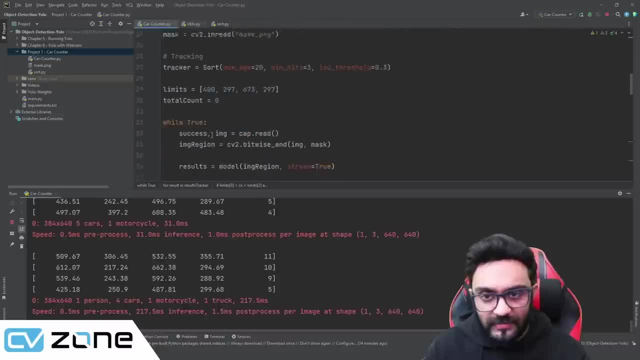 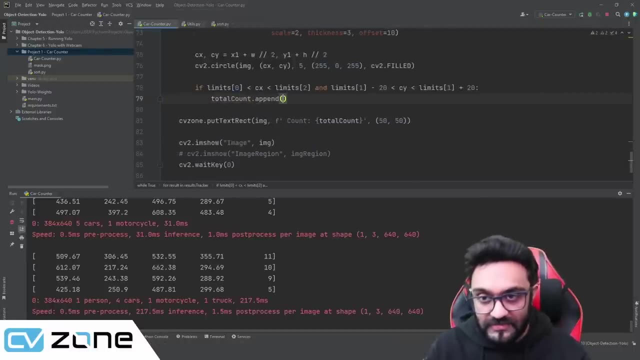 OK, so how will it look like? So, total count. we will make it a list And then we will go down and here we will say total count, dot append, And we are going to append the value of the ID. OK, But how can we check if it's already there or not? 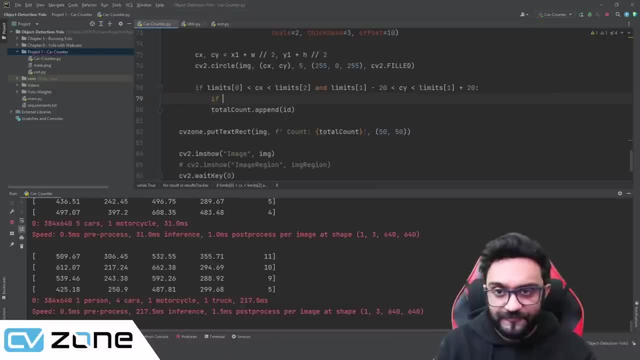 In the total count. we will check, We'll write. if the total count, dot count of the ID equals zero, then do this. Now, what does this mean? So basically, we are telling it to find the number of times when we write dot count. 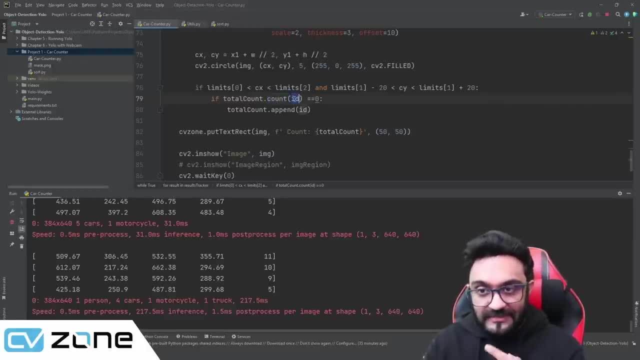 It means count the number of times This ID is present in this list. So, for example, if it was five here, it will count the number of times five is available here. If five is not available, it will be zero. If there were two fives, it will be one. 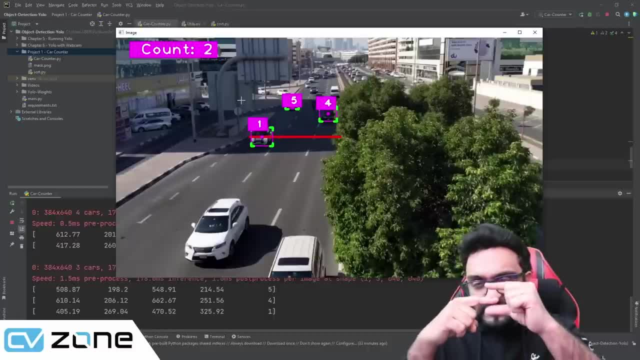 there it's counted it as two. now, if we make this region very small, it might not, it might not count it at all because it's very low. but if it make it, if we make it very big, then it it will have multiple counts. so we need to make sure that we make sure that we make sure that we make sure that. 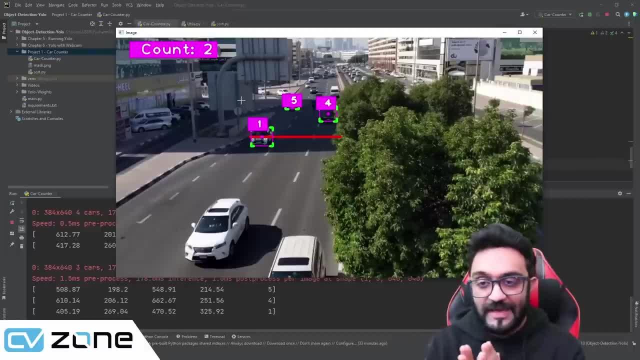 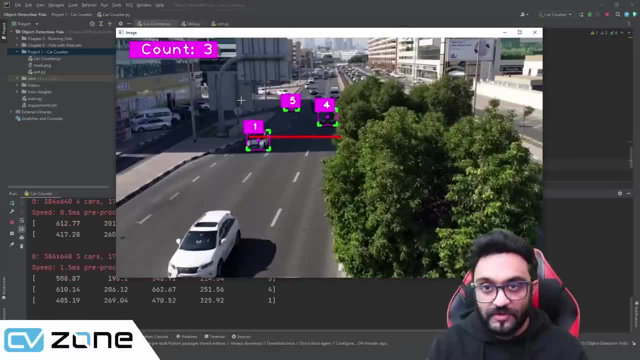 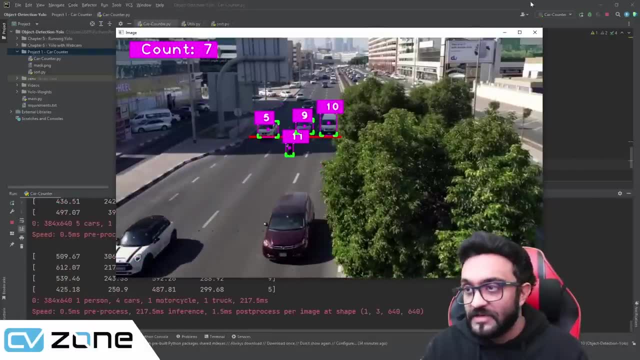 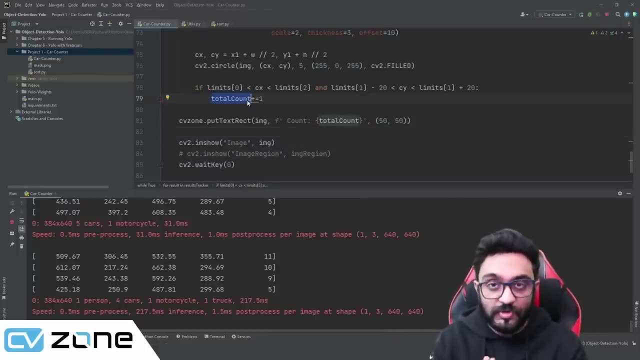 to the counter. that's how we will fix this issue, because if i run it again at that same point, it has counted three times, so that's not good. okay, so how can we do that? instead of making it a variable, we will make it a list. uh, i'm talking about the total count. 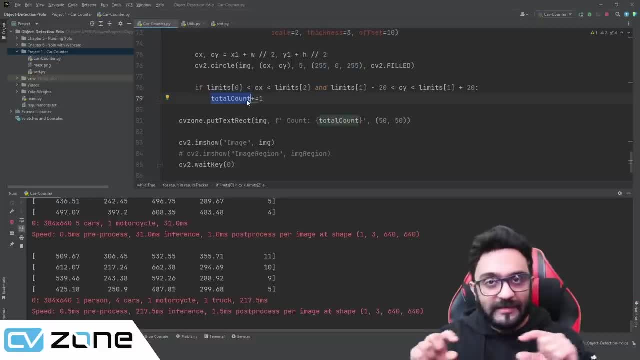 so instead of making total count a variable, we'll make it a list, and in that list we will put ids, so one, two, five, eight, nine things like that. so then, whenever we detect a new count, we will check if that id is already present. we will not count it if it's there, we will not count if it's not. 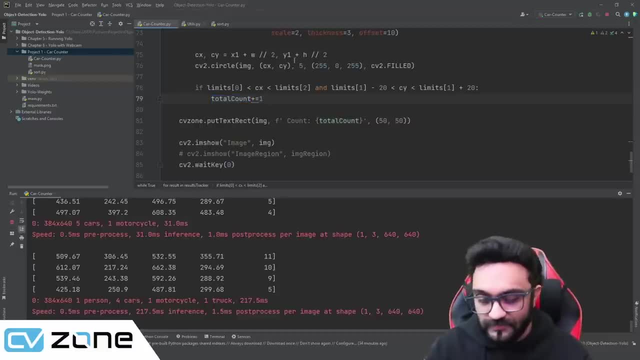 there, we will add it, okay, so how will it look like? so, total count. we will make it a list and then we will go down and here we will say total count, dot append, and we are going to append the value of the id. okay, but how can we check if it's already there or not in the total count? 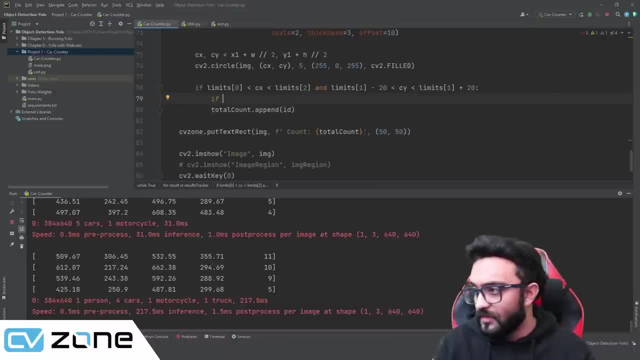 we will check, we will write. if, uh, the total count, dot count of the id equals zero, then do this now. what does this mean? so basically, we are telling it to find the number of times. when we write dot count, it means count the number of times this id is present in this list. 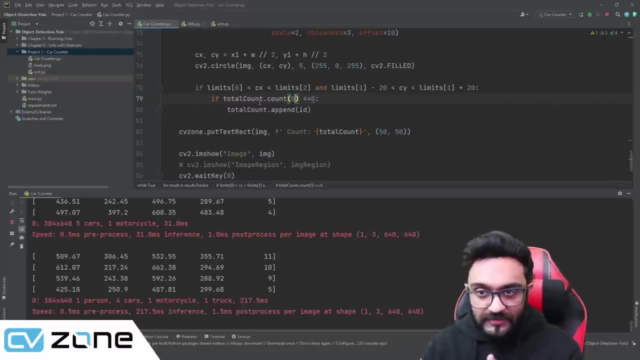 so, for example, if it was five here, it will count the number of times five is available here. if five is not available, it will be zero. if there were two fives it will be one- oh sorry, two- and then if there is no five, it will be zero. so this is what we are saying. so we are saying: 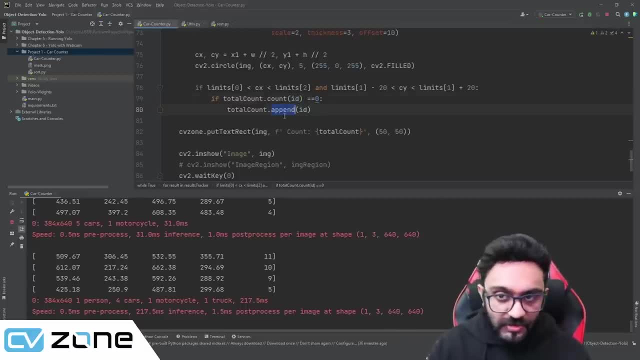 if this id is not already present, then total count dot- append id. so this time it should be correct. but now it is a list, it is not an actual value that we can just write here. so all we have to do is we have to find the length of this list, so that will be the total count. so 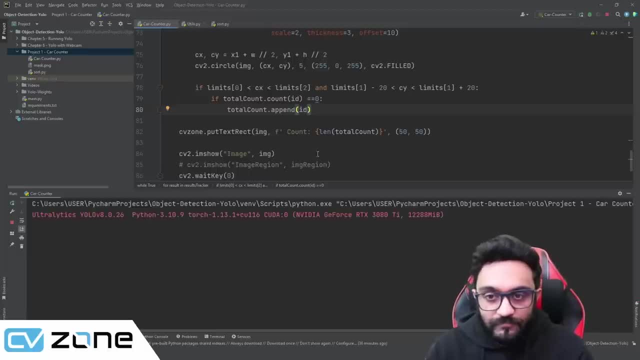 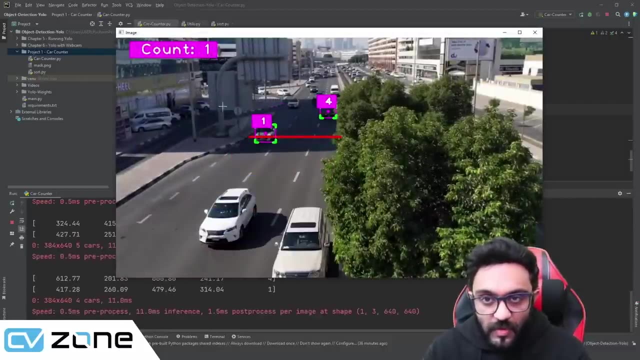 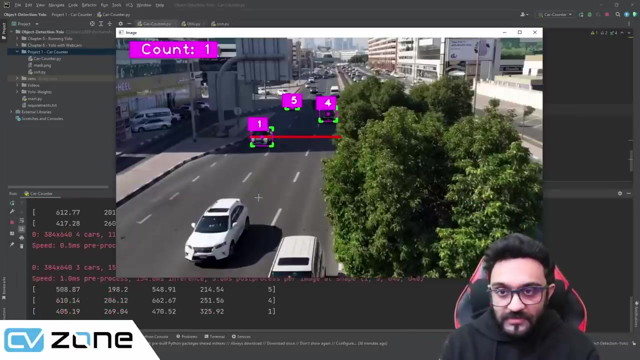 let's stop that and run it again. and this time around, if we click, this is count is one. now, if i go to the next frame, it should not count. there you go, didn't count. if i go again to the next frame, it should not count, didn't count. 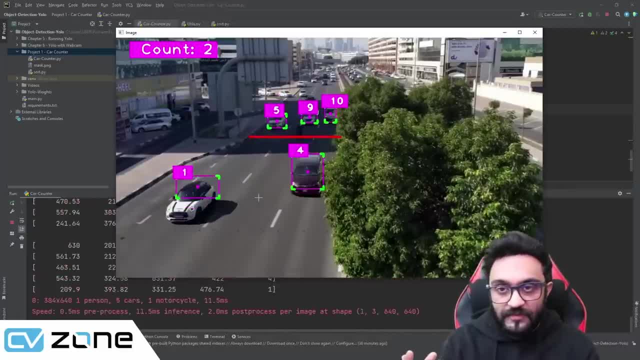 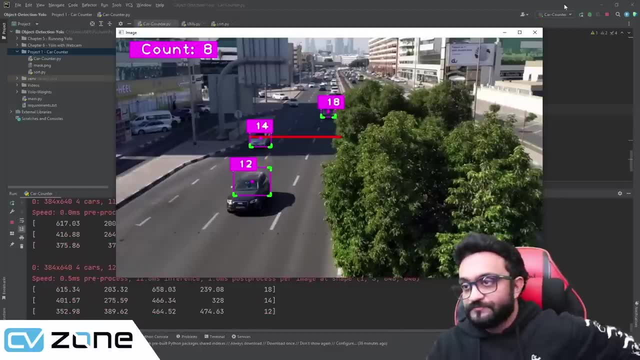 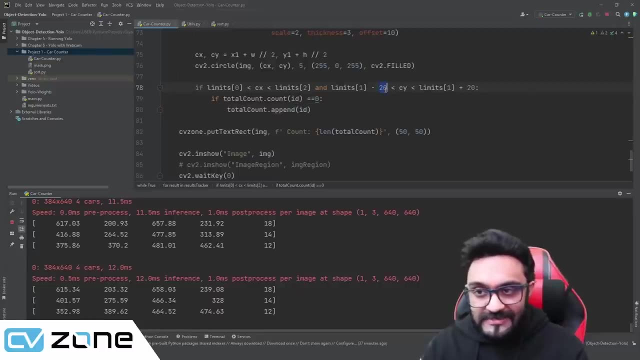 now it should count because that's the second id. then it should count third id, fourth, fifth, sixth, seventh, eighth and so on. so if you, if you see that some of the detections are missing, uh, what you can do is you can increase this value, you can make it 30, because right now we have another check, that is: 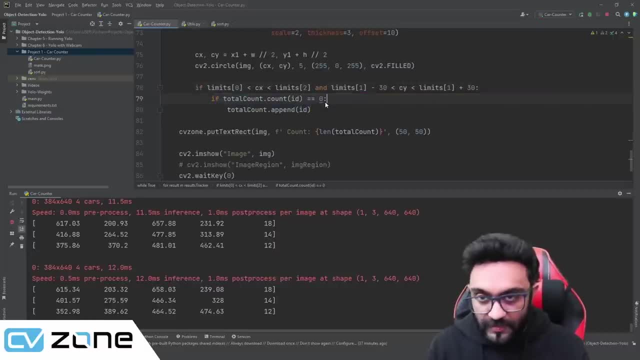 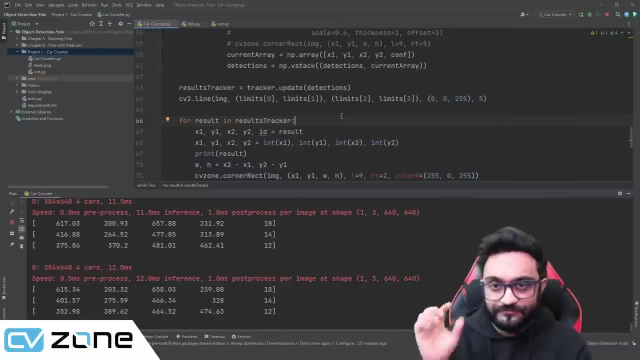 checking whether it's a duplicate or not, so we don't have to worry about that. and the second thing we can do is we can change the color of this line. we can change the color of this line so that whenever it's detected something, it turns green, so it's an indication that it had a count. 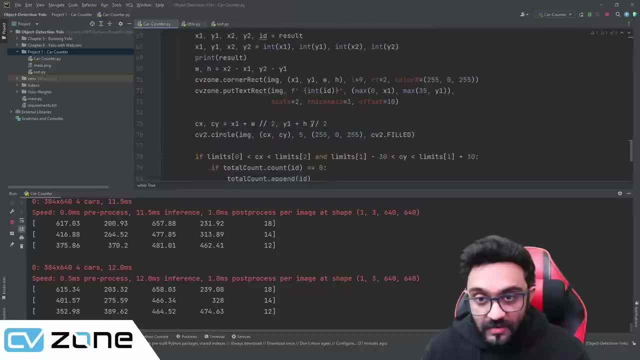 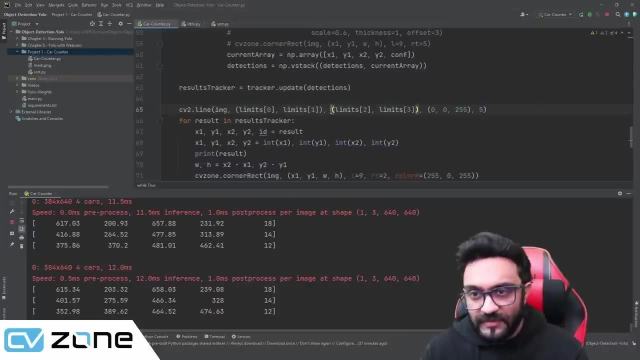 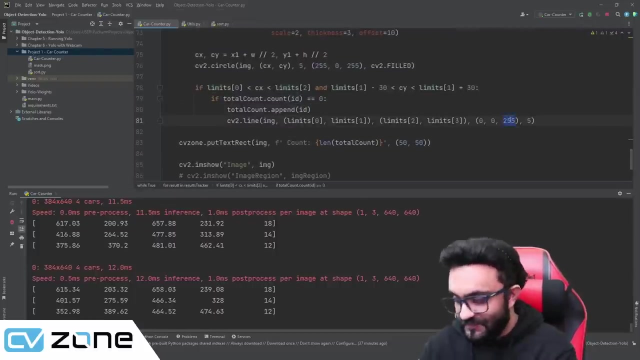 so we can print it, uh, maybe here at the end, or or we can simply print it again in red color. i know it's it's a weird way to do this, but you can do this. uh, you can just simply print it again, and instead of red, 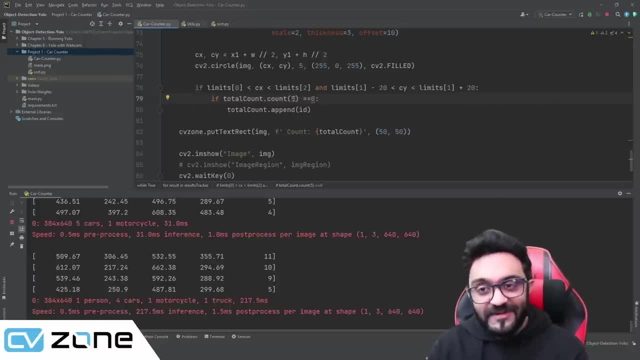 Oh sorry. two, And then if there is no five, it will be zero. So this is what we are saying. So we are saying, if this ID is not already present, then Then total count dot append ID. So this time. 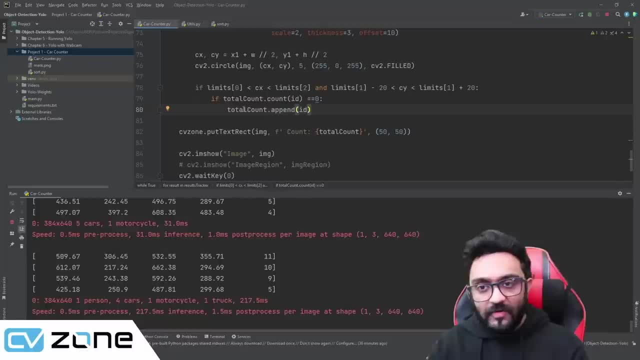 It should be Correct. But now it is a list, It is not an actual value that we can just write here. So all we have to do is we have to find the length of this list. So that will be the total count. 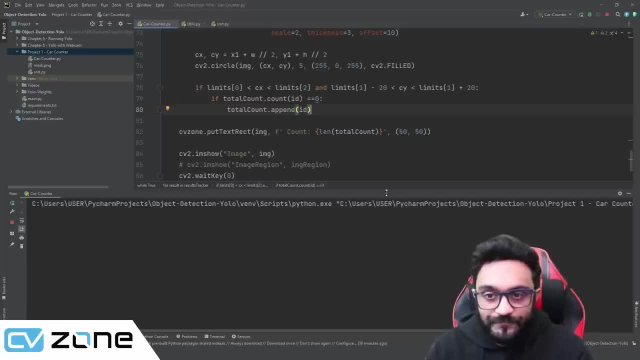 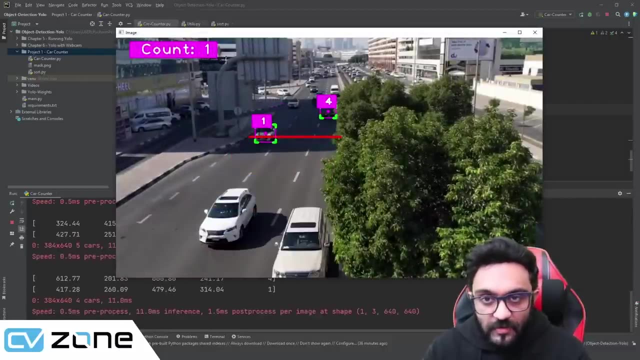 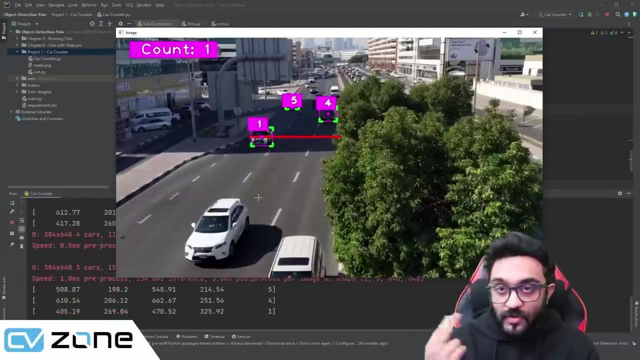 So let's stop that and run it again, And this time around, if we click This is, count is one. Now, if I go to the next frame, it should not count. There you go, Didn't count. If I go again to the next frame, it should not count. 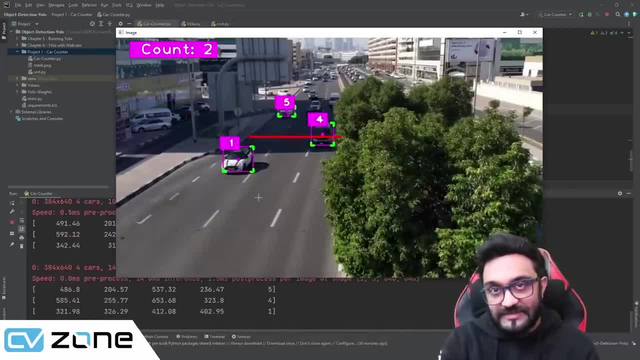 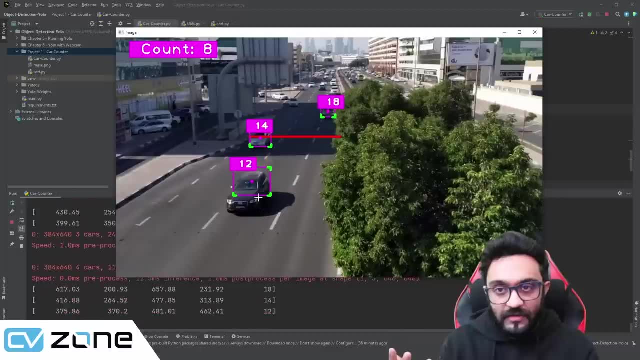 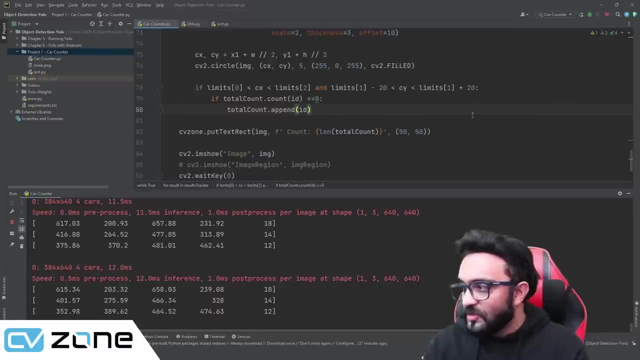 Didn't count, Now it should count because that's the second ID. Then it should count third ID, fourth, fifth, sixth, seventh, Eight and so on. So if you, if you see that some of the detections are missing, what you can do is you can increase this value. 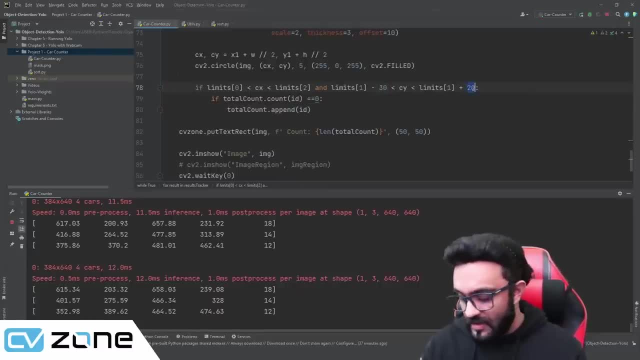 You can make it 30. Because right now we have another check that is checking whether it's a duplicate or not. So we don't have to worry about that. And the second thing we can do is we can change the color of this line. 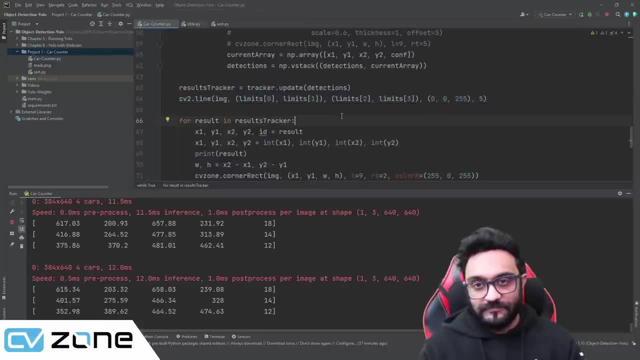 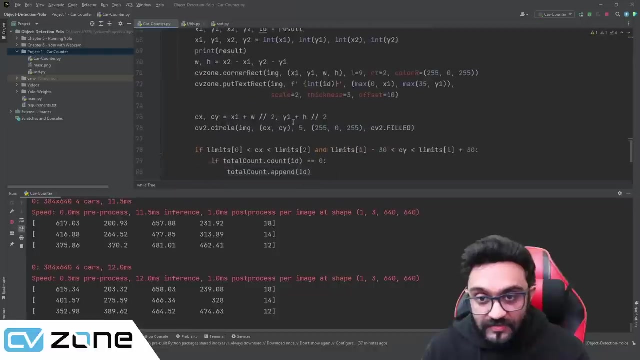 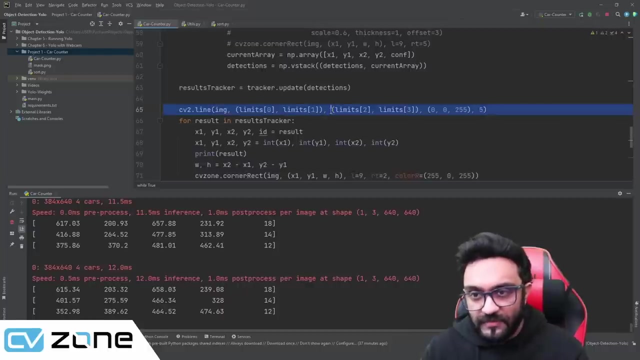 We can change the color of this line so that whenever it's detected something, It turns green, So it's an indication that it had a count. So we can print it, Maybe here at the end, Or or We can simply print it again in red color. 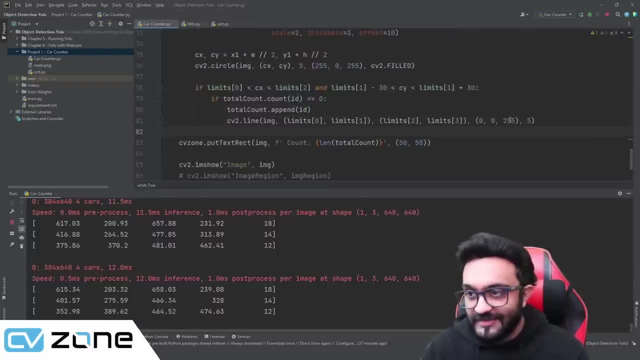 I know it's it's a weird way to do this, but you can do this. You can just simply print it again And instead of red I will print it as green, So it's basically overlaying on top of it, Okay. 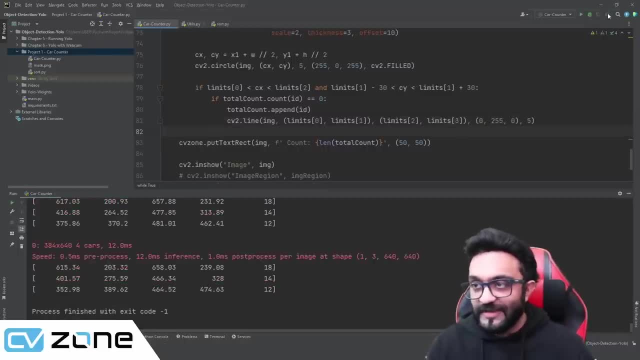 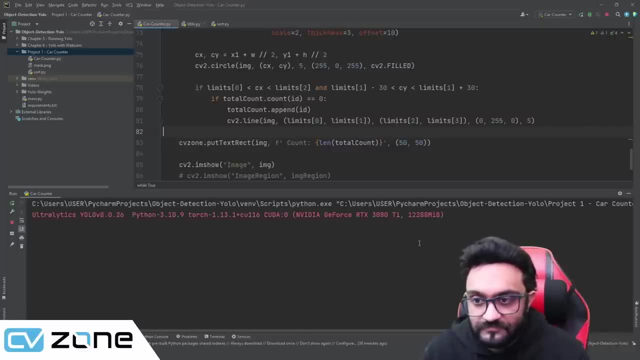 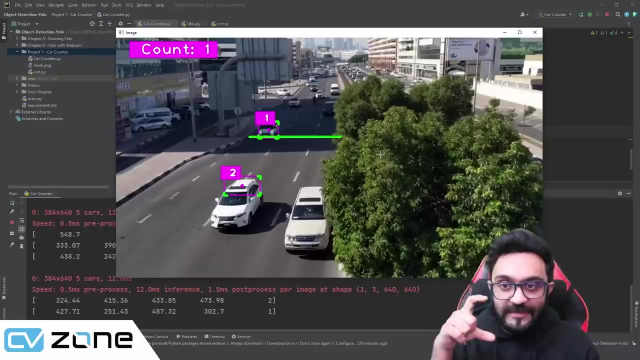 i will print it as green, so it's basically overlaying on top of it. okay, there you go. so if we run this now, at this point, it is detecting as a count because it's within that region, and then it's detecting. maybe it's too early. 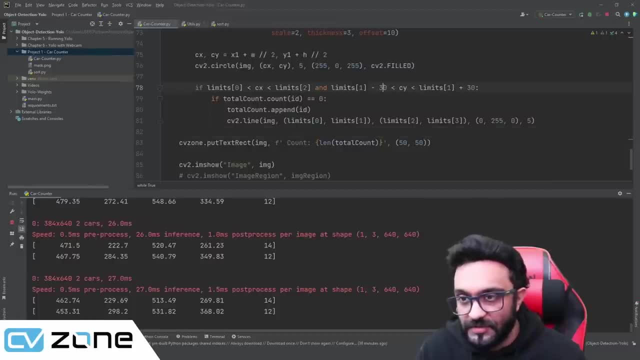 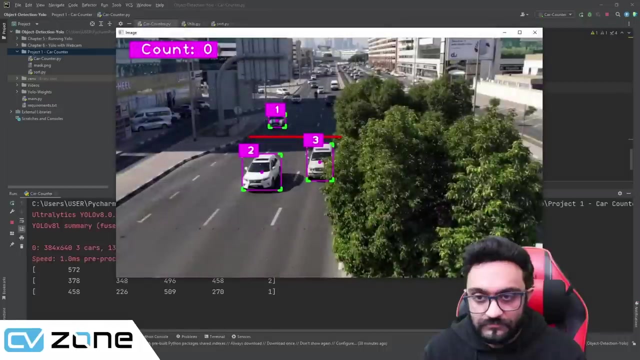 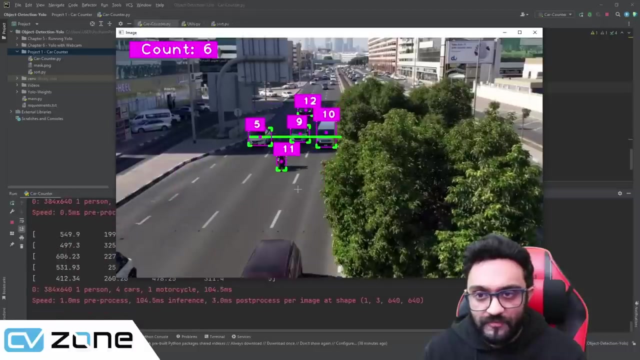 okay, maybe it's too early. early, let's reduce this to 20 back, or let's put it as 15, and let's put this as 15 as well. yeah, i think that's better. two, three, four, five, six, that's correct. then seven, that's correct, uh. 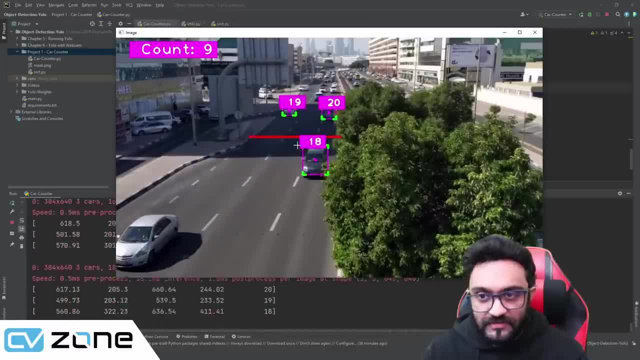 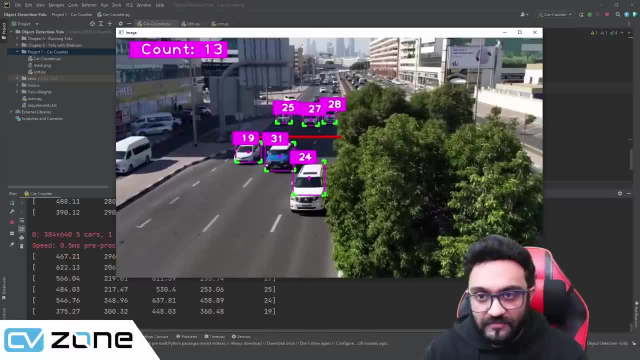 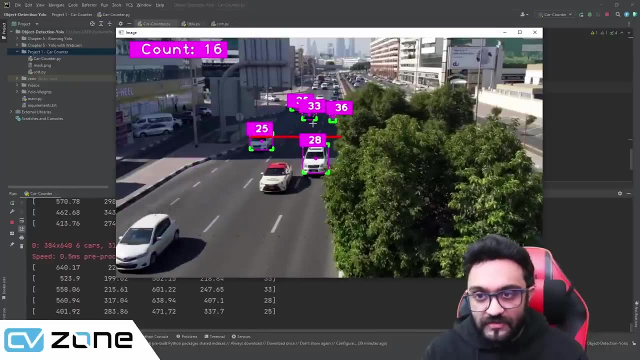 then we have eight, that's correct. nine, this will be 10, this will be 11, 12, 13, 14, so it should be 14 till here. uh, then 15, 16, it should be 16 when it crosses these all. 16, that's correct. then 17, 18, 19. 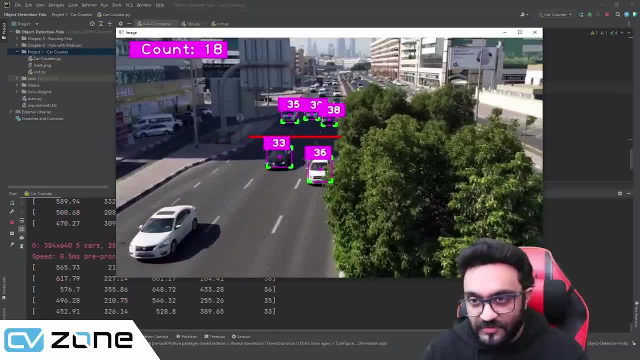 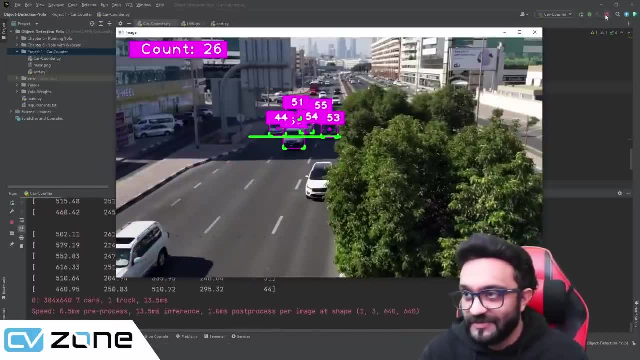 17, 18. that was 19, then 20, 21. it should be 21. after this, this is 22. okay, this is getting confusing. that's why we have the computer to actually find it for us. so what we can do now is we can go down. 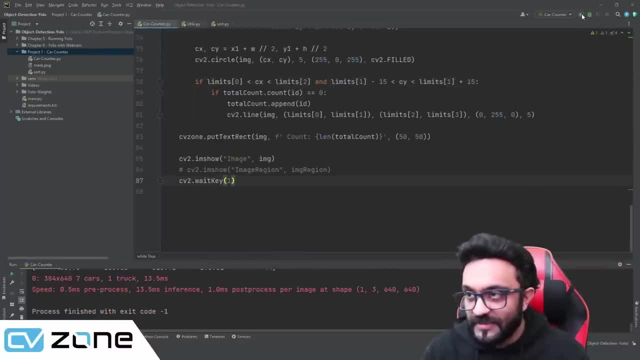 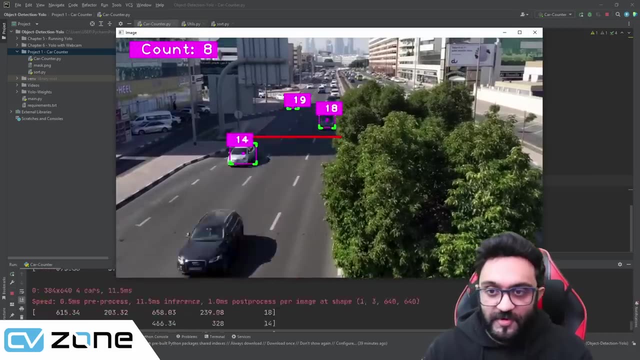 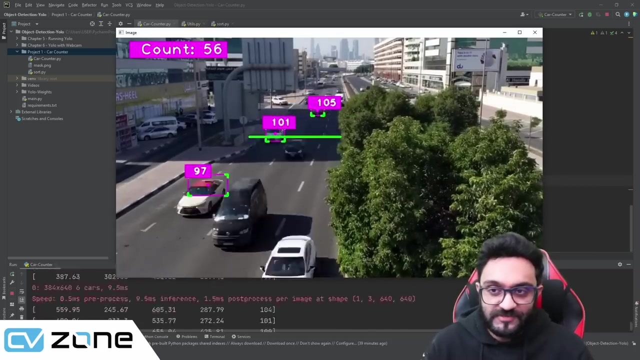 and we can put it as one, and let's see the magic happen. so there you go, it's really fast and it's detecting all those counts and and of course, it's using the gpu. that's why it's so fast. 62, 66, 64, 75, blah, blah, blah, blah. 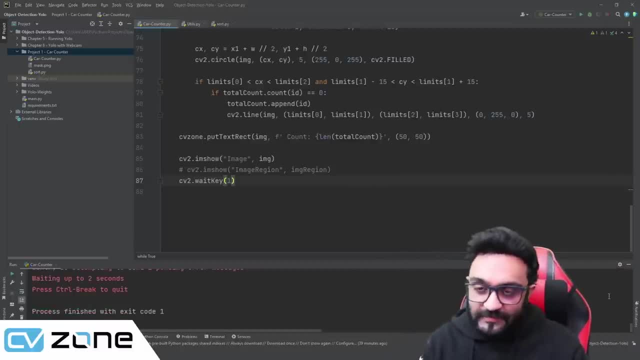 so that's good. so, um, so now everything seems to work fine. but what we can do next is add a little bit of graphics so that it looks a little more appealing. so i have a graphics file here again. you can find it on our website within the zip folder. it's free to download, just go. 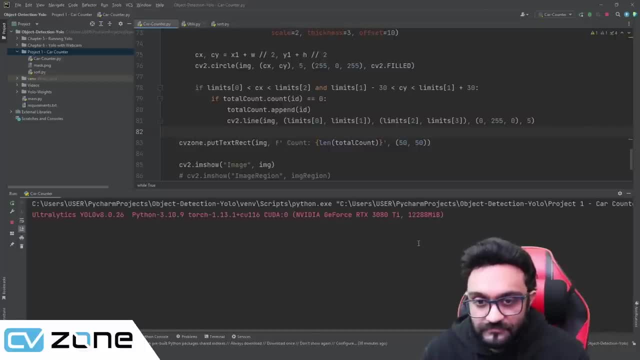 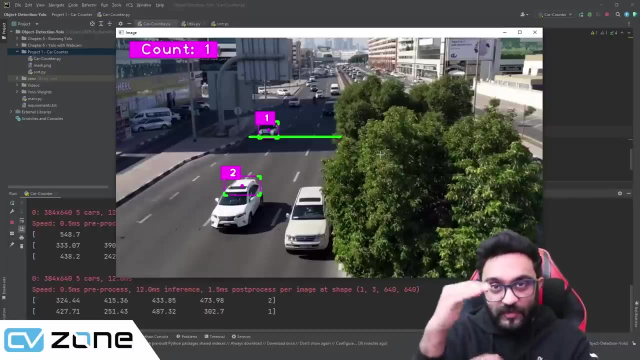 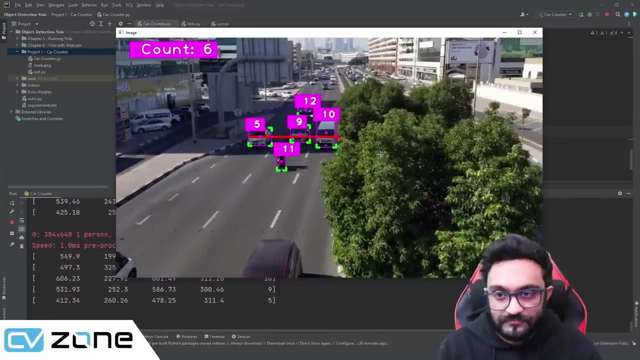 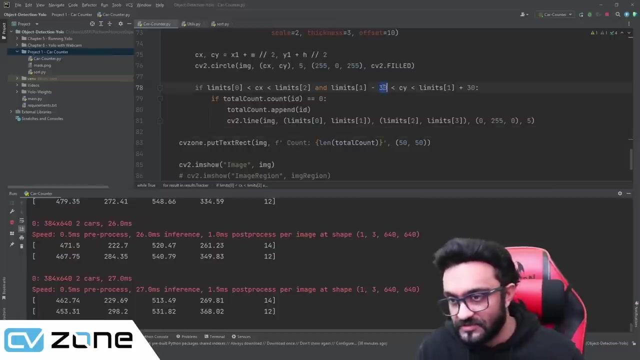 There you go. So if we run this now, at this point, it is detecting as a count because it's within that region, And then it's detecting. Maybe it's too early. Okay, Maybe it's too early. Let's reduce this to 20 back. 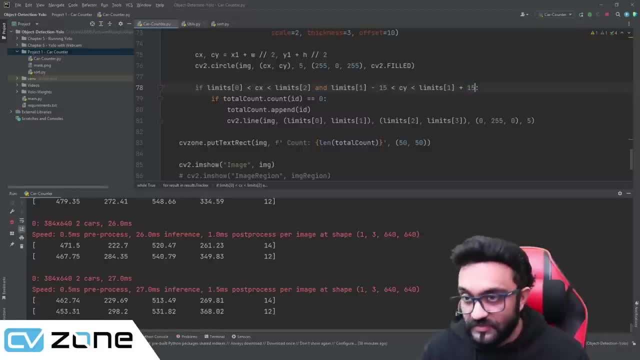 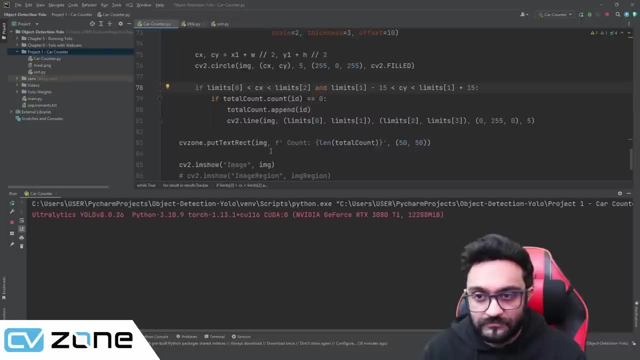 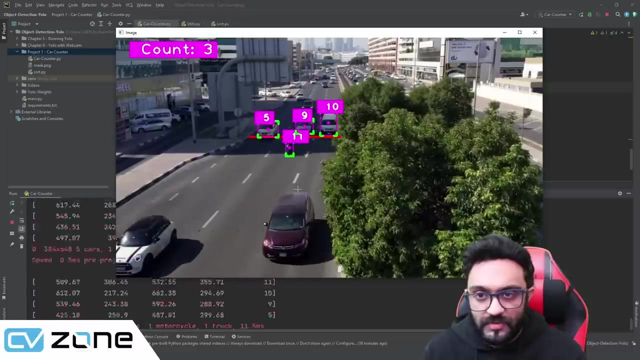 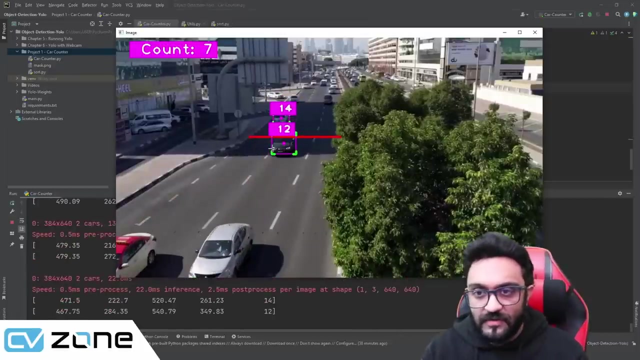 Or let's put it as 15.. And let's put this as 15 as well. Yeah, I think that's better. Two, three, four, five, six, That's correct, Then seven, That's correct, Then we have eight. 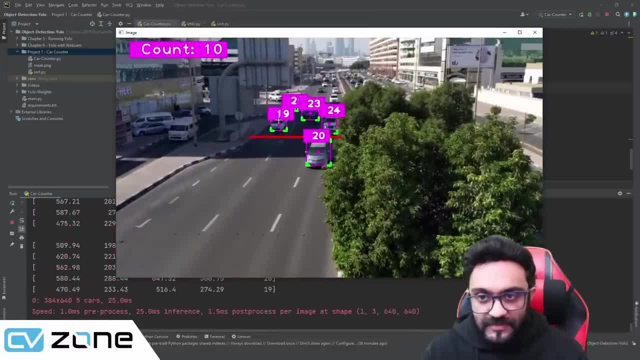 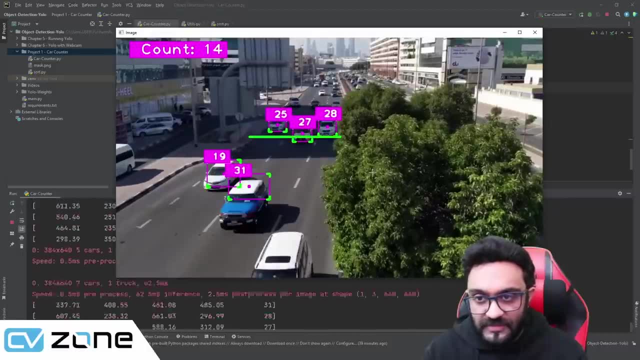 That's correct. Nine, This will be 10.. This will be 11,, 12,, 13,, 14.. So it should be 14 till here, Then 15, 16.. It should be 16 when it crosses these all. 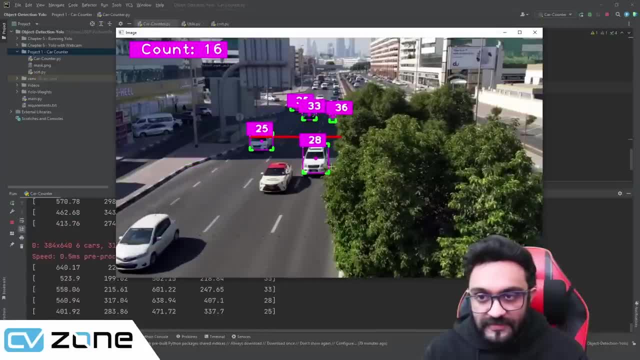 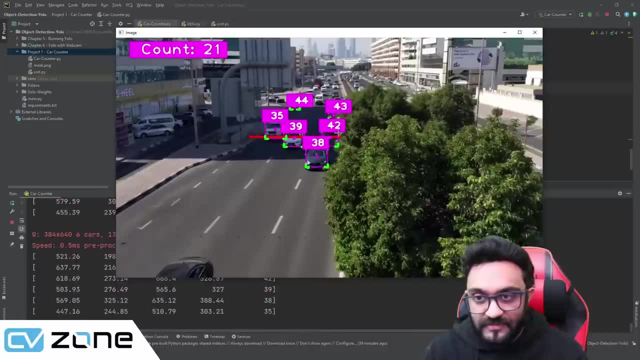 16. That's correct. Then 17, 18, 19.. 17, 18.. That was 19.. Then 20, 21.. It should be 21 after this. This is 22.. Okay, This is getting confusing. 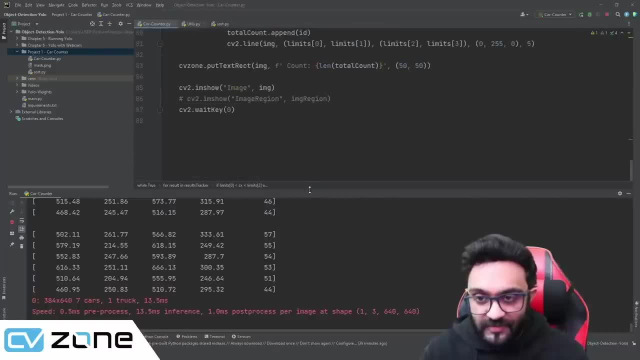 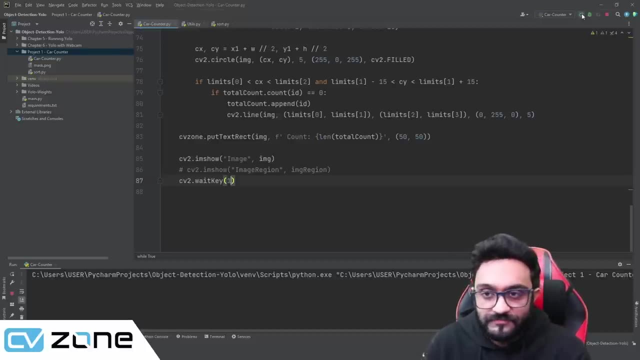 That's why we have the computer to actually find it for us. So what we can do now is we can go down And we can put it as one And let's see the magic happen. So there you go. It's really fast. 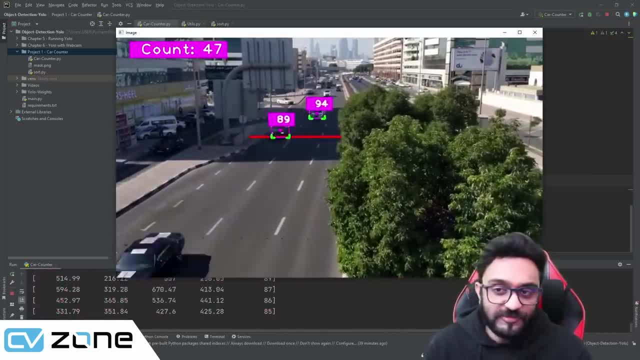 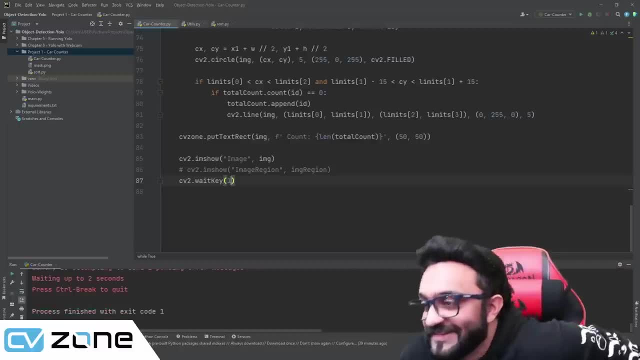 And it's detecting all those counts And, of course, it's using the GPU. That's why it's so fast. 62,, 63,, 64, 75, blah, blah, blah, blah blah. So that's good. 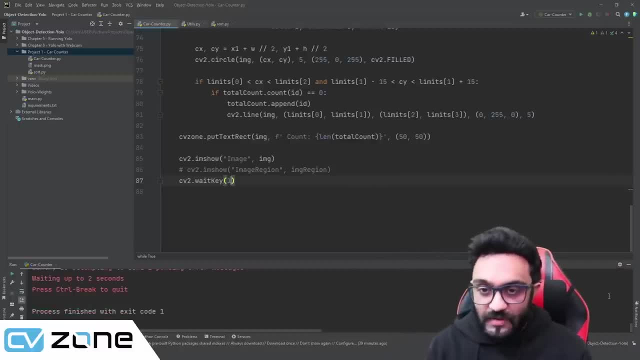 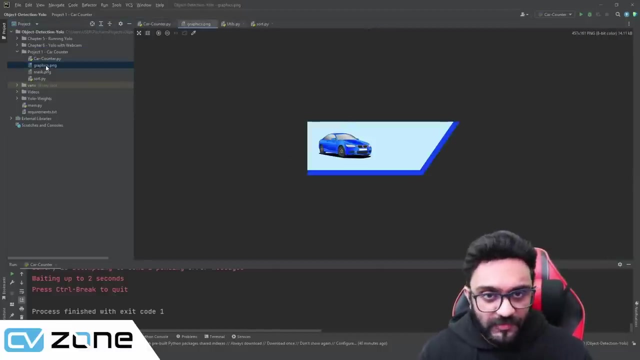 So now everything seems to work fine. But what we can do next is add a little bit of graphics so that it looks a little more appealing. So I have a graphics file here Again. you can find it on our website within the zip folder. 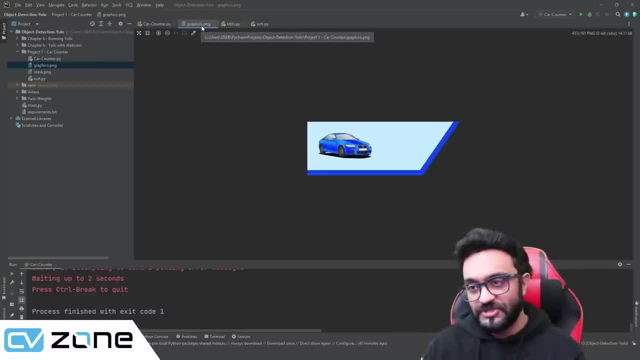 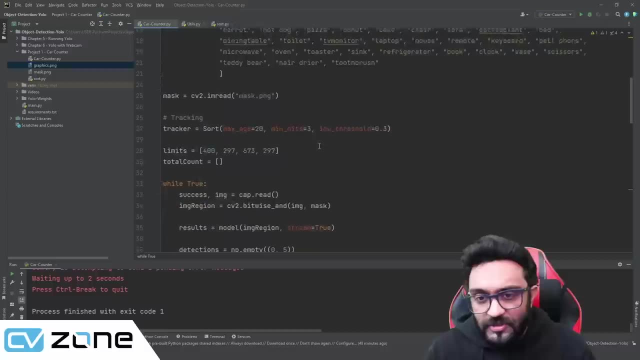 It's free to download. Just go ahead and download. So this is the graphicspng, We are going to overlay it on our main video And then we are going to display the numbers on this. So how can you do that? We are going to read this file. 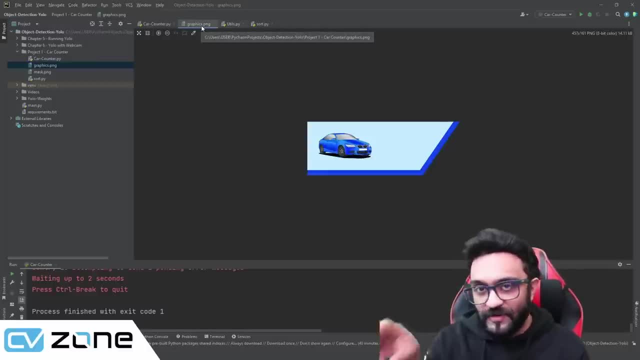 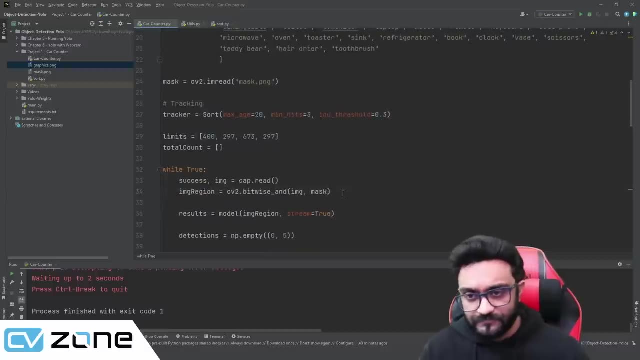 ahead and download. so this is the graphicspng, we are going to overlay it on our main video and then we are going to display the numbers on this. so how can you do that? we are going to read this file. we are going to say: image graphics equals cv2.im. read now the reason we are importing. 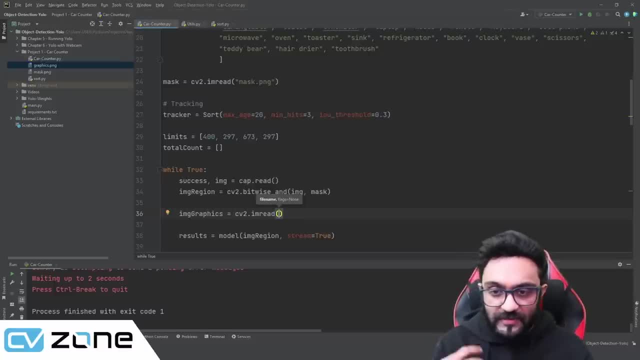 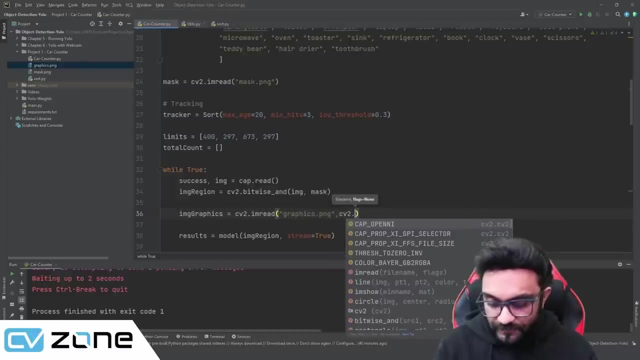 it within the while loop is because if you don't do that, the graphics quality will be really bad over time it will be. it will give very bad results. so you have to import it every single iteration. so graphicspng, and we will write: cv2 dots unchanged. image unchanged. i am read: unchanged. 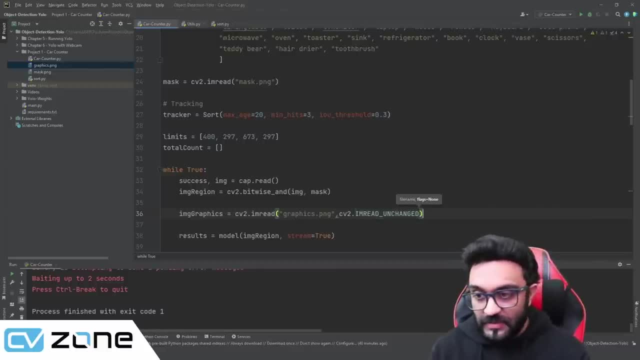 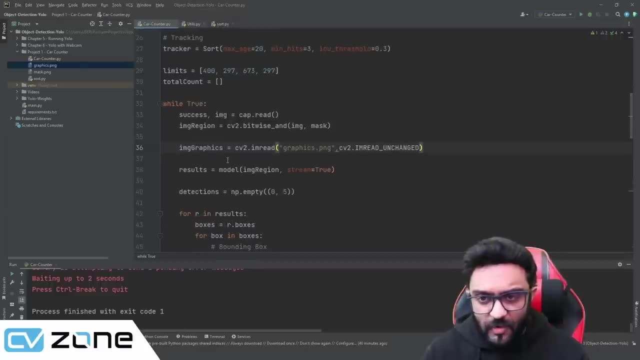 so you have to write that, otherwise it will not work properly because we are going to remove the transparency. so then what we need to do is, at the very end we can overlay the image, or, yeah, we can overlay it over here as well, it doesn't matter. so here we are going to write that: cv zone dot overlay. 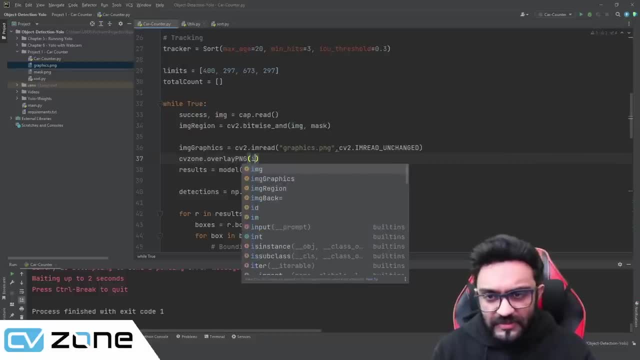 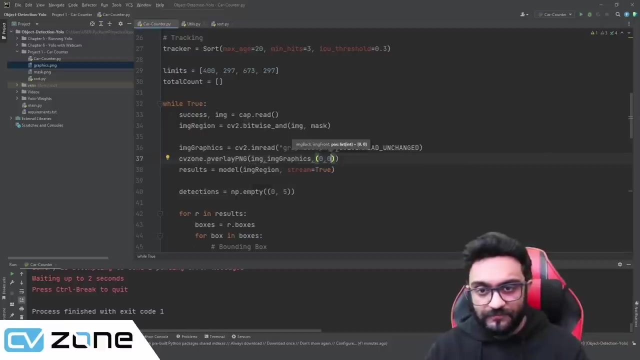 png. so image, uh, the first one is the background, or the. the first one is the background. this word is the background, so this will be image and the second one is our image graphics. it will overlay. and where is the position? the position is 0: 0. it's right at the corner and 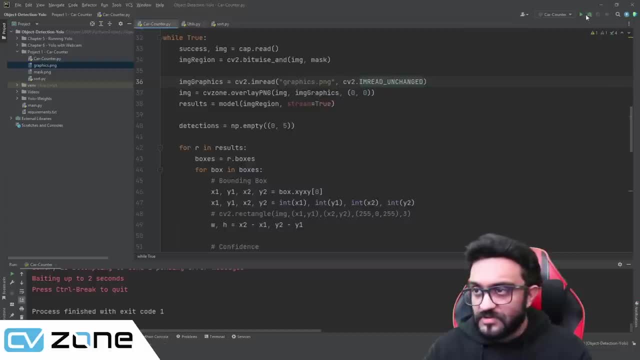 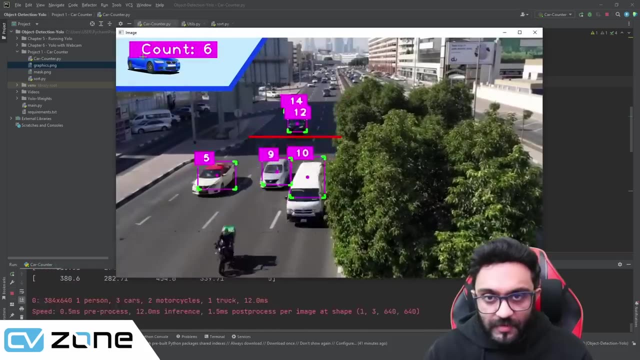 we will put it back to our image in the main file. so let's run that and see if it's in the correct position. if it is, then we will overlay the count on it. there you go. so now the image is there, looks good, and now we will remove this rectangle. 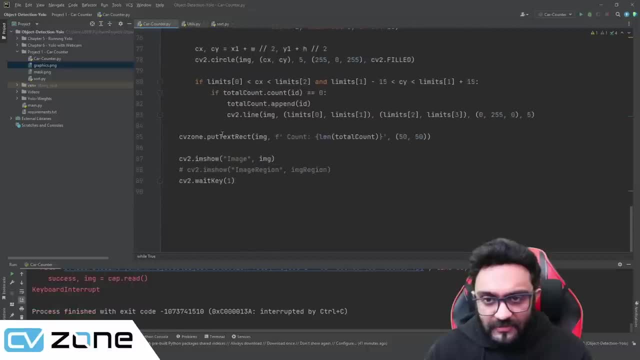 comment and paste in the defined location. now we do that over here so we can see that image will idea angular count and instead of this count we are going to simply write cv2 dot put text and we are going to write the image. the text will be basically string of the length of the total. 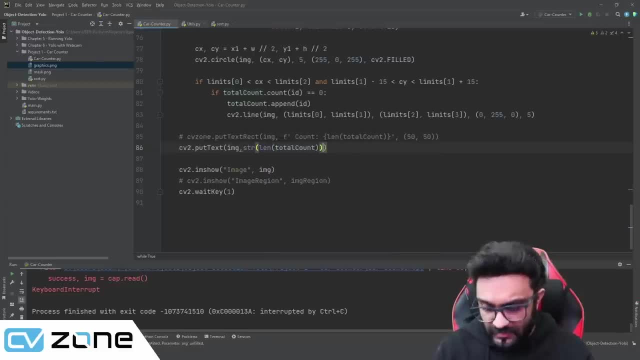 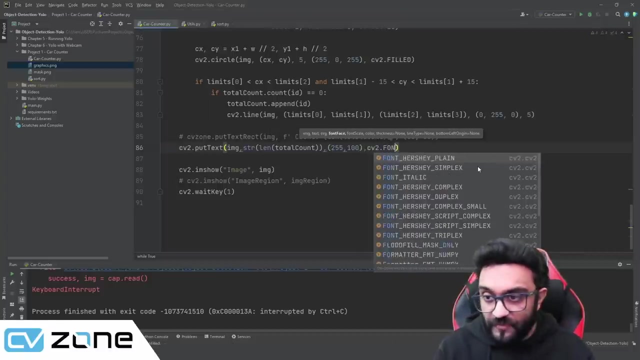 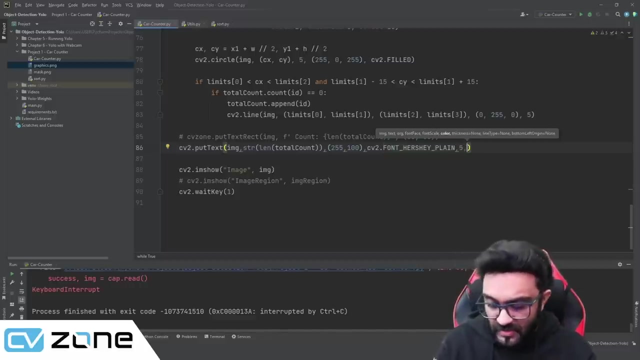 count and then we will have. what do we have next? the origin, uh, the origin, let me check. it should be 255 and 100. then we have cv2, dot font, hershey plane. and then the, the font scale: let's put it as five. uh, the color: let's put it as black, or let's put it as red, 50, let's less red. 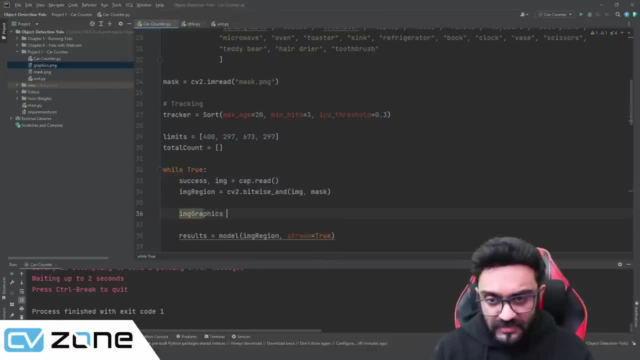 We are going to say image Graphics. Graphics equals cv2.imread. Now, the reason we are importing it within the while loop is because if you don't do that, the graphics quality will be really bad over time. It will give very bad results. 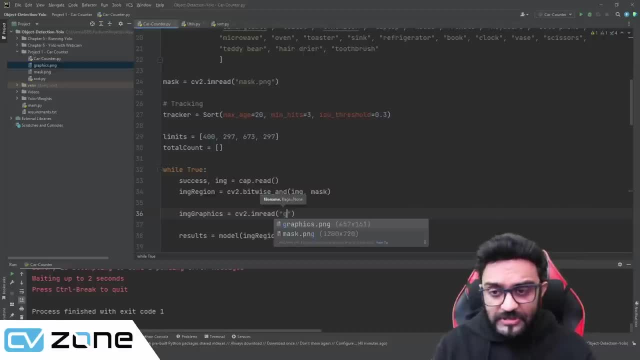 So you have to import it every single iteration. So graphicspng, And we will write cv2.imread unchanged. So you have to write that, Otherwise it will not work properly, Because we are going to remove the transparency. So then what we need to do is, at the very end we can overlay the image. 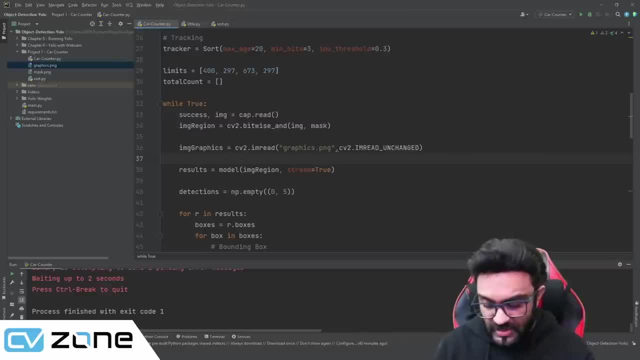 Yeah, we can overlay it over here as well, It doesn't matter. So here we are going to write that cvzoneoverlaypng, So image. The first one is the background, So this will be image And the second one is our image graphics. 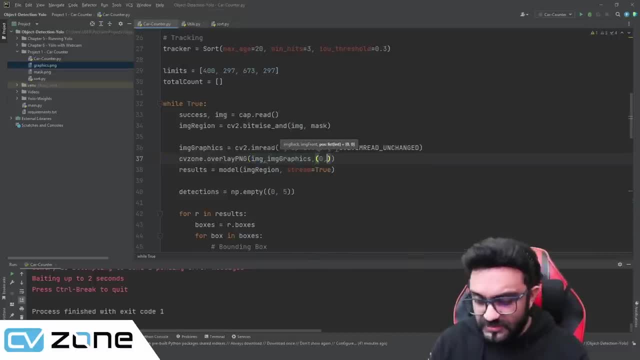 It will overlay. And where is the position? The position is 00.. It's right at the corner And we will put it back to our image in the main file. So let's run that and see if it's in the correct position. 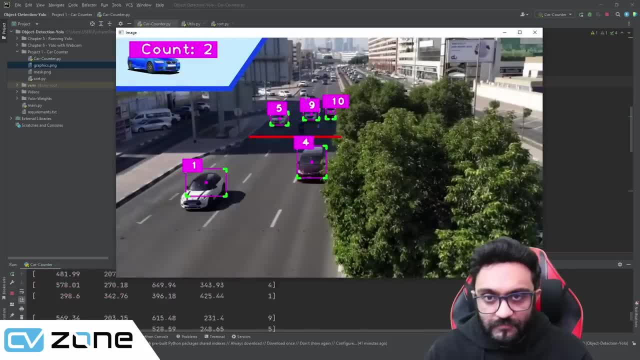 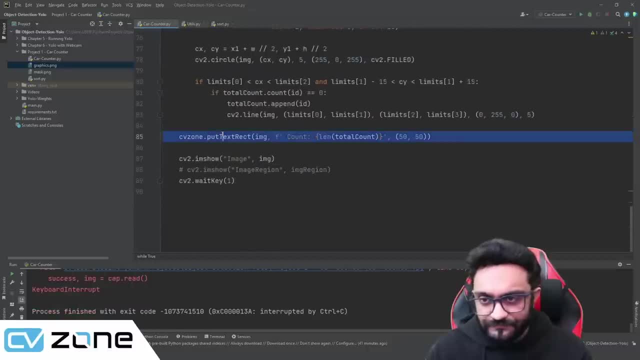 If it is, then we will overlay the count on it. There you go. So now the image is there, Looks good, And now we will remove this rectangular count, And instead of this count, we are going to simply write cv2.puttext. 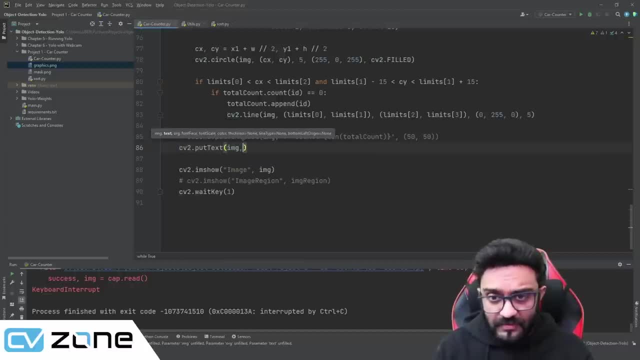 And we are going to write the image. The text will be basically string of the length of the total count And then we will have. what do we have next? The origin. The origin- let me check It should be 255 and 100.. 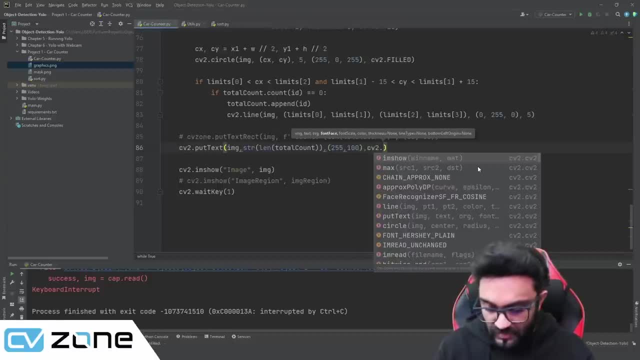 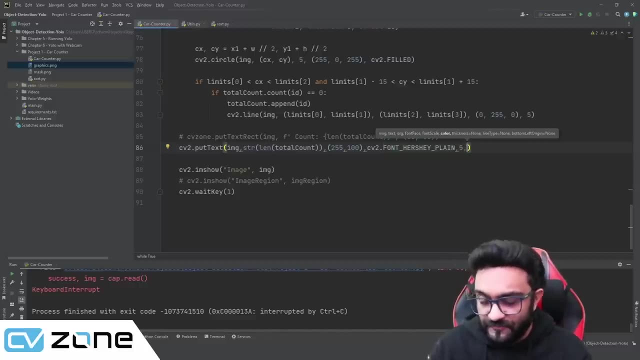 Then we have cv2.font-hershey-plane, And then the font scale: let's put it as 5.. The color: let's put it as black, Or let's put it as red, Less red, 50,, 50,, 255.. 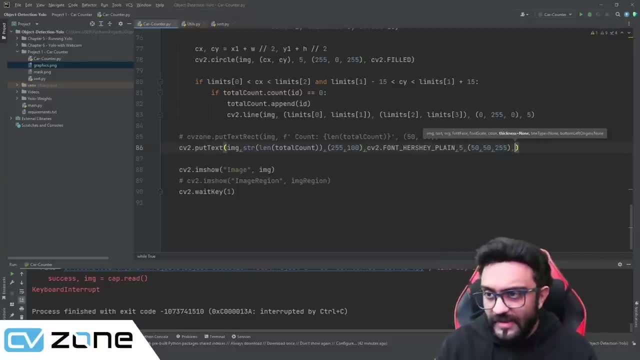 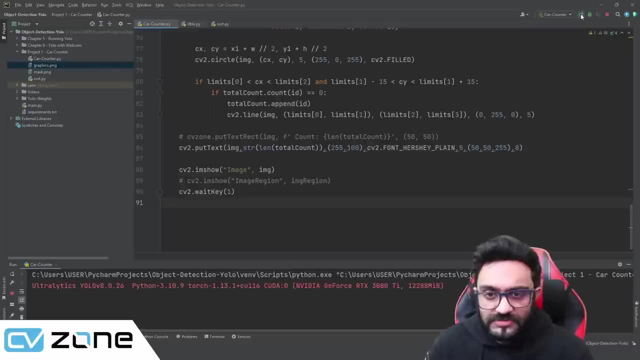 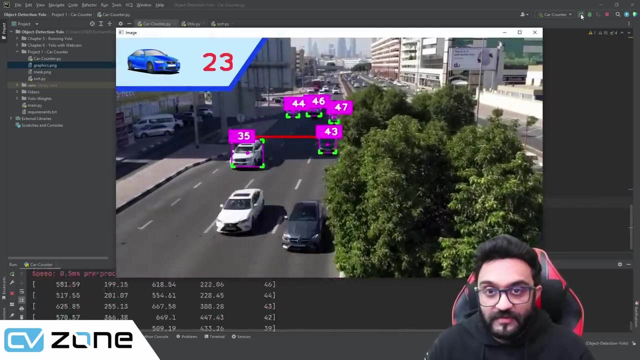 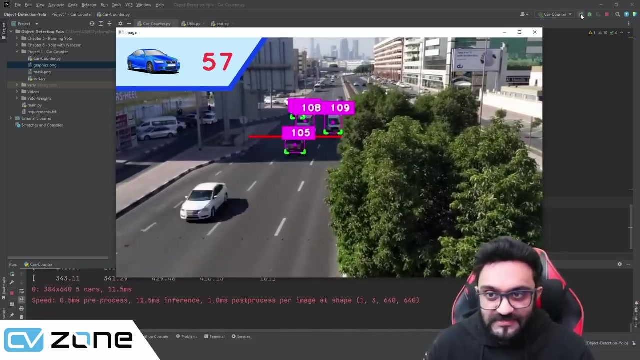 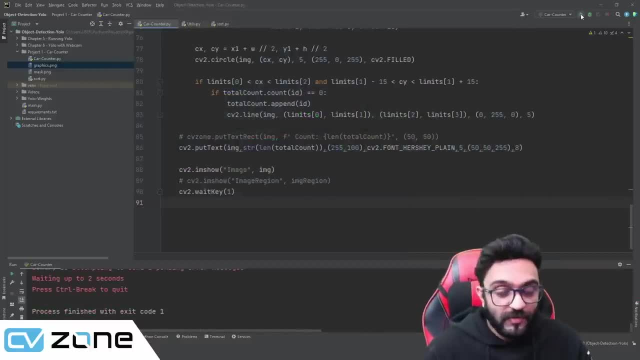 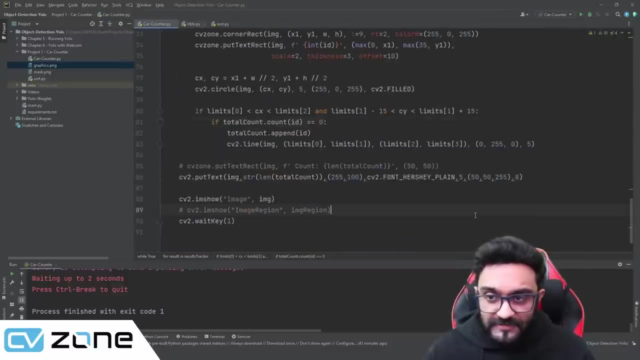 so, finally, the, the robots or the AI is helping us solve problems. so this was our project for. so, finally, the robots or the AI is helping us solve problems. so this was our project for. so, finally, the robots or the AI is helping us solve problems. so this was our project for car counter and it was a really, really simple and, as you can see, it's very fun to do and it is very informative. so i will see you in the next one. 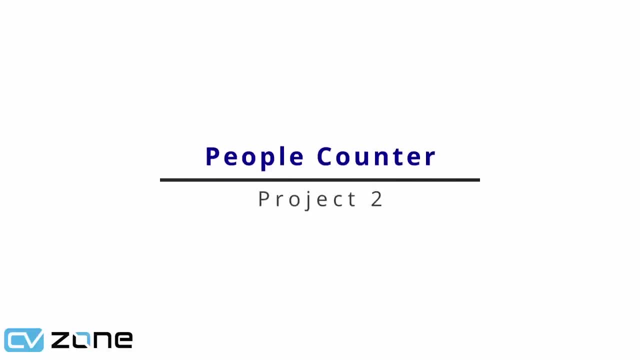 car counter and it was a really, really simple and, as you can see, it's very fun to do and it is very informative. so i will see you in the next one car counter. and it was a really, really simple and, as you can see, it's very fun to do and it is very informative. so i will see you in the next one. 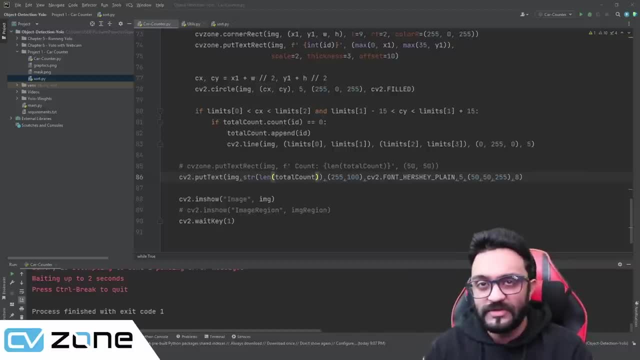 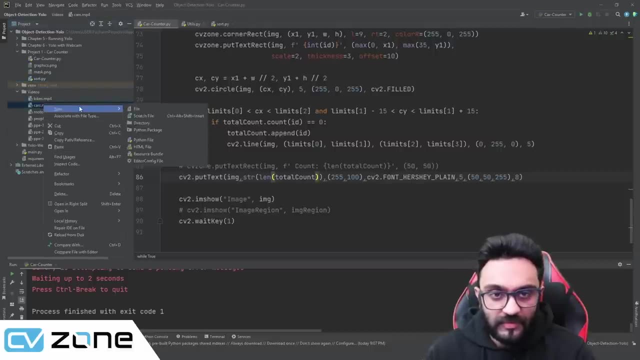 so, now that we have completed our car counter project, we are going to do a similar project to that which will be people counter. so the difference between car counter and people counter will be that we will have multiple directions that we are counting in. so if we go to our video people 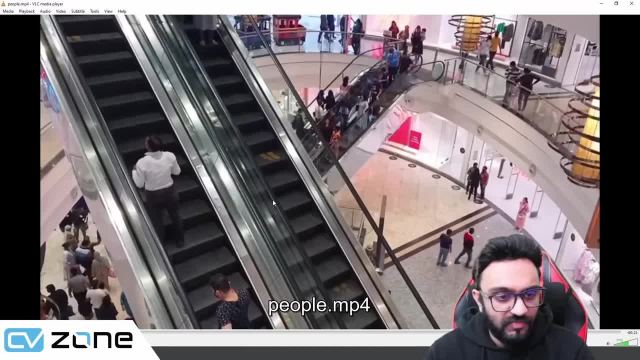 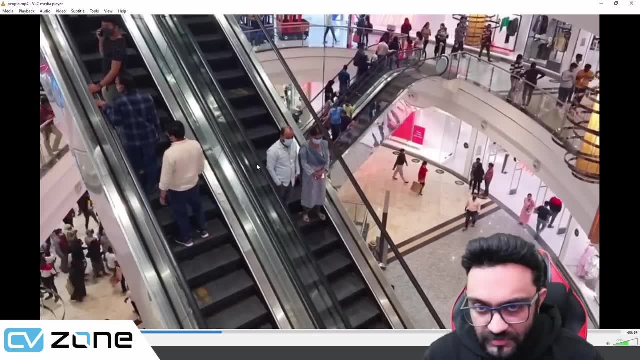 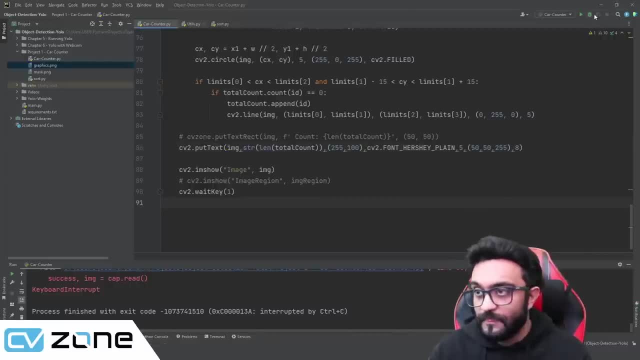 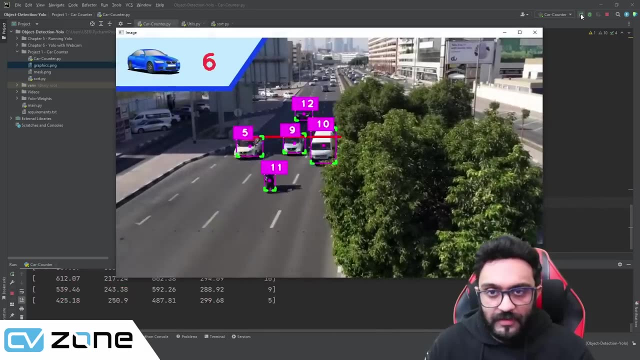 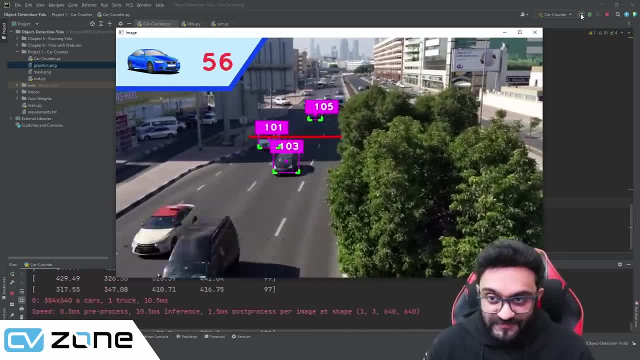 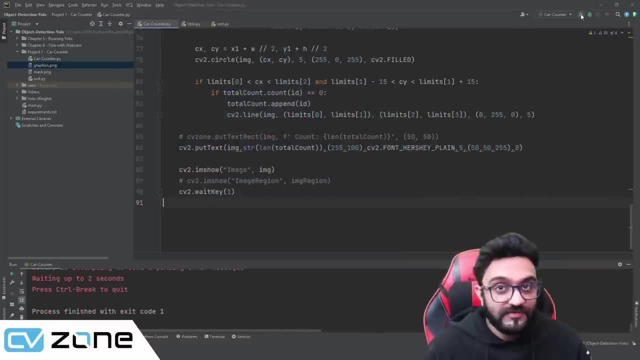 So normally you won't be able to count this fast. So finally, the robots or the AI is helping us solve problems. So this was our project for CarCounter And it was really really simple And, as you can see, it's very fun to do. 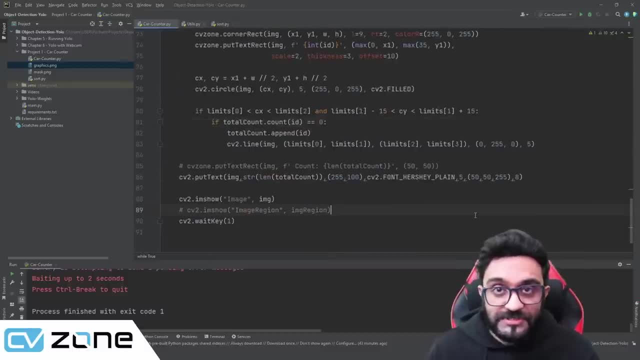 And it is very informative. So I will see you in the next one. So, now that we have completed our CarCounter project, we are going to do a similar project to that which will be PeopleCounter. So the difference between CarCounter and PeopleCounter. 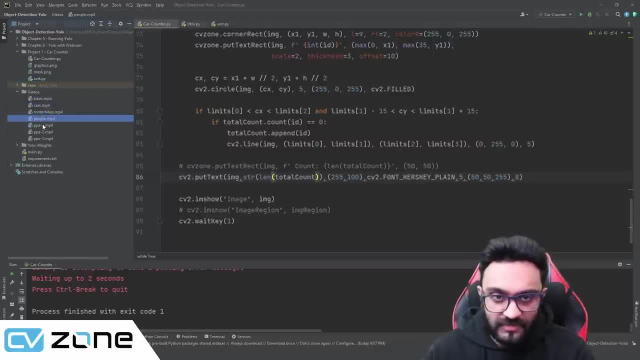 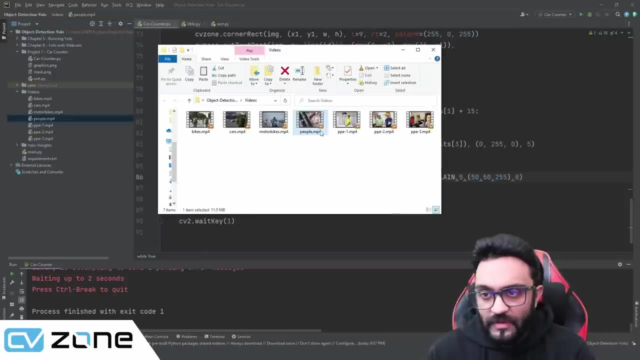 will be that we will have multiple directions that we are counting in. So if we go to our video people, peoplemp4, and we have a look at the mp4, you can see that we have an escalator that has two directions. 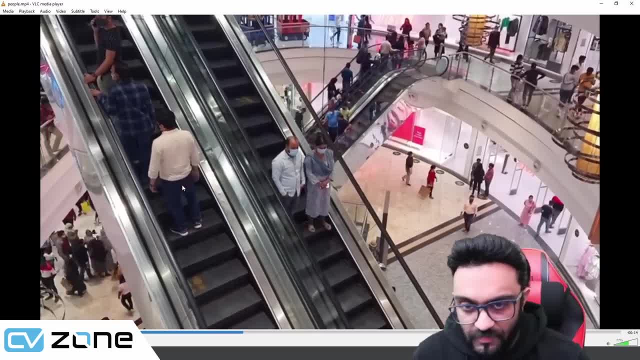 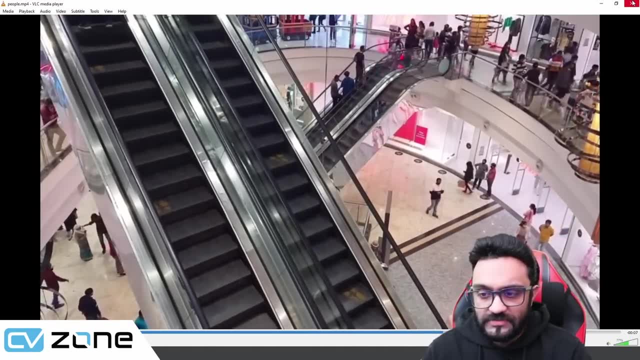 One is going up and the other one is going down. So there are people going down, There are people going up. So we are going to count how many people went up and how many people went down. So that will be the task for this project. 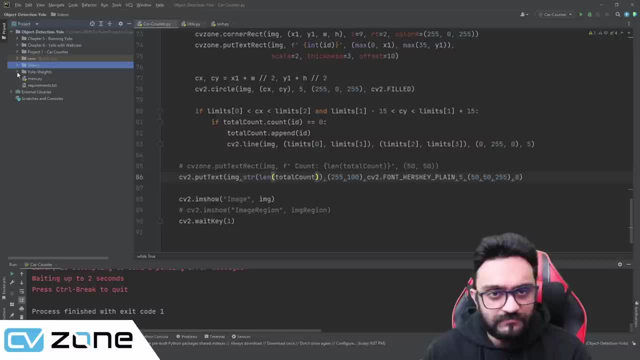 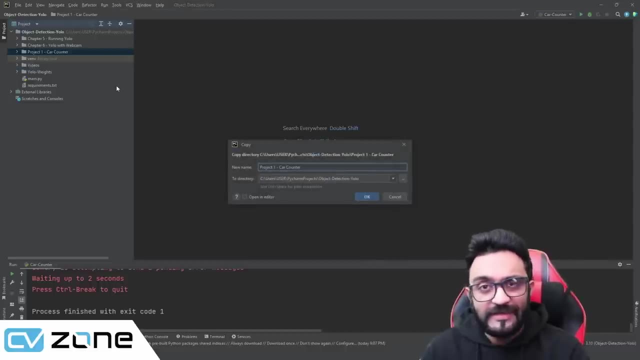 So what we will do is, first of all, we will copy, which is the best thing ever. We will copy and paste our complete project. Now, what this will allow us to do is to use our previous code and we can adjust it to our new video. 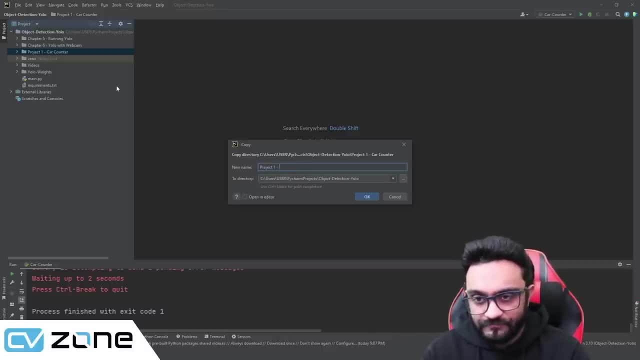 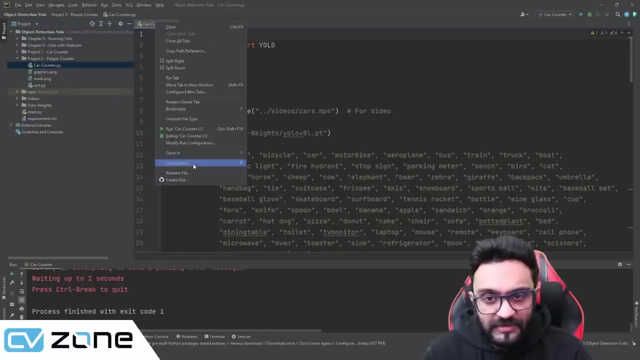 and our new purpose. So we can write here PeopleCounter and this is project number two, So we will hit OK. So project number two: PeopleCounter. first of all, we will open it up and we will rename it. where is the rename? 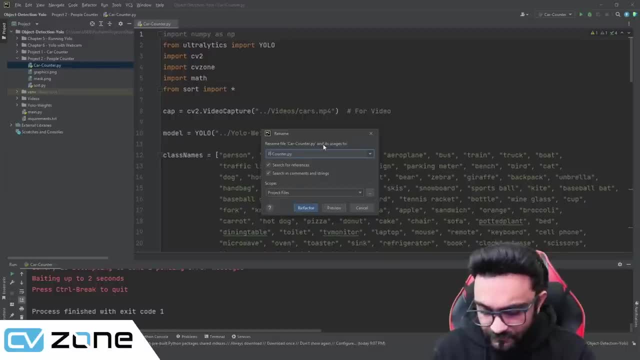 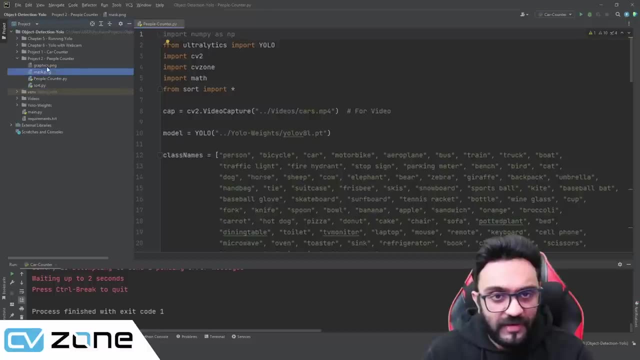 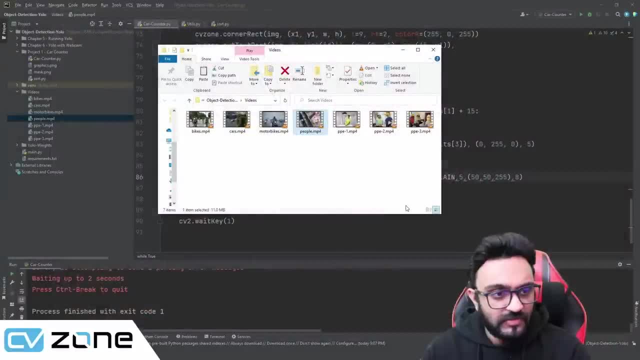 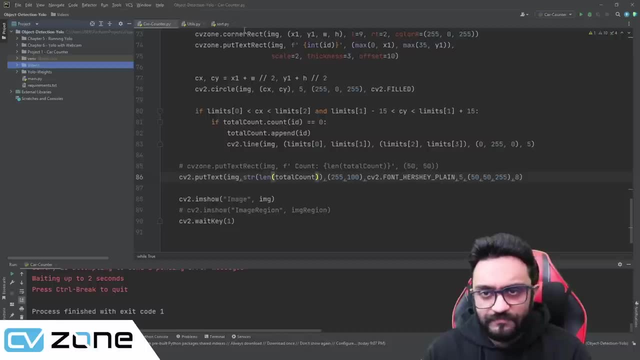 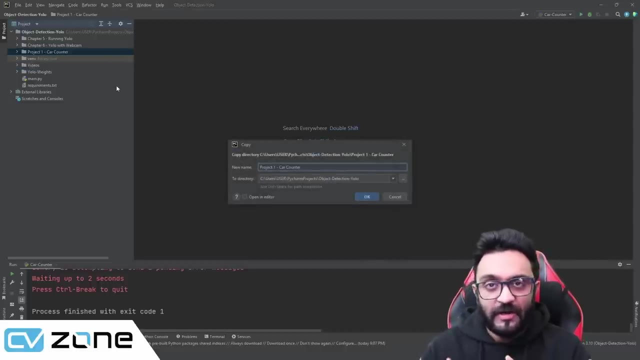 peoplemp4 and we have a look at the mp4, you can see that we have an escalator that has two directions: one is going up and the other one is going down. so there are people. afa, that would be the task for this project. so what we will do is, first of all, we 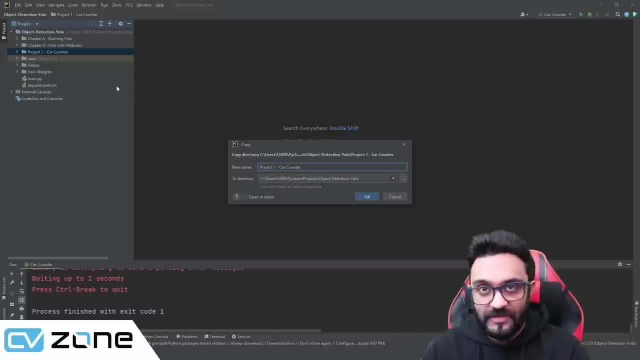 will copy, which is the best thing ever. we'll copy and paste our complete project. now, what this will allow us to is to use our previous code and we can possible thrown on a righteousness, on a söy�� to our Genesis code. it doesn't give you the identity you're looking for. come on. 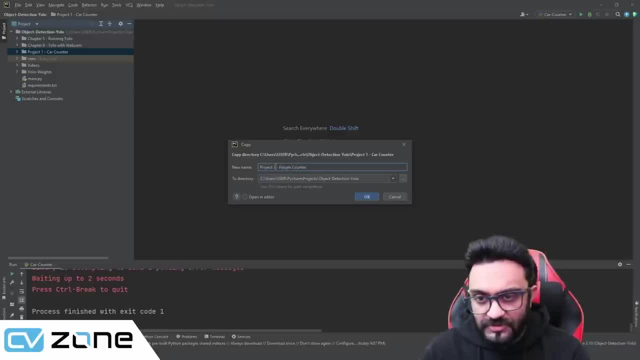 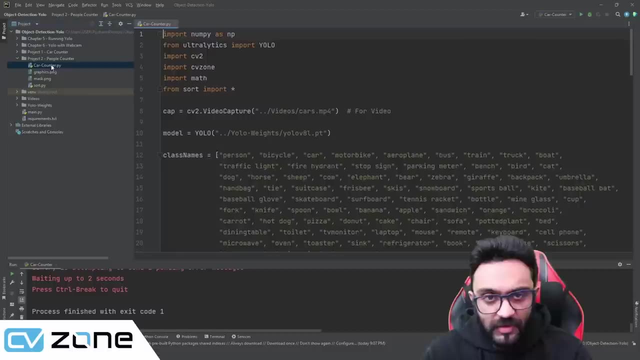 people counter and this is project number two, so we will hit: okay. so project number two: people counter. first of all, we will open it up and we will rename it. uh, where is the rename? here is the rename. so we will write: here: people counter, there you go. so we'll write: people counter here. 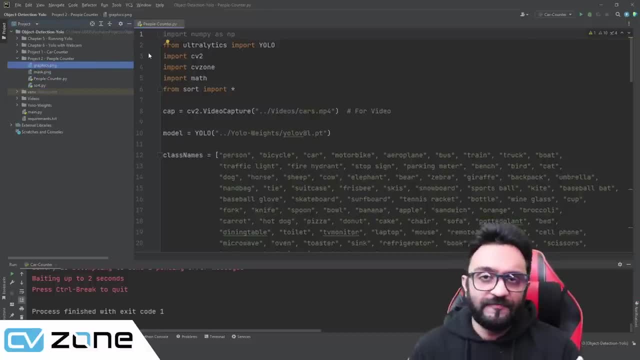 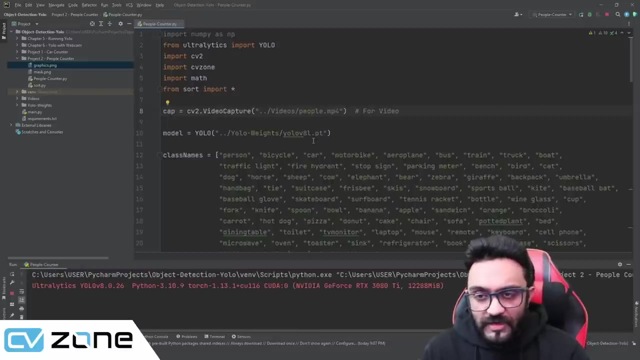 we have sort mask and graphics. now the mask and graphics are going to change, but for now, just to make sure everything works fine. uh, first of all, we are going to change the video. we will write here people, and then we are going to run it to see what happens. so, as you can see, we are still. 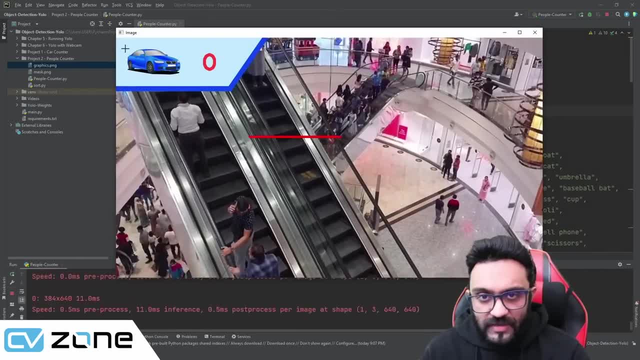 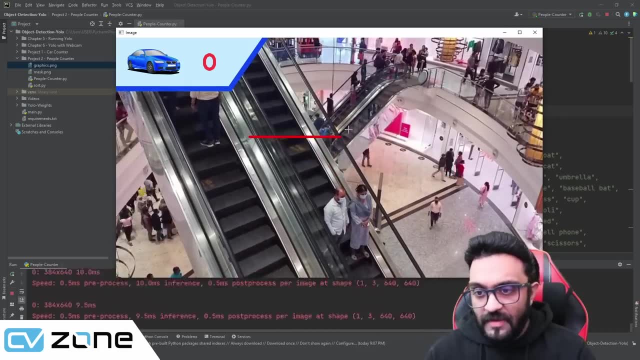 using the large version. so there you go. so we have the graphics over here, which is for the car, and we have a line here which is basically counting. but, as you can see, it is not going to be a lot of work. it's not counting anything because it's not detecting anything, because, if you remember, we 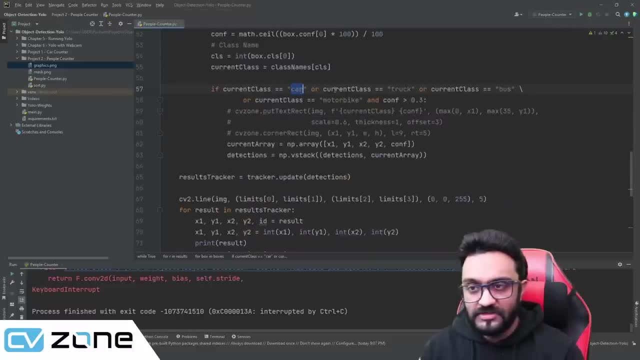 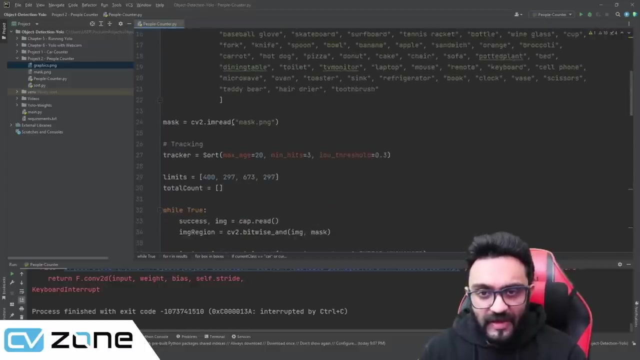 asked it to only detect, uh, cars, bikes, trucks and, um, motorbikes, so that that are, those are the four classes that we want to detect. so that is not being detected here. that's the first thing. the second thing is that we have the mask which is being overlaid in the wrong place. we need to. 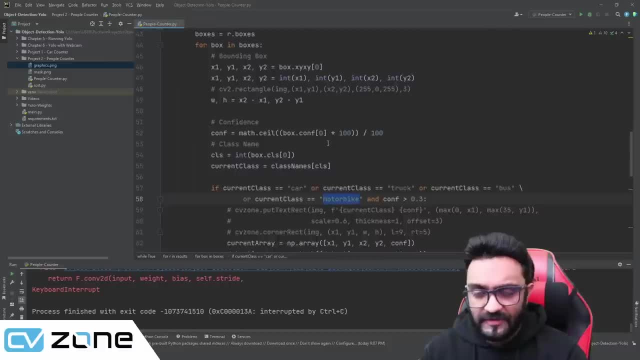 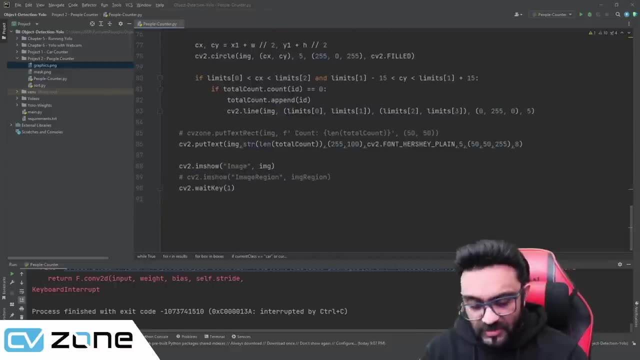 remove that too. and then we also have the counter, or the graphics, which which is wrong as well. so first of all, let's bring in the graphics again. you will find the graphics, um, in the zip file when you download it from our website, so i've created this earlier and this is how it looks. so this is the graphics. 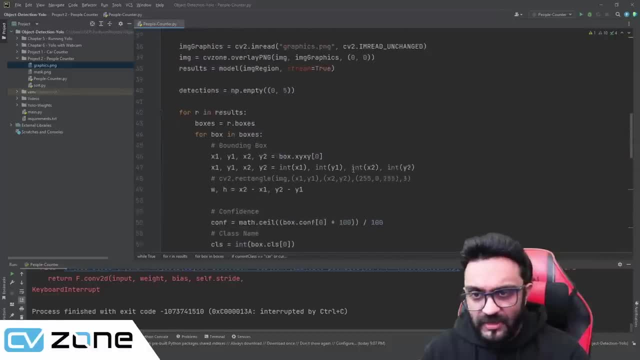 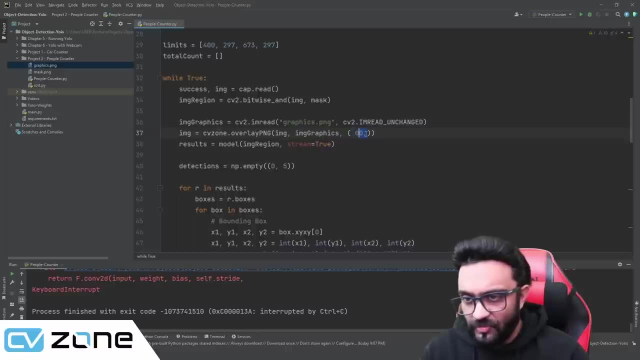 so what we can do is we can simply replace this graphics right away, so that we have one less thing to worry about. so here in the graphics, we have graphics right here. so we have graphics right here, which is our png, and we will not put it at zero zero. what we will do instead is: let me check the. 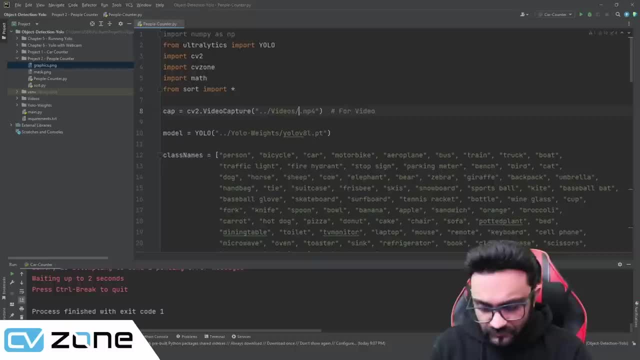 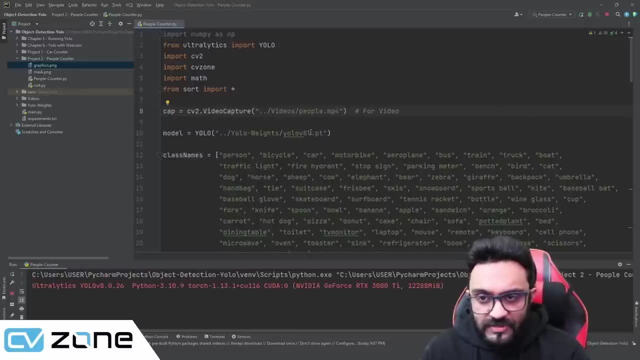 first of all, we are going to change the video. We will write here, People, and then we are going to run it to see what happens. So, as you can see, we are still using the large version. So there you go. So we have the graphics over here. 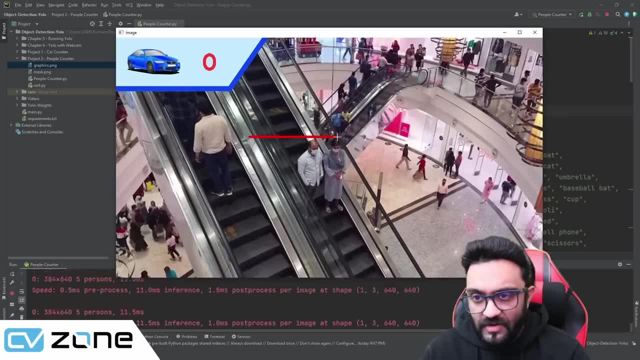 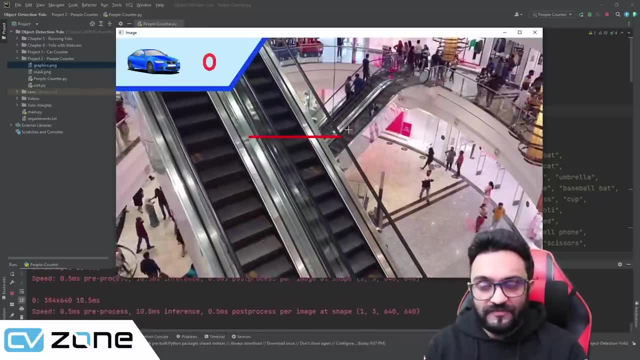 which is for the car, And we have a line here which is basically counting, But, as you can see, it is not counting anything. because it's not detecting anything? Because, if you remember, we asked it to only detect cars, bikes. 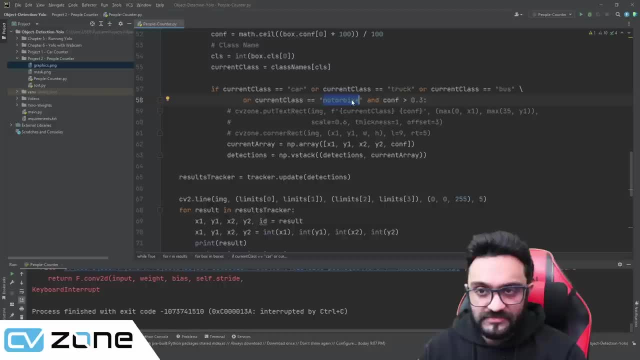 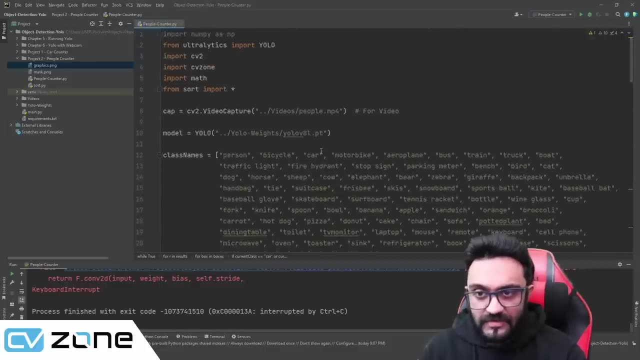 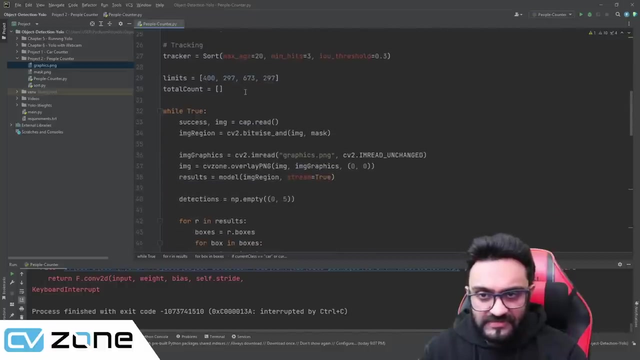 trucks and motorbikes. So those are the four classes that we want to detect. So that is not being detected here. That's the first thing. The second thing is that we have the mask, which is being overlaid in the wrong place. 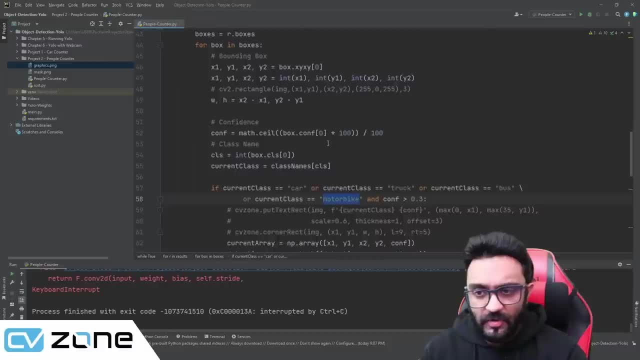 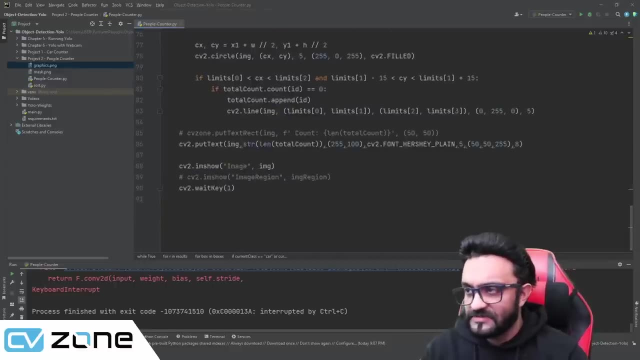 We need to remove that too. And then we also have the counter or the graphics, which is wrong as well. So first of all, let's bring in the graphics Again. you will find the graphics in the zip file when you download it from our website. 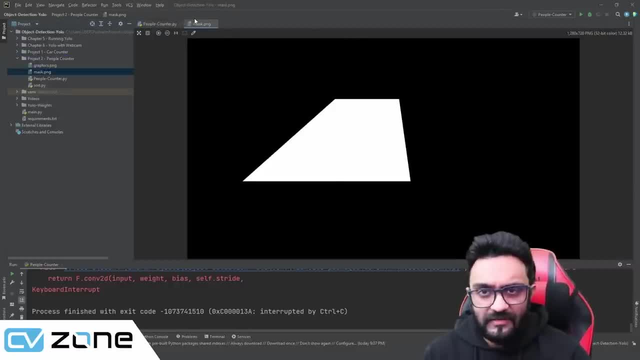 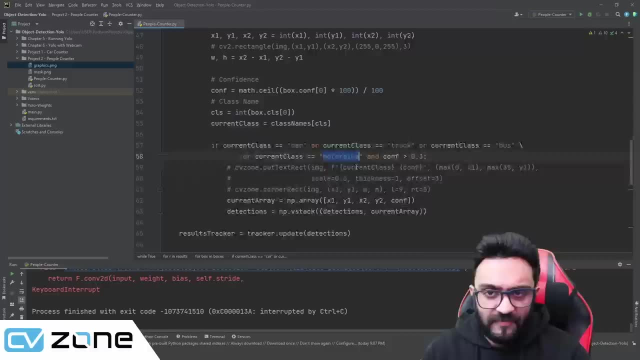 So I've created this earlier And this is how it looks. So this is the graphics. So what we can do is we can simply replace these graphics right away, so that we have one less thing to worry about. So here in the graphics: 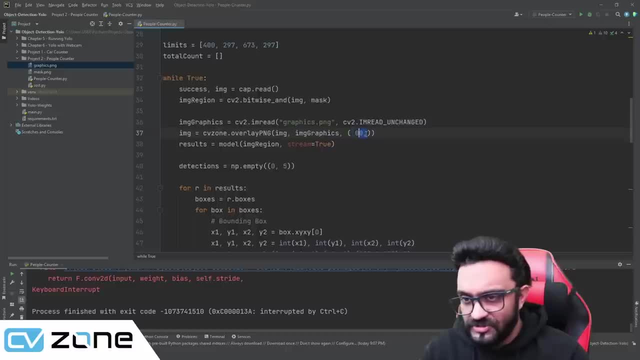 we have graphicspng and we will not put it at 00.. What we will do instead is let me check the exact values: It's 730,, 730 and 260.. So this is the exact position where it should be So, if we run this now, 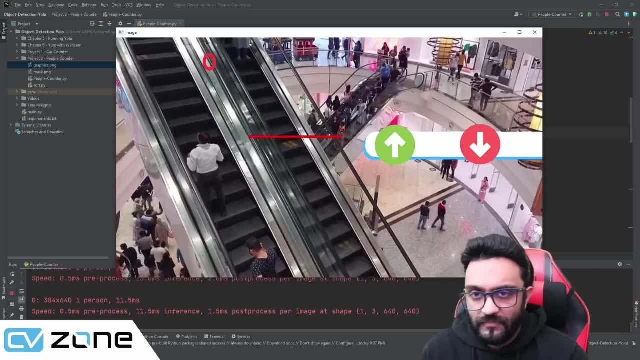 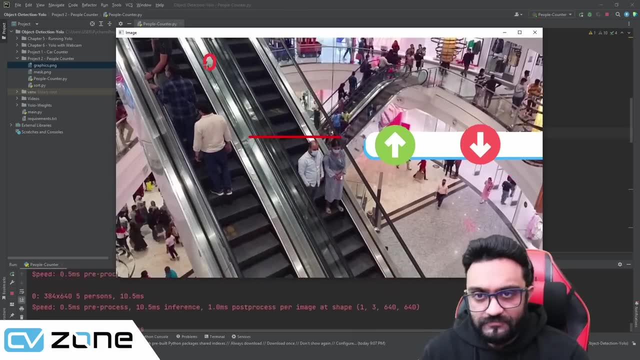 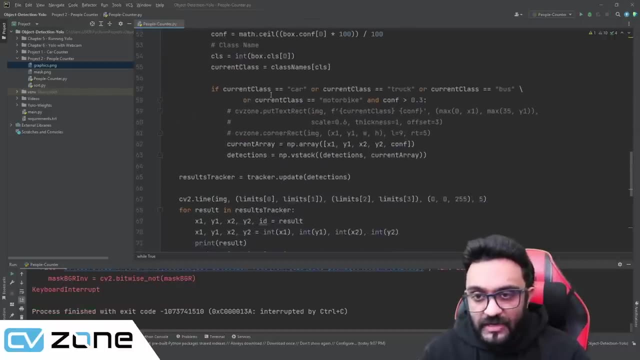 we will have the graphics being shifted. There you go, So we have the graphics over here. So that is the first thing done towards our people counter project. Then the second thing that we can do is we can open up the detections for people. 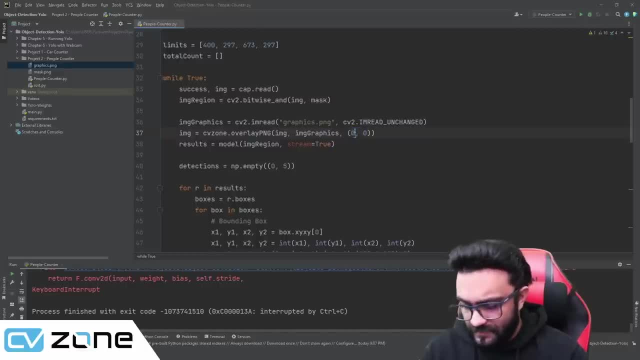 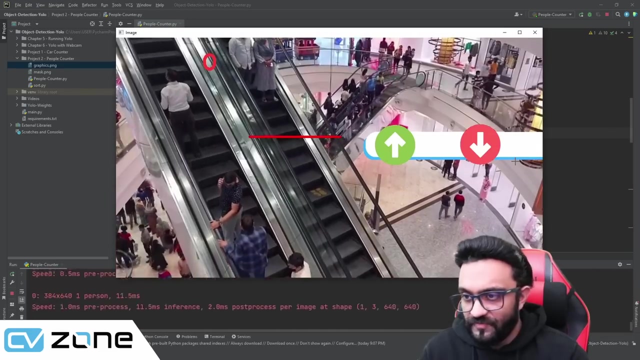 exact values. it's 730, 730 and 260, so this is the exact position where it should be. so if we run this now, we will have the graphics being shifted. there you go. so we have the graphics over here. so that is the first thing done towards our people. counter project. 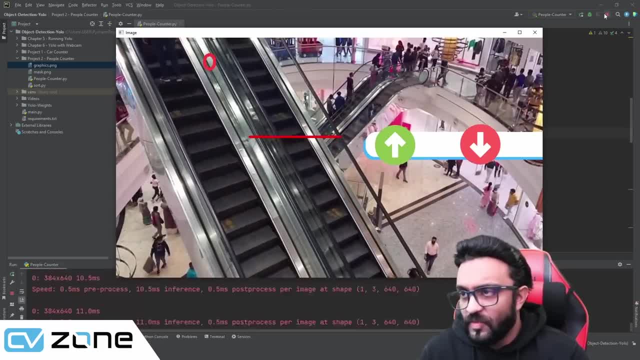 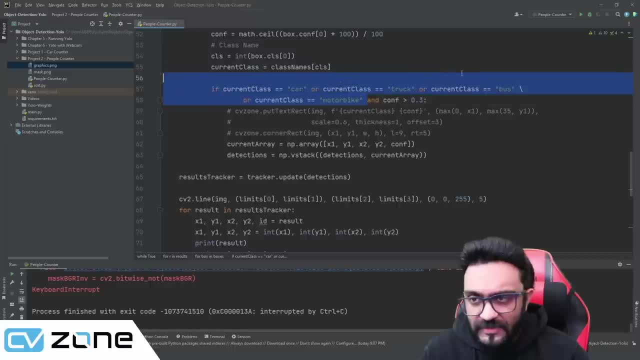 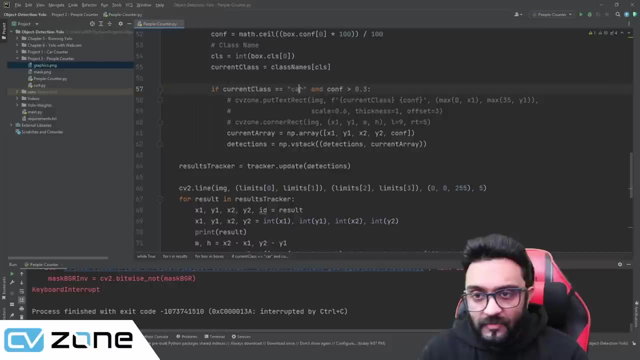 the second thing, uh, that we can do is we can open up the detections for people. so here we have car and here we have the confidence. so the confidence will keep the same. the rest we will delete and we will write here: person, if the current class is person and the confidence is greater than 0.3. 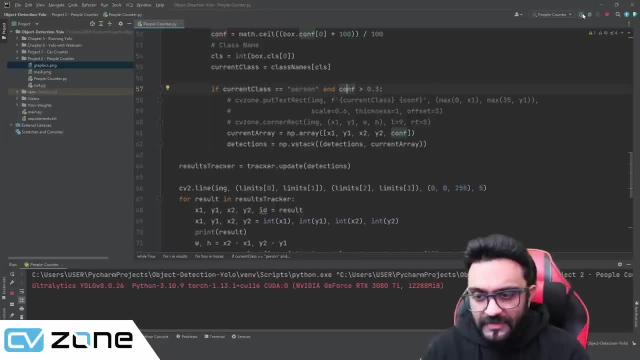 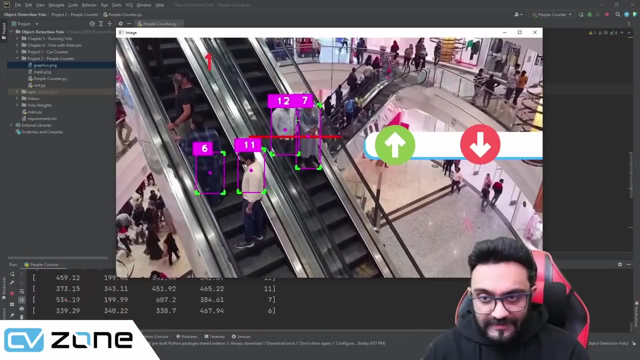 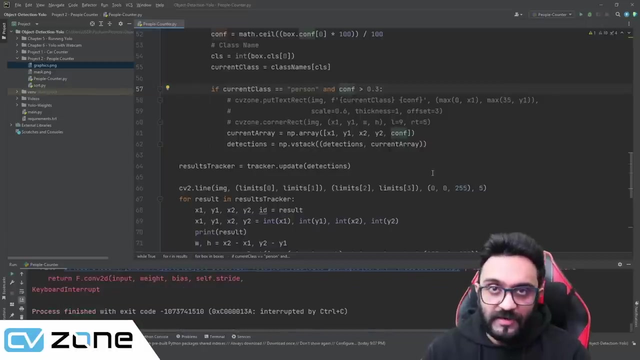 so now it should give us the detections, but we will have the issue of the mask because, as you can see, the mask is around here, so it's only detecting in this region. so the mask is completely wrong. so what we need to do, we need to go ahead and create our new mask. 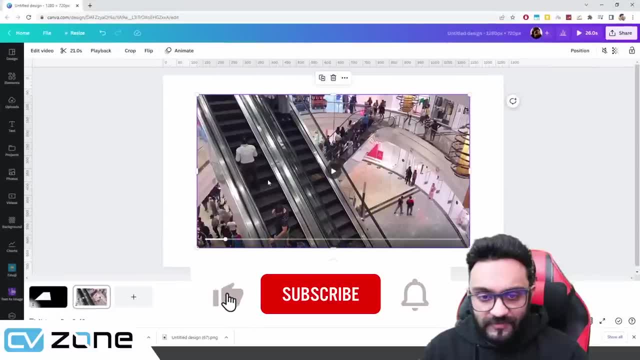 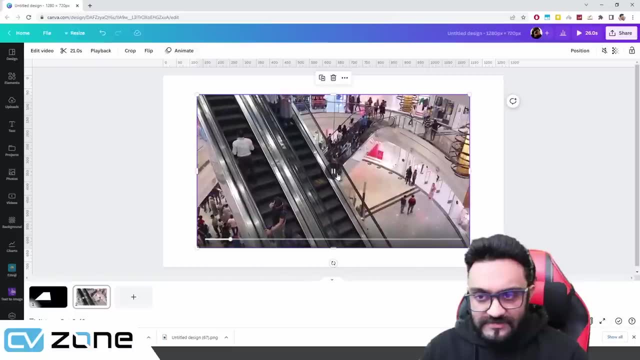 so let's go ahead and do that. so we are back here in canva and, as you can see, it's the same file. we had this mask earlier, and now we are going to create a new mask, and this is the same video that we saw earlier and, first of all, we are going to fill it up. 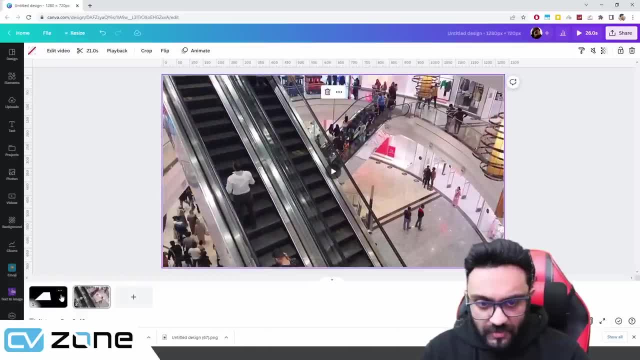 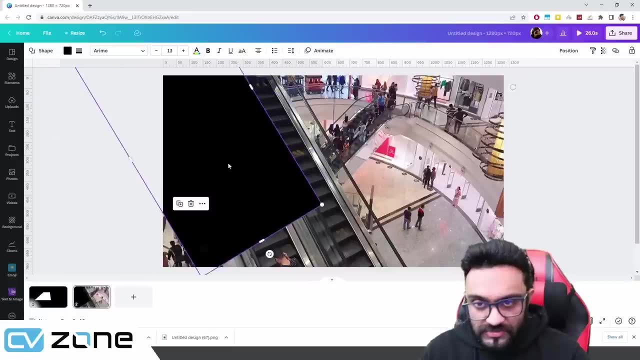 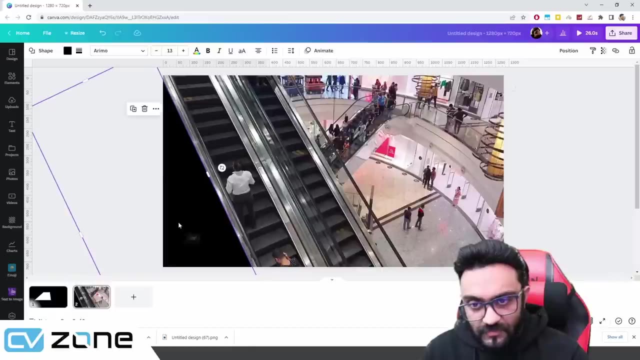 in the space, and now we are going to start creating our mask. we can go back and simply copy one of the rectangles so that it will be easy for us to work with. so here we will rotate it like that, maybe a little bit lower. there you go. i think that's good. we will copy that. 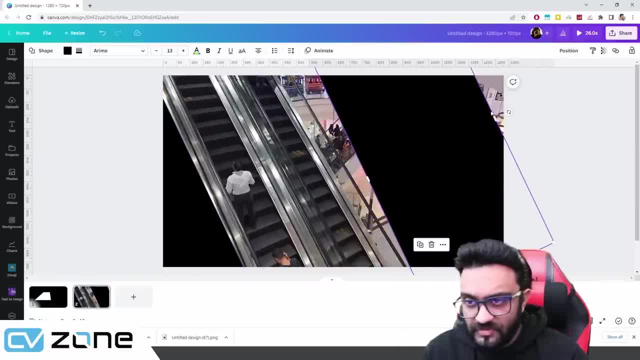 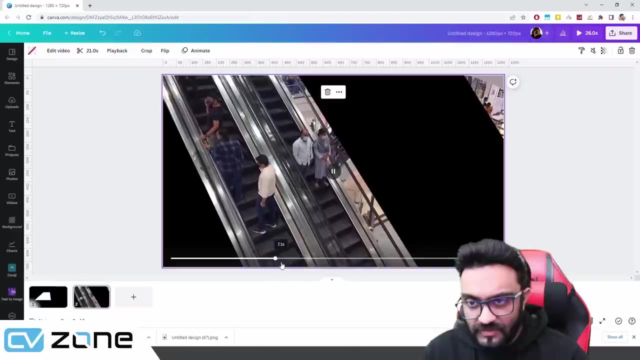 and we will paste it here. okay, it's not straight, it's not aligned with the, with the escalator, so maybe around like that. so let's play the video so that we can see till what points do we get the people coming in out. there you go. so i think, yeah, maybe a little. 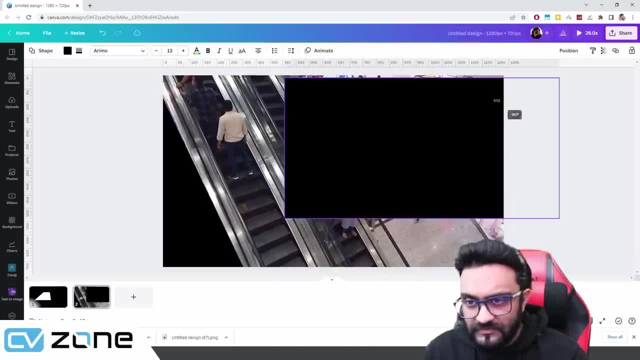 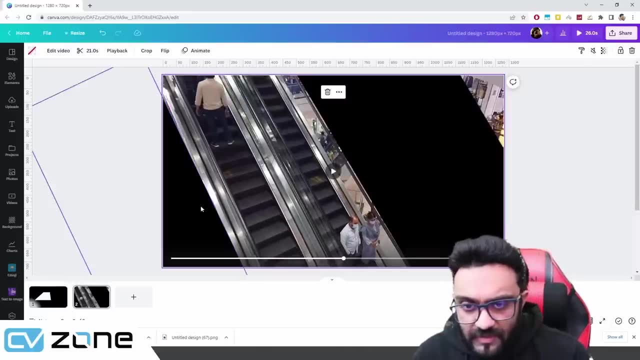 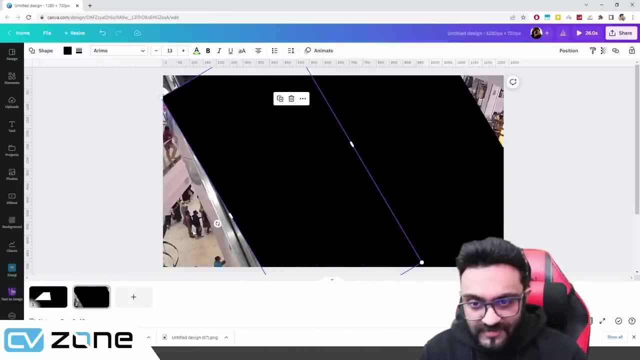 bit lower and maybe a little bit tilted. why does it start in the wrong position? there you go. so, yeah, i think that should be fine and we can remove this, because this is correctly aligned and we can now rotate it here so that we can see how it looks. so we're going to rotate this mask. 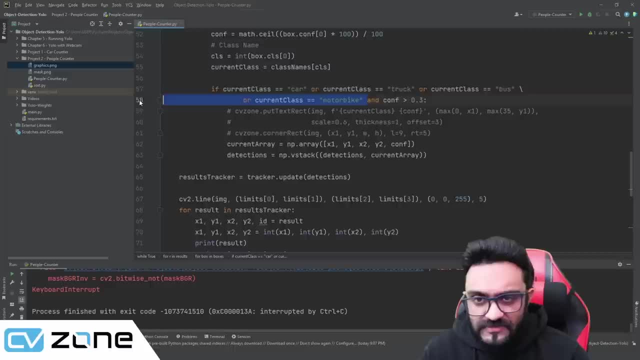 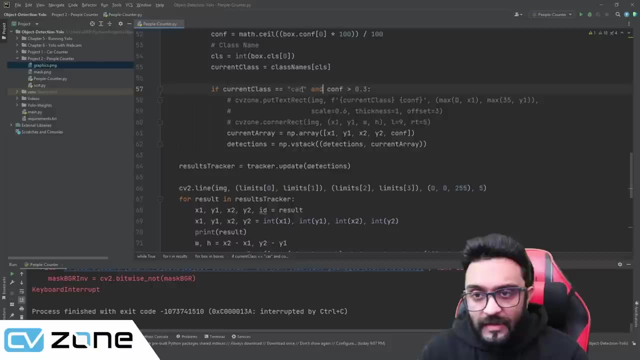 So here we have car and here we have the confidence. So the confidence will keep the same. The rest we will delete And we will write here: person, If the current class is person and the confidence is greater than 0.3.. So now it should give us the detections. 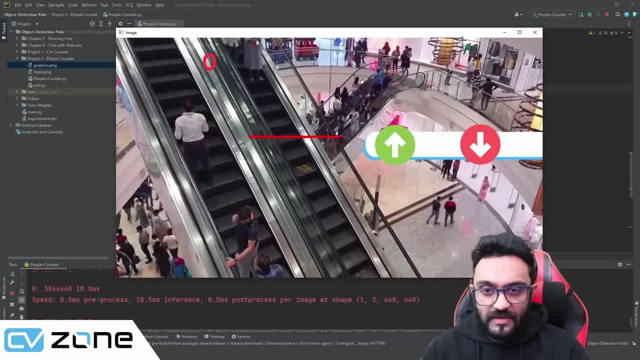 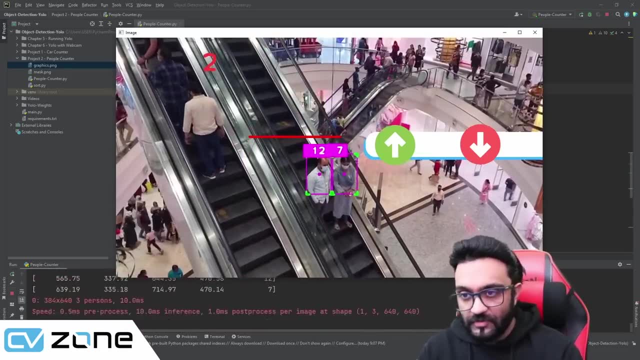 But we will have the issue of the mask because, as you can see, the mask is around here, So it's only detecting in this region. So the mask is completely wrong. So what we need to do, we need to go ahead and create our new mask. 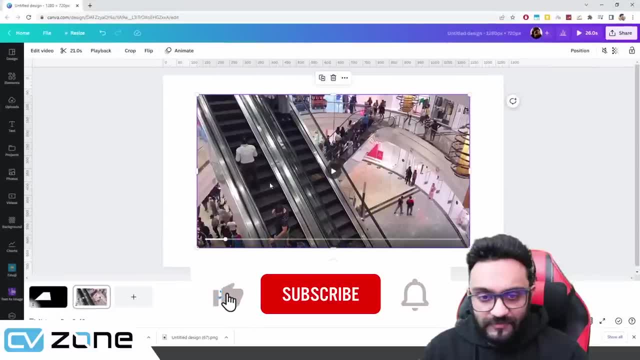 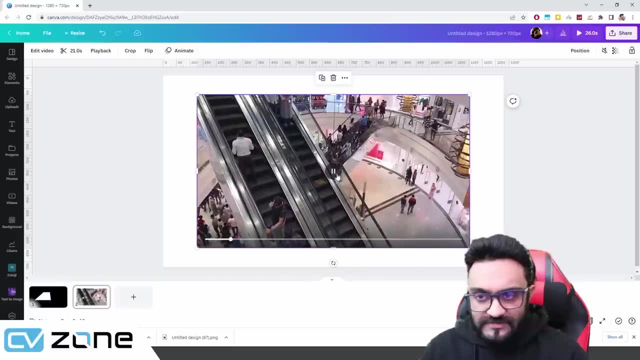 So let's go ahead and do that. So we are back here in Canva And, as you can see, it's the same file. We had this mask earlier, And now we are going to create a new mask, And this is the same video. 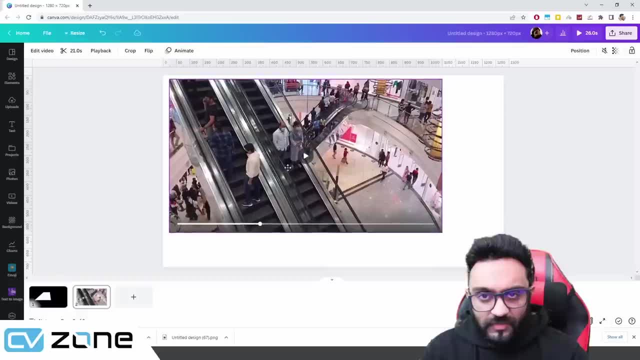 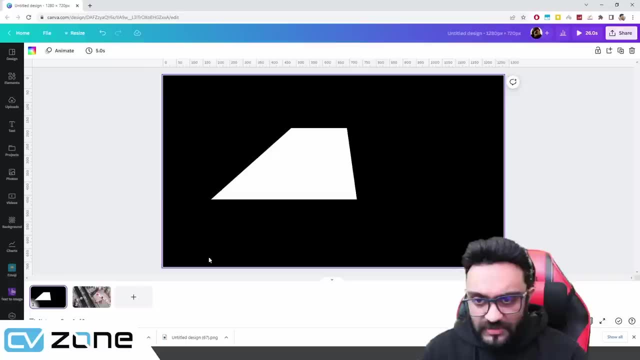 that we saw earlier, And first of all, we are going to fill it up in the space, And now we are going to start creating our mask. We can go back and simply copy one of the rectangles so that it will be easy for us to work with. 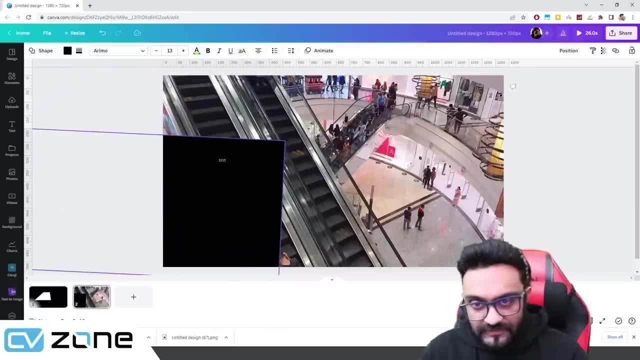 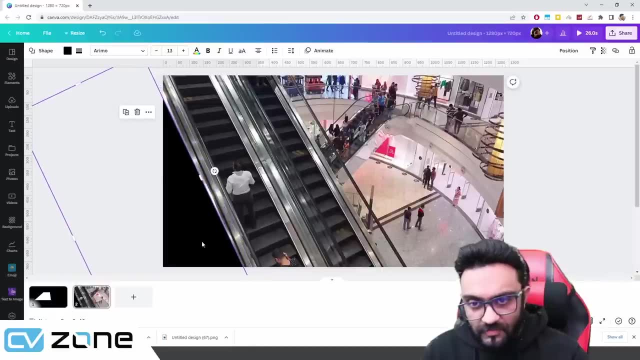 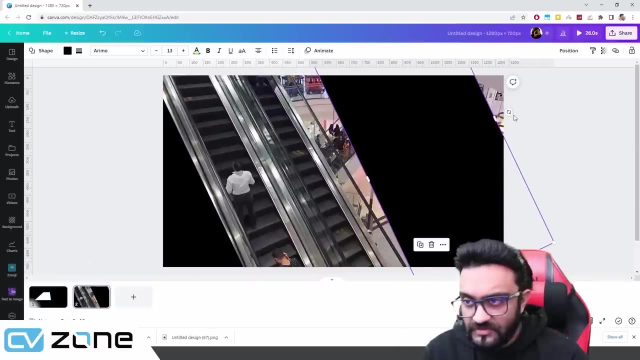 So here we will rotate it Like that, Maybe a little bit lower. There you go, I think that's good. We will copy that and we will paste it here. Okay, it's not straight, It's not aligned with the escalator. 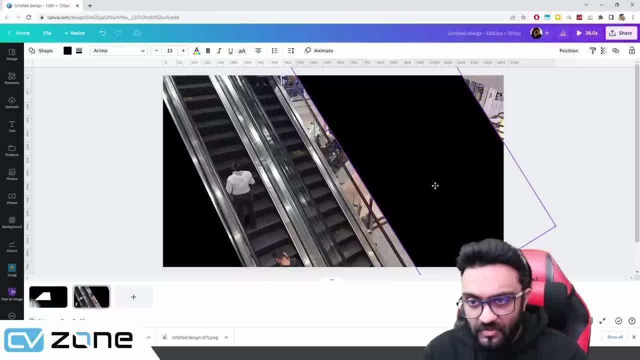 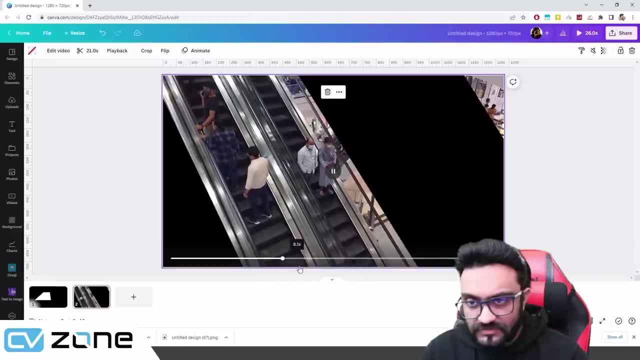 So maybe around like that. So let's play the video so that we can see till what point do we get the people coming in and out. There you go. So I think, yeah, maybe a little bit lower And maybe a little bit tilted. 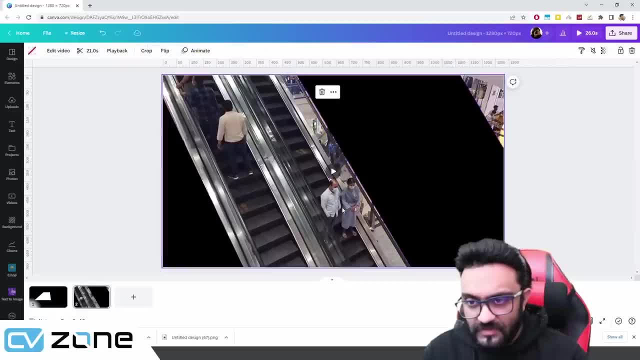 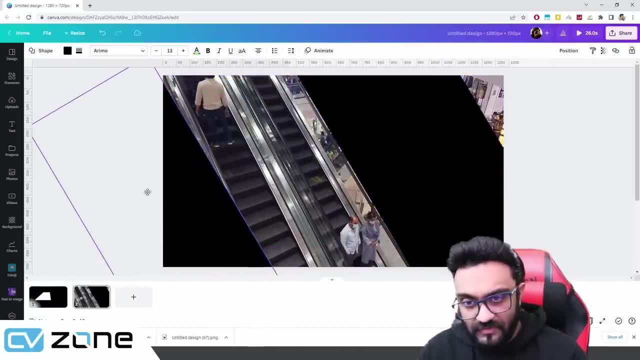 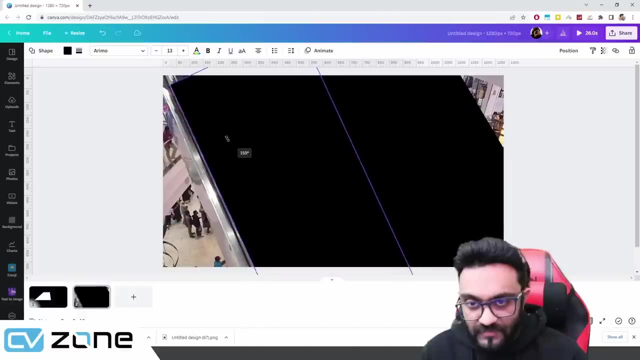 Why does it start in the wrong position? There you go. So yeah, I think that should be fine And we can remove this, because this is correctly aligned and we can paste it here. Oh no, the angles are different. Okay, so we need to rotate it again. 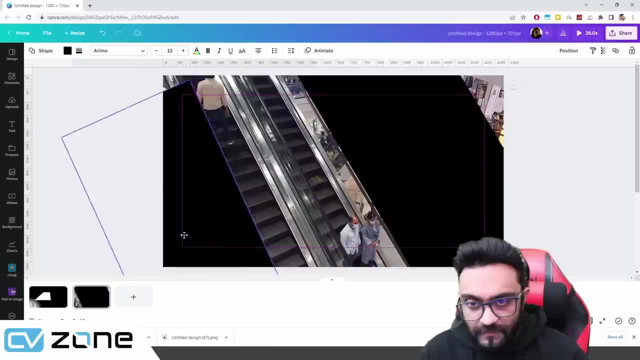 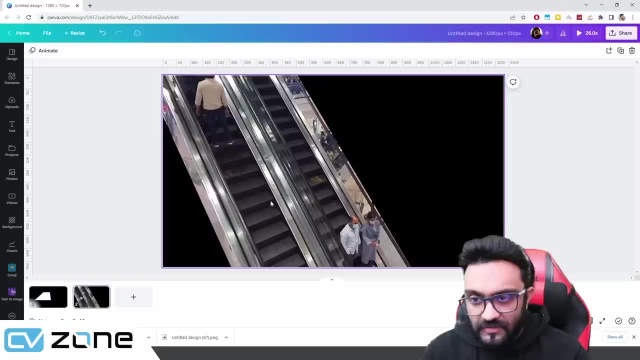 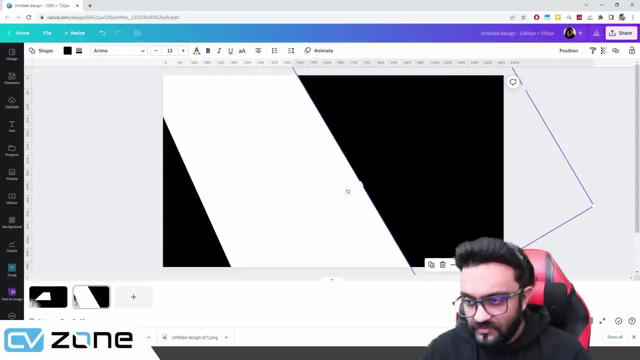 Maybe like that And we will put it here. There you go. So this should be our new mask and we can push this back here And we will delete this video so that becomes white. We need to fill this gap. There you go. 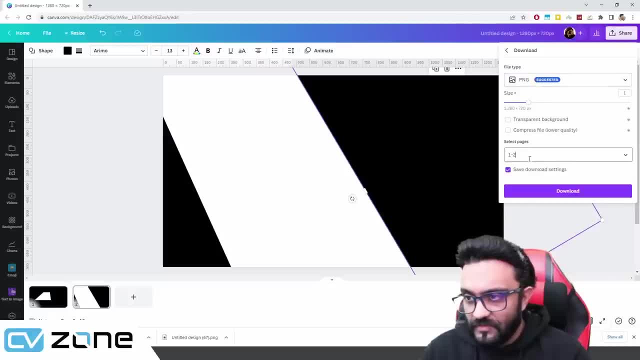 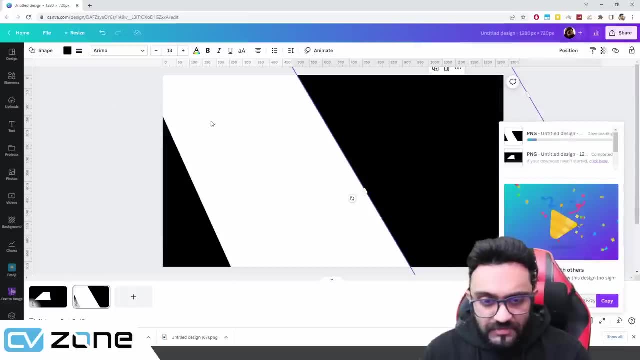 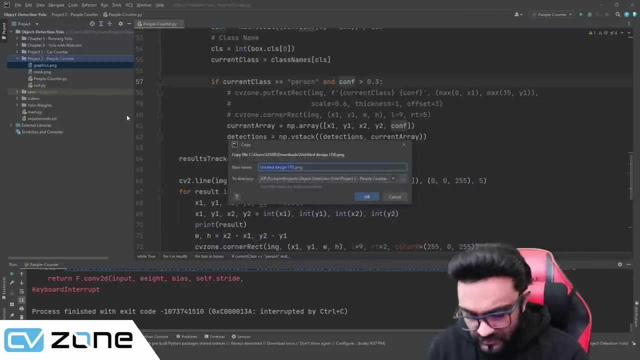 So we can download this mask. Now we need to select which page We're talking about- page number two, and we don't want any transparency or any compression. And now it's downloaded, So we will drag it in to our people counter and we will write here: mask. 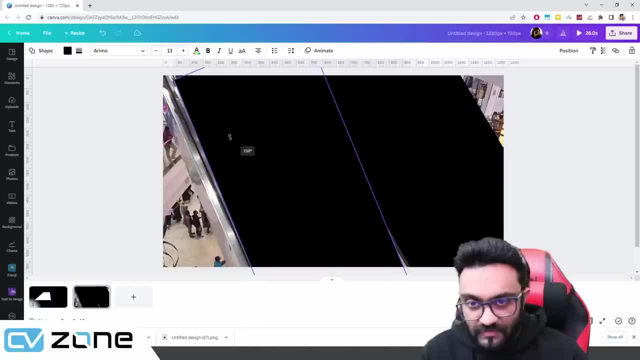 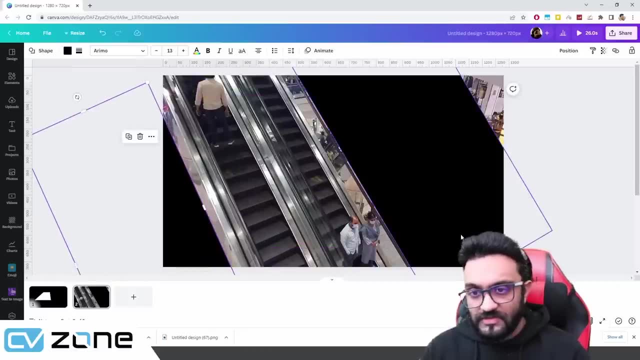 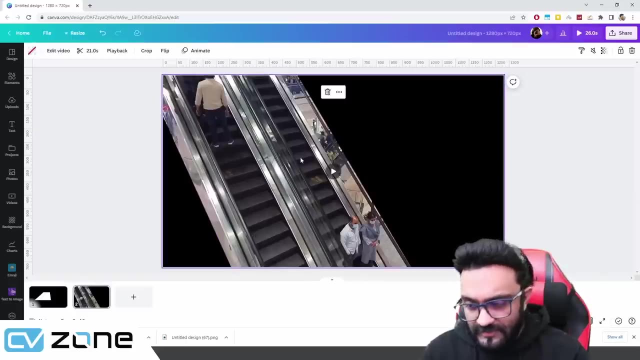 so we're going to rotate it here. oh no, the angles are different. okay, so we need to rotate it again, maybe like that, and we will put it here. there you go. so this should be our new mask and we can push this back here and we will delete this video. so that becomes white. we need to fill this cap there. 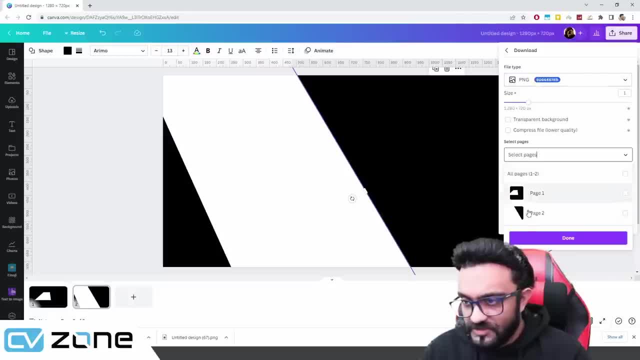 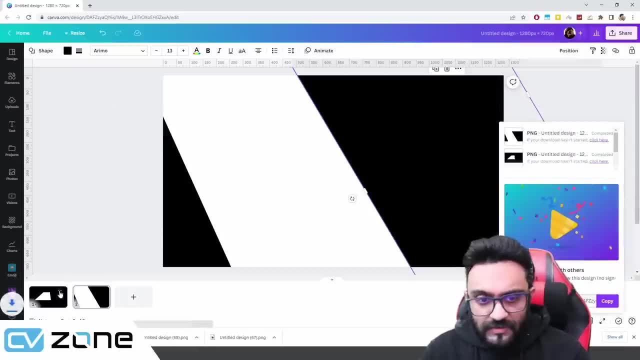 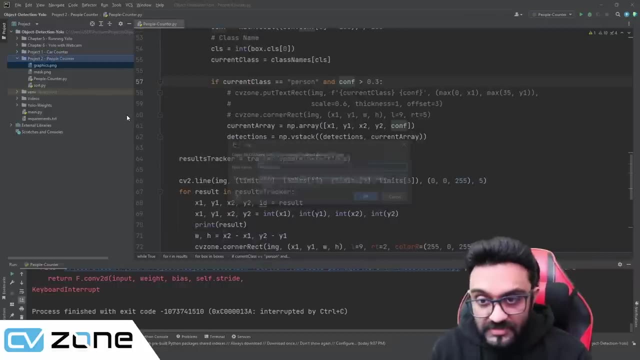 you go so we can download this mask. now we need to select which page we're talking about- page number two- and we don't want any transparency or any compression. and now it's downloaded, so we will drag it in our people counter and we will write here: mask the reason. 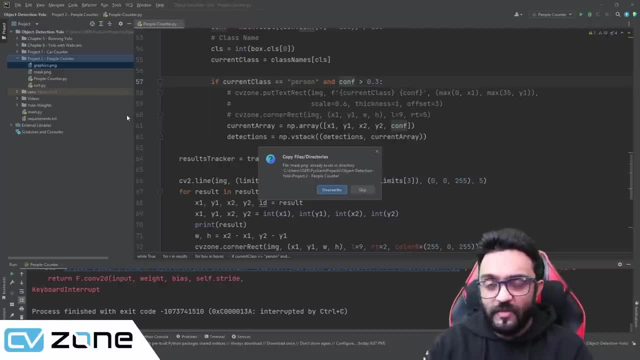 I'm showing this is because if you have a different video or if you are working on a different project, you can actually do it yourself. otherwise, for me to just copy and paste, it's very easy because I've already done this, but I'm showing you this so that you can do it yourself for your own project as well. so this is. 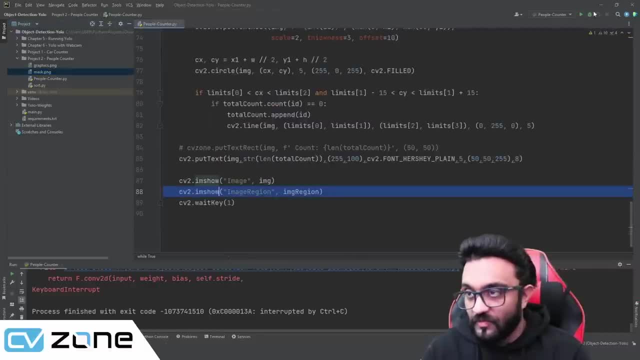 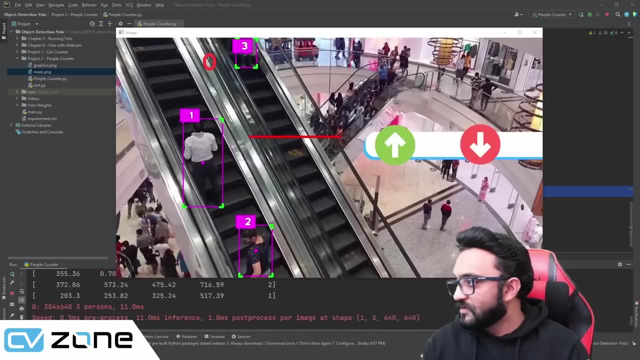 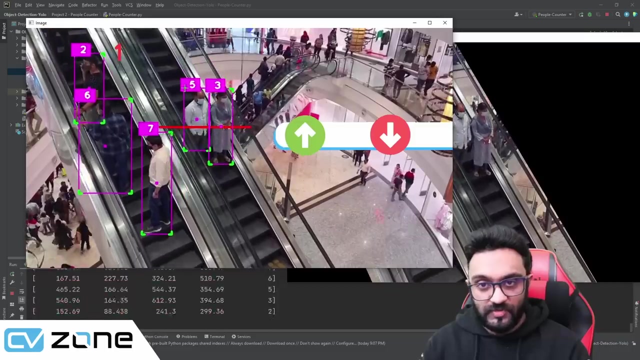 the mask, and now let's open up the region as well, so that we are 100% sure that it is working as we expect it to. so there you go. so this is the mask and, as you can see, it is detecting very well. so one, two, three, four, five, six, seven and 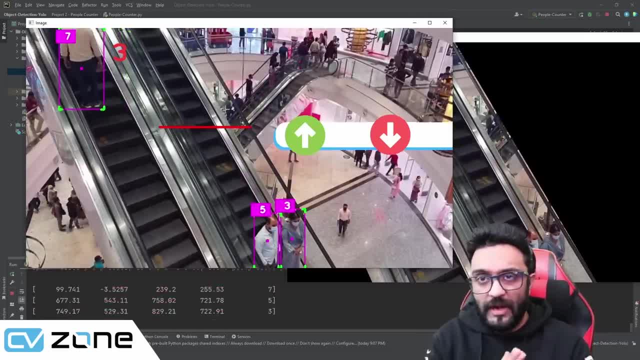 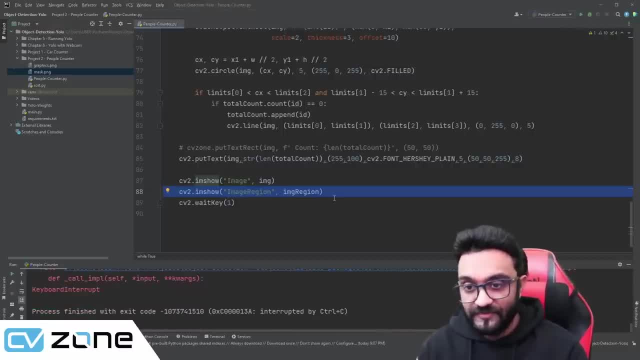 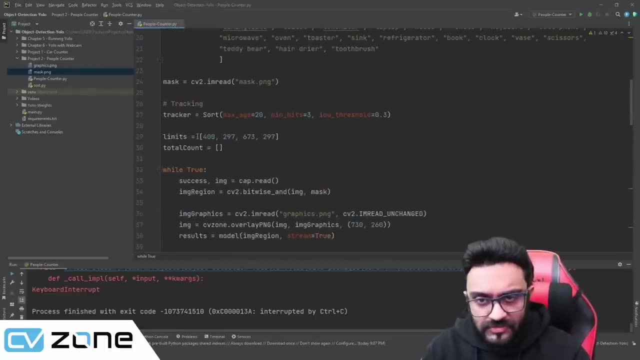 now we need to fix the counter. so how many people are going up and how many people are going down? so in this case we will have two lines, so we don't have just one line, we will have two limits. first of all, let's comment this out and we will go up and in the count or in the 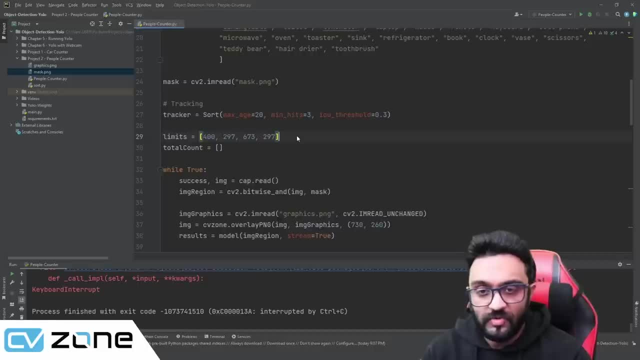 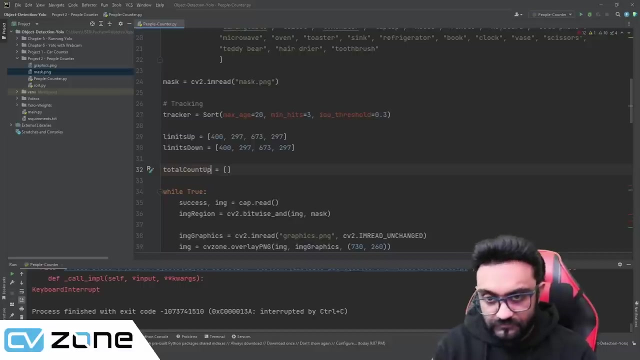 limits. we will have two of each. so we will have limit limits up and limits down, limits down, and then we have total count up and total count down. so we need to put the lines here. so I have the lines for up. it is one zero three, one sixty one and two, nine six. two, nine six and one six one, and then 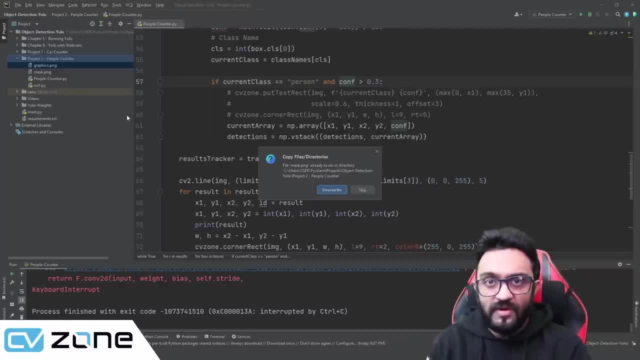 The reason I'm showing this is because if you have a different video or if you are working on a different project, you can actually do it yourself. Otherwise, for me to just copy and paste is very easy, because I've already done this, But I'm showing you this. 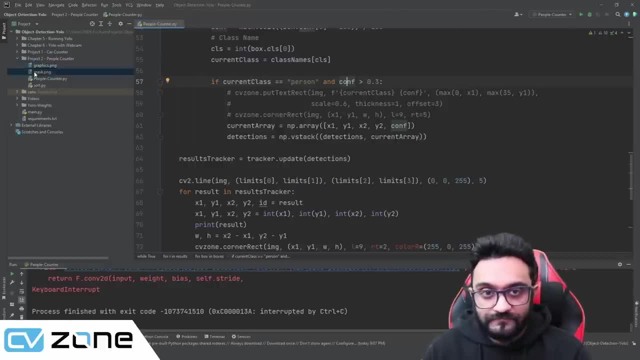 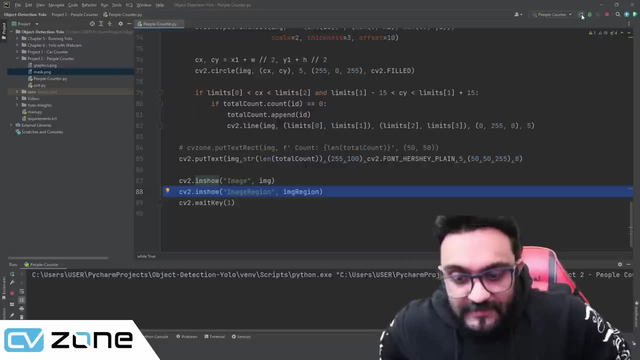 so that you can do it yourself for your own project as well. So this is the mask, And now let's open up the region as well, so that we are 100% sure that it is working as we expect it to. So there you go. 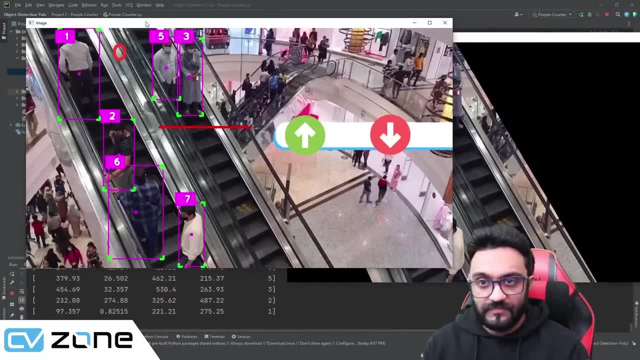 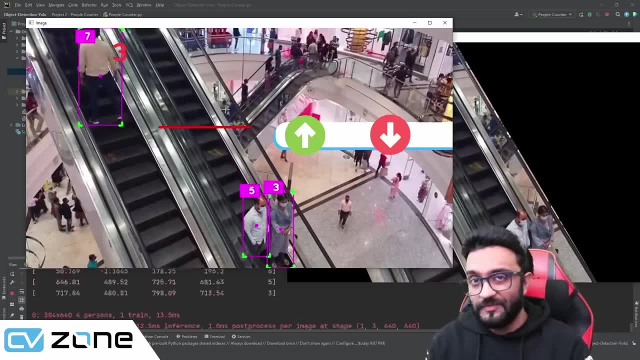 So this is the mask And, as you can see, it is detecting very well. So one, two, three, four, five, six, seven, And now we need to fix the counter. So how many people are going up and how many people are going down? 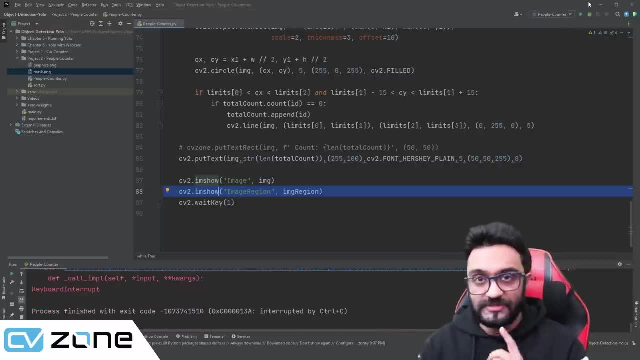 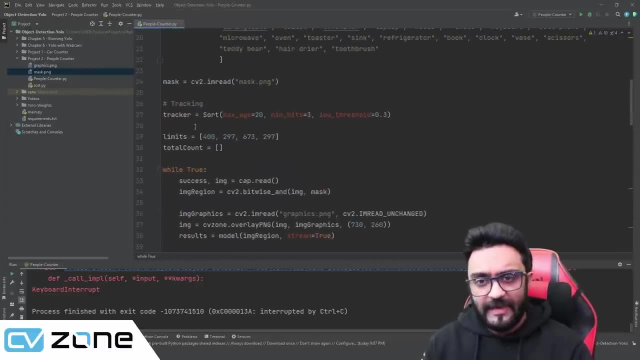 So in this case we will have two lines, So we don't have just one line, We will have two limits. First of all, let's comment this out and we will go up, And in the count or in the limits, we will have two of each. 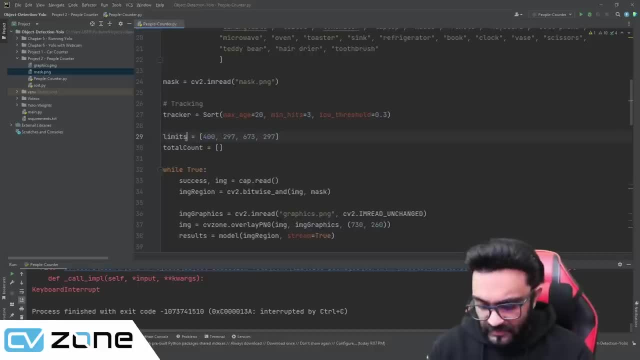 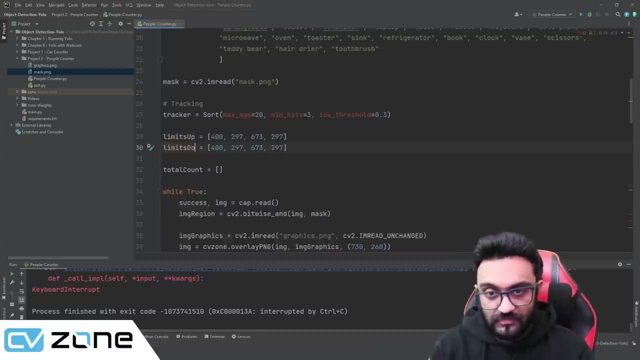 So we will have limits- limits up and limits down, Limits down- And then we have total count up and total count down. So we need to put the lines here. So I have the lines. for up, It is 103, 161. 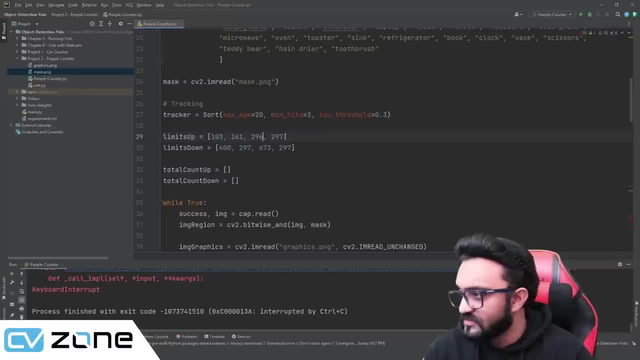 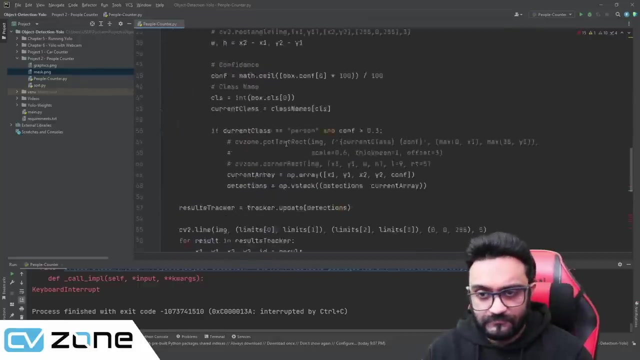 and 296, 296 and 161.. And then for the limit down is 527, 489 and 735 and 489.. 735 and 489.. Yeah, So, yeah, that's good, And here we have limits, because now we'll have some headers. 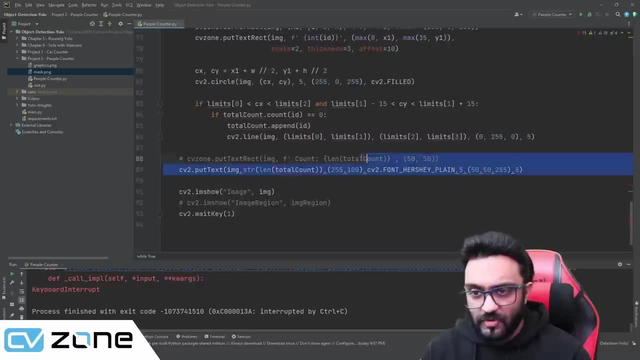 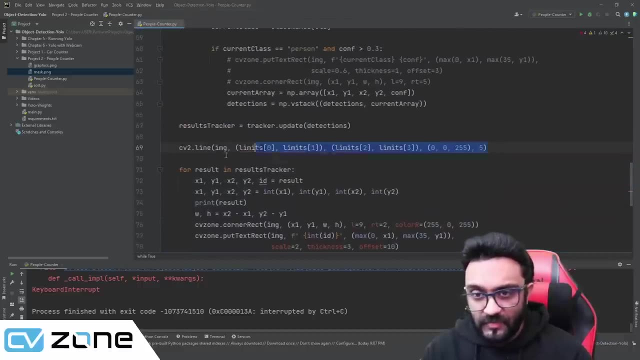 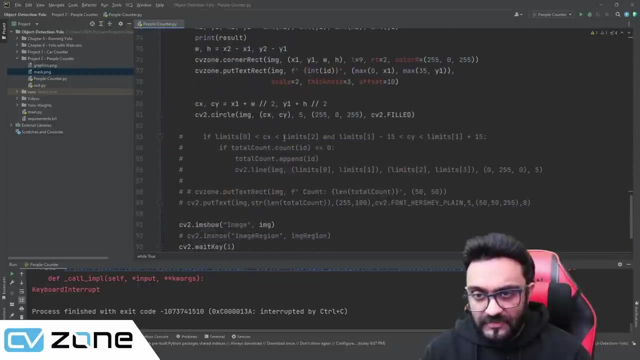 because limits is not actually there. So what we can do is we can comment all these headers, We can comment this control and slash is how you comment, And then we will comment this as well, And anything else, No. Okay, So now that this is commented, 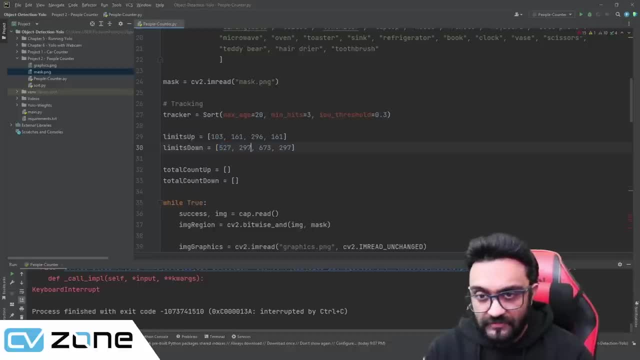 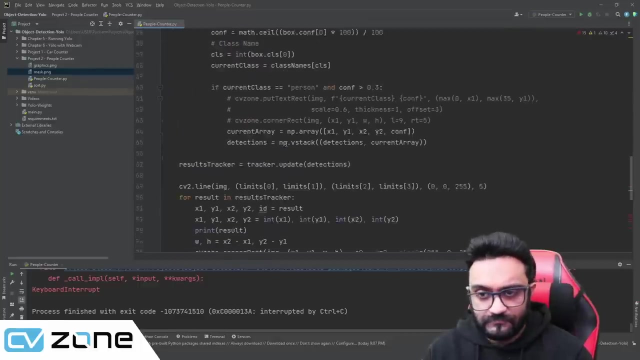 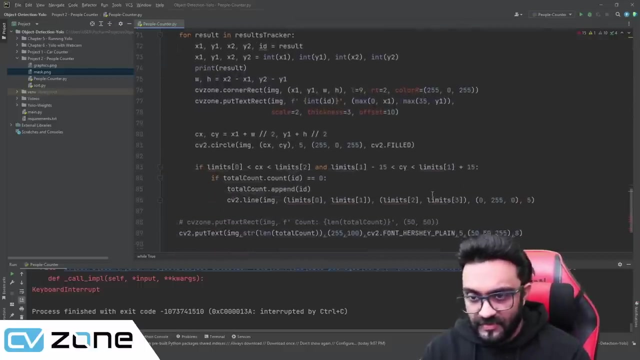 for the limit down is five, two, seven, four, eight, nine and seven, thirty five and four at night, seven, three, five and our eight, nine, yeah. so yeah, that's good, and here we have limits, because now we'll have some headers, because limits it's not actually there. so what we can do is we can. 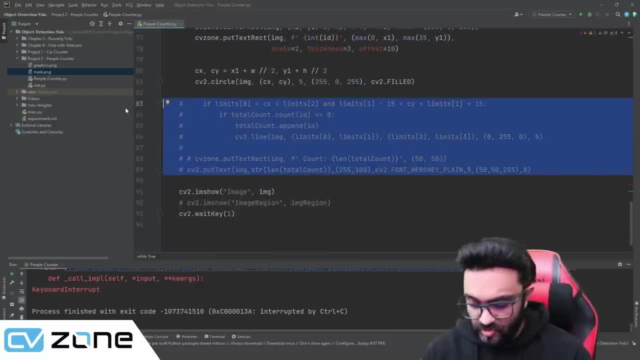 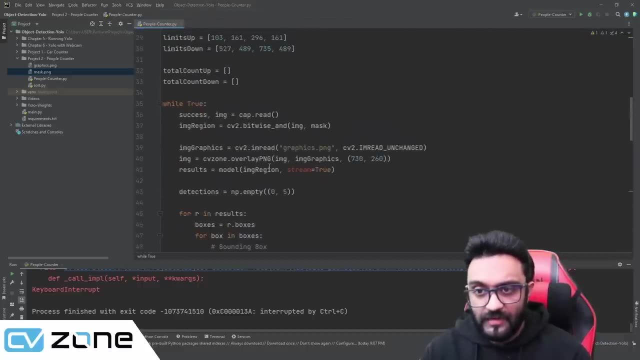 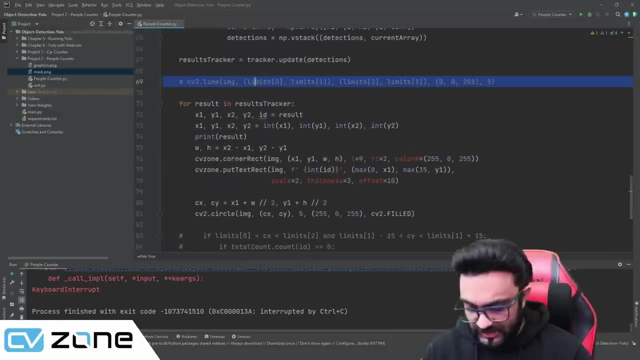 comment all these errors. we can comment this. control and slash is how you comment, and then will comment this as well and anything else, no, okay. so now that this is commented and we know there will be no errors, what we can do is we can change this line, for example, to limits up. 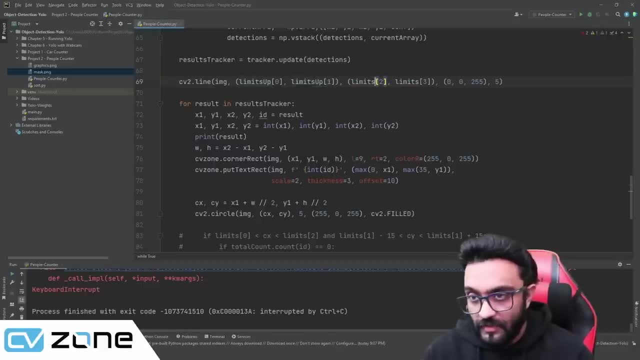 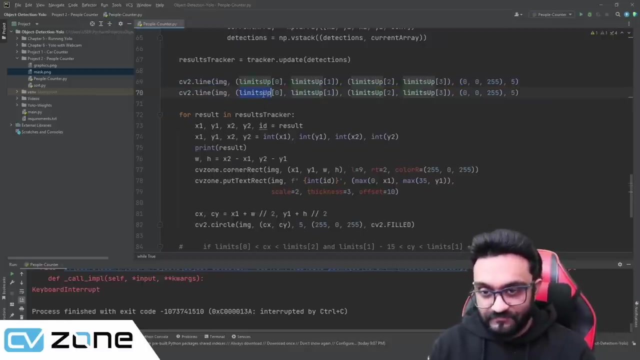 and we can write here up and up. why am i writing it wrong up and up? okay, and then we will write again for the other line. we will write down limits down and i'm going to copy it so that i don't have to manually write it again, again. okay, 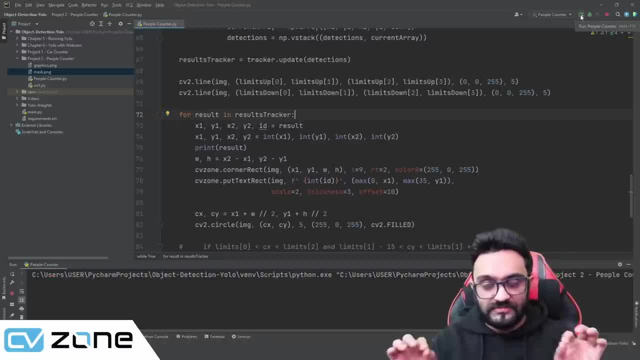 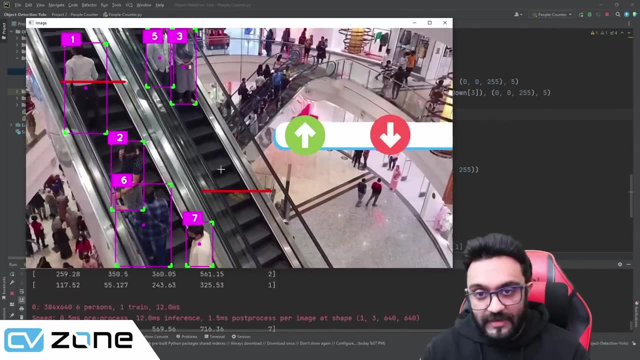 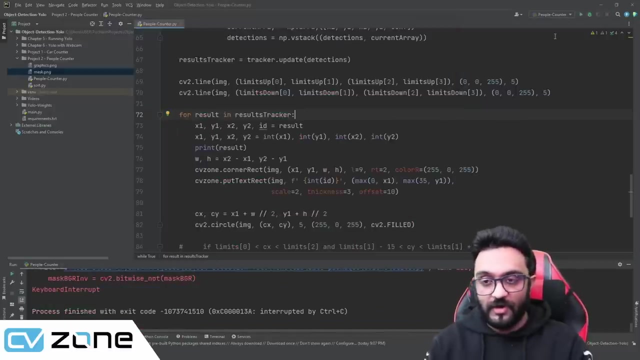 so let's run that and hopefully we will have two lines, uh, one for going up and one for going down. there you go. so this line is for going up and this line here is for going down. so we need to check for both of these individually. uh, how many people are crossing that line and how many people? 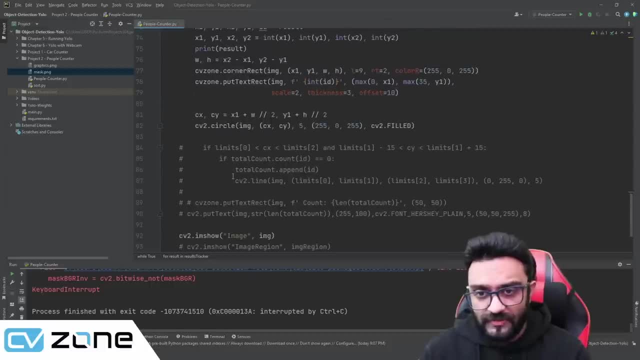 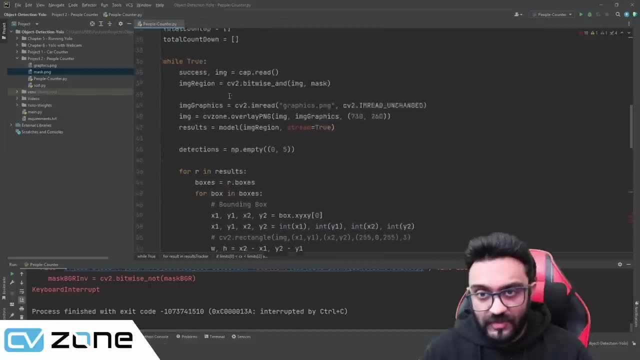 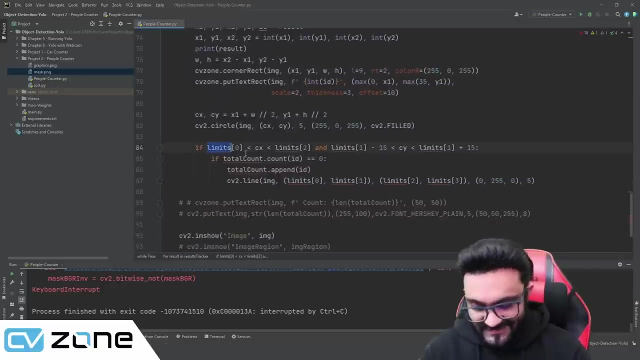 are crossing that line. okay, so then we will come to the limits. so here let's do for one. so instead of limits, we will write limits up. see how lazy i am, i'm going up just to copy it, the limits up. i'm going to paste everywhere. uh, you can actually do a search and replace. 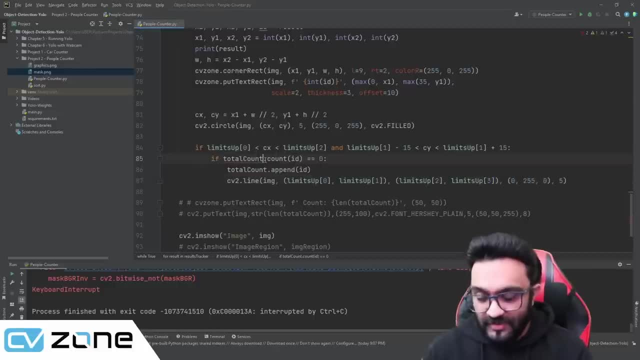 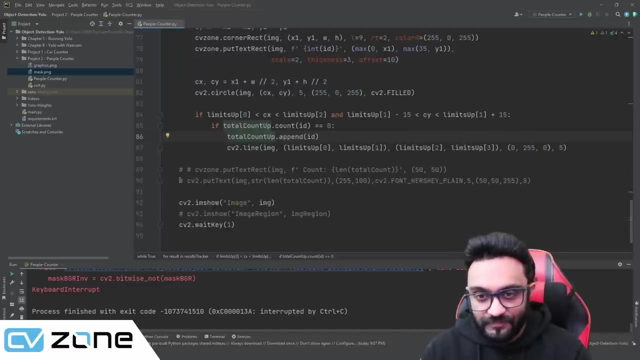 but again, you see how lazy i am. okay, total count, we will put up why i, i don't know why. okay, total count up dot, band id and blah, blah. and here in the, in the put text, we are going to write up: okay, so let's run that and let's see. uh, what kind of results do we get? are we getting anything to? 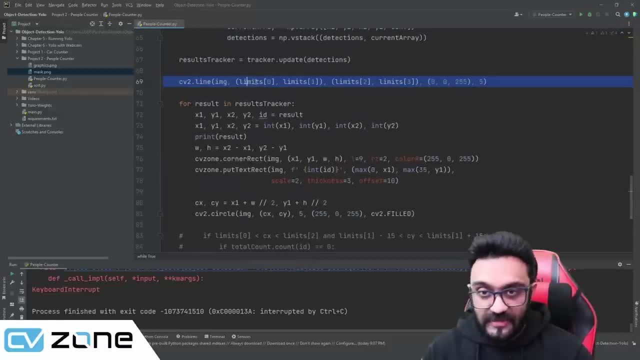 and we know there will be no headers. what we can do is we can change this line, for example, to limits up, And we can write here up and up. Why am I writing it wrong? Up and up, Okay, And then we will write again. 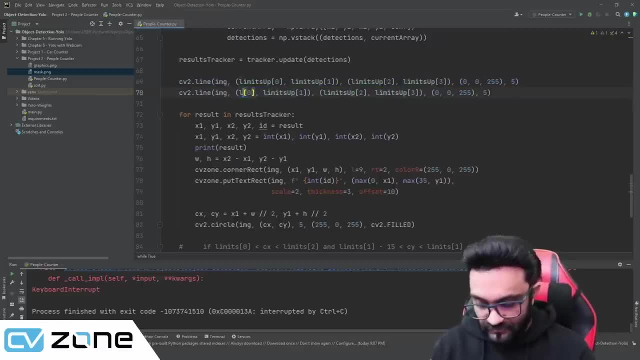 for the other line, we will write down Limits down And I'm going to copy it so that I don't have to manually write it again and again. Okay, So let's run that And hopefully we will have two lines, one for going up. 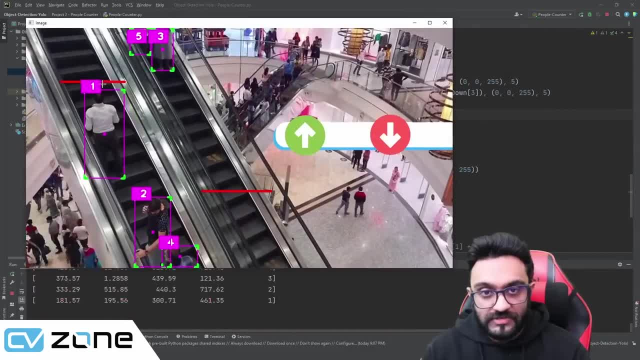 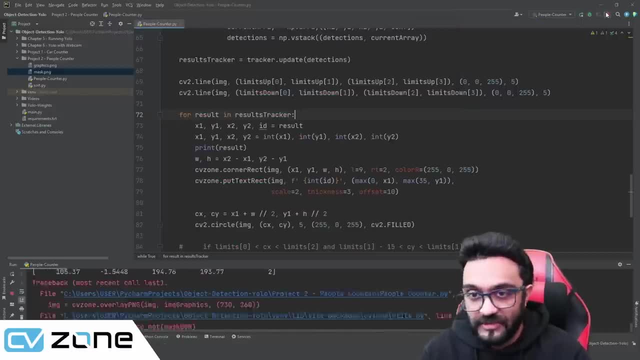 and one for going down. There you go. So this line is for going up and this line here is for going down. So we need to check for both of these individually: how many people are crossing that line and how many people are crossing that line. 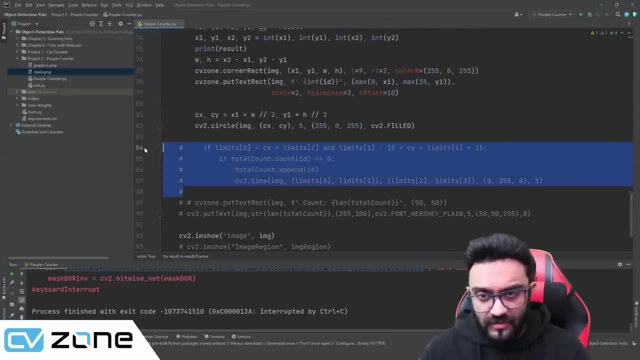 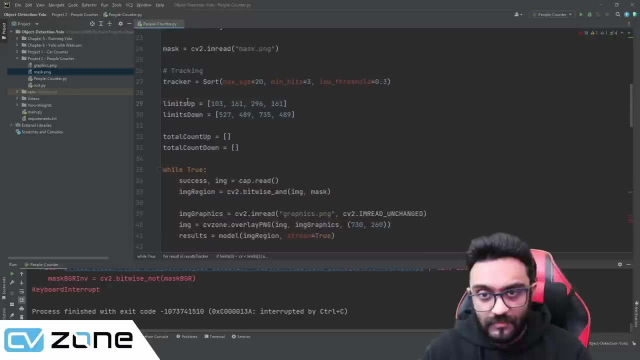 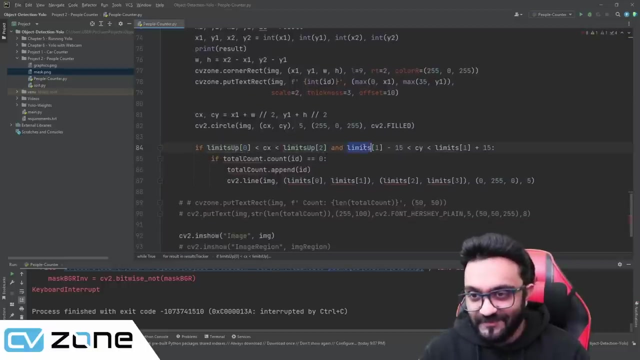 Okay, So then we will come to the limits. So here let's do for one. So instead of limits, we will write limits up. See how lazy I am, I'm going up just to copy it. So limits up, I'm going to paste everywhere. 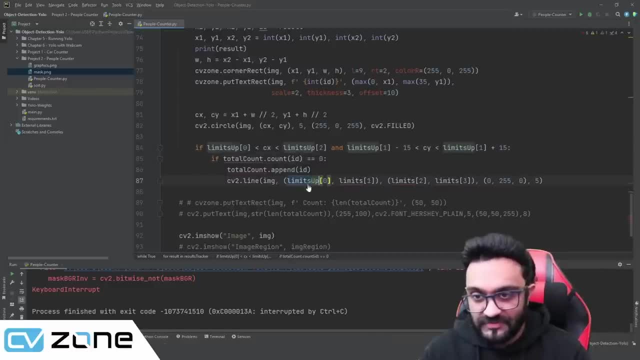 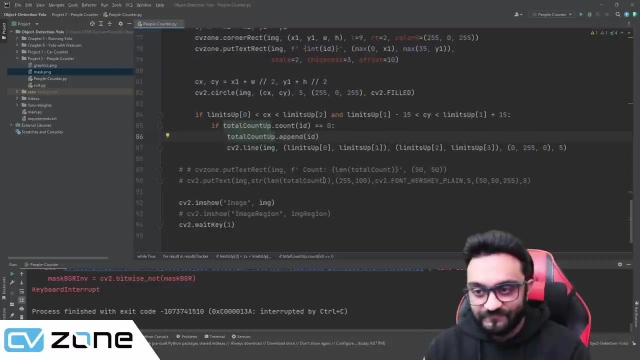 You can actually do a search and replace, But again, you see how lazy I am. Okay, Total count, we'll put up Why I, I don't know why. Okay, Total count up dot, append Up, dot, append ID, and blah blah. 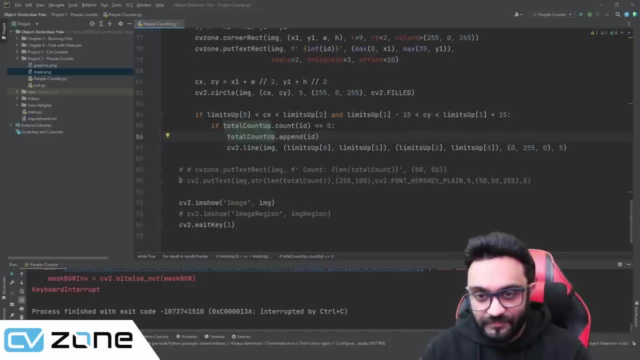 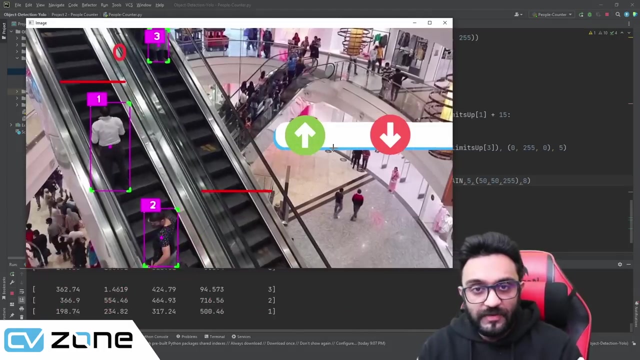 And here in the, in the put text we are going to write up: Okay, So let's run that and let's see what kind of results do we get. Are we getting anything good? Because it is supposed to get red green. 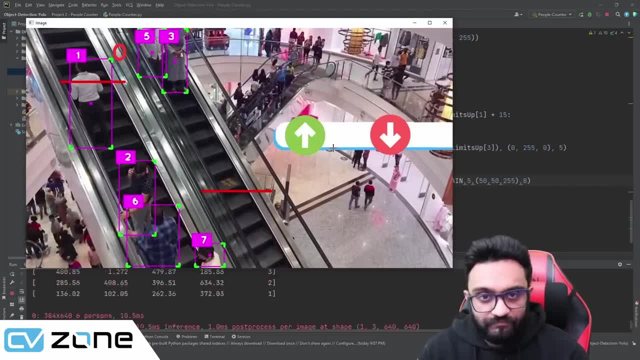 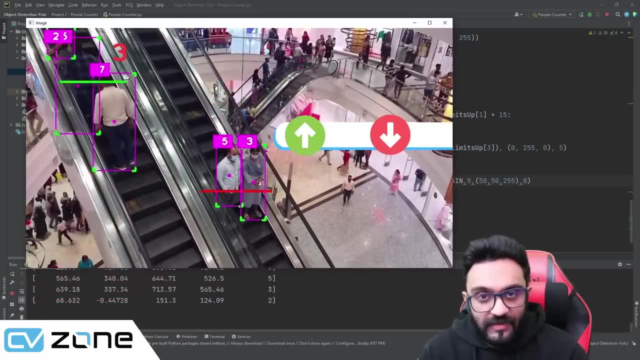 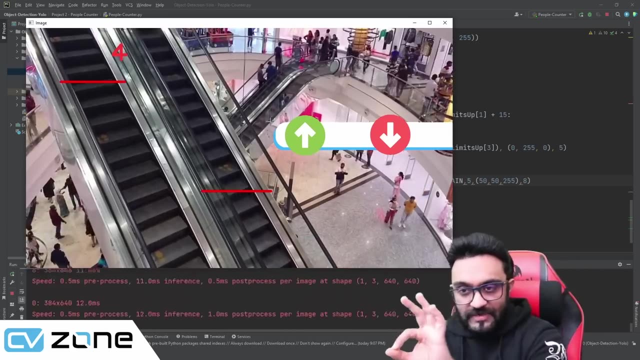 it because it is supposed to be: uh get red, uh green. yeah, so there you go, it went green. one count, two count and three count. there we go and four count. excellent, so this is working fine. all we need to do now is take that and put it down, uh, in the correct region and make it green instead of 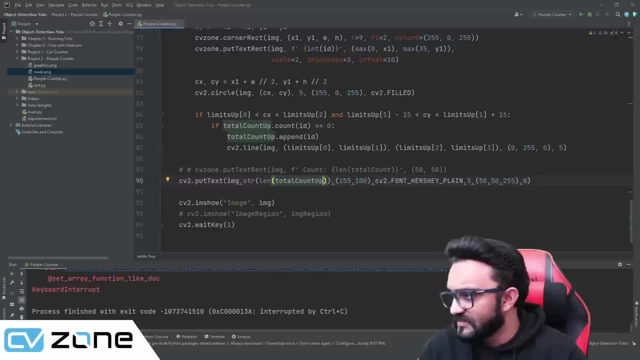 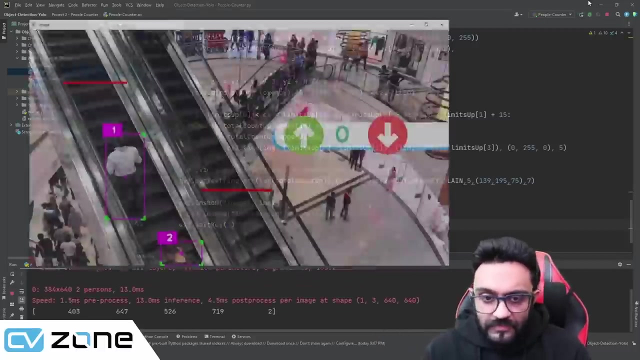 red. so let me check the values. exact values for the count is 929 and 345.. three, four, five and hershey plane five and seven, and this should be 139, 195 and 74.. so we're giving it a bit of a green color. uh, green is for up, red is for down. so there you go. so here you have zero. 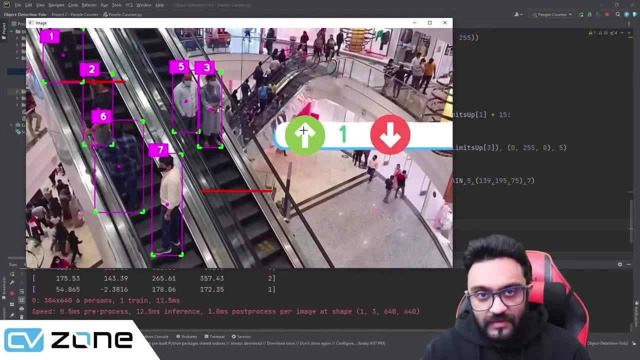 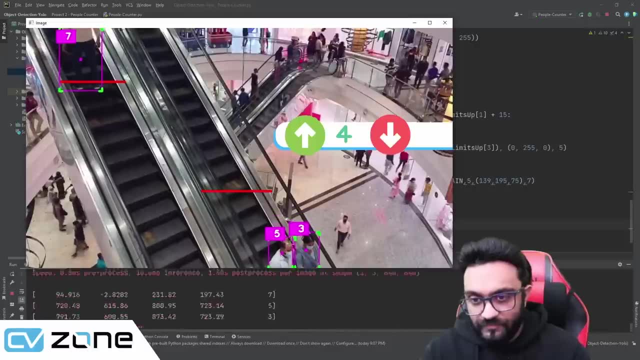 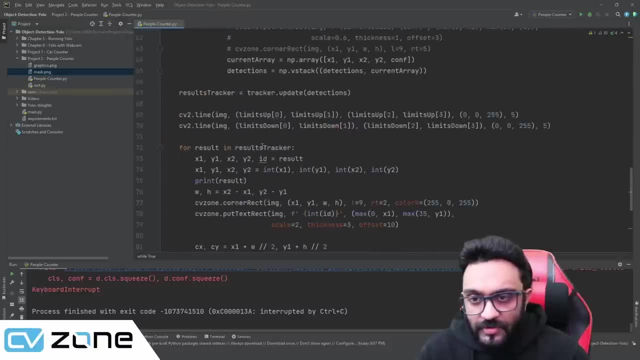 so the first one goes, so you get one, and then the second one is two and the third one is three. so now we need to do for the people going down. okay, so for the people going down, it's very simple. all you have to do is you have to. 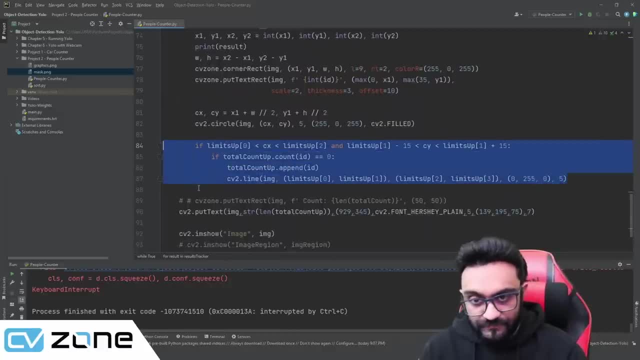 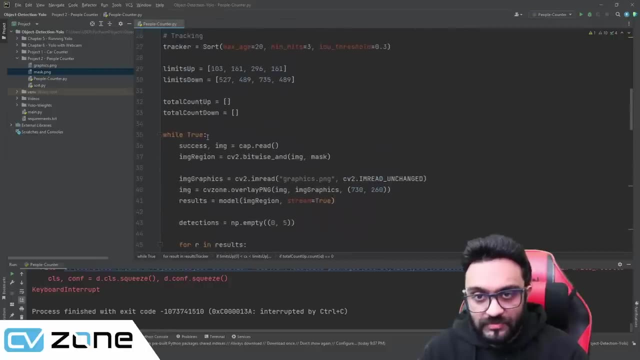 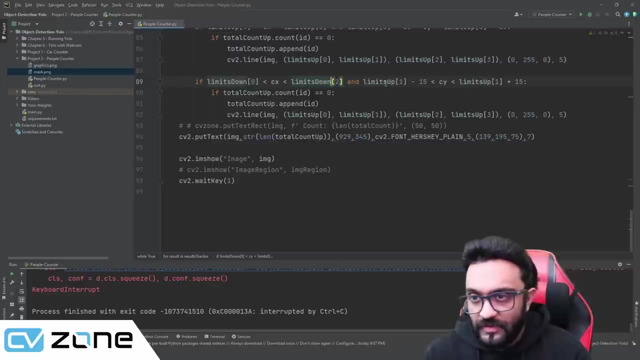 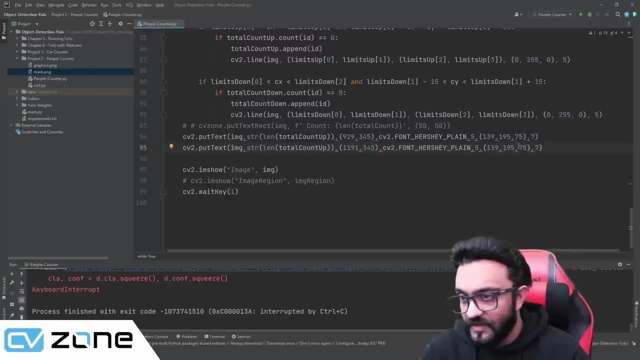 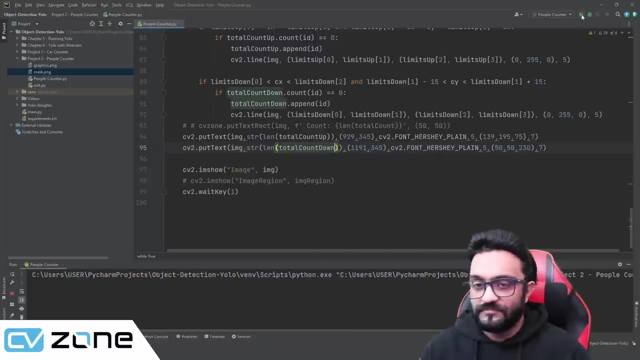 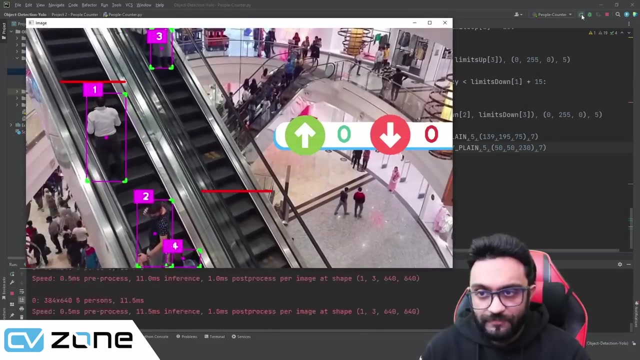 values are one, one, nine, one and three, four, five, and the color will be fifty, fifty and two thirty, so this should be total down. so let's run that and see if it works. there you go. so we have the red part here, the green part here, so this is going up. 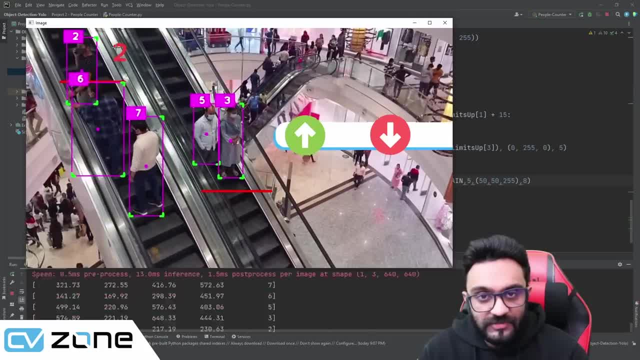 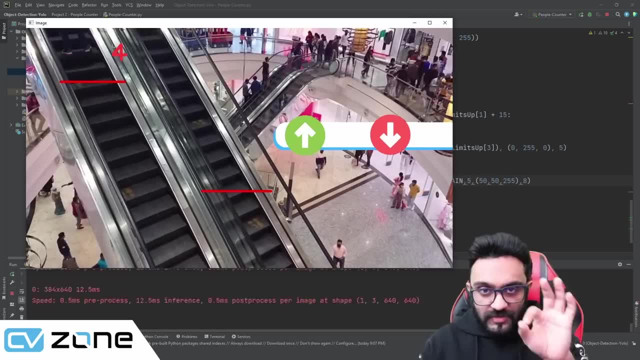 Yeah, So there you go, It went green. One count, two count and three count. There we go And four count. Excellent, So this is working fine. All we need to do now is take that and put it down in the correct region. 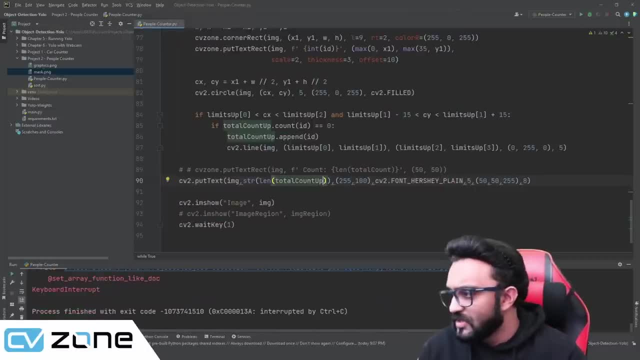 and make it green instead of red. So let me check the values. Exact values for the count is 929 and 345.. 345.. And Hershey, plane five and seven, And this should be 139,, 195, and 74.. 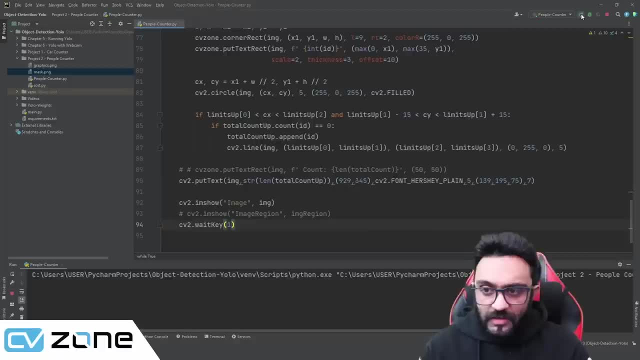 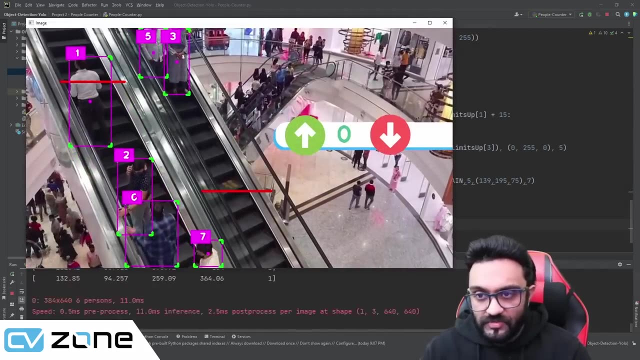 So we are giving it a bit of a green color. Green is for up, red is for down. So there you go. So here you have zero. So the first one goes, So you get one, And then the second one is two. 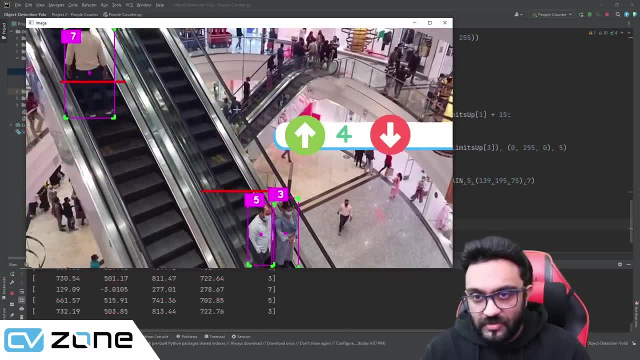 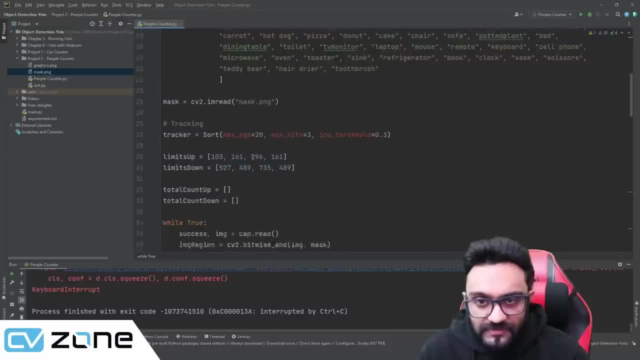 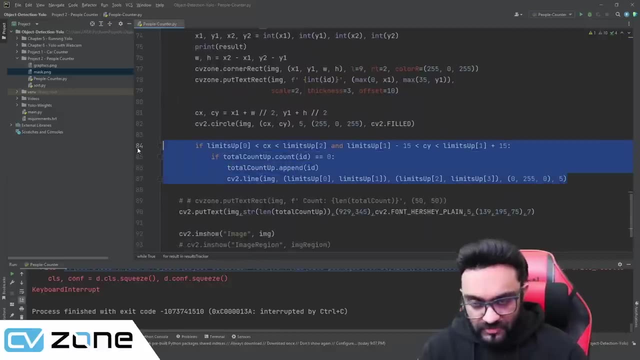 And the third one is three. So now we need to do for the people going down. Okay, So for the people going down, it's very simple. All you have to do is you have to hear the if condition, copy that and paste it. 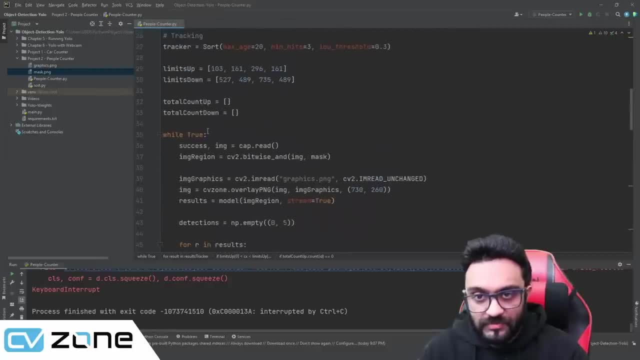 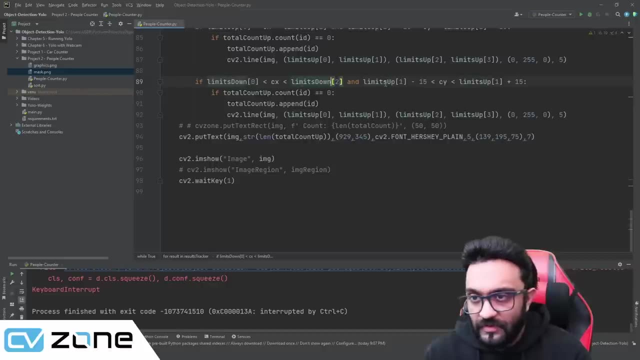 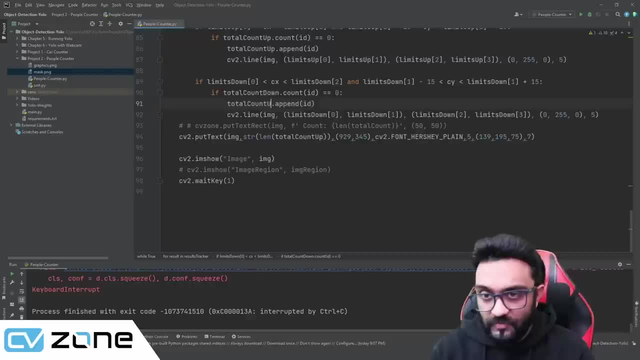 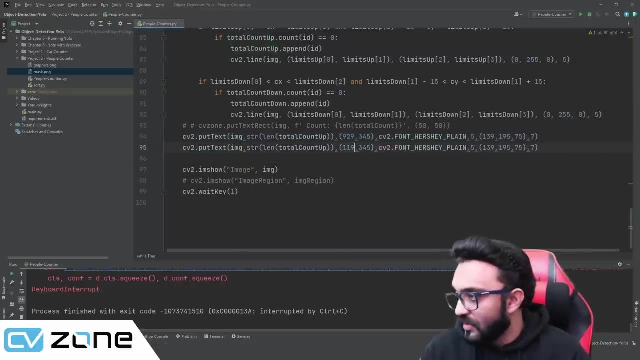 So that will become down. Count up will become down. We will copy the text And here the values are 1191 and 345.. And the color will be 50,, 50, and 230.. So this should be total down. 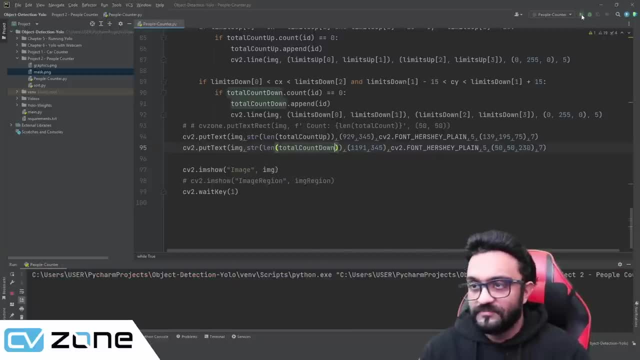 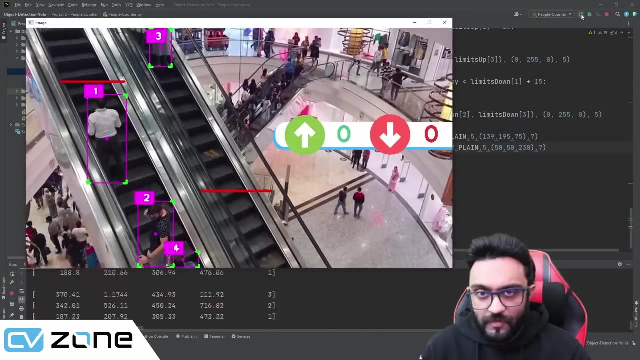 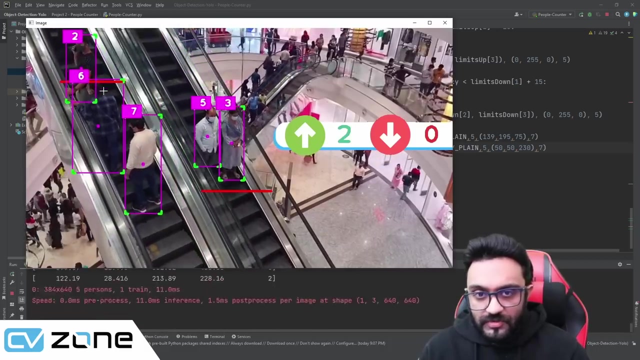 So let's run that and see if it works. There you go. So we have the red part here, the green part here. So this is going up: One, two, three, And now it should detect these two as well: One and two. 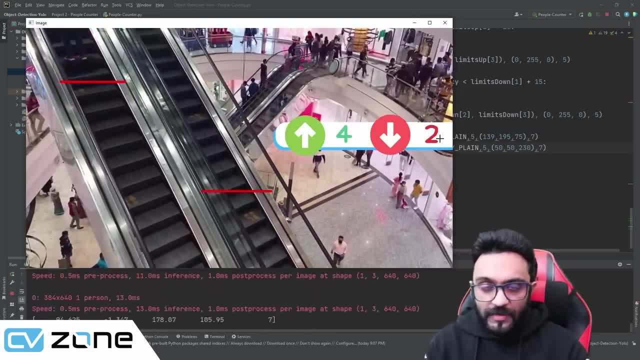 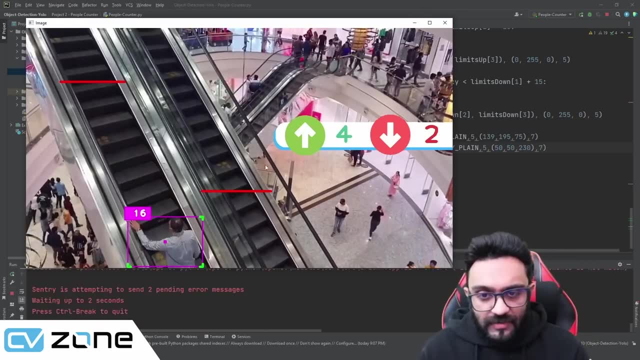 There you go. So we have a total number of people- four people going up- And we have a total number of two people going down. So again, if it was crowded, it will detect all the other people as well And it will do the calculations. 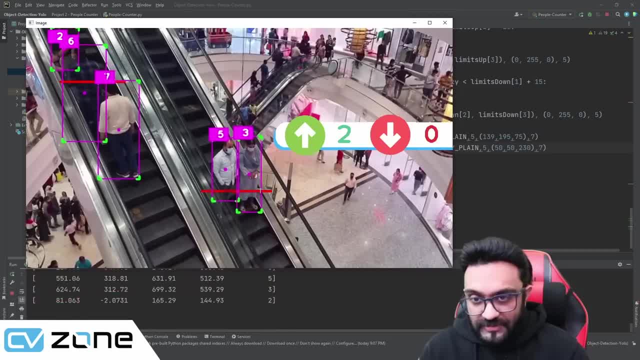 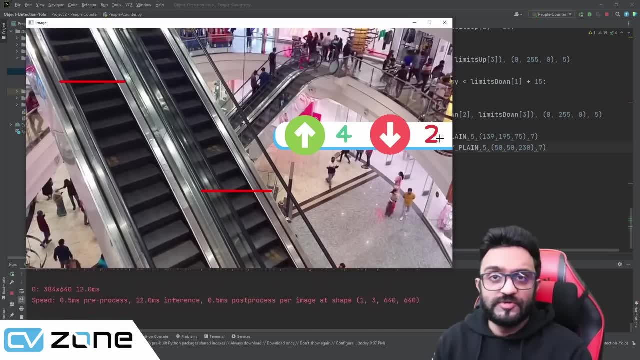 one, two, three, and now it should detect these two as well. one and two. there you go, so we have a total number of people- four people- showing up, so let's copy that down. this is a private growth going up and we have a total number of two people going down. so again, if it was crowded, it will. 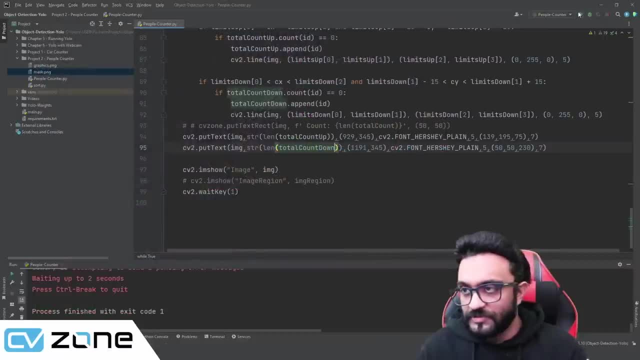 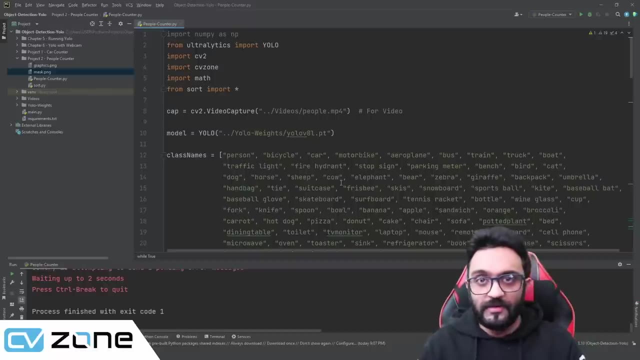 detect all the other people as well and it will do the calculations. so, as you can see, it's very easy to actually change the code a little bit and cater it to your own project, and it is very fun to play around with these values and because this is something that you can implement in real time. 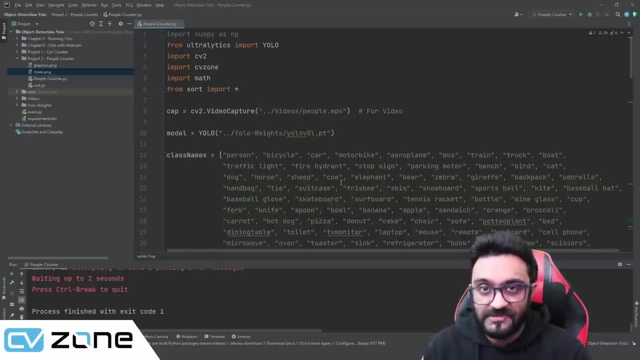 and it is something you can implement it as a real world application. that's why it's really informative and fun to do as well, and in the next part we are going to learn how to create your own custom model so you can create your own data set and use that data set to train your model and 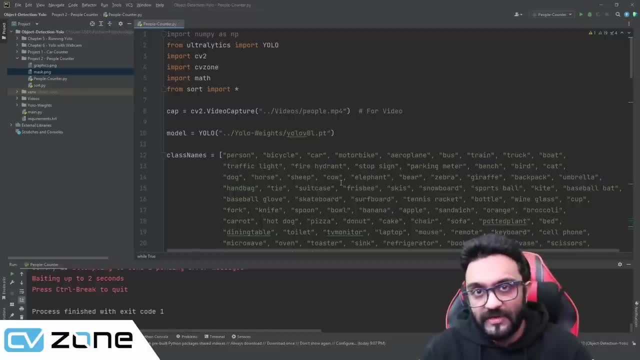 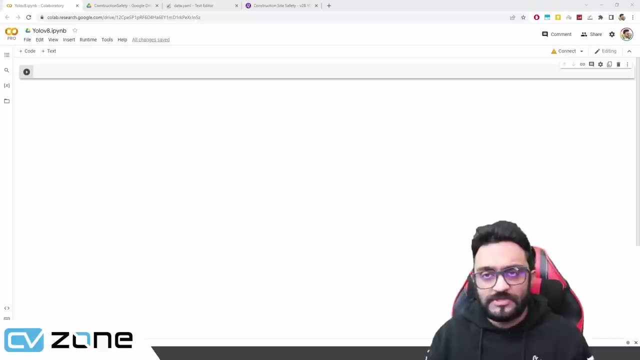 using that model, you can create your project. so that is what we are going to do next, so let's go ahead. so now we have already seen that. we have already seen that we have already studied and already learned how actually we can use pre-trained model to 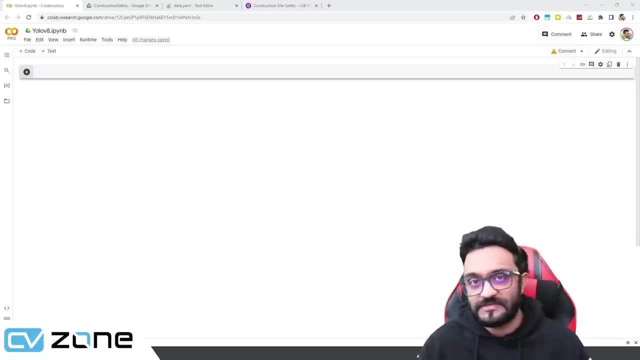 create our projects. but now we are going to create custom trained models with our own data set and we are going to use it in our projects. so how can we do that? so we can do that by using either nvidia's graphic card or we can use it by running google collab online. so we will be 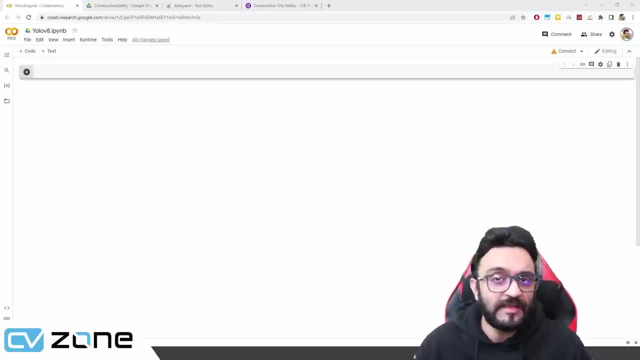 using google collab, since everyone has access to it and it's free to use, and if you have your own graphics card installed, you can do pretty much the same thing offline as well. pretty much the same code to run it on your own pc. so here we have a google collab opened up and it's called yolo. 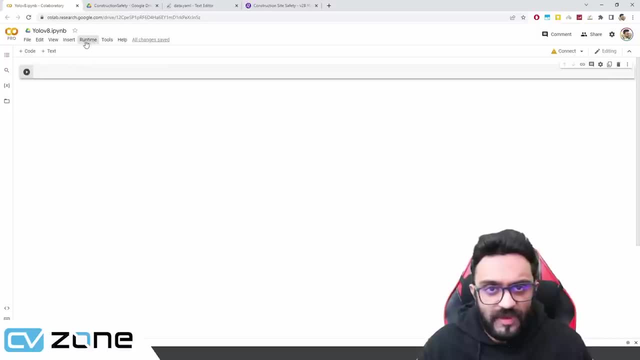 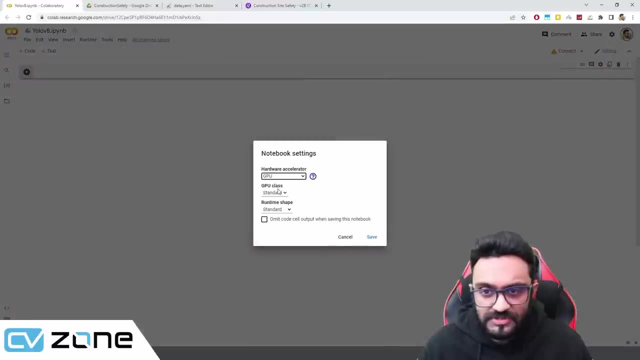 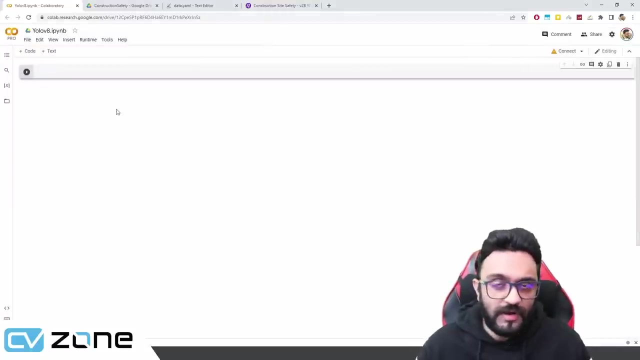 version 8 and right now it's empty and what we have to make sure is that the runtime is. if you go to change, we have to make sure that the runtime is gpu. we are going to save that now. uh, before we actually go and write some code on how to train your custom model, we need to know what kind of 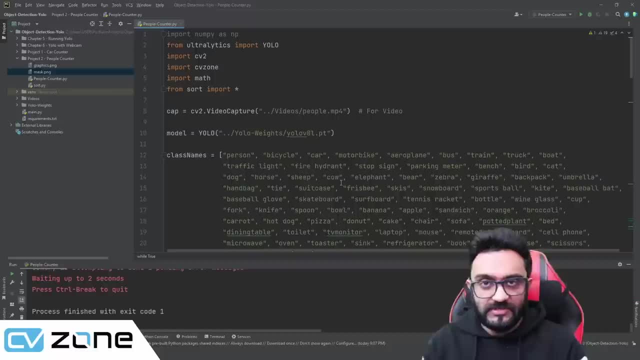 So, as you can see, it's very easy to actually change the code a little bit and cater it to your own project, And it is very fun to play around with these values, And because this is something that you can implement in real time and it is something you can implement it as a real world application. 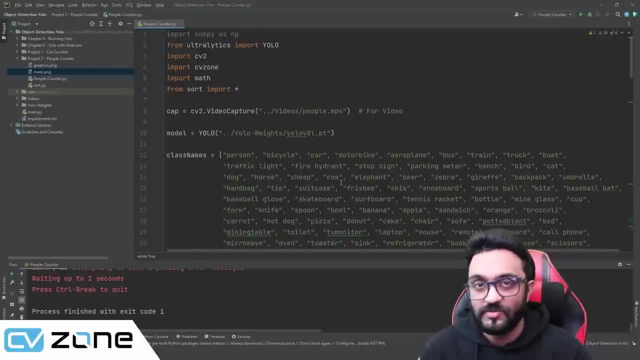 that's why it's really informative and fun to do as well. And in the next part we are going to learn how to create your own custom model so you can create your own data set and use that data set to train your model And using that model. 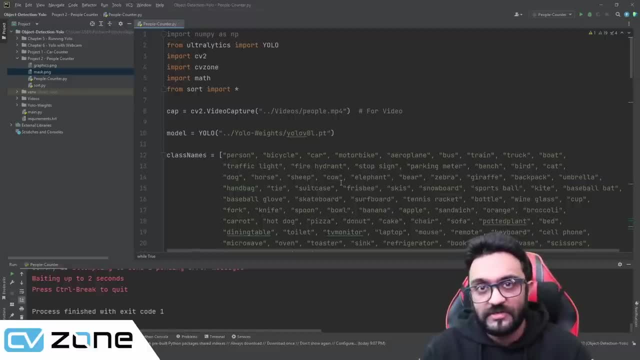 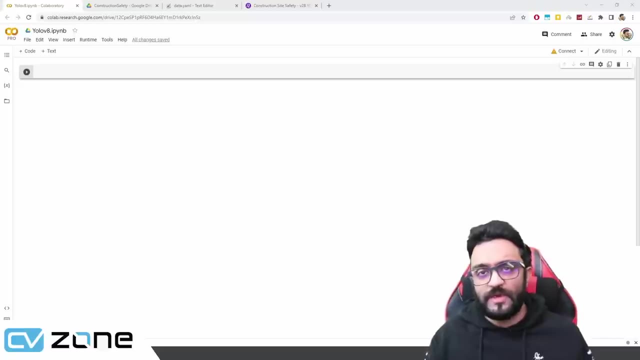 you can create your product. So that is what we are going to do next. So let's go ahead. So now we have already studied and already learned how actually we can use pre-trained model to create our projects, But now we are going to create custom trained models. 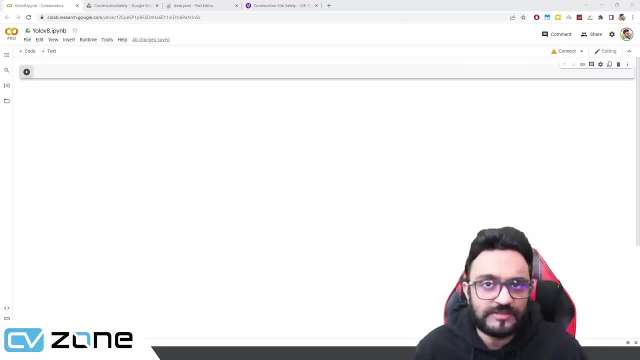 with our own data set And we are going to use it in our projects. So how can we do that? So we can do that by using either Nvidia's graphic card or we can use it by running Google collab online. So we will be using Google collab, since everyone has access to it. 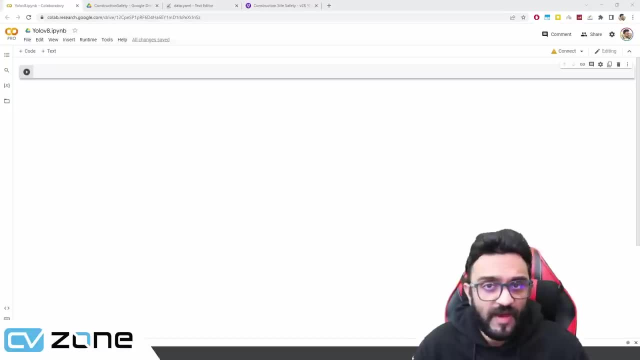 and it's free to use. And if you have your own graphics card installed, you can do pretty much the same thing offline as well. Pretty much the same code to run it on your own PC. So here we have a Google collab opened up. 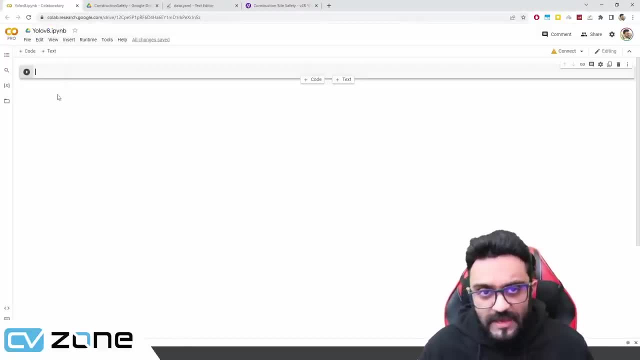 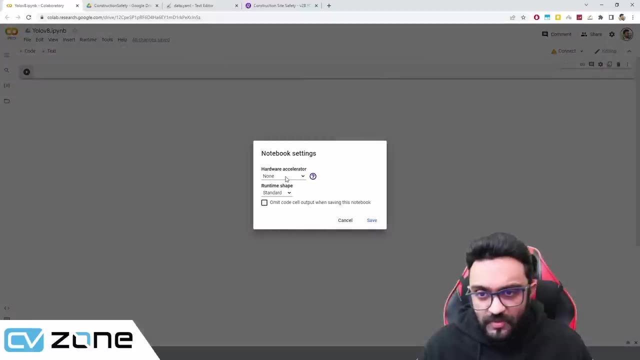 and it's called YOLO version 8.. And right now it's empty And what we have to make sure is that the runtime is. if you go to change, we have to make sure that the runtime is GPU. We are going to save that. 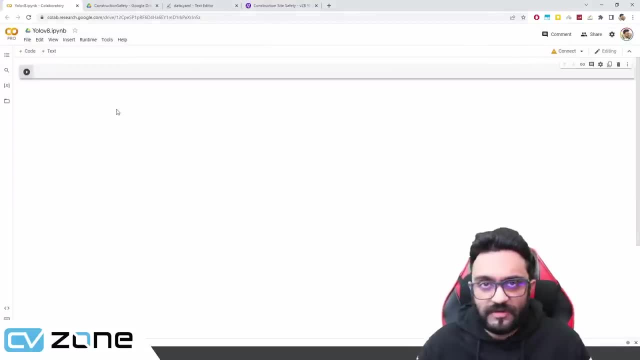 Now, before we actually go and write some code on how to train your custom model, we need to know what kind of data set that we need. So the project that we are going to do today is called the PPE detection, or the personal protective equipment. 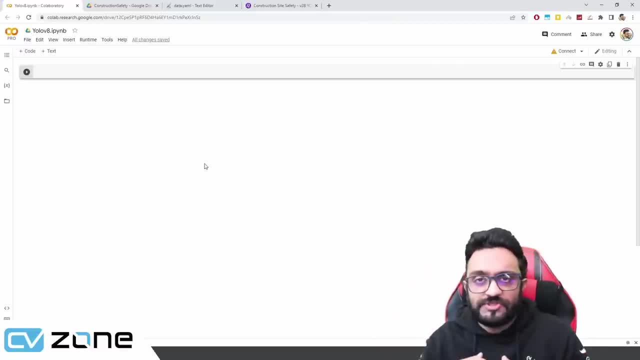 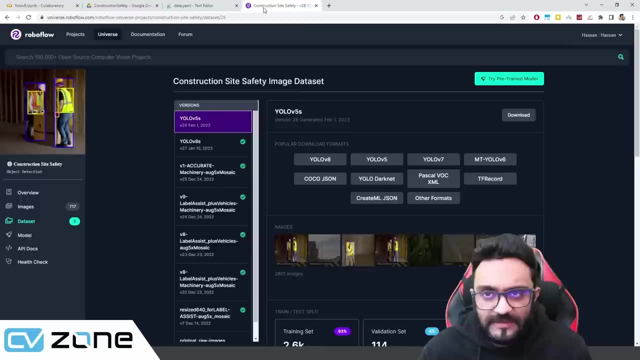 Basically the hard hat and the construction jacket and the mask. So we need to find whether a person is wearing that or not. So we have this data set available on RoboFlow and you can see we have the version YOLO 8 as well. 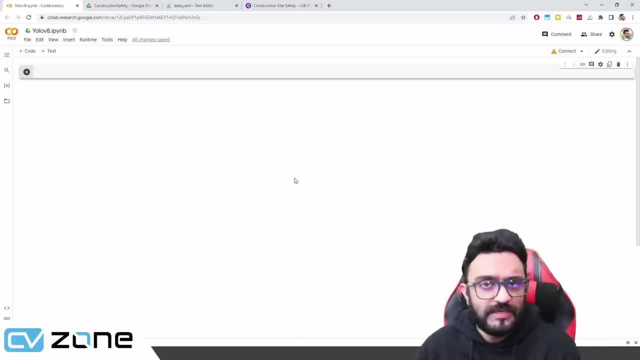 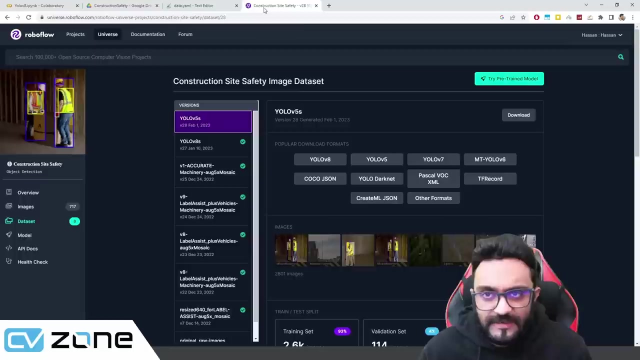 data set that we need. so the project that we are going to do today is called the ppe detection, or the personal protective equipment, basically the hard hat and the construction jacket and the mask. so we need to find whether a person is wearing that or not. so we have this data set available. 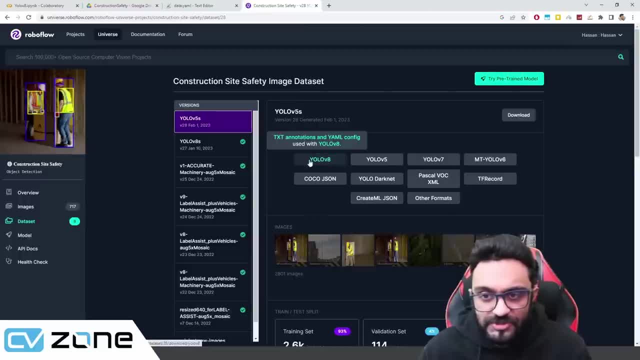 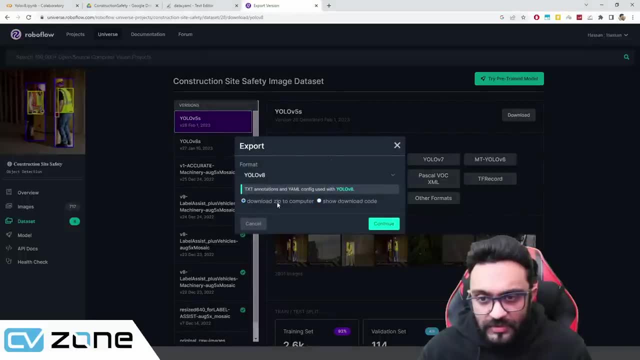 on roboflow and you can see we have the version yolo 8 as well. you can simply download it from here. so if you click on that and you can download uh zip to computer and you can press continue now. by doing this, what will happen is that you will get the data set as well as the 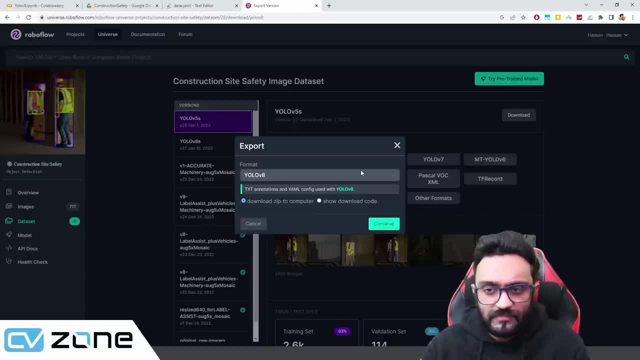 yaml file that will allow you to run with yolo version 8.. now, if you don't have a data set available online and if you wanted to create your own data set, then you actually need to know what is the format of the data set that you want to use. and if you want to create your own data set, 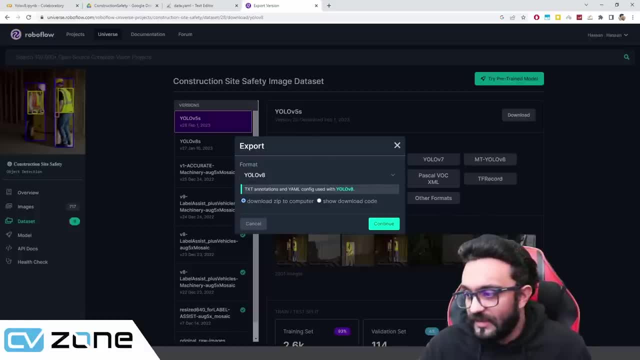 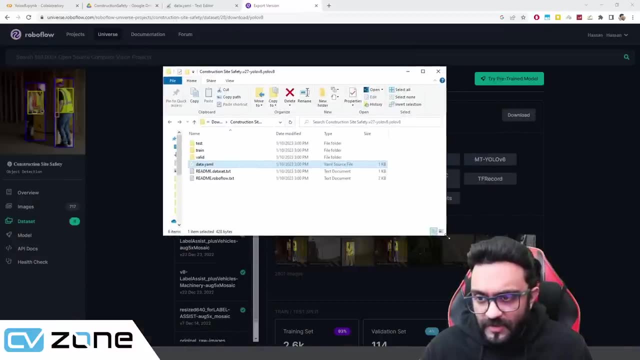 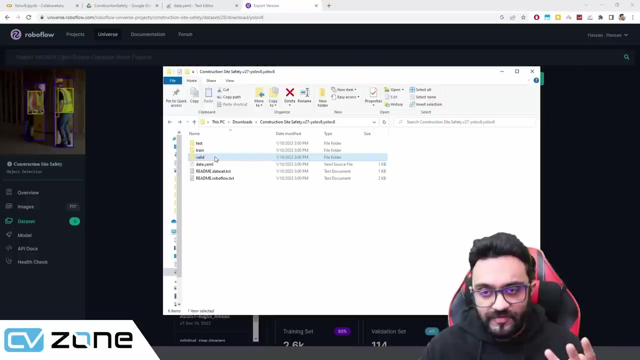 then you need to know what is the format in which the data set should be so in order to understand that we are going to open up this construction data set. so here is that data set. if you download it in a zip format and if you extract it, you will have test, train and valid. these are the three. 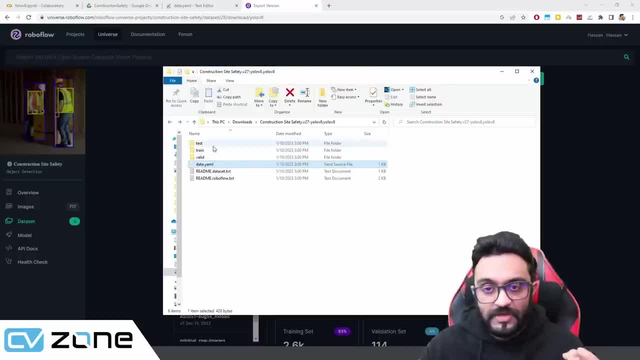 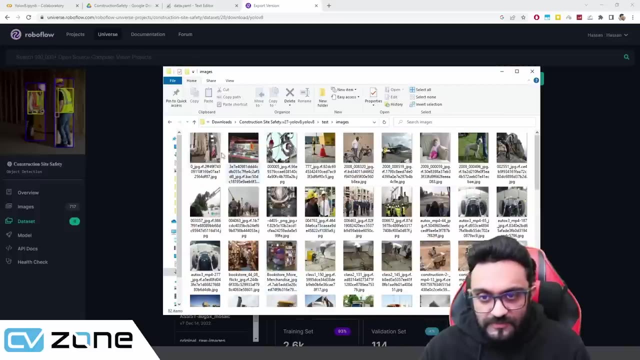 folders and then you will have a data file. so in the test file you will have images and labels. in the train file you will have images and labels and valid also images and labels. so if you open up test file, if you open up images, you will see all of these different images that 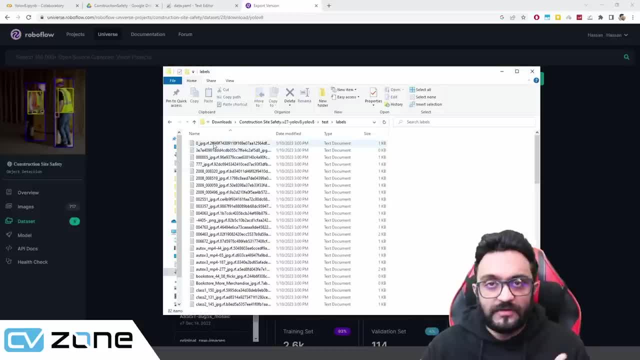 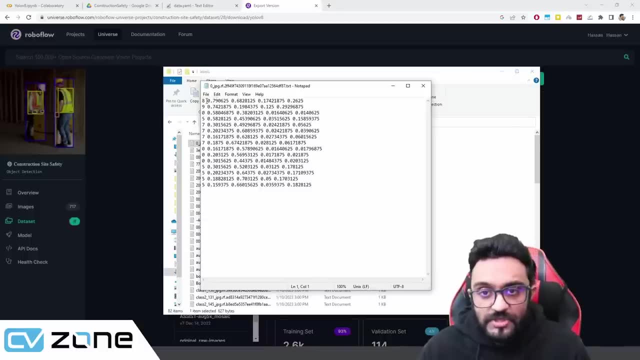 you have, and each image will have a corresponding um text file and in that text file you will see all the different classifications. so, for example, you will find the class number 8 at this at these coordinates. so these are basically normalized values. it means they are from 0 to 1 in between. 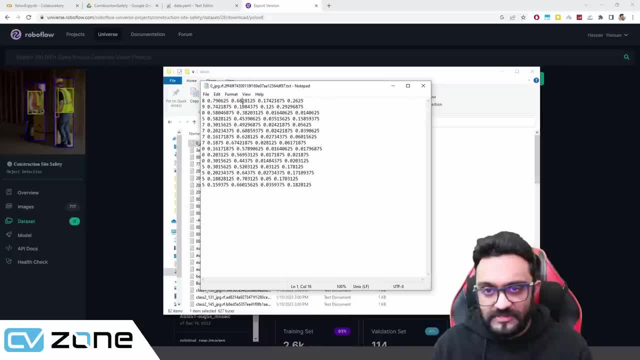 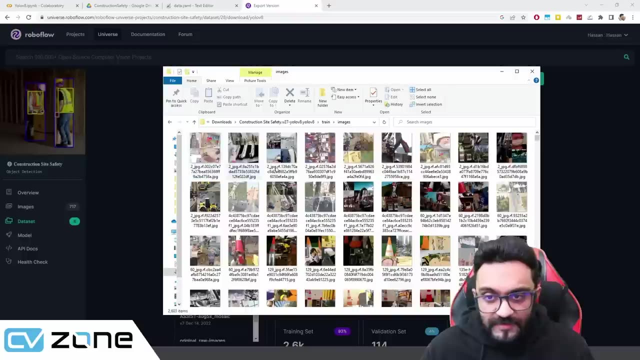 those values. so if you multiply it with the actual image size, you will get the pixel values. so these are the four values: x1, y1 and the width and the height. so you can find all these values for all these different classes, for all these different images. so if you go to, for example, train, you will find 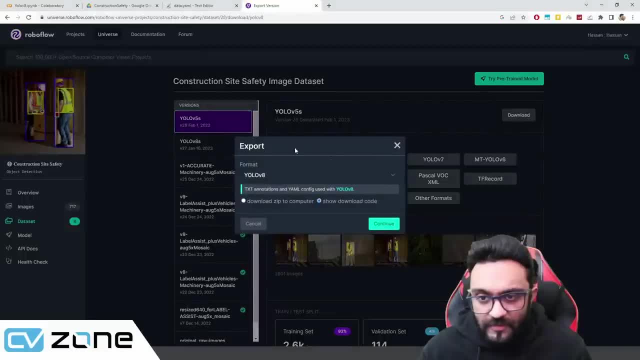 You can simply download it from here. So if you click on that and you can download zip to computer And you can press continue Now. by doing this, what will happen is that you will get the data set as well as the YAML file that will allow you to 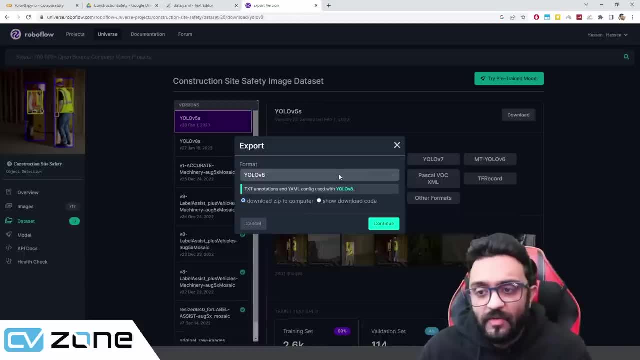 run with YOLO version 8.. Now, if you don't have a data set available online and if you wanted to create your own data set, then you actually need to know what is the format in which the data set should be. So, in order to understand that, 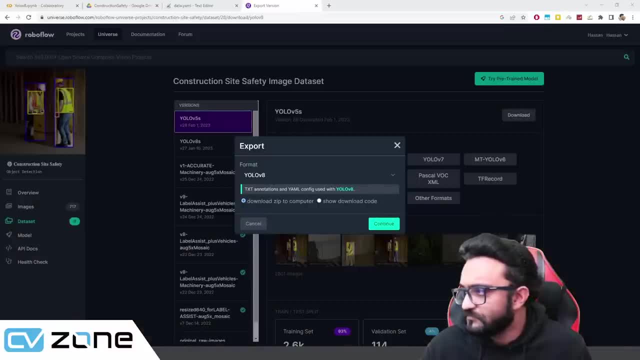 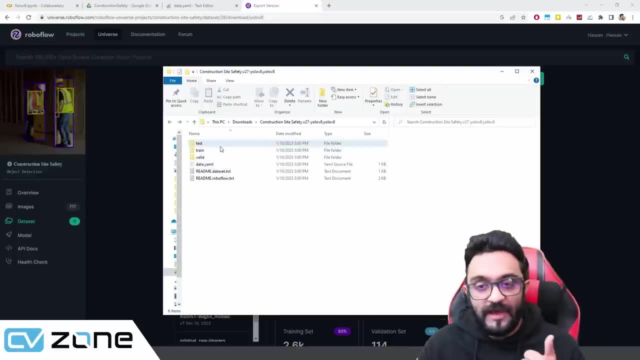 we are going to open up this construction data set. So here is that data set. If you download it in a zip format and if you extract it, you will have test train and valid. These are the three folders and then you will have a data file. 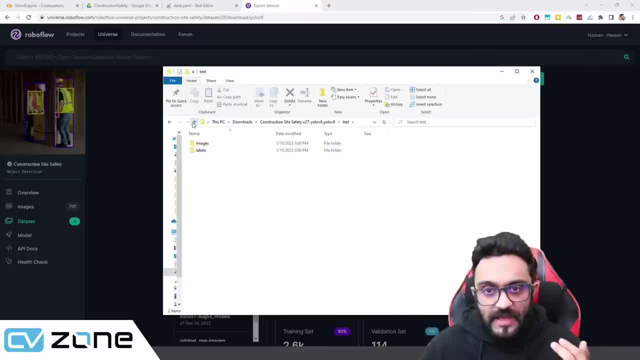 So in the test file you will have images and labels. In the train file you will have images and labels and valid also images and labels. So if you open up test file, if you open up images, you will see all of these different images that you have. 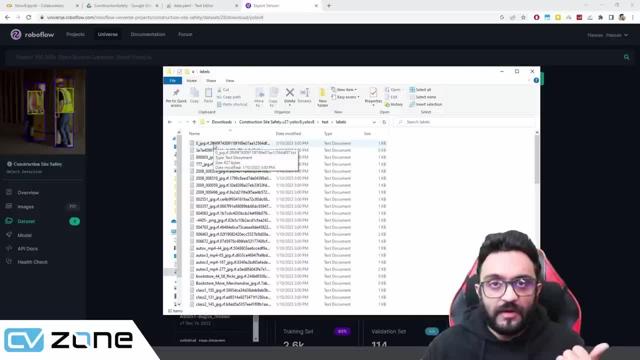 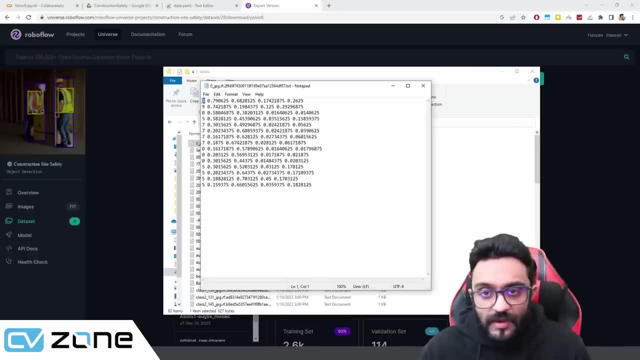 And each image will have a corresponding text file And in that text file you will see all the different classifications. So, for example, you will find the class number 8 at these coordinates. So these are basically normalized values. It means they are from 0 to 1. 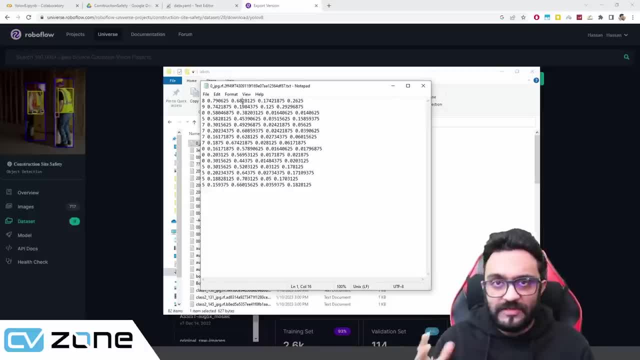 in between those values. If you multiply it with the actual image size, you will get the pixel values. So these are the four values: X1, Y1, and the width and the height. So you can find all these values for all these different classes. 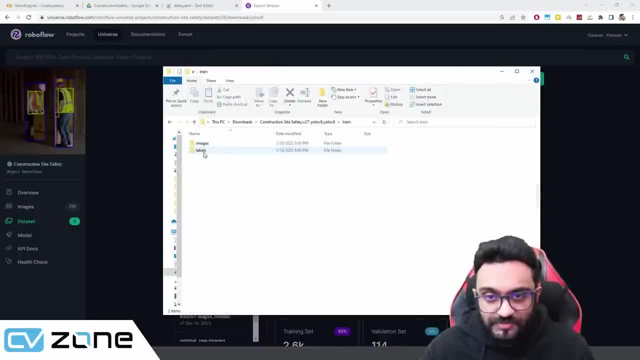 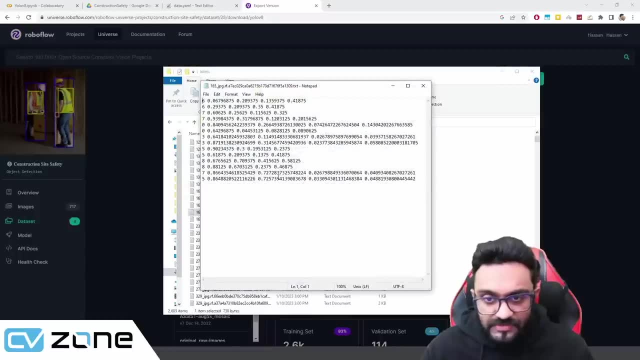 for all these different images. So if you go to, for example, train, you will find images and within these images you will find these labels, and within the labels you will find all these corresponding coordinates. So this is the file format. 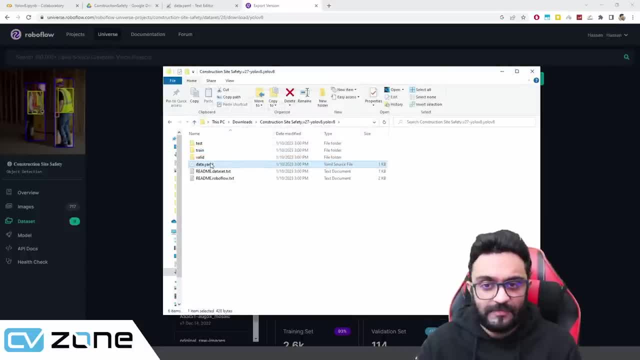 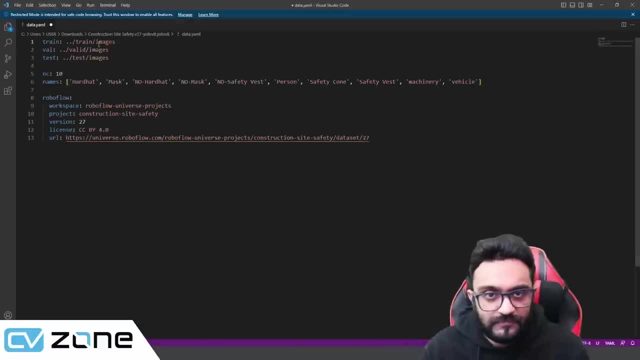 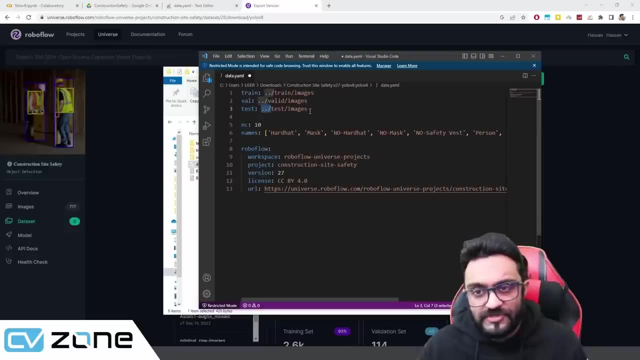 And then the important thing to have is the data. So the data YAML file, basically it gathers all this information into one place And if you open that up, you will see that you have train validation and test folders. So you have to mention where these folders are. 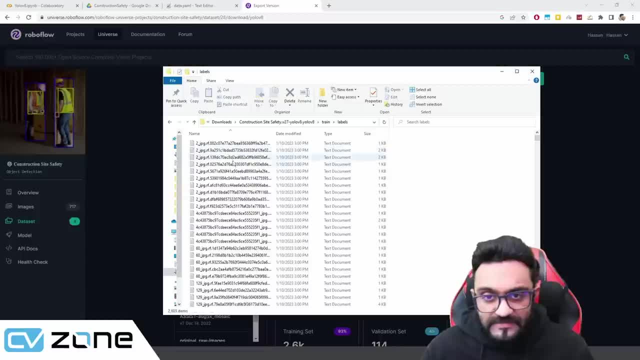 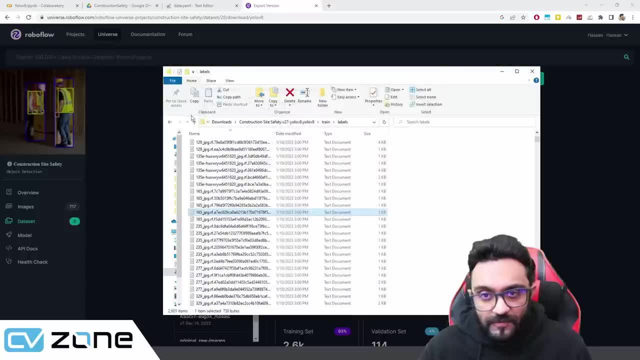 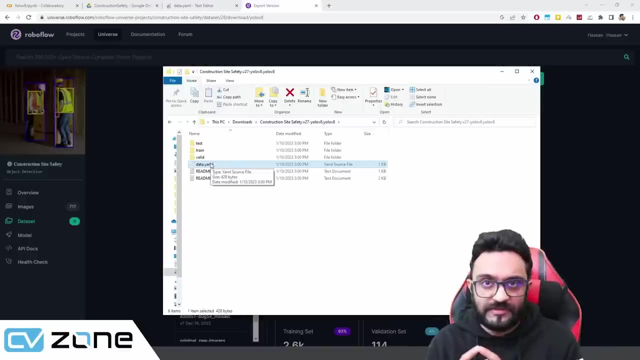 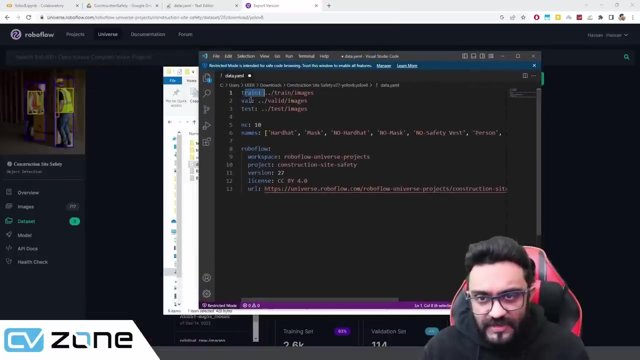 images and within these images you will uh find these labels and within the labels you will find all these corresponding uh coordinates. so this is the file format and then the data. so the data yaml file. basically it gathers all this information, uh, into one place and if you open that up, you will see that you have train validation and test folders. so you 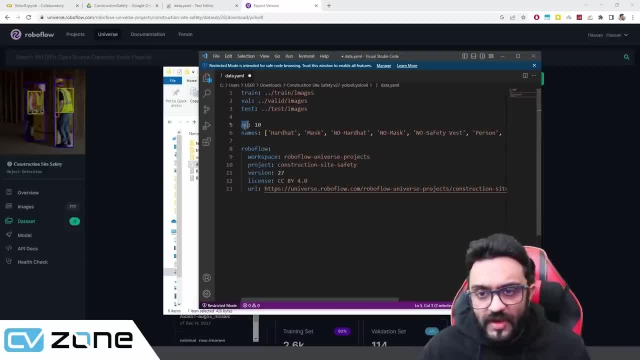 have to mention where these folders are. and then you have the number of classes- that is equal to 10 in this case- and you have the names of all these classes. so you have hardhat mask, no hardhat, no mask, safety vest person and safety cone, safety vest machinery, and so on. so, and the rest of this, 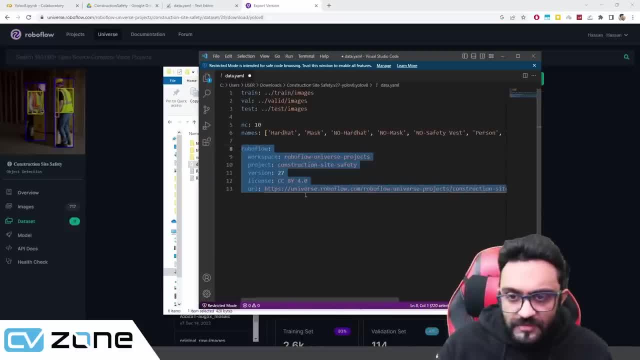 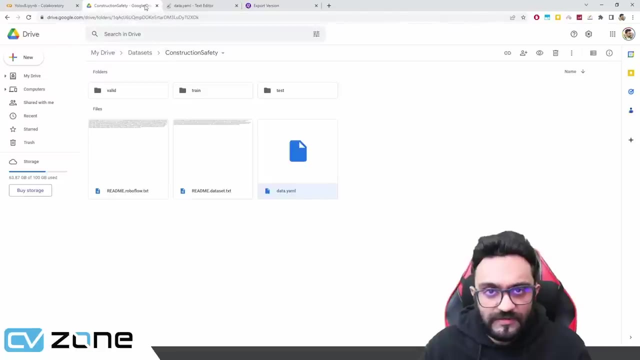 is not very important. this is just for the copyrights and all that. so what you can do is- and there is one more thing we need to add- when we bring it to google collab. so what we will do is we will copy all of this data to google drive. so if you go to my drive right now, i have a datasets. 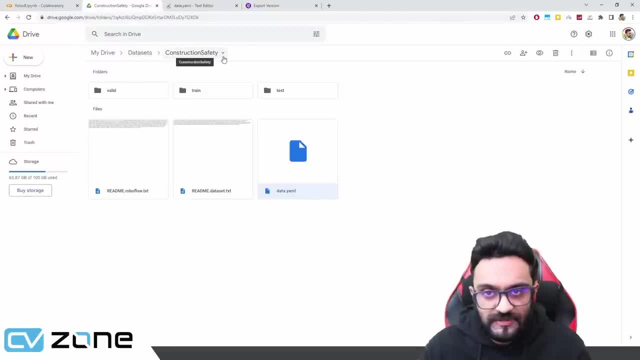 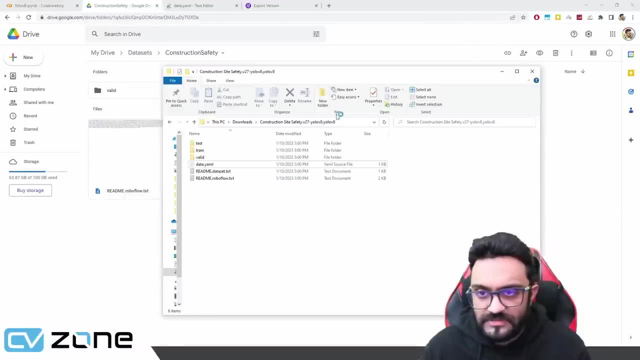 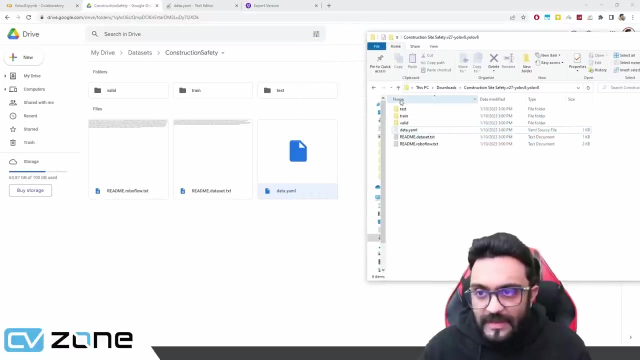 folder and within that dataset we have construction safety. So this is the exact same folder. You can see here, you can see here construction safety. So you have read me, read me. and then you have the datayaml and then you have the test train and valid. These are the three folders If you open that. 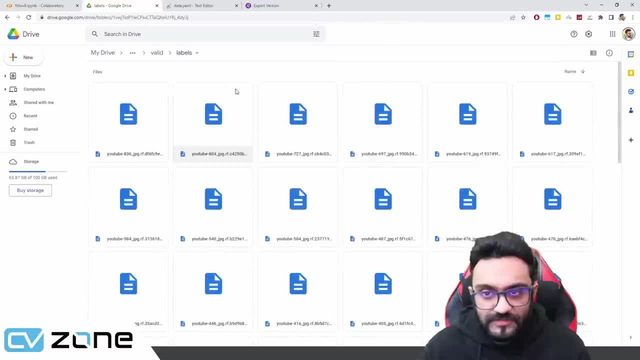 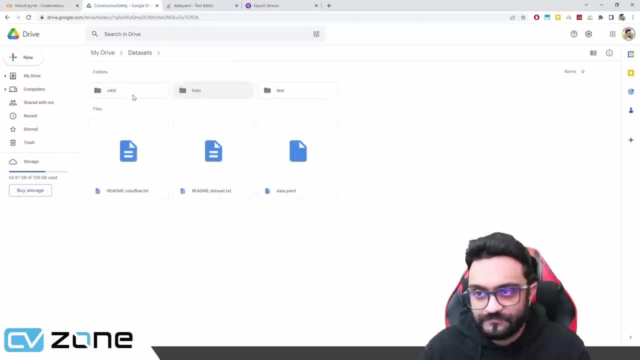 up. each folder will have labels and images inside of it. There you go. So this is the basic idea. If we go back to our data sets, construction safety and this is the main thing. So here, datayaml, we have to make some changes here. So here in the file you'll. 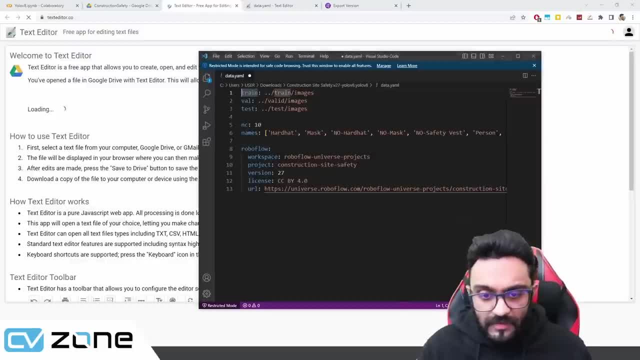 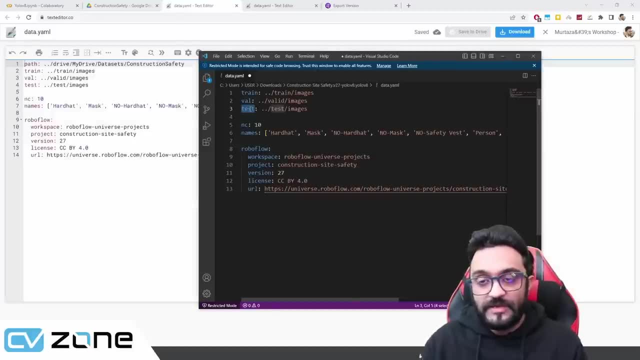 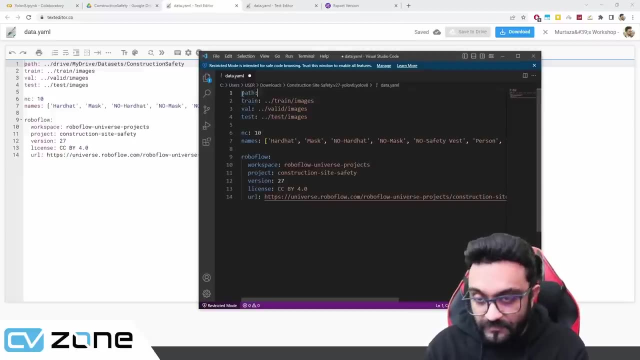 go to the text editor. If you remember, here our file contains train, validate and test. These are the folders that we have, but we need to define the path where these are present. So we have to write here: Okay, Path. And then we have to define the path in our drive, in the Google drive, So that 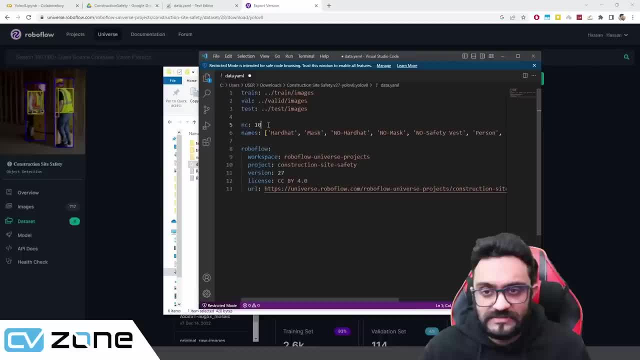 And then you have the number of classes- that is equal to 10 in this case- And you have the names of all these classes. So you have hard hat mask, no hard hat, no mask, no safety vest person and safety cone, safety vest machinery, and so on. 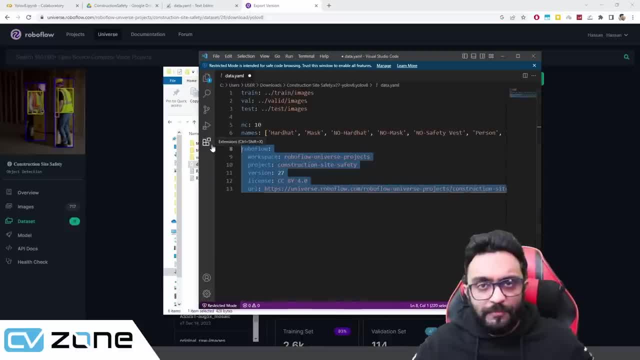 So- and the rest of this is not very important- This is just for the copyrights and all that. So what you can do is- and there's one more thing we need to add- when we bring it to Google Colab. So what we will do is: 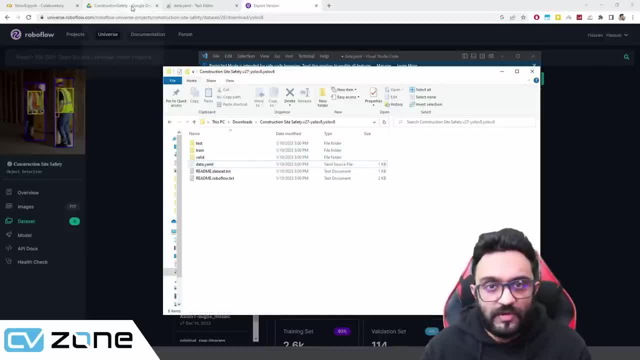 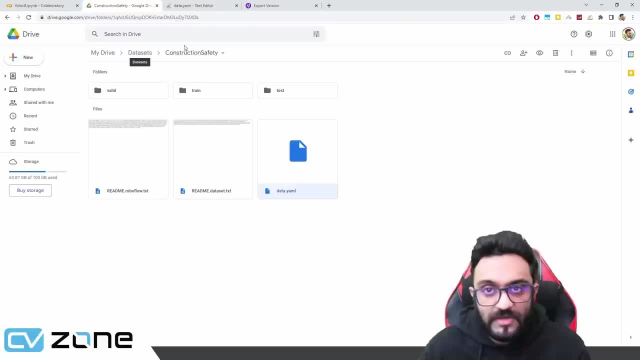 we will copy all of this data to Google Drive. So if you go to my drive right now, I have a data sets folder and within that data set we have construction safety. So this is the exact same thing as we did in the previous folder. 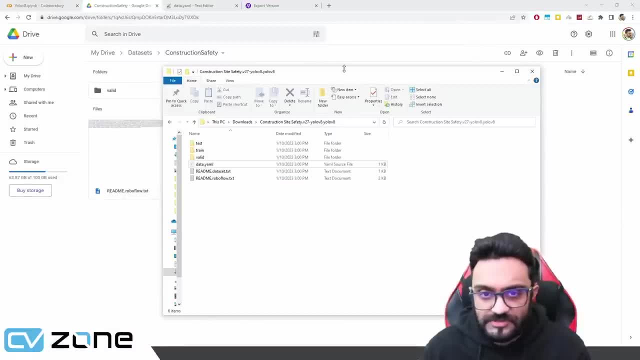 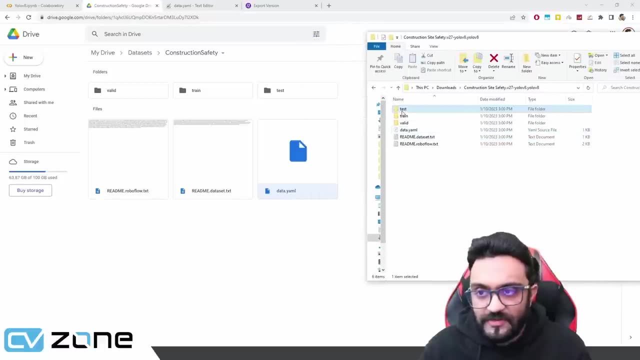 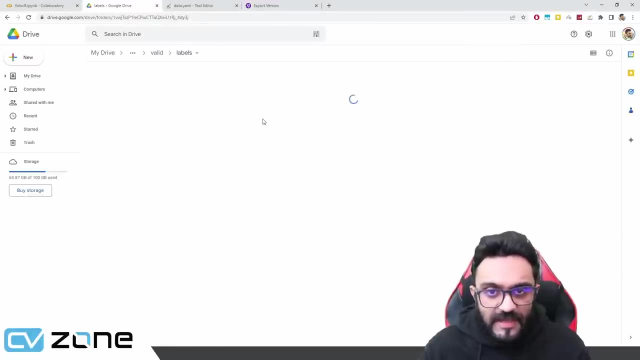 You can see here. you can see here construction safety. So you have read me, read me, and then you have the datayaml, and then you have the test, train and valid. These are the three folders. If you open that up, each folder will have labels. 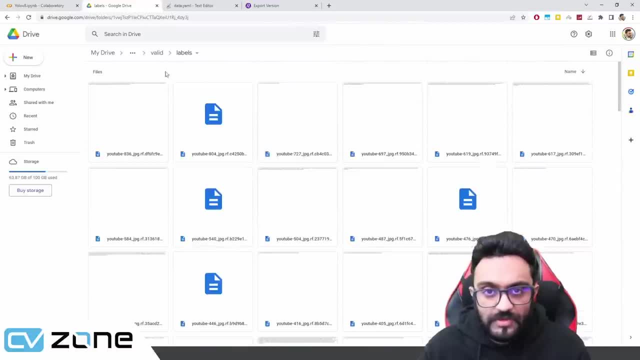 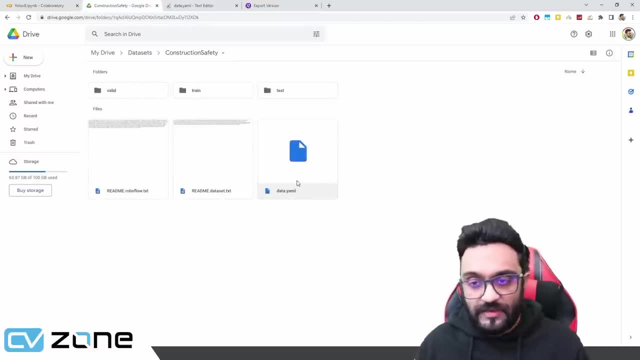 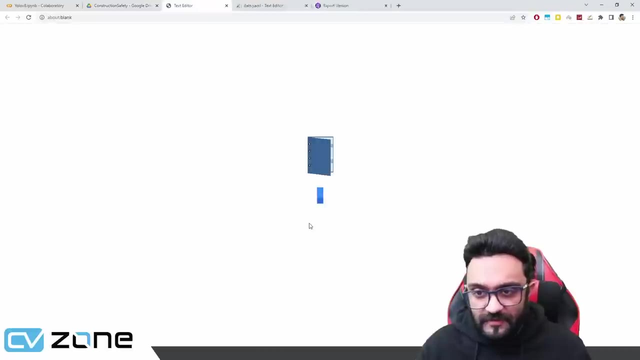 and images inside of it. There you go. So this is the basic idea. If we go back to our data sets, construction safety and this is the main thing. So here, datayaml, we have to make some changes here. So here in the file, 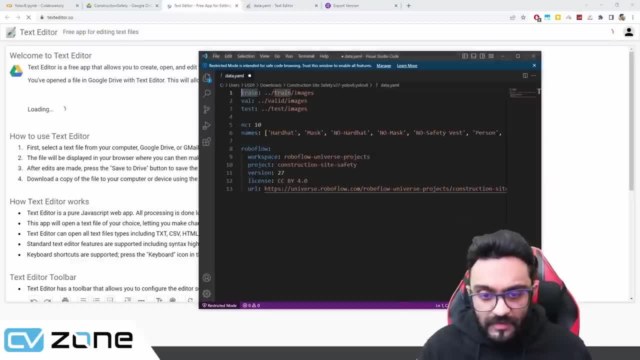 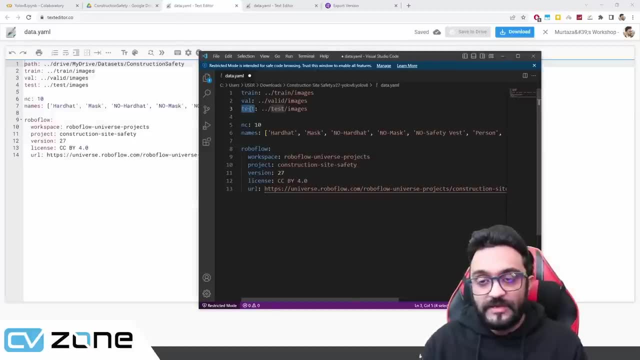 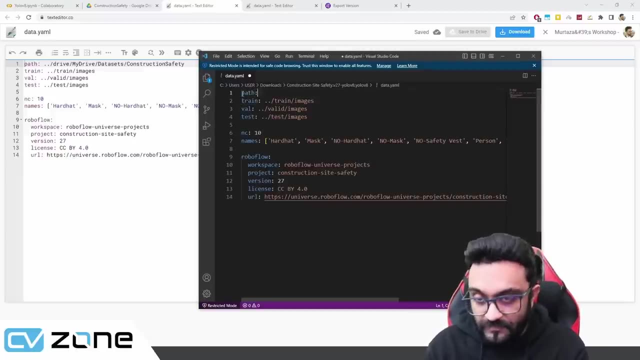 you'll go to the text editor. If you remember, here our file contains train validate and test. These are the folders that we have, but we need to define the path where these are present, So we have to write here: path. 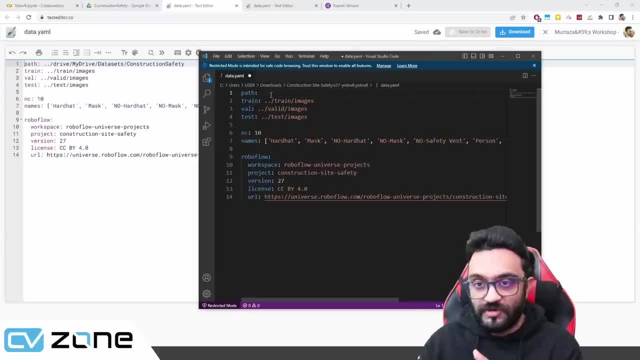 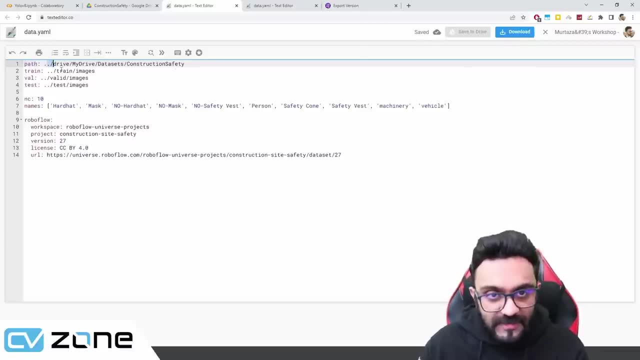 and then we have to define the path in our drive, in the Google drive. So that is what we have done here. So you will open that up and you will write here path and inside that you will write drive, my drive and then whatever your folder is. 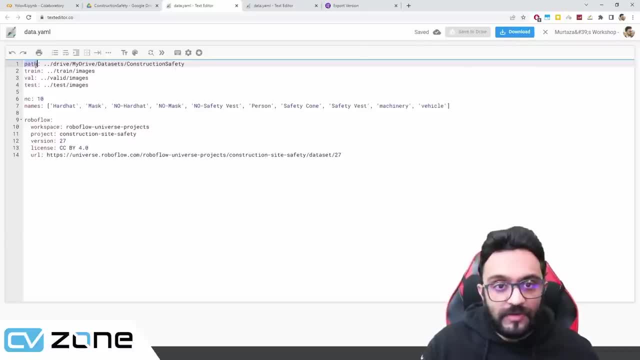 is what we have done here. So you will open that up and you will write here path And inside that you will write drive, my drive, and then whatever your folder is. So for me, inside my drive I have the folder data sets. Inside that I have the construction safety. 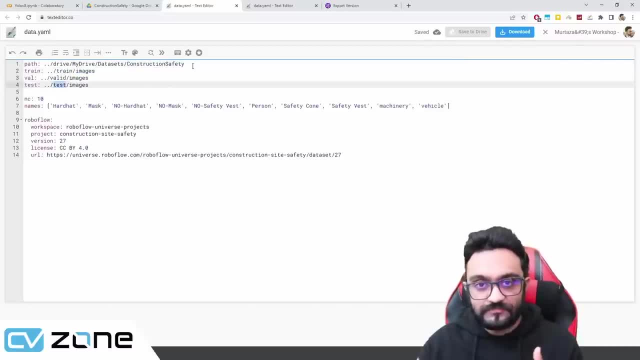 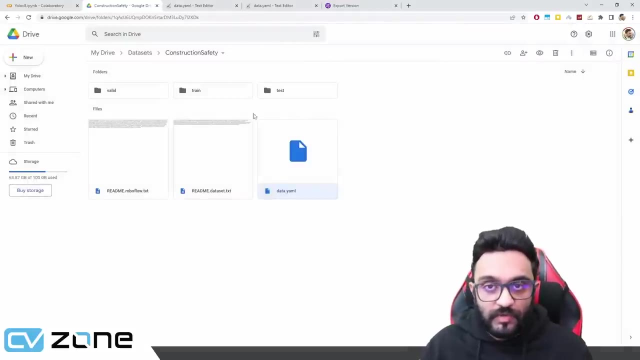 and inside that we have train, valid and test. So you have to write this path. The rest of it remains the same. So this is the basic idea of how you can upload your files to Google drive and how you can edit it to run it using Google collab. So that's the 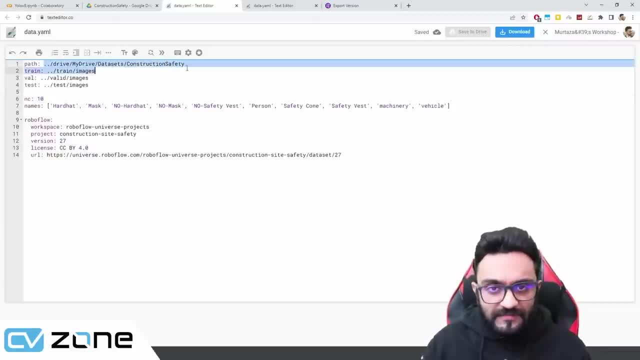 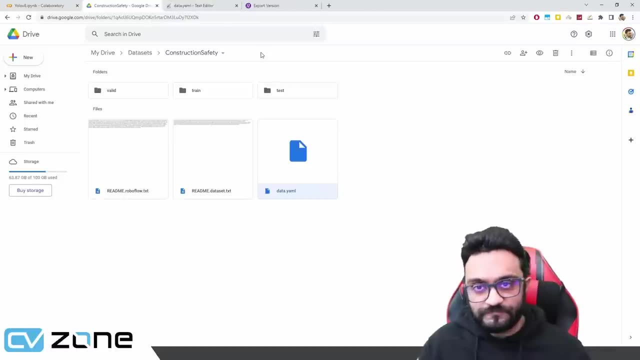 only thing you have to do, You have to write here path and you have to give in the path file. I will show you it. I will show you this again once we go into our Google drive. Okay, That's done. But what if you have your own images and you want to create this? if 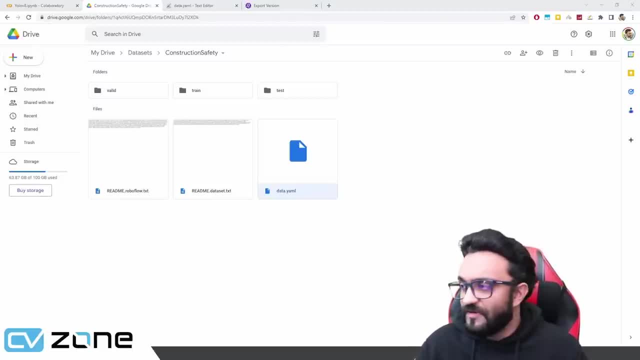 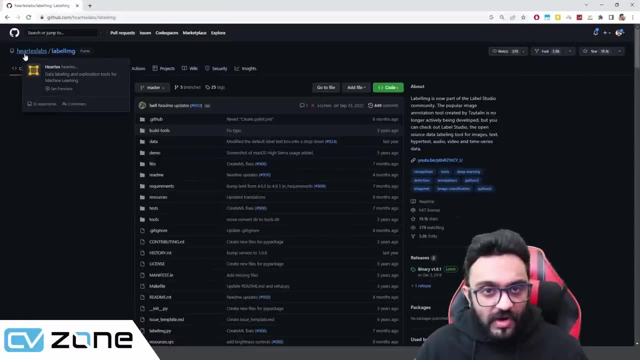 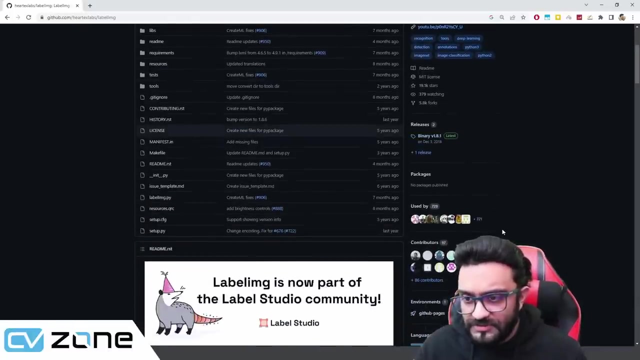 you want to label it. what can you do, then? Now to do that, we have a very famous label, IMG project. uh, that is available on GitHub and you can see it is by heart, uh, ex labs. So thanks to all the contributors and the creators. So what you have to do is you have 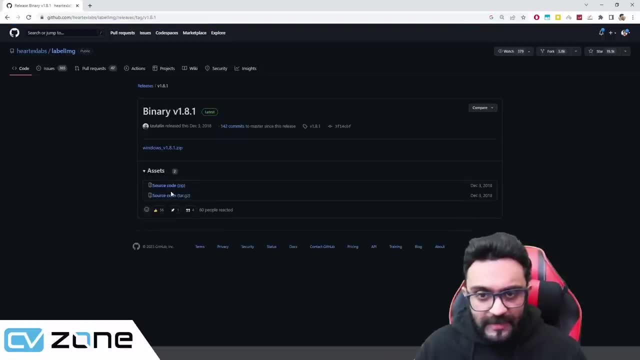 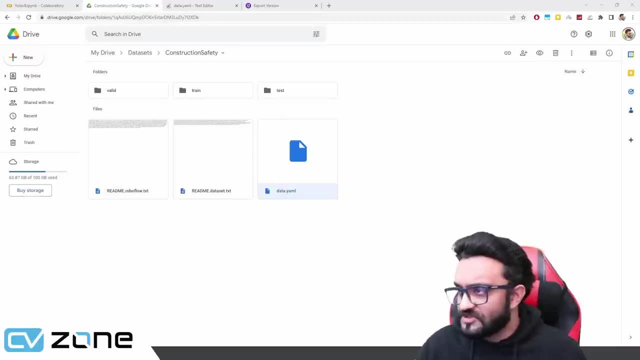 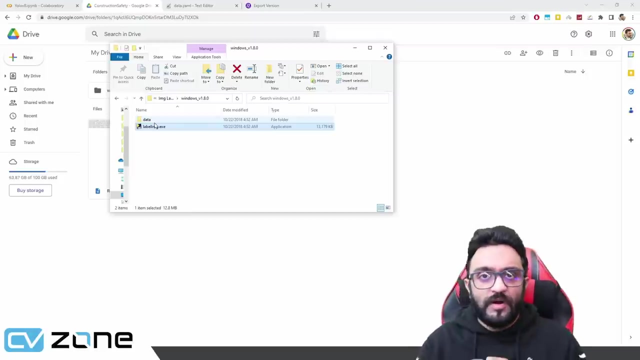 to go to the releases, You can click on binary and here you can download the zip file. Once you download the zip file, You can extract it, And once you extract that, you will get something like this label: image dot exe. Now, for example, if you were to uh find the poker chips, if you were. 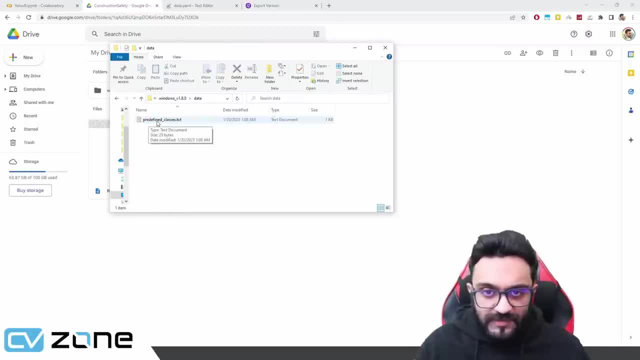 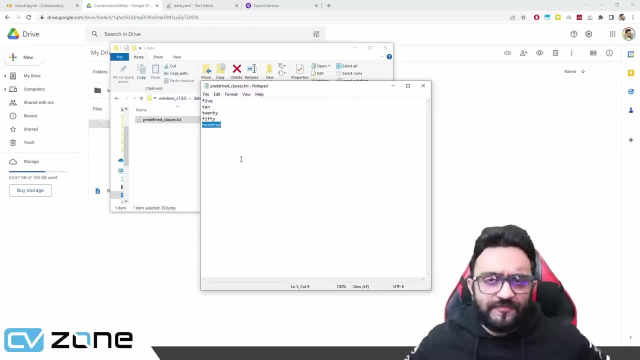 detecting poker chips. here in the data, you will go to predefined classes And here I have given five: 10,, 20,, 50, and a hundred. These are our five classes. in case of construction safety, We have hard hat, no hard hat, uh, um, a jacket, no jacket, and stuff like that. 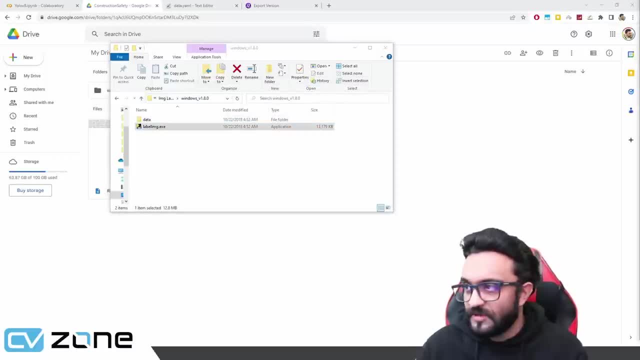 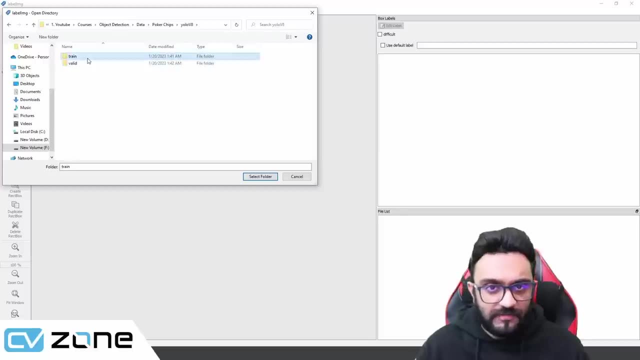 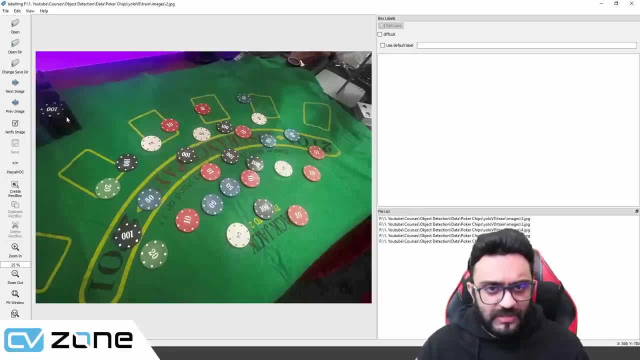 So you will do that and then you will go back and click on label image dot exe. Once you open that up, you can open directory. You can select, for example, these are the images I want to label, or whatever. So, for example, these are the images. So then you can press. 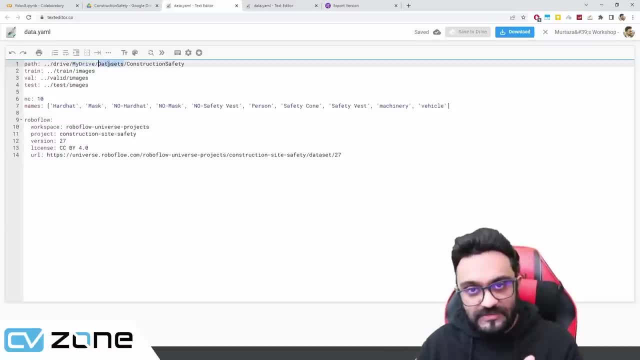 So for me, inside my drive I have the folder data sets, Inside that I have the construction safety And inside that we have train, valid and test. So you have to write this path. The rest of it remains the same. 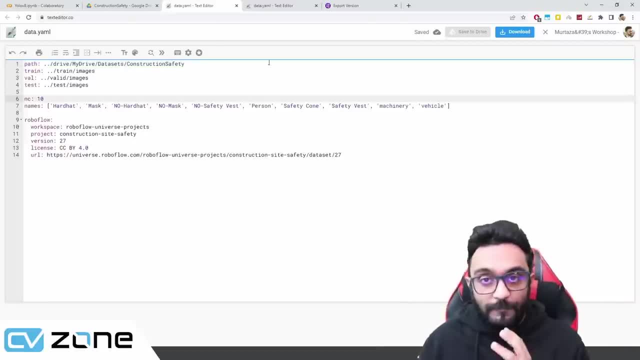 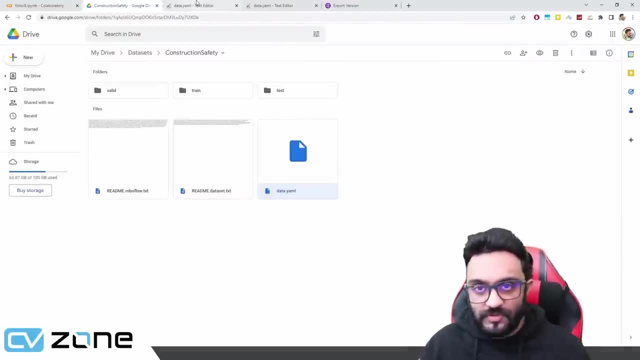 So this is the basic idea of how you can upload your files to Google Drive and how you can edit it to run it using Google Colab. So that's the only thing you have to do: You have to write here path and you have to give in the path file. 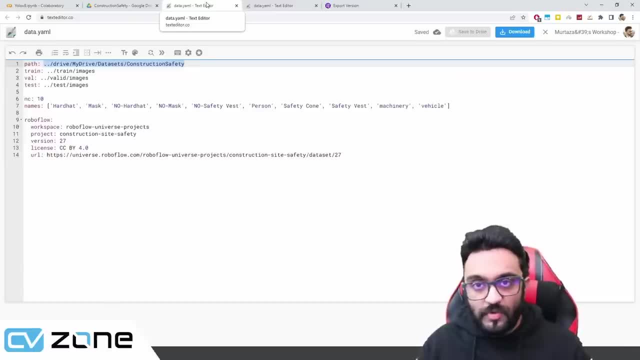 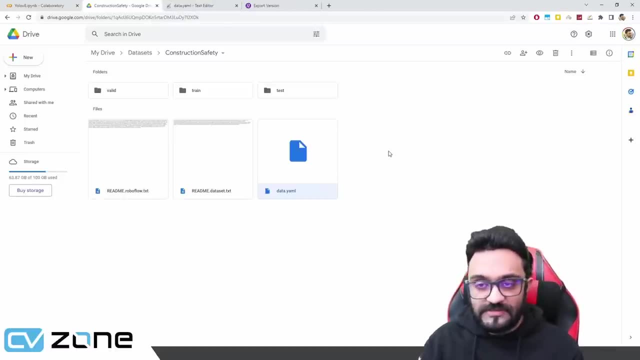 I will show you it. I will show you this again once we go into our Google Drive. Okay, that's done. But what if you have your own images and you want to create this, if you want to label it? what can you do then? 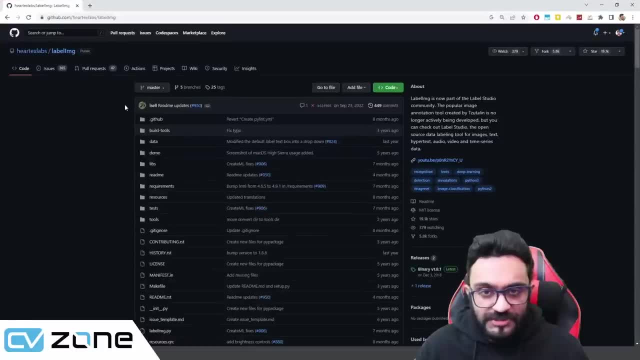 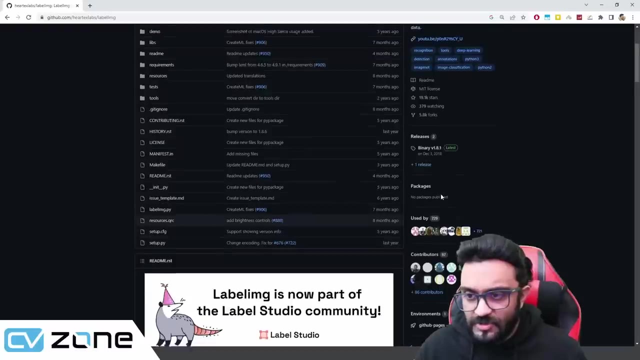 Now, to do that, you have a very famous label, IMG project- that is available on GitHub and you can see it is by Heart EX Labs. So thanks to all the contributors and the creators. So what you have to do is you have to go to the releases. 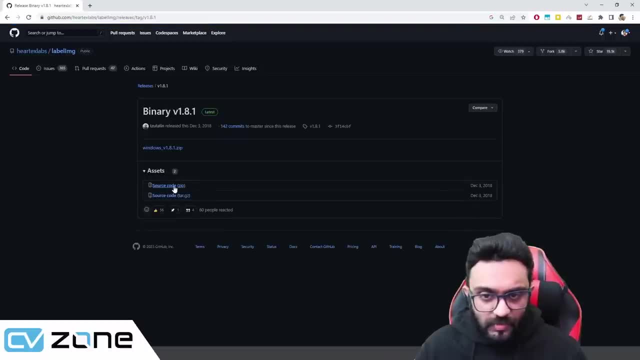 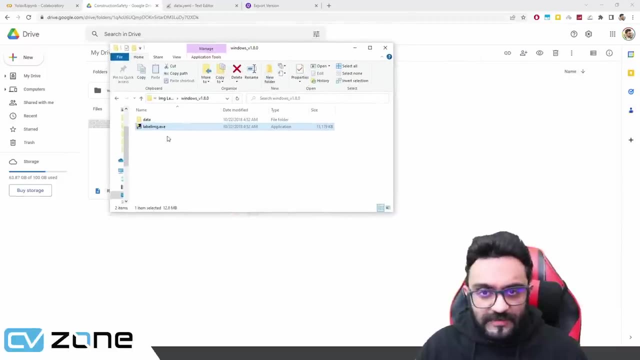 You can click on binary and here you can download the zip file. Once you download the zip file, you can extract it, And once you extract that, you will get something like this label: imageexe. Now, for example, if you were to find the poker chips, 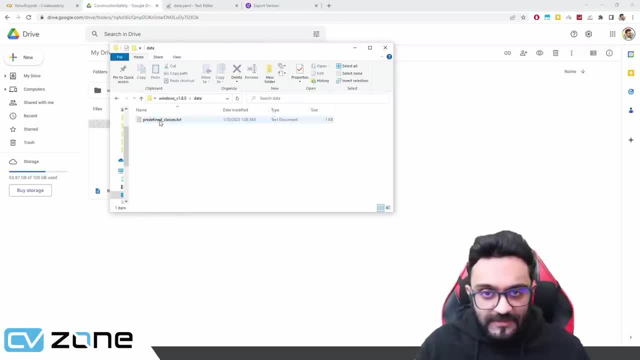 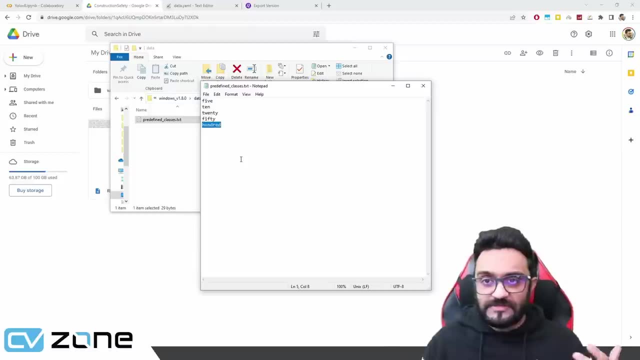 if you were detecting poker chips here in the data, you will go to predefined classes, and here I have given 5,, 10,, 20,, 50 and 100.. These are our five classes. In case of construction safety, we have hard hat, no hard hat. 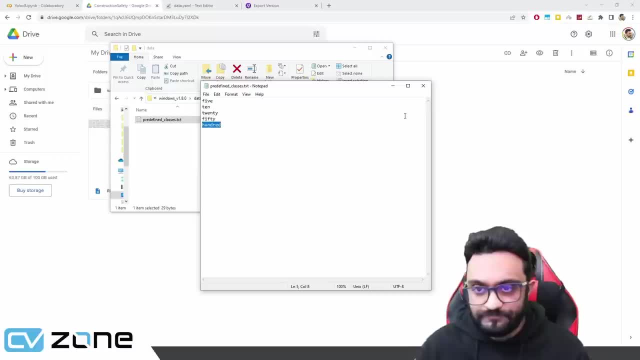 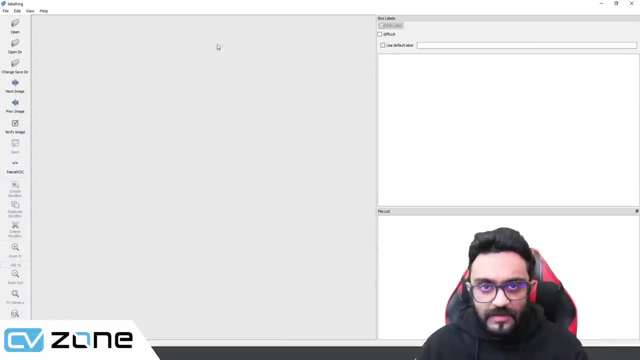 a jacket, no jacket and stuff like that. So you will do that and then you will go back and click on label imageexe. Once you open that up, you can open directory. You can select, for example: these are the images. 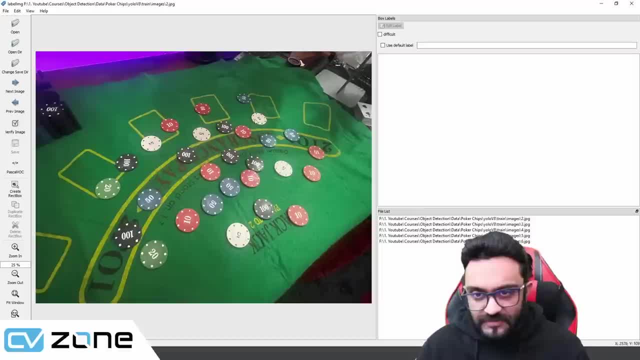 I want to label or whatever. So, for example, these are the images. So then you can press R- sorry, you can press W to actually select And you can define: for example: this is class number five and hit OK. So this will create this label. 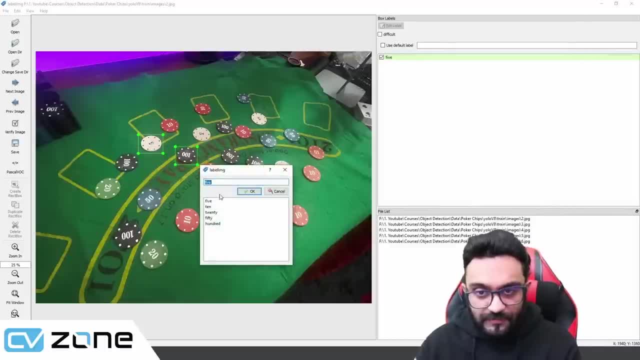 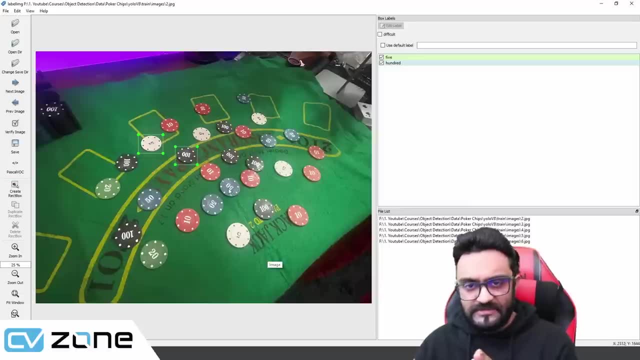 Then you will press W again, and this is, for example, for 100,. you will click on 100 and press OK. Now the easy way to do this is do all the fives first, then all the 10s, then all the 100s. 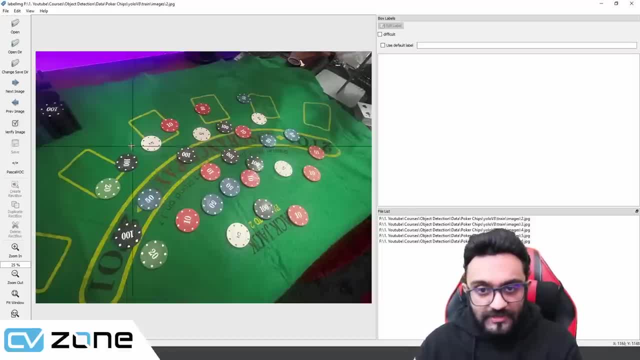 R. uh sorry. you can press W to actually select and you can define, for example, this is class number five and hit Okay, So this will create this label. Then you'll press W again, And this is for example for: 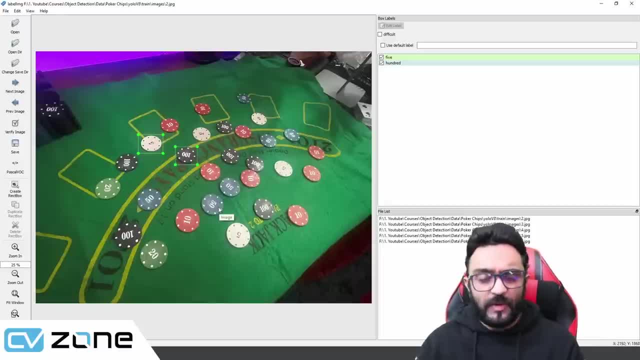 a hundred, you'll click on a hundred and press Okay. Now the easy way to do this is do all the fives first, then all the tens, then all the hundreds, all the twenties, things like that, And once you want to export, you will make sure that this here it's Yolo format. 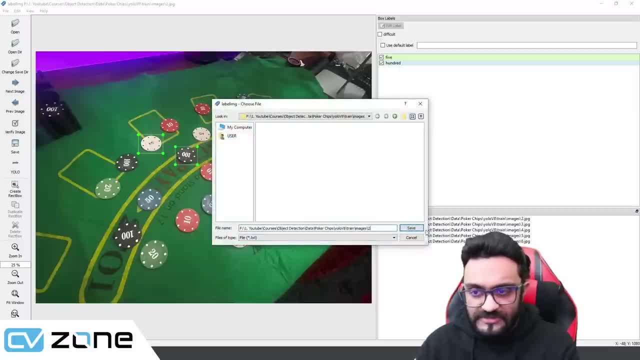 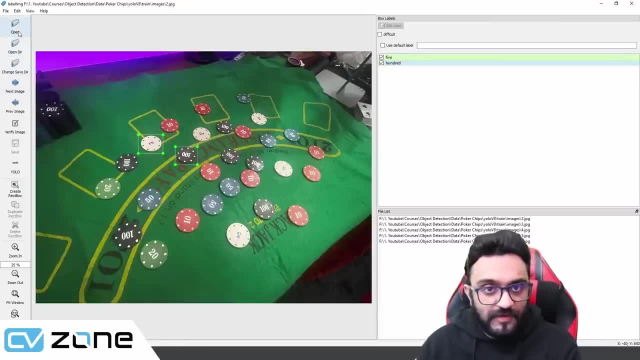 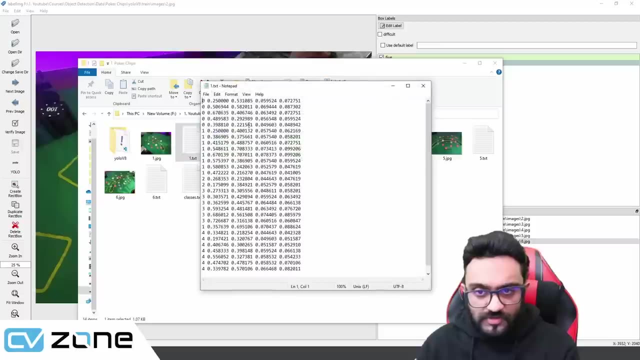 and you will click on save and here it will save the file. If you hit save, it will save the file. Uh, in that Location. So if we open the directory, so here we have this directory, So let's say we save this one. So if we open that up you can see it's the same format. So zero is for. 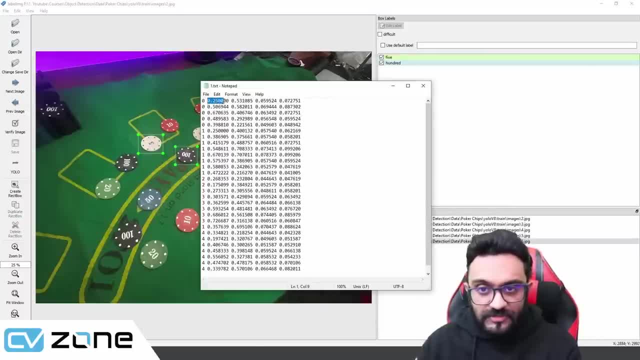 I think five, uh, that's for five, Uh. so the location of this is at this point. So these are the coordinates for that. And then class number one is present here, Uh, class number two, uh, you have here, and so on. So this is how you can label these images. So, 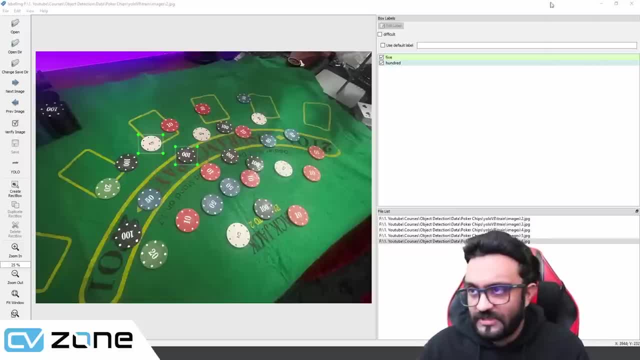 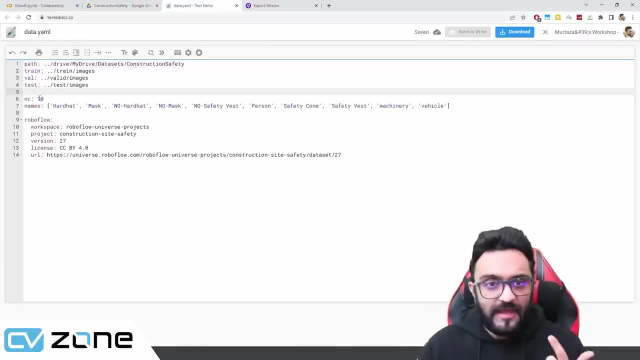 the YAML file you can create yourself. As I've mentioned. it's very easy to do. Uh, all you have to do is you have to write the path, the train, the validation and the test folders, And then you have to write number of classes and the names of the classes. That's it, And 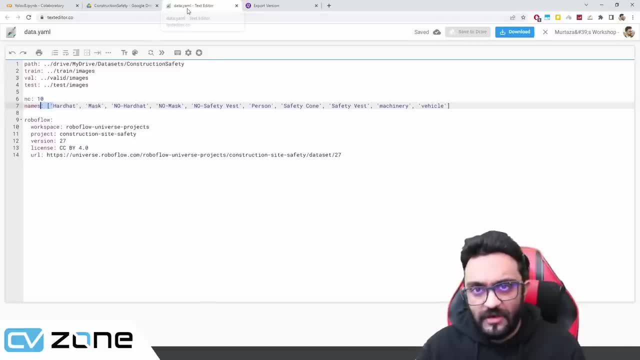 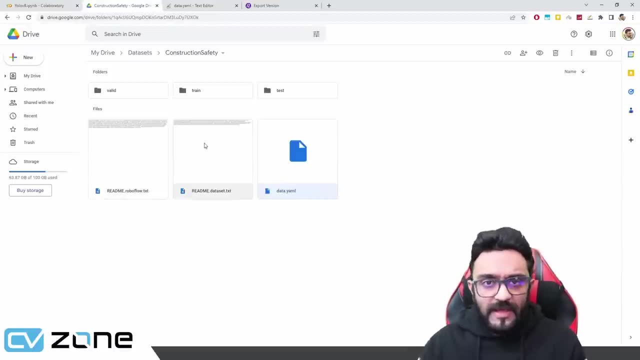 you will save the file. It's a simple text file, basically uh, by the format dot, Y, M, L. So once you have done that, now we can simply go ahead and upload everything, Uh, for example, in this case, uh, we can download it from here. 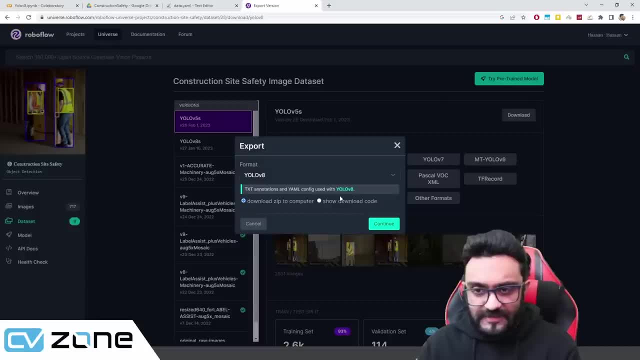 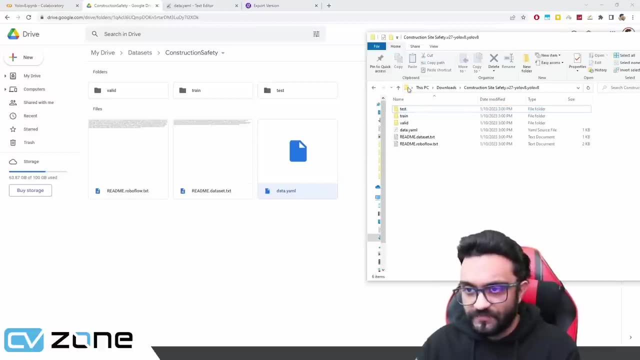 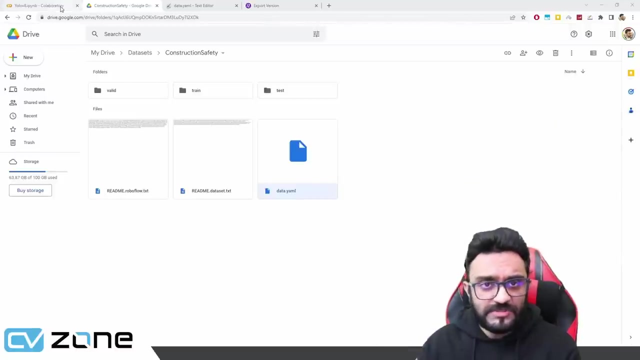 The um construction safety image data set And once we have that, we can upload it to our Google drive. Once Google drive- uh, these are the basically the files- we'll select all and drag, but I will not do that now, Then once you have that, because it will take. 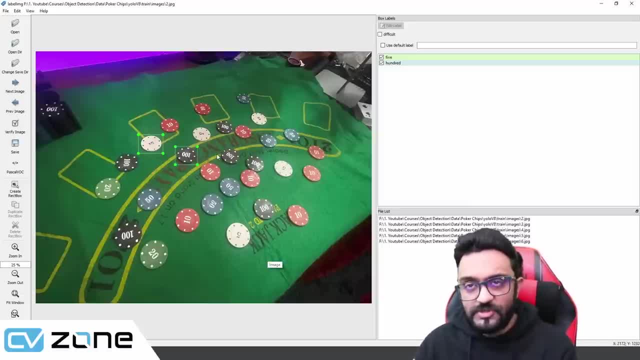 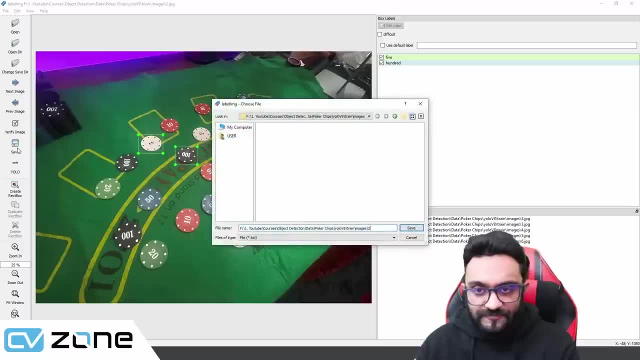 all the 20s, things like that- And once you want to export, you will make sure that this- here it's YOLO format and you will click on save And here it will save the file, If you hit save. 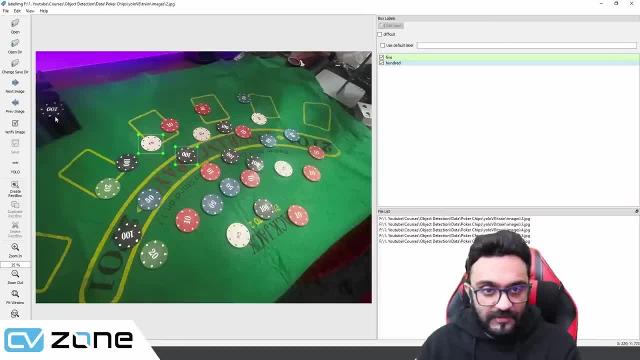 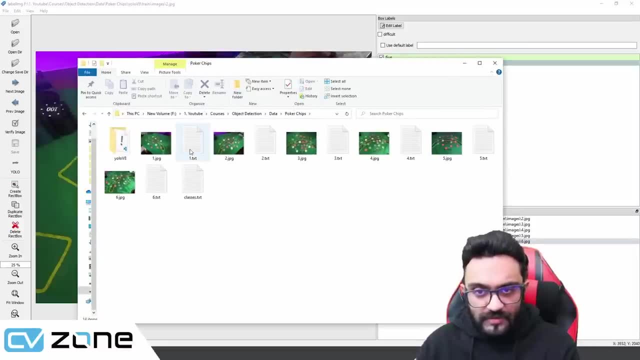 it will save the file in that location. So if we open the directory, so here we have this directory, So let's say we save this one. So if we open that up you can see it's the same format. So zero is for. 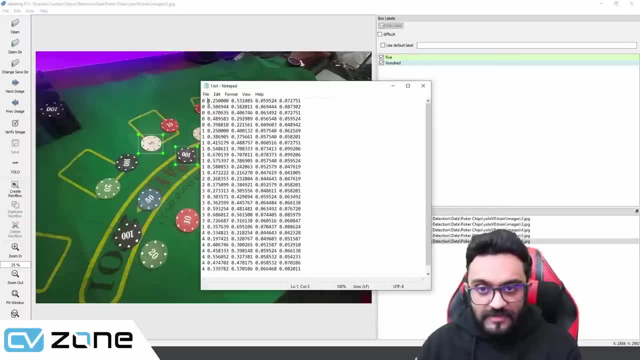 I think five, That's for five. So the location of this is at this point. So these are the coordinates for that. Then class number one is present here, Class number two you have here, and so on. So this is how you can label these images. 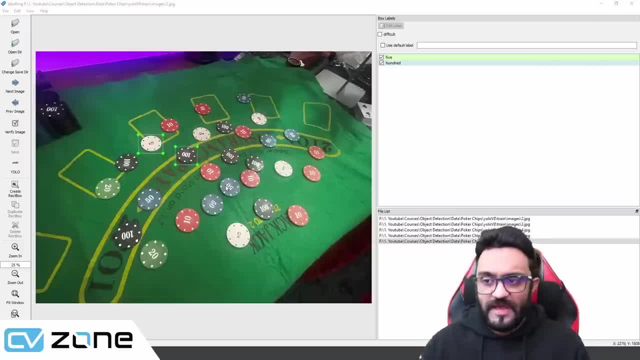 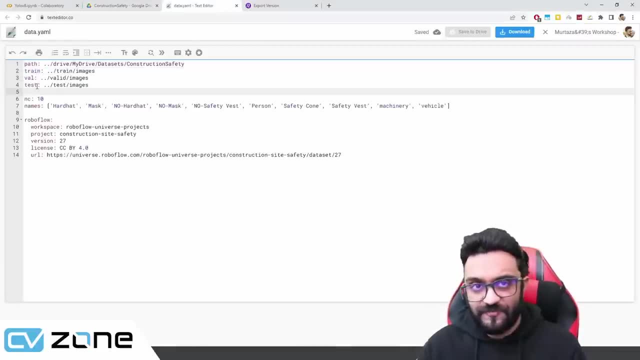 So the datayml file you can create yourself. As I've mentioned, it's very easy to do. All you have to do is you have to write the path, the train, the validation and the test folders, And then you have to write. 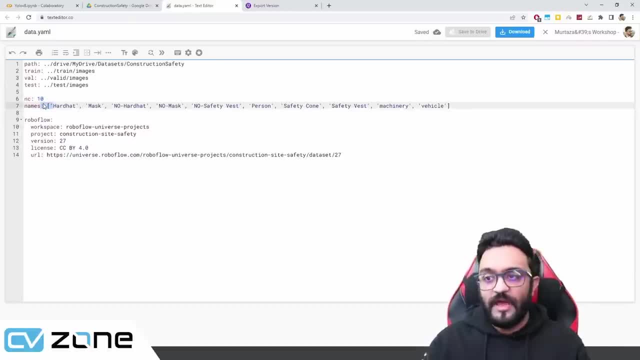 number of classes and the names of the classes. That's it, And you will save the file. It's a simple text file, basically by the formatyml, So once you have done that, now we can simply go ahead and upload everything. 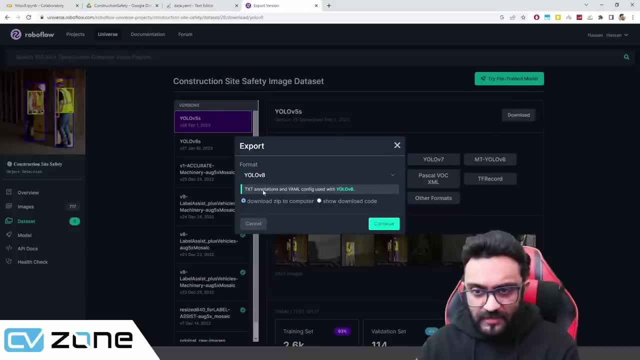 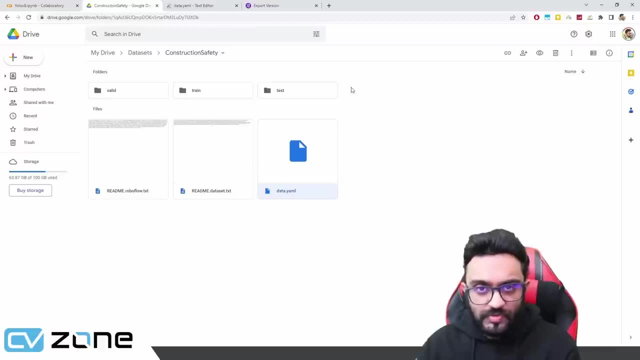 For example, in this case we can download it from here- The construction safety image data set- And once we have that, we can upload it to our Google Drive. Once Google Drive, these are basically the files. We'll select all and drag. 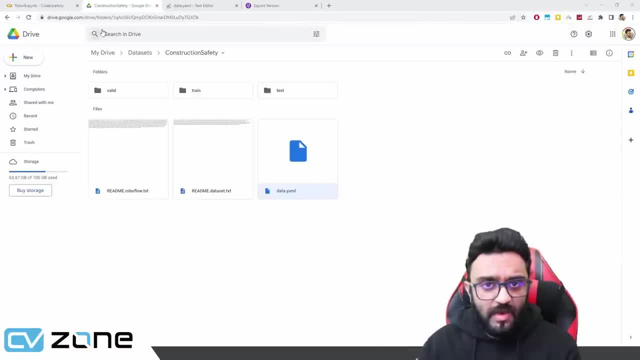 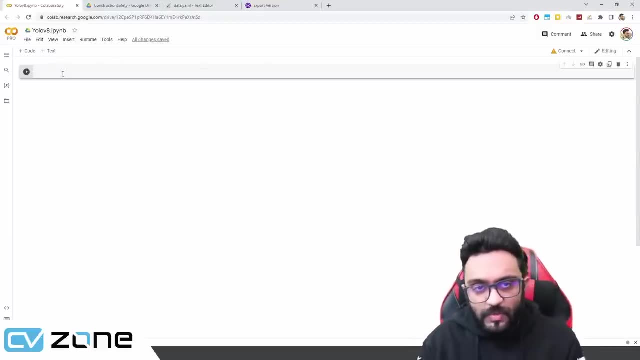 but I will not do that now, Then once you have that, because it will take some time- then we have Yolo version eight. This is our Google collab file. So what we have to do is, first of all, you will go to folder. 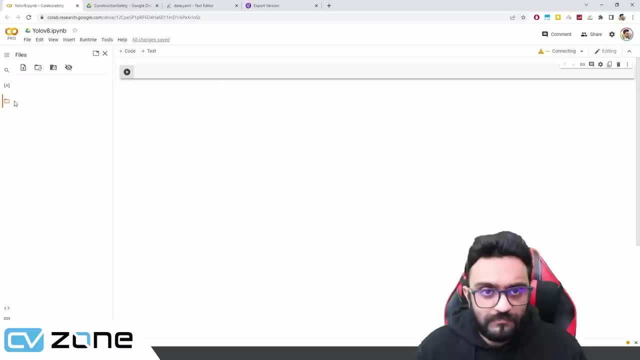 and here in the folder you will see that we have an option here to connect your drive- mount drive. So make sure you click on that and it will mount your drive. It will ask you to give access. Once you give the access, 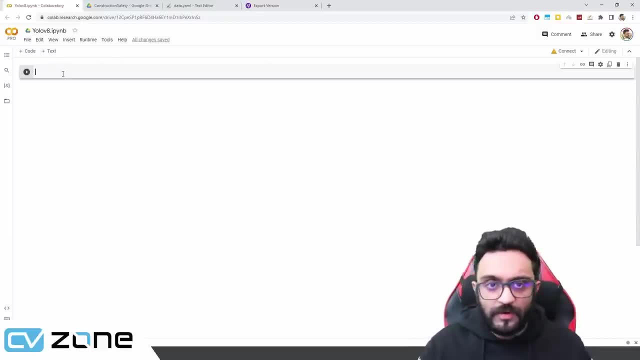 some time. then we have Yolo version eight. This is our Google collab file. So what we have to do is, uh, first of all, you will go to folder and here in the folder we have, you will see that we have an option here to connect your drive mount drive. So make. 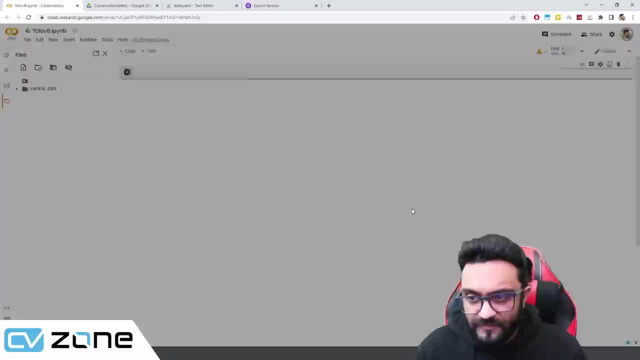 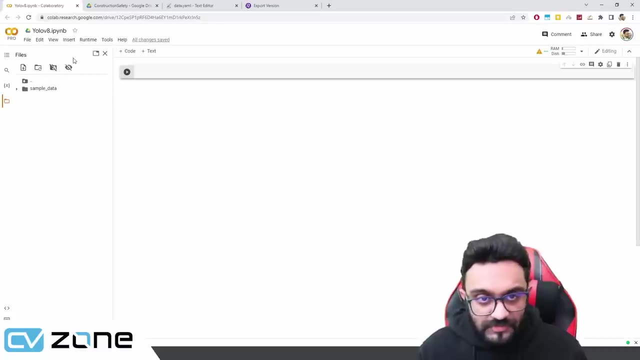 sure you click on that and it will mount your drive. It will ask you to give access. Once you give the access, this will have a cross. It means it has been mounted. So if you go back and you click on content, not the bin the content- uh, I think it's still loading. 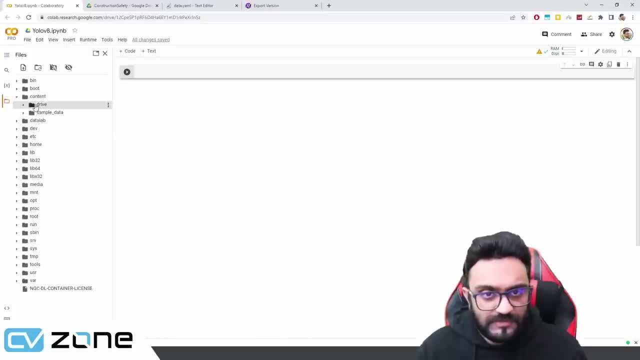 Let's wait for it. Content: There you go. So now you have the drive. So if I click on the drive and then my drive, and then I can go to data sets, and inside the data sets we have construction safety, and inside construction safety we have test train, valid and datayaml. 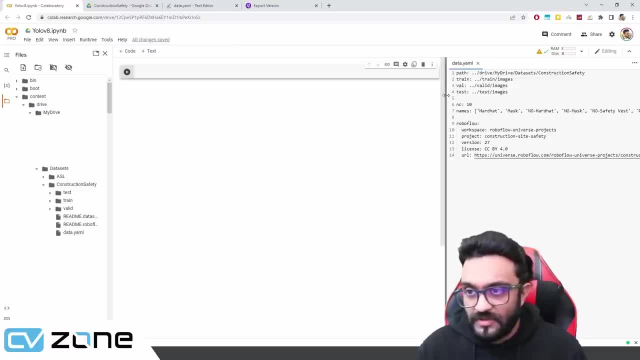 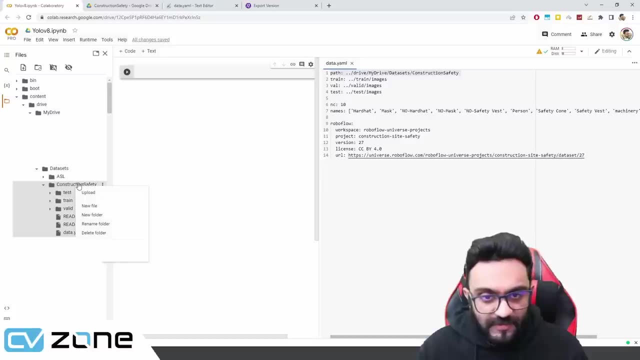 If you double click, that this is what we have to make sure. So this path should be correct. So if I right click here, let's say construction safety, If I right click and I can say copy path and then I can paste it here, So this is the path that we need to have content drive. 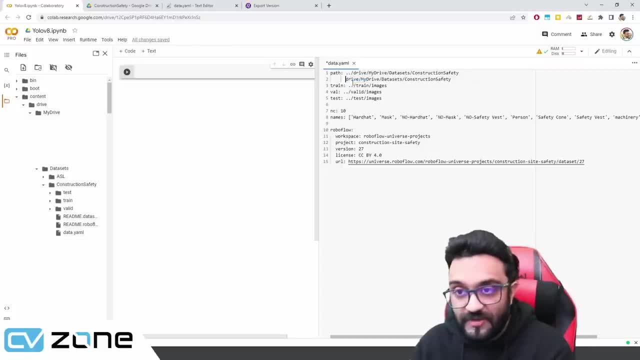 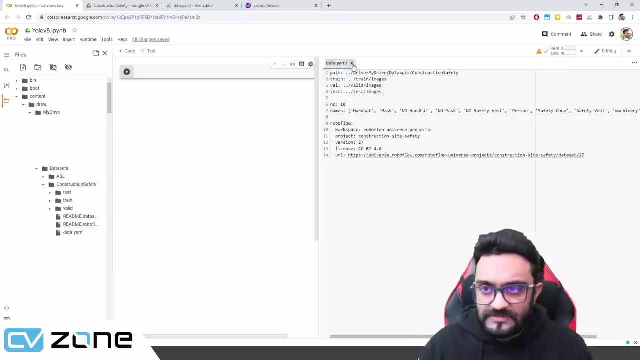 So after content, uh, we need the drive. So from drive we are going to write my drive data sets, construction safety. So this is what we need, So we need to make sure it is at the path over here. So once that is done, we can close this and we can close all of that, And now we can start. 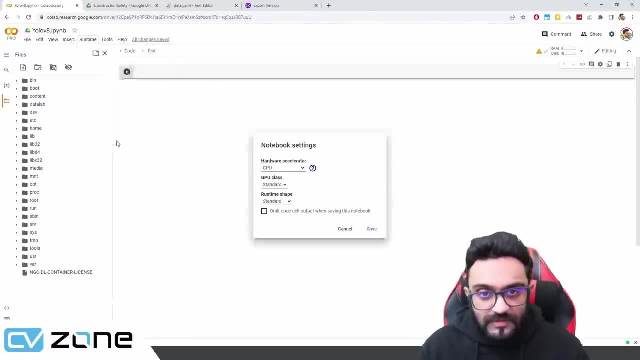 writing some code again. just make sure the runtime is GPU and we will save this. And over here we are going to first of all write a few lines of code. That's it. We will need five lines of code and we will have our Yolo running and we will have our Yolo training. 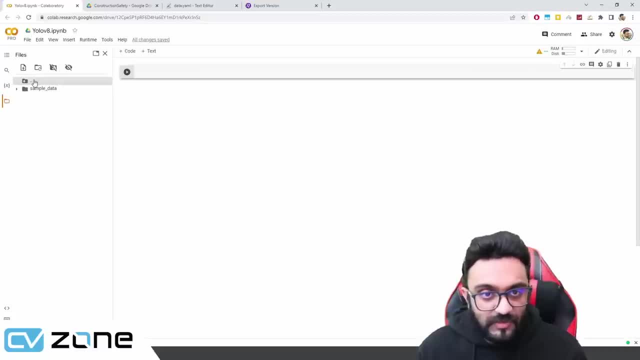 this will have a cross. It means it has been mounted. So if you go back and you click on content, not the bin, the content, I think it's still loading. Let's wait for it. Content- There you go. So now you have the drive. 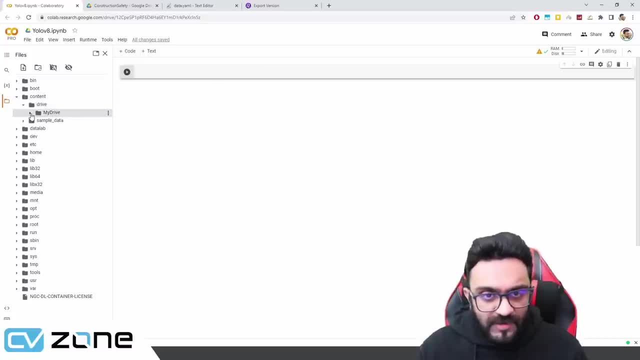 So if I click on the drive and then my drive and then I can go to data sets And inside the data sets we have construction safety And inside construction safety we have test strain valid and data dot YML, If you double click that 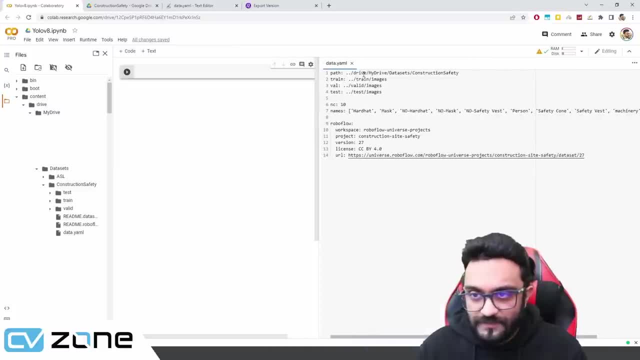 this is what we have to make sure. So this path should be correct. So if I right click here, let's say construction safety, If I right click and I can say copy path and then I can paste it here. So this is the path. 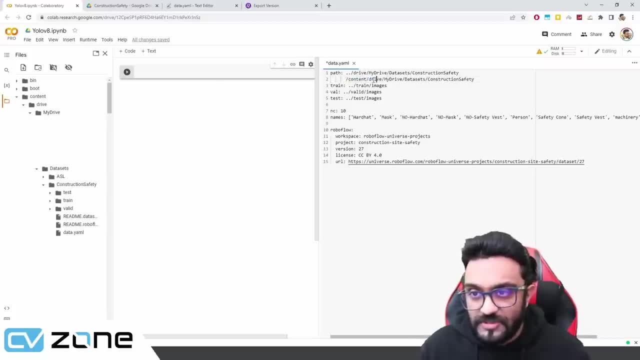 that we need to have Content drive. So after content, we need the drive. So from drive we are going to write: my drive data sets, construction safety, So this is what we need. So we need to make sure it is at the path over here. 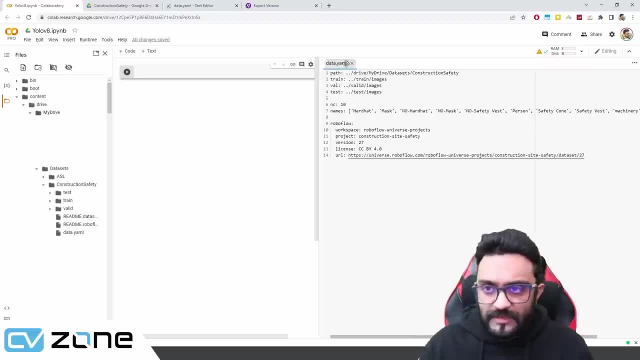 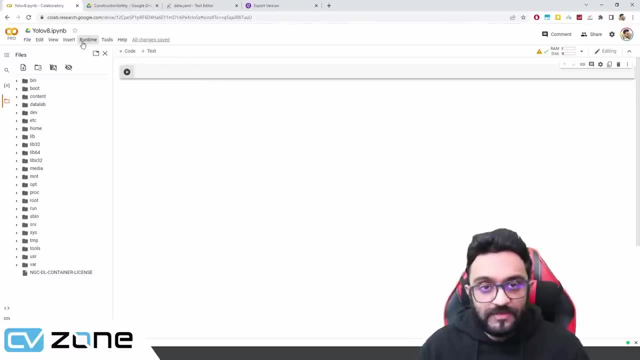 So once that is done, we can close this and we can close all of that, And now we can start writing some code Again. just make sure the runtime is GPU And we will save this. And over here we are going to. 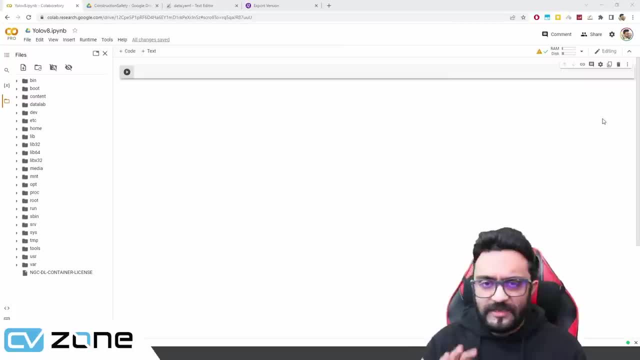 first of all write a few lines of code. That's it. We will need five lines of code and we will have our YOLO running and we will have our YOLO training. So first of all, we need to check whether we are. 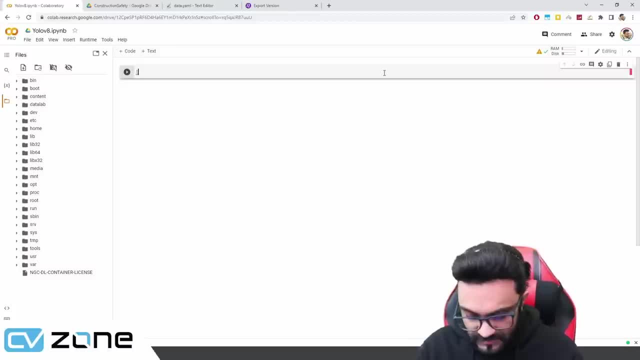 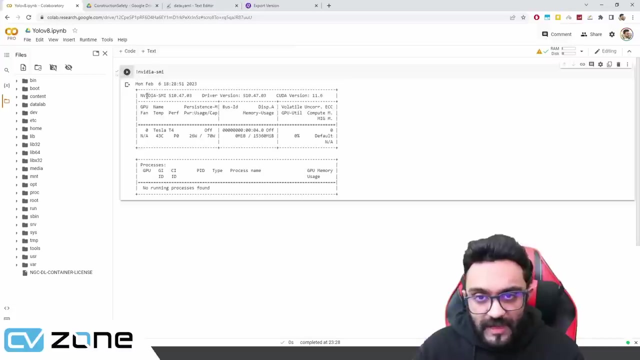 using a graphics card or not. So we will write here: NVIDIA SMI, dash SMI, And then we are simply going to run it. So once we run this, we will have some information. So here you can see Tesla T4.. We are actually using 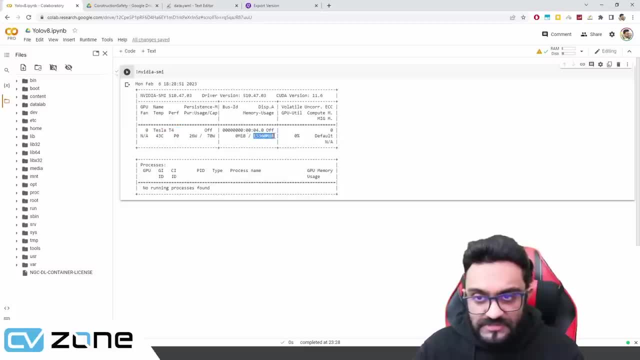 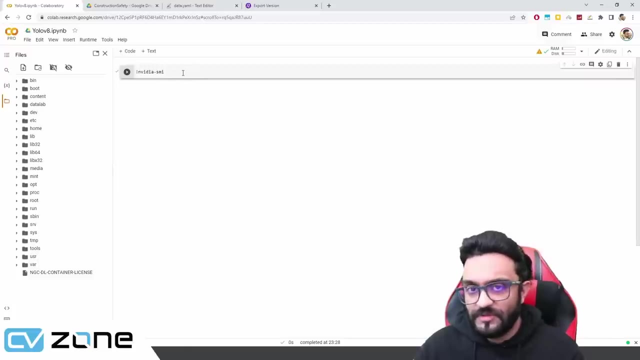 15360 MBs. So that's good. So we are actually using a graphics card, So that's done. Now, what I'd like to do? I like to clear all the outputs whenever we do that, So then we can write. 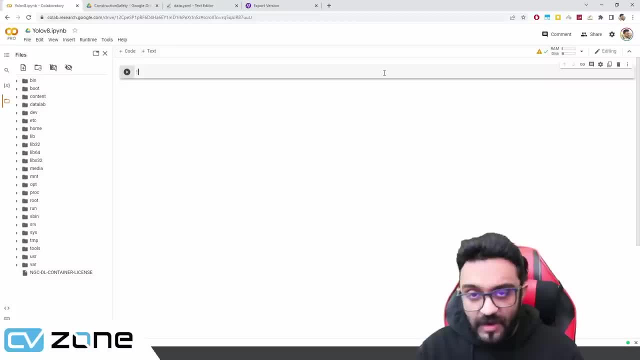 So first of all, we need to check whether we are Uh using a graphics card or not. So we will write here: uh NVIDIA SMI, uh dash SMI, and then we are simply going to run it. So once we run this, we will have some information. 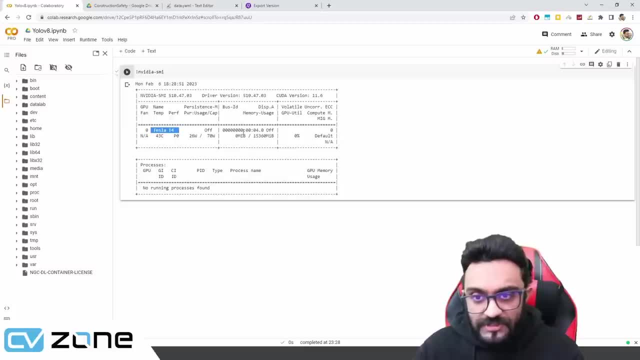 So here you can see a Tesla T4.. We are actually using 15360 MBs, So that's good. So we are actually using a graph Graphics card, So that's done. Now, what I like to do? I like to uh, clear all the outputs. 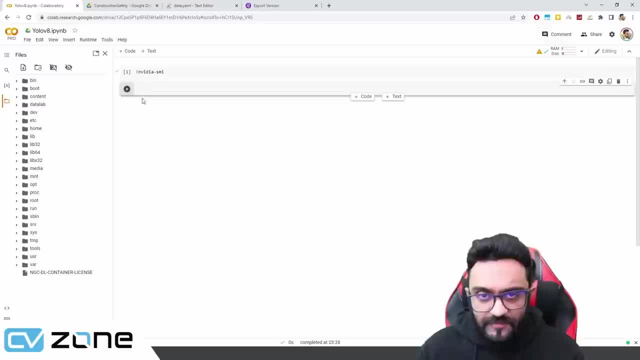 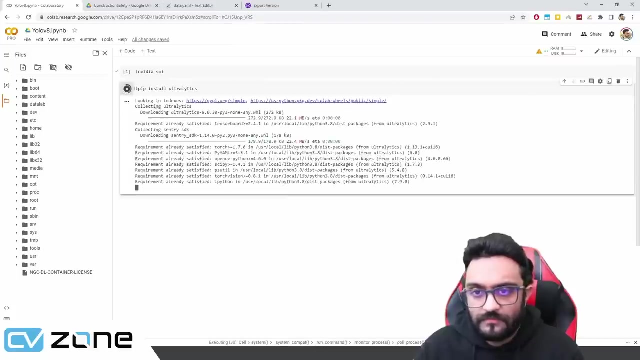 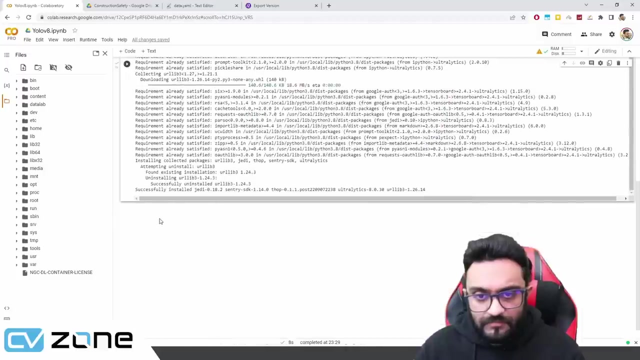 whenever we do that. So then we can write another line of code. Now in this we are going to install Ultralytics, So we will write here: pip, install Ultralytics. We will hit enter. Oh sorry, Let's play. 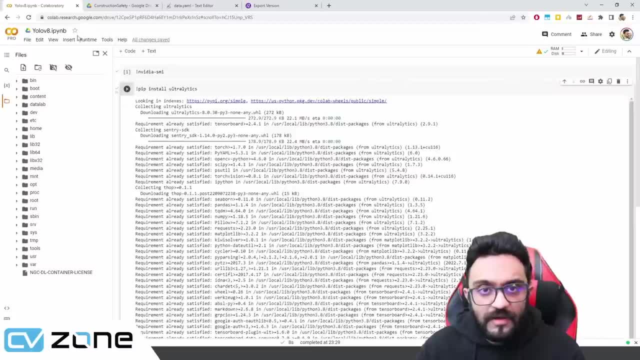 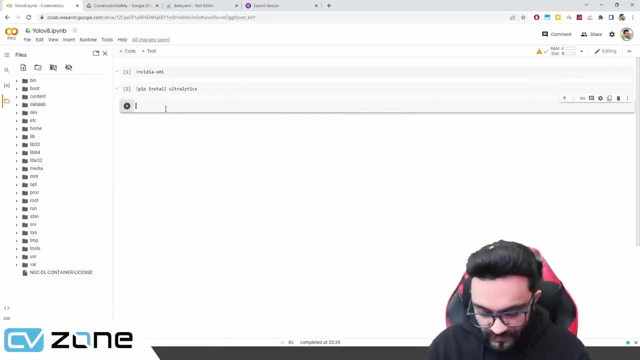 So now it's done installing. So that's done. Again, I will go back to edit and clear outputs because I don't like them. Then we are going to go and we are going to import Yolo. So, like we did earlier, from Ultralytics import. 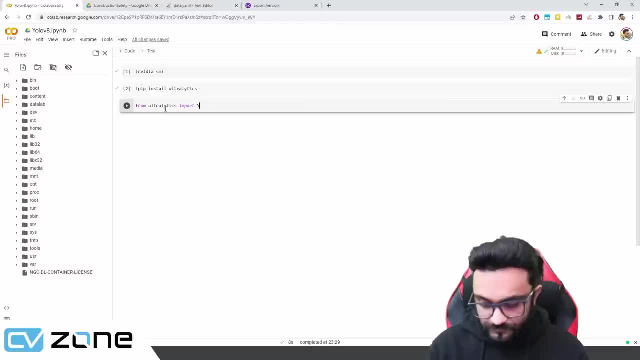 Okay, Okay. So we are going to go and we are going to print out Yolo, Uh, Yolo is capital. And we are going to press enter and there you go, It has been executed. So now we are going to write the actual command that will run Yolo and detect it on an image. So, first of 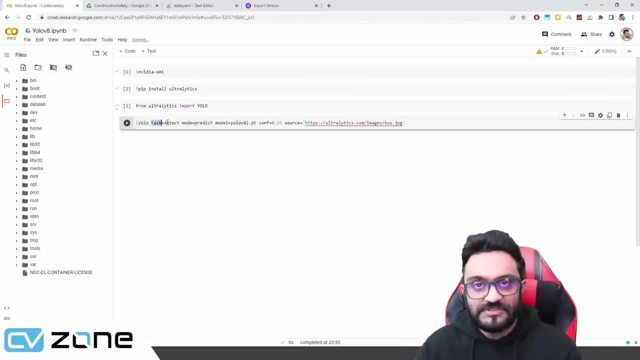 all. we are going to write Yolo and then we will define the task to detect. from an image We need to detect objects. It also has the option of classification And it also has the option of segmentation, But for now we will just do detection. You can write segmentation. 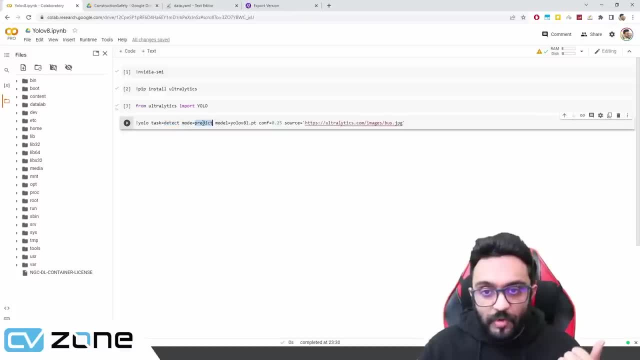 as well. if you wanted to segment, Then we have more to predict. Uh, there is training as well, There's validation as well, But right now we are using the mode as predict, Then the model. So which model we are using? 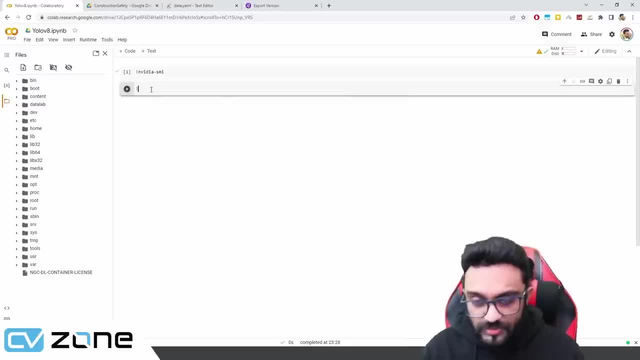 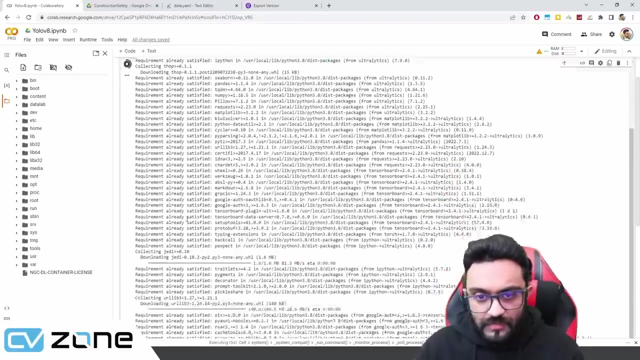 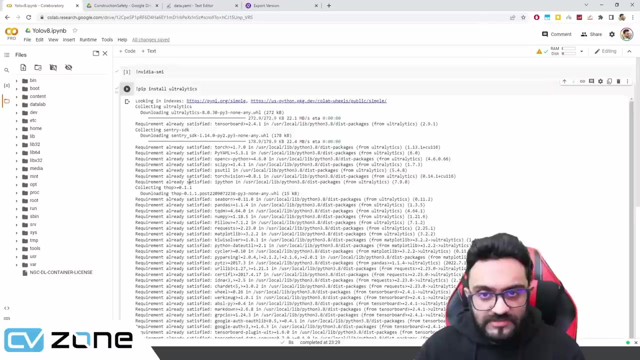 another line of code. Now in this we are going to install Ultralytics. So we will write here: pip, install Ultralytics. We will hit enter. Oh sorry, we'll hit play. So now it's done installing. So that's done. 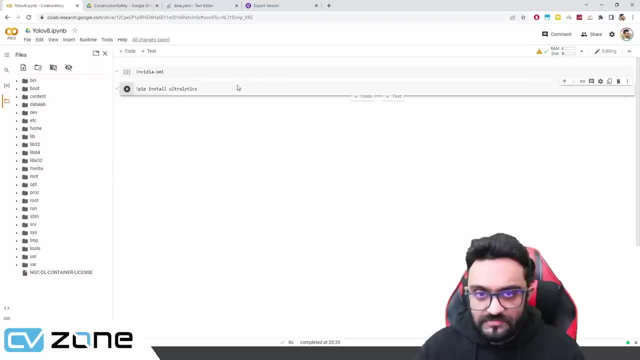 Again, I will go back to edit and clear outputs because I don't like them. Then we are going to go and we are going to import YOLO. So, like we did earlier, from Ultralytics, import YOLO. YOLO is capital. 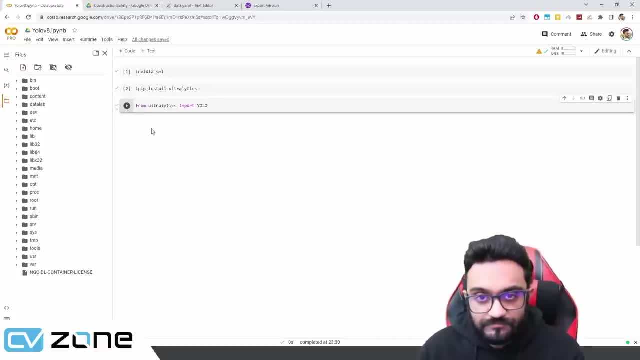 And we are going to press enter. And there you go, It has been executed. So now we are going to write the actual command that will run YOLO and detect it on an image. So first of all we are going to write YOLO. 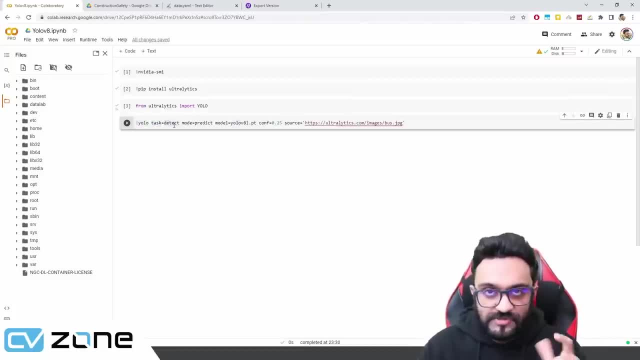 And then we will define the task to detect. from an image We need to detect objects. It also has the option of classification and it also has the option of segmentation. But for now we will just do detection. You can write segmentation as well. 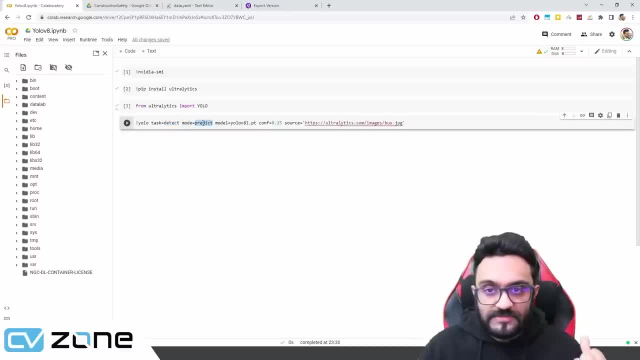 if you wanted to segment, Then we have mode predict. There is training as well, There's validation as well, But right now we are using the mode as predict. Then the model. So which model we are using? We are using YOLO 8 version. 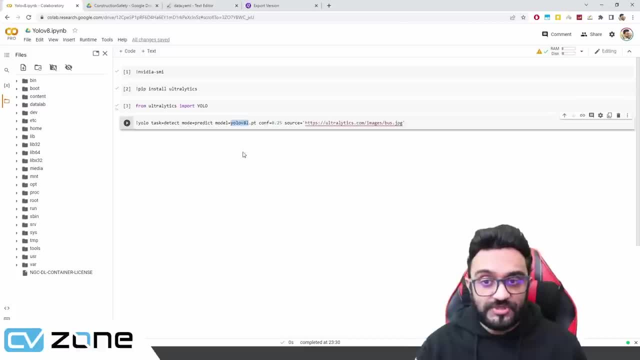 YOLO version 8, which is large. So we are using the large model And the confidence level minimum should be 0.25.. And what is the source? The source is basically the image, So it can be here in your drive. 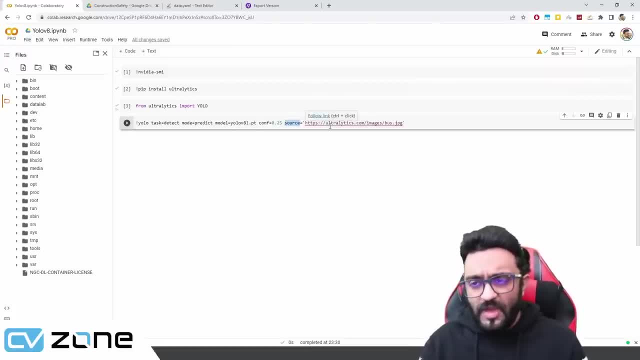 or you can give an online source. So for now we are just giving it an online source. This is basically ultralyticscom slash images- slash busjpg. If you had your own image, you can import it here and test it out, Or if you have an image online, 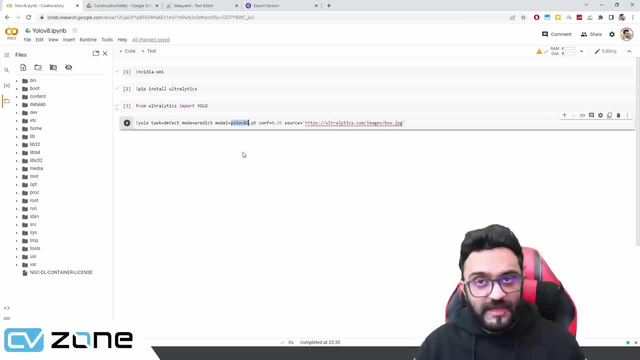 We are using Yolo eight version uh, Yolo version eight, which is large. So we are using the large model and the confidence level minimum should be 0.25.. And what is the source? The source is basically the image, So you it can be here in your. 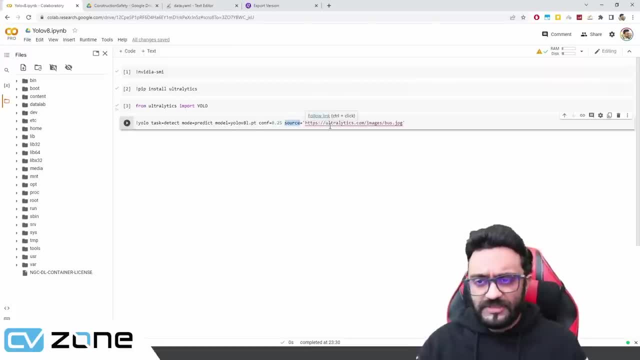 drive or you can give an online source. So for now we are just giving it an online source. This is basically ultralyticscom slash images- slash busjpg. If you had your own image, you can import it here and test it out. Or if you have an image online, you can test. 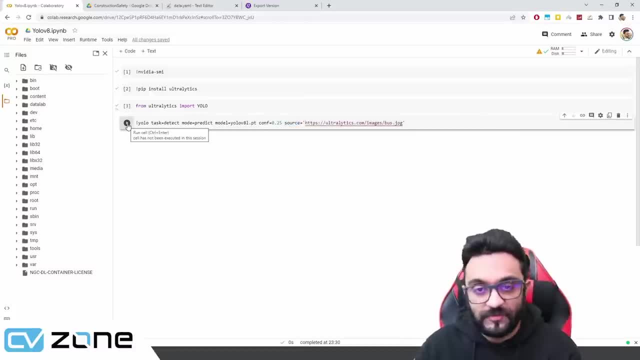 it from there as well. So once that is done- this is the moment of truth- We will press control enter and then it will execute this command. So first of all, as always, it is going to download the weights, because it already does not have that. That is done, Now it is. 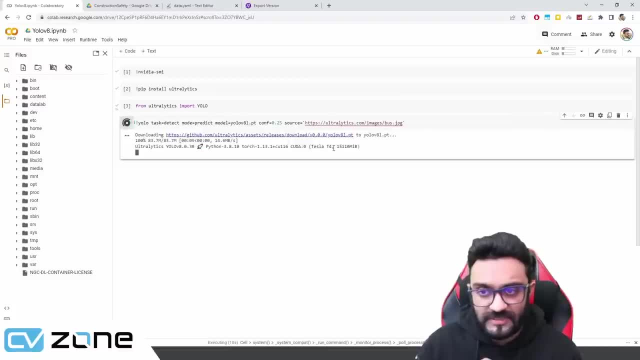 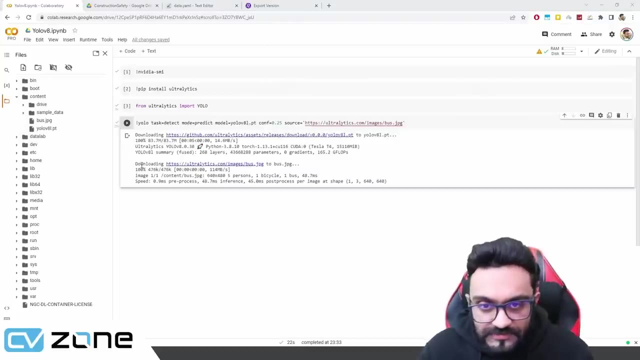 running and it is using CUDA zero Tesla T four. This is the GPU that it's using, So that's good. We know that it's working. It's downloading the image and the image has been downloaded and it has executed everything. As you can see, this is now done and you can see it downloaded the file and then it gave. 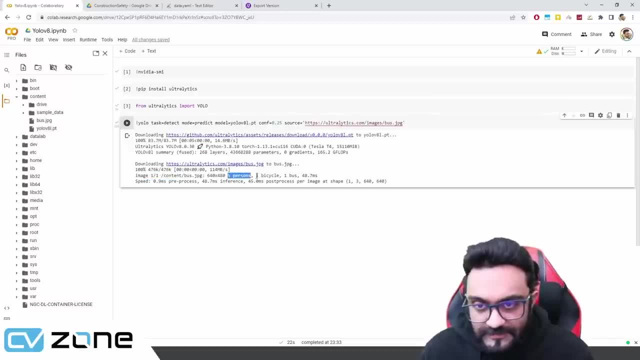 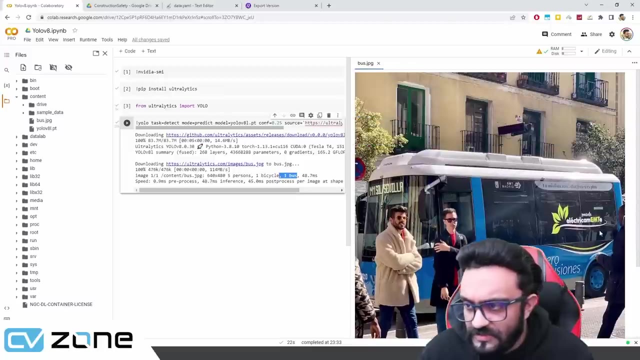 us the result that there were five people detected, one bicycle and one bus. So if we open this up it will not actually show you the bounding boxes and all that. but we will need to write some code for that, But for now you can see there's one person here. second, 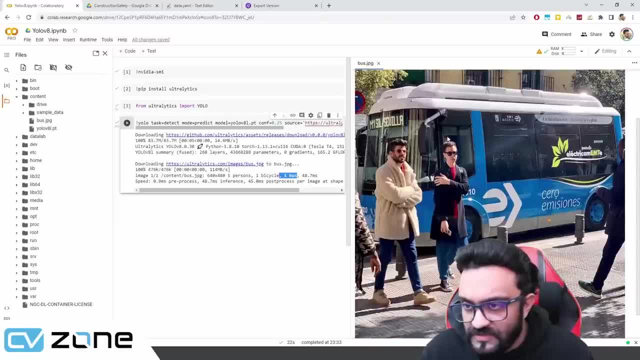 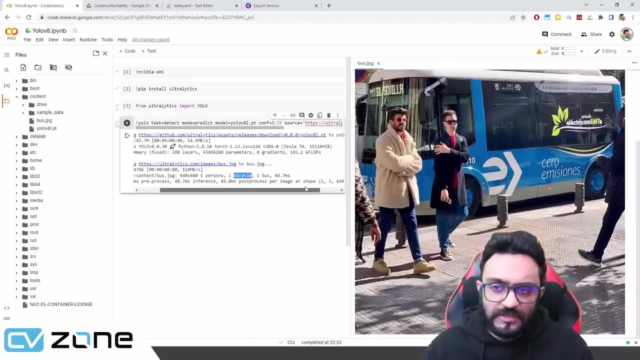 here, third here, fourth here and maybe a fifth inside Well over here. So five people, one bicycle, one bus. So this is the bus. I'm not sure where the bicycle is, though, And yeah, so that's the idea. So it means it is working. So what we need, we don't need. 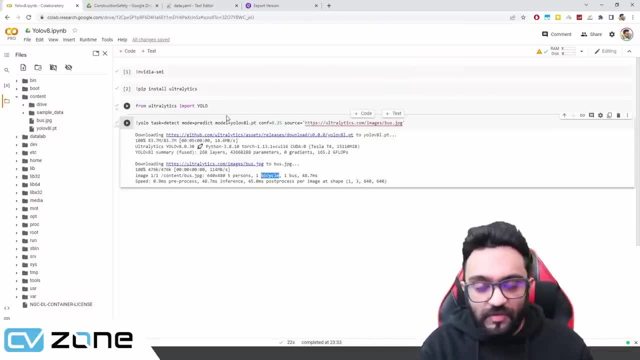 to test any images here. We can run it on our actual offline code and we can write the same code here and it will work fine as well. But we just wanted to check whether it's working or not, whether the installations are working or not. 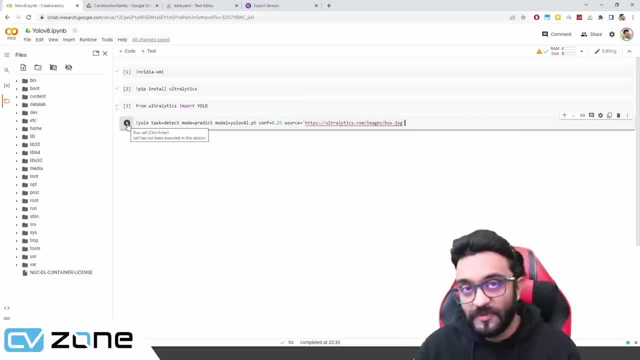 you can test it from there as well. So once that is done, this is the moment of truth. We will press enter, control enter, and then it will execute this command. So first of all, as always, it is going to download the weights. 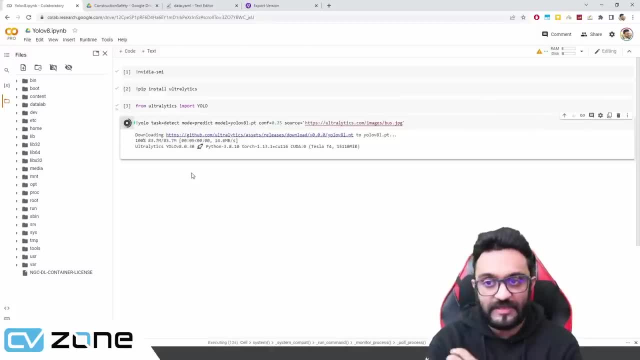 because it already does not have that. That is done. Now it is running and it is using CUDA 0, Tesla T4.. This is the GPU that it's using. So that's good. We know that it's working. It's downloading the image. 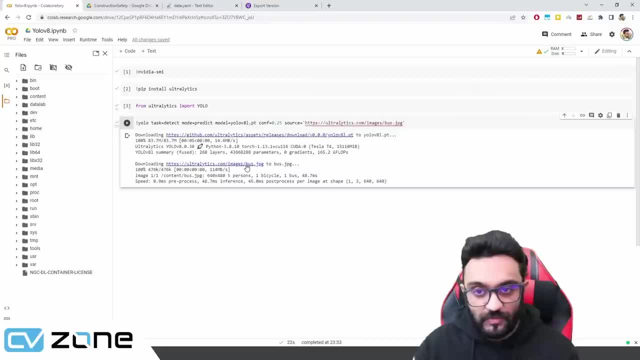 And the image has been downloaded and it has executed everything. So, as you can see, this is now done and you can see it downloaded the file and then it gave us the result that there were five people detected: one bicycle and one bus. So if we open this up, 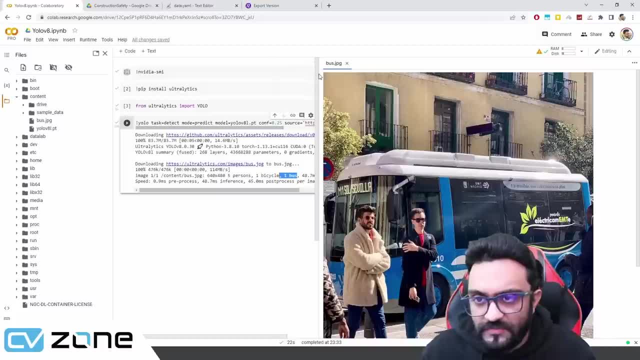 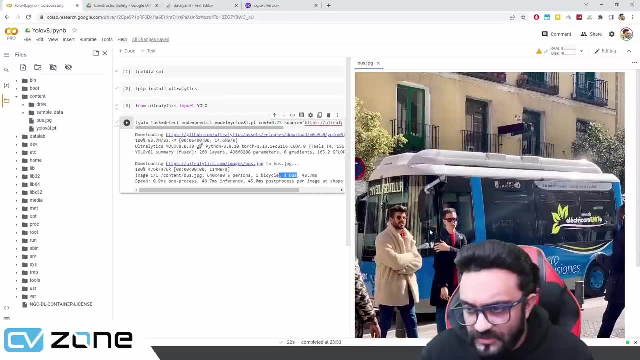 it will not actually show you the bounding boxes and all that, But we will need to write some code for that. But for now you can see: there's one person here, second here, third here, fourth here and maybe a fifth inside. 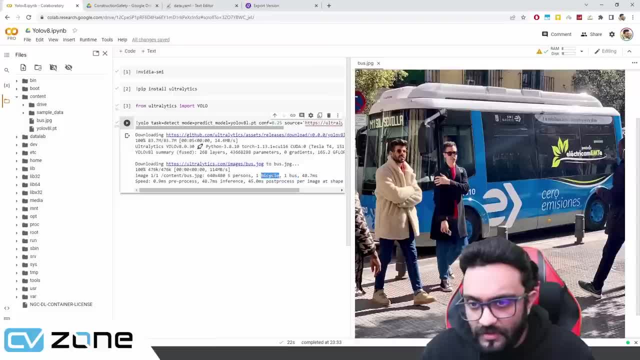 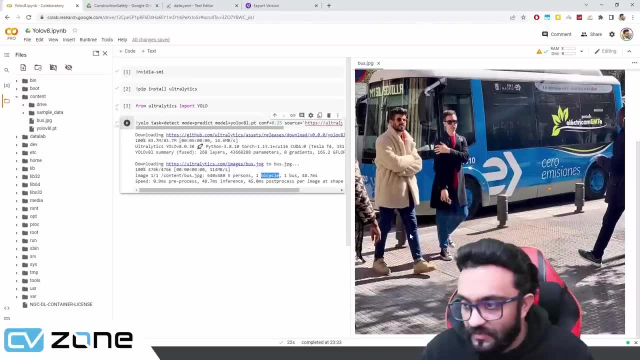 Well over here. So five people, one bicycle, one bus. So this is the bus. I'm not sure where the bicycle is, though, And yeah, so that's the idea, So it means it is working. So what we need. 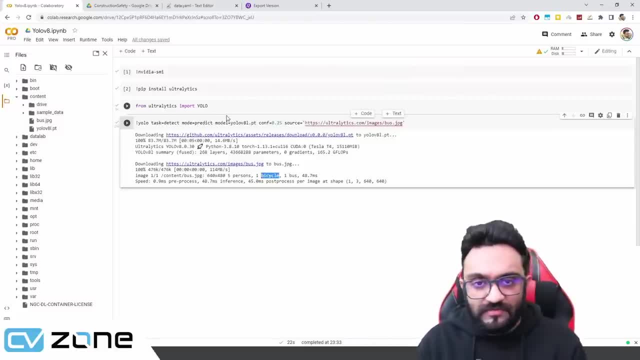 we don't need to test any images here. We can run it on our actual offline code and we can write the same code here. It will work fine as well. But we just wanted to check whether it's working or not, whether the installations are working or not. 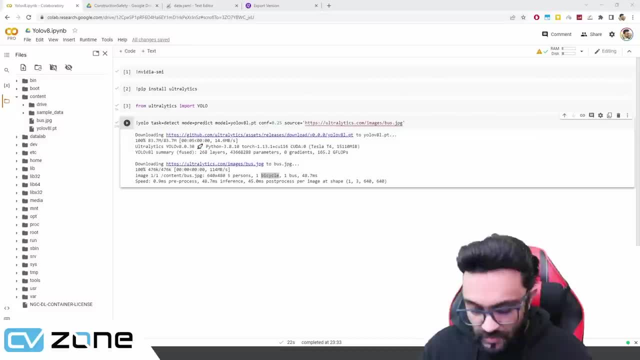 So, once we have confirmed that the installations are done, what we need is a simple one line code to actually do our custom training. Oh, custom data training. So that's it. And then what we will do: we will add our code and I'm going to paste it here. 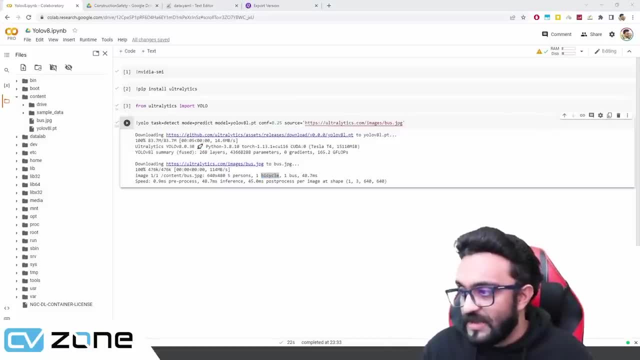 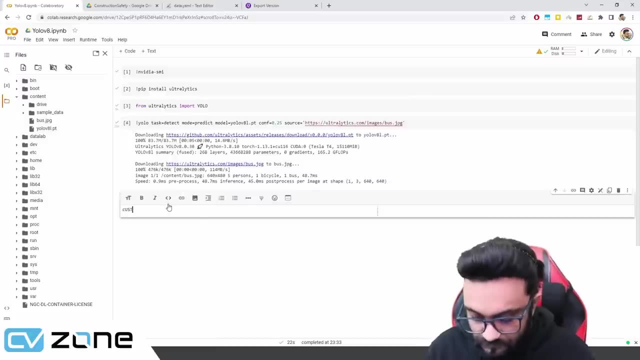 So, once we have confirmed that the installations are done, what we need is a simple one line code to actually do our custom custom training. Oh, custom data training. So that's it. And then what we will do. we will add our code and I'm going to paste it here. 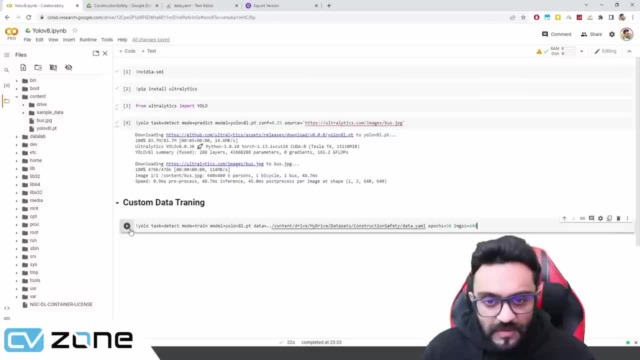 So now we have a similar command, like before. We have Yolo, Then we have task, Again we have detection, But this time around the mode is training, not prediction. It is training, and it is training based on, again, the large. what do you call the model? You can use the? 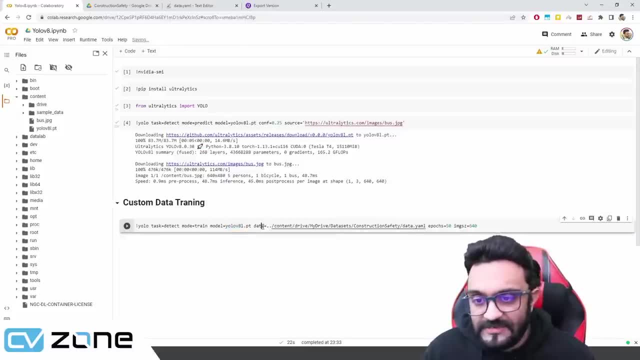 nano, small or medium as well, And where exactly is the data? So this is what you have to define, This is what you have to change. So data, These are the actually equals double dot slash content drive. So this is the exact path that 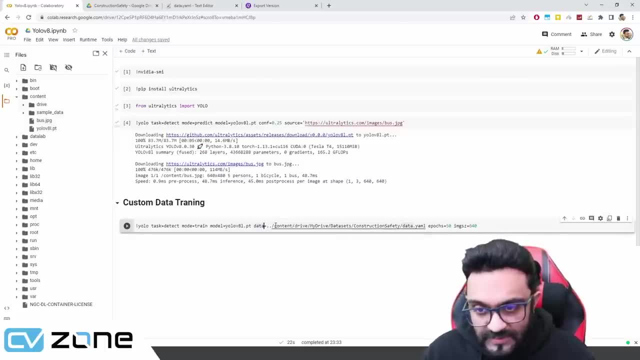 you will copy and paste here. So double dash back, a double dot back content drive: My drive: data sets, construction safety slash datayaml. So you have to give that file. That file is the linking file for all the dataset. So you need to give the location. 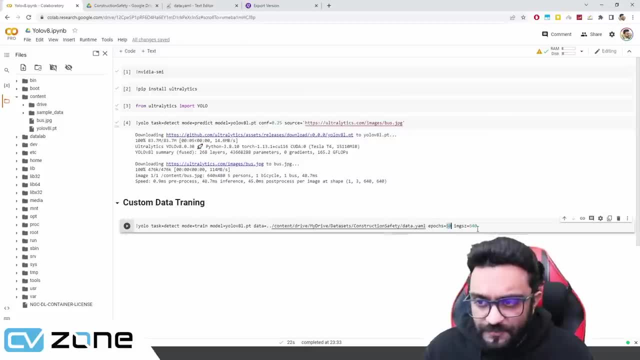 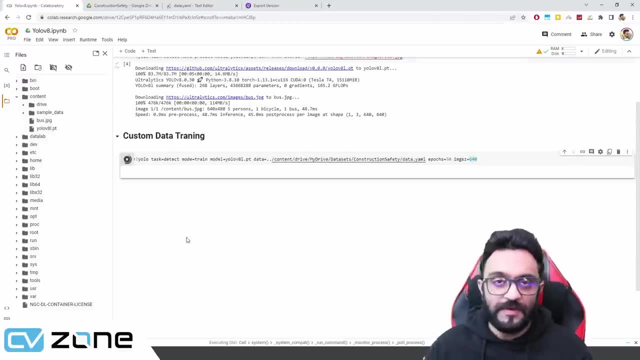 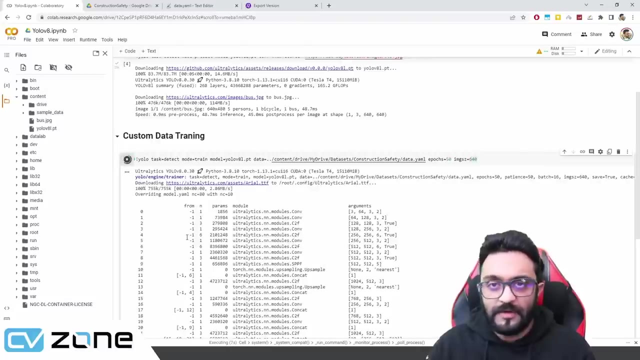 of that file. Then you can define the number of E-pods and the initialization image size. so that's pretty much it, and now all you have to do is press run and see the magic happen. so it will take a while to actually train. so we will let it train and then we will come back. 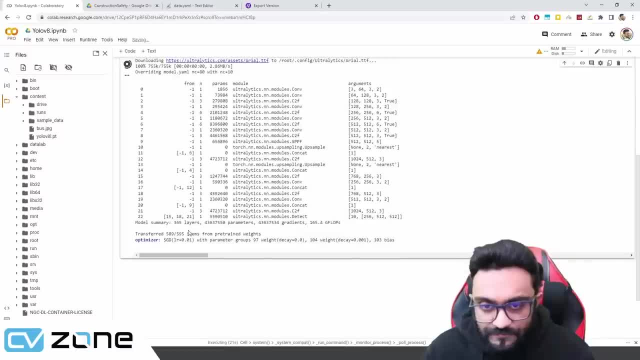 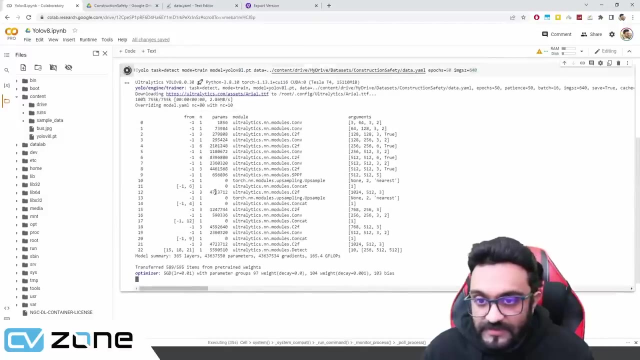 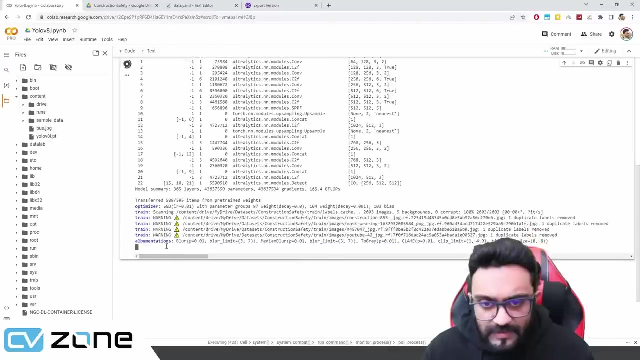 to it. so first of all, it is setting up all the weights. here you can see 589 of 595 items from pre-trained weights. so we are using the pre-trained weights to actually train our own model. you can say it is transferred learning as well. so the optimizer is has a learning rate of 0.01, and let's 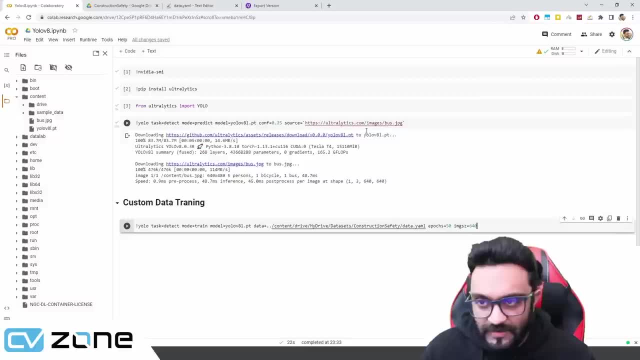 So now we have a similar command, Like before. we have Yolo, Then we have task, Again we have detection, But this time around the mode is training, not prediction. It is training, and it is training based on again. 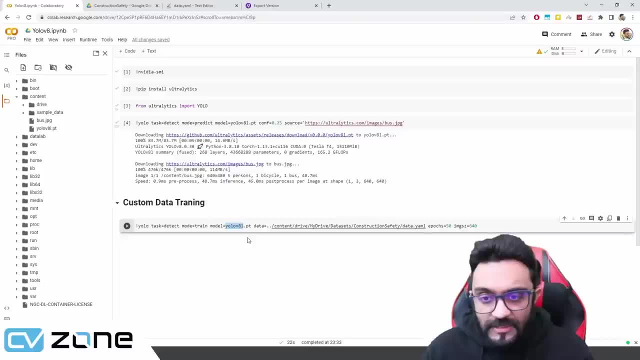 the large. what do you call the model? You can use the nano, small or medium as well. And where exactly is the data? So this is what you have to define, This is what you have to change. So data basically equals. 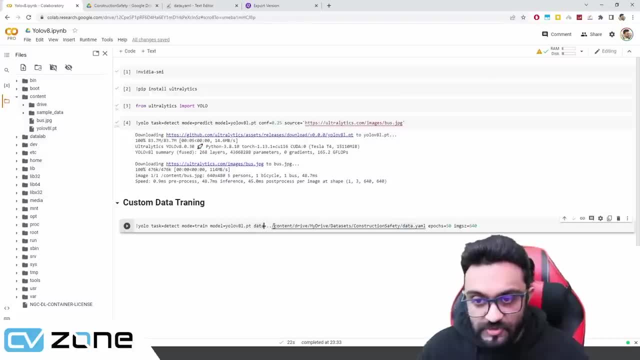 double dot slash content drive. So this is the exact path that you will copy and paste here. So double dash back. double dot back content drive. my drive data sets: construction safety slash data dot YAML. So you have to give that file. 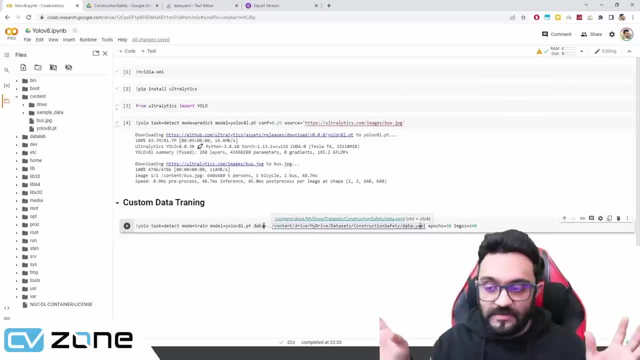 That file is going to be the linking file for all the data set. So you need to give the location of that file, Then you can define the number of epochs and the image size. So that's pretty much it, And now all you have to do 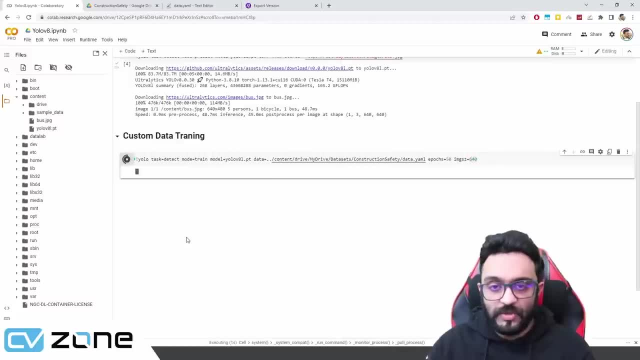 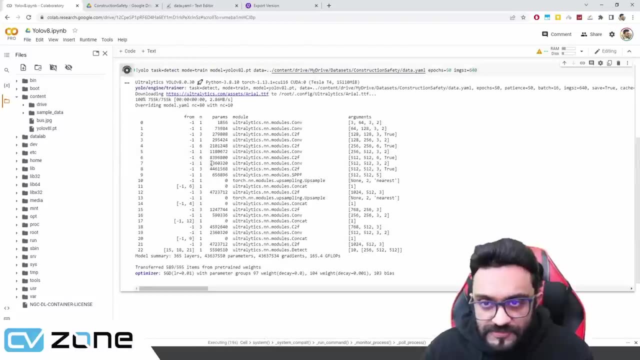 is press run and see the magic happen. So it will take a while to actually train. So we will let it train and then we will come back to it. So first of all, it is setting up all the weights. Here you can see. 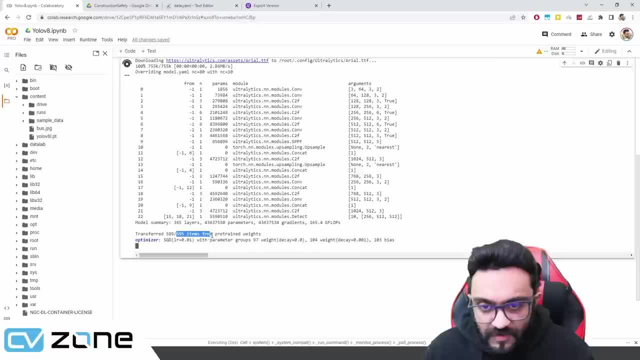 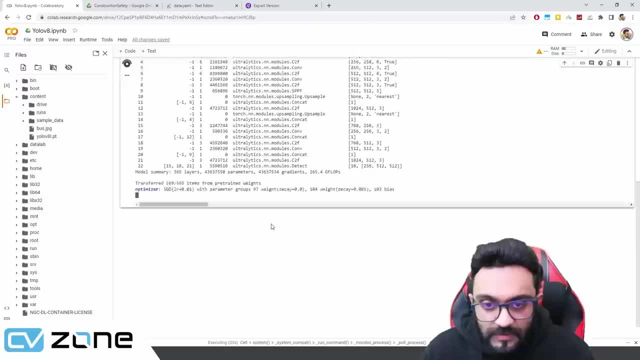 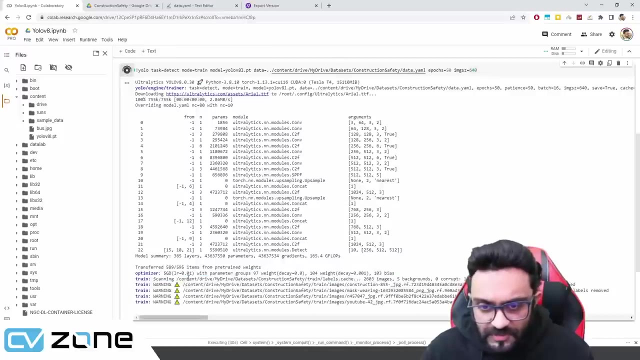 589 of 595 items from pre-trained weights. So we are using the pre-trained weights to actually train our own model. You can say it is transfer learning as well. So the optimizer has a learning rate of 0.01.. And let's see. 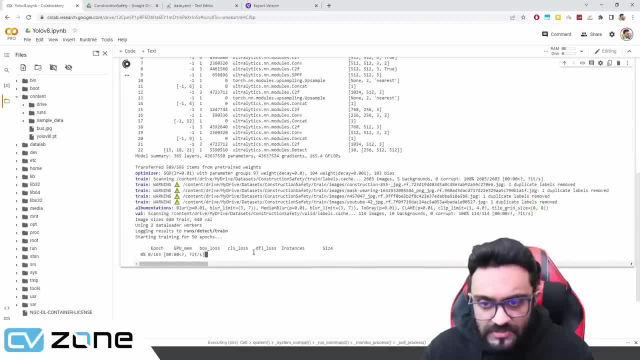 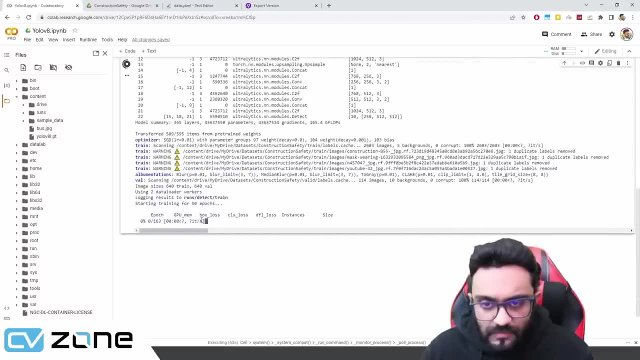 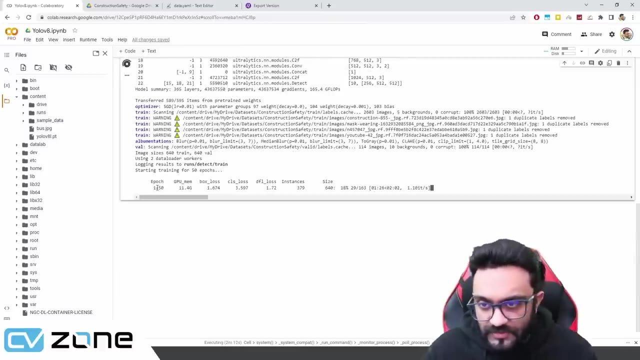 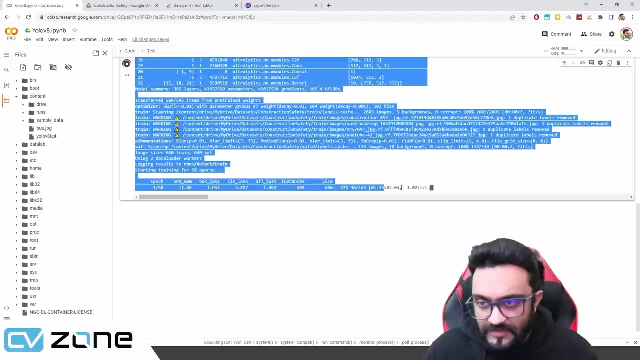 see. when does it start? so there you go. so right now it has started. so this is epoch number one did start not yet. let's wait for it to start. so now you can see the epoch has started, the counter has started, and here you can see the time that has taken already and the estimated time that is left. so this is basically the idea. so 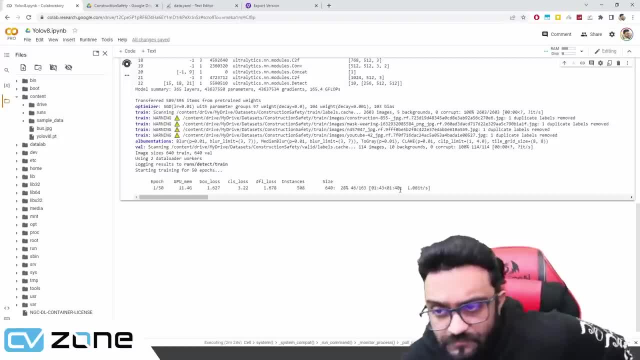 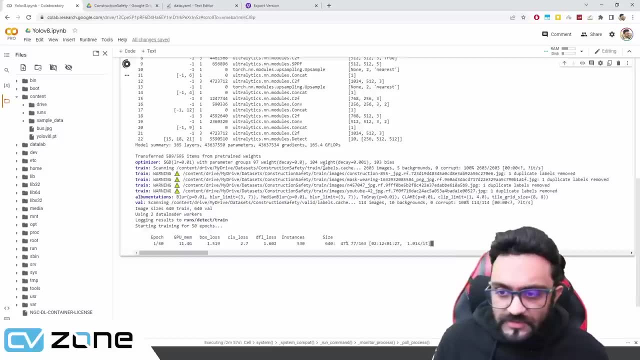 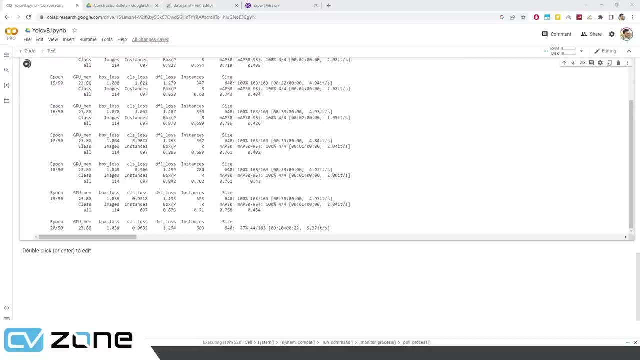 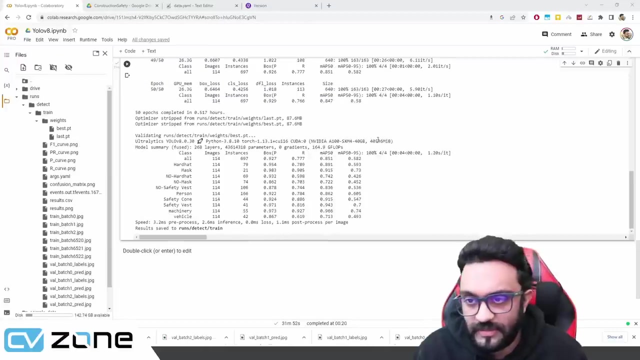 each one of these will take, for example, two minutes or three minutes, so you can calculate from there. it will take, for example, 150 minutes. so, anyways, let's wait for it to finish and i will see you once it's done. so now you can see that the process has completed, the training is completed and 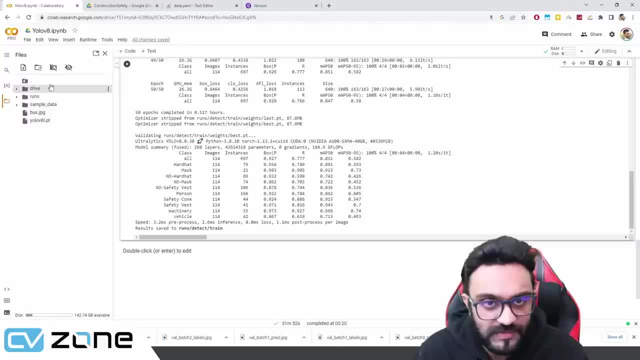 if you go to runs. this is basically in our content. if you go to runs and in detect you go to train, you will see all these files generated. so the main thing that we need to uh look at is the best dot pt. these are the weights and this is the best dot pt, and this is the best dot pt and this is the. 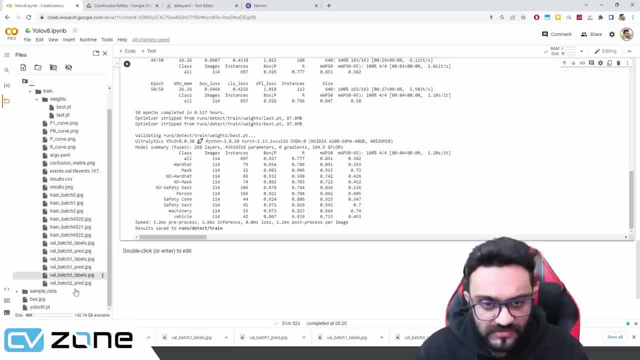 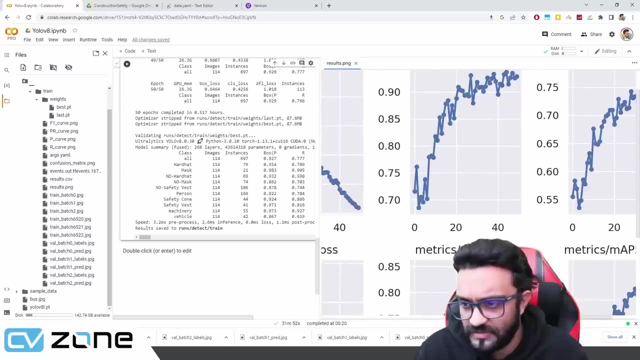 the last weight dot, pt. so and the rest of these are basically the parameters, the response of our model. so, for example, you can see over here resultspng. you also have the, so here you can see the mean average position values and you also have the recall and the precision values and you have 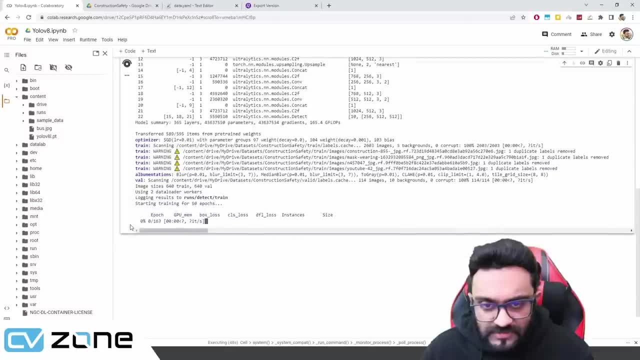 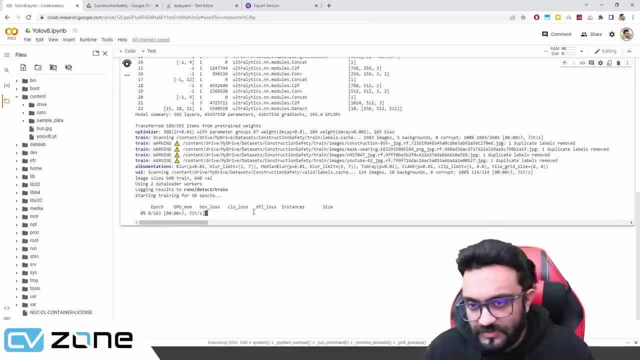 when does it start? So there you go. So right now it has started. So this is epoch number one. Did it start? Not yet. Let's wait for it to start. So now you can see, the epoch has started, The counter has started. 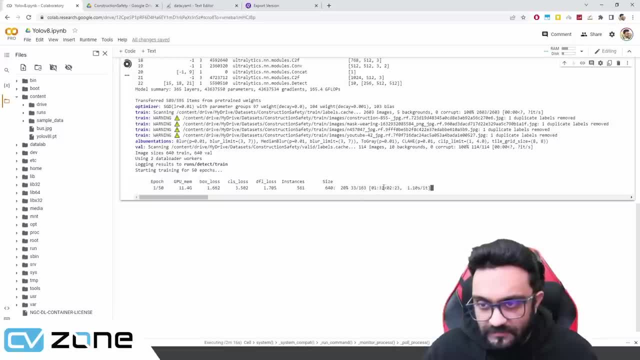 And here you can see the time that has taken already and the estimated time that is left. So this is basically the idea. So each one of these will take, for example, 2 minutes or 3 minutes, So you can calculate from there. it will take, for example, 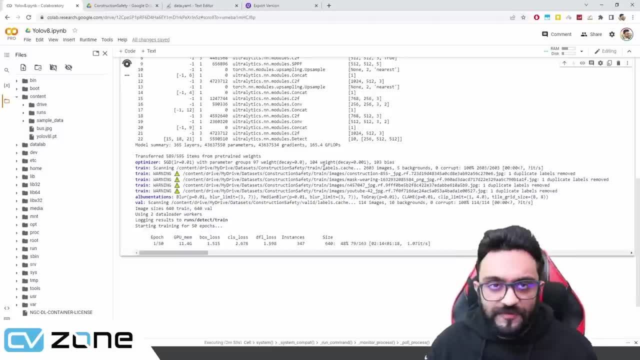 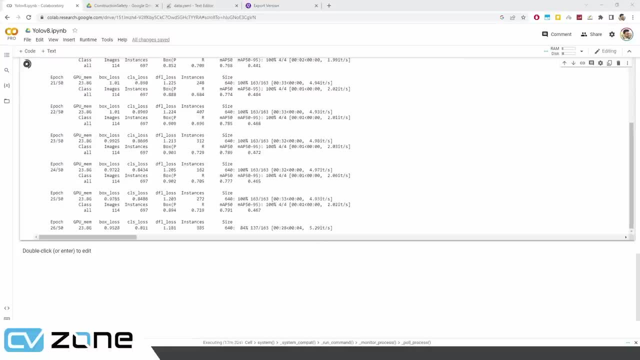 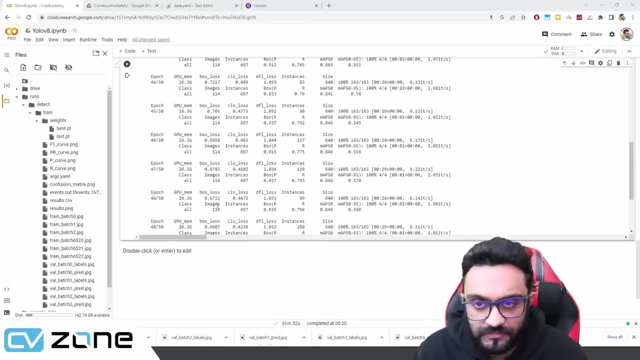 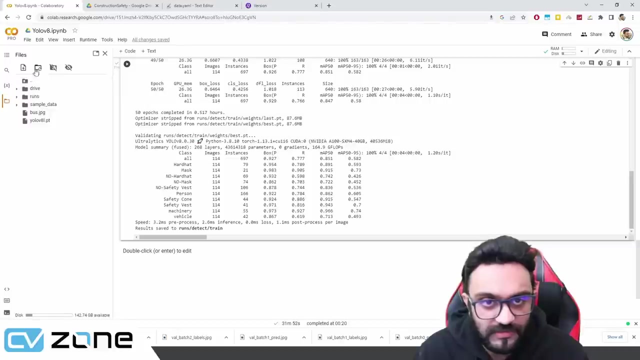 150 minutes. So, anyways, let's wait for it to finish and I will see you once it is done. So now you can see that the process has completed, the training is completed and, if you go to runs, this is basically in our content. if you go to runs, 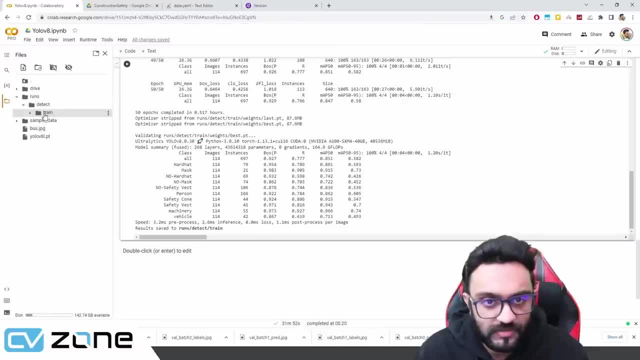 and in detect, you go to, you go to train, you will see all these files generated. So the main thing that we need to look at is the bestpt. these are the weights and this is the last weightpt, So, and the rest of these are basically. 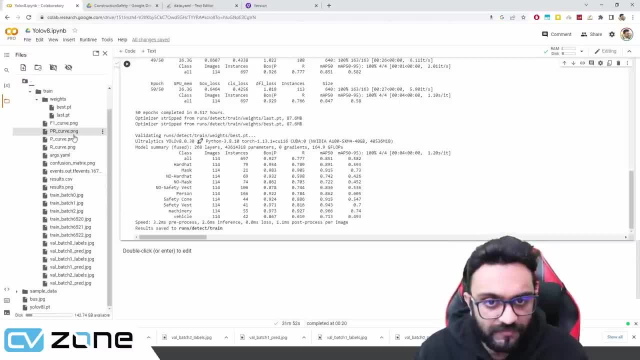 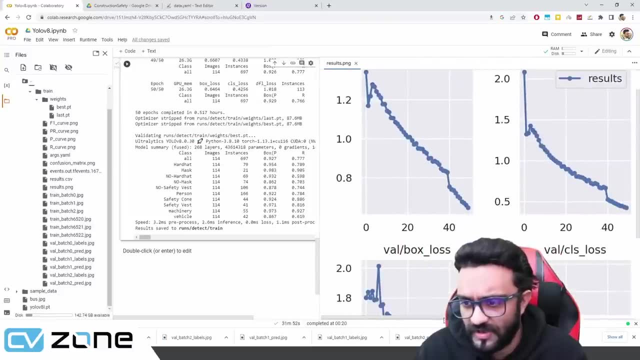 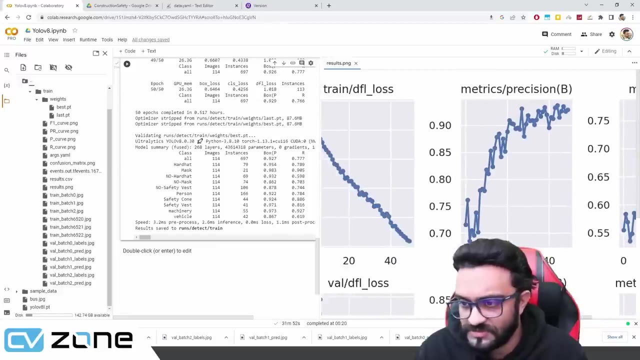 the parameters, the response of our model. So, for example, you can see over here resultspng. you also have the, so here you can see the mean average position values and you also have the recall and the precision values and you have the training loss for the class. 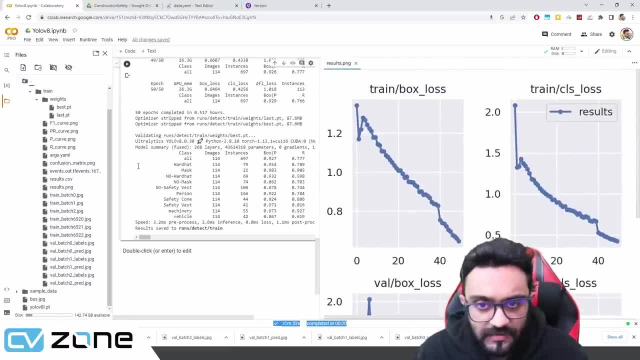 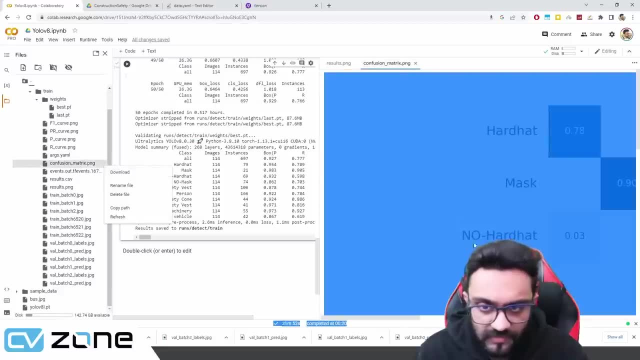 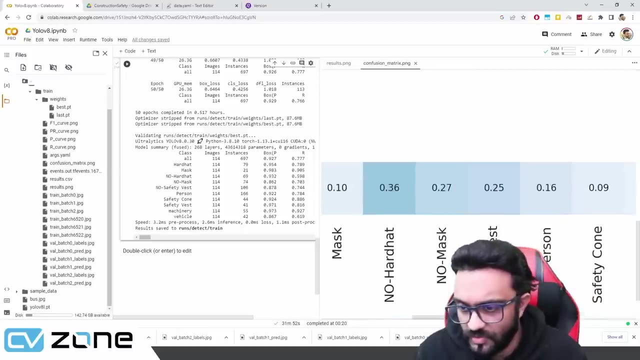 and also for the box. and then you also have the confusion matrix. So all of these things you can download. you can click here and download. it will be easier to see. otherwise, you can open it up on Google Colab as well. So here you can see. 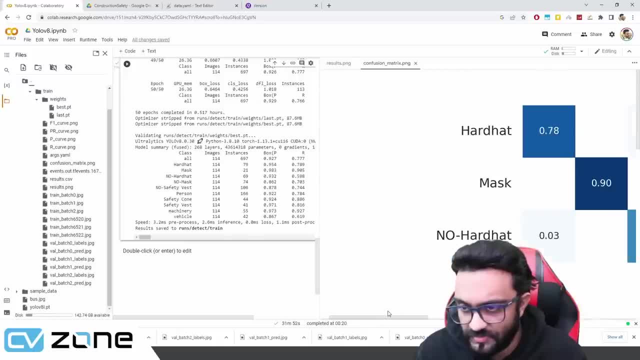 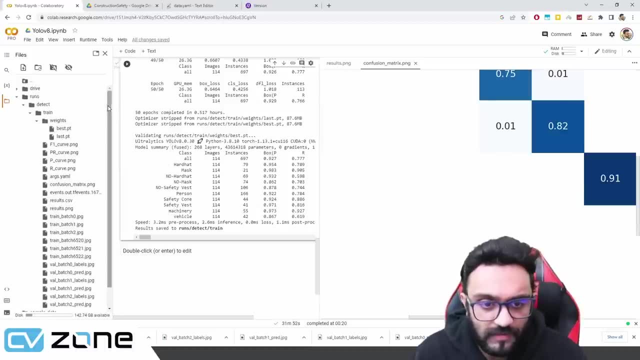 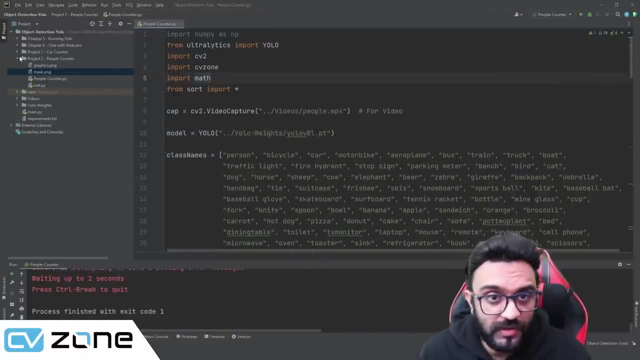 the confusion matrix of how well it responded to the training. So then, what you will do is you will download the best file and once that is downloaded, you are going to bring it to our project. So here we are going to name our project, so we will copy: YOLO with webcam. 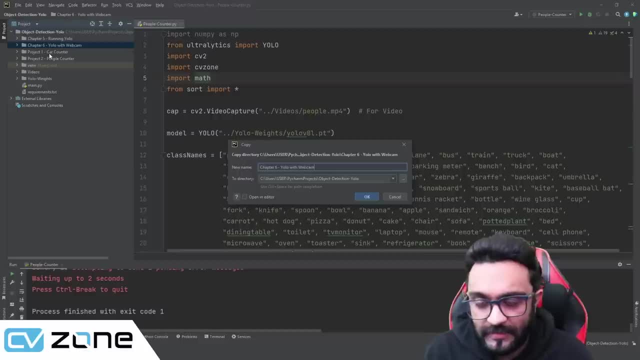 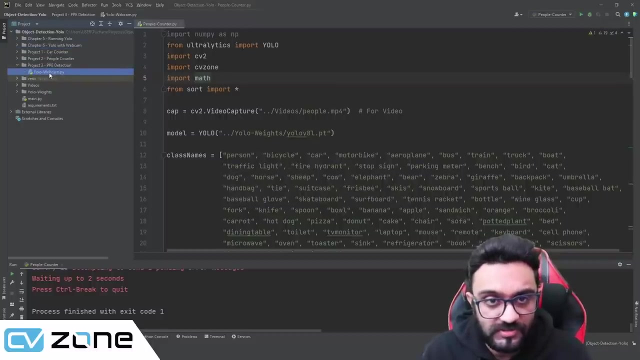 because that's pretty much what we are doing. we are running it with webcam and what we will do is we will remove all of this and we will write project 3, and here we will write PPE Detection. so this is our project 3 and it says YOLO webcam. 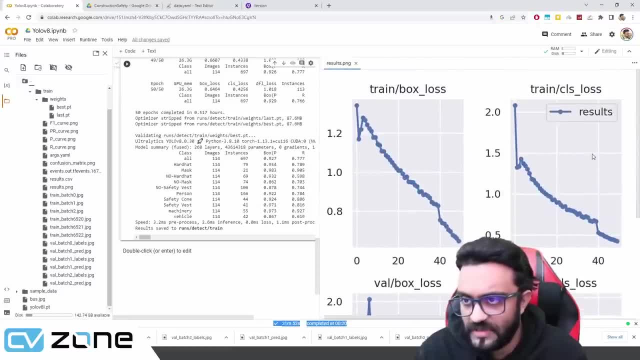 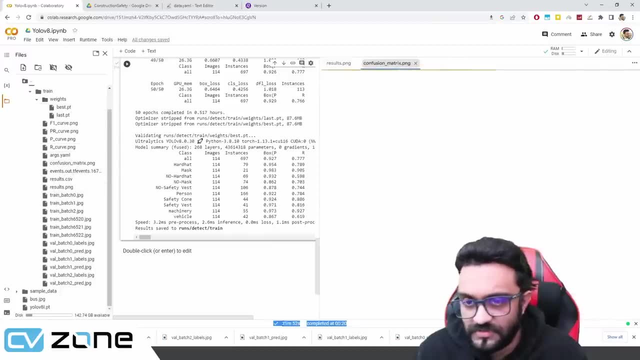 the training loss for the class and for also for the box. and then you also have the confusion matrix. so all of these things you can download. you can click here and download. it will be easier to see. otherwise you can open it up on google collab as well. so here you can see the confusion matrix. 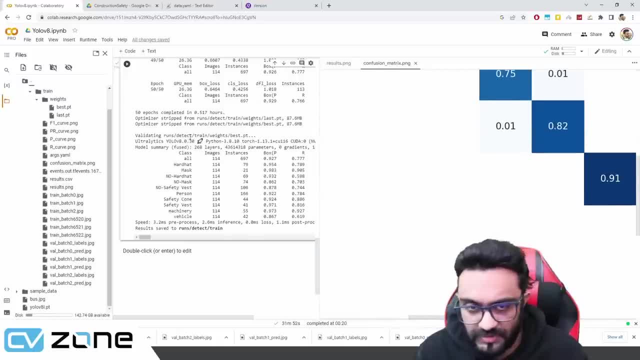 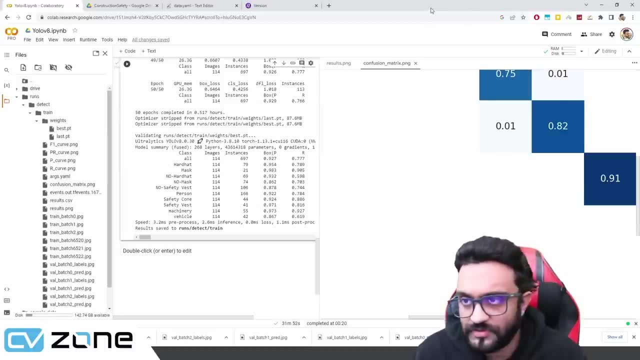 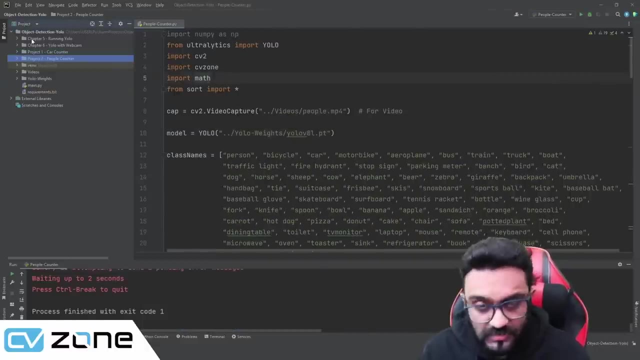 of how well it responded to the training. so then what you will do is you will download the best file and once that is downloaded, you are going to bring it to our project. so here we are going to name our projects, so we will copy. yolo with webcam. 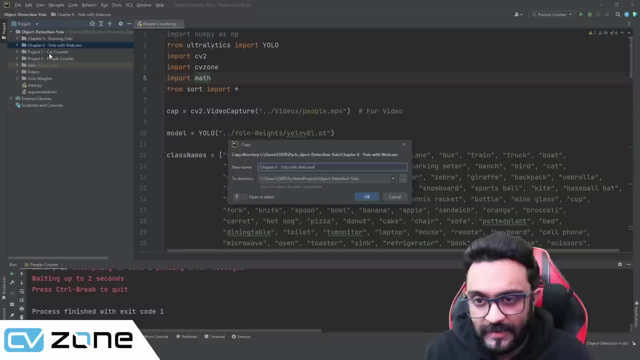 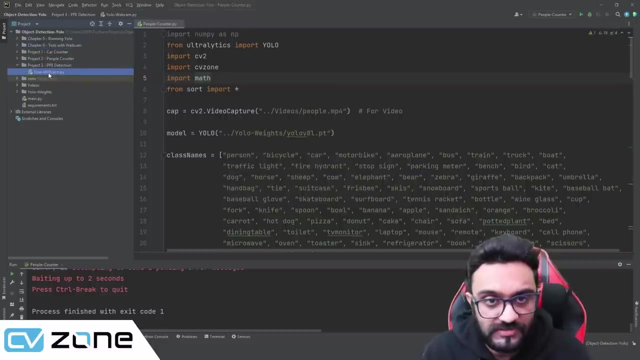 because that's pretty much what we are doing. we are running it with webcam and what we will do is we will remove all of this and we will write project three, and here we will write ppe detection. so this is our project three and it says yolo webcam. so we will double click that. 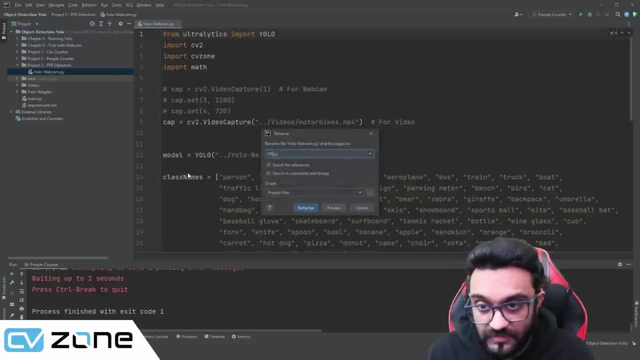 and right click and rename and we will write ppe detection. there you go. so now what we can do is we can use the ppe videos. so if we go here, we can open in our explorer and you can see we have these three videos. this is the first one. 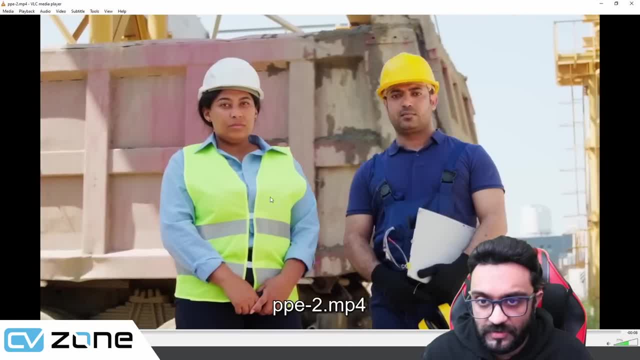 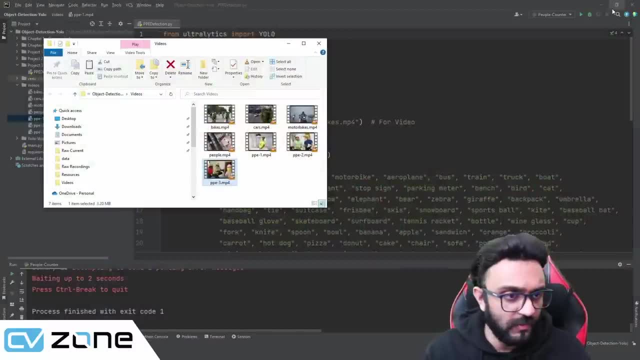 this is the second one, and this is the third one, so we are going to test on all three and we'll also test on the webcam. i do have a hard hat and, uh, i'm pretty sure we can find a mask, and i also have the construction jacket, so maybe we'll try that as well. so, uh, let's write here ppe. 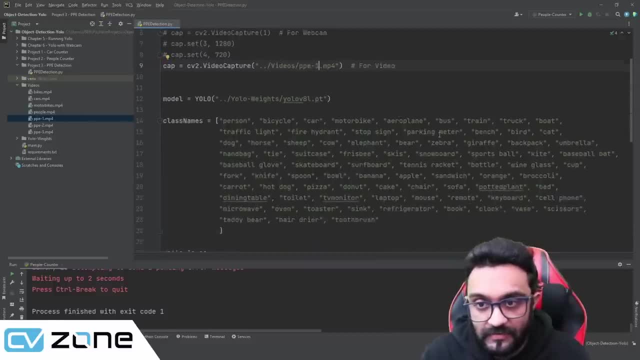 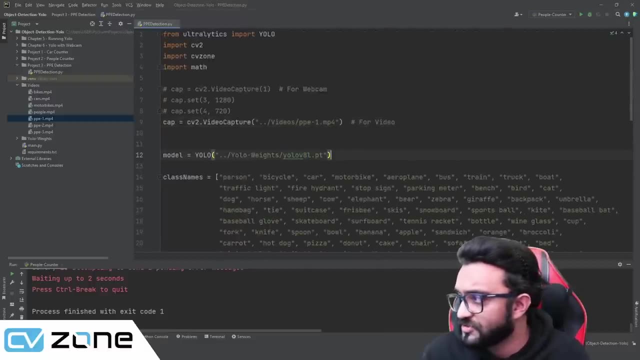 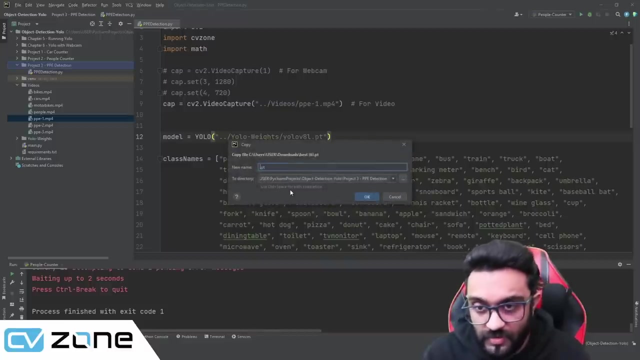 dash one, i believe that's the name. and uh, yeah, that's good. and then we have to change the uh model. so here we are just simply going to drag and drop. so here, this is the model. so we are going to drop it here and we are going to call it ppe. so here we will change it to ppe. 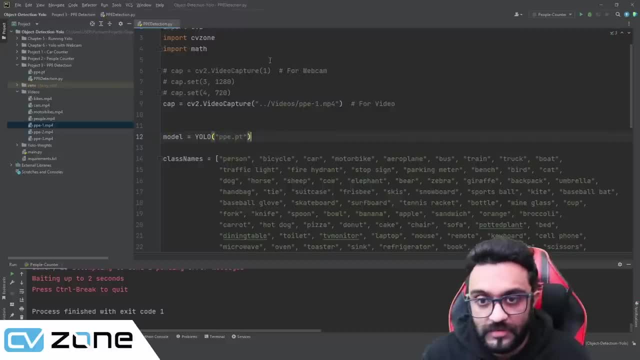 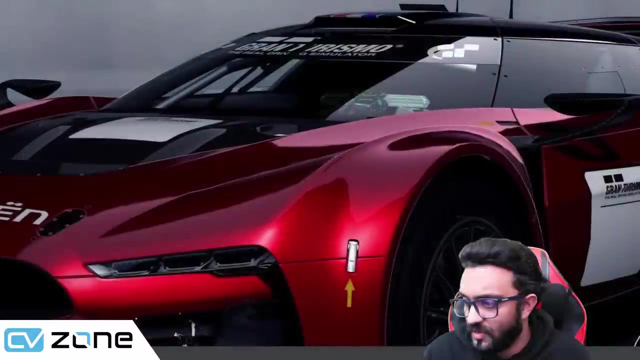 and we will remove all of this. so let's go ahead and run it. so let's- uh, actually one more thing i forgot: we do have to change the class names. so if we open up our files- uh, that we got the data dot yml file- we have the names of all the classes. 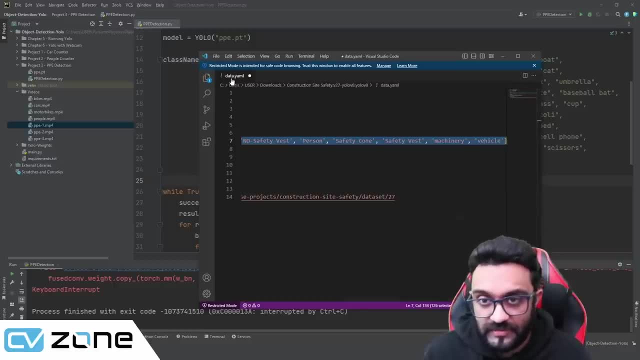 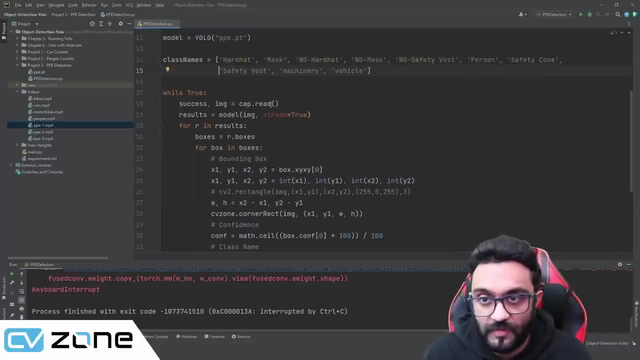 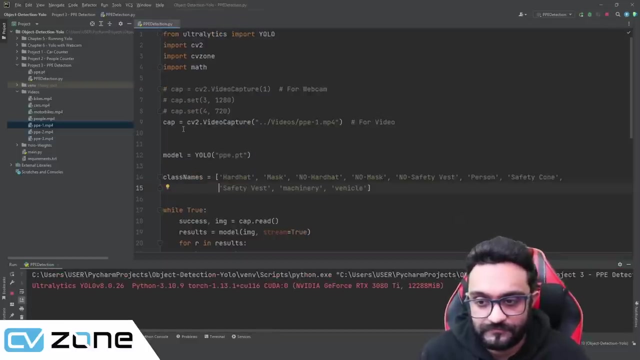 so we can simply copy it from there. so this is in the datayml file and we can replace it with our class names. there you go, so these are the class names, and now, if we run it, it should work fine. there you go. so it's detecting the person, it's detecting the hard hat. 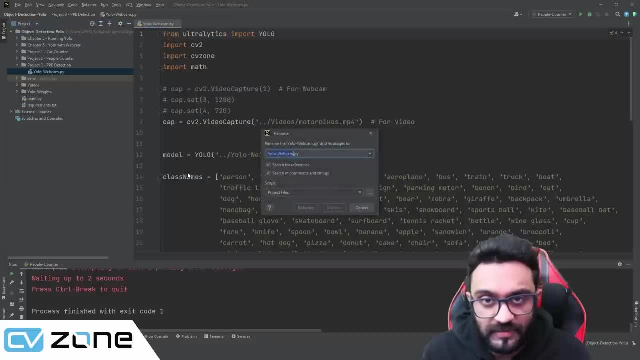 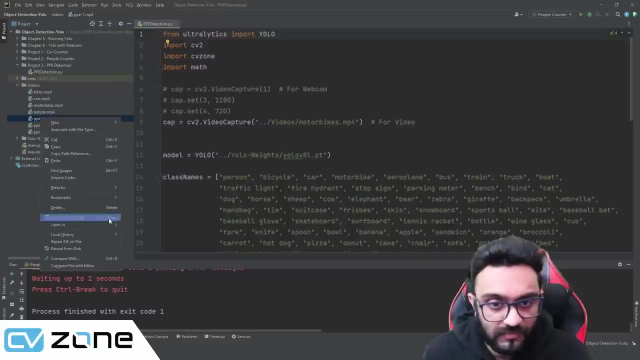 so we will double click that and right click and rename and we will write PPE Detection. there you go. so now what we can do is we can use the PPE videos. so if we go here we can open in our explorer and you can see we have these three videos. 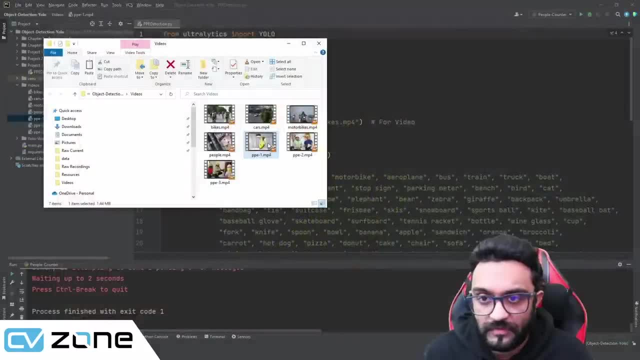 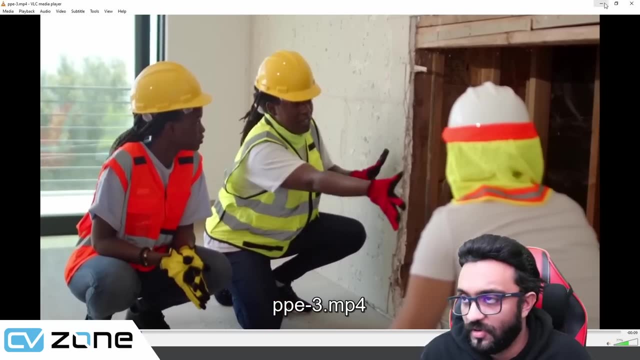 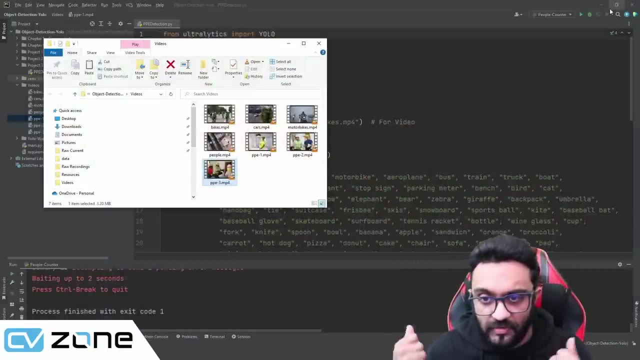 this is the first one, this is the second one and this is the third one, so we are going to test on all three and we will also test on the webcam. I do have a hard hat and I am pretty sure we can find a mask, and I also have the construction jacket. 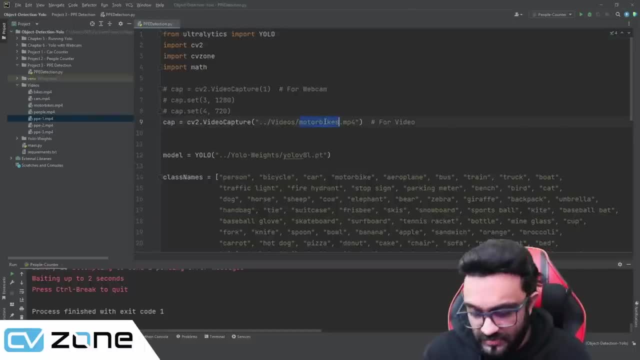 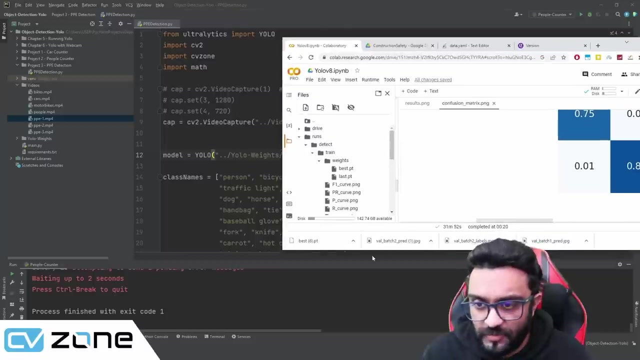 so maybe we will try that as well. so let's write here: PPE, PPE-1- I believe that's the name, and, yeah, that's good. and then we have to change the model. so here we are, just simply going to drag and drop. so here, this is the model. 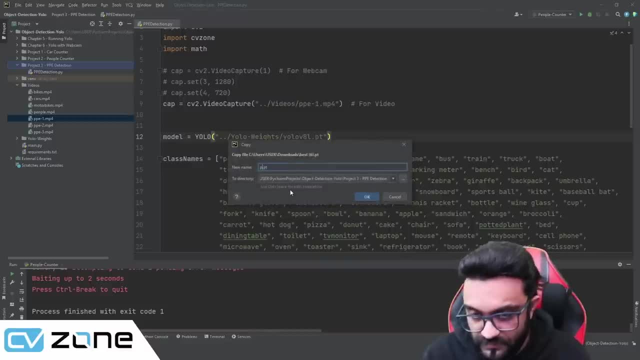 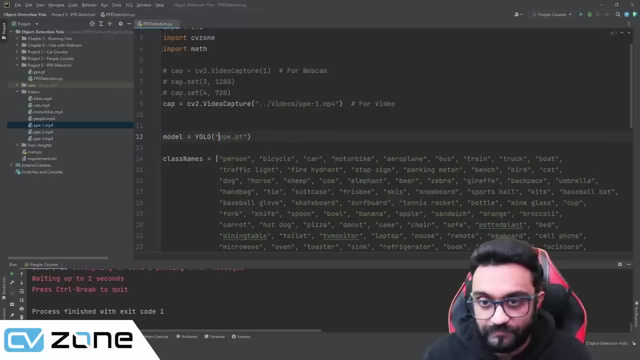 so we are going to drop it here and we are going to call it PPE. so here we will change it to PPE and we will remove all of this. so let's go ahead and run it. so let's actually one more thing I forgot: we do have to change the class names. 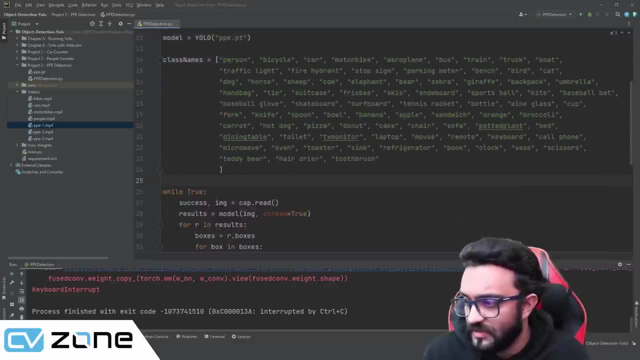 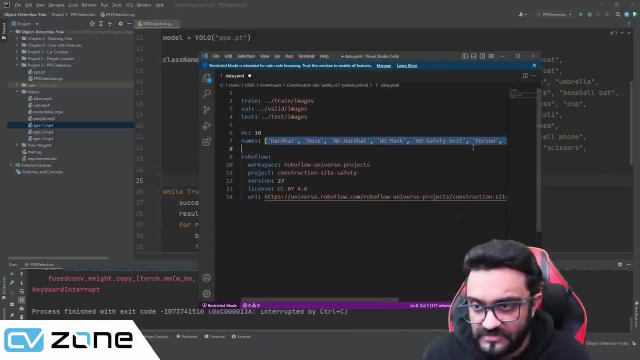 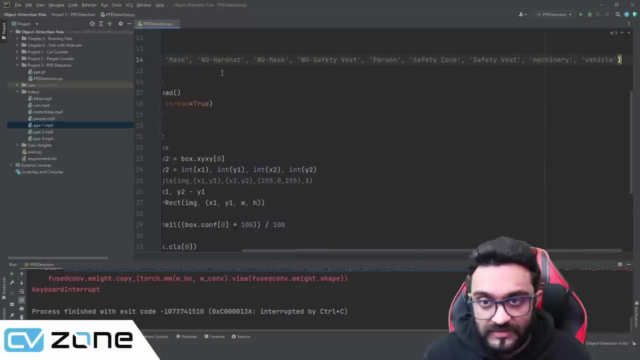 so if we open up our files that we got the datayaml file, we have the names of all the classes, so we can simply copy it from there. so this is in the datayaml file and we can replace it with our class names. there you go. so these are the class names. 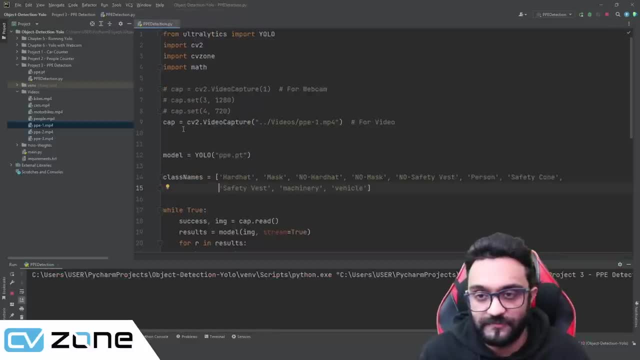 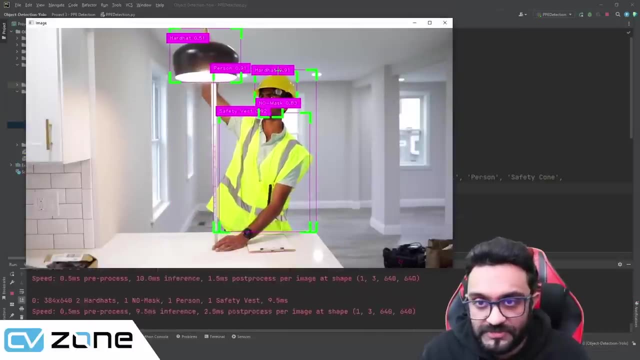 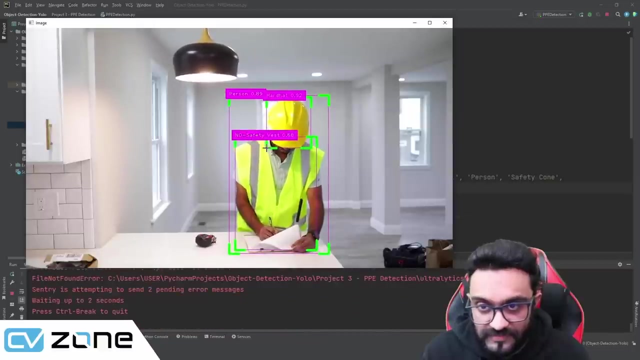 and now, if we run it, it should work fine. there you go. so it's detecting the person, it's detecting the hardhat, no mask, and you can see. it also detects safety or no safety vest. so it's not the most accurate, but it is giving us some good readings. 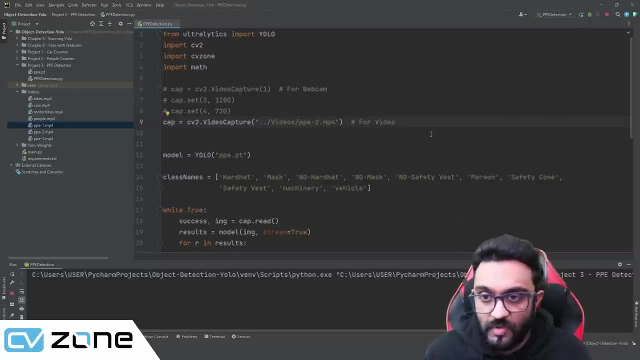 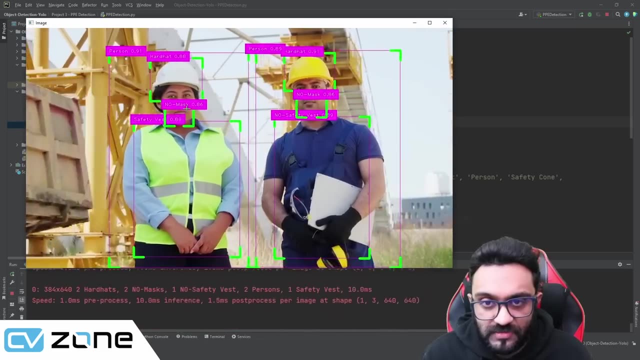 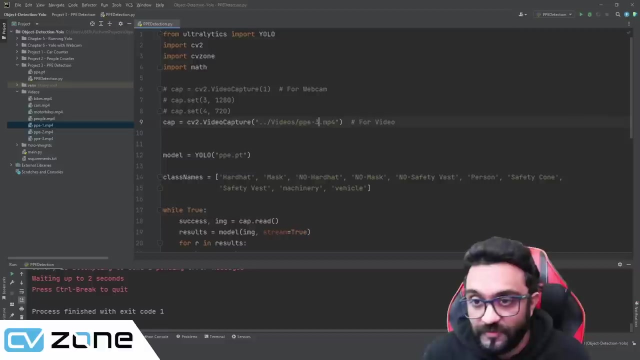 so what you can do is you can train it with more dataset and for longer epochs, for more epochs to get better results. so here you can see: safety vest- no mask, hardhat. and person- person- hardhat, no mask. and there you go. let's try for number three. 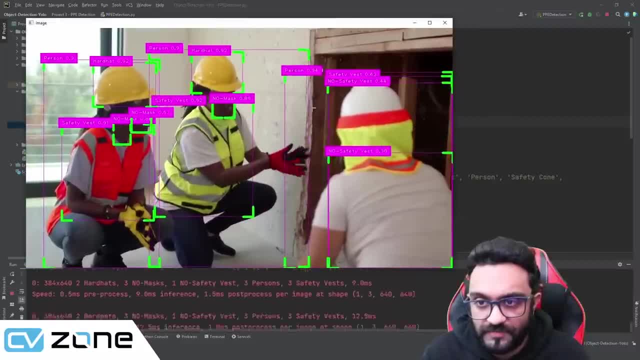 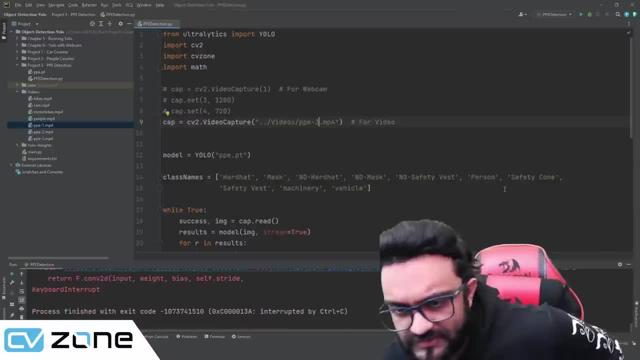 there you go. we have safety vest- hardhat person. no safety vest here. we have no mask safety vest- hardhat okay. so what we can do is this is a little bit difficult to see what exactly is being detected and what's not being detected, so what we can do is: 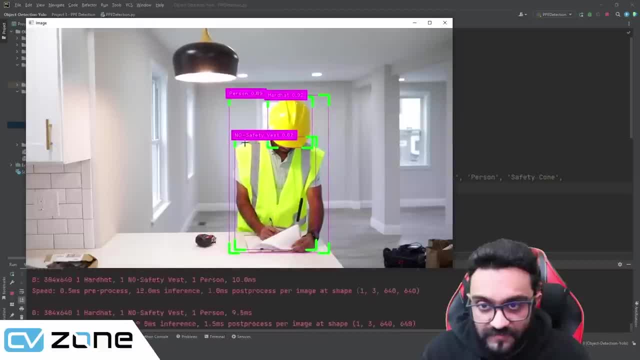 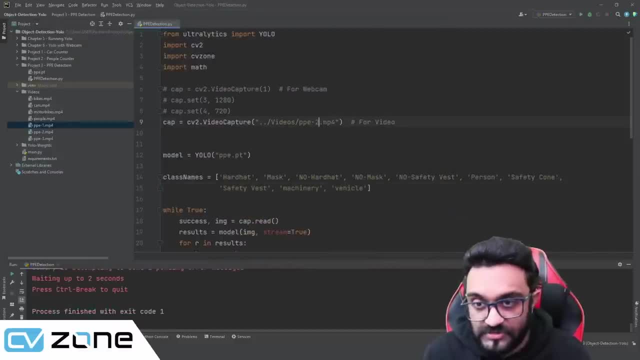 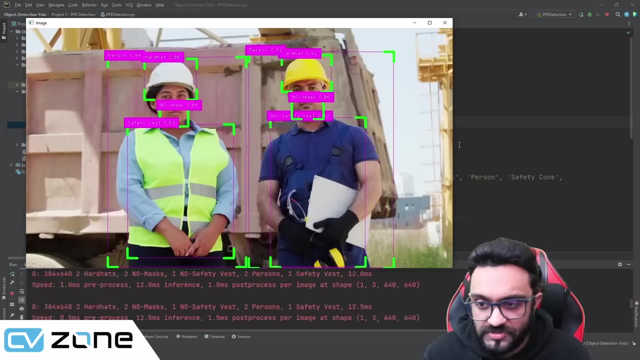 no mask and you can see it also detects safety or no safety vest. so it's not the most accurate, but it is giving us some, uh, good readings. so what you can do is you can train it, uh, with more data set and for longer epochs, for more epochs, to get better results. 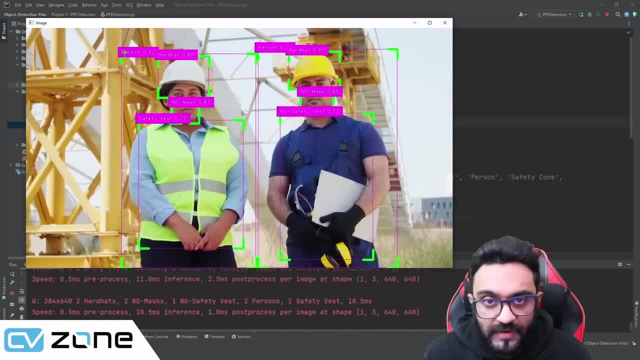 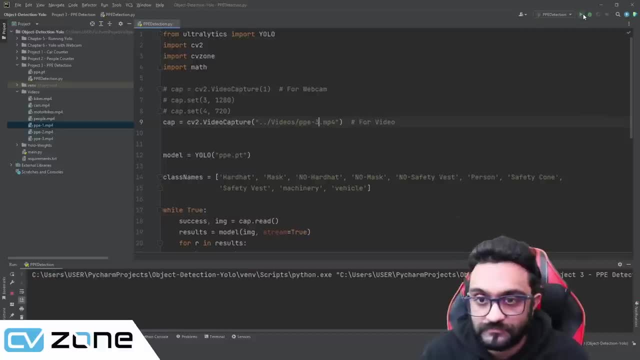 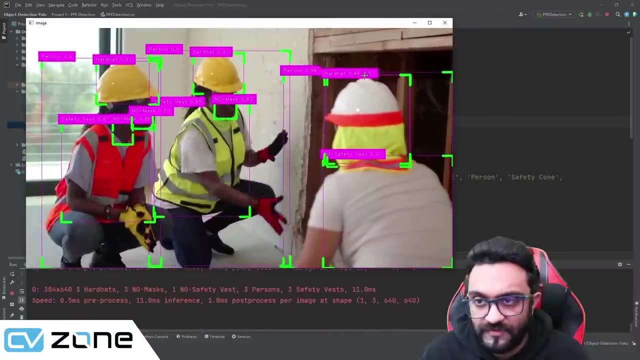 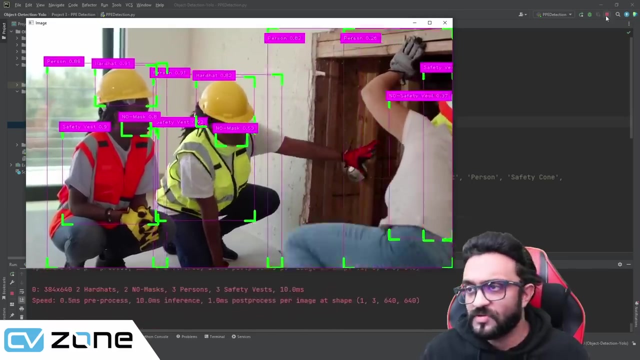 so here you can see: safety vest- no mask, hard hat and person- person, hard hat, no mask. and there you go. uh, let's try for number three. there you go, we have safety vest, hard hat, person- no safety west. here we have no mask. safety vest: harder- okay, so what we can do is: uh, this is a little bit. 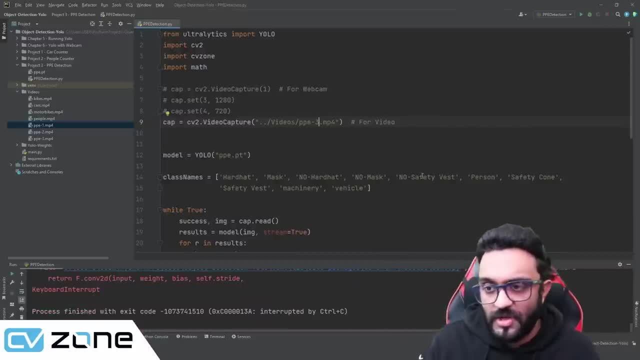 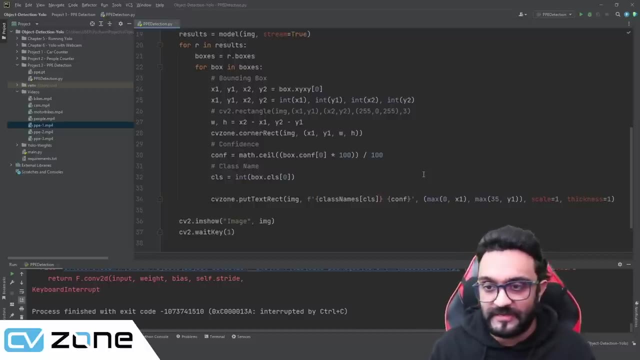 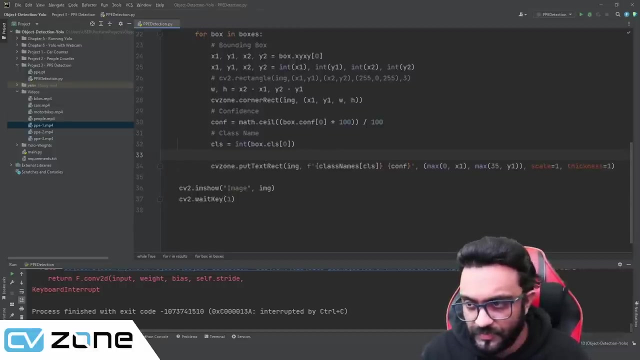 difficult to see what exactly is being detected or and what's not being detected. so what we can do is we can check which classes are we detecting and based on that we can assign a color. so here we can put a normal rectangle, or do we need to put yeah? 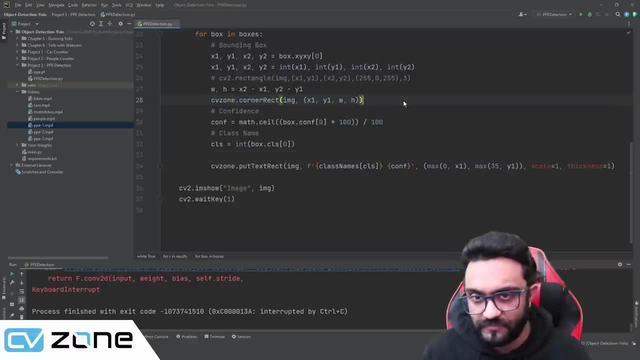 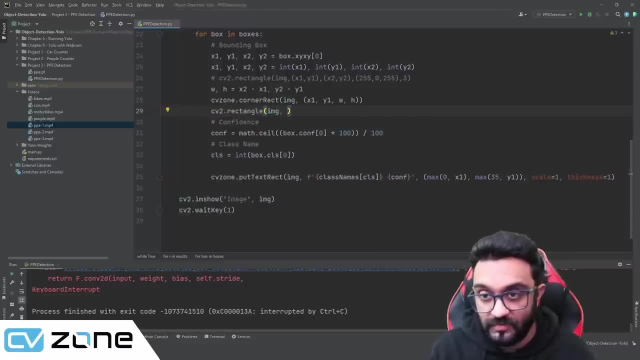 let's put a normal rectangle instead of the corner rect. so we will write here: cv2, dot rectangle and image and we will give in the X 1, Y 1 and the X 2 and the Y 2, and then we are going to give in the color. so this will be my color. let's say: 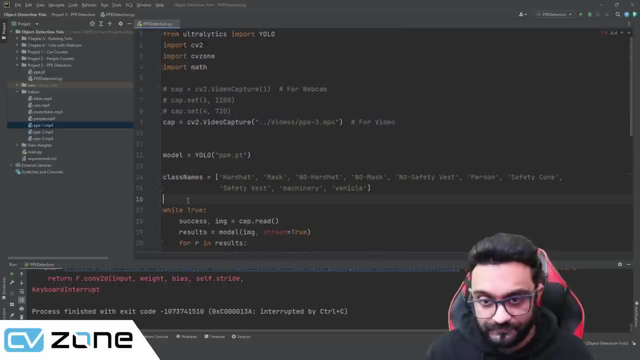 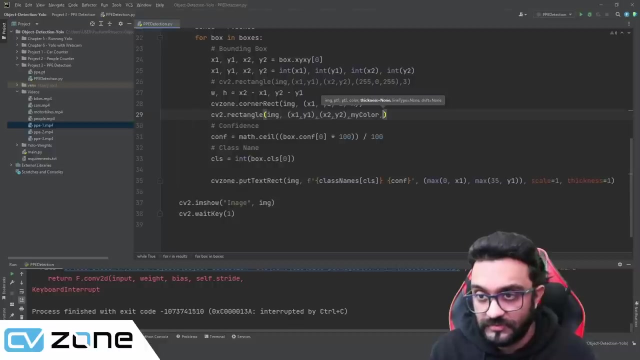 my color. so, by default, my color, my color, equals red. so 0, 0, 2, 5, 5. and then we are going to write down the thickness. the thickness, let's say it's 3, and that's pretty much it so. and then for: 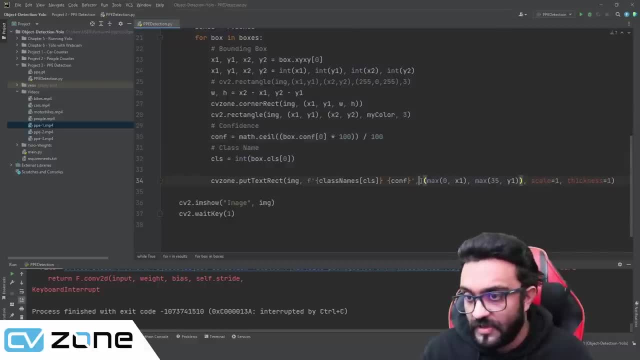 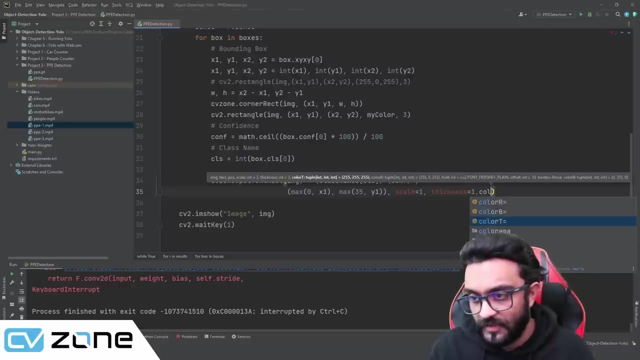 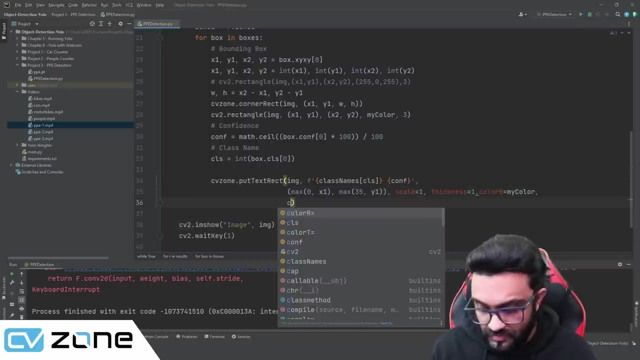 this part here. put text rect. we are also going to assign the color color for the rectangle or color for the background and color for the text. so the color for the background, let's make it my color, and for the text, we have to make it white color for the text we are going to. 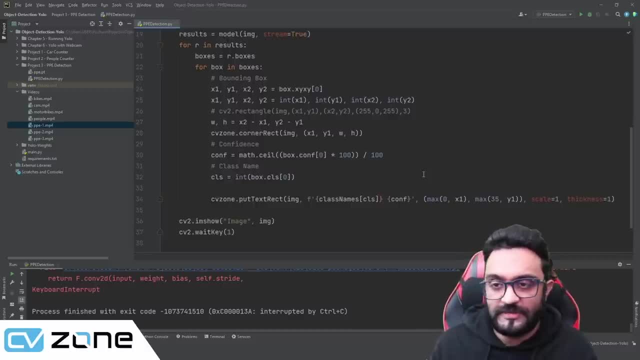 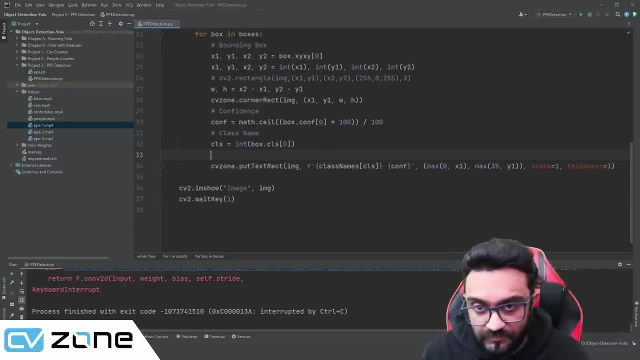 we can check which classes are we detecting and based on that we can assign a color. so here we can put a normal rectangle, or do we need to put? yeah, let's put normal rectangle instead of the corner rect. so we will write here: cv2.rectangle and image. 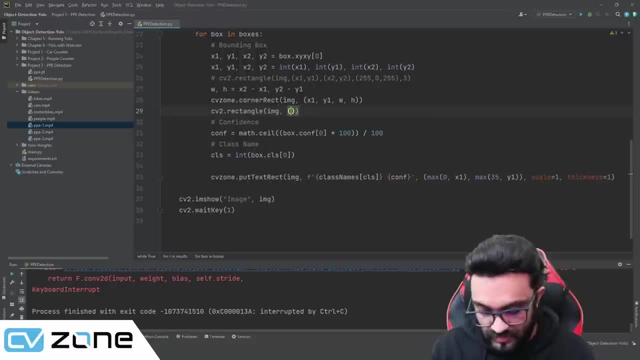 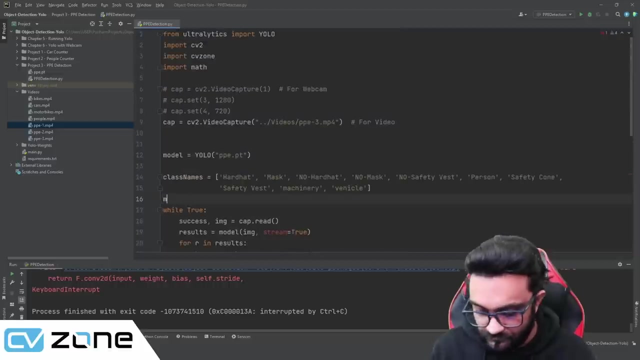 and we will give in the x1, y1 and the x2 and the y2, and then we are going to give in the color. so this will be my color, let's say my color. so by default, my color, my color, equals red, so 00255. 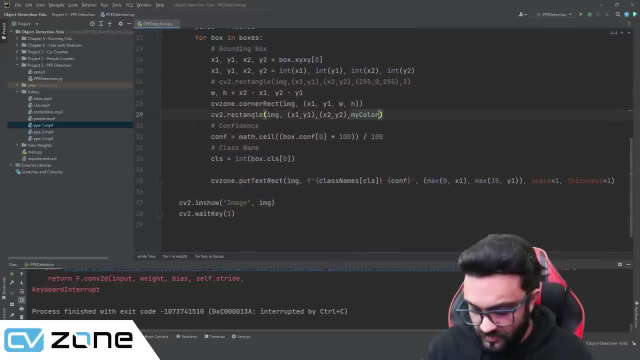 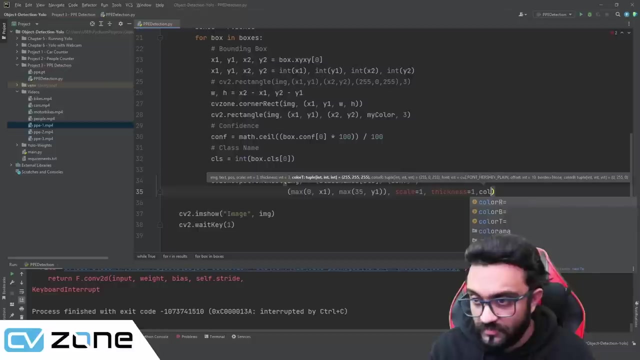 and then we are going to write down the thickness. the thickness let's say it's 3 and that's pretty much it so. and then for this part here, put text rect. we are also going to assign the color: color for the rectangle or color for the background. 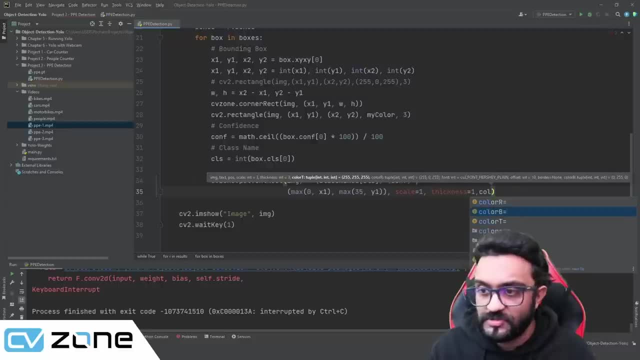 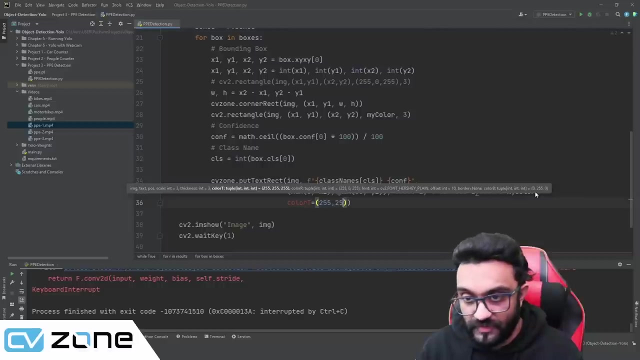 and color for the text. so the color for the background: let's make it my color, and for the text: we have to make it white. color for the text: we are going to make it white. so 255, 255 and 255. so let's run this. 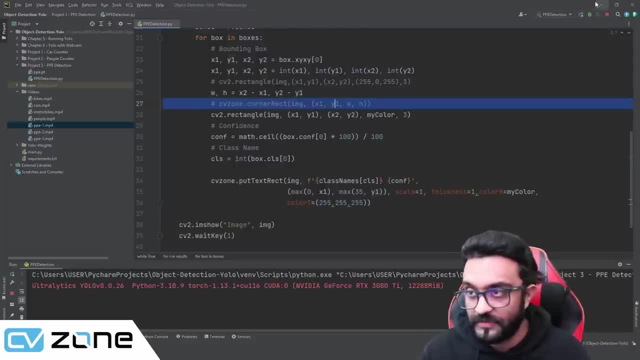 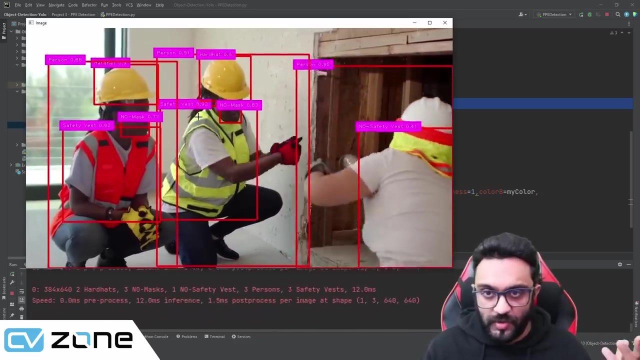 and see what happens. now we need to remove the corner rectangle. so what we are trying to do is that it should detect, it should show us the red color and, in the case where there's no mask or no hard hat, and in case it is present, it should give us green. 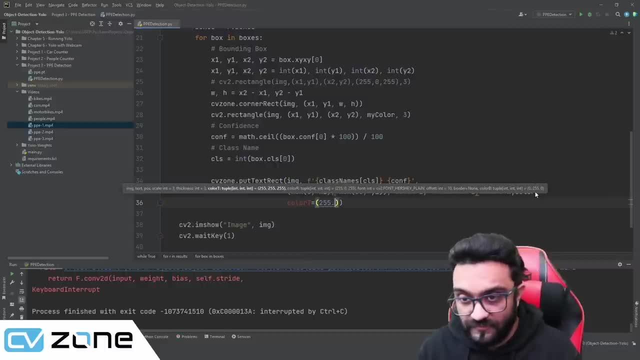 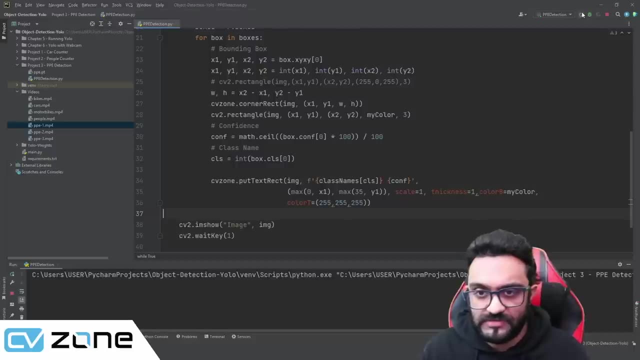 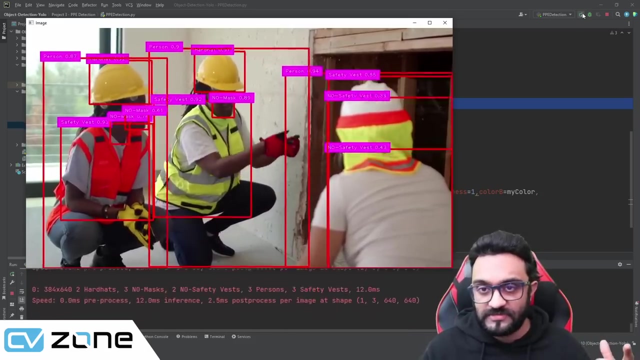 make it white. so 2, 5, 5, 2, 2, 5, 5 and 2, 5. so let's run this and see what happens. now we need to remove the corner rectangle. so what we are trying to do is that it should detect, it should show us the red color and, in the case where there's, 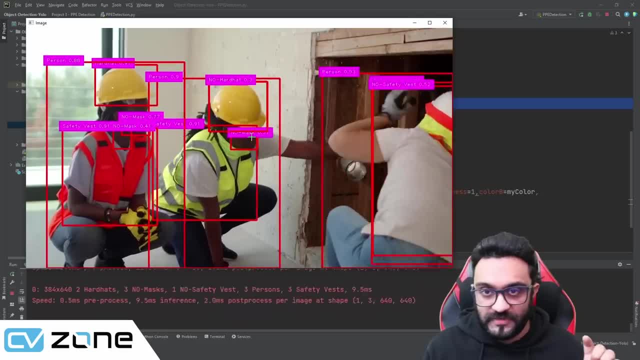 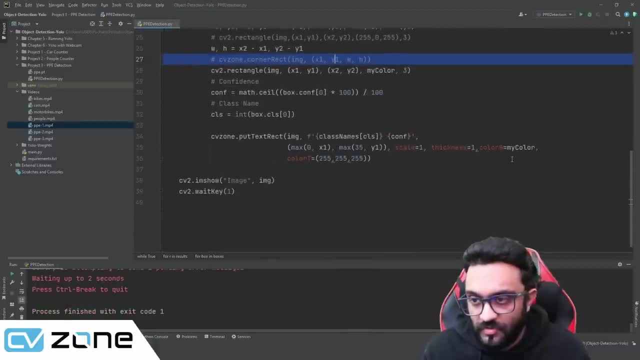 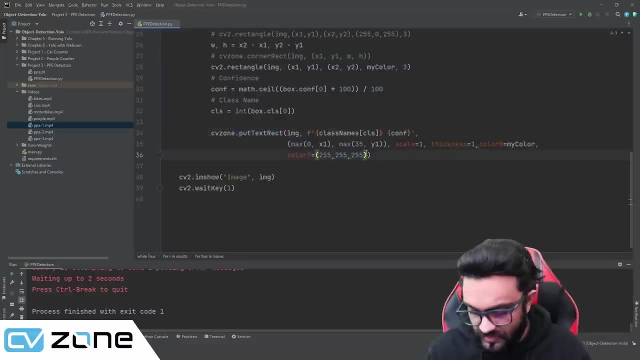 no mask or no hardhat and in case it is present, it should give us green. so okay, so yeah, now it's my color is showing, but it didn't show for the put text rect. let's put it for the color rect, as my color as well. 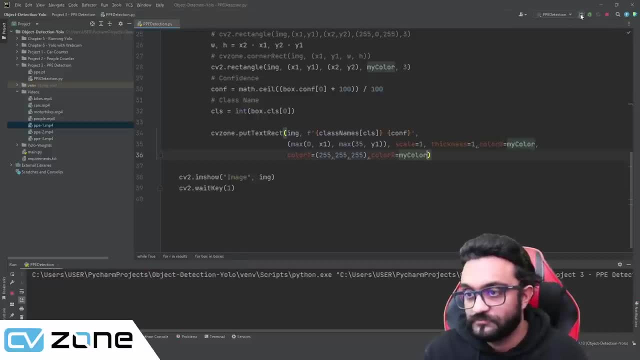 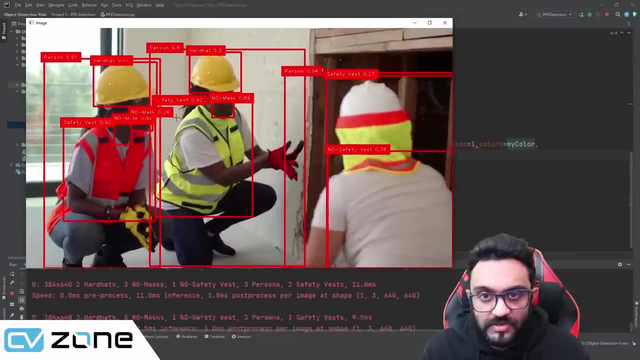 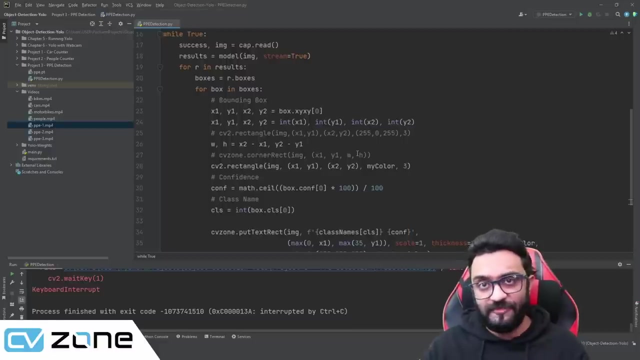 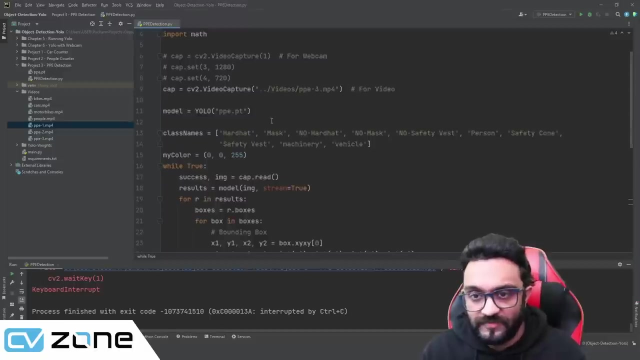 yeah, now it's good. so it's showing red for all of these. so now we need to make sure if, by default, it will be red. if we are detecting one of those classes that have the green, then it should detect green. for example, we have the hardhat. we 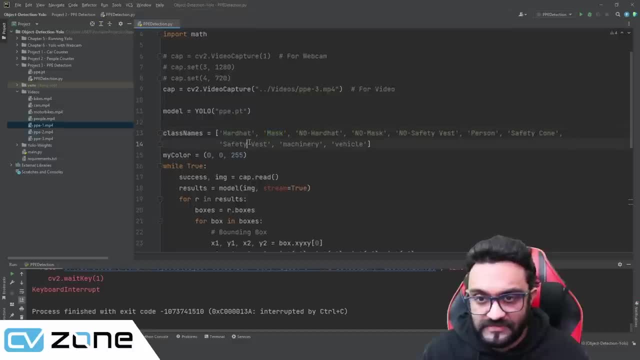 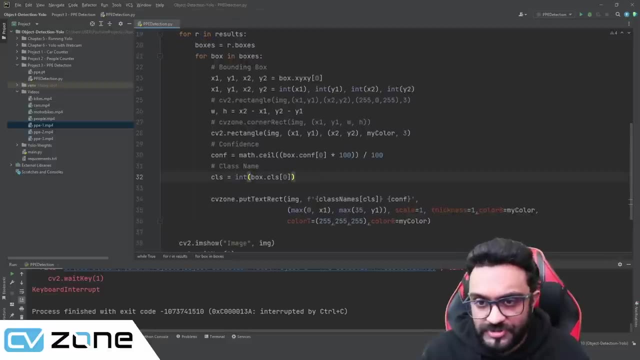 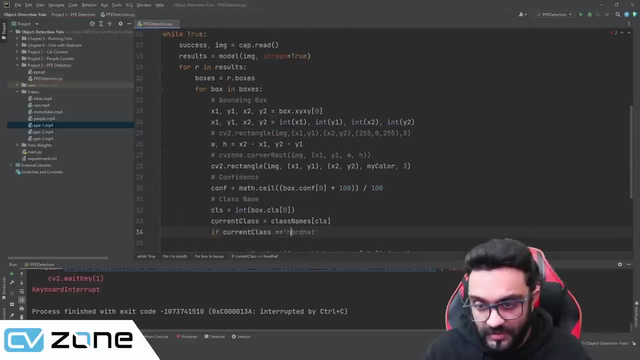 have the mask and we have the safety vest. so these are the three classes. so what we will do is we are going to check now. first of all, we will write here: current class equals class names at CLS. and if current class equals hard hat, is it capital? yes, hard hat. and. 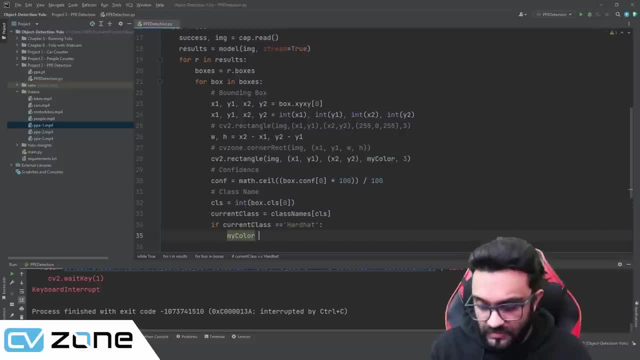 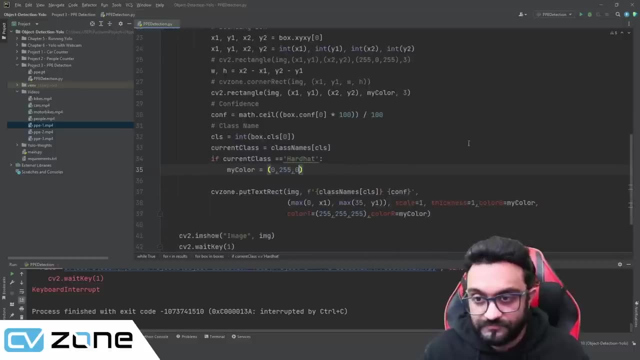 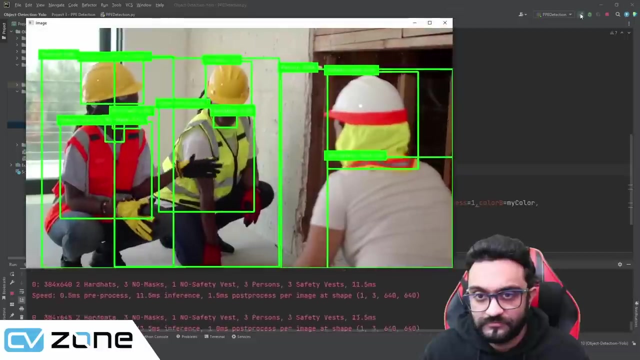 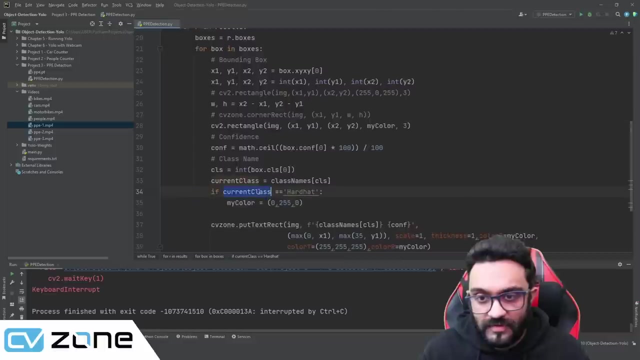 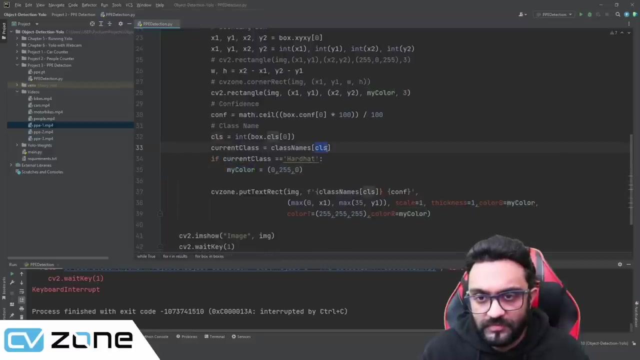 then my color equals zero, two, five, five and zero. let's try that out. so now all of them are green. so what's the issue? if current class equals hardhat, my color is 0, 2, 5, 5. current class is coming from here for text and we need to give it after so the 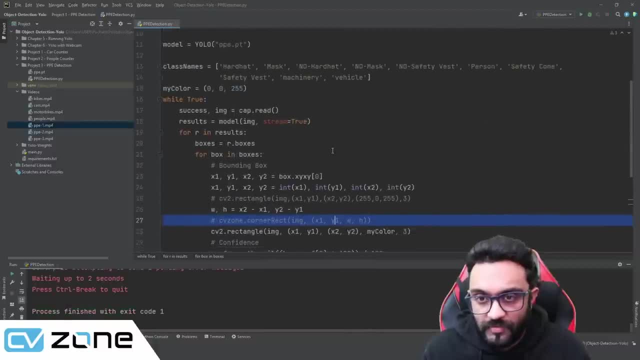 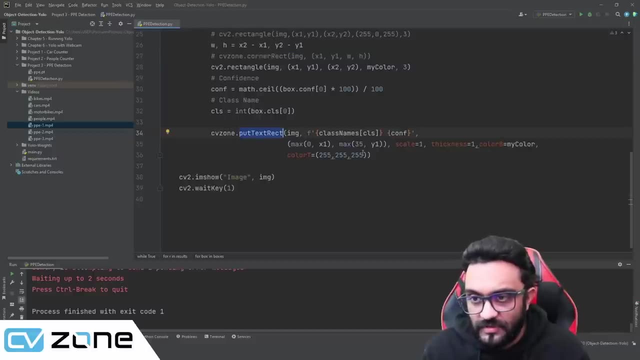 so okay. so yeah, now it's my color is showing, but it didn't show for the put text- rect. let's put it for the color rect as my color as well. yeah, now it's good. so it's showing red for all of these. so now we need to make sure. 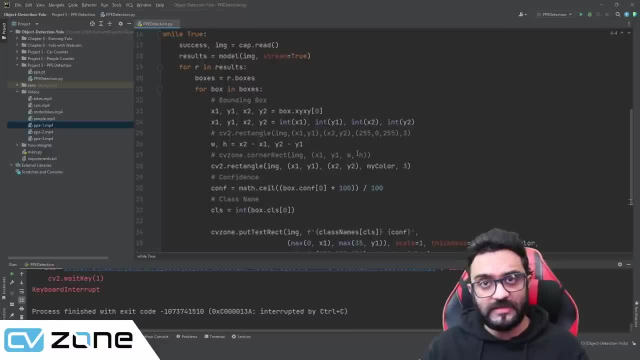 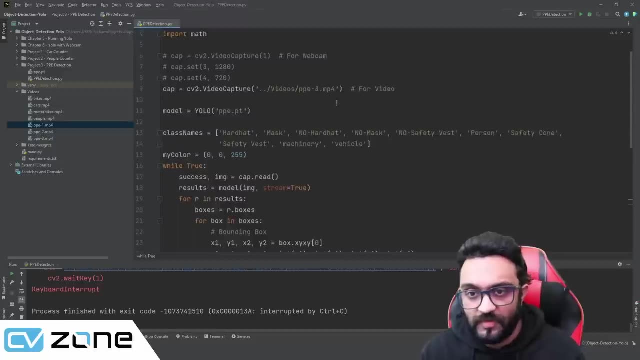 if, by default, it will be red. if we are detecting one of those classes that have the green, then it should detect green. for example, we have the hardhat, we have the mask and we have the safety vest. so these are the three classes. so what we will do is: 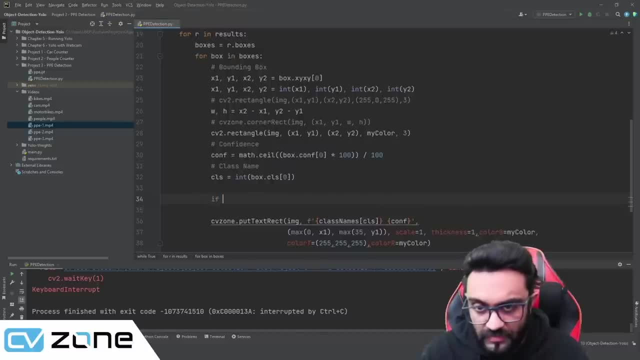 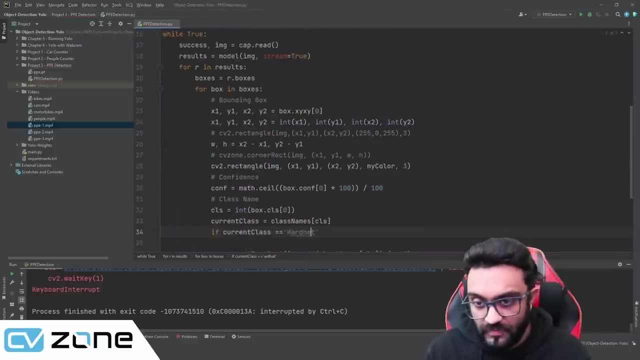 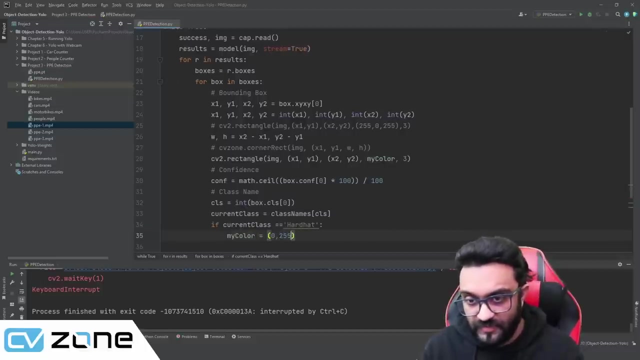 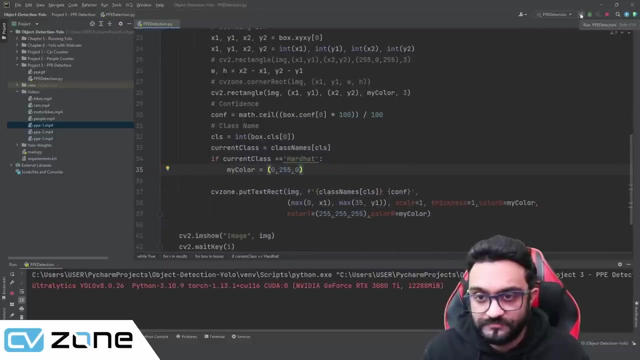 we are going to check now. first of all, we will write here: current class equals class names at cls, and if current class equals hard hat, is it capital? yes, hardhat. then my color equals 0, 2, 5, 5 and 0. let's try that out. 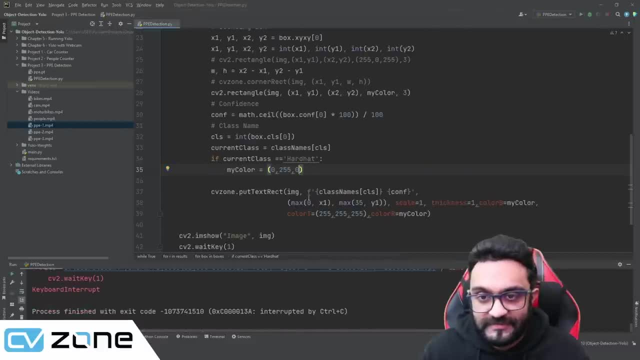 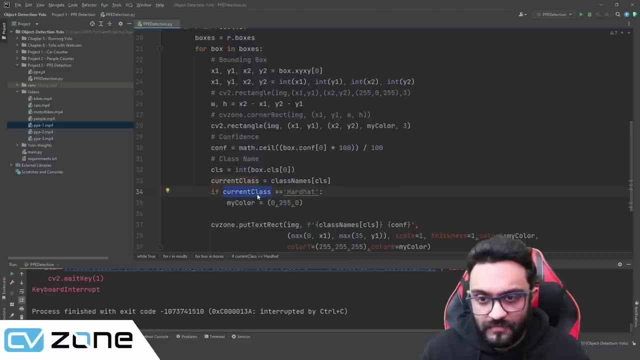 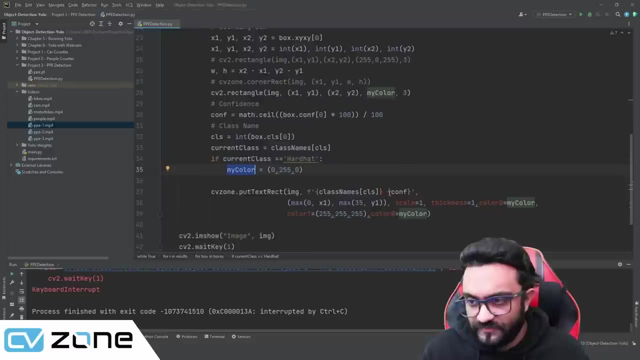 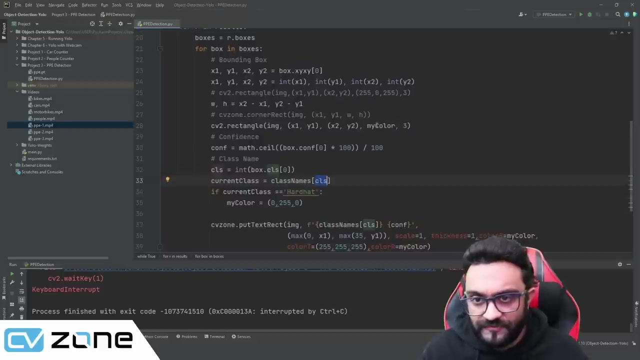 so now all of them are green. so what's the issue if current class equals hardhat? my color is 0 2, 5, 5 um. current class is coming from here for text and we need to give it after so the rectangle, because this has my color. 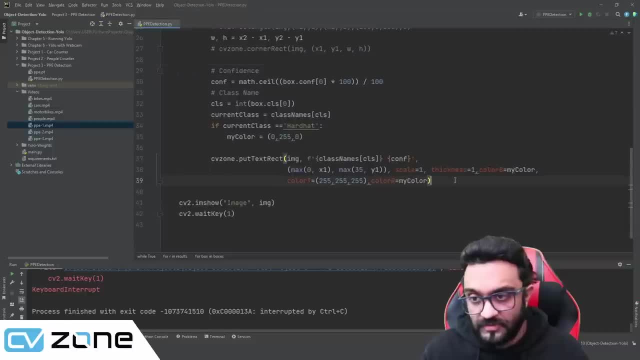 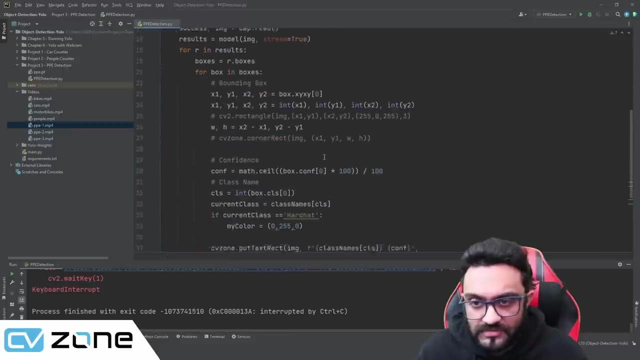 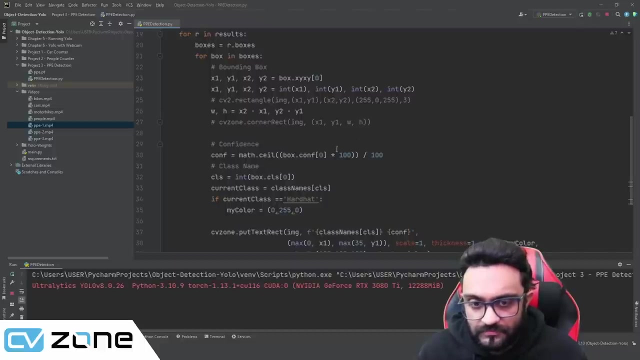 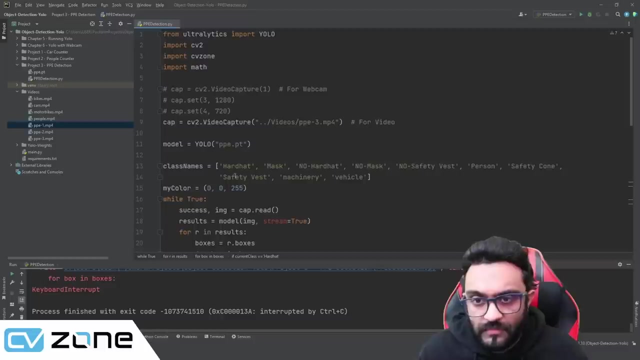 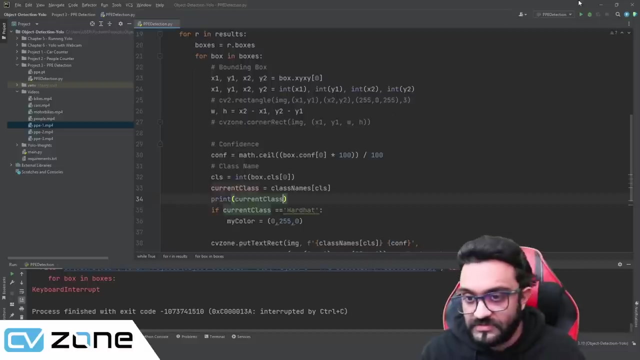 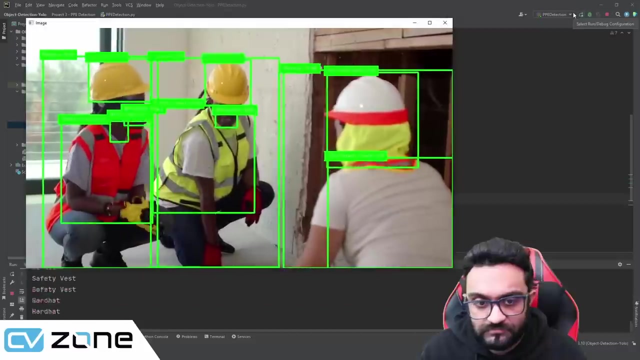 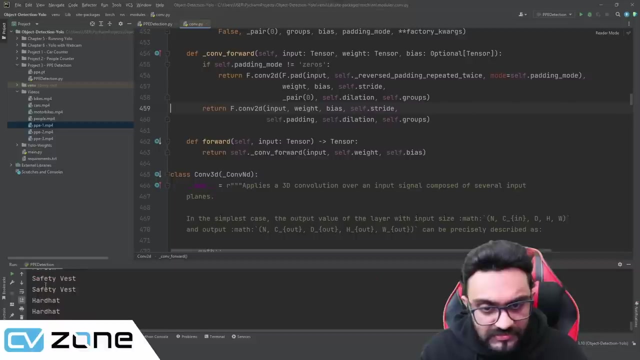 rectangle, because this has my color, needs to be here, so you will put it here. and current class equals hard hat, hard hat. why did it show all of them green? that's weird. let's print the current class. so when we are printing the current class, it shows person safety. 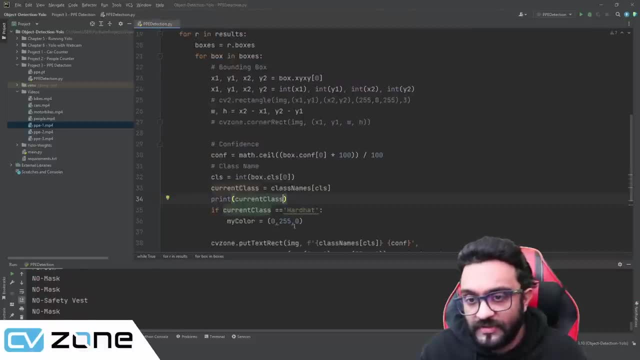 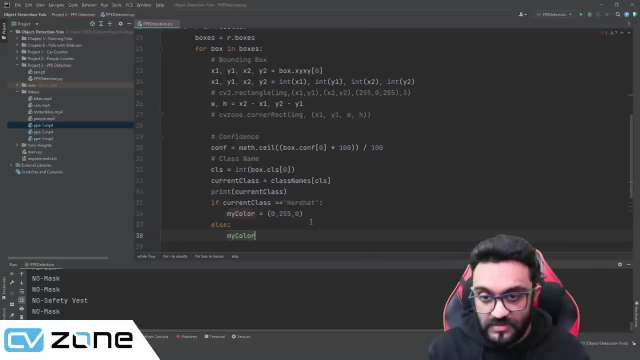 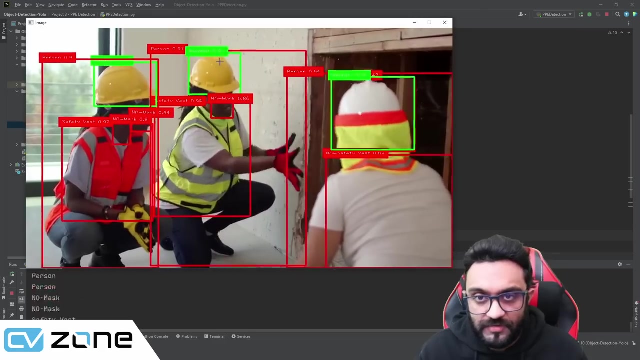 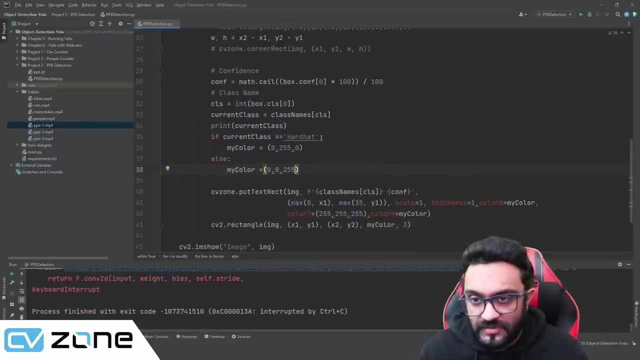 value: best safety, best, safety, best. oh, we need to write else, uh else, because it's not changing after that. my color equals: my color equals: uh, zero, uh, two, five, uh, zero, zero and two five, five. now, hopefully it will be better. yeah, so there you go. we have green for hard hat and the rest are red. okay, so if my current class 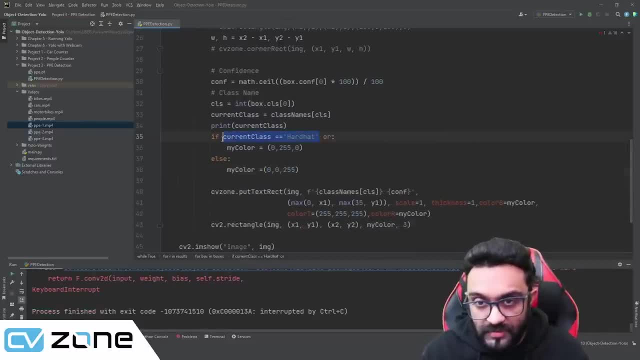 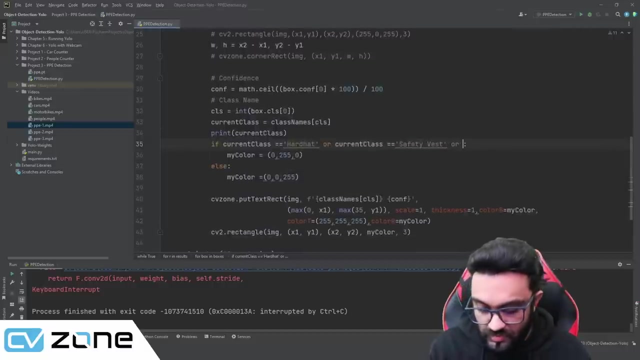 is hard hat, or my current class is safety vest. uh, safety vest and mask, or my current class equals visuals mask. then it is this. otherwise the rest of them are red. um, and what else can we do? we can make it smaller because scale is not that good. um, we are using the put text rect. we can make the. 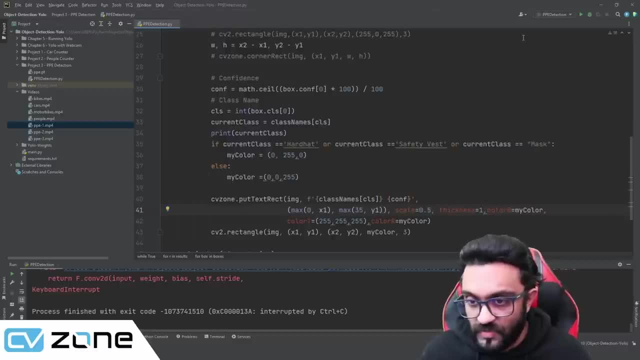 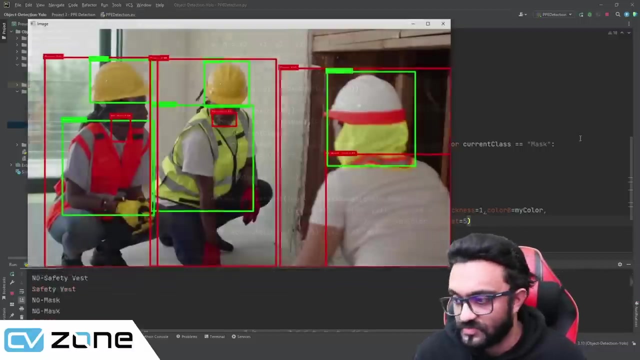 scale, 0.5, let's say, and the thickness is one, that's fine, um, and the offset, offset. let's make it 5 instead of 10, so it will be a little bit smaller, so that it's easier to know what is going on. uh, there you go it's. there's a lot of overlap, that's why it's a little bit. 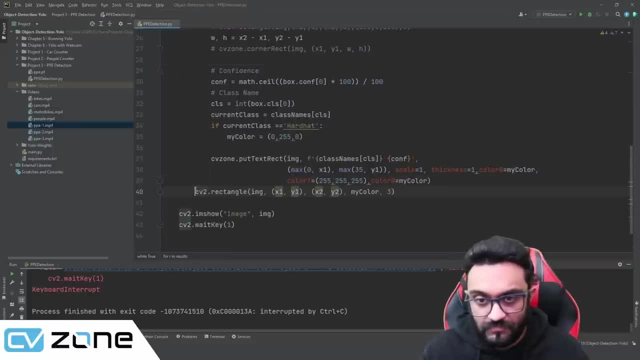 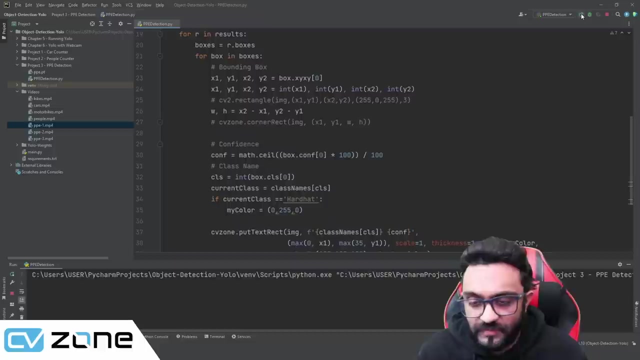 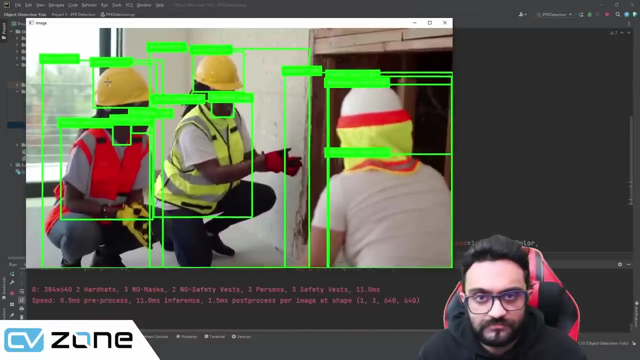 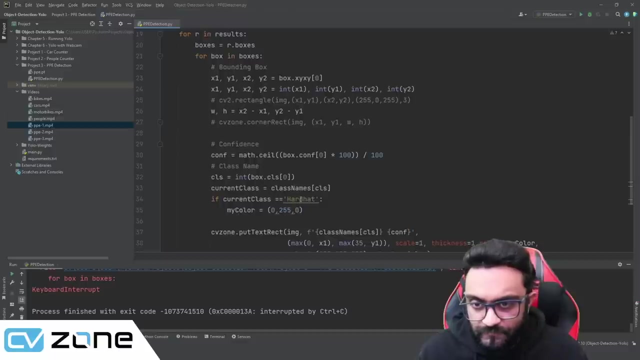 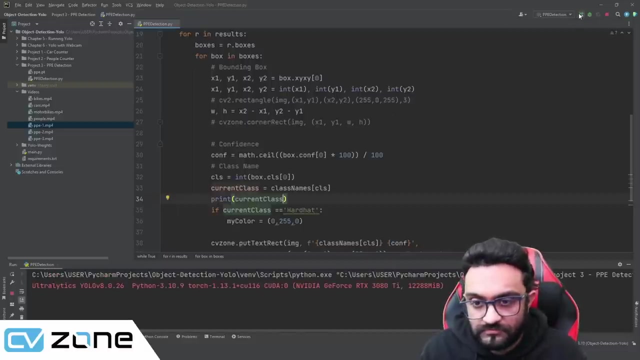 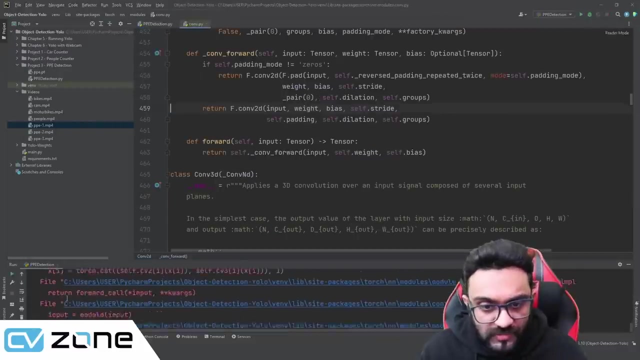 needs to be here, so we will put it here. and then current class equals hardhat, hardhat. why did it show all of them green? that's weird. let's print the current class. so when we are printing the current class, it shows person safety vest, safety vest. 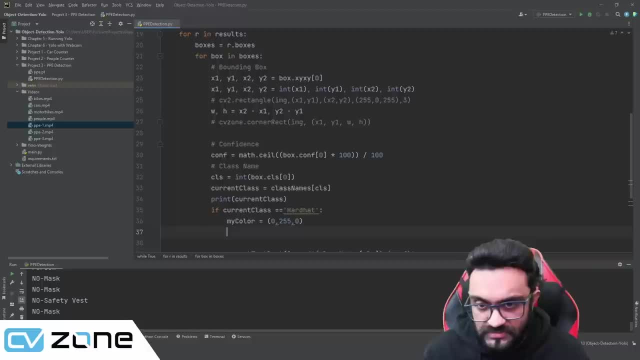 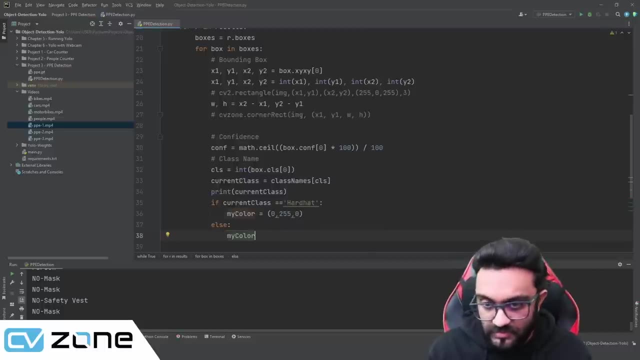 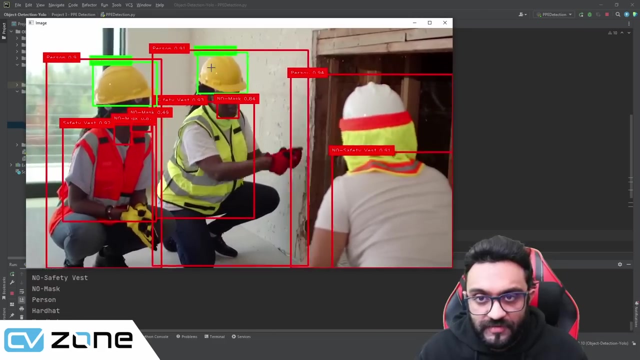 safety vest. oh, we need to write else, uh, else, because it's not changing after that. my color equals. my color equals uh, 0, uh, 0, 0 and 255. now, hopefully it will be better. yeah, so there you go, we have green for hardhat. 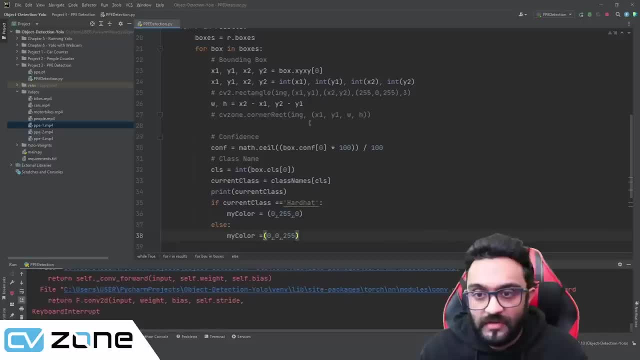 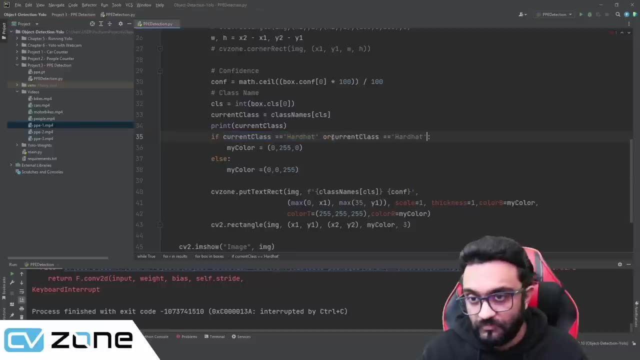 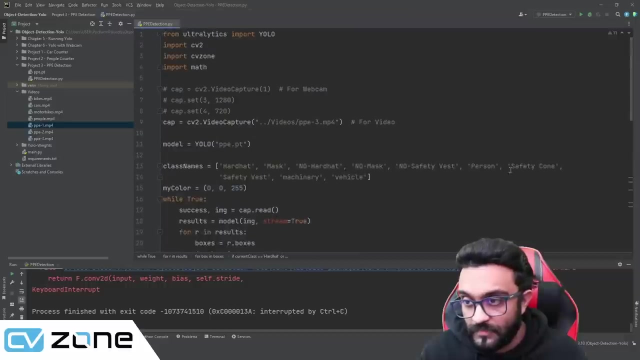 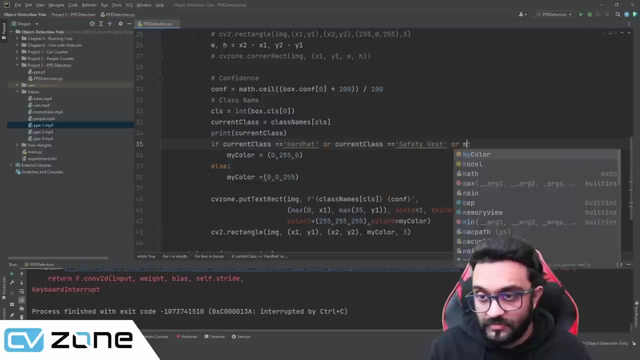 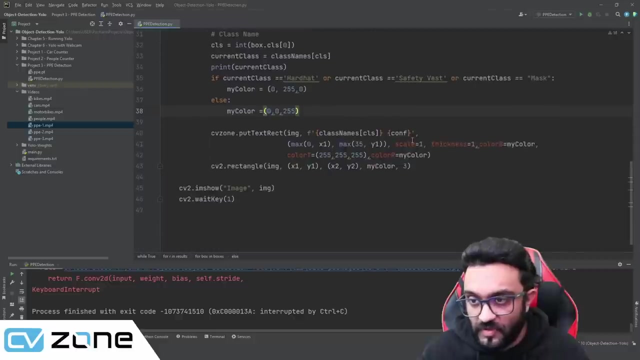 and the rest are red. okay, so if my current class is hardhat or my current class is safety vest- uh, safety vest and mask, or my current class equals mask, then it is this. otherwise the rest of them are red. um, and what else can we do? we can make it smaller because 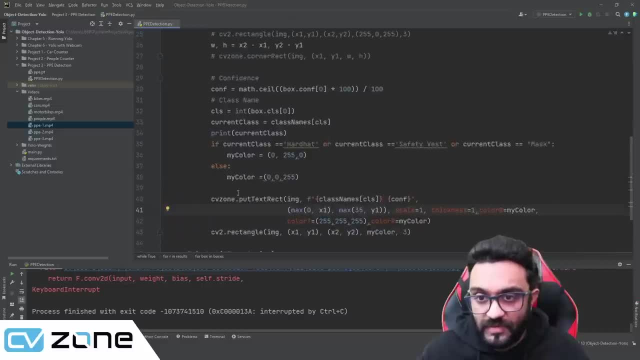 scale is not that good. um, we are using the put text rect. we can make the scale 0.5, let's say, and the thickness is one that's fine. um, and the offset, offset. let's make it 5 instead of 10.. so it will be a little bit smaller. 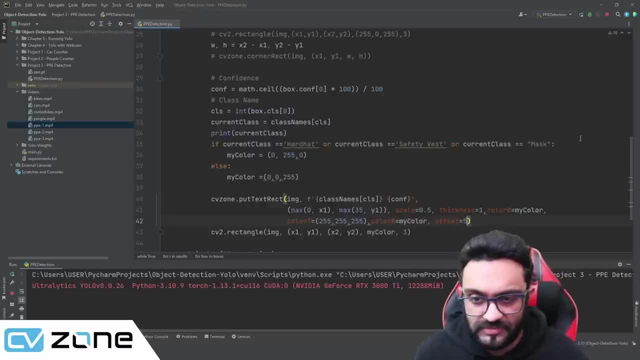 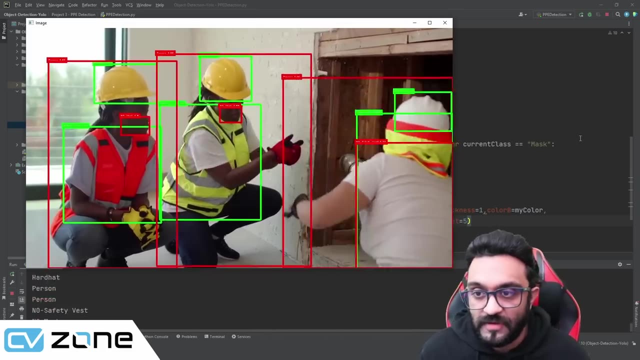 so that it's easier to know what is going on. uh, there you go it's. there's a lot of overlap, that's why it's a little bit confusing, but you can see that when it's uh, the hardhat it's detecting, it's showing a screen. 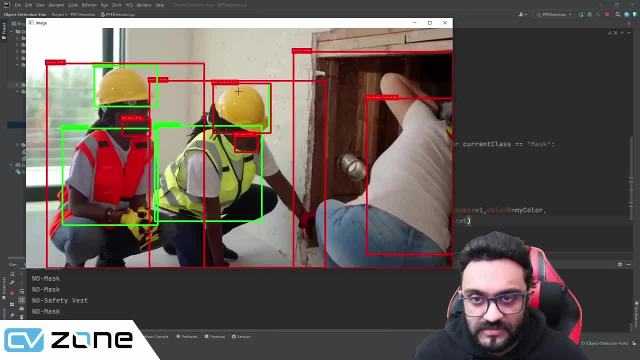 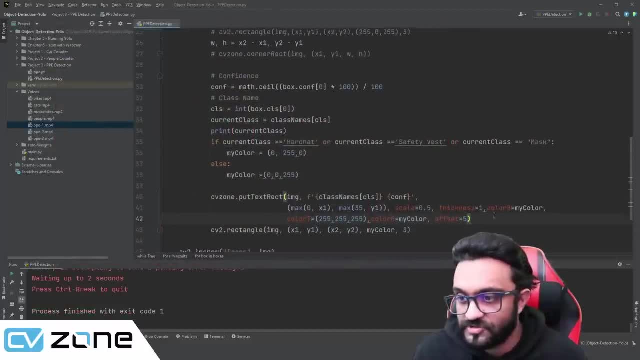 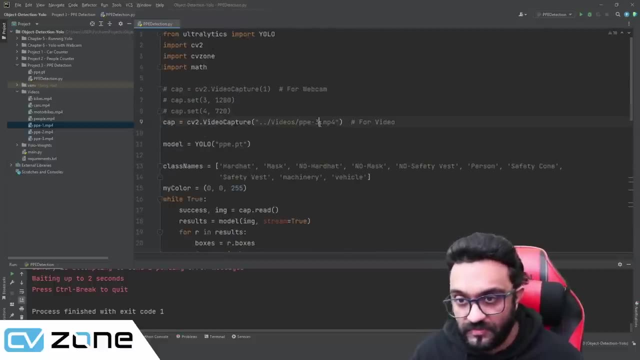 confusing, but you can see that when it's, uh, the hard hat it's detecting, it's showing us green. when it's not, it's showing us red. uh, let's try it. actually the scale is very small, um, so, let's try one and let's try another video. the first one was the most clear. 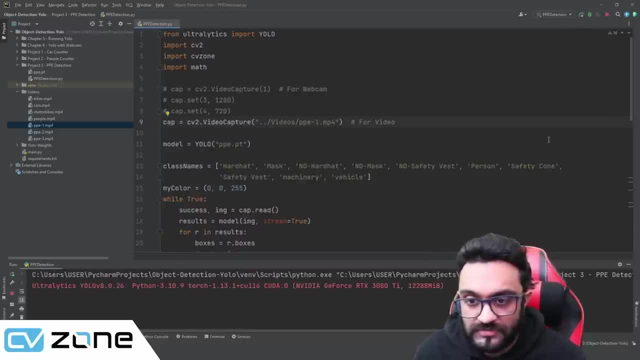 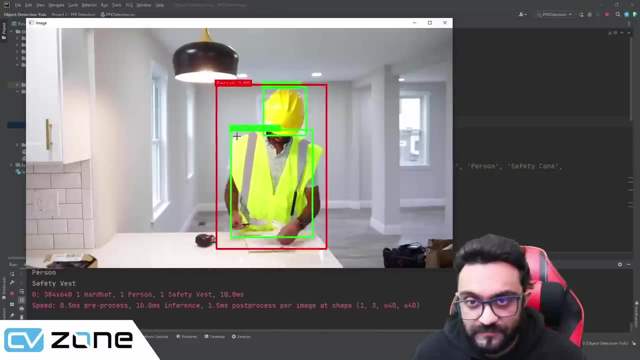 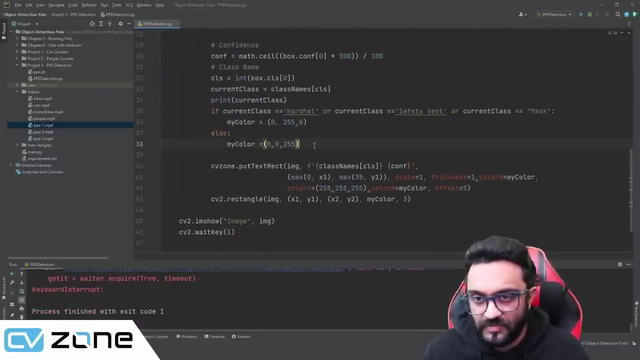 let's try that one out. there you go. so we have the hard hat, we have the person, no mask and safety vest, uh, or what we can do is we can assign a third color as well, because if it's a person, then we don't need to worry about that. so all the red colors and all the green colors, and then we give. 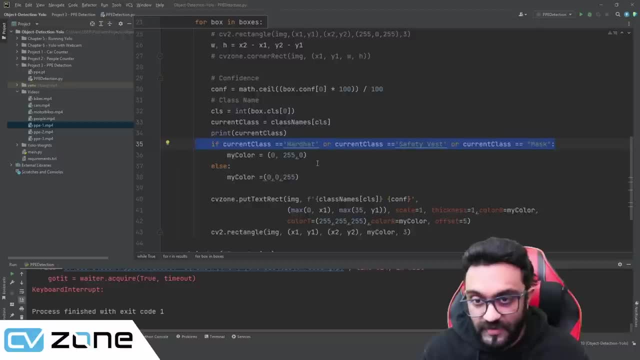 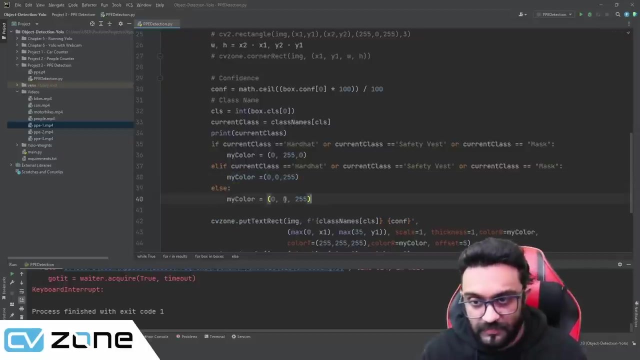 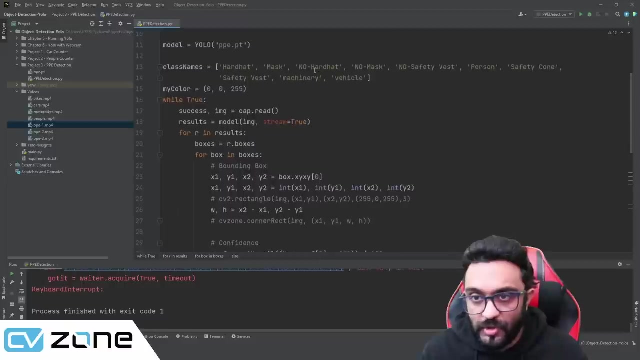 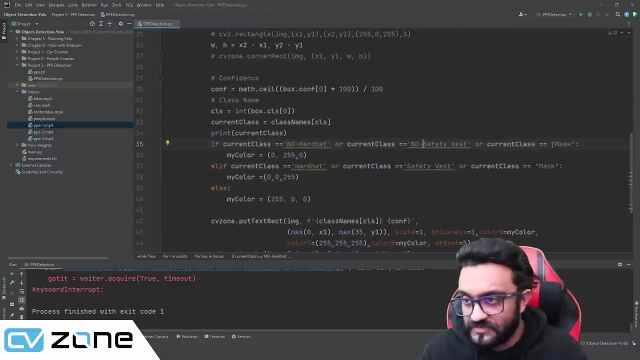 an else. so if it's current mask and all of that, we can assign a third color as well, then we can write else, if else, if, and then we can write else else. my color is purple, or let's say, blue, two, five, five, zero and zero. okay, so, uh, it's no hard hat, no hard hat, and no safety vest and no mask. 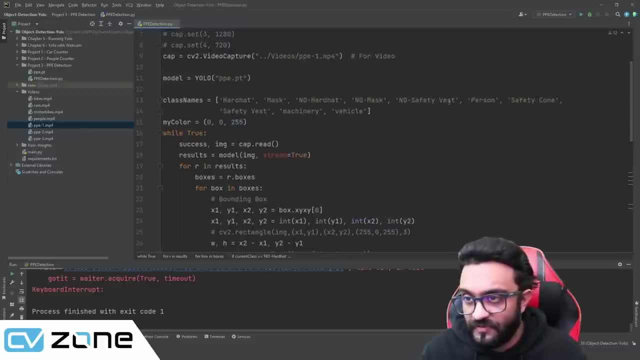 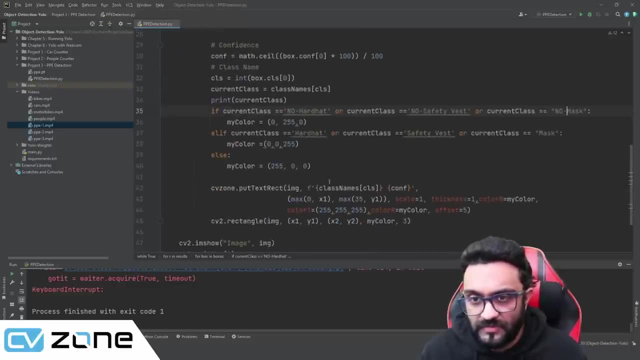 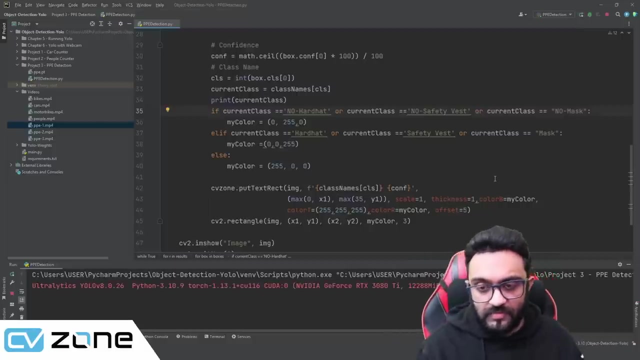 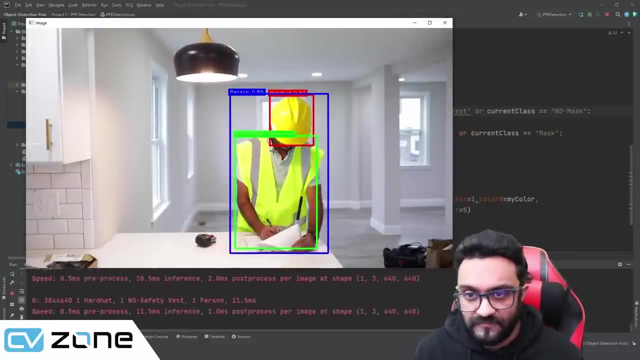 yep, these are the ones for red. uh, then safety cone, safety vests- we don't really care about that. the the rest are blue, so let's run that. so the person now should be blue and we should have green, for okay, it's opposites, hard hats, safety vests, and we also need to give in. 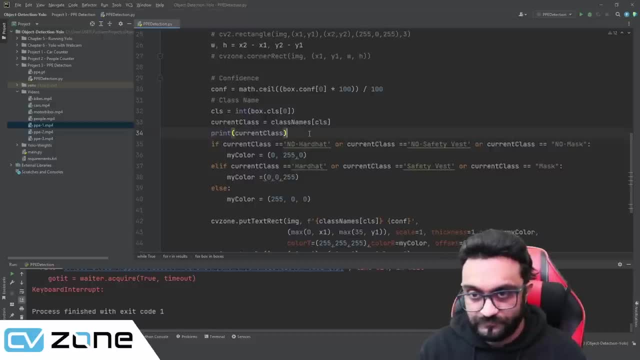 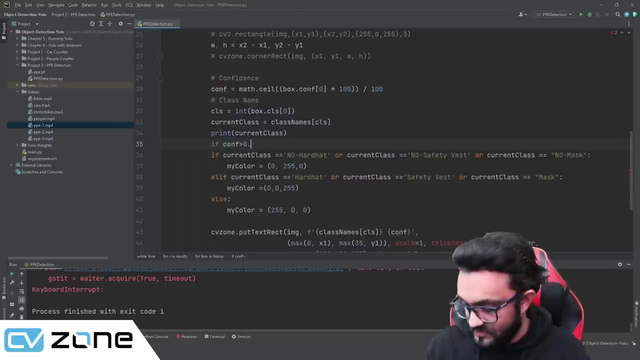 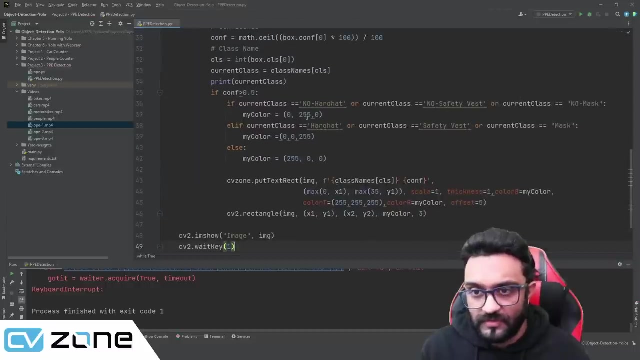 maybe a threshold so that we don't get a lot of wrong detections. if the confidence level is greater than 0.5, let's say, then only we'll do all of that. so yeah, we were talking about the color, so no hard hat. uh, all of this is is supposed to be red. 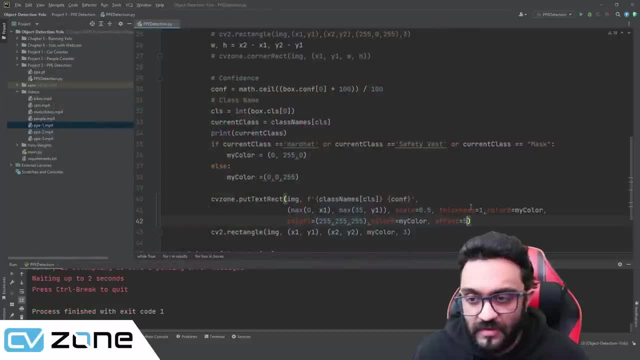 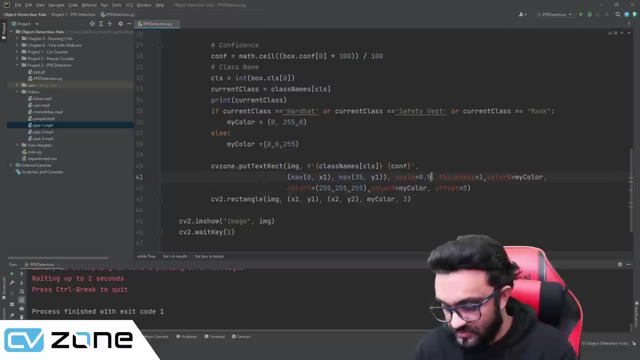 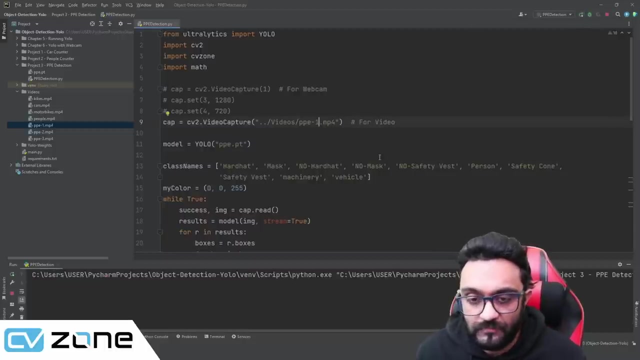 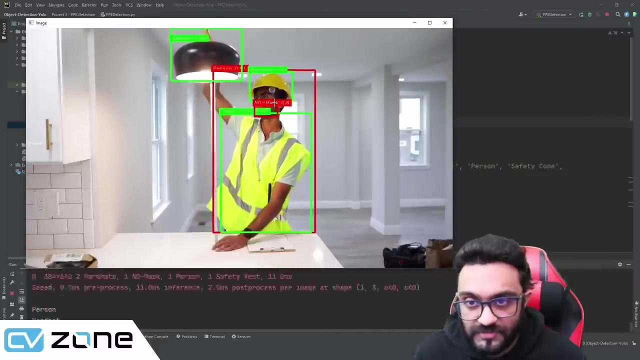 when it's not, it's showing us red. uh, let's try it. actually, the scale is very small, so let's try it. uh, so let's try one. and let's try another video. the first one was the most clear. let's try that one. out, there you go. so we have the hardhat, we have the person. 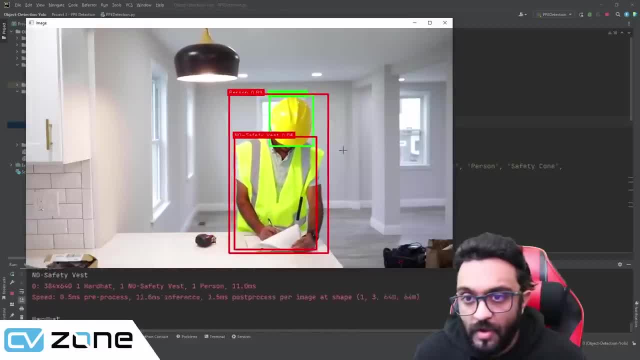 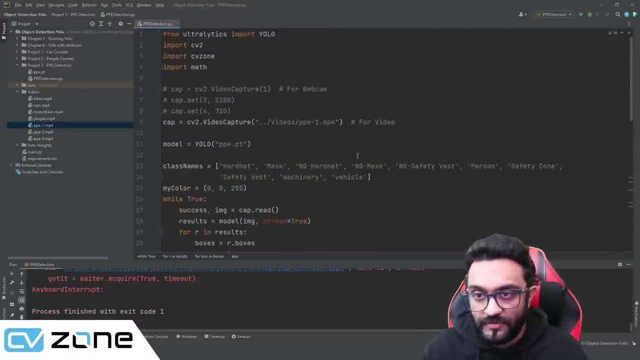 no mask and safety vest. uh, or what we can do is we can assign a third color as well, because if it's a person, then we don't need to worry about that. so all the red colors and all the green colors, and then we give an else. 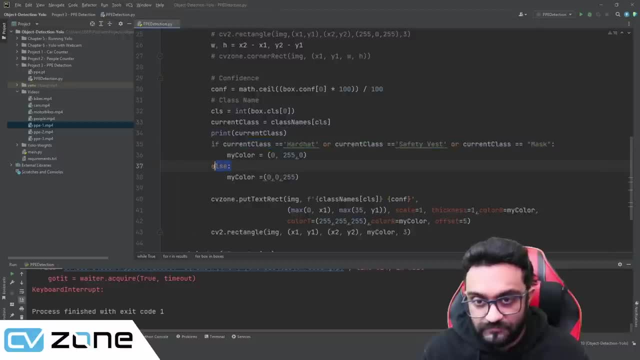 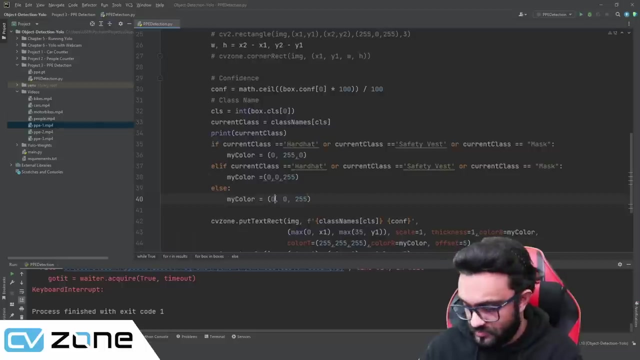 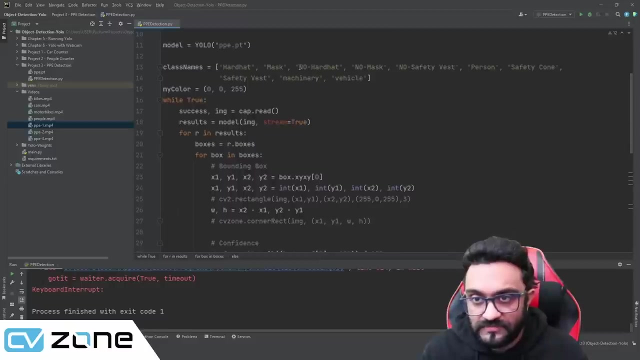 so if it's current mask and all of that, then we can write else, if else if, and then we can write else else. my color is purple, or let's say, blue. two, five, five, zero and zero. okay. so, uh, it's no hardhat, no hardhat. 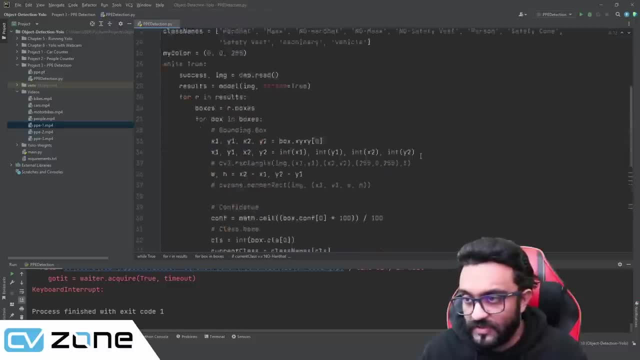 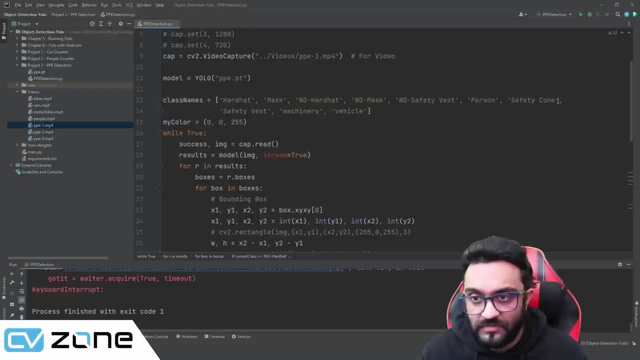 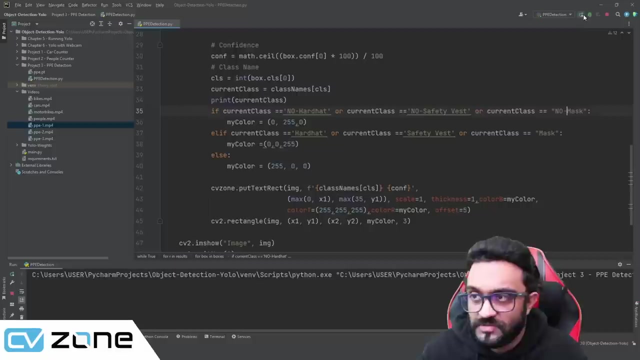 and no safety vest and no mask. yep, these are the ones for red. uh, then, safety cone, safety vest, we don't really care about that. the the rest are blue, so let's run that. so the person now should be blue and, uh, we should have green for. 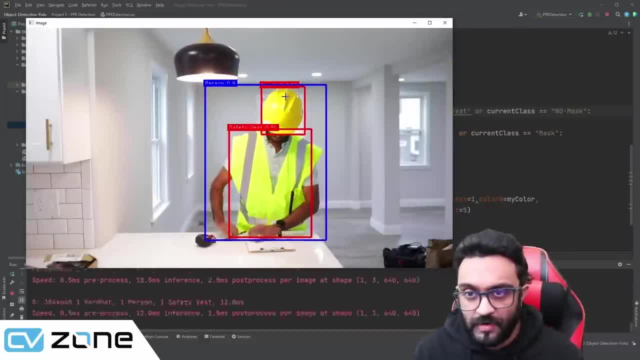 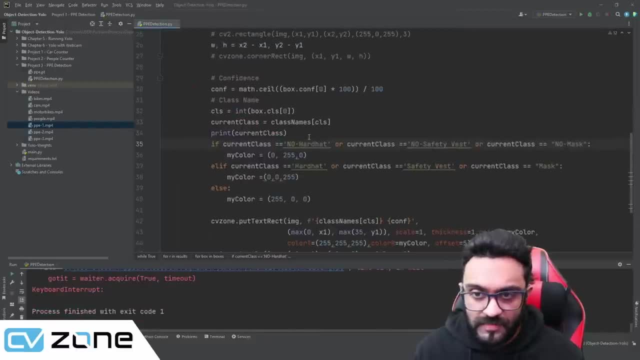 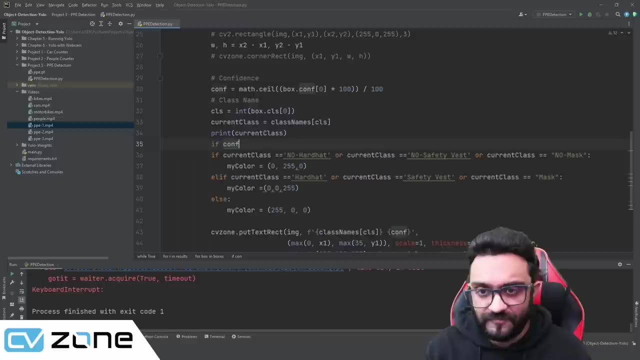 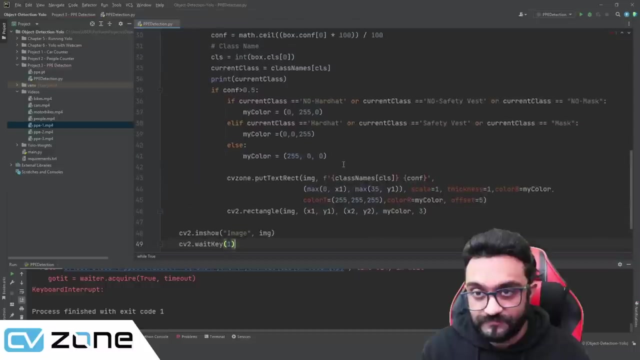 okay, it's opposite hardhat safety vests, and we also need to give in maybe a threshold so that we don't get a lot of wrong detections. if the confidence level is greater than 0.5, let's say, then only we'll do all of that. 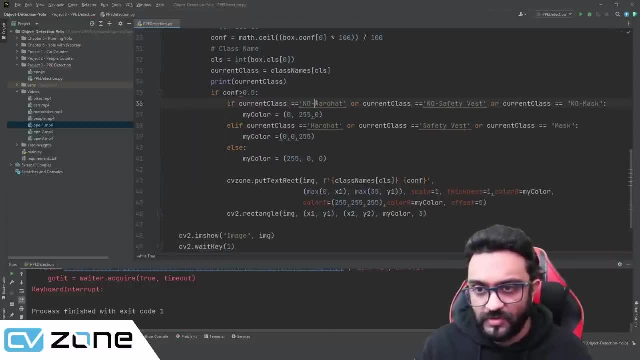 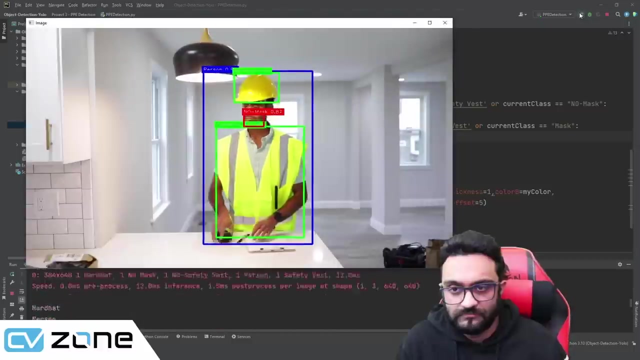 so yeah, we were talking about the color, so no, hardhat. uh, all of this is is supposed to be red, these are supposed to be green, so, and the rest are blue. let's run that again. there you go. so we have the safety vest, safety hardhat and the person. 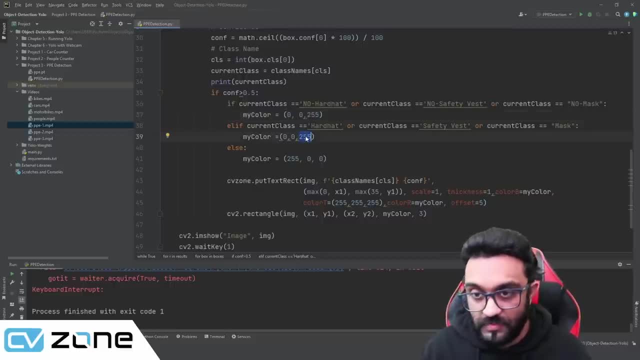 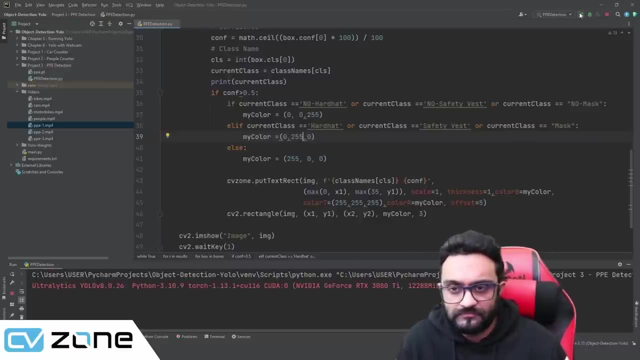 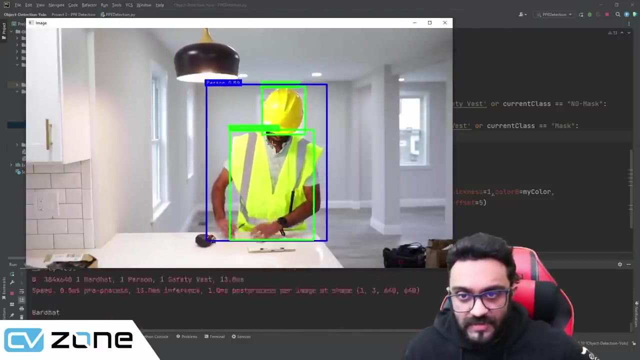 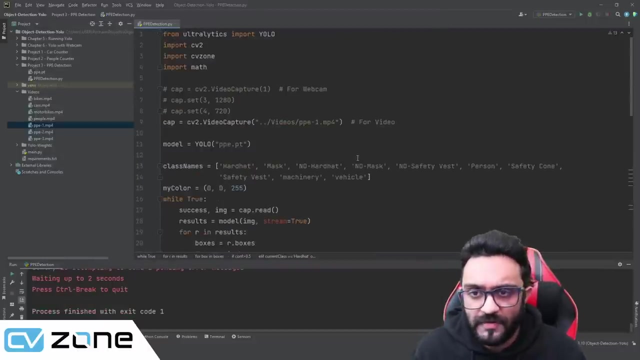 these are supposed to be green, so, and the rest are blue. let's run that again. there you go. so we have the safety vest, safety hard hat and the person, and then we have the no mask. so when it's not very clear it's not giving good results, but overall it seems to work fine. 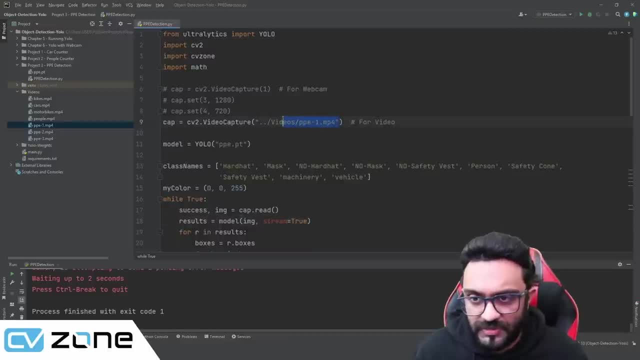 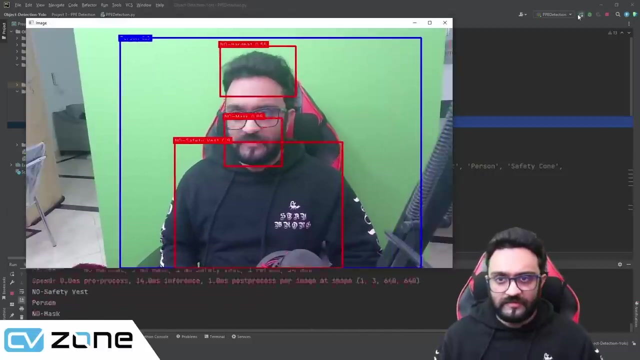 so now we can also try it with the webcam. so i will put it in the background, so i will put it in the it. okay, let's keep it for video and for webcam. we can open this up and let's try it out. so, as you can see, i'm not wearing a hard hat, no mask and no safety vest, but it's detecting the person. 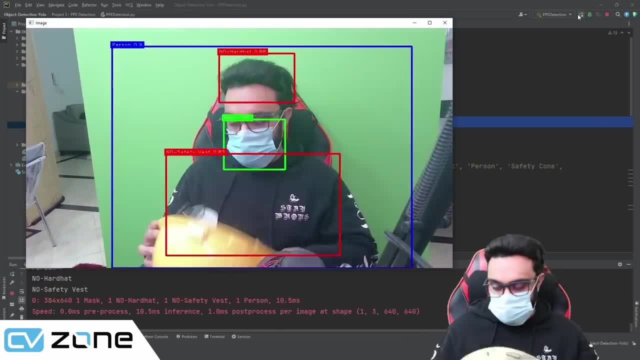 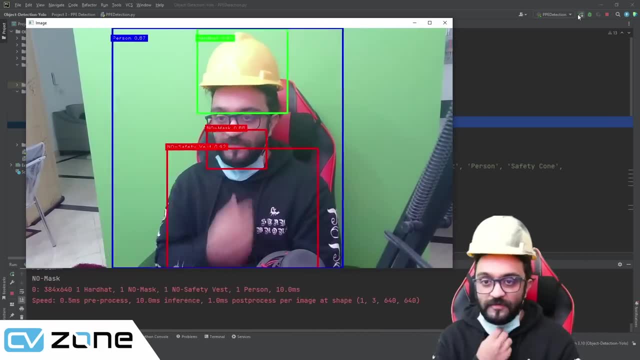 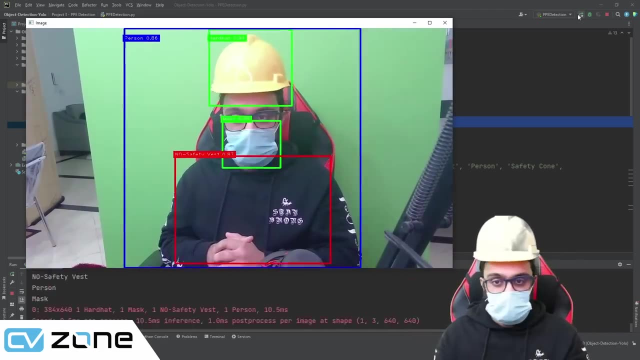 so if i wear a mask, you can see it's detecting the mask. and if i wear the hard hat, you can see it detects the hard hat. there you go. if i remove the mask says no mask, there you go. and we have the hard hat and no safety vest. 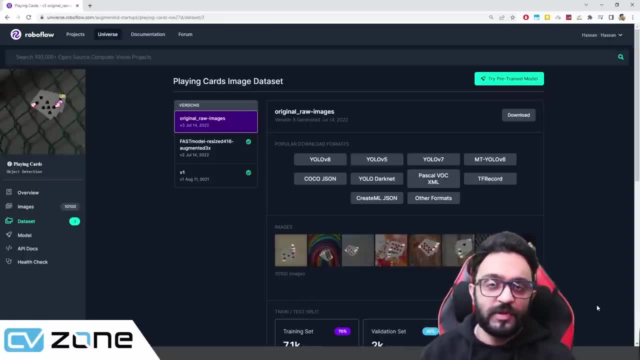 so now we are headed to project number four, and in this project we are going to create a poker hand detector in which we will first of all detect all the different cards and, once we have the card, we are going to take a look at the card, and we are going to take a look at the card and we are 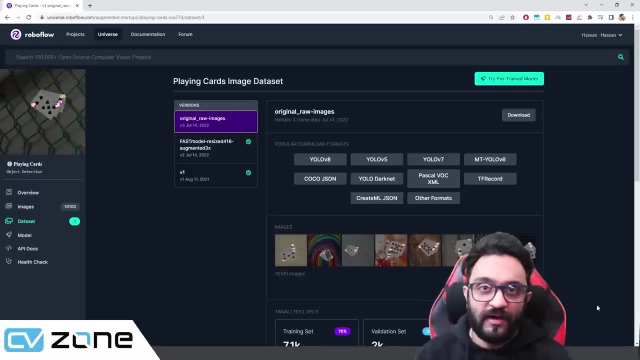 going to take a look at the card and we are going to determine what poker hand do we have. so this is a very interesting project because it has multiple layers, and the first one is to actually detect the cards, which we will do by yolo, and the second one is actually classifying: uh, what um hand do we have? 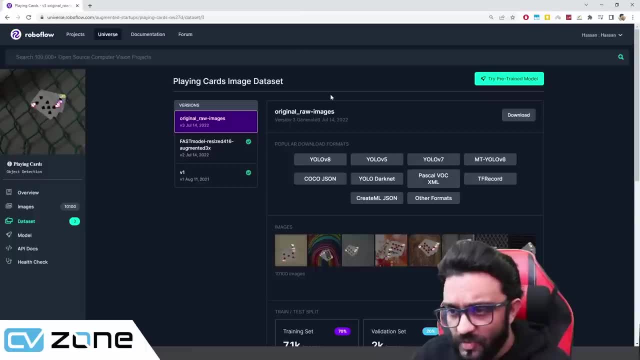 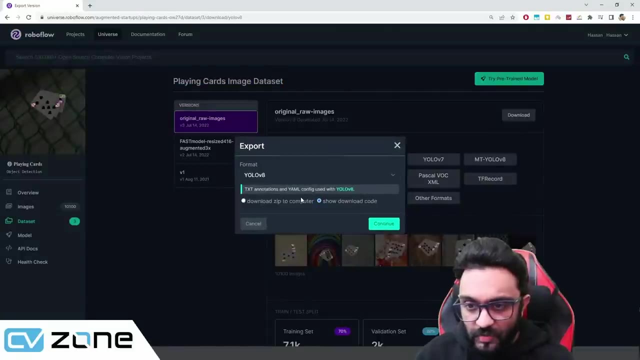 so there will be a little bit of code involved there. so where are we getting the data from? the data is available on robo flow universe and we are downloading the playing cards image data set and we will download the yolo version 8 so you can simply click on that download zip to computer. 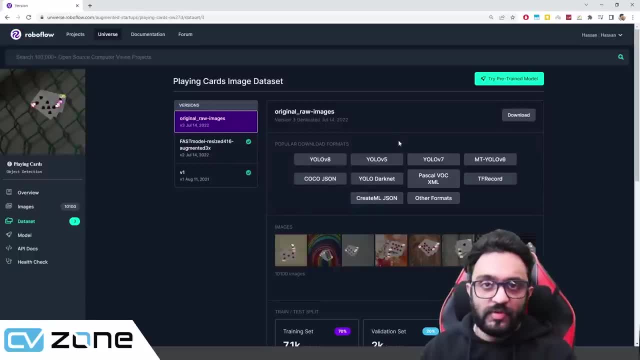 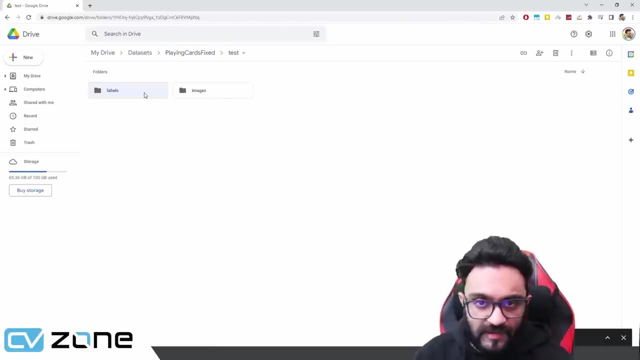 and you can press continue. once it is downloaded, you upload it to the google drive. so let me show you, uh, where that is. so this is the playing card data set. so we have validation, training and test data set. so we have labels and we have images for each of these labels. 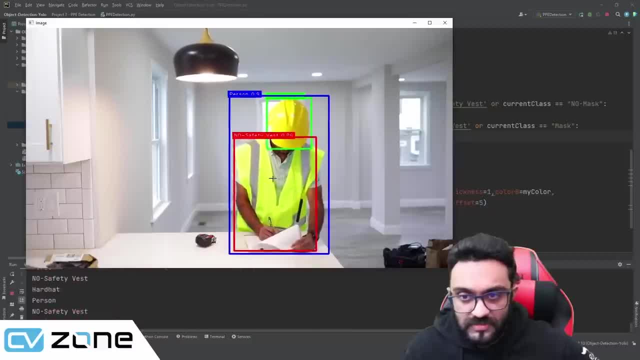 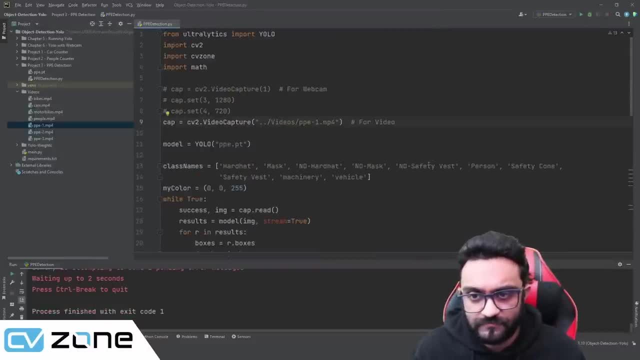 and then we have the no mask. so when it's not very clear, it's not giving good results, but overall it seems to work fine. so now we can also try it with the webcam. so i will put it: okay, let's keep it for video and for webcam. 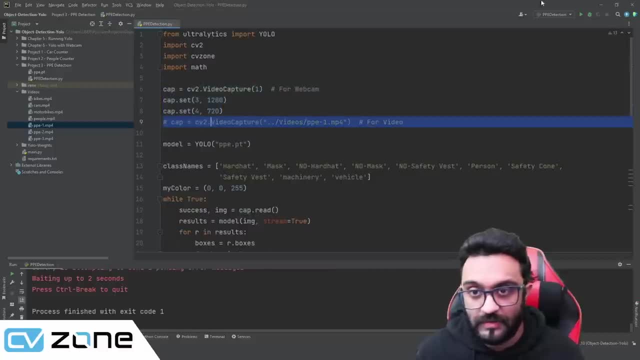 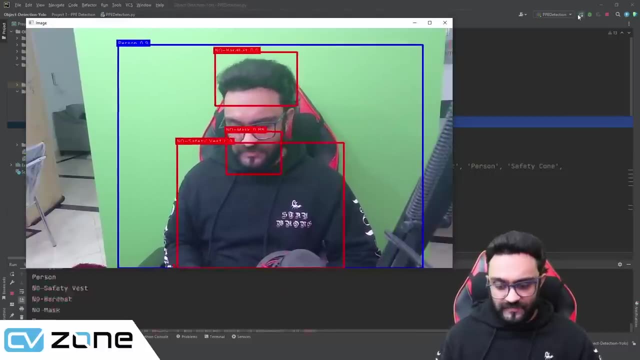 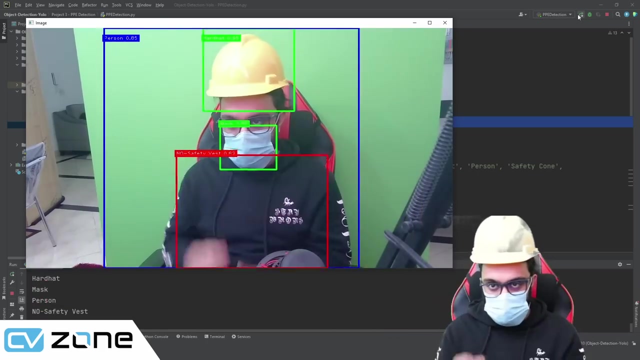 we can open this up and let's try it out. so, as you can see, i'm not wearing a hardhat, no mask and no safety vest, but it's detecting the person. so if i wear a mask, you can see it's detecting the mask, and if i wear the 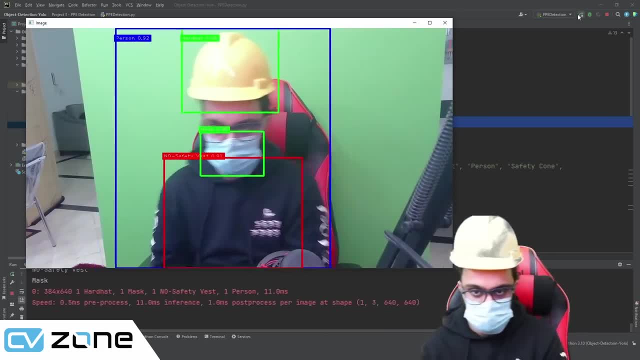 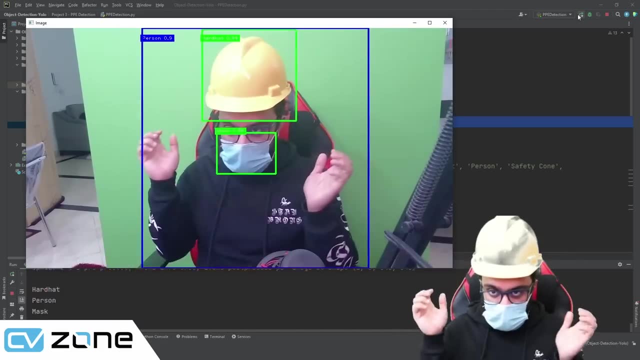 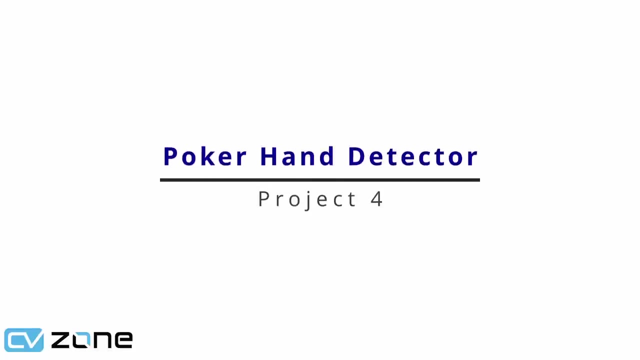 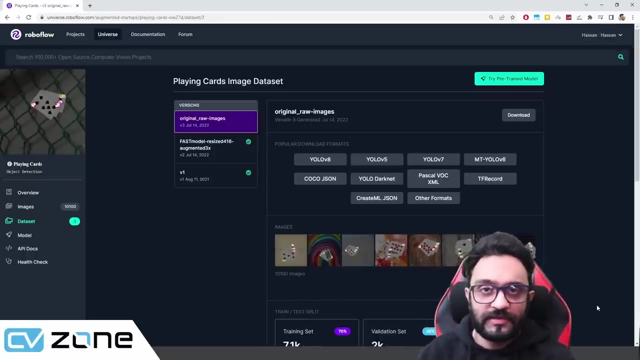 hardhat. you can see it detects the hardhat. there you go. if i remove the mask, it says no mask. there you go, and we have the hardhat and no safety vest. so now we are headed to project number four, and in this project we are going to create a poker hand detector. 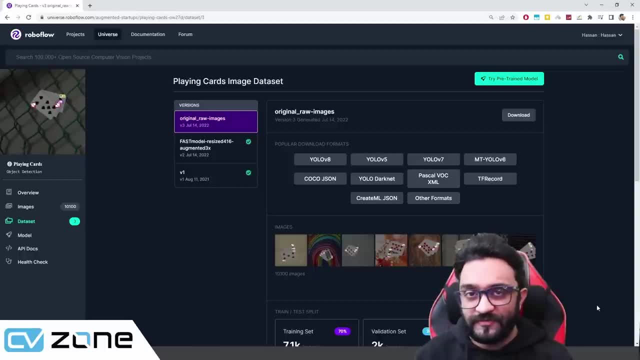 in which we will first of all detect all the different cards and once we have the cards, we are going to determine what poker hand do we have. so this is a very interesting project because it has multiple layers, and the first one is to actually detect the cards. 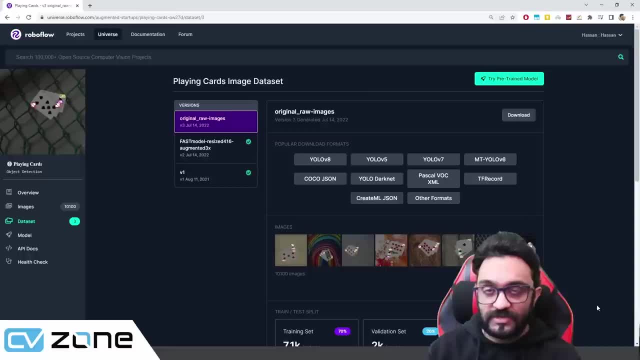 which we will do by yolo, and the second one is actually classifying what hand do we have, so there will be a little bit of code involved there. so where are we getting the data from? the data is available on roboflow universe and we are downloading the playing cards image data set. 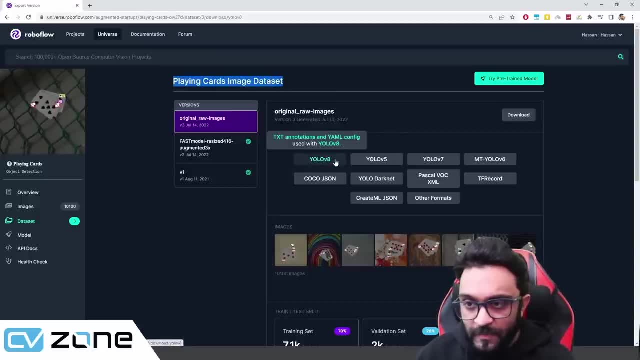 and we will download the yolo version 8. so you can simply click on that download zip to computer and you can press continue. once it is downloaded, you upload it to the google drive. so let me show you where that is. so this is the playing card data set. 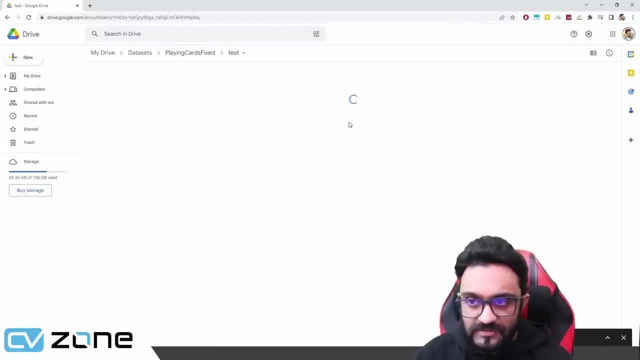 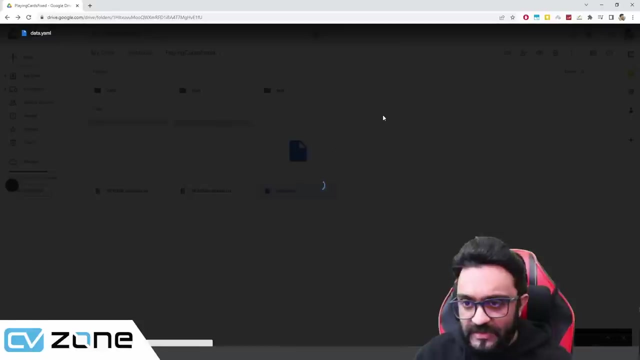 so we have validation, training and test data set, so we have labels and we have images for each of these labels. so, like we have seen before in our bbe project, it is the same format and the thing that is different is, again, the datayaml file. so let's open that up in a text editor. 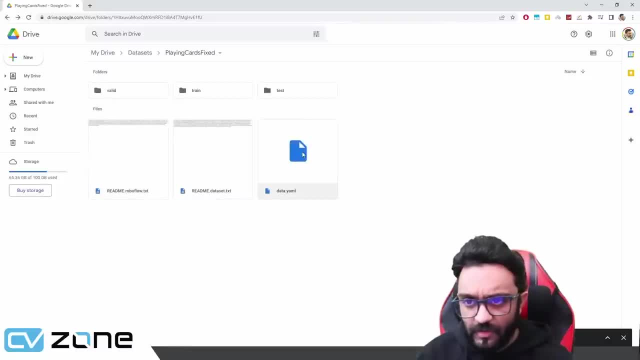 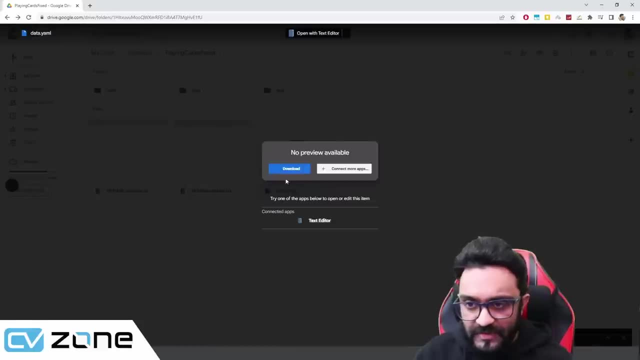 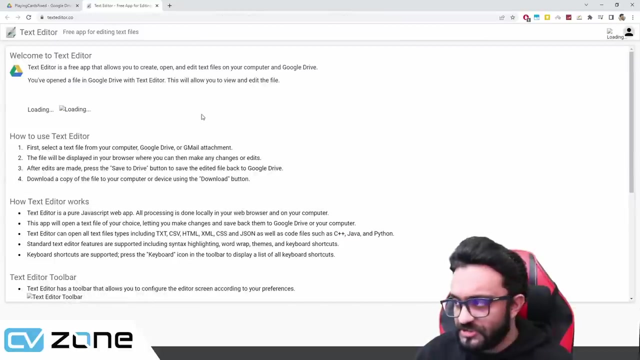 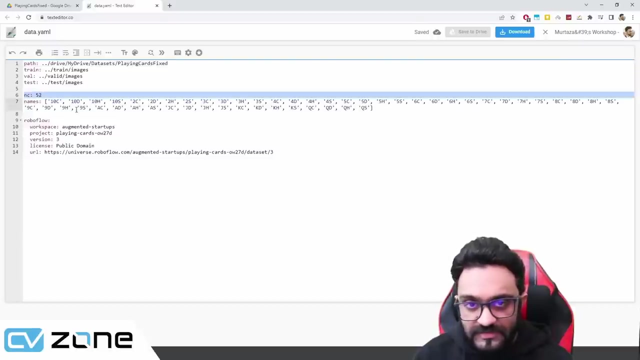 and we have values for each of these labels. so, like we have seen before in our bve project, it is the same format and the thing that is different is again the datayml file. so let's open that up in a text editor and let's see what changes have we made there. so this is our datayml file and 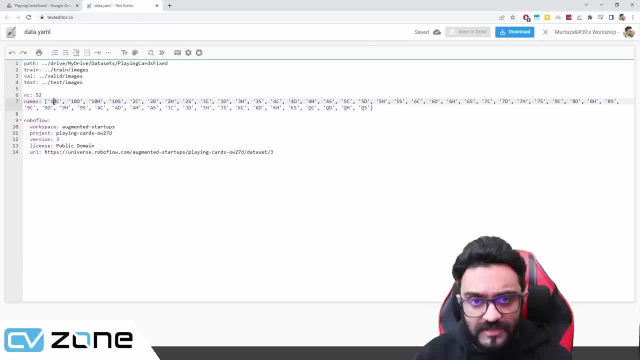 here you can see, we have number of classes as 52, and all of these classes are based on the rank, the suit. so here it's 10 of clubs, 10 of diamond, for example. so all of these, as you can see, we have here. and then we have, uh, the training, validation and test folders, but we also have 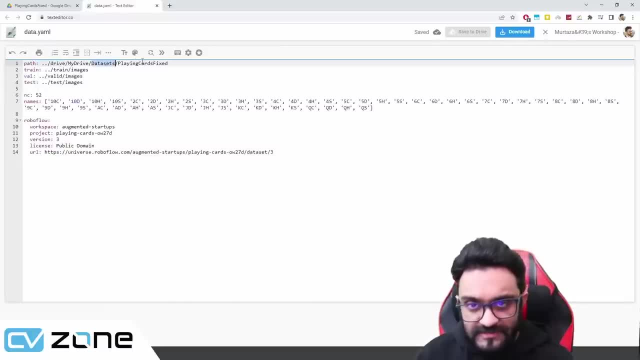 defined the path, so the path is drive, my drive data sets and playing cards fixed. so they had an issue earlier where they had a duplicate, so i believe it's fixed now. earlier they had 53 classes because there was a duplicate, but now it's fixed so i had to upload it again and use this as playing. 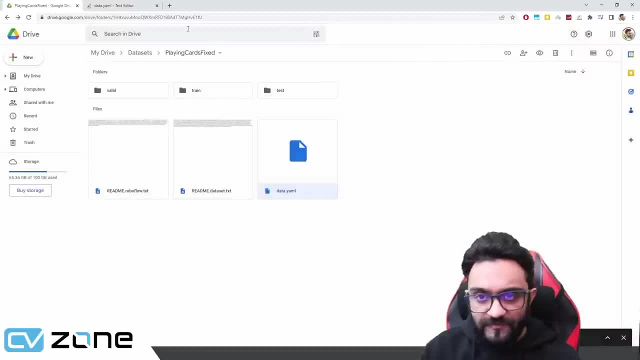 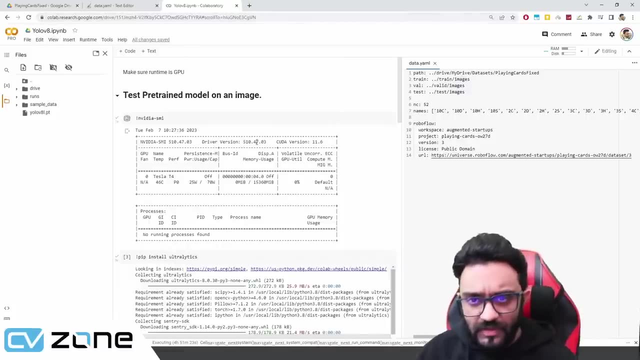 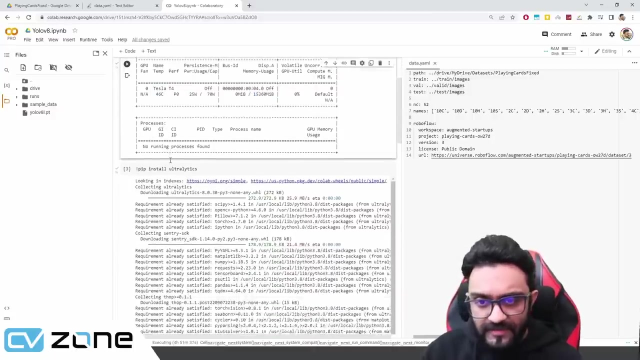 cards fixed. so this is what we have, and then what we do next. what i did next is actually to save some time, i ran the exact same google collab. so you check the nvidia driver or the nvidia graphics card and we have the similar one that we had earlier, which is tesla d4. it is 16 gb of memory, and then we install. 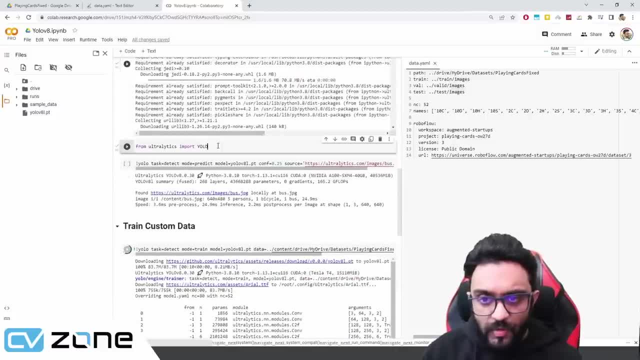 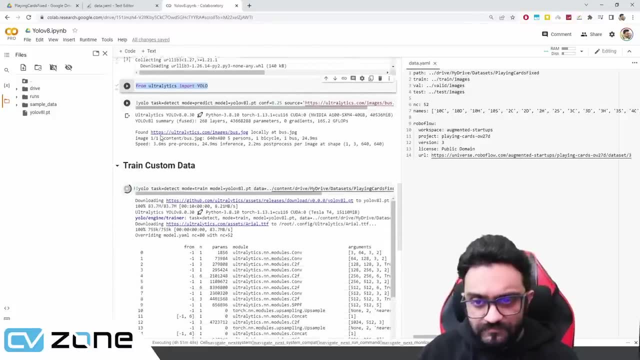 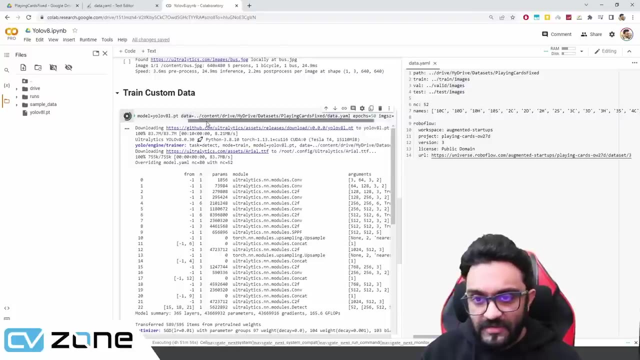 ultralytics, and after that we import yolo from ultralytics, and this you don't have to perform, just to make sure it's running. you can do that, and then you start the training process. so in the training process, all you have to do is you have to change the data path so it will be content drive. 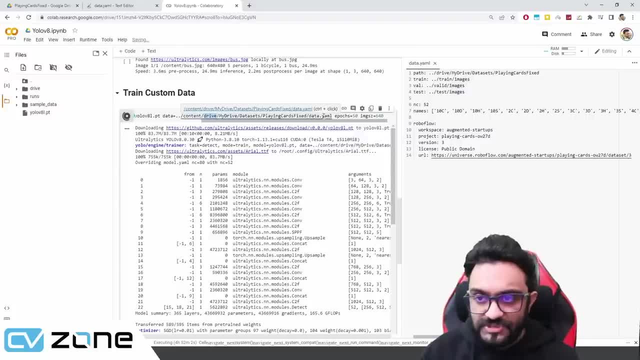 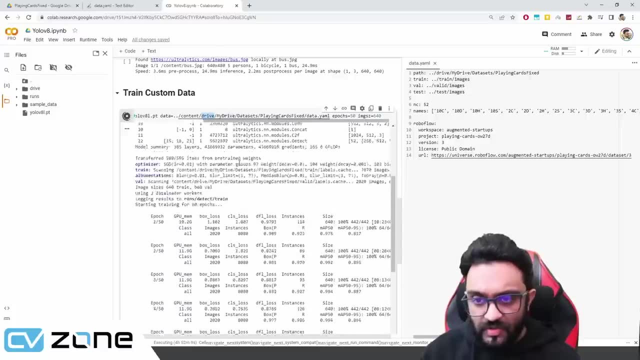 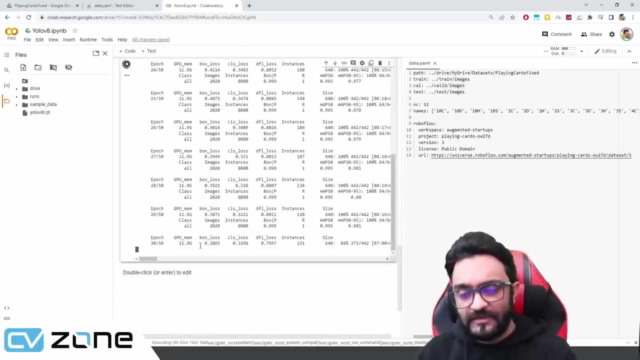 my drive data sets, playing cards, fixed slash data dot y aml. so this is what we have to do and, uh, we will have 50 epochs. so right now it's taking a long time. so meanwhile, it's training. we are going to go ahead and understand the basic concepts of poker and how we can create a classifier for 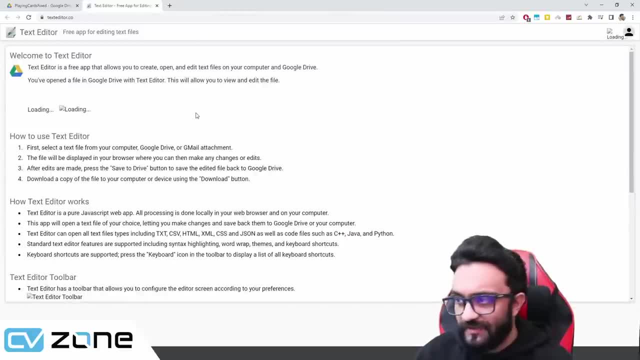 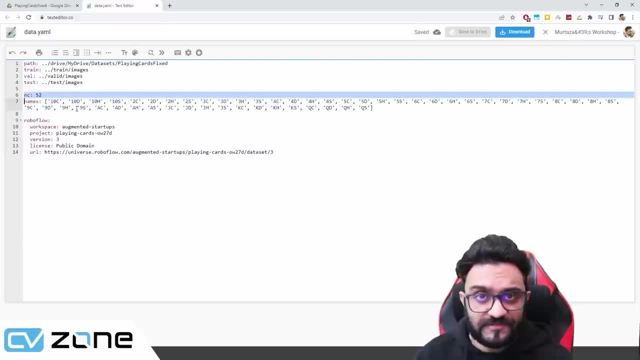 and let's see what changes have we made there. so this is our datayaml file and here you can see we have number of classes as 52, and all of these classes are based on the rank and the suit. so here it's 10 of clubs. 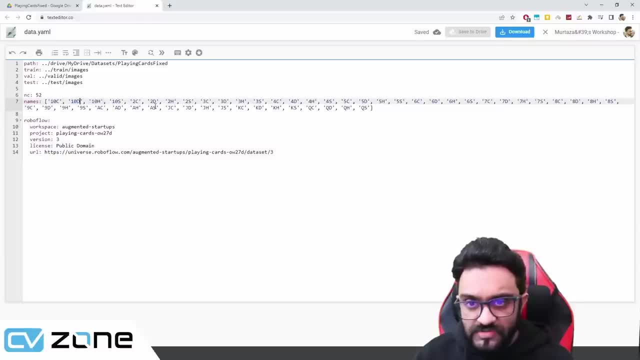 10 of diamond, for example. so all of these, as you can see, we have here, and then we have the training, validation and test folders, but we also have defined the path. so the path is drive, my drive, data sets and playing cards fixed, so they had an issue earlier. 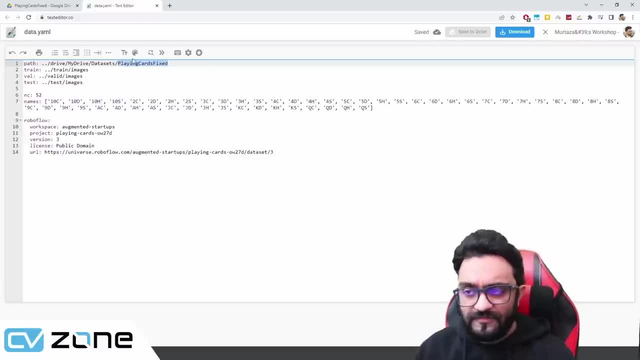 where they had a duplicate. so i believe it's fixed now. earlier they had 53 classes because there was a duplicate, but now it's fixed so i had to upload it again and use this as playing cards fixed. so this is what we have and then what we do next. 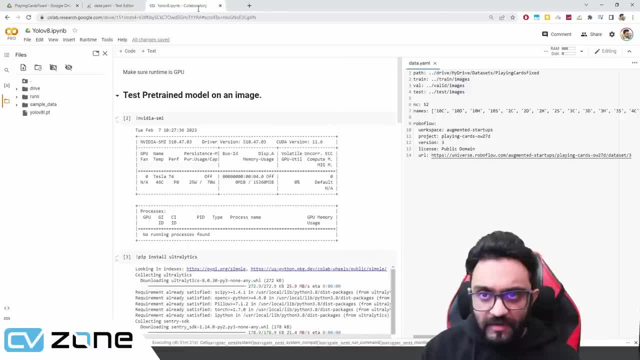 what i did next is actually, to save some time, i ran the exact same google collab. so you check the nvidia driver or the nvidia graphics card and we have the similar one that we had earlier, which is tesla d4. it is 16 gb of. 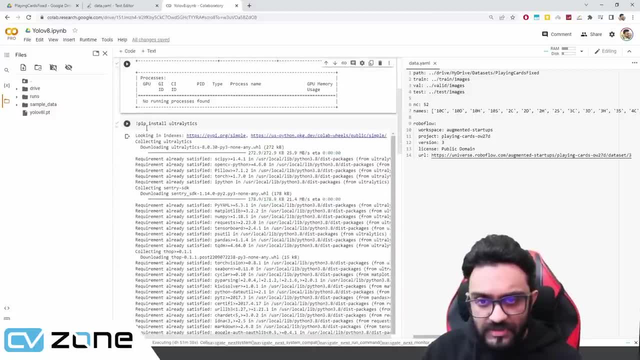 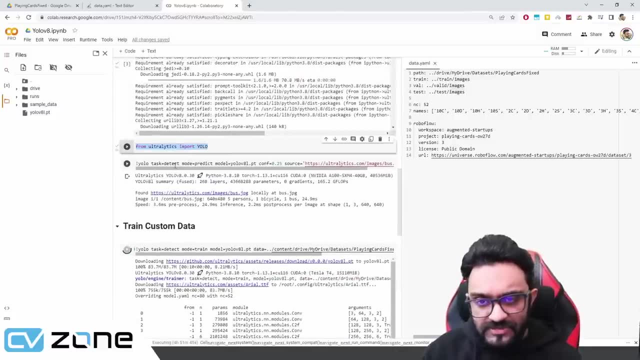 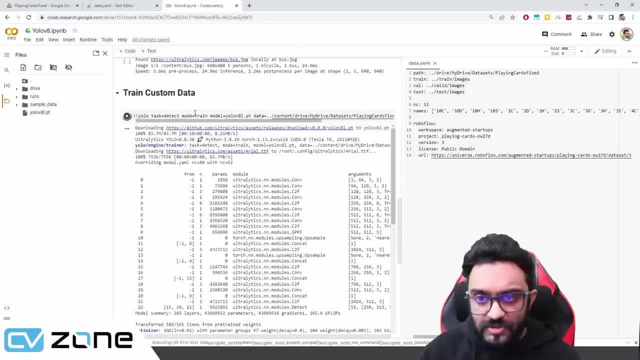 memory, and then we install ultralytics and after that we import yolo from ultralytics, and this you don't have to perform, just to make sure it's running. you can do that, and then you start the training process. so in the training process all you have to do is 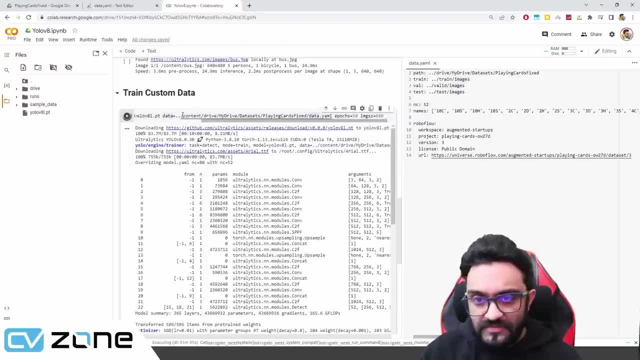 you have to change the data path so it will be content drive. my drive data sets, playing cards, fixed slash data, dot y a, m l. so this is what we have to do and we will have 50 epochs. so right now it's taking a long time. 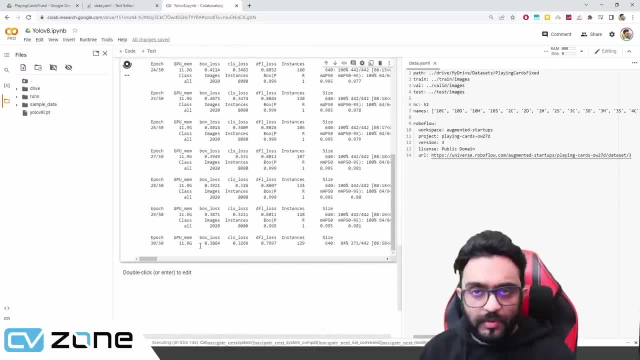 so meanwhile it's training. we are going to go ahead and understand the basic concepts of poker and how we can create a classifier for poker. so that part does not involve object detection but it is quite crucial to the project. so we will first go through that meanwhile. this will finish. 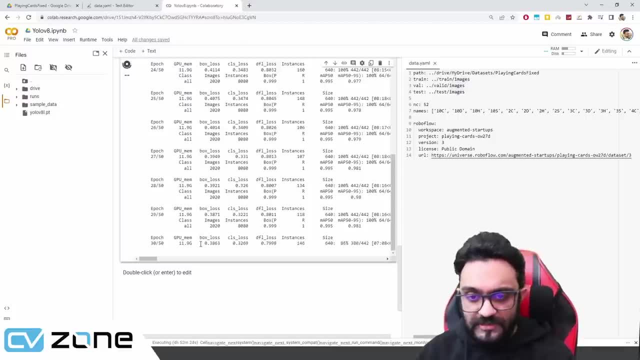 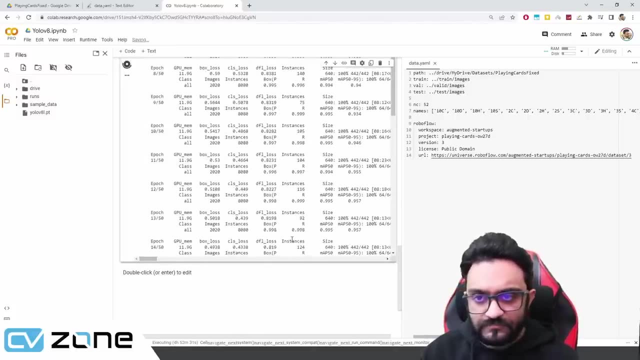 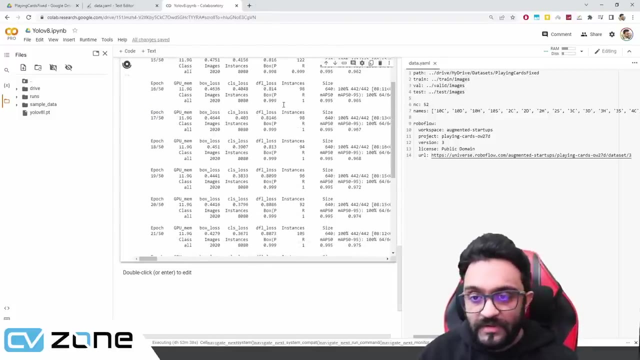 poker. so that part does not involve object detection, but it is quite crucial to the project. so we'll first go through that. meanwhile, this will finish what do you call training, and then we can take the data and start, uh, the detection as well. so this is up and running and, by the way, this is the datayml file. you can see it's here as: 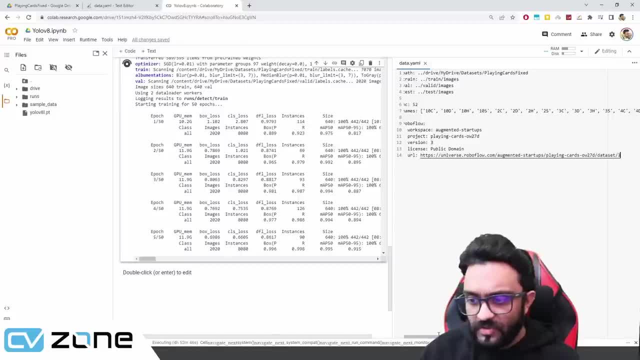 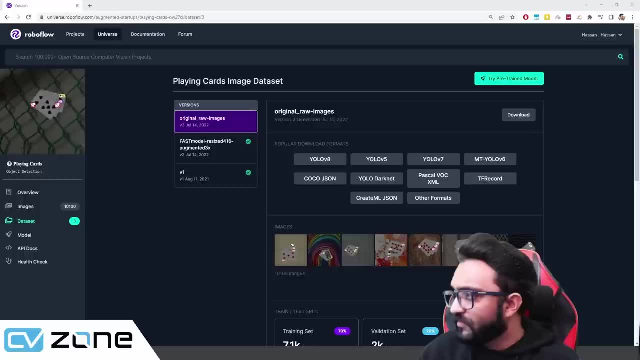 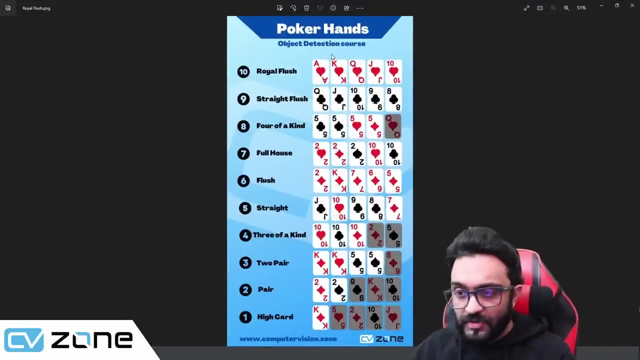 well, so that's good. so let's go back and try to understand what exactly is a poker game and how we can create a classifier for it. so to do that, i've created a simple classifier and i'm going to show you how you can create a classifier for it. so let's go ahead and 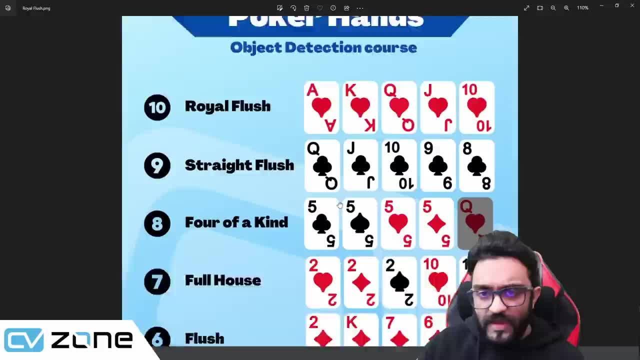 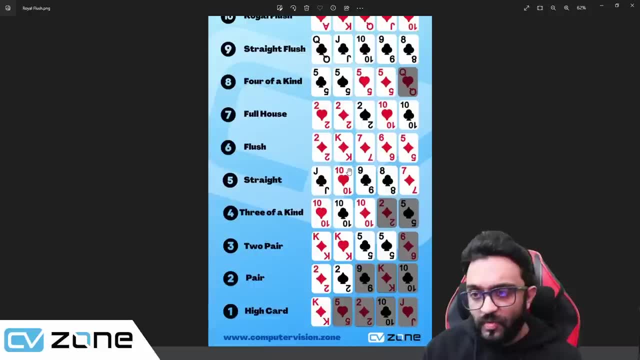 see what we have here. so we have a total of 10 different classes, so high card pair, two pair, three of a kind and so on. so we will start by understanding that first of all, you have to compare five cards. so everyone has two cards and the rest are laid out, uh, in in public domain. so 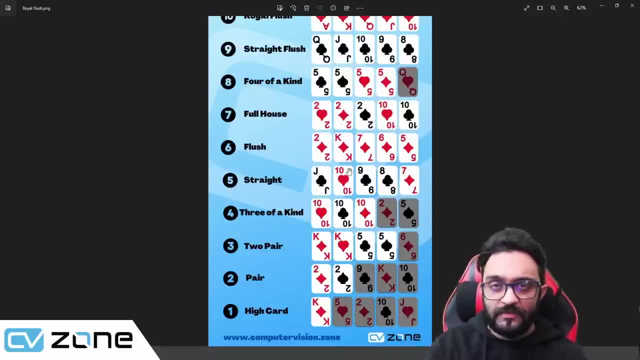 everyone has access to those cards that are in public domain. so we have a total of 10 different cards that are in public domain, but the two cards that you have are only for you to view. so what you have to do is you have to check your two cards and you have to check the rest of the. 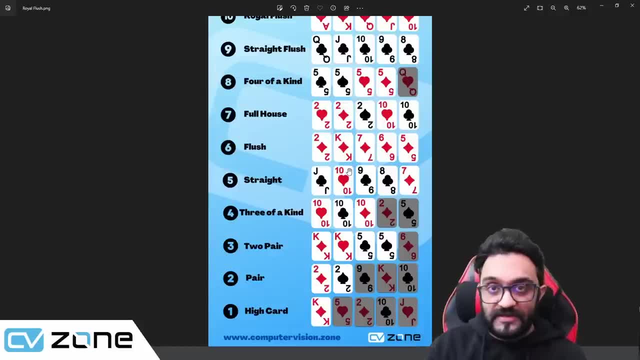 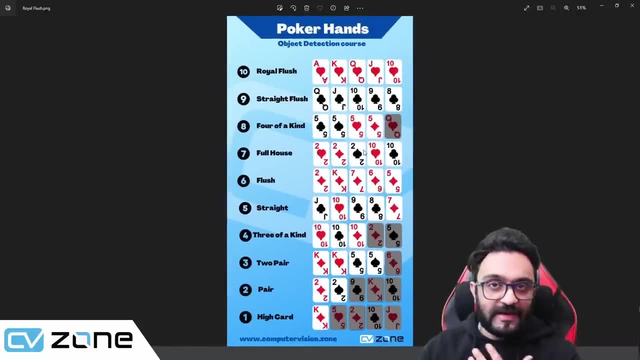 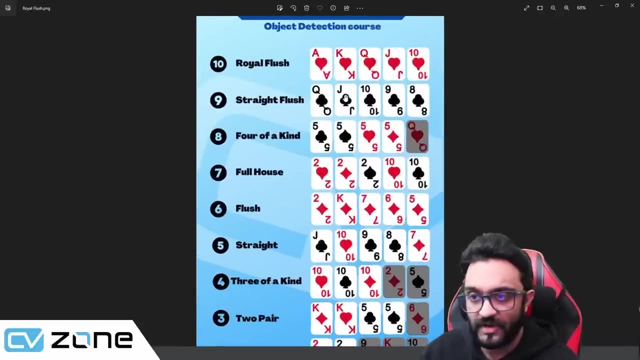 cards that are in public domain to find the best possible scenario, so the biggest hand. so whenever we have these five cards, we call it a hand. so we have a total of 10 types of hands and to understand these we need to understand what is rank and what is suit. so in. 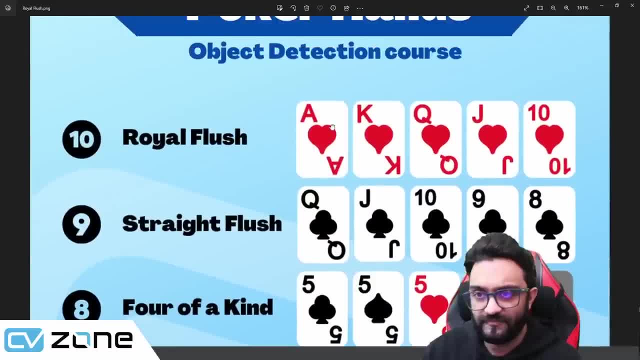 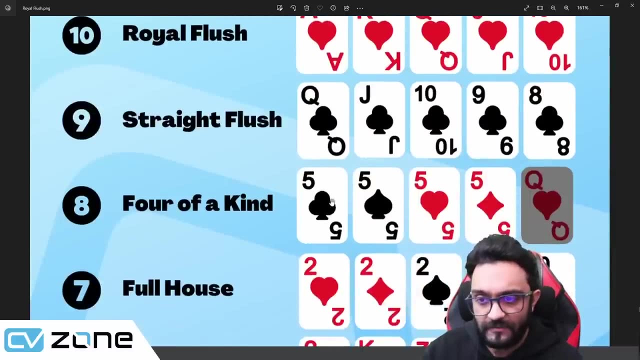 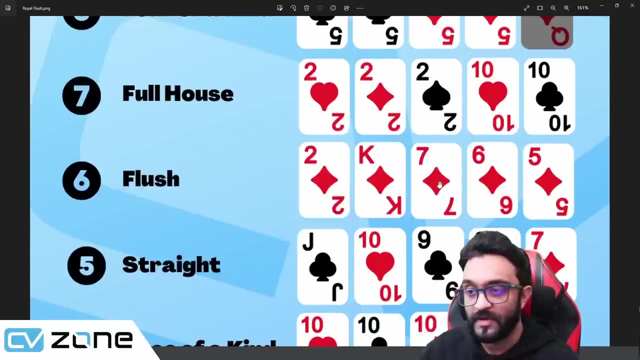 poker, uh, or in playing cards we actually have, for example, this is an a of hearts, this is queen of clubs. so a is basically the rank and hearts is basically the suit. so five is a rank and clubs is a suit. so, similarly, we have seven as the rank and diamond as the suit. so what we need to do is: 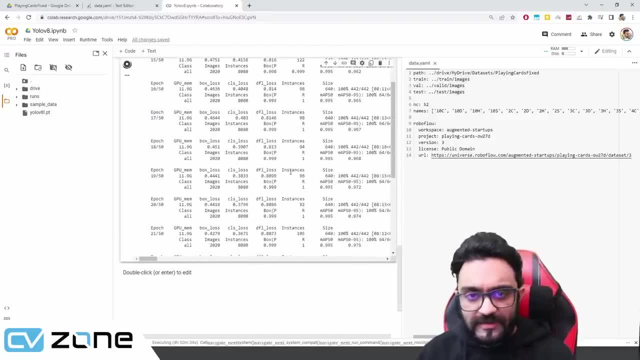 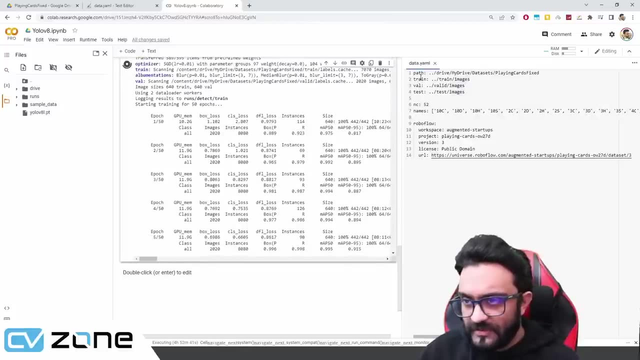 what you call training, and then we can take the data and start the detection as well. so this is up and running. and, by the way, this is the data dot y a m l file. you can see it's here as well, so that's good. so let's go back. 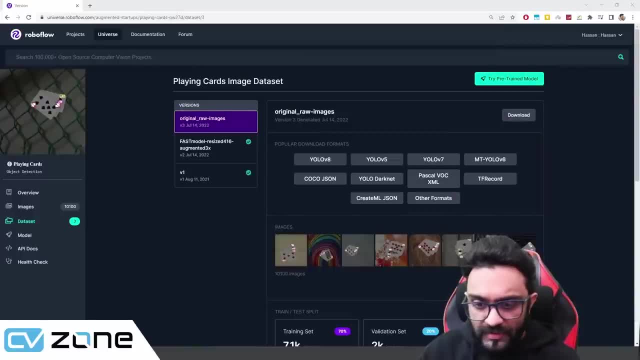 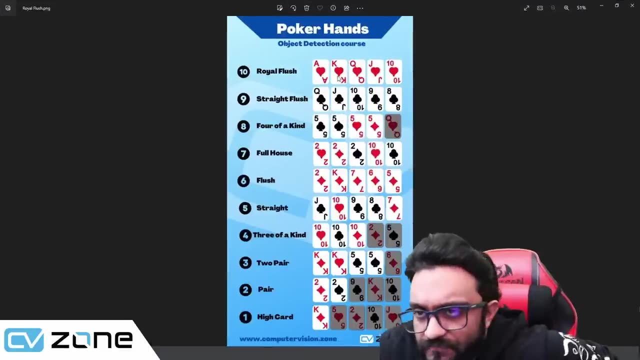 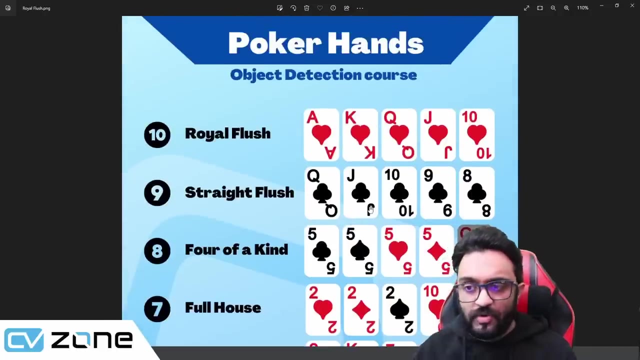 and try to understand what exactly is a poker game and how we can create a classifier for it. so to do that, I've created a simple poker hands. what do you call classifier, or? you can see, this is the data sheet or the cheat sheet. so we have a total of 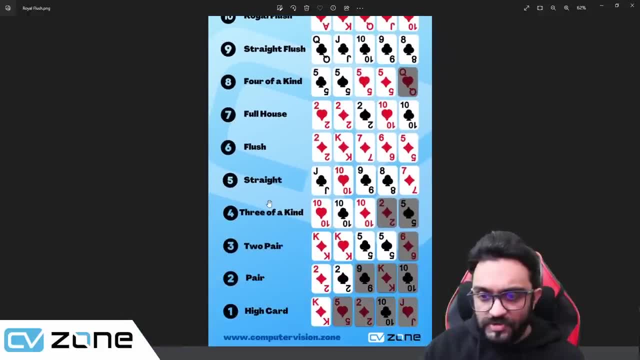 ten different classes, so high card pair, two pair, three of a kind and so on. so we will start by understanding that first of all you have to compare five cards, so everyone has two cards and the rest are laid out in public domain, so everyone has access to those. 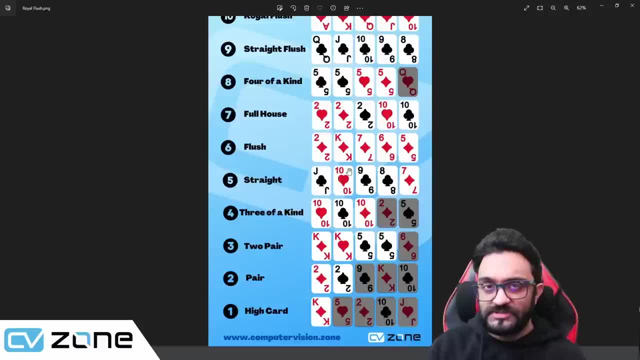 cards that are in public domain, but the two cards that you have are only for you to view. so what you have to do is you have to check your two cards and you have to check the rest of the cards that are in public domain to find the best possible scenario. 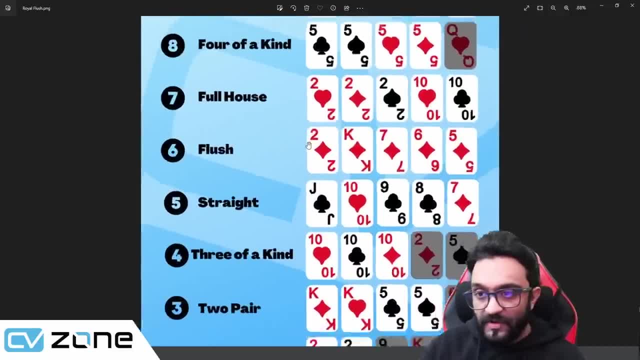 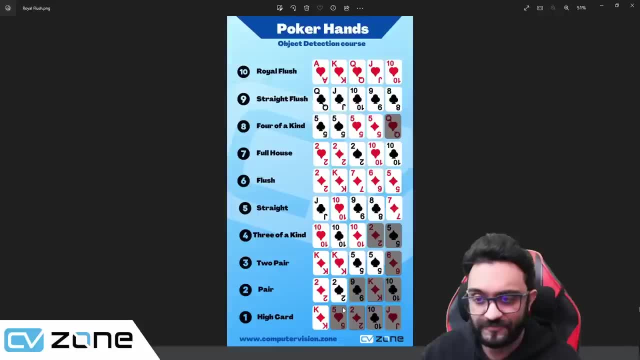 so the biggest hand. so whenever we have these five cards, we call it a hand. so we have a total of ten types of hands and to understand these we need to understand what is rank and what is suit. so in poker or in playing cards, we actually have 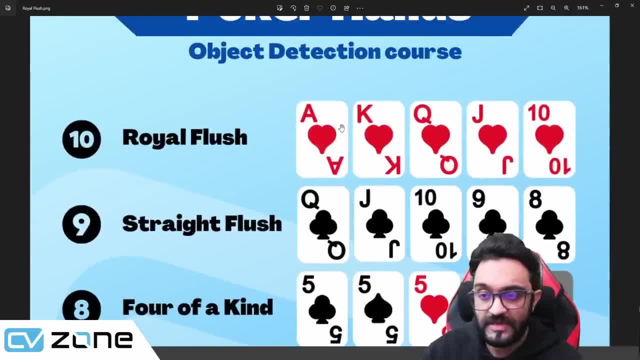 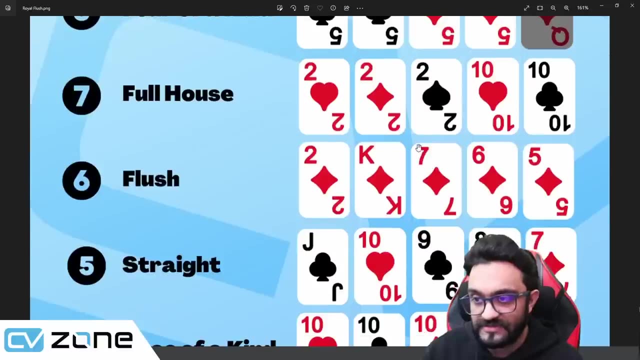 for example, this is an A of hearts. this is queen of clubs. so A is basically the rank and hearts is basically the suit. so five is a rank and clubs is a suit. so similarly, we have seven as the rank and diamond as the suit. so what we need to do is 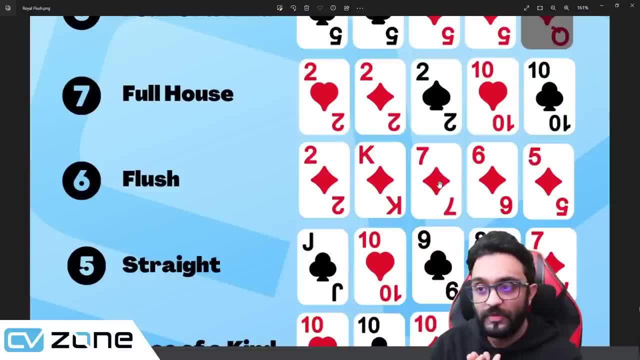 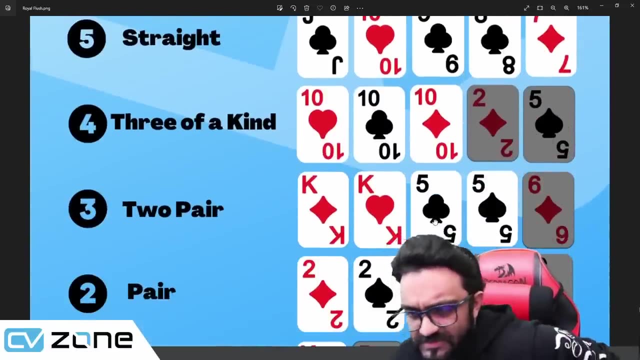 we need to understand that. first of all, we will differentiate these two. some hands are based on just the ranks and some hands are based on just the suits, and some of them are a combination. so let's start with the easiest one, which is a pair. we will get to the high card later on. 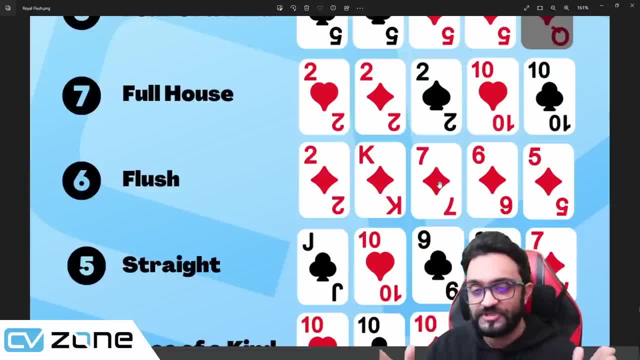 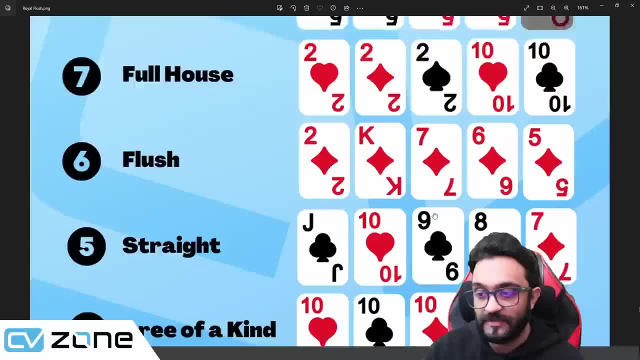 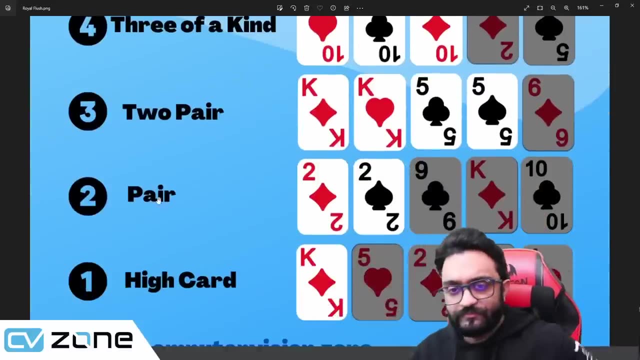 we need to understand that, first of all, we will differentiate these two. some hands are based on just the ranks and some hands are based on just the suits and some of them are a combination. so let's start with the easiest one, which is a pair. we will get to the high card later on, but let's start with the pair. the pair. you have same rank. 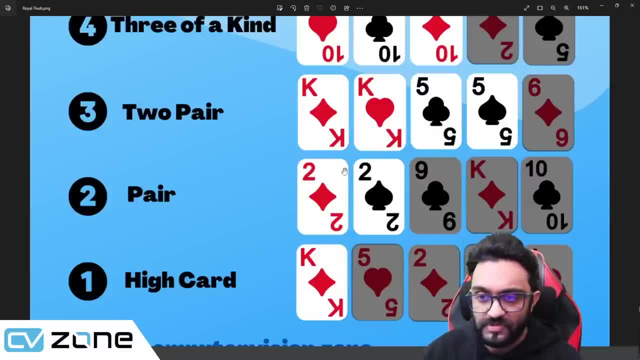 of two cards. so the rest of them they don't match, but two of them they match. so it can be two, two, it can be five, five, it can be seven, seven, it can be a, a. so whatever the card is, you should have a pair of the rank, not the suit of the rank. 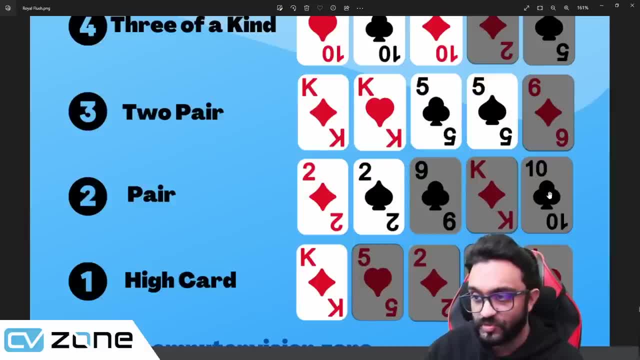 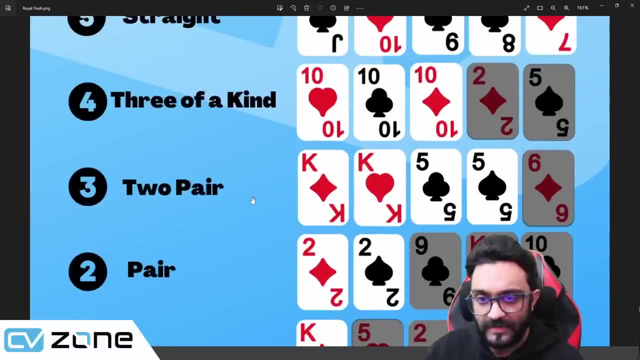 so, for example, you can see this is a pair of suit, but that does not count, so you don't have a pair of suit, you only have a pair of rank. okay, then we have two pair. two pair is similar to one pair, instead that you have two of them instead of one. so you have a king, king and five, five. so that's. 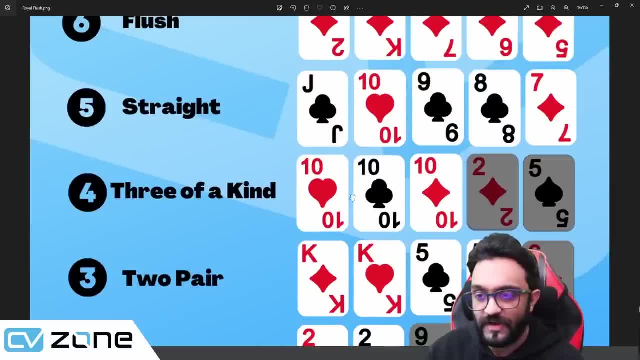 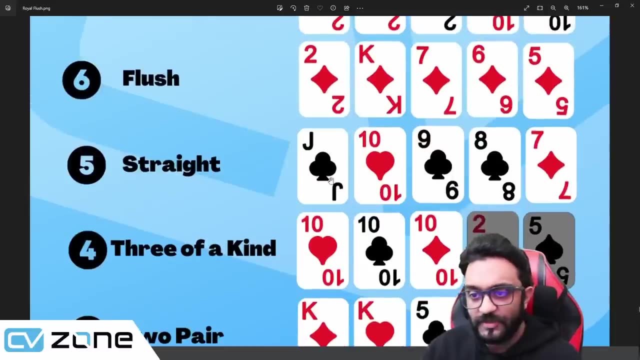 two, pair, then you have three of a kind. in three of a kind you have three of the same ranks, so it can be seven, seven, seven, eight, eight, eight, king, king, king, queen, queen, queen, or ten, ten, ten. in this case, the other two they don't matter. then you have a straight in straight, you have consecutive. 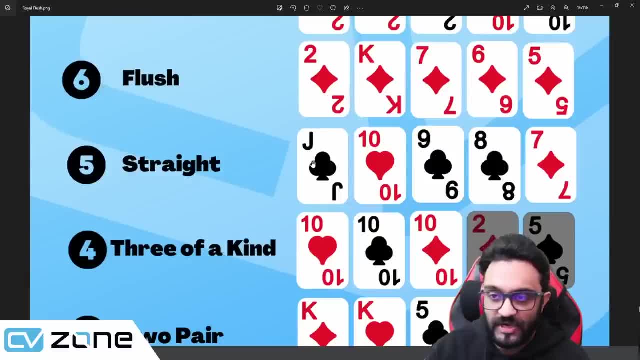 numbers. so for example, seven, eight, nine, ten jack. now, here again the rank matters, not the suit. we are not looking at the suits at all till this point. so for example, you have two, three, four, five, six, that is also a straight. then you have, uh, seven, eight, nine, ten jack. then you can also have nine. 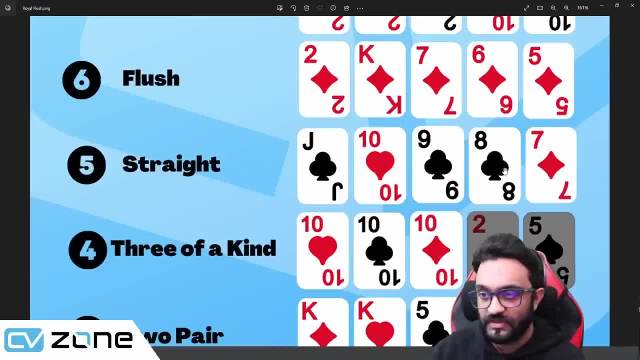 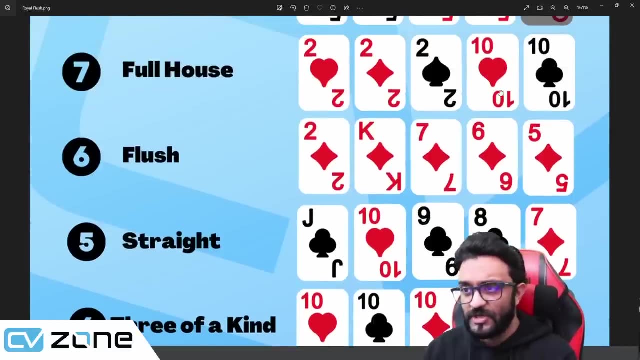 ten, jack queen king. that is also a straight, so you should have consecutive ranks. so if you do seven plus one, that should be the next one. eight plus one, nine. so that's the idea. by the way, rank for jack is eleven. so after ten you have uh, jack queen king and ace, so jack is eleven. 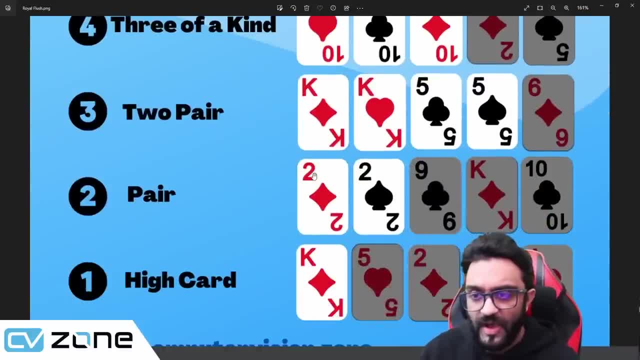 but let's start with the pair. the pair, you have same rank of two cards, so the rest of them they don't match, but two of them they match. so it can be 2-2, it can be 5-5, it can be 7-7. 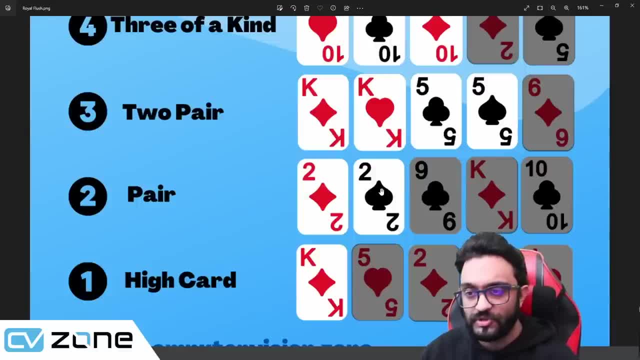 it can be A-A. so, whatever the card is, you should have a pair of the rank, not the suit of the rank. so, for example, you can see this is a pair of suit, but that does not count. so you don't have a pair of suit, you only have a pair of rank. 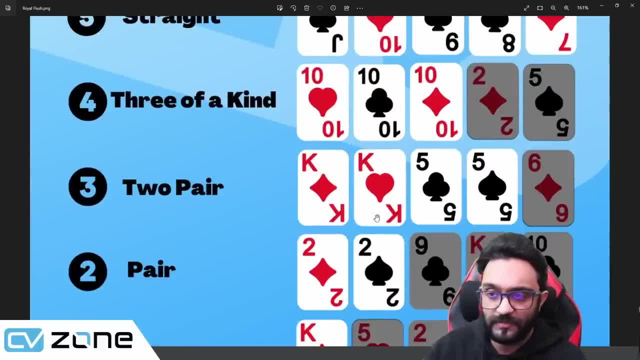 okay, then we have two pair. two pair is similar to one pair, instead that you have two of them instead of one. so you have a king-king and 5-5, so that's two pair. then you have three of a kind in three of a kind. 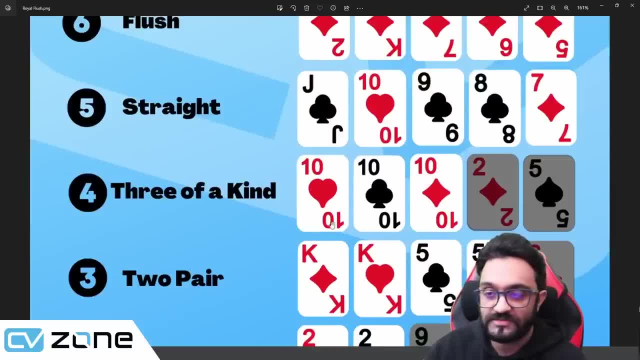 you have three of the same ranks, so it can be 7-7-7, 8-8-8, king-king-king, queen-queen-queen or 10-10-10. in this case, the other two they don't matter. then you have a straight. 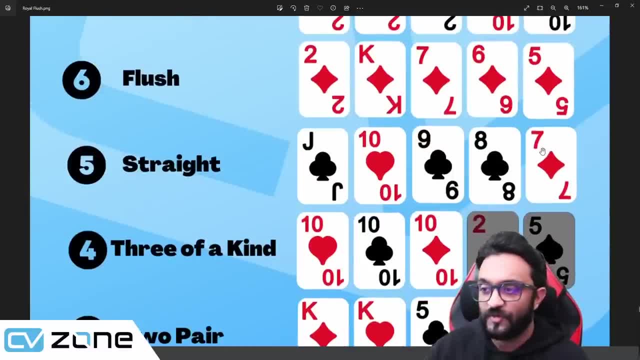 in straight, you have consecutive numbers. so for example, 7-8-9-10 jack. now, here again, the rank matters, not the suit. we are not looking at the suits at all till this point. so for example, you have 2-3-4-5-6. 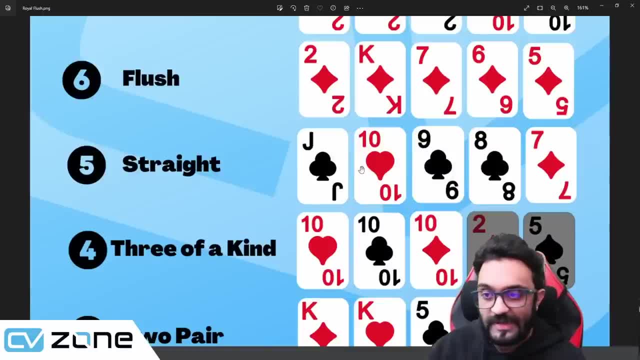 that is also a straight. then you have 7-8-9-10 jack. then you can also have 9-10 jack- queen-king- that is also a straight. so you should have consecutive ranks. so if you do 7 plus 1, that should be the next one. 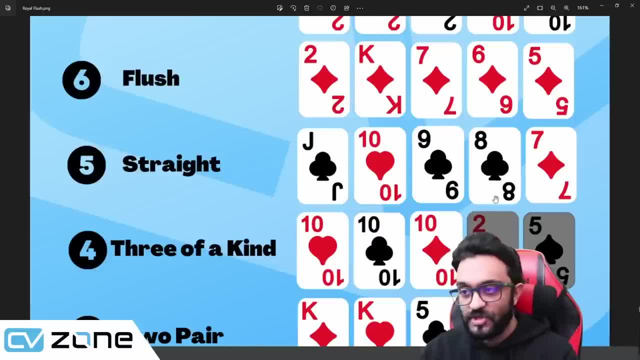 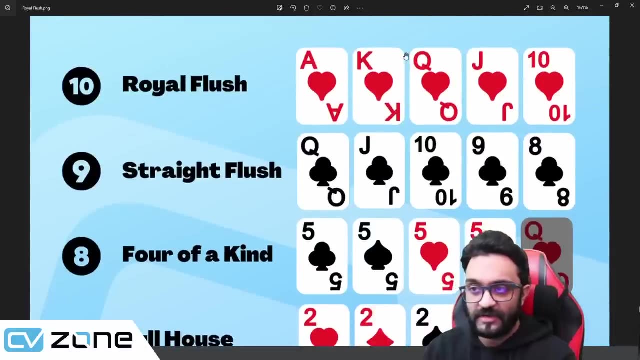 8 plus 1- 9. so that's the idea. by the way, the rank for jack is 11, so if you do 7 plus 1, that should be the next one: 8 plus 1, 9, 9, 9, 10, 11. 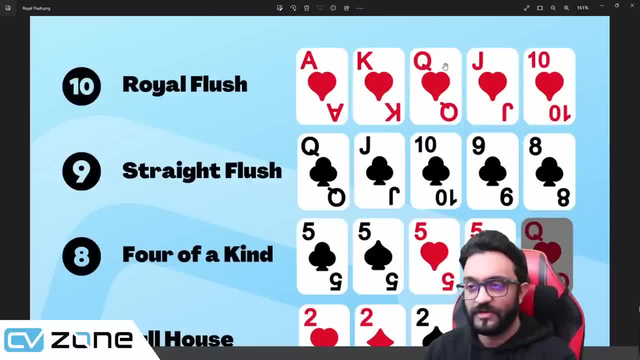 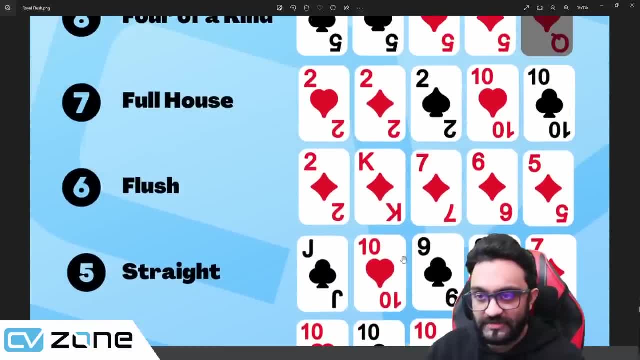 so after 10 you have jack, queen, king and ace. so jack is 11, rank number 11, queen is 12, king is 13, a is 14. so that's the biggest rank. ok, after straight now comes the suits. so if you have all the same suits, 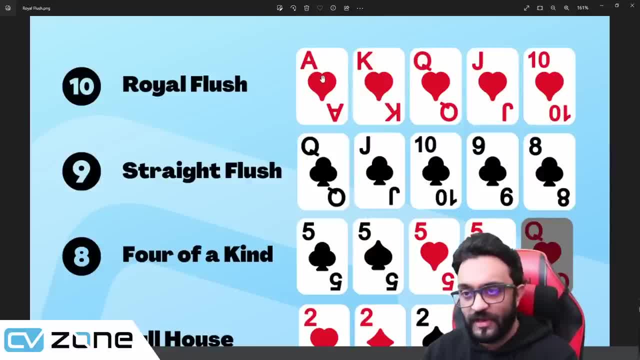 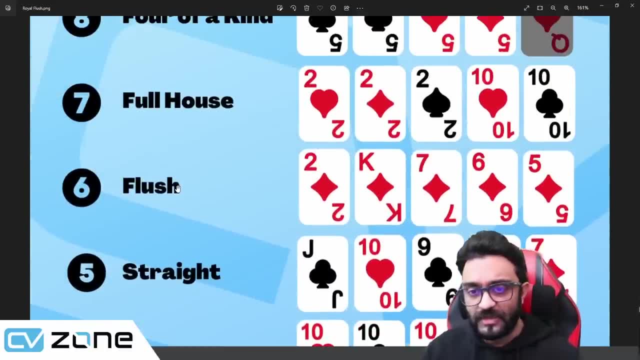 rank number eleven, queen is twelve, king is thirteen, a is fourteen, so that's the biggest rank, okay, uh, after straight now comes the suits. so if you have all the same suits, then you have a flush. so it can be all diamonds, it can be all hearts, it can be all uh clubs. 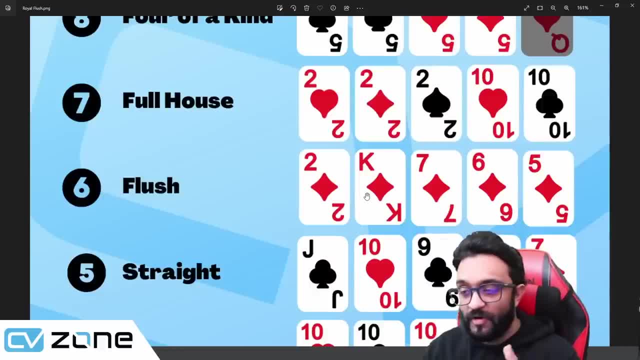 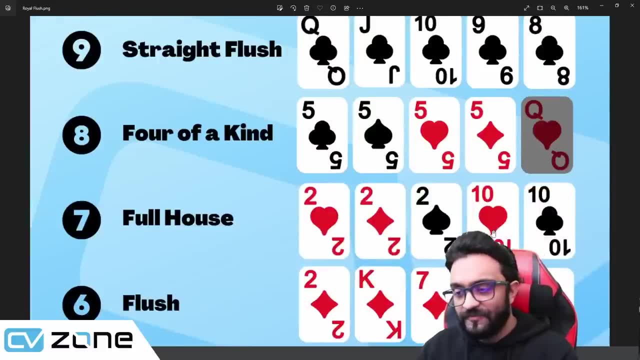 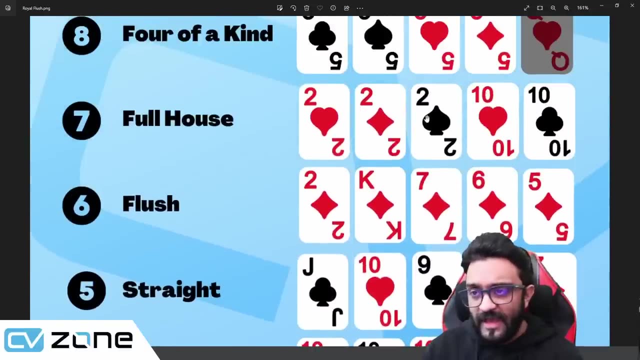 spades, whatever it is, um, if all of them, or or five of them, uh, are of the same suit, then it is a flush. then you have a full house. in full house, you have three of a kind, which is you have three cards that are of the same rank and then you have a pair. so you have two, two, two, and then ten, ten. 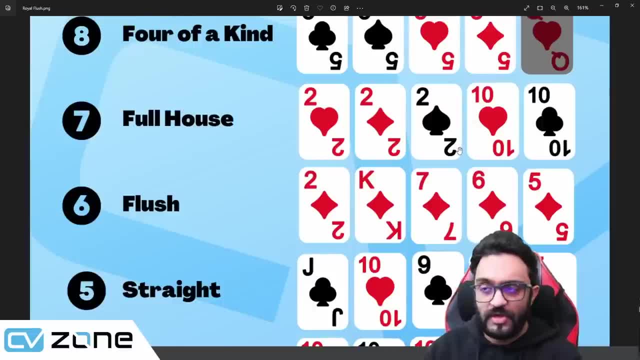 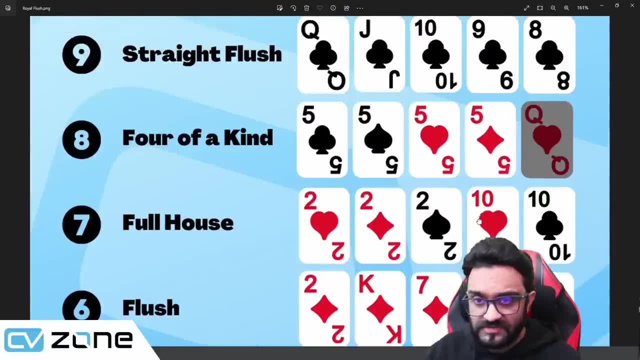 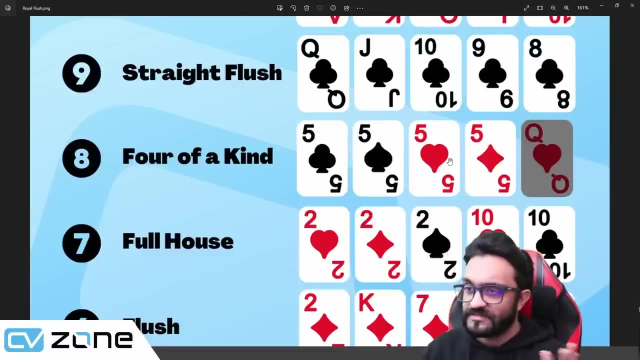 it can be five, five, five and seven, seven, so three of a kind plus a single pair, that is your full house. then you have four of a kind, which is very simple. you have four of the same racks. so five, five, five, five, seven, seven, seven, seven, nine, nine, nine, nine. 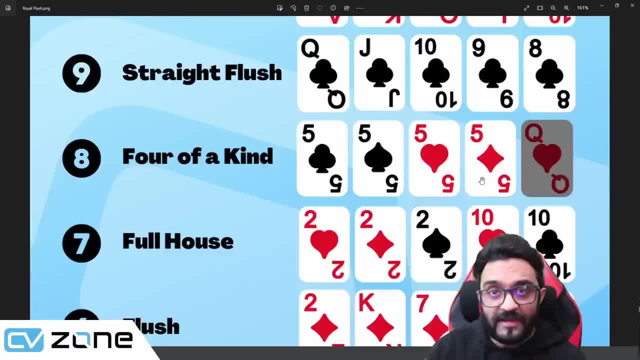 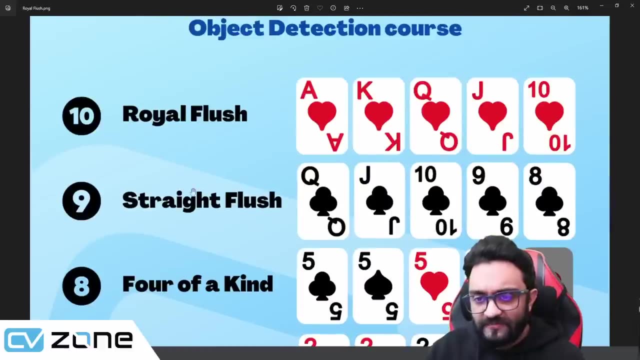 king, king, king, king and so on. so the ranks are pretty much the same. again, we don't care about the suits, actually the suits, you will have all the suits. so uh, it's, it's obvious. and the last card? we don't care about the last card, okay, uh, then we have a straight flush. 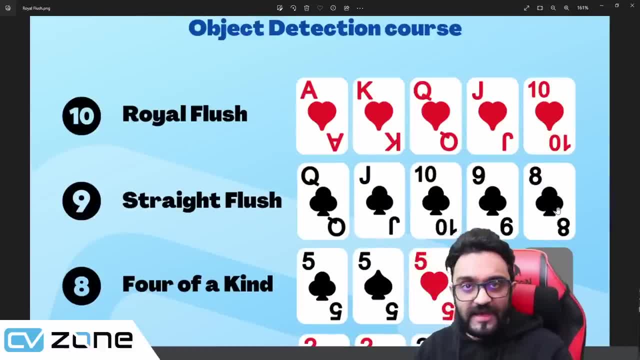 in the straight flush. we have a straight and a flush, so we have the ranks and we have the suits as well. so the suits, as you can see, all of them are uh clubs and uh straight is eight, nine, ten. jack queen, again, it can be two, three, four, five, six or any other, uh, any other formation. 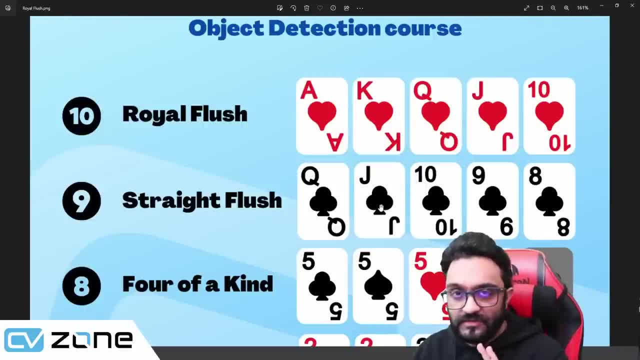 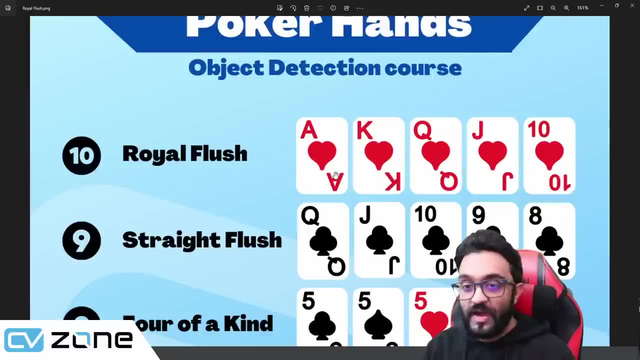 but it also has to have the suits as the same. and the last one, which is the highest, it is that you have, you have a straight, but starting from ace, so ace, king, queen, jack, ten, so that is the highest straight, plus you have a flush, so that is a royal flush. so, uh, you have, for example, hearts, hearts, hearts, hearts, and then 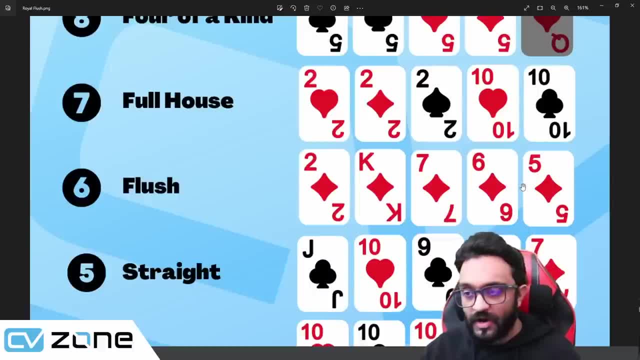 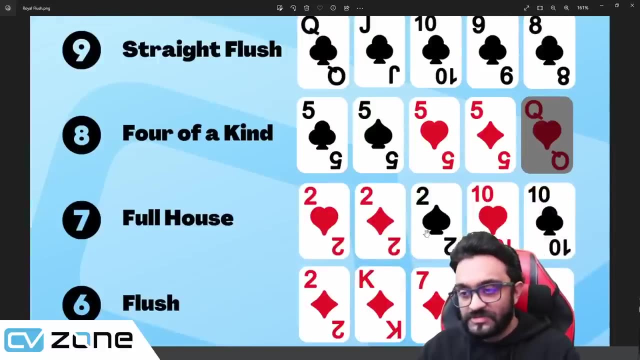 then you have a flush, so it can be all diamonds, it can be all hearts, whatever it is. if all of them, or 5 of them, are of the same suit, then it is a flush. then you have a full house. in full house you have 3 of a kind. 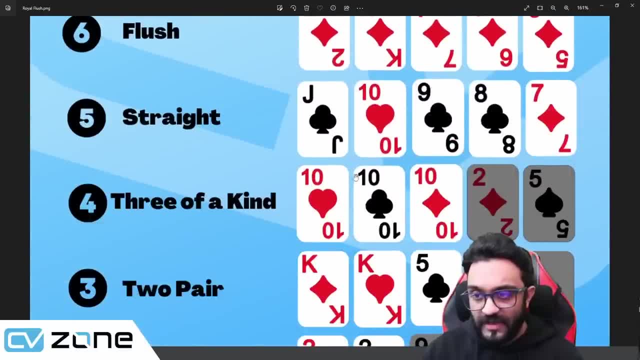 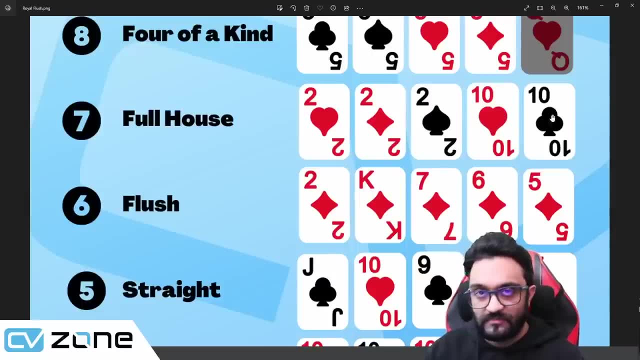 which is you have 3 cards that are of the same rank and then you have a pair, so you have 2, 2, 2 and then 10, 10. it can be 5, 5, 5 and 7, 7, so 3 of a kind. 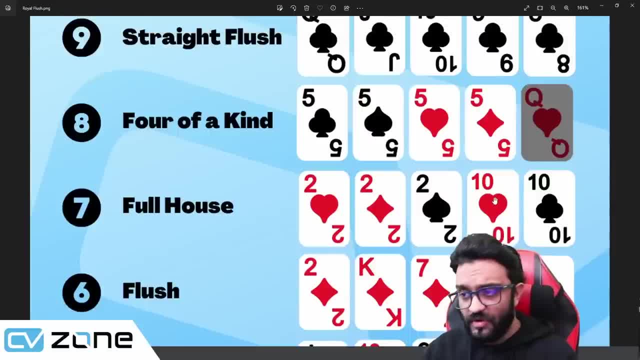 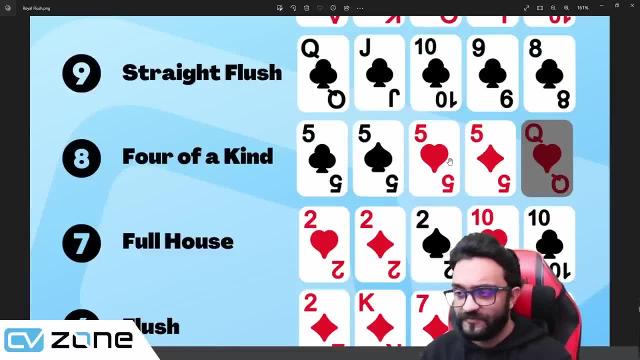 plus a single pair, that is your full house. then you have 4 of a kind, which is very simple. you have 4 of the same racks. so 5, 5, 5, 5, 7, 7, 7, 7, 9, 9, 9, 9. 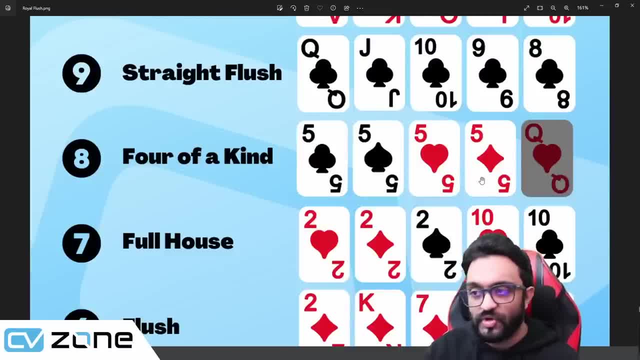 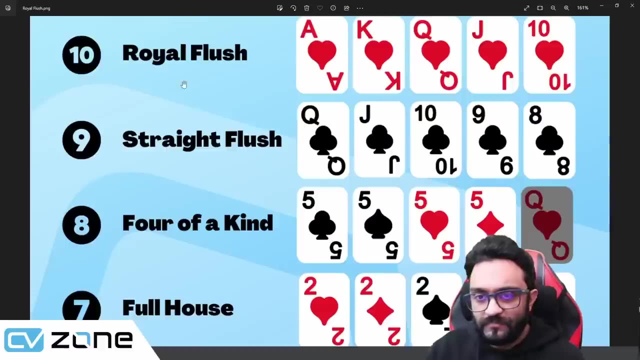 king, king, king, king and so on. so the ranks are pretty much the same. again, we don't care about the suits, actually the suits, you will have all the suits, so it's it's obvious. and the last card? we don't care about the last card, ok. 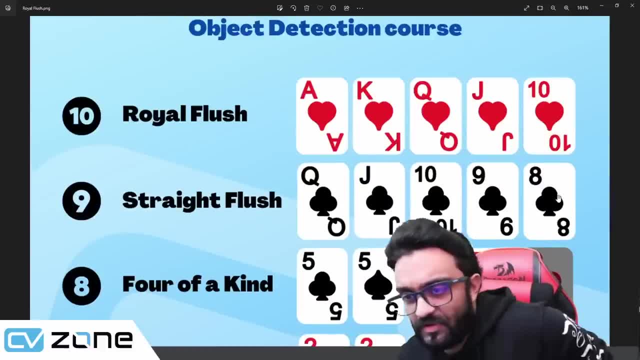 then we have a straight flush. in the straight flush we have a straight and a flush. so we have the ranks and we have the suits as well. so the suits, as you can see, all of them are clubs and straight is 8, 9, 10. jack queen. 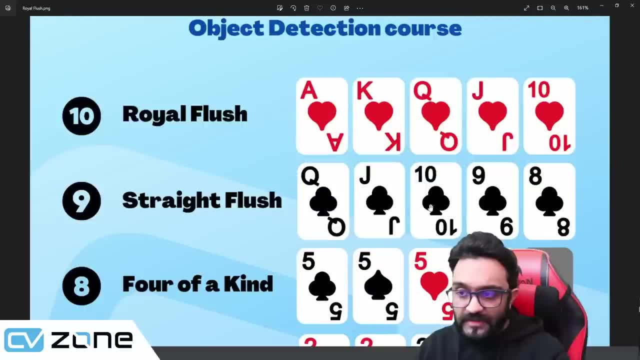 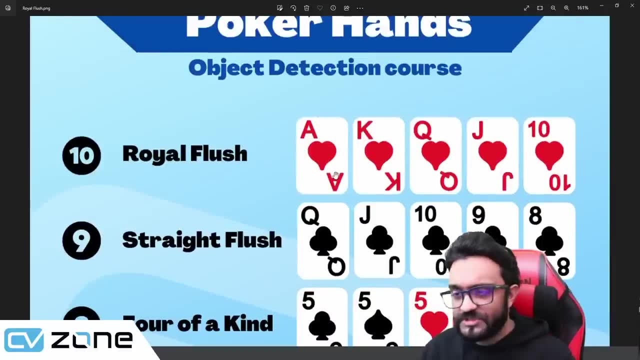 again, it can be 2, 3, 4, 5, 6 or any other, any other formation, but it also has to have the suits. so the last one, which is the highest one, it is that you have. you have a straight, but starting from ace. so 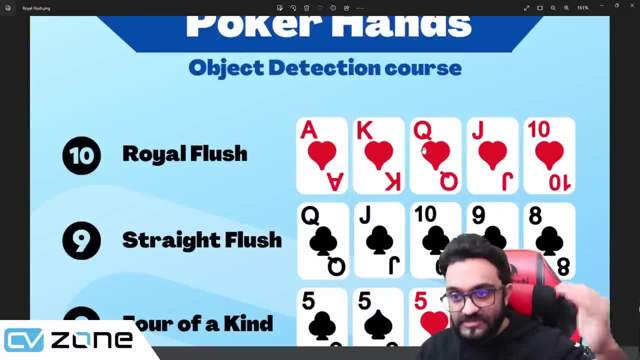 ace king queen jack: 10, so that is the highest straight, plus you have a flush, so that is a royal flush. so you have, for example, hearts, hearts, hearts, hearts, and then you have a king queen jack, if it starts from queen king, king queen jack: 10, 9. 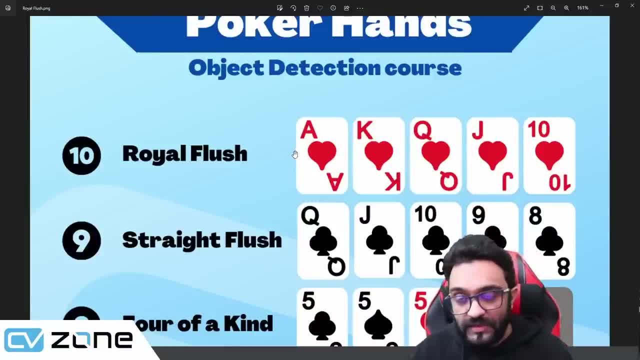 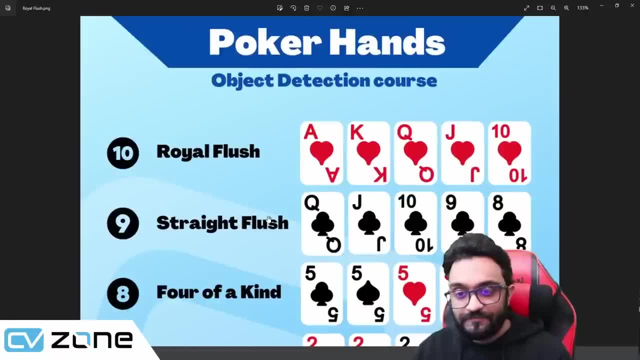 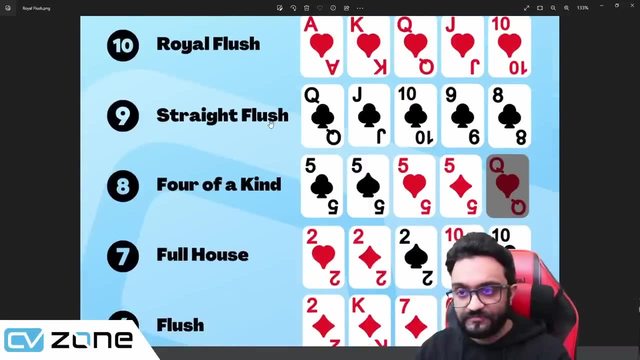 you have a king queen jack if it starts from queen or if it starts from king, king queen jack ten nine. so it's not a royal flush. in that case it is simply uh, a straight or a flush. so, uh sorry, straight flush, in that case it's a straight flush. so that is the basic idea. and the last one, if you 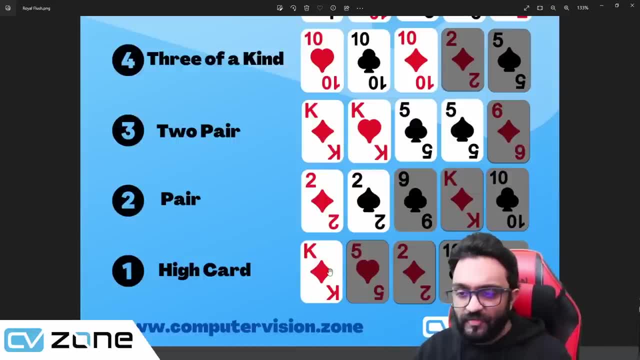 don't have any combination, then you have the highest card, so the biggest card. so, for example, if somebody um had a pair and you had the highest card, the peer will win, so with the higher card. in the previous video i mentioned that, that card Valley in it. it is one of those great spect Tet prior. player players and we will do a little test on it here. so just go ahead, if someone knows why, and suggest that you want to play with your other dream. Regarding the royal flush, like i said earlier, summon the Royal flush, since everyone goes to an essence. Ice spell in the Kings upgrader will win. 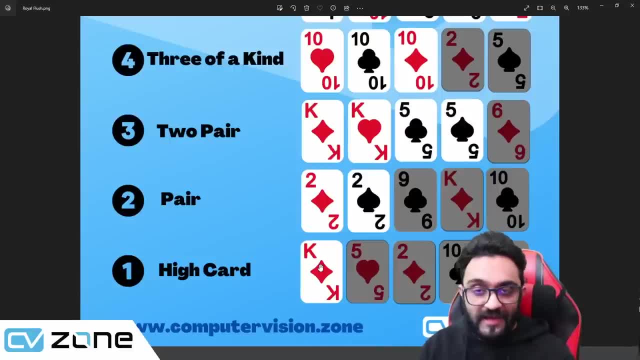 the relationship with the Royal flush. so if the simultaneously consideration includes: 1. realize the player is a child, one who does not win itqué, one player who does any particular team will win. then take on an higher card. if both of you don't have anything like there are two players playing against each. 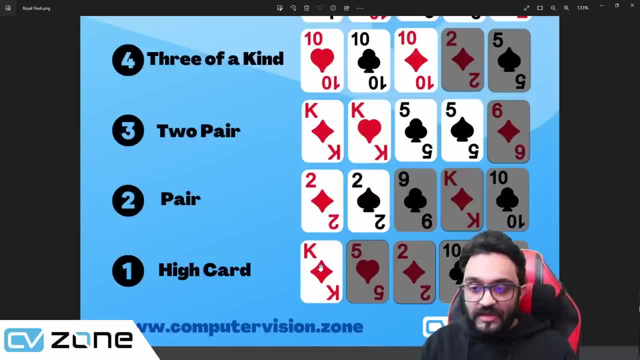 other, your five cards versus their five cards. if both of them have no classes at all- none of them- then you check which one has the highest card. so if you have the king and the other one has queen, then you win. so that's the idea. so what we will do is we will classify one hand. so we'll not do. 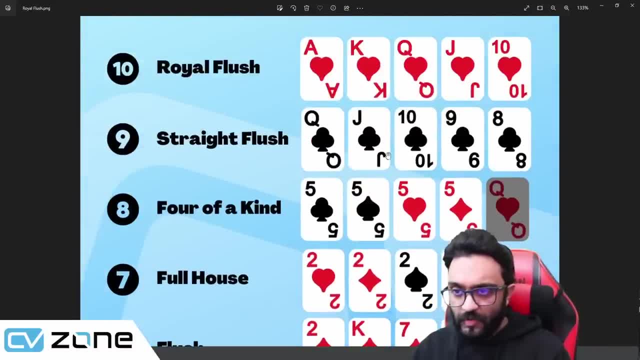 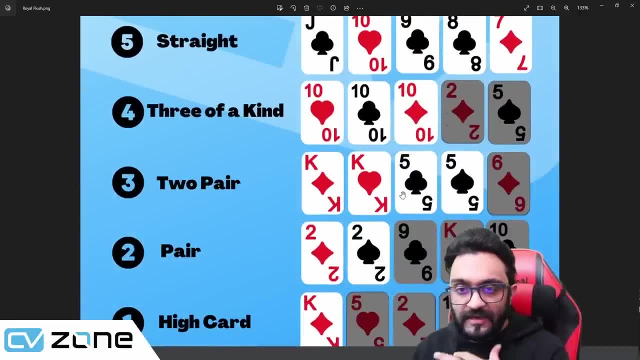 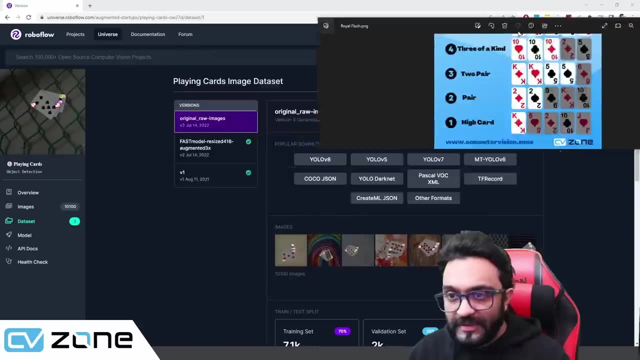 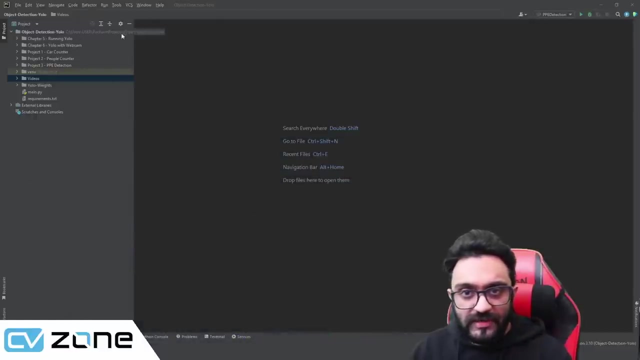 two hands. we'll do just one hand of our own hand. so we will send in five values as strings and it will output us the name of the hand. so that will be interesting to accomplish. so we will keep this image open and I will put it on the side and we will come back to it every now and then. so let's. 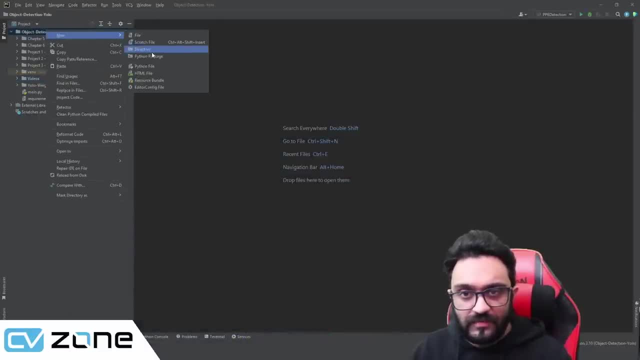 start by creating the folder- and we are going to call it project for poker hand detector. so, poker hand detector, you're going to start off with that, okay. so what we'll do is we will create a function and this function, we will input it- five strings or. 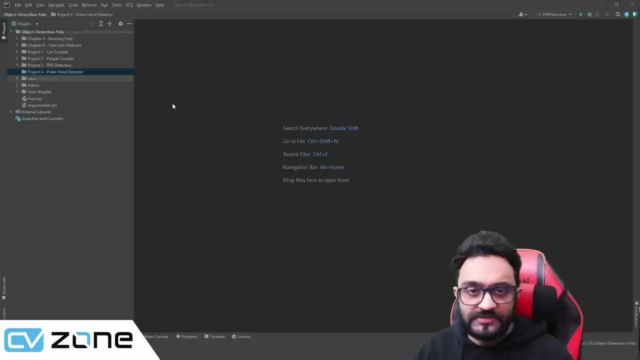 you can say a list with five strings and it will output us the result. so we will create it as a module, so that it is a separate code in a separate file and we can simply link it to our project. so here we will create a new python file and we will 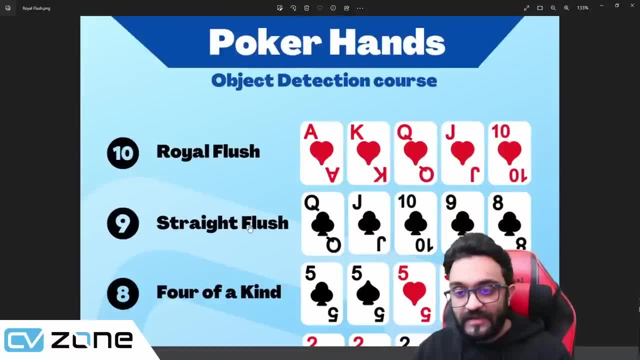 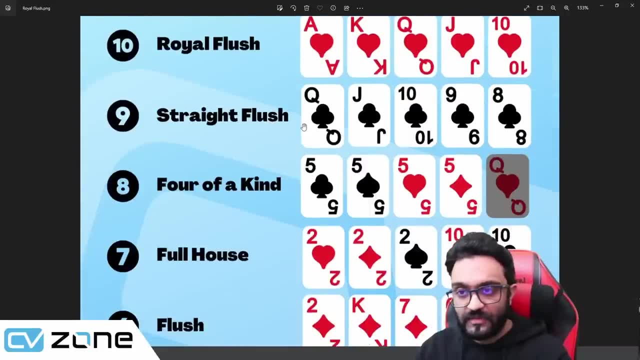 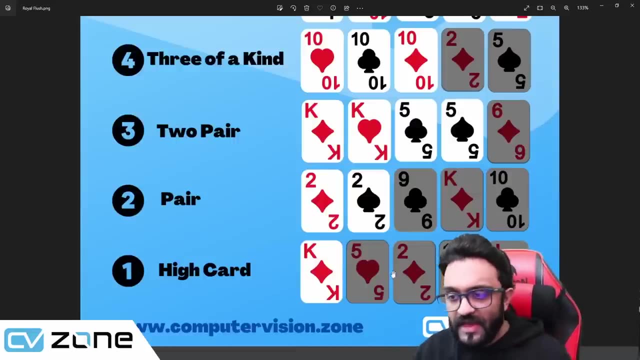 no, it's not a royal flush. in that case it is simply a straight or a flush. so sorry, straight flush. in that case it's a straight flush. so that is the basic idea. and the last one: if you don't have any combination, then you have the highest card. 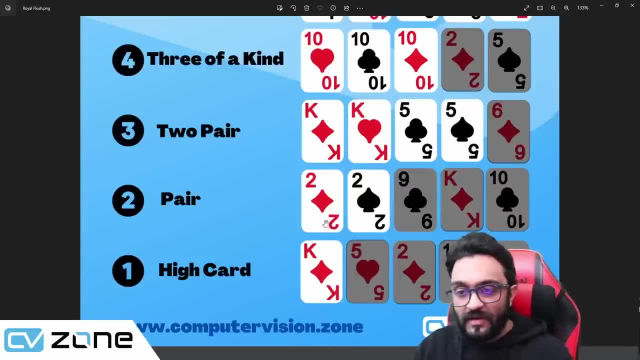 so the biggest card. so, for example, if somebody had a pair and you had the highest card, the pair will win, so with the high card. if both of you don't have anything like there are two players playing against each other, your five cards versus their five cards. 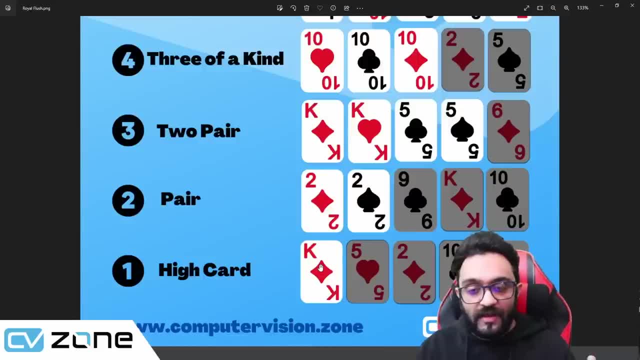 if both of them have no classes at all- none of them- then you check which one has the highest card. so if you have the king and the other one has queen, then you win. so that's the idea. so what we will do is we will classify one hand. 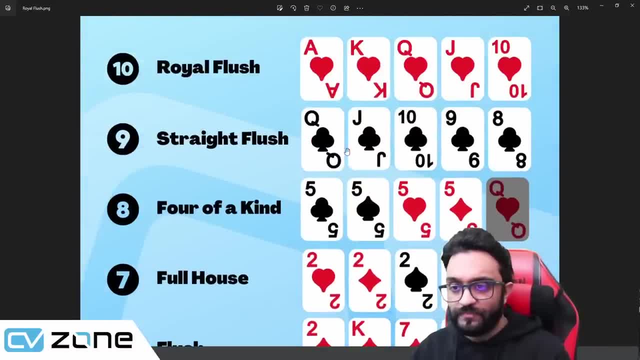 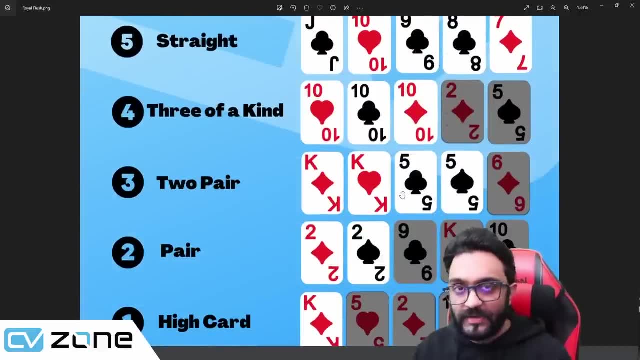 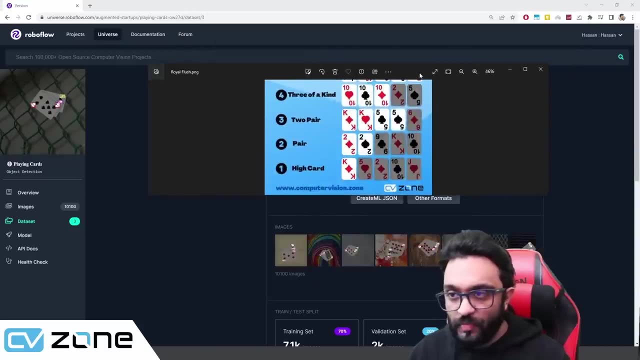 so we'll not do two hands of our own hand, so we will send in five values as strings and it will output us the name of the hand. so that will be interesting to accomplish. so we will keep this image open and I will put it on the side. 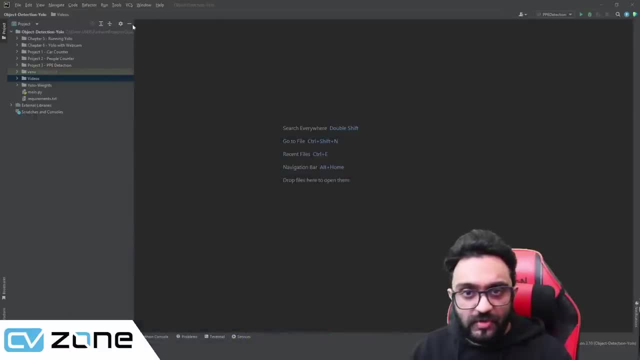 and we will come back to it every now and then. so let's start by creating the folder, and we are going to call it project for poker hand detector. so poker hand detector. we are going to start off with that, okay. so what we will do is we will create. 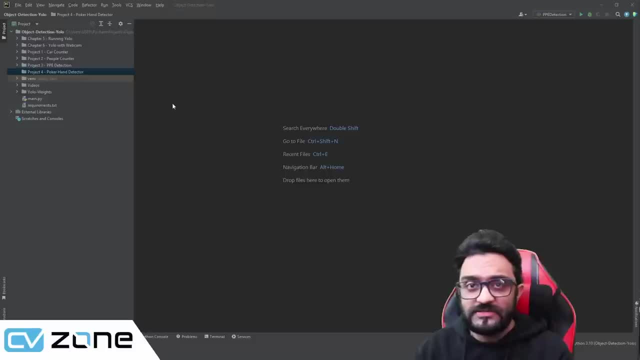 a function and this function we will input it five strings, or you can say a list with five strings, and it will output us the result. so we will create it as a module, so that we can simply link it to our project. so here we will create a new python file. 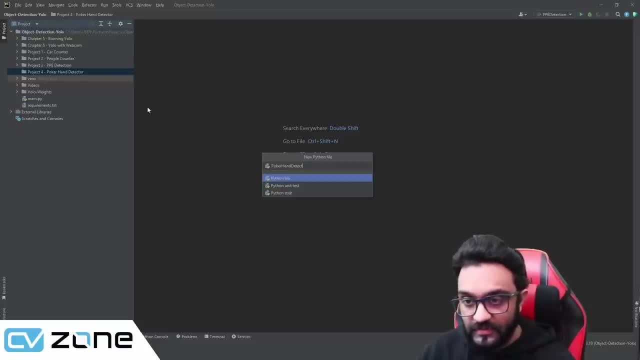 and we will call it poker hand detector function. let's call it. so here we are going to write: def find poker hand. so that's how you write what you want to write. so you will have this in this folder there, because you have to return something and 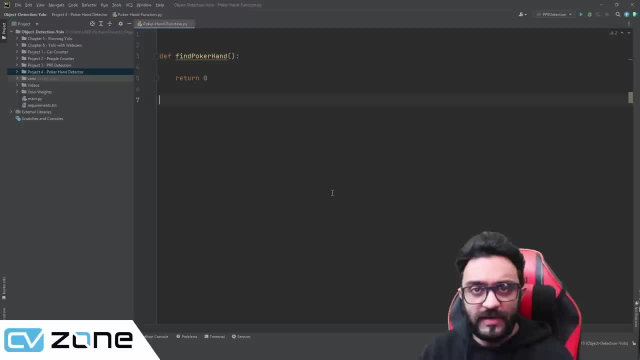 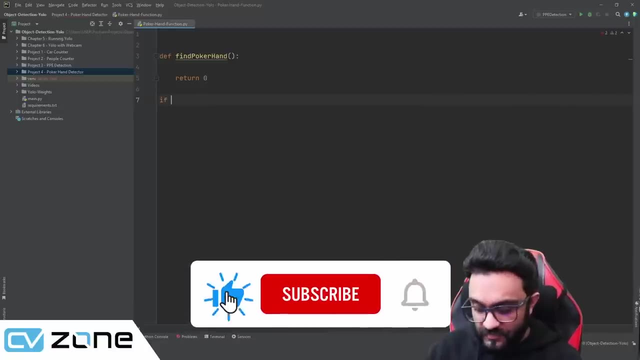 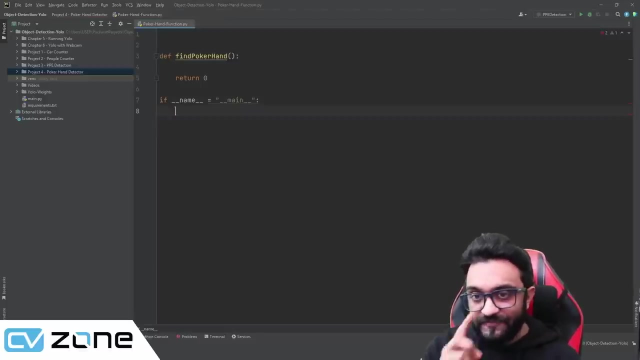 right now we will return zero. okay, so that's good, and then what we have to do is we will be testing it as well. so this means that it is checking. if this is the main file that is running, then it will run this code. if some other file is calling this function, it will not run this code. so, yeah, we have to put. 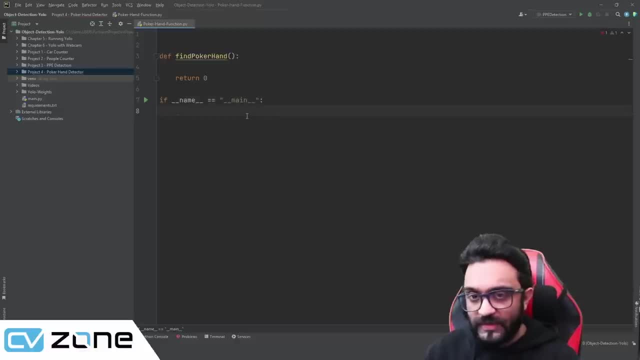 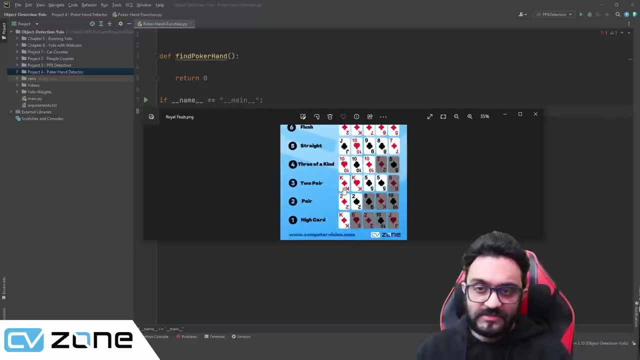 double equal. there you go. so now what we can do is we can send in a few, what do you call hands. so let's start off. so here is our image. so let's start off by creating all these hands and, one by one, we are going to send it to see what it gives. so, first of all, let's start. we are going to start. 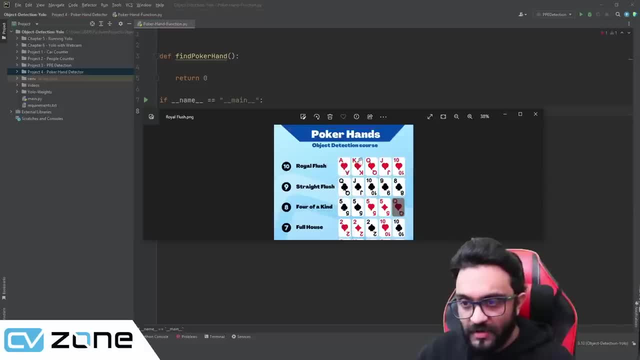 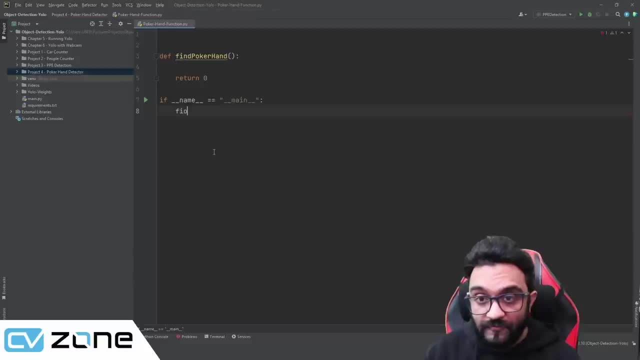 at the top we'll start with royal flush. so a of hearts, k of hearts, queen, and so on. so here we will write find, find, poker hand and we will send in a list and inside the list we will give a of hearts, then k of hearts, then we will give queen of hearts, then we will give jack of hearts. 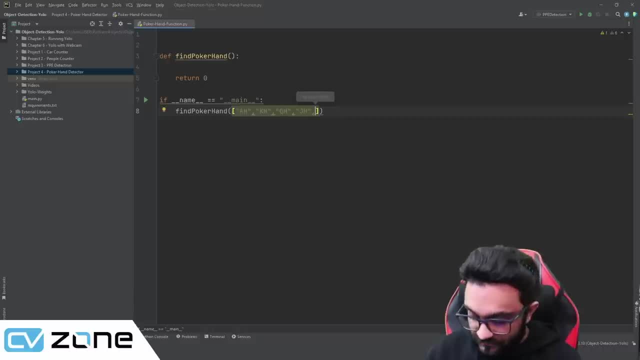 jack of hearts and then we are going to give 10 of hearts. so this will be our royal flush, and And in front of it we are going to write Royal Flush, And then we will copy this and we are going to paste. And then the second one we will do is Straight Flush. 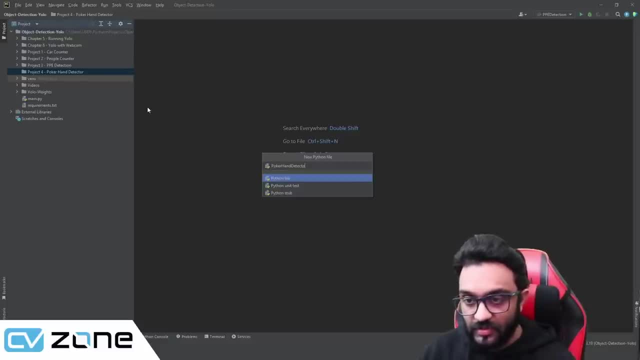 call it poker hand detector. uh, function, let's call it. so here we are going to write: uh def, find poker hand. so that's how you write. uh, what do you call a function? and we have to return something, and right now we will return zero. okay, so that's good. and then what we have to do is: uh, we, we will be testing it as well. so we need 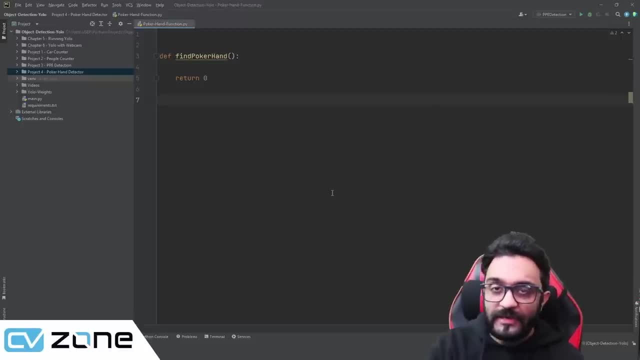 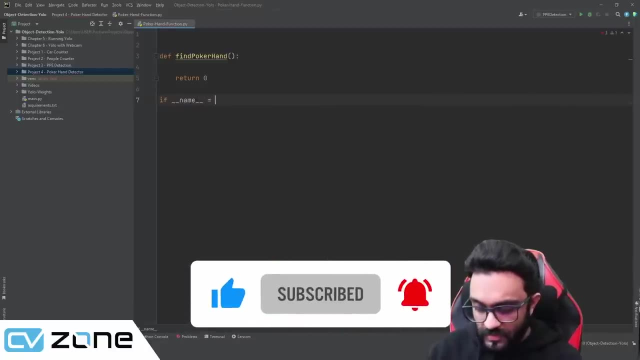 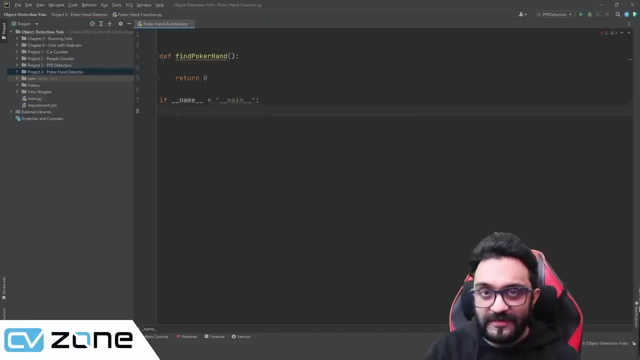 to make sure that we run this individually and then we will integrate it to our project. so we will write if underscore underscore name equals underscore underscore main. so this means that it is checking. if this is the main file that is running, then it will run this code. if 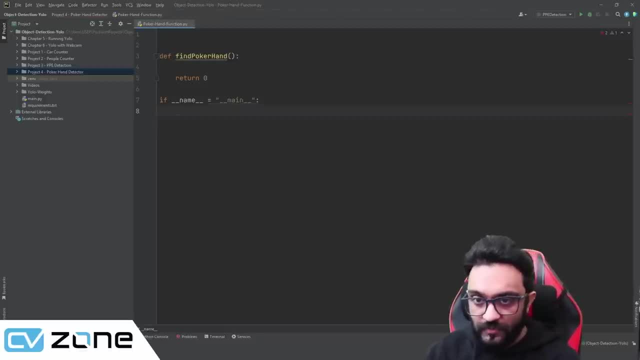 some other file is calling this function, it will not run this code. so, yeah, we have to put double equal. there you go. so now what we can do is we can uh send in a few- uh, what do you call hands? so let's start off. so here is our image. so let's start off by creating all these hands. 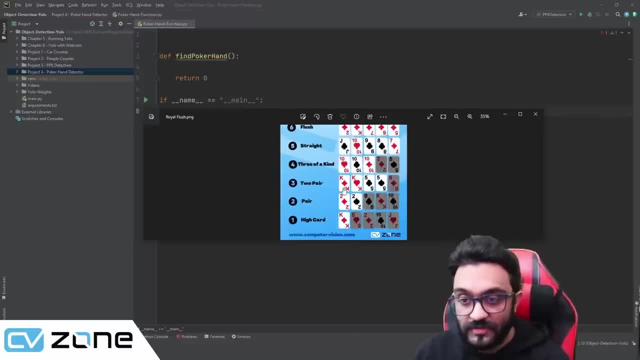 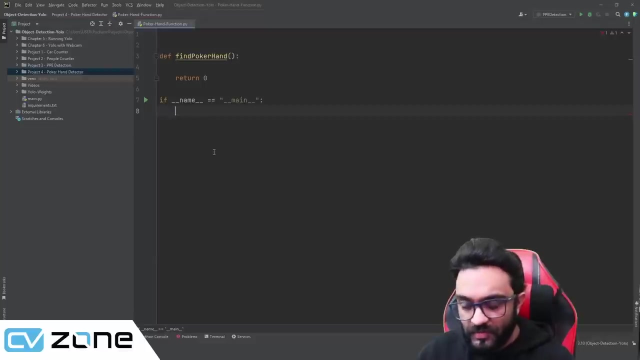 and one by one, we are going to send it to see what it gives. so first of all, uh, let's start. we are going to start at the top. we'll start with Royal flush, so a of hearts, K of hearts, queen, and so on. so here we will write, uh, find poker hand, and we will send in a list and inside the list we will 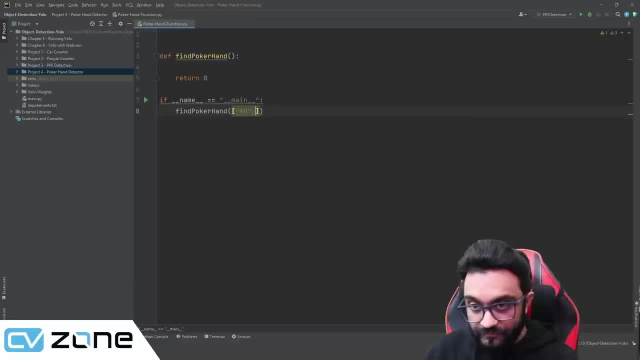 give a of hearts, then K of hearts, then we will give a queen of hearts, then we will give jack of hearts, jack of hearts, and then we are going to give 10 of hearts. so this will be our Royal flush, and in front of it we are going to write royal flush. 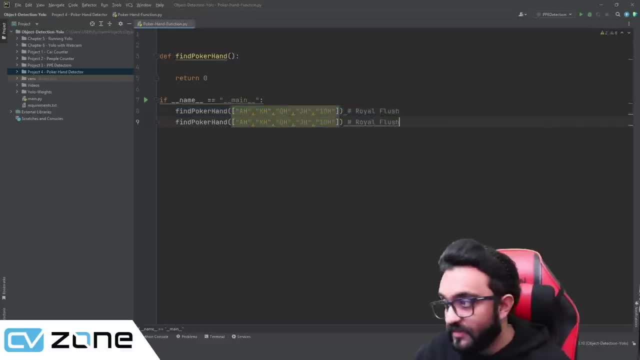 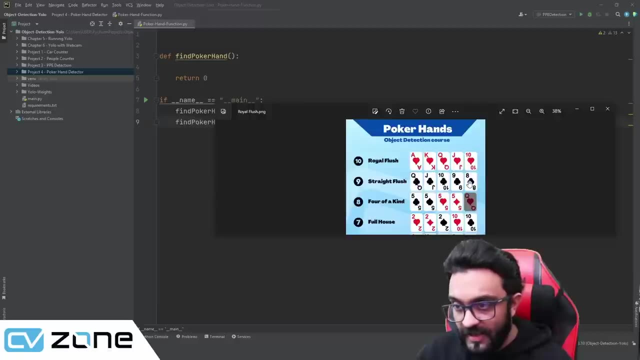 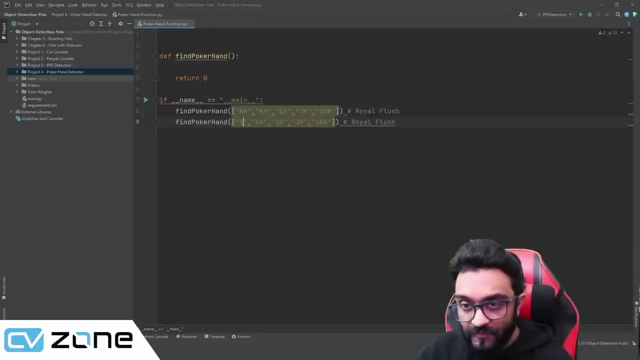 and then we will copy this and we are going paste, and then the second one we will do is straight flush. so again, queen, jack, ten, nine, eight, but all of them are clubs. so queen, queen of club, then jack of club, then ten of club, nine of club and eight of club. so this is not a royal flush, it is a straight s-t-r-a-i-g-h-t straight. 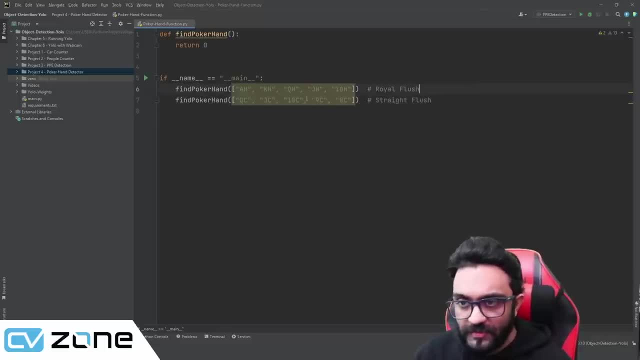 flush. so these are the two that we are starting off with. so let's run that and see what do we get? so no, actually we'll get nothing. so what we have to do is we have to return. uh, let's return. we will put here hand and we will return the hand. okay or no, we'll not return the hand. we want to print it. 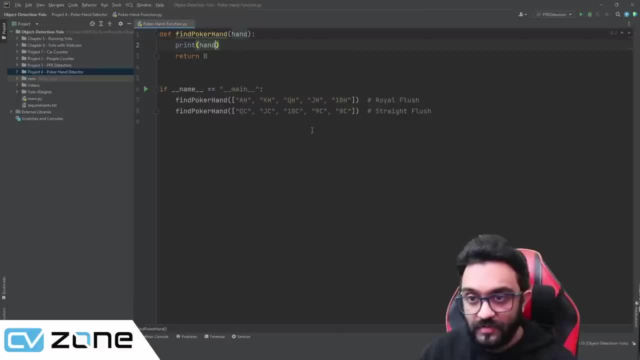 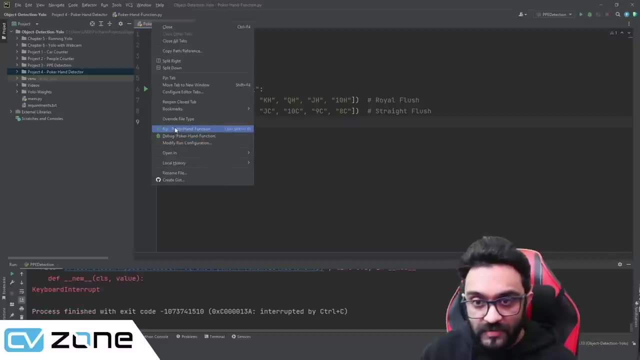 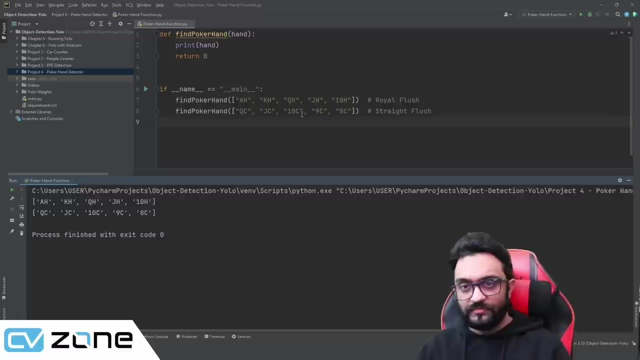 so we will print the hand, okay, so let's run that and see what do we get. uh, no, we are running the previous one. right click and run and there you go. so now we are getting this: uh, these two as the output. so that's good, we have started. 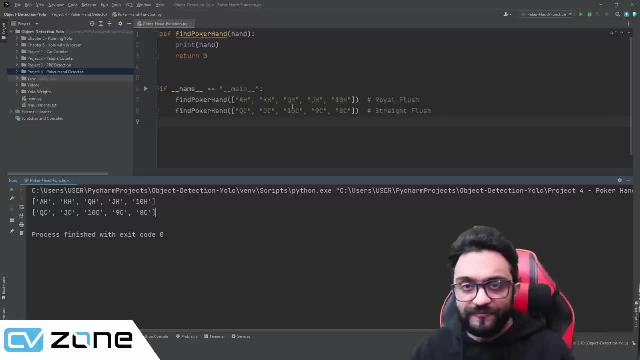 and the first thing we will do is we are going to bring here a classic soccer club will do is we will find the ranks and we'll find the suits individually and put them in a list, because what we are trying to do is we are trying to understand some of them. we will classify based 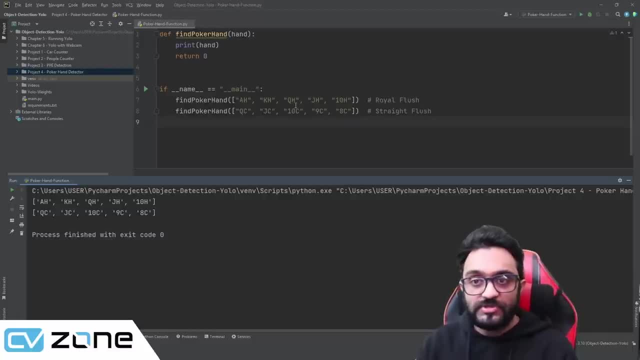 on ranks, some of them classifying based on suits. so if we have them in a list we can play around with them very easily. so that will be our first step. we need to make sure that we have the ranks and the suits all in two different lists. so here we will write: ranks equals a list and then suits. 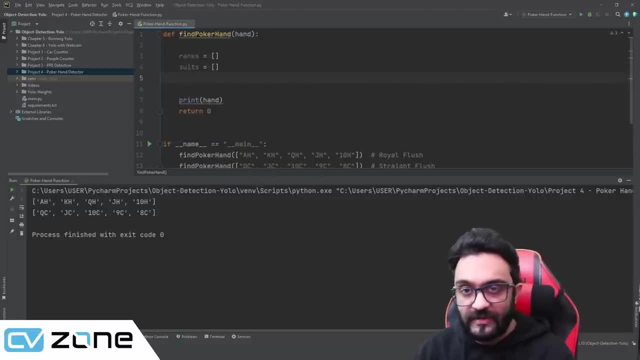 equals a list. so these are the two lists that we have and we are going to loop through the hand and, for card in hand, we are going to loop through the card and, first of all, what we can do is if, if i wanted the rank, for example, i want the rank, which is the first. 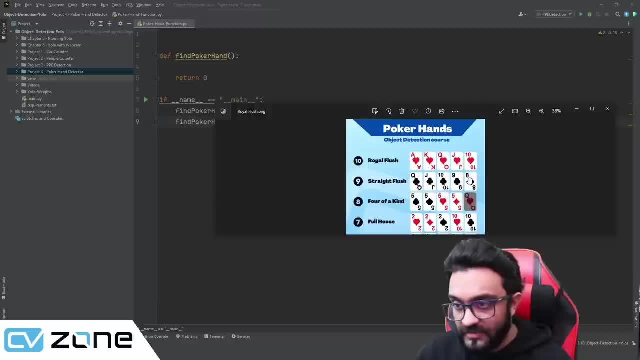 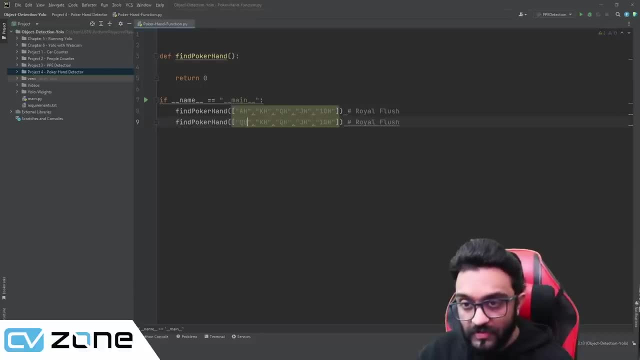 So again Queen, Jack, 10,, 9,, 8.. But all of them are clubs. So Queen, Queen of Club, then Jack of Club, then 10 of Club, 9 of Club and 8 of Club. 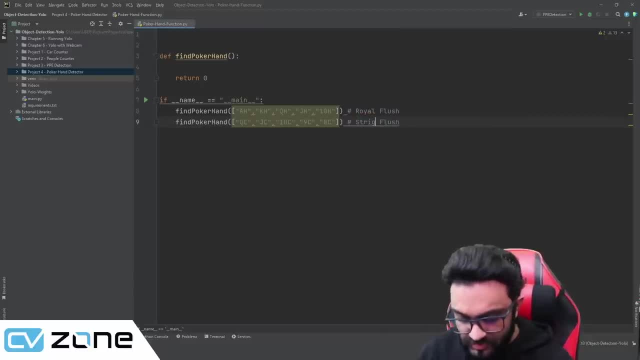 So this is not a Royal Flush, It is a Straight Flush. So these are the two that we are starting. So let's run that and see what do we get? So no, actually we will get nothing. So what we have to do is we have to return. 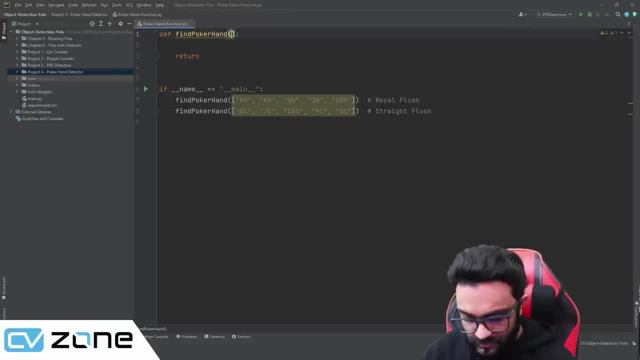 Let's return. We will put here Hand And we will return the Hand. Okay Or no, we will not return the Hand, We want to print it, So we will print the Hand, Okay. So let's run that And see what do we get. 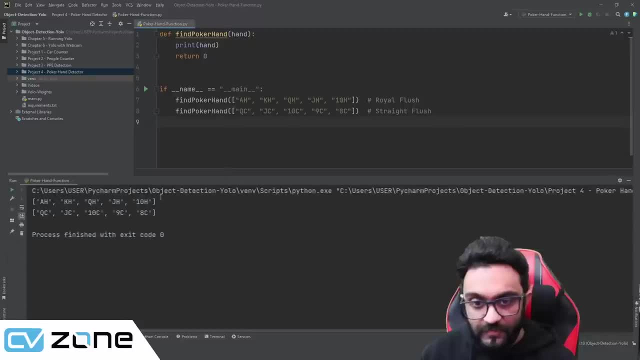 No, we are running the previous one. right Click and run And there you go. So now we are getting this, these two, as the output. So that's good, We have started And the first thing we will do is we will find the ranks and we'll find the suits individually and put them in a list. 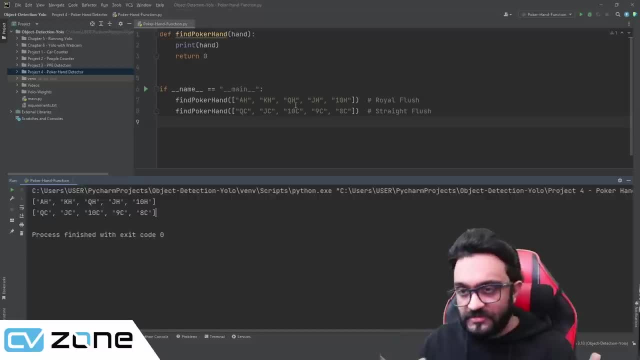 Because what we are trying to do is we are trying to understand. some of them We will classify based on ranks, Some of them Classifying based on suits, So if we have them in a list, we can play around with them very easily. 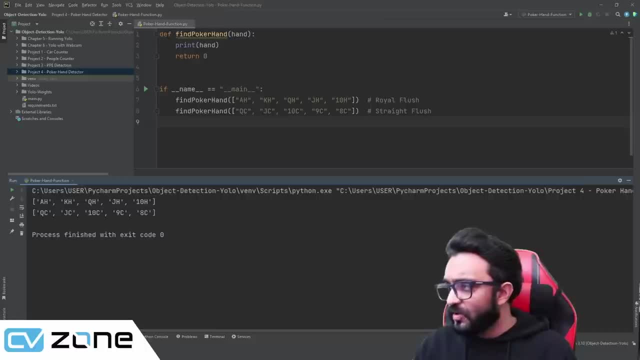 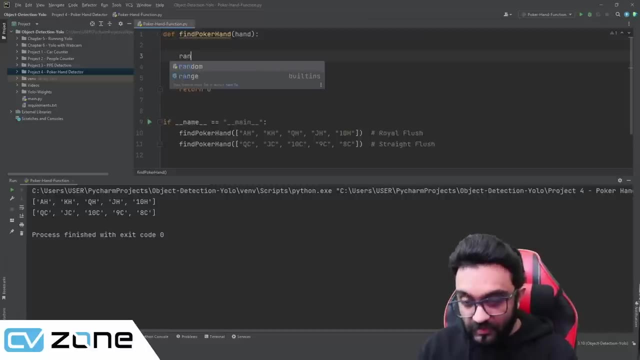 So that will be our first step. We need to make sure that we have the ranks and the suits all in two different lists. So here we will write: ranks equals a list and then suits equals list. So these are the two lists that we have and we are going to loop through the hands. 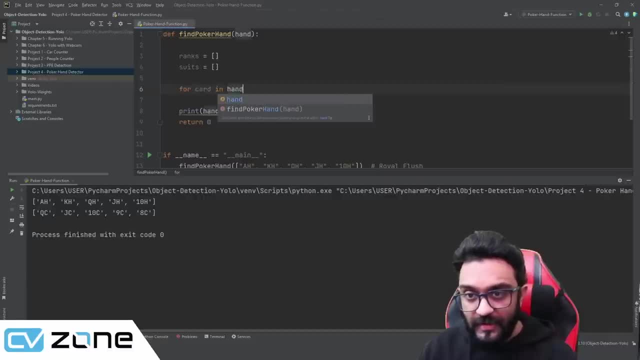 And for card in hand. we are going to loop through the card And, first of all, what we can do is, if I wanted the rank, for example, I want the rank, which is the first element here. So all I have to do is I have to say: card at zero, right. 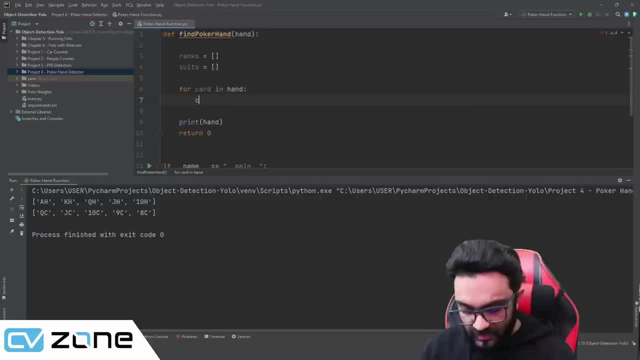 element here. so all i have to do is i have to say: card at zero, right? so let me print that out. so if i write that, that will be my rank. so i'm getting a, i'm getting k queen jack one and all that. so basically i'm getting what i need. but if you 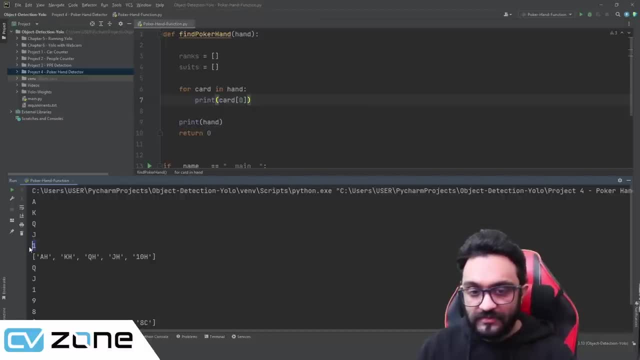 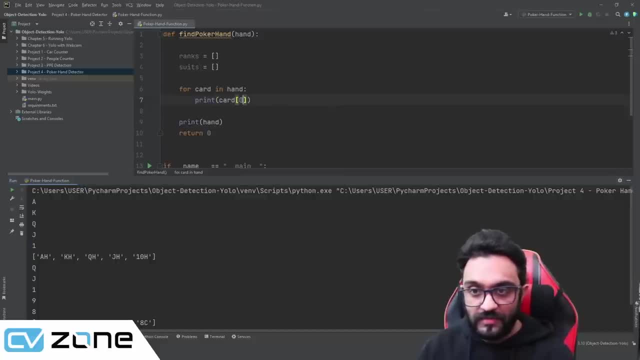 so then i will take two values instead of one. so i need to get zero and i need to get till one- uh sorry, till two, because that's not inclusive. so then i will get ten, but for the rest of them i should not get two, i should get only one. so that's the idea. so i have to check here. 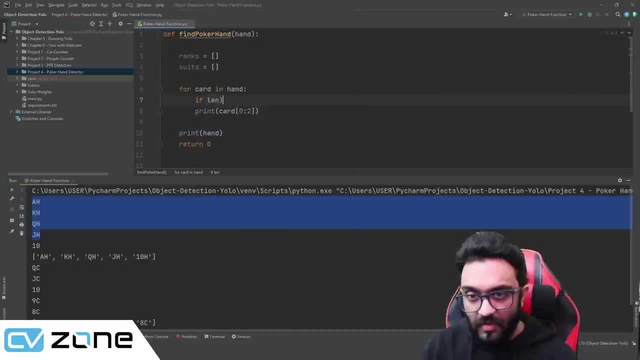 if the length of card equals two, or should we write yeah equals two, then it will be: rank equals uh, card at zero. else, rank equals card at uh, zero. sorry, zero, two, two. so now if we print, print the rank, then it will show us. so for a king queen jack, it's fine, it's getting one, and for ten, it is getting two. 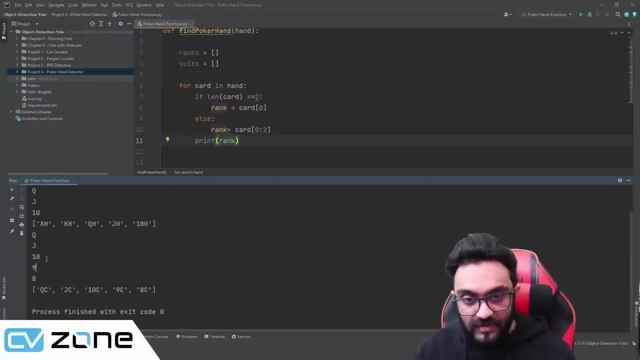 so that's the idea. so for eight, nine, it's fine, for ten, it is getting the two. that is exactly what we needed. so this way we are basically, uh, getting the rank and we also need the suits. so if, if, if the card has the length of two, then the suit is the next value. right? so the suits. 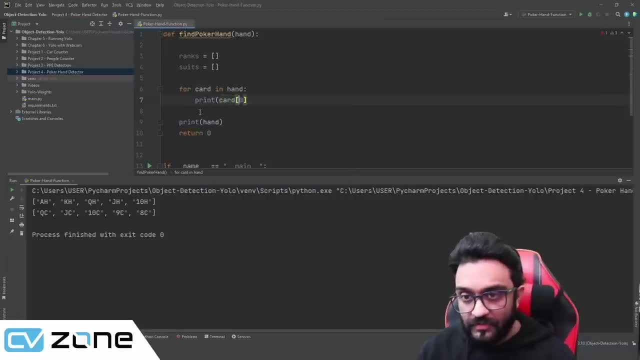 So let me print that out. So if I write that, that will be My rank. So I'm getting a, I'm getting K Queen Jack one and all that. So basically I'm getting what I need. But if you look at the last one, I'm getting one. 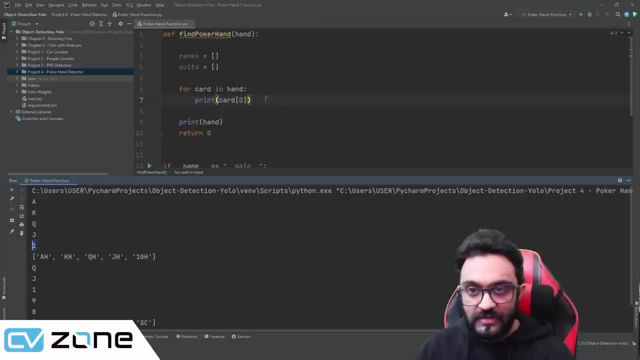 That's wrong. That's not the actual rank. So what I can do is I can I can put an if statement that if the digits are three, Then it means It is a ten. Okay, So then I will take two values instead of one. 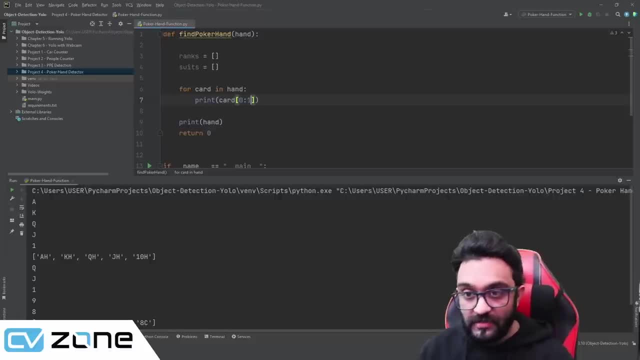 So I need to get zero and I need to get till one- sorry, till two, because that's not inclusive. So then I will get ten, But for the rest of them I should not get two, I should get only one. 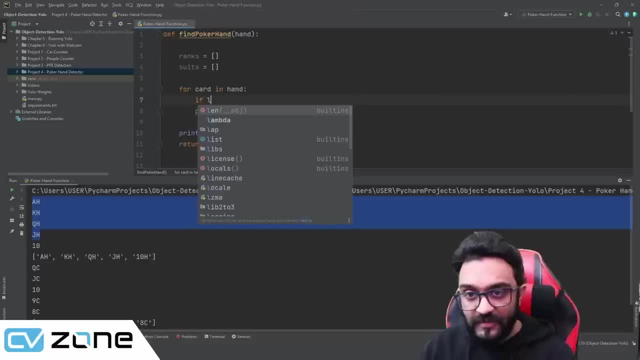 So that's the idea. So I have to check here. If the length Of Card Equals Two, Or should we write Equals two, Then it will be Rank Equals Card At zero, Else Rank. 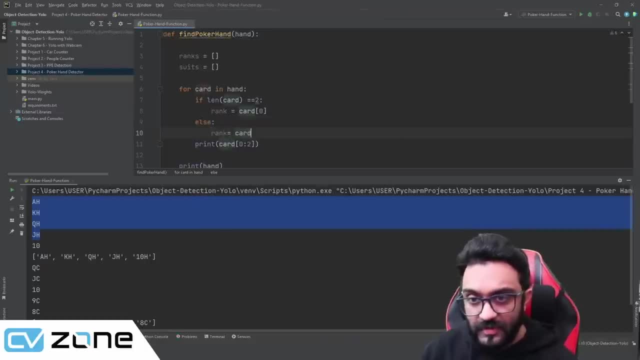 Equals Card At Zero. Sorry, Zero Two, Two. So now if we print, Print The rank, Then it will show us. So for a king queen jack, it's fine, It's getting one. 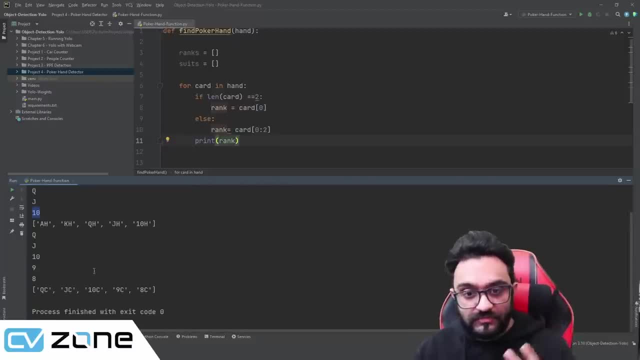 And for ten it is getting two. So that's the idea. So for eight, nine, it's fine, For ten, it is getting the two. That is exactly what we needed. So this way We are basically Getting the rank. 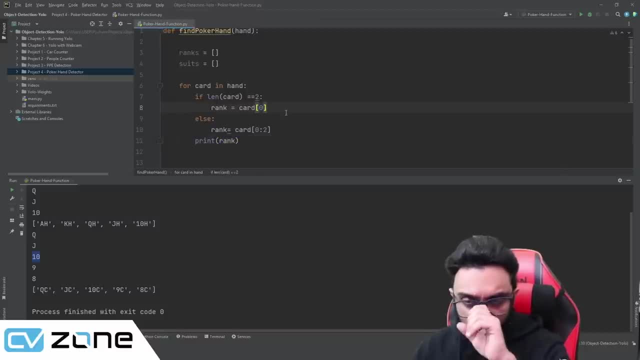 And we also need the suits. So If, If, If the card Has the length of two, Then the suit Is the next value, Right, So the suits Equals Card At one. But if that's not the case, 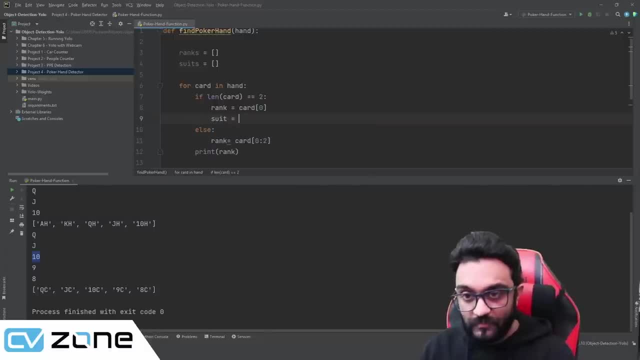 Then the suit Is the next value Right. So the suits Equals Card At one. But if that's not the case, Then the suit Is the next value Right. Then the suit Is basically Card At. 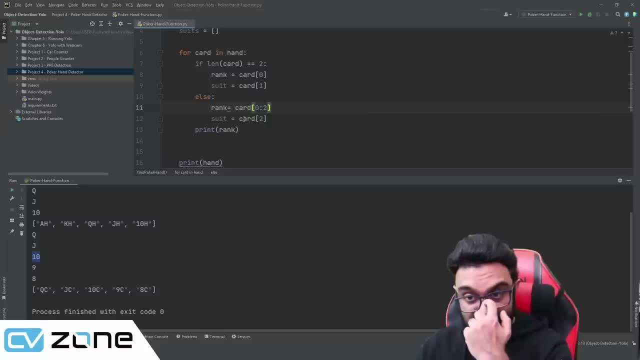 Two. So Zero, One Two. So That's the idea, And now We will have the Rank And the Suit, So they will be Separately detected. There you go, So, A Of hearts. 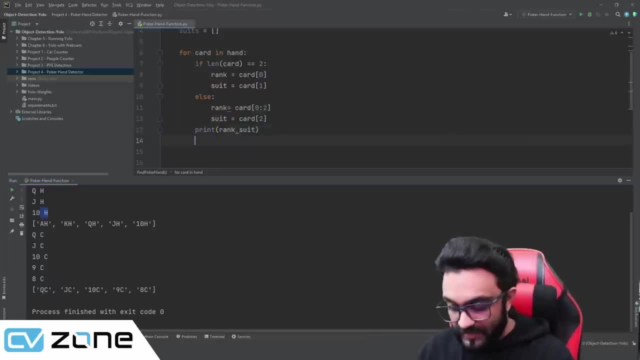 King Of hearts, Queen Of hearts, Ten of hearts, And so on. So now we have it Separately, And the next One, And the Suit, Is The Rank, And That's The. 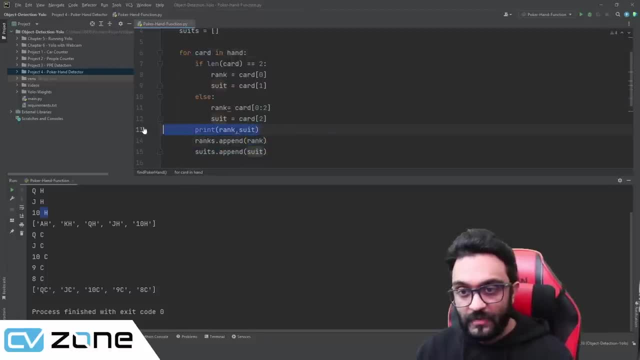 So We will Say Ranks- Dot- Append Rank And Suit- Dot Append Suit, And we have to do it for each card. So this should be Inside And we can remove that. So once that is done, 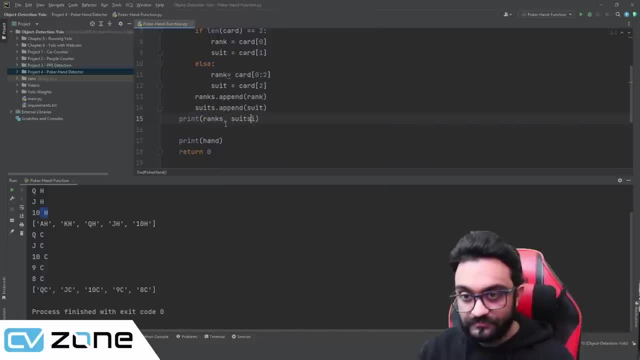 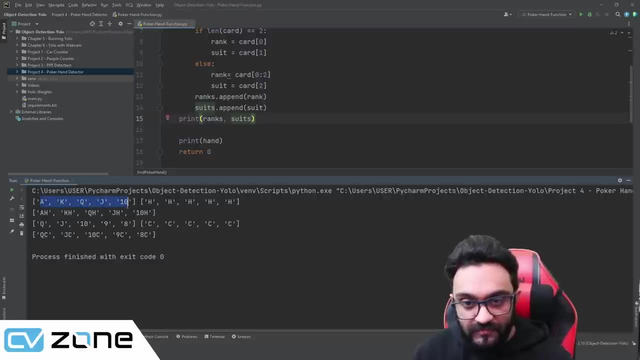 Just To make sure, suits. There you go. So we have the list of ranks and we have the list of suits. We have the list of ranks, We have the list of suits. So that's good. So now, first of all, we are going to start. 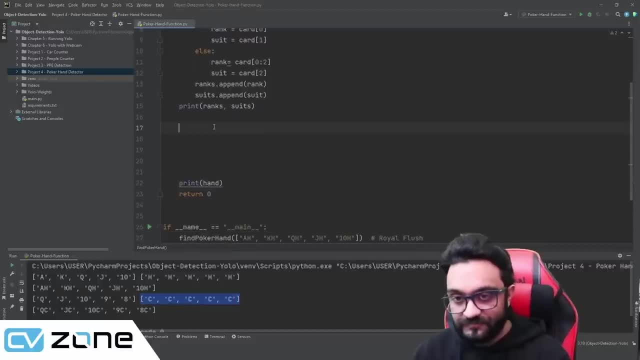 off by Royal Flush. So here we are going to check for Royal Flush Flush and we'll check the rest later on. Now, how can we check for Royal Flush In Royal Flush? the first thing we need to check is whether it is a flush or not. If all of them are same, if all of them are same in the suits. 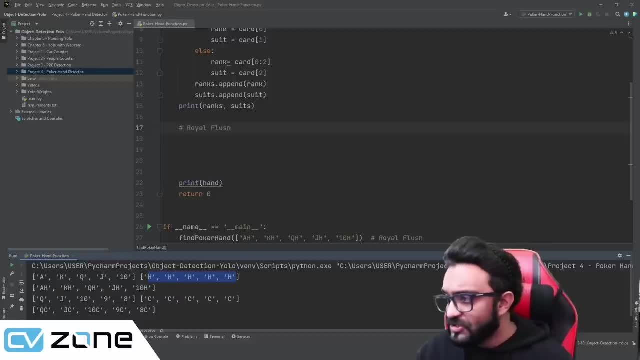 then it is a flush. So how can you do that? So basically, what you can do is you can check if, or let me just print it so that it's easier to see actually what is happening. So what we can do is we can check. 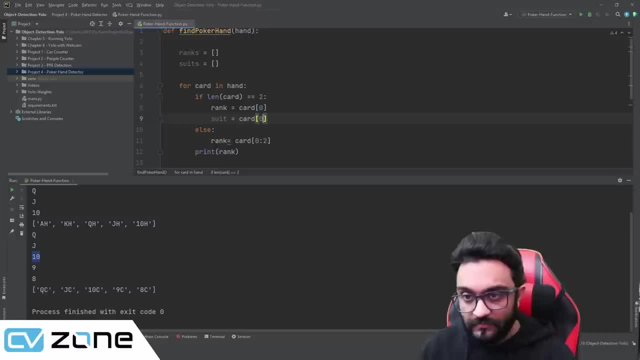 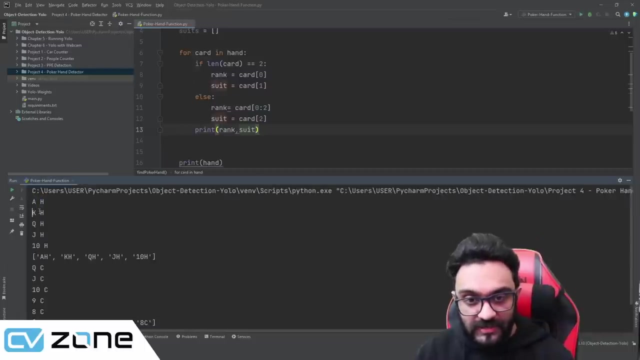 equals card at one. but if that's not the case, then the suit is basically card at two. so zero on two. so that's the idea, and now we will have the rank and the suit, so they will be separately detected. there you go. so a of hearts, king of hearts, queen of hearts, ten of hearts, and so on. so now we have 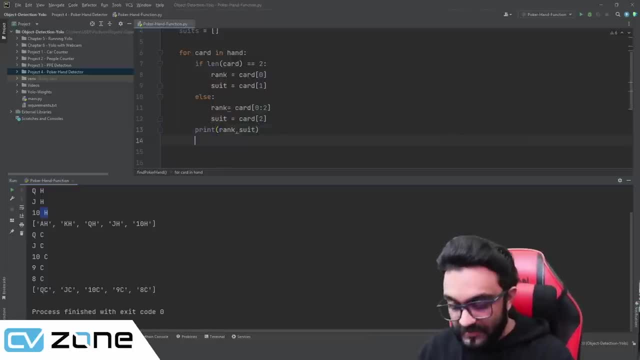 it separately. so all we have to do now is we have to append it to our list. so here we will say ranks- dot- append rank, and suits- dot- append suit, and we have to do it for each card. so this should be inside and we can remove that. so once that is done, just to make sure we are headed in the 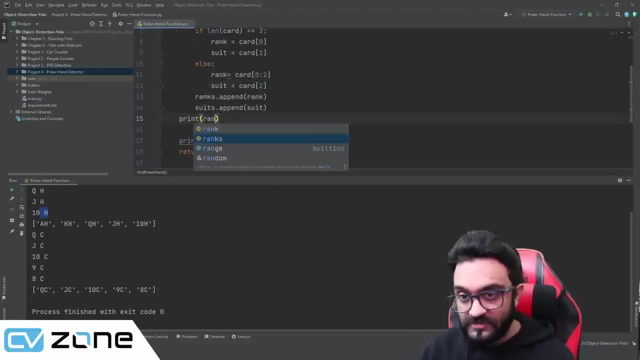 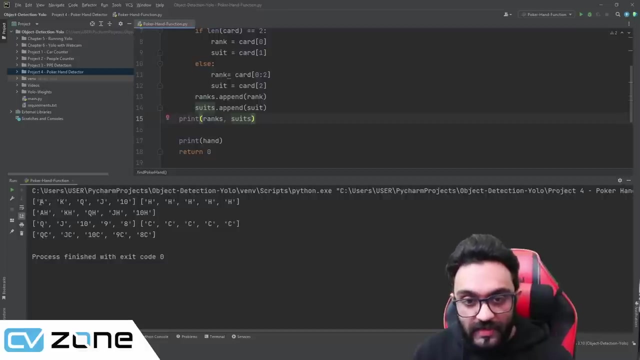 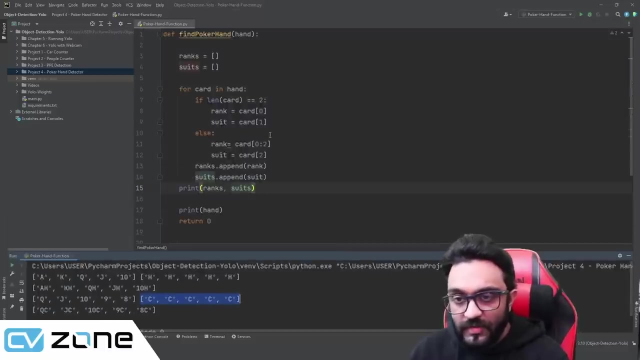 right direction. we will print the ranks. this will be a list of ranks, and then we will also print suits, suits. there you go. so we have the list of ranks and we have the list of suits. we have the list of ranks, we have the list of suits. so that's good. so now, first of all, uh, we are going to start off. 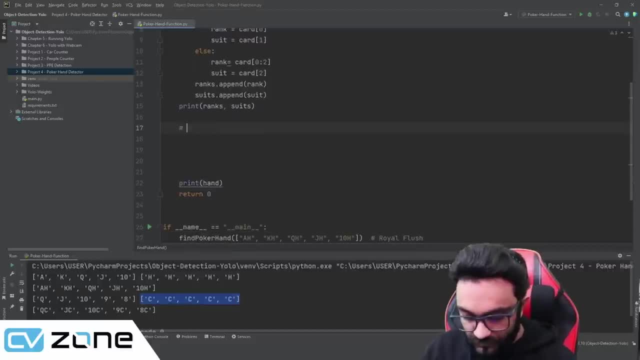 by royal flush. so here we are going to check for royal flush, flush and uh, we'll check the rest later on. now, how can we check for royal flush in royal flush? the first thing we need to check is whether it is a flush or not, if all of them are same, if all of them are same in the suits. 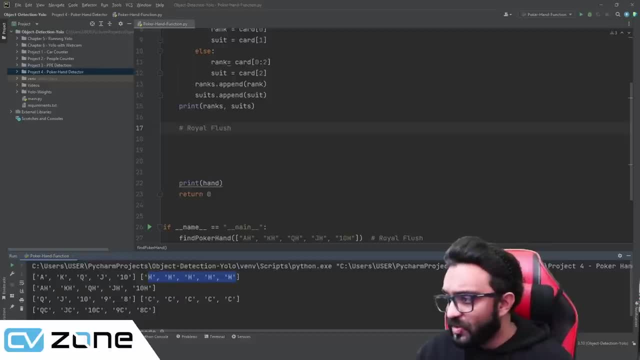 then it is a flush. so how can you do that? so basically, what you can do is you can check if, or let me just print it so that it's easier to see actually what is happening. so what we can do is we can check for the suits. 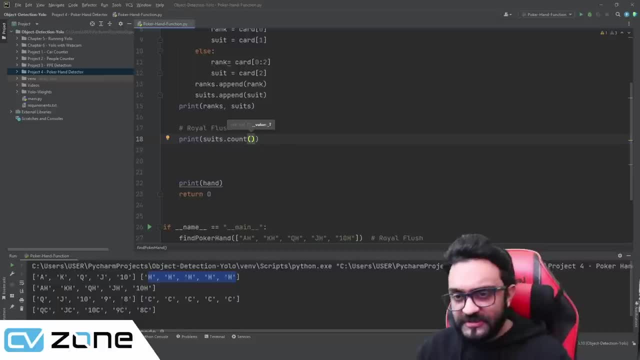 dot count the first element. okay, it can be anything, because all of them have to be same in order for this to be true. so you can pick any element from the list, so you can write suits at zero. so basically, we are asking it to count the number of times you are getting this element. so 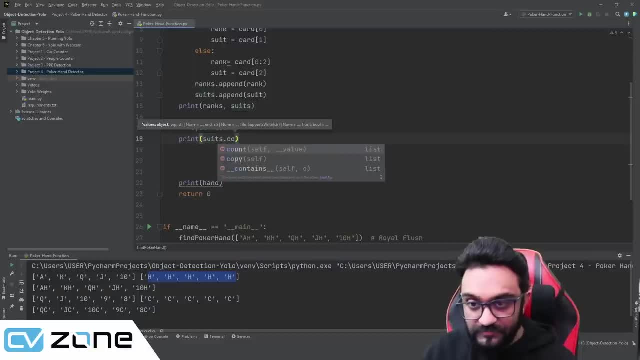 for the suitscount, the first element. It can be anything, because all of them have to be same in order for this to be true. So we can check for the first element, So we can check for the second element, So you can pick any element from the list, So you can write suits at zero. So 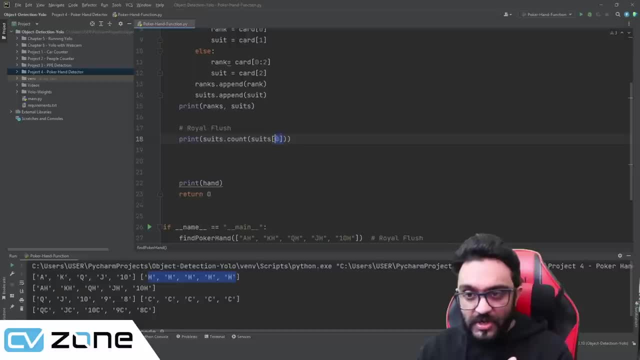 basically, we are asking it to count the number of times you are getting this element. So, for example, it will take H and it will count how many times we have H in this list. If that is equal to five, then it means all of them are. 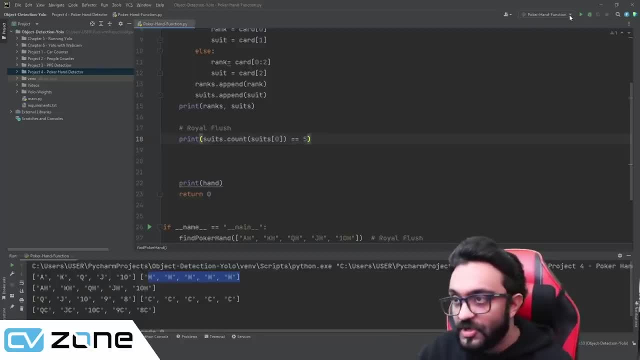 a flush, Then all of them are the same, then it's a flush, So let's run it. So in the first one it's true, And in the second one it's also true, But let's put another hand, poker hand. we are going to. 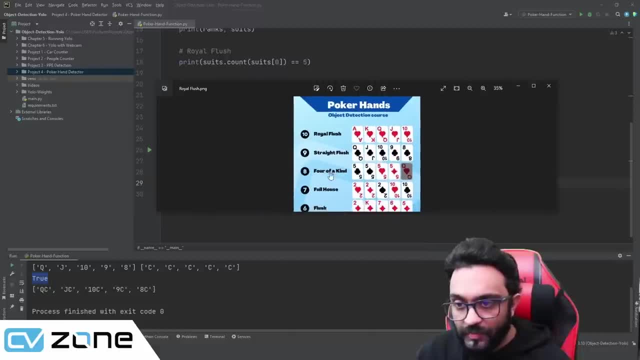 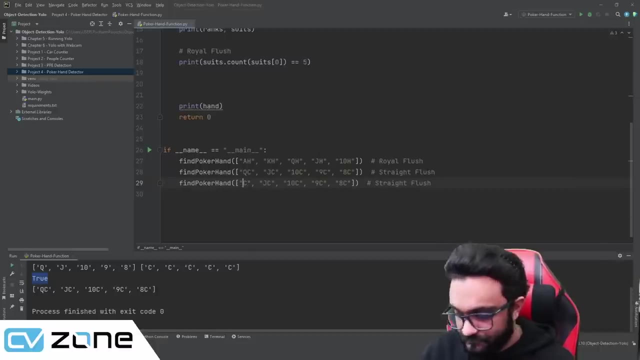 put. let's say we will put another hand. Let's put four of a kind which is next, So it is 5555, and queen, So it is five of club, five of spade, five of hearts, five of diamond, And we have queen of hearts. 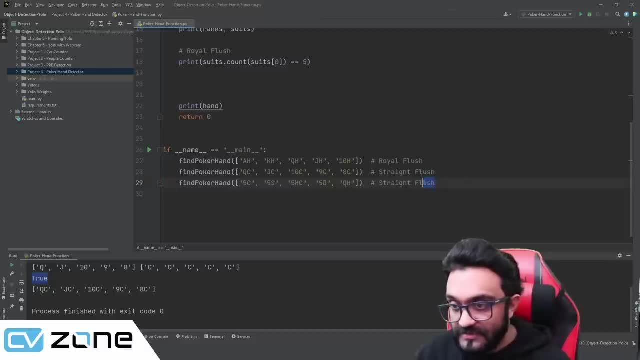 queen of hearts. So this is what is it? four of a kind? So in that case, it will be four of a kind. So in that case, it will give us a false because all of them are not same. So the last one, it is giving us false because it is not a. 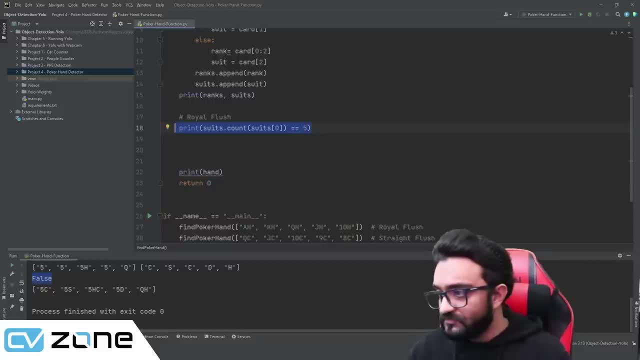 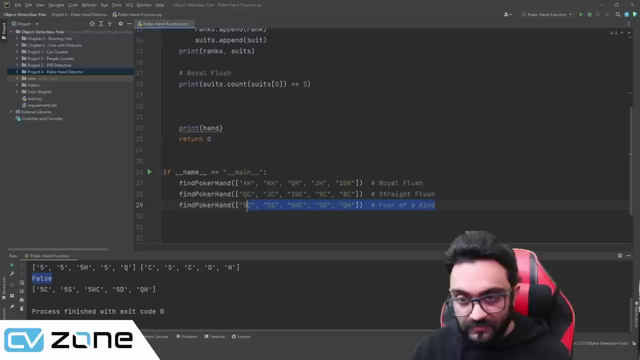 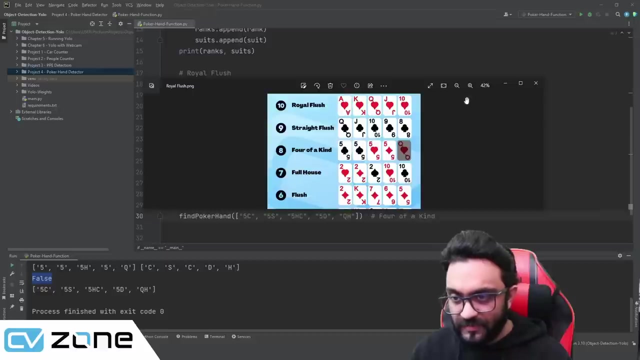 flush. So this is only checking for a flush. By the way, the next one, no, the one after that is a flush. So let's put a flush as well. So we'll have another one. So let's just put full house as well. We'll put full house and flush both of. 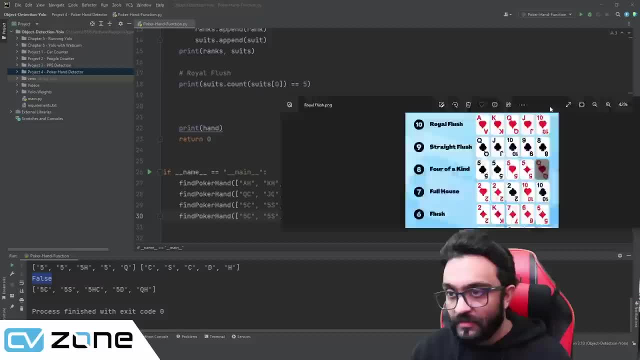 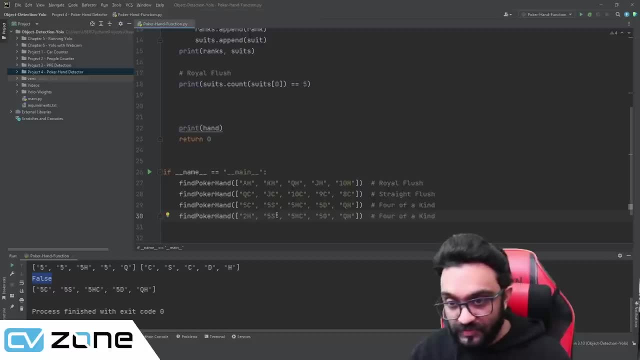 them. So these are two to two to 1010.. So two of. so I'm writing it exactly like it is, so that there is no confusion of what we are doing: Two of diamonds and two of spade. Two of spade, two of spade. What is this? Why is that like this? It should be hearts, not. 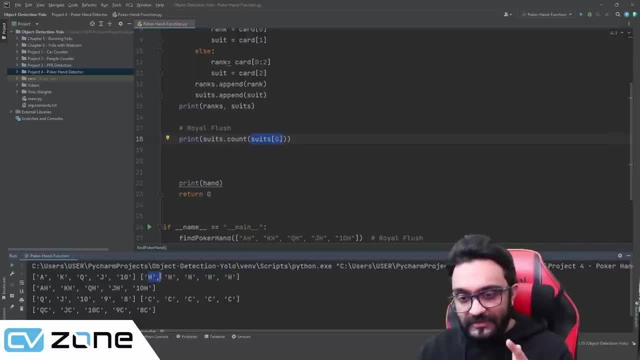 for example, it will take h and it will count how many times we have h in this list. if that is equal to five, then it means all of them are- uh, it's a flush. then all of them are the same. then it's a flush. let's run it. so in the first one it's true, and in the second one it's also true. 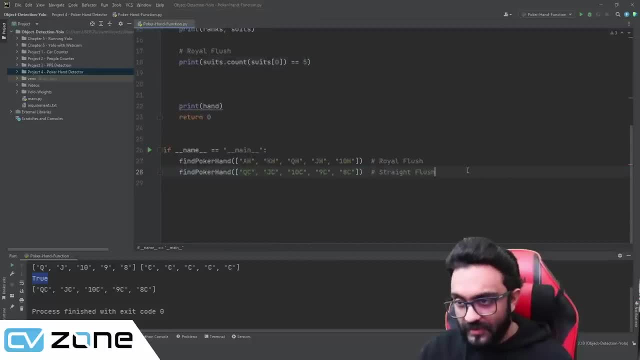 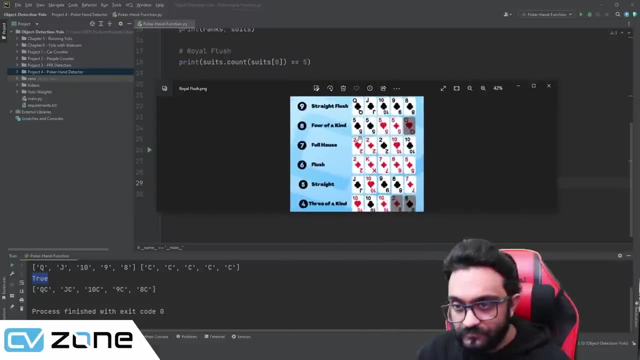 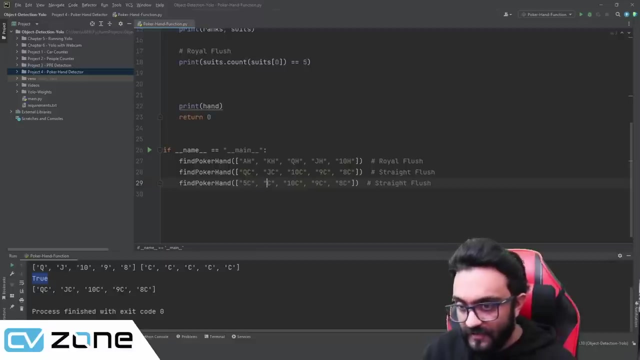 but let's put another hand, poker hand we are going to put, let's say, say we will put another hand, let's put four of a kind which is next. so it is five, five, five, five and queen. so it is five of club, five of spade, five of hearts, five of diamond. 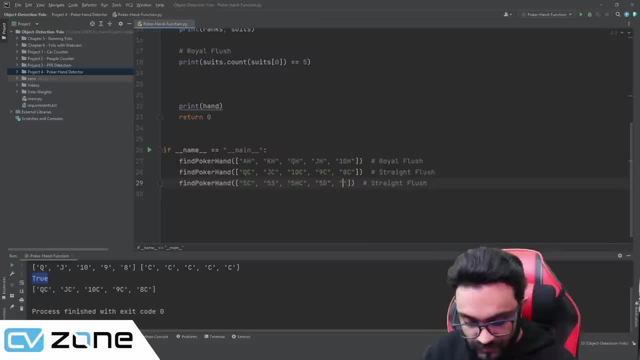 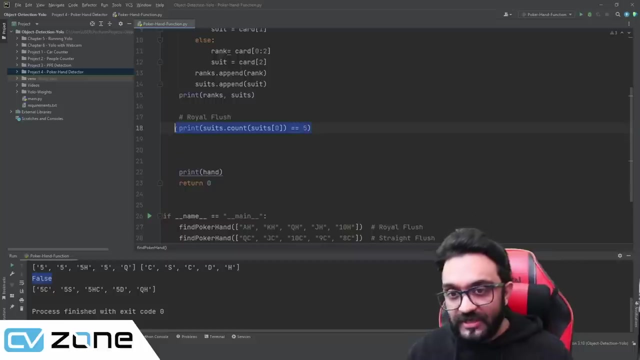 and we have queen of hearts, queen of hearts. so this is what is it? four of a kind. so in that case, it will give us a false because all of them are not same. so the last one: it is giving us false because it is not a flush. so this is only checking for a flush. by the way, the next one: 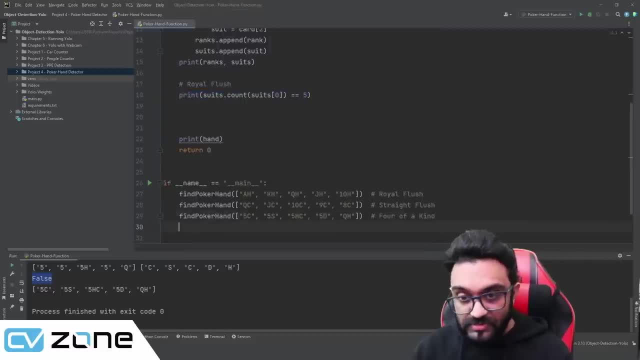 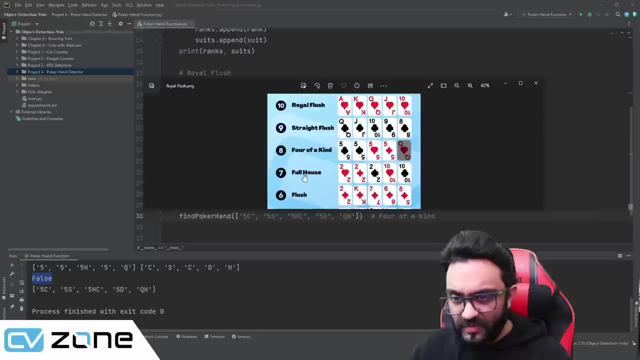 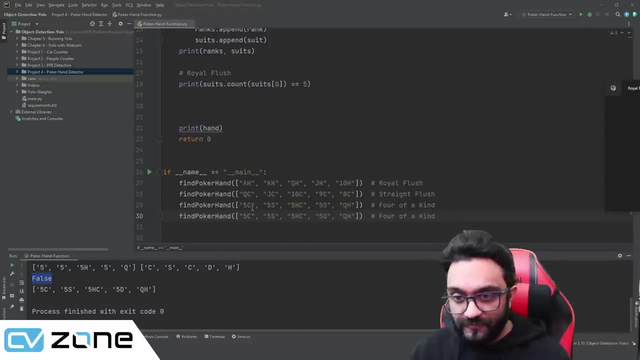 no, the one after that is a flush. so let's put a flush as well. so we'll have another one. so let's just put full house as well. we'll put full house and flush both of them. so these are two, two, two, two and ten, ten. uh, so two off. so i'm writing it exactly like it is so. 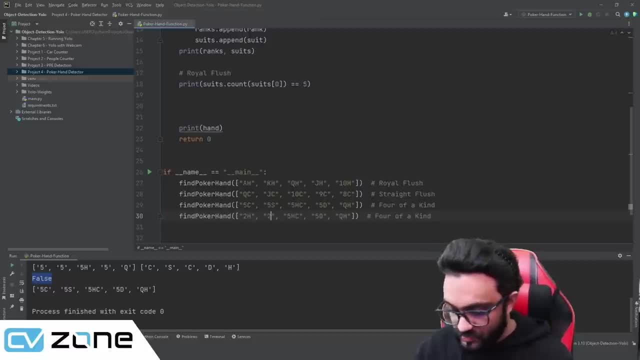 that there is no confusion of what we are doing. uh, two of diamonds and two of spade. to of spade, two of spade. so what is this? why is that like this? it should be hearts, not club. okay, two of spade and then 10 of hearts and then 10 of spade. club. there you go. so this one is what is it full house? uh, full. 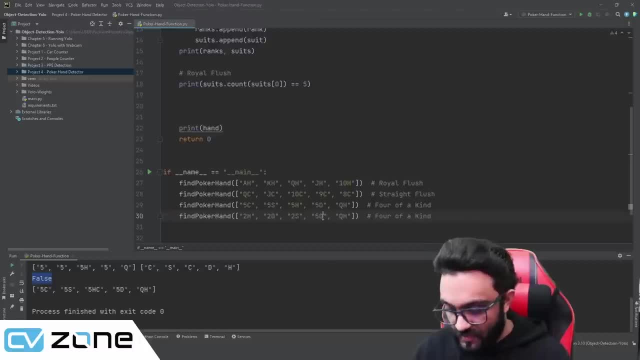 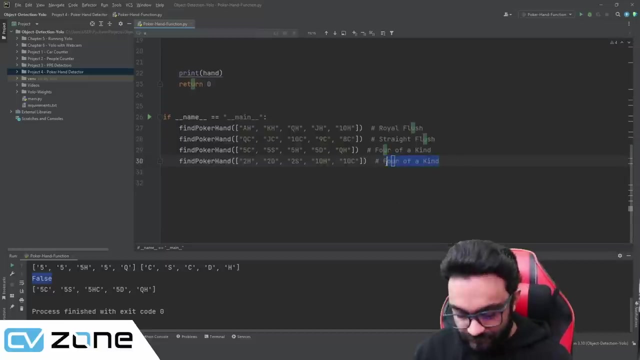 club: Okay, two of spade and then 10 of hearts, And then 10 of spade. club: There you go. So this one is what is it? Full house, Full, full house. And the next one, Next one, will be flush. 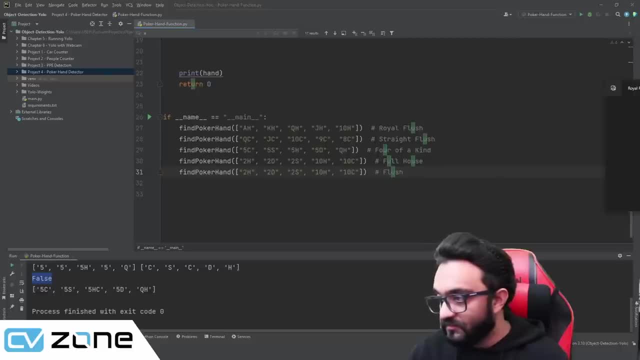 So in flush you have- I'm using again the same one- two of diamonds, Then all of them they will be diamonds. So this will be king of diamonds. This is seven of diamond, Then we have six of diamond, six of diamond and five of diamond, Five of diamond. So let's run that. 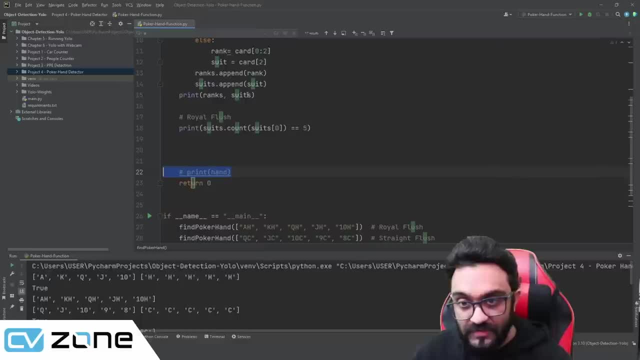 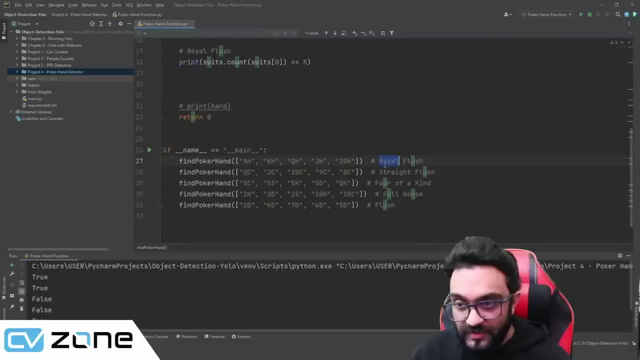 giving us a lot of outputs. So let's not print the hand and let's not print the ranks and suits, And we run that and there you go. So the first one has a flush. So it's true. the second one is also a. 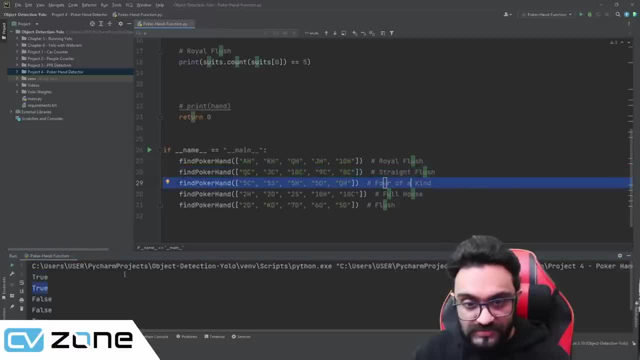 straight flush, so it's true. The third one is four of a kind, so it's false. The fourth one is also false because it's a full house And then we also have another flush, so it's true. So this means this methodology. will first of all tell us, whether will first of all tell us, whether will first of all will tell us whether it's a flush or it's not. So it's the first of all fact which will believe us. So here it's: three by three, by three, which means this cards match that. 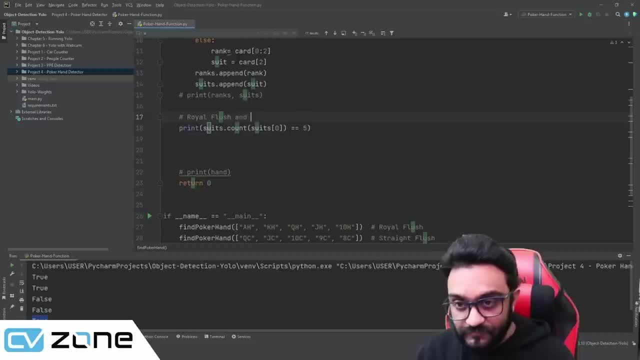 or not. so we can check for royal flush and we can check for straight flush and we can also check for flush. so we can check three of these things right away. so if we go in, if we have this first condition, if that is true, it means it is a flush. now, once we know it is a flush, we can get to the 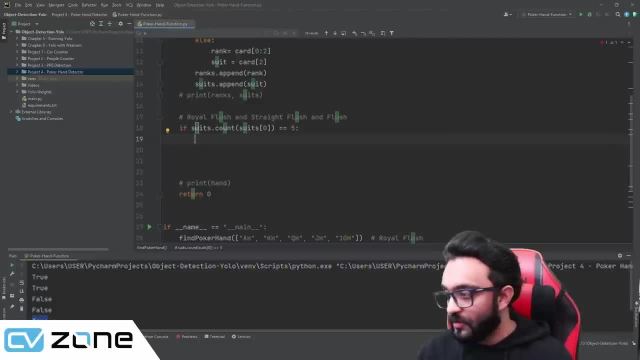 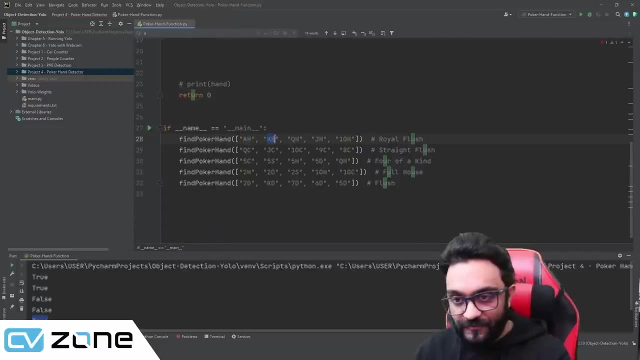 second step, checking whether it's a royal flush or not. so in in the royal flush we must have the ranks. so uh, but. but the thing is that it might be a of hearts, king of hearts, but it might be, um, sorted wrong. so we need to make sure, first of all, that they are sorted properly. so the biggest 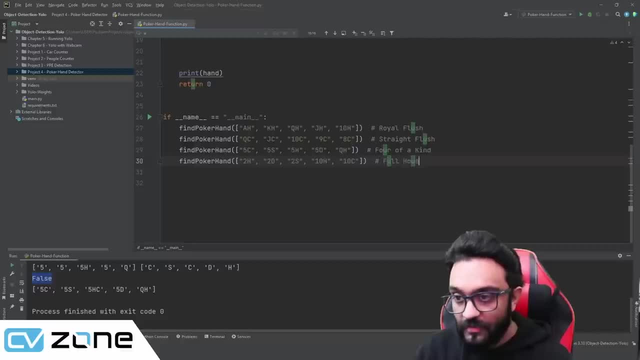 full house. and the next one, next one will be uh flush. so in flush you have- uh- i'm using again the same one- two of diamonds, then all of them, they will be diamonds, so this will be king of diamonds. this is seven of diamond, then we have six of diamond, six of diamond and five of diamond. 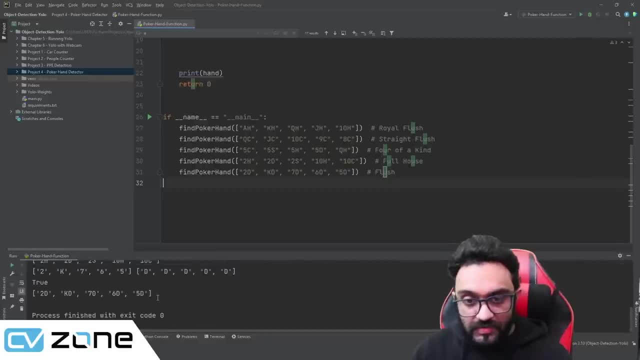 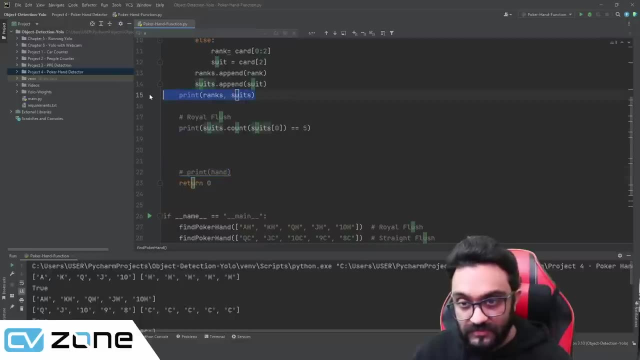 five of diamond. so let's run that. uh, it's giving us a lot of outputs, so let's not print the hand and let's not print the ranks and suits. uh, and we run that. and there you go, so the first one has a flush. so it's true. so let's run that. and there you go. so the first one has a flush. so it's true. 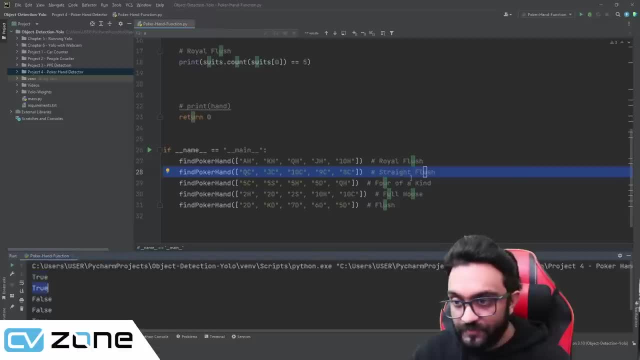 ready, so it's true. the second one is also a straight flush, so it's true. the third one is four of a kind, so it's false. um, the fourth one is also false because it's a full house and then we also have another flush, so it's true. so this means this methodology will, first of all, 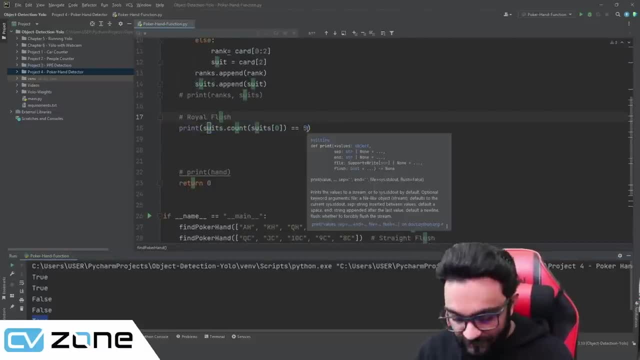 tell us whether it's a flush or not. so we can check for royal flush and we can check for straight flush and we can also check for flush. so we can check three of these things right away. so if we go in, if we have this first condition, if that is true, 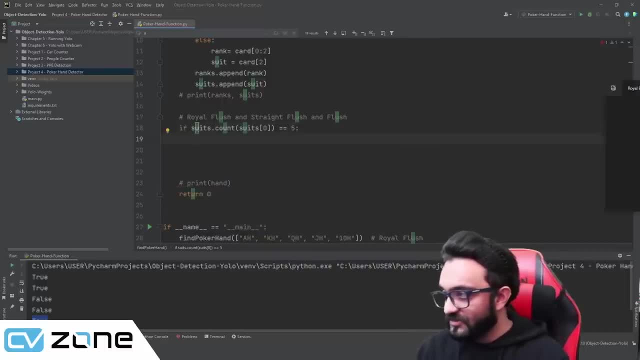 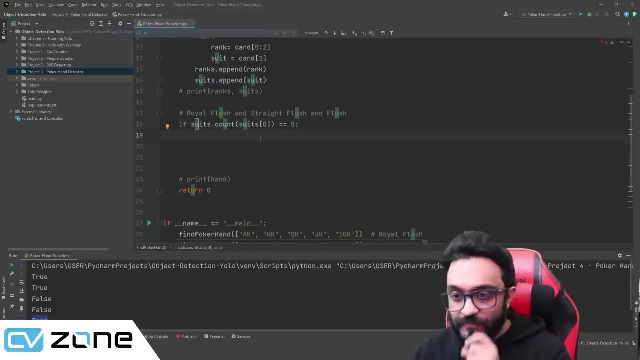 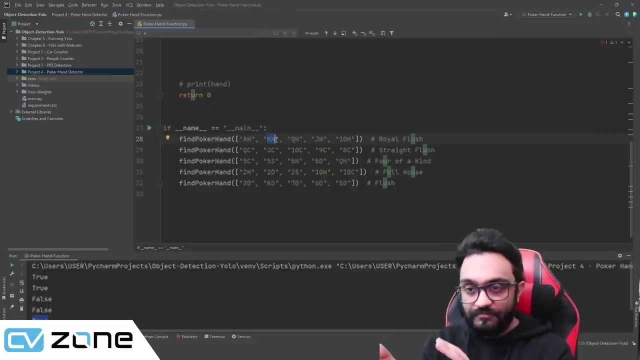 it means it is a flush. now, once we know it is a flush, we can get to the second step, checking whether it's a royal flush or not. so in in the royal flush, we must have the ranks. so uh, but, but the thing is that it might be a of hearts, king of hearts, but it might be um, sorted wrong. so 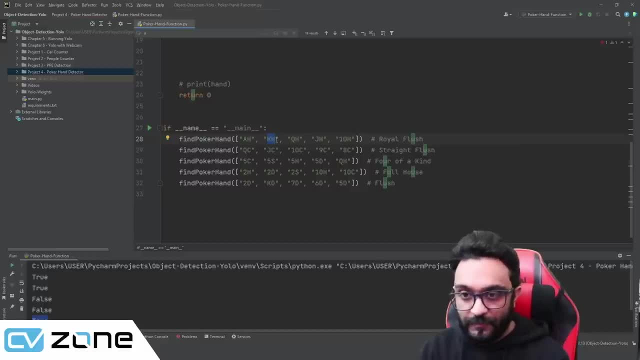 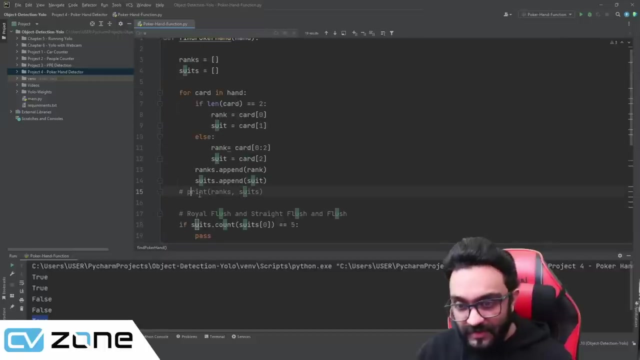 we need to make sure, first of all, that they are sorted properly. so the biggest one, the highest rank, should be the first. but a king queen does not have a rank yet, because if we print it out, if we print out the ranks, uh, let's just write pass here. if we print out the ranks, 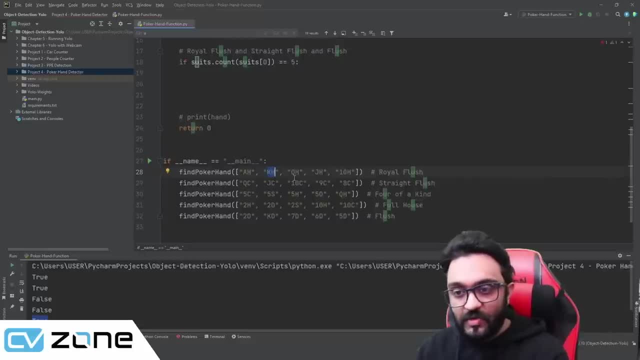 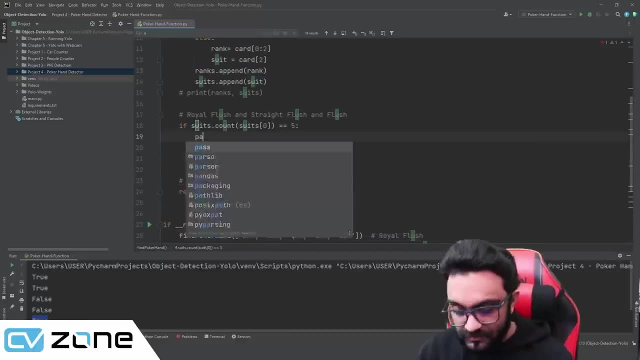 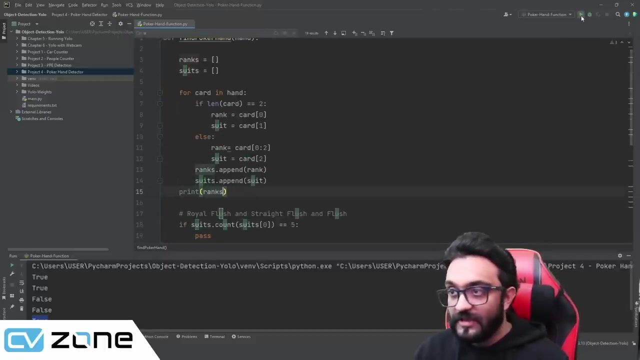 one. the highest rank should be the first, but a king queen does not have a rank yet, because if we print it out, if we print out the ranks, uh, let's just write pass here. if we print out the ranks, it will not give us for a king and queen, it's simply writing a king, queen, jack, which is which is wrong in our case, because 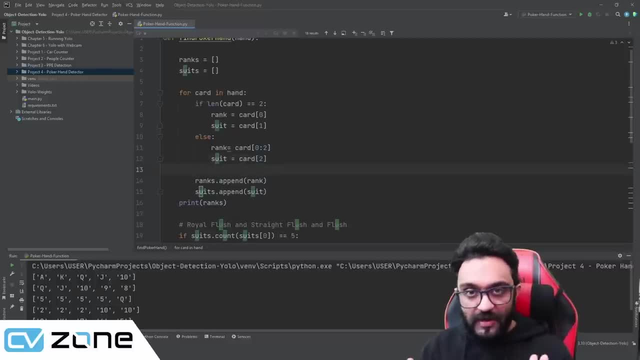 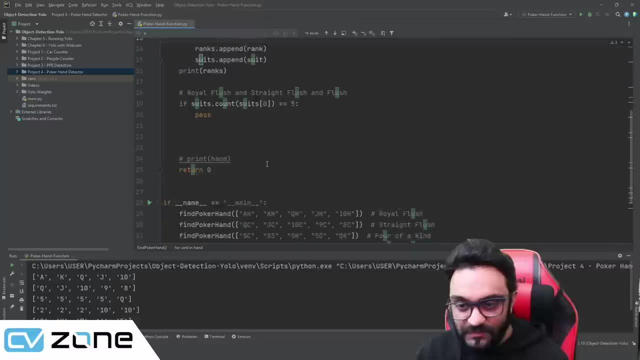 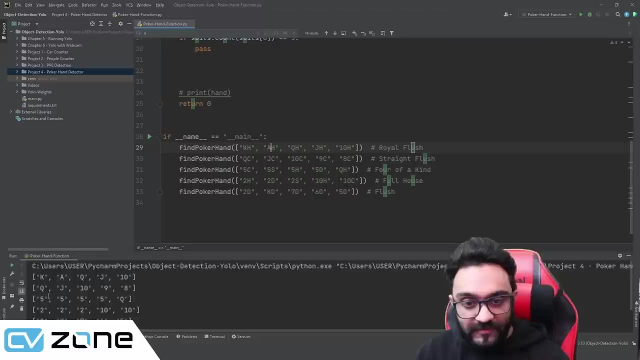 uh, we need to work with values. uh, when we sort them out, we want uh 14 to be a instead of just writing a. otherwise it will not be organized, because if i put, if i remove a here and i put a here, then it will give us k first and a second, which is still a royal flush, but it's not in sequence. so we 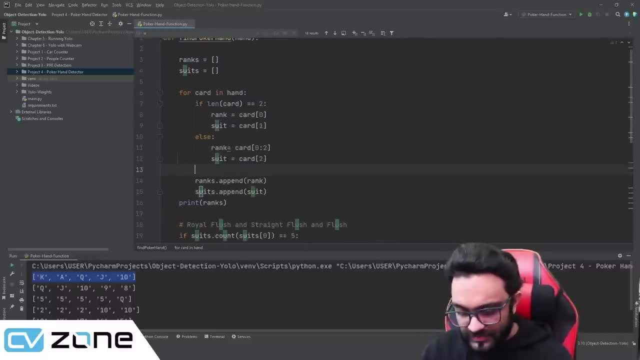 are not able to get the rank properly. so what we'll do here, we'll simply write: if rank equals a, then rank rank equals 14.. uh, that's how simple it is. so else, if rank equals king, we'll copy that, paste and paste. okay. so rank is a, drank will be 14. rank is k, it will be 13.. rank is q. 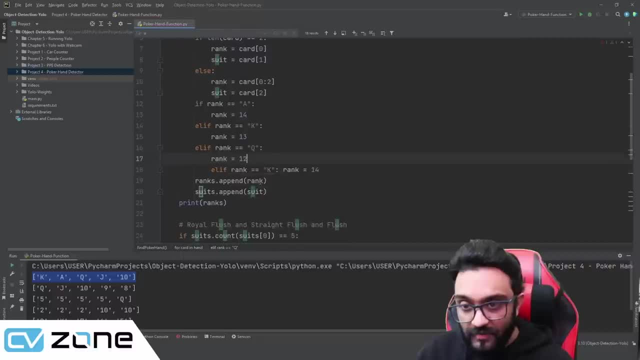 it will be 12. rank is jack, it will be 11.. there we go. so now, if we run it, we will have numbers. so 13, 14, 12, 11, 10.. now what we need to make sure is that they are sorted properly. if they are sorted properly, then it will be easier. 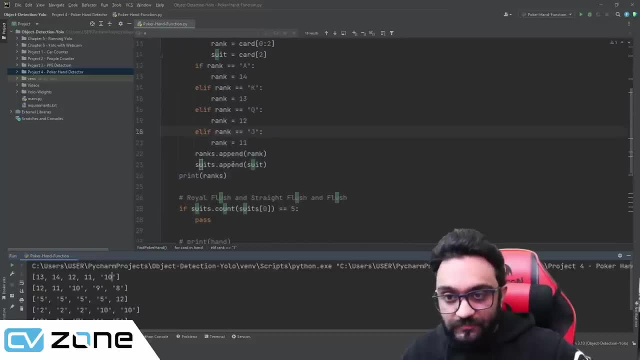 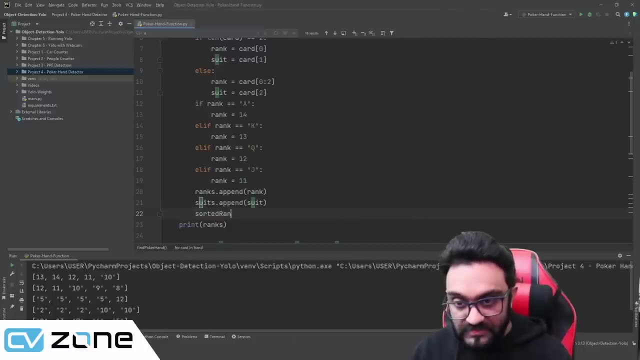 is that they are sort appropriate. if they are sorted proper, then it will be easier for us to uh check for royal flush. so what we can do is, since we all know that there are numbers here, so that we can simply write sorted, so sorted ranks. actually, we will do it after the sorted ranks. 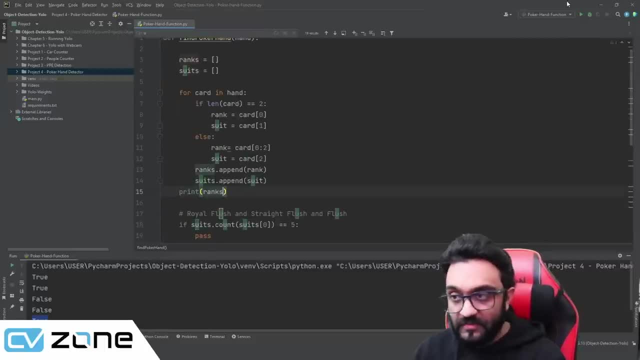 it will not give us for a king and queen. it it's simply writing a king, queen, jack, which is which is wrong in our case, because we need to work with values when we sort them out. we want 14 to be a instead of just writing a. 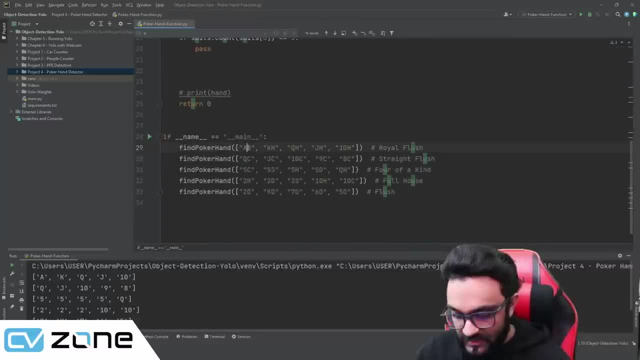 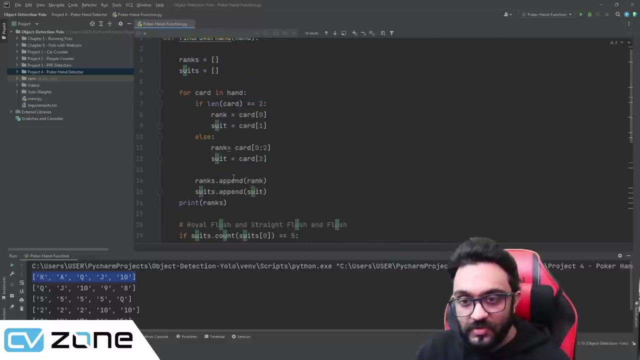 otherwise it will not be organized. because if i put, if i remove a here and i put a here, then it will get a us k first and a second, which is still a royal flush, but it's not in sequence. so we are not able to get the rank properly. so what we'll do here, we'll simply write if rank equals a. 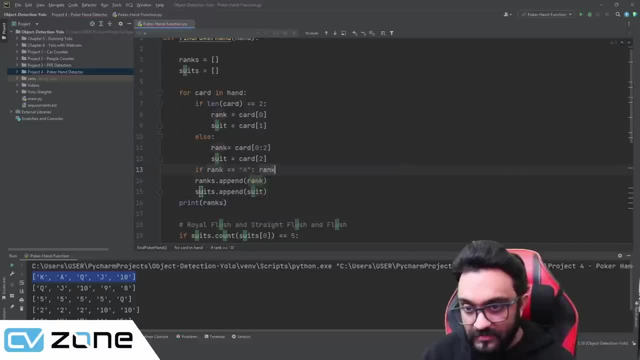 then rank. rank equals 14.. that's how simple it is. so else, if rank equals king, we'll copy that, paste and paste. okay. so rank is a drank, it will be 14. rank is k, it will be 13. rank is q, it will be 12. 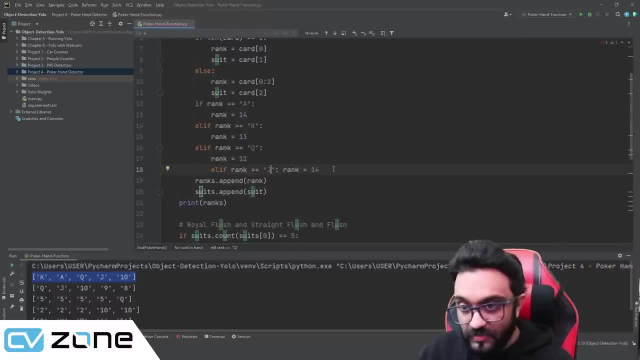 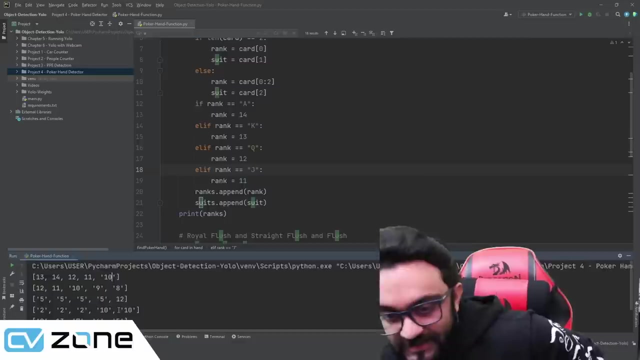 rank is jack, it will be 11.. so that's the way we're going to run it. then, if rank equals k, we'll take an antony rank свое rank over there. there you go. so now, if we run it, we will have numbers. so 13, 14, 12, 11, 10. now what we need to make sure is that they are sorted properly. 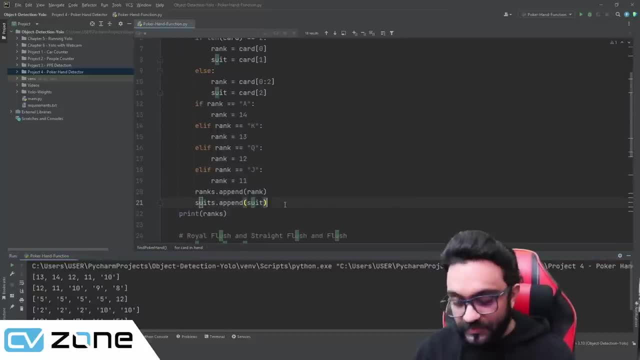 if they're sorted properly, then it will be easier for us to check for royal flush. so what we can do is we can simply write sorted, so sorted ranks will do it after the sortedRanks equals sorted and we will give in our ranks. That's it. 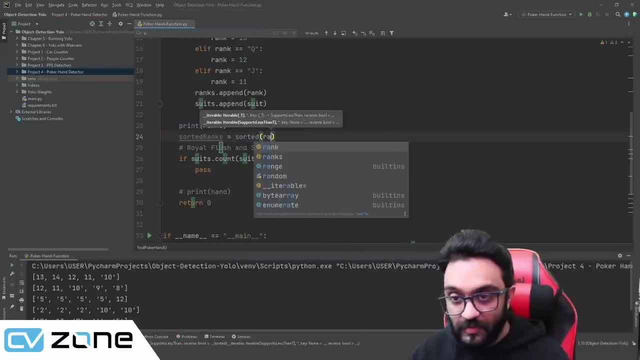 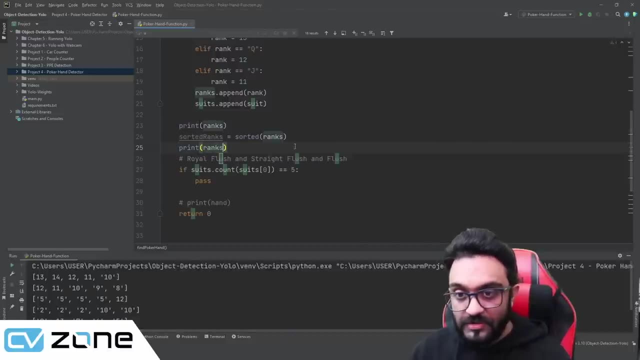 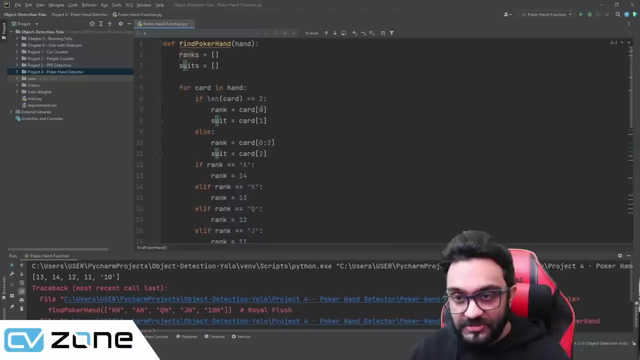 equals sorted and we will give in our ranks. that's it. so if we print ranks again, you will see that now it will be sorted. okay, so ranks, when we are sending them in, uh, they are not integers, they are, um, they are strings. so we need to convert it into integers. there you go. so now you will see. 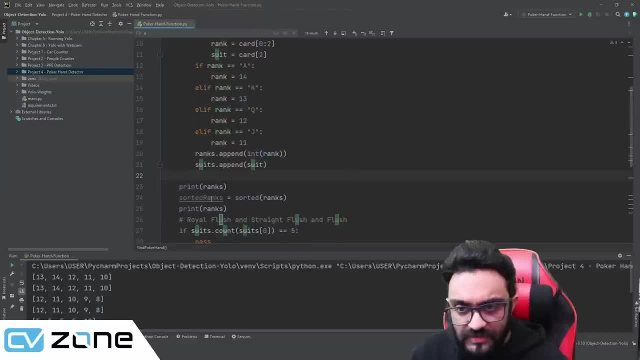 uh, actually it didn't do anything. why is that? oh, because we need to convert it into integers. so we need to convert it into integers- printed ranks, not sorted ranks. okay, let's run that again and you will see. for the first one you will see this one is 13, 14, 12, but now you can see it's 10, 11, 12, 13, 14. so it has sorted it. 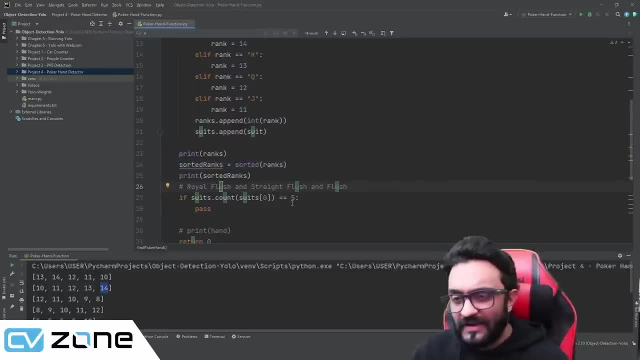 so now what we can do is: um, actually, let's, let's forget about the sorted rank, because, or we can use the sorted ranks, but what we can do is, uh, instead of saying that the first one is 10 and the second one is 11, we can just say: 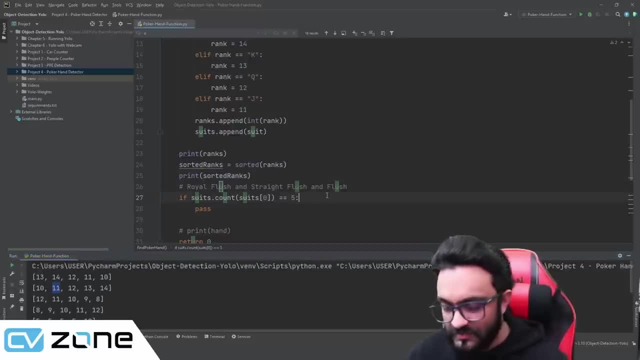 if it's in this uh, that that should work as well. so we can write if uh 14 in sorted ranks, and so that's how you can check if 14 is present in the sorted ranks, and uh, and then we will write another, and then another, and 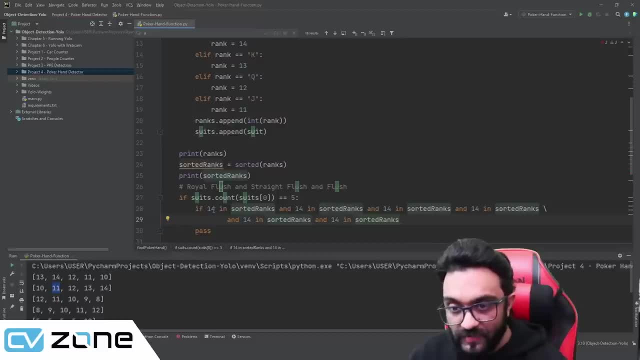 then we will write another and and then another, and so if 14 is there, then 13 is there, then 12 is there, then 11 is there, and then 10 is there. uh, i wrote one extra. if that is the case, then it means it is a royal flush, so we will print royal. 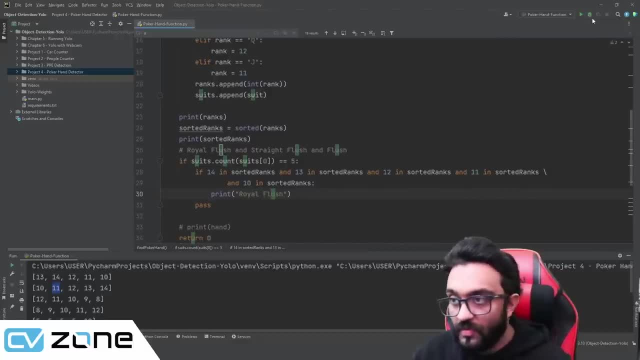 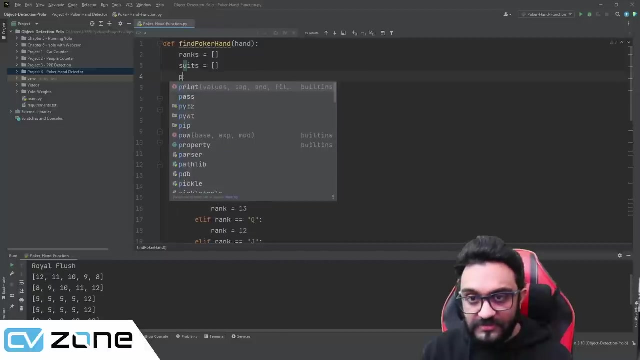 royal flush. so let's run that and there you go. so here you can see, it says royal flush, because this is true for this. the rest of them it's not true. so what we will do is, in order to get the output, we are going to save, uh, the, we are going to create a list called possible. 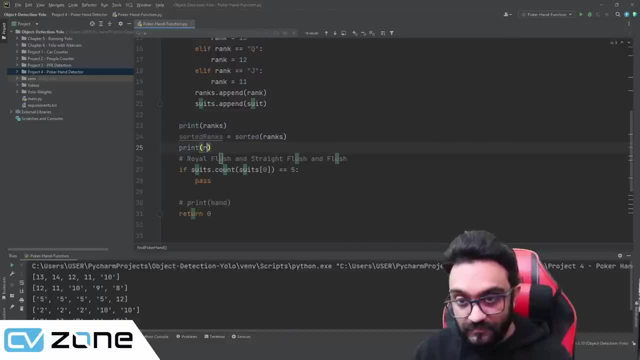 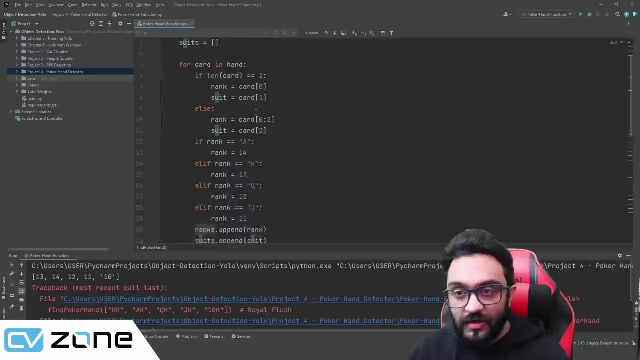 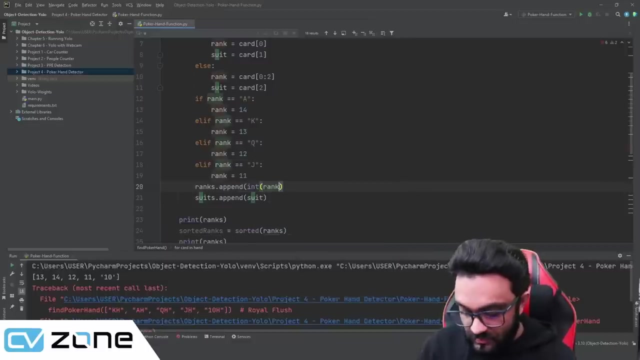 So if we print ranks again, you will see that now it will be sorted. Okay, so ranks, when we are sending them in, they are not integers, they are strings. So we need to convert it into integers. There you go. So now you will see. actually it didn't do anything. Why is? 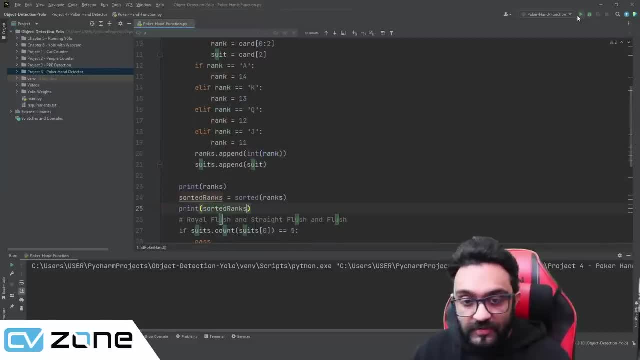 that? Oh, because we printed ranks, not sortedRanks. Okay, let's run that again and you will see. for the first one, you will see this one is 13,, 14,, 12, but now you can see it's. 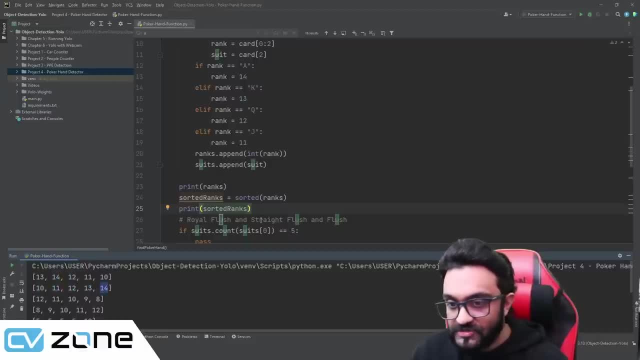 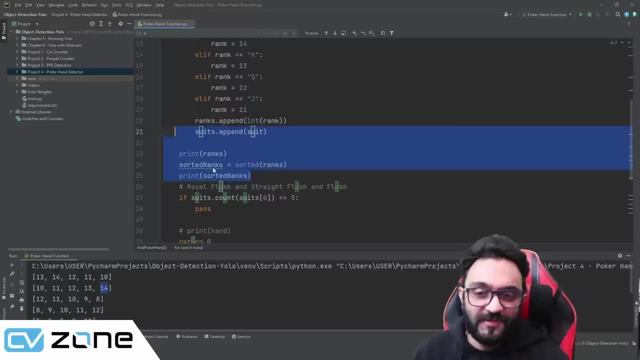 10,, 11,, 12,, 13,, 14.. So it has sorted it. So now what we can do is actually: let's forget about the sortedRank, because what we can use the sortedRanks, but what we can do is instead. 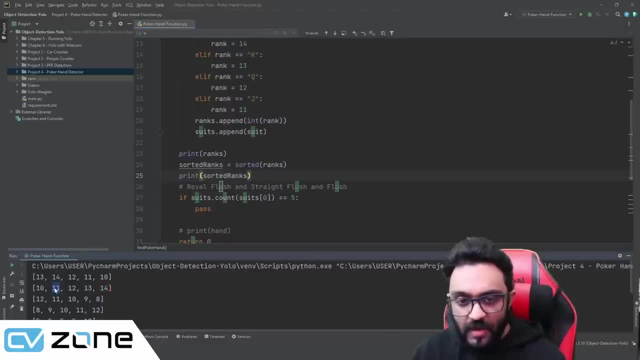 of saying that the first one is 10 and the second one is 11,. we can just say: if it's in this, That should work as well. So we can write: if 14 in 10,, 12,, 13,, 14,, 12,, 13,, 14,. 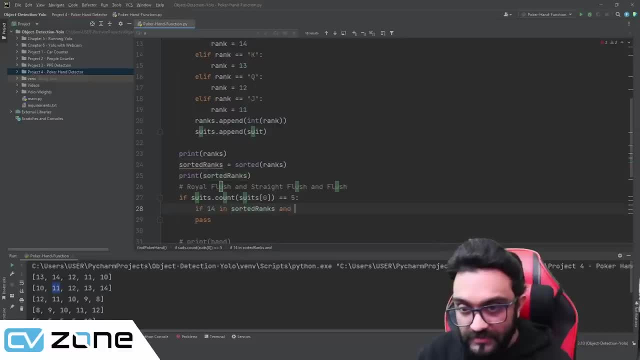 14 in sortedRanks, and so that's how you can check: If 14 is present in the sortedRanks, and then we will write another, and then another, and then we will write another, and and then another, and So if 14 is there, then 13 is there, then 12 is there. 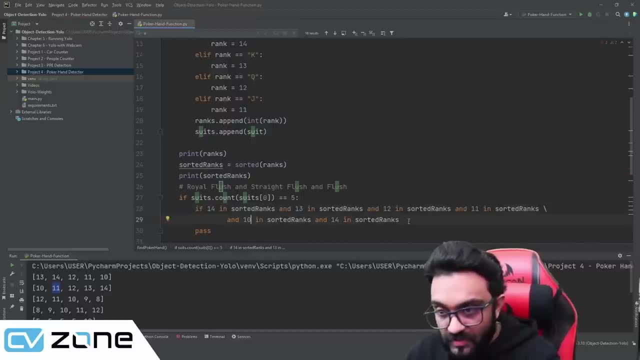 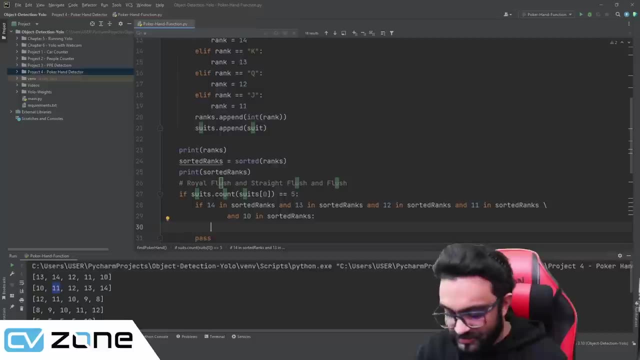 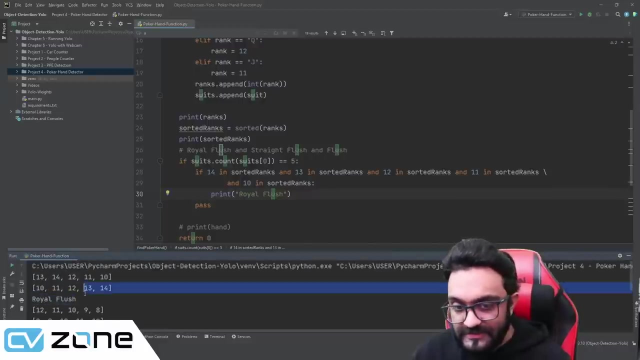 Then 11 is there and then 10 is there. I wrote one extra. If that is the case, then it means it is a Royal flush. So we will print Royal flush. So let's run that, and there you go. So here you can see. it says Royal flush. because this is true for this. The rest of them, you. 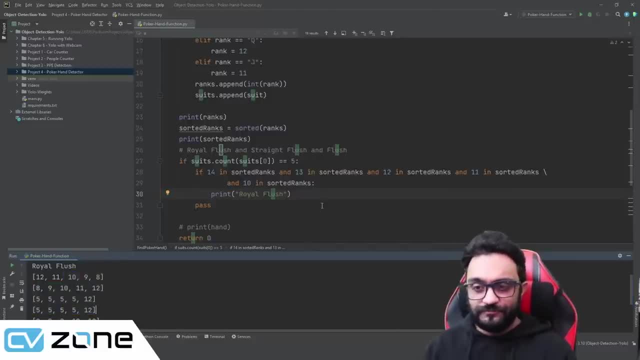 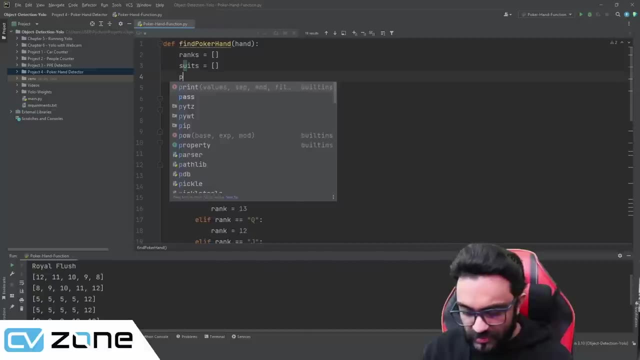 know it's not true. So what we will do is, in order to get the output, we are going to save the. we are going to create a list called possible, possible ranks, And this list will contain all the possible ranks. So if, for example, we are getting a Royal flush, we 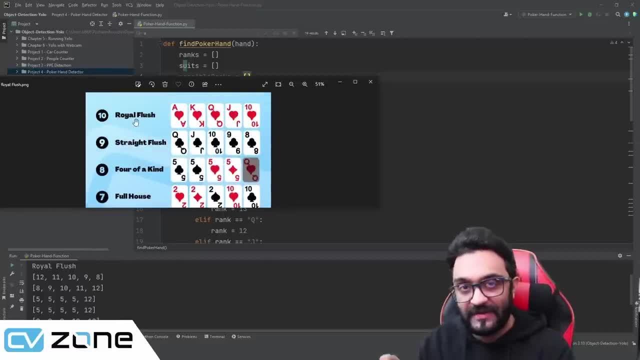 are going to put the value of 10 inside it. We are going to append, Because sometimes what you can have, we can also detect a single pair when it's two pair, right, So we need to find the highest one. So we will put all the possible scenarios. 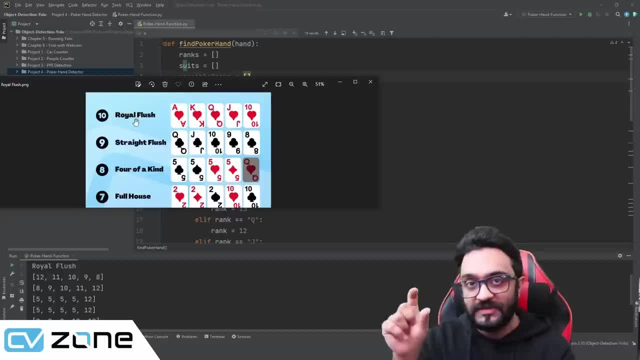 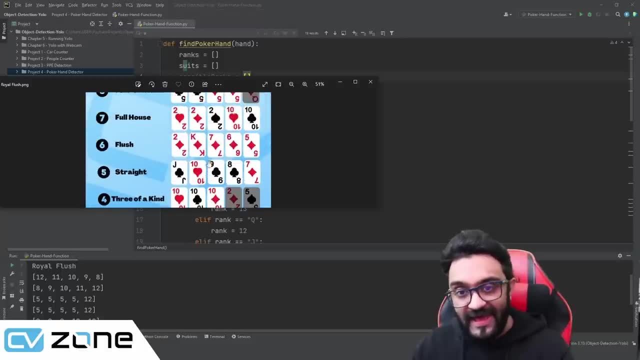 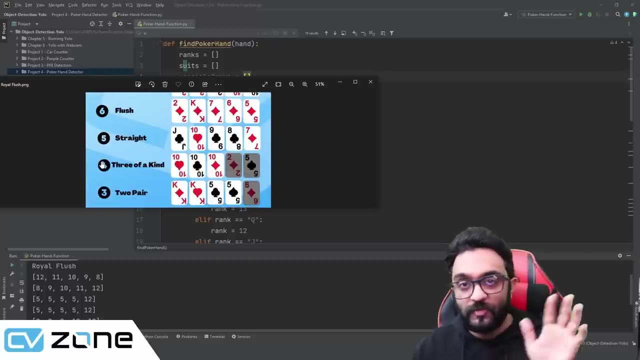 inside this list and we will pick the highest one. So if it was, for example, if it detected that it is a three of a kind and it also detected it is a full house, then for full house it will be seven and for three of a kind it will be four. So we will pick seven. 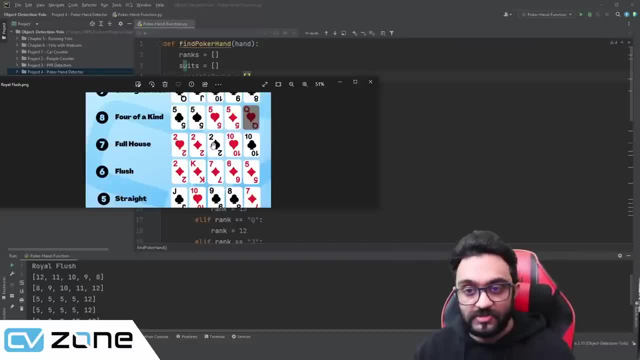 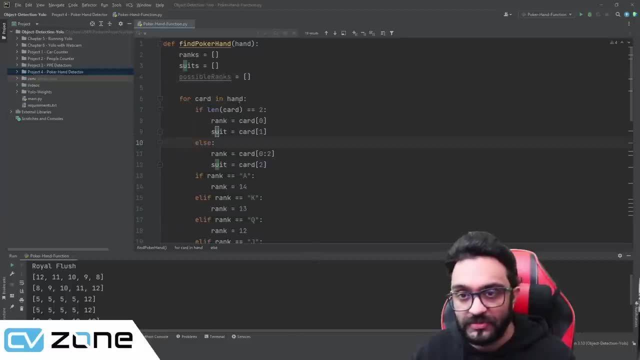 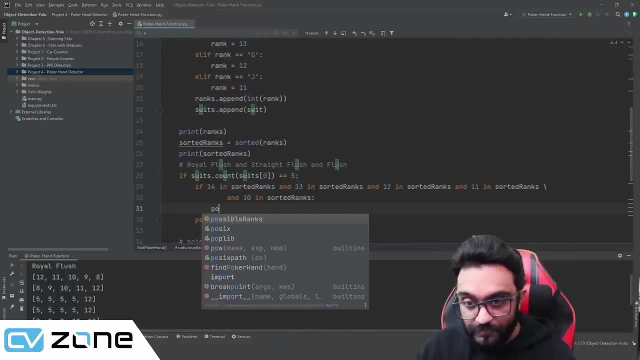 and that will be our highest hand. So that's what we are going to do. So in this case our Royal flush is 10.. So we are going to put inside here we are going to write possible ranks, dot append 10.. 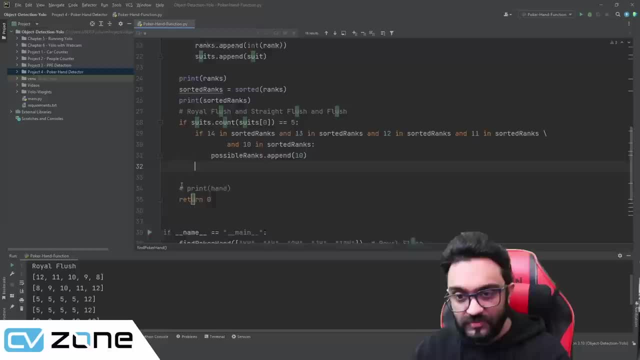 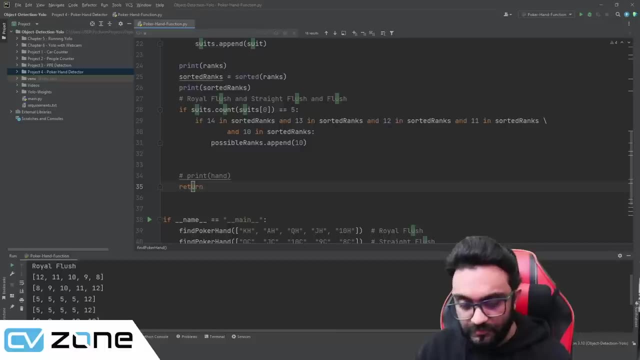 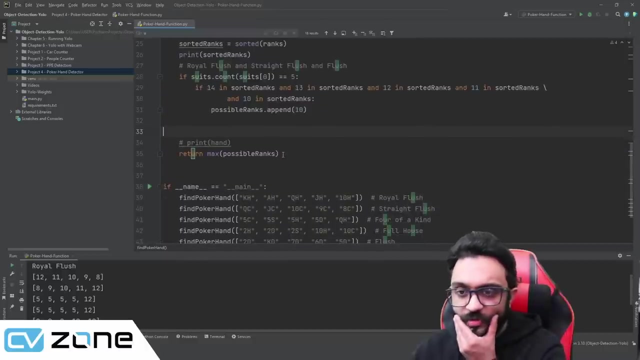 So we are going to append that. And one more thing: once we do that, in the return we are going to return the possible ranks maximum value. so that's the basic idea. um, or should we return? no, that will return only a number. wait, what we can do is we can write the poker: poker and ranks equals. uh, we are going to. 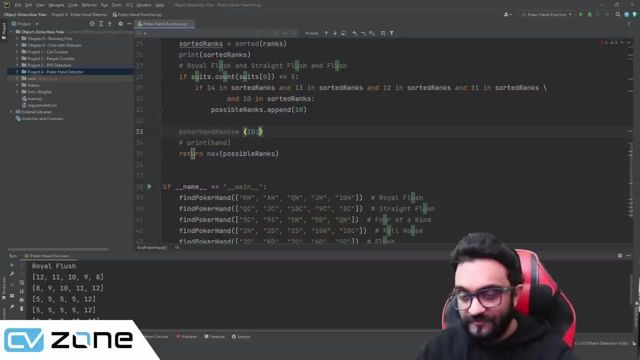 create a dictionary and for each one of them we are going to give a number and a name, so it will be royal lush. then for the second one, for number nine, uh, it will be straight flush, and for number eight will be four of a kind, then for number seven it will be full house. 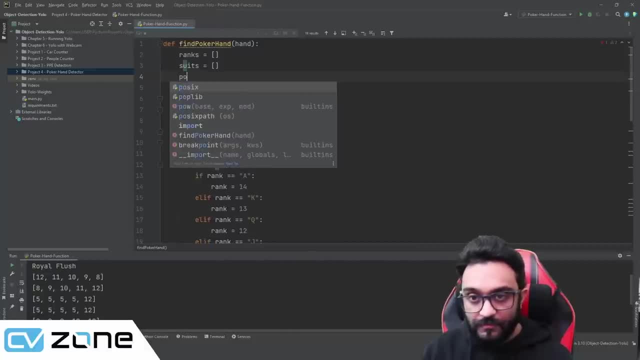 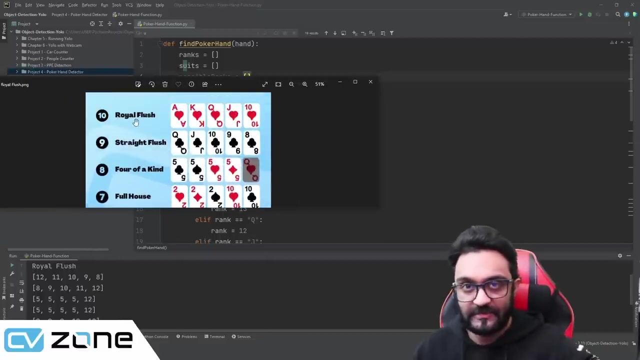 possible ranks, and this list will contain all the possible ranks. so if, for example, we are getting a royal flush, we are going to put the value of 10 inside it, we are going to append, because sometimes what you can have, we can also detect a single pair when it's two pair, right. so we need to find 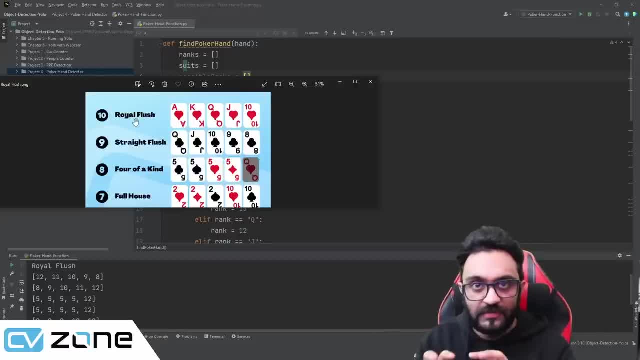 the highest one. so we will put all the possible scenarios inside this list and we will compute 4 in order to query what the actual number is. but in this case, the r fii for these only lists and we will pick the highest one. so if it was, for example, if it detected that it is a three of a, 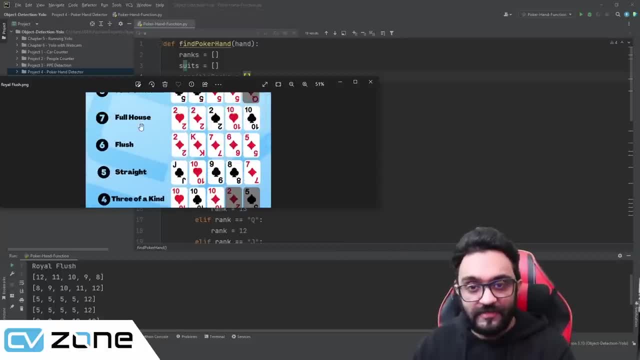 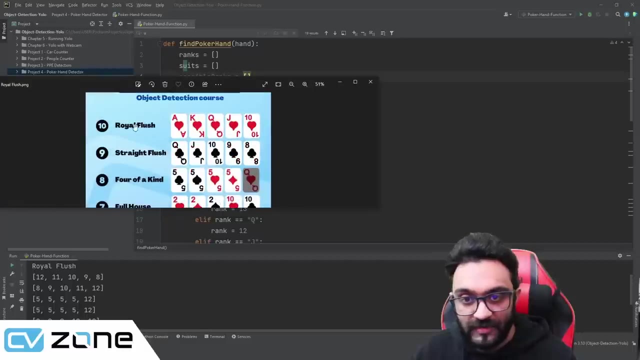 kind and it also detected it is a full house. then for full house it will be seven, and for three of a kind it will be four. so we will pick seven and that will be our highest uh hand. so that's what we are going to do. so in this case our royal flush is 10, so we are going to put um inside here. 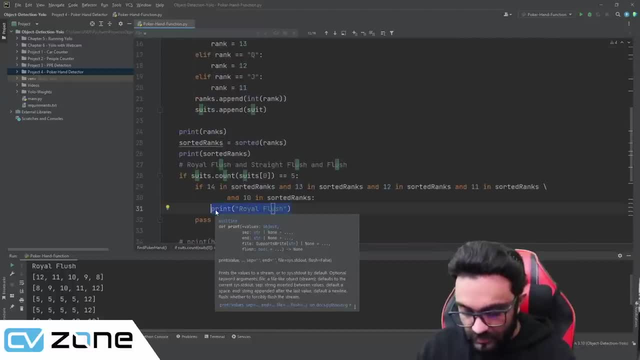 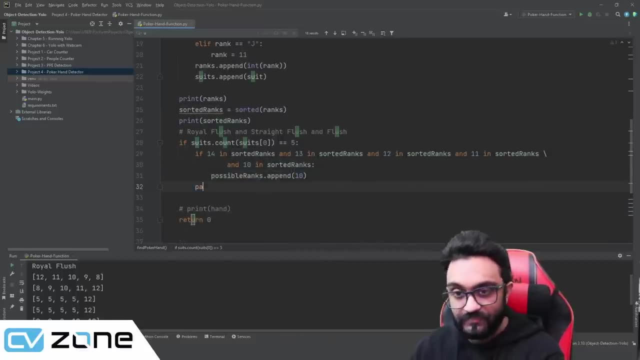 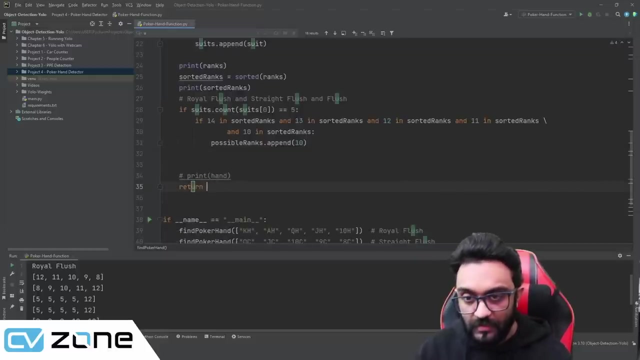 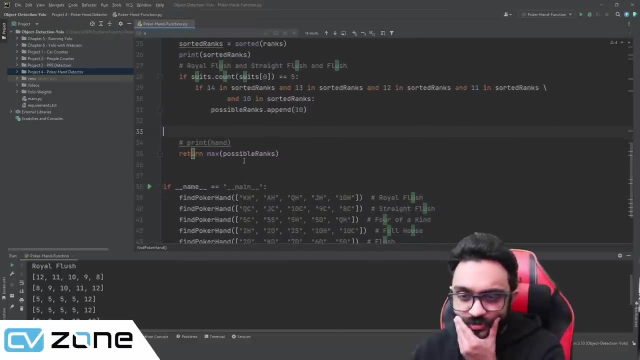 we are going to write uh possible ranks, dot, append 10. so we are going to append that and once we do that, uh, in the return, we are going to return, uh, the possible ranks, maximum value. so that's the basic idea, um, or should we return? no, that will return only a number. 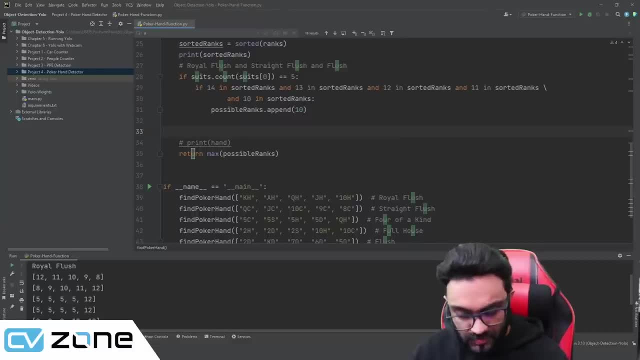 wait, what we can do is we can write the poker: poker and ranks equals. uh, we are going to create a dictionary and we are going to write a dictionary and we are going to write a dictionary and for each one of them, we are going to give a number and a name. so it will be royal. 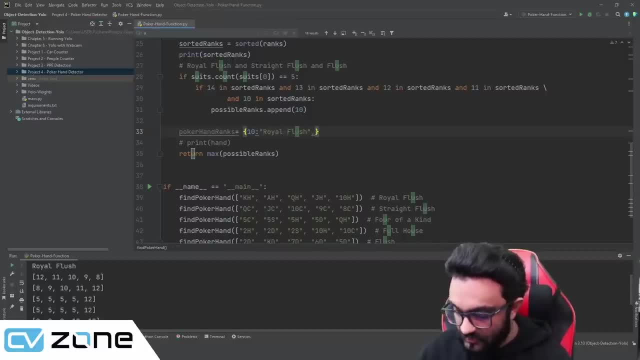 lush, then for the second one, uh. for number nine, uh, it will be straight flush, and for number eight will be four of a kind, then for number seven it will be full house, then for number six it will be flush, then for number five it will be straight. 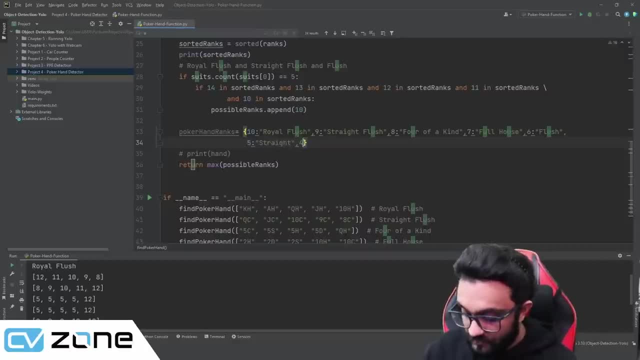 ght. and then for number four, it will be three of a kind. then for number three, it will be two pair pair. for number two, it will be pair. for number one, it will be icon. so these are all our ranks, and now what we can do is we can. 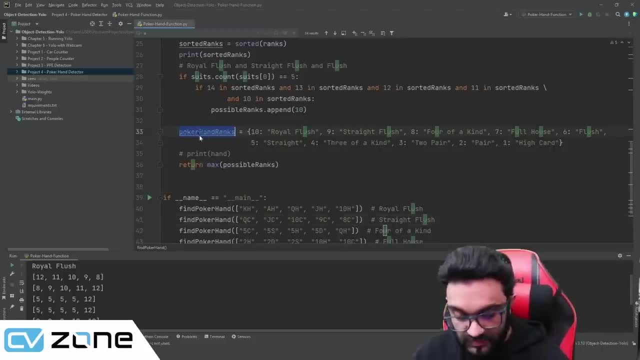 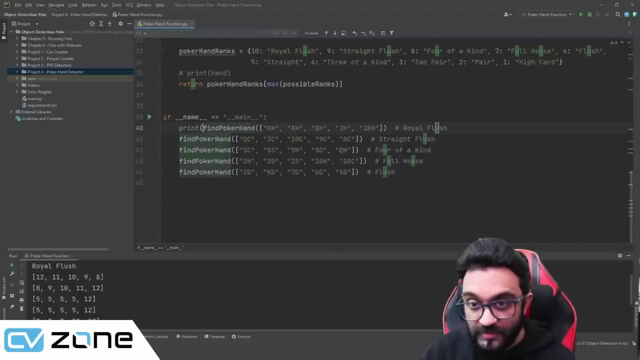 um, check the max possible, and then we can write here: poker ranks at this value, so we will return that and we can simply print that out. so here, for each one of them, we can simply write: print, print, print, print. there we go. so, uh, now let's remove all the prints. 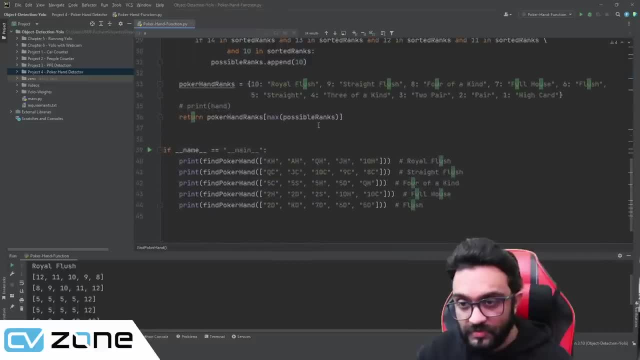 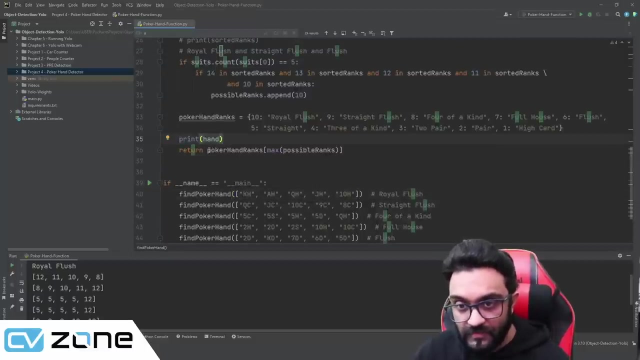 and um. what we will do is: or should we print here? no, let's not print here, let's print it inside, so we'll not have to write it again, again. so we will print that out hand and we will print what it is like. what did it detect? so here, print hand and print this. 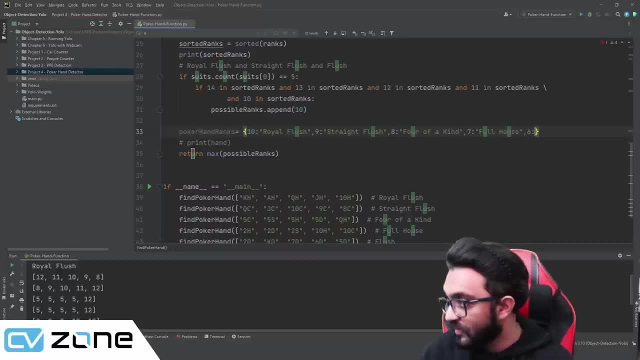 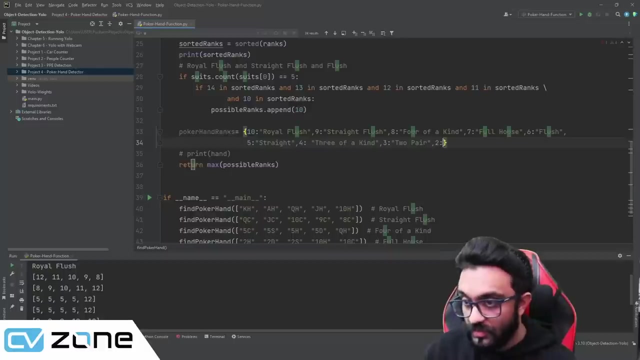 then for number six it will be flush, then for number five it will be straight ght, and then for number four it will be three of a kind, then for number three it will be two pair, pair. for number two it will be pair, for number one it will be: i god. so these are all our ranks, and now what we can do is: we can. 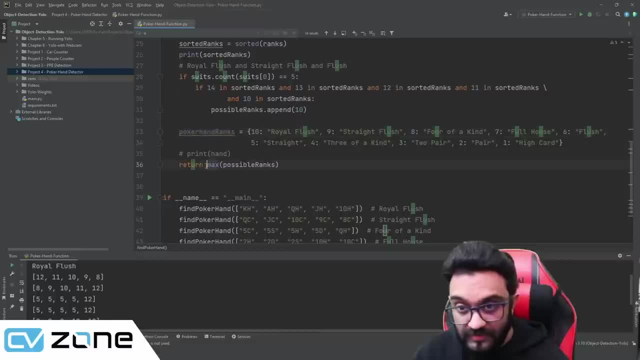 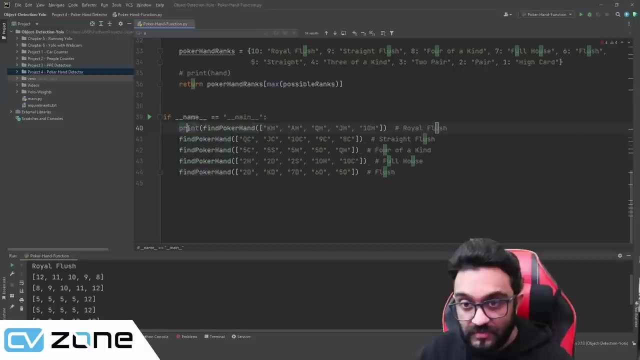 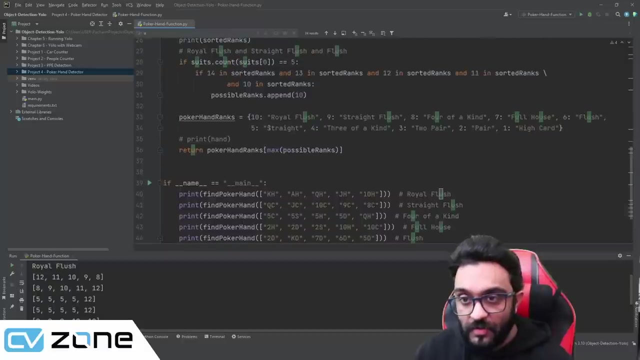 check the max possible and then we can write here: poker ranks at this value, so we will return that and we can simply print that out. so here, for each one of them, we can simply write: print, print, print, print. there you go. so, uh, now let's remove all the prints. 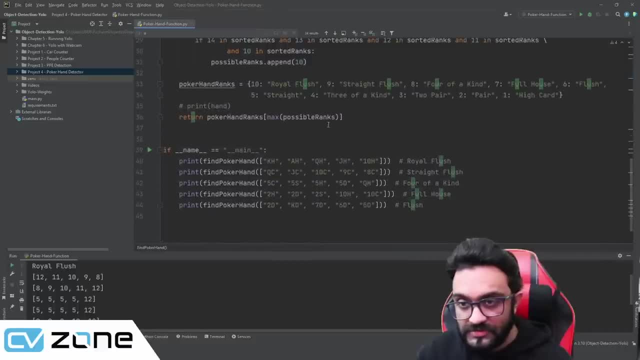 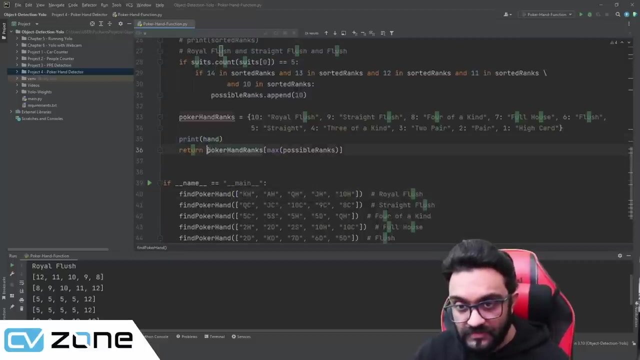 and what we will do is: or should we print here? no, let's not print here, let's print it inside, so we'll not have to write it again, again. so we will print the hand and we will print what it is like. what did it detect? so here, print hand and print this. 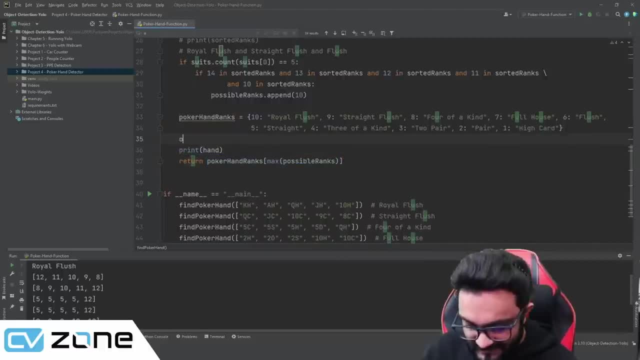 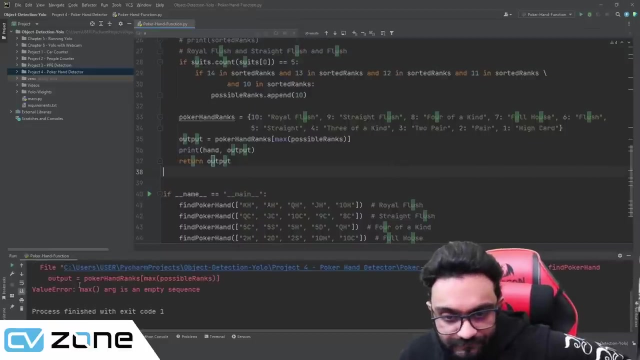 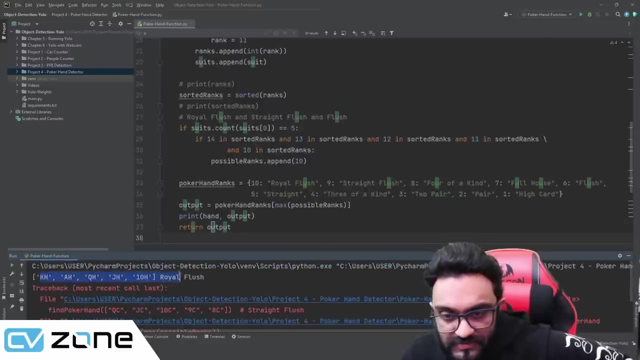 or let's give it: uh, let's, let's call it: output is this, and then print the output and then put the output here, return the output. there you go. so yeah, let's run that and see what we get. max argument is an empty sequence, so the first one you can see it is a royal flush. 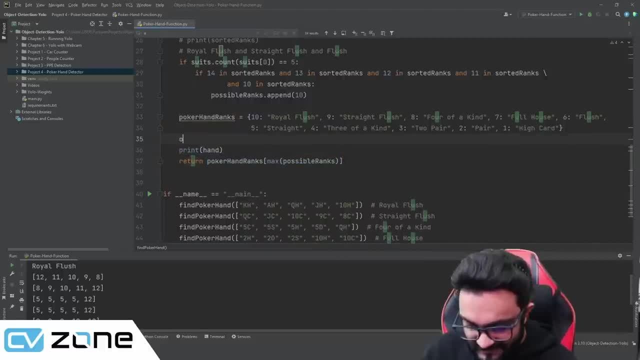 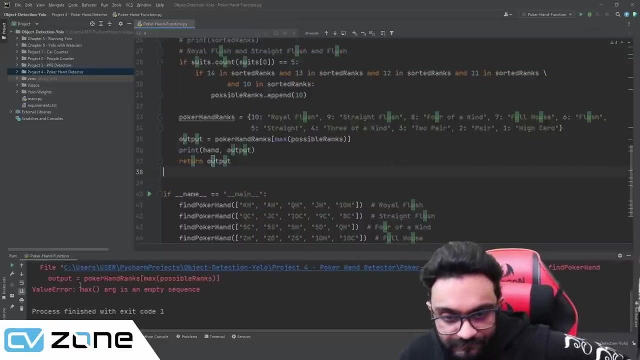 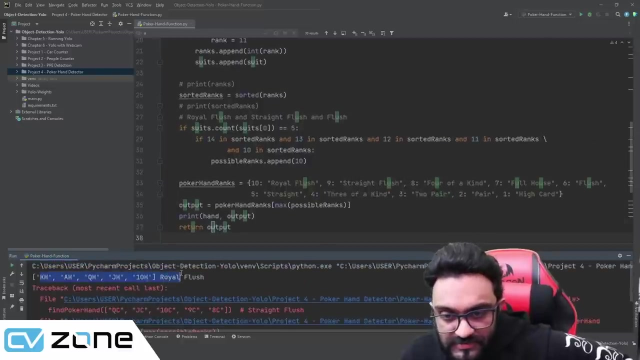 or let's give it: uh, let's, let's call it: output is this, and then print the output and then put the output here, return the output. there you go. so yeah, let's run that and see what we get. max argument is an empty sequence, so the first one you can see it is a royal flush. 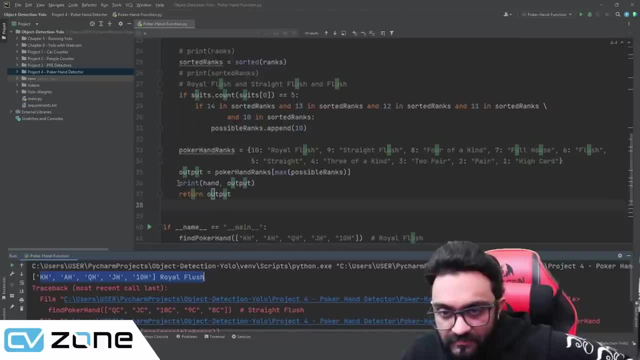 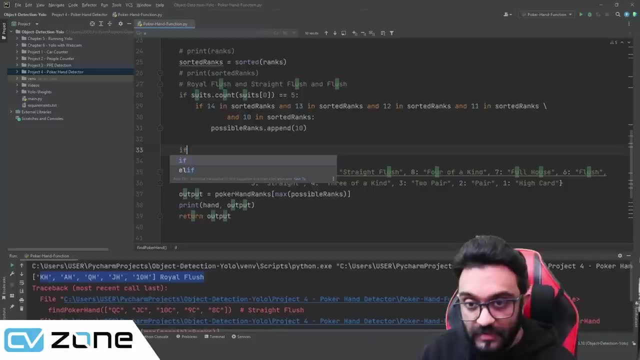 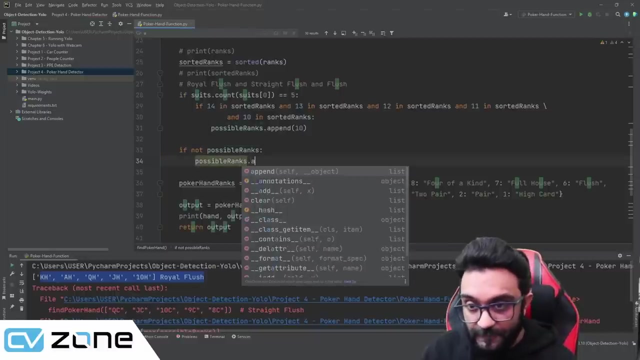 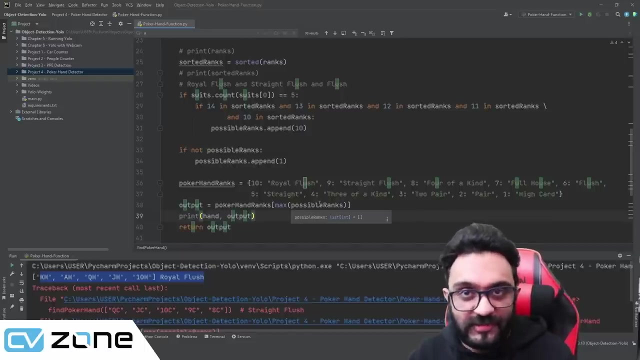 so it is returning that if nothing is there, uh. if if there are no, we can simply write: if uh, not possible ranks. it means if possible ranks is empty, then possible ranks. dot append one. it means it is high card. right. if we have not actually coded for the flush or the straight or full house, for now it will just say, uh, high card. 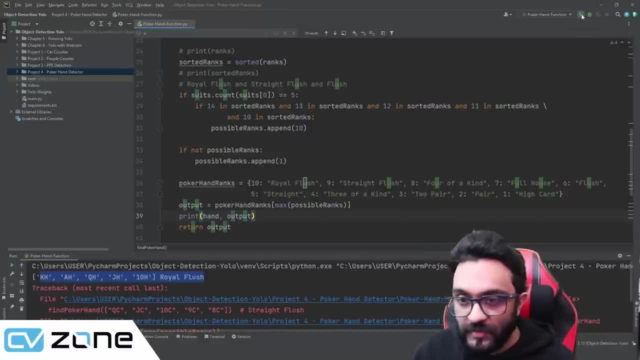 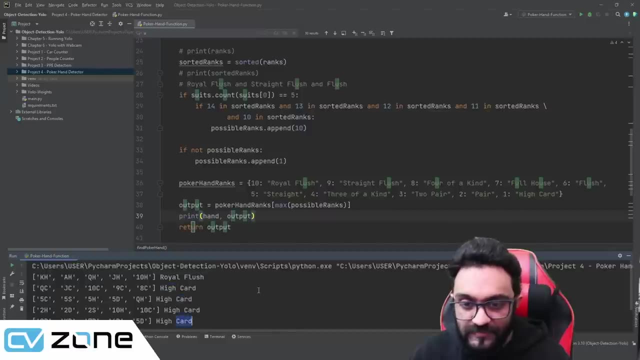 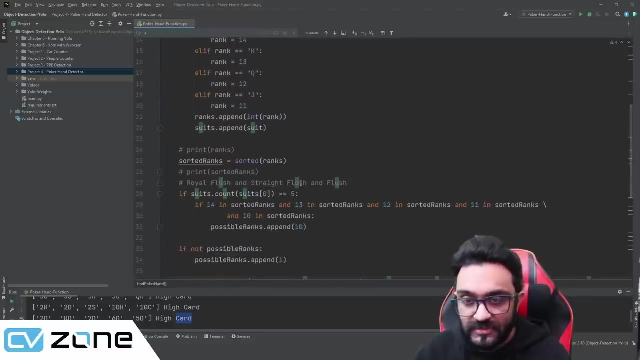 so as we go along and we keep adding, uh, it will keep fixing. so for now, you can see, it says royal flush for the first one, for the second, third, fourth and fifth it says high card. so for now we are heading in the right direction, we are getting a good output, we can see the results. 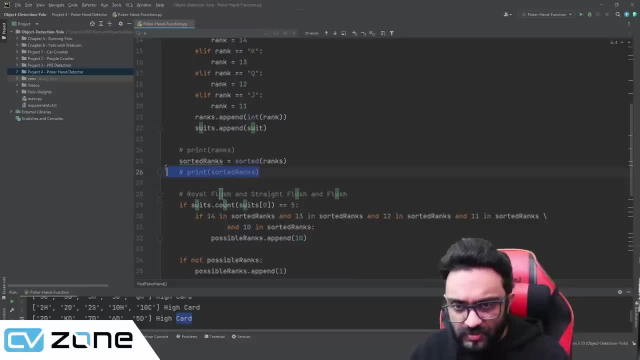 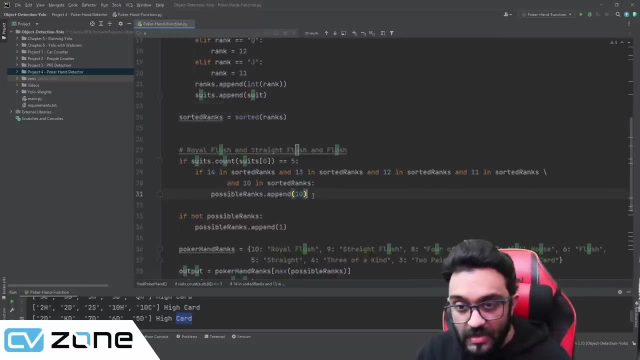 and here we are checking for this: sorted ranks. let's keep it for now. maybe we will need it later, but actually we don't really need it for now. so once we check that, if this is the case, uh, the second one we are going to check is for straight flush. so if we know how to check for 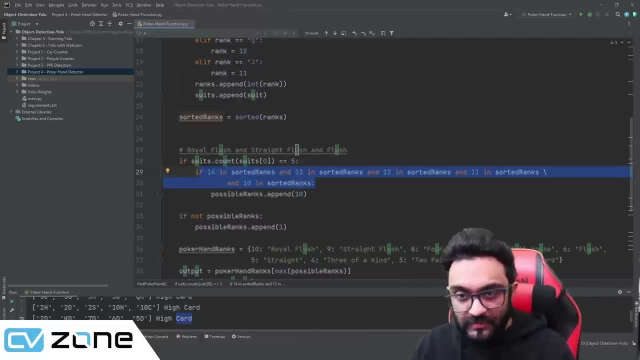 straight. we can. uh, if we are going to check for this, then it will show us that we can get an output. can just put the straight code inside this if statement and it will become straight flush because this statement is checking for flush, because if we write here else else possible dot. 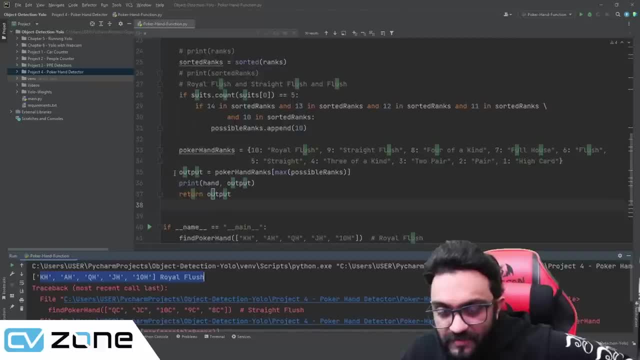 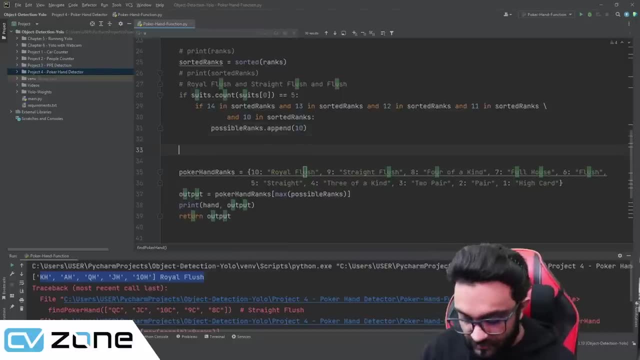 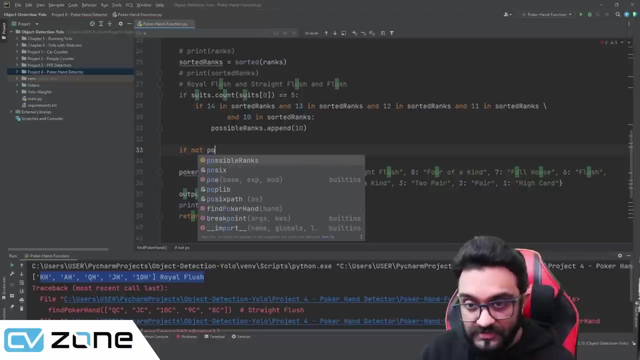 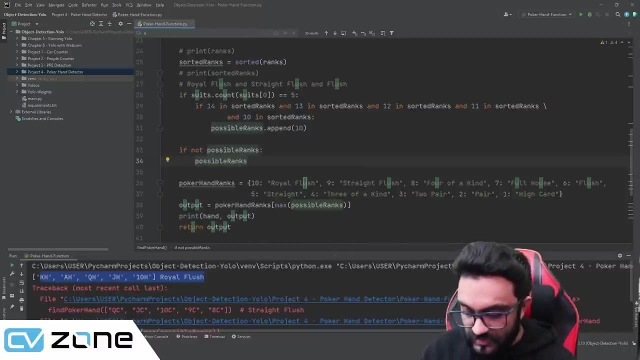 so it is returning that if nothing is there, uh. if if there are no, we can simply write: if, uh, not possible ranks. it means if possible ranks is empty, then possible ranks. dot append one. it means it is high card right. if we have not actually coded for the flush or the straight or full house, for now it will just 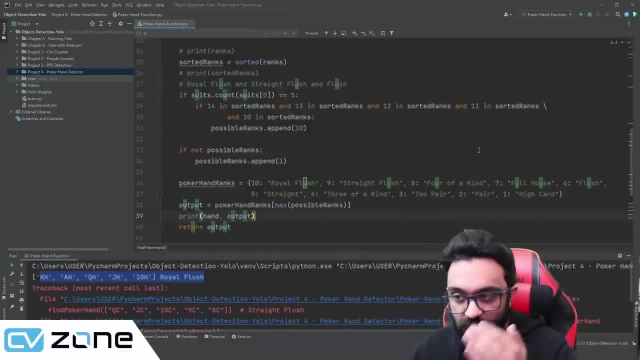 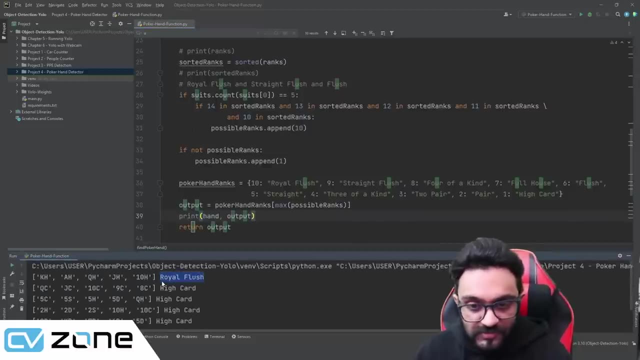 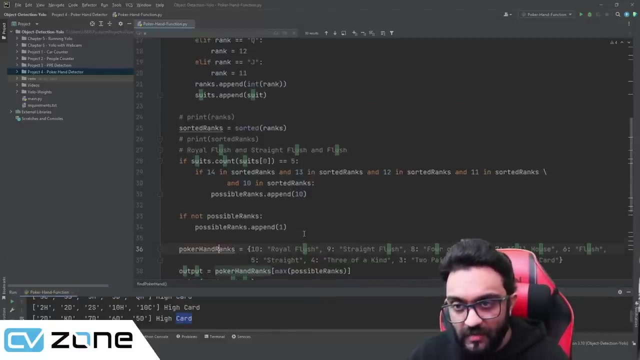 say, uh, high card. so as we go along and we keep adding, uh, it will keep fixing. so for now you can see, it says royal flush for the first one. for the second, third, fourth and fifth it says high card. so now we are heading in the right direction, we are getting a good output. 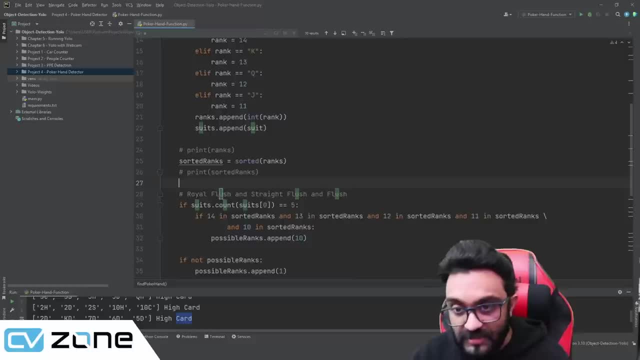 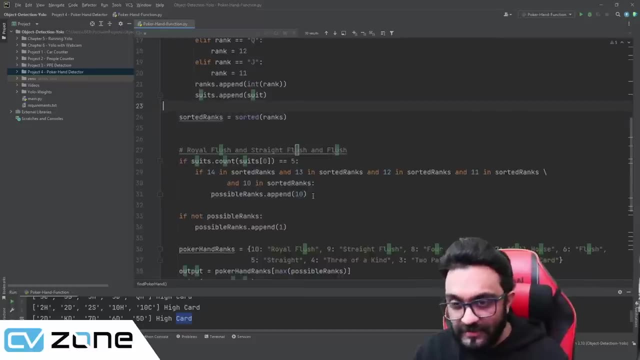 we can see the results and here we are watching the final input. so we are checking and we are also checking for: uh, this sorted ranks. let's keep it for now. maybe we will need it later, but actually we don't really need it for now. so once we check that, if this is the case, the second one we are going to. 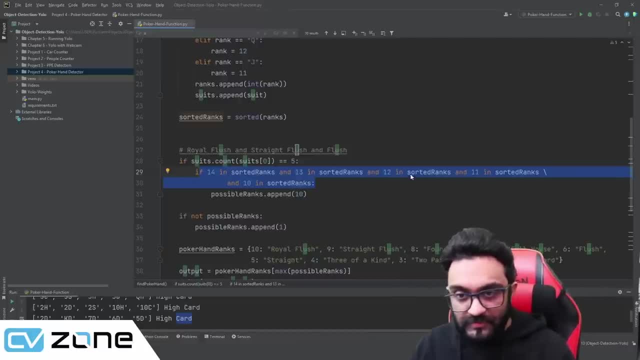 check is for straight flush. so if we know how to check for straight, we can just put the straight code inside this if statement and it will become straight flush, because this statement is checking for flush. so this is the first time we will be checking for flush. okay, so as you can see, it is. 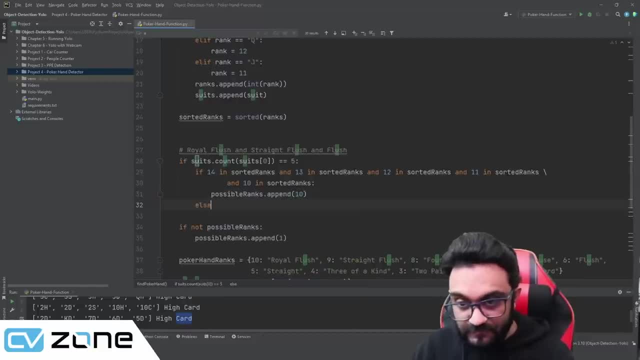 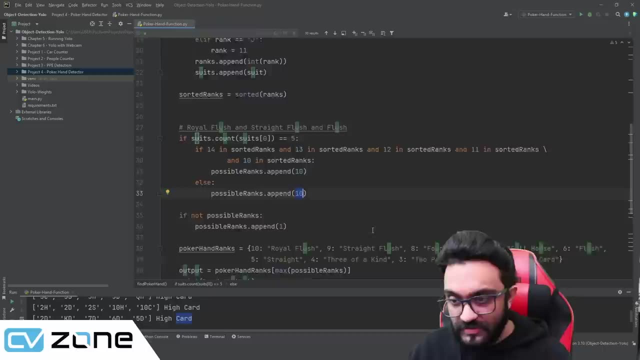 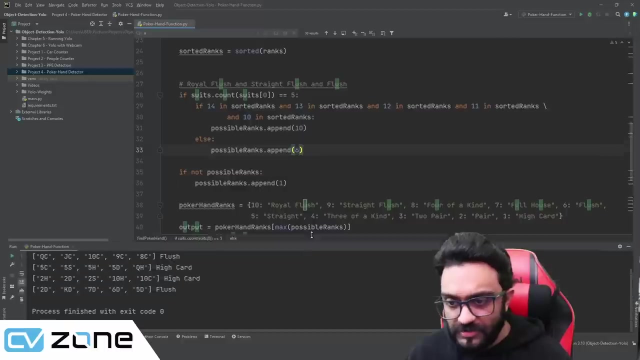 having a very valid first thing, and it's not going to be necessary to just go ahead and make this for flush, because if we write here else else possible dot append is: uh, what is flush? flush is number six. so we'll put here six and if we run this now, you will see that this one is detected as 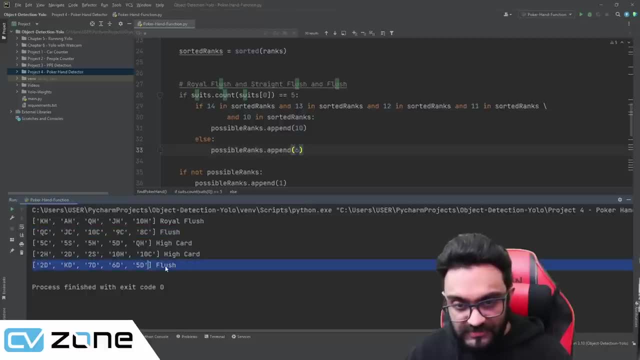 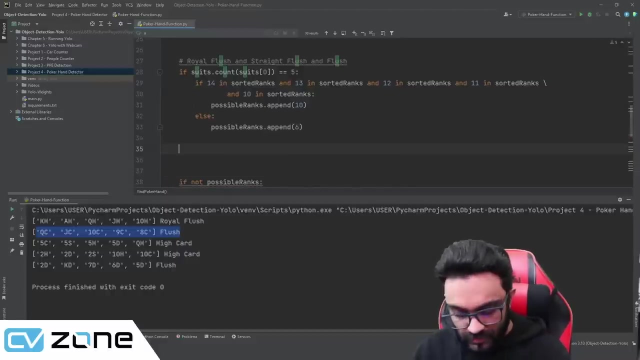 a flush and this one is detected as a flush, so this one is correct, it's a flush, but this one is a straight flush, so we need to fix that. we need to add another if statement here to check for straight. how do you check for straight? let's do that first. so here we are going to write straight. 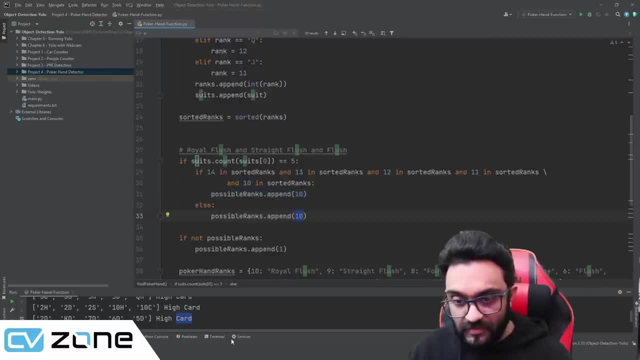 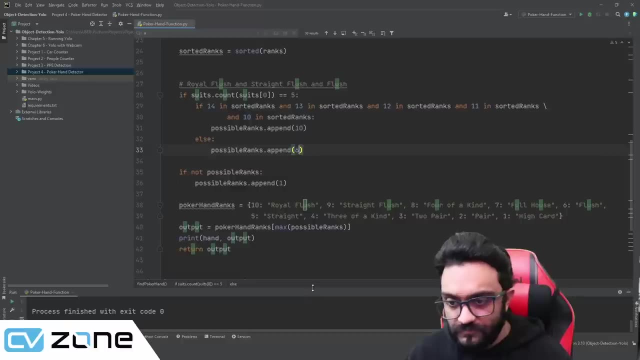 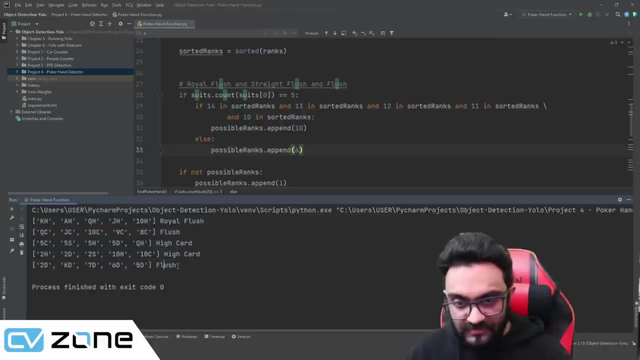 append is: uh, what is flush? flush is number six, so we'll put here six and if we run this now, you will see that this one is detected as a flush and this one is detected as a flush. so this one is correct, it's a flush, but this one is a straight flush. so we need to fix that. we need to add: 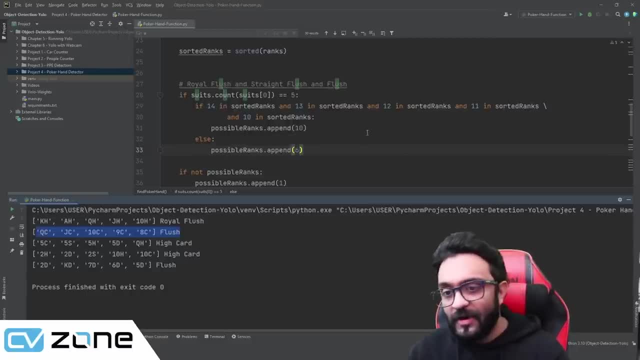 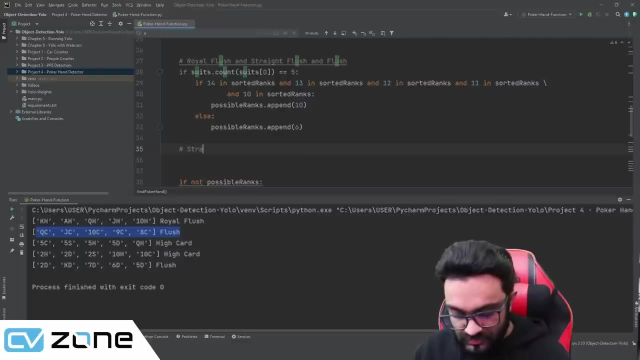 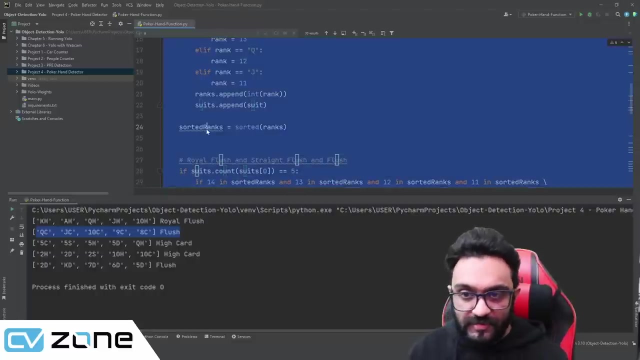 another if statement here: to check for straight: how do you check for straight? let's do that first. so here we are going to write straight. okay, so what happens is, in order to check for straight now, we need the sorted ranks. So, for example, we will have in the sorted ranks, we will have, let's 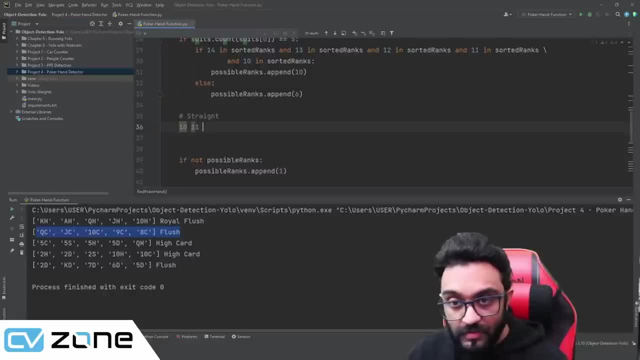 say 10,, 11,, 12,, 13,, 14.. So this is our sorted ranks. So what can we do? We can take the first element, or we can take this element and we can say: check the element before this. 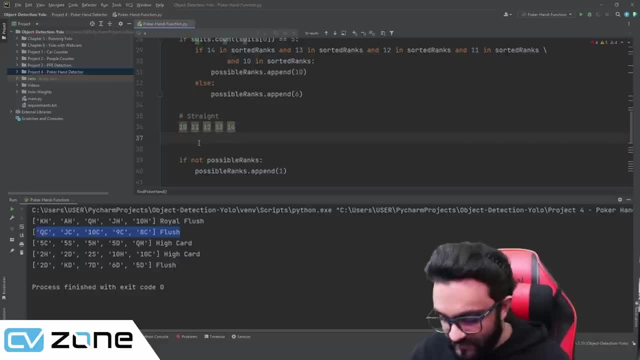 and add one to it. So right now we are talking about 11.. We will take 11 and then we will take the element before this, which will be 10, and we will write here 10 and we will say that: add one to that element plus one and check if they both are equal. So then it will. 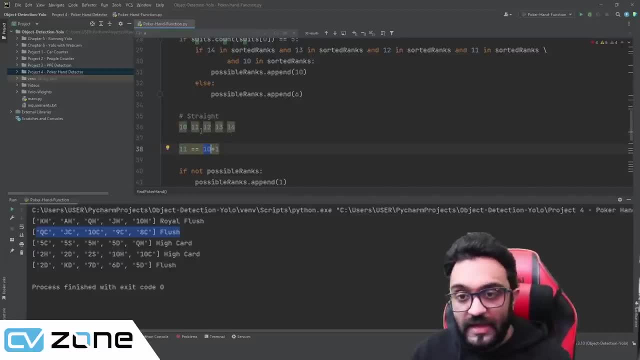 become 11 equals 11.. So that is true. Then it will go to the next element, So it will go to 12.. Then it will check the one before it. It will be 11.. So it will write 11 and it will add plus one. So it will check if 11 plus one is 12.. If 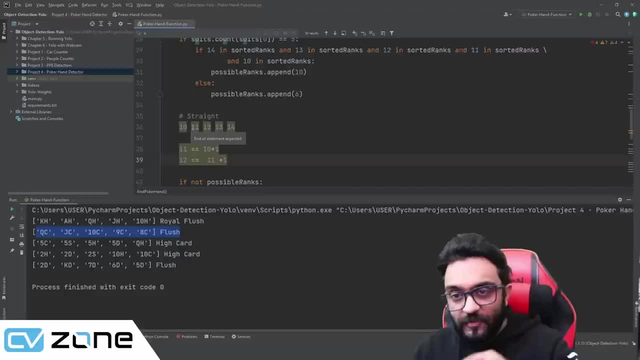 that is true, it will become true. So we will keep checking for all of them. So if all of them give us true, true, true, true, true, true, true, then we will say, okay, it's a straight If even one of them gives us something else. for example, this one is: let's say: 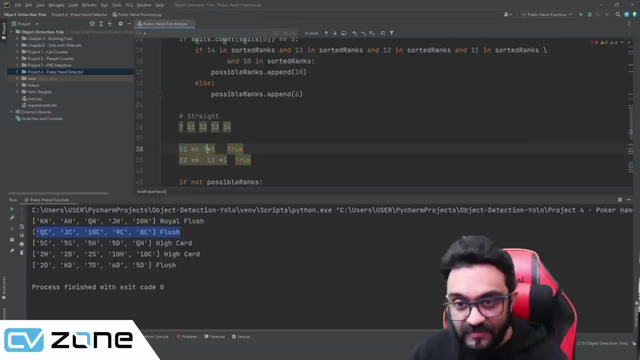 11.. So we write here 11 and it checks: seven plus one is eight. This one is false, but the rest of them are true. Then it's not a straight. So that's how we will check it. So to do that, we are going to write some efficient code. So we are going to write for. 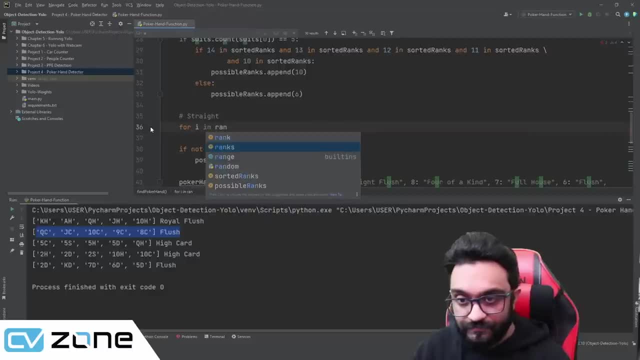 I in range. So we are basically looping, uh, and we need to loop through one because we are starting off. uh, let me put it back, because we are starting off with this value, not this value. We will pick this value and add one to it. Uh, sorry, add one to the previous one, because 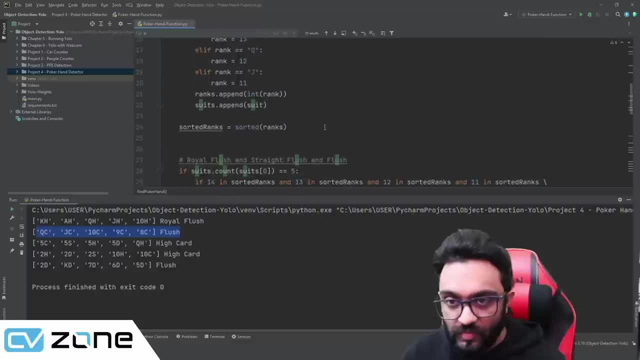 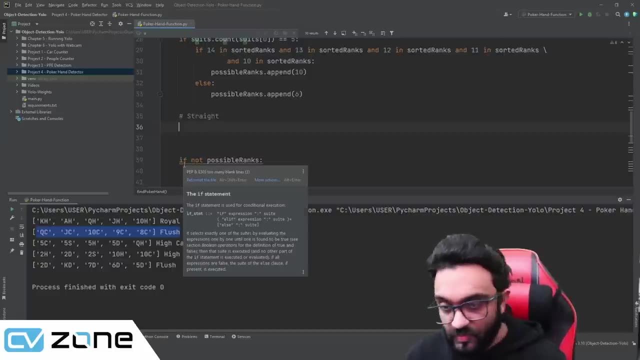 okay. so what happens is, in order to check for straight now, we need the sorted ranks. so, for example, we will have in the sorted ranks we will have, let's say, 10, 11, 12, 13, 40. so this is our sorted ranks. so what can we do? we can take the first element. 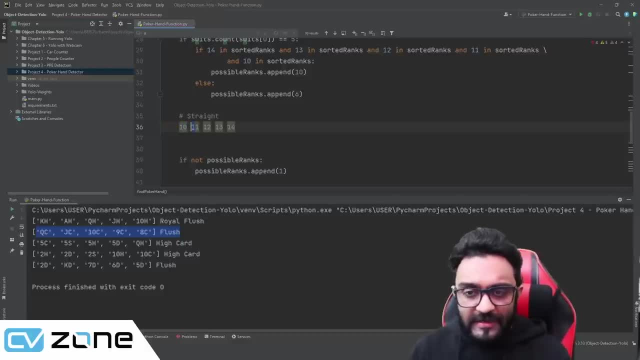 or we can take this element and we can say: check the element before this and add 1 to it. so right now we are talking about 11, we will take 11 and then we will take the element before this, which will be 10, and we will write here 10 and we will say that add. 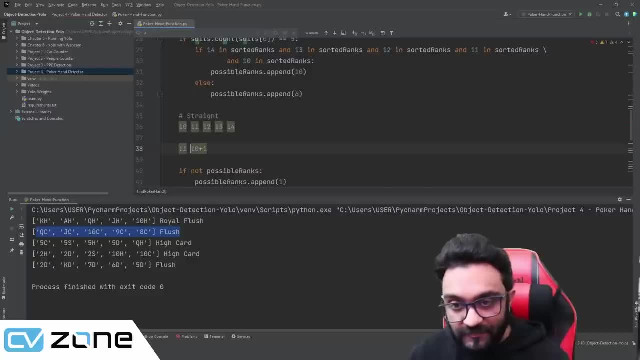 to that element plus 1 and check if they both are equal. so then it will become 11 equals 11. so that is true, then it will go to the next element, so it will go to 12. then it will check the one before it. it will be 11, so it will write 11 and it will add plus 1. so it will check if 11. 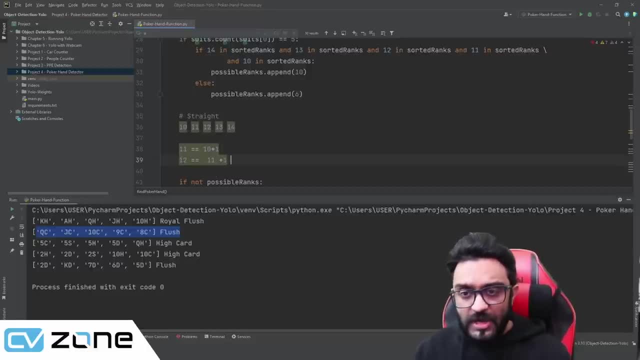 plus 1 is 12. if that is true, it will become true. so we will keep checking for all of them. so if all of them give us true, true, true, true, true, true, true, then we will say: okay, it's a straight. if even one of them gives us something else, for example, uh, this one is, let's say, 7.. so we write here: 11. 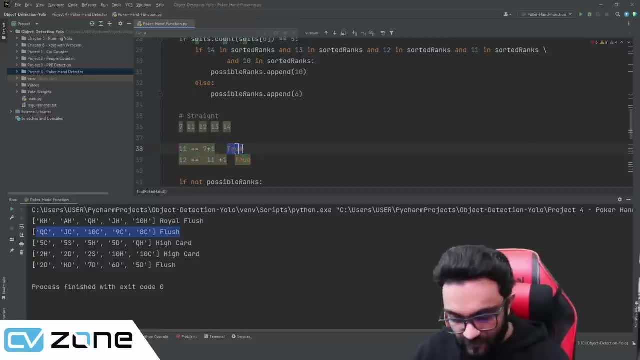 and it checks: 7 plus 1 is 8. this one is false, but the rest of them are true. then it's not a straight. so that's how we will check it. so do that. we are going to write some efficient code. so we are going to write for i in range. 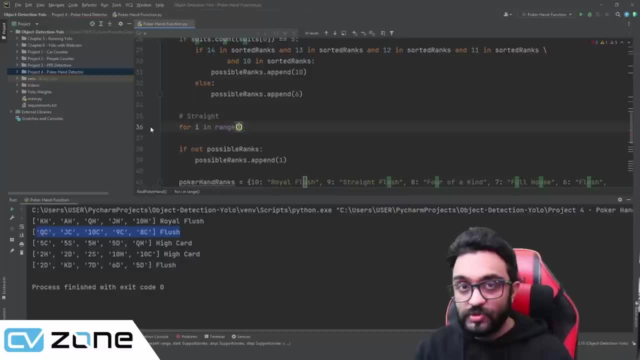 so we are basically looping, uh, and we need to loop through one because we are starting off. uh, let me put it back, because we are starting off with this value, not this value. we will pick this value and add one to it. sorry, add one to the previous one, because this value does not have a previous value. 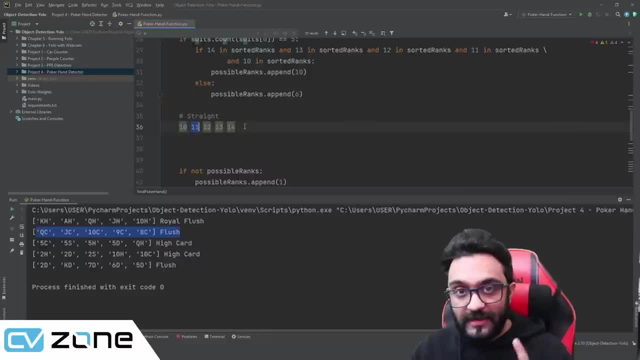 this value does not have a previous value, So we will start from one and not zero. So here we are going to write for I in a range One till the length of our range, which I length of our sorted ranks. it will be five. so it should be fine, but we are still writing it. so 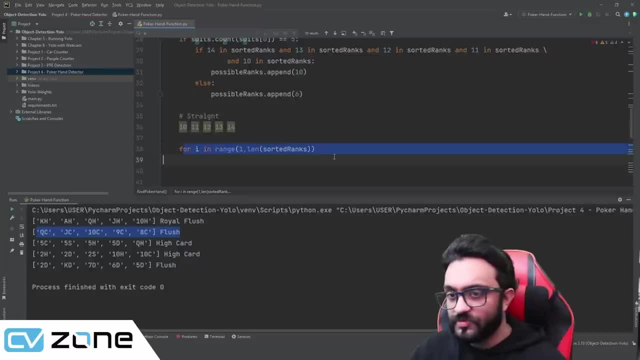 if that is the case, so to make it a little more efficient, we are going to write a single line for loop. so instead of writing it after, we will write it before that. so what exactly are we writing? we are writing that: sorted ranks at I. so sorted ranks at I, not one, not in ranks at I so. 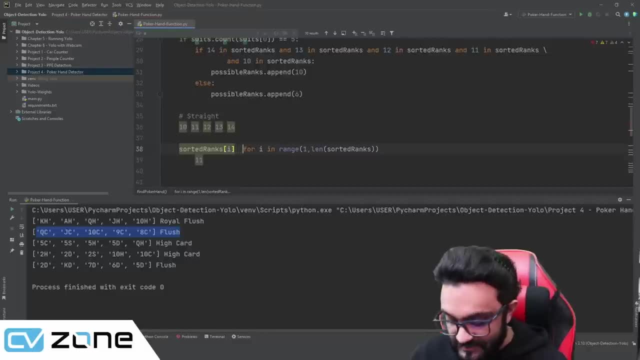 this will be, for example, 11. this is equal to sorted ranks at by minus 1 plus 1. so this is what we are doing. we are putting 11 equals 10 plus 1, right? if that is the case, and what we can do is we will keep getting the answer. 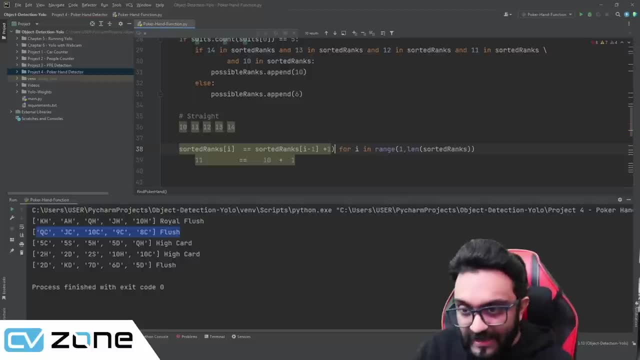 and all of this will be stored in a list. so in that list we can just write here: all. if all of them are true, then it will give us true. if even one of them is false, it will give us false. so that's the basic idea. so we need to put another bracket here and we will write it after that. 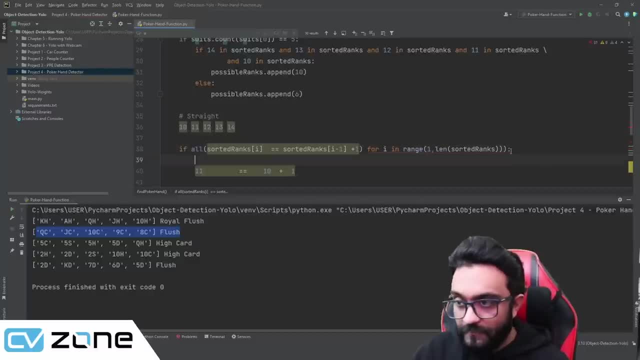 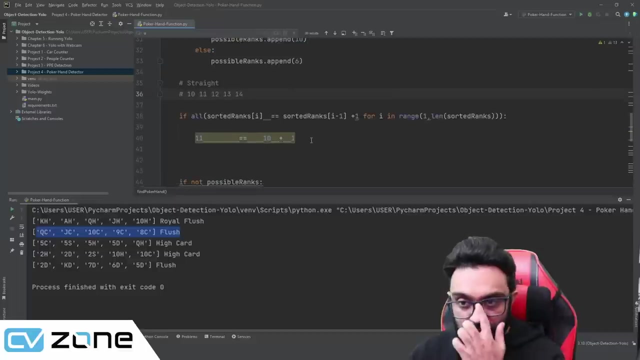 we will put an if statement, or is there a problem? one, two, two, three, okay, there should no, not be a bracket here. okay, so that's the idea. let me comment this as well. um, let me put this as well here, so that you understand what exactly happened. so, if that is true, it means it is a straight. 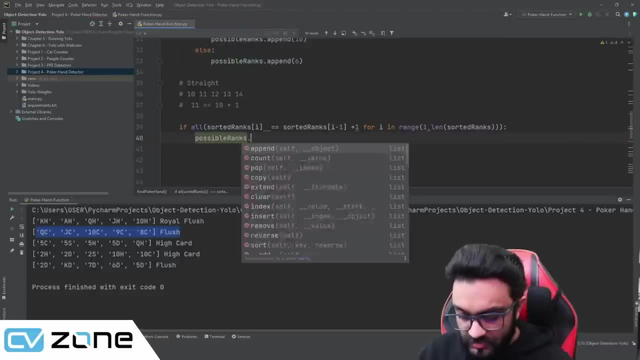 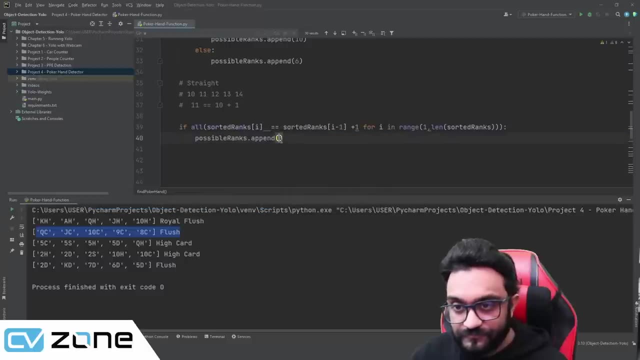 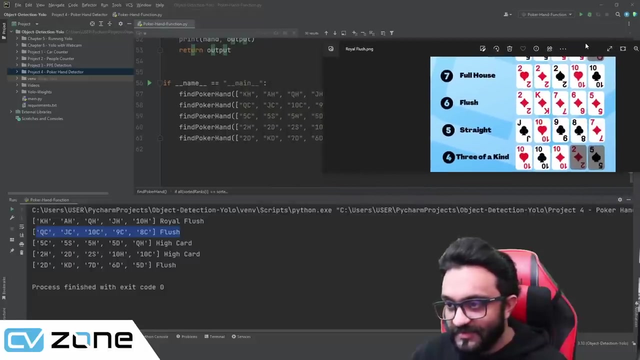 so we can write possible ranks. uh, dot append. what is a straight? a straight is number five, number five. did we add a straight so far? no, actually, let's add all of them, because that that's annoying, you know, going back and forth. so after flush we have straight. 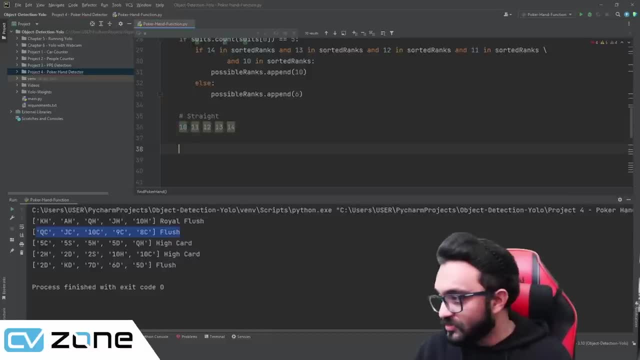 so we will start from one and not zero. so here we are going to write for i in range one till the length of our sorted ranks. it will be five. so should be fine, but we are still writing it. so if that is the case, so to make it a little more efficient, we are going 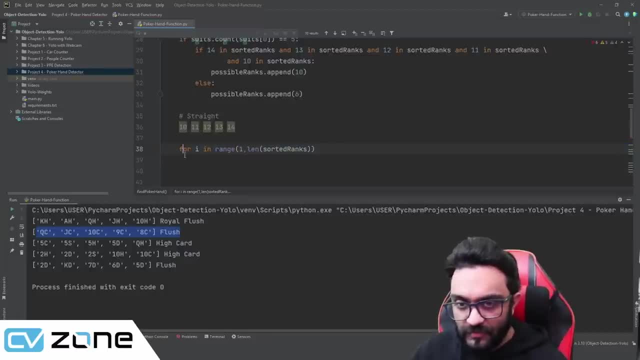 to write a single line for loop, so instead of writing it after, we will write it before that. so what exactly are we writing? we are writing that sorted ranks at i. so sorted ranks at i, uh, not one, not in ranks at i, so this will be, for example, 11.. this is equal to sorted ranks at i minus one. 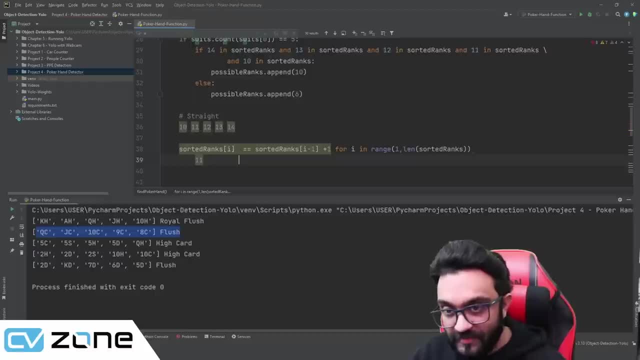 plus one. so this is what we are doing. we are putting 11 equals 10 plus one, right, if that is the case? and what we can do is we will keep getting the answer and all of this will be stored in a list. so in that list we can just write here all. 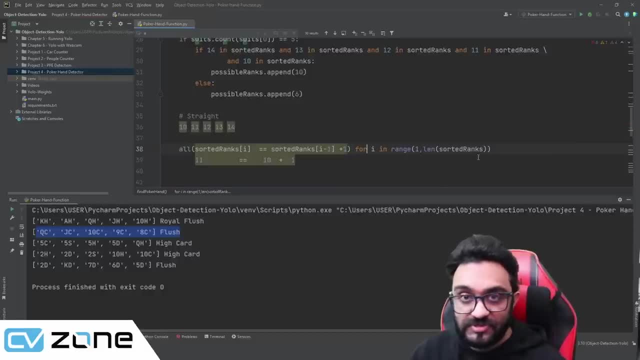 if all of them are true, then it will give us true. if even one of them is false, it will give us false. so that's the basic idea. so we need to put another bracket here and we will put an if statement, or is there a problem? one, two. 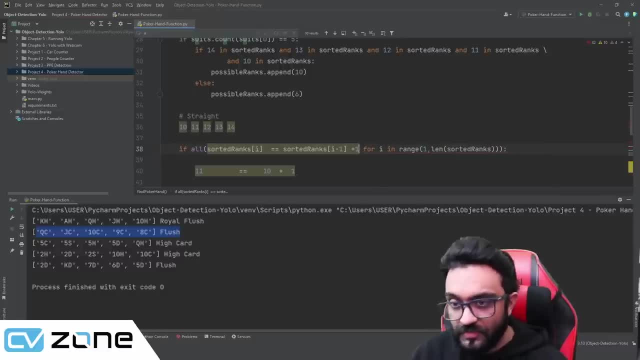 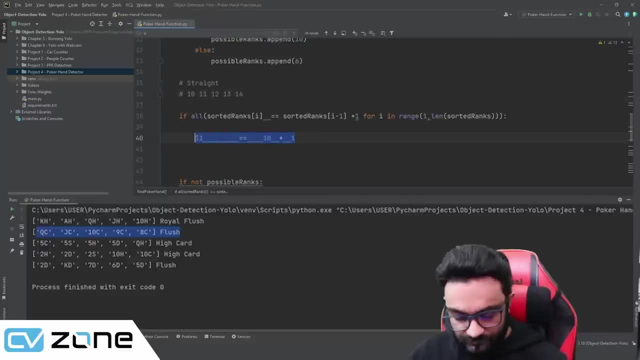 two, three. okay, there should not not be a bracket here, okay, so that's the idea. let me comment this as well. um, let me put this as well here so that you understand what exactly happened. so, if that is true, it means it is a straight, so we can write possible ranks. dot append. 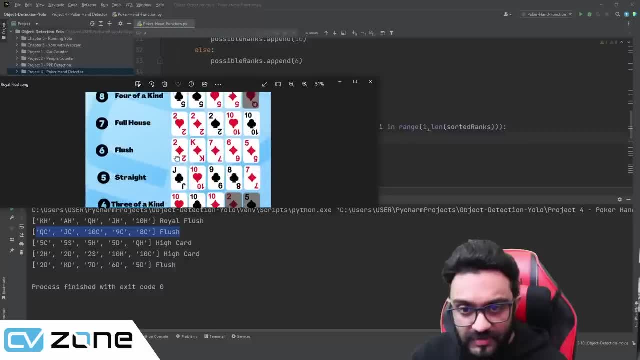 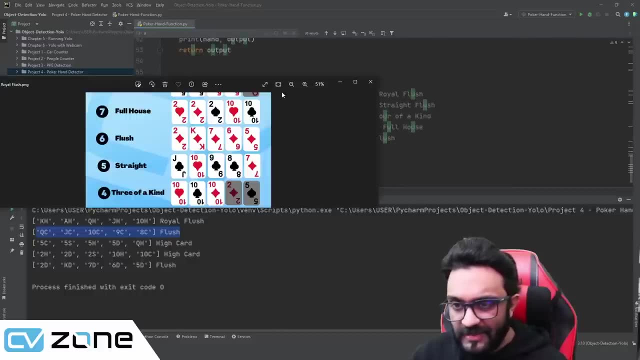 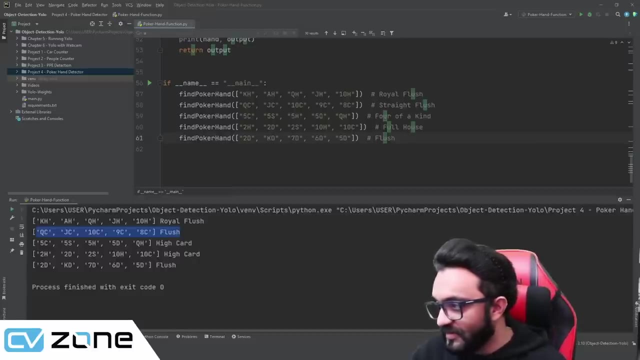 what is a straight? a straight is number five. number five. did we add a straight so far? no, actually, let's add all of them, because that that's annoying, you know, going back and forth. so after flush, we have straight, we have straight. then three of a kind, two pair, pair and high card. so flush, then we have straight. 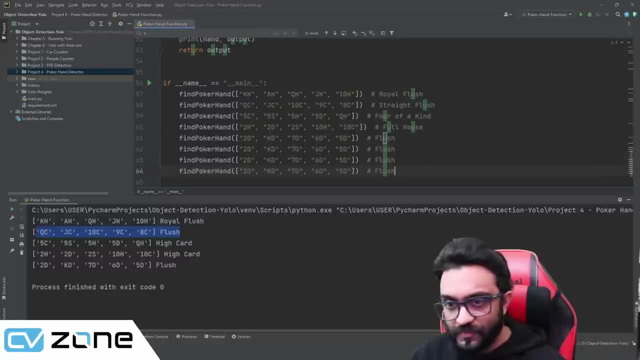 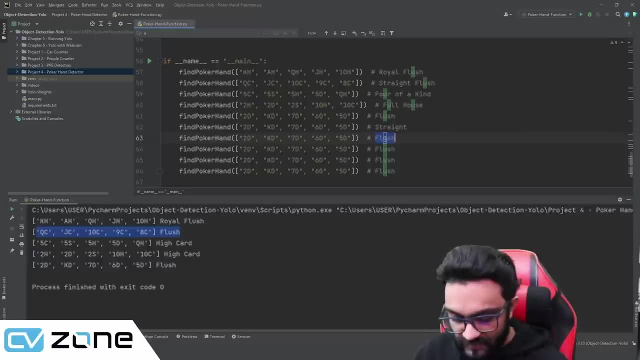 we have straight, then three of a kind: two pair, pair and high card. so flush, then we have straight, then we have three of a kind, uh, then we have two pair, then we have pair and then we have high card. there you go. so now we did till flush, now we 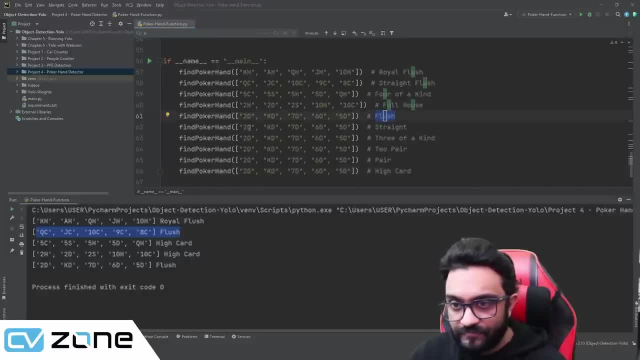 are going to do straight. so, for straight, we have Jack of spades, uh, clubs, Jack of Club. then we have 10 of hearts, then we have nine of Club, then we have eight of Club and then we have seven of Diamond. so this is our straight. and then poker hand, three of a kind. we have 10 of hearts, 10 of hearts, then 10 of. 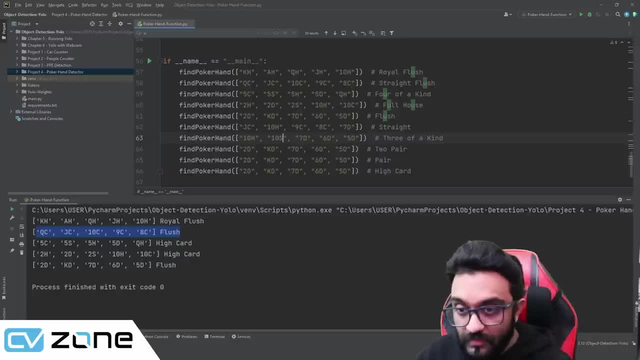 spades, 10 of spades, or is it? no, it's not spade, it's club. my bad uh. 10 of clubs and then 10 of diamonds. 10 of diamonds and then two of diamonds. two of diamonds and then two or five of uh. spades. 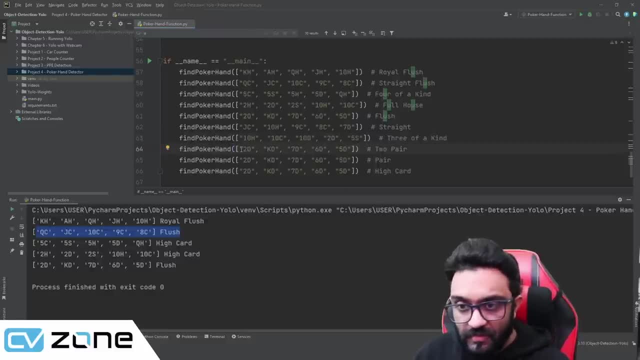 then two pair. we have king of king of diamond, then we have king of hearts, then we have five of clubs, then we have five of spade and then we have six of diamond. then we have a pair where we have two of diamond, two of two, of what is it? spades. then we have nine of nine of clubs and we have king of diamond. 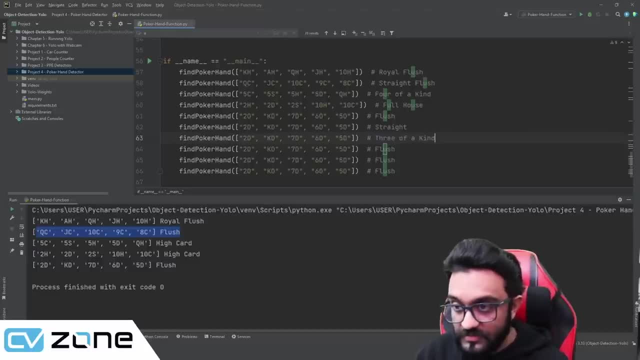 then we have three of a kind uh, then we have two pair, then we have pair and then we have high card. there you go. so now we did till flush, now we are going to do straight. so for straight, we have jack of spades, uh, clubs, jack of club. 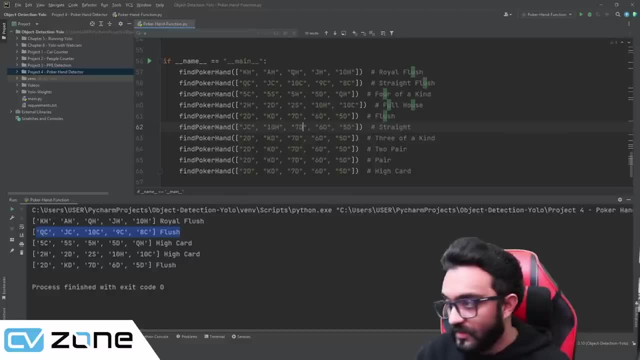 then we have ten of hearts, then we have nine of club, then we have eight of club and then we have seven of diamond. so this is our straight. and then poker hand, three of a kind. we have ten of hearts. ten of hearts, then ten of spades. 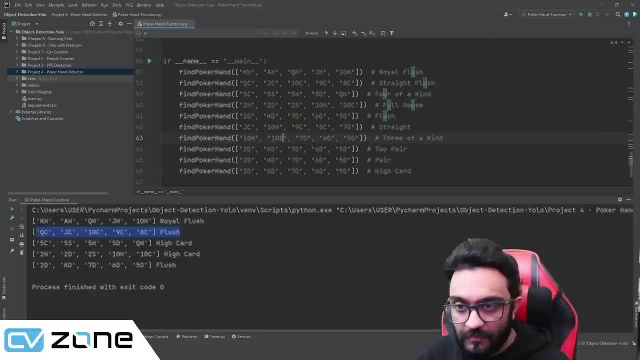 ten of spades, or is it? no, it's not. spades club, my bad. uh. ten of clubs. and then ten of diamonds. ten of diamonds and then two of diamonds. two of diamonds and then two or five of uh, spades, then two pair. we have king of king of diamond. 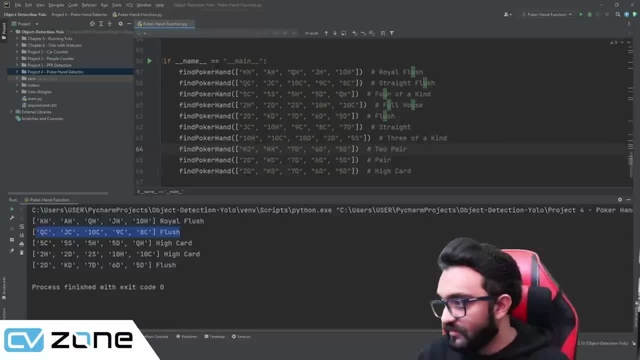 then we have king of hearts, then we have five of clubs, then we have five of spade, and then we have six of diamond. then we have a pair where we have two of diamond, two of two of- uh, what is it? spades. then we have nine of nine of clubs and we have king of diamond. 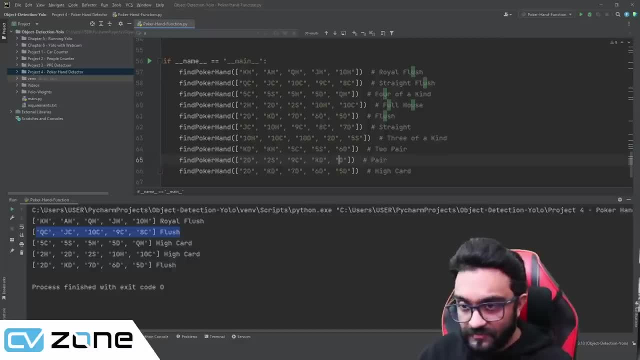 then we have ten of clubs. the last one is king of diamonds. so, king of diamonds, five of diamonds, then two of diamond, or five of diamonds, oh, five of hearts, my bad. five of hearts, two of diamond, and then ten of clubs, and then jack of diamonds, jack of hearts. i'm getting mixed up, okay, so that's the idea. and now 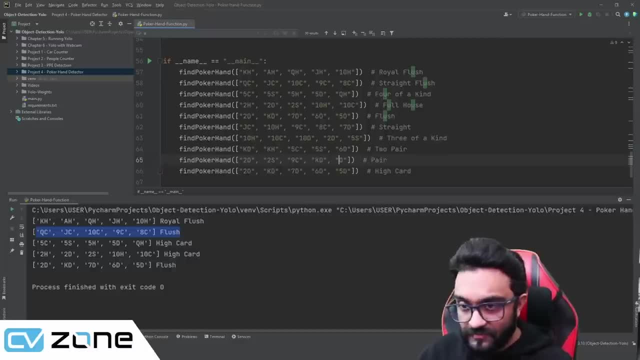 then we have 10 of clubs. the last one is king of diamonds. so king of diamond, five of diamonds, then two of diamond, or five of diamonds of hearts- my bad. five of hearts, two of diamond, and then ten of clubs, and then jack of diamonds, jack of hearts. i'm getting mixed up, okay? so that's the idea, and now let's run it um and see what do. 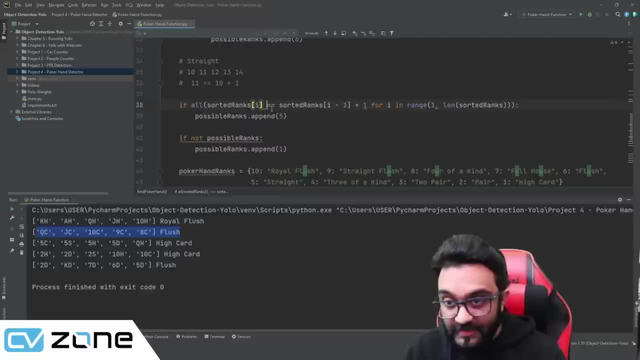 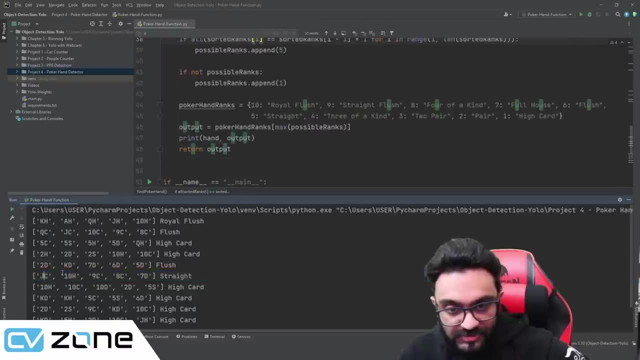 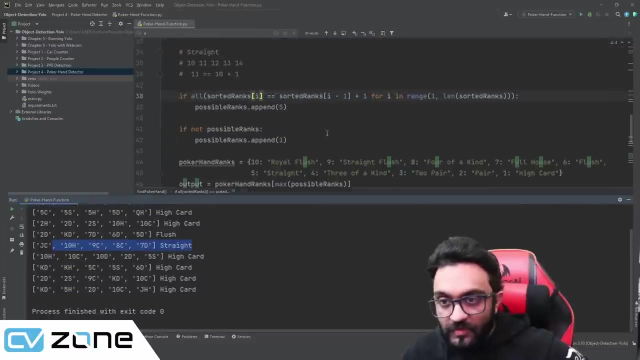 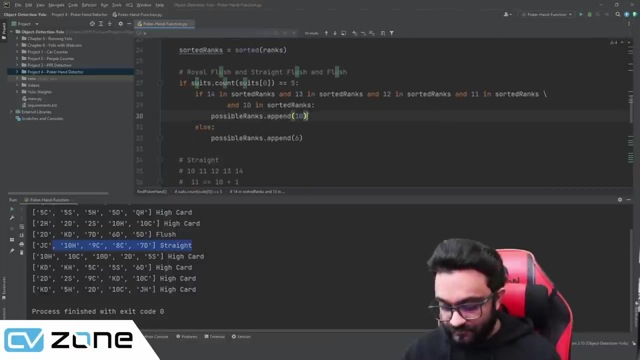 we get, so we should have the correct straight. so if we run this now for straight, this is straight. it is uh jack, ten, nine, eight, seven, and it is correct. so this is straight. now what we need to do is we need to take this straight part and we need to add it to our if statement here. so we will put else if. 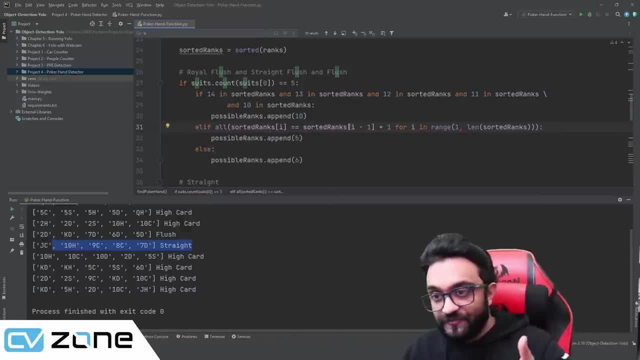 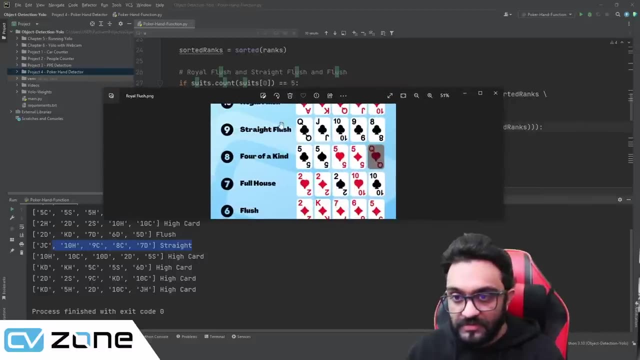 so first it will check if it's a flush and then it will check if it is a straight, then it will become straight flush. so straight flush is number nine. so you can see here: this is straight flush, so it will become number nine. so if we run, 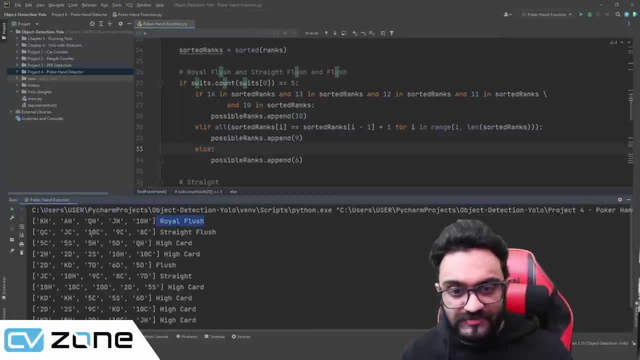 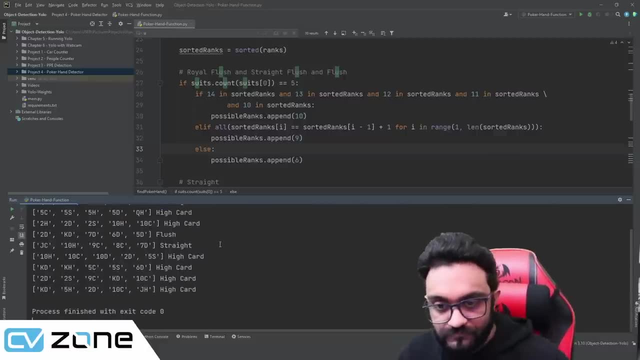 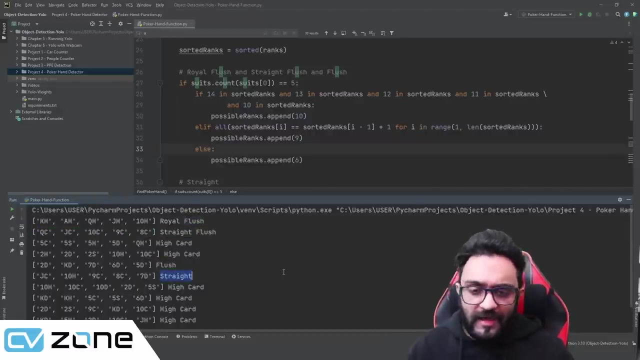 that now over here we have the royal flush. it's fine. the straight flush is now being detected as well, so that's very good. so we have the straight flush here, okay, so we have done one, two, uh, three and four. so we have done four, and we have also done the fifth, which is the high card. 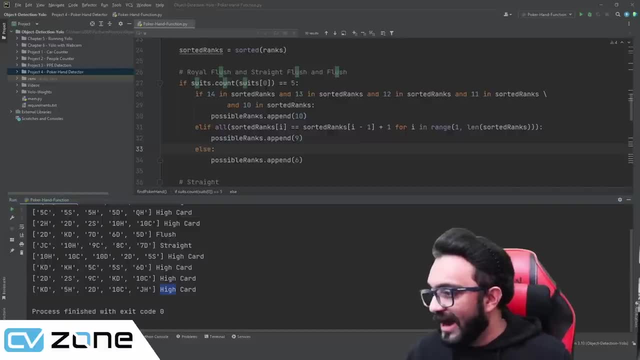 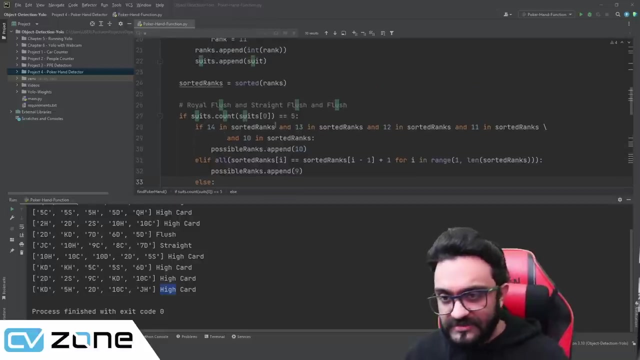 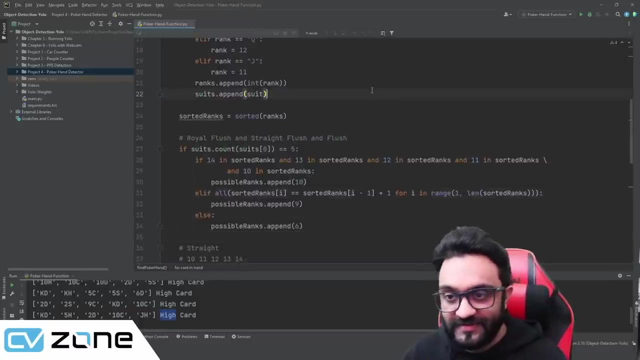 so we have done five out of ten, so we are halfway done. now what we will do is we are going to check for, uh, four of a kind, then we will check for three of a kind, then two pair and then a single pair. so, uh, to understand, how can we check, or why is it showing a search to move that? 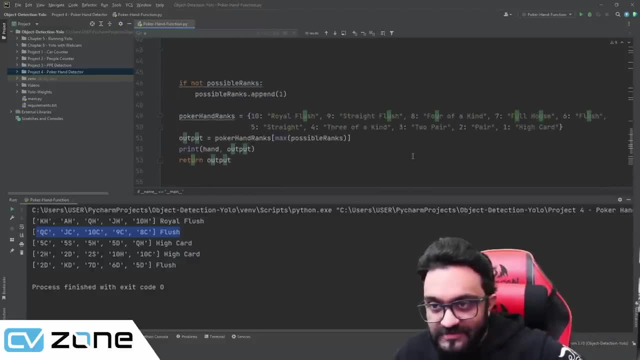 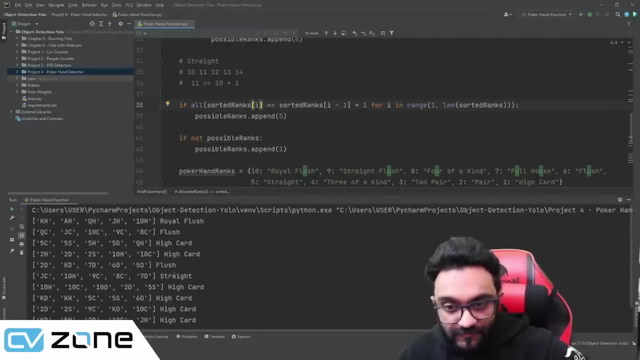 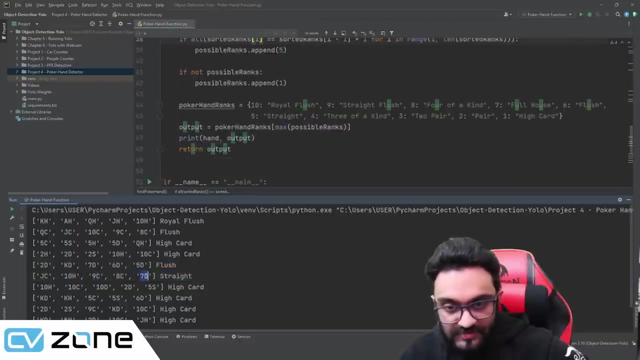 let's run it um and see what do we get. so we should have the correct straight. so if we run this now for straight, we should have a straight. so if we run this now for straight, we should have a straight for straight. this is straight, it is jack: 10, 9, 8, 7 and it is correct. so this is straight. 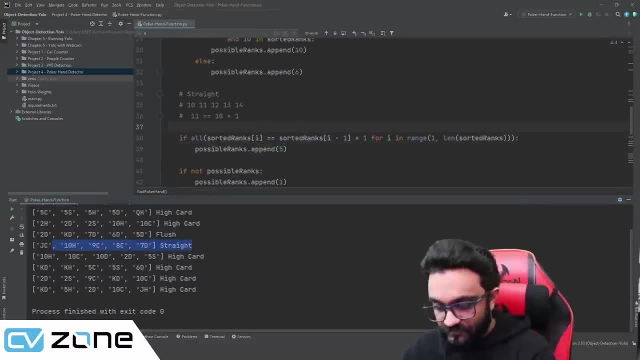 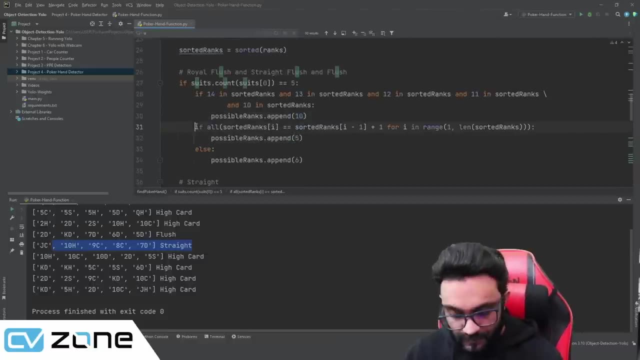 now what we need to do is we need to take this straight part and we need to add it to our if statement here, so we will put else. if so, first it will check if it's a flush and then it will check if it is a straight. then it will become. 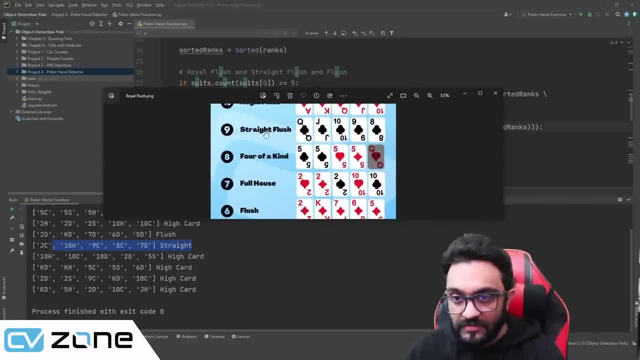 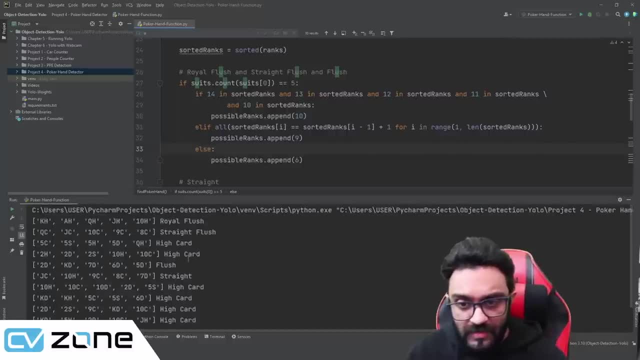 straight flush. straight flush is number nine, so you can see here this is straight flush, so it will become number nine. so if we run that now over here, we have the royal flush. it's fine. the straight flush is now being detected as well, so that's very good. so we have the straight flush. 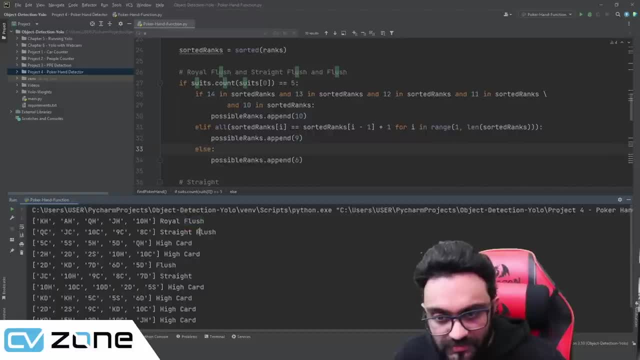 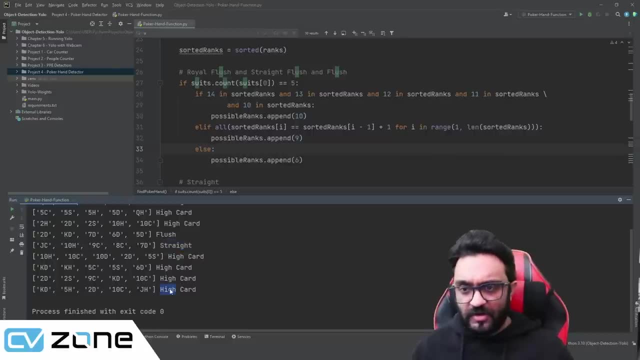 here. okay, so we have done one, two, uh, three and four. so we have done four. and we have also done the fifth, which is the high card. so we have done five out of five. so we have done five out of five, ten. so we are halfway done. now what we will do is we are going to check for, uh, four of a kind 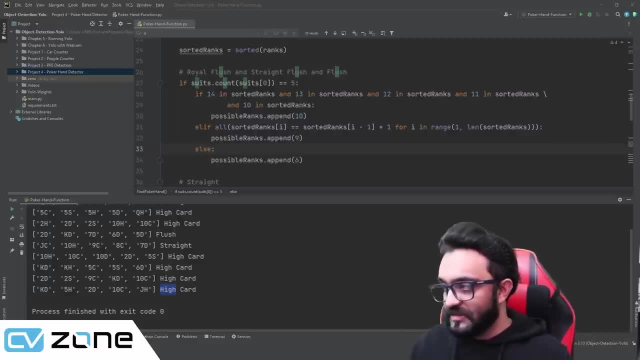 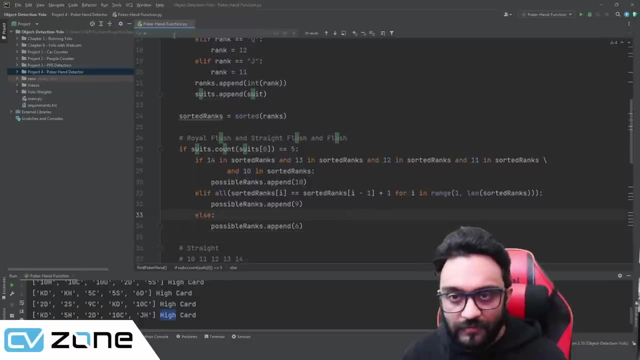 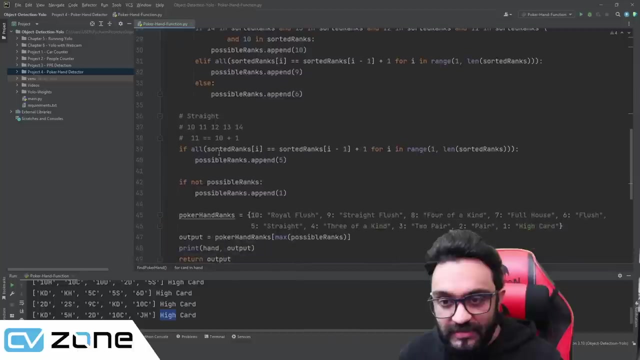 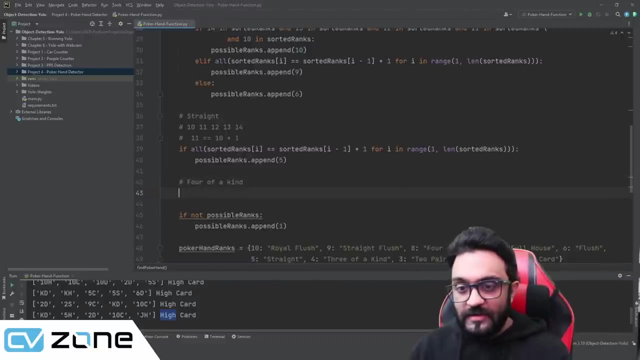 then we will check for three of a kind, then two pair and then a single pair. so, uh, to understand, how can we check? or why is it showing a search? let's remove that, okay. so to check, let's do it after straight. this is four of a kind. now four of a kind. if you have a list right, uh, four of a kind will have. 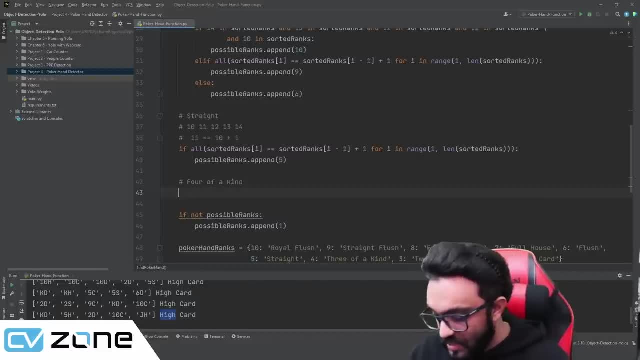 four of them as the same and one card will be different. so, for example, you will have three, three, three, three and then five. so three of uh, four of them are same and one of them is different, right? so what we can do is we can tell it. 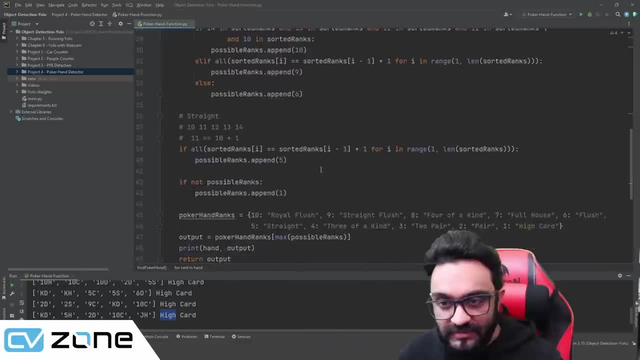 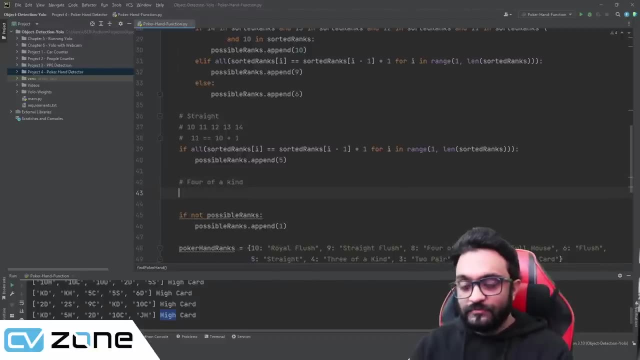 okay. so to check, let's do it after straight. this is four of a kind. now, four of a kind, if you have a list, right, uh, four of a kind will have four of them as the same and one card will be different. so, for example, you will have three, three, three, three and then five. so three of uh, four of them. 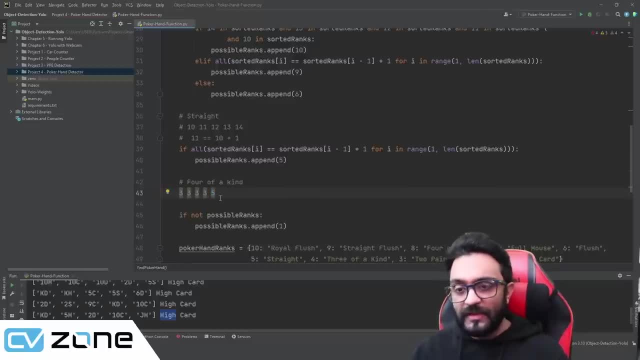 are same and one of them is different, right? so what we can do is we can tell it. we can tell the computer to find, to create a set. what does a set do? a set will put all these three together and it will put this as separate. so when you do a set to this, 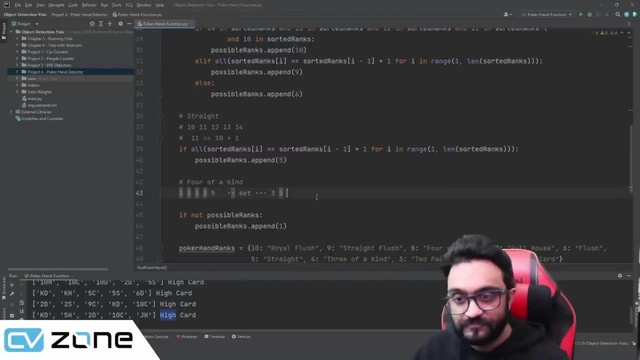 when you do a set, this will become three and five, so we can check how many do we have. we have three and five, so after completing the set, how many values do we have? if we have two values, this means it might be four of a kind, because 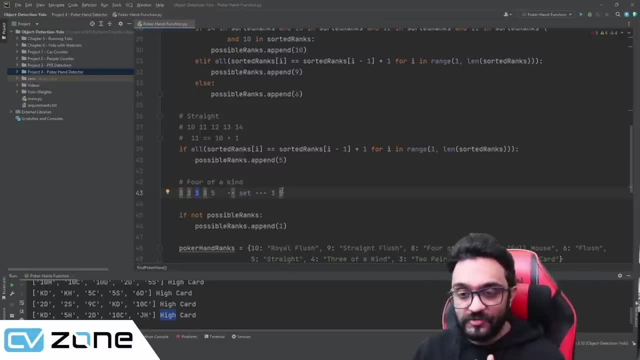 there is another condition where you can have two set, and that is when you have, let's say, three, three, three, three, three, three and five and five, five. So in that case if you do a set, then also it will give you three and 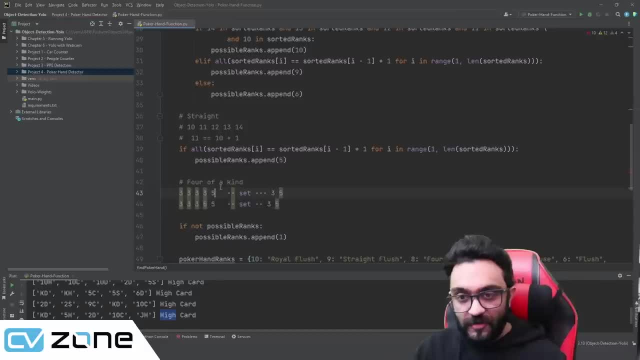 five. So we need to check first of all whether, when we convert it into a set, does it give us two values. If that is two, then we need to check whether this value comes three times or four times. If it comes three times, then it is four of a kind. If it comes three times, 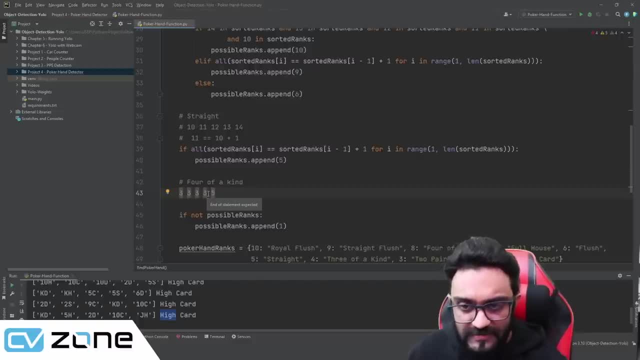 we can tell the computer to find, to create a set. what does a set do? a set will put all these three together and it will put this as separate. so when you do a set to this, when you do a set, this will become three and five, so we can check how many do we have. we have three and five, so 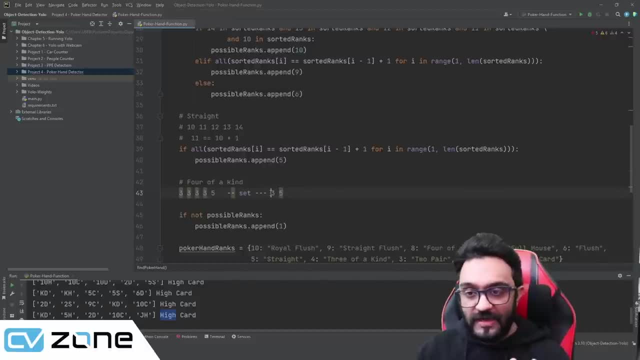 how many do we have? now? we have three, we have one and then a set. the set is one, then another, and two and then another, and so on. as we are doing a set, we will be getting four of a kind, and after completing the set, how many values do we have? 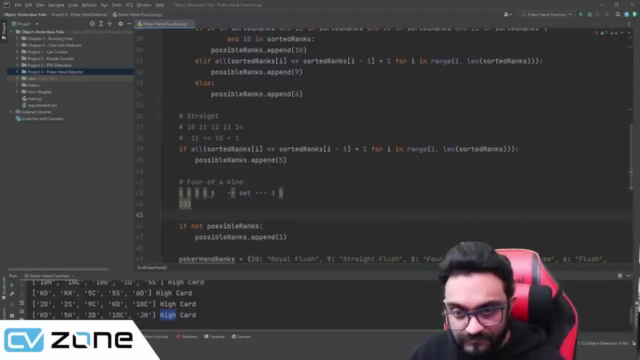 if we have two values, this means it might be four of a kind, because there is another condition where you can have two set and that is when you have, let's say, three, three, three, three, three, three and five, five, you, three and five. so we need to check first of all whether, when we convert it into a set, 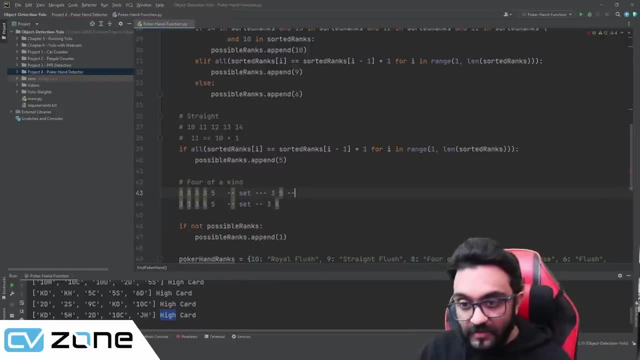 does it give us two values? if that is two, then we need to check whether this value comes three times or four times. if it comes three times, then it is four of a kind. if it comes three times, then it is full house, because these are three, three of a kind, and this is. 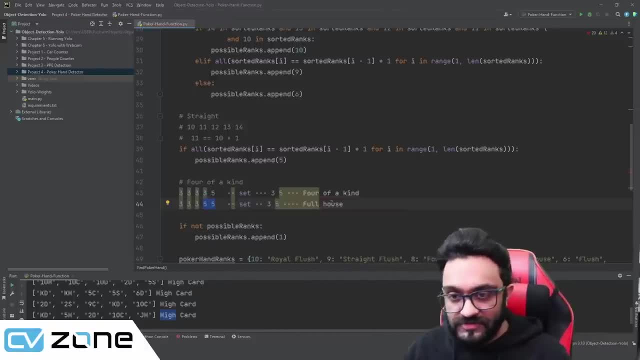 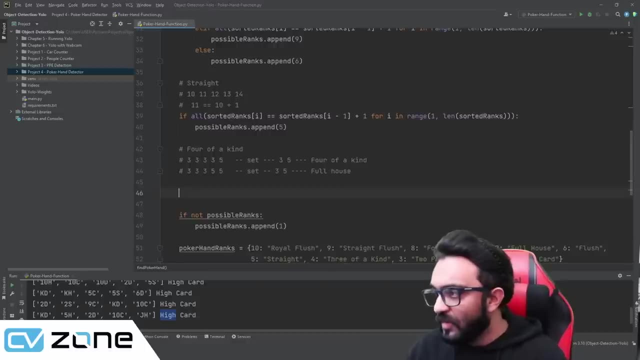 a pair, so it becomes full house. so how can we do that? first of all, what we will do is we will get unique values, so hand unique values equals set, set, set of sorted ranks, sorted ranks. but this will be a set. you cannot use it as a list, so we 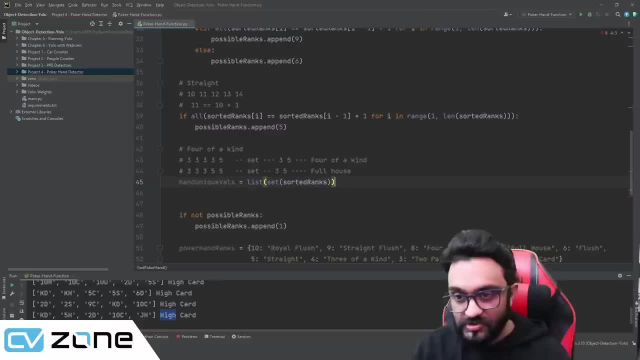 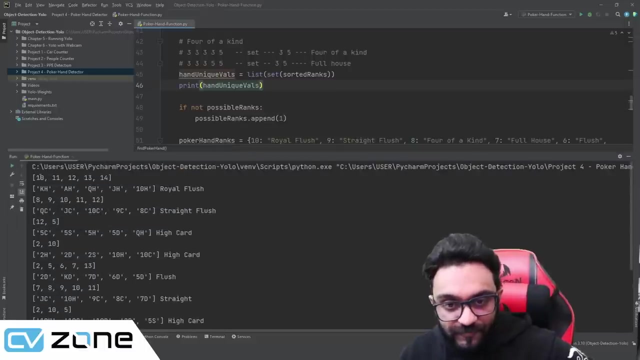 will convert it into a list to make it easier for us to work with. so we will do that. so if i print unique hands now print unique, oh hand unique values. so let's print that and for each hand it will print the unique values. so for the first one, 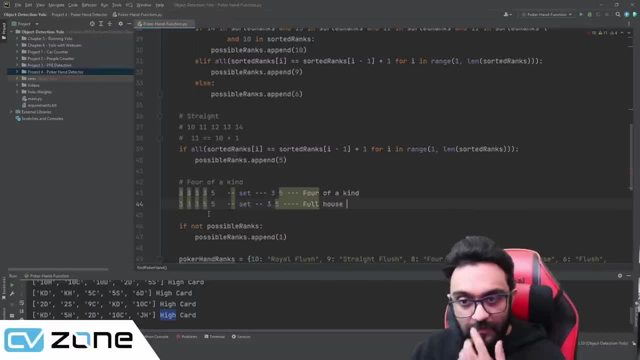 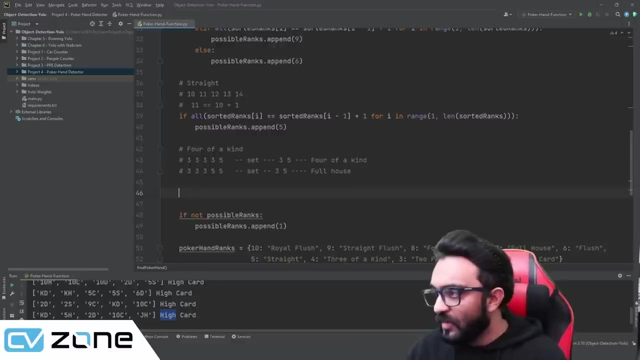 then it is full house, because these are three, three of a kind, and this is a pair, So it becomes full house. So how can we do that? First of all, what we will do is we will get unique values. So hand unique values equals, set of sorted ranks, sorted ranks, But this will be a set. 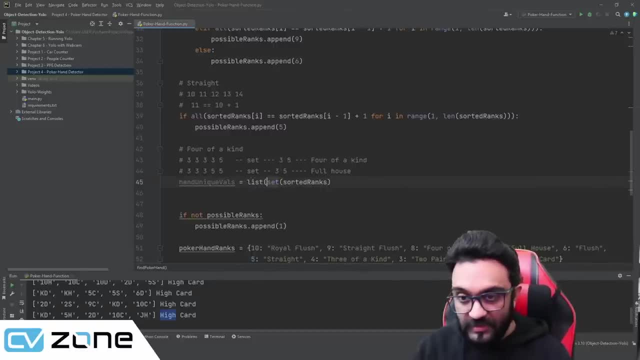 You cannot use it as a list, So we will convert it into a list to make it easier for us to work with. So we will do that. So if I print unique hands now print unique values. Oh, hand, unique values. So let's print that And for each hand it will print the. 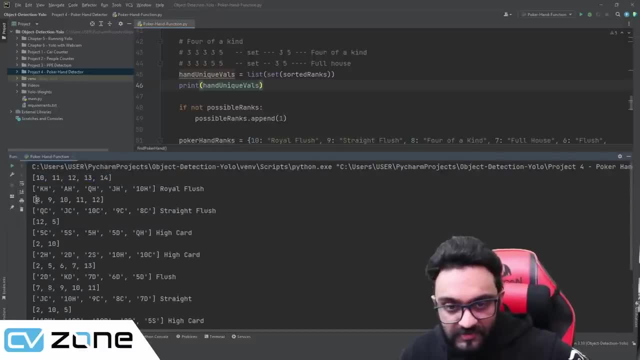 unique values. So for the first one there are no unique values. So eight, nine, 10,, 11,, 12.. So it's printing that For the second one again. oh sorry, the first one was here. 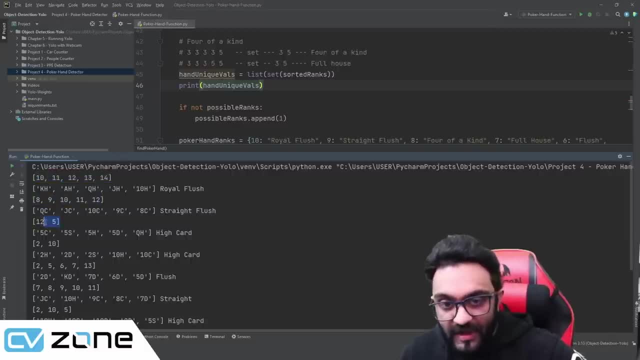 The second one: no unique values. In the third one, you have unique values, So you have five, five, five. It's three of them. Four of them are five, So it's giving us five, And one of them is a 12. So it's giving us 12 and five. So this one is basically four of a kind, And after four, 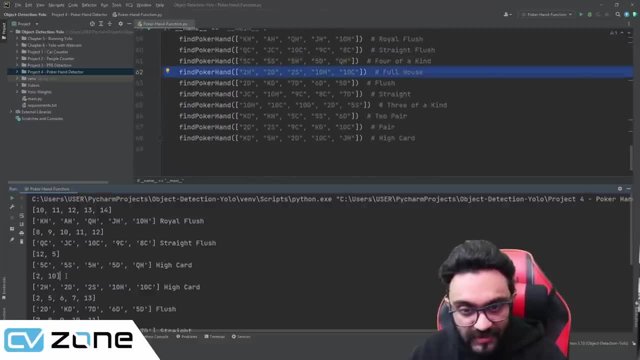 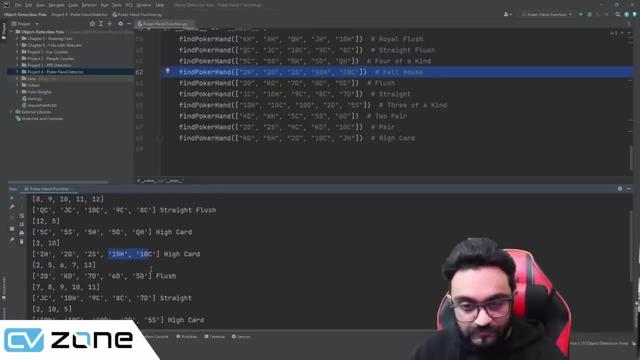 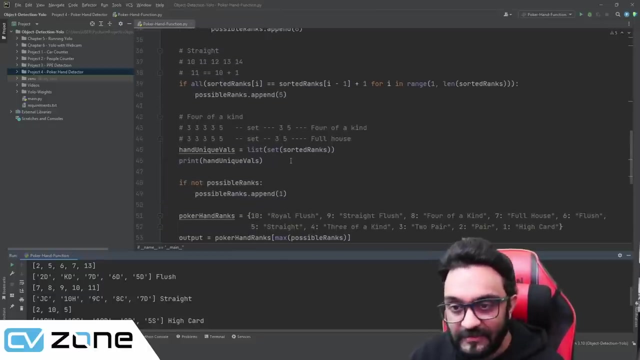 of a kind we have a full house, So that is also giving us two. So it was giving us two and 10.. So these are three and this is two. So now we need to check if the unique hand list basically has two. 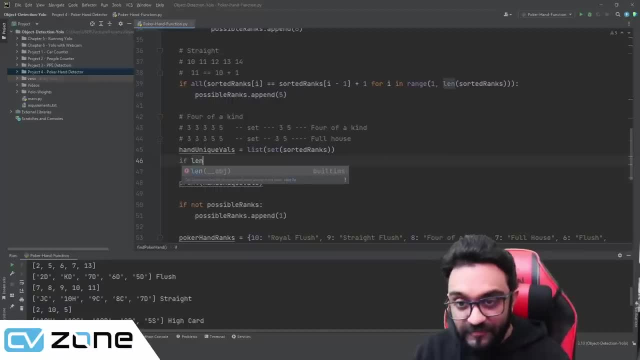 Values. So first of all, we need to check if it has two values, If the length of hands- unique values- equals two. if that is the case, then it will be one of these four of a kind or full house. Actually, we should, we should put this here somewhere, but it took. I think we should put. 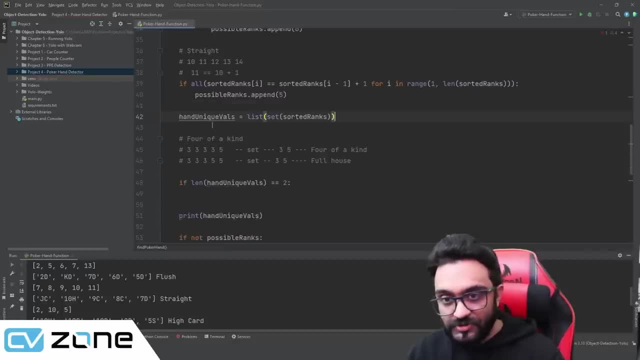 this one outside, because this one is journal. It will also be used for three of a kind. It will also be used for full house, for two pair and so on, because this is unique values. So now we are checking for four of a kind. So now what we will do is we are going to check. 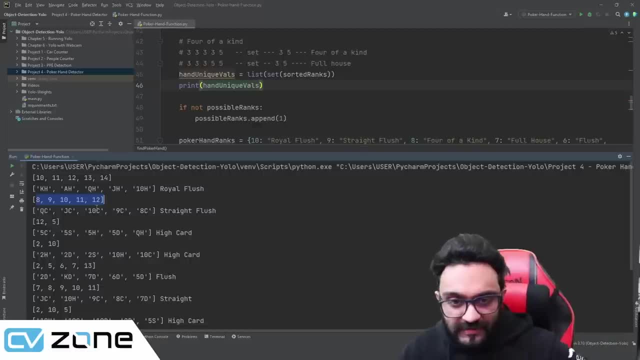 there is no unique values, so 8, 9, 10, 11, 12. so it is printing that for the second one again. oh sorry, the first one was here, the second one: no unique values. in the third one you have unique values, so you have five, five, five. it is three of them. four of them are five, so it is. 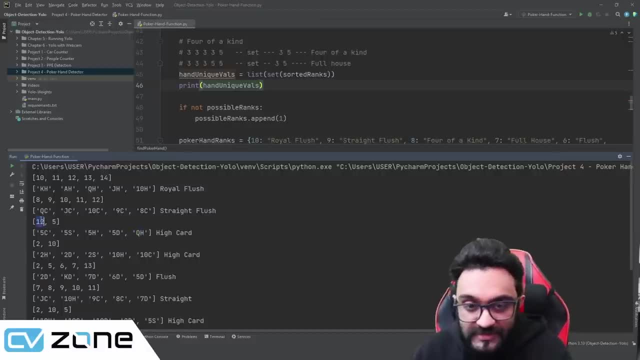 giving us five, and one of them is 12, so it is giving us 12 and 5, so this one is basically 4 of a kind and after 4 of a kind. do not give those values. there is a 2 at first, so the second is 12, which means 12, and the 3 is the 5th person. not sure about whether they are one vs the other, but they are 4 in the last 3 and the rest are four. 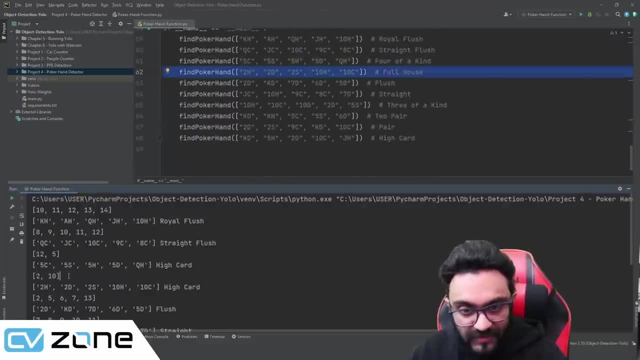 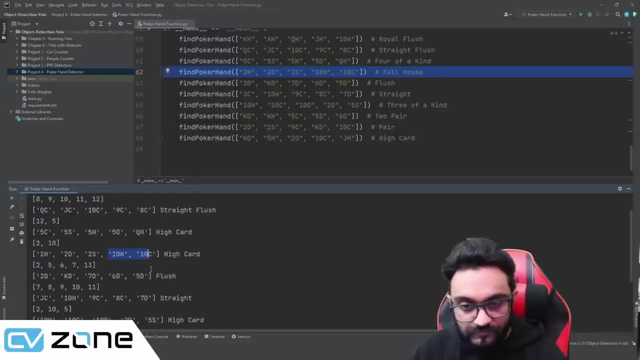 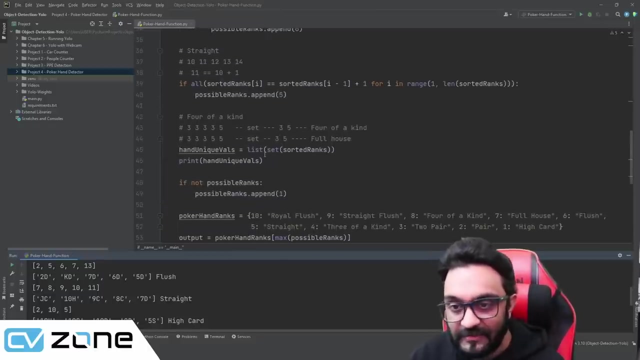 of a kind we have a full house, so that is also giving us two. so it was giving us two and ten. so these are three and this is two. so now we need to check if, if the unique hand list basically has two uh values. so first of all we need to check if it has. 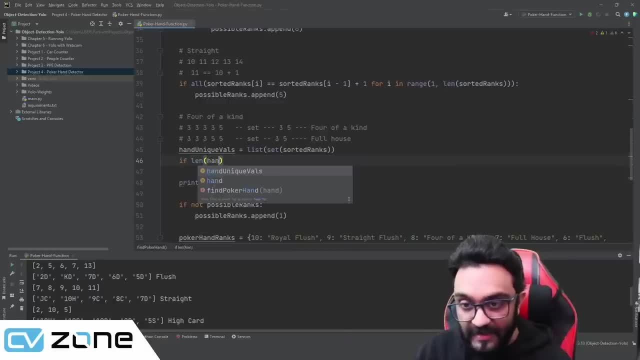 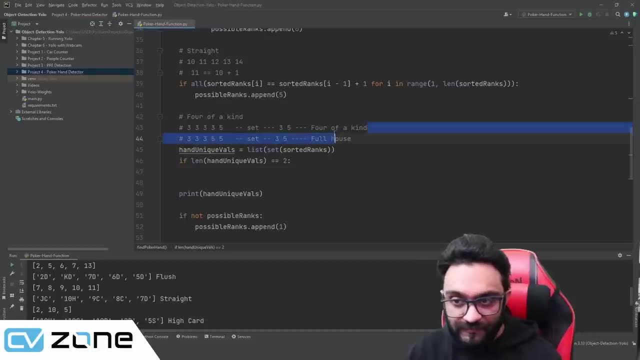 two values if the length of hands- unique values- equals two. if that is the case, then it will be one of these four of a kind or full house. actually we should, we should put this here somewhere, but it's okay, i think we should put this one outside, because this one is journal. it will also be used. 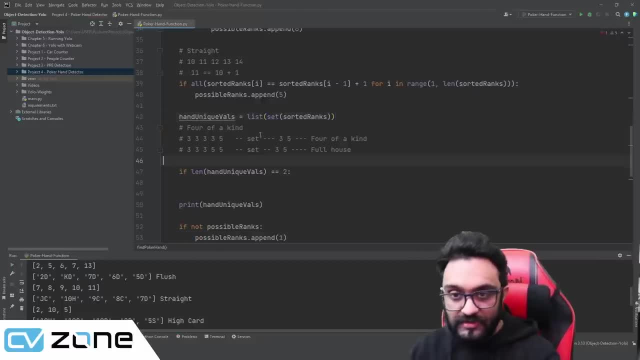 for three of a kind. it will also be used for full house, for two pair and so on, because this is unique values. so now we are checking for four of a kind. so now what we will do is we are going to check, we are going to loop through all the values. 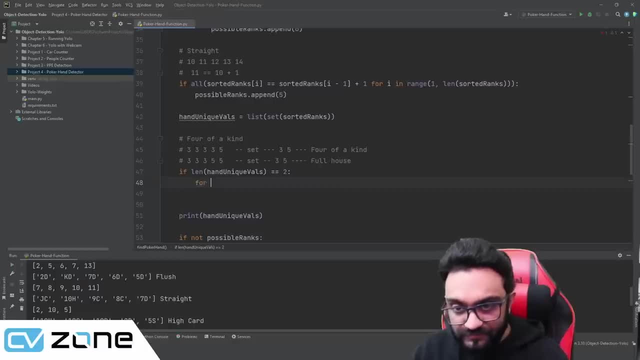 for: okay, for value, value in hand, unique values. so it will loop through the values, which will be 12 and 5. okay, so for each value we need to count how many times is it present in our complete list? so we will say that, how many times the value of, let's say, uh. 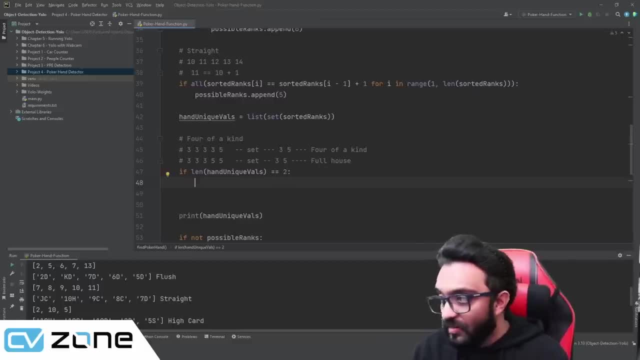 we are going to loop through all the values For- okay for value, value in hand, unique values. So it will loop through the values which will be 12 and five. Okay, So for each value we need to count how many times is it present. 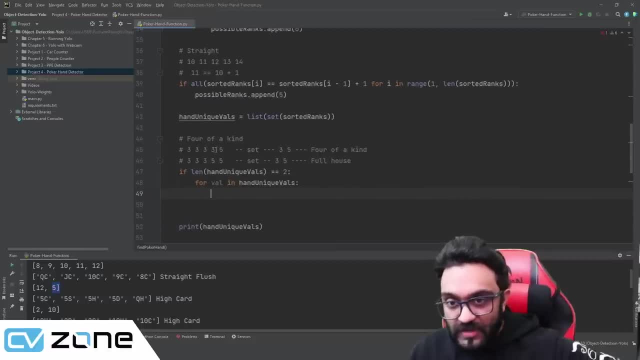 In our complete list. So we will say that how many times the value of, let's say, uh, uh, three is present in this whole uh list? We need to check that. So we will say that sorted ranks dot count. 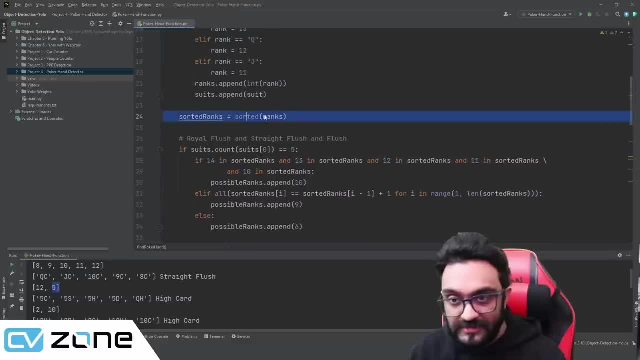 So this is our sorted list. Where is it? This sorted list is basically eight, nine, 10,, 11,, 12.. Or in this case it is five um, five, five, five, five. Q, right, Uh? or queen is 13.. Uh, no. 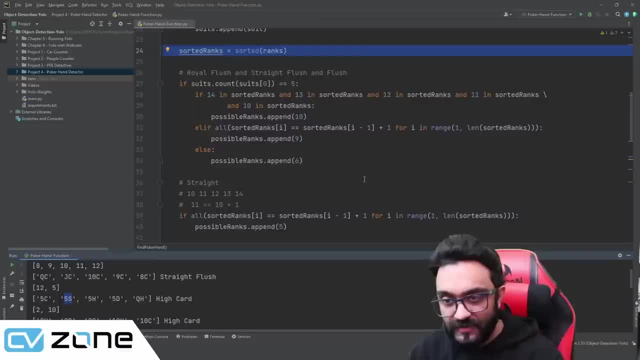 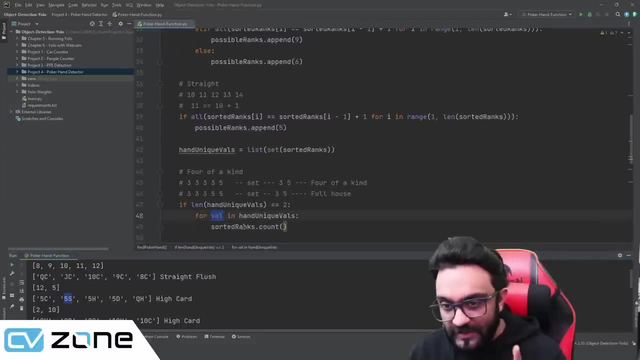 it's 12.. So it's: uh, five, five, five and then 12.. So that's our sorted. So we are going to check this value. How many times does it come in the main list? So we will write here: val. 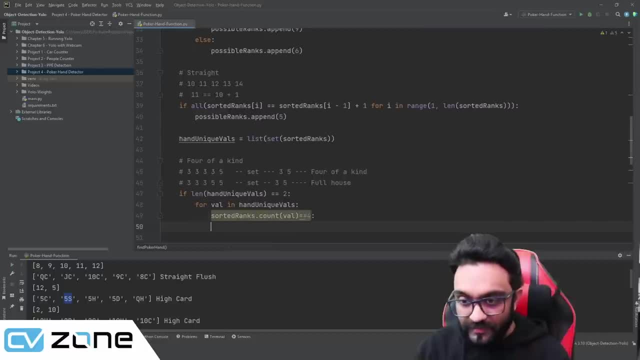 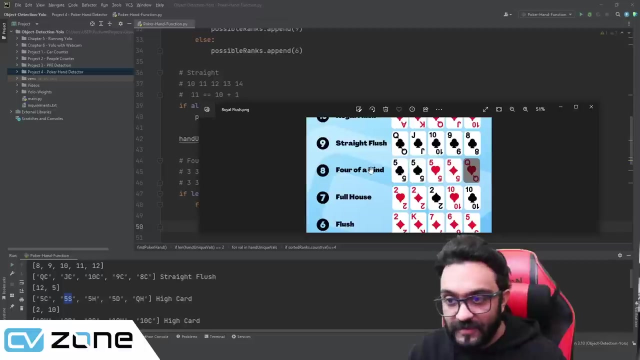 And if that comes four times, then we are going to write. uh, we need to write. if that is the case, then we will write possible rank dot append. Uh, what is four of a kind? four of a kind is number eight, So we will append eight. 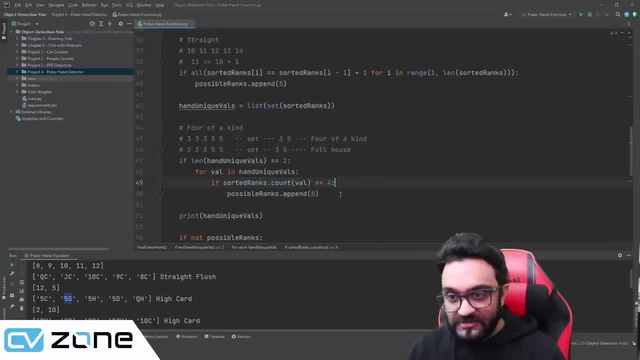 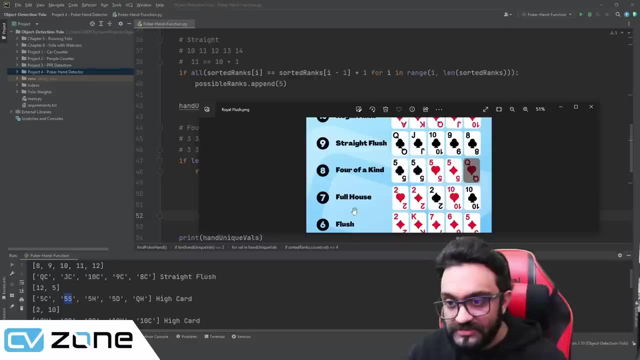 And if it is not four times, if it's three times, then it means it is number seven, which is full house. If it's three times and the the, the set is two. This is a. this is a unique value. This is a unique value, The set is: 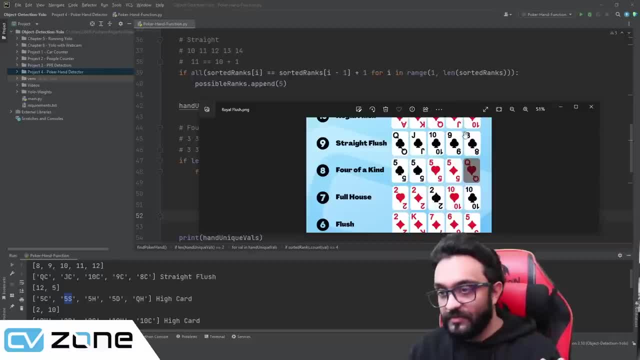 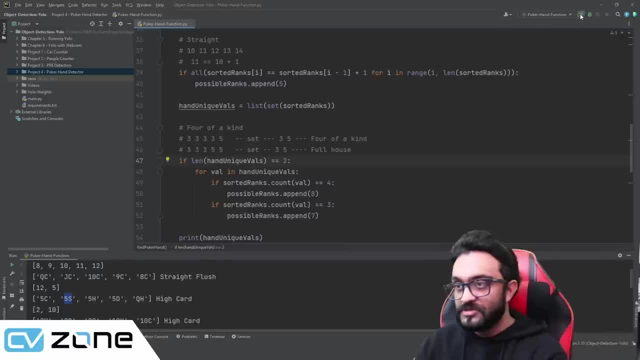 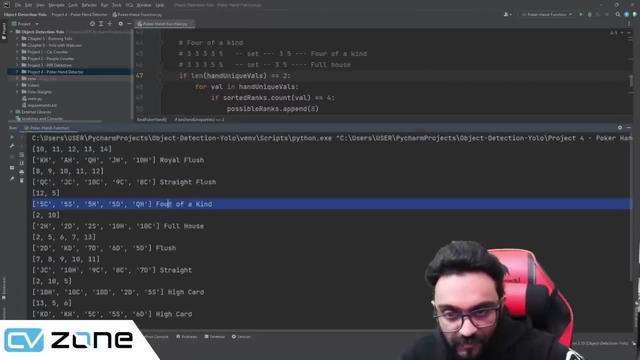 two And one of them is three, It means the other one will be two automatically. So we know that if it's three, then the rank is seven. So if we run this now, you will see that here we have the royal flush straight: four of a kind. It's detected properly. This is four of a kind, And if it's 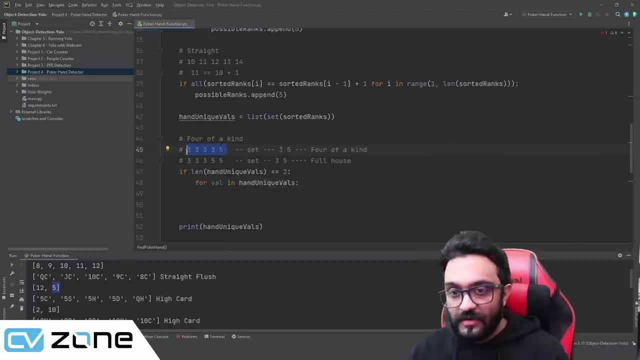 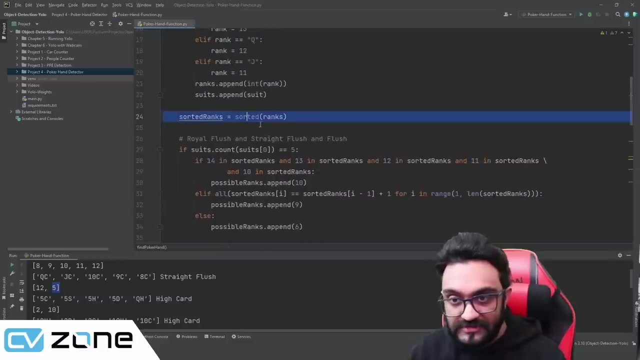 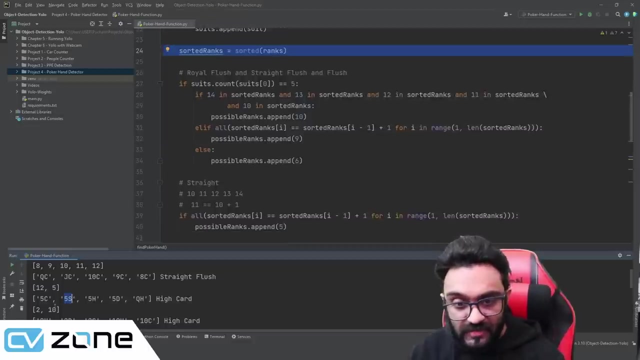 three is present in this whole uh list. we need to check that. so we will say that sorted ranks dot count. so this is our sorted list. where is it? this sorted list is basically eight, nine, ten, eleven, twelve, or in this case it is five, um, five, five, five, five, q, right, uh, or queen is thirteen. no, it's twelve. so it's five, five, five and. 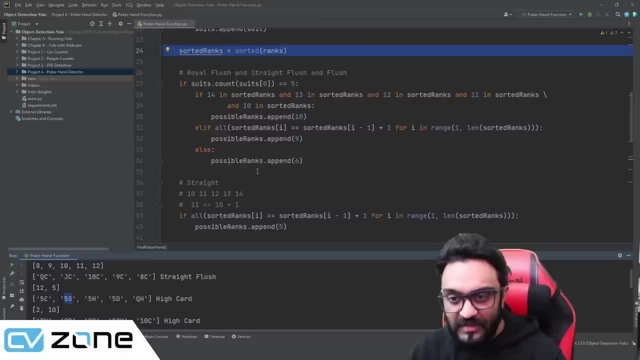 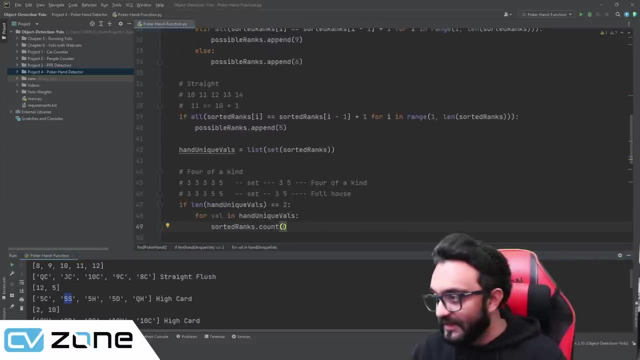 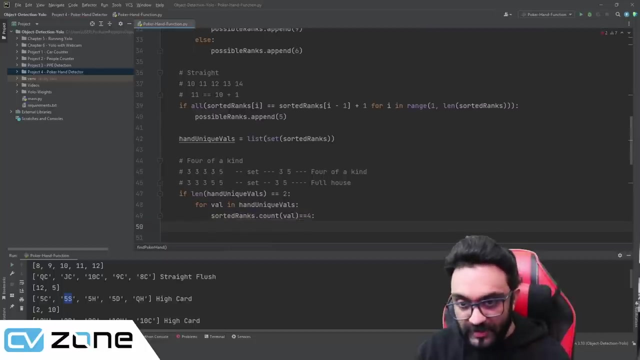 then twelve, so that's our sorted. so we are going to check this value. how many times does it come in the main list? so we will write here, val, and if that comes four times, then we are going to write. we need to write if that is that here in the list we can't see it, so we have to write if that is the. 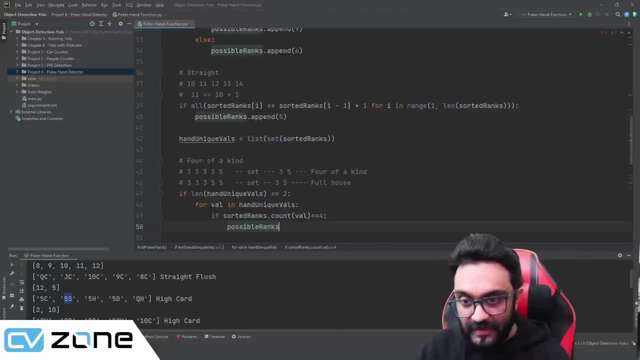 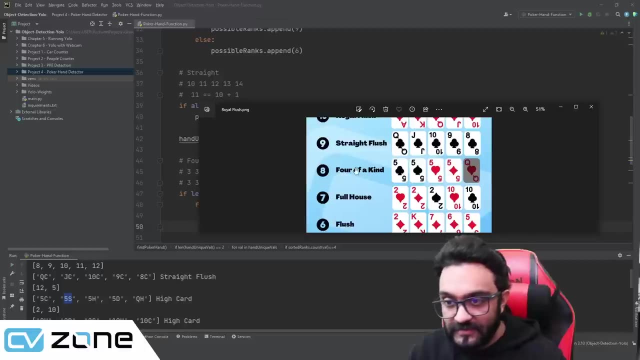 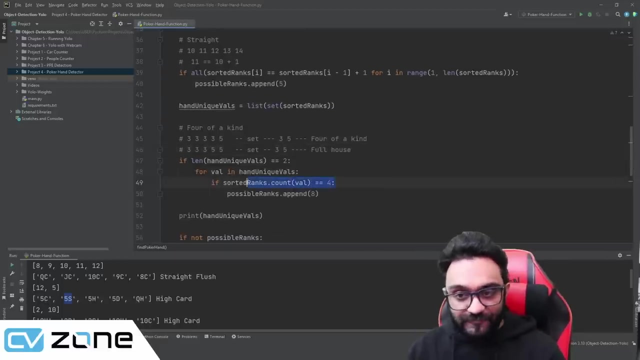 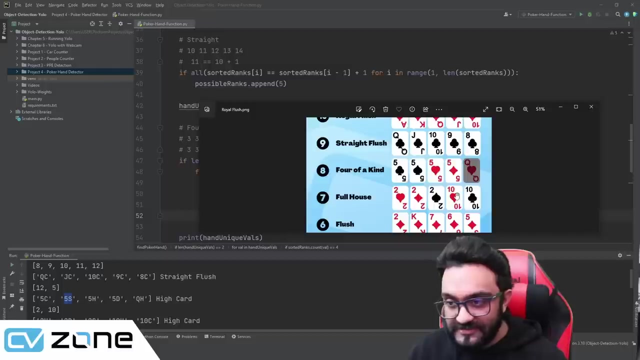 that is the case, then we will write possible rank dot append what is four of a kind. four of a kind is number eight, so we will append eight and if it is not four times, if it's three times, then it means it is number seven, which is full house. if it's three times and the the set is two, this is a. 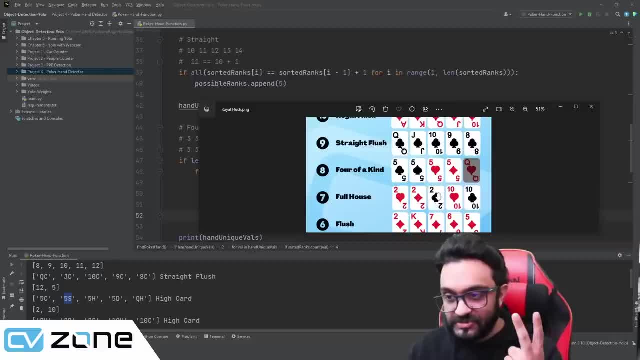 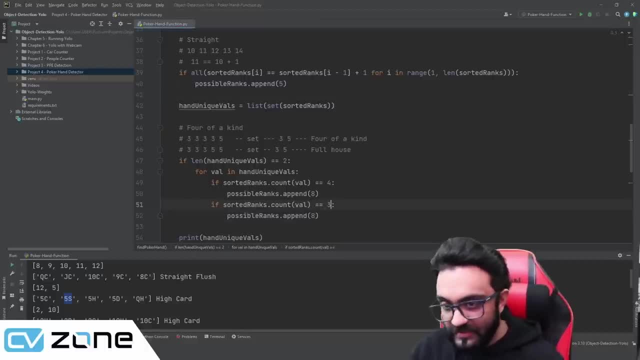 this is a unique value. this is a unique value. the set is two and one of them is three. it means the other one will be two automatically. so we know that if it's three, then the rank is seven. so if we run this now, you will see. 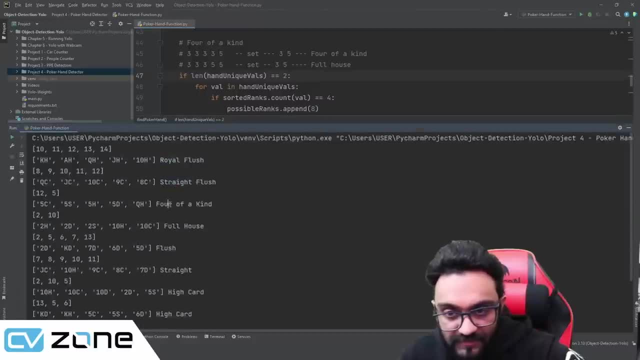 that here we have the royal flush straight. four of a kind. it's detected properly. this is four of a kind. there you go, and then if we have a full house, it is also detected properly. oh sorry, this is full house. this is, uh, four of a kind. so here we have two and ten. so this is full house and this is. 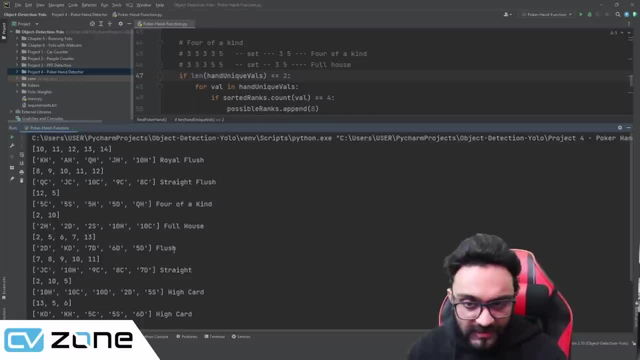 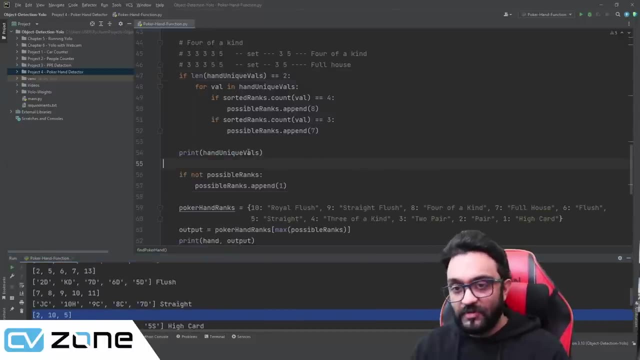 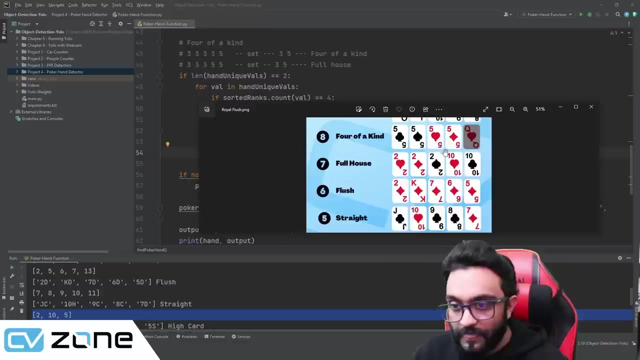 four of a kind. there you go, and already we have the flush and the straight working. so that's good. so this is the same pattern we are going to use with, uh, the next, the next one, which is three of a kind. so here we have done the flush, we have done the straight, now we are going to three of a kind. so 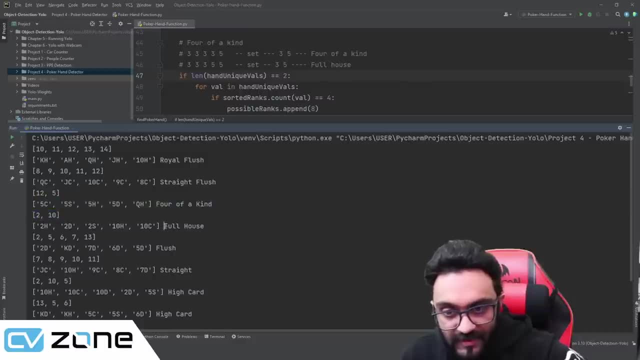 four of a kind. there you go, And then, if we have a full house, it is also detected properly. Oh sorry, This is full house, This is a four of a kind. So here we have two and 10. So this is. 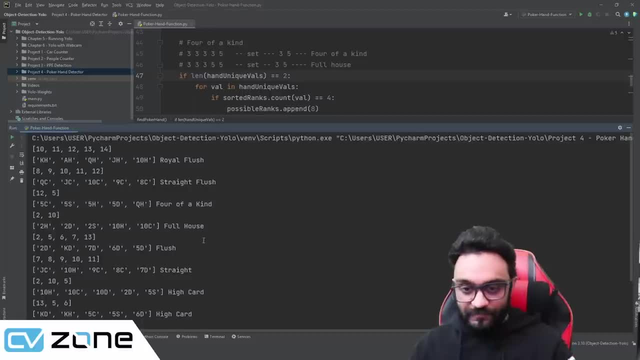 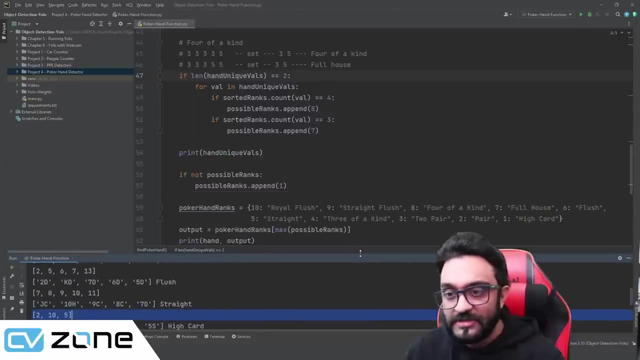 full house, and this is four of a kind. There you go, And already we have the flush and the straight working. So that's good. So the same pattern we are going to use with, uh, the next, the next one, this three of a kind. So here we have done the flush, We have done the straight, Now we are going. 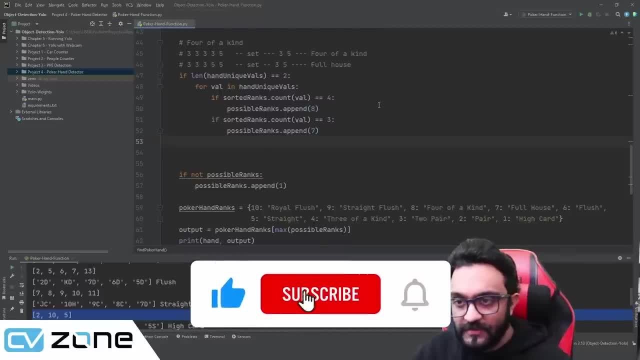 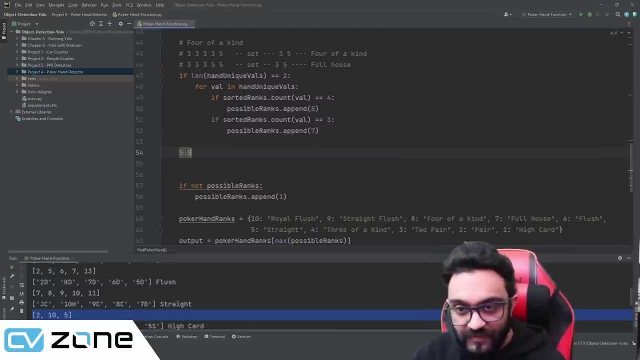 to three of a kind. So now we are going to three of a kind and two pair. So if let's say we have a three of a kind, so we will have five, five, five, five and five, and we will have, uh, let's say, 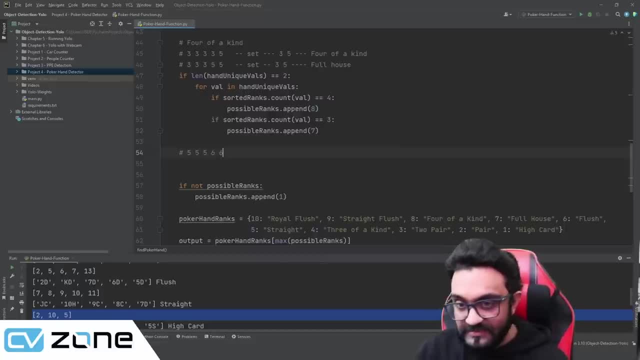 six and seven, because if we have six, six, it becomes a full house. We are not talking about that, right? Uh, we are not, Because we have already done that. So if it's six and seven, then it will give us how many unique. 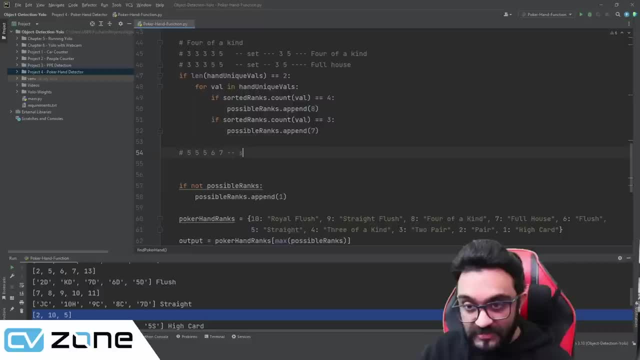 values. It will give us three unique values because when we send it to a set, the set will be five, six and seven. So it will give us three values. Uh, we can also have three values in another scenario. What is that scenario where you have, let's say, eight, eight, this is a pair. 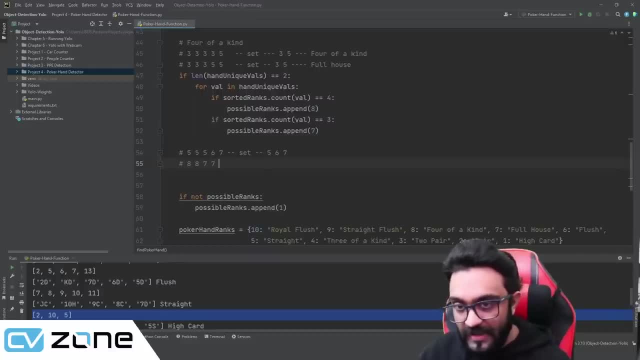 Then you have seven. seven, That's also a pair. And then you have three, let's say uh, or let's say two. So when you create a set of this, so you will have eight, seven and two. So how many unique values you have. Unique. 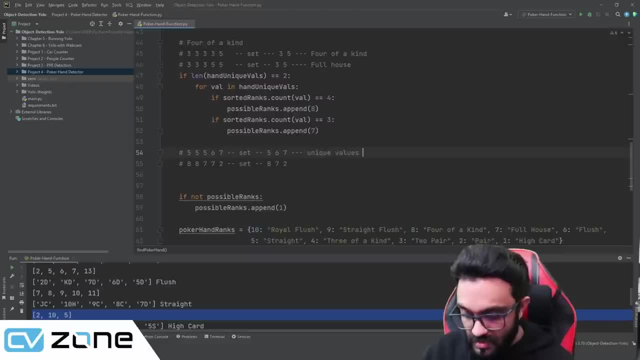 values are three. Also here, unique values equals three. So in both cases you will have eight, seven and two. So you will have eight, seven and two. So in both cases it's three. In this case it is uh, three of a kind. And in this case, 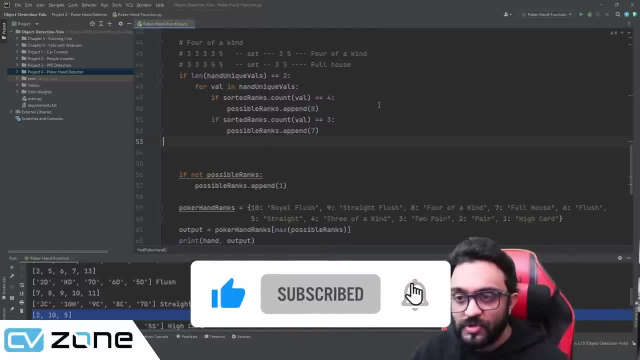 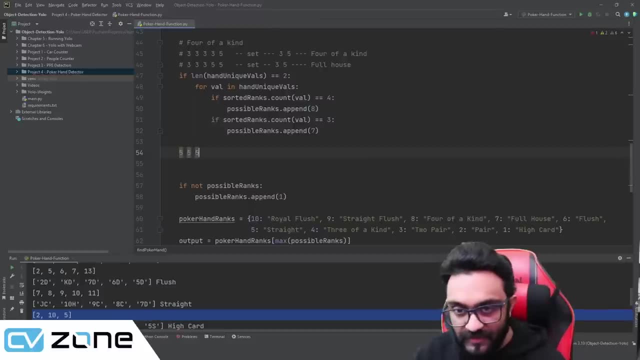 now we are going to three of a kind and two pair. so if let's say we have a three of a kind, so we will have five, five, five, five and five, and we will have, uh, let's say, six and seven, because if we have six, six, it becomes a full house. we are not talking about that, right? uh, we. 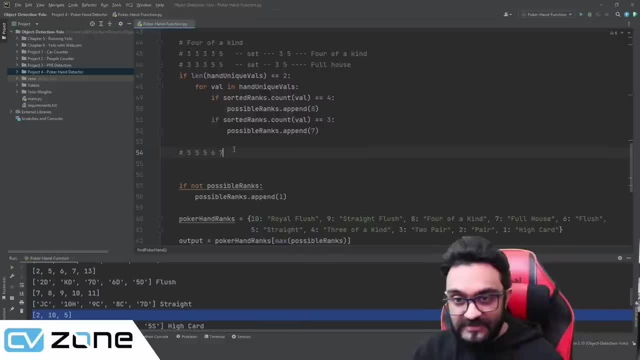 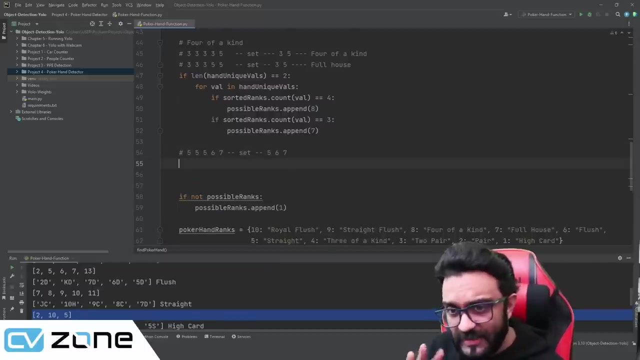 are not talking about that because we have already done that. so if it's six and seven, then it will give us how many unique values? it will give us three unique values, because when we send it to a set, the set will be five, six and seven, so it will give us three values. uh, we can also have three. 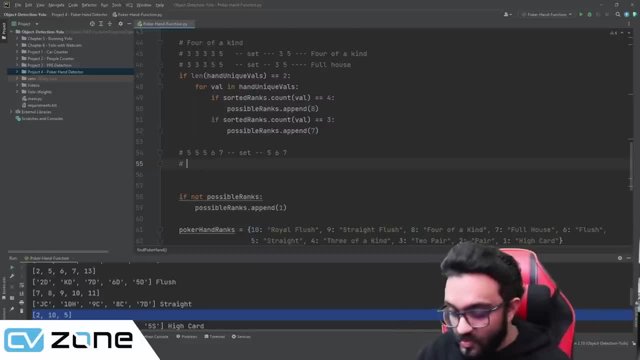 values in another scenario. what is that scenario? where you have, let's say, eight, eight, this is a pair. then you have seven, seven, that's also a pair, and then you have three, let's say, or let's say two. so when you create a set of this, so you will have eight, seven and two. 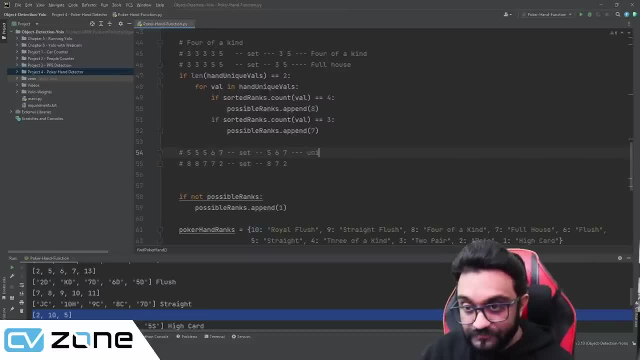 so how many unique values you have? unique values are three. also here you, unique values equals three. so in both cases it's three. in this case it is uh three of a kind, and in this case it is uh two pair right. so we need to check first of all if they are three, actually we can write. 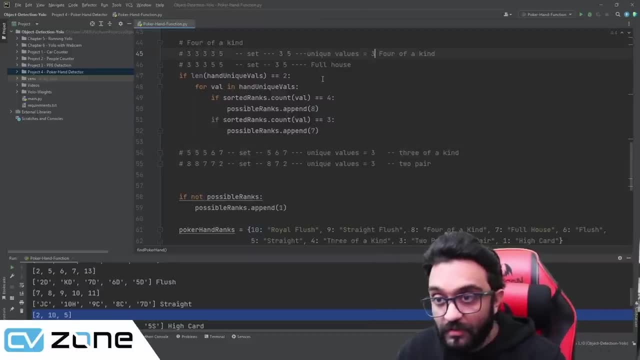 here as well. unique values are two and unique values are two. there you go. so four of a kind, full house and that okay. so here we need to check if the length of unique values is basically three. so here we are checking four of a kind and a full house. 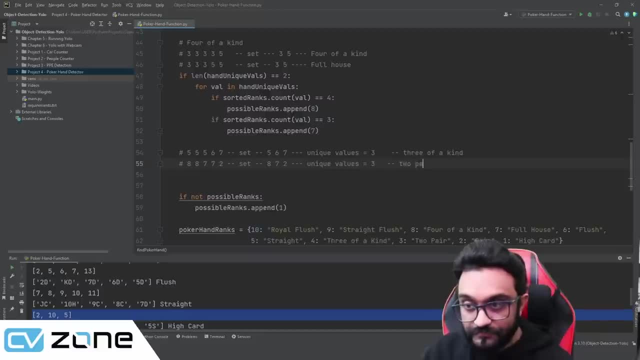 it is, uh, two pair, right. So we need to check first of all if they are three. Actually we can write here as well: Unique values are two And unique values are two. There you go, So four of a kind full house and that Okay. So here we need to check if the length 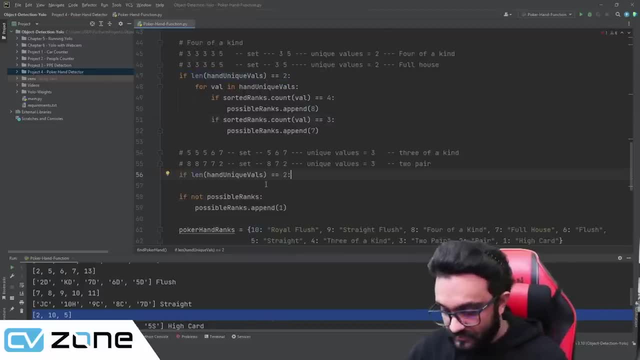 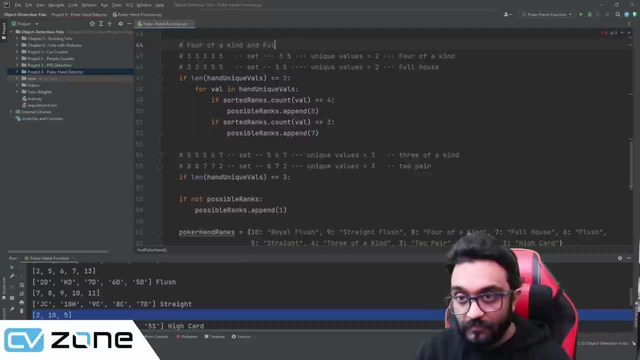 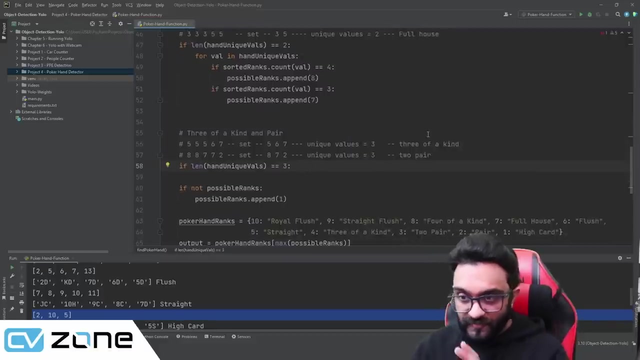 of unique values is basically three. So here we are checking four of a kind and uh, full house. Here we will be checking three of a kind and pair. There you go. So, uh, for both of them we first need to check the unique values. There are three. 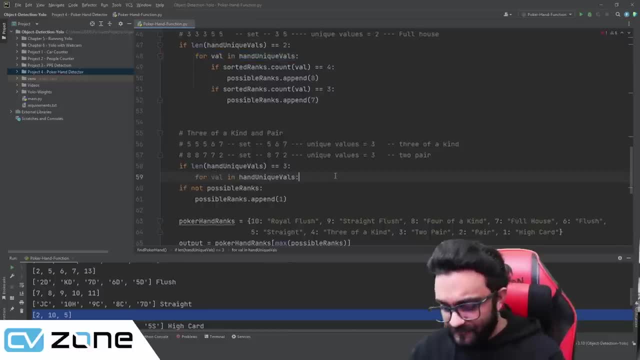 Then we will check the values. If the value comes, how many times We will loop through the value? And if the value comes, so here the value will come three times. So if the value comes three times, then it is a three of a kind, So a three of a kind. then it is a three of a kind, So a three of a kind. 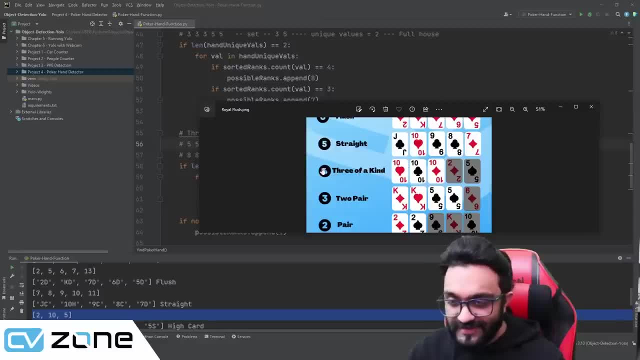 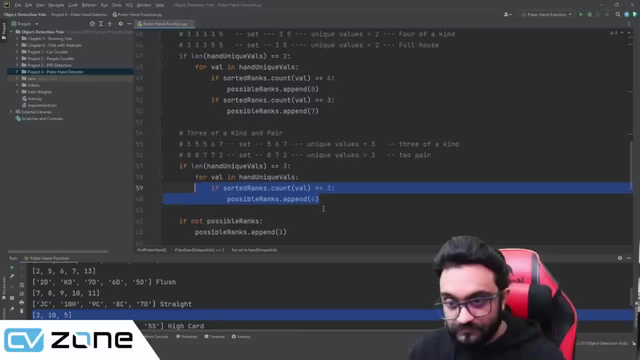 is 10.. It's not 10.. It's four. So the three of a kind is four, And if the value comes two times, which means here, for example, is 2 and here, for example, it's 2,- 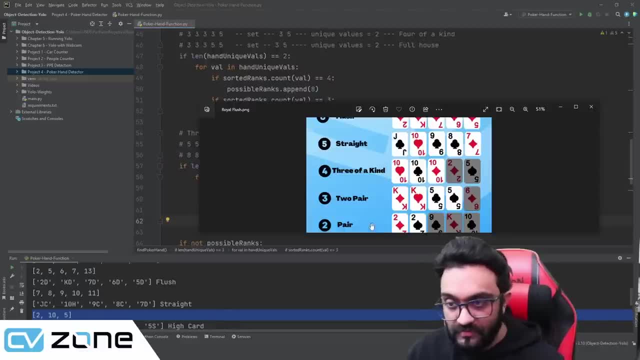 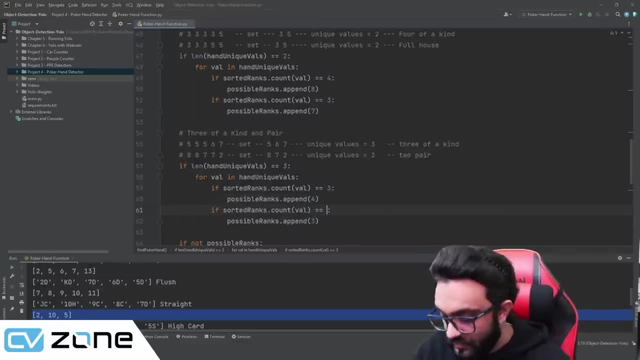 then it is a, then it is a two pair, which is three. There you go, Uh sorry, When it comes two times. So if it's three times and then there is a two pair, three times it is three of a kind. if it's two times it is two pair. we can write it here as well. 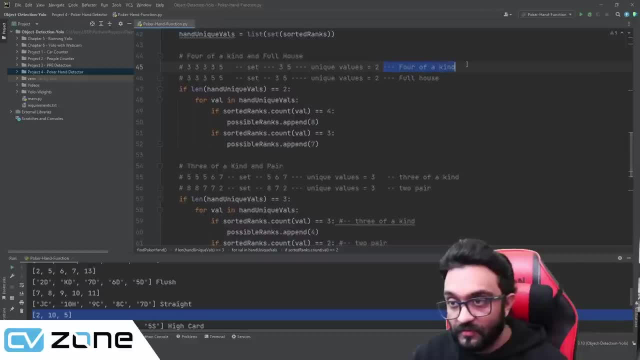 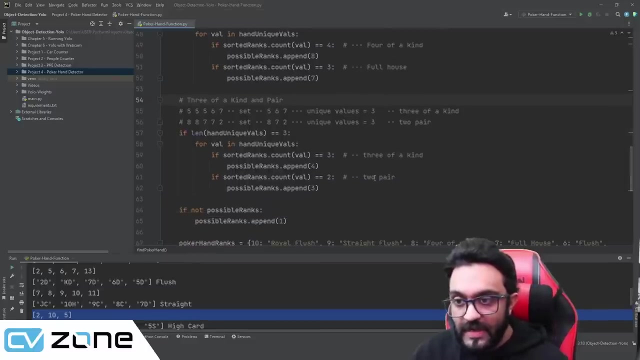 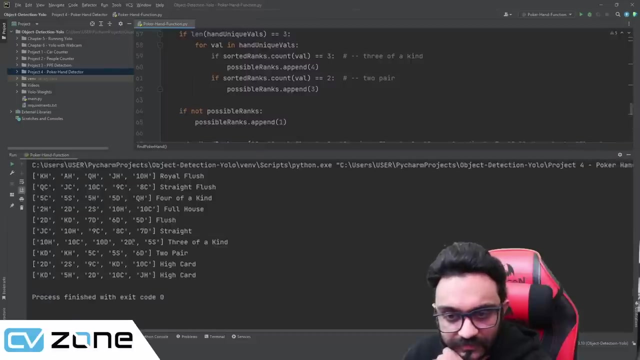 so it's easier to know what's going on here. also, we can write four of a kind, and this one is full house, so it's it's pretty easy. all you have to do is just think a little bit, how exactly can we do this? and i believe, uh, only one is left. let's run this first, and there you go. this is three of a. 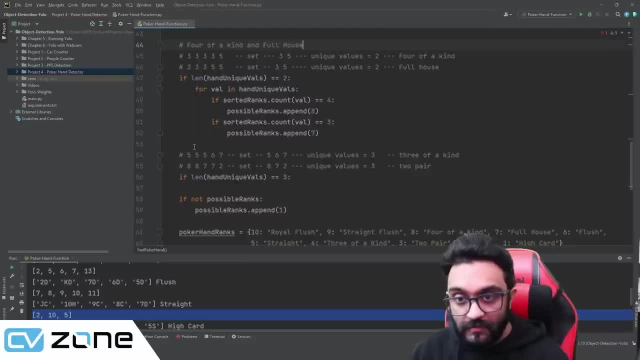 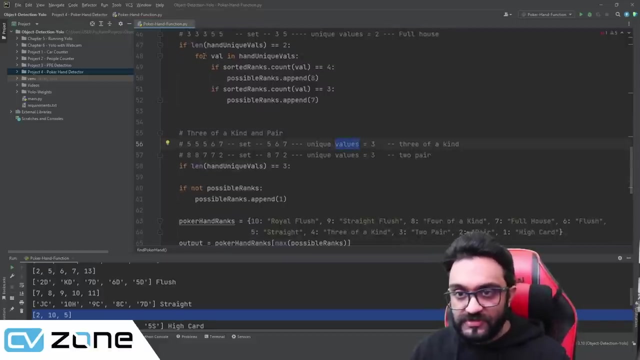 here we will be checking three of a kind and pair. there you go. so for both of them we first need to check the unique values. there are three. then we will check the values. if the value comes, how many times we will loop through the value and if the value comes, so here the value will come. three: 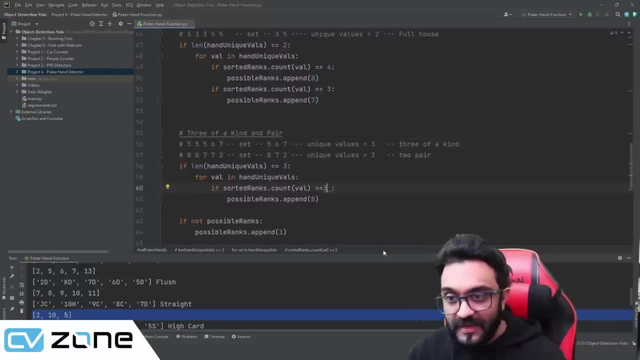 times. so if the value comes three times, then it is a three of a kind. so a three of a kind is ten, not ten, it's four. so three of a kind is four. and if the value comes two times- which means here, for example, is two, and here, for example, it's two- then it is a and it is a two pair. 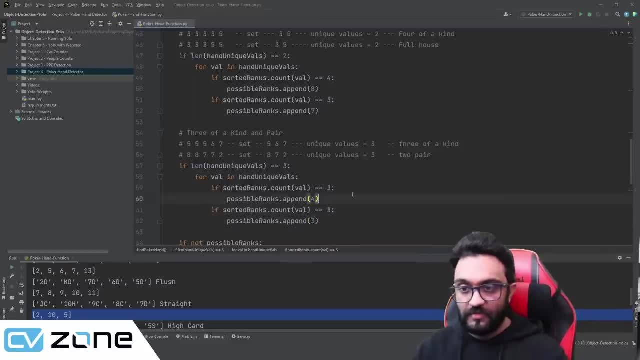 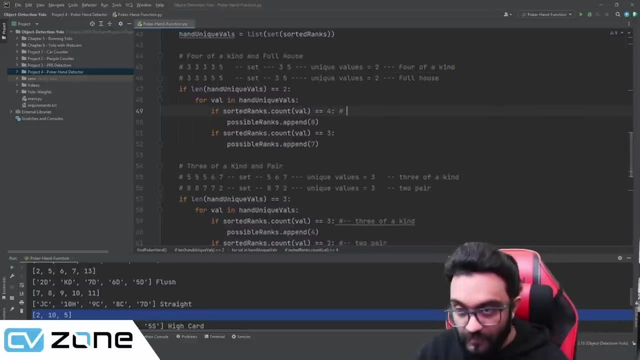 which is three. there you go, sorry when it comes two times. so if it's three times, it is three of a kind, if it's two times, it is two pair. you can write it here as well, so it's easier to know what is going on here. also, we can write four of a kind, and this one is full house, so it's it's pretty easy. 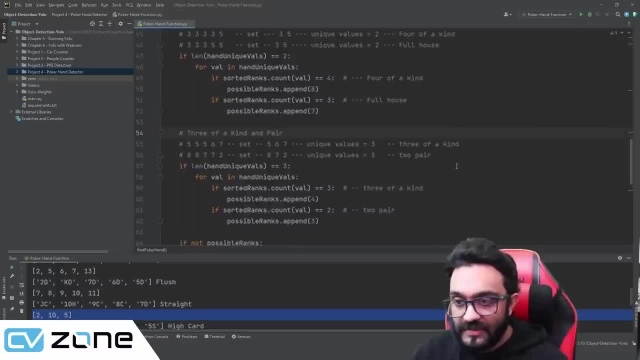 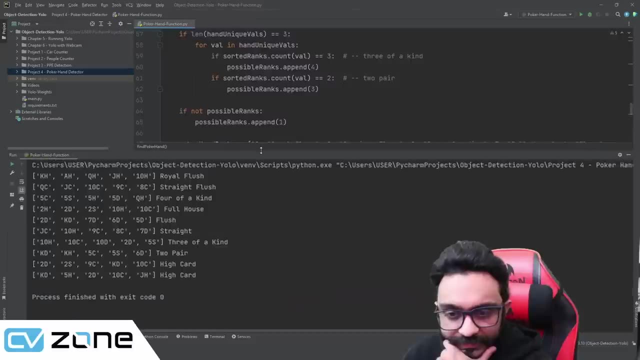 all you have to do is just think a little bit, how exactly can we do this? and I believe only one is left. let's run this first, and there you go. this is three of a kind, because we have ten, ten and ten and the other two are different, so it's not a full house, it's three of a kind. 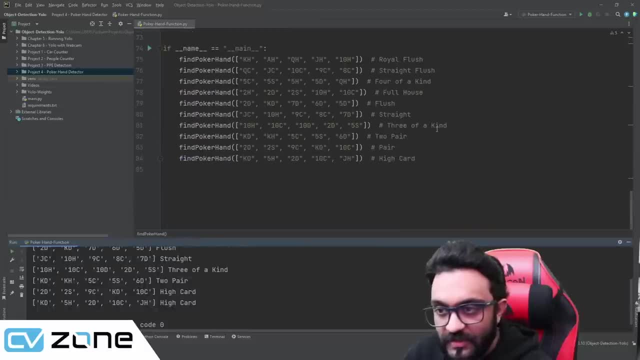 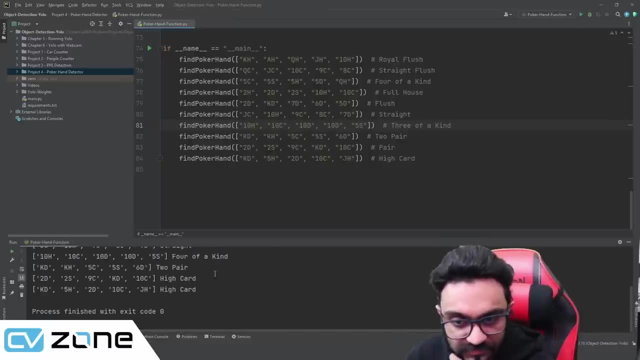 and uh, actually, let's change it to full house here. three of a kind will make it full house. uh, if we write here 10 as well, let's see if it detects as a full house. there you go. so where is it full house? there you go. no, full house is here. and then it's a four of a kind. sorry, I made. 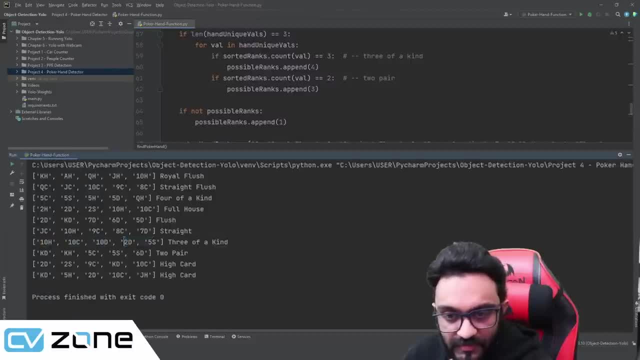 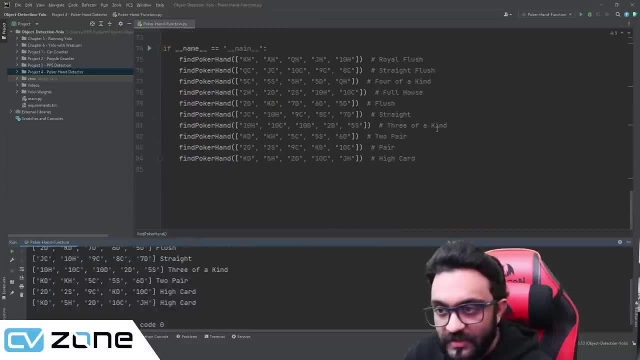 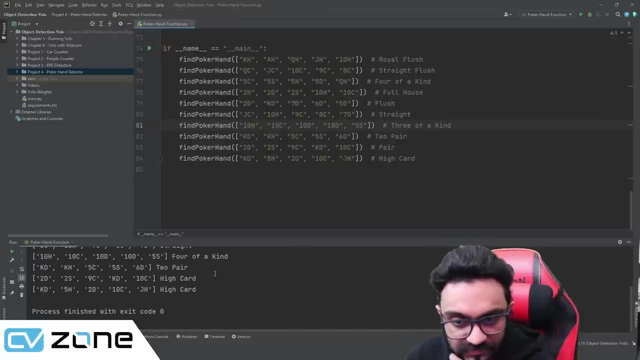 kind, because we have 10, 10 and 10 and the other two are different. so it's not a full house, it's three of a kind. and uh, actually, let's change it to full house here. three of a kind will make it full house. uh, if we write here 10 as well, let's see if it detects as a full house. there you go, so where? 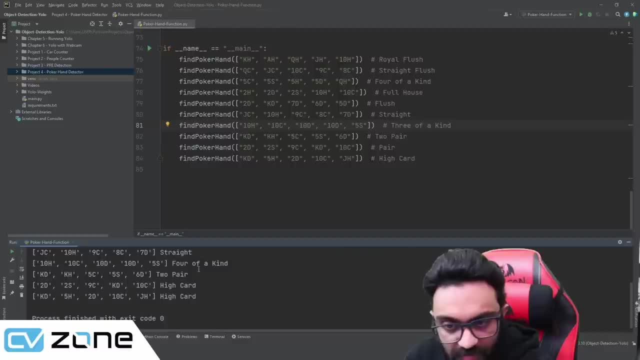 you go: no, full house is here, and then it's a four of a kind. sorry, i made it four of a kind, my bad. uh, i wanted to make it full house, which means this is 2d, so this will be also 2d. my bad, so this will. 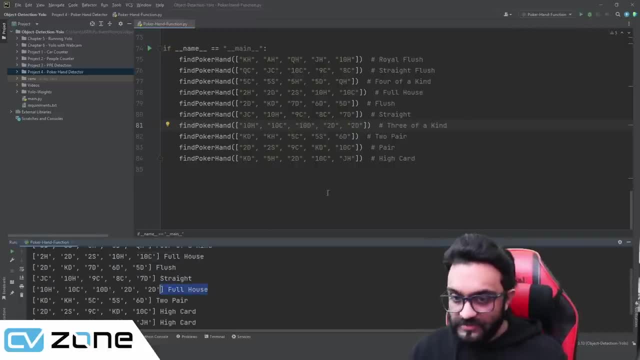 become a full house. there you go see. now it's a full house, it means our methodology is working fine. so we have three of a kind working properly. then we have two pair. so king king is working fine. five, five, that is a two pair, excellent. so now we have these, uh, unique values, and then 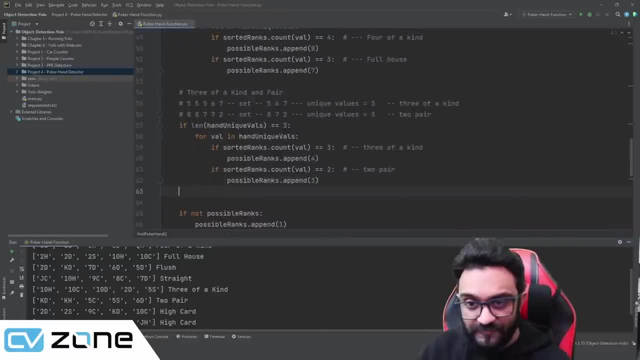 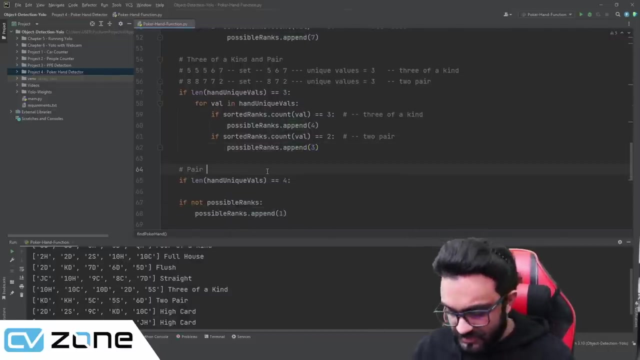 the last one is very simple. um, we are checking for a pair. pair is simply when you have four values. so, for example, you have- let me share an example here- so you have five, five and then three, six, uh, seven and eight. so the set of this. did i write more? i think yeah. so the set for this. 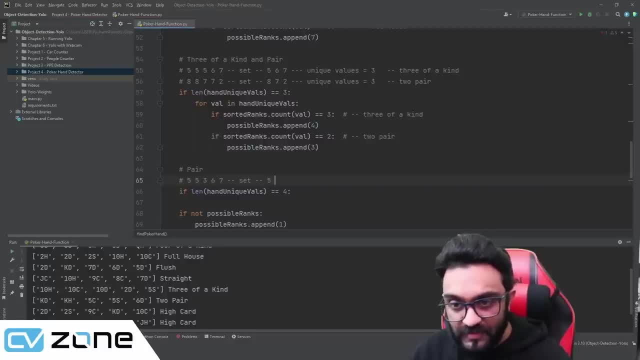 will be five, five, uh will be five, three, five, three, six and seven, which are four. unique. unique values equals four, which means a pair. that's how simple it is. so, um, you will simply write possible rank dot append and you will write two, because one is already there and that is your high card. so if we run this now and 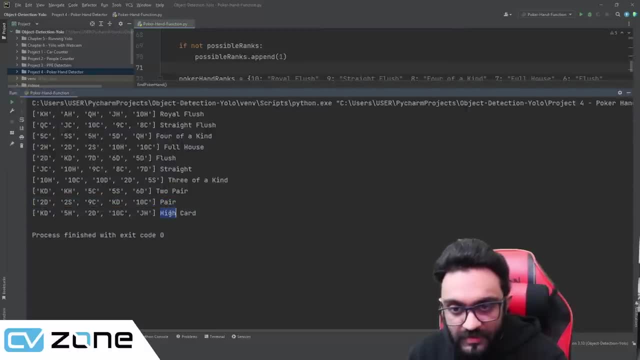 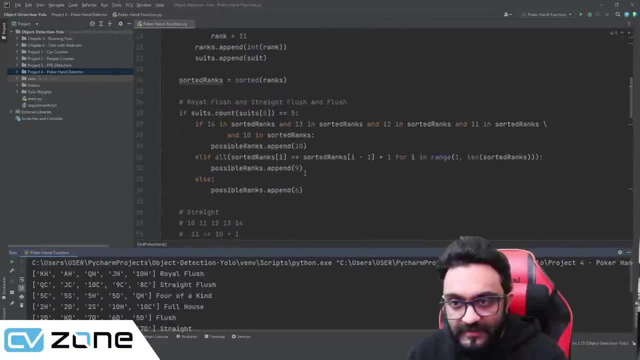 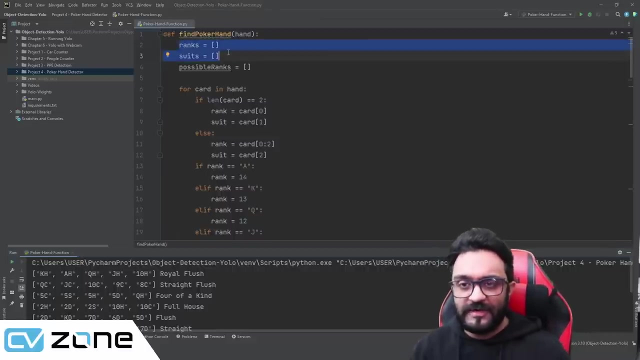 we go down and there you go. so here you are getting a pair, here you're getting a high card. so this is basically how we can um get these values. so, to repeats, or to summarize what we have done, we have first of all extracted the ranks and the 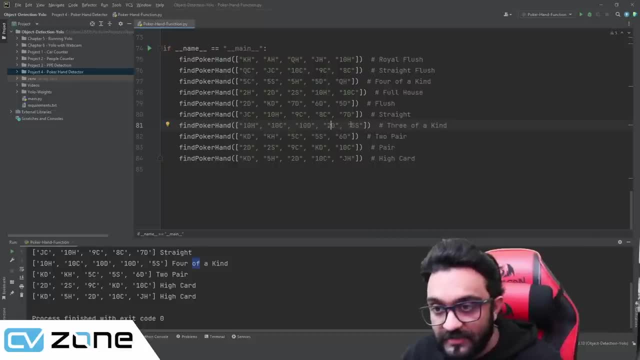 it four of a kind my bad. uh, I wanted to make it full house, which means this is 2D, so this will be also 2D, my bad. so this will become a full house. there you go see. now it's a full house. it means our. 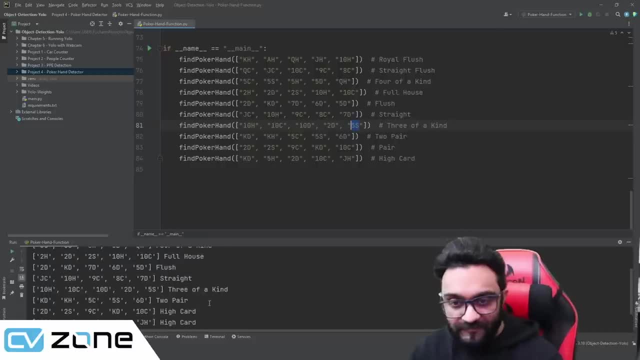 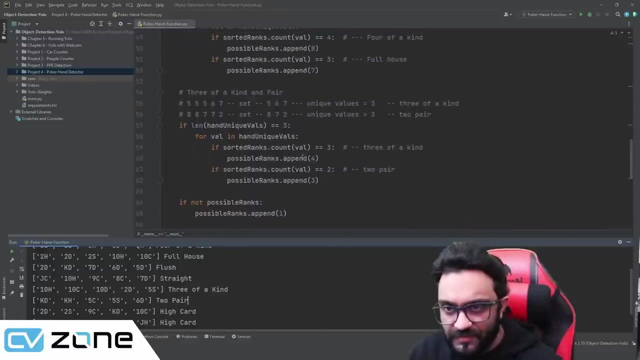 methodology is working fine, so we have three of a kind working properly. then we have two pair, so king, king is working fine. five, five, that is a two pair. excellent. so now we have these, uh, unique values. and then the last one is very simple. um, we are checking for. 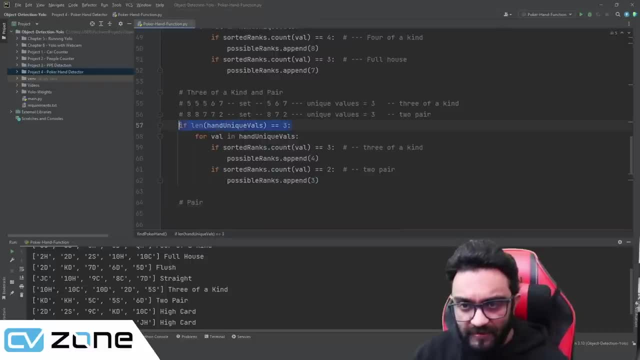 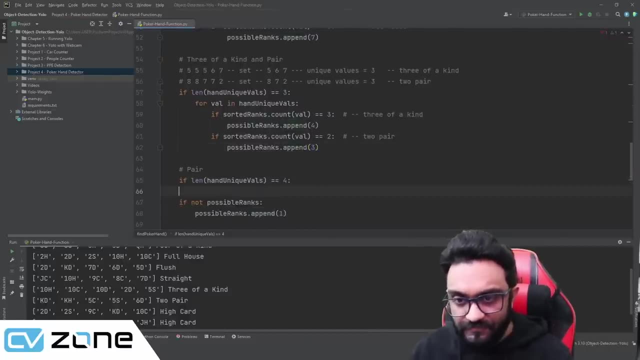 a pair. pair is simply when you have four values. so, uh, for example, you have- let me share an example here. so you have five, five, and then three, six, uh, seven and eight. so the set of this? did I write more? I think yeah, so the set for this will be five, five, uh will be five. 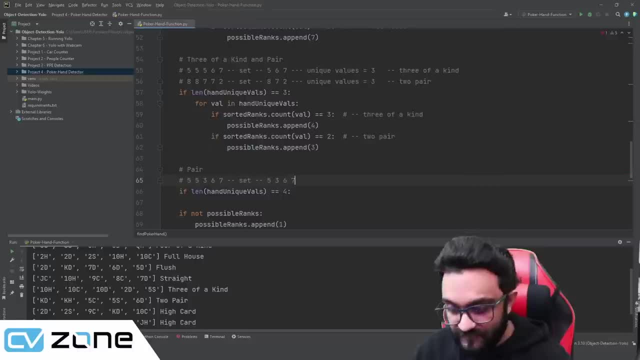 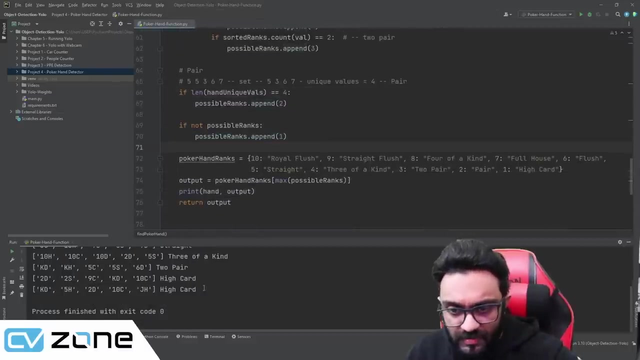 three, five, three, six and seven, which are four unique. unique values equals four, which means a pair. that's how simple it is. so, um, you will simply write possible rank dot append and you will write two, because one is already there. that is your high card. so if we run this now and we go down, and there you go. so here you're getting. 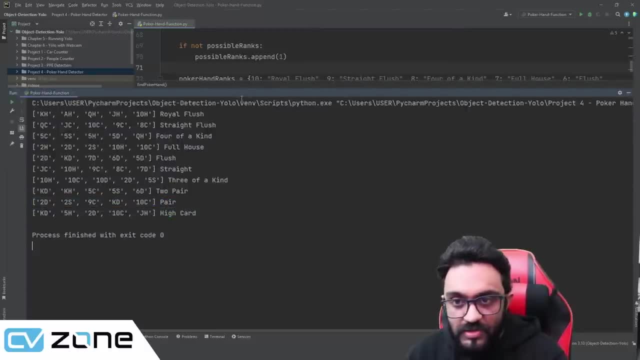 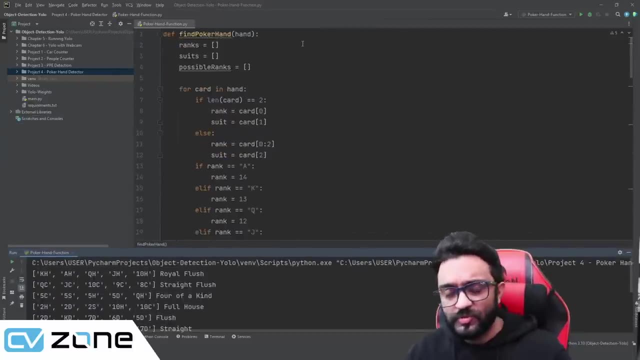 a pair. here you're getting a high card. so this is basically how we can um get these values. so, to repeats, or to summarize what we have done, we have first of all extracted the ranks and the suits and we have created a variable called possible ranks. uh, not a variable, a list in which we will. 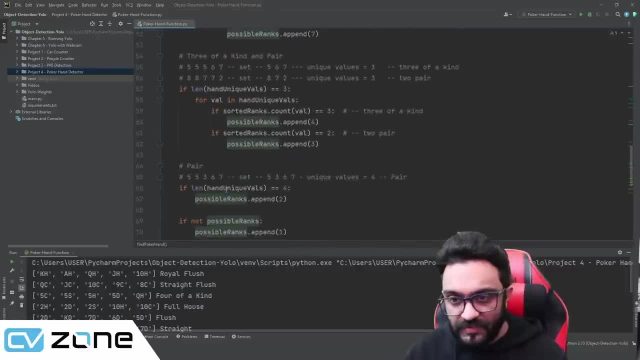 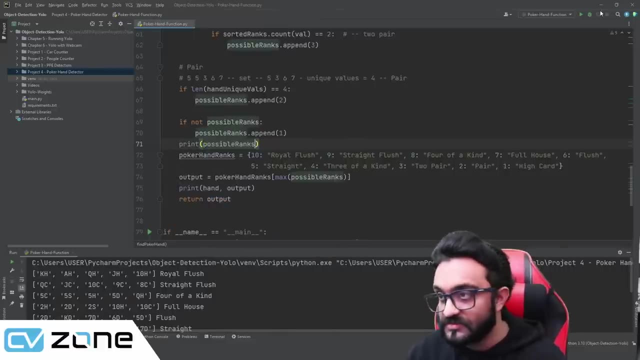 store all those uh ranks. uh, actually, let's print out the possible ranks, uh, before we uh print possible racks, and let's see if there are more than one. yeah, here you can see it's three, three, uh, both of them are three, so it's nine and five. so it is also a flush and it is also a. 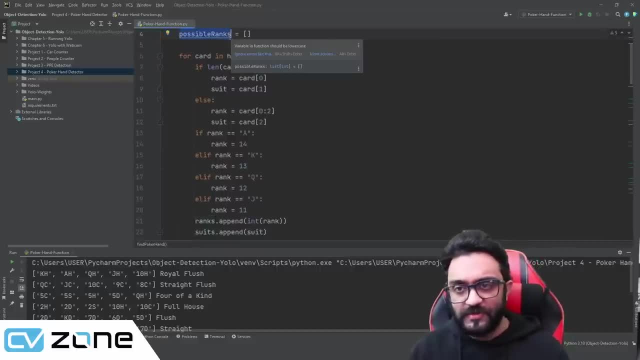 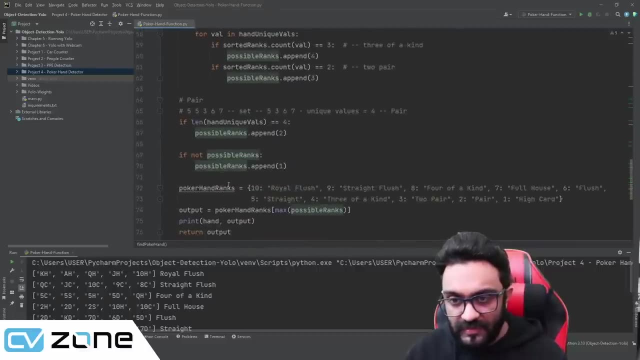 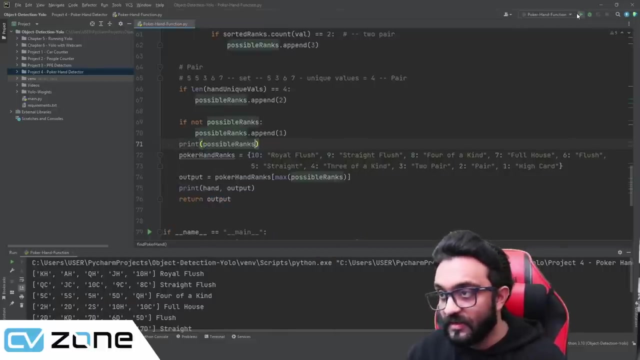 suits and we have created a variable called possible ranks, not a variable, a list in which we will store all those ranks. actually, let's print out the possible ranks before we print possible ranks, and let's see if there are more than one. yeah, here you can see, it's three, three. 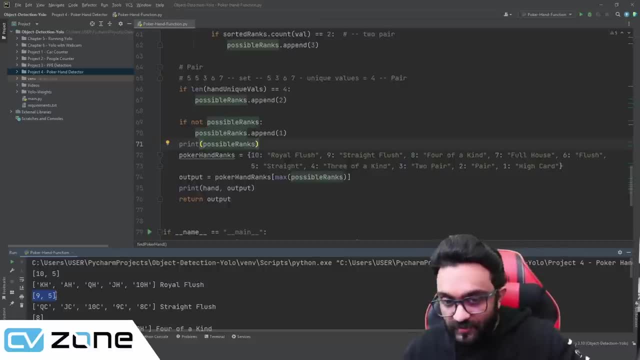 both of them are three, so it's nine and five, so it is also a flush and it is also a straight, so yeah, and then it is both of them together, so it's straight flush. and then here you have four for kind, so the rest of them, they don't have multiples. 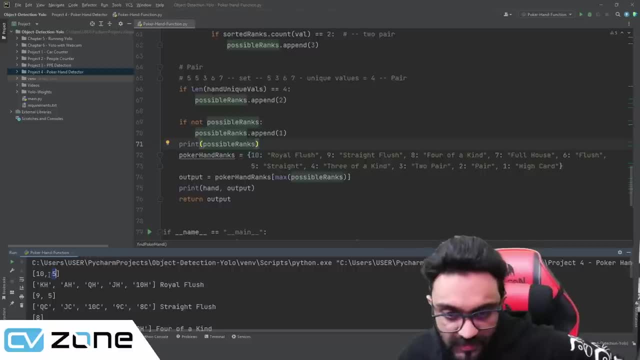 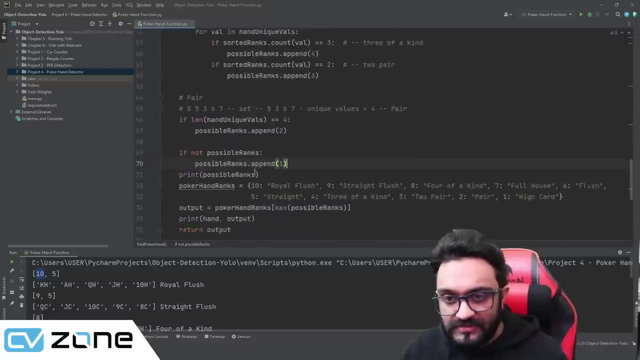 but this one has multiple as well, uh, because it is a flush as well and it is, uh, a royal flush as well, so it will take the bigger one, which is royal flush. so, yeah, that's the idea. and then, uh, as we were mentioning, so you extract. oh, so you know what to do with multiple. you extract on a 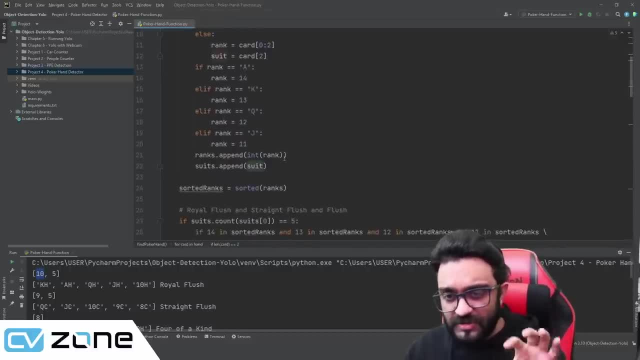 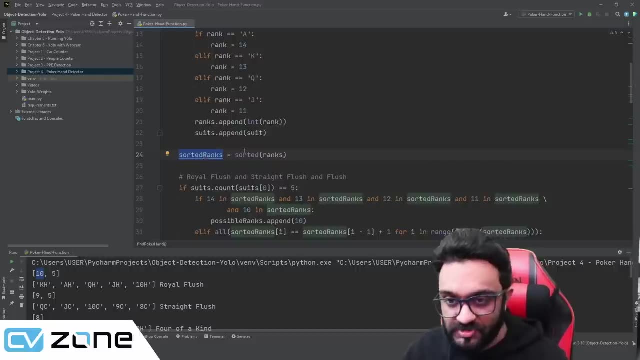 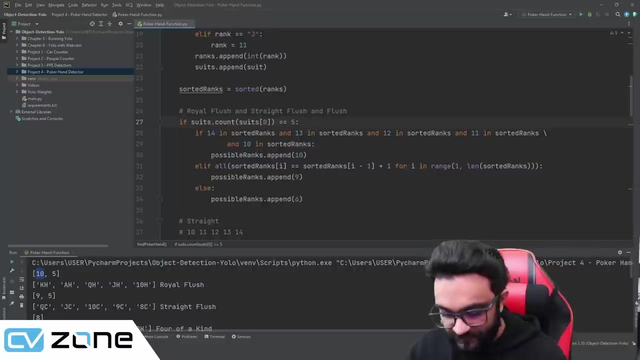 all the ranks and all the suits. once you have them in lists, you sort them, because sorting them will make it easier, especially when you are finding the straight. that will make it much easier. so you will first check for the royal flush. no, you will first check for the flush, so check. let me write here. 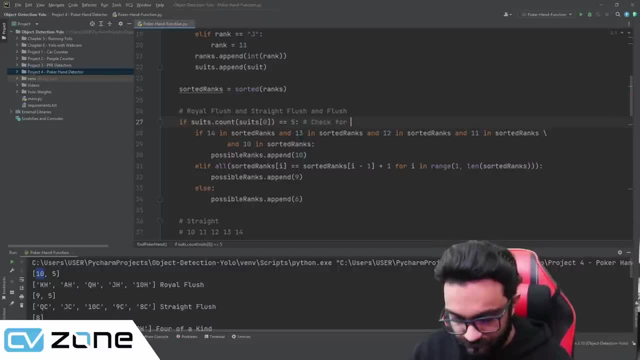 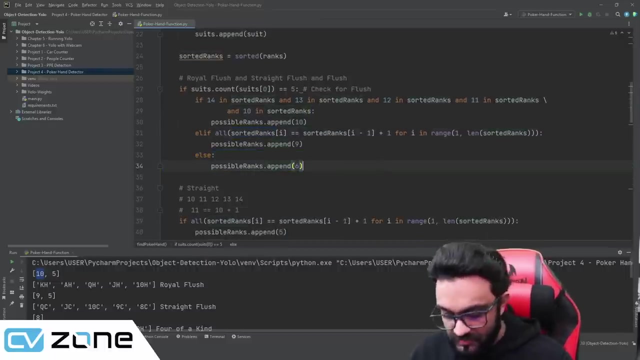 check for flush and then it will check for royal flush over here and then it will check for straight. if it is flush and it is royal, then it will be royal flush. if it's flush and it is straight, then it is straight flush. otherwise it will be simply flush. so this is flush, basically. 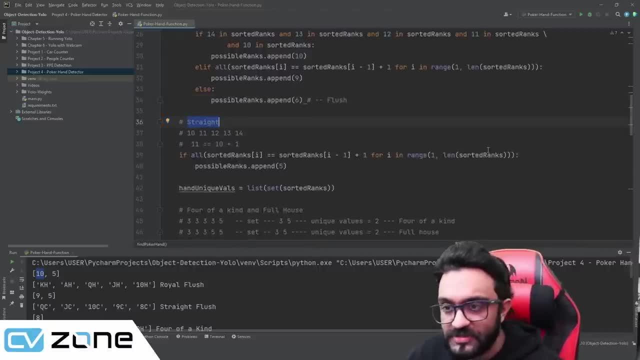 then we have straight in straight. what we are doing is we are we are checking the previous value and we are adding one to it and comparing it with our current value. so 11 is being compared with 10 plus 1, 12 is being compared with 11 plus 1. if all of them give us true value, if they are same, then it 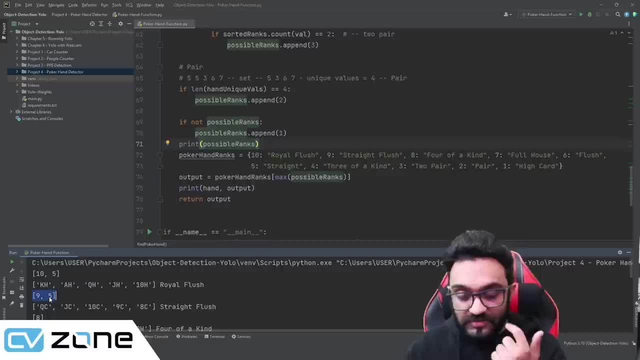 straight, so, uh, and then it is both of them together, so it's straight flush, um, and then here you have four of a kind, so the rest of them they don't have multiples, but this one has multiple as well, uh, because it is a flush as well and it is a royal flush as well, so it will take the bigger one, which is royal flush. 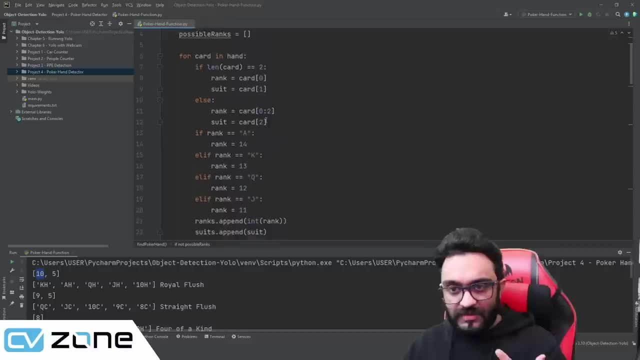 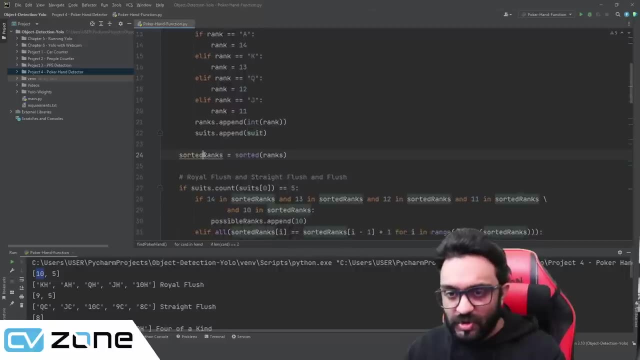 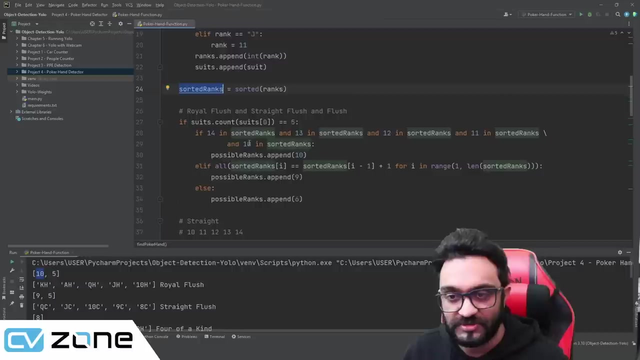 so, yeah, that's the idea. and then, uh, as we were mentioning. so, you extract all the ranks and all the suits. once you have them in lists, you sort them, because sorting them will make it easier, uh, especially when you are, uh, finding the straight, that will make it much easier. so you will. 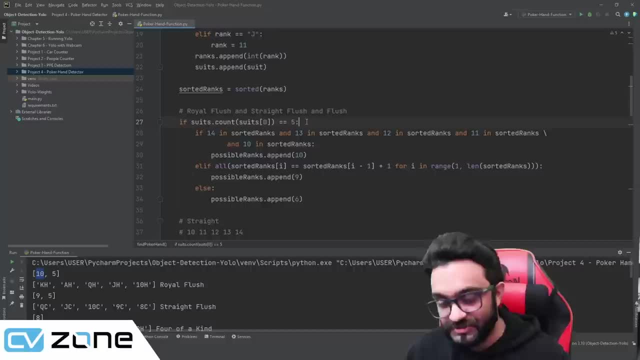 first check for the royal flush. uh, no, you will first check for the flush, so check. let me write here: uh, check for blush, and then it will check for royal flush over here and then it will check for straight. if it is flush and it is royal, then it will be royal flush. if it's flush and it is. 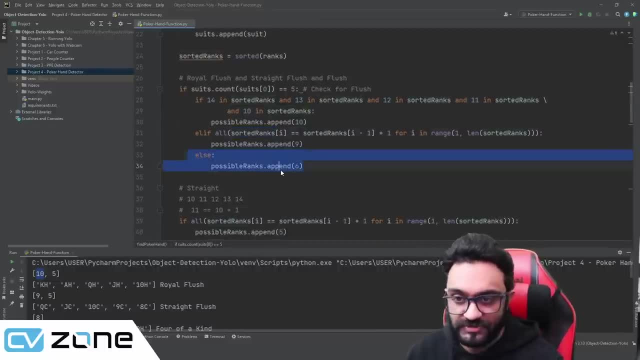 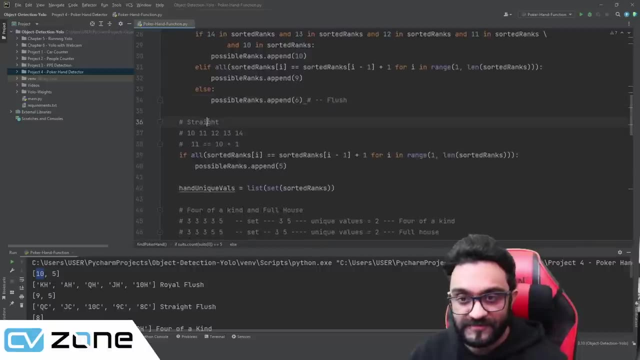 straight, then it is straight flush, otherwise it will be simply flush. so this is flush. basically, then we have straight in straight. uh, what we are doing is we are we are checking the previous value and we are adding one to it and comparing it with our current value. so 11 is being compared with 10. 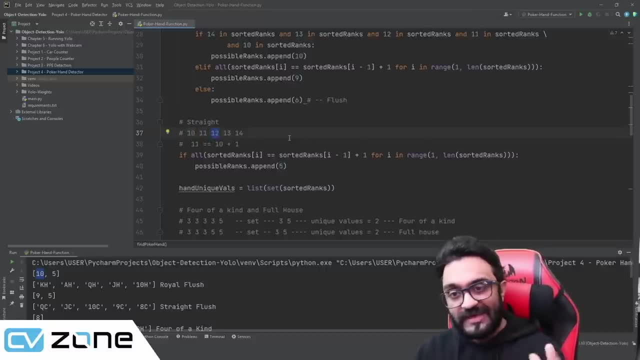 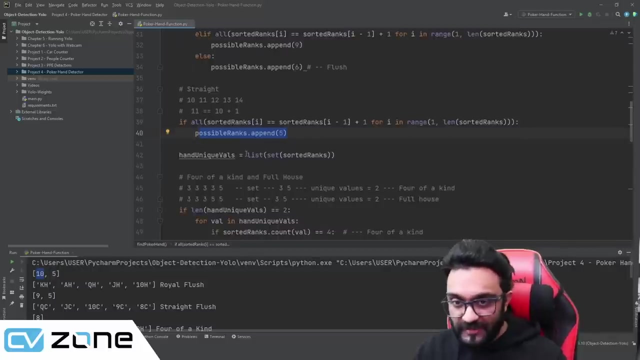 plus 1, 12 is being compared with 11 plus one. if all of them give us true value, if they are same, it becomes all of them are consecutively listed and ranked. so that's why we will write it as straight. then comes the unique values. so we will check the unique values by putting a set. 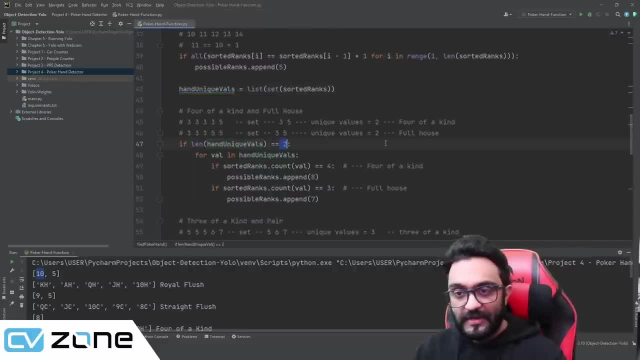 to the sorted ranks. if the unique values are two, it can have two possibilities: four of a kind or full house. if one of the values has four uh counts, then it is a four of a kind. if one of the values has three counts uh, then it is full house. same way we are checking the unique values. 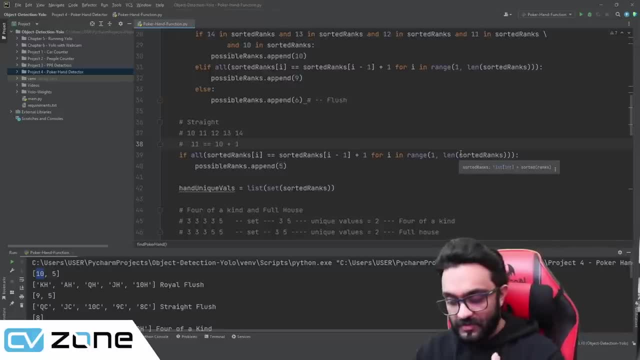 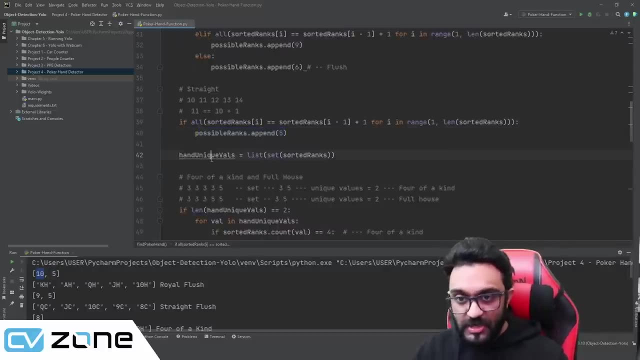 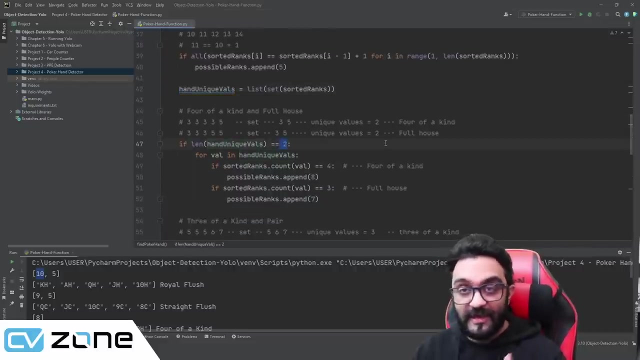 becomes. all of them are consecutively listed and ranked, so that's why we will write it as a straight. then comes the unique value. so we will check the unique values by putting a set to the sorted ranks. if the unique values are two, it can have two possibilities: four of a kind or full house, if one of the values has four. 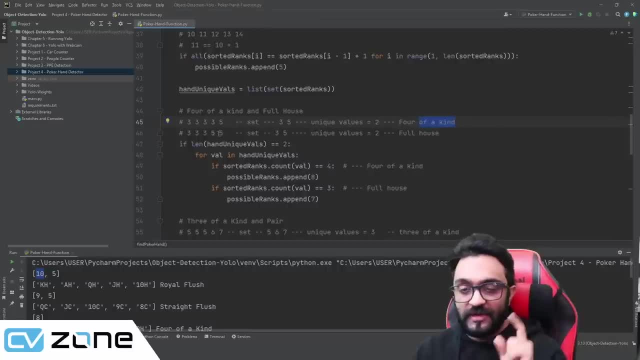 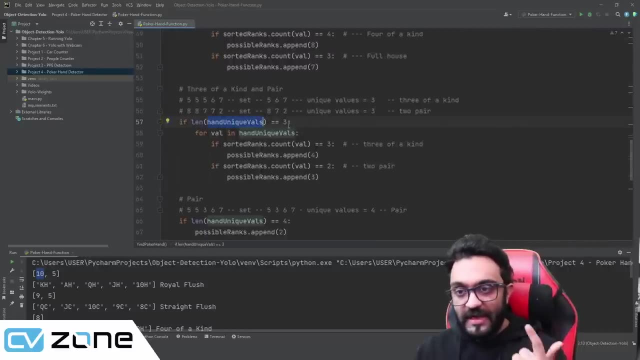 uh counts, then it is a four of a kind. if one of the values has three counts, uh, then it is full house. same way, we are checking the unique values, and if the unique values are three, there are two possibilities. one of them is three of a kind if 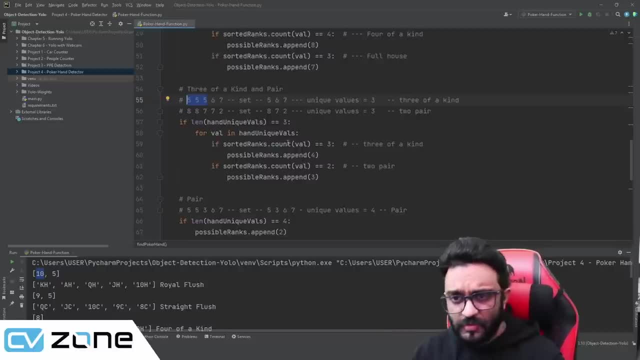 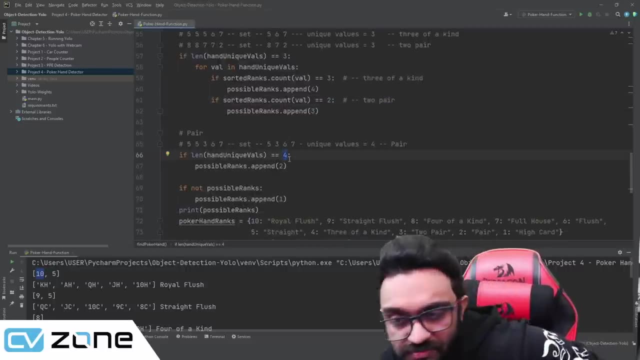 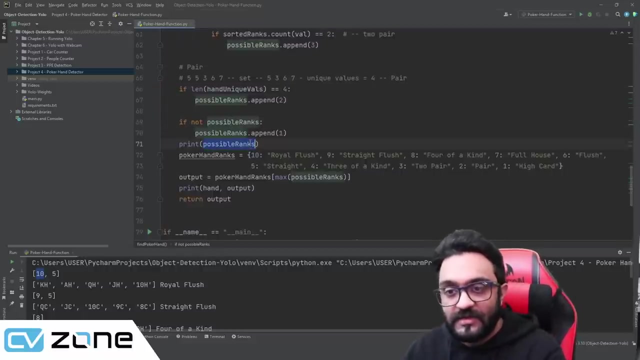 uh, the value uh has the count of three, and if the value has a count of two, it means it's two pair, and then, if it's single pair, then the unique values, the set, will have a count of four, and if, if nothing else works out, then it is um high card. and once that, once all of that is done, we. 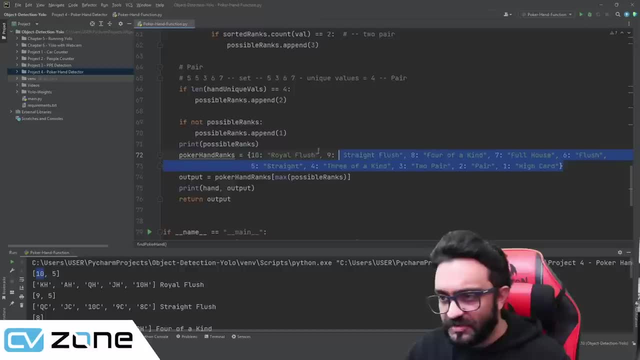 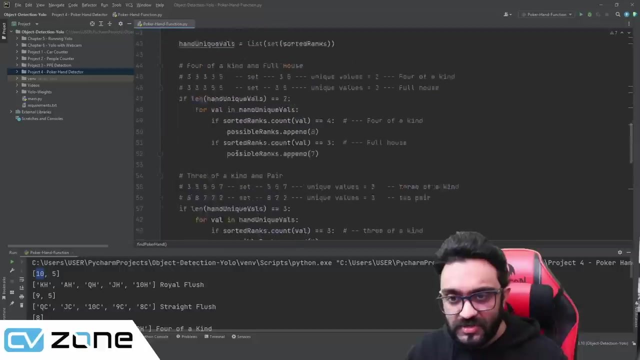 have our uh- what do you call? dictionary, with all the rankings and the numbers, and then from that we uh extract. what output do we get? what is our result? so let me, let me, remove all the prints so that it is neat and clean. we don't want, uh, too many things printed. 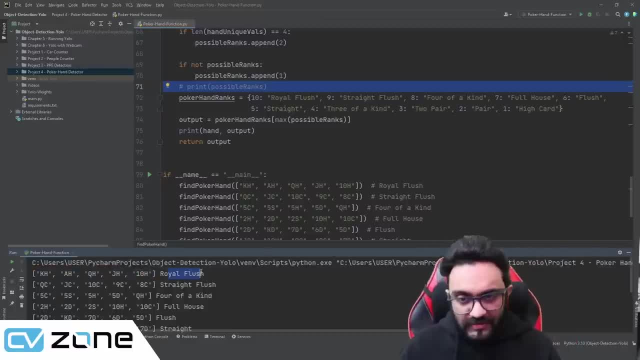 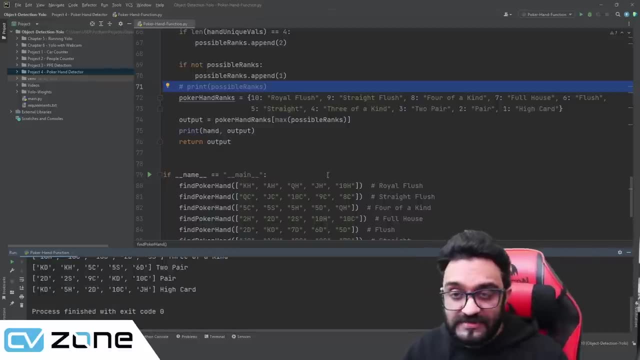 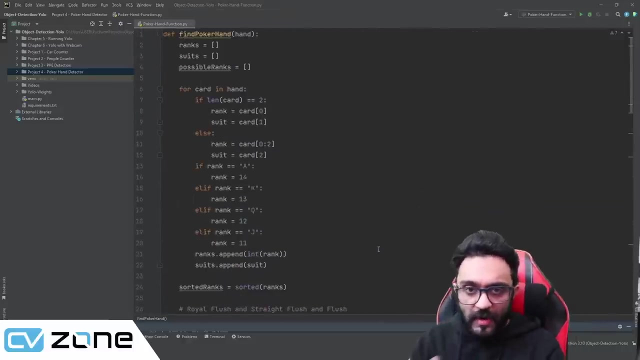 yeah, so then we only have the hand and what it is, uh, detected as so royal flash, straight flash four of a kind, two pair and so on. so this is basically how we can classify our poker hand and Now, once we have written this code, now we can go and use our trained model to find. 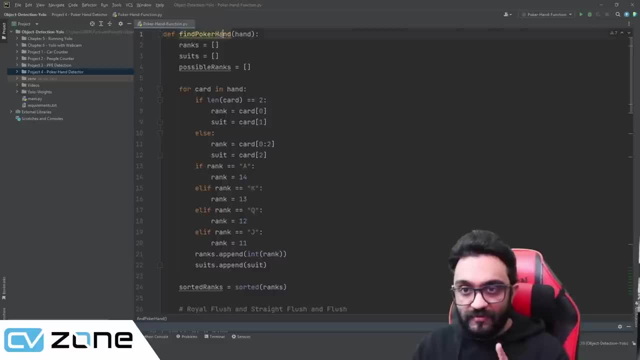 to detect that hand, and then we will send it to our find poker hand and it will give us the output of what type of hand it is. So let's go ahead and do that. Okay, so now our process has been completed. 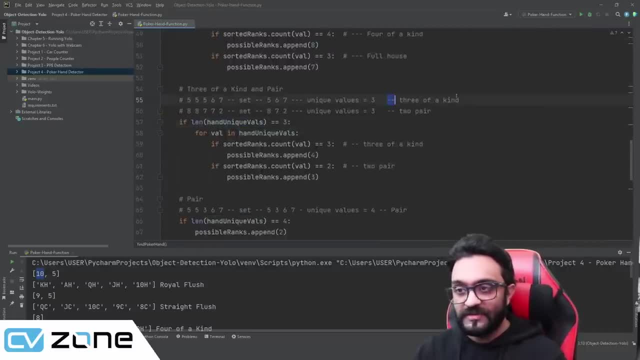 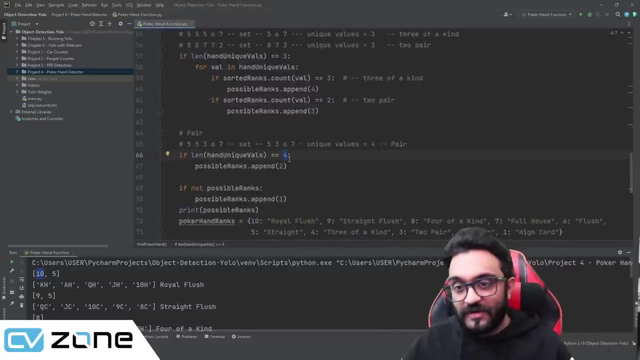 and if the unique values are three, there are two possibilities. one of them is three of a kind. if the value uh has the count of three, and if the value has a count of two, it means it's two pair, and then if it's single pair, then the unique values, the set will have a count of four. and 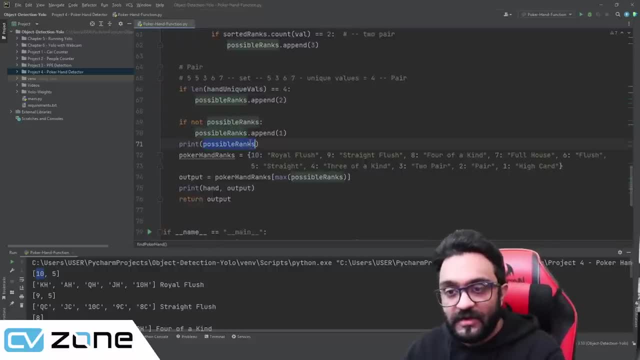 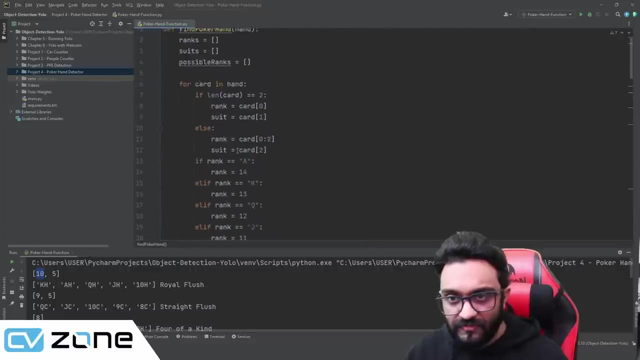 if, if nothing else works out, then it is: uh, high card. and once that, once all of that is done, we have our uh- what do you call? dictionary with all the rankings and the numbers, and then from that we extract. what output do we get? what is our result? so let me, let me, remove all the prints. 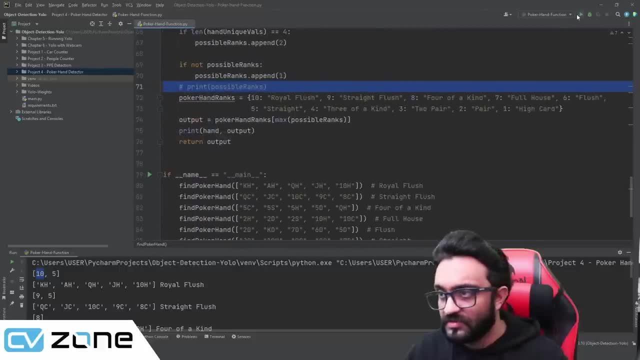 so that it is neat and clean. we don't want, uh, too many things printed. yeah, so then we only have the hand and what it'll let us do is, if we all, uh, to learn our code, we also need to know what actually allow the keyras out of the world. and then copy that and, yes, print and enter our code, and this is. 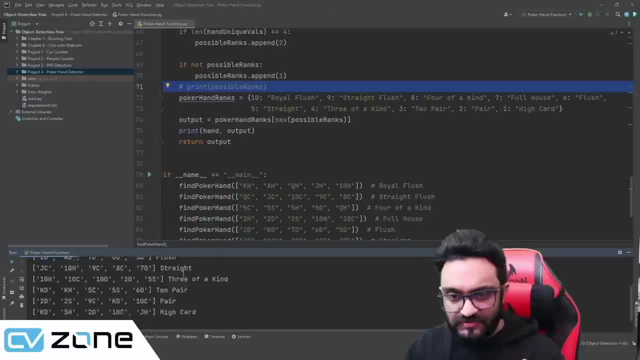 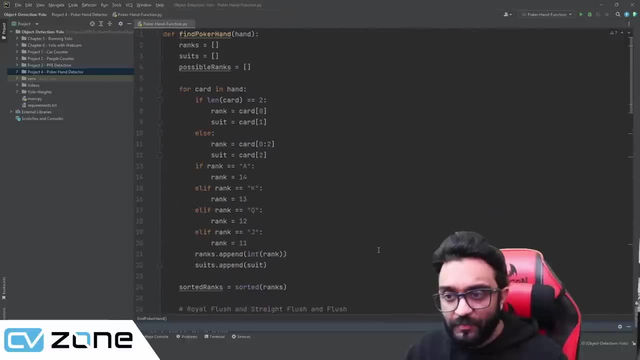 is detected as so royal flush, straight flash for of a kind to pair, and so on. so this is basically how we can classify our poker hand and now we, once we have written this code, now we can go and use our trained model to find, to detect that. 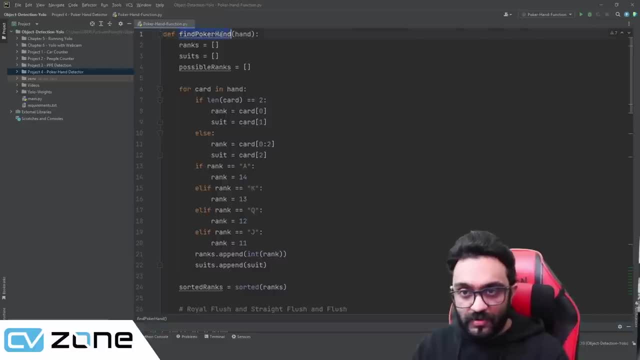 hand and then we will send it to our find poker hand and it will give us the output of what type of hand it is. so let's go ahead and do that, okay? so now our process has been completed, the training is done and we had 50 epochs. 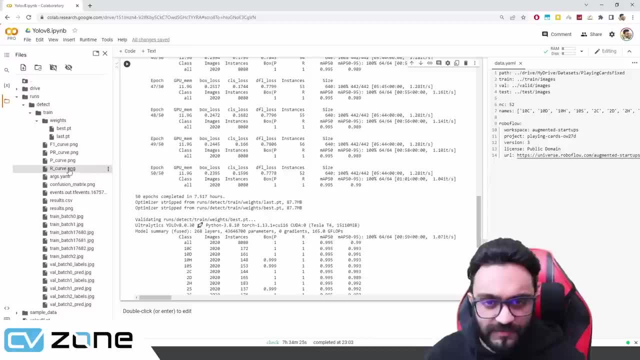 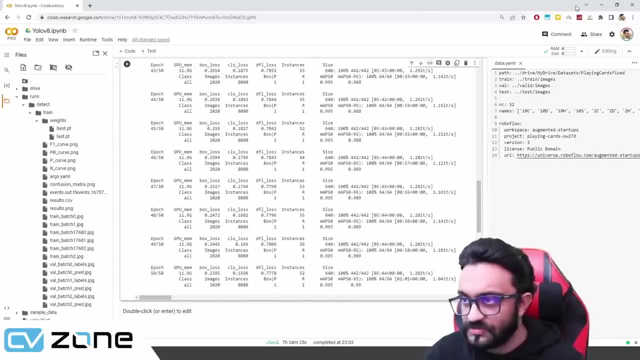 completed in 7.5 hours. so for further details, you can look at the precision and recall curves, and we also have the confusion matrix and all these training and validation but batches. so what we will do now is we will download the best one and we are going to use that in. 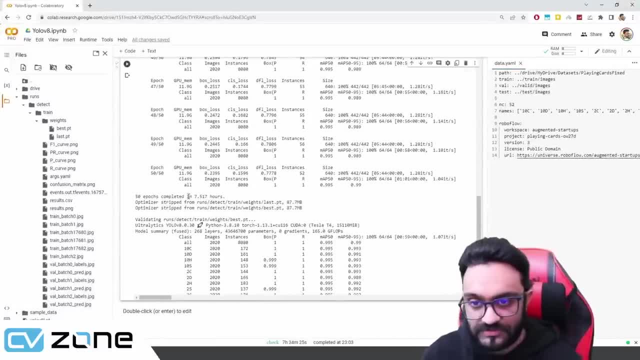 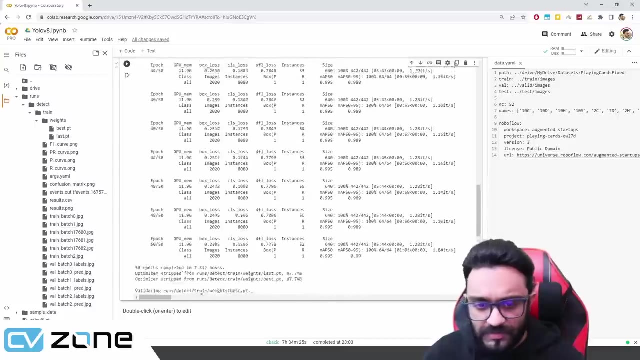 The training is done and we had 50 epochs completed in 7.5 hours. So for further details, you can look at the precision and recall curves, and we also have the confusion matrix and all these training and validation batches. So what we will do now is we will download the best one and we are going to use that. 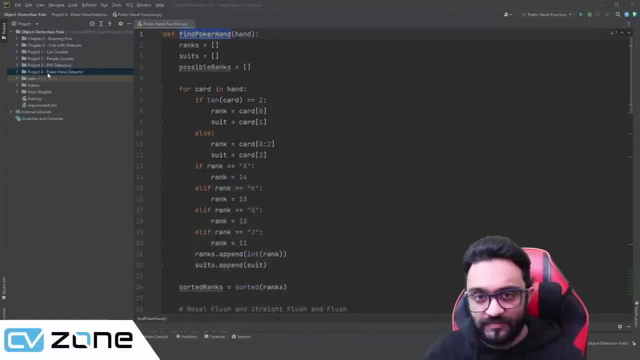 in our project. So we already have project 4 listed and we have created our poker hand function, and now what we will do is we will copy YOLO webcam, because we will be using our webcam to run it. So we will simply. 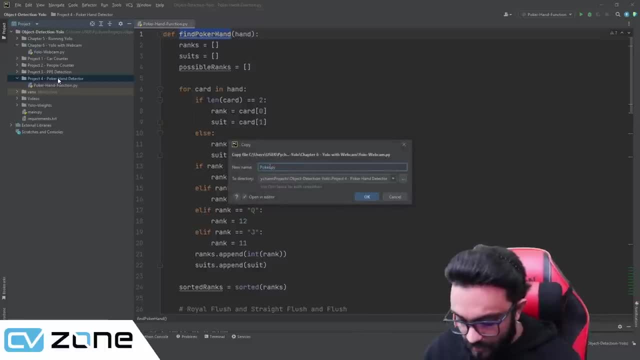 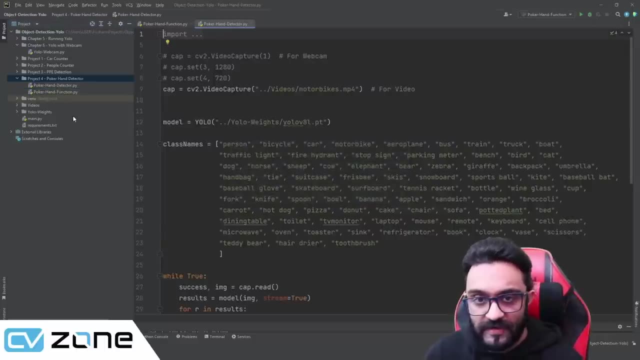 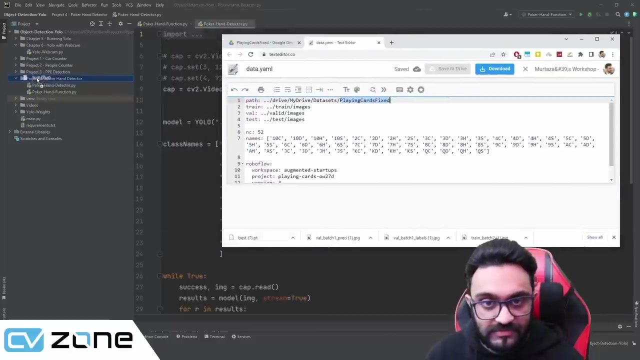 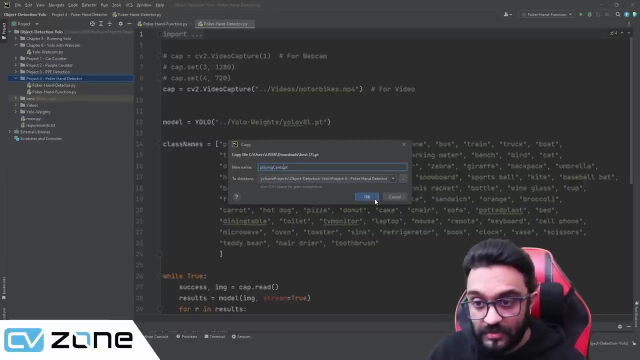 Copy that and we will name it poker hand detector. So once we have that, we will bring in our model. So here you can see, this is best 7.. So let's drag that in and we will call it playing cards, dot, PT. and over here now we. have to make the changes, So we will call it playing cards dot, PT and over here. now we have to make the changes, So let's drag that in and we will call it playing cards dot, PT and over here now we. 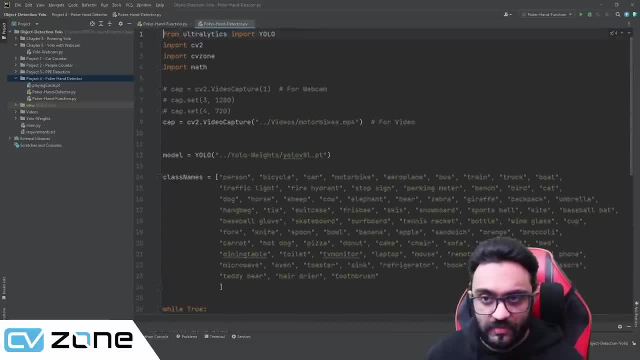 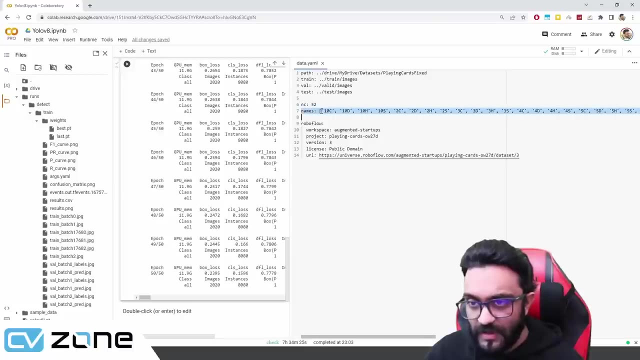 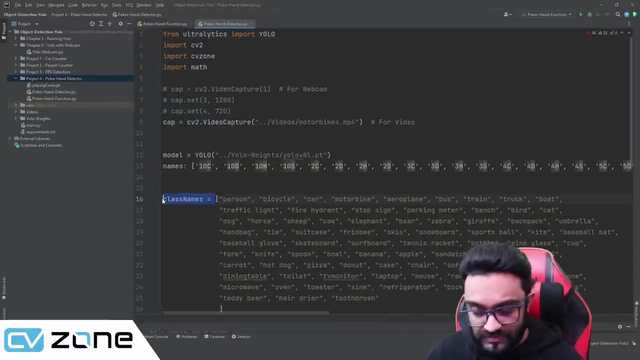 have to make the changes So that it detects these. So first of all, the class names we need to change, So to change that we can go back to our data dot YML file and we can copy all the names and we can simply paste them here. and we can just cut this and paste it here. 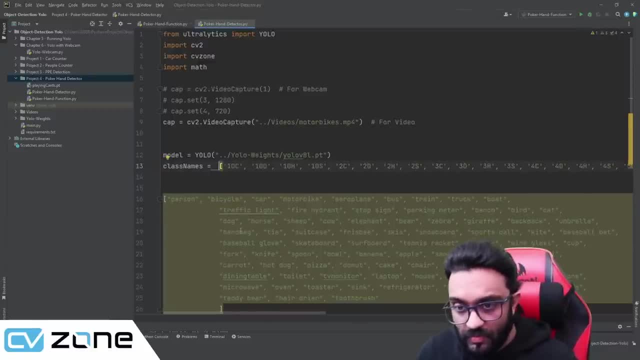 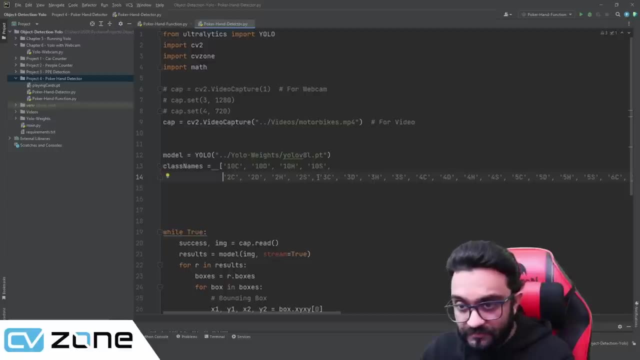 There you go. So to make it easier to understand what's going on, and we have all the classes- we can simply press enter after each of the ranks are done. So after two is done, then three, four, five, six, seven, eight, nine, ace, jack, king and. 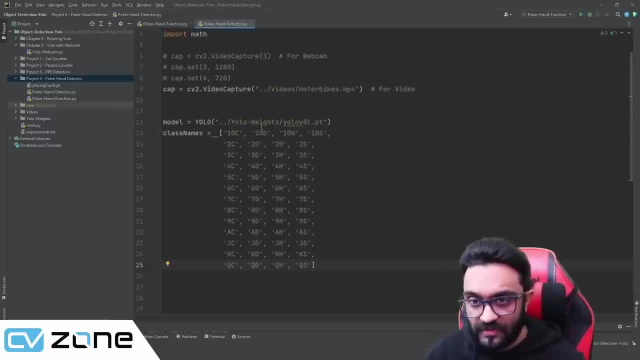 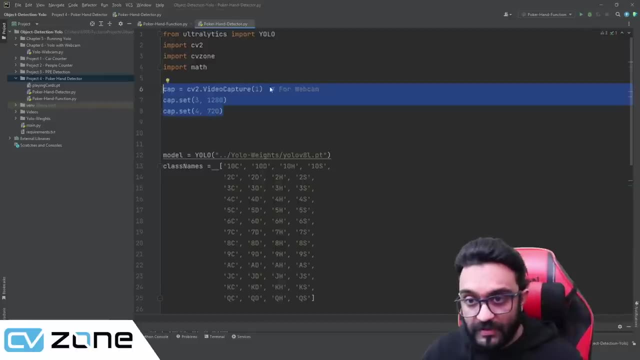 queen. So, as you can see, we have all the classes listed here and the video. we are not going to use any video, so we can remove that and we can open up the webcam and we will be using webcam one and this is the size and we will be using our own weight, which is 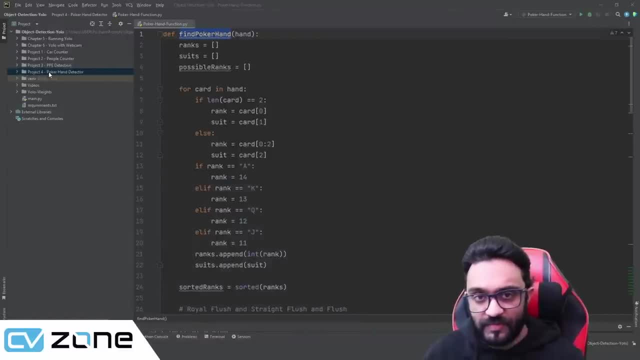 you our project. so we already have project for listed and we have created our poker hand function, and now what we will do is we will copy Yolo webcam, because we will be using our webcam to run it. so we will simply copy that and we will name it. 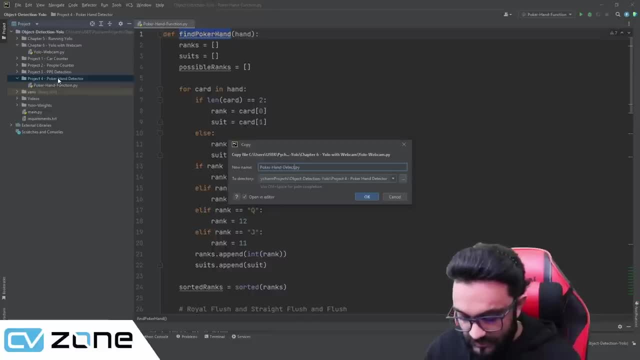 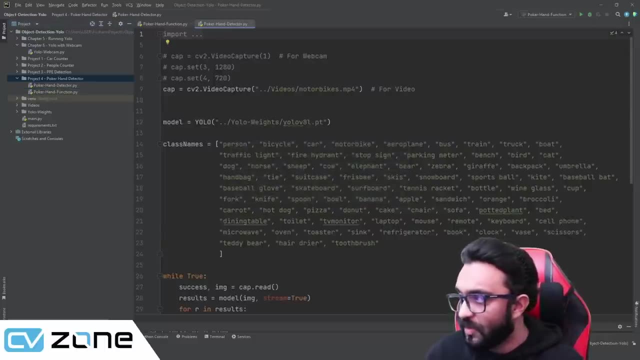 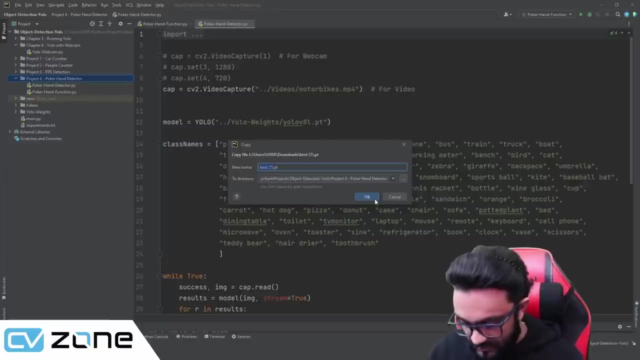 poker hand detector. so once we have that, we will bring in our model. so here you can see, this is best seven, so let's drag that in and we will call it playing cards dot, PT and over here. now we have to make the changes so that it detects these. so first of all, 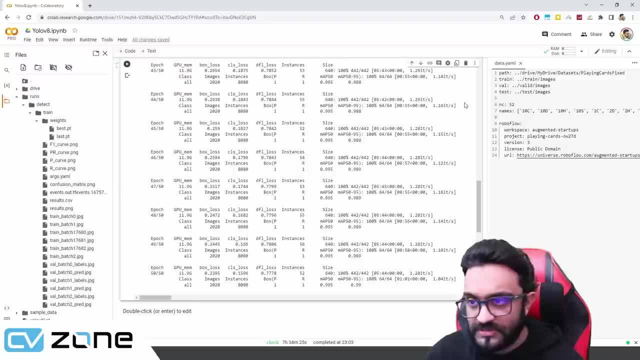 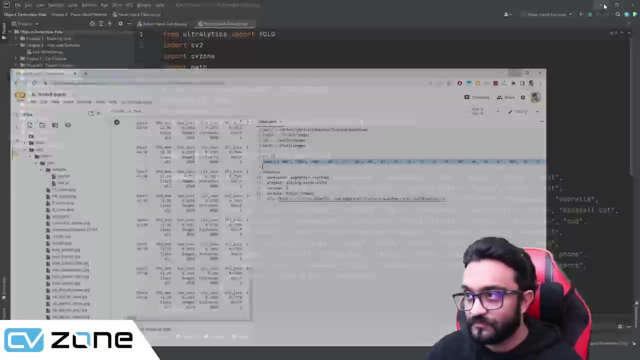 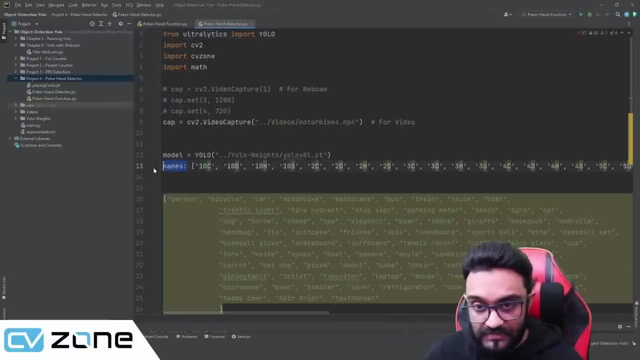 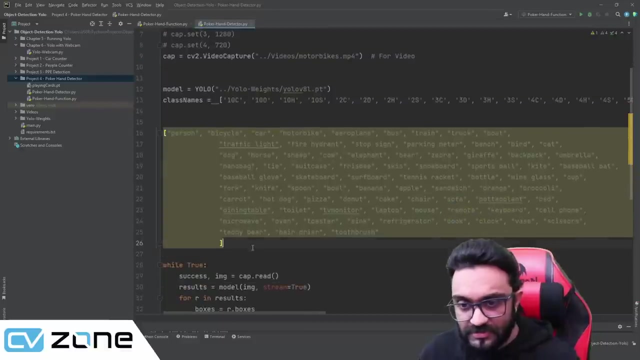 the class names we need to change. so to change that, we can go back to our data dot YML file and we can copy all the names and we can simply paste them here here and we can just cut this and paste it here. there you go, so to make it easier to understand. 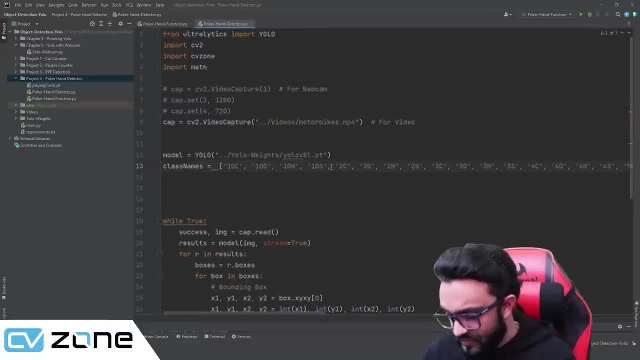 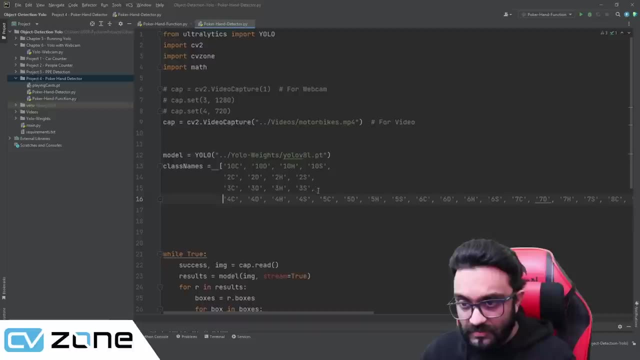 what's going on and we have all the classes. we can simply press enter after each of the ranks are done. so after two is done, then three, four, five, six, seven, eight, nine, ace, jack, king and queen. so, as you can see, we have all the classes listed here and the the video we are not going to use. 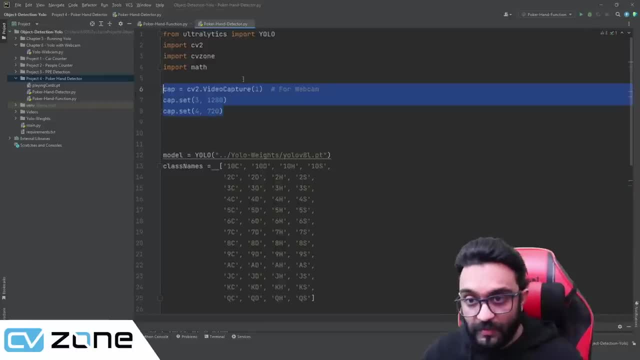 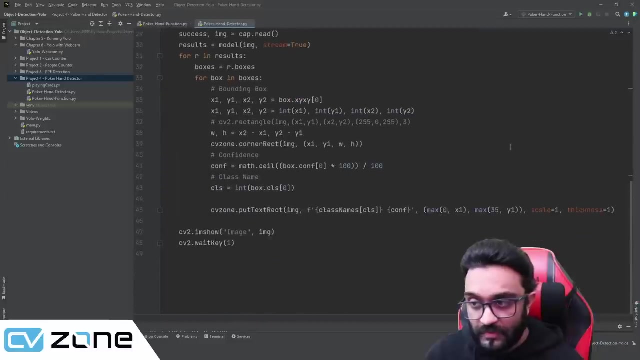 any video so we can remove that and we can open up the webcam and we will be using webcam one and this is the size and we will be using a our own weight, which is playing cards, dot, pt. and let's run this now and see if it works. 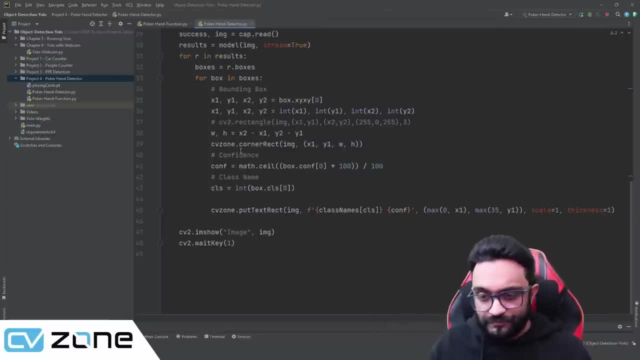 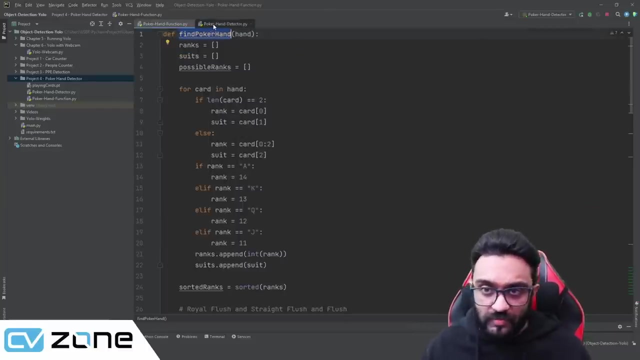 so i have my webcam upside down and we have some playing cards here and we are going to test them out one by one and see how it performs. once we know that all of these are detected properly, we can go ahead and merge our poker hand function with it, so that we don't have any 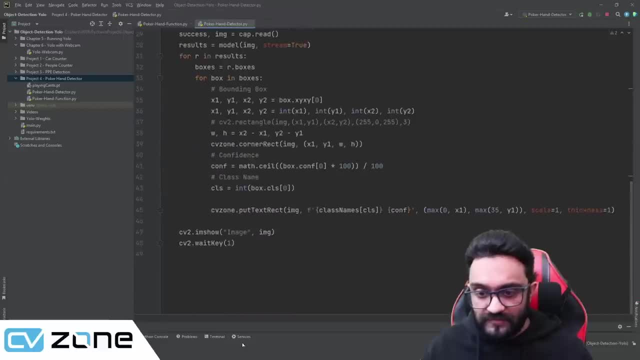 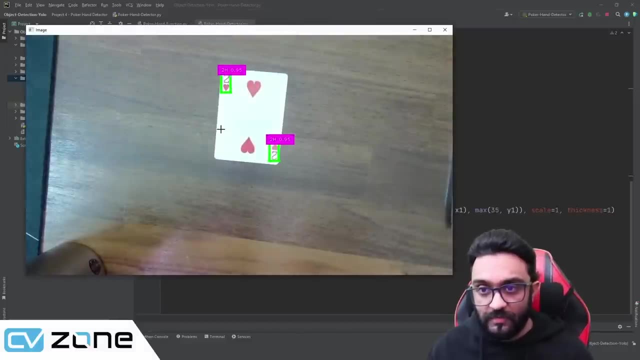 issues. so let's see if that works. it's actually running at the background, so here let's put in two. there you go. we are getting two edge, which is basically two of hearts. then we have jack of clubs, that's good. we have queen of spades. 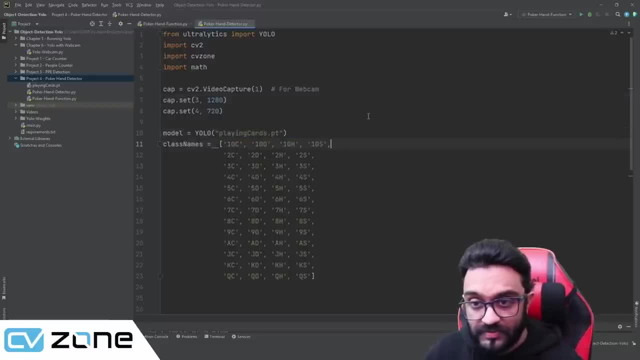 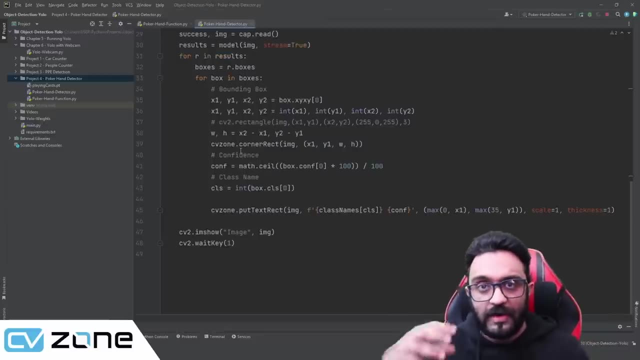 playing cards, dot, PT and let's run this now and see if it works. So I have my webcam upside down and we have some playing cards here and we are going to test them out one by one and see how it performs. Once we know that all of these are detected properly, we can go ahead and merge. 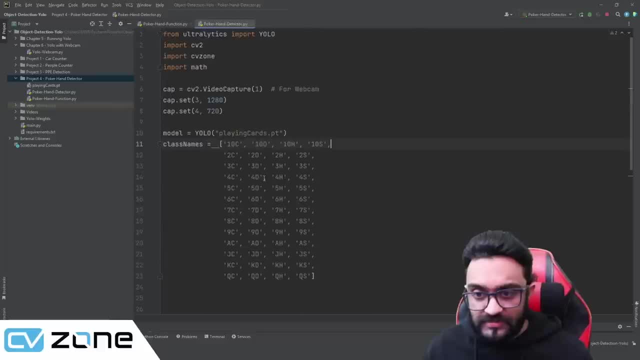 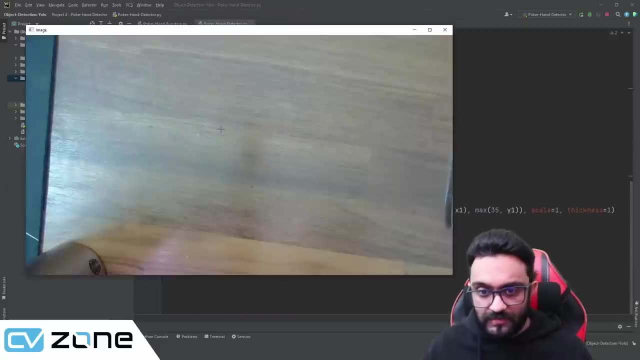 Our poker hand function with it so that we don't have any issues. So let's see if that works. It's actually running at the background, So here let's put in two. There you go. We are getting two edge, which is basically two of hearts. 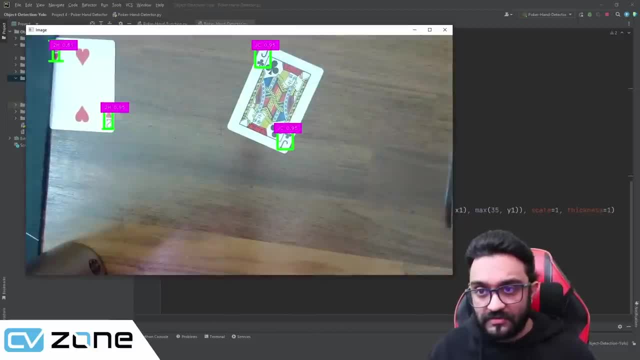 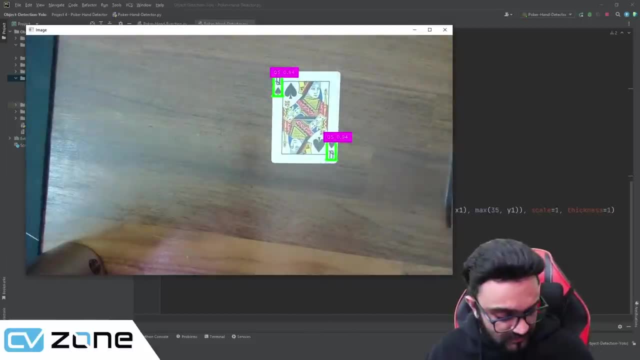 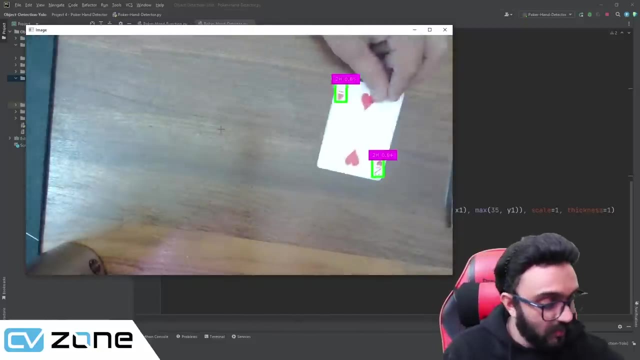 Then we have jack of clubs- That's good. We have queen of spades- That's good. So, in order to make it a little bit more efficient, what we can do is we can put all of the twos together and see if they work fine. 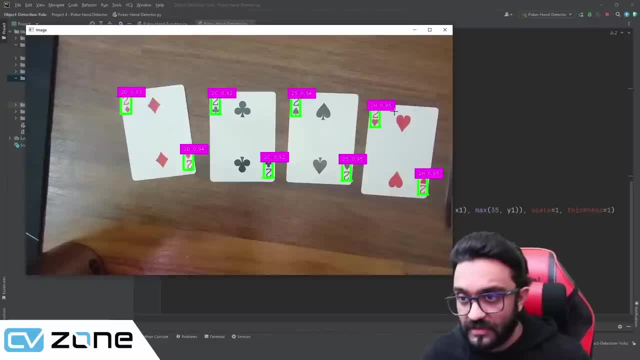 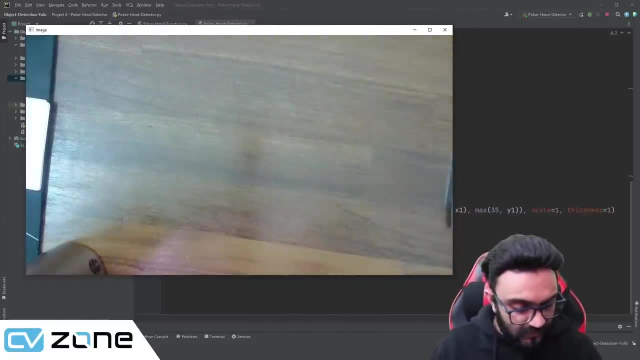 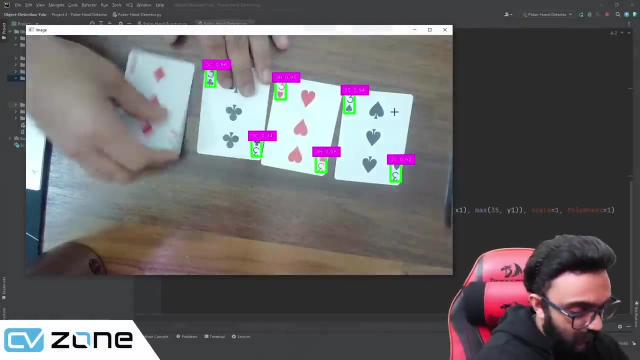 There you go: Two of diamond, two of clubs, two of spades and two of hearts. So we are detecting them properly. That's good. Then we have the clubs. Oh sorry, the threes, Let's try those. 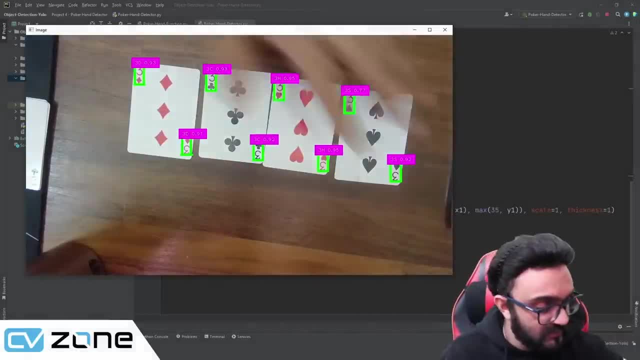 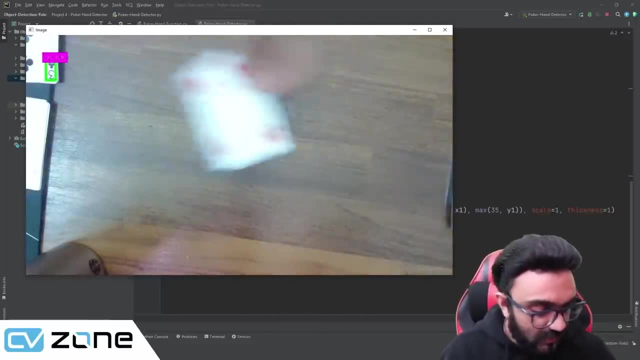 And three of diamond, three of club, three of heart, three of spades. That's working fine as well. We have to do this to make sure everything is working fine. There might be one or two classes that are not detected properly, so we have to make. 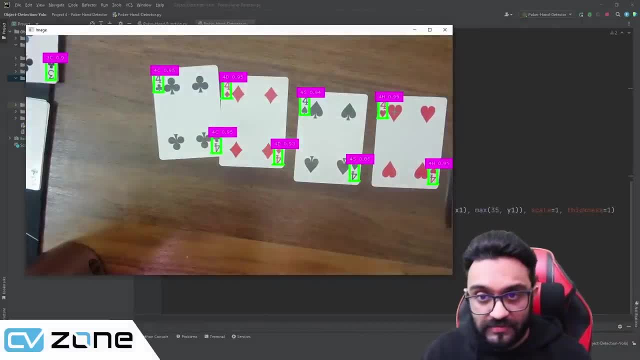 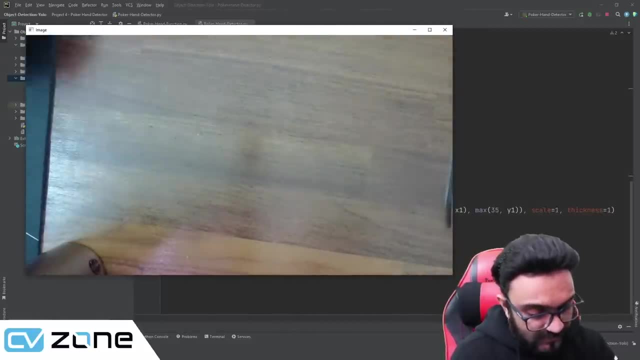 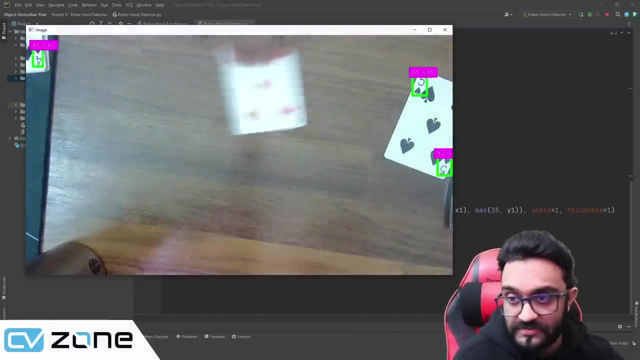 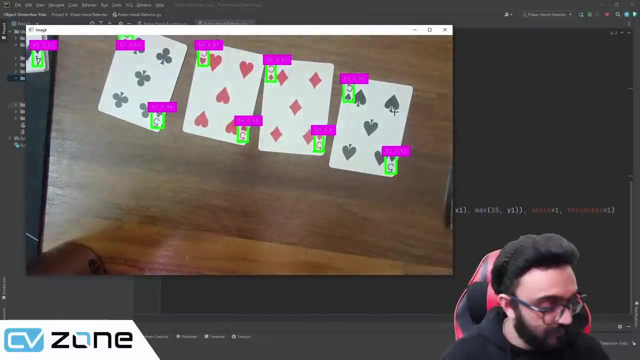 sure all of them are correct: Heart, spades, diamond and clubs. So those are fine as well. So so far it is giving us really good results and it's very fast as well, as you can see. So this is five of spade, five of diamond, heart and club. 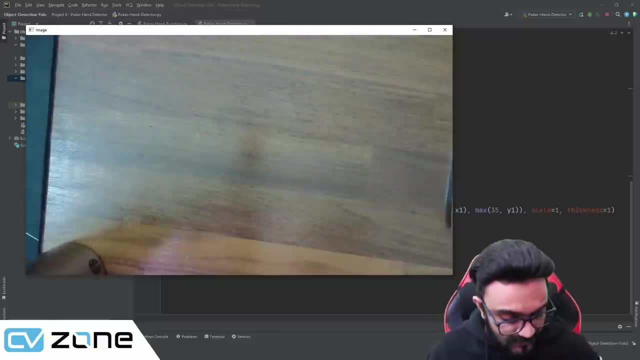 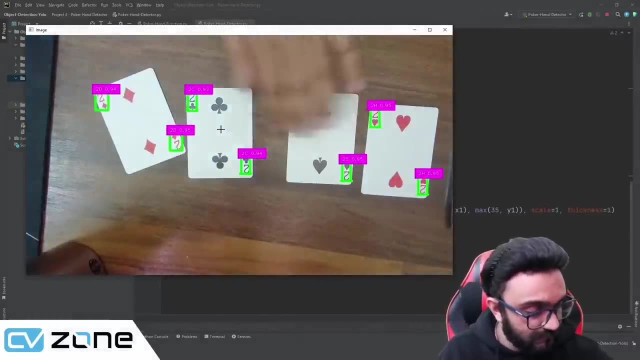 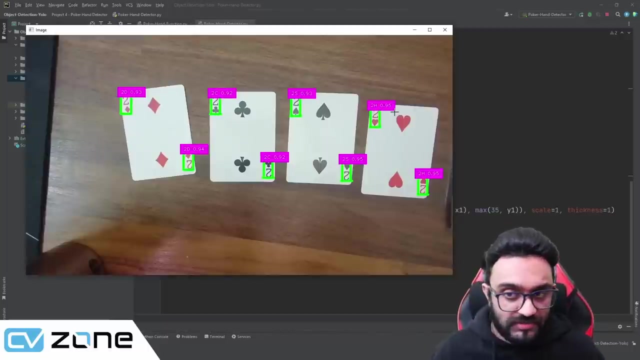 good. so, in order to make it a little bit more efficient, what we can do is we can put all of the twos together and see if they work. fine, there you go: two of diamond, two of clubs, two of spades and two of hearts. so we are detecting them. 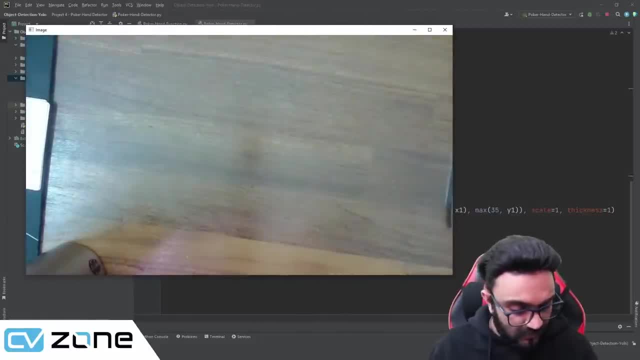 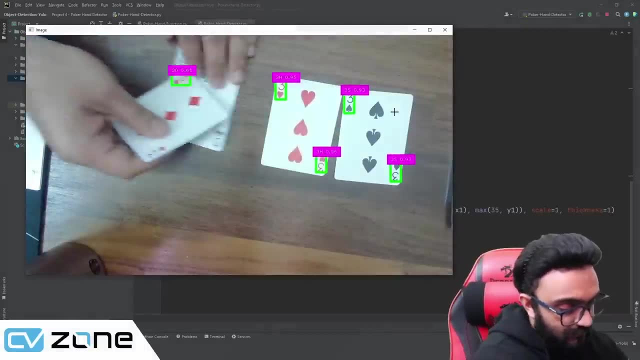 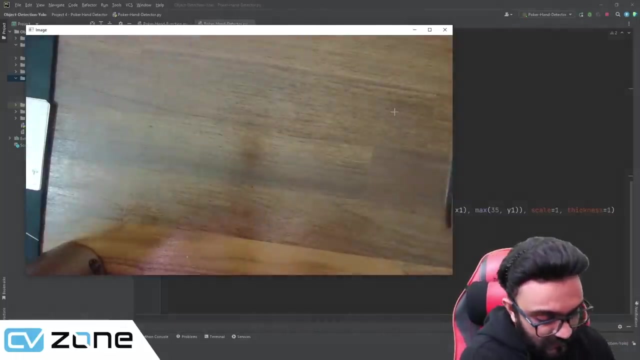 properly. that's good. then we have the clubs. oh, sorry, the threes, let's try those- and three of diamond, three of club, three of heart, three of spades. that's working fine as well. we have to do this to make sure everything is working fine. there might be one or two classes that 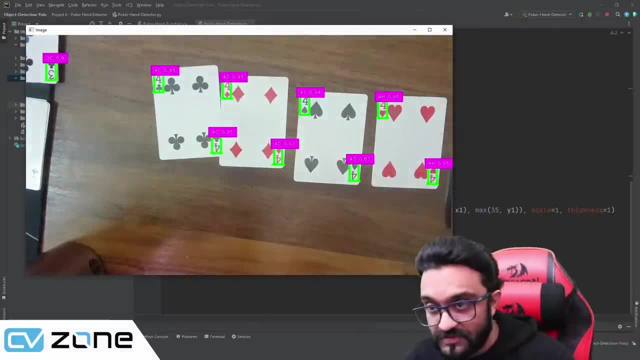 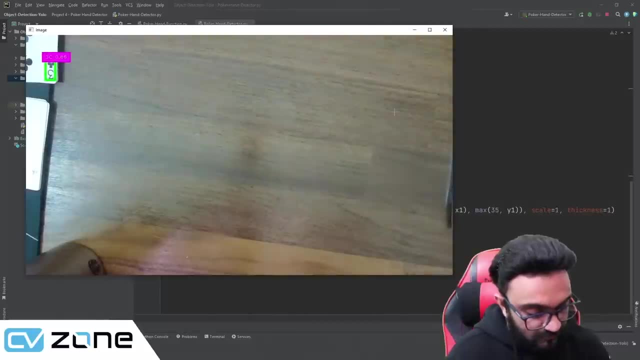 are not detected properly. so we have to make sure all of them are correct: hearts, spades, diamond and clubs. so those are fine as well. so so far it is giving us really good results, so that's good. so, yeah, all right, let's hopefully we have it work, but let's try again and see if we can find any other problems with. 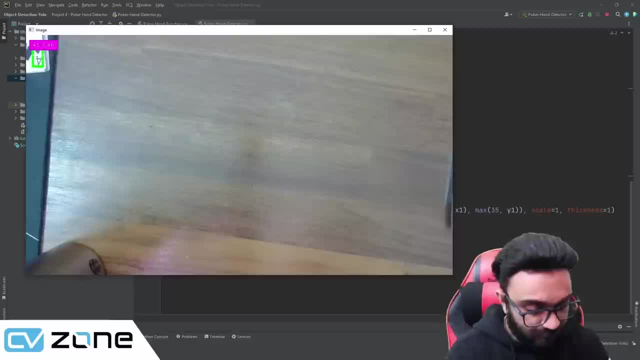 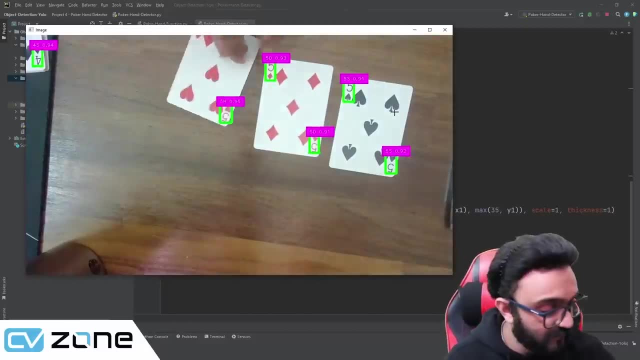 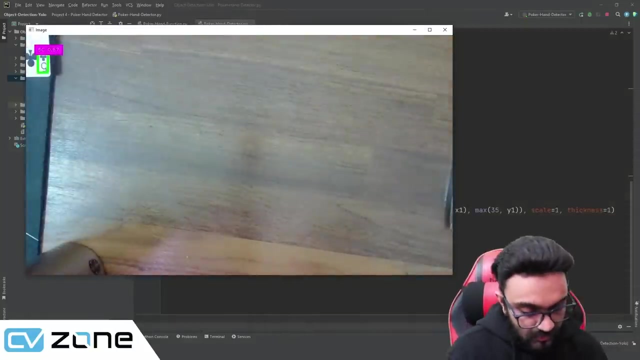 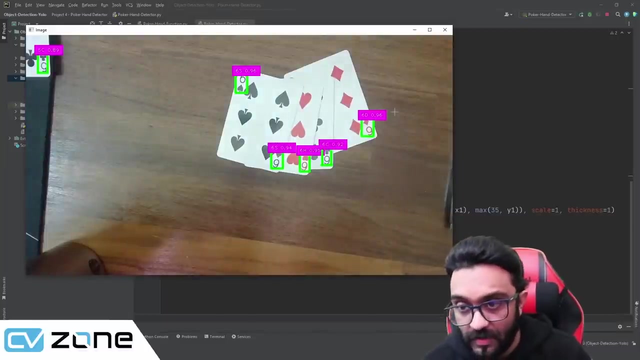 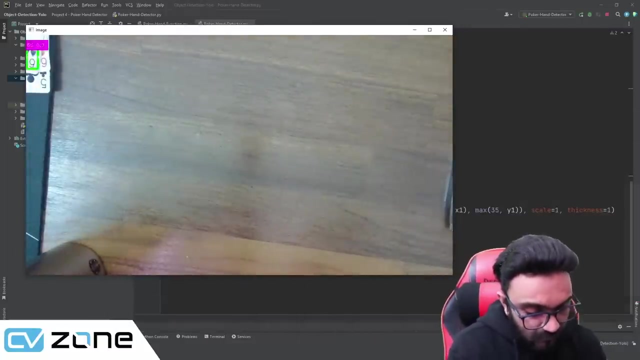 good results and it's very fast as well, as you can see. so this is five of spade, five diamond, heart and club. there you go. then let's check the six. let's put them like that: diamond, club, heart and spade. that's fine. then let's put seven. let's try it like that. seven. all of them are correct. 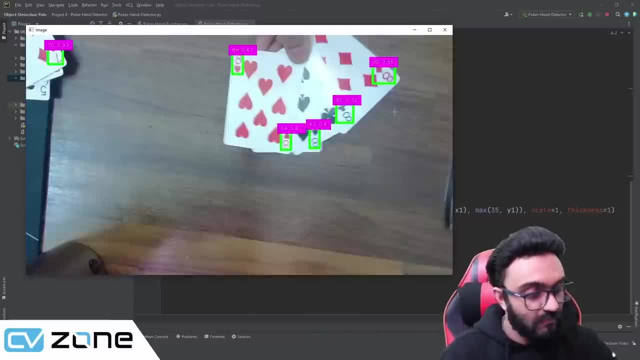 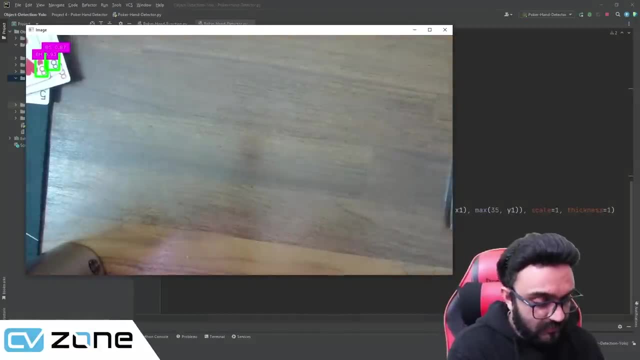 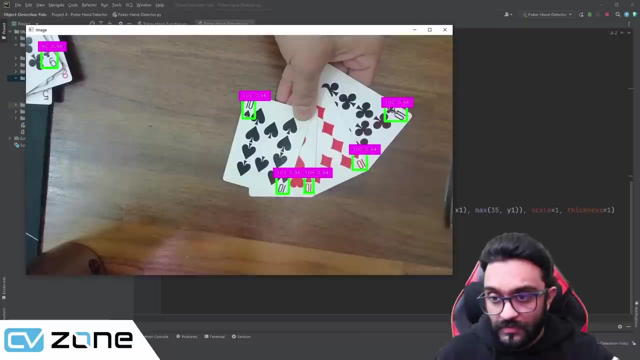 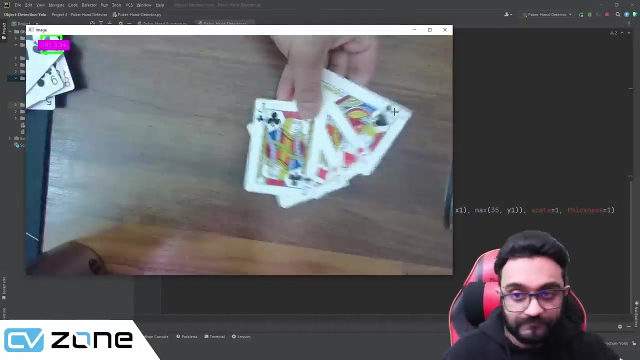 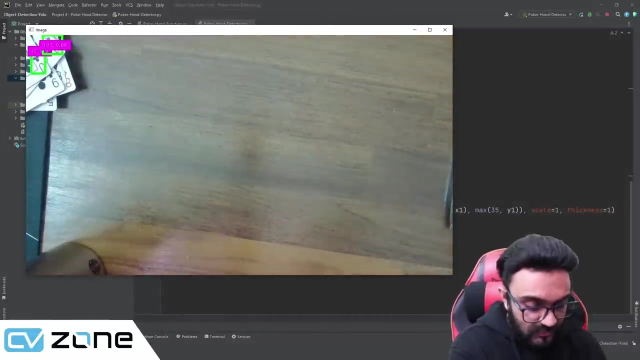 let's try eight. eight, all of them are correct. nine: yep, all of them are correct. and yep correct. then we have jack- yep correct. then let's try the queen- yep correct. let's try the kings. wait, i'm missing a king. oh, what happened? i am missing a king. 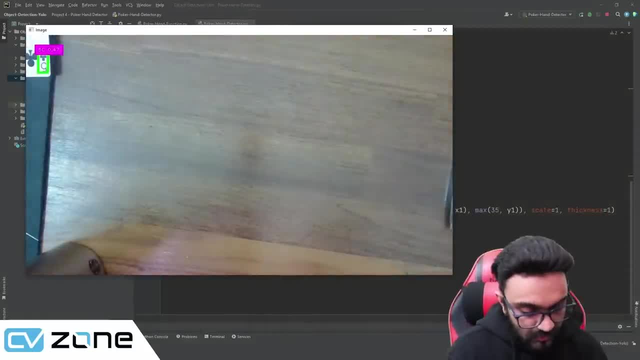 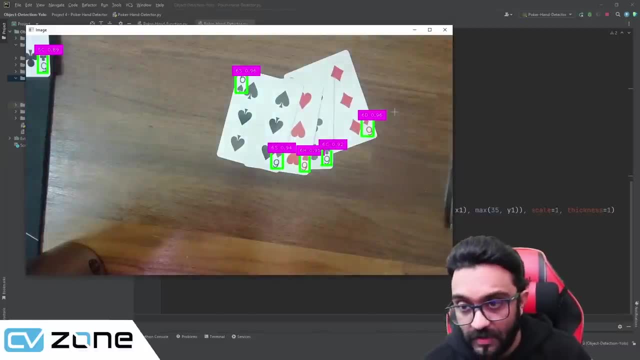 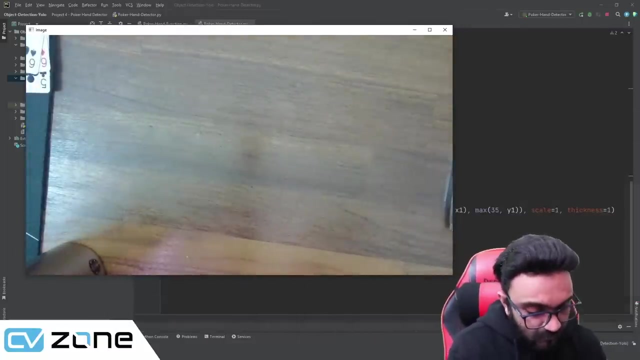 There you go. Then let's check the six. Let's put them like that: Diamond club, heart and spade. That's fine. Then let's put seven. Let's try it like that: Seven, all of them are correct. 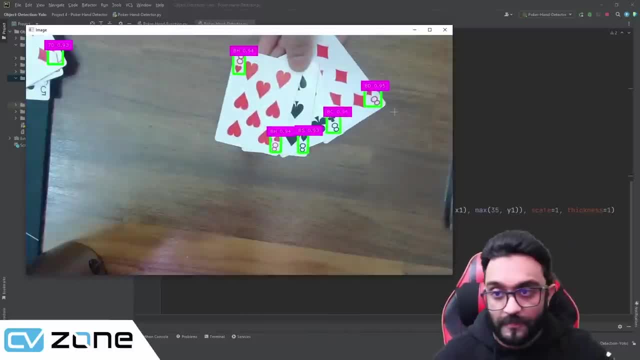 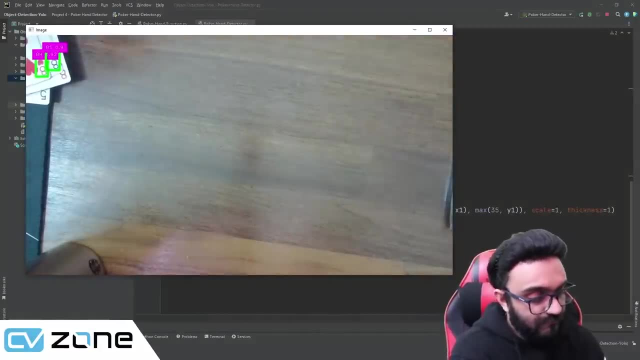 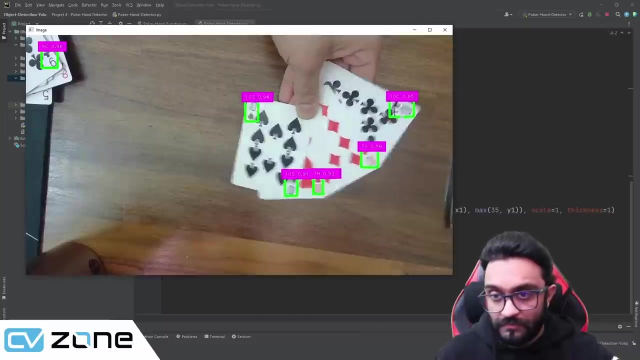 Let's try eight- Eight- all of them are correct. Nine- Yep- Eight- all of them are correct. Ten, Yep- correct. Then we have jack, Yep, correct. Then let's try the queen Yep correct. 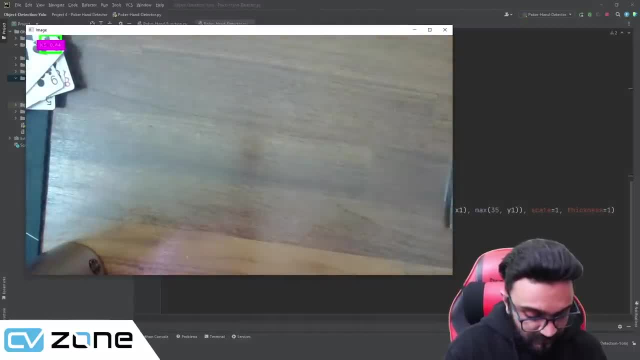 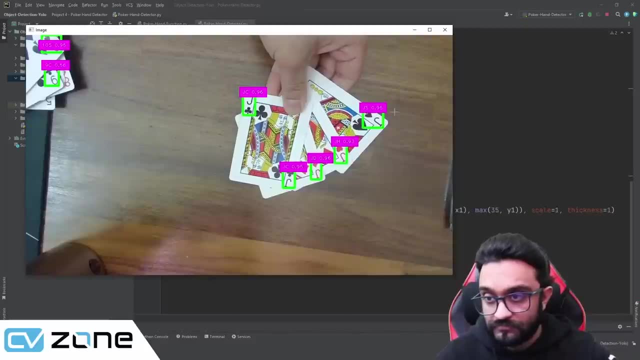 Then let's try the queen Nine: 10. 10., 11., 12., 13., 15., 16., 17., 18., 19., 21., 20., 21., 22.. 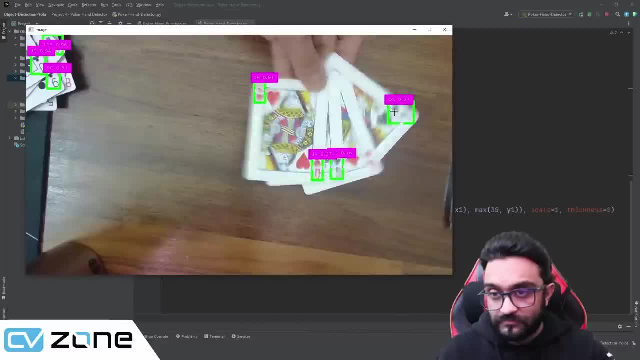 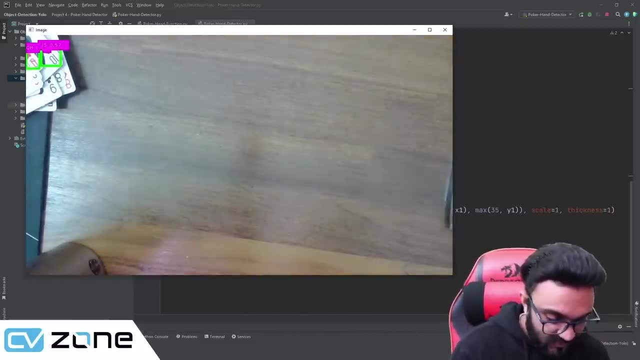 23. 24. 25. 26.. yep, correct, let's try the kings. wait, I'm missing a king. oh, what happened? I am missing a king. okay, so let's let's. let's try with the cards we have. oh no, I found it never. 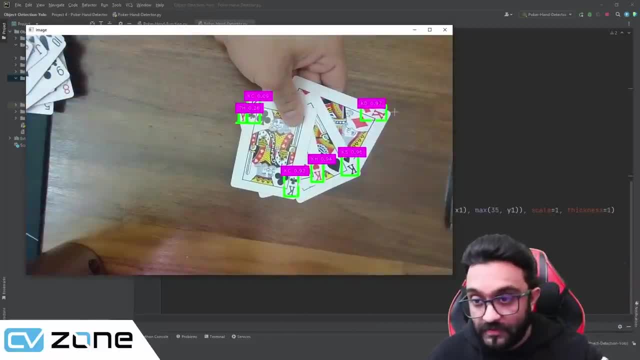 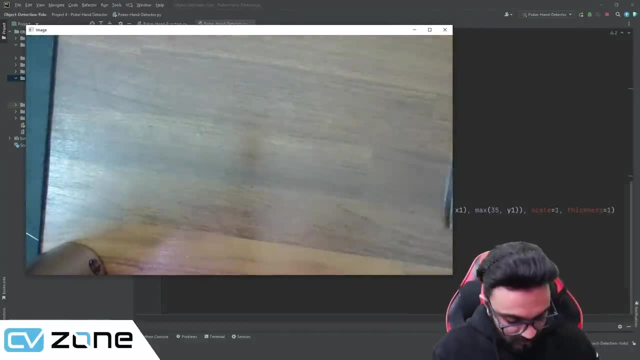 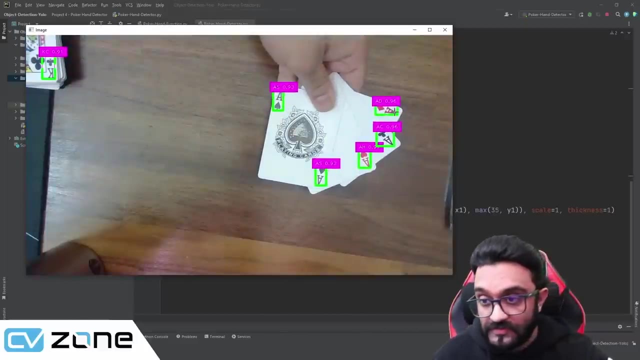 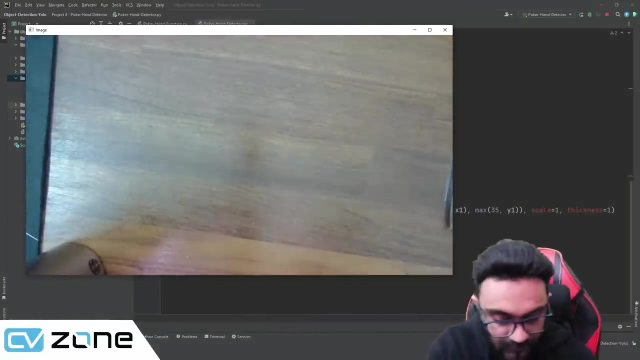 minds. okay, club, heart, spade, diamond- excellent. and now the moment of truth, the last one, the ace, ace of spade, heart club and diamond- perfect. so we have 100 out of 100 being detected properly. actually, 52 out of 50,, 52,. so what we will do now is we: 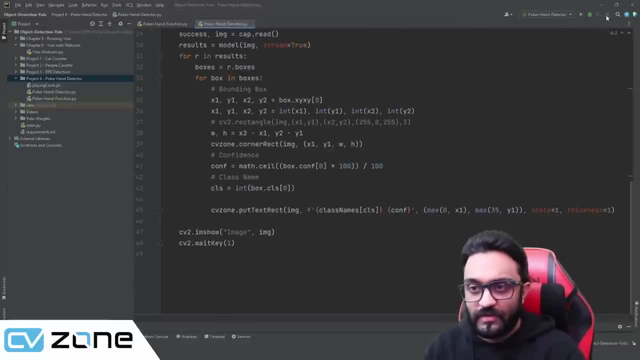 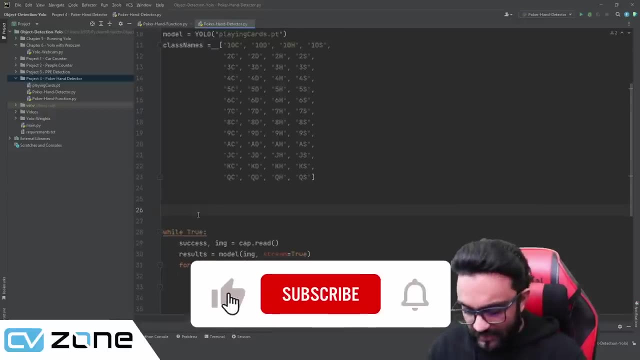 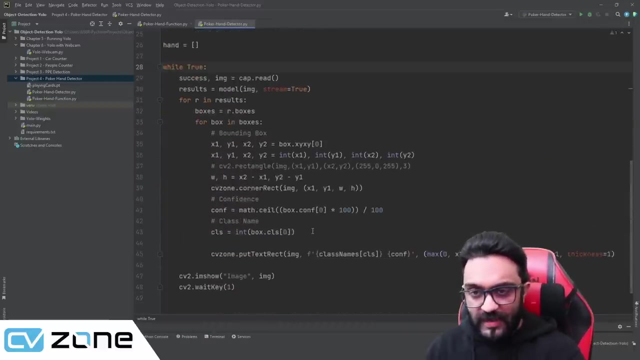 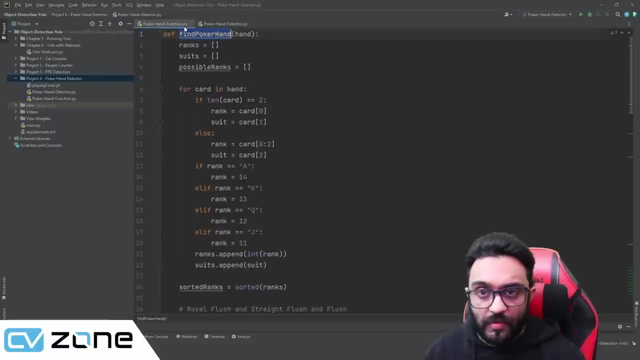 will detect. first of all, we. we are already displaying it. we are going to put it in a variable called hands or hand. hand is equal to empty. now, once we have this, we are going to send this hand to our poker hand function. so here, if we import now in order to import, 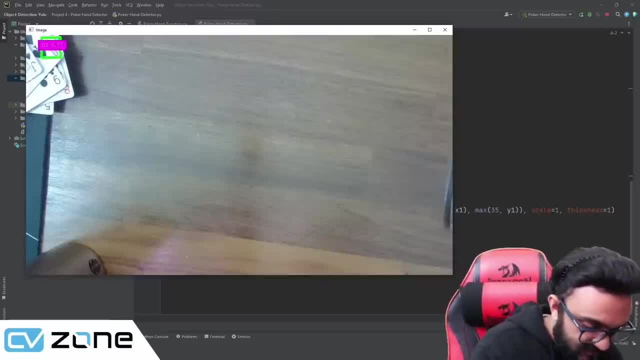 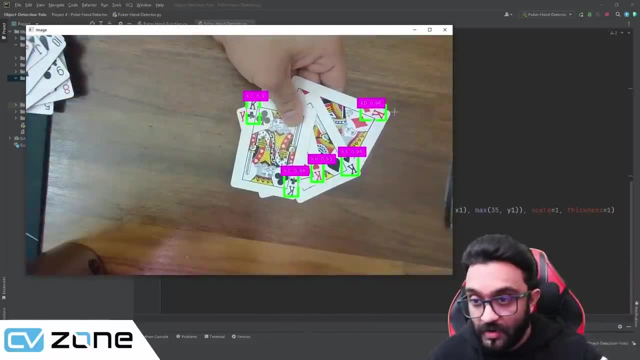 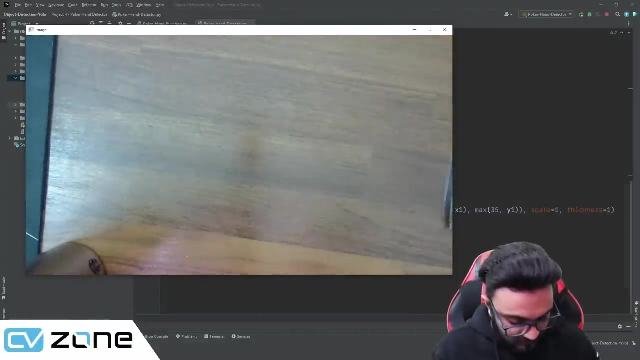 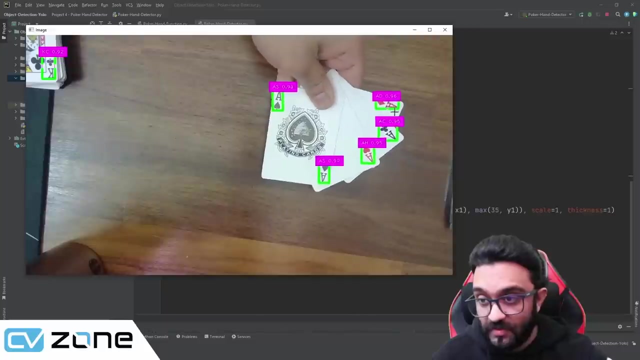 okay, so let's, let's just try with the cards we have. oh no, i found it, never mind, okay. club, heart, spade, diamond- excellent. and now the moment of truth, the last one, the ace. ace of spade, heart, club and diamond- perfect. so we have 100 out of 100 being detected. 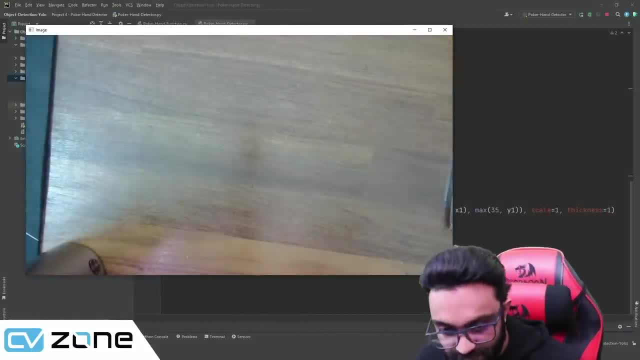 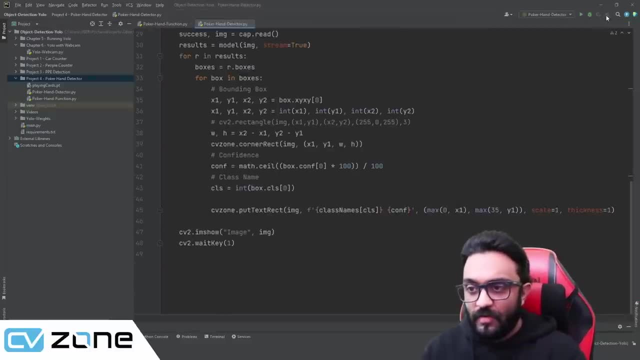 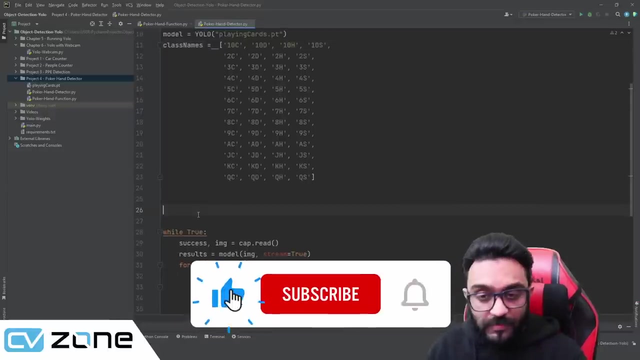 properly. um, actually 52 out of 50, 52. so what we will do now is, once we detect this- first of all we we are already displaying it- we are going to put it in a variable called hands or hand. hand is equal to empty. now, once we have this, 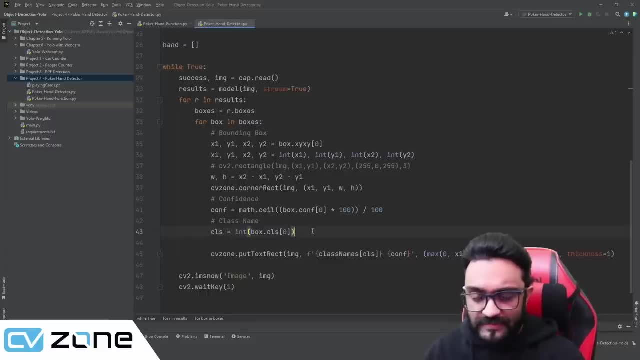 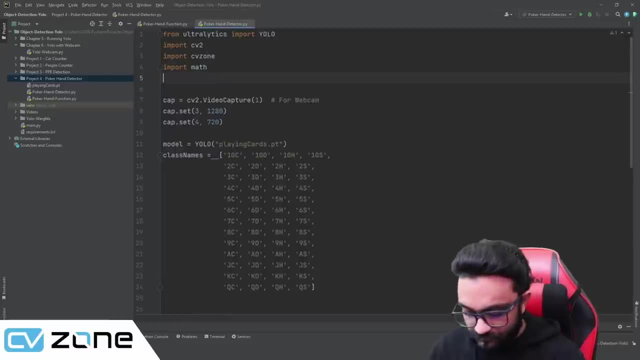 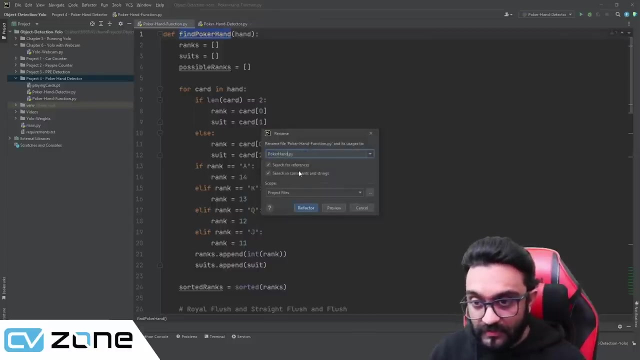 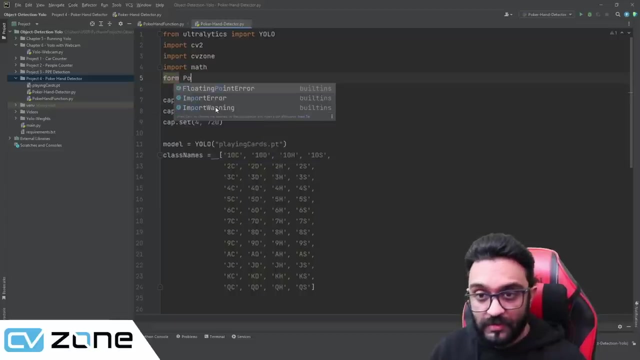 we are going to send this hand to our poker hand function. so here, if we import now, in order to import this we will have to rename it, rename file and we will write it poker hand function without the dashes so that it's easily imported. so we'll write here from poker so we can write here: imports poker and function. so now we will. 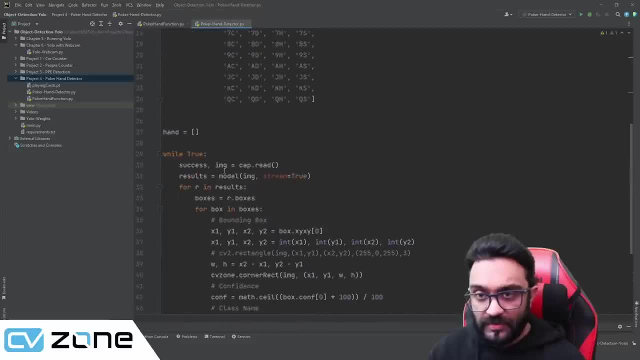 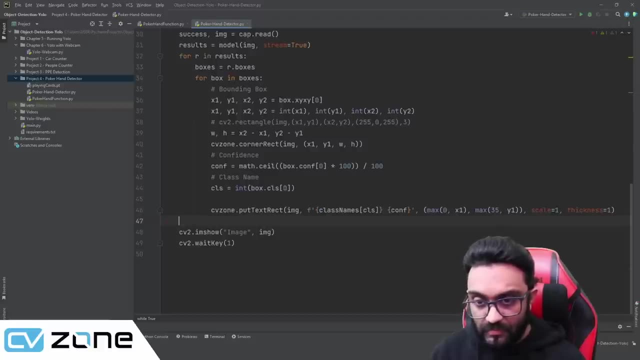 have the ability to use find poker hand, so we can go down here and we can send it to find. so we can write: poker hand function dot. poker hand function dot. find poker hand and we will send in our hand. so we will check the results equal this and what we have to do is we have to first of all. 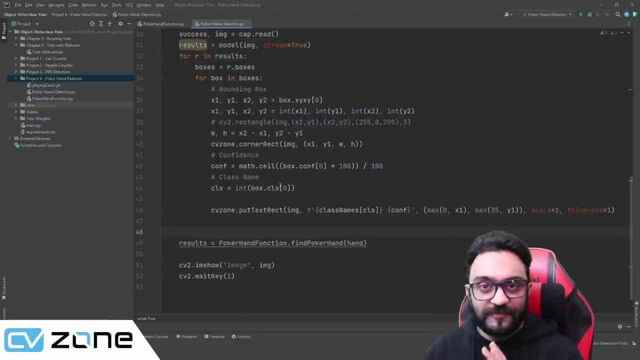 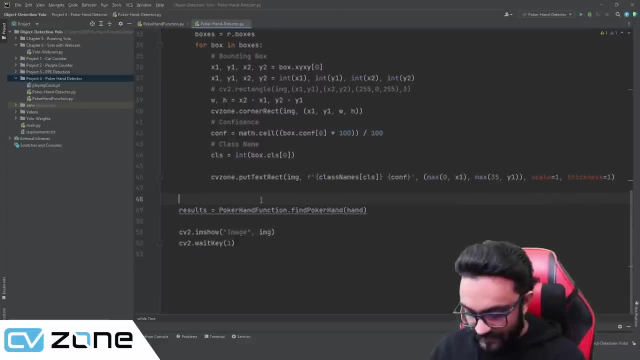 make sure that we have five different cards. so if there are four or two or three, that then it should not work. so we should have a total of five. so if the length of hands, if the length of hand equals five, then only we are going to send this. if it's more or less, we. 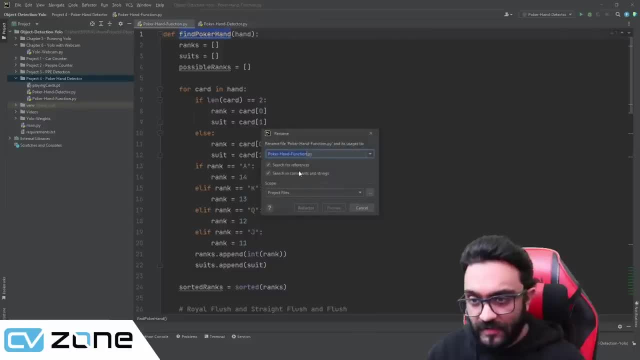 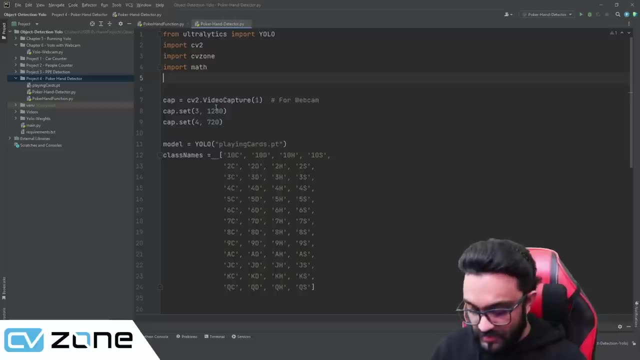 this. we will have to rename it, rename file and we will write it poker hand function without the dashes, so that it's easily imported. so we'll write here from poker so we can write here: import poker hand function. so now we will have the ability to use find poker. 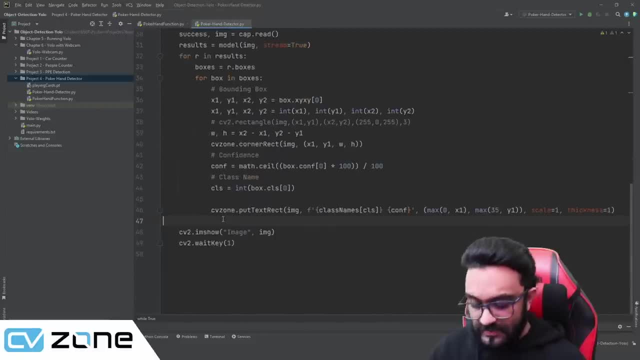 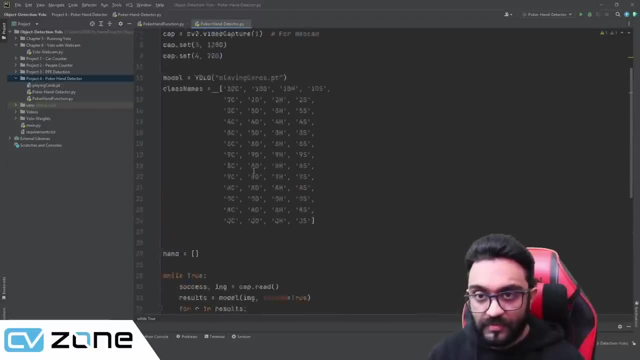 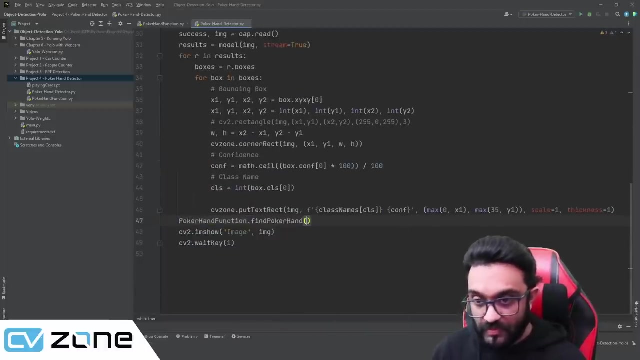 hand so we can go down here and we can send it to find. So we can write: poker hand function dot. poker hand function dot. find poker hand. and we will send in our hand so we will check the results, equal this and what we have to do. 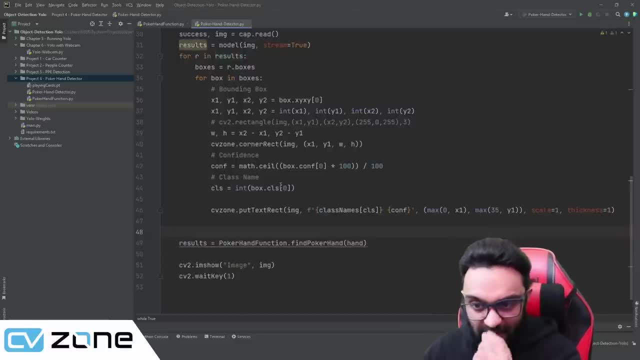 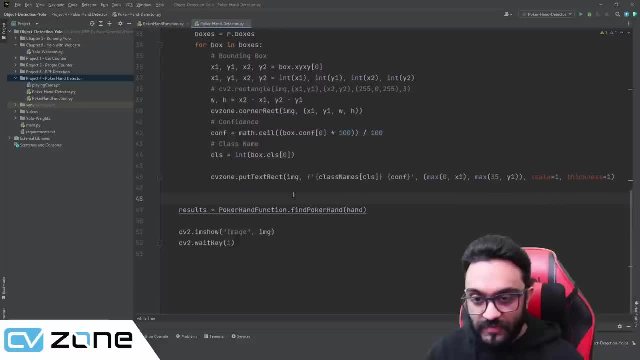 four or two. we have to make sure that we have five different cards. so if there are, or two or three, that then it should not work, so we should have a total of five. so if the length of hands, if the length of hand equals five, then only we are going to send this. if it's more, or 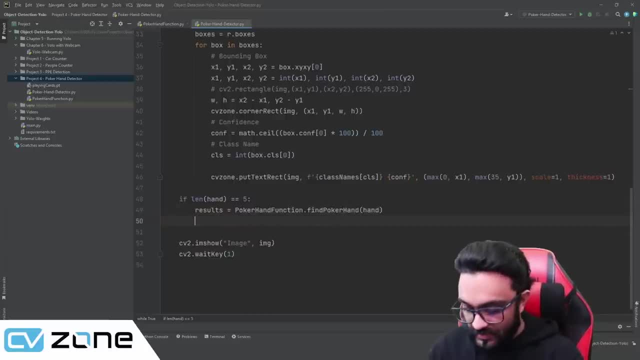 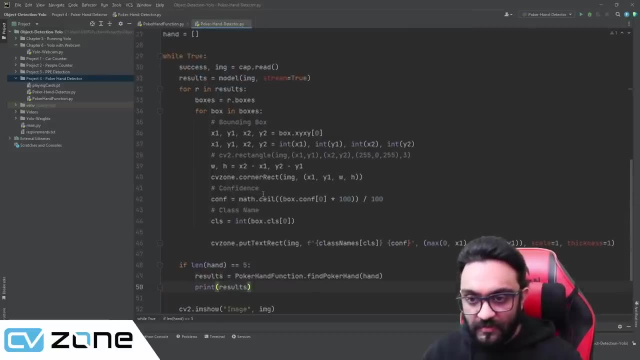 less. we should not send it. so once that is done, we can simply print the results. we can display it. we will display it now, but for now we'll do that. okay, so once we are actually detecting this, we can put, for example, a limitation that if the confidence level is greater than 0.5. 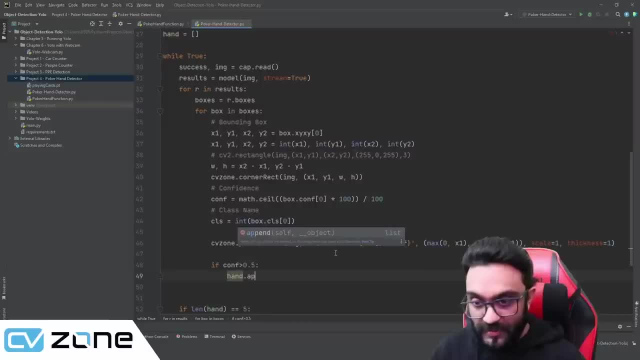 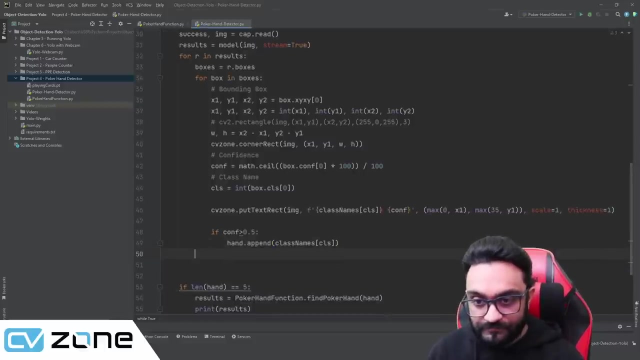 then hand dot append. we are going to append the class name. so the class name is basically cls. so this is not actually the class name. the class name is class names of cls. there you go, so we will append that. so what we can do is we can, we can print. 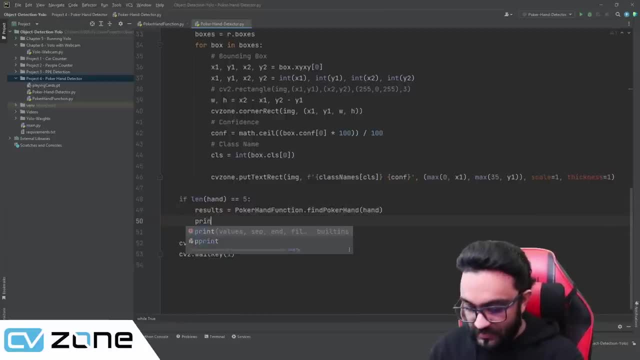 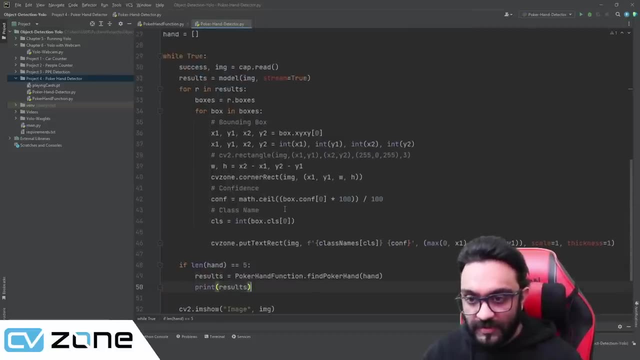 should not send it. so once that is done, we can simply print the results. we can display it. we will display it now, but for now we'll do that. okay, so once we are actually done with this, we can go to our host, Toni, so we can sometime input this. then we can also send another link there as well. so 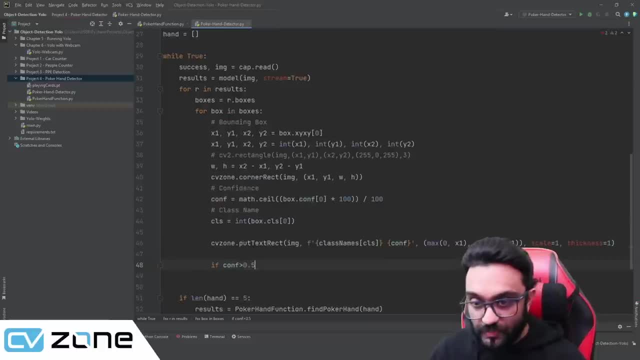 we can have an element, and when you cannn, you can also send this a mama as well. so let's have a moment over here for a minute so that we can put this world. now we are actually detecting this. we can put, for example, a limitation that if the confidence 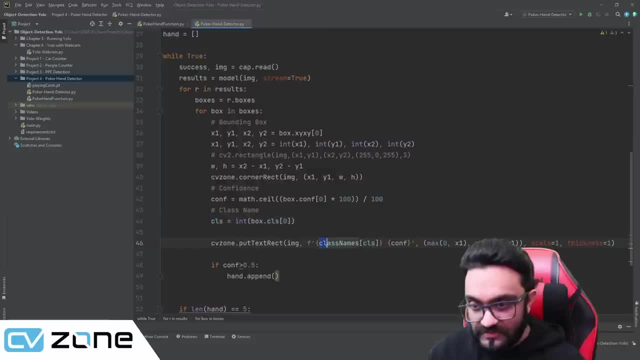 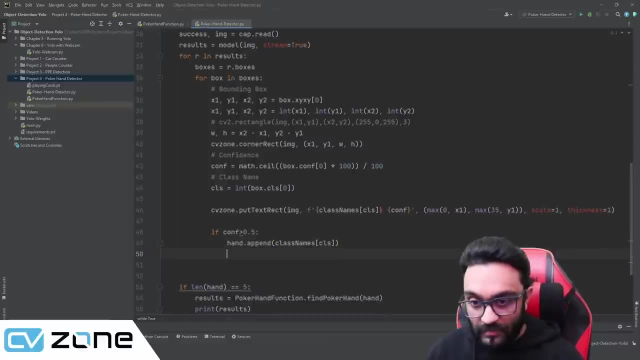 level is greater than 0.5, then a hand dot append üğ. so we will append that. so what we can do is we can, we can print a hand. so let's try that out and see how it works, because we want to see what exactly are we sending before we actually see the results. so 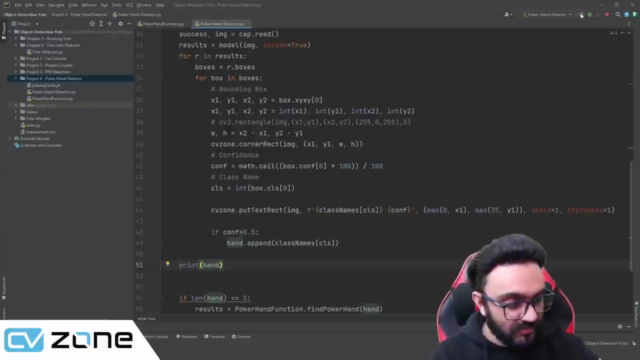 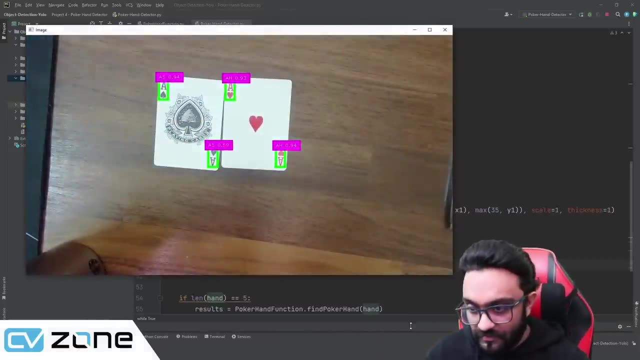 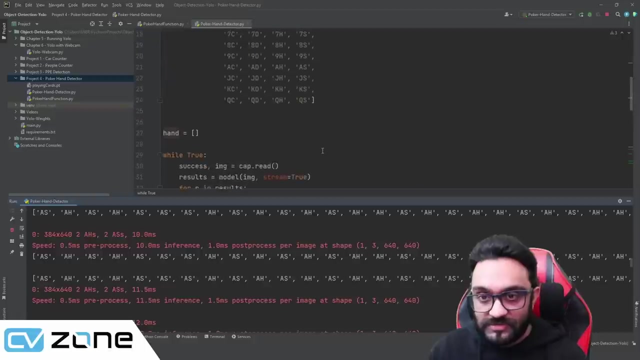 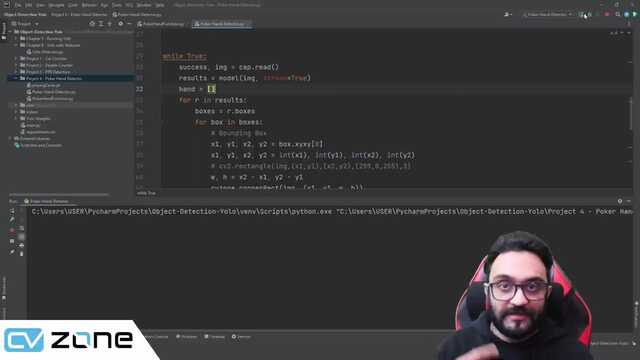 let's put two cards in and let's see what result do we get. so there you go. we have, uh, some results here. so there you go. uh, it is appending. oh, oh, it keeps adding to it, which is not good. the hand should be after each iteration, it should update and it should clear out. so we need to have a fresh start. 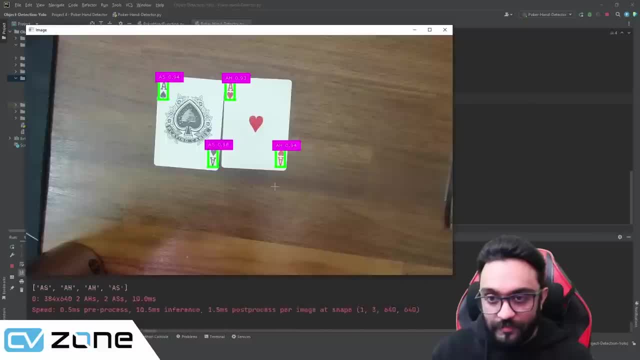 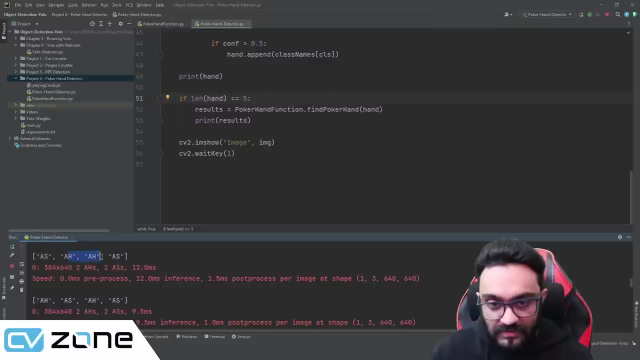 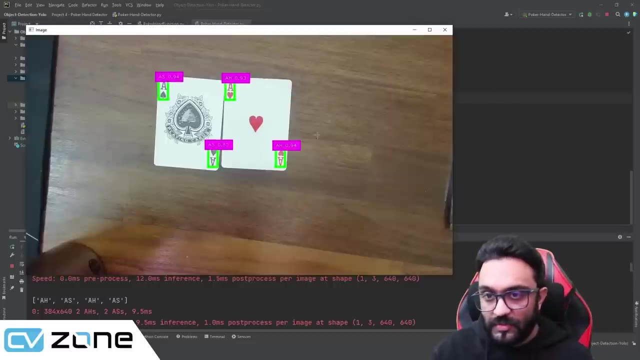 every time it runs an iteration. so there you go, we have. we have these. you a s a h and a h a s, h and h. okay, so the problem here is that it's showing it twice, so that's not good. so what we need to do is we need to create a set and send it back to a list. 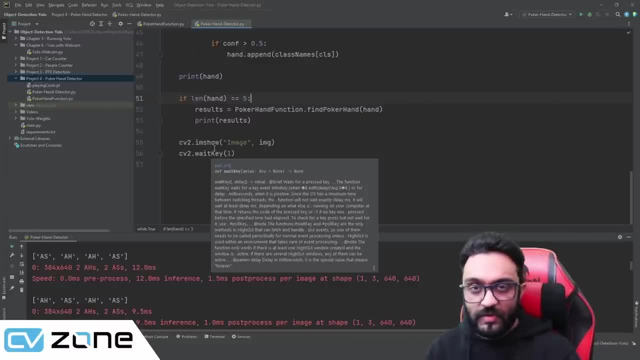 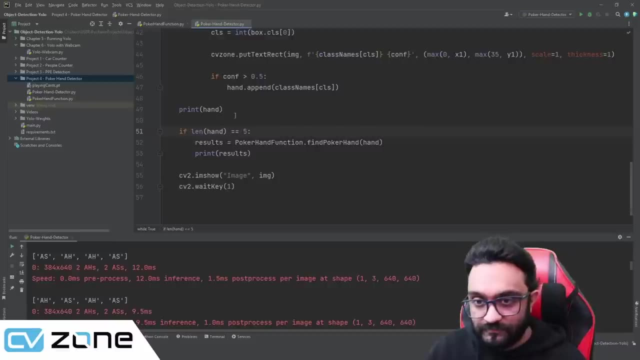 so this way it will only have unique values, because we cannot have two of the same cards. it cannot be possible. so we can simply just do a set and then it should work fine. so here we can write: hand equals set of hand, and then we can put it in a list again. 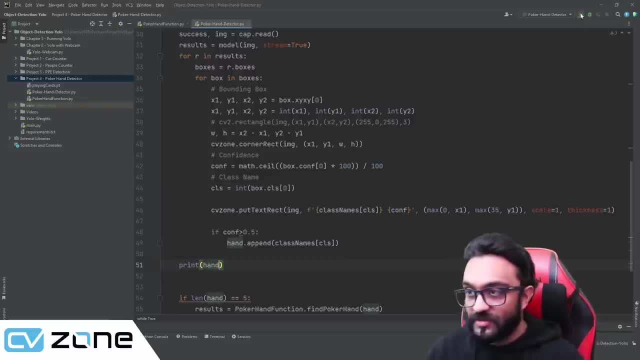 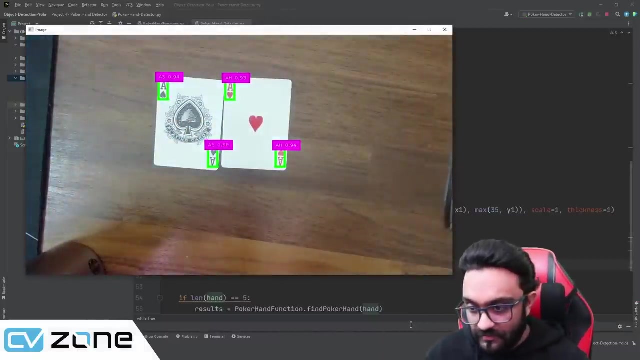 a hand. so let's try that out and see how it works, because we want to see what exactly are we sending before we actually see the results. so let's just put two cards in and let's see what result we get. so there you go. we have some results here. so there you go. uh, it is appending. oh. 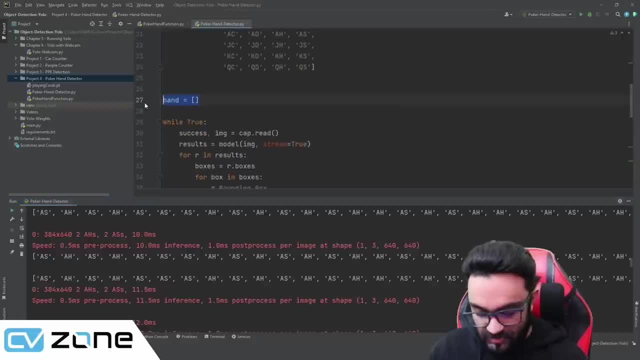 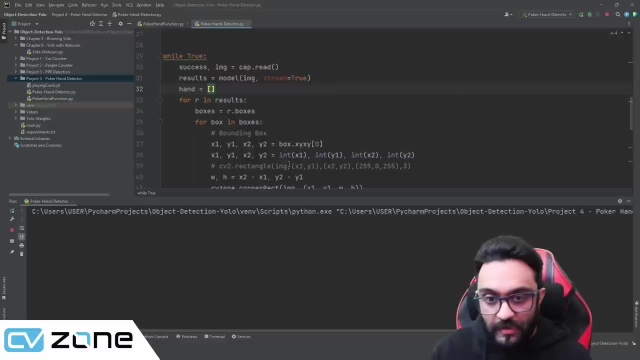 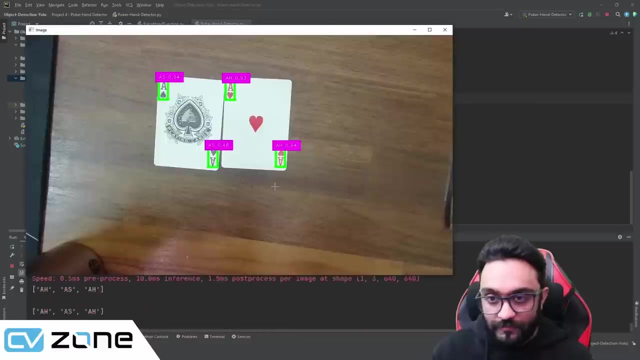 oh, it keeps adding to it, which is not good. the hand should be after each iteration, it should update and it should clear out. so we need to have a fresh start every time it runs an iteration. so there you go, we have. we have these as ah and ah. 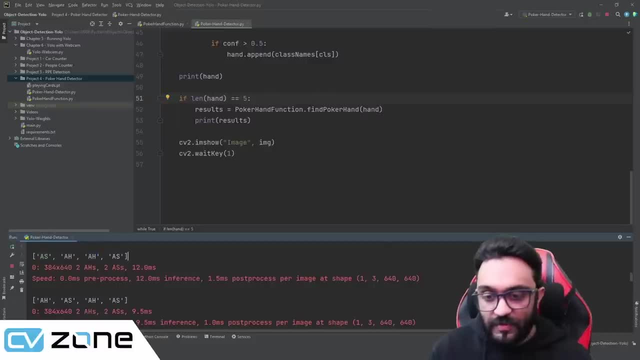 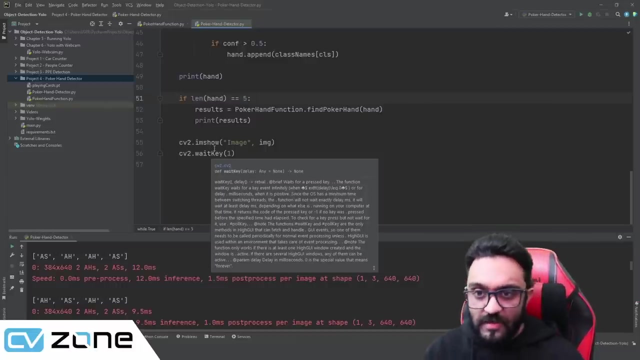 as ah and ah. okay. so the problem here is that it's showing it twice, so that's not good. so what we need to do is we need to uh, create a set and send it back to a list, so this way it will only have unique values, because we cannot have two of the same cards. it cannot be possible, so we can. 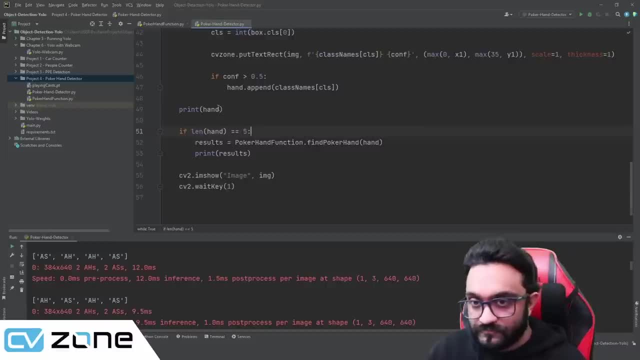 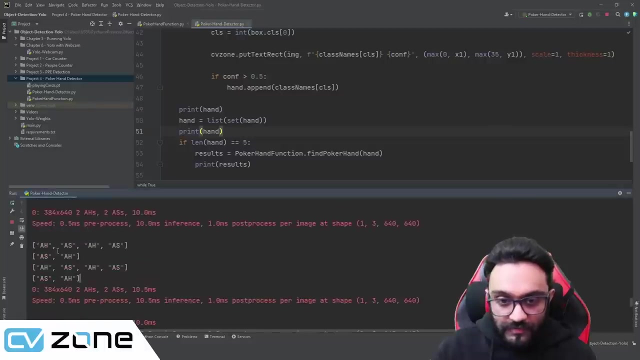 simply just do a set and then it should work fine. so here we can write: hand equals a set of hand, and then we can put it in a list again and we will print it before and we will print it after. so so there you go. so if this is the case, then the set is like this, so we are getting one of each. 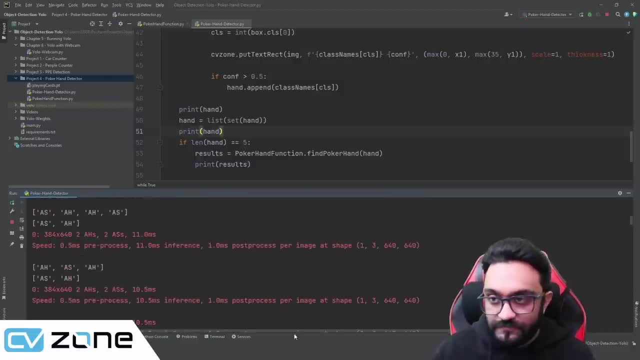 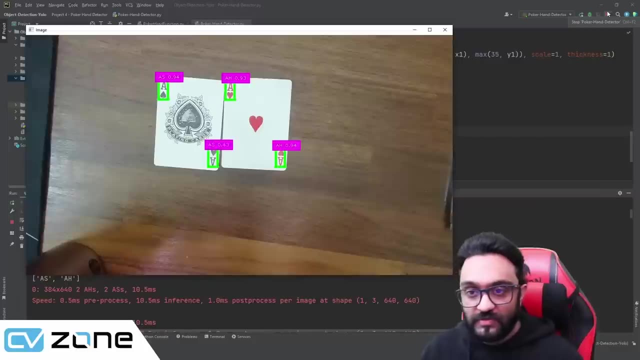 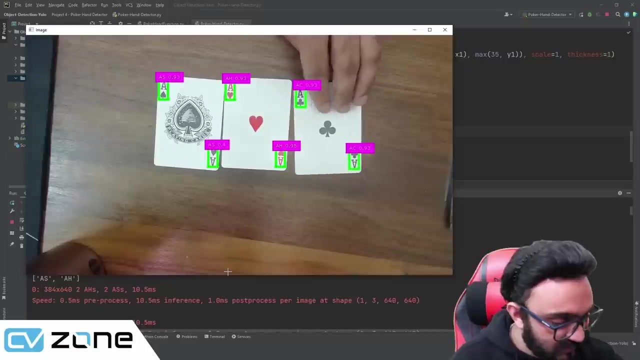 so that's good, that's exactly what we want. so, as you can see here, it is detecting, but we are getting one of them. okay, so now what we can do is we can add five of these and it should give us the result. so let's put four of a kind, which, because it's really easy here- i have already. 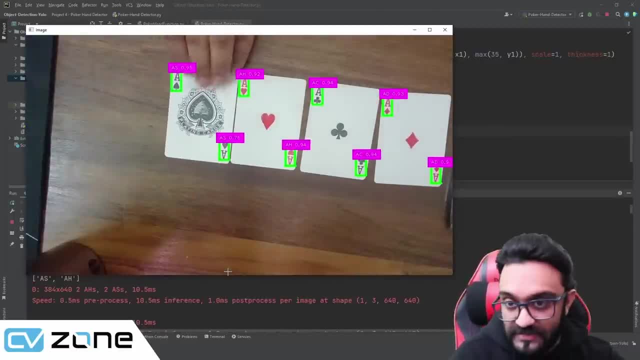 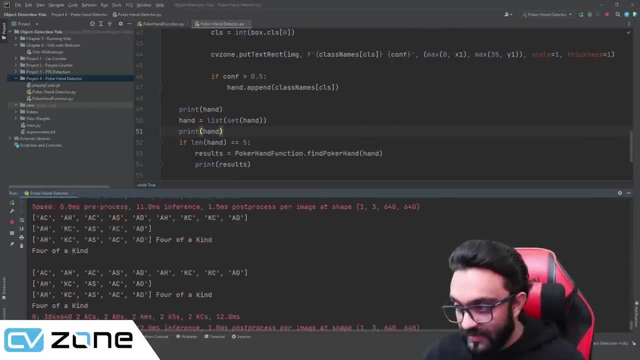 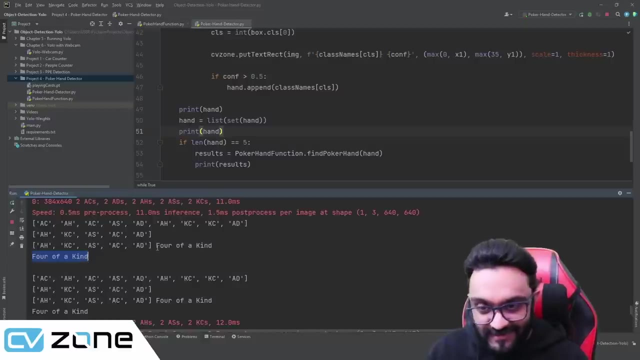 a's lined up, so and we have these a's, and then we can add simply another card which is a king, and we should get an output here. so let's go at the end and let's see. so there you go, we are getting four of a kind. so the moment of truth has been revealed and we're getting a four of a kind. 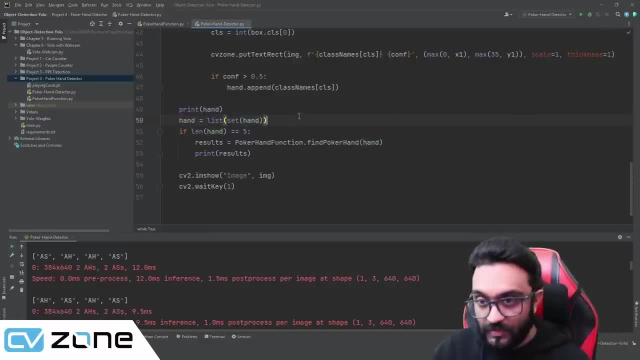 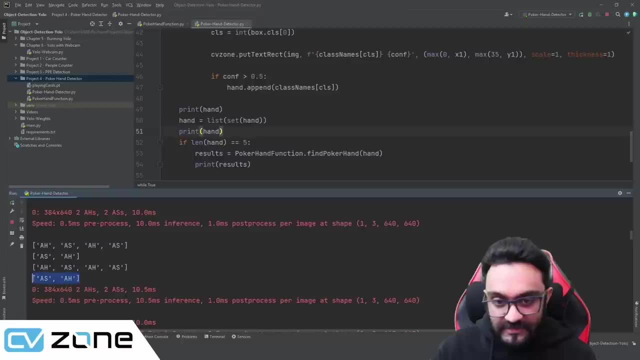 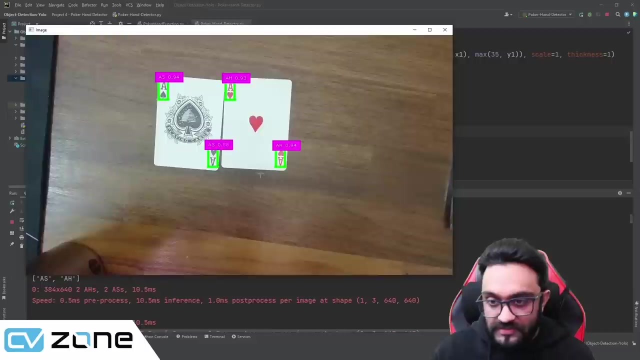 and we will print it before and we will print it after. so there you go. so if this is the case, then the set is like this, so we are getting one of each. so that's good, that's exactly what we want. so, as you can see here, 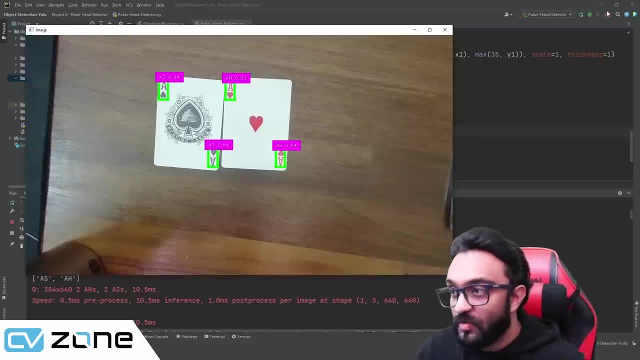 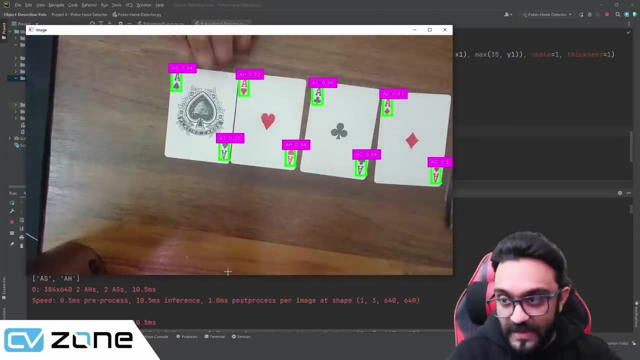 it is detecting, but we are getting one of them. okay. so now what we can do is we can add five of these and it should give us the result. so let's put a four of a kind which- because it's really easy, here i have already a's lined up and we have these a's and then we can add simply: 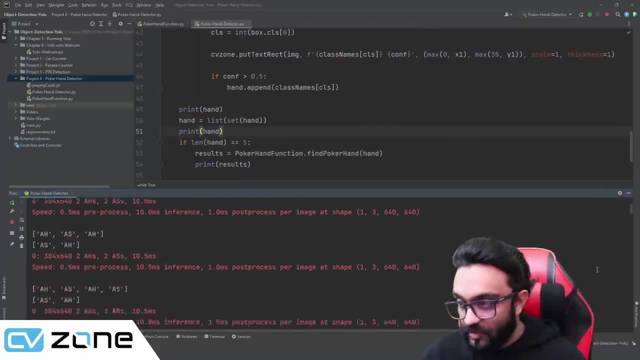 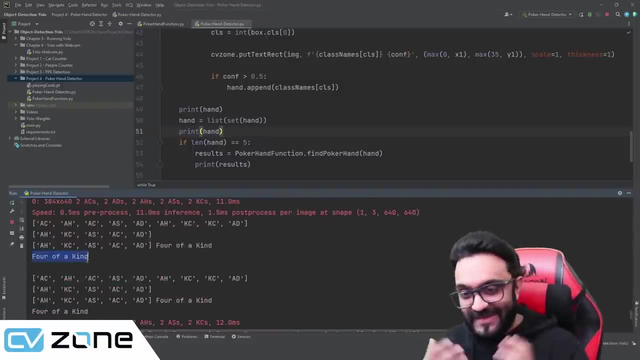 another card which is a king, and we should get an output here. so let's go at the end and let's see. so there you go, we are getting four of a kind. so the moment of growth has been revealed. and we're getting a four of a kind- excellent. so that is really amazing to see. 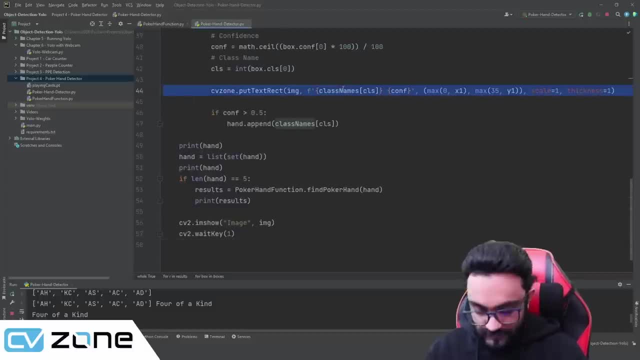 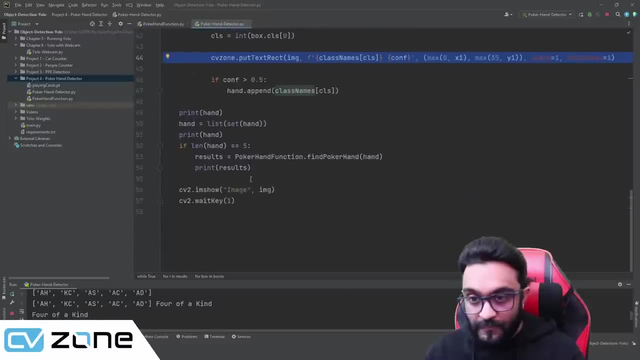 how it works. now what we can do is we can simply put it on on display so that we can see it in real time. so here, cv's on put text. we can copy that and we can paste it here and instead of the class name, we'll do the result, our results and 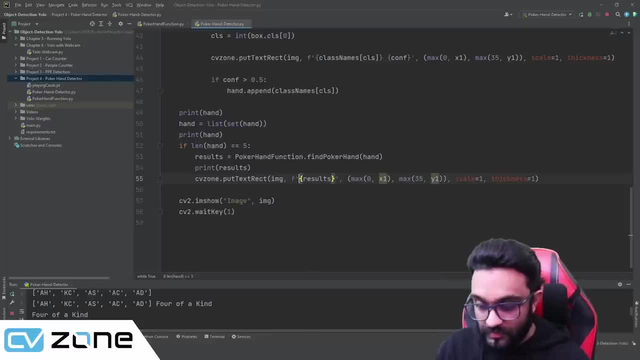 we will write. so here we are, going to give in the position of zero and zero. let's say: or should we put it in the middle? let's do a little bit in the middle. what's the size? 1280, maybe 300, and the height may be 50. and the scale? we want it big, so let's put it at five. so it's going to be a little bit. 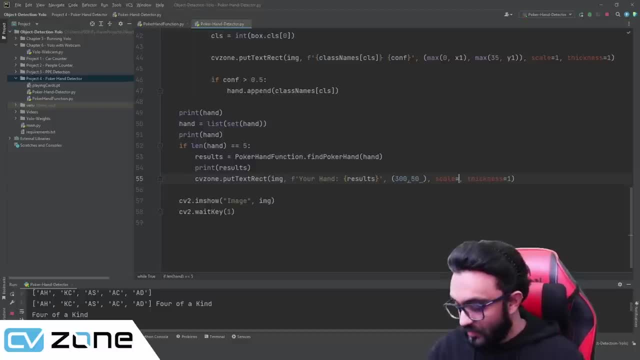 bigger, and then we're going to put a little bit lower. so we're going to put the number, so we're going to put it in the middle, so let's do it in the middle. and then we're going to put a little bit at five and the thickness let's put it at six. um, hopefully this will give us some good results. 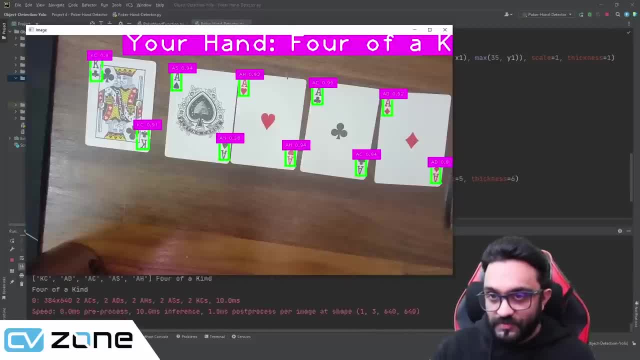 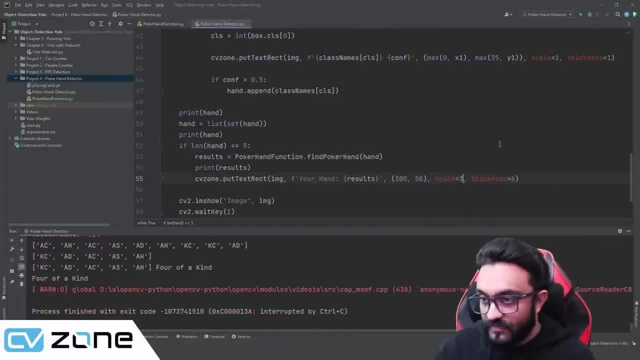 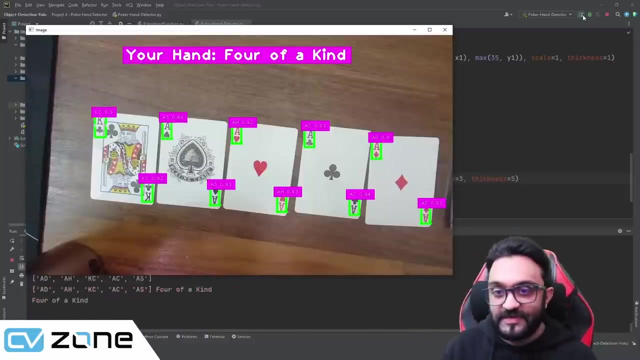 okay. so it's too big. we need to push it down a little bit and we need to make it a little bit smaller. so maybe three and thickness is five and we push it down further to 75.. let's run that. there you go, your hand. four of a kind, excellent. so what if? what if i remove one of the ace? 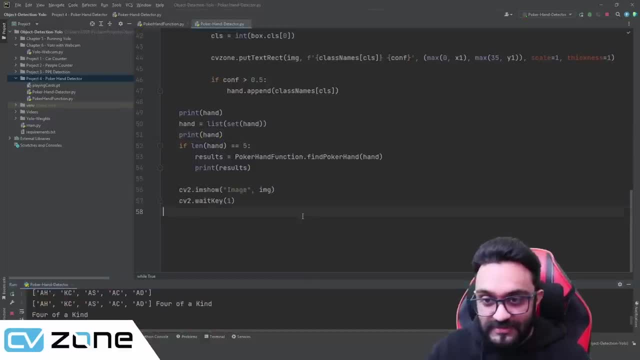 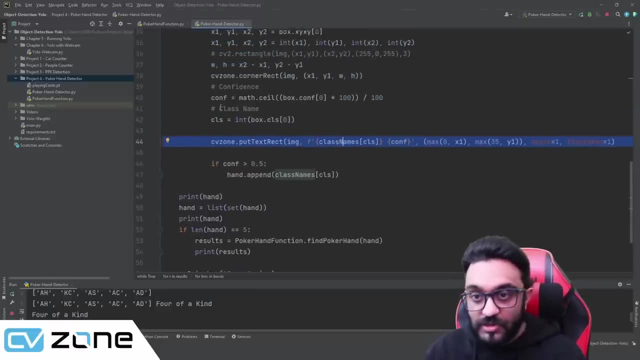 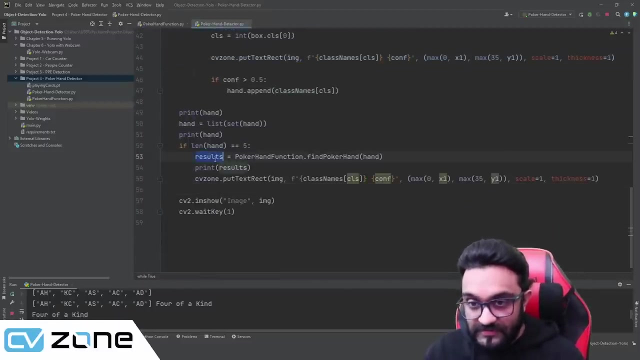 excellent. so that is really amazing to see how it works. now, what we can do is we can simply put it on on display so that we can see it in real time. so here see, we don't put text, we can copy that and we can paste it here and, instead of the class name, we'll do the result. 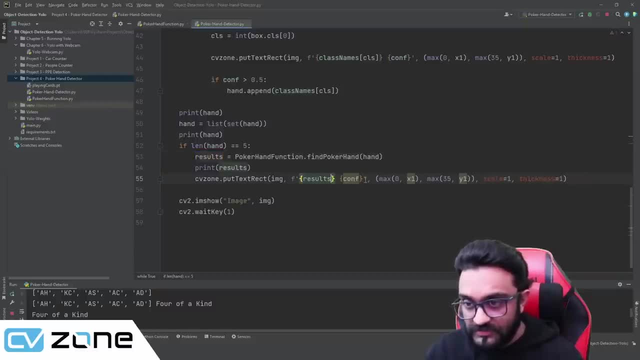 results and we will write your hand and we will write it like that. so here we are, going to give in the position of zero and zero. let's say, or should we put it in the middle? let's do a little bit in the middle. what's the size? 1280, maybe 300, and the height? maybe 50. 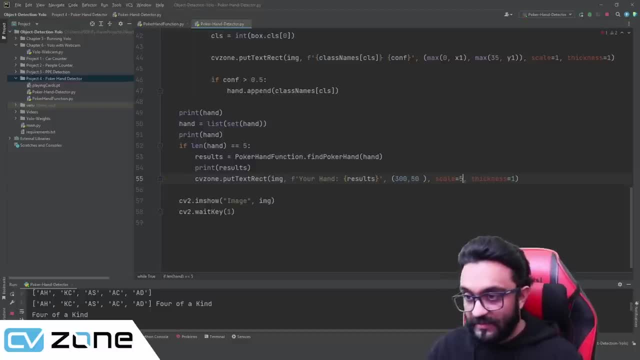 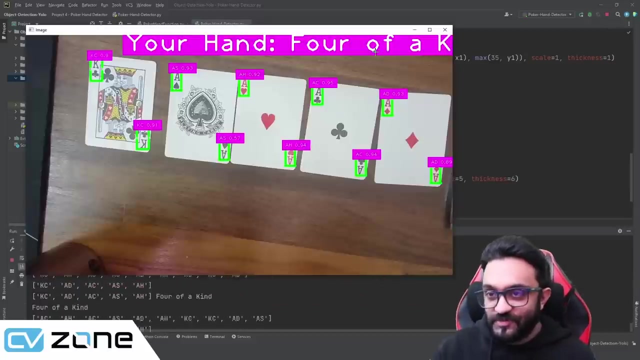 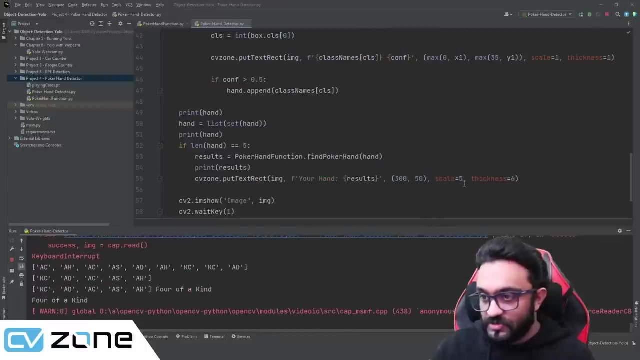 and the scale. we want it big, so let's put it at five. and the thickness: let's put it at six. um, hopefully this will give us some good results. okay, so it's too big. um, we need to push it down a little bit and we need to make it a little bit smaller, so maybe three and thickness is five. 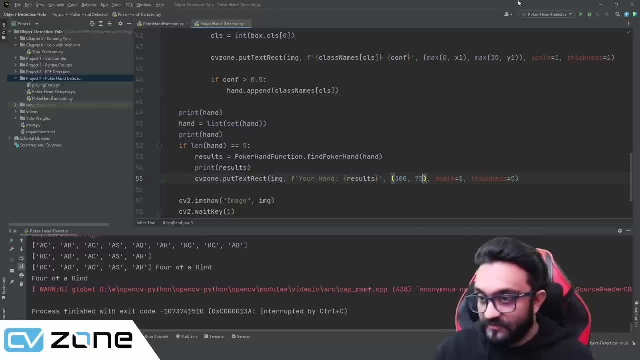 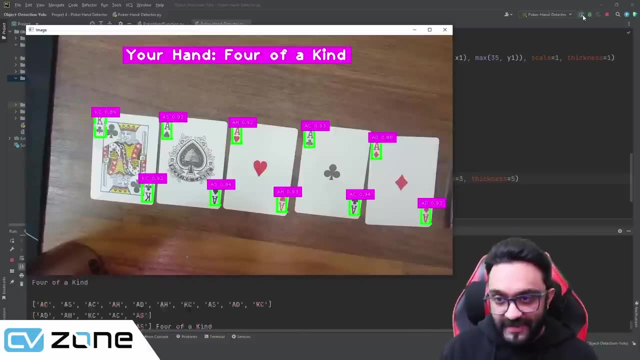 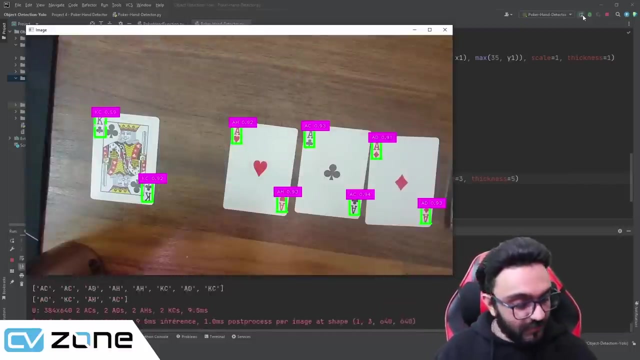 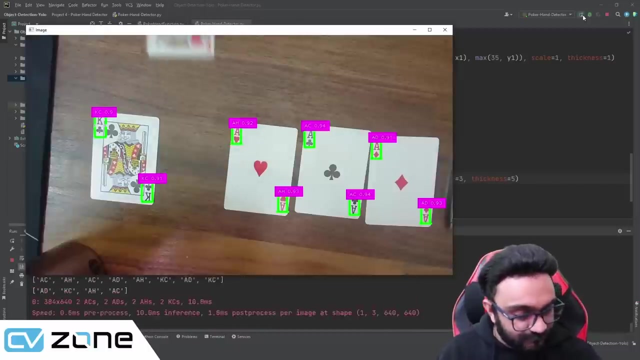 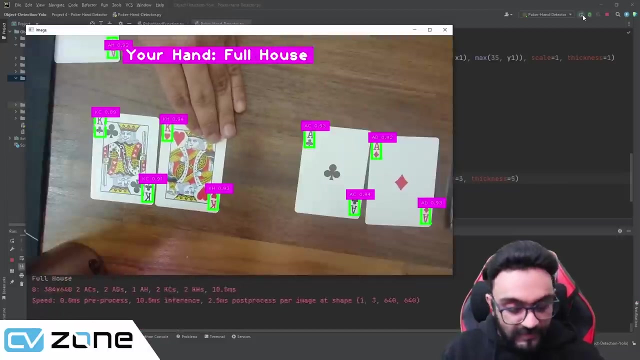 and we push it down further to 75.. let's run that. there you go, your hand, four of a kind, excellent. so what if? what if i remove one of the ace and i put a king there? then it becomes full house. your hand is a full house, that's excellent. and what if i put instead of an ace, i put another king? 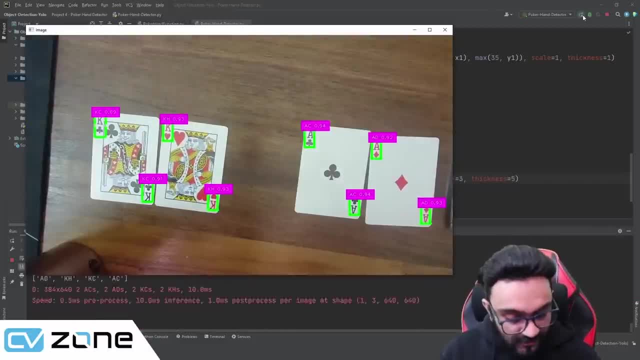 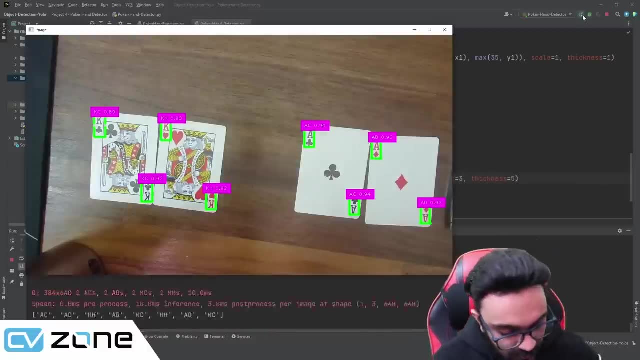 and: okay, where is this? okay, i need to remove that. and then i put a random card. let's say six, then it should be two pair, excellent. so what we'll do is we'll go one by one and we will test out each of these scenarios. so let's put it together. 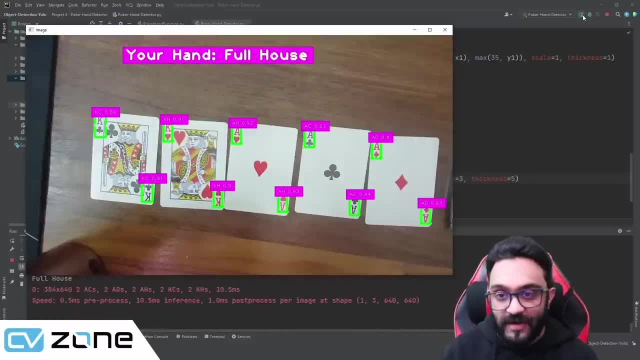 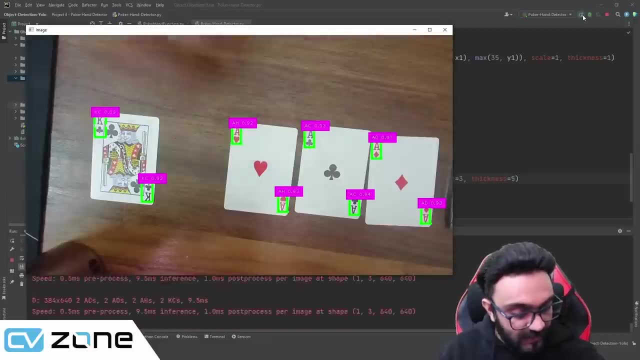 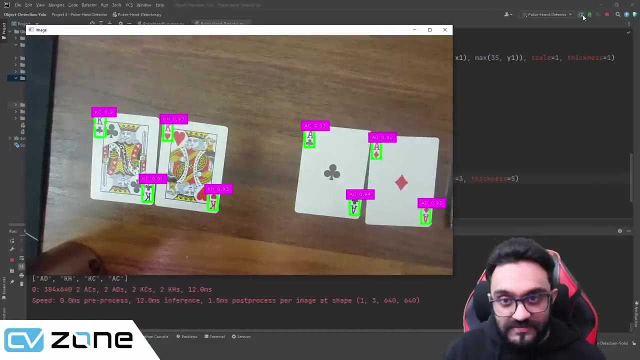 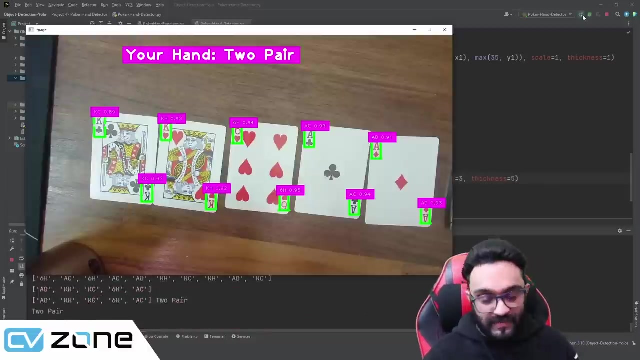 and i put a king there, then it becomes full house. your hand is a full house. that's excellent. and what if i put, instead of an ace, i put another king, and okay, where is this? okay, i need to remove that. and then i put a random card, let's say six, then it should be two pair, excellent, so what we'll? 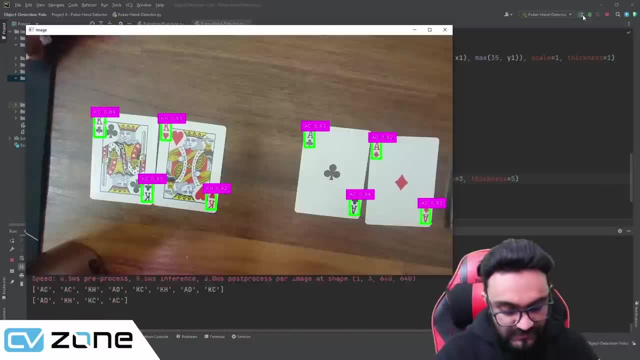 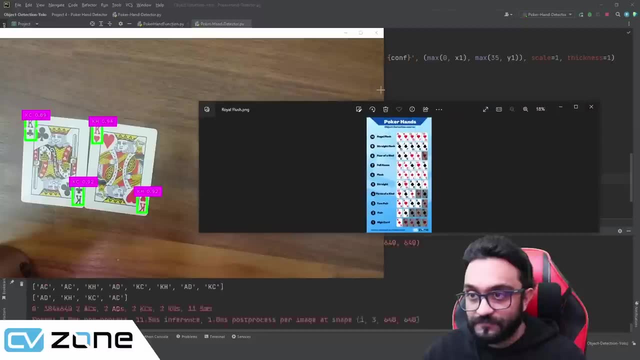 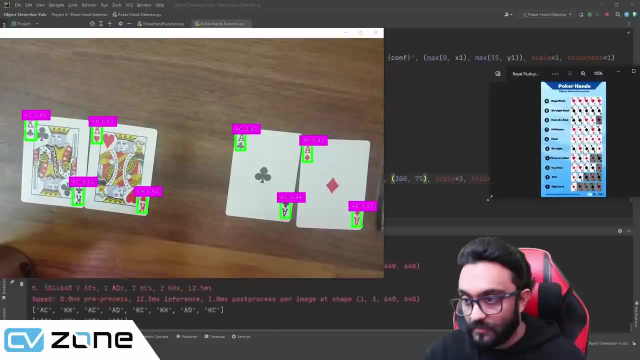 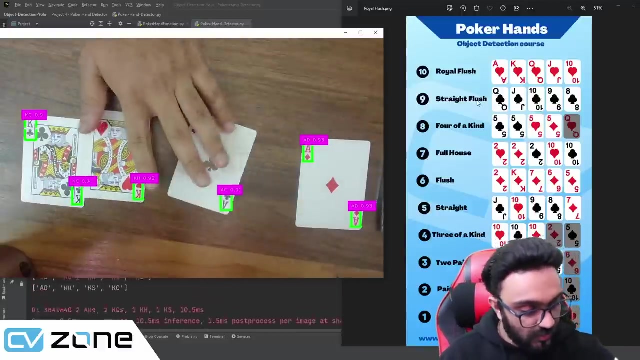 do is we'll go one by one and we will test out each of these scenarios. so let's put it together and let's see what do we get. so let me try to put this here. so the first one we are going to do is royal flush, so in which we have ace. uh, then we have 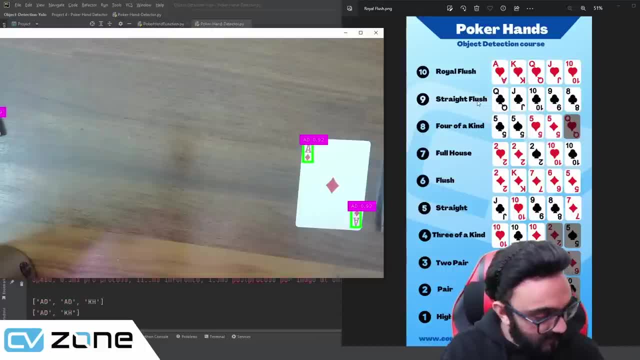 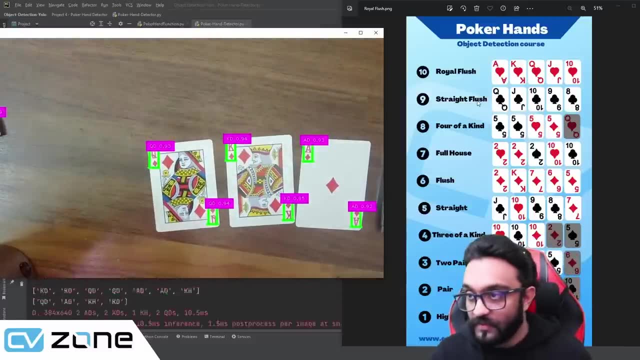 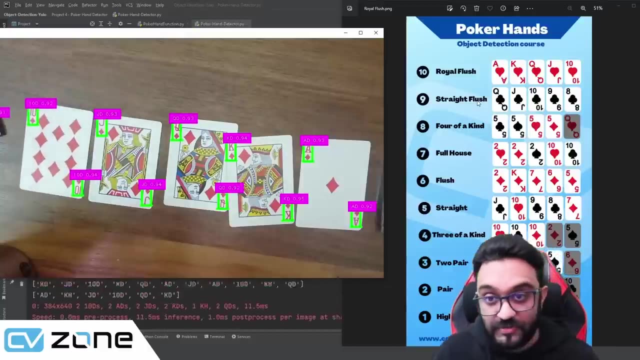 uh, of the same type. so we will have the king of diamond, then we have the queen of diamond, and then we have the jack of diamond, and then we have the 10 of diamond. so that should give us royal flush. so there is another card coming in here. 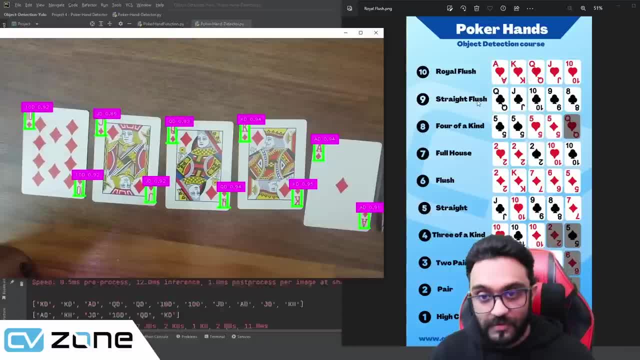 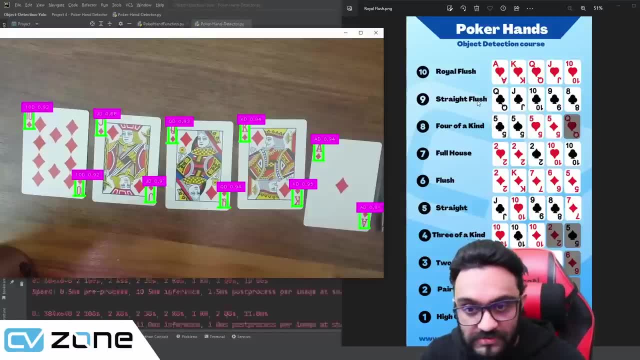 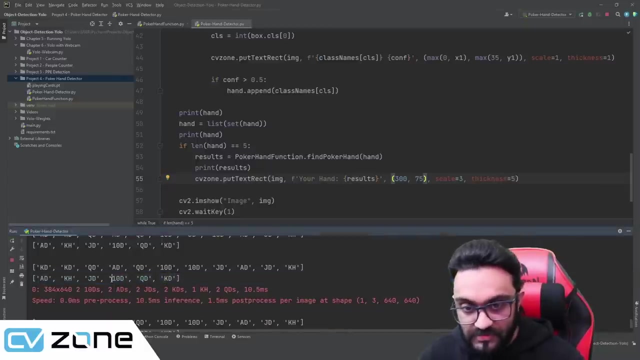 let's put them straight. there you go. so now it should give us the result, but it's not. uh, what is the issue 10 of diamond? j, d, q, d, k d and a d? uh, what seems to be the issue a, k, h, j d, 10 d, q d and k d? so there's a 10 d somewhere, for some reason. 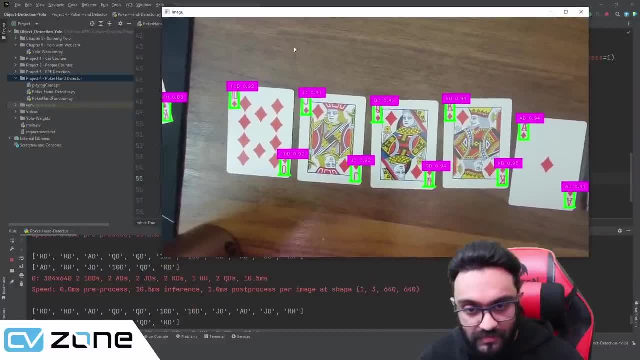 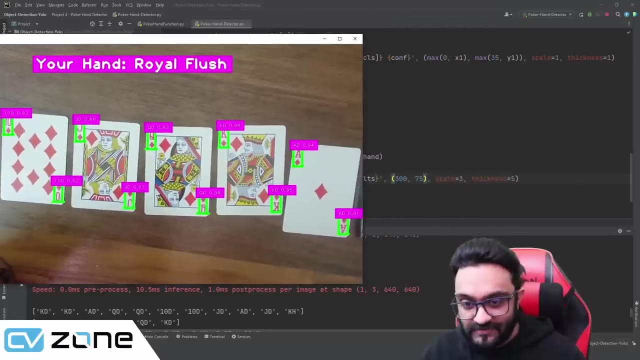 yeah, there is a 10 d. yeah, 10 d is supposed to be there. a k j. there's another k k h. where is the k h? oh, okay, so it's detecting it here. my bad, so there was another card, uh, on the side. that's why it was detecting that, okay, so there you go, so you have a royal flush. 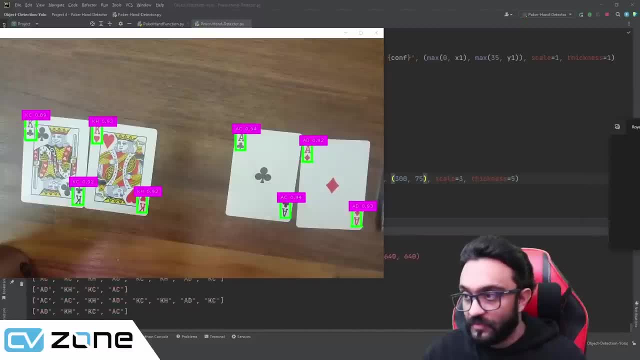 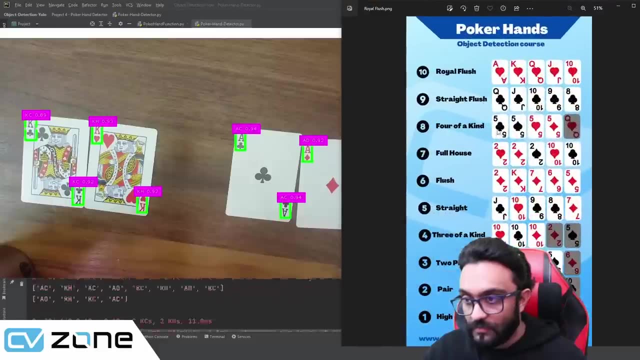 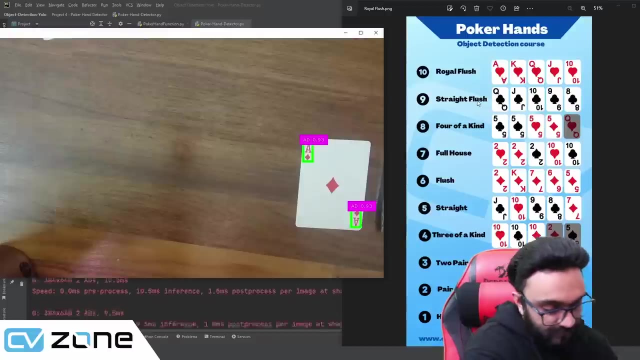 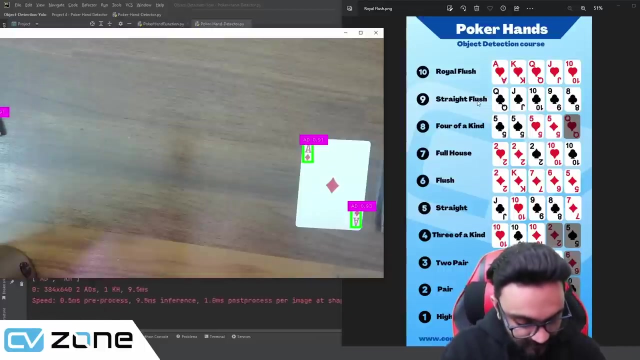 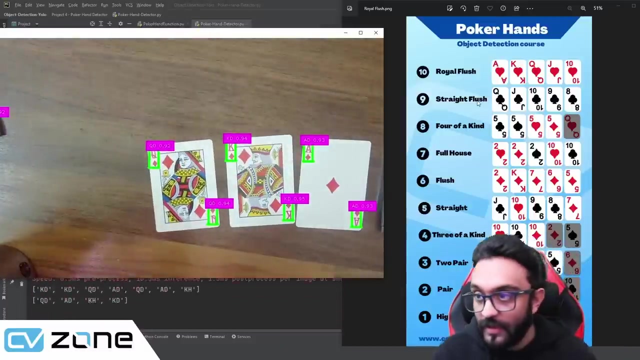 let's see what do we get. so let me try to put this here. so the first one we are going to do is royal flush, so in which we have ace, then we have of the same type, so we will have the king of diamond, then we have the queen of diamond, and then we have 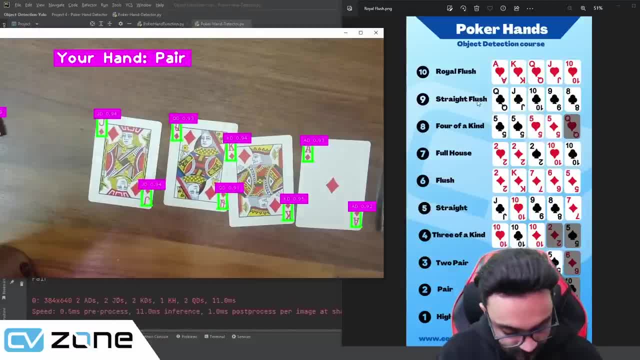 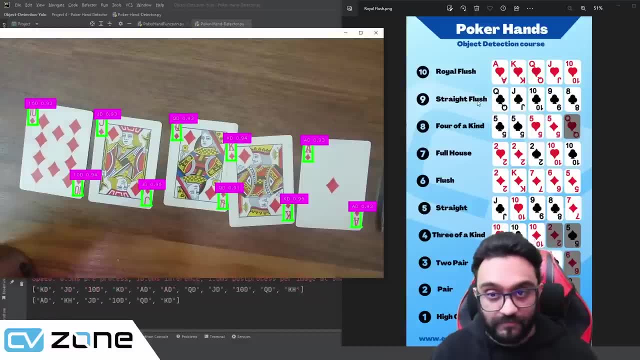 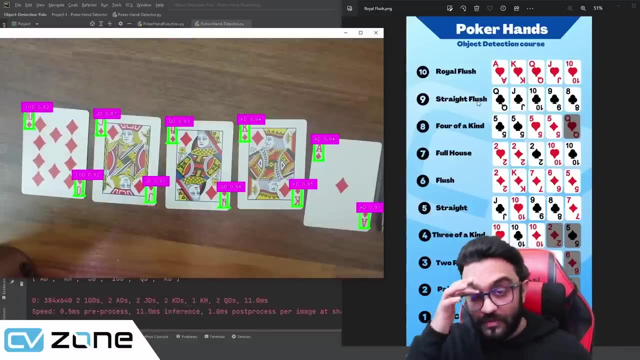 the jack of diamond and then we have the ten of diamond. so that should give us royal flush. so there is another card coming in here. let's put them straight. there you go. so now it should give us the result, but it's not. uh, what is the issue? ten of diamond, j, d, q, d, k, d and a d? uh, what seems to be? 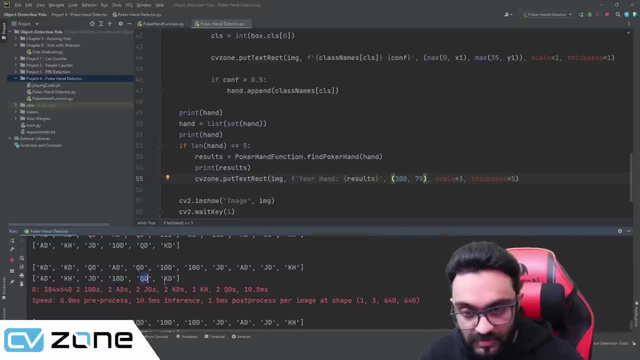 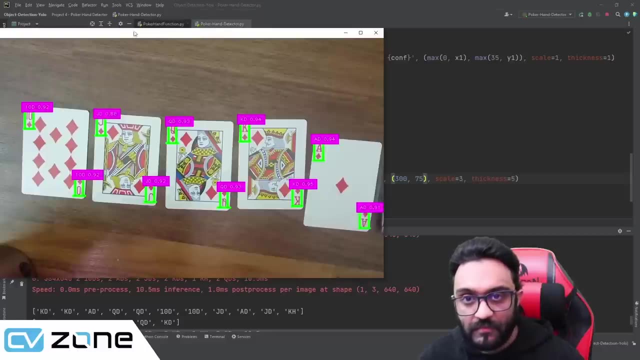 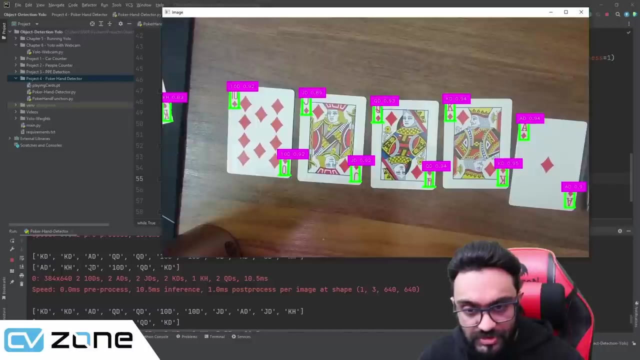 the issue: a k h, j d, 10 d, q, d and k d. so there's a 10 d somewhere for some reason. yeah, there is a 10 d. yeah, 10 d is supposed to be there. a k j. there's another k k h. where is the k h? oh, okay, so it's detecting it here. my bad, so there was. 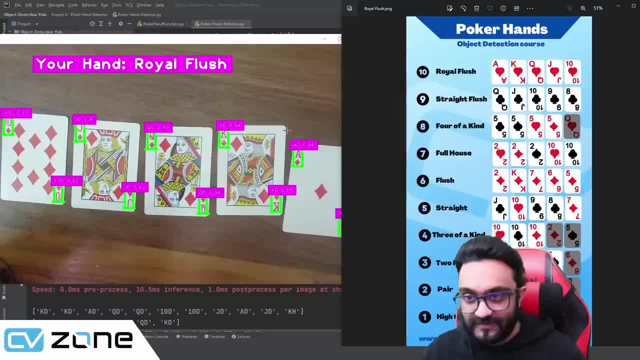 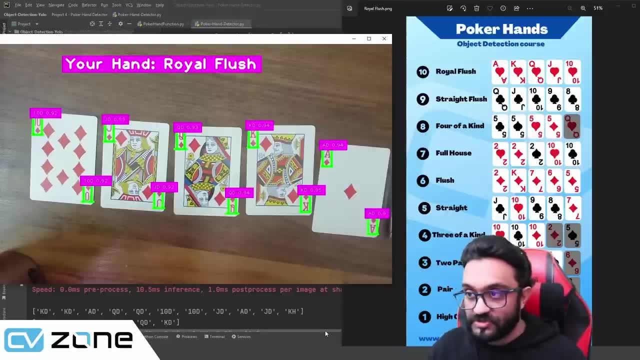 another card, uh, on the side. that's why it was detecting that. okay, so there you go. so you have a royal flush. excellent, now let's try a straight flush. so, uh, we have, let's say, king, queen, jack, 10, and if we put a nine, uh, nine, of diamond, then it will become a straight flush, because it will not be a royal, it will be. 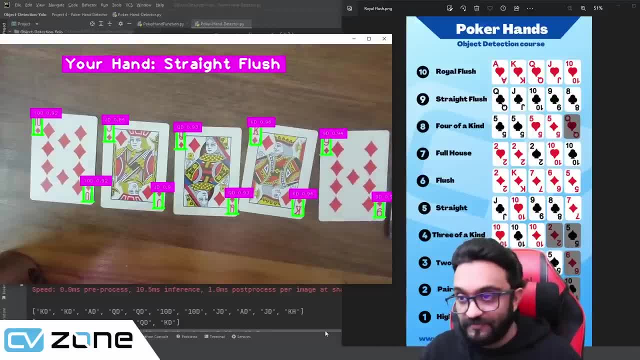 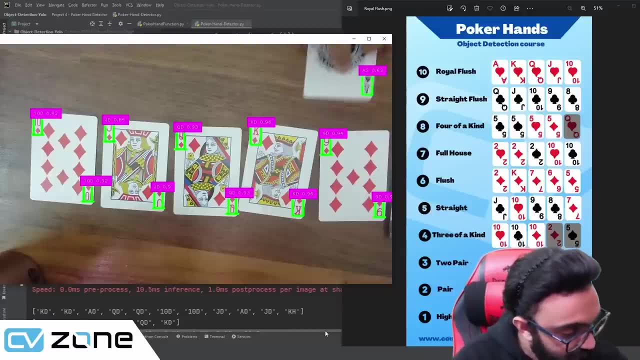 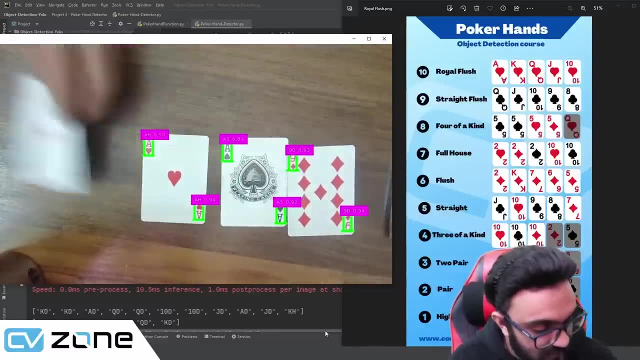 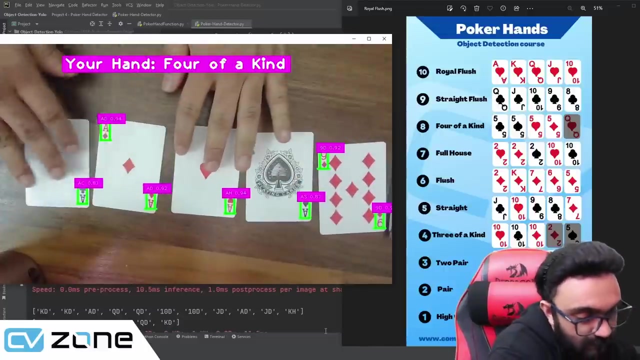 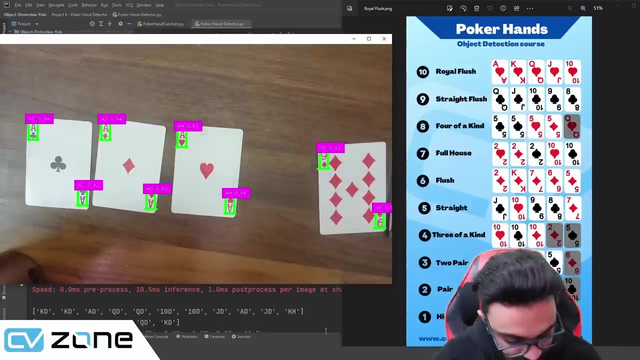 a straight flush, there you go. so now it is a straight flush and let's try four of a kind. so we are going to add ace, ace, ace, and a king, so, or a nine, so ace, ace, ace. and where is the other ace? there you go, there you go, hand four of a kind. that's perfect. then we will try a full house, so we will remove. 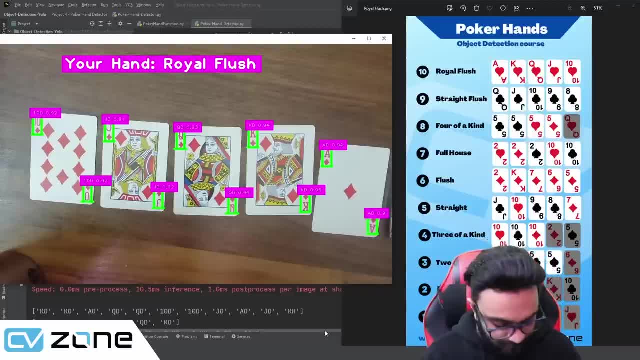 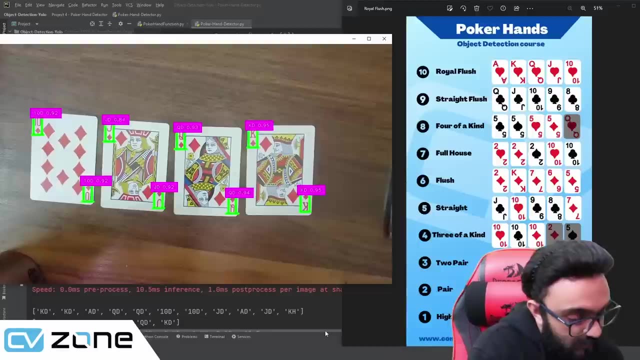 excellent. now let's try a straight flush. so we have, let's say, king queen jack 10, and if we put a nine, uh nine, of diamond, then it will become a straight flush, because it will not be a royal, it will be a straight flush. there you go. so now it is a straight flush, and 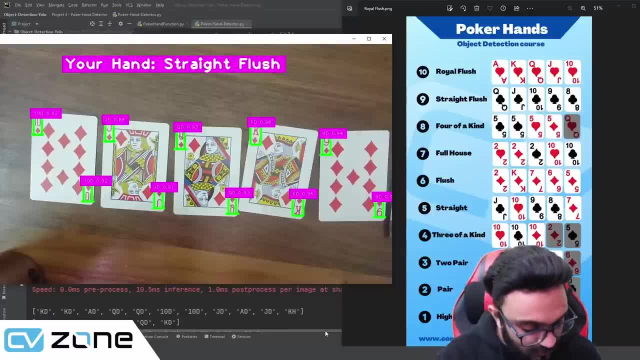 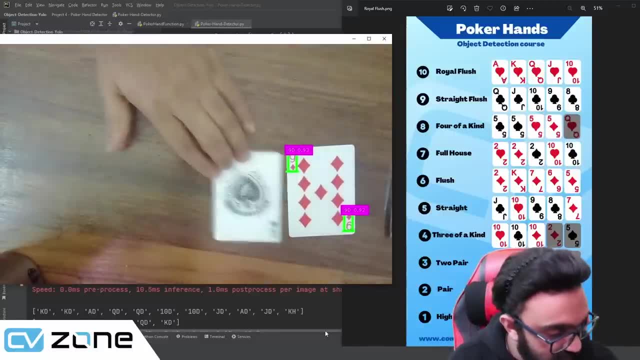 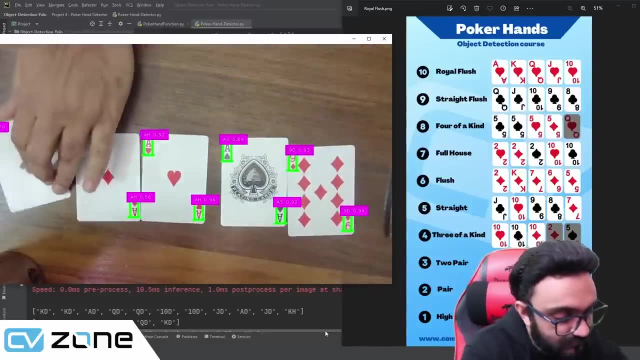 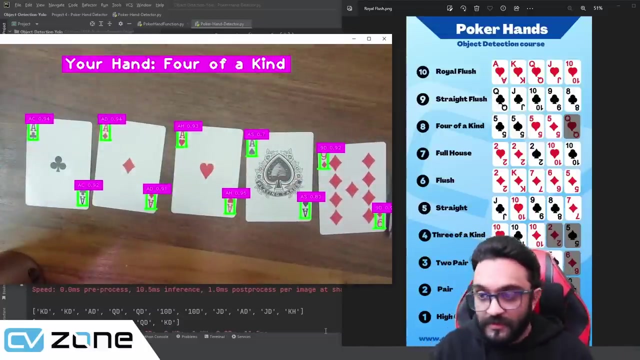 let's try four of a kind. so we are going to add ace, ace, ace, and a king, so, or a nine, so ace, ace, ace. and where is the other ace? there you go, there you go, hand four of a kind, that's perfect. then we will try a full house, so we will remove. 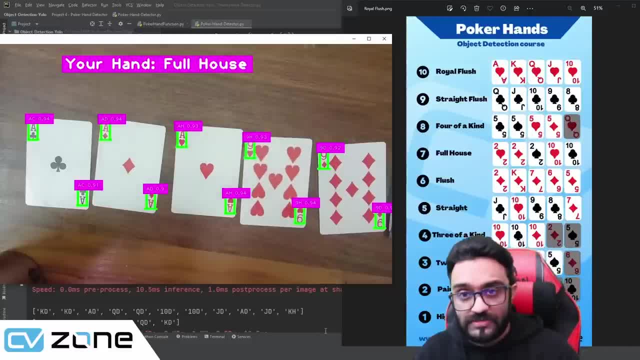 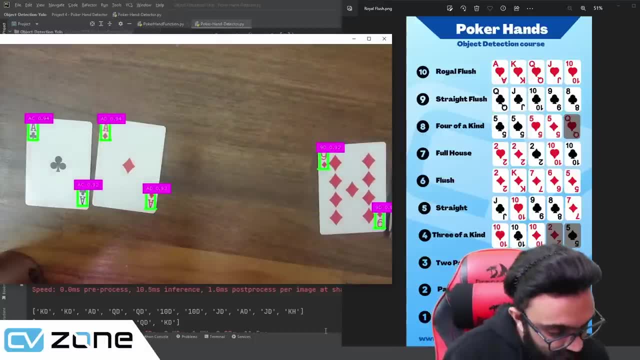 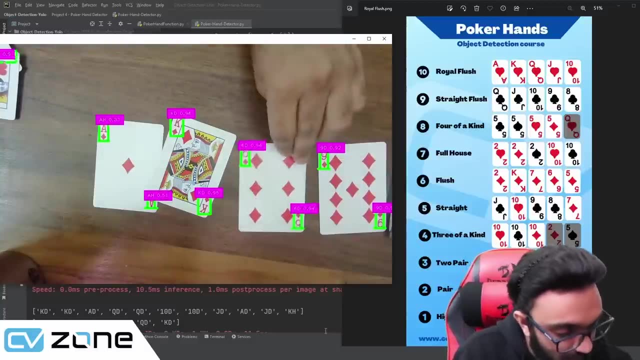 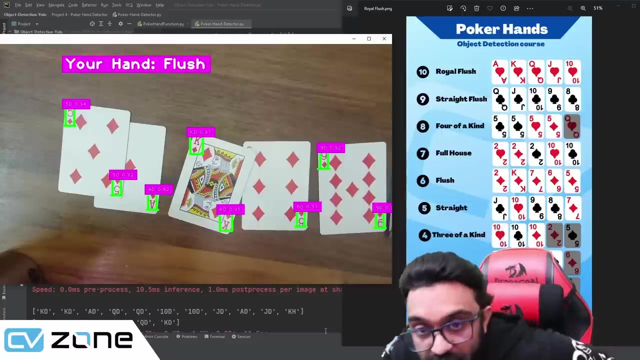 the a and we will put a nine. so that is a full house. excellent. now we will try a flush. so let's put all diamonds. so random, random diamonds doesn't have to be straight or anything. so we are going to put six and a five, there you go, and we have another one. so there you go. so even if they are, 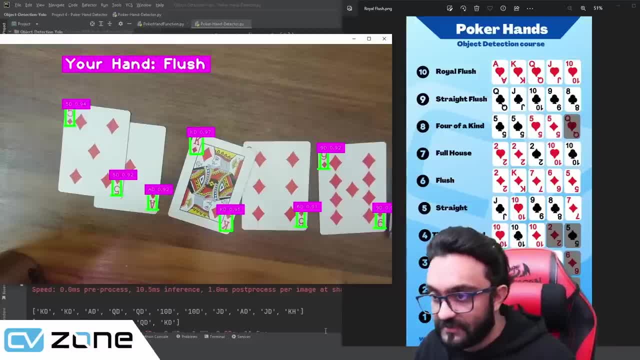 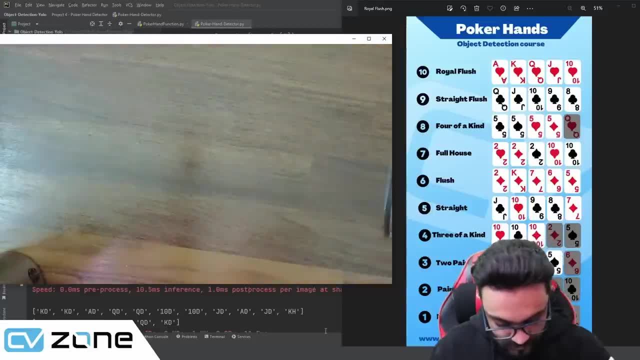 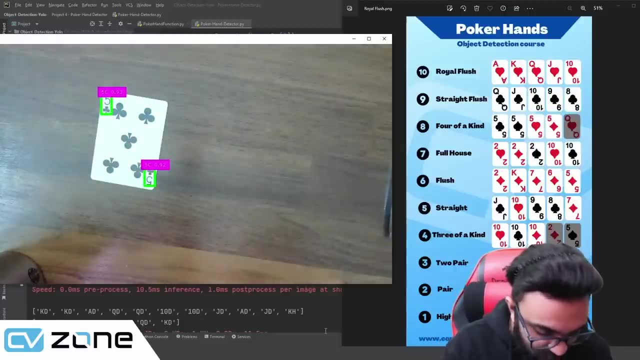 um, not exactly straight, it will still detect them. so full house. uh, then we had a flush. the flush is working fine. now let's try out a straight. so, uh, let's try out five. then we will try. um, two, three, two, three. now we need a four. 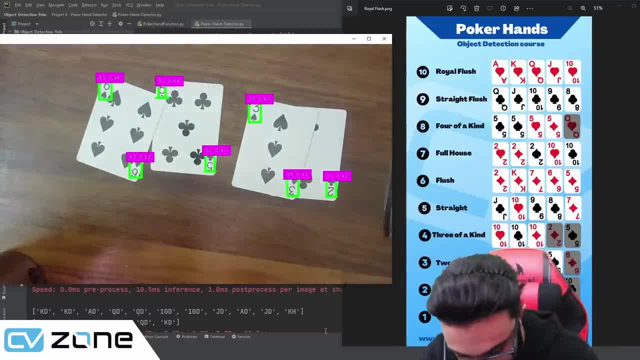 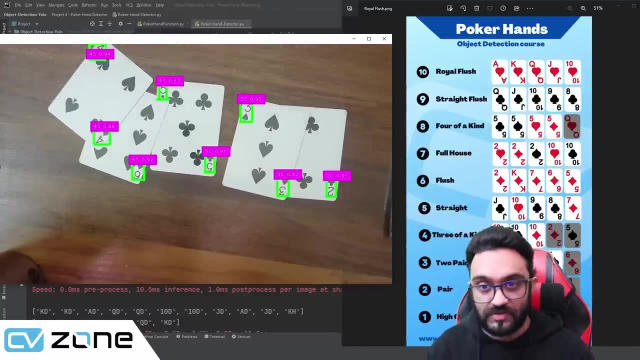 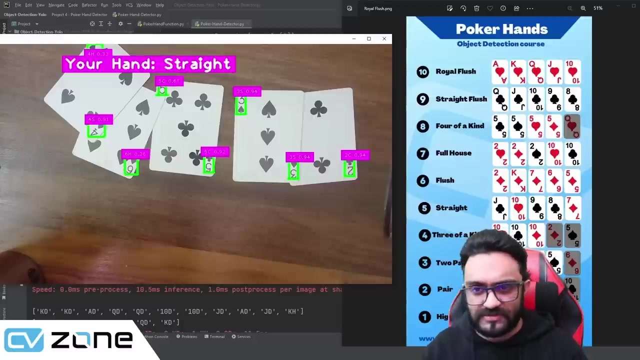 we also need a six, and where is the four? come on, where is the four? there you go. so we have four. so there you go, your hand is straight. so it's upside down. it's not really organized, but still you're getting a straight. it's not very stable. 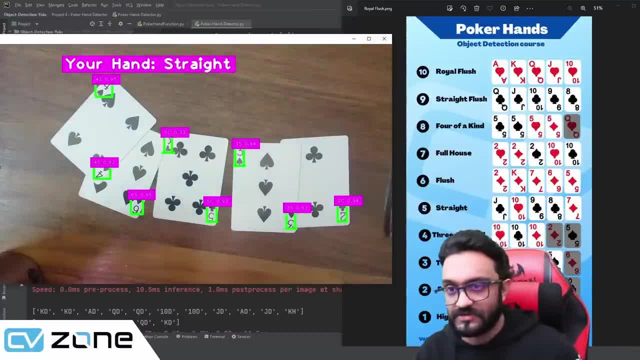 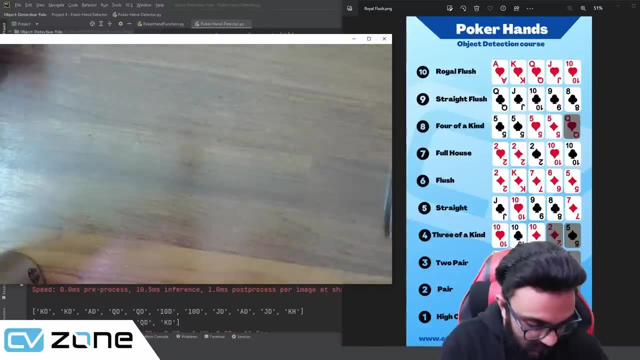 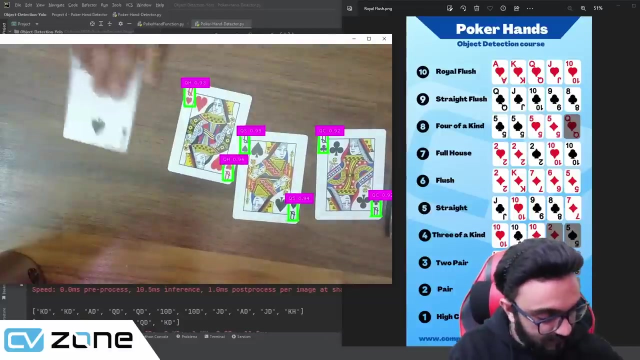 i'm not sure why. if you push it further, yeah, there you go. now it's much um stable, much more stable. so we're getting a straight. uh, that's perfect. then we have to try a three of a kind. so let's try with queens. so these are three queens, and then we have a two and a king. so your hand is three of a. 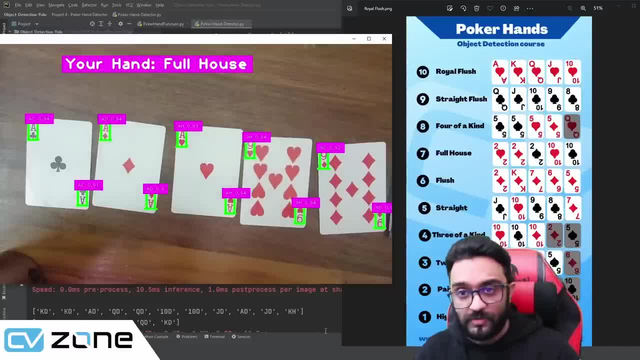 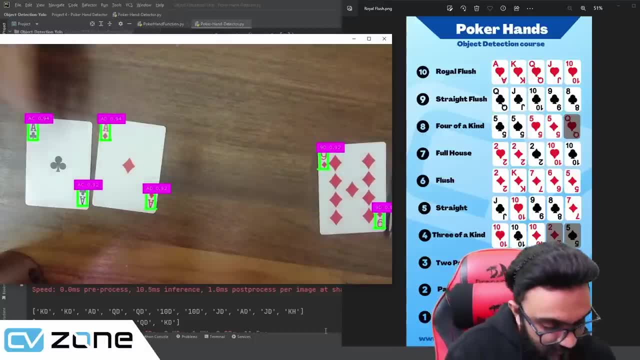 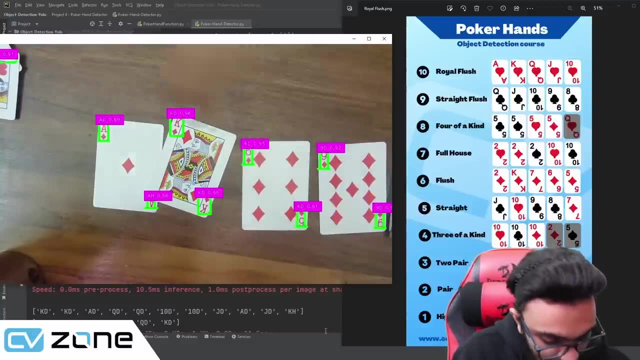 the a and we will put a nine. so that is a full house. excellent. now we will try a flush. so let's put all diamonds. so random, random diamonds. uh, doesn't have to be straight or anything. so we are going to put six and a five. there you go. 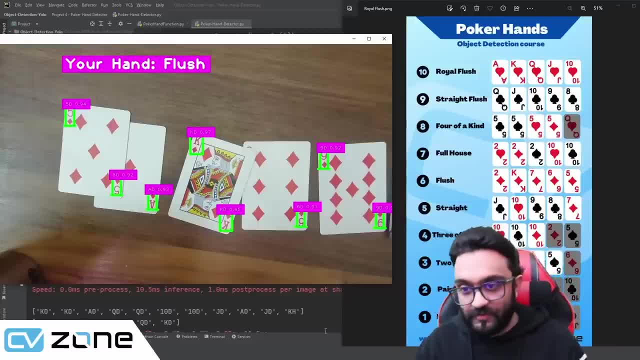 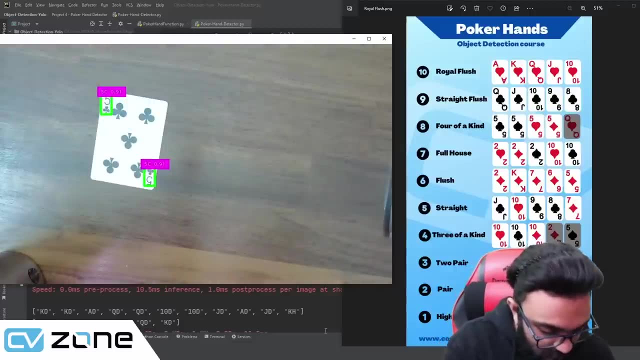 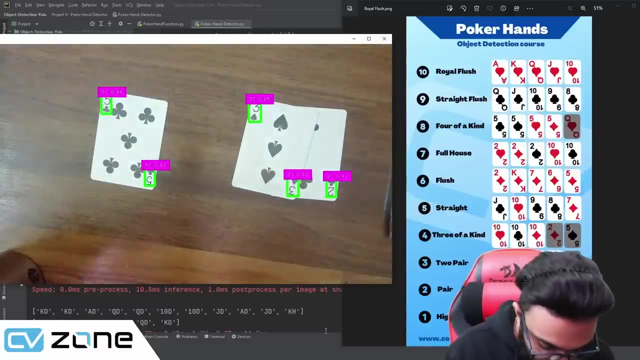 and we have another one. so there you go. so, even if they are um not exactly straight, it will still detect them. so full house. uh, then we had a flush. the flush is working fine. now let's try out a straight. so, uh, let's try out five. then we will try um two, three, two, three. now we need a four. 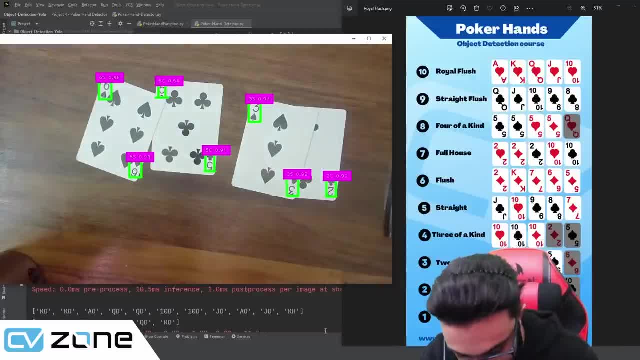 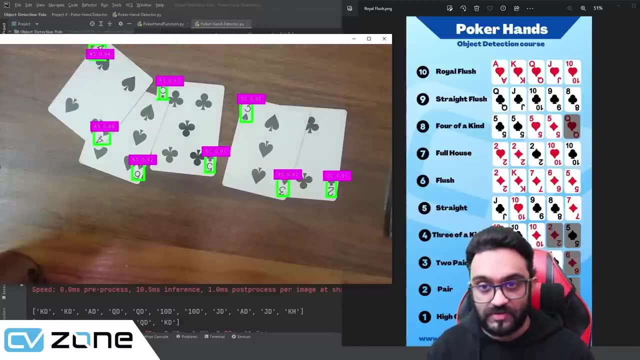 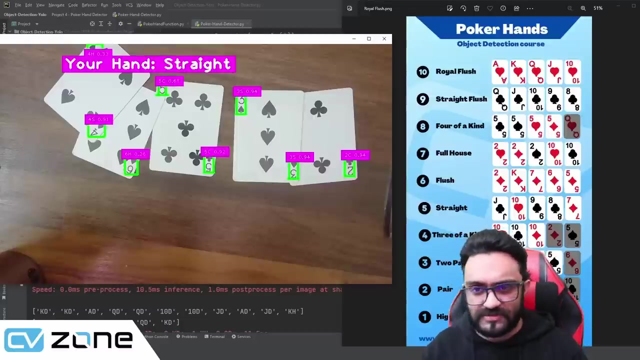 we also need a six. and where is the four? four, come on. where is the four? there you go. so we have a four. so there you go. your hand is straight. so it's upside down. it's not really organized, but still you are getting a straight. it's not very stable, I'm. 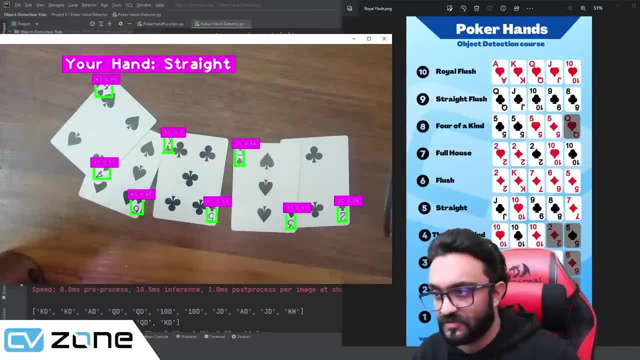 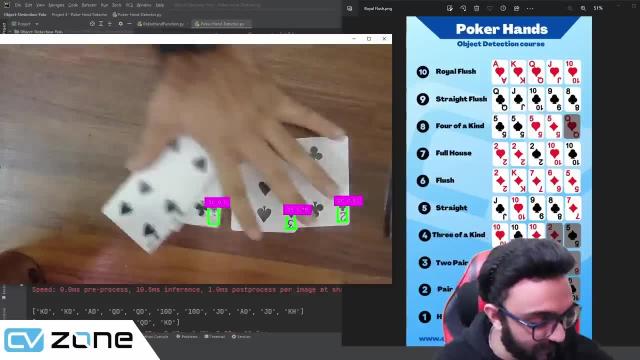 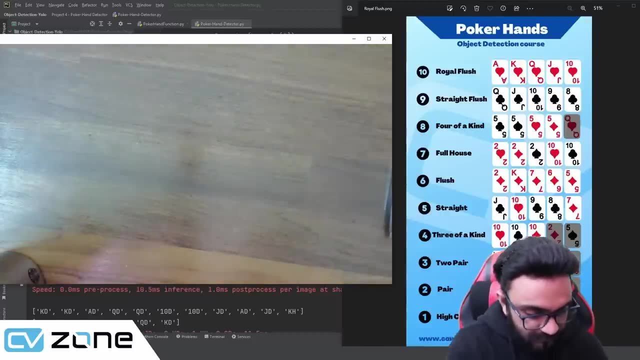 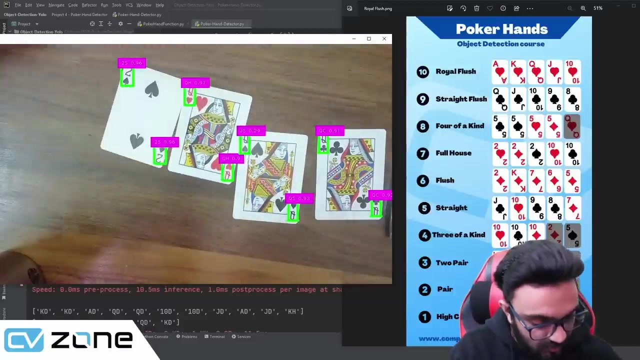 not sure why. if you push it further, yeah, there you go. now it's much um stable, much more stable. so we are getting a straight, uh, that's perfect. then we have to try a three of a kind. so let's try, uh, with Queens. so these are three Queens, and then we have a two and a king. so your hand is three of. 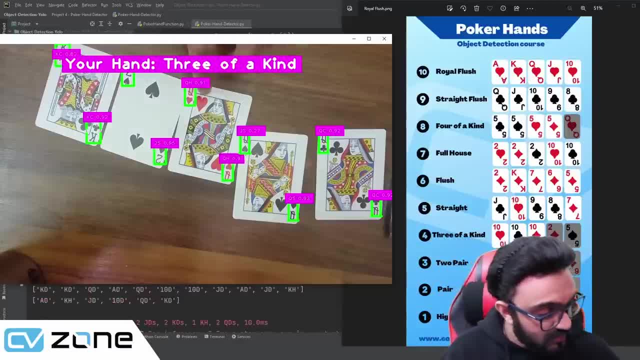 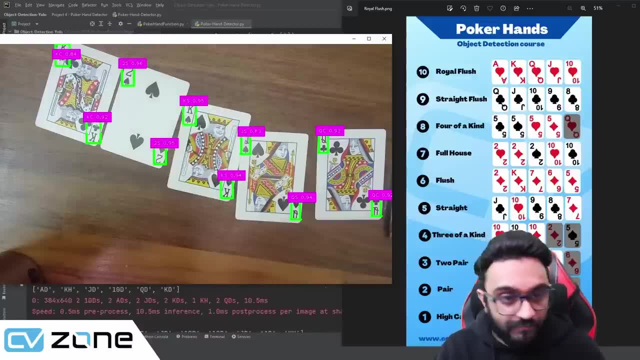 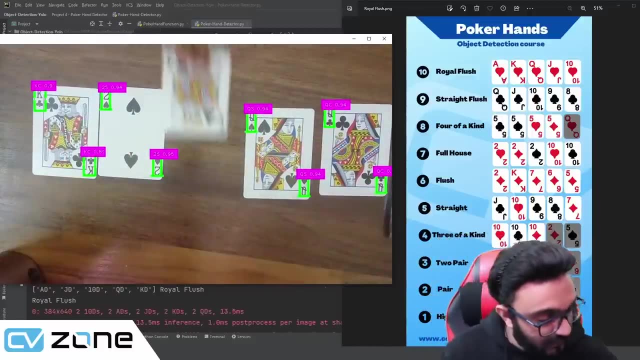 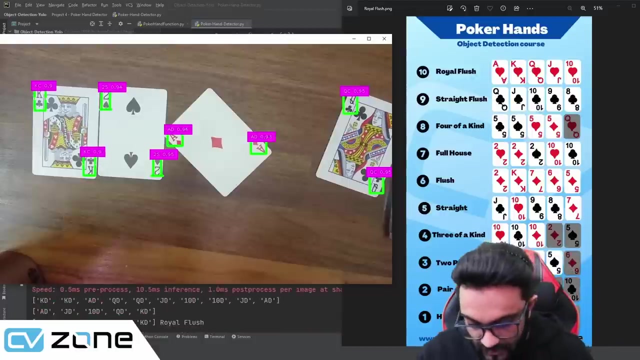 a kind perfect. uh, then we have two pair, so let's remove the queen and let's add a king, so that will become two pair. what happened? um, there you go, it becomes two pair. and that then let's try a single pair. there you go, your hand is a pair, and uh, let's remove the queen and let's put a five here. 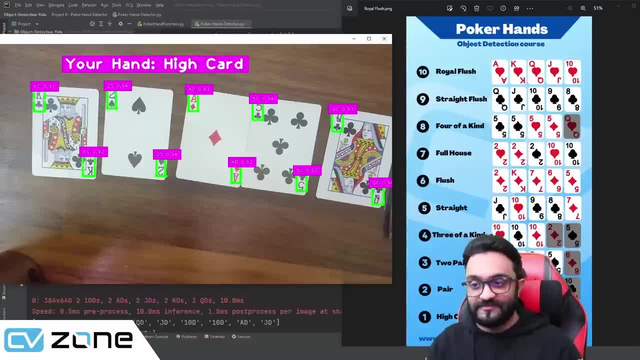 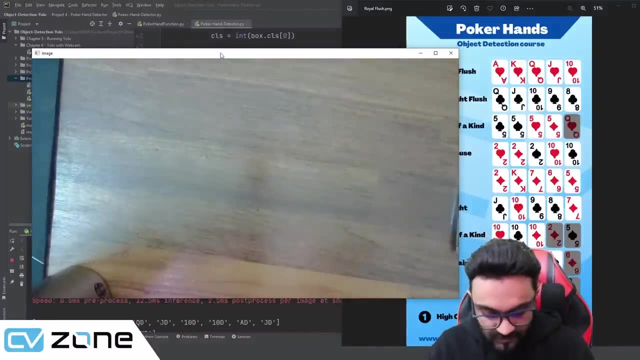 and that should give us high card. there you go: it gives us high card. so this is basically our project successfully done and it looks really good and we are getting real-time and let's, let's try to try it in our hand and see what it gives us. there you go: it gives us high. 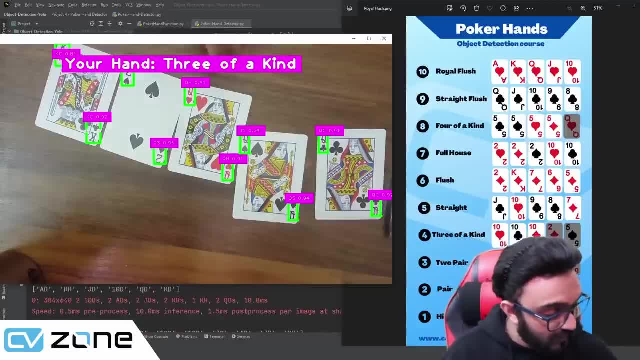 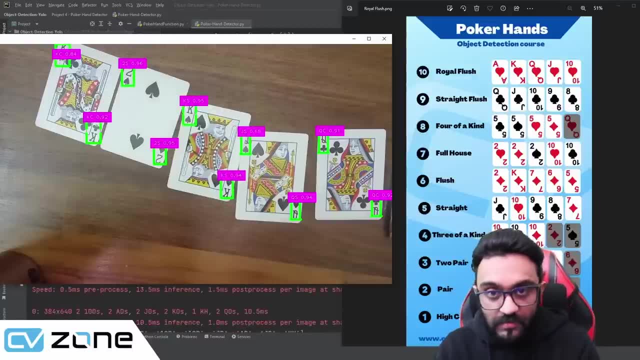 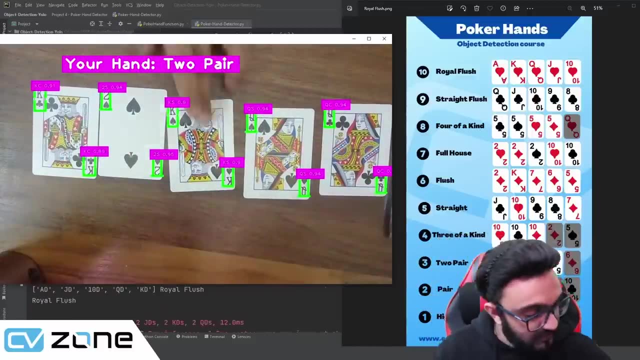 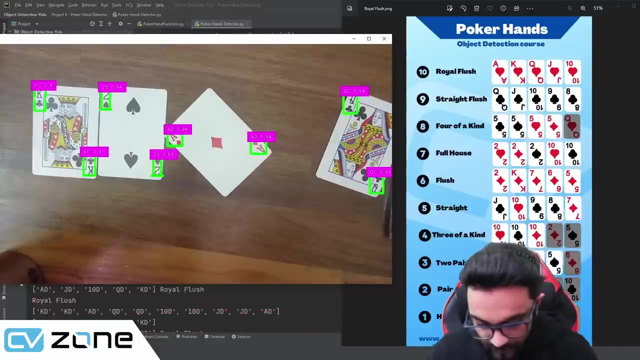 kind: perfect. uh, then we have two pair, so let's remove the queen and let's add a king, so that will become two pair. what happened? um, there you go, it becomes two pair, and that then let's try a single pair. there you go, your hand is a pair, and uh, let's remove the queen and let's put a five here. 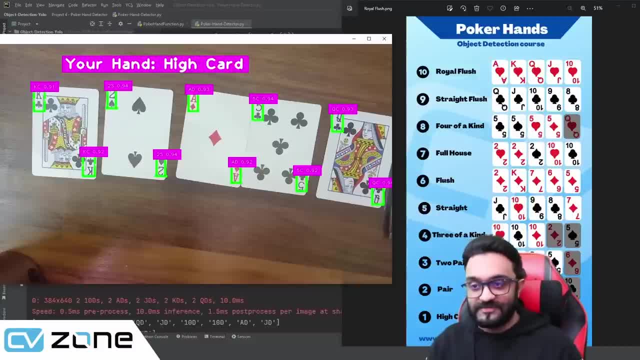 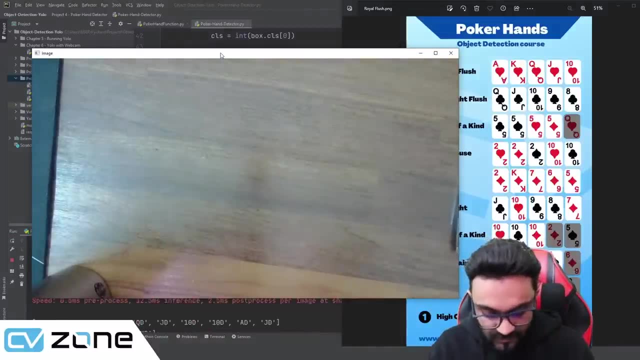 and that should give us high card. there you go: it gives us high card. so this is basically our project successfully done and it looks really good. and, uh, we are getting real-time output and let's, let's try to try to try it in our hand and see what it gives us. there you go: it gives us high card, so it gives us. 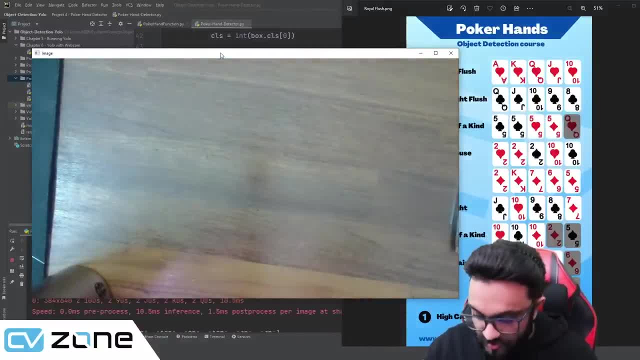 high card and, uh, let's try it, uh, with a pair or something, so that we can see if it works properly or not. um, there you go. so it is a pair, it is a pair, and then let's put another king here, it will become three of there you go, three of a kind. 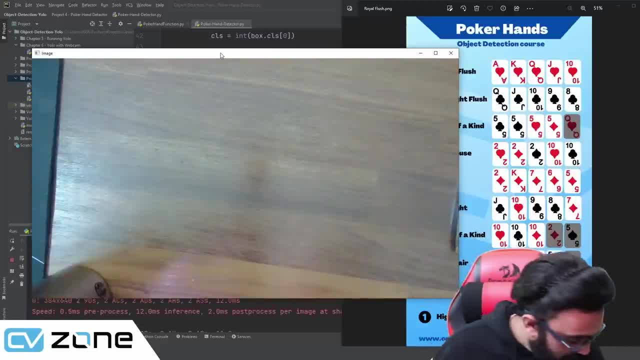 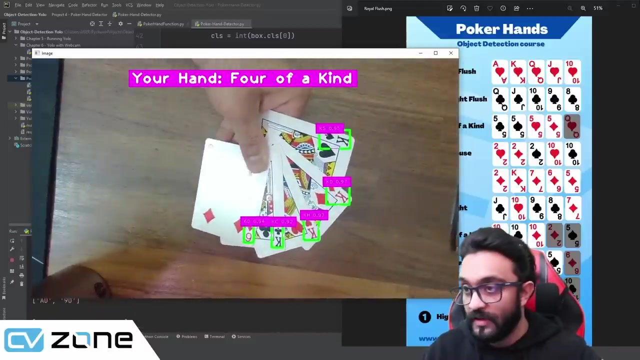 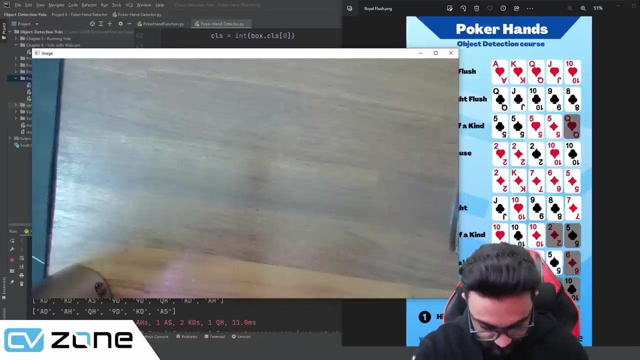 three of a kind, and then let's make it four of a kind. i think it filled up. no, um, we need another king. where is the king? there you go, so we'll get four of a kind. you have four of a kind, and then let's try flush. so let's make a flush of diamonds. 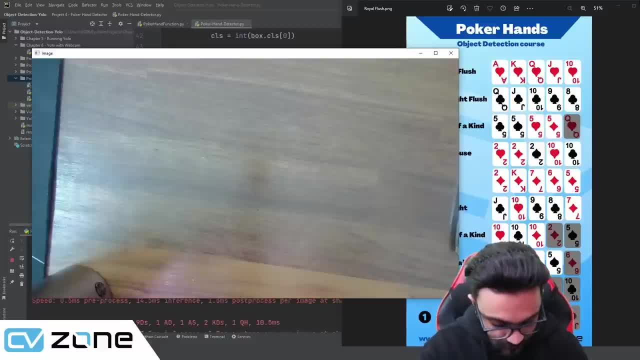 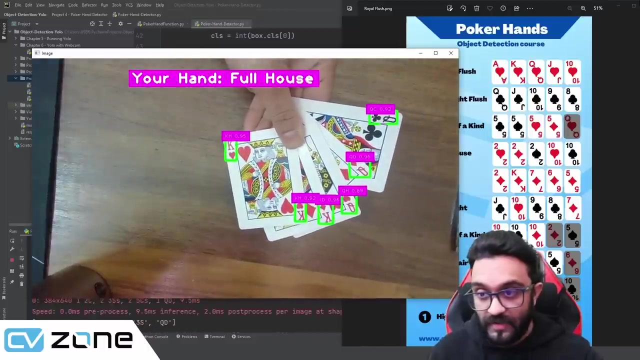 flush of diamonds, there you go. it's a flush, excellent. what else can we try? let's try a full house. so we have queen, queen and king and a king and we need another queen. there you go. so this should be a full house. full house, yep. and if we remove 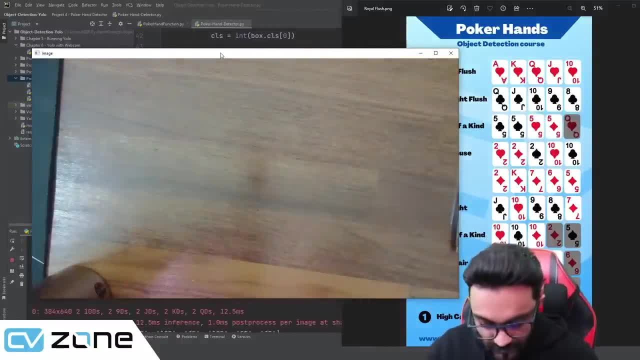 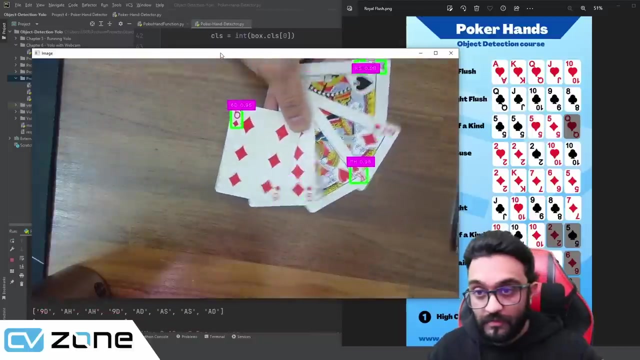 card, so it gives us high card. and uh, let's try it, uh, with a bear or something, so that we can see if it works properly or not. um, there you go. so it is a bear, it is a bear, and then let's put another king here, it will become three of there you go, three of a kind, three of a kind, and then let's. 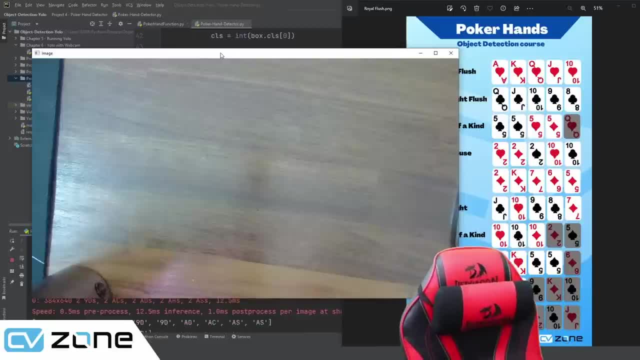 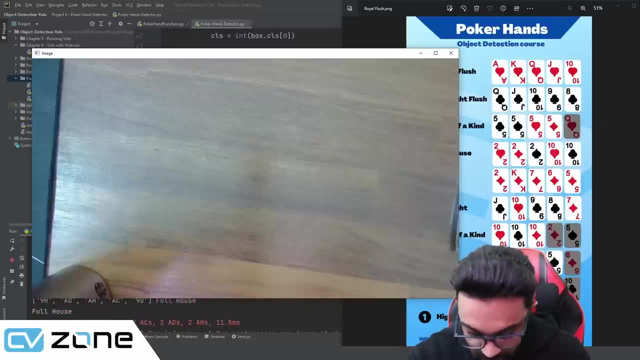 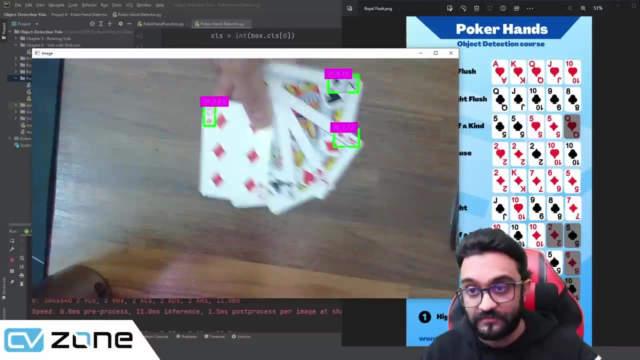 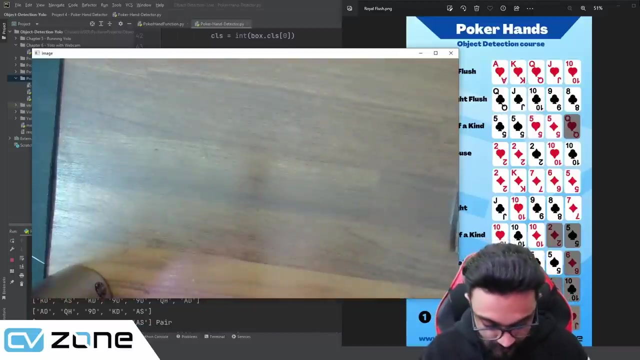 make it four of a kind. i think it filled up. no, um, we need another king. where is the king? there you go. so we'll get four of a kind. yeah, we have four of a kind. and then let's try a flush. so let's make a flush of diamonds. 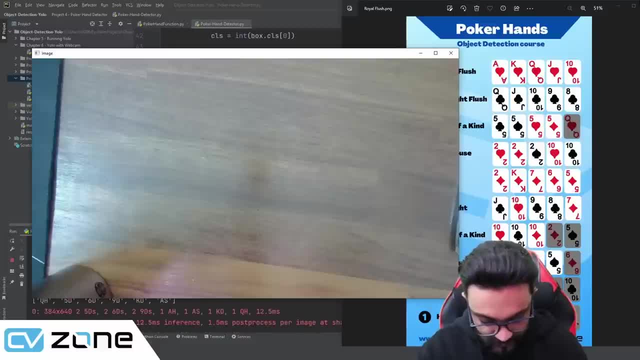 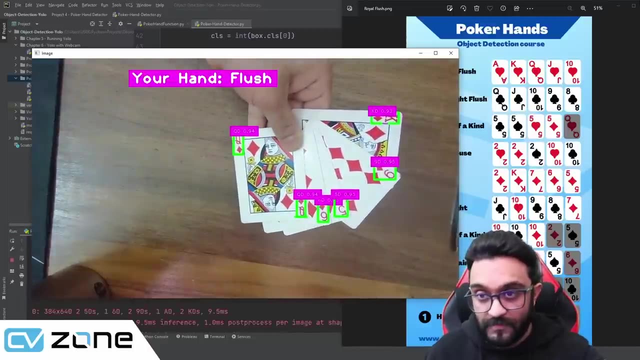 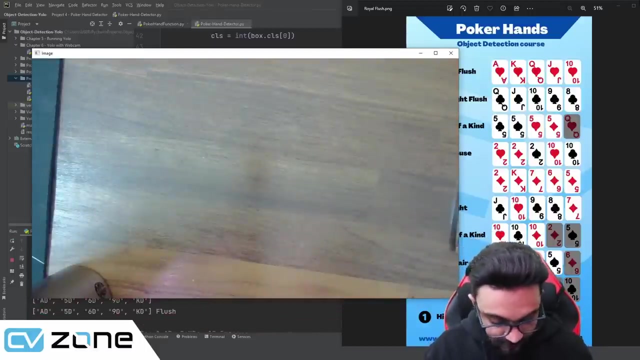 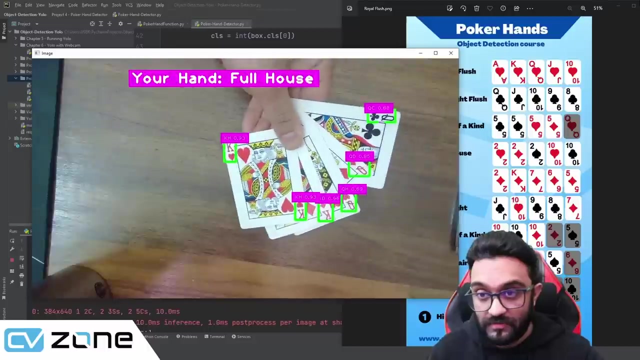 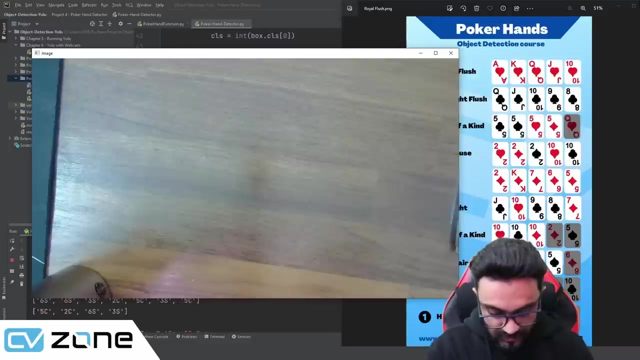 flush of diamonds. there you go. it's a flush, excellent. and what else can we try? let's try a full house. so we have queen, queen and king and a king and we need another queen. there you go. so this should be a full house. full house, yep. and if we remove the queen and put, let's say, two, then it will become two pair. 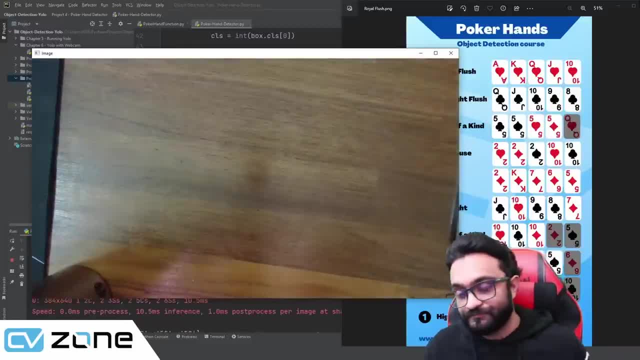 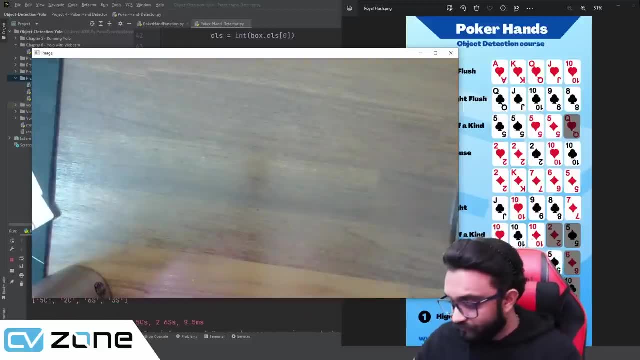 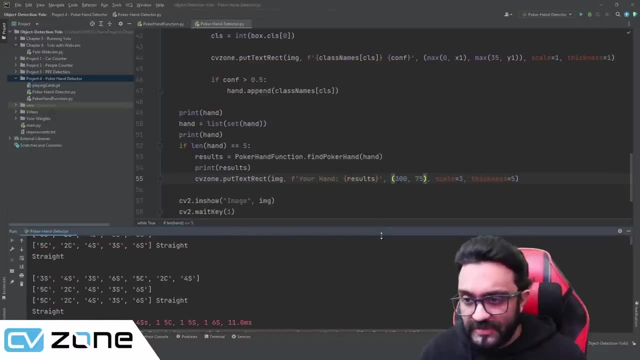 there you go, so that's pretty good. so, as you can see, um our object detection model is working really good, and our poker hand detector is also very working very good. so this was our project. as you can see, you can put all these things together and it really creates a great project and it gives you 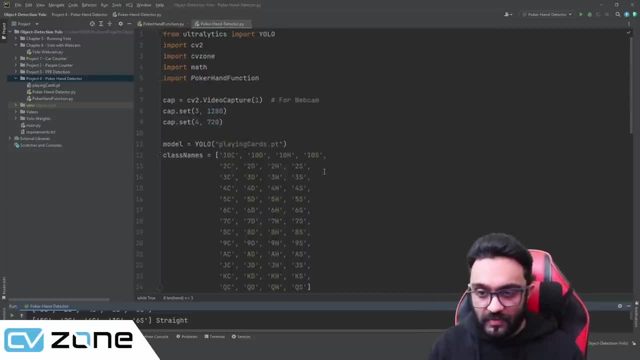 a lot of information and it is fun to play around with as well. so object detection is like a superpower. once you understand how to create a project and how to create a project and how to train your custom models, you can really explore the possibilities and create some really good.